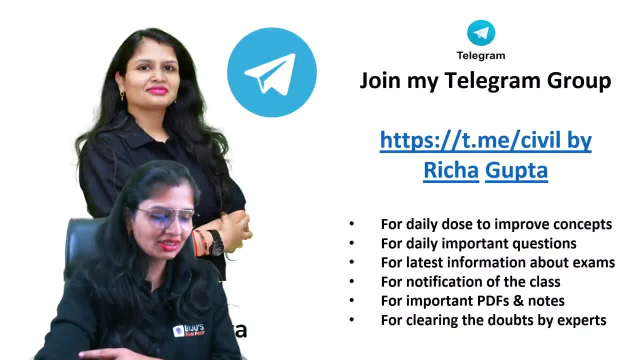 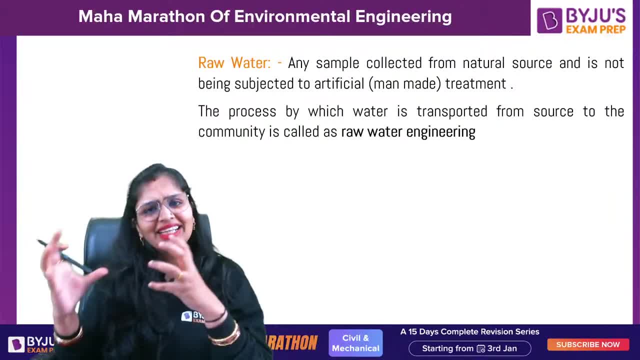 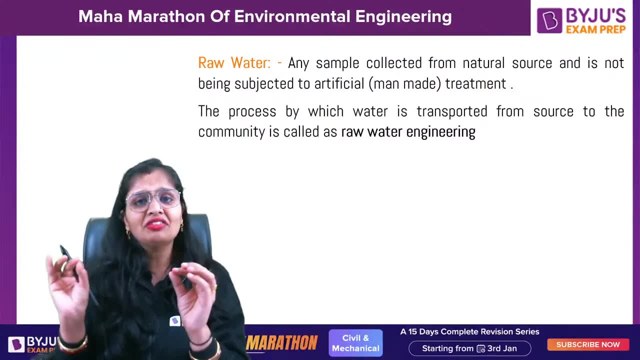 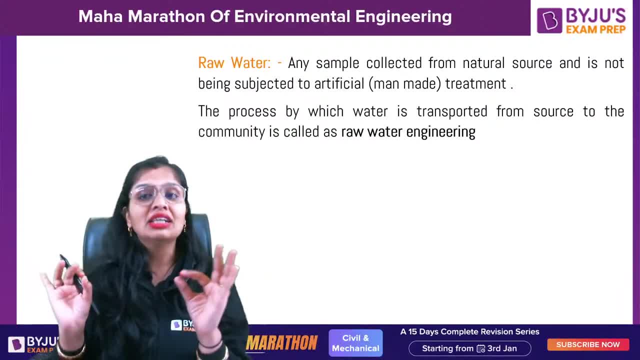 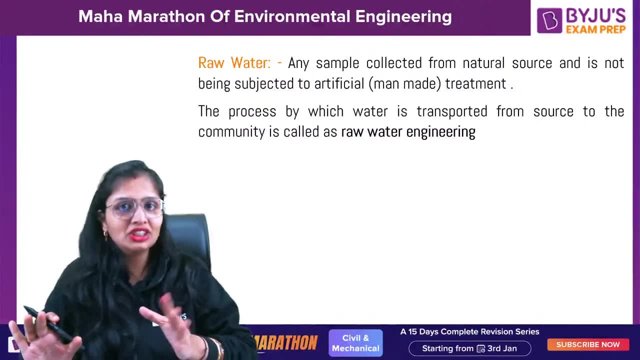 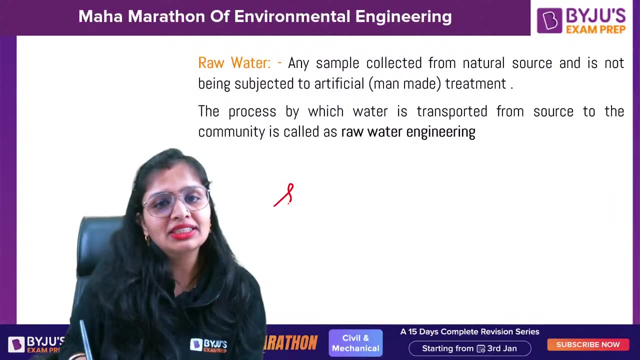 interfered by the humans. that means the manmade interference should not be there. Okay, So that is known as raw water. That s why, when you studied the first part, it is treatment of raw waters, sources of raw water. Okay, Now the portion comes: the whole process. 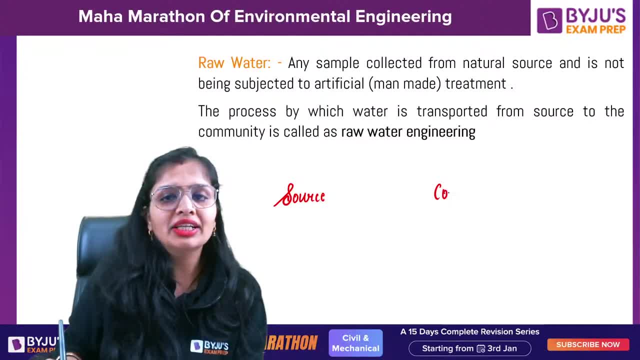 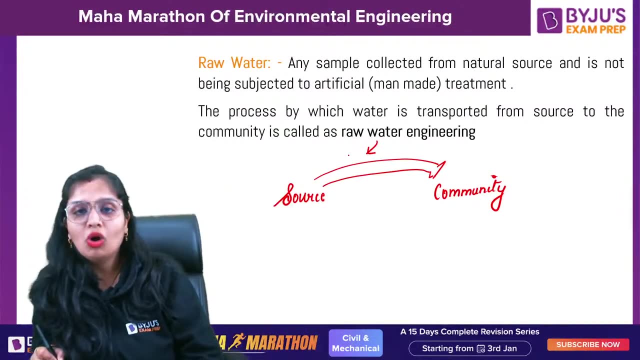 ths is the source. from the source the water is transported to the community. so the whole process, from where the water gets transported from source to the community, is known as raw water engineering. so it's very much important to understand what you mean by raw water, that is, that sample which 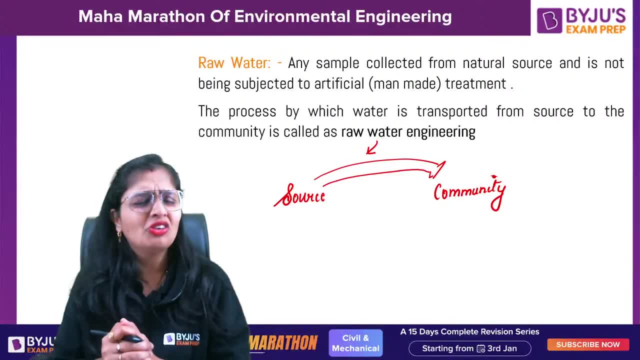 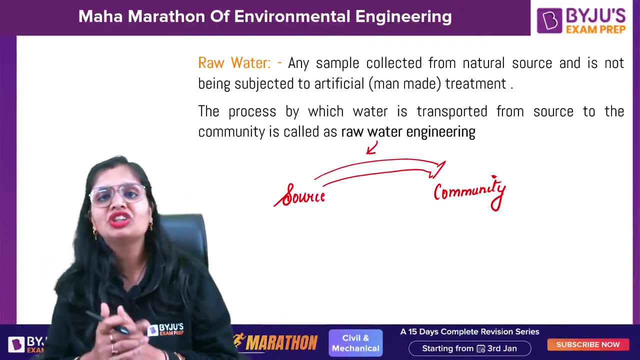 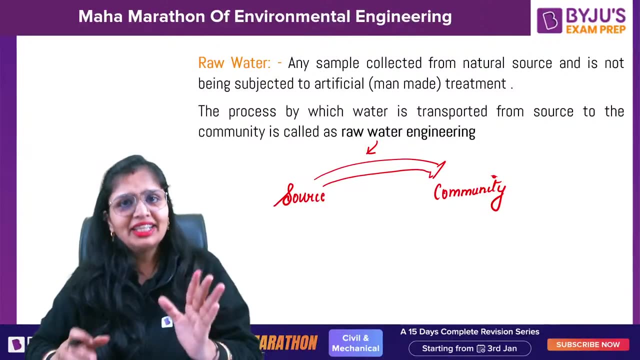 is connected, collected, and it is not treated because of a, because it may be pure, okay, then no treatment is required, and if it is not pure, that we will check how much treatment is to be given. now the next question comes. now the next question comes. tell me, is it possible specifically, 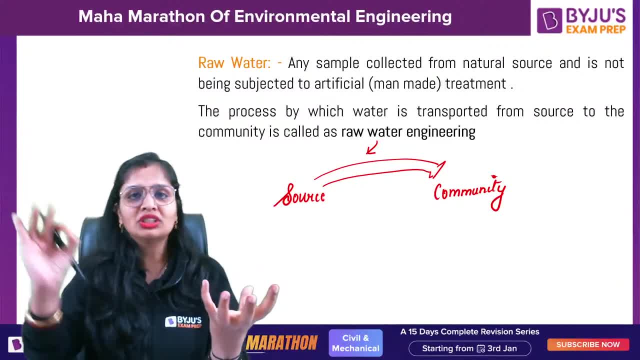 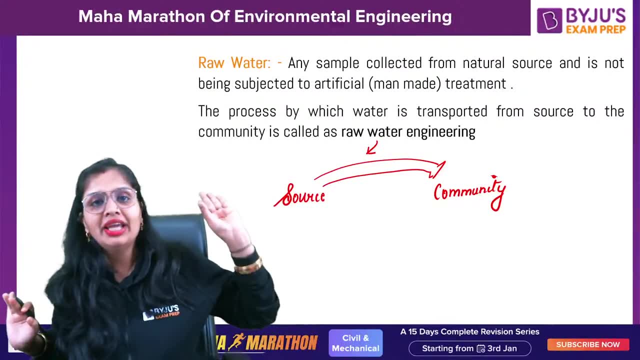 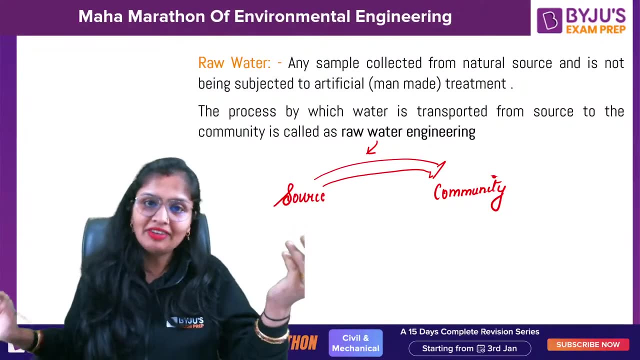 in india that whatever water you get from the source is pure, you don't need any treatment. is it possible? i'm asking on majorly basis: say yes or no. yes or no is it possible? is it possible? is it possible that we get a water from the source which is 100 pure? obviously no, everybody knows. that is the 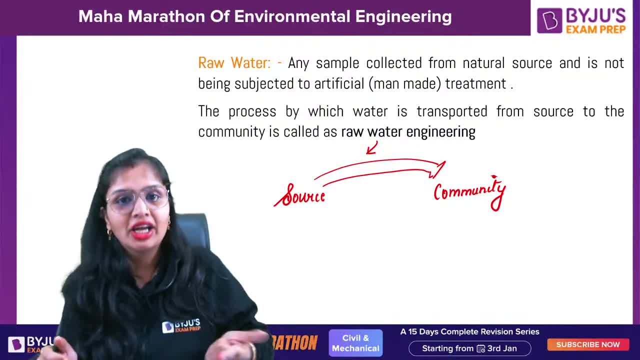 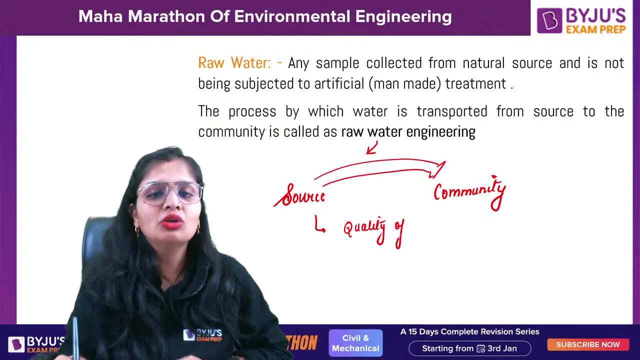 reason. see, if you study something, you should know why we are studying it. so, from the source, first you will check the quality of the water. once you check the quality of the water, then you will go for the treatment of water. okay, so that is the reason we study in this sequence. but the question 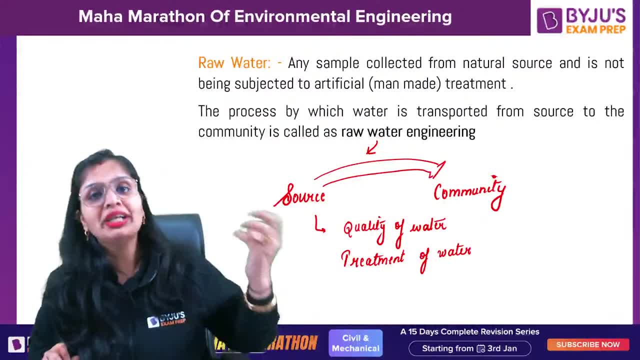 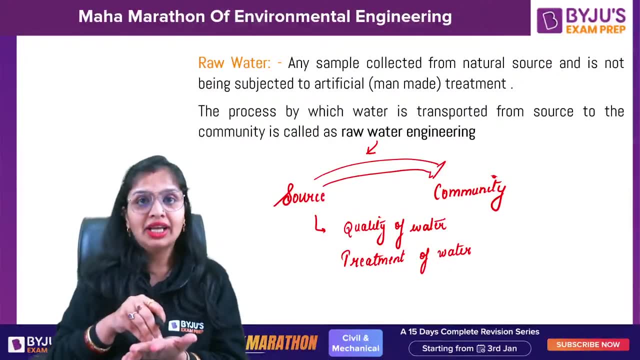 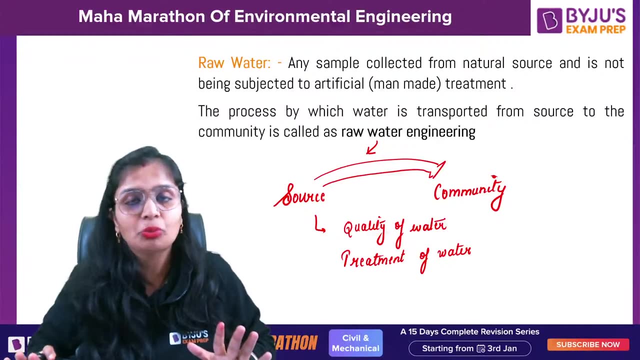 how much? how much water is to be taken? based on that we will select the source. so first i want to know that. how much water is the demand of the people, the demand of water? i have to calculate. that is the reason the first chapter comes out to be water demand. now, quickly. this was the basics. 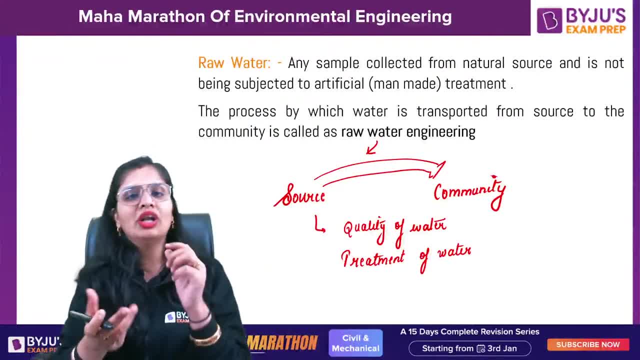 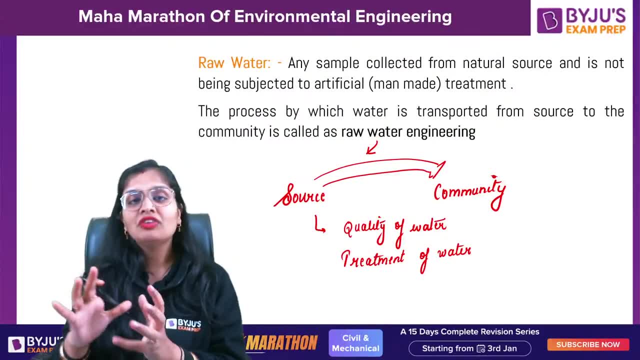 that yeah, source to community, the whole process, quality of water treatment, distribution- all these comes under raw water engineering, in that first of all, when you select the source, you have to think that if i'm selecting this source, will it be able to fulfill the needs of the people. so first you have to calculate the 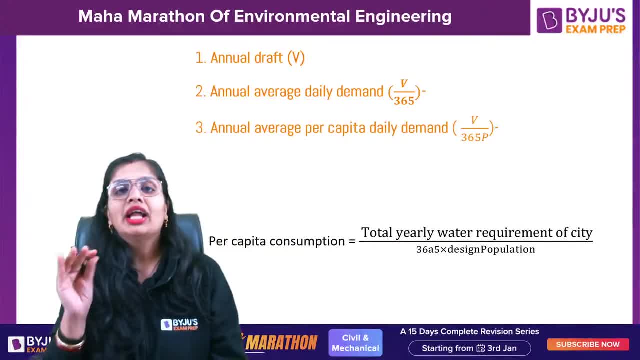 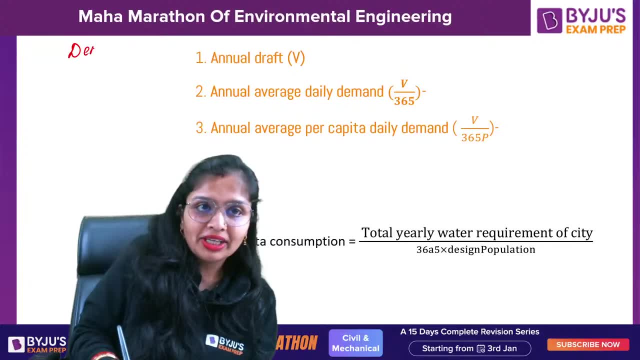 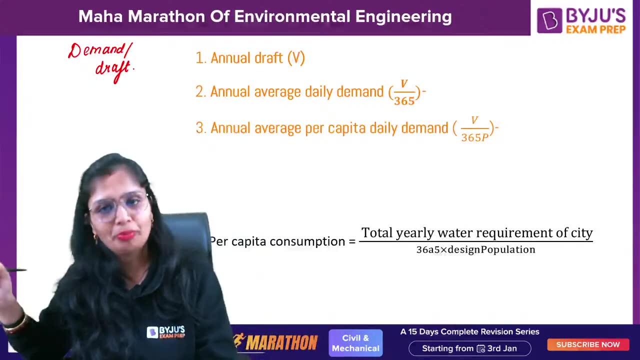 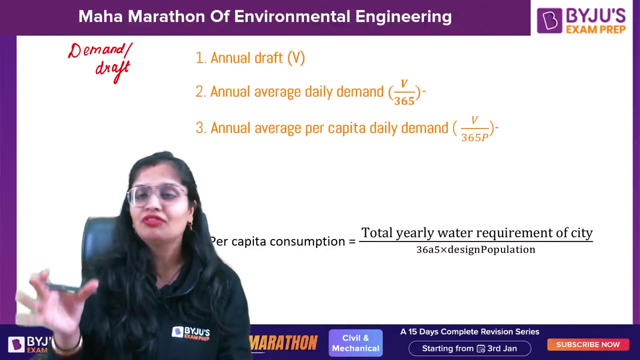 water demand. so the topic comes water demand. now, before telling you the method, there are very important things which you should know: demand, in the case of water demandェand driver- both are same. so generally till now they have asked questions long back in this topic. But you cannot say that they can't ask questions because if you see the mechanical paper, they were asking questions last year from untouched topics. 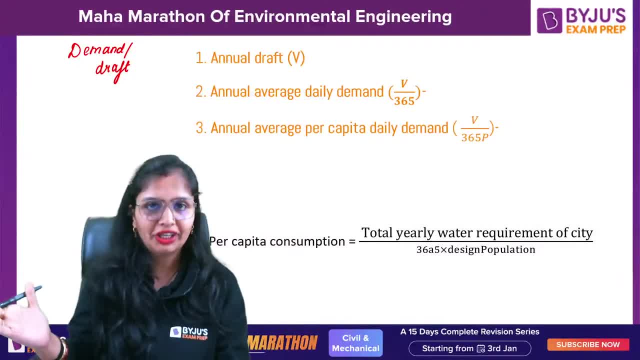 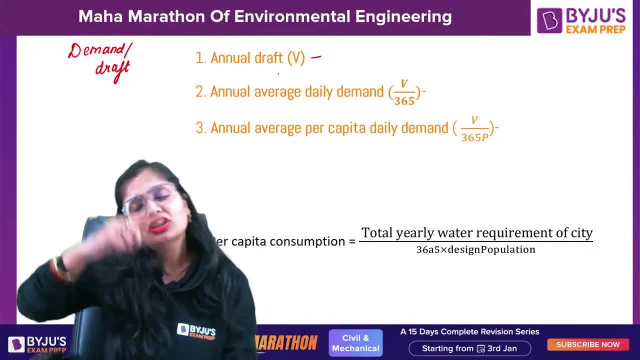 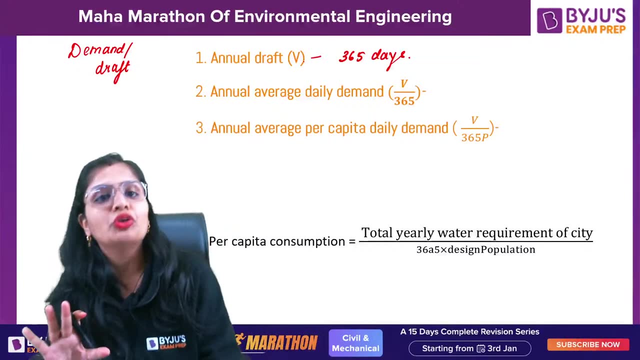 So similarly GATE can do for environmental, for civil engineering also. OK, so annual draft, or you call it annual demand: It is the yearly water requirement for the whole year, for the 365 days. How much water is required in terms of volume? 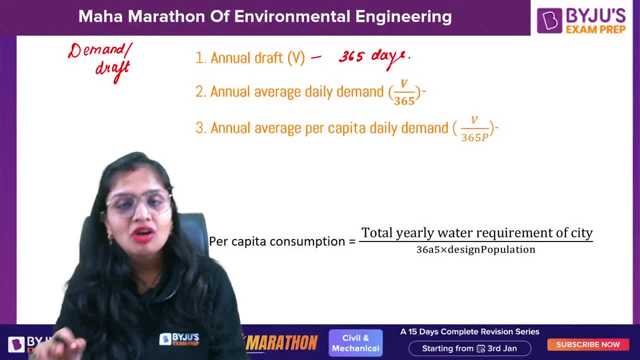 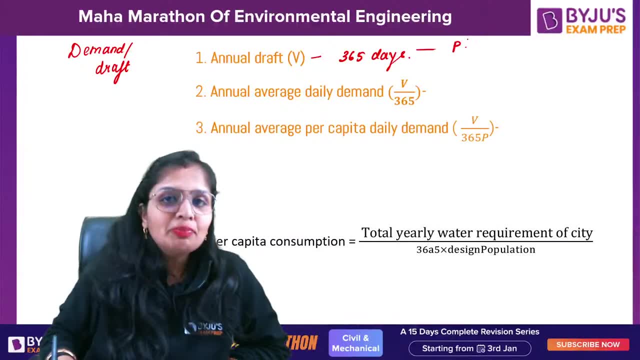 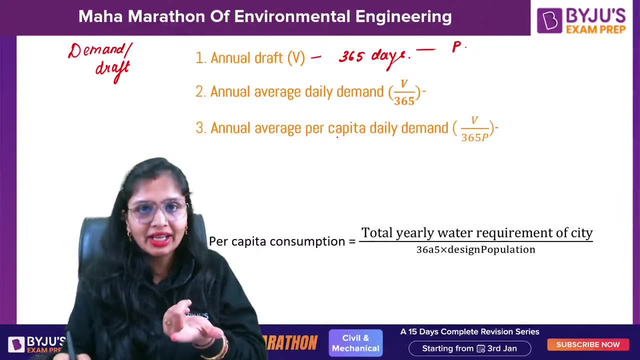 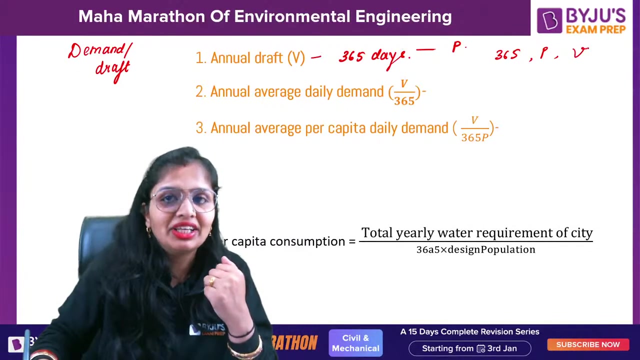 That is known as annual draft for the population P. Now, annual average daily demand for that population, P: how much will be the water demand for a single day? Daily means what A day. So if for P population for 365 days for P population the demand is V, 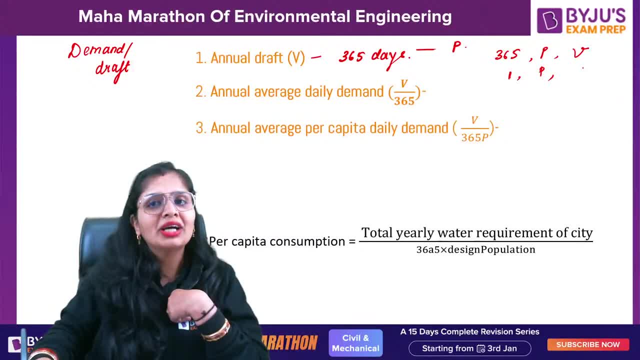 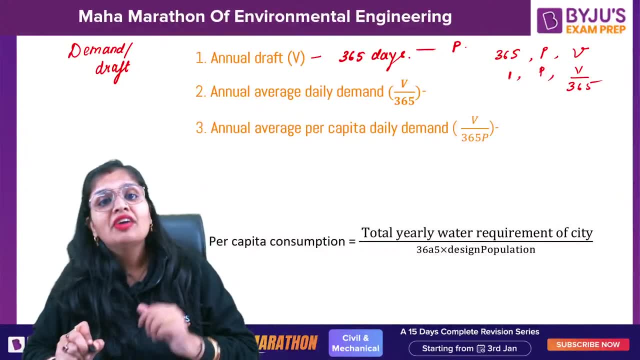 So for one day, for P population, the demand will be: how much V by 365.. Just applying the unitary method. Similarly, similarly, when you say annual average, per capita, daily demand, capita means person, but they can give you per capita per person per head. 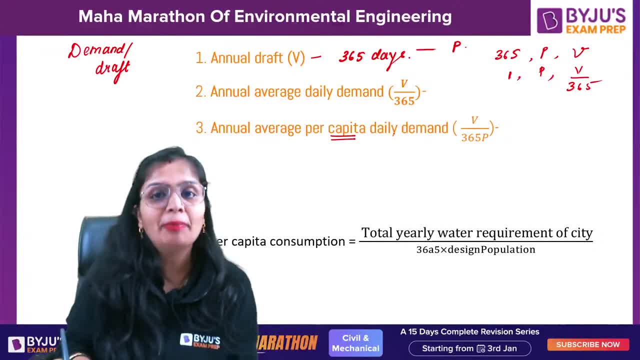 All means the same. So annual average per capita daily demand: That means one person on one day requires how much quantity of water or what is the demand of it. So one person one day, One person, One person will require how much water. 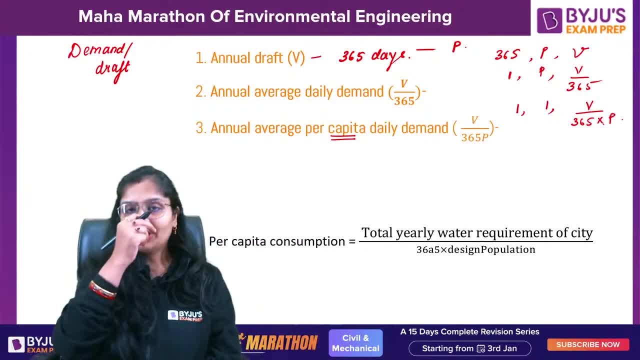 365 into P. Okay, So that is the reason the per capita consumption comes out to be V upon 365 into P. V is the annual demand of the population. P V by 365 is the total demand of the population for a single day. 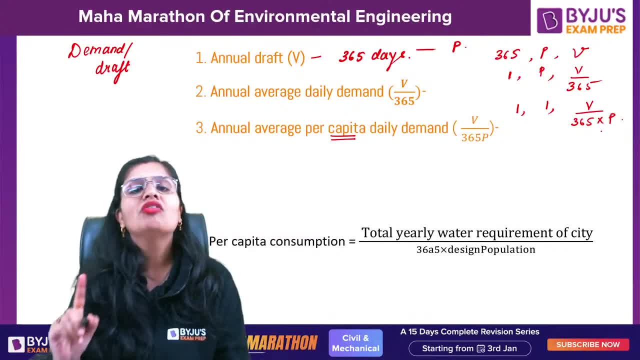 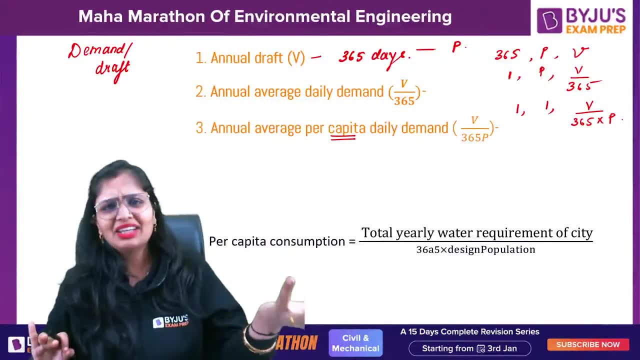 And you divide it by the population, You will get the demand for a single day for a single person, Just like whenever you. basically. when you take milk, you say that one liter milk, two liter milk. When you take rice, you say one kg, 10 kgs, quintals tons. 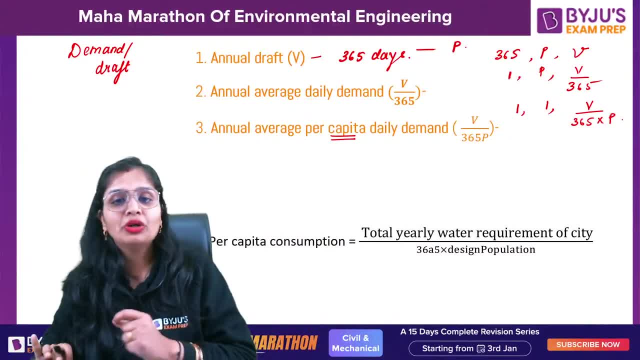 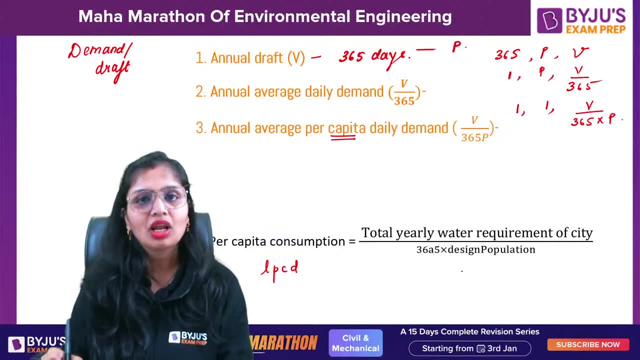 Similarly, when you want to report water demand, you report it in terms of LPCD- Liters per capita per day. Okay, So this is in short. we say LPCD. This is the official denotations. Okay, So that is what is written here. 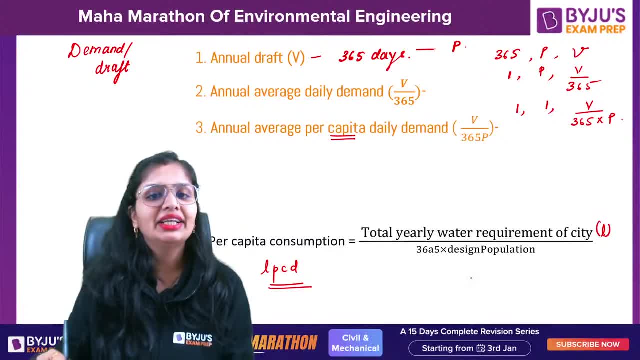 Total yearly water requirement. This will be in Liters 365- 365. That is, when you divide it by 365, you will get get for one day, And when you divide it by the population, you will get for per person. 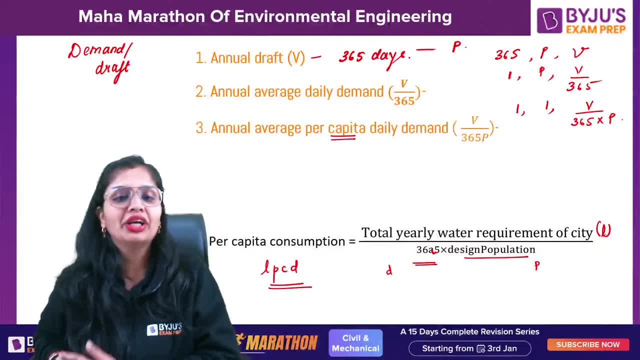 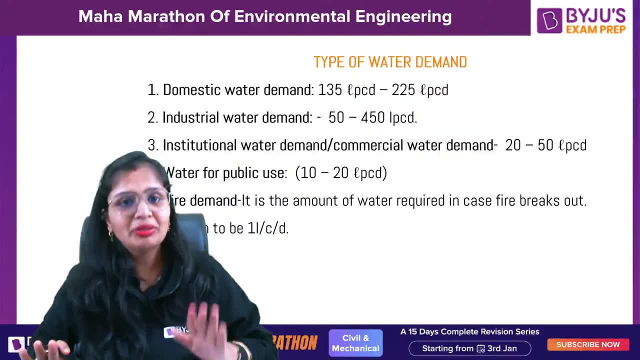 So per capita, per capita consumption is reported in terms of LPCD. Okay, Now let's be quick. These are the demands. have not been asked, but they can ask you in terms of statement, wise portions, or they won't. They can ask you in the following portion: 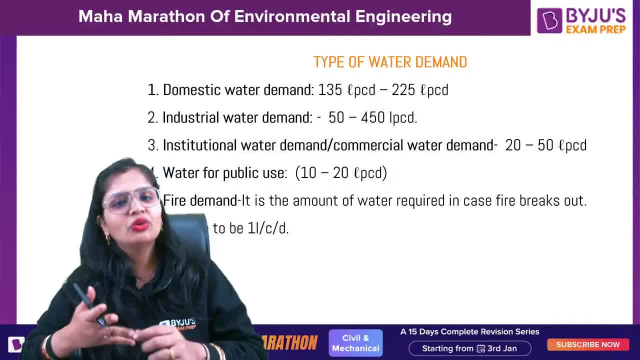 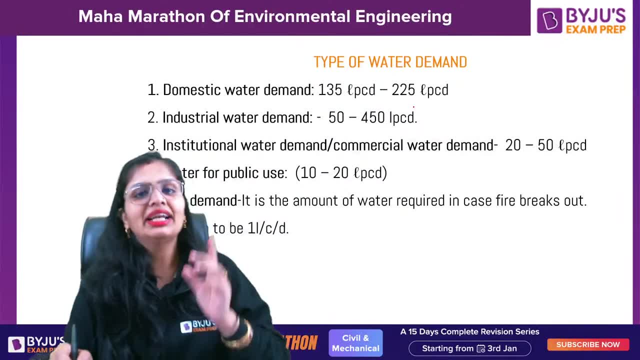 Domestic water demand: The water which is required for drinking, Cooking, washing. This is known as domestic water demand. It varies from 135 LPCD to 225 LPCD. Let me tell you one thing: 135 LPCD is for low income group and 225 LPCD is for high income group. 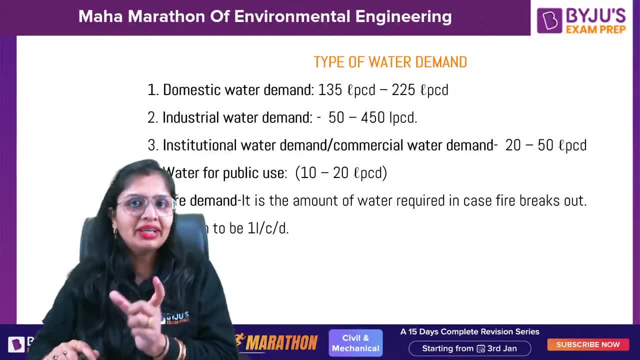 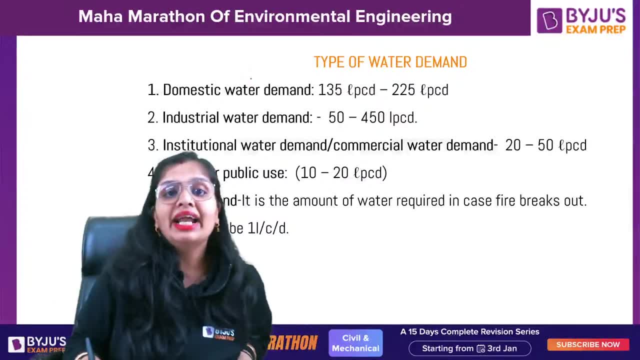 So we say LIG and HIG. Okay, Why I'm telling you these basics things? because in MSQ generally they ask you: statement wise quotient, So you should know this. Then industrial water demand: It varies from 50 to 450.. 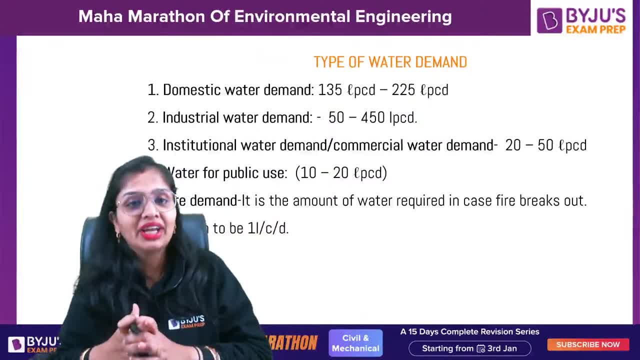 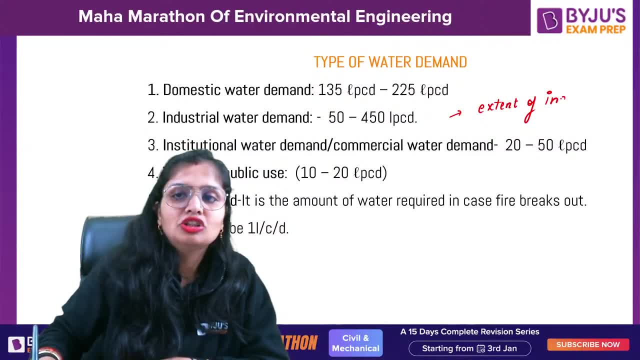 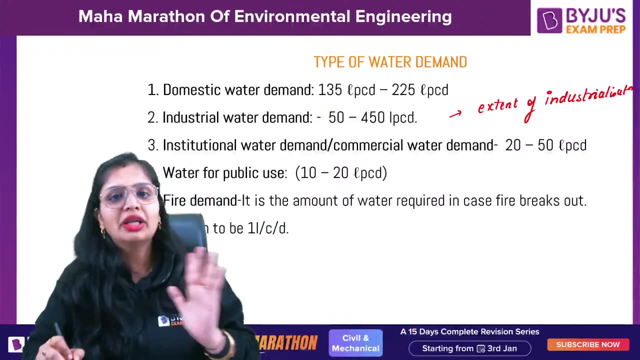 Now you can ask me, ma'am, why there is a huge gap in the race? because it depends upon the extent of industrialization: Smaller industries, bigger industries, Some industries require more water, Some industries require less water. So it depends upon that. 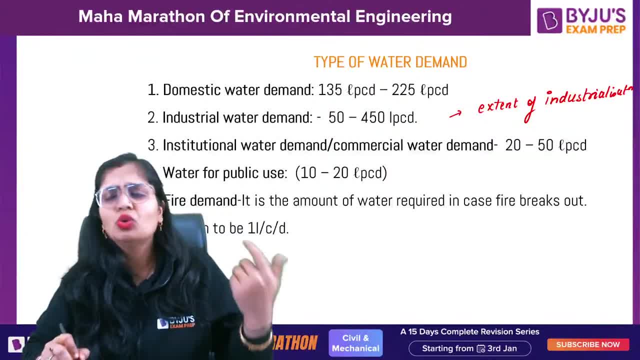 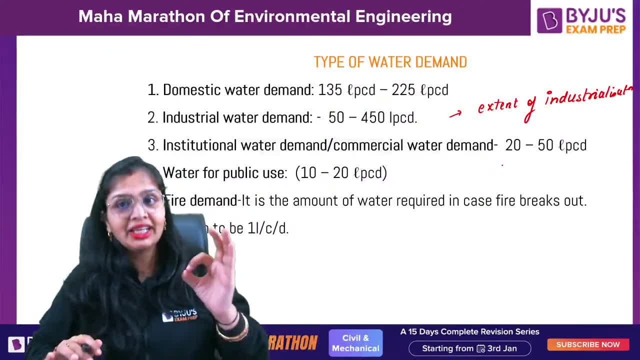 Institutional water demand, like coaching centers, You can say schools, hospitals. So they require 20 to 50 LPCD as the water. Now you will say that, ma'am, it is mandatory That 20. Or 50. This will be the range. 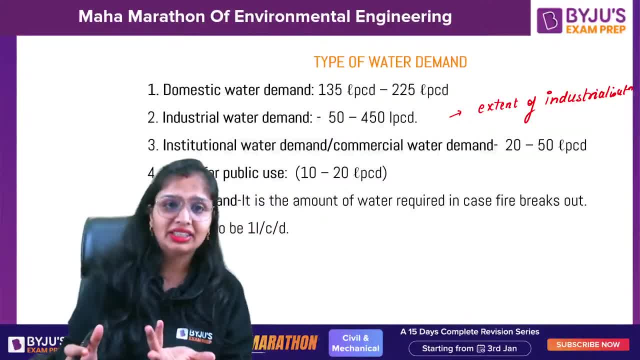 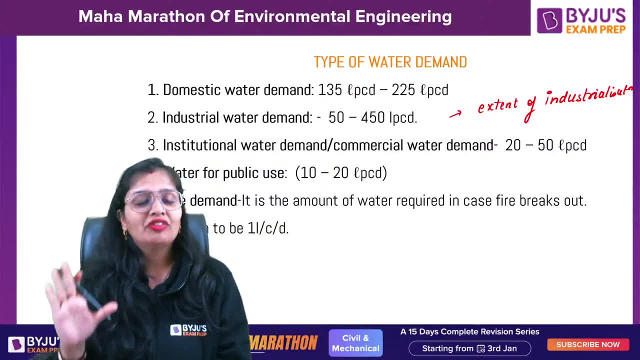 No, It can be greater than this, It can be lesser than this. Okay, Water for public use, That is, 10 to 20 LPCD. Then coming to the important one: Water for public use, If you want to know, like when you wash the roads and all. 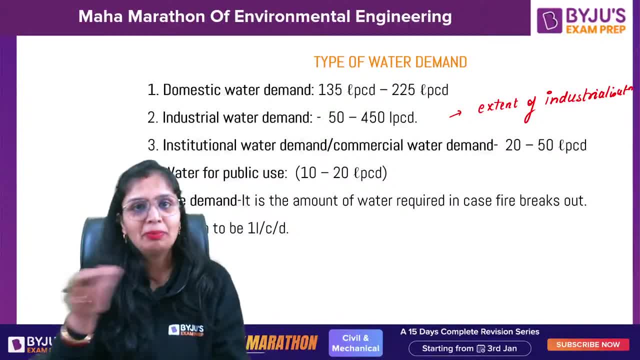 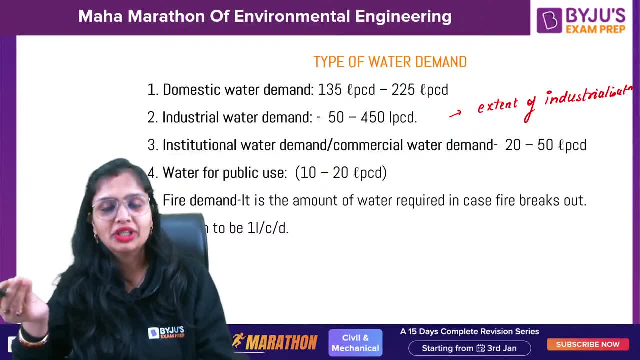 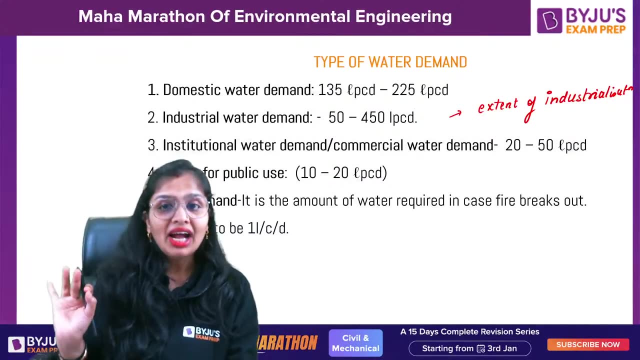 For that purposes also water is needed in public parks and all for basically watering the plants and all. So for that purpose water is needed. So that is the reason: 10 to 20.. LPCD now fire demand. important fire demand is if certainly a fire breaks out in your city. 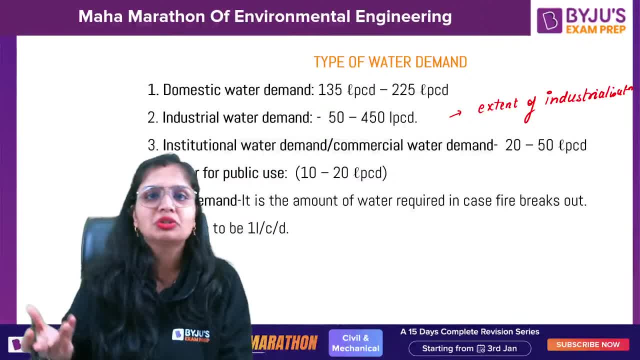 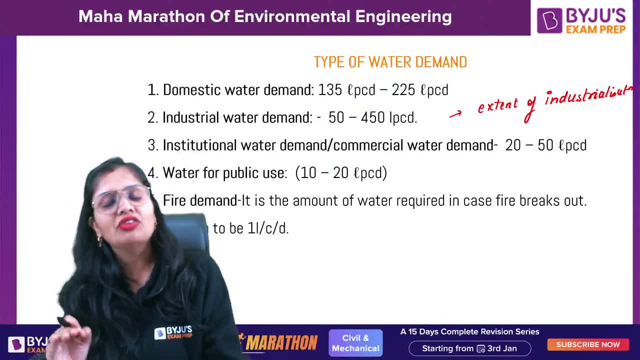 So you will be like: okay, fine, We'll open the tap and we'll bring the water. notes practically not feasible. You have to store a certain amount of water. So the amount of water needed for fire demand is very minimum. That is one LPCD. 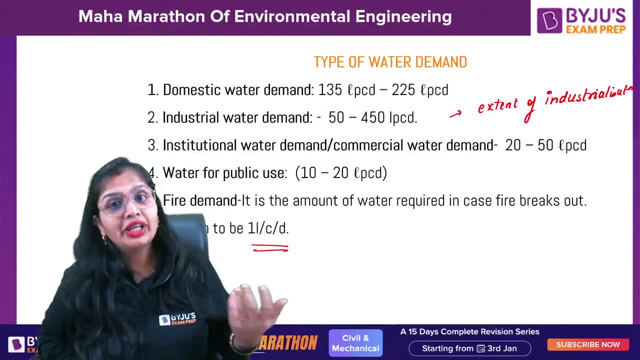 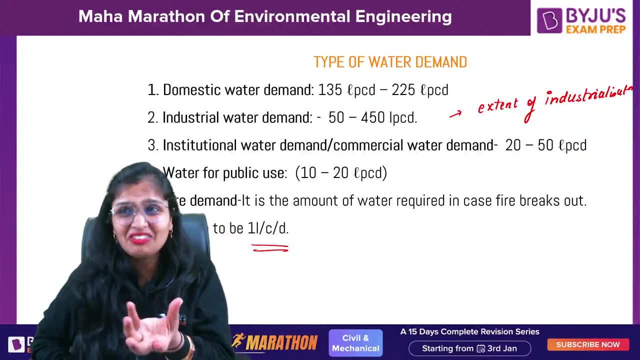 Now you will say: ma'am, such a less quantity of water. You're telling: domestic demand, is this much industrial demand, is this much in fire demand? So let's one LPCD. Can you believe one LPCD? Yes, because the outbreak of fire does not happen every time. 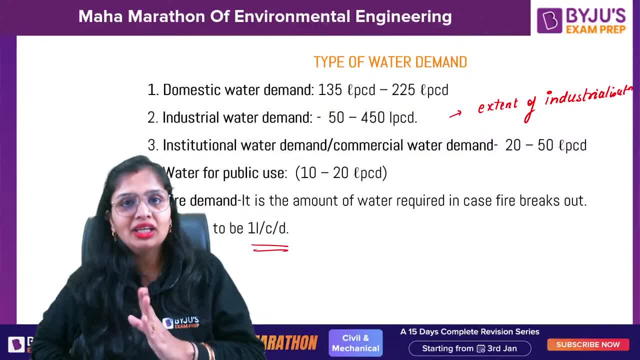 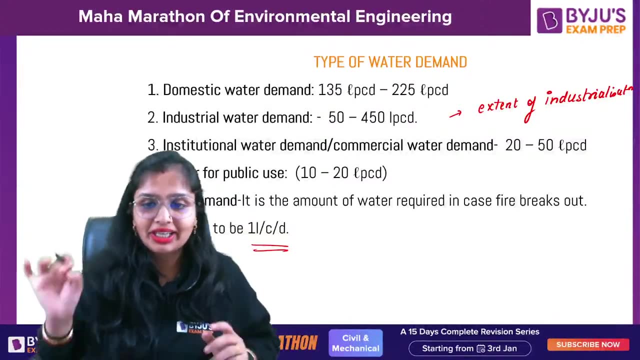 Okay, That's the reason you should know. but there are empirical formulas which they can, basically they can give you which are the formula to be used for fire demand and these are empirical formulas. Whenever I say empirical, empirical means units, observation based formula, and units has to be taken care of. 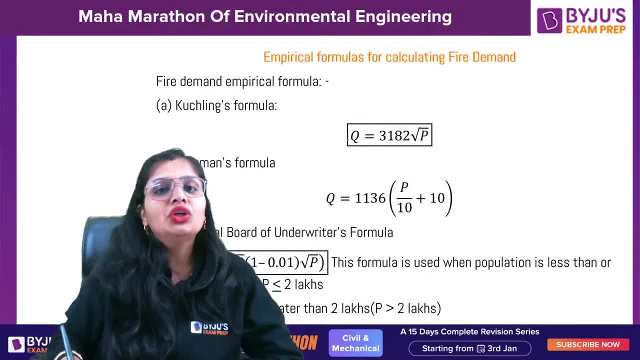 So first is kuchlings. formula Q is equal to 3182 root P. Let's be quick in this. everywhere, The discharge which you will get will be liters per minute. The population will be in thousands. Don't worry, We'll do a numerical also. 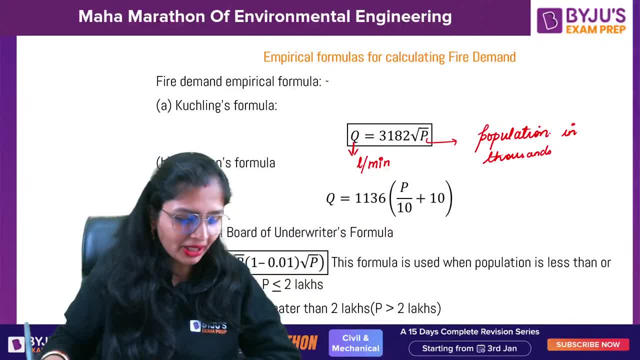 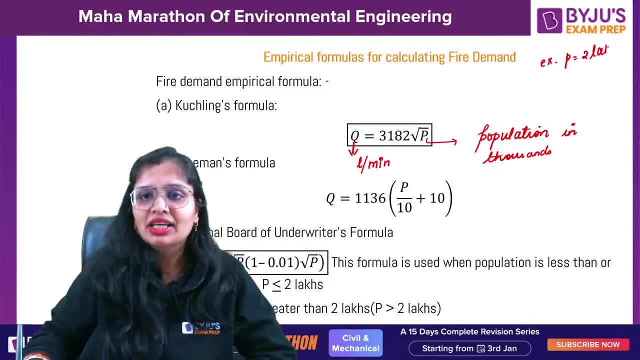 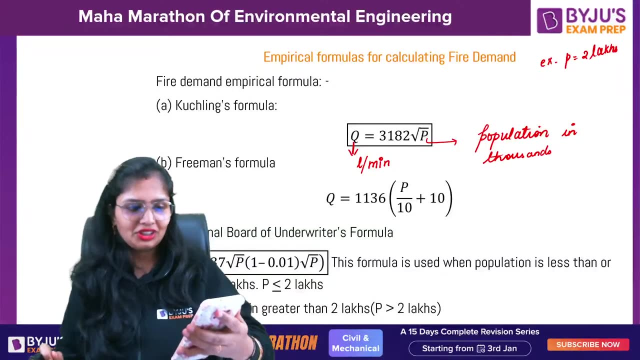 Population in thousands. So, guys, let's be quick. Let's, if the population is, let us suppose, 2 lakhs, So what you will substitute here? You don't mind. last words, I'm not visible. Where should I shift If I'll shift here? 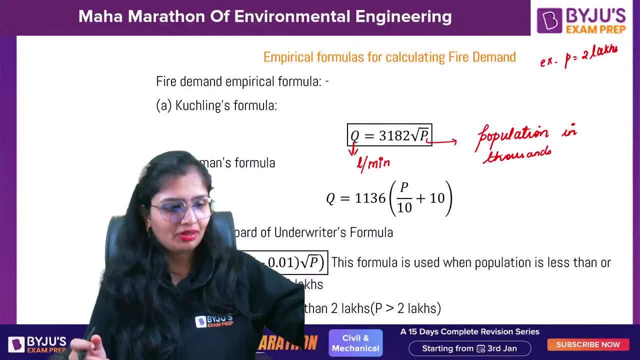 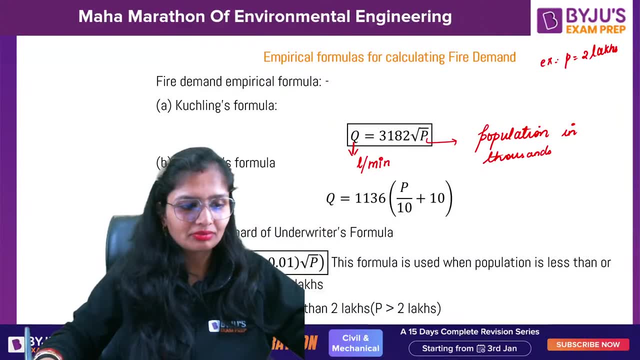 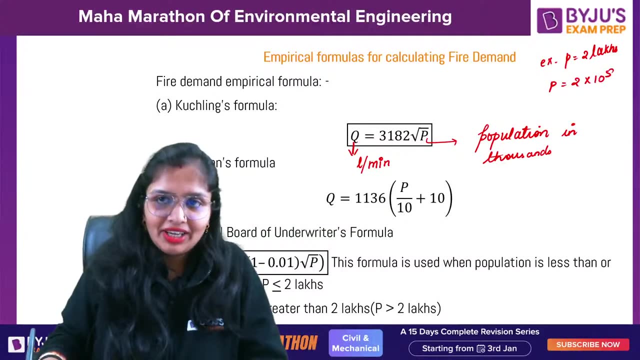 Okay, Now is it visible. Let me check it out first. 200, how I opposite. I did opposite. P is 2 into 10, raised to power, 5 divided by a thousand. So this will become 200. Okay. 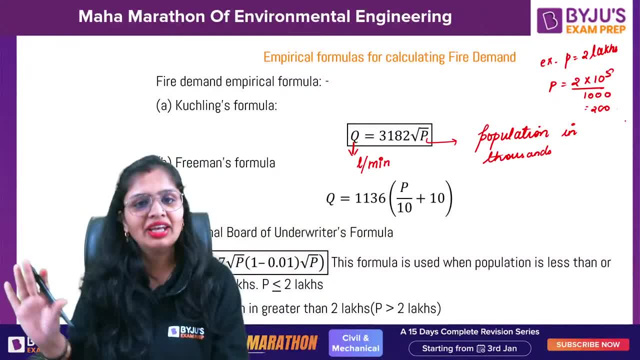 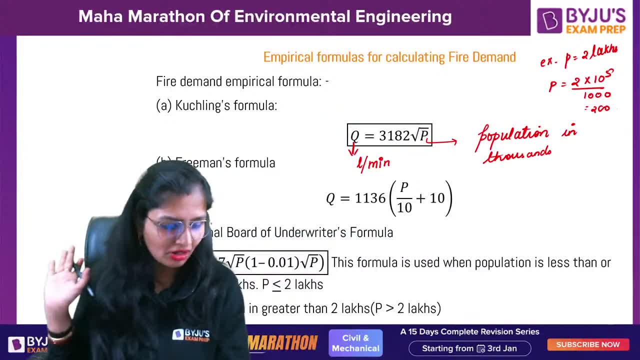 So you have to To substitute here to a hundred. So everywhere in all the formulas you have to do this. Now, one doubt which you guys have is population in thousands. Yeah, already substituted. fine, Now the one question which I wanted to ask you and basically tell you. basically, in some books you find they write it as 1: 1, 3, 5, P by 5 plus 10.. 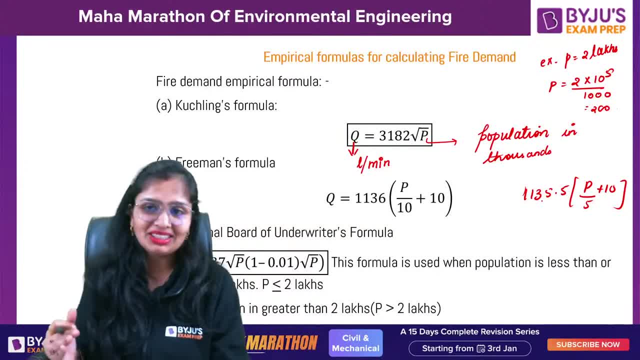 Sometimes they write 1, 1, 3, 6, P by 5 plus 10. See, this is observation based, So ambiguity will be there. But generally when You use 1, 1, 3, 5. 5, then you use P by 5, general basis. 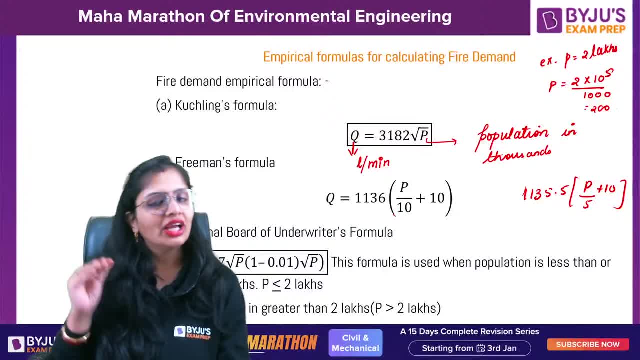 When you take 1, 1, 3, 6, you write P by 10 plus 10.. So actually many students ask me the same thing, So I have confirmed it right now. Okay, Q is liters per minute. P is in population in thousands everywhere. 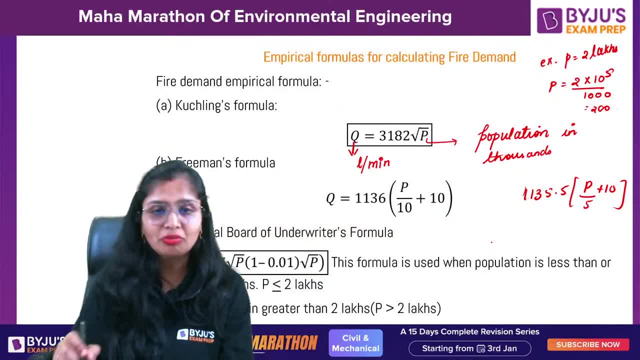 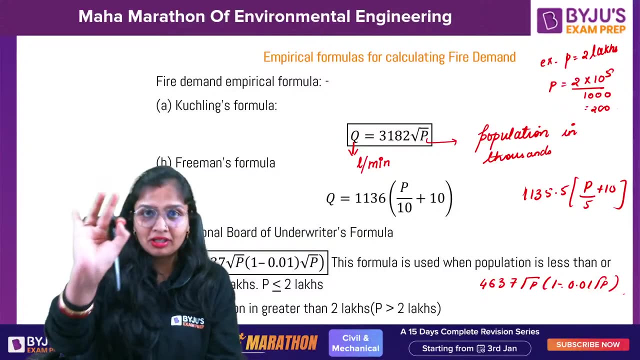 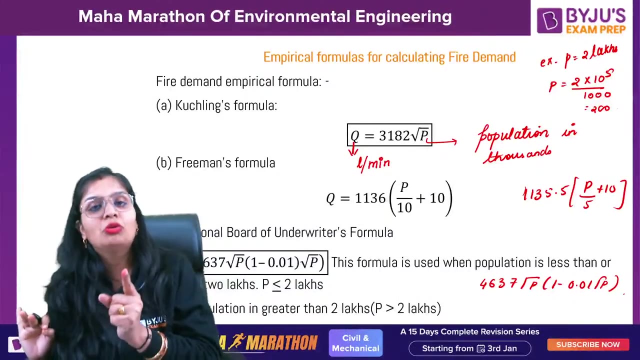 You will get the same thing. National Board of Underwriters formula. This, Alec, I'll tell you this is a 10, 4, 6, 3, 7 root P. 1 minus point 0, 1 root P. Okay, but remember again a statement, wise question, or they can judge you also. this formula is applicable only when the population is less than or equal to 2 lakhs. 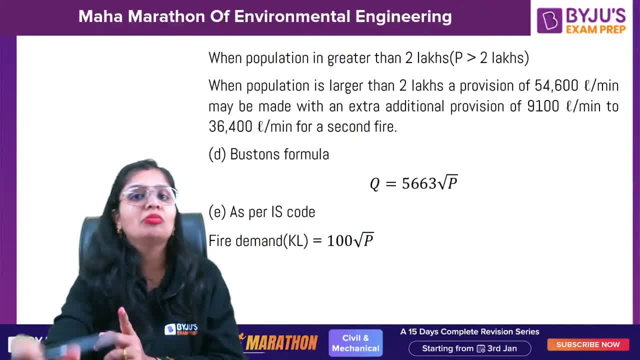 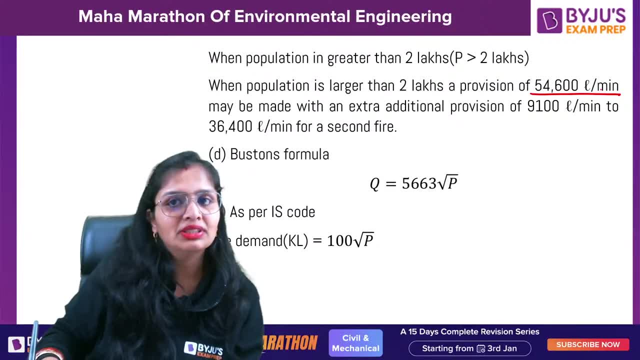 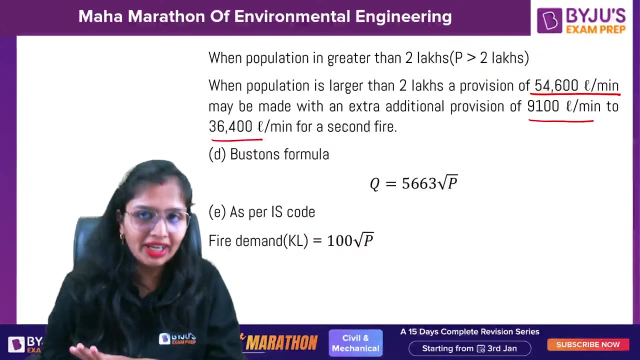 If the population is greater than 2 lakhs, you cannot apply this formula for that. They have generally given you the provision that 54,600- 600 liters per minute will be there. that will be the world demand for Fire. additional 9100 liters per minute to 36,400 liters per minute will be there in case an outbreak of second fire takes place. 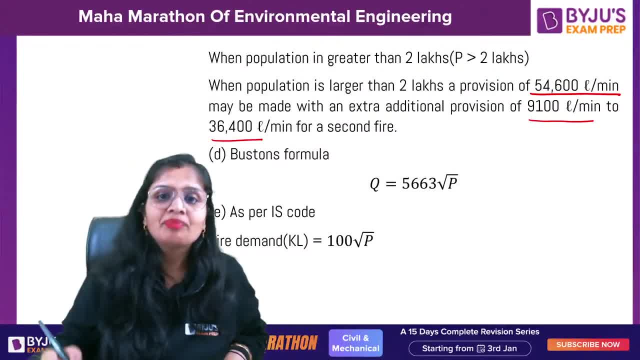 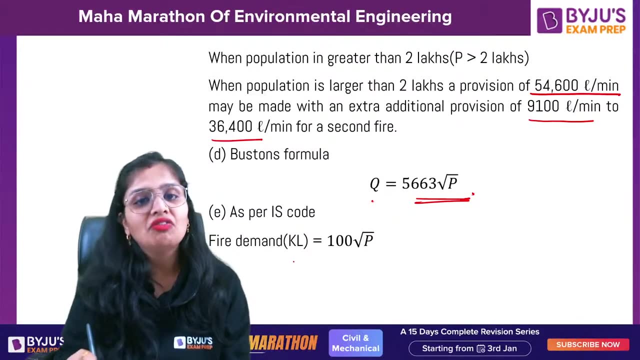 Okay, again a statement, wise thing They can ask you guys. Okay Now Buston's formula: 5 double 6, 3 root P, where discharge is in liters per minute piece, the population in thousands. last, This is important one, If you go through the Indian standard codes, the fire demand. 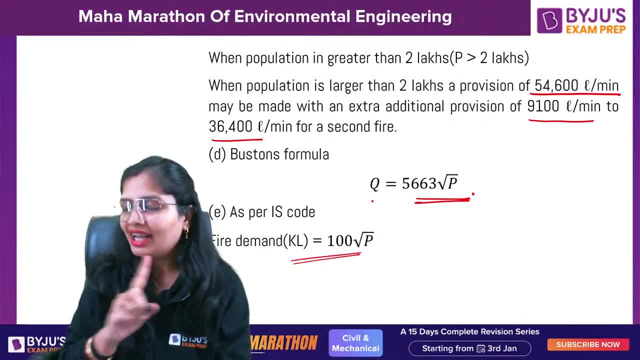 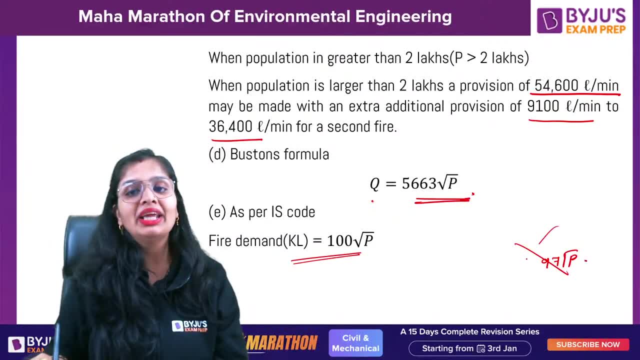 Which you get is in kilo liters. Remember this, never, ever. They have asked till now. So if in books, if you see the old books, they have written 97, root P. This was prior to 2012 for the modified version. 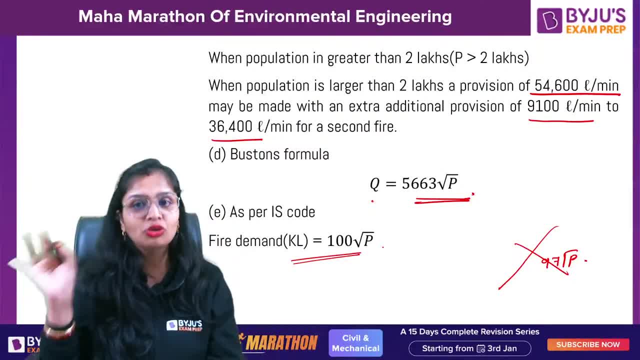 Now you get 100 root P. So if you study from the old books gets your fact check better, because now it is modified. So as far as code the fire demand comes out to be 100 root P here the fire demand, You will get it in. 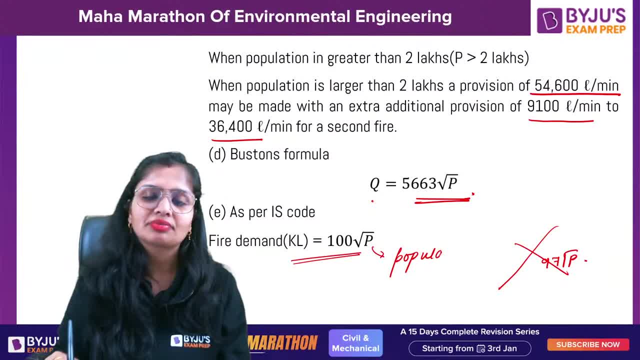 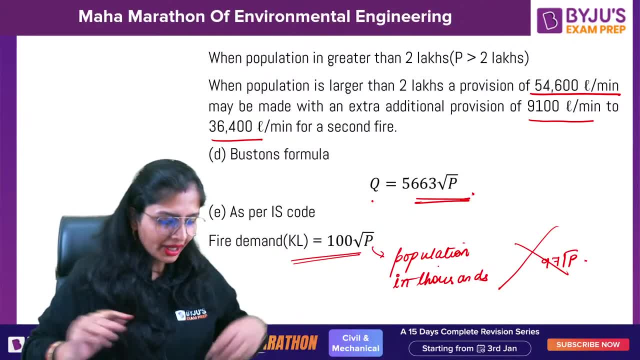 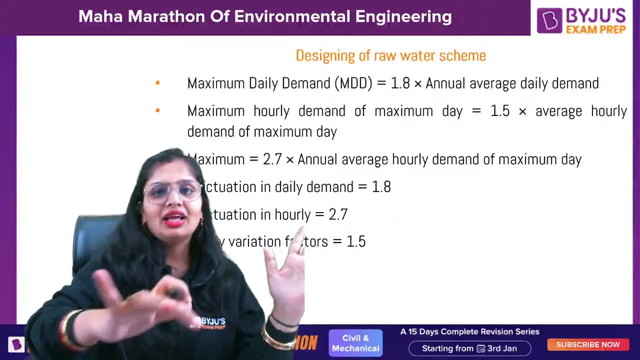 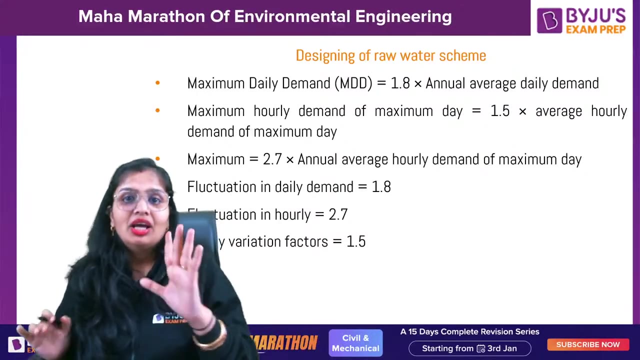 Kilo liters and the population will be in thousands. Okay, double put formula, Okay, fine. So till here any doubts. Now, this is a very important thing. I am talking about designing of raw water scheme. final, So let me tell you fun. some things like like: 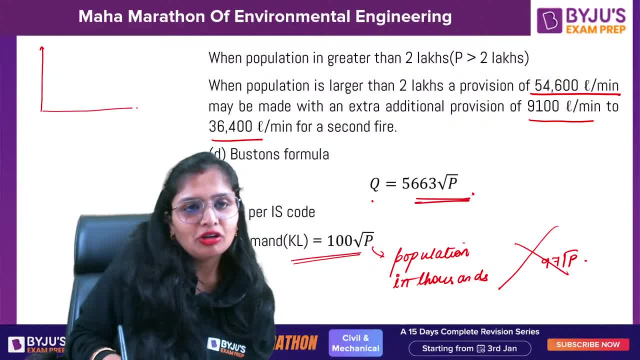 If I talk about generally, if I talk about if the this is the discharge and this is that, so it's. let us suppose it's morning, 12 to 6, 6 to 12, then 12 to 6 pm, Then 6 to 12 pm. 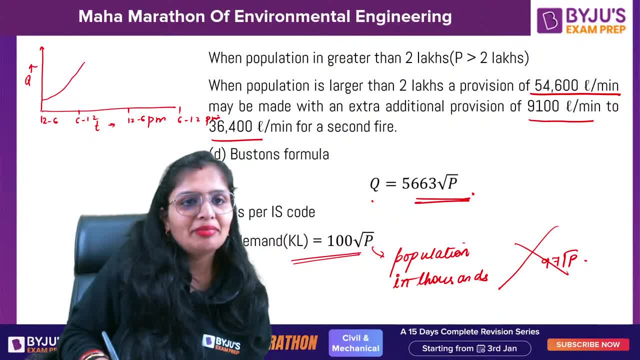 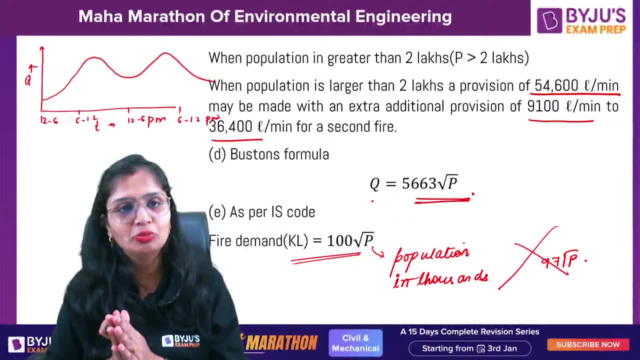 And so on. So, generally, your water demand will be like this time: It will be more than it. This is the time, This is more, and so on, and this varies from person to person. This varies from person to person. Now, I believe that 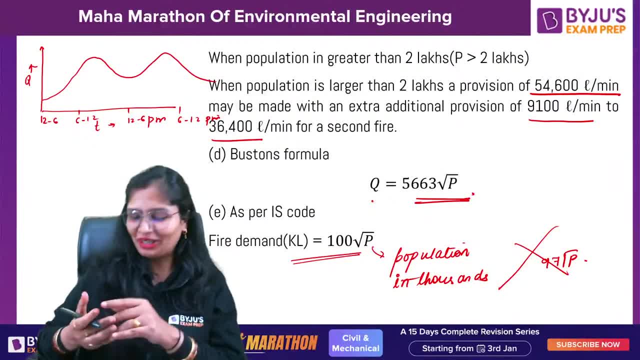 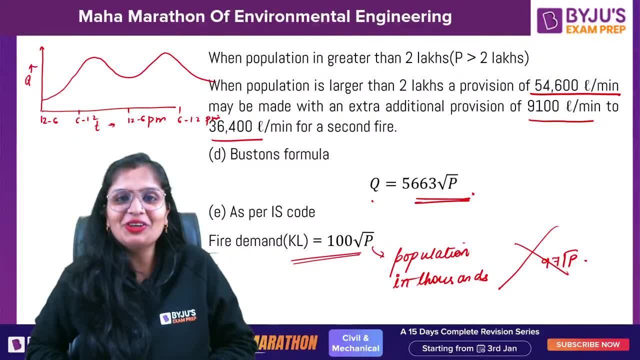 You guys take a bath in winter season. Okay, specifically boys, because generally boys don't take a bath in winter season, Is it? I don't know everybody. So you are saving the water, I know that. so actually, the water demand varies from person to person. 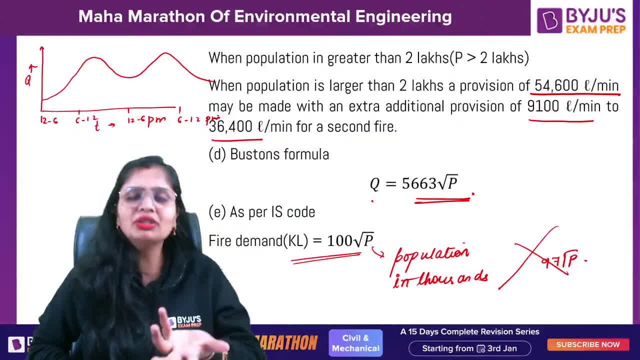 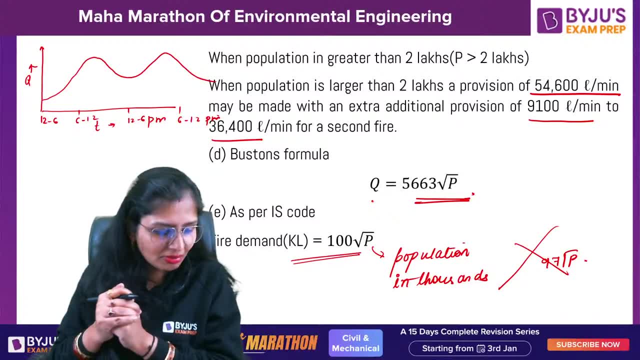 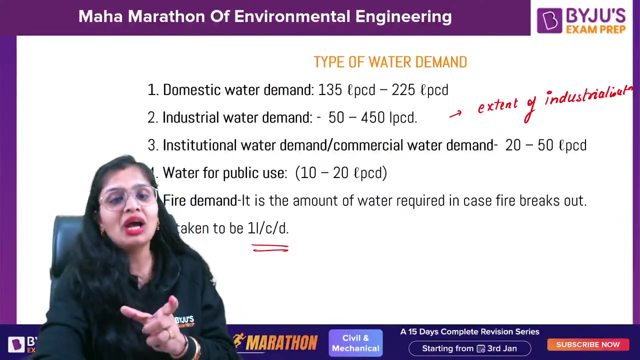 Okay. So now the question comes: if for one person the demand is waiting, what will happen to the entire Man? for hospitals will be no water demand. If there, means, how much such will be a said this water demand better. This is for institutional, commercial fixed value. 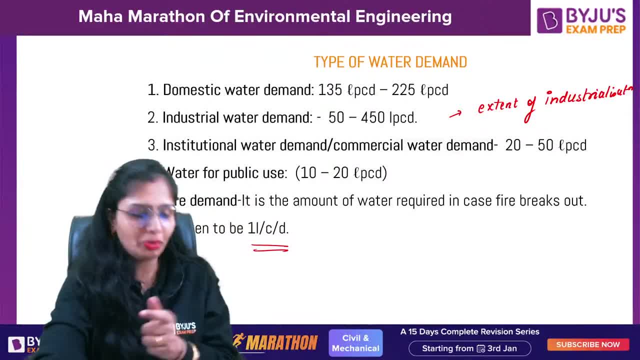 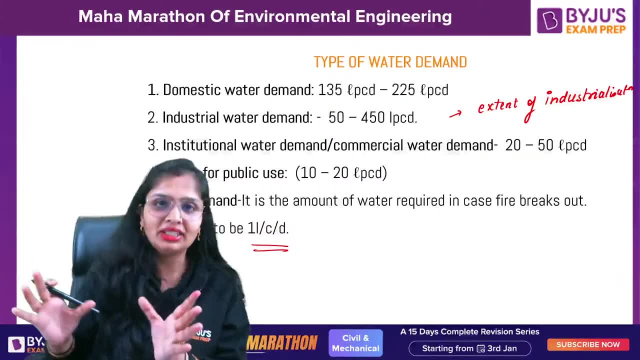 How much it is there, because if you see the code, it is written for hospitals. If you're asking the 50 beds, hundred beds. So if you see the code in detail, it has given for how many beds which are there in hospital. based on then the, based on that, the water demand. 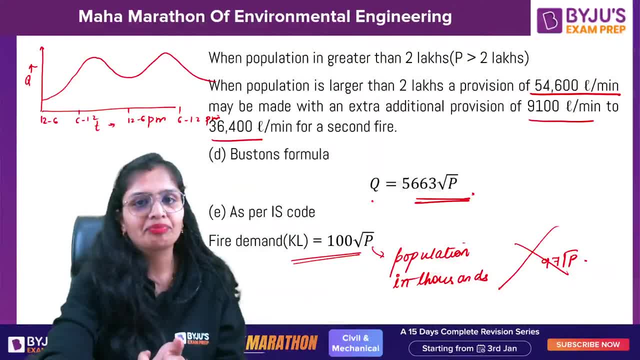 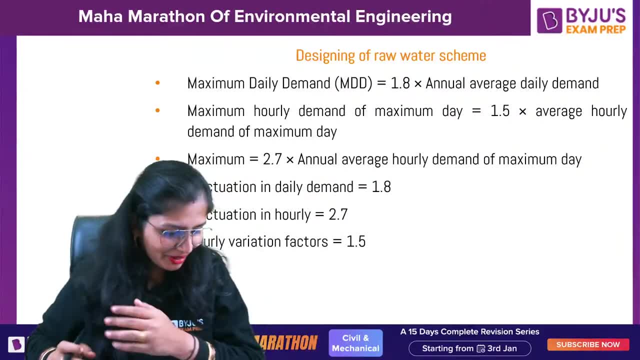 I've just given you a range of it. Okay, If you see the codes, I don't think you need to learn the whole code. But yeah, you can go it. Okay, such will be a minute. We shall add voltage. Oh my God, Arun. 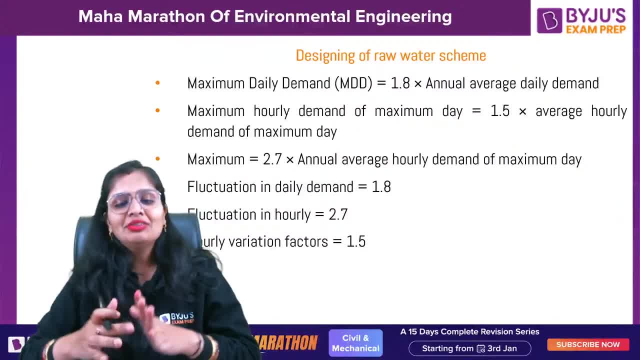 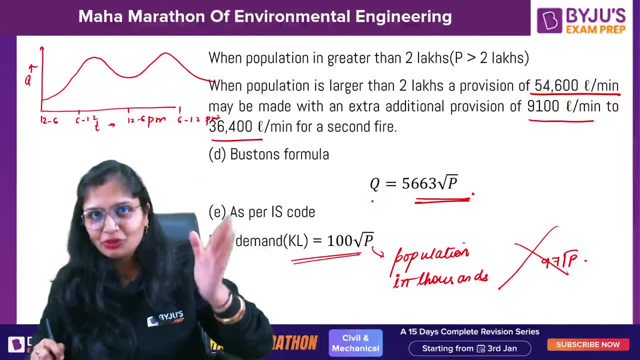 Now you wasted the water, Okay. So now the question comes. the question comes, the demand for a single person fluctuate. like you guys, for today marathon, I also woke up early, Otherwise I wake up at 9. Okay, So what will happen? 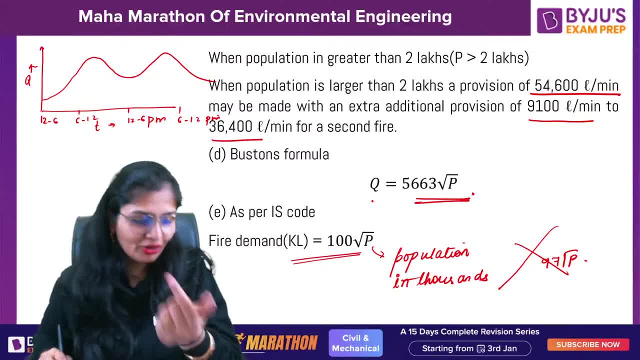 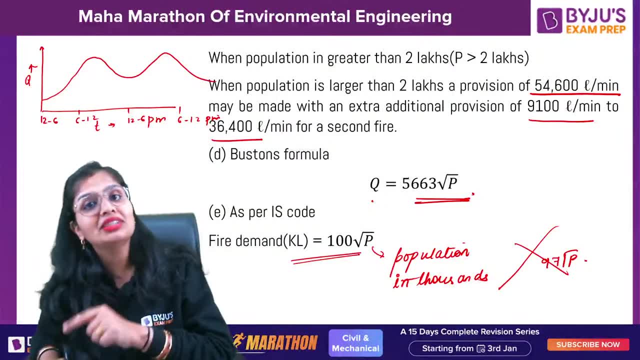 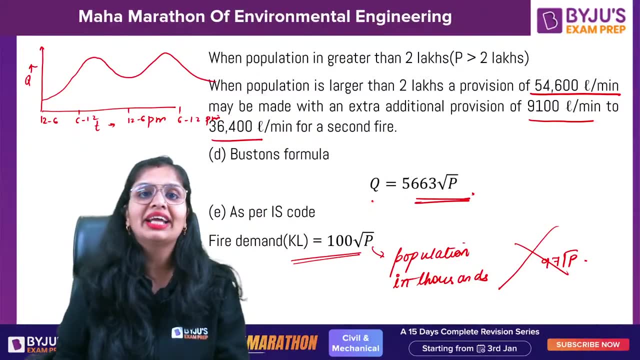 My water demand will Start from 9 am. If Arun wakes up that 7, his water demand will start from 7 am. So person to person water demand is varying and person to person the peak demand also varies. But if I consider a single person, it will not be possible for me to design the raw water scheme. 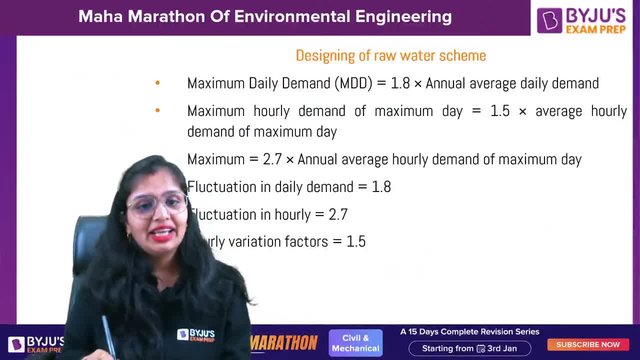 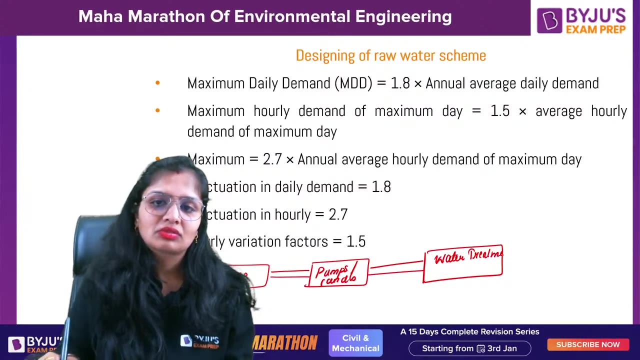 Now you will come on designing. Yes, if you see there is a source. From the source, There is a pipe which takes To pumps and canals. From here It goes to the water treatment plant. From water treatment plant It goes to the service reservoir. 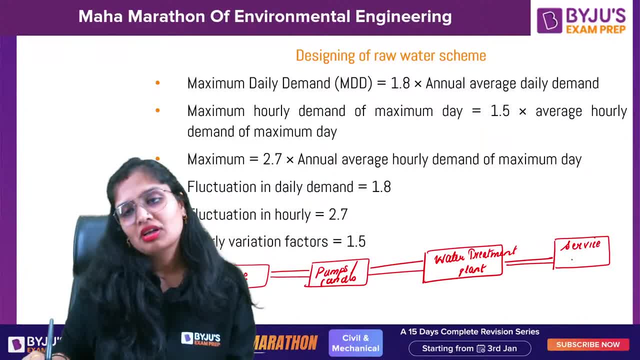 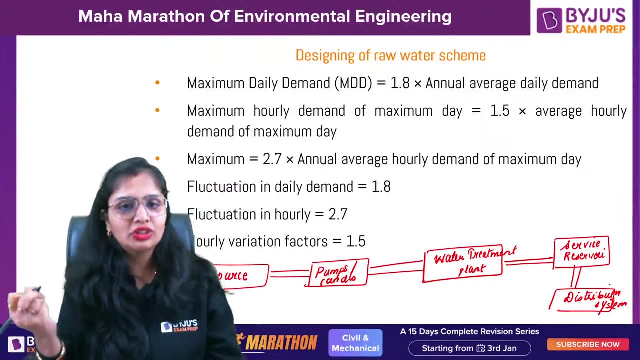 That is paniki tanki in your locality And from service reservoir It goes into the distribution system. So, Basically, guys, you need to design it for all these components. It's not randomly We can use it. No, we have to design it. 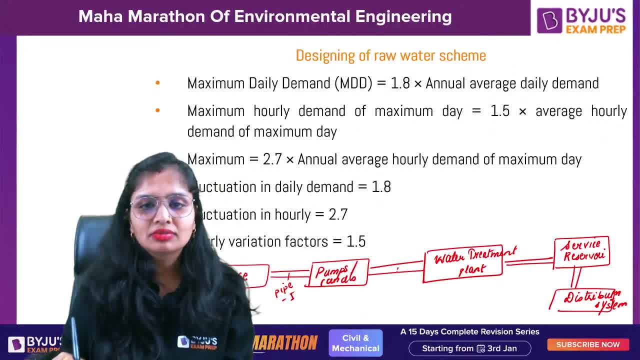 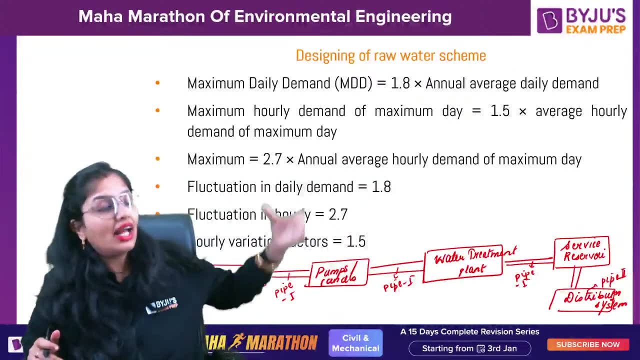 So this is pipe one Piper. So even the capacity of pipes and all this you have to design. You have seen those are. now it is the concrete sewer pipes are also being installed and the normal laying of pipe. So everything is to be designed. 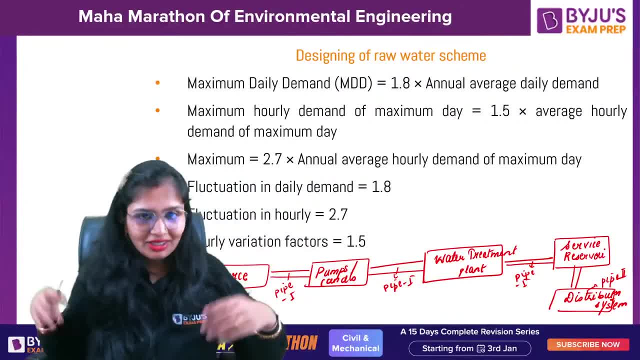 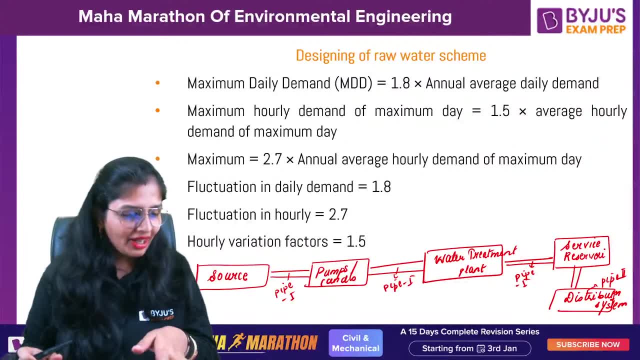 Okay, So To the right. Okay, fine, I'll do right, Is it okay, Fine? So now the question comes. Now the question comes when you design, when you design the source. Now is it visible? Okay, fine, 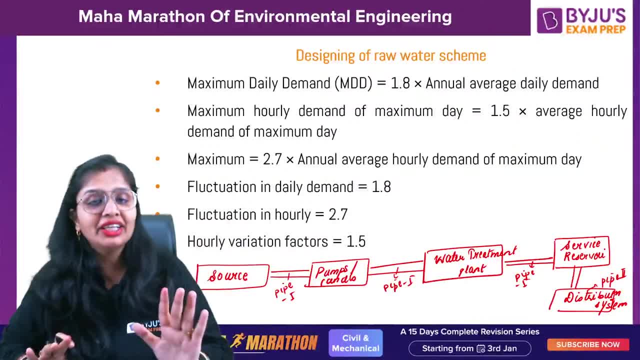 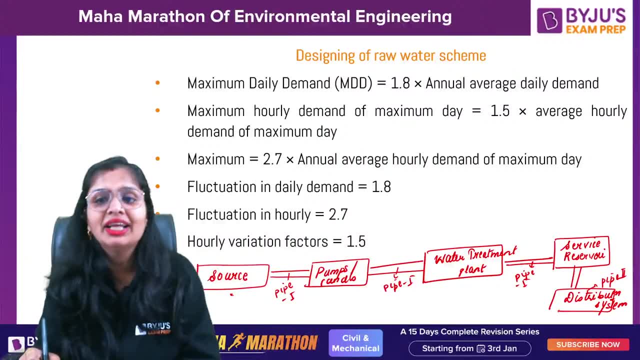 So the source, pumps, water treatment service is the way everything is to be designed. So there are terms which you should know. This is the whole raw water, This whole process from the source To the community distribution system, that is, to your homes. This exactly is the whole raw water engineering. 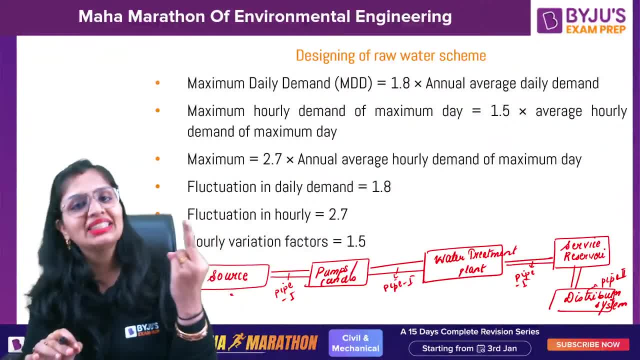 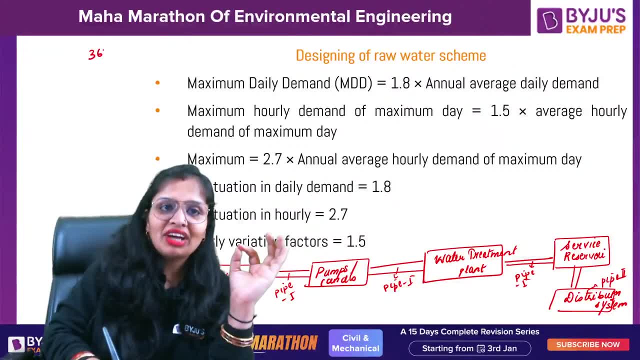 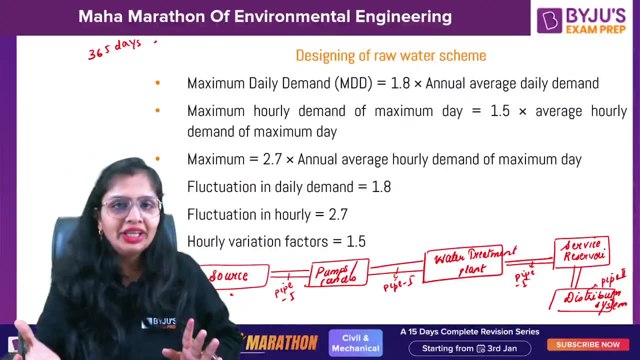 Now comes the question. There are two terms which you need to know: maximum daily demand and maximum hourly demand. maximum daily demand means, out of the 365 days, There will be a day where the demand of water will be maximum. What might be a day of Holi? 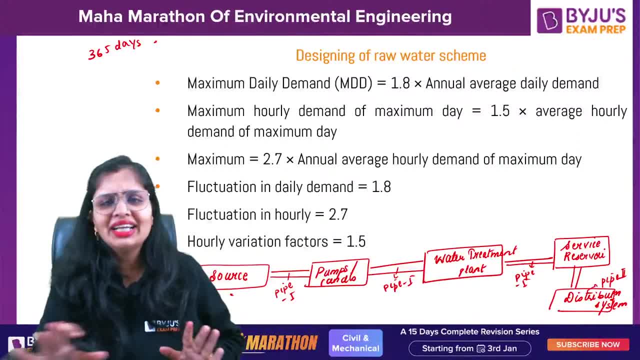 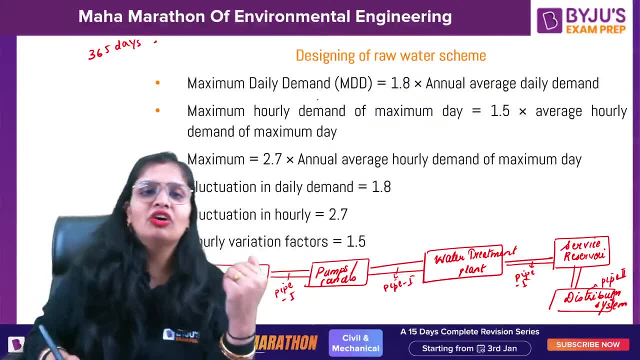 It might be the day of anything like Diwali or any date can be there where the demand Of water will be maximum. So that is known as maximum daily demand. Let us suppose today is what 6th January. So let us suppose the demand on 6th January is the maximum. 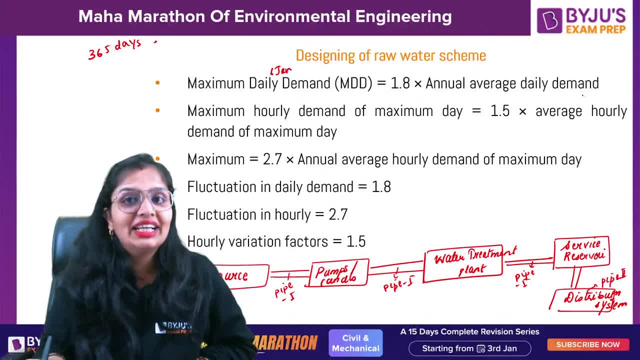 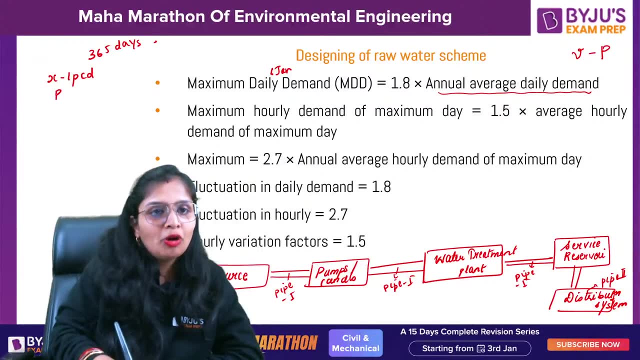 So what I can write: 1.8 annual average daily demand. annual average daily demand is means for the whole population P. What is the water demand for a single day? So if you say for one person, if the demand is X, so for the whole population P, the demand will be how much? 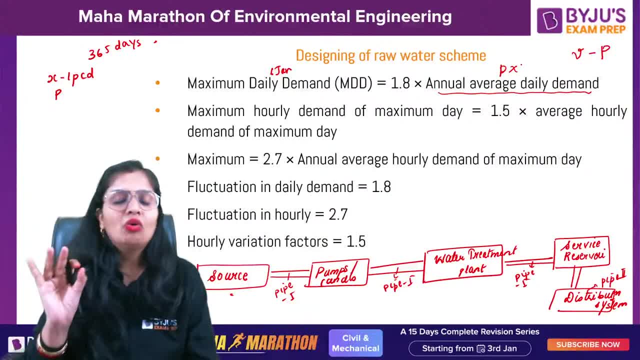 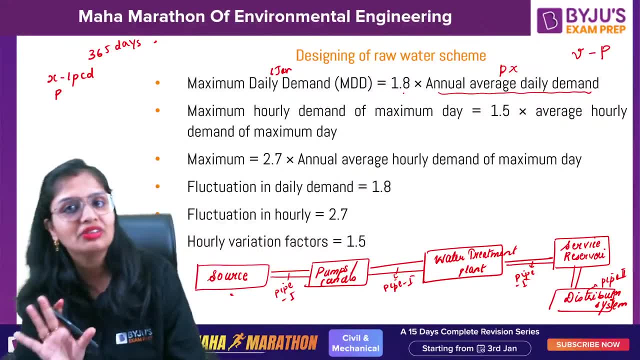 P into X. Okay, Now one thing which is very important. You should know. you will ask me that, man, from where this 1.8 is coming. this 1.8 is observation based. Okay, now, maximum hourly demand. I told you, don't make this mistake. 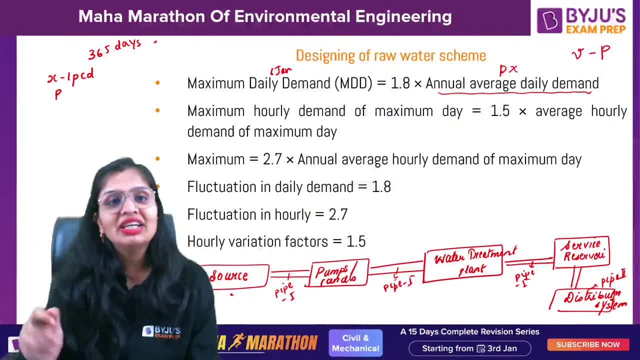 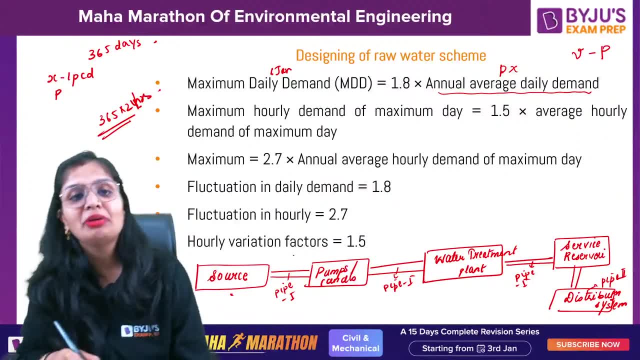 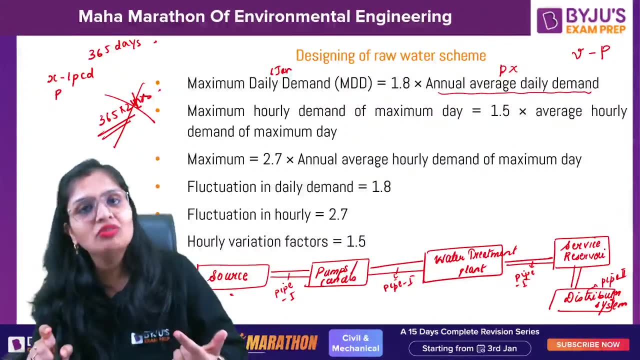 If they give you. also remember, maximum hourly demand does not mean that out of 365 into 24 hours, which will be the one hour when the demand will be maximum. No, This is a wrong concept. It means that let us suppose if 6th January water demand is maximum on 6th January, 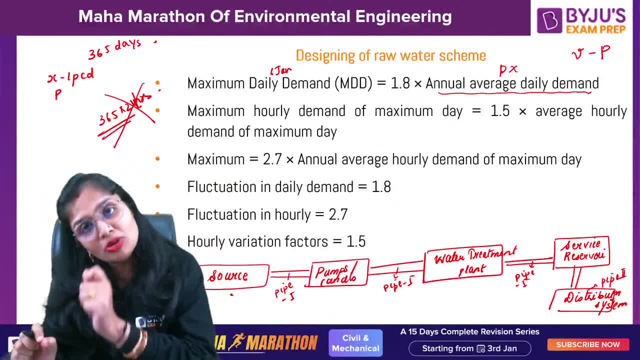 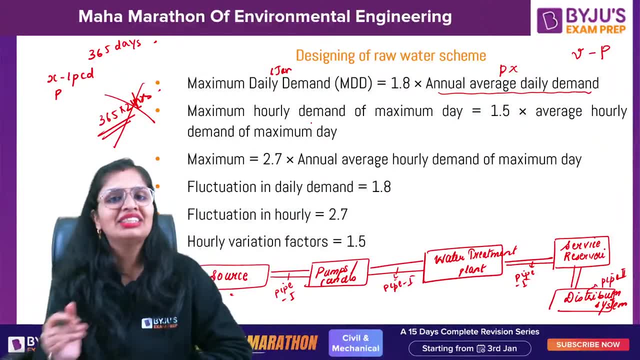 There will be one hour when the water demand will be maximum. So I'm talking about that power of 6th January. So, Max, generally in books you will see they write MHD, MHD, MHD, You learn it. maximum hourly demand, maximum hourly demand. but they don't mention because they assume that you understood maximum hourly demand of maximum. 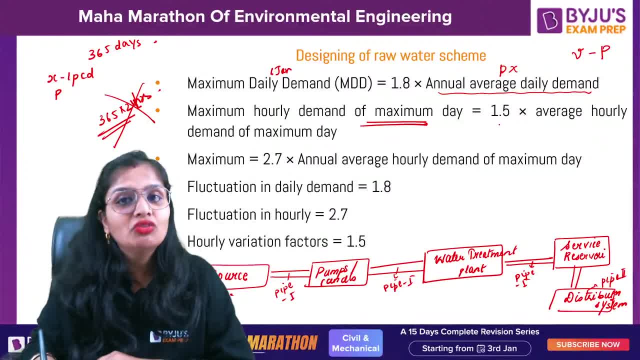 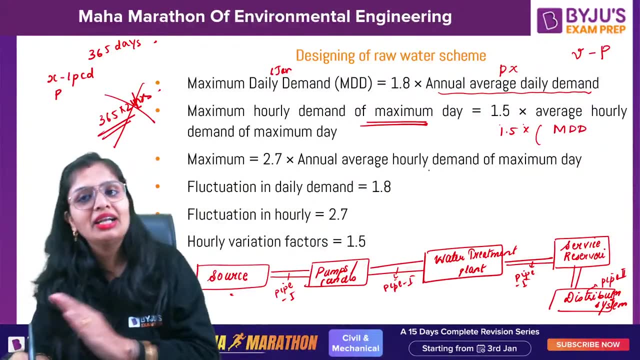 Okay, so which is equal to 1.5 average hourly demand of maximum average hourly demand. How you calculate, you do what you add all the hours, water demand, So it will come out to be maximum daily demand divided by 24, because you need it average. fine. 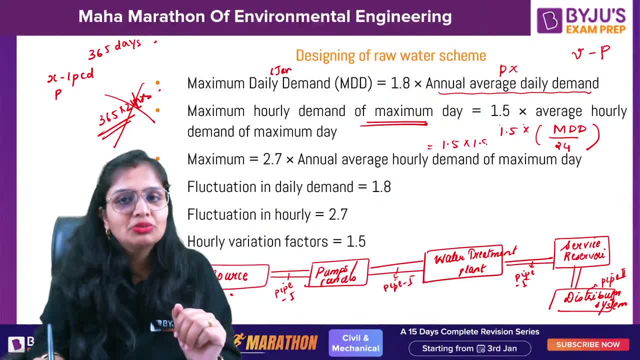 So when you substitute in place of maximum daily demand, you can substitute 1.8.. I'll write it Annual average daily demand. in short, I'm writing it 24.. So this comes out to be this: 1.5 into 1.8 will come out to be 2.7 and this will come out to be annual average hourly demand of maximum. 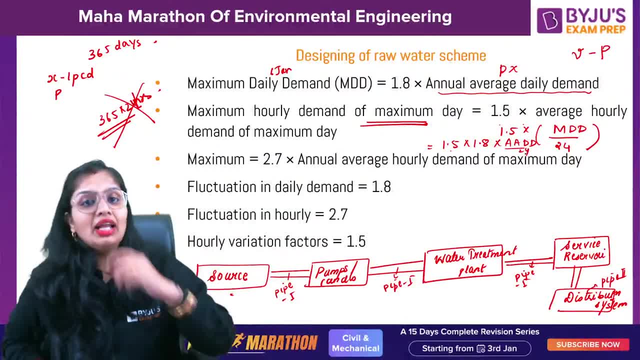 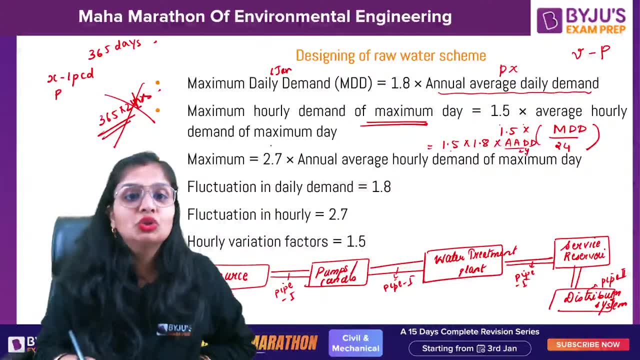 Okay, so this you should know, correct 2.7.. Now again one question. Generally they have asked in EAC and your state level questions. till now They haven't asked in gate fluctuations, this word fluctuations. Let me tell you fluctuation. 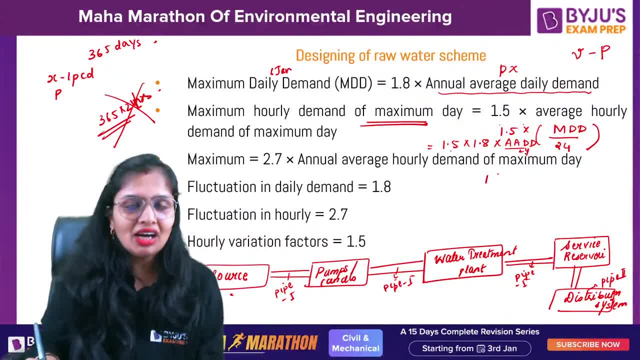 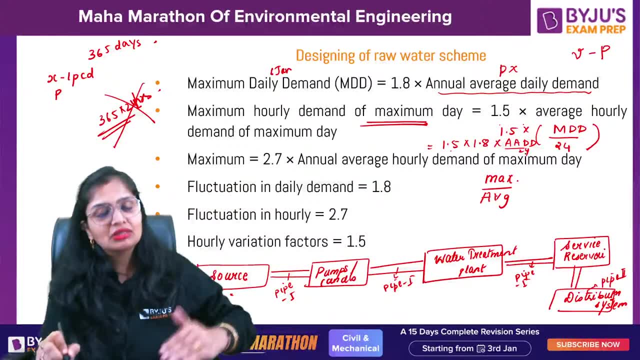 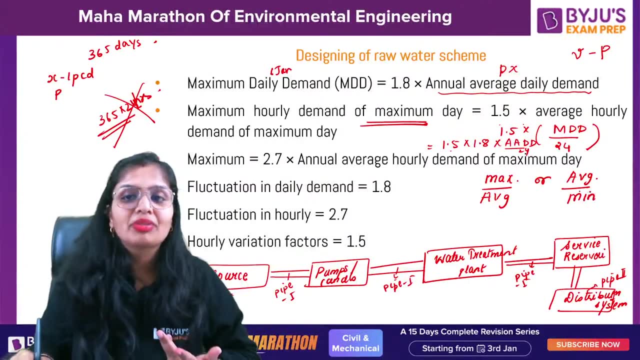 Any parameter. Let us take P So Ellen. in our case, fluctuation is for water demand, So it is the ratio of maximum to average. How many times maximum water demand is more than the average? or you can say how many times average water demand is more than the minimum. 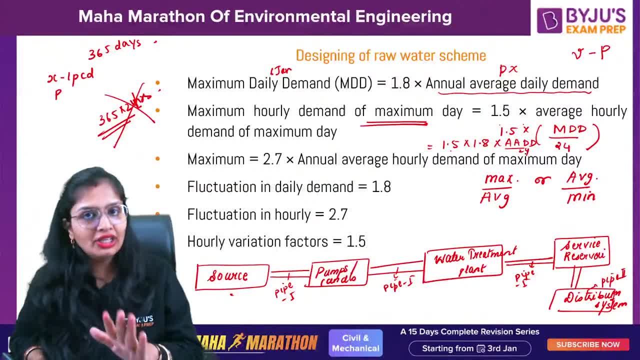 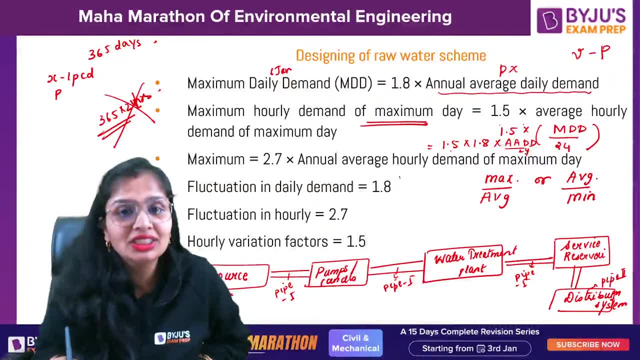 So this is known as the fluctuations: right now not asked in gate again telling you asked in your state level examination AEG papers and your ESE. so fluctuations in daily demand is 1.8. fluctuations in hourly demand is 2.7 important. 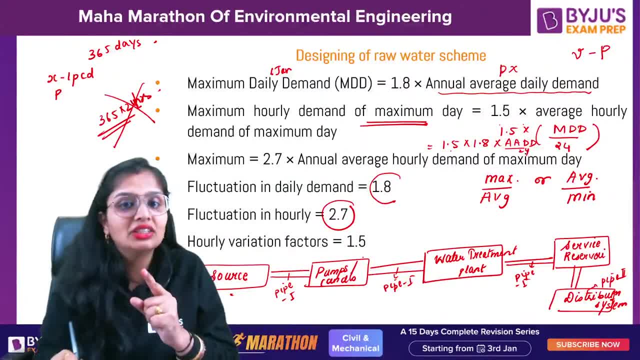 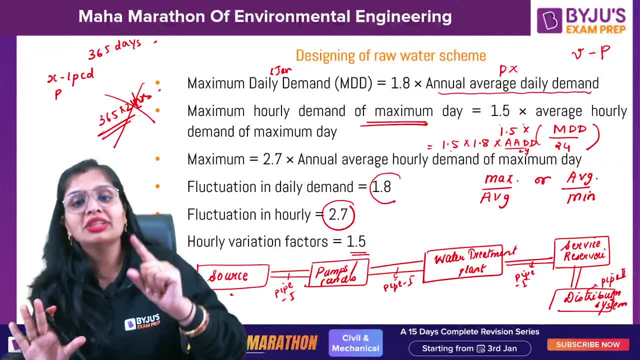 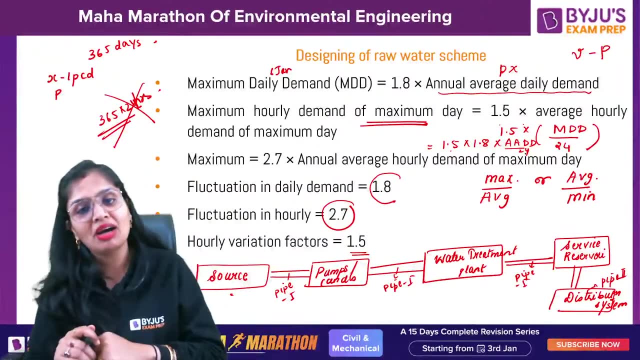 Okay, and the hourly variation factor? It is 1.5. statement wise, They can ask you clear. So this you should know. now comes the question, man, So source will be designed for how many years and for maximum daily demand or maximum hourly demand? 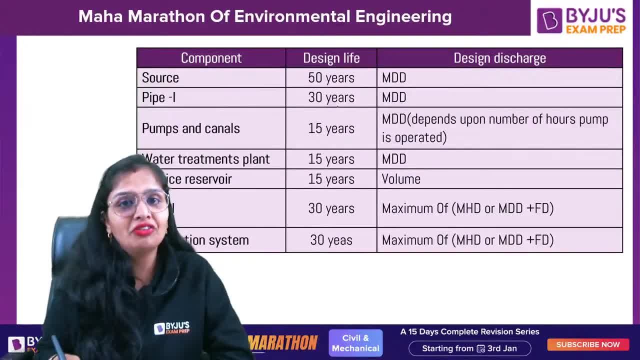 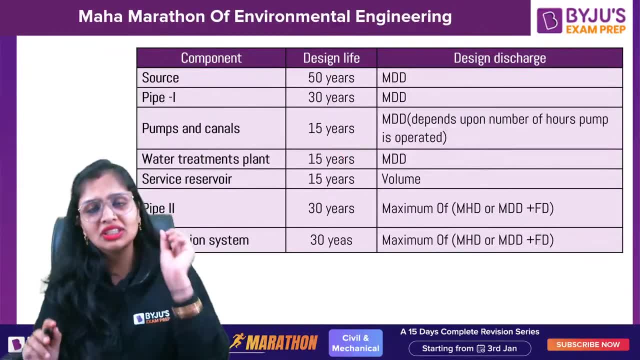 So let's check it out. first, The source: we design it for 50 years. pipes: We design it for 30 years. first question which comes into picture: Why is source designed for maximum number of years? Come on, guys, Answer me. 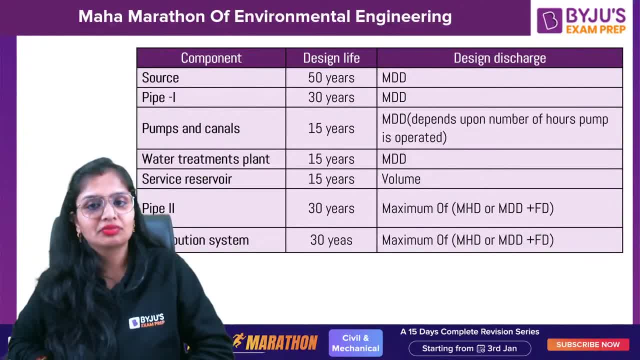 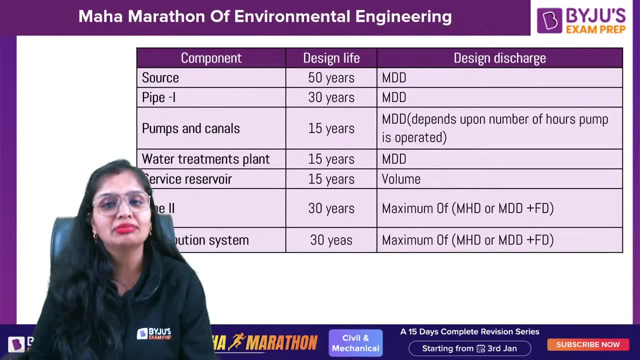 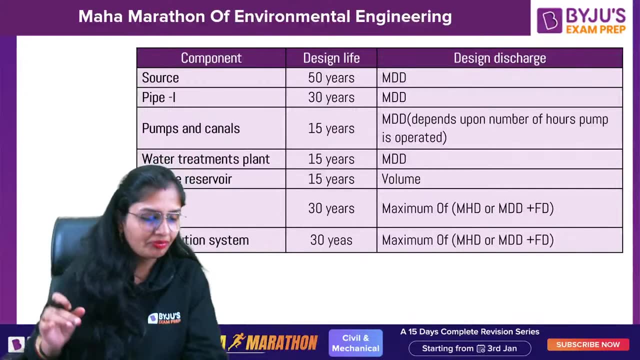 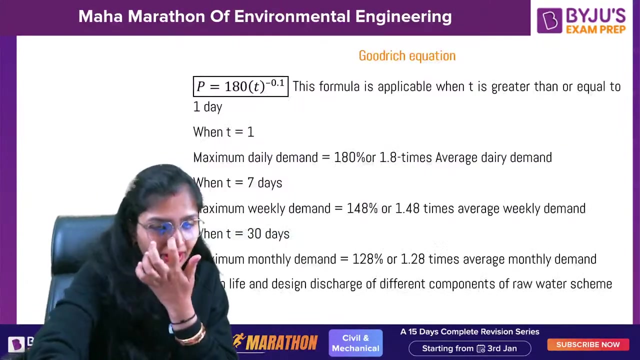 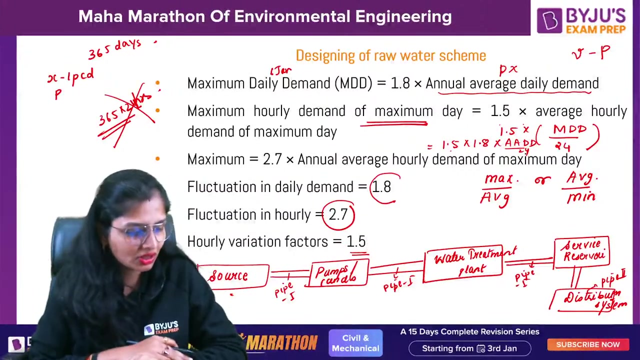 Why stores is designed for maximum number of years. Why, Come on? I want the answer Why stores is designed for maximum Arun Pankaj, everybody Has to serve MVS, Anything else. See this whole, this whole. treatment units are based on the source: long-term purpose use. 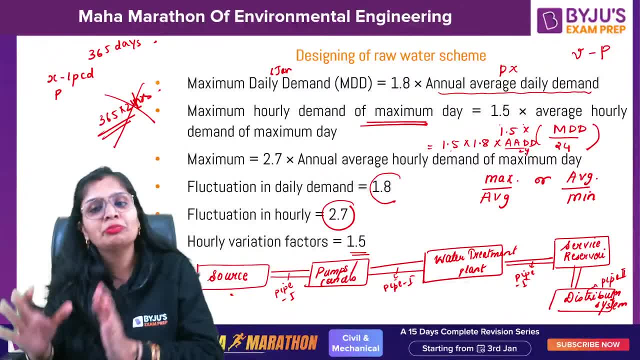 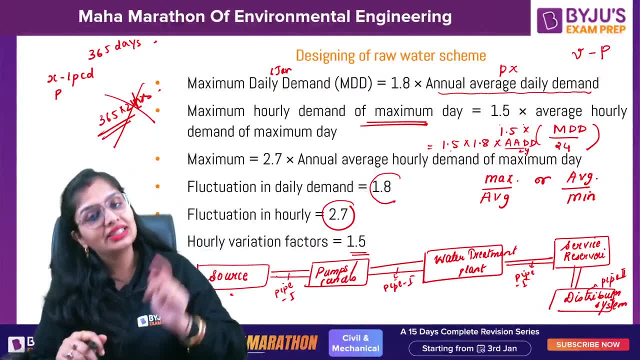 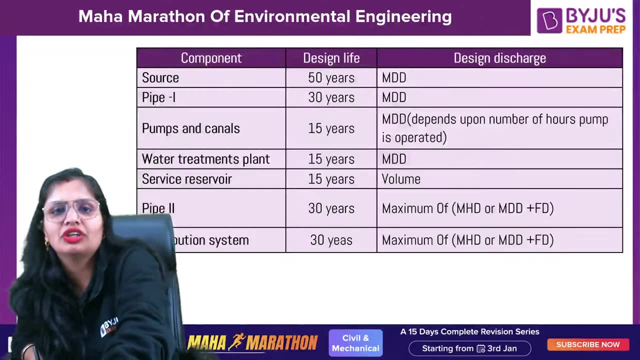 Yeah, huge investment is then, moreover, these pumps, by this pipes, water treatment. Everything is basically dependent on the source. That's why source is designed for maximum number of hours. We don't construct source, We take the construct, intake structures for it. Okay, so that's the reason it is designed for 50 years. 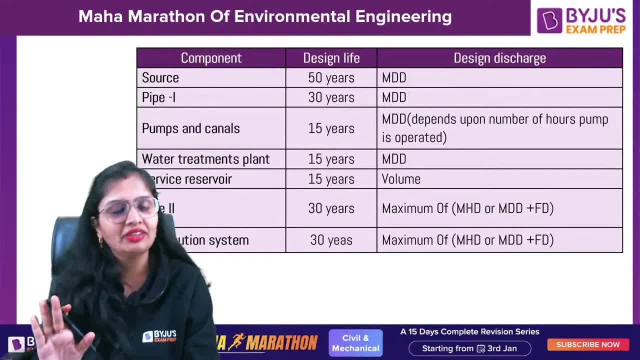 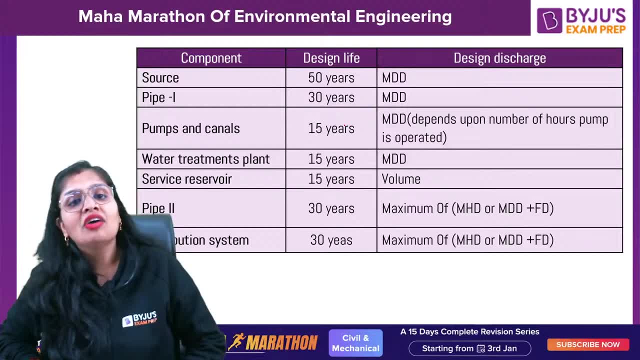 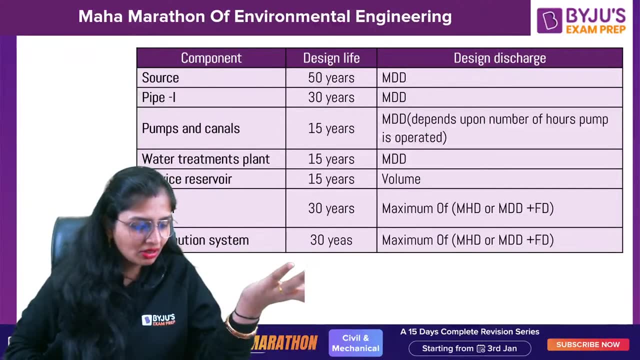 Pipes are designed for 30 years. distribution systems are designed for 30 years. pumps, water treatment unit, service reservoir I designed for 15 years. now again comes the potions why they are designed for lesser number of time. reason: reason, just like your mobile phone Serviceability. all sessions require whole syllabus will be covered in this session. 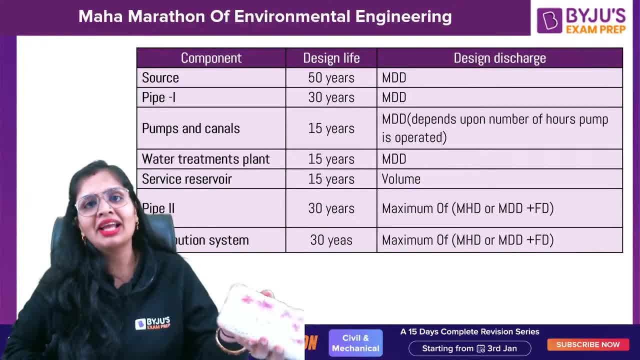 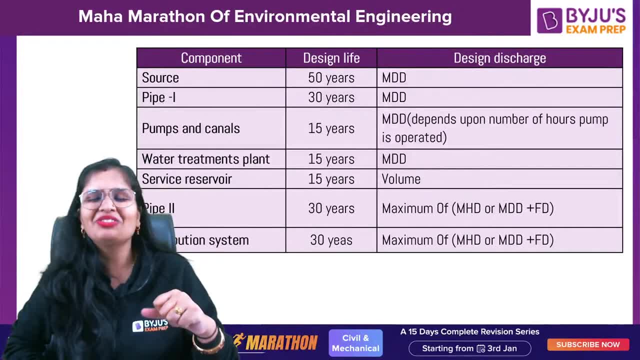 Yes, Now, just like this mobile phone, like you know Apple, every year it launches a new thing with new camera, with new- you can say, new- features in it. So what happens? you feel like now I should sell one of my kidney and buy another one. 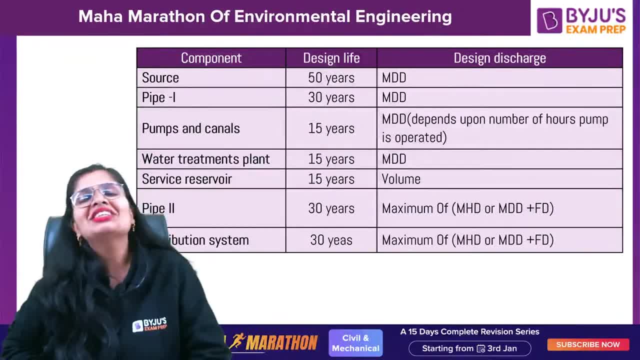 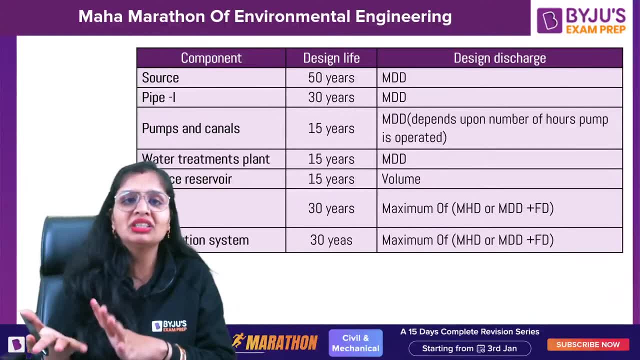 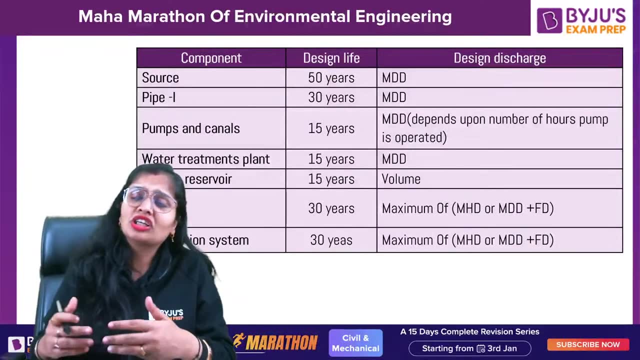 Just kidding, but you feel you get tempted, right. So the question comes: there is a technical updation, which takes place similarly in the case of pumps, water treatment, service, Reservoir. there is an updation, techniques, new techniques comes. So what, man? let us, let us construct a bigger one. 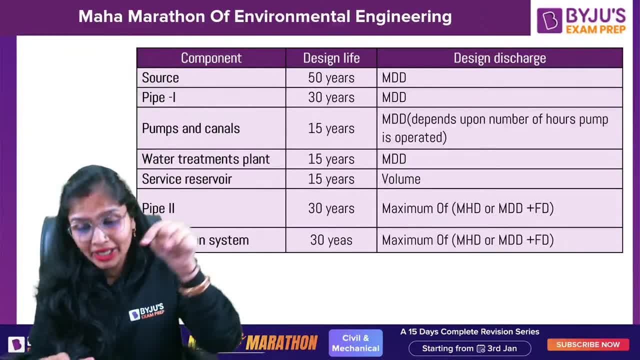 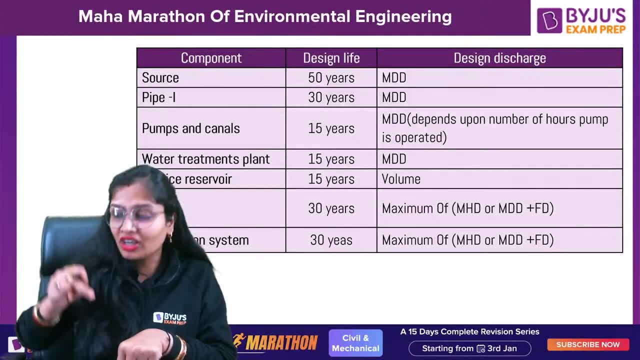 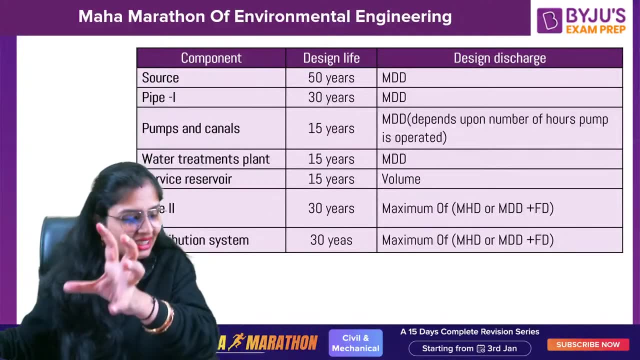 We will use it for 30 years. If you are doing that, you are investing large amount of money now, and you are. if you are investing large amount of money now for a longer period of time, You have to use the outdated technology. Yeah, that is the reason. this is designed for lesser number of years. the question now: 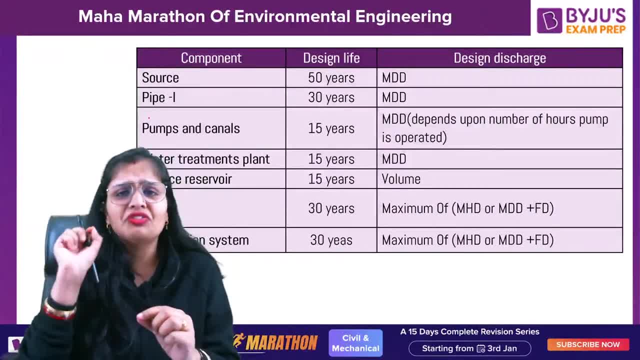 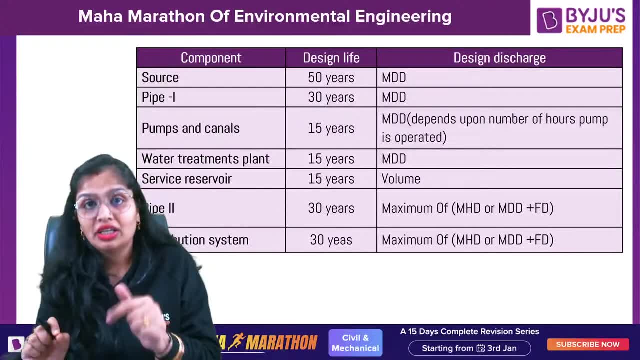 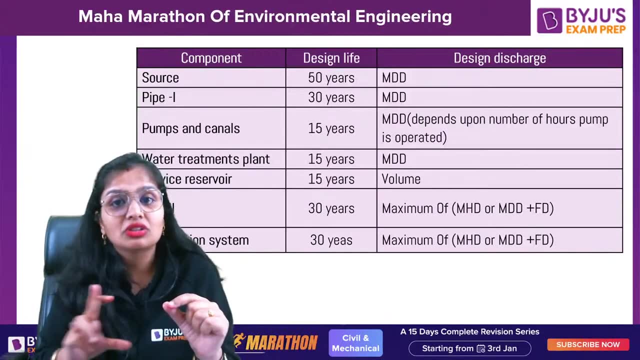 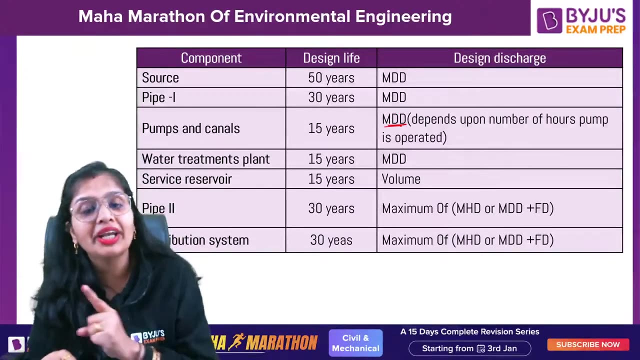 One thing: pumps and canals. This is very important. weather, This is very, very important, specifically when you study it in irrigation engineering also, and if any question comes in your environmental engineering: pumps and canals generally does not operate for 24 hours. Okay, MDD, you say it, but generally it's not MDD. also why? because it does not operate for 24 hours. 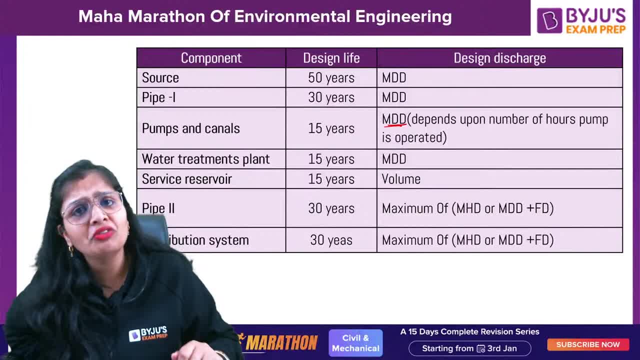 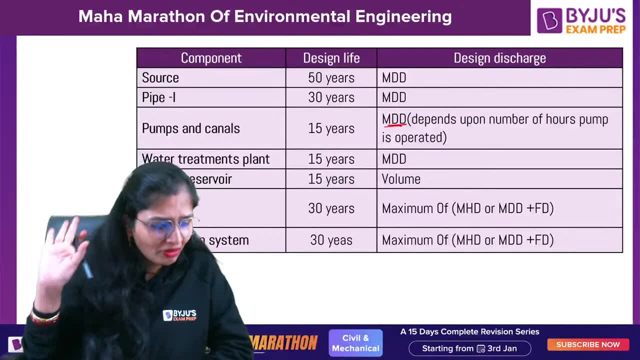 Remember this. why, man? Why pumps will not operate for 24 hours. beta G: you have to give electricity bill also. Okay, that's the reason I tell you. you tell me one thing, you tell me one thing: one is 240 liters. You need 240 liters. 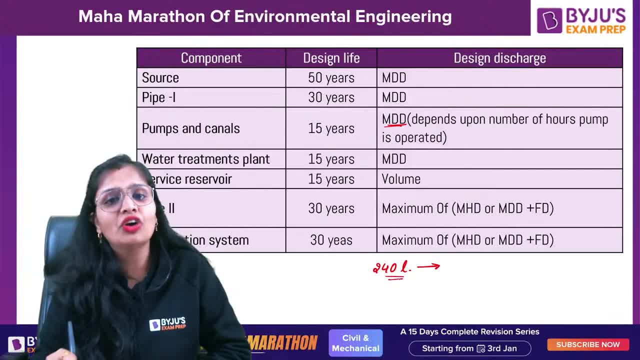 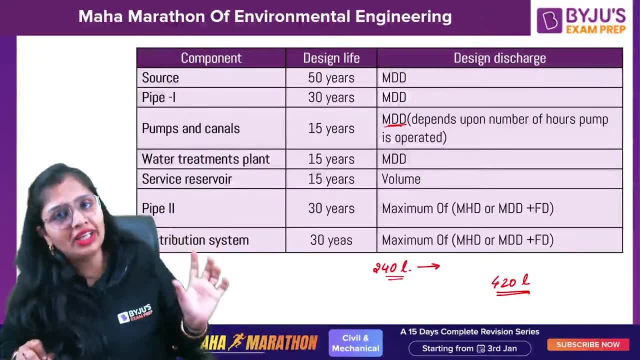 So you will design, or you will take a pump which has 240 liters of pumping capacity, or you will take it for 420 liters. Come on, guys, based on your knowledge, Tell me you need 240 liters of water per day. So you will take a pump of 240 liters of 420 liters. 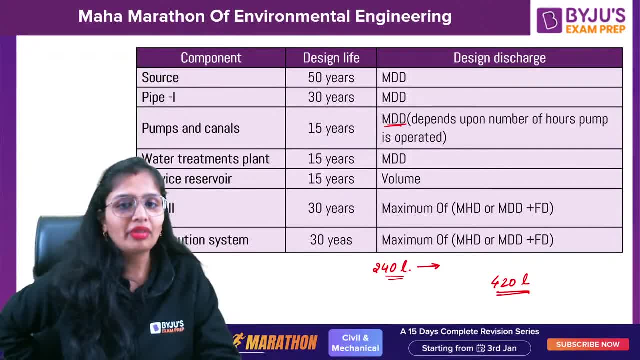 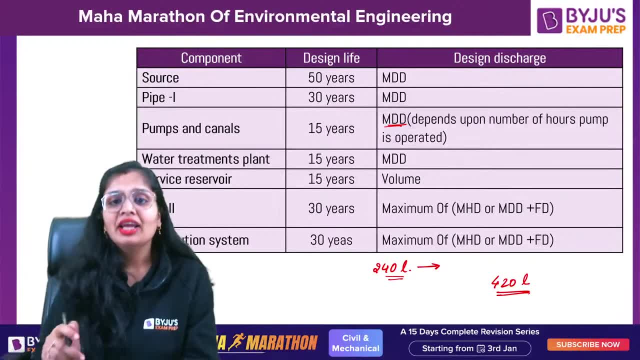 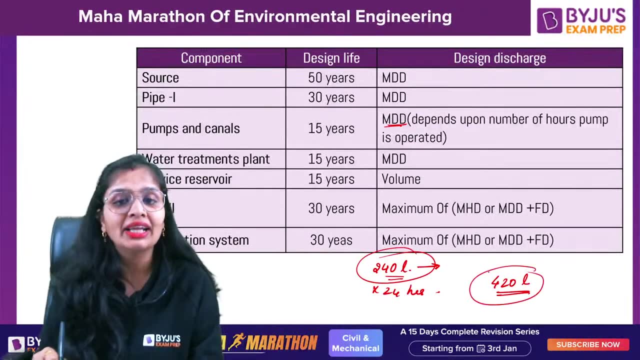 420, fast, fast, fast 420. why? because if I need 240 liters per day, I have to pump for 24 hours, But if I need for, I have basically purchased 420 liters pump capacity, So I will operate for 12 hours. 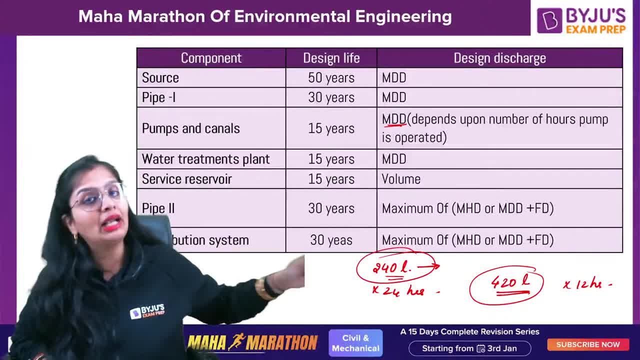 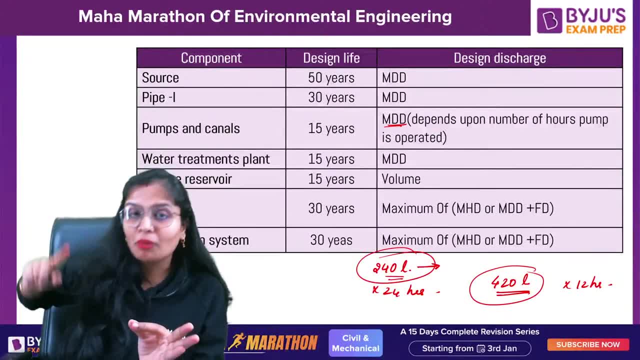 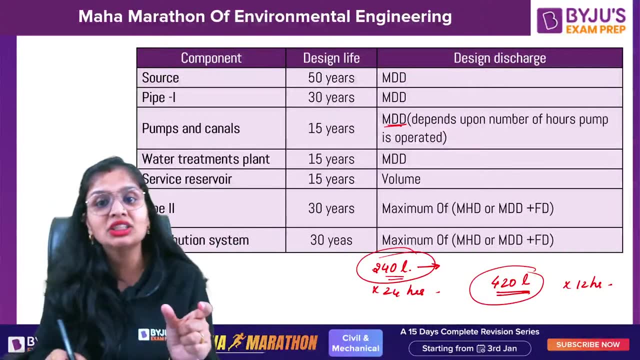 So what man? you spend it. the money for 420 liters. that pump would have been costly, Yes, But initial investment cost is more, but operation cost is less. Remember these technical terms: initial cost is less for this one. initial cost is less, but operation cost is more. 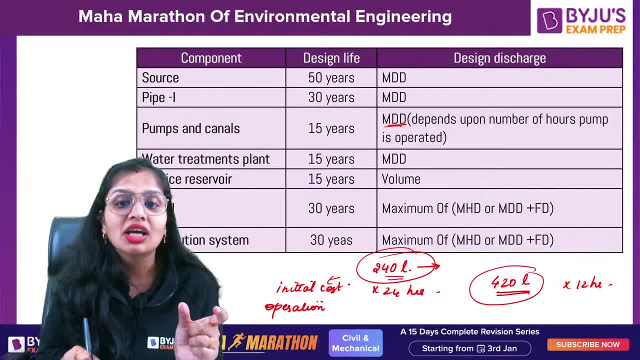 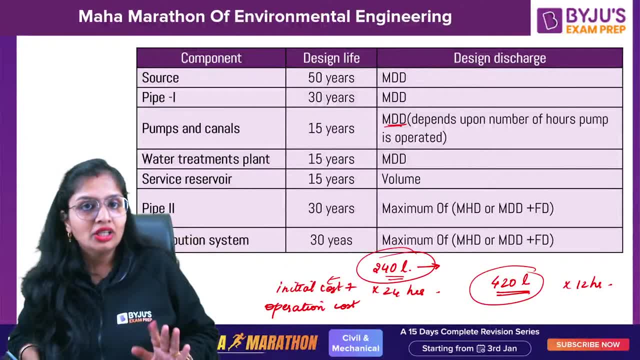 because the pump will be operating for 24 hours to 420 liters. Initial cost is more, operation cost is less because I'll be operating only for 12 hours, So generally in environment and irrigation, Whenever They'll give you questions, maximum number of times. 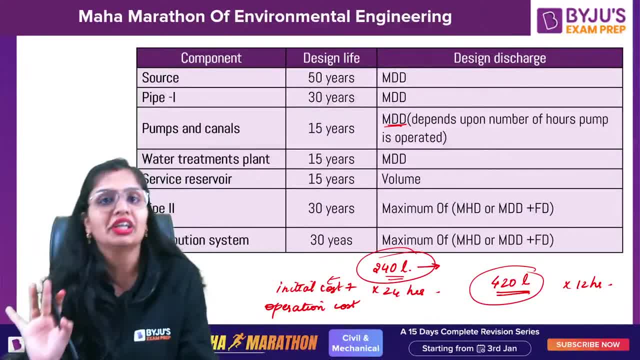 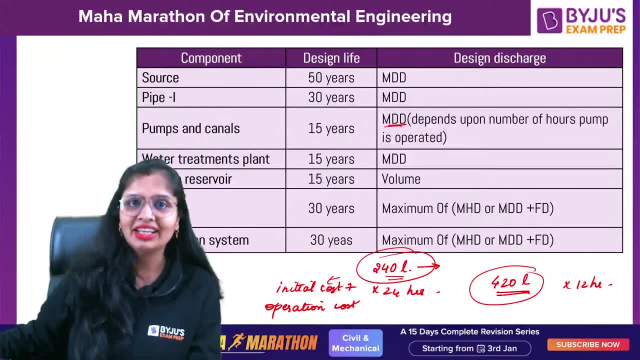 They'll specify. the pump is operating for 8 hours. The pump is operating for 10 hours. And you why? you want to get that example? take it in your home. We say na paani chadha rahe. in Hindi you say that mummy paani khatam ho gaya paani chadha rahe. switch on the pump. 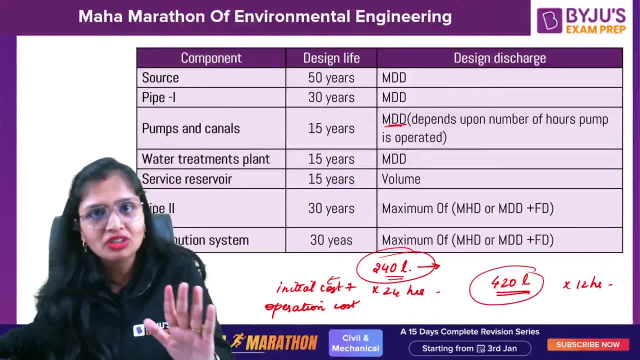 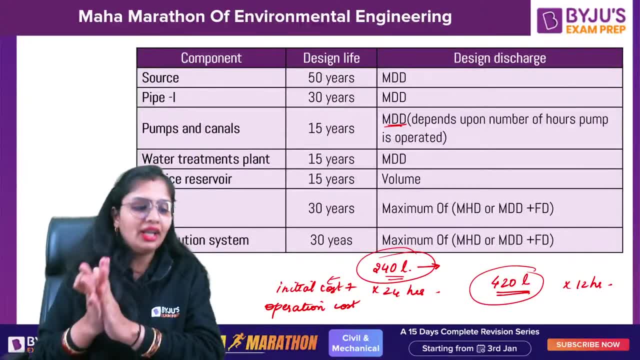 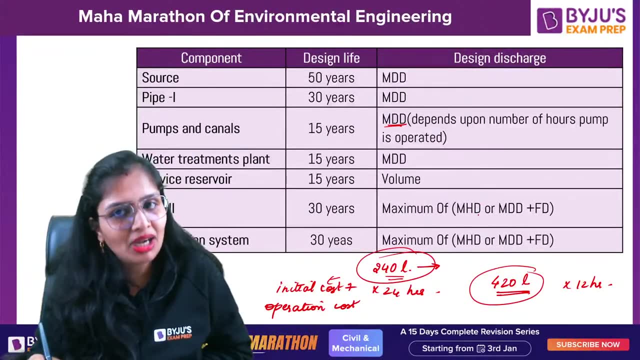 There is no water. So do you operate the pump for 24 hours? No, you don't do that, Okay, because it requires electricity. That is the reason. clear now. Next comes pipe and distribution system. They are designed for maximum of maximum hourly demand, or maximum daily demand plus fire demand. 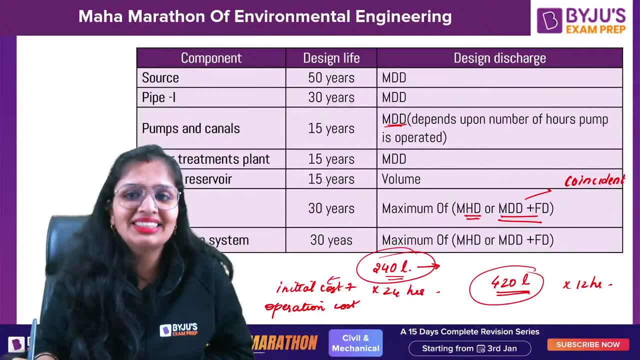 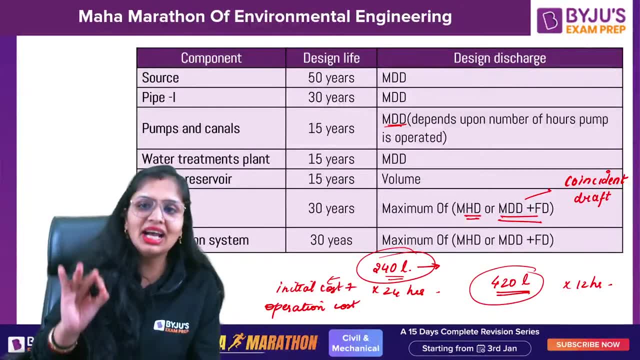 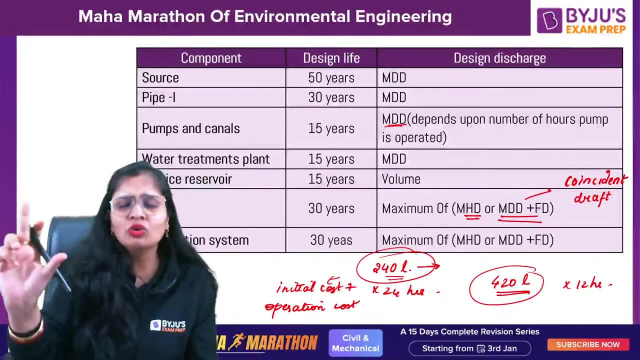 This is known as coincident draft in some cases. in many exams I've asked: actually coincident draft is mdd plus fire demand. Remember, sometimes they ask you coincident draft. Sometimes they ask you distribution system is designed for. both are different. Now one question. maximum students get confused. 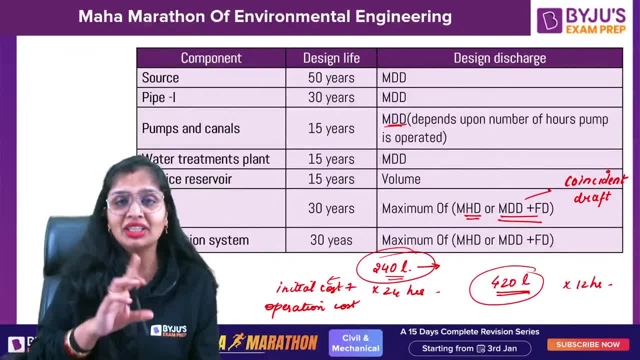 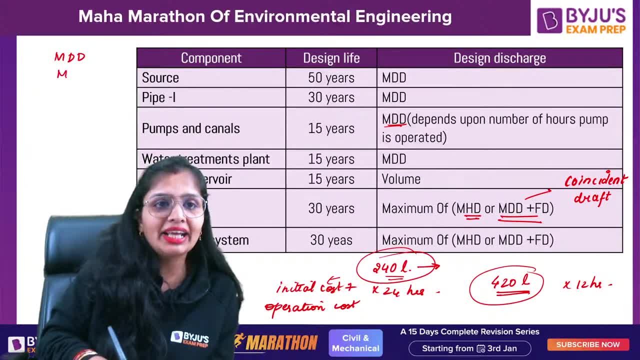 In your a exams, in your ESE exams, in your gate examination. It has been asked sometimes what they say distribution system is designed for. they write mdd, They write mhd, They write this fire demand, but they will write mdd and they will write the fourth option. maximum of this is a, b, c, d, maximum of a and b. 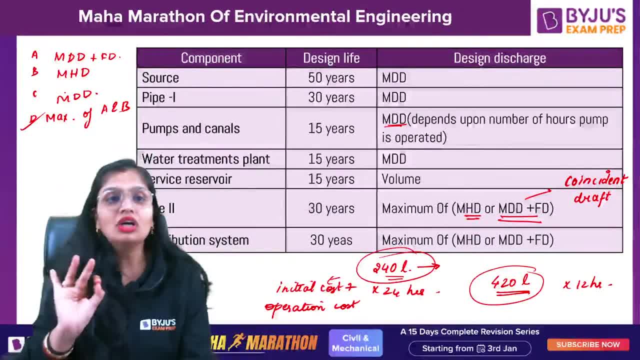 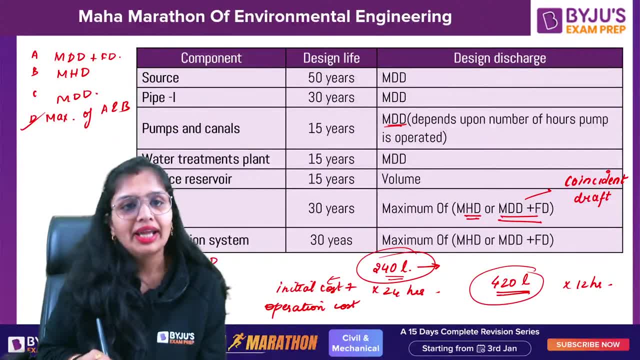 If this question comes, you mark it at T. Now let us suppose Secondary format. They judge you is. they write only mdd, mhd and they write any other things are also. let us suppose fire demand, and they will write none of these. 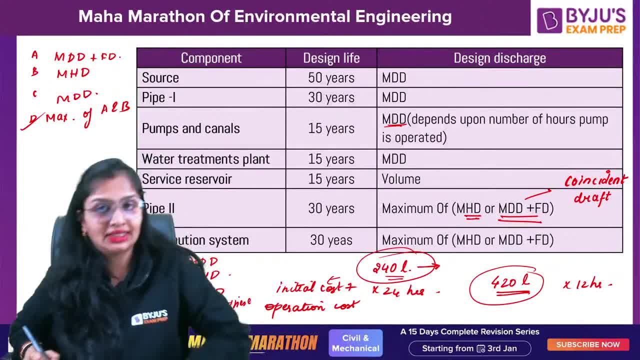 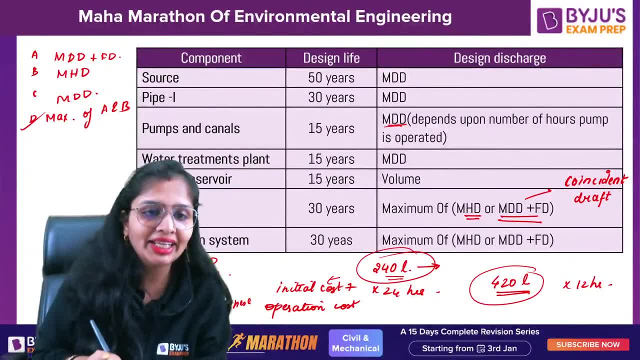 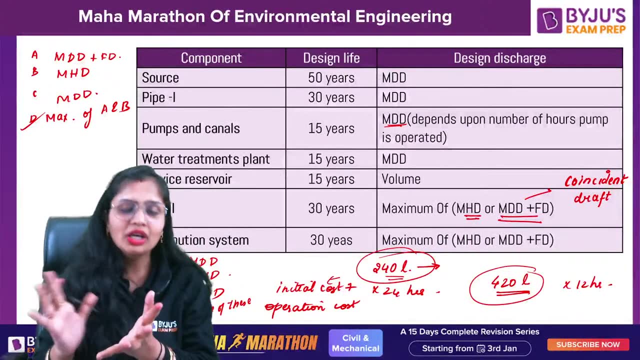 So in this case, if they give you option like this, suppose if such option comes in your exams, So generally the answer which they take is maximum hourly. Okay, So, based on the options you have to, you have to do what you have to do what you have to modify your answers. 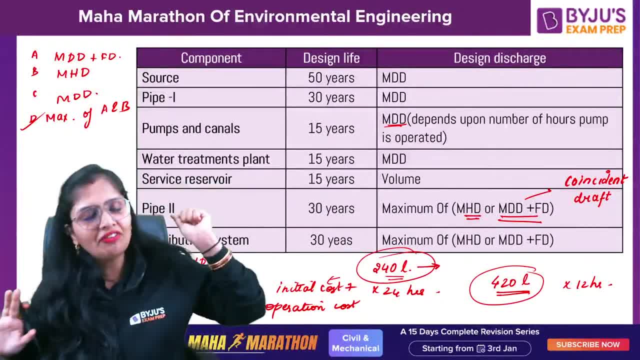 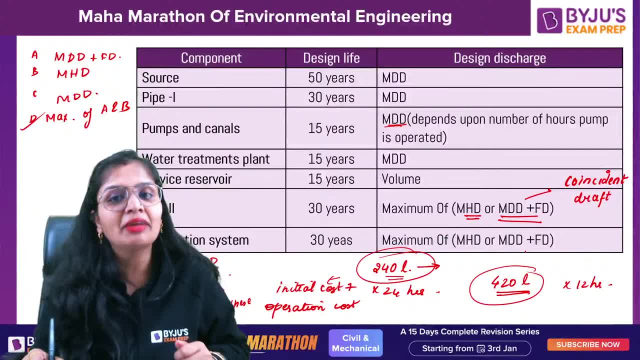 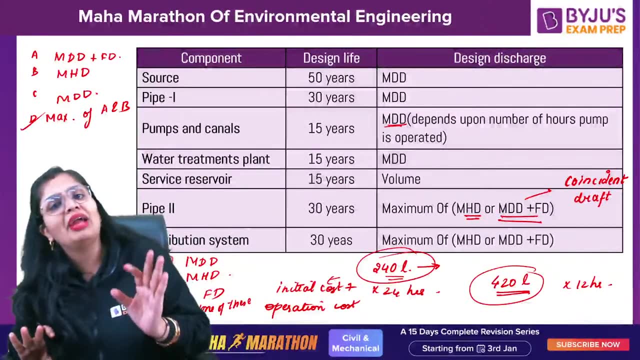 Okay, Now let me tell you 95% of the times in numericals, which has been asked: maximum daily demand plus fire demand comes out to be maximum. Okay, wherever if you are giving the test series and all 95% of the time, mdd plus fire demand comes out to be maximum. 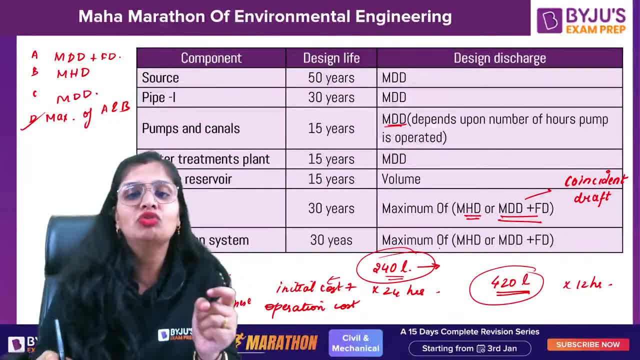 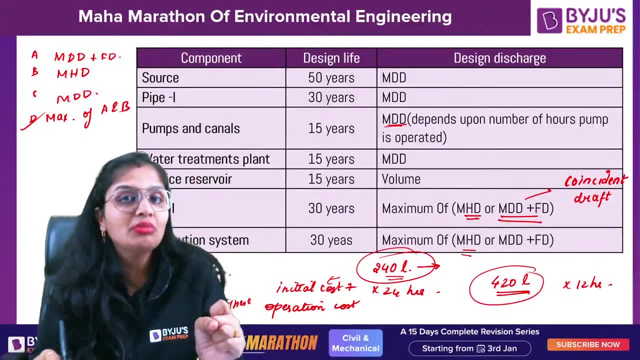 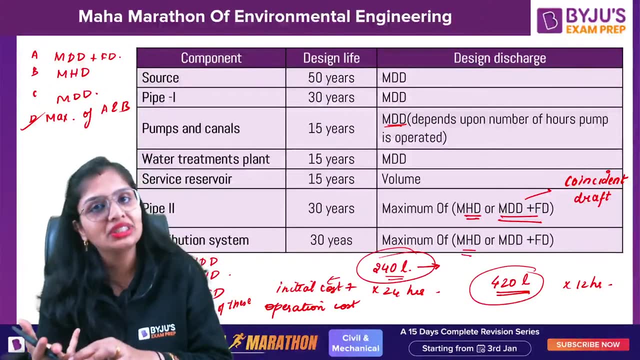 But that doesn't mean in the examination You won't calculate mhd. don't do this mistake. They can set the data in such a format that maximum hourly demand will come out to be maximum. Okay. So that is the reason: calculate mhd, calculate coincident draft: which of the maximum will come? don't do that. 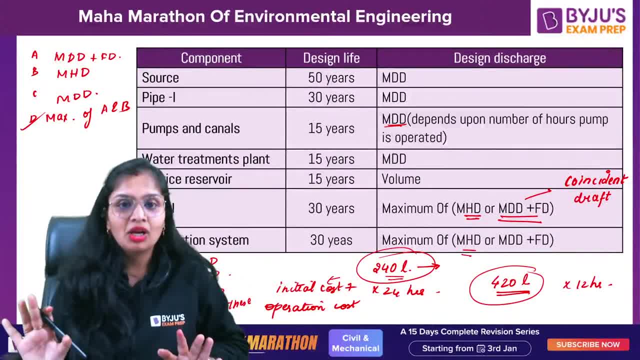 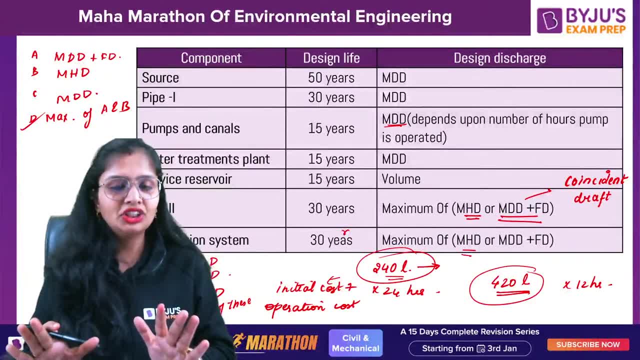 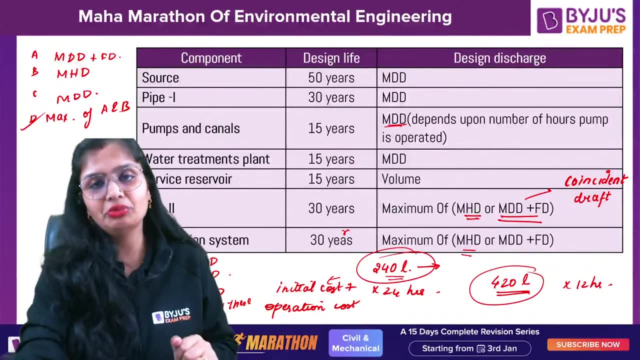 Okay, take that into account, So don't be in overconfidence. Okay, So till here, any doubt? guys Enjoying the session. Rishabh, everybody's speed is okay Fast. Actually, there's 20 seconds lag in YouTube. 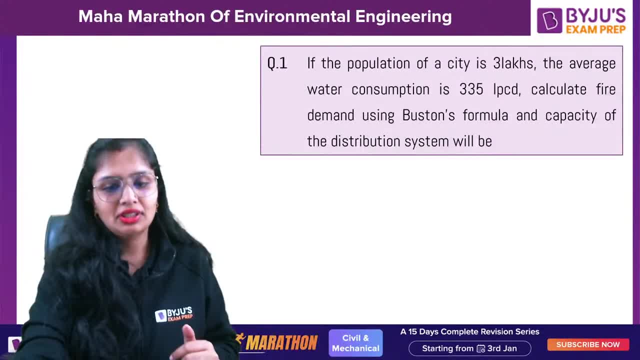 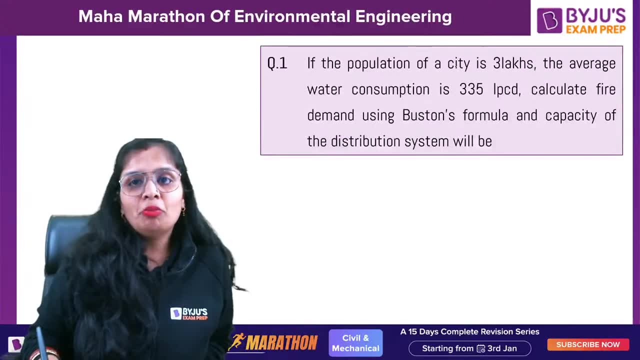 So whatsoever I said we just do after 20 seconds. Okay, I on it straight, fine. So this is the question for you: The population is given to you, average water consumption is given. you have to calculate the bird were fire demand in mld and the capacity. 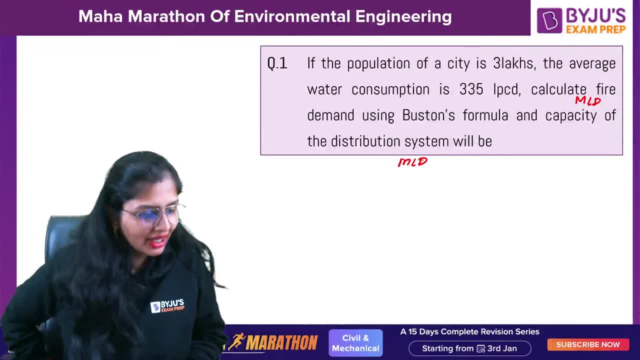 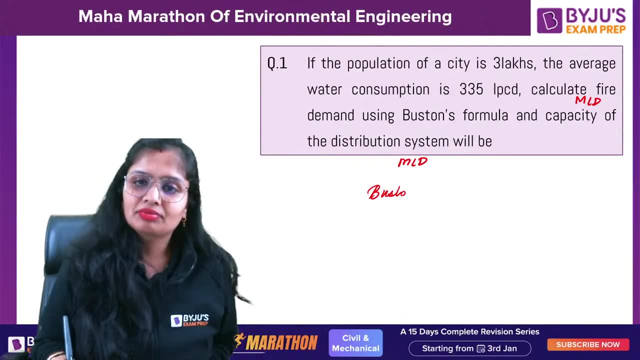 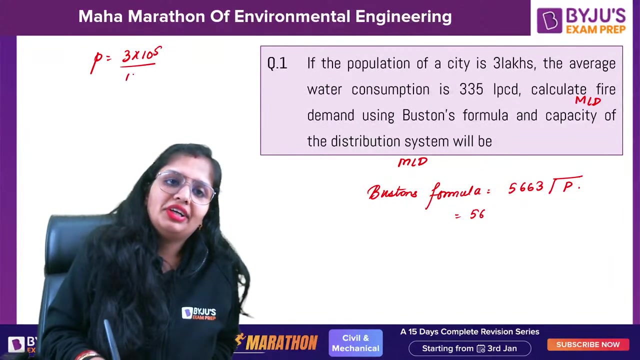 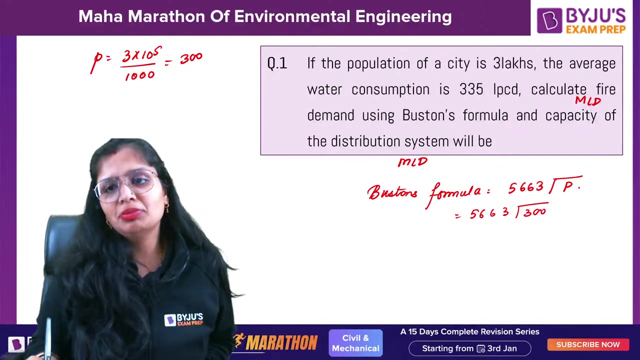 Of the distribution system in mld. Come on, guys, faster. Population is 3 lakh bus tons. formula Population in thousands, So 3 into 10, raised to power, 5 divided by thousand. Okay, Get the answer in liters per minute. 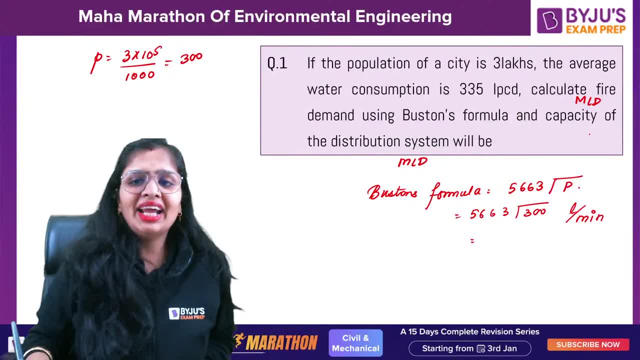 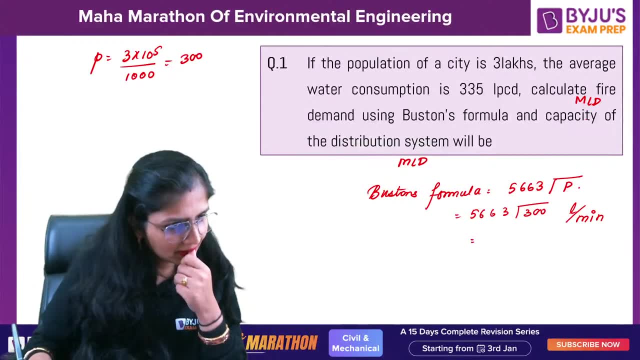 After that you have to convert it into liters per day. Get me this answer in liters per day. That will be better Calculate On mld also. Come on guys, first liters per minute. It will come how much it is coming. 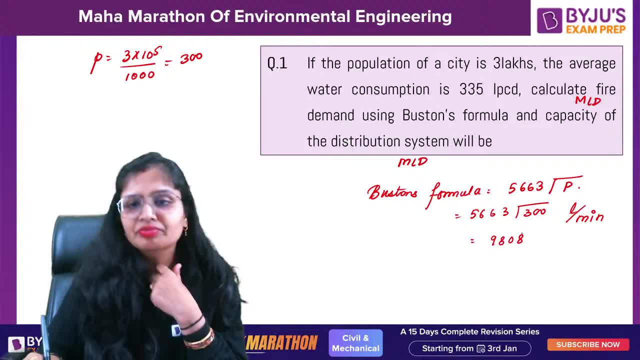 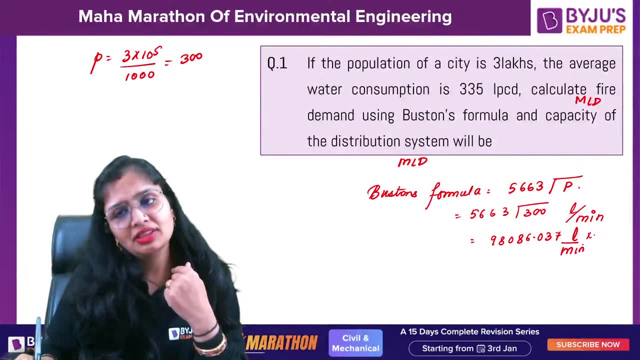 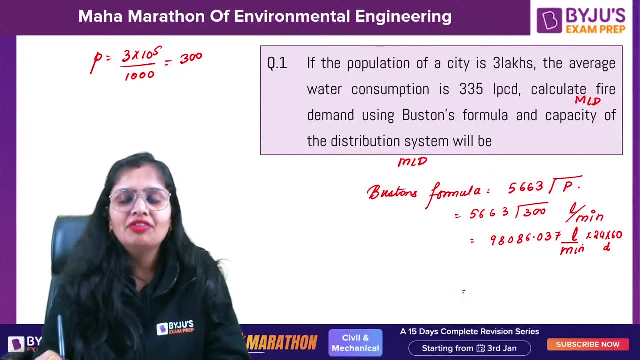 Anybody Letters per minute. So if you call want to convert it into days, Multiply 24 into 6. It will be 1 upon, So it goes into the multiplication side. Okay, And for mld divided by 10, raised to power 6.. 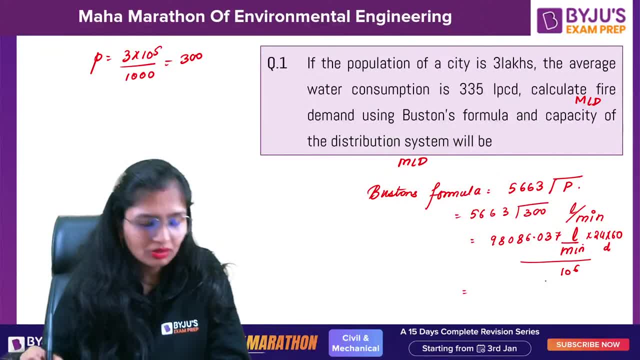 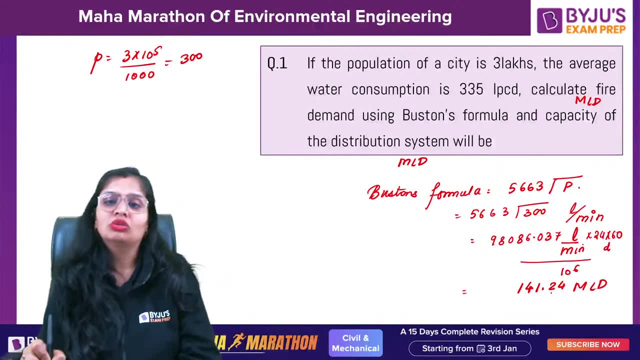 How much it will come. I'm asking in mld. Just check it out. I might write wrong Also calculations. You have to check it out. So this is the bus tons fire demand which you are getting: 140, correct, Correct Girish. 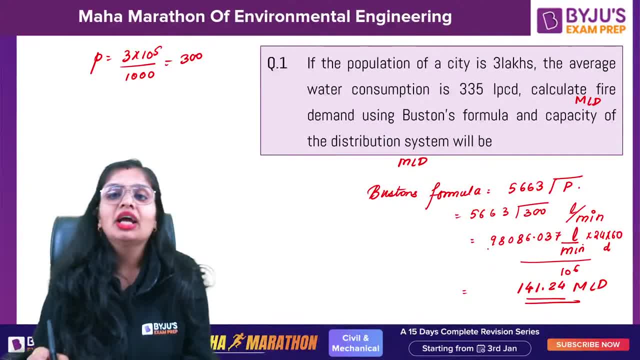 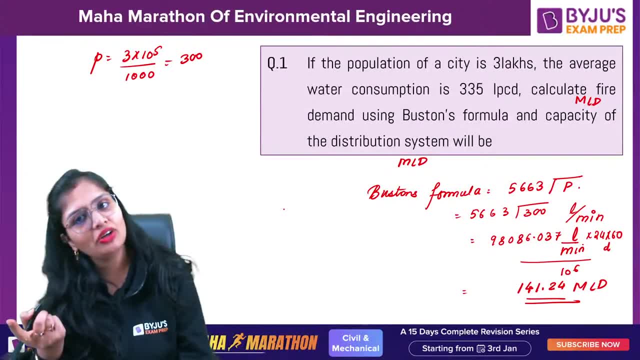 Okay, So this is the by bus tons formula, This is the fire demand. Now, if you want to know the capacity- capacity of distribution system- So you have to calculate mdd also, You have to calculate mhd also. So mdd is what? 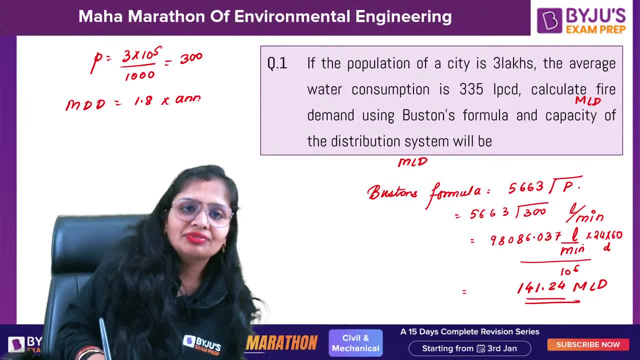 1.8. Times annual average Daily demand. So one person requirement is 335 liters per day. How much will be required? by 3 lakhs, Calculated in mld, divided by 10, raised to power 6, and tell me. 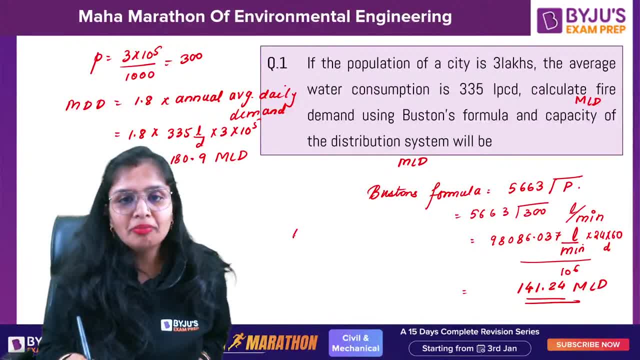 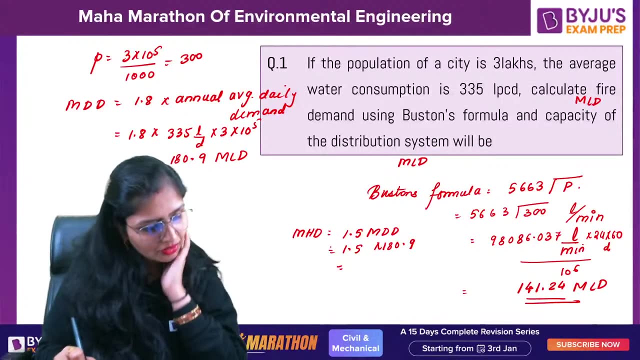 This is maximum Daily demand. Now, if you talk about maximum hourly demand, that will be 1.5 times. So maximum daily demand: 141.24. that I got it, This one. How much it will come? 180.9.. 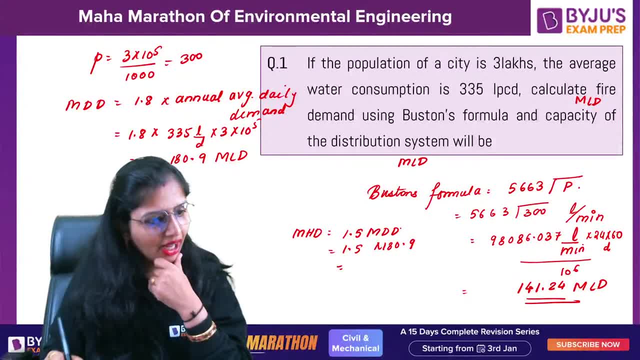 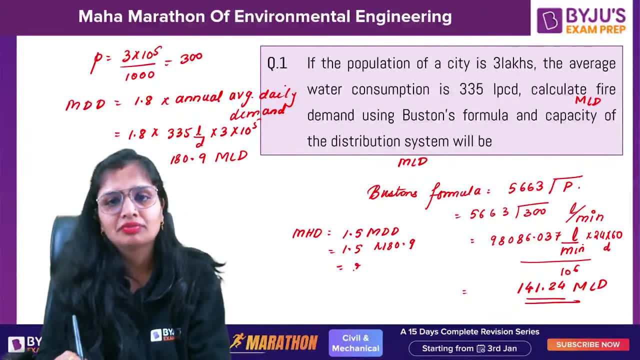 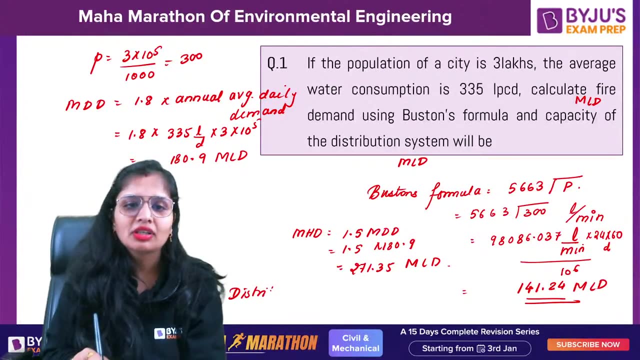 Okay, and this one Or I have to calculate 1.5 into 180.9. Million liters. So distribution system will be what Maximum of mdd plus fire demand And mhd How much it is coming, mdd plus fire demand. 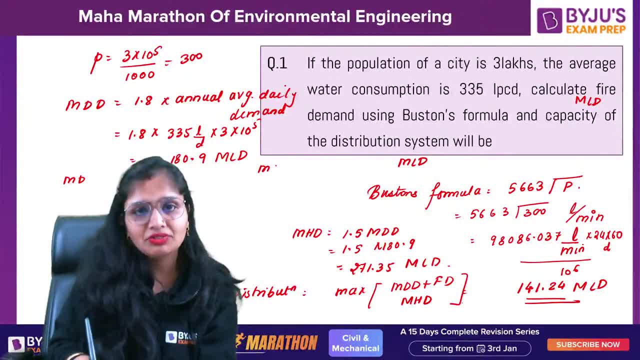 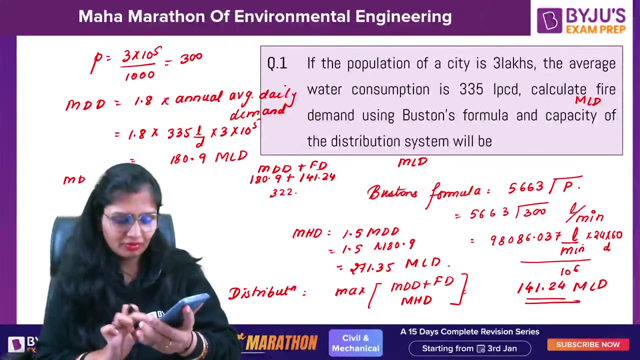 It is going above my head out: mdd plus fire demand: 180.9. fire demand is: how much? 141.24.. How much it is coming? How much it is coming 180.9? 141.24.. This comes out to be 322.14 mld. 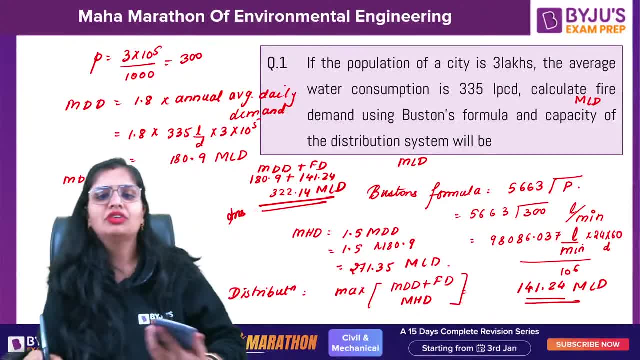 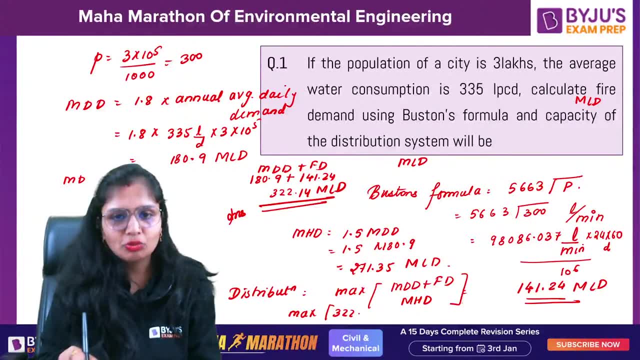 So the distribution system is designed for 322.14.. So this is going to be 322.14 mld. Why? Because mhd is 271.35.. So maximum of 322.14. And 271.3.. Clear. 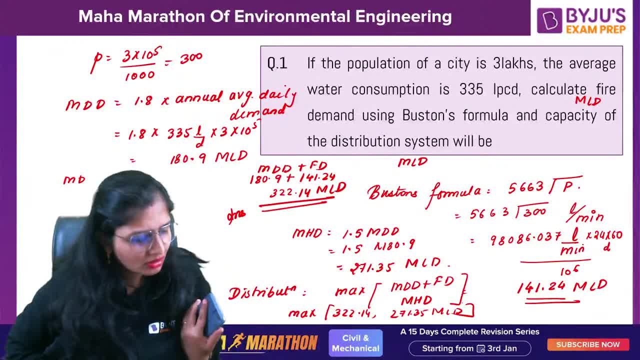 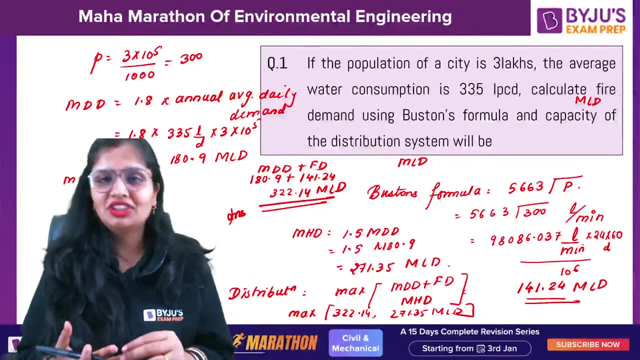 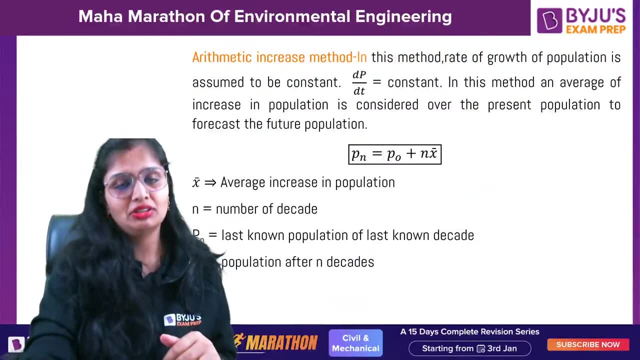 331 it is coming. 322, it is there. Dinesh, check it out once again. Okay, so this is the simple questions which they can ask. Fine, So now coming for the the population forecasting methods. Population forecasting methods. Why? Because you need to. 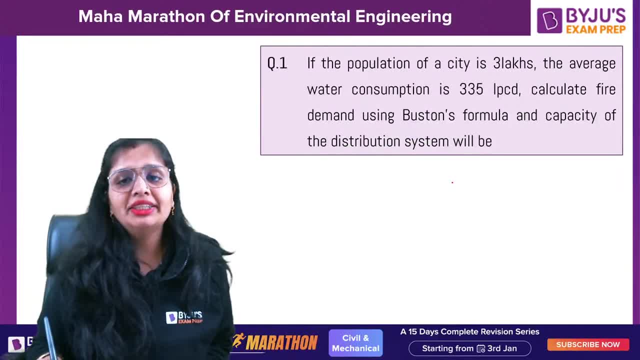 forecast the population Now, before that. the population depends upon many factors, like it depends upon the birth rate. You know that, right? The population, we are second and we are proud in India. okay, Out of the whole country, After China, we are the second in producing the 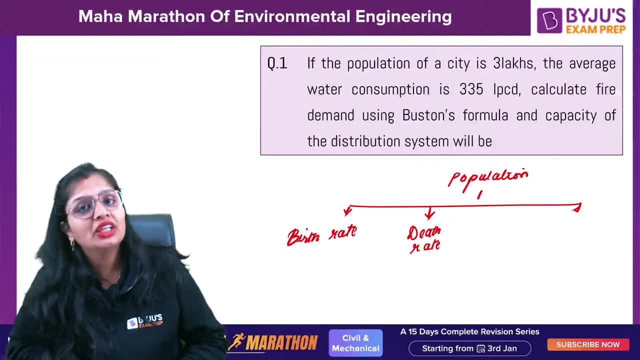 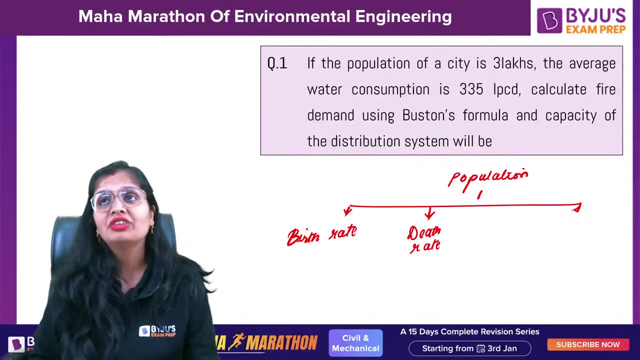 population. So birth rate: it affects the population, Death rate: it affects the population. Nowadays death rate has reduced also, you can say, and you can say increased also. Now you say increased and reduced, both because nowadays there are new types of diseases which are coming. 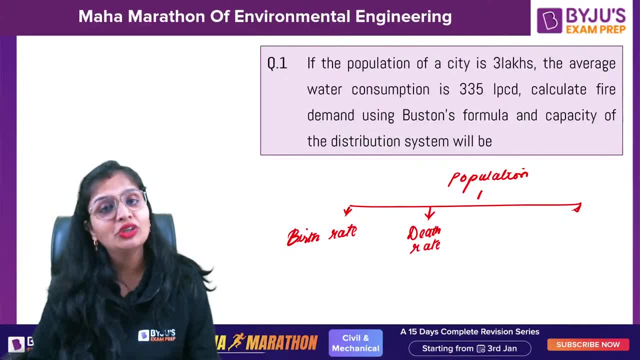 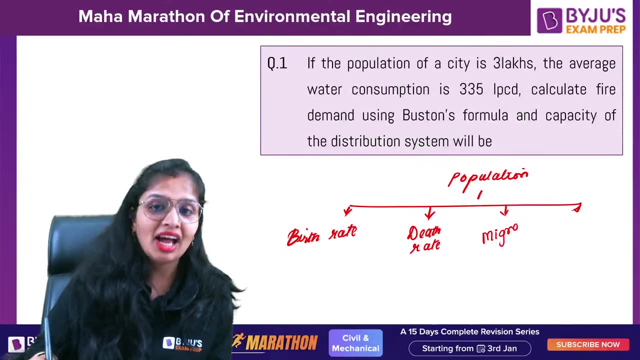 which you have never, ever heard of. okay, Secondly, reduced because we have- now everybody has- money and we have latest technological advancement in the medical science also, So death rate is reduced because of that. Then there is migration. Migration, there is a word which, again, they: 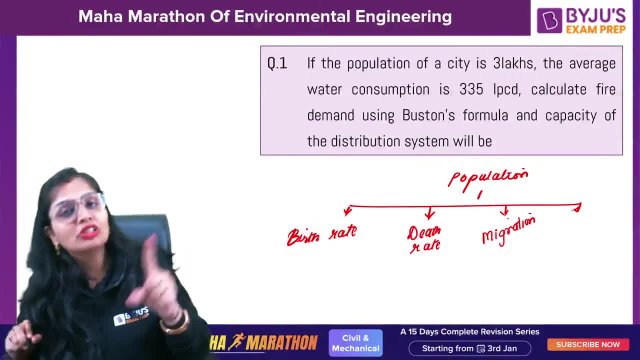 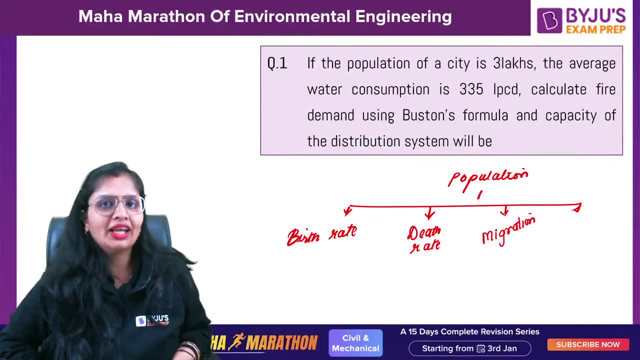 haven't asked in statement wise questions, but they can ask you: is positive migration and negative migration? Positive migration if you shift from a place. let us suppose I am living in Bhilai and I want to shift to Noida, So from here I am shifting to Noida, So, Noida, there will be a. 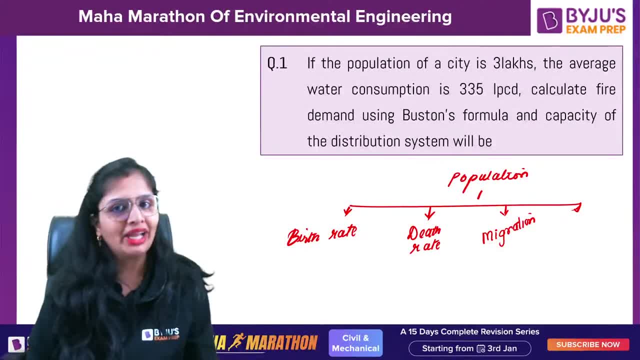 positive migration. but if you shift to Noida, you will have a negative migration. So you have, in Bhilai, there will be a negative migration. okay, Because the population is what Reduced, because I, along with my family, shifted to Noida. okay, So this is migration. Then there is one. more thing: increased due to annexation. Now, what you mean by annexation means in Hindi we say kabja karna. Let us suppose if we do annexation of any nearby country I won't take the name, otherwise there will be a case on me also that I am planning it. 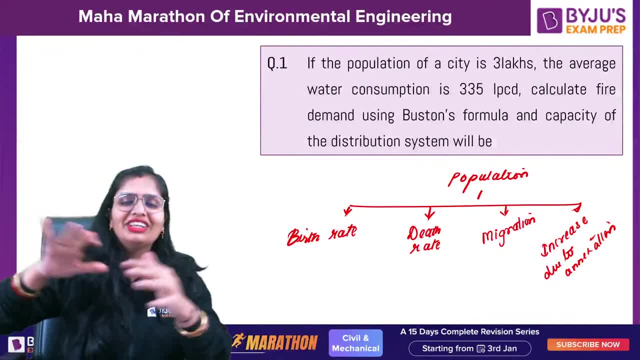 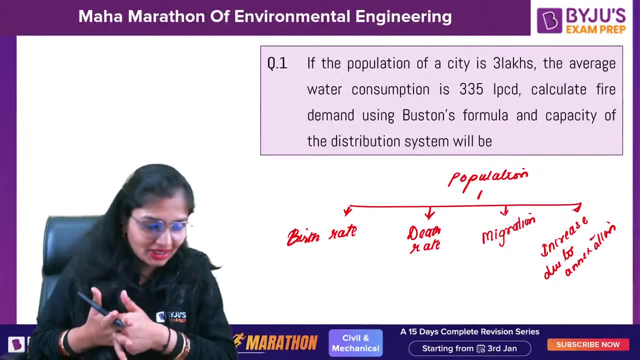 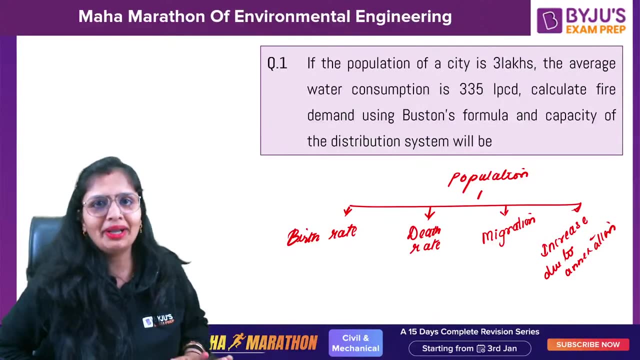 So if I want to basically annexate any of the neighboring countries, so what will happen is what will happen is the population will eventually increase. okay, So there are n number of factors like pandemic and epidemic. I guess you know the difference between pandemic and epidemic. 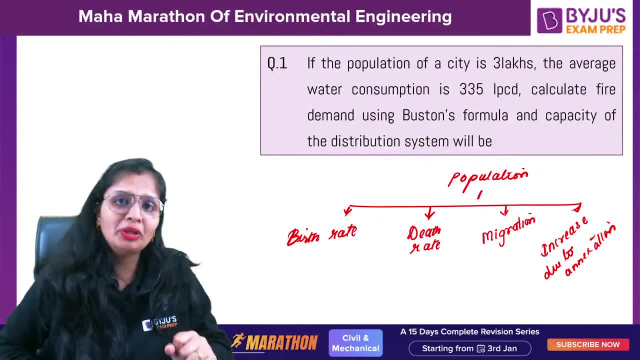 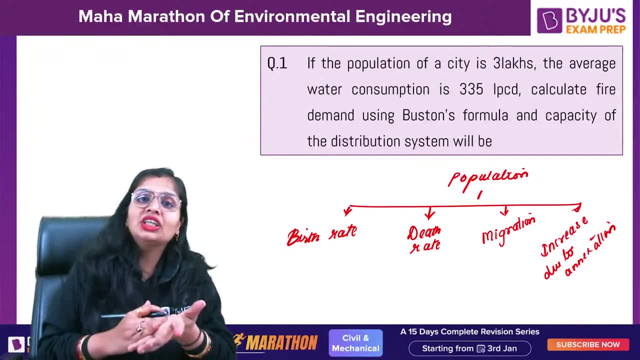 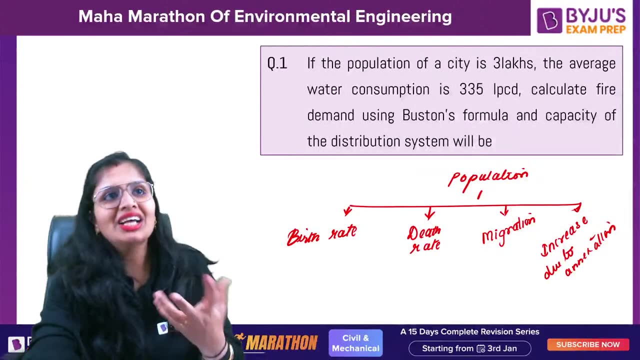 okay, Like COVID came lots and lots of people died. So that is what it happens- one in 100 years. So because of that, the population initially decreased. So that can also be a reason, okay. So now when you forecast the 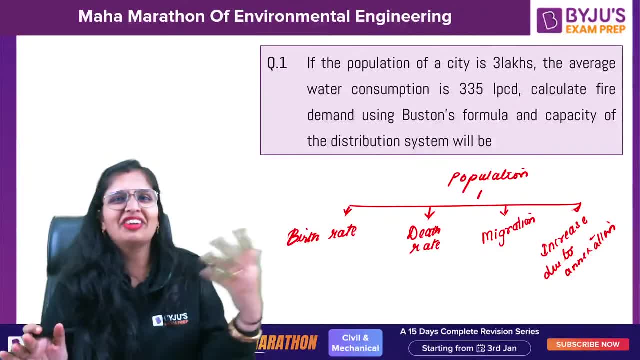 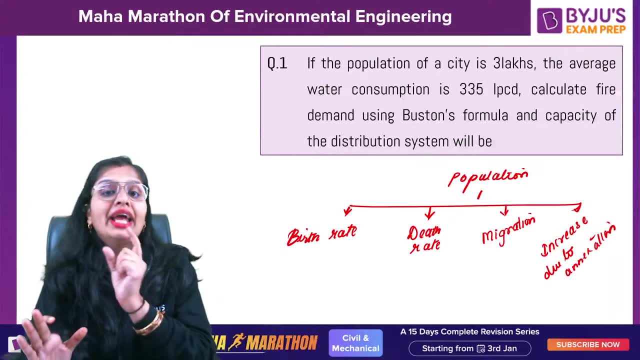 population? there is. no, every city is not similar. You know, some cities are very old, some cities are now only formed. So that is the reason: population forecasting methods wait. It is not at all necessary that in the gate examination they will give you which method. 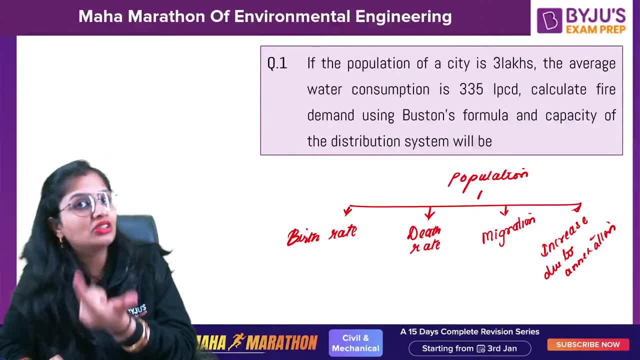 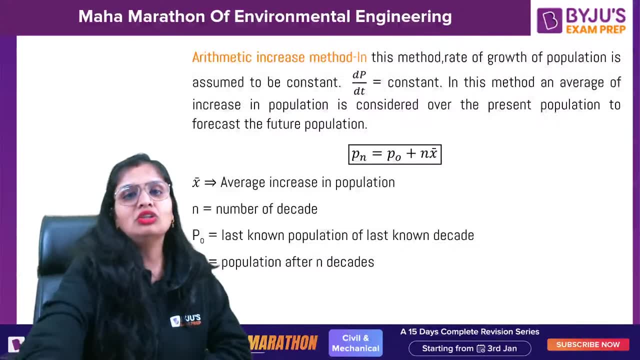 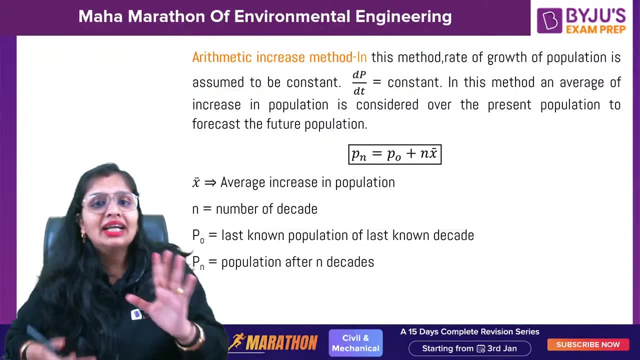 to apply. They can give you certain sentences based on that which you have to apply. your brain, whether to go by arithmetic, geometric or whatsoever methods, are there. So this is the first arithmetic increase method. What happens In this? you assume that the growth of population is constant. It is constant, That is. 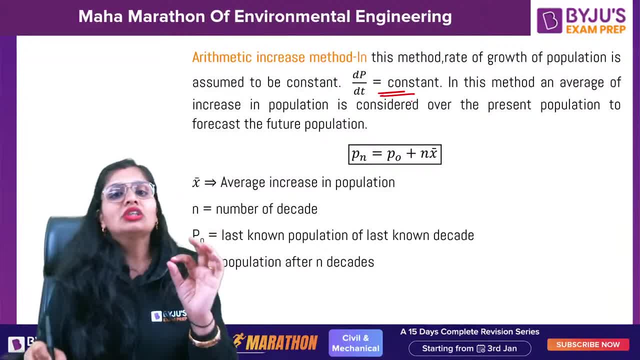 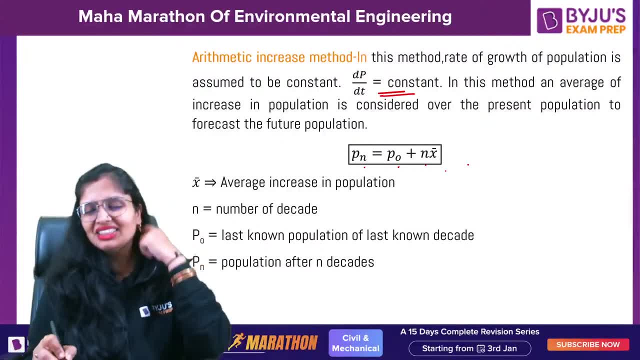 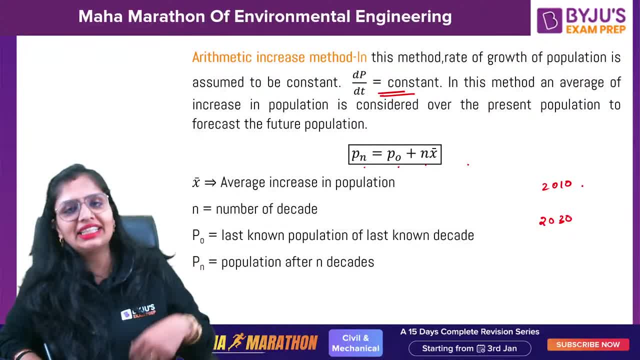 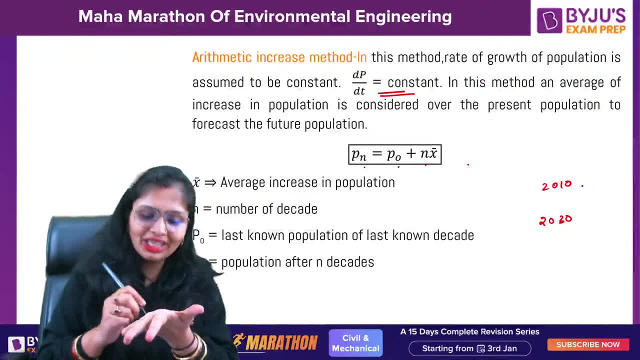 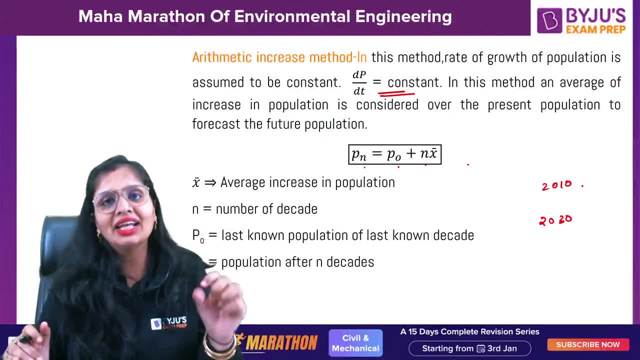 call it as Jann Ganna. So they come to your home. how many are males, how many are females, how many are females, how much they are educated. So everything is mentioned, Basically taking the data, and it is mentioned in the census. So every ten years, the census is being taken. So 2010, if let us suppose, was the last recorded census and you need to forecast operating the population in 2013.. Now first question comes: when do we need to forecast the population of Pn in 15, 15 years or near? So what I mean is commonkay Last population. 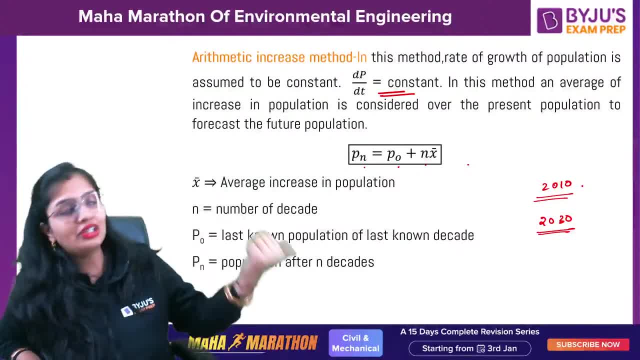 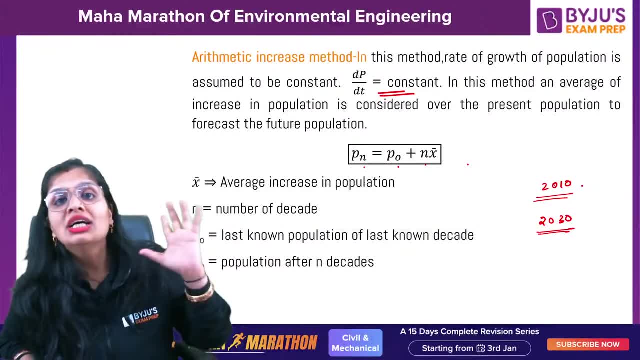 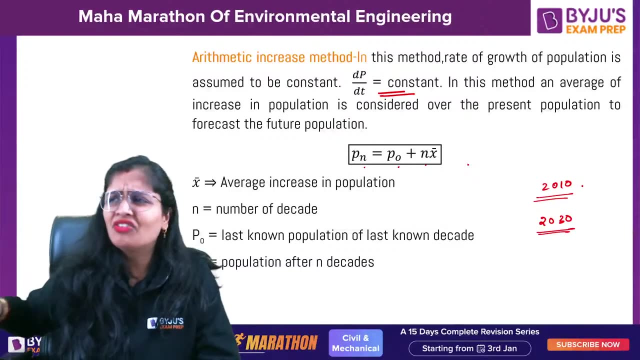 the population. because if you design the water pumps and canals or service reservoir for present condition, your whole this equipment will fail. because obviously it is by default true that next time the population will increase- worst cases happens, like covid and all then only the population will decrease. otherwise, 100% chances are there that it will increase. okay, so that is. 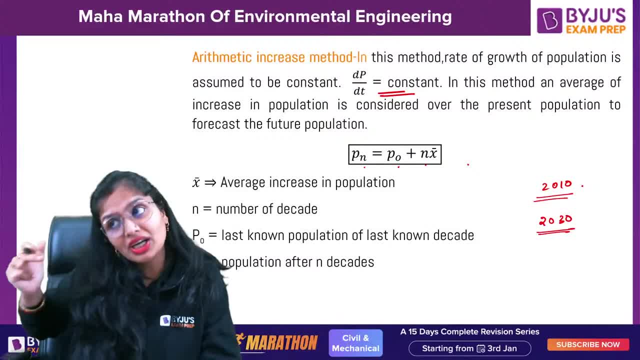 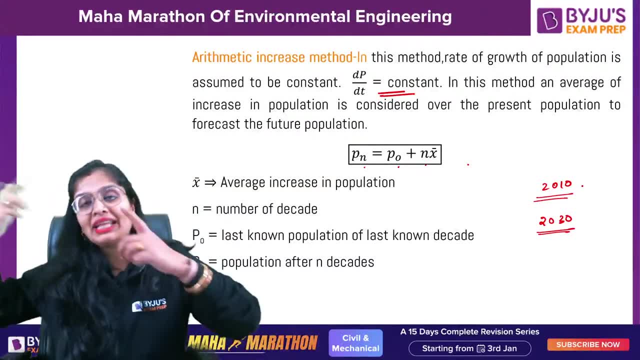 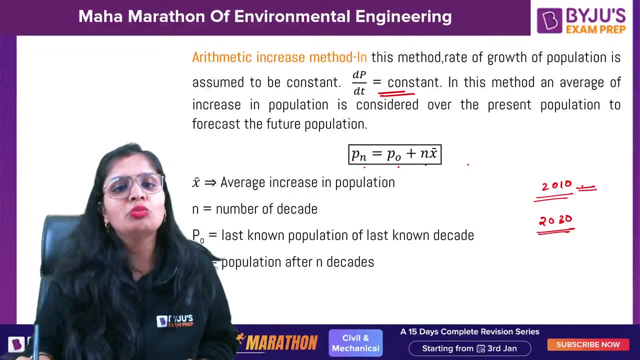 the reason. that is the reason we design it. we forecast is like: suppose, if we design it for 50 years, after 50 years, whatsoever is the population? keeping that in mind, we are designing it today. okay, so that is the thing. so 2010 is the last known population, so it will be p0. 2030 is the 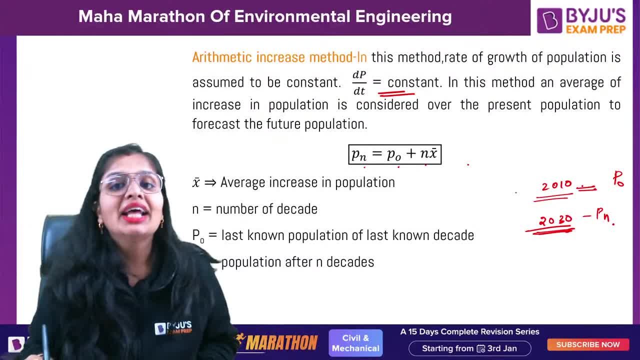 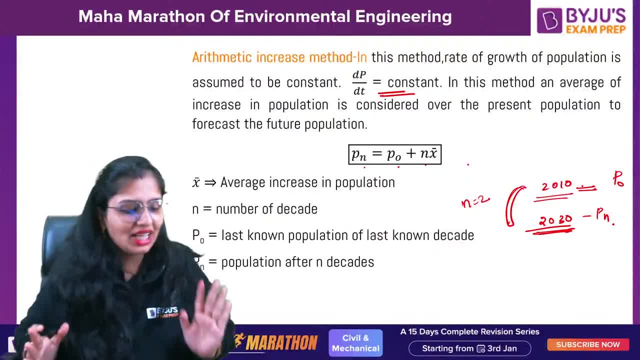 20 years, so n is 2 and x bar is 20 years. so n is 2 and x bar is 20 years. so n is 2 and x bar is 20 years. much increase in population on average basis has taken place, just like china, russia. yeah, that's true. 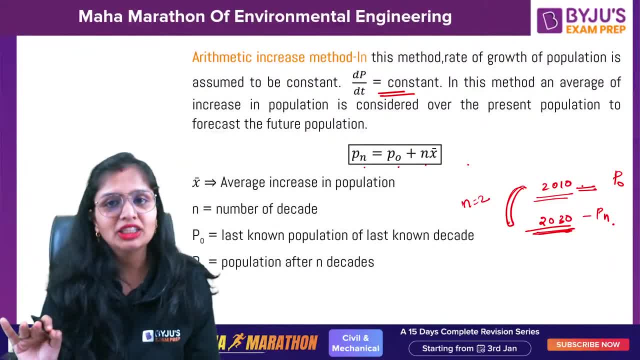 okay, so this is the arithmetic increase population. you use it for old cities nowadays or in the examination they will say: compute the population in this method. in this method, what is assumed rate of growth of population is assumed to be constant. they will not mention arithmetic increase method. 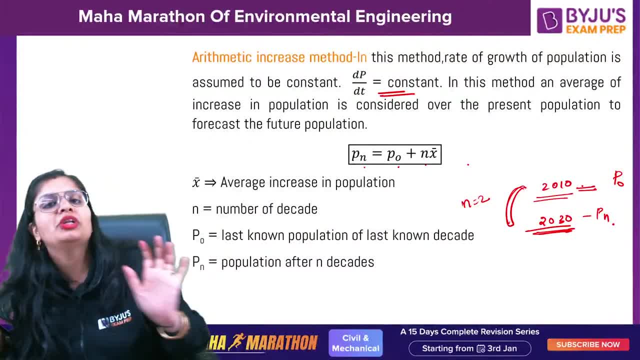 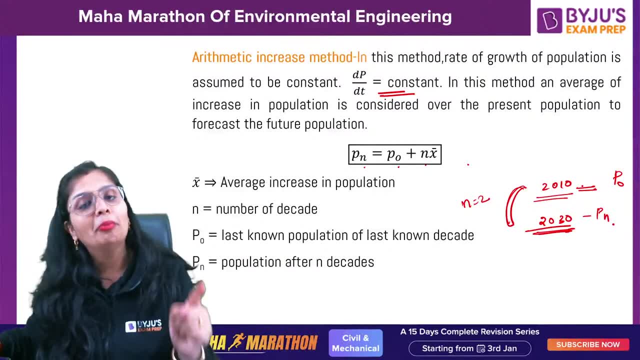 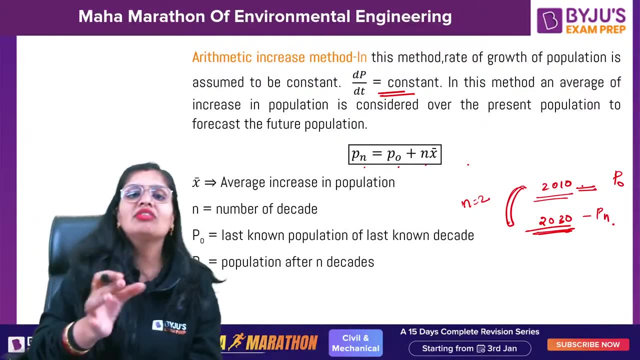 they will mention assuming, Assume rate of growth of population is as a constant. If they mention like this: remember this is practically not true, But in arithmetic increase method this assumption is taken And if in the quotient they mention this line, you have to go for arithmetic increase method. 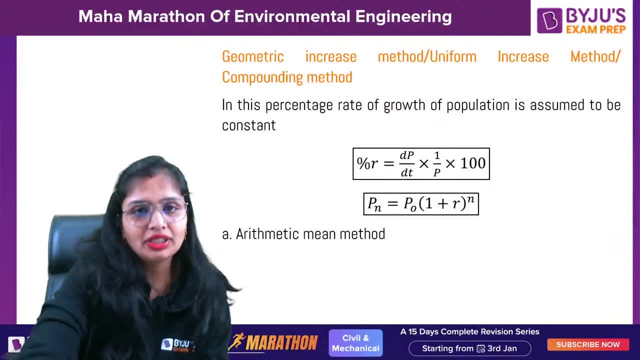 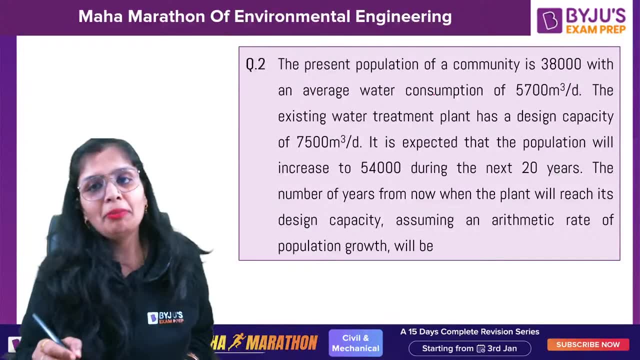 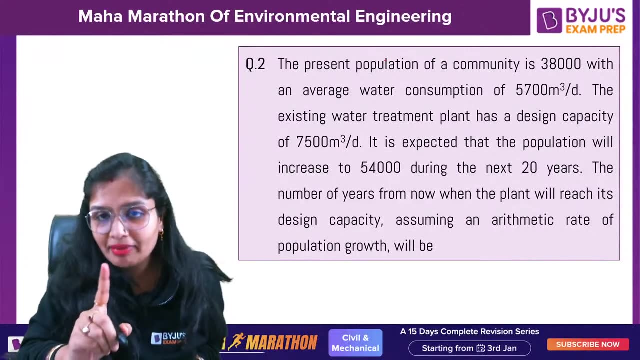 Okay, Now let's solve this quotient. Let's solve this quotient first. Come on, This is the quotient, And similar pattern of quotient has been asked in your GATE examination also. This was a good quotient. Same quotient, dicto same quotient. 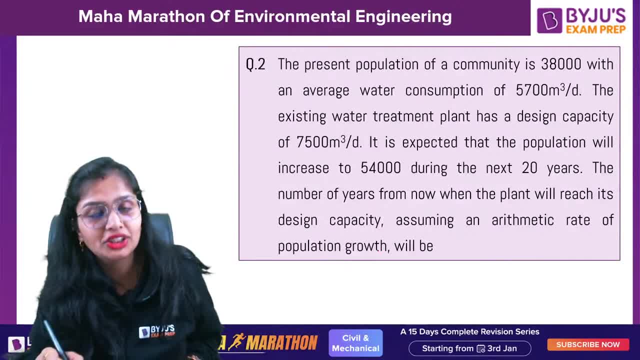 Right now, they told you, assume an arithmetic rate of population growth Dicto. they can ask you for geometric rate also. Okay, I'll tell you where the difference will come. First let us study geometric rate also, Then I can tell you where the difference will come. 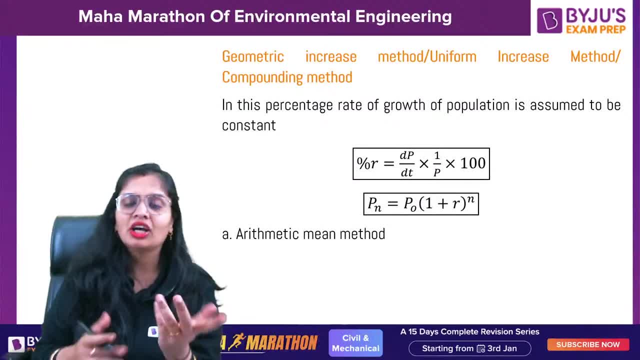 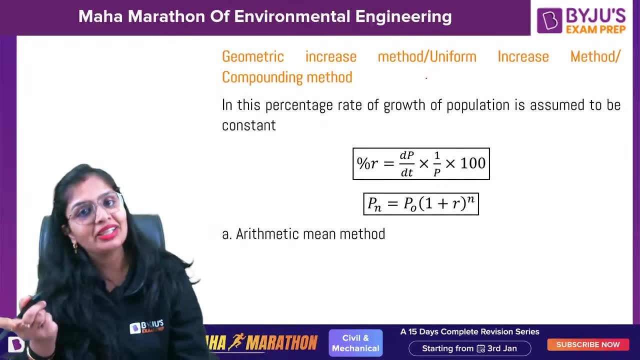 Okay, Because right now they have asked for arithmetic, Now they can ask for geometric also. So geometric, I'll tell you. geometric increase method, uniform increase method, compounding method, All these three means the same. In the arithmetic method, DP by DT was constant. 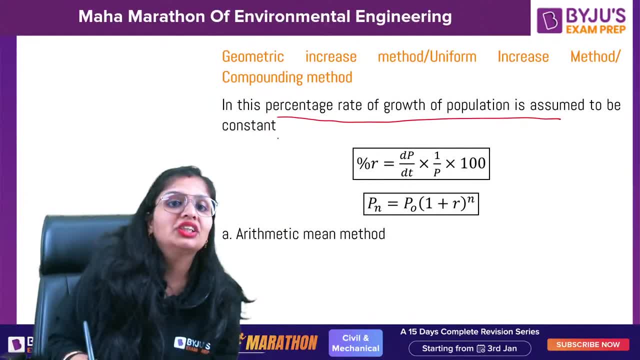 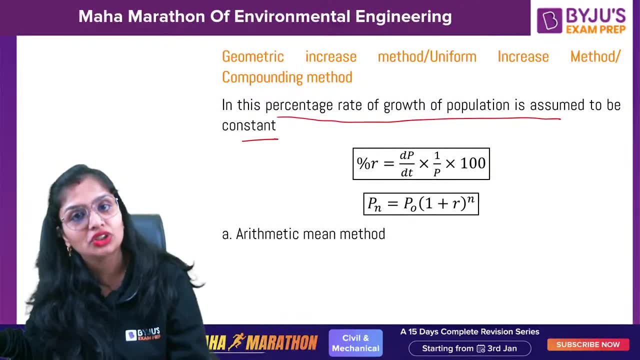 In this percentage rate of growth of population is constant. So again, if they want, they can write this and they will say: compute the population, forecast the population. So you have to apply your brain that this time it is asking to calculate by geometric increase method. 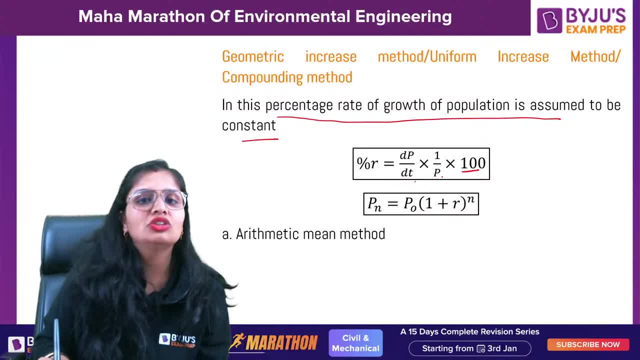 The percentage R will be. Rate of growth is assumed to be constant. So here Pn is equal to P0, 1 plus R to the power 100.. Now, very important thing, Pn is same Population after indicates. P0 is the last known population. 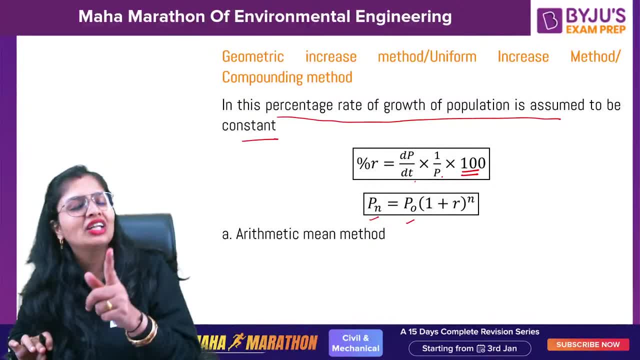 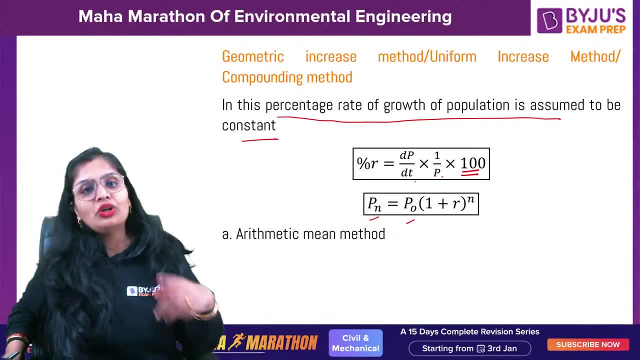 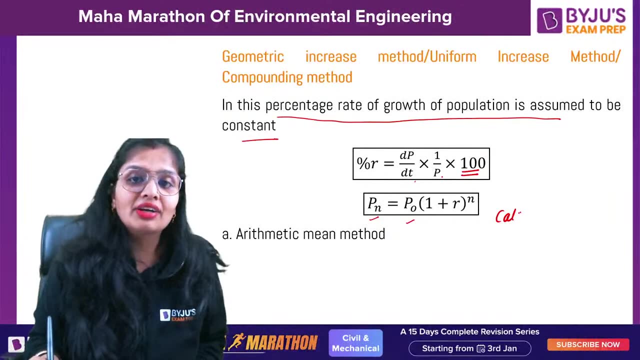 You remember Arun and everybody. you remember. once I told you that formula: revision of environmental engineering. There everybody made a mistake. I told you arithmetic increase method, geometric increase method, But for calculation of, If you want to, calculation of R, that is, percentage rate of growth. 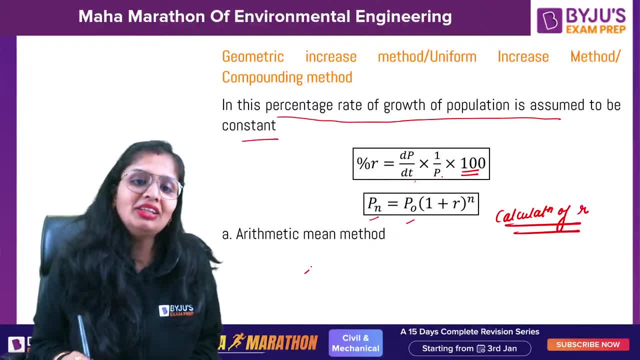 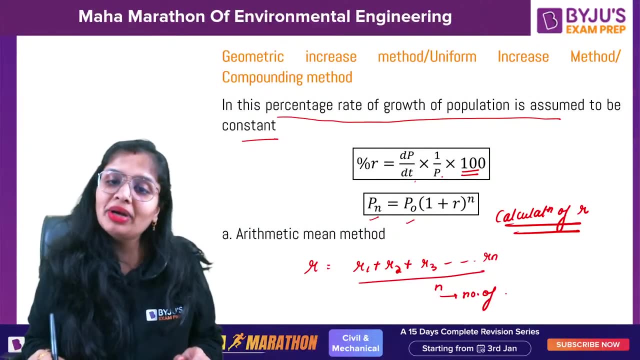 There are two methods. One is arithmetic method, and that is R1 plus R2 plus R3. dash, dash n. Remember this: n is not number of decades, This is number of rates. Now, what do you mean by number of rates? 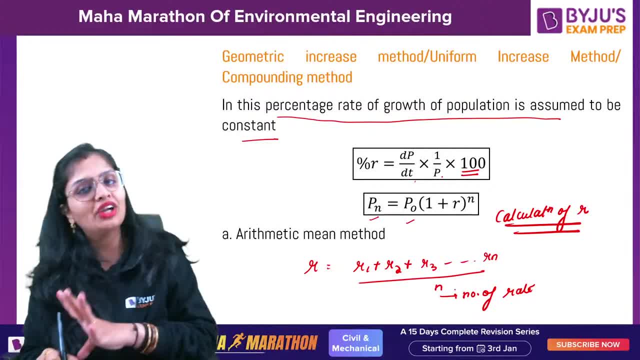 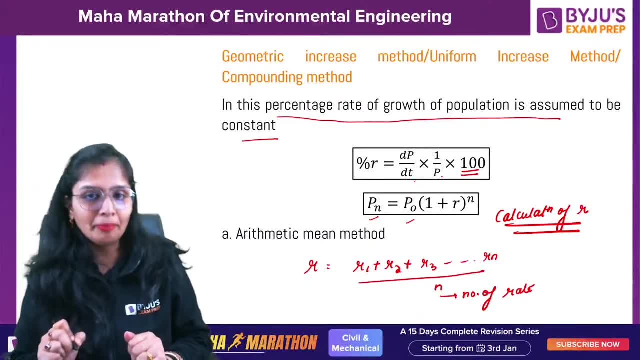 If R is 4, you write it 4.. Like, if 4 R, you have taken, write it 4.. If 5.. If 5 R you have taken, write it 5.. Okay, So this is arithmetic mean method for calculating R. 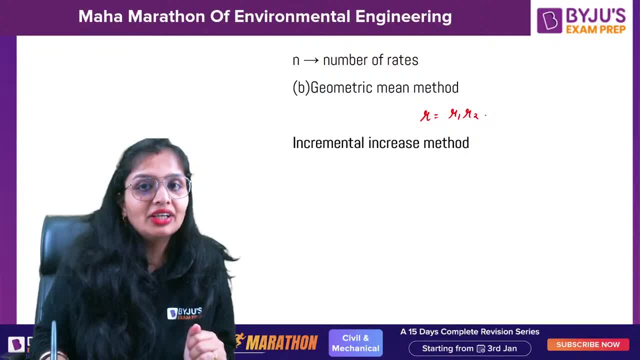 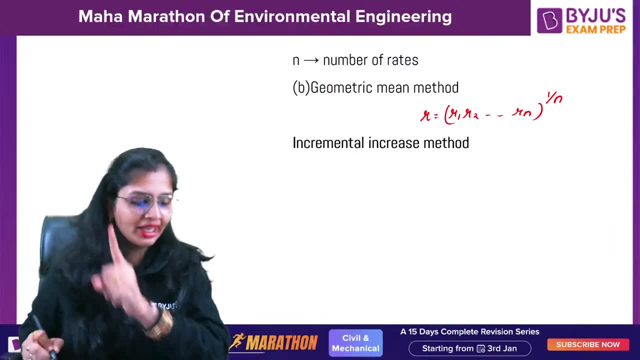 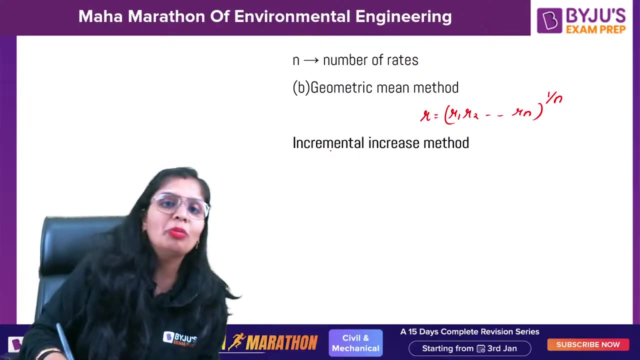 Geometric mean method. R is R1, R2, Rn, 1 by n. This is geometric mean method, Very important. Again, I am telling you a statement. wise thing: If in examination they are not telling you how to calculate R, go by geometric mean method. 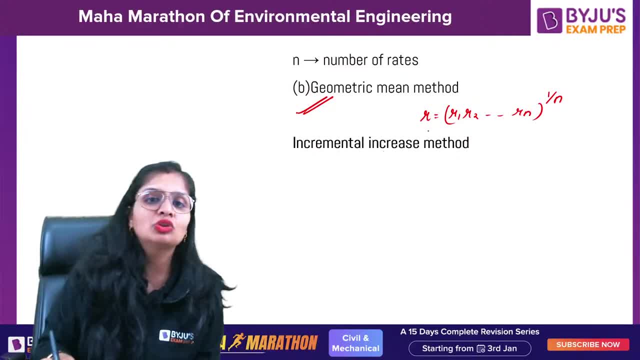 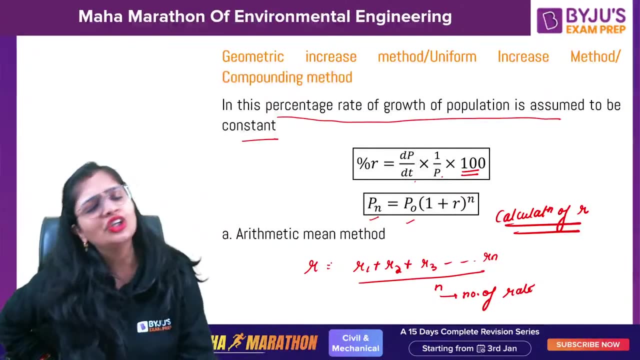 Because because, as per your code, It has told to take the R value as geometric mean method. If you go in the field and all, or if any interview question comes there, generally maximum times the engineer takes this value to calculate. Now you will say, mom, it is cheating. 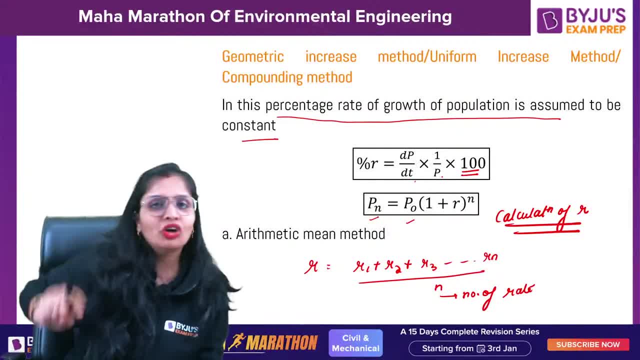 In the code it is telling you to do by geometric mean method. You taught us this, But when we went to the field. it is telling us to go by arithmetic mean method. What is this discrimination? Reason is: by arithmetic mean method. 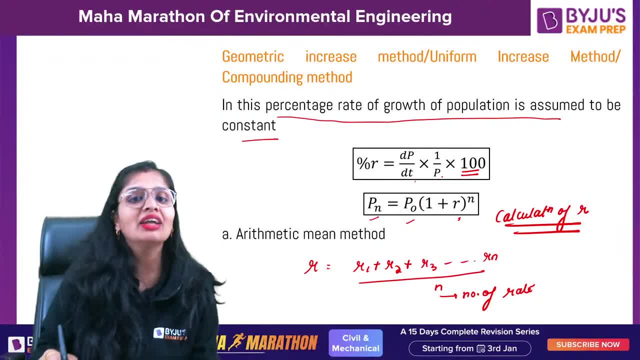 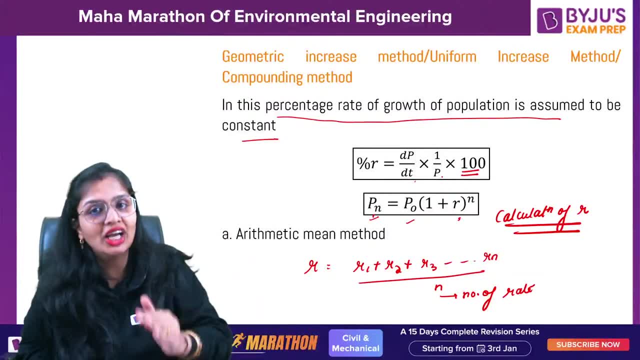 You get More value of R. More value of R means more value of the predicted population. Everybody wants to be on the safe side. The engineer in charge, who is doing all this calculation, also wants to be on the safe side, So he forecast more population. 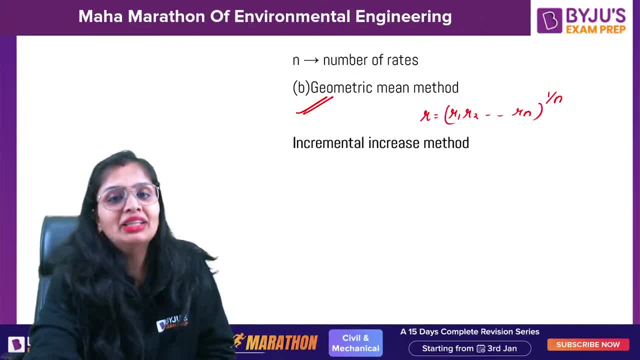 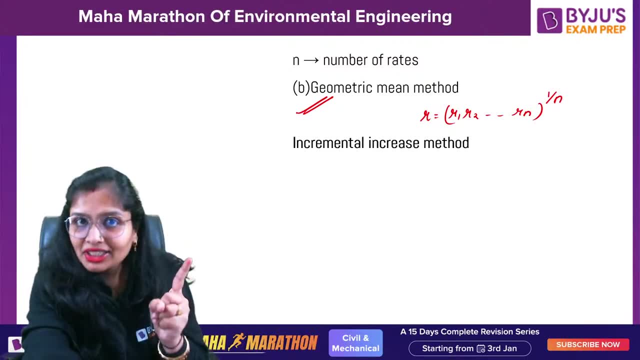 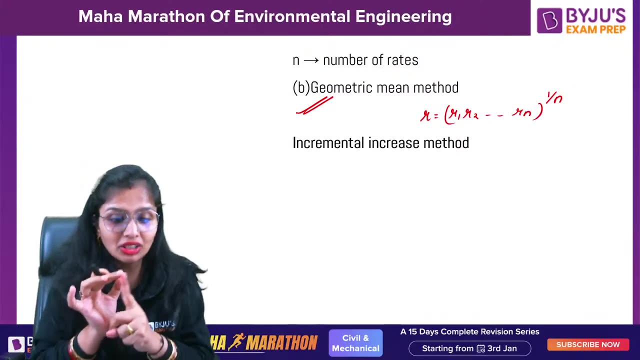 That's it, Okay. So these are the method of calculating. If not mentioned, go for geometric mean method For calculating R. Remember arithmetic increase method, Geometric increase method As method For population forecasting. Arithmetic mean method and geometric mean method are method for calculating percentage rate of growth. 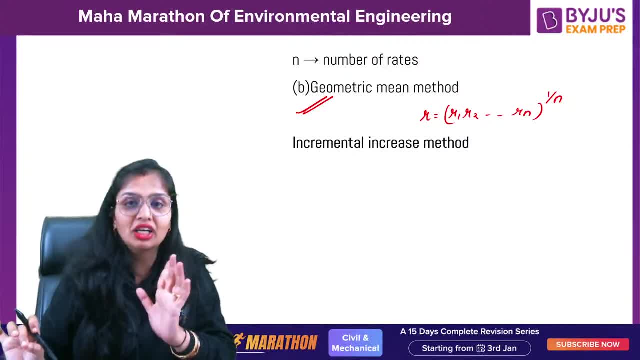 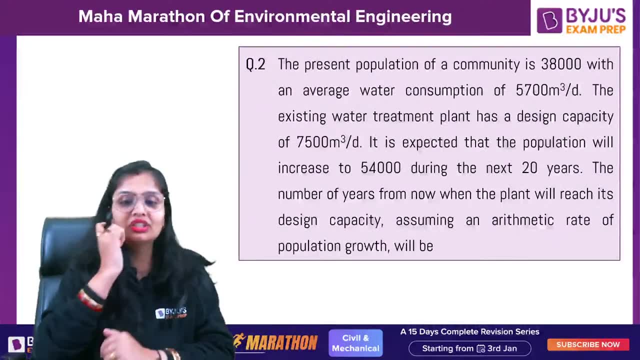 That is R. So there is a difference between the two things. Don't get confused, because you guys got confused in formula revision also. Now let's talk about this question First. I will tell you first. I will tell you by arithmetic and I'll tell you where the changes will be. 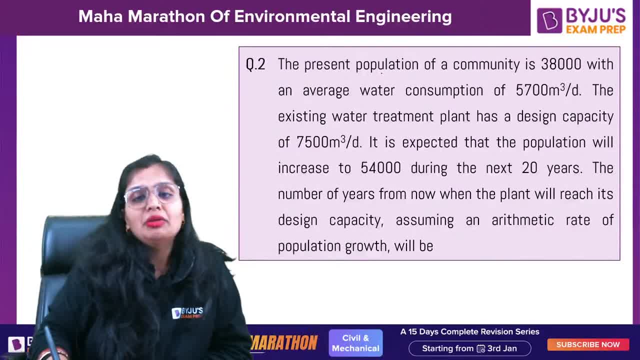 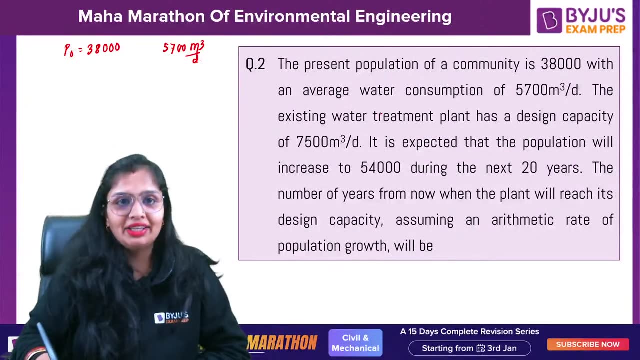 There is same portion is asked by geometric method. The present population of a community Is 38,000.. Okay, fine, And average water consumption is 5700 meter cube per day. Now the existing the water consumption is 5700 meter cube per day, but the plant has a design capacity of 7500 meter cube per day. 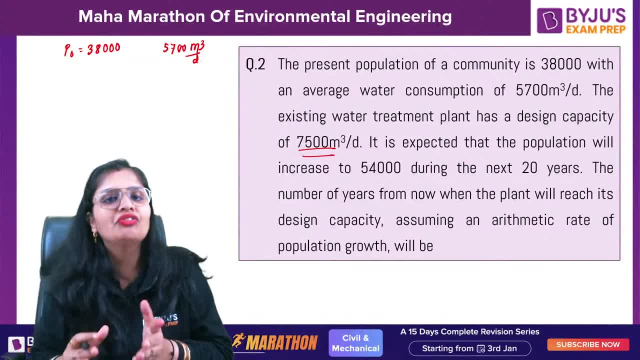 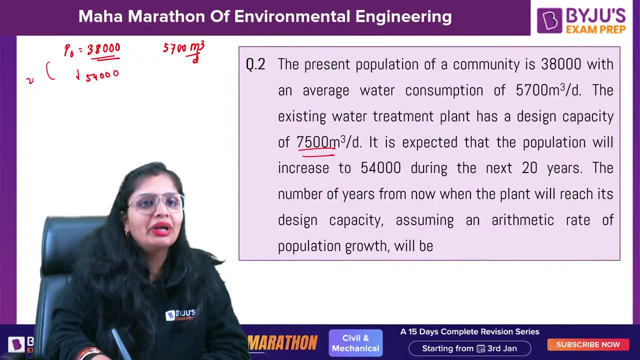 And it is expected that the population will increase to 54,000.. So right now, if the population is 38,000, it will increase to 54,000 in the next 20 years. So let us suppose Pn is equal to P0 plus an X bar. 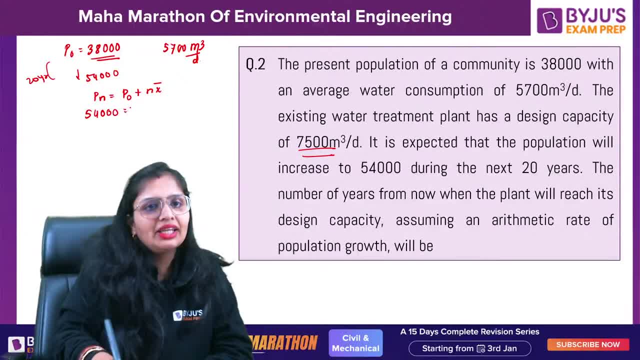 In the portion it is giving me that 54,000, and here it is 38,000, and it will increase in next 20 years. 20 years means two decades, because one decade is equal to 10 years. So can you calculate, guys, and tell me what will be the X-bar? 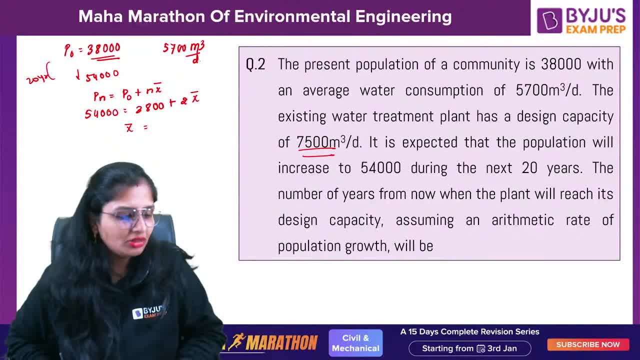 What will be the X bar? Yeah, arithmetic mean is greater than What will be the X-bar. Yeah, arithmetic mean is greater than What will be the X-bar. Yeah, arithmetic mean is greater than What will be the X bar. guys, Faster, faster. 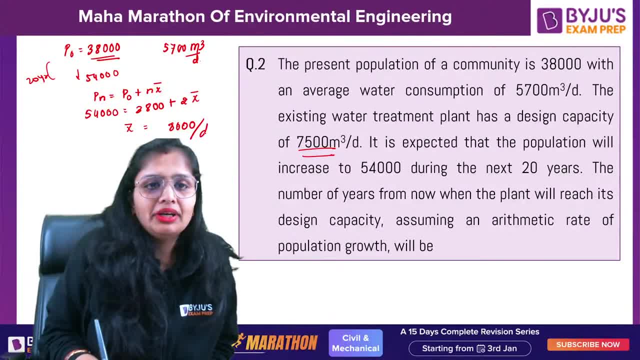 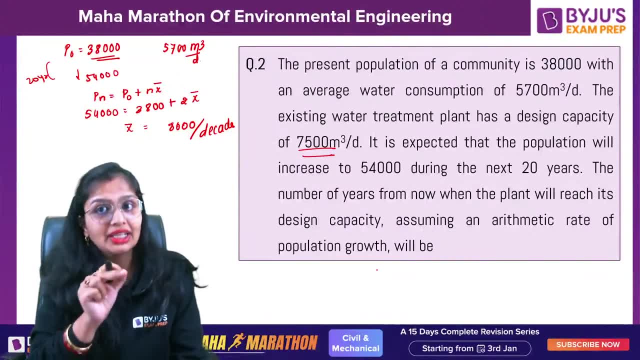 8,000.. So 8,000 per decade. Now in the question it is not asking me X bar, It is asking me the number of years from now, that is, from 38,000 population. What will be the number of years when the plant will reach its design capacity? 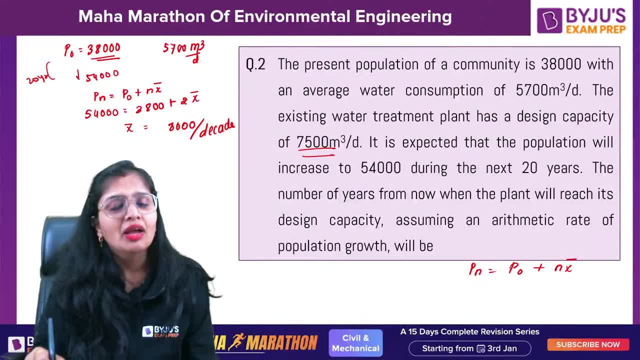 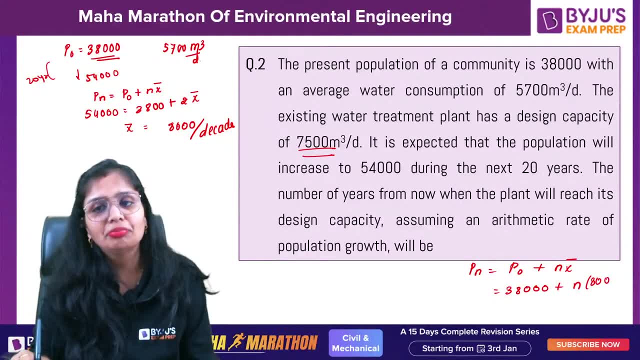 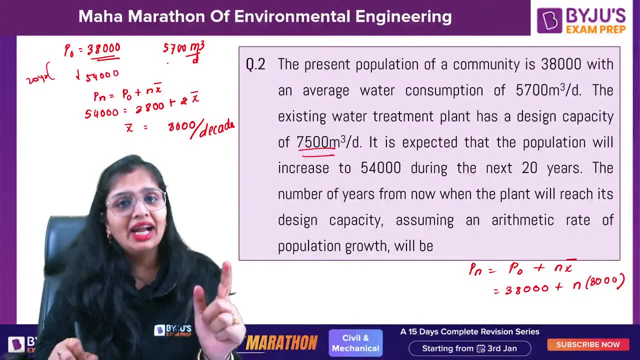 So Pn is equal to P0 plus NX bar P0. I know 38,000.. Number of decades: I need to calculate X bar. I already know 8,000 per decade. So let us suppose right now: if 5700 meter cube per day is the demand and 38,000 is the people, what will be the demand of one person? 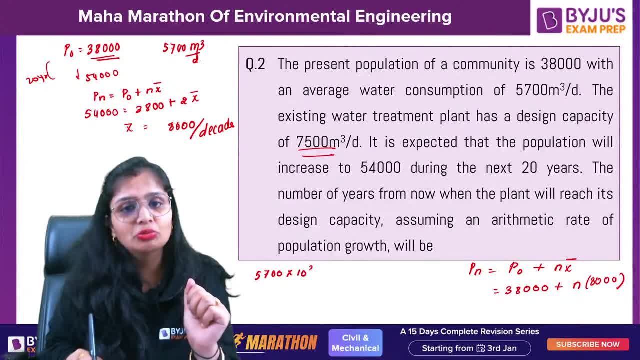 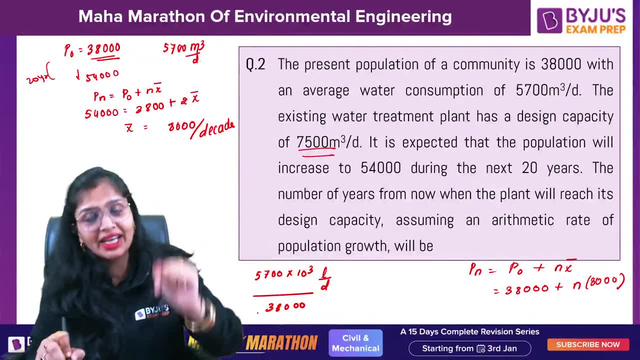 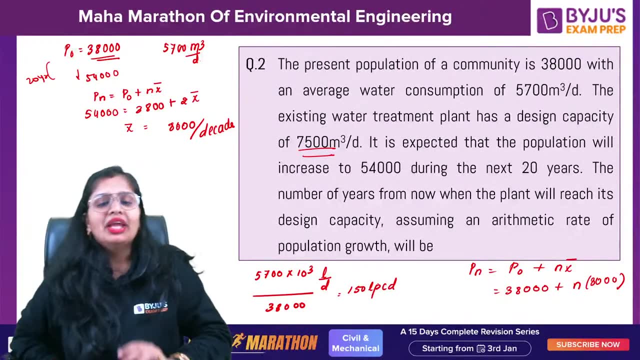 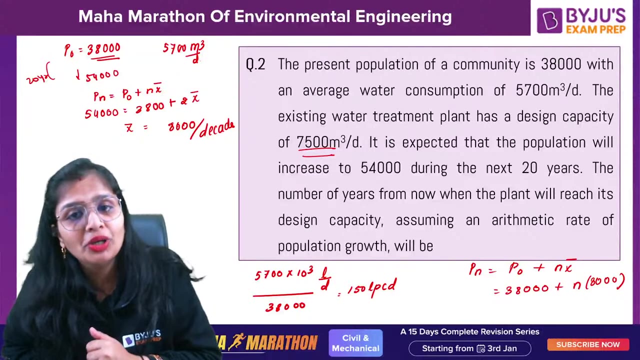 So 5700 meters, That is 10 raised to power, 3 liters per day divided by 38,000.. This will give me the demand currently for one person one day. It comes out to be 150 LPC. Now if 150 liters is the demand for one person for 7500 meter cube per day of demand, how many people's demand is there? 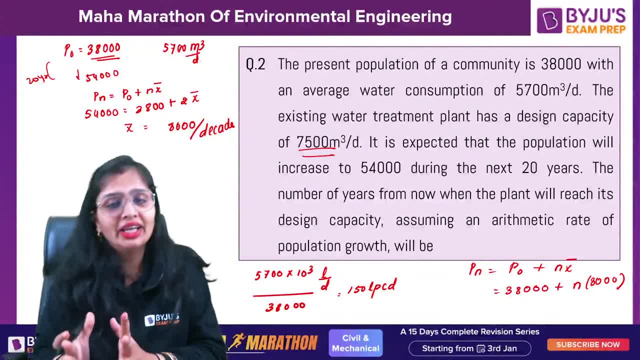 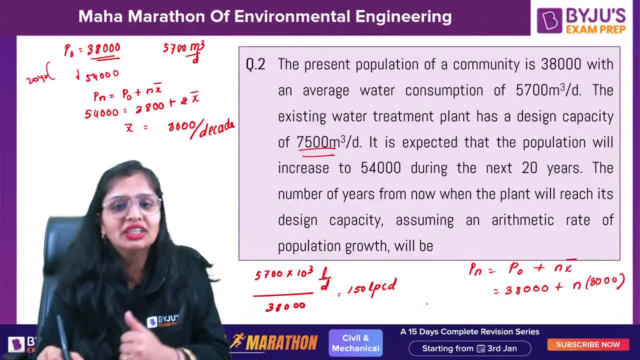 Or you can say how much population has to be there. The demand becomes 7,500 meter cube per day. So you can calculate this. just reverse it. how you reverse it: 7,500 into 10, raised to power, 3 liters per day divided by 150 LPC. go through the units. 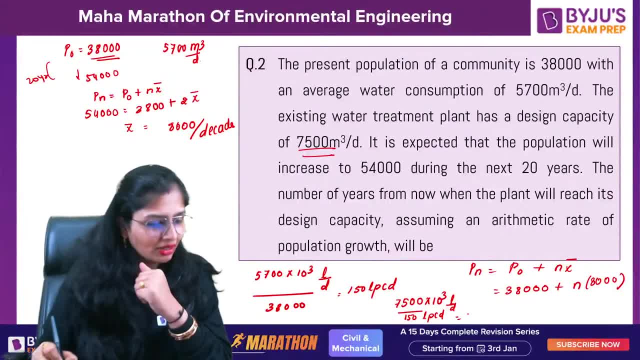 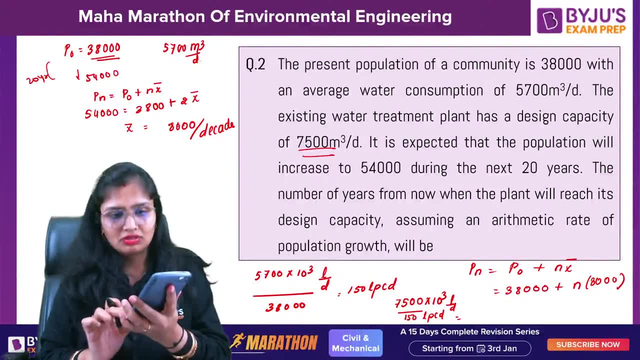 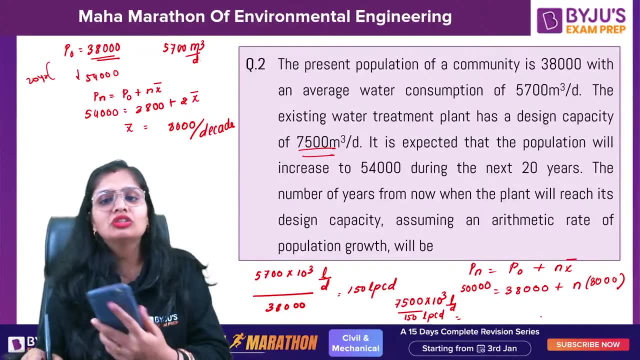 This will tell you how many population is there. Tell me calculate 7.. 7.. Let me see it again: 7.. 7,500.. 50,000, 2, 3, 4, So you will solve it. 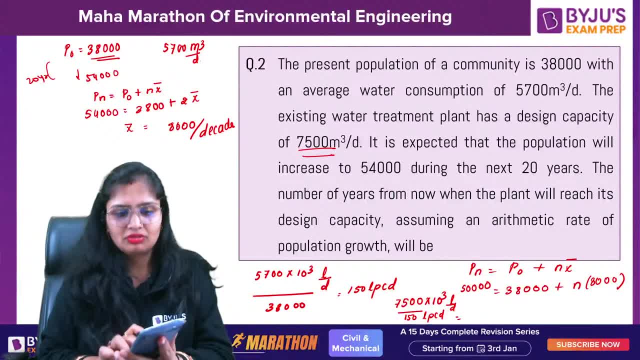 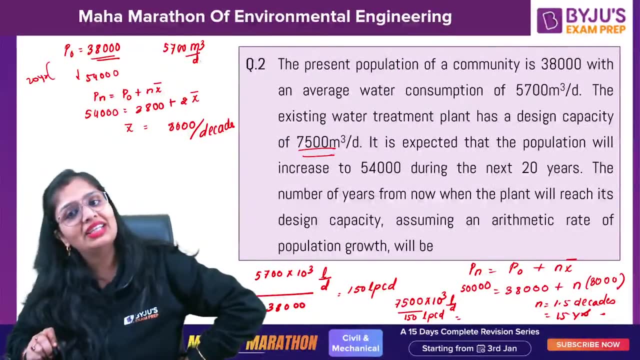 This will come out to be how much? 1.5 decades, That is 15 years. Okay, If you want similar question, they can ask you. Only difference will come. They will tell you geometric method. This will remain same. This will remain same. Only change will be done is: 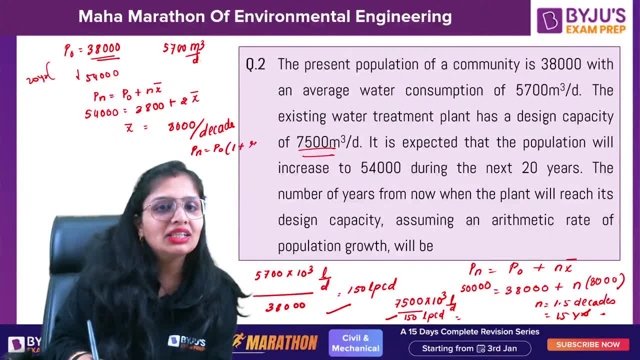 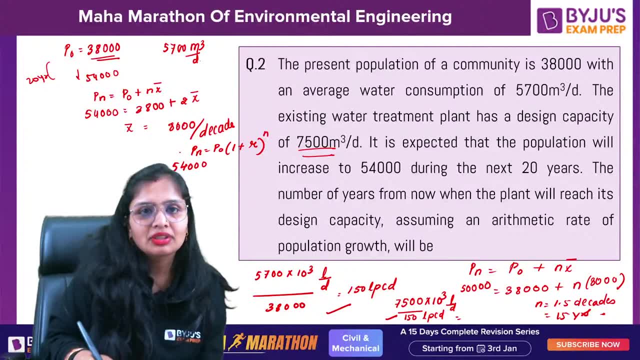 Pn is equal to P0, 1 plus R into N. Okay, In this question, this will be 54,000, This is 38,000, This will be 38,000. Okay, You need to calculate R And this is 2. Okay, So from here you will calculate R. 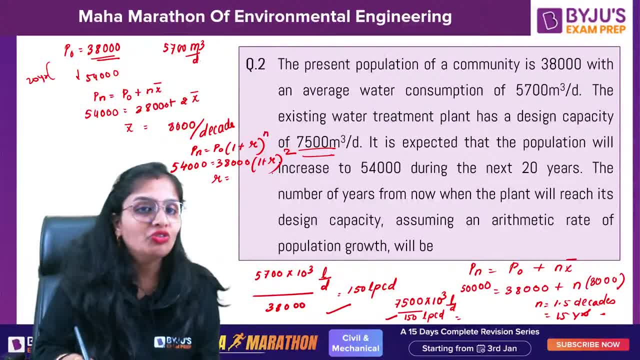 If this question would have been in geometric increase method. So with the help of it you will calculate R here And again you will get, You will use this formula: Pn is equal to P0, 1 plus R into N. Okay, And here you will substitute 50,000. 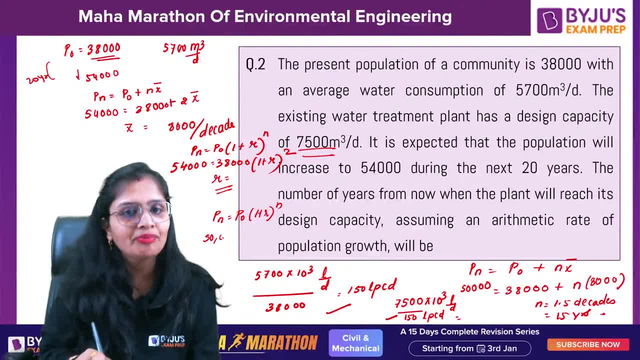 As it came, 38,000, 1 plus R to the power. N R you already calculated You will get N, But this time you have to use log For calculating the value of N. So everything concept will remain the same, Only the formula will change. Clear everybody. 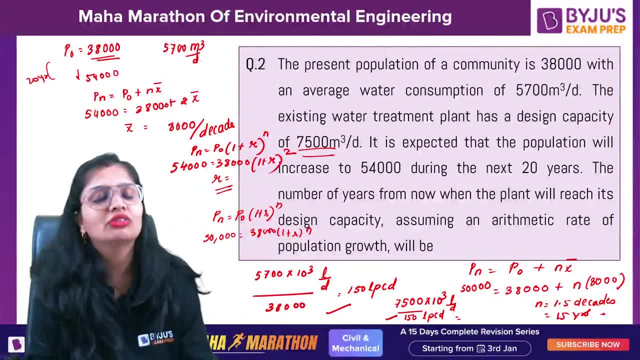 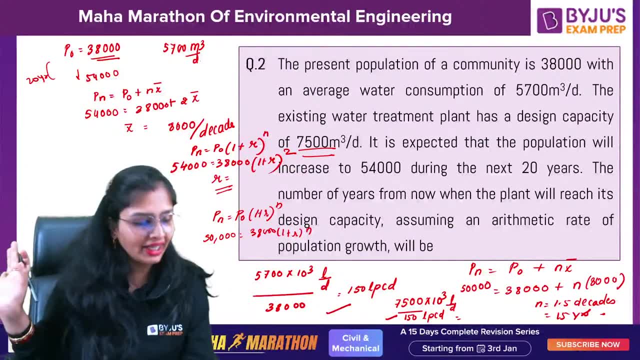 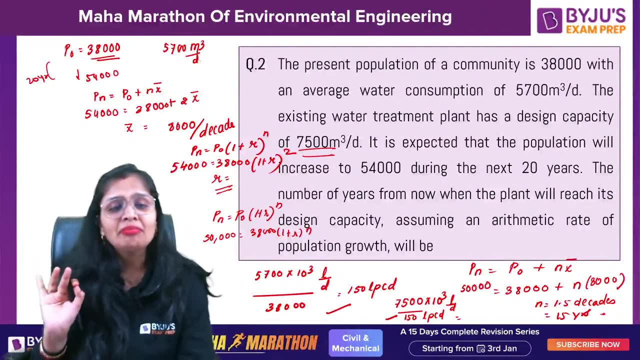 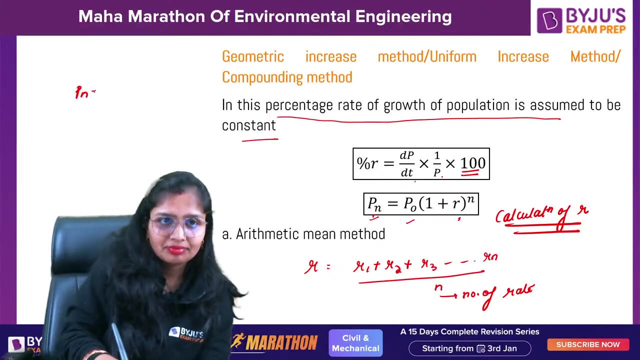 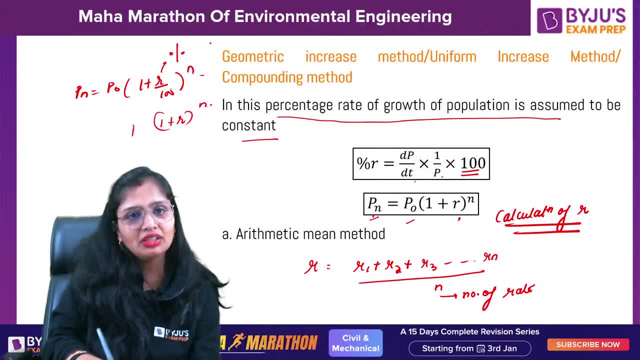 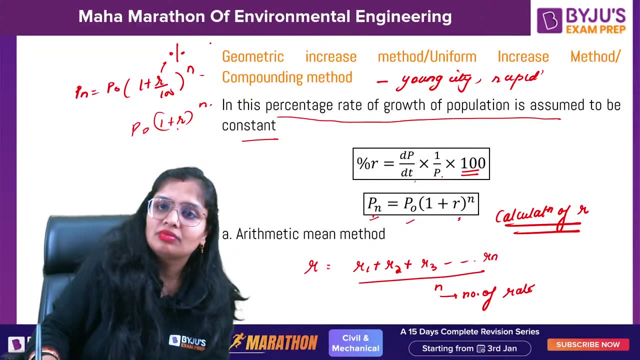 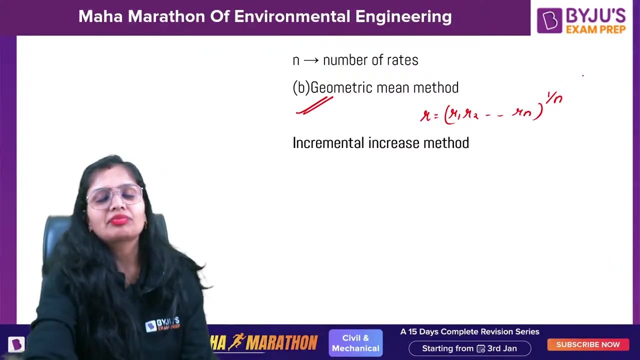 If they write like this, You have to Substitute R in decimals. Okay, So this you should. This is geometric increase method. increase method. this is used for young cities, or you can say, rapidly growing cities, remember, okay. now coming to incremental increase method, always remember: geometric increase method gives. 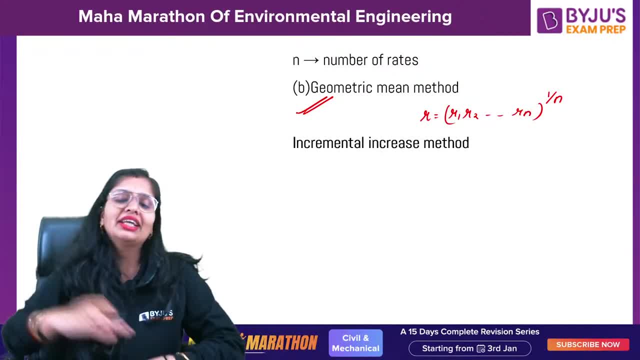 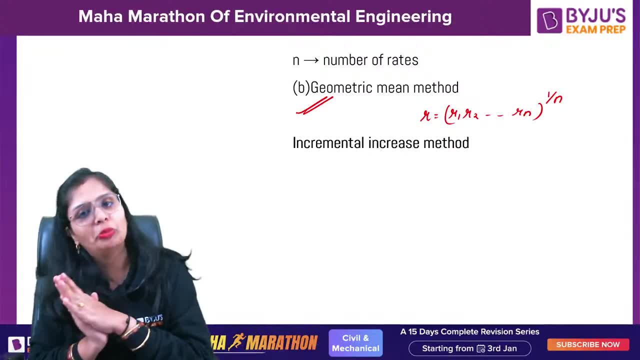 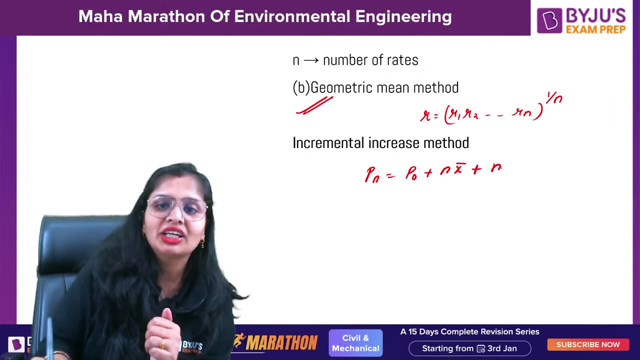 you a higher value of population forecasting. arithmetic increase method gives you a lower value of population forecasting, but incremental increase method gives you a moderate value of population forecasting. okay, if you remember, there was one question asked in gate examination where they didn't mention which method to use. okay, and generally it was done by incremental increase. 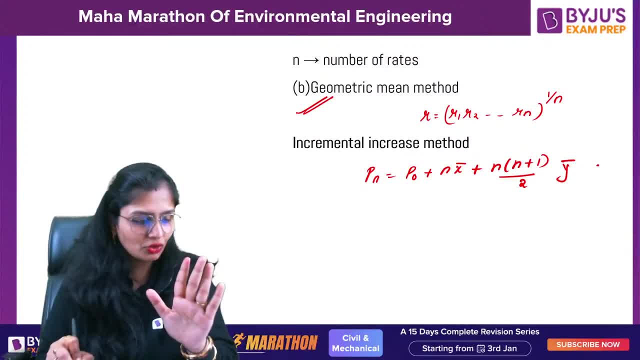 method, but don't worry, nowadays they won't ask that sort of questions with you. so pn population after n decades. p- not last known population. n is number of decades, x bar is, as already told you, how much is the population value of population forecasting and n is number of decades. 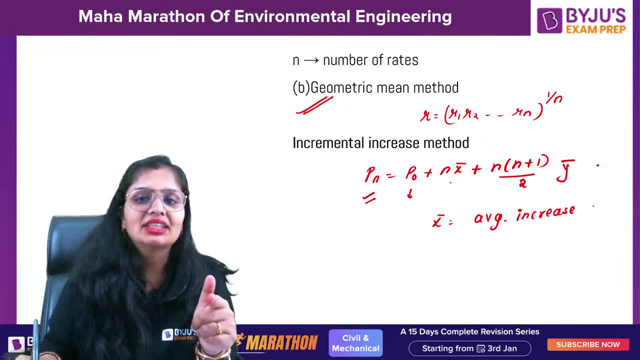 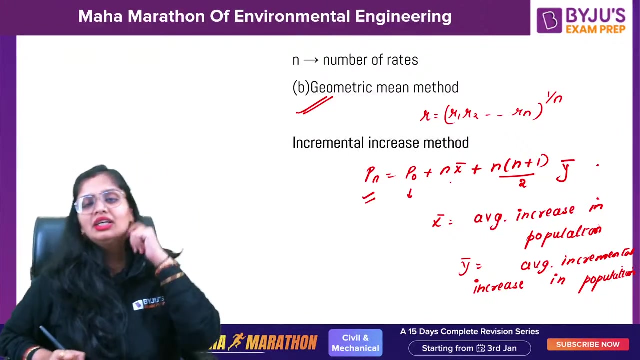 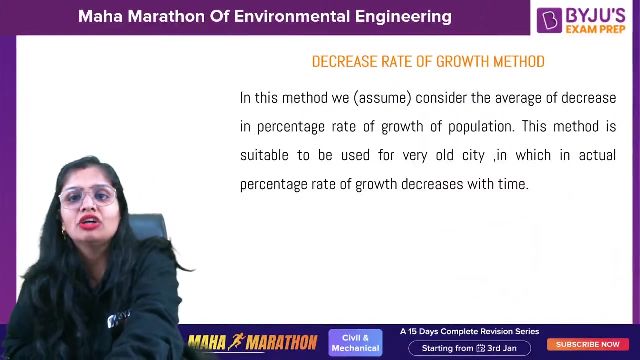 much on an average basis. population is increased. So average increase in population and y bar is how much increase in average has taken place. So incremental increase in population. So this was till here. now talking about decrease rate growth method, this is very important. 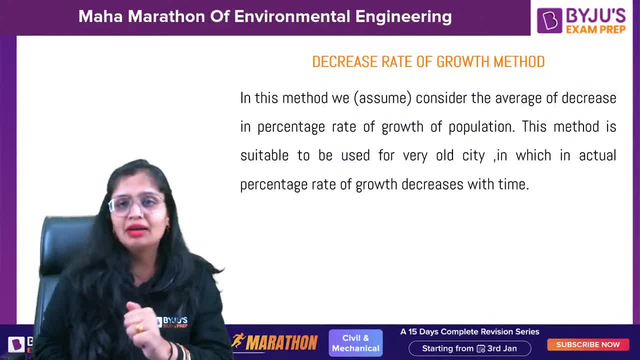 because what is happening? let us suppose I give you this example. let us suppose initially Girish example I'll take. Okay, Girish used to eat two chapatis. then I said: Girish, I'm cooking food for you. Is there any other word? that's in the middle of the sentence. 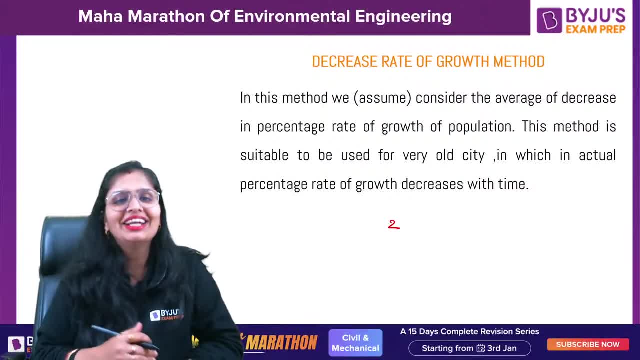 Okay, so Girish used to eat two chapatis. then I said, Girish, I'm cooking food for you. Is there anything that's in the middle of the sentence? you are my good student. you topped the examination, treated on my side so fine. we went to the hotel. 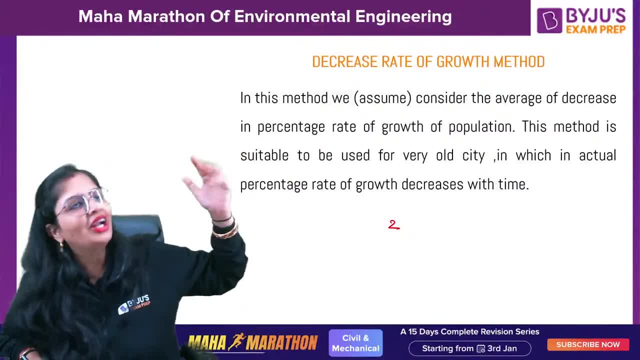 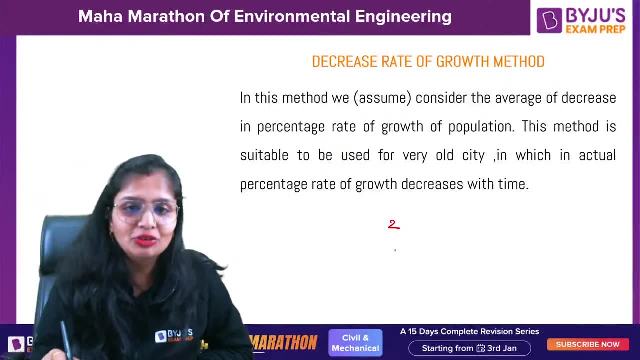 because Girish scored AIR rank 1 and I told him that order. so Girish told that, ma'am, my diet is 2 chapatis. I will say: no, today is your day, eat 4 chapatis. so he ate 4 chapatis then, Prince also. 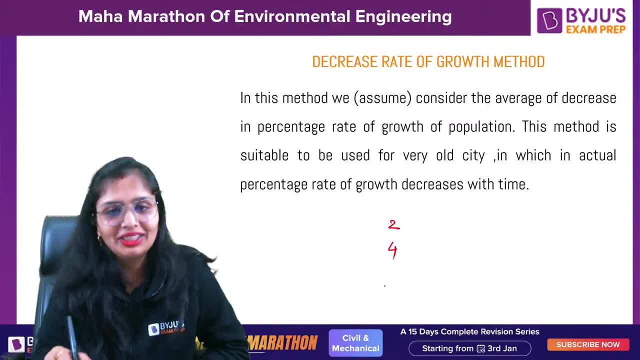 said: bhai, today is your day, eat 1 more chapati. so then he ate 5 chapatis. so initially Girish diet. increased to how much percentage? 50 percentage and then from 4 to 5, the Girish 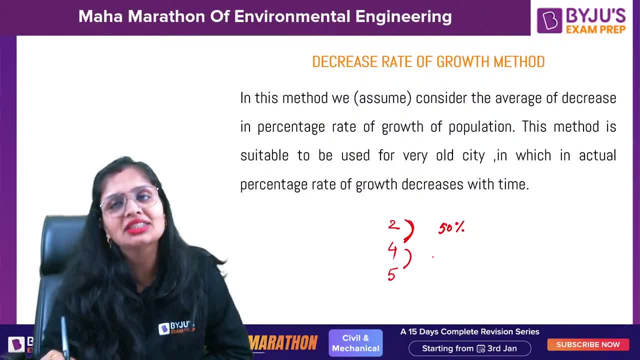 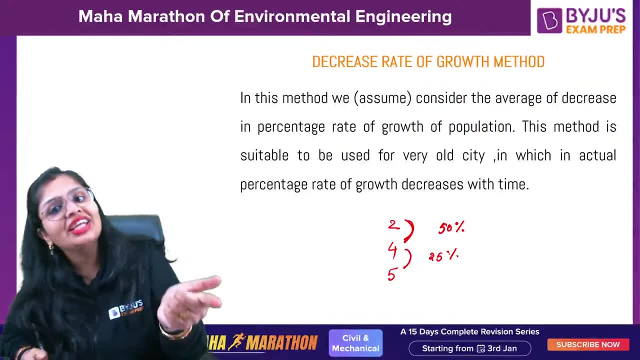 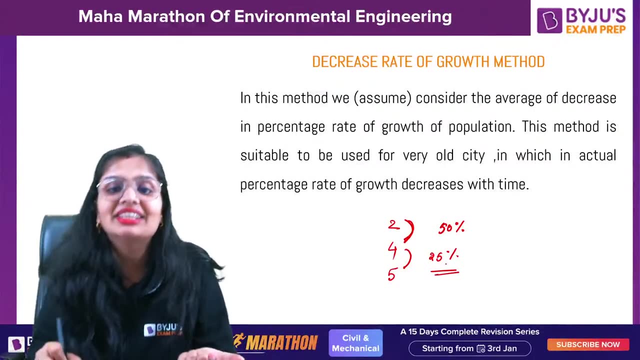 diet increased. to how much percentage? 1 by 4 into 100, that is 25%, right? so what is happening? what is happening? the diet of Girish is increasing, but the percentage at which its diet is increasing is decreasing. getting it obviously. you can see 2,, 4,, 5, the chapatis. 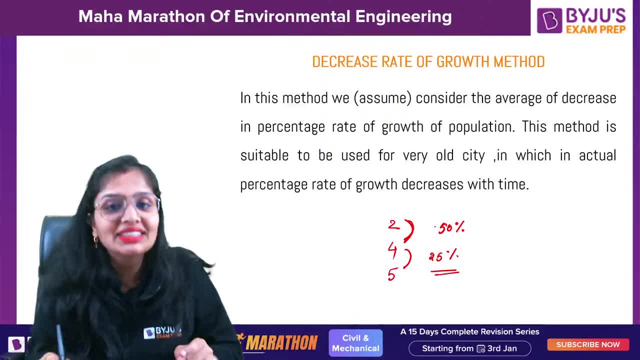 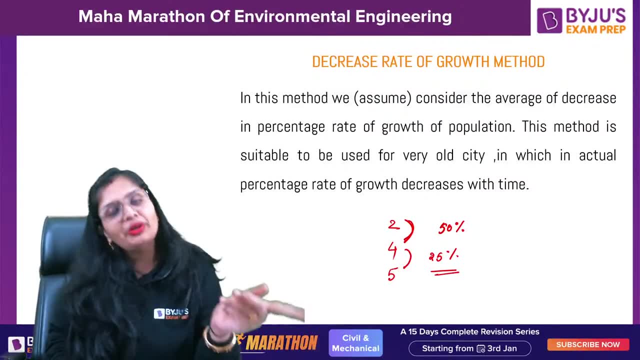 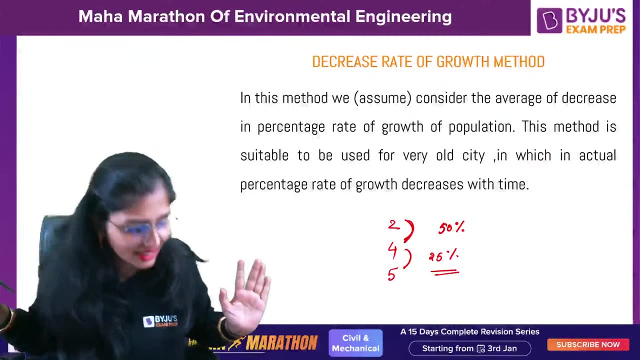 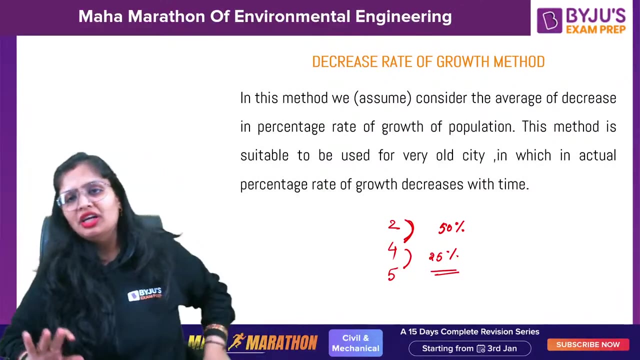 which he is eating is increasing, but the percentage is decreasing. similarly, when you talk about decreased rate of growth method, the population increases, but the percentage at which the population increases is decreasing. clear, clear, understood what I meant to say. guys, faster, faster, you can give a thumbs up, don't need to write heavy statements and all. 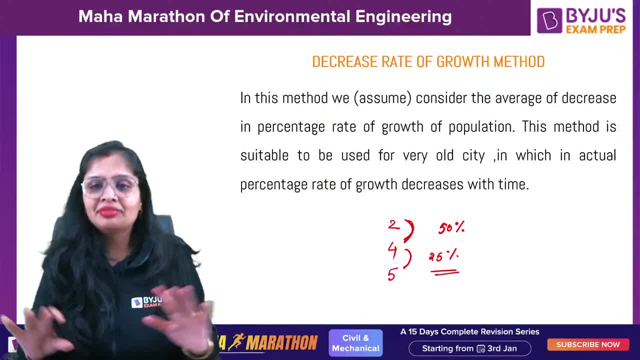 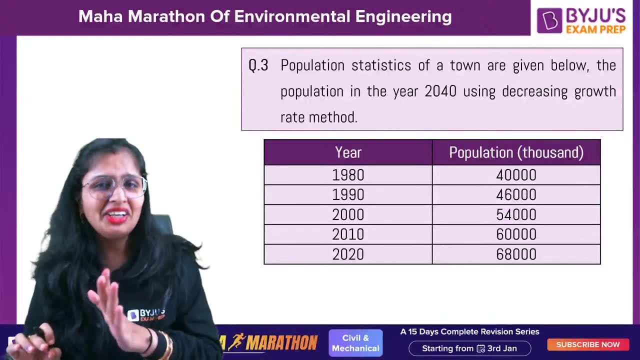 clear, clear, Girish, Girish, Prince, everybody. okay, so now this method. this method is trickier. there is one difficult formula. I didn't wrote it also and I don't want you to remember that formula also. 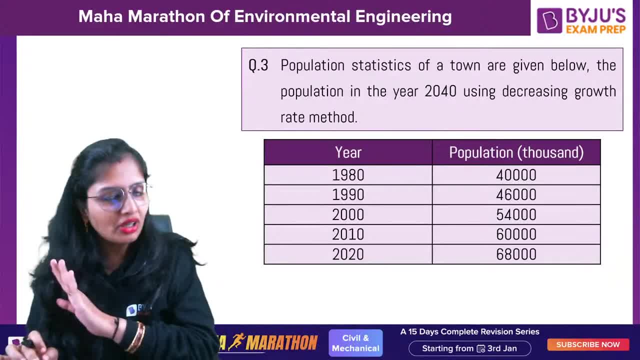 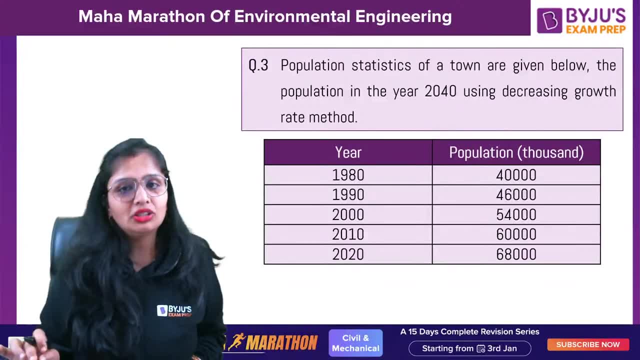 because in civil engineering, n number of formulas are there. don't remember that formula for decreased growth rate method. I will tell you a simple method to solve it. simple method to solve it. how. let's talk about it: 2020 year, the population is. 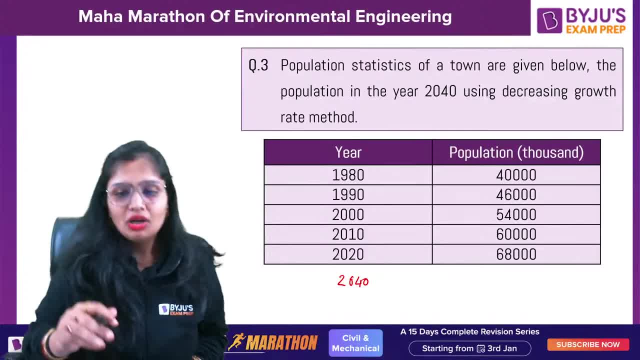 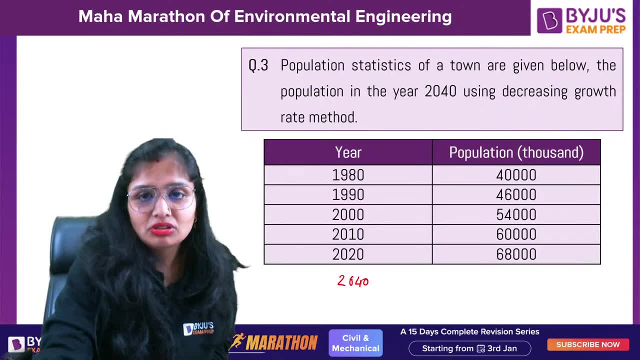 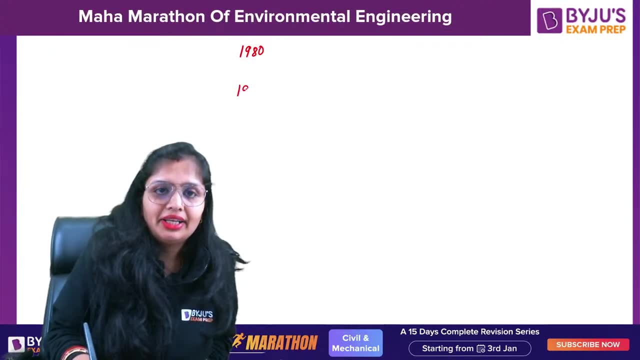 given to you and it is asking you in 2040, okay, now see, I have taken a blank slide because I want to make columns and all. so 1980 till 2020, okay, 1980,, 1990,, 2000,, 2010,, 2020,. 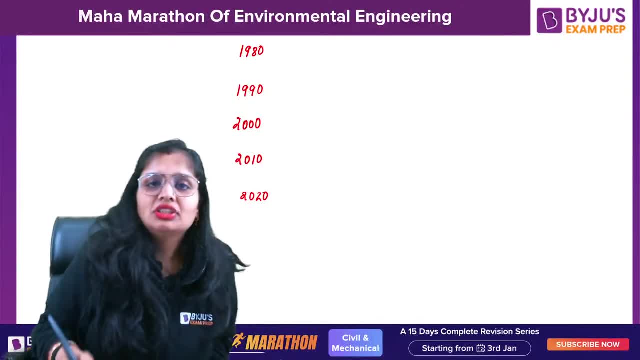 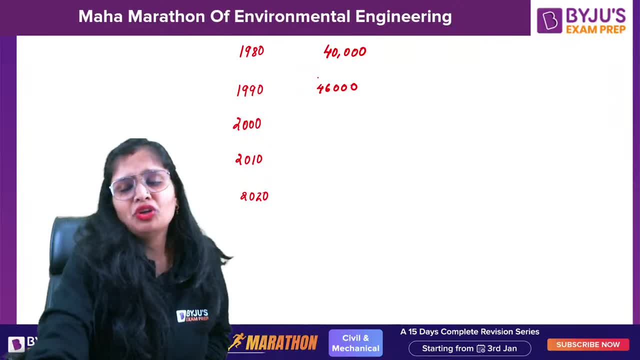 46,000,. if you don't remember the formula, that will be good. only because obviously in your brain lots of more formulas are there. so why to waste time? 60,000, 68,000,, 60,000, 68,000, okay. 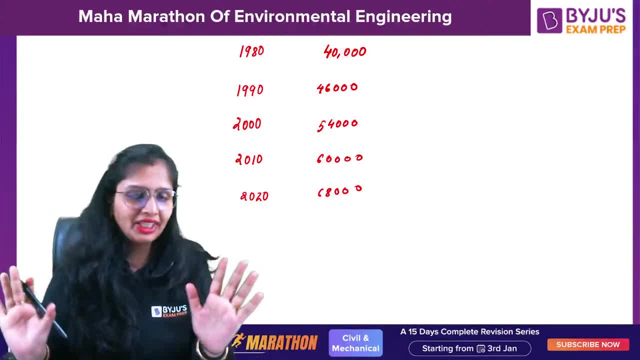 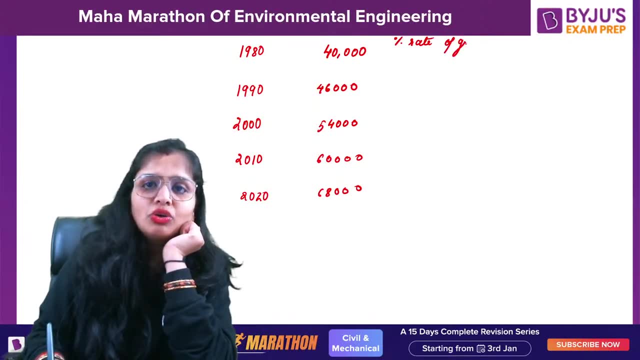 so this is the, this is what this is the population, this is the year. now how to calculate. first, you will calculate the percentage rate of growth, how much growth has taken place, how you will calculate, come on. 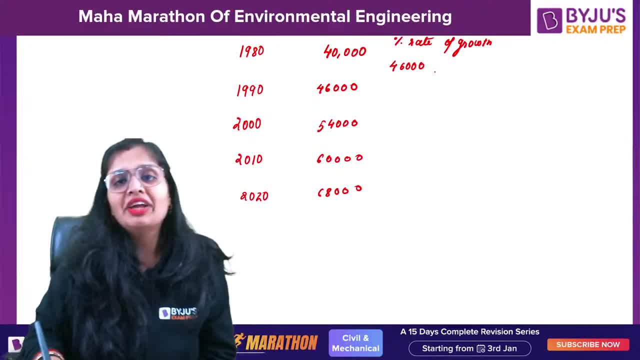 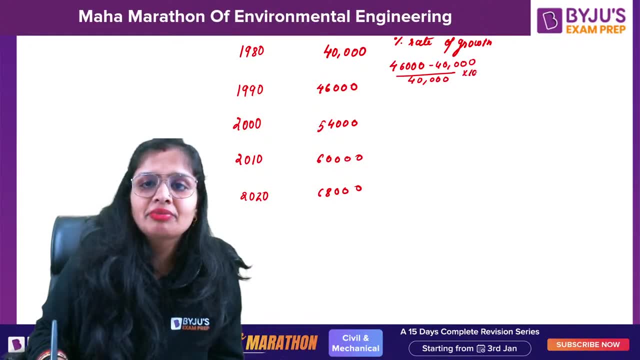 guys be with ready with your calculator, our own MVS, everybody. 40,000 divided by 40,000 into 100, how much it is coming? similarly, 54,000 minus 46,000 divided by 46,000 into 100,. 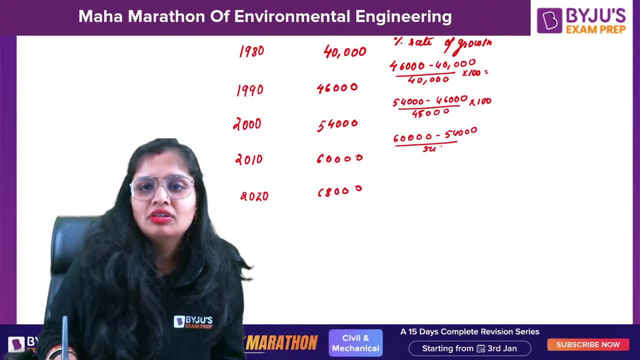 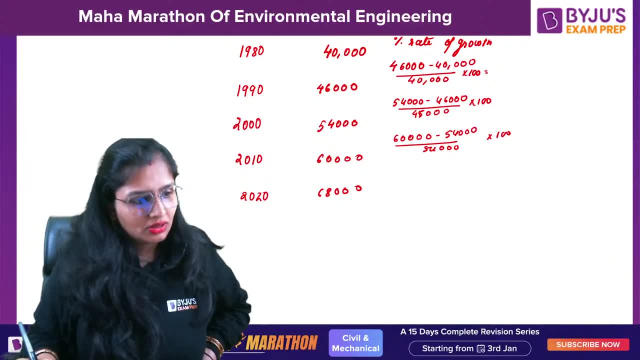 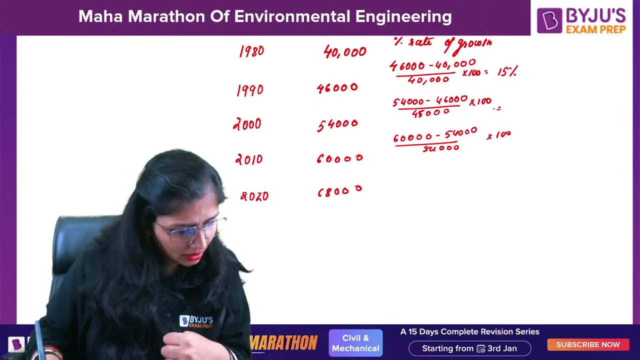 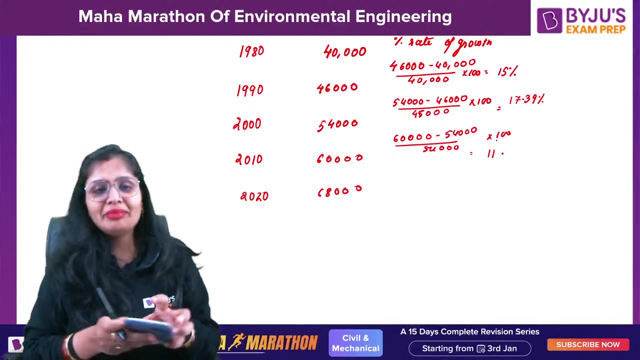 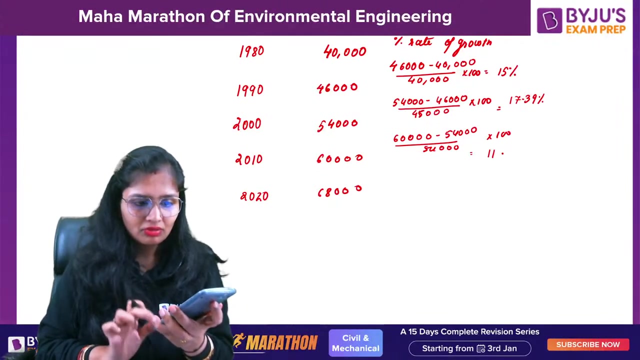 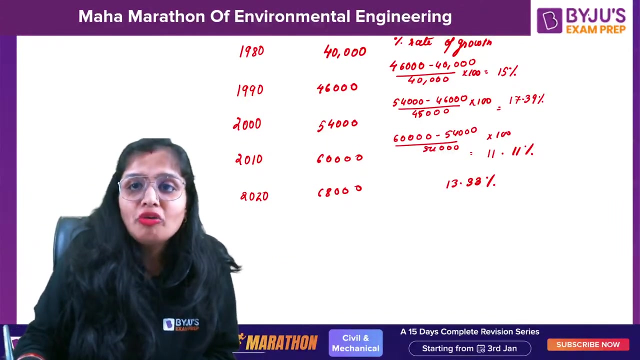 54,000, similarly. calculate everything and be fast fast: 15 percentages for the first one, then 17.39,, then 11.39,, then 11.39,, then 11.39, percentage right, okay, this is percentage rate of growth. now how much decrease is taking place? 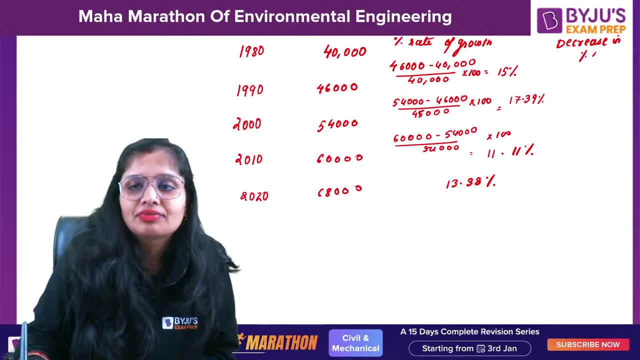 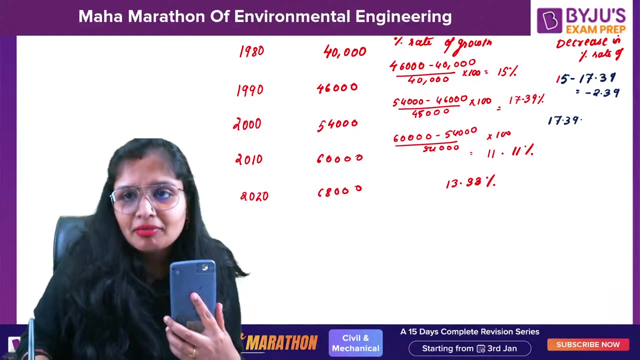 decrease in percentage rate of growth. so this will be 15. i'll take other color pen, if any color pen you're having problem, then let me know that. also: 15 minus 17.39, how much it is coming? how much decrease it is coming? 15 minus 17.39 minus 2.39. then then again 17.39 minus 11.11. 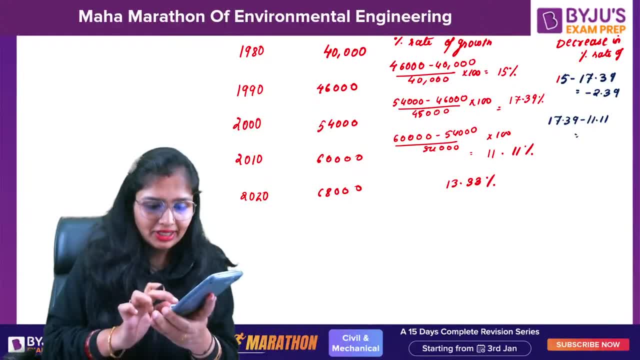 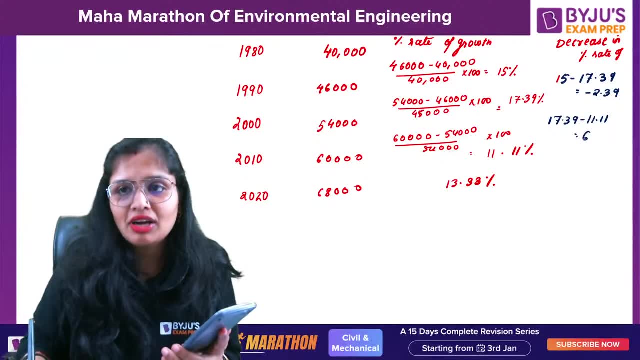 how much it is coming: 17.39 minus. anyway, if you do the formula also you have to do this. so don't think that if you do the formula you don't have to calculate. then also you have to calculate 6.28 percentage, then 11.11 minus 13 point. it was 33 na 33. 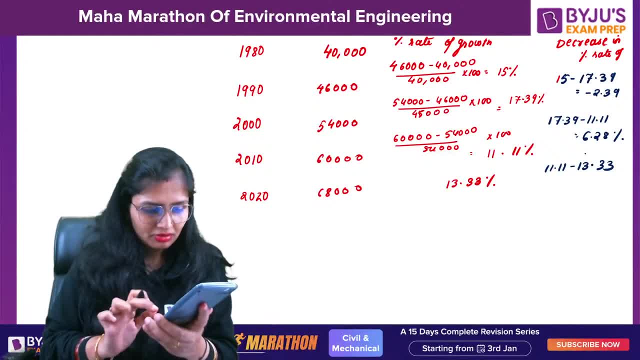 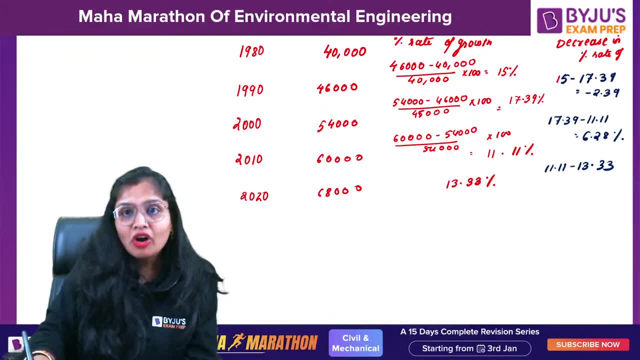 plus 2.39, no beta. no plus no, no. no, that's the wrong thing, bhanot. always from this to this, whenever, everywhere you used to do from the higher one to the lower one, okay, or from the current one to the previous one, but remember, when you calculate decrease, i will do from the initial. 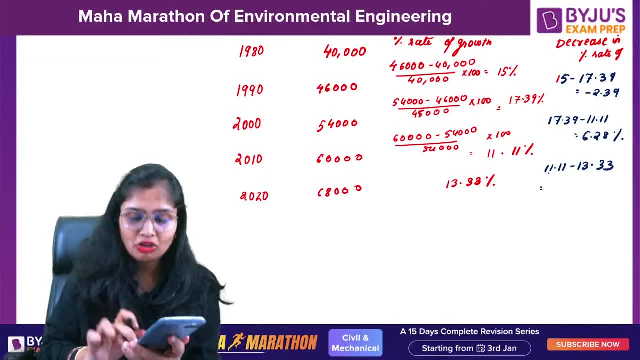 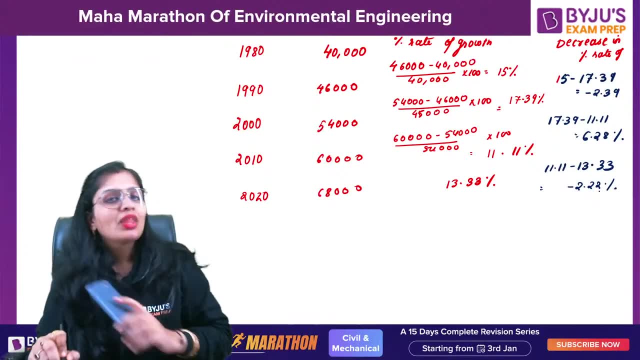 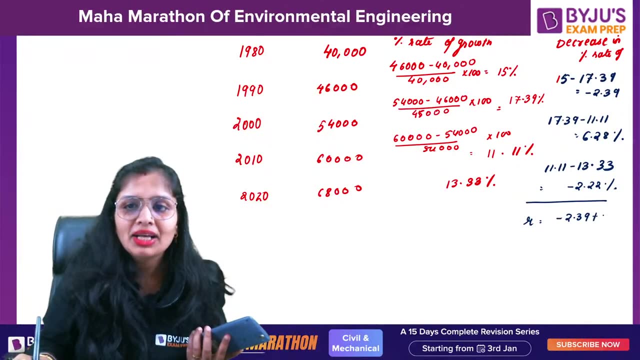 to the final. okay, so this will come out to be how much minus 2.22 percentage. okay, so from here, if you want to calculate our, that is, that will come out to be minus 2.39 plus 6.28. you have to take the sign also into. 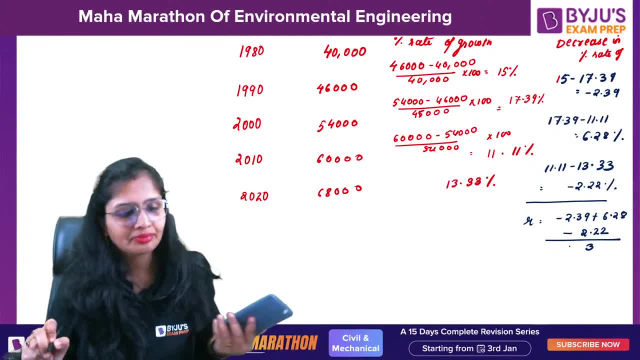 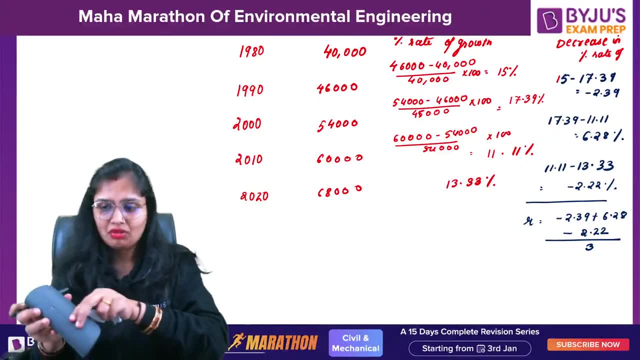 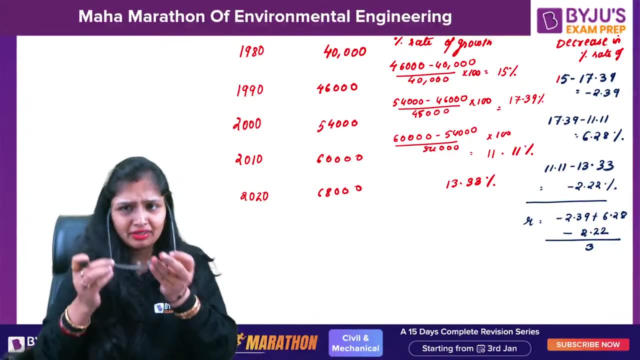 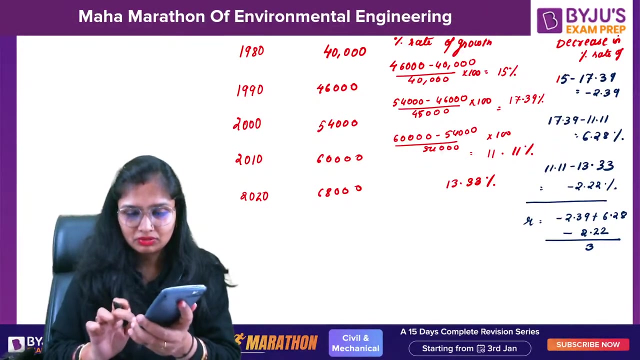 consideration: divided by 3, how much you are getting you, you, How much you are getting? 2 point minus you are getting, Just let me take it out- 0.566.. Yeah, 1.67.. How come Divide by 3.? 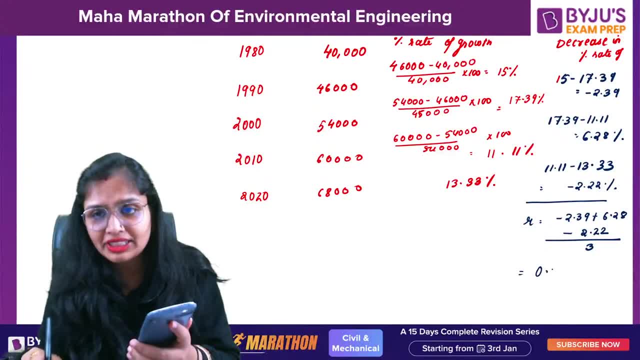 You guys have done it. If point yes, Devanshu and I got the same answer: 0.556 per decade. Now remember that means in this there is no direct formula. If you go through the method of formulas also, you have to calculate. 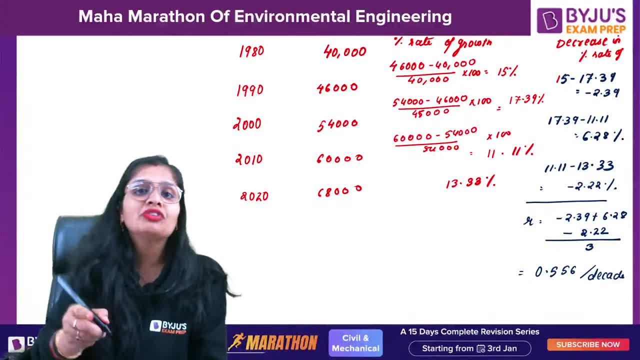 If it has asked you 2040, then also, first you have to calculate for 2030.. It is mandatory. You have to go here in sequence format. That means the percentage is decreasing. If in 2020, the percentage is 33%. 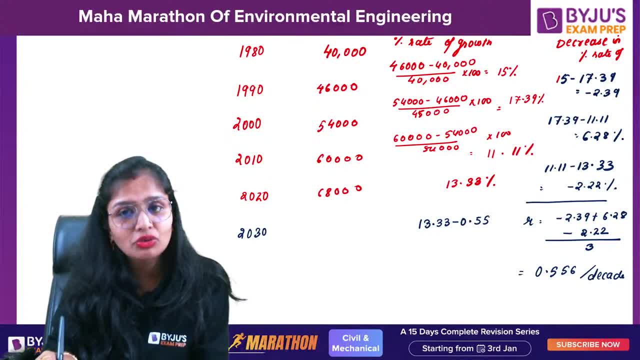 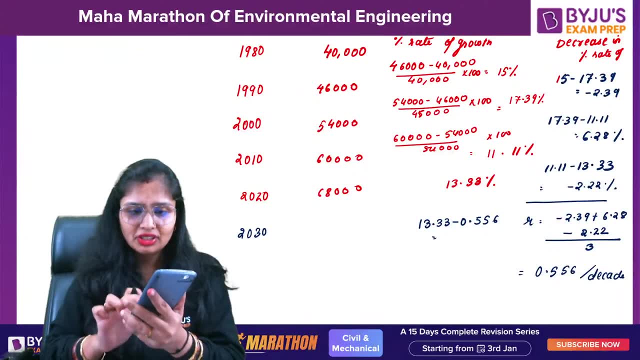 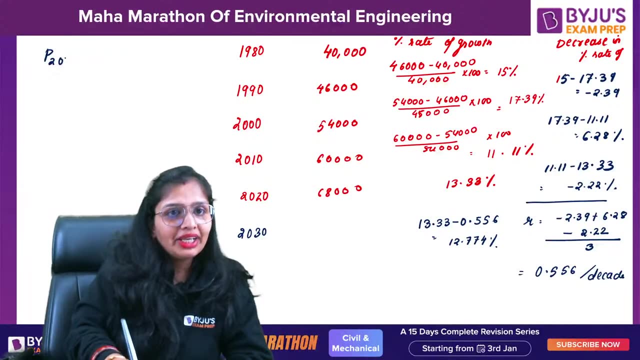 The percentage will reduce. That's why it is decreased rate of growth method. So it will be how much? 13.33 minus 0.556.. So this will come out to be 12.774%. So that means the population in 2030, although it has not been asked, but you have to calculate. It will be 68,000 plus 12.774% of 68,000.. Guys, calculate And tell me fast. I don't have the answer with me. 76686.32, 76686.32, Now talking about 2040. 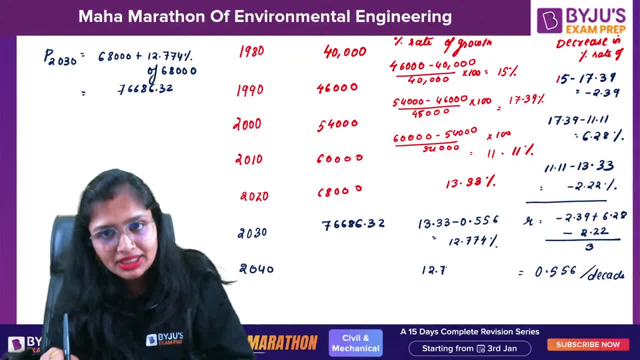 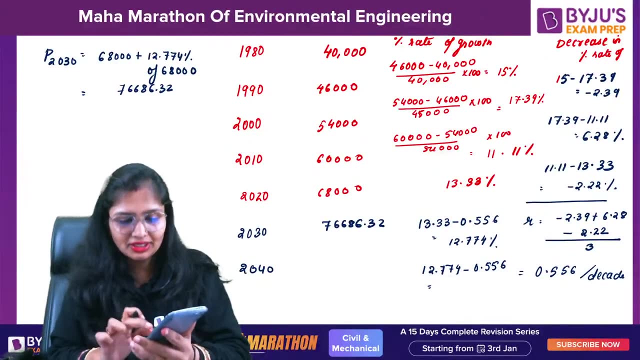 Similarly, if for 2030, the percentage rate of growth was 12.774.. If you subtract minus 0.556, you will get it. So this will come out to be 12.774 minus 0.556. This comes out to be 12.218%. 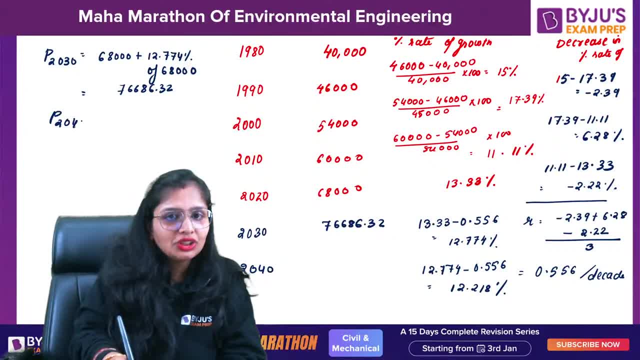 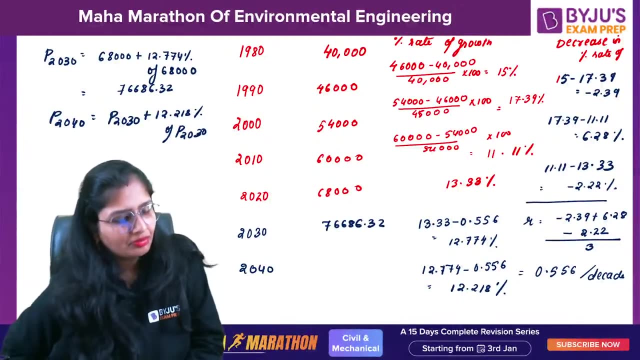 So the population in 2040, which is asked in the question, will be population in 2030 plus 12.21% of population in 2030.. Now, guys, tell me the answer In this manner, you will proceed. 86055.85. 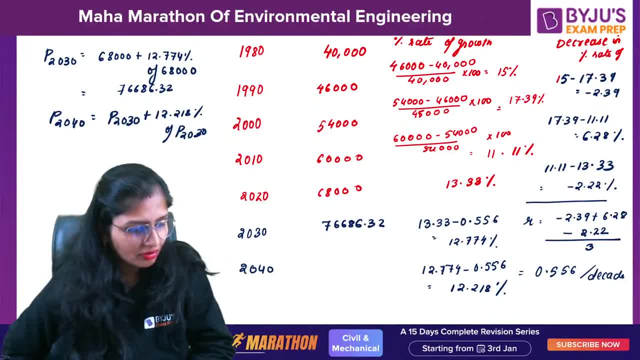 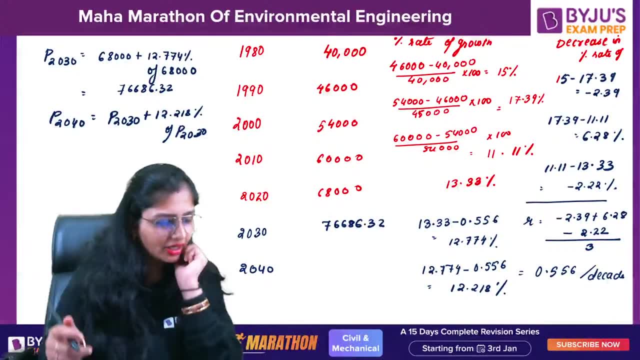 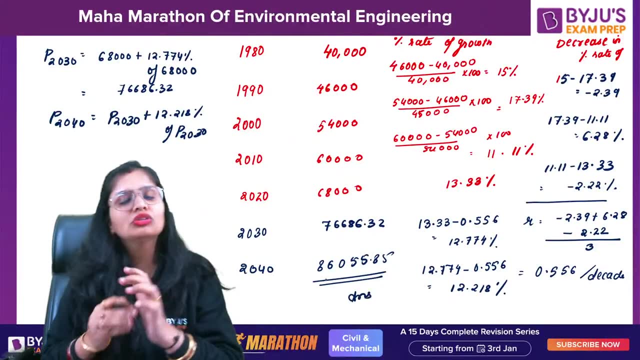 Clear How much it is coming. Calculate and tell me fast: 86055.85. So this will be the answer. So if you go through the formula or any method, you have to go like this, only So better. don't go through the formula, go through the logic. 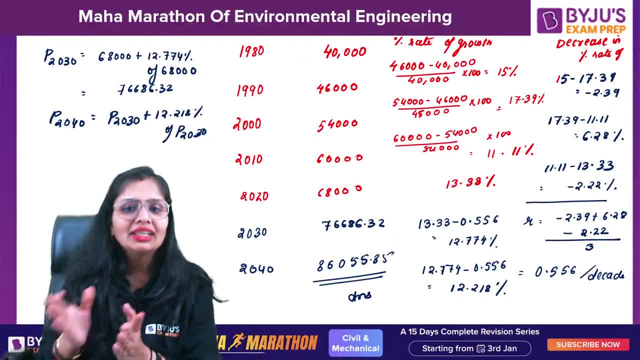 Calculate the decrease in percentage, Okay, And then subtract it. Now one mistake: don't do it. Some people do the wrong method. They say that if you want to calculate for 2040, do what? 13.33 minus 2 times of 0.556.. 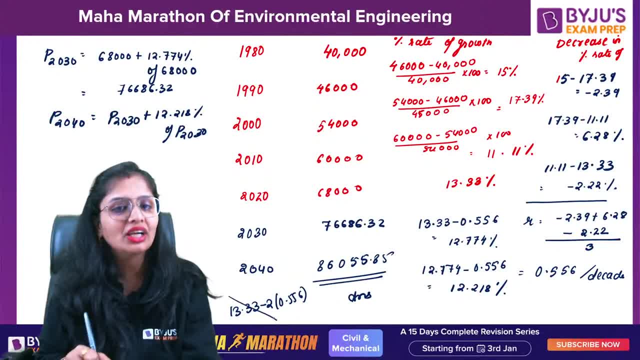 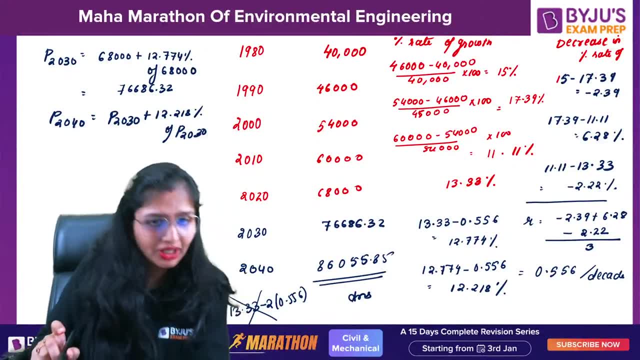 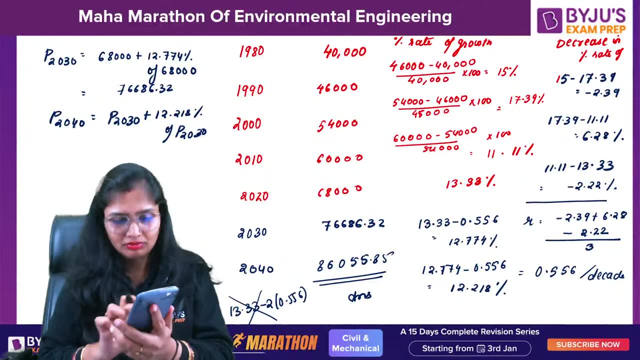 And then do 68,000 plus how much it comes. That is the wrong approach. Don't go by that method. Okay, Everybody is getting different Arun. you are getting different answer beta. Just check it everybody: 86055, Arun, wrong answer beta. 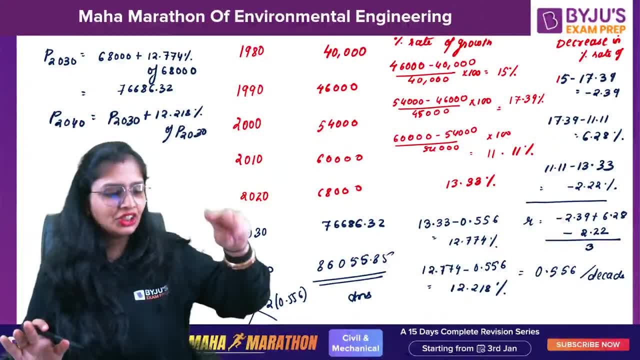 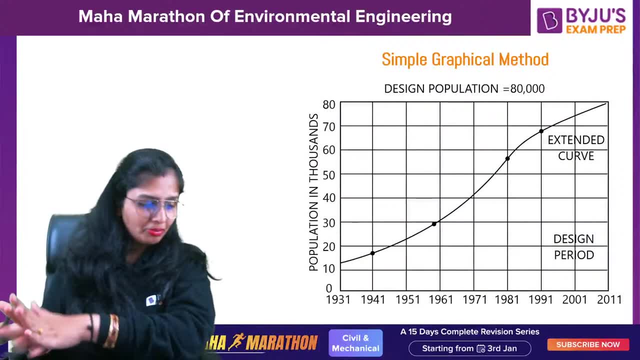 Fine, Clear. This method is clear. everybody, Deepak, Girish, Tiksha, everybody, it is clear. So this is the method. Now, talking about simple graphical method: Mistake, Okay, fine, Do mistakes here, not in your gait exam. 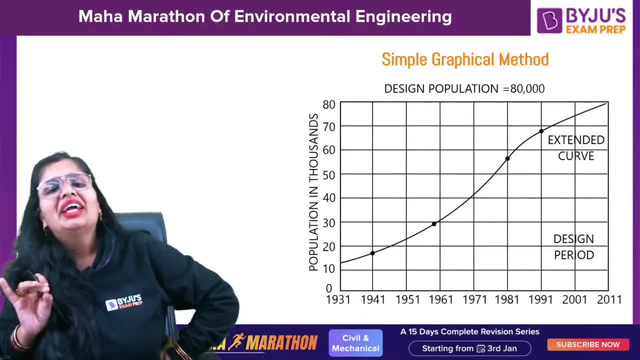 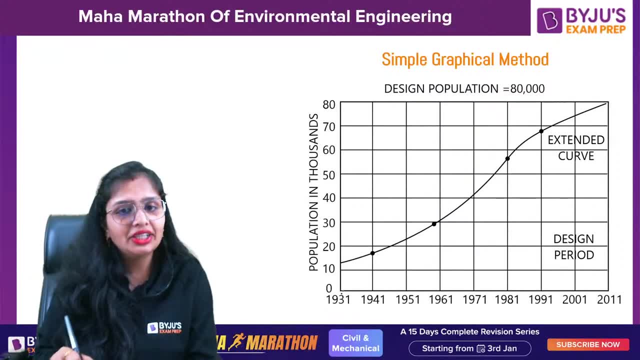 Now simple, graphical, Not used Basic. It is based on upon the experience and intelligence of the designer. Now, let us suppose in 1931, you know the population. In 1941, you know the population. 1951, you know the population. 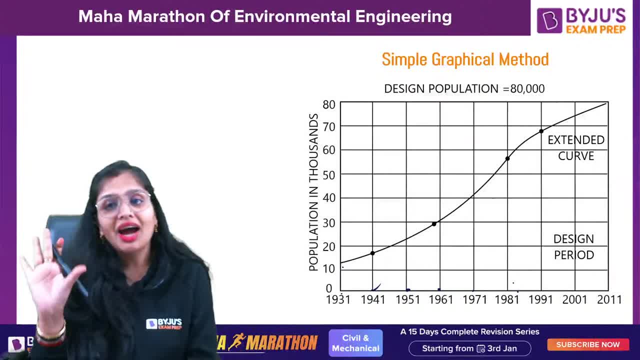 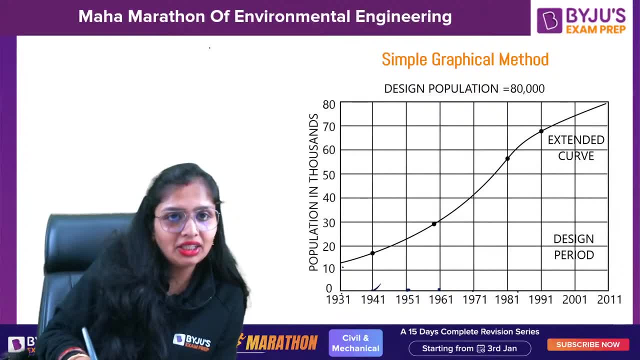 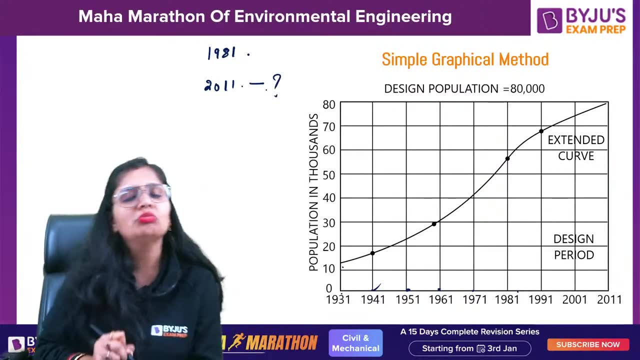 61,, 71,, 81,. you know the population. After that, you want to compute the population for 2011.. Okay, For 10 years, it happens. 1981 was the last population you know, And let us suppose, 2011,. you want to know the population. 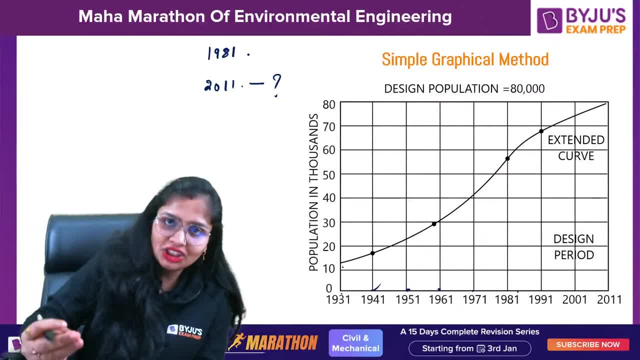 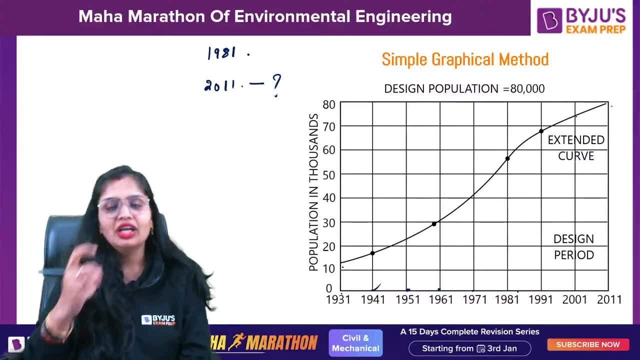 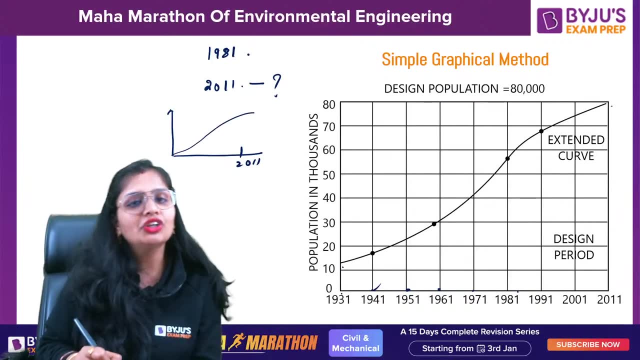 Based on the pattern, the engineer, the designer, will extend this graph. Okay, Will extend this graph. Now, what will happen? Let us suppose if this is the graph, what will happen if he has extended the graph like this? So what he will do? he will draw a line parallel to the y-axis from 2011.. 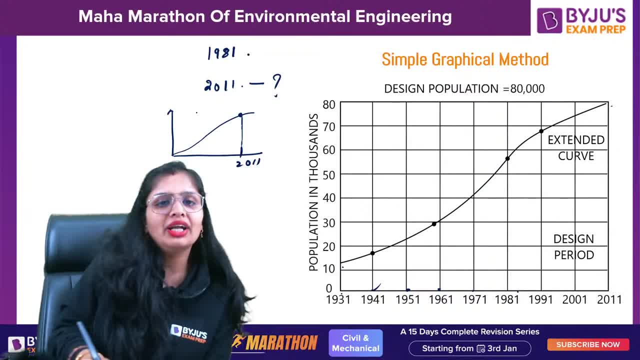 The point it will touch The point, it will touch the curve. from that point it will draw a line parallel to x-axis, The point at which it will cut the graph on the y-axis, that will be the population. Simple as that. 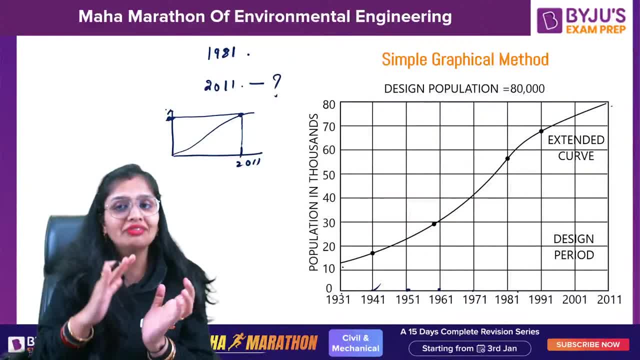 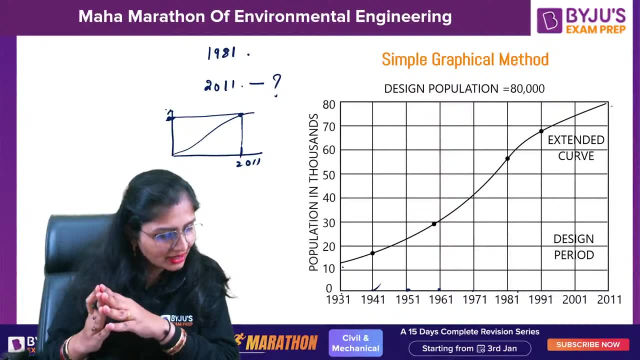 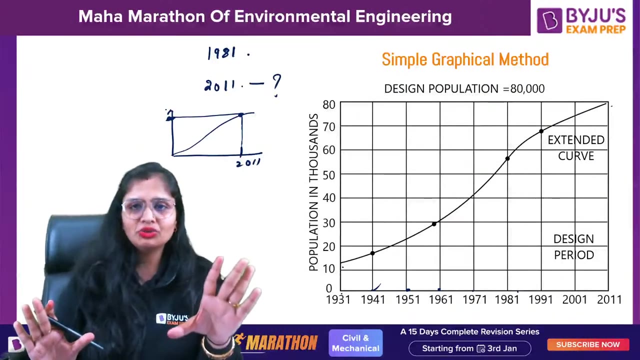 But how the curve is extended, that depends upon the experience of the designer. Okay, So this you should know. Okay, Fine, So this is the thing which you should know. Okay, Practice, Practice session. Okay, So this is simple graphical method, not used that much. 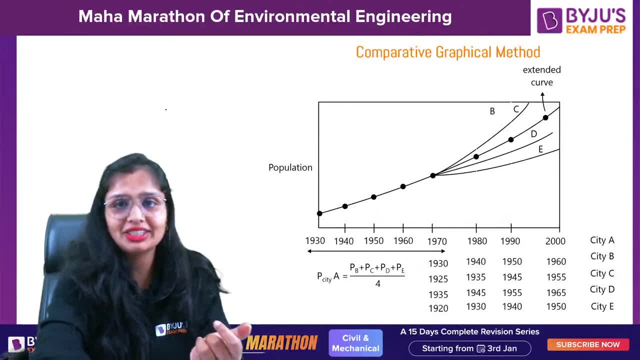 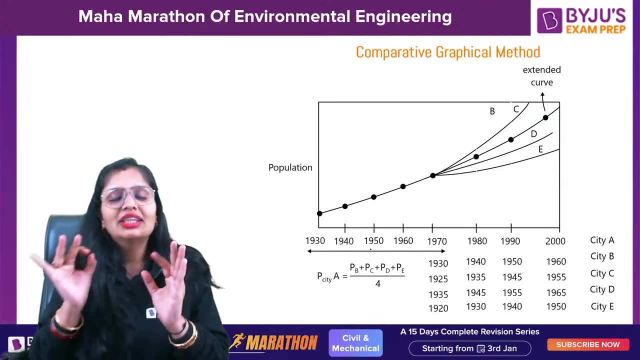 But if it comes, so I told you, it depends upon the intelligence and experience of the designer. This is the comparative graphical method, or comparative graphical method, which is used. Now, what happens here? What happens here is basically- let us suppose this is used because the new city is developing in a similar manner as compared to the previous city. 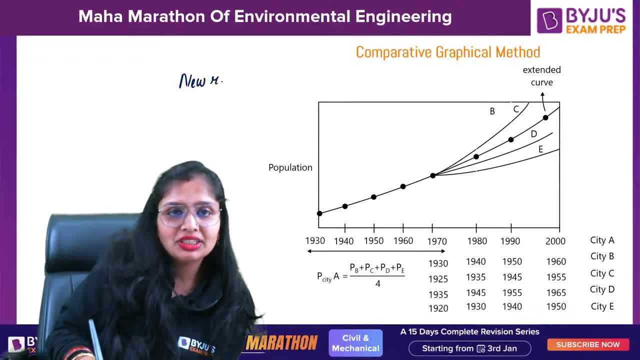 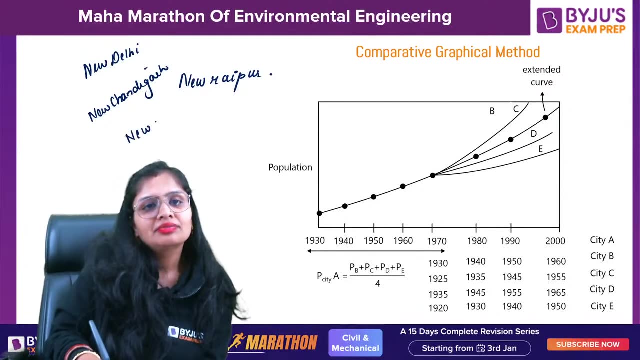 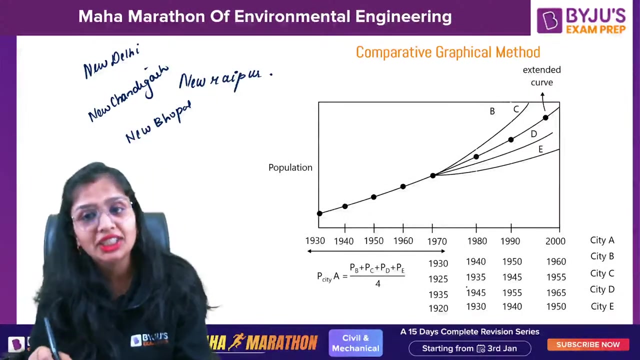 Let us suppose, if you talk about, in my area, new Raipur is developed. Now new Raipur is developing in similar manner, like new Delhi, like new Chandigarh, like new Bhopal. Okay, So now what happens for city A, for which I need to forecast the population? I came to know that city B, city C, city D and city E are developing in the similar manner. 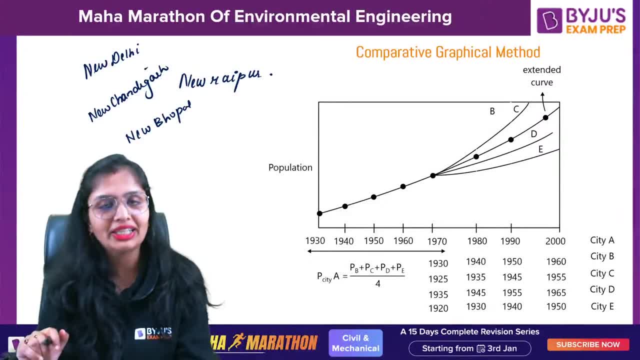 Of course the year will be different, but yeah, they are developing. they have developed in the similar manner. Like I will read it: 1970, what was the population in city A Similar was for city B, 1930.. 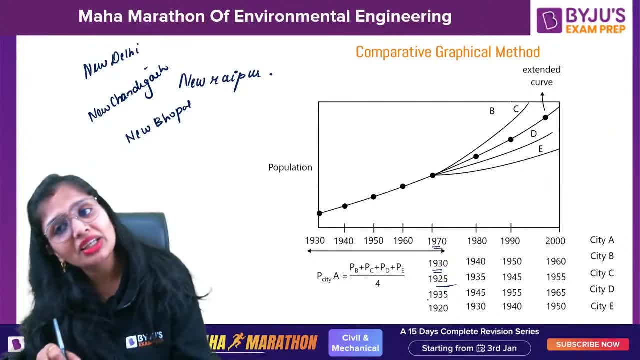 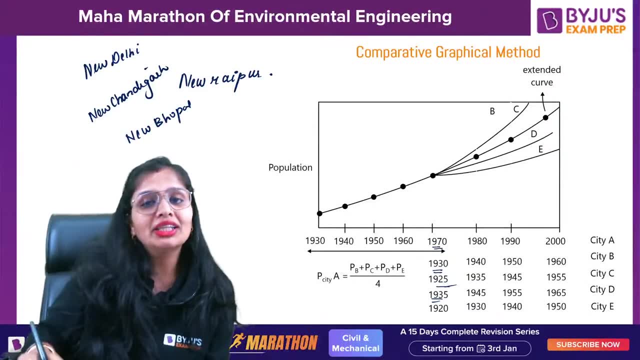 Similar population was there for city C in 1925.. Similar was the population for city D in 1935. And similar was the population for city D in 1920.. So what they will do is what they will do is the curve for every other is given to you. 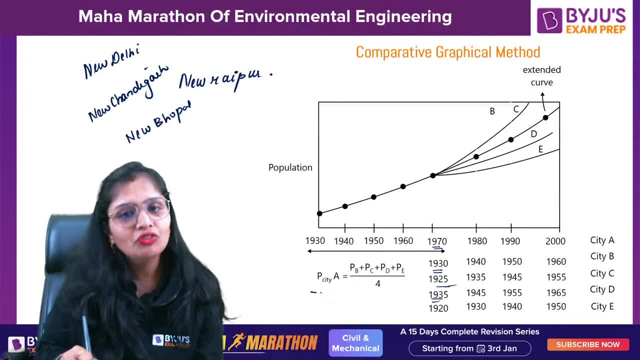 Okay, Okay, Okay, based on those, what you will do, you will you know the population for 1980, what will be the population. that will be the same population for city B, 1940, 1935, for city C, and so on. 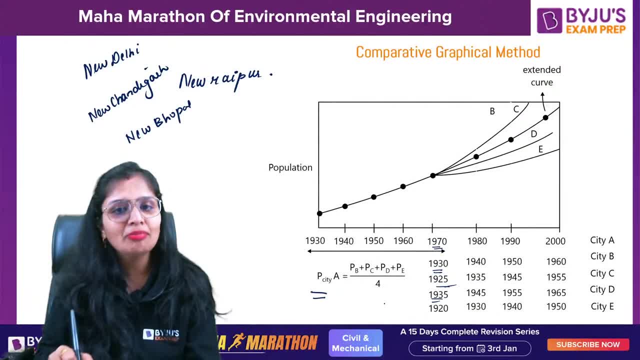 So you will add the population for those cities, divide it by 4, because you have taken 4 cities and you will plot it. Then you will plot it, then you will plot it. So this is simple, Okay, Simple, but yet logical. 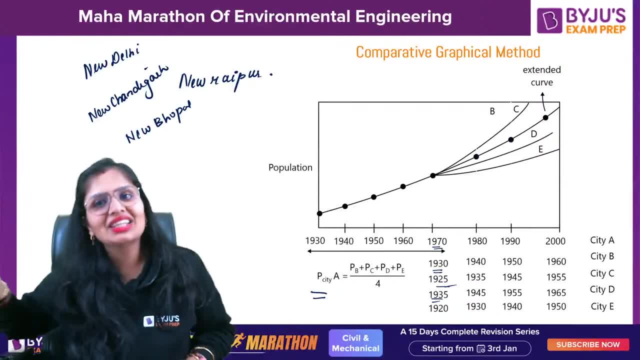 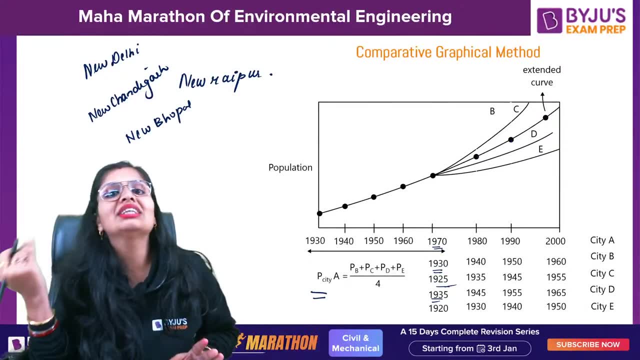 Why? Because it is not based upon the experience of the designer that he can extend. This is purely logical. Why? Because you have selected those cities which have developed in the similar manner as compared to the city for which you are forecasting the population. 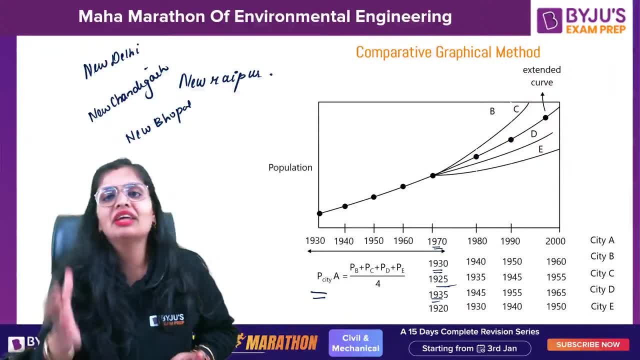 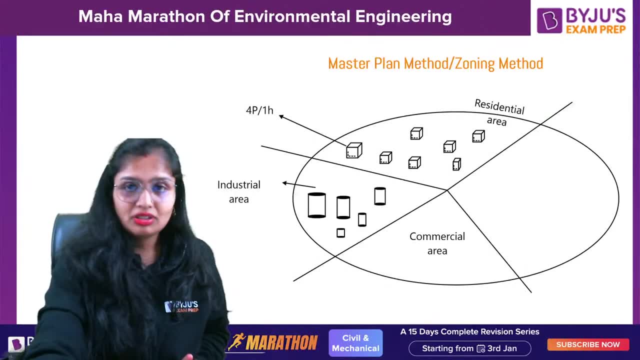 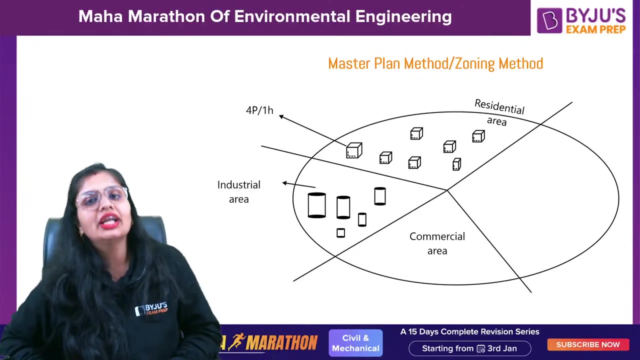 So this is because you are doing a comparison. this is known as comparative graphical method. Clear everybody. Last method, second last method, last, not last. This is the master plan method, or zoning method. Master plan, zoning method. If ever, if you are living in a, let us suppose, a municipal corporation, area, Nagar Nigam, which we call it, you just type it in Google: the zone plan of your city. you will get it. 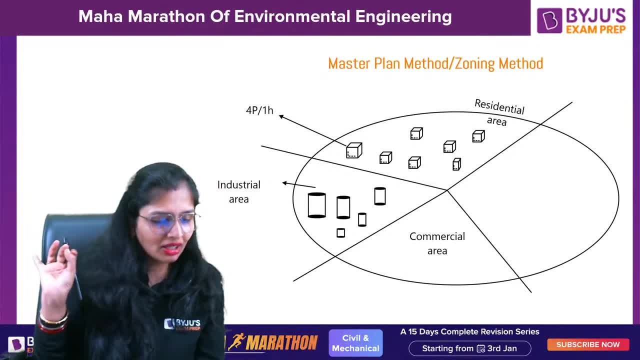 Remember, have you guys ever basically repeat what Sashi? Have you guys ever thought that? or you have read it in the papers: Sarkari zameen par kabza karke logo, ko loota. Basically what they have done. they have taken the government land. 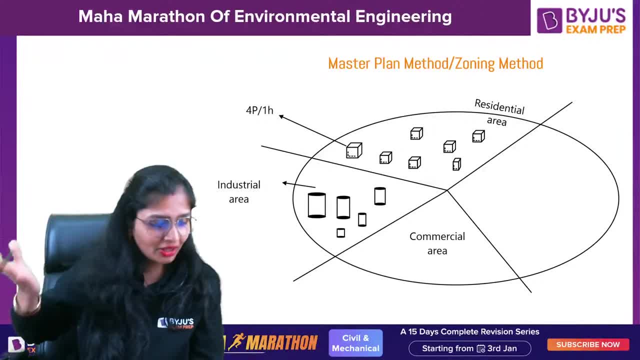 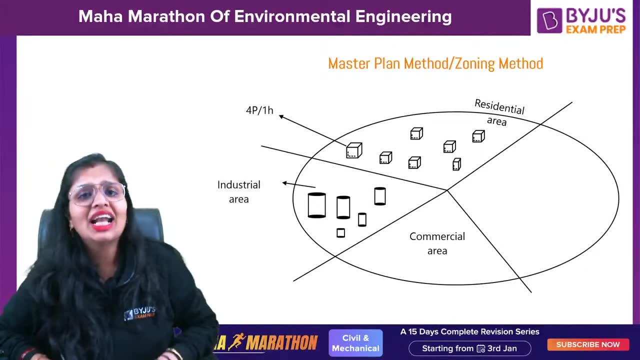 And these contractors and all sold that land. You guys have read it, Okay, You guys have read that. So, basically, what is happening? basically what is happening? And the question comes why they know that it was a government building- or government, you can say- that land. 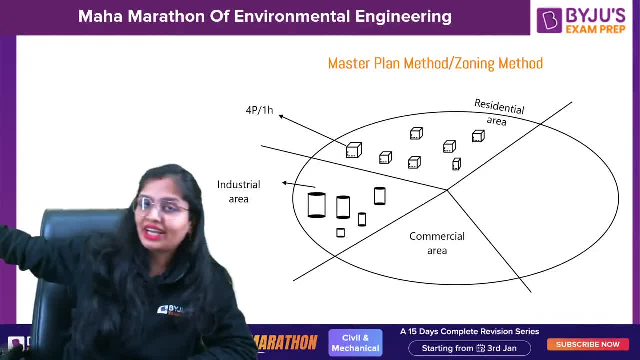 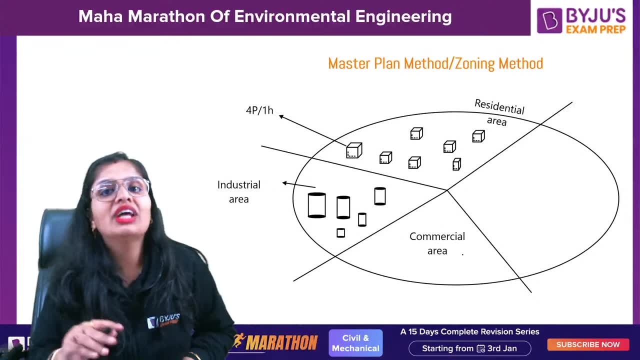 Because when the city was being constructed, it was said that this is railways property, This is a state government's property, and so on. Okay, So that is the master plan of that city. Okay, So let us suppose if it is saying that the this area is residential area, this area is industrial area, this is commercial area or any other area, 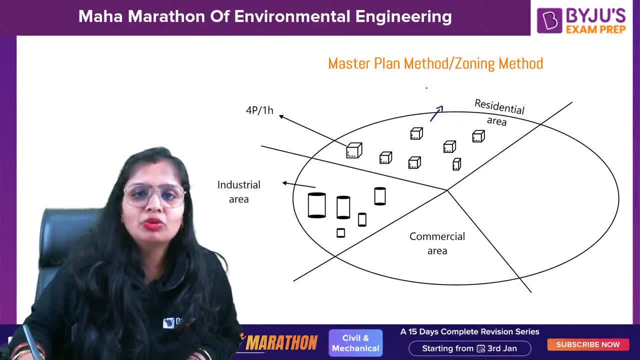 So mention that densities also like: if let us suppose like 50 kilometers square area is there, Okay, So let us suppose a hundred people are required per kilometer, if a hundred people are there per kilometer square, and let us suppose 50 kilometers square area is there. 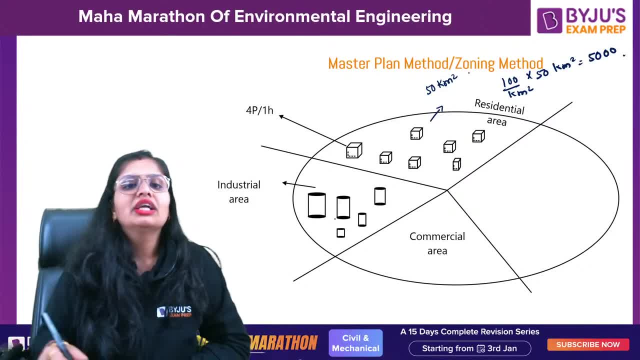 So how much people will be there? 5,000.. Similarly, the industrial area. it is telling you: let us suppose 20 people are there per kilometer square and a hundred kilometers square area is there. So how much people will be there here? 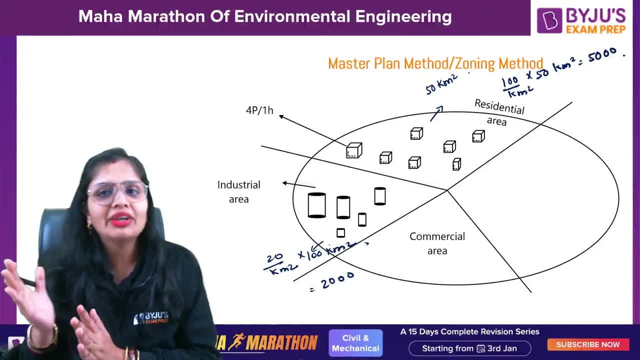 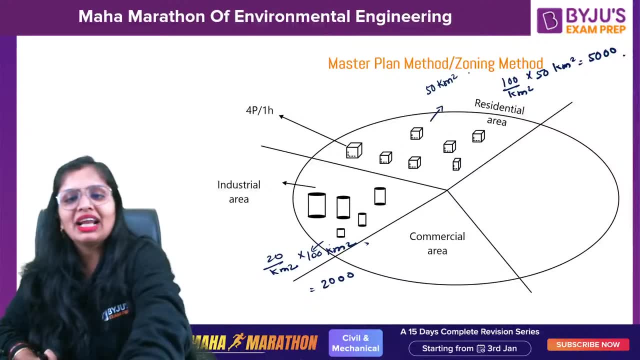 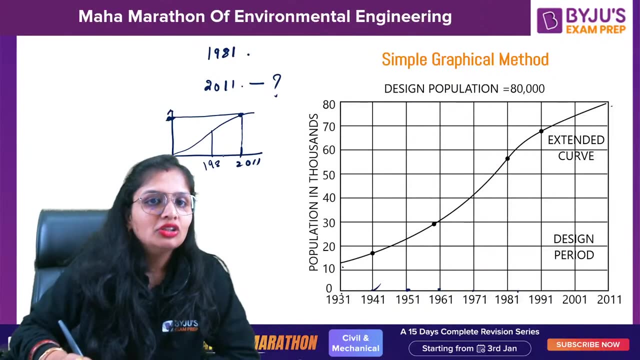 2,000.. So in this manner, you will add all of them and you will get how much is the population there. So this is also the method, Okay, A simple graphical method. simple graphical method is better If, let us suppose, you know the last population of 1981, so you extended this curve. you extended this curve. 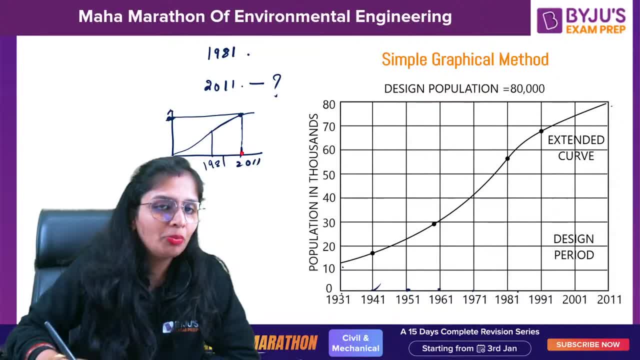 Okay, Now, from 2011,. you want to get the population, So you have drawn a line perpendicular, or basically first parallel to y-axis. it will touch the graph at a certain point. From this point, draw a line parallel to x-axis, the place at which it touched the y-axis, you will get the population. 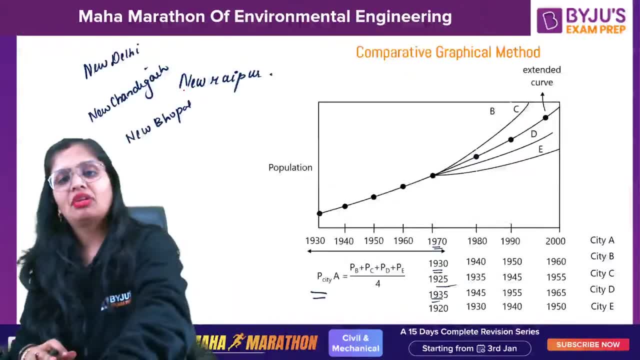 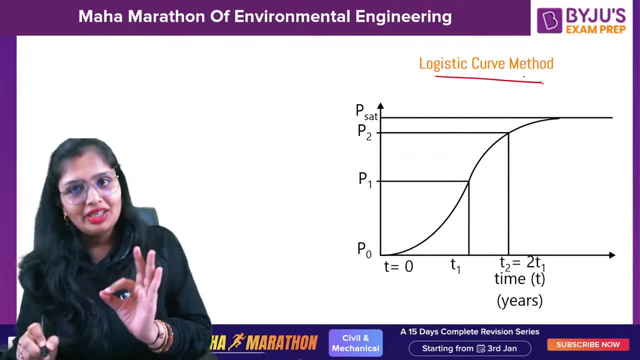 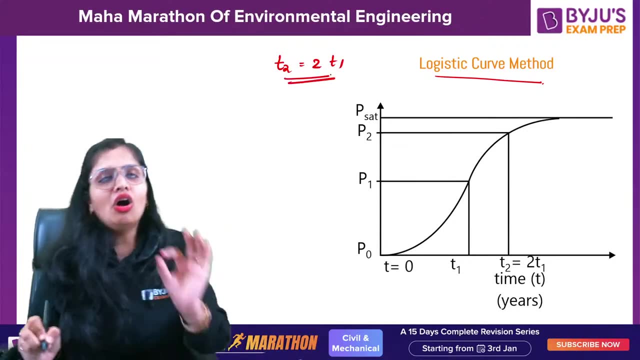 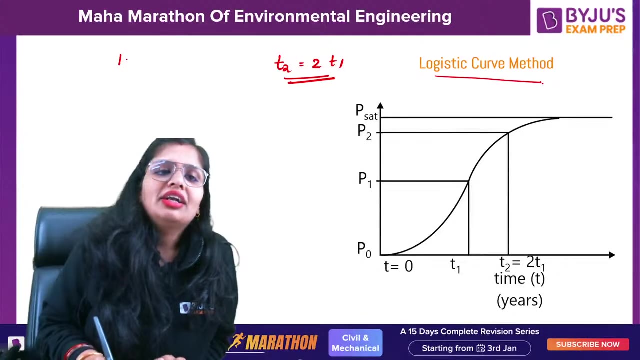 Clear. So from here you will get the population of 2011.. Last method: logistic curve method. Remember. this method you will able to apply only when t2 is twice of t1.. All calculations are done from the base year. Now you will tell me- already told you- 1990,, 2010,, 2015.. 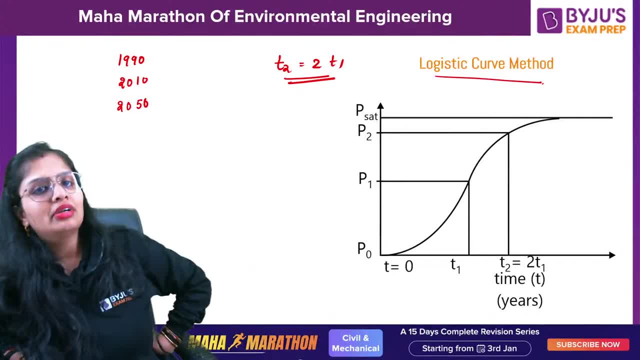 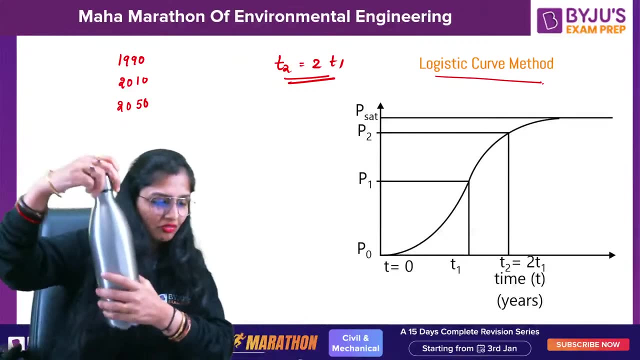 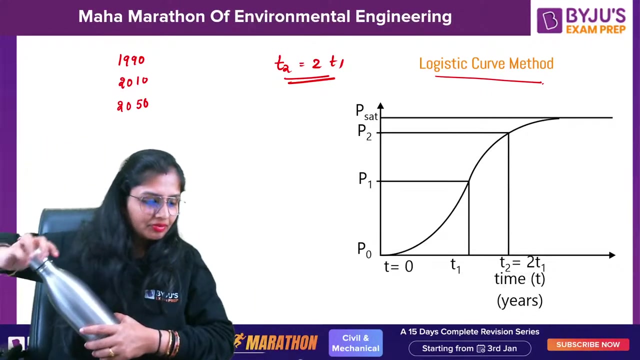 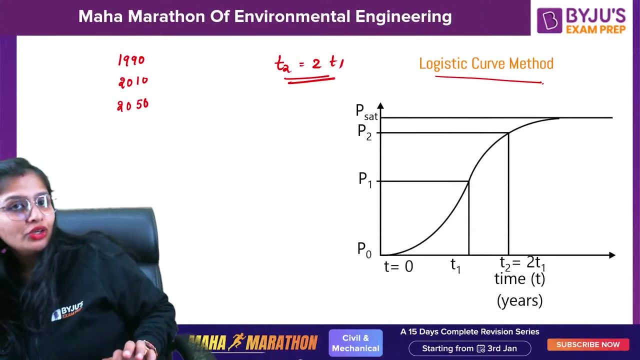 Can you apply logistic curve method here? Can you apply logistic Logistic curve method here? yes or no? Fast, I want the answer fast, Fast, fast, Arun, everybody, Alekh. No, you cannot. I told you all calculations are done from the base year. 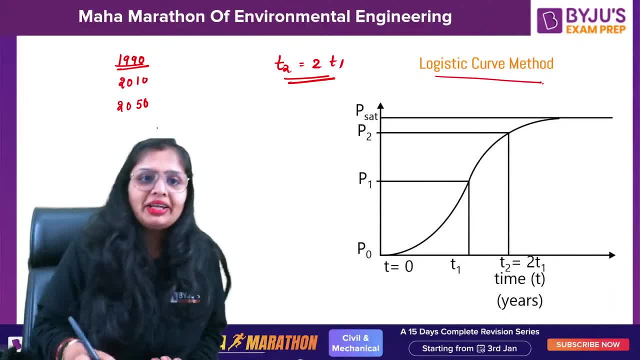 1990 is the base year. What you guys thought, let me tell you: 1990 to 2010, it is 20, and from 2010 to 2050, it is 40.. 2010 to 2020, 30,, 40,, 50.. 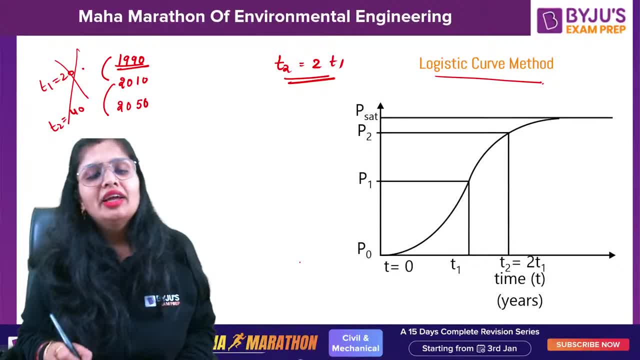 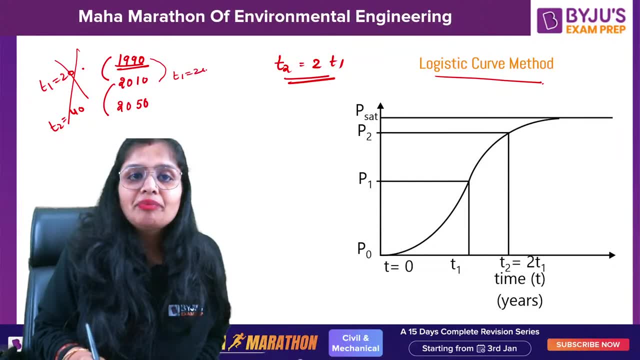 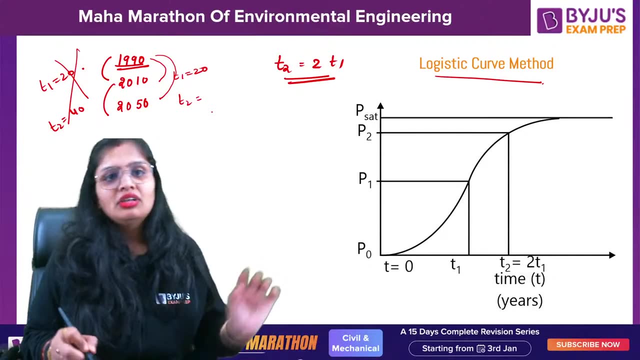 So you thought we can apply No. Why? I will tell you: Because 1990 to 2010,. it is 20.. 1990 to 2050.. How many decades, How many decades. 2000.. 2010.. 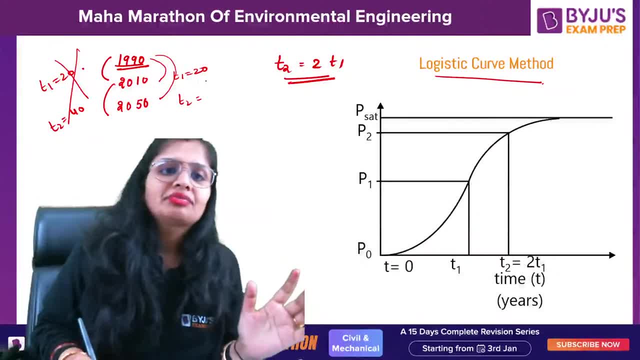 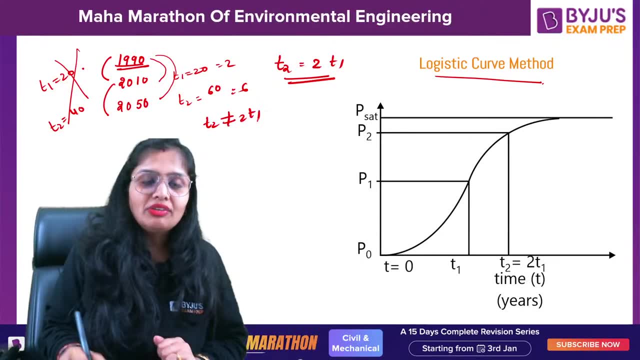 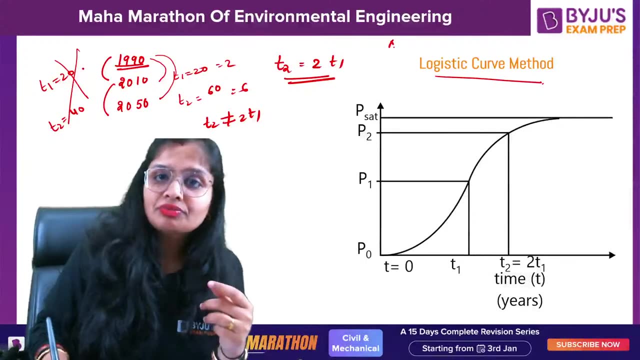 2020.. 30. 40., 50.. 2 decades. this is 6 decades. Can you apply? T2 is not equal to 2 times t1.. All calculations are done from the base year. I will write it also so that you do not. 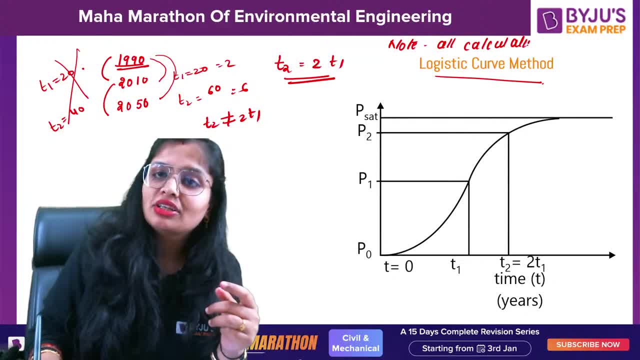 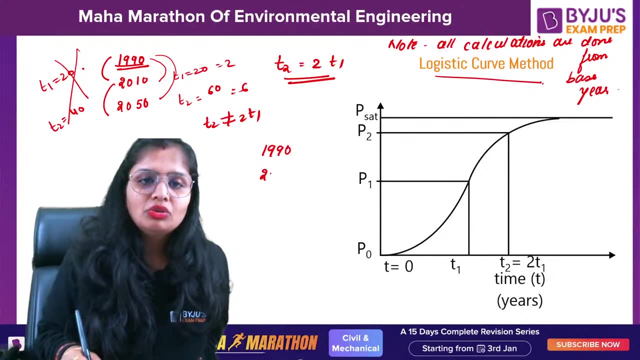 I just shout and shout, but again you do the same mistake. All calculations are done from the base year, are done from base year. okay, now tell me this one: 1990,, 2010,, 2013,. now tell me Tiksha. 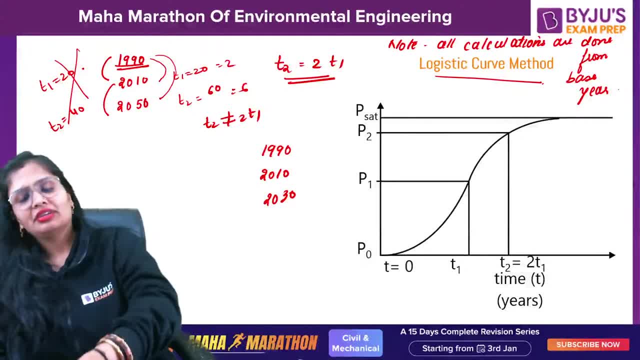 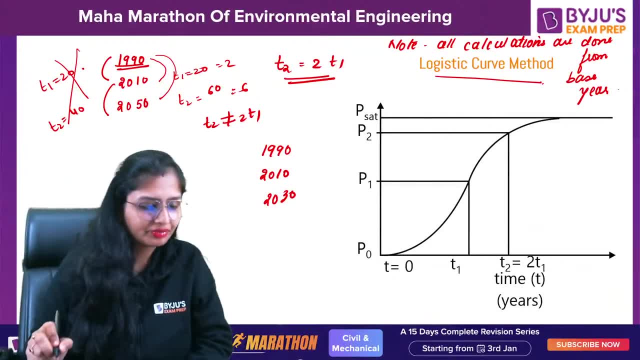 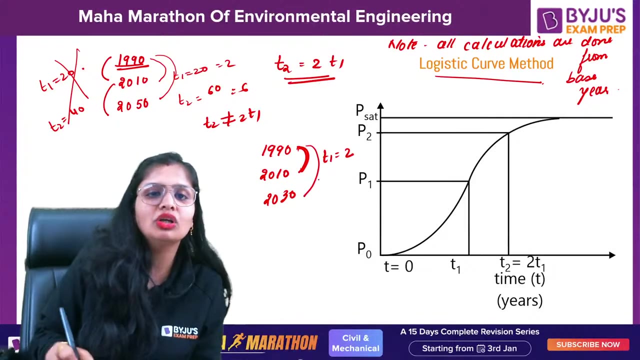 everybody. Sashi, can I apply yes or no? yes, why? because 1990 to 2010,. two decades, 1990 to 2013,. four decades. so you can see T A2 is twice of T1, so yes, here you can apply logistic curve. okay, generally when you. 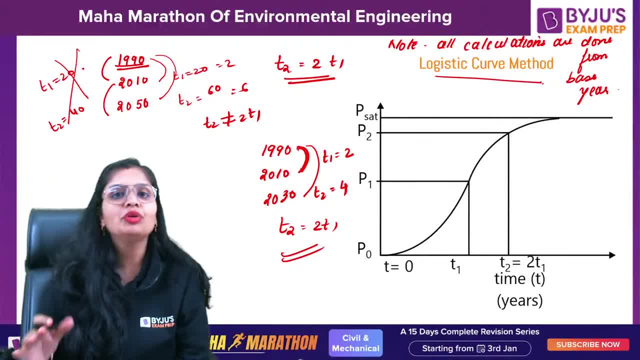 see the variation of population with respect to time. you get a S curve like you can see it here. it appears like S, so you call it as logistic curve, you call it as autocatalytic curve, you call it as S curve. now you know this word: saturated. I am done, I am saturated. 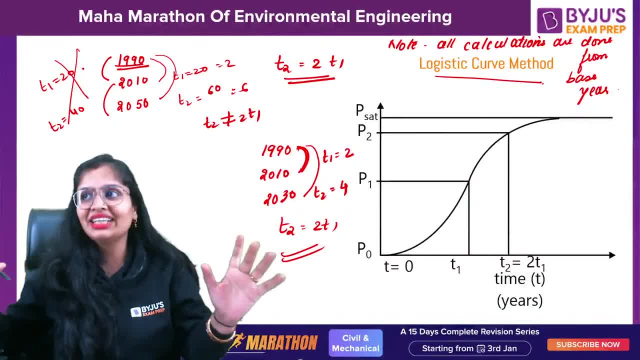 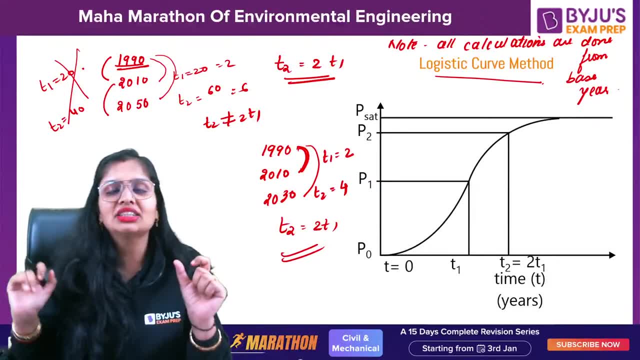 this is over. so I am saturated. similarly, when the city has reached to its maximum, now, more than that it cannot accommodate. so that is the saturation population. that is the saturation population, let us suppose at T0, the population. 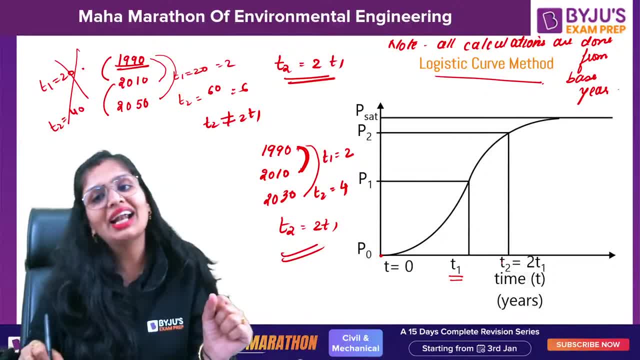 was P0,, at T1, the population is P1, and at T2, the population is P2, now you want to calculate. let us suppose, at P, at any, basically at any time, T, what will be the population? 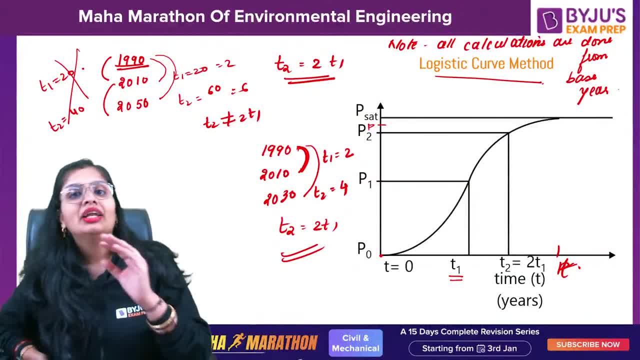 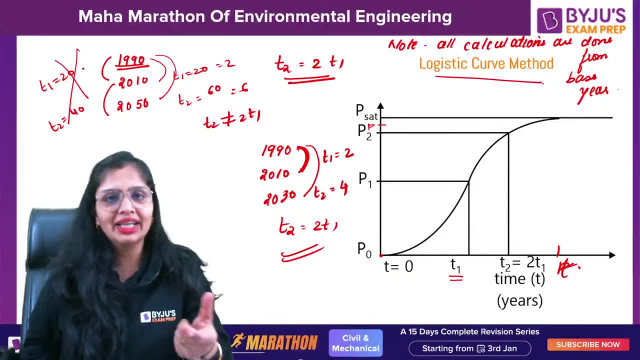 P, so we will go by logistic curve method. now these, this method, this method. this is generally, as in your ESE, conventional. This is purely formula based. They can ask you in gate examination for 1 month to check out whether you know the formula or not. Okay, So this is the. 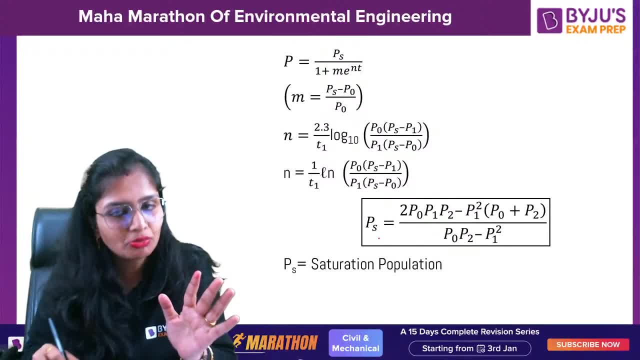 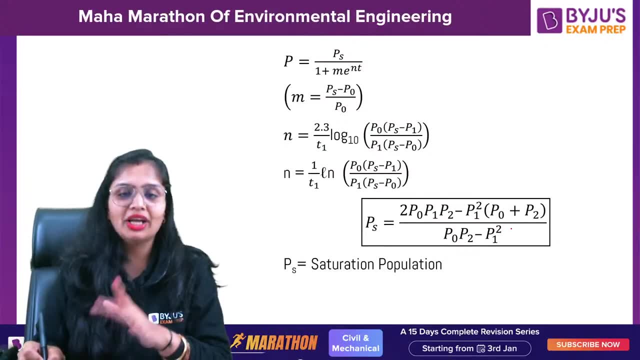 formula for this. First you need to calculate the saturation population, which is 2 P0, P1, P2 minus P1 square, P0 plus P2, P0, P2 minus P1 square. I know this is tough, but do 2-3 equations. you. 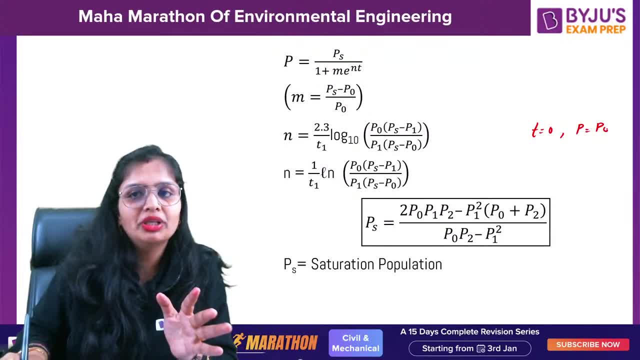 remember this: At T is equal to 0,, P is equal to P0.. At T is equal to T1, P is equal to P1.. At T is equal to T2, P is equal to P2.. Okay, So this, you should not remember. This. you can apply only. 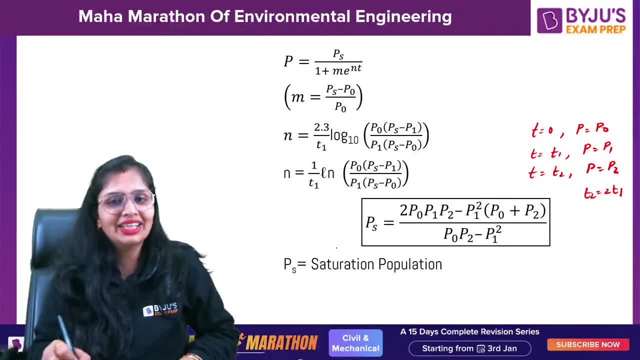 when T2 is twice of T. So for this, in 1 month, they can ask you what is the saturation population If they want you to predict the population, forecast the population. So it is: P is equal to PS1 plus ME to the power NT. 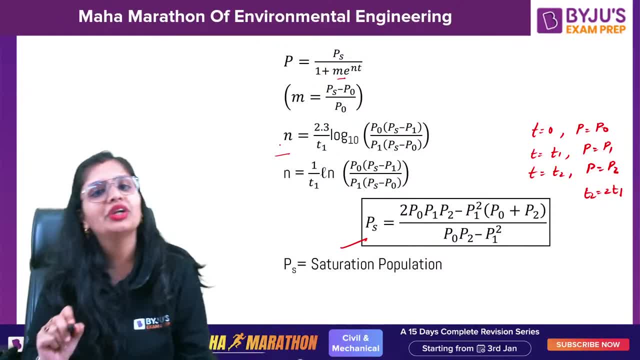 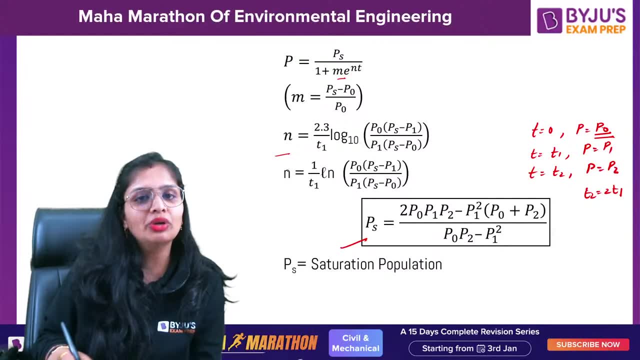 Okay, And M and N. again formula you need to know: M is PS minus P0, the population of the base here. Okay, Remember this, you can do it in any manner. N value, you can do it for log based N. 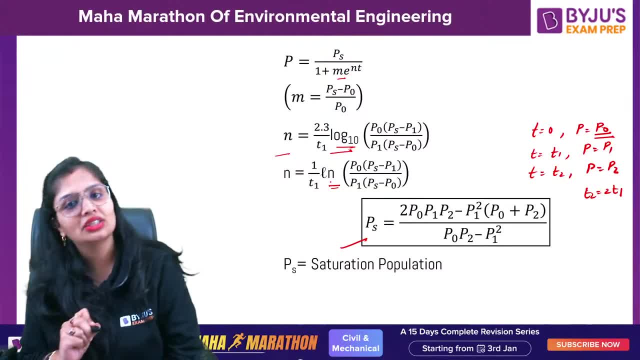 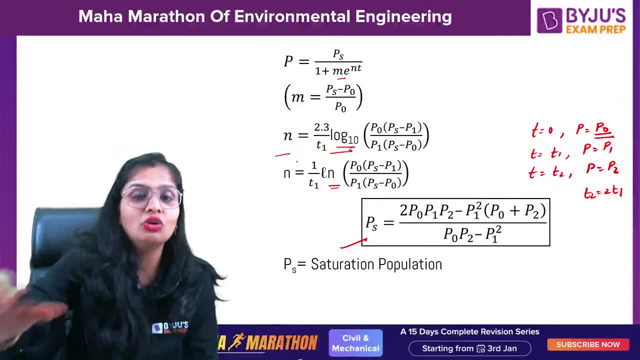 just multiply 2.3. or if you want natural log, you can do it like this. But when you substitute T1, beta, always from base here, Always from base here, Otherwise your whole calculation will be gone. Okay, This formula, with the help of it. 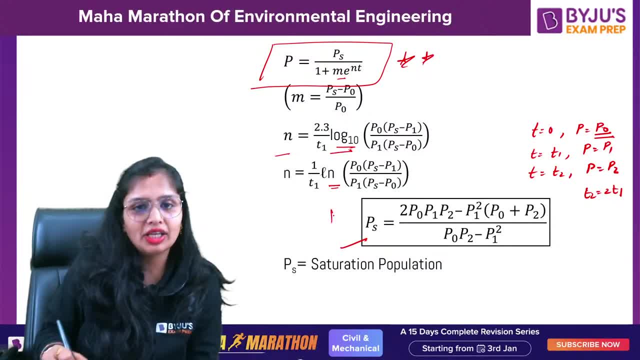 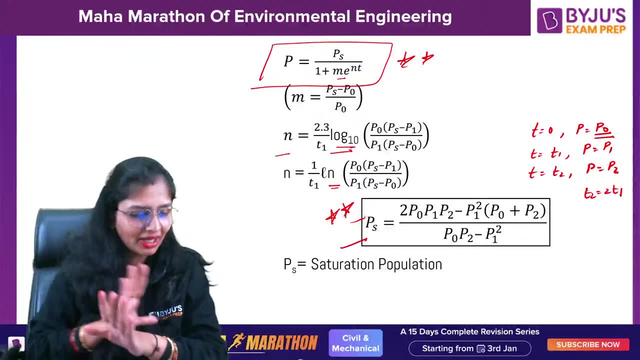 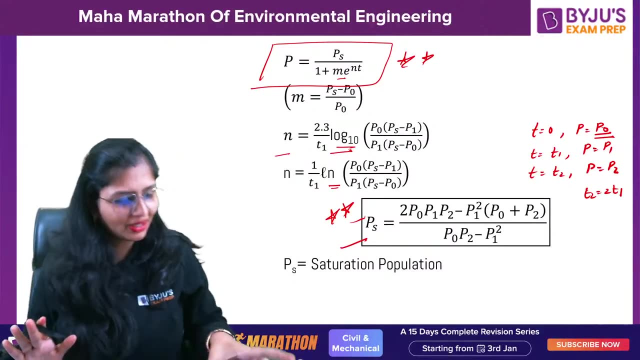 you can calculate the population. This is an important one. This is an important one. Okay, So this completes your first water demand. Any doubt, Any doubt, Guys, so many people right now, I saw, and so less likes, Not fair. 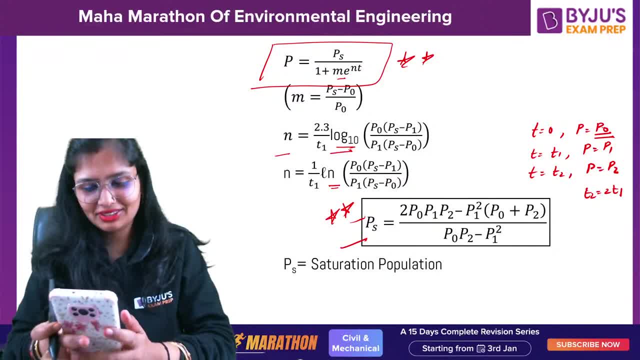 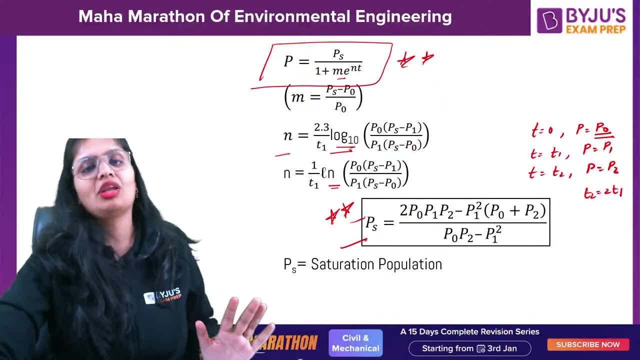 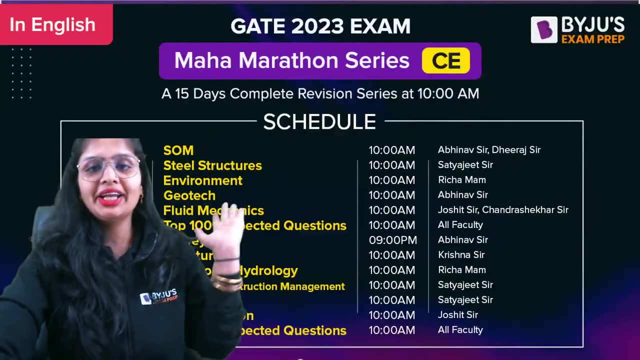 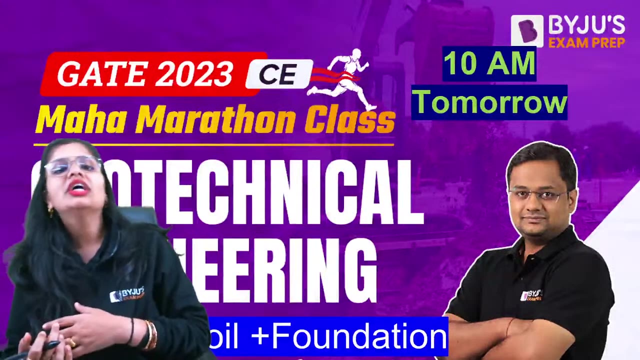 Not at all fair, You guys, becoming miser nowadays. Okay, Clear, everybody, Okay. So now ready for the next chapter. Ready, Important chapter Schedule once again shown to you and guys. tomorrow you will be having the geotechnical marathon by Abhinav sir, 10 am tomorrow. complete soil and foundation Link has already been given. 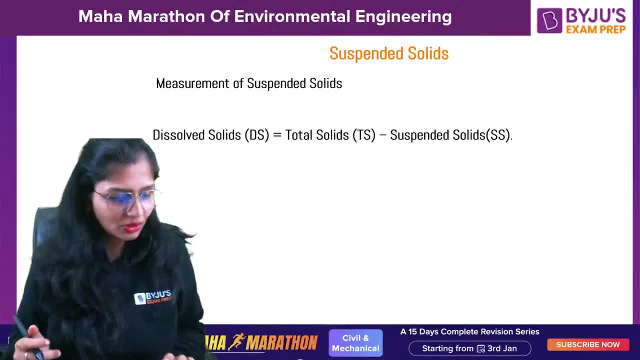 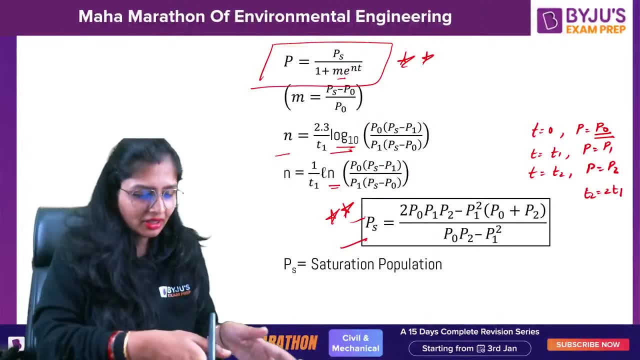 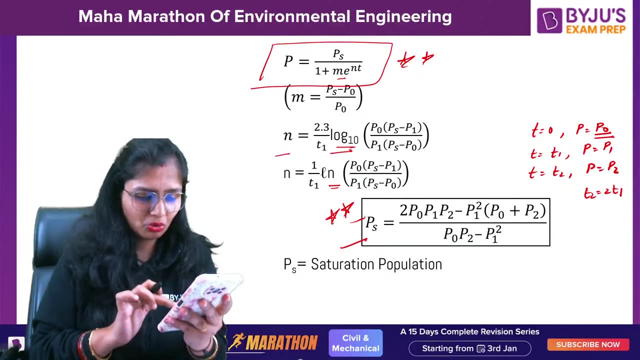 You can set a reminder, Okay, So problem on last method. problem on last method. if you want, fine, i'll do it. well, well, it was not given because it's just a calculation method. but if you want, i will give you. just wait a second. 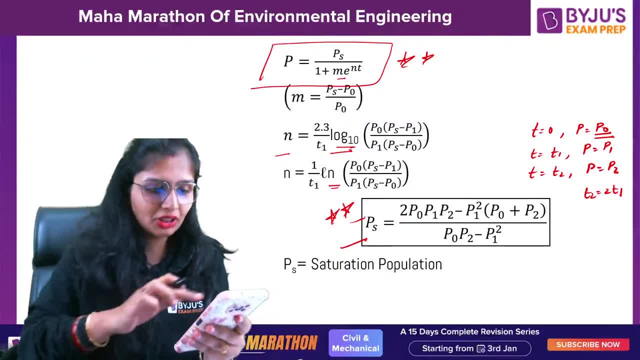 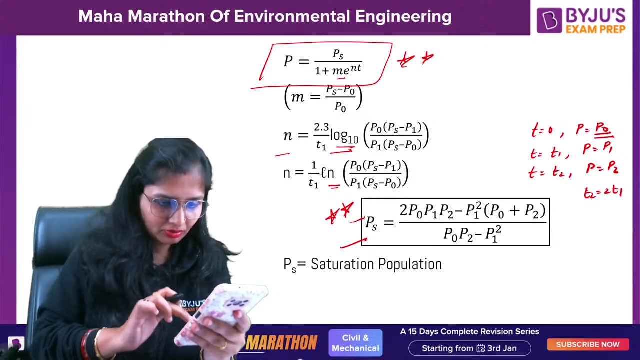 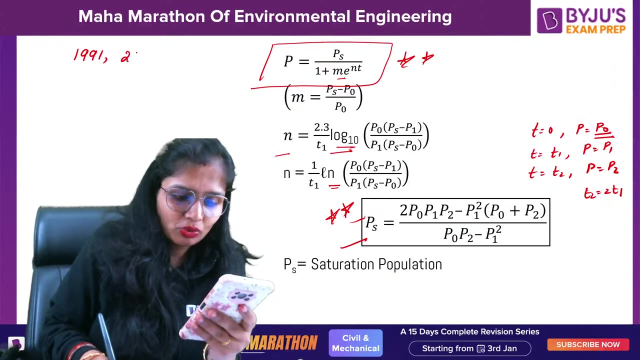 um, basically, they can ask you to calculate saturation population, and all only okay. they can ask you to calculate saturation population and all have it from here. population of a city in three consecutive years. three consecutive years, that is, 1991, 2001 and 2011. the population is given to you as 80 000. 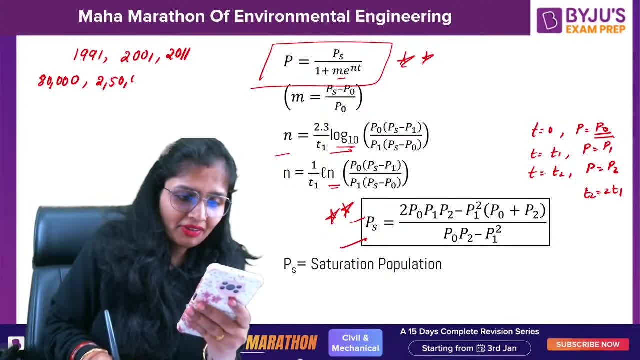 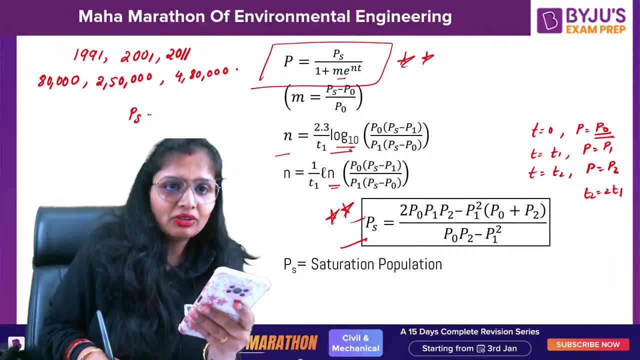 and the population is given to you as 80 000 and the population is given to you as 80 000, two lakh fifty thousand and four lakh eighty thousand. okay, and it is asking you first to calculate the saturation population. first it is asking you to calculate the saturation population. 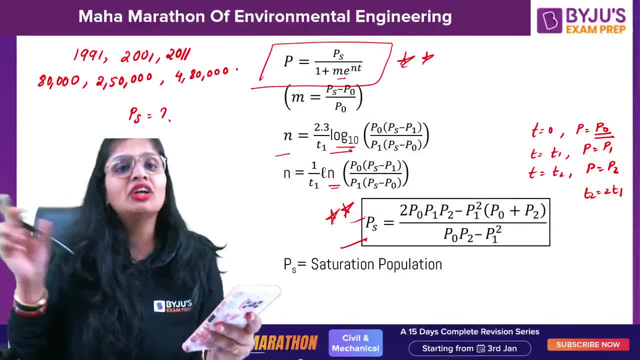 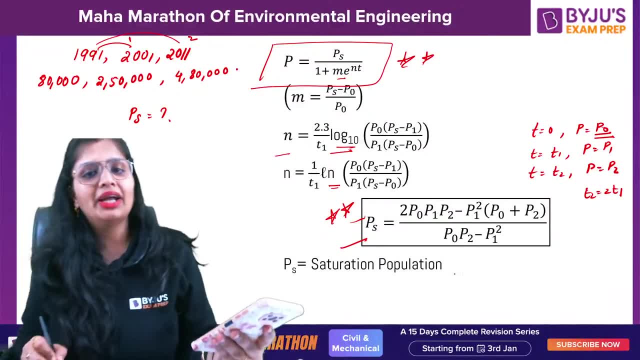 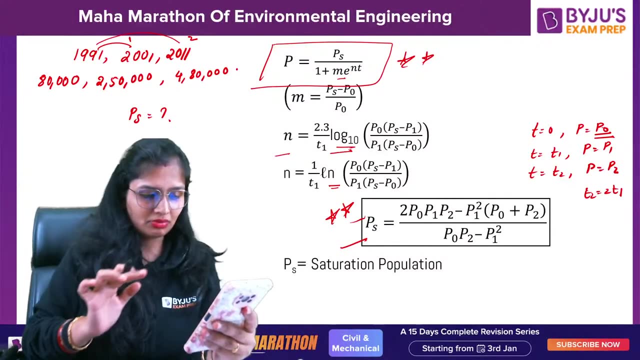 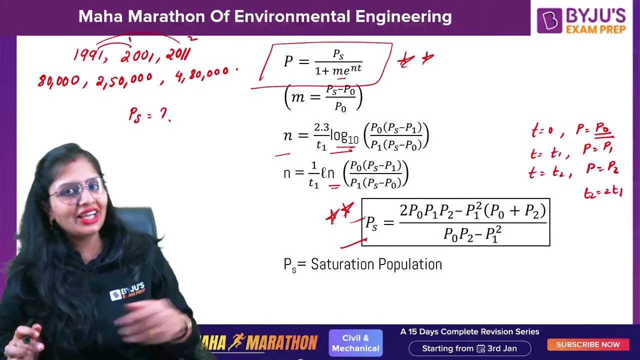 if such question comes first, you have to check it whether logistic curve is applied or not. check it out. from here to here it is one decade. from here to here it is two decades. yes, you can apply it. use the formula. calculate the saturation population. five minutes break. let us do a roshit quality of water, then a break. 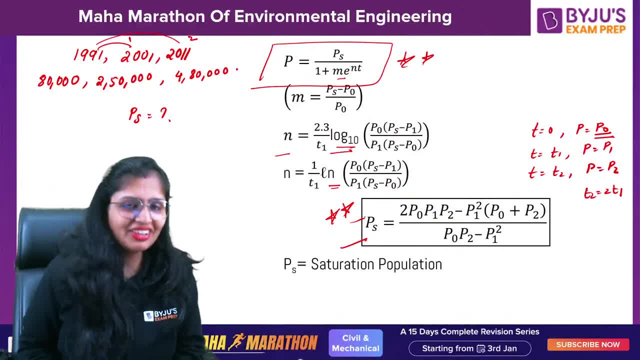 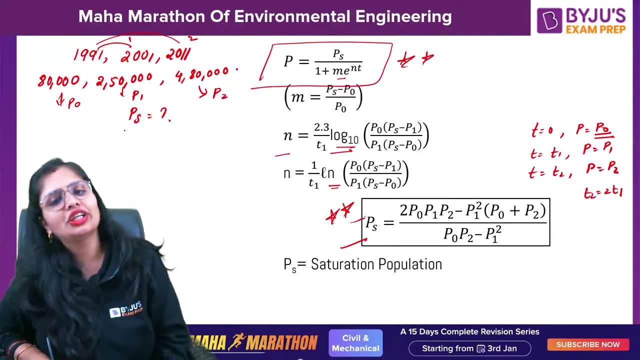 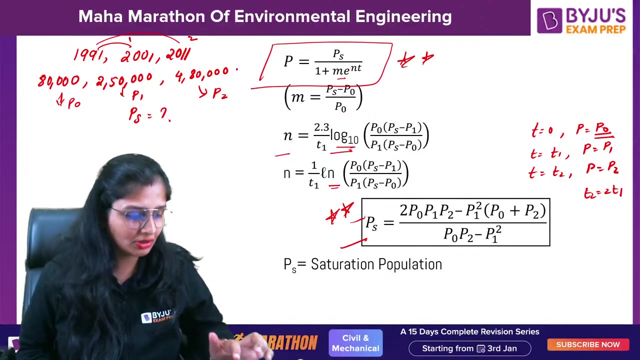 previous year. question has not been asked from this topic. come on guys, this is p naught, this is p1, this is p2. you have to calculate saturation population. no, no, no, not on our gate, so you guys can solve it in gate. they have not asked in eac conventional and all questions has been there from this topic. 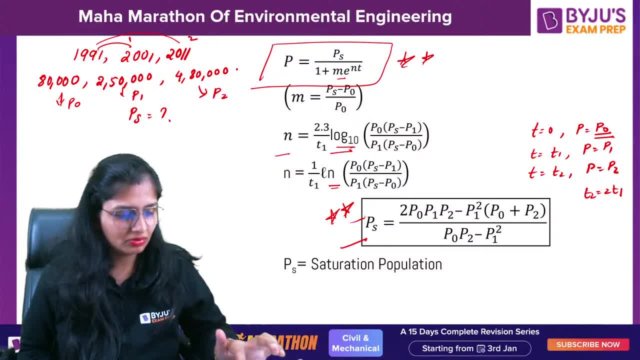 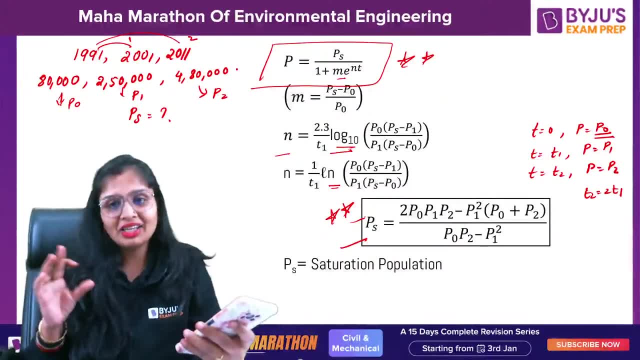 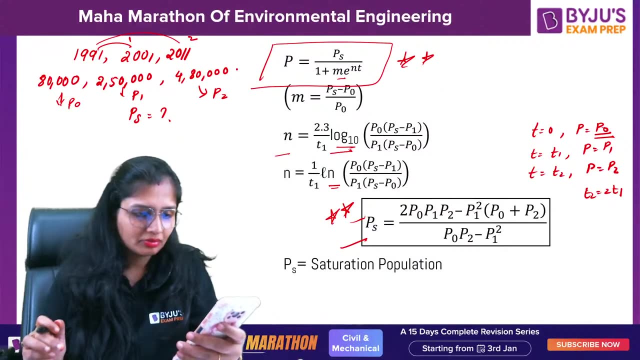 solve it. i know it is. it takes time, so better take out the zeros to be common. well, i have the answer for this one. the saturation population comes out to be 655602. so just check it out. just check it out so they can ask you, in one marks, these questions. 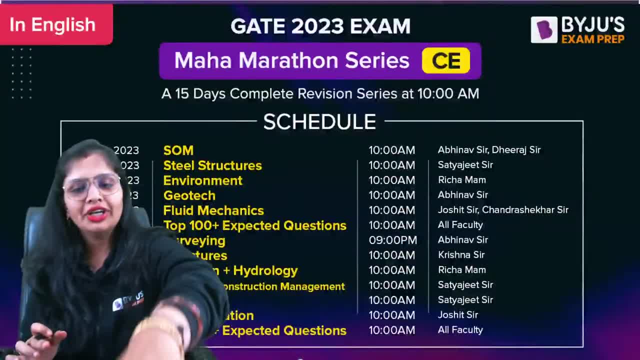 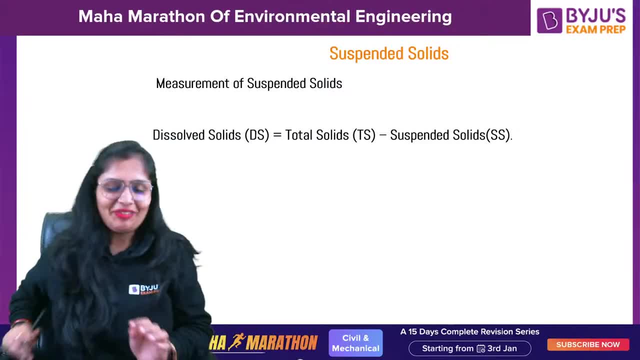 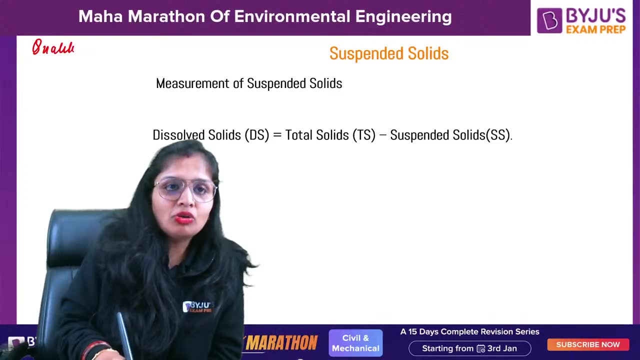 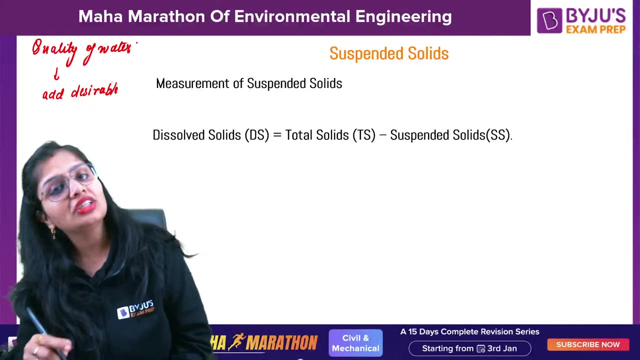 okay. so, guys, first we will do quality of water, then a break if you guys want. otherwise i thought of having it at two o'clock, okay, so fine. so now, talking about quality of water, i am going to talk about quality of water. when you talk about quality of water, when you talk about quality of water, the aim of quality of water is to add desirable quality. if it is not there, see, certain minerals are required by your body. but if it is not there, it is added. but if certain minerals are there more than which is required by your body, that has to be taken out. okay, so add desirable quality. if it is not there, it is added. but if certain minerals are there more than which is required by your body, that has to be taken out. okay, so add desirable quality. if it is not there, it is added. but if certain minerals are there more than which is required by your body, that has to be taken out. okay, so add desirable quality. if it is not there, it is added. but if certain minerals are there more than which is required by your body, that has to be taken out. okay, so add desirable quality. if it is not there, it is added. but if certain minerals are there more than which is required by your body, that has to be taken out. okay, so add desirable quality. if it is not there, it is added, but if certain minerals are. 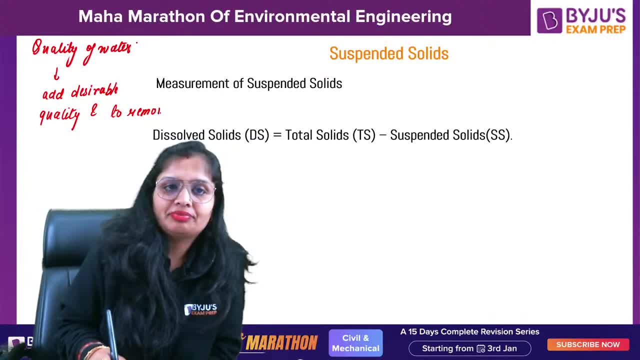 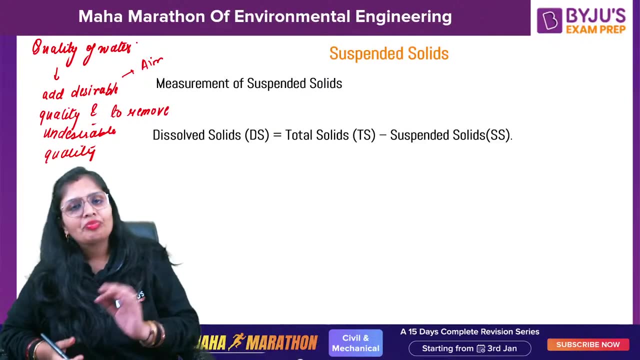 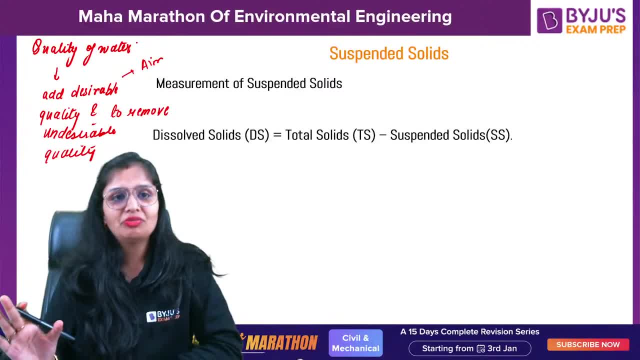 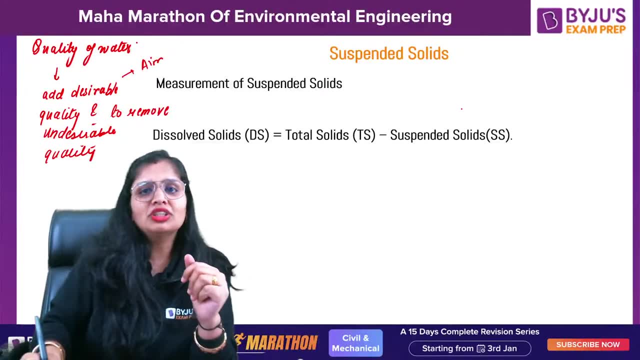 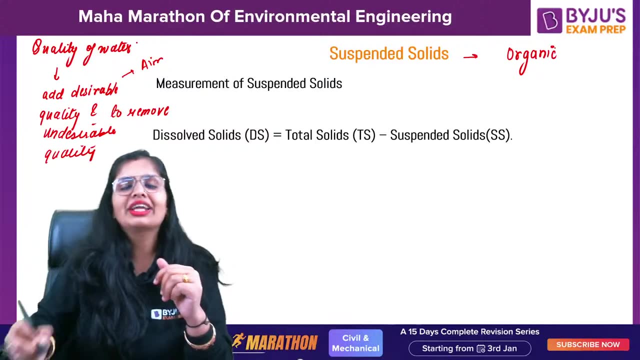 So when you talk about parameters in physical parameters, physical is something which you can touch, feel and see. Now, when you talk about suspended solids, the suspended solids, if you talk about the source, source can be organic. Generally we say organic, you know organic. 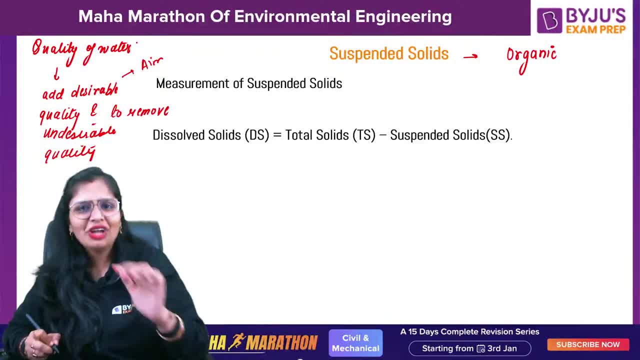 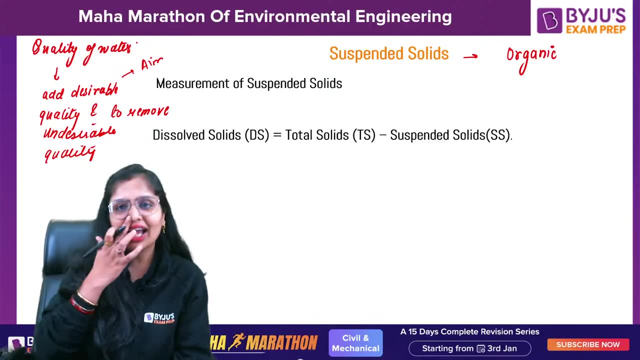 vegetables are coming. nowadays You have the standard. you know I don't take normal sugar, I take organic sugar. I prefer organic rice. you know those kind of people. So organic is where you get carbon in, that okay, And organic particles are there, or inorganic like sands. 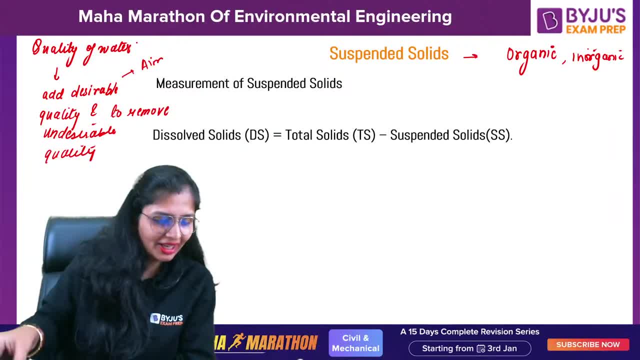 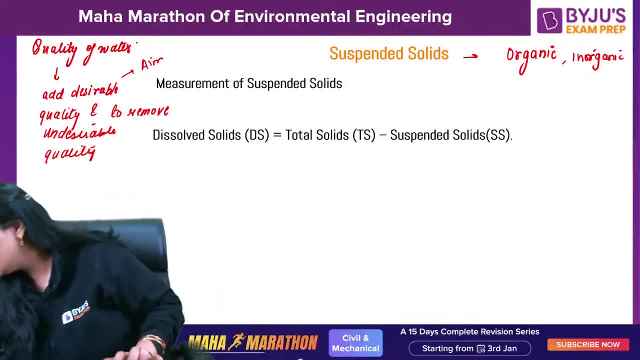 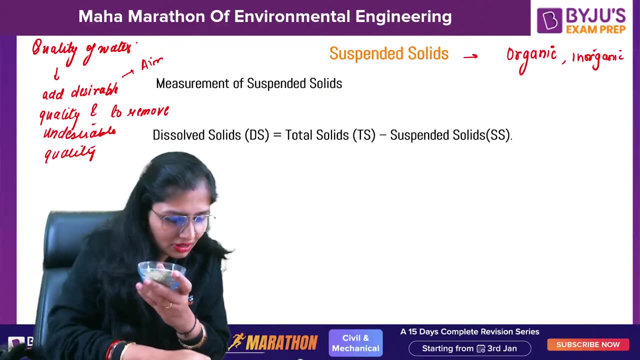 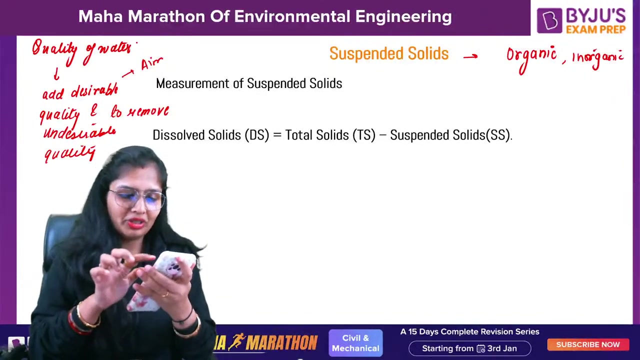 silts are there. okay, Now let's do it. I have a glass of water with me right now. okay For showing it. I have taken a glass and I have some. is it visible or not? Okay, Actually, in my phone it is going two minutes slow, So I need to. fine Now I can show you in the 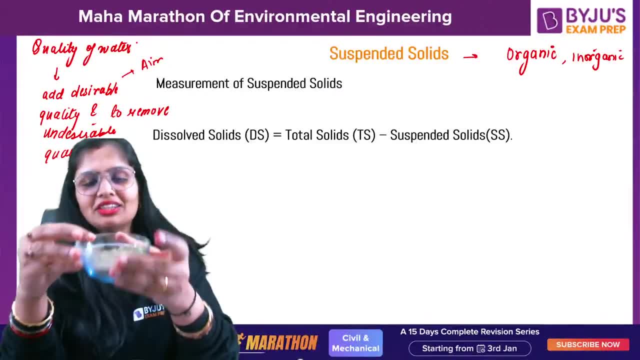 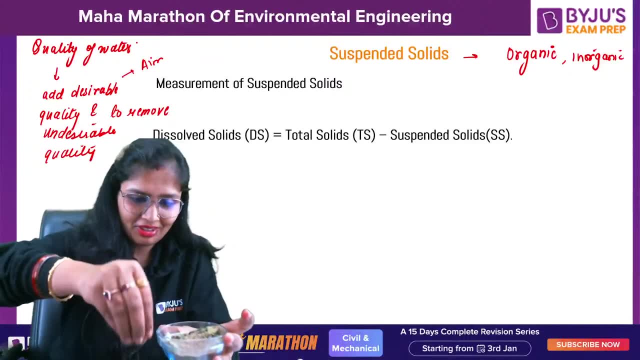 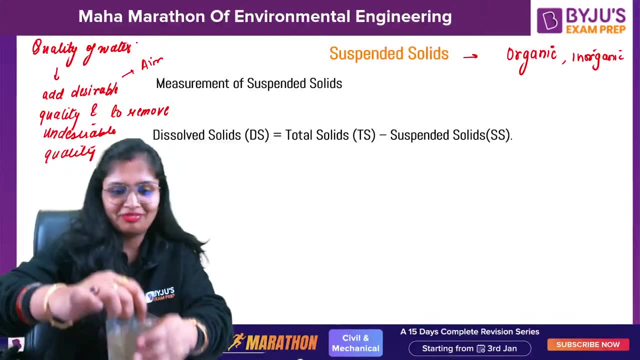 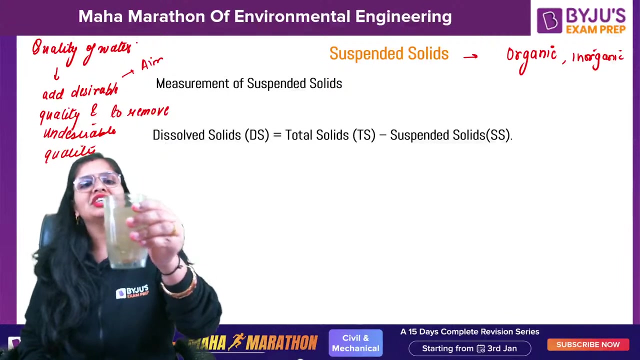 camera. I guess you can see some sands, silts, particles are there, So I will pour this now. Let me stir it also now. So a water. initially it was a clear water. okay. Now this is the water. Will you drink this? 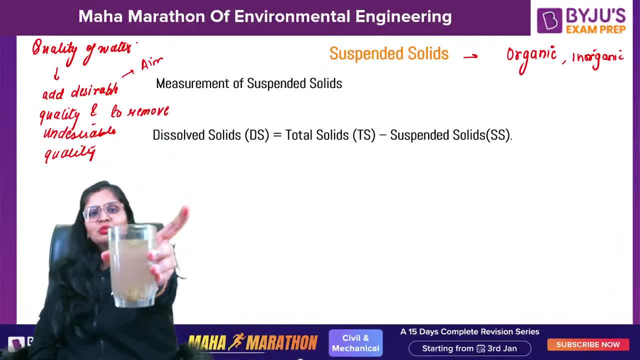 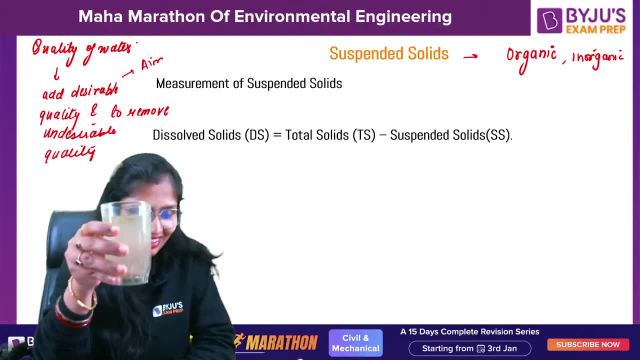 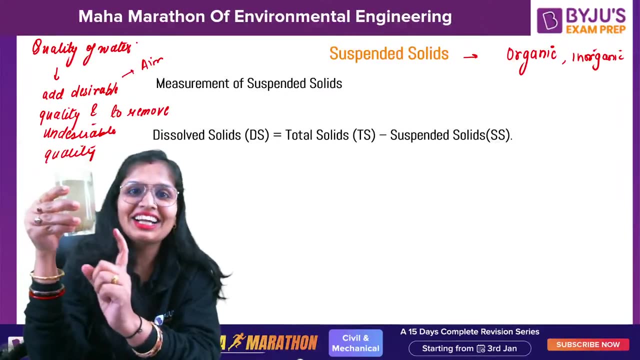 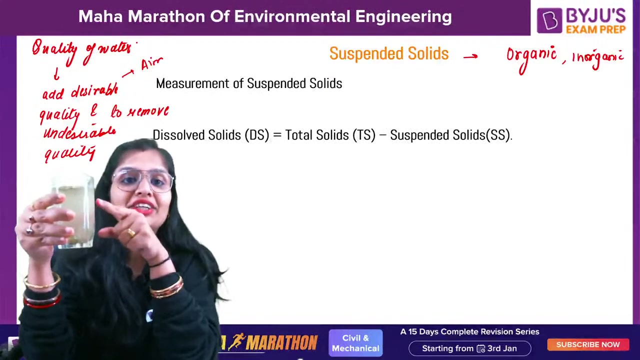 water, guys, Will you have this water? Come on, everyone, everybody. Will you have it? Why, If I would have told you that this is Jaljeera, then you guys would have have it Suspended. solids, Organic sources, organic and inorganic. Now tell me the impact. 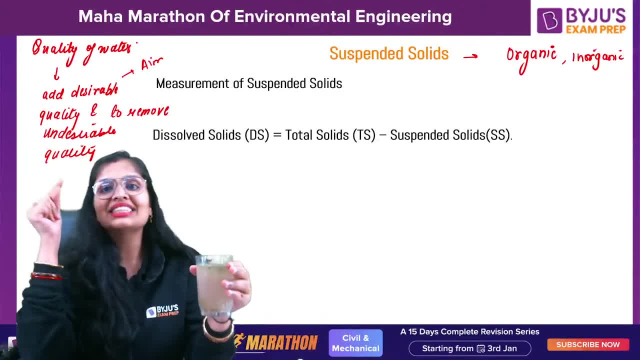 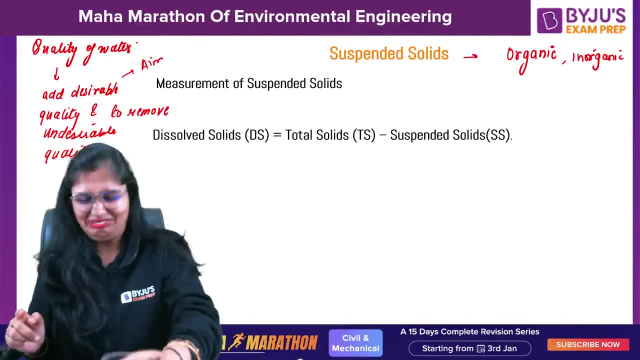 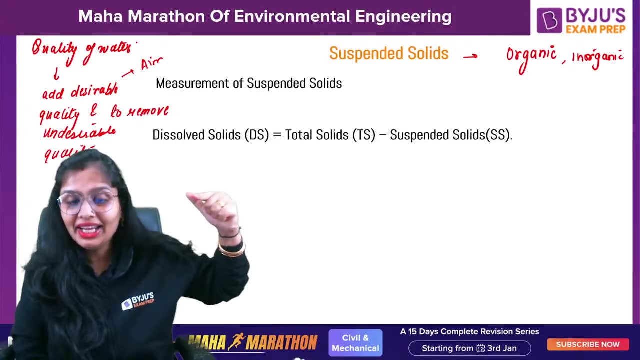 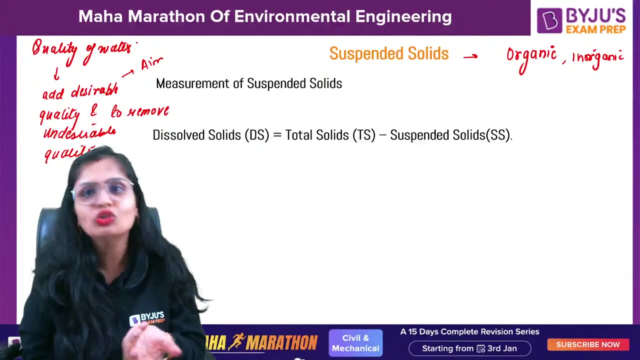 The first impact which came right now is psychological impact. The moment you saw it, you felt: I can't have it Disgusting. This is psychological impact. Okay, So this is because it doesn't look good. We say in Hindi: dikhne mein acha nahi hai, to hum nahi pih rahe hai. The thing which doesn't 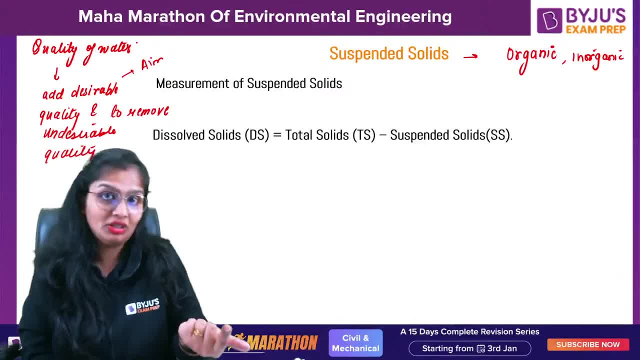 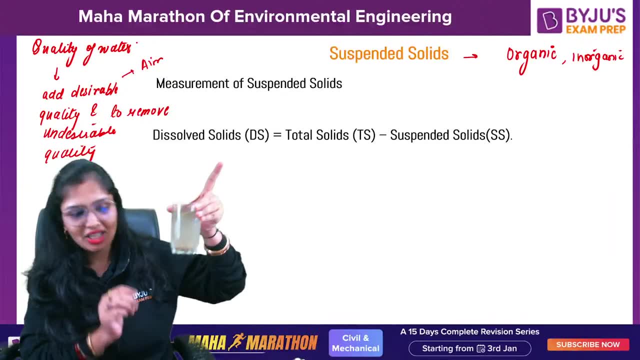 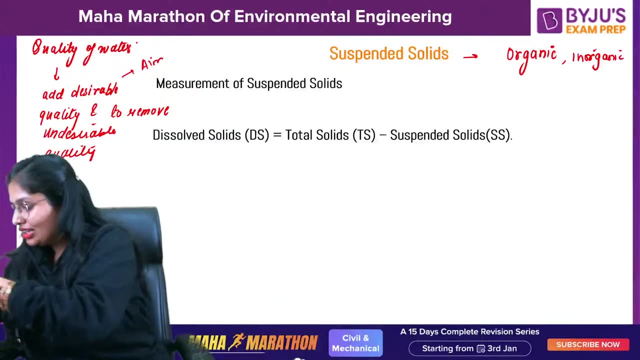 looks good, we have that perception that it won't be good. Okay, So this is because it is aesthetically displeasing or unpleasing to our eyes, So we won't drink this. Okay, I'll use this for turbidity also, Wait. Okay, So this is for suspended solids Now. 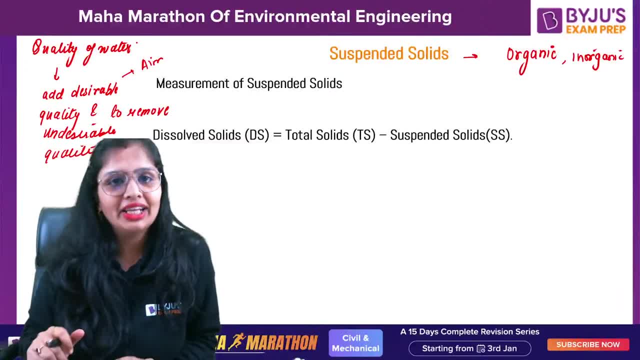 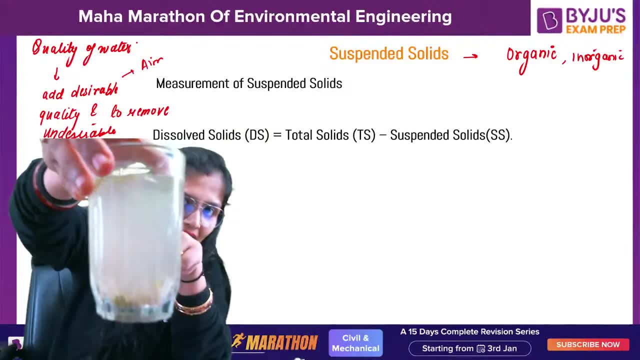 what happened? What happened in this organic and inorganic are there? Now comes the question In this: what was happening? If you see some solids are dissolved, You can see the color. I'm putting it in front of camera. You can see some solids have settled down, which you guys. 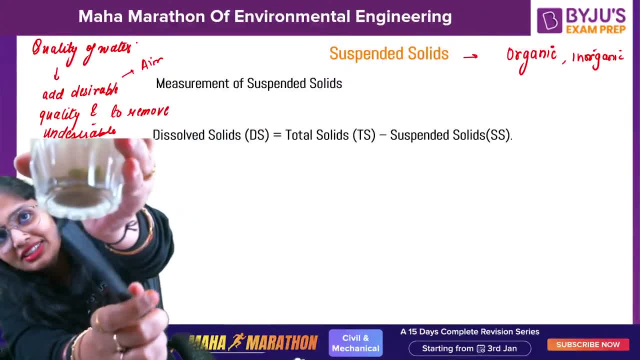 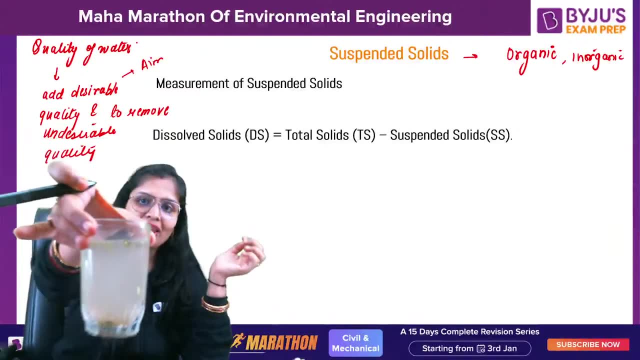 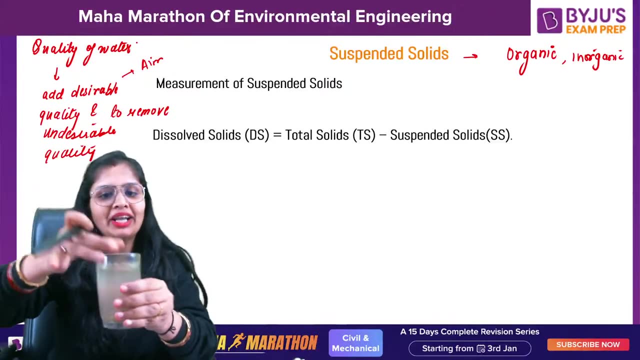 won't be able to see. I guess, If you can see, the solids have settled down also, Okay, And some solids are dissolved also, which you can see it here. Okay, So that suspended solids, or basically first the total solids, can be suspended or it can be dissolved. So 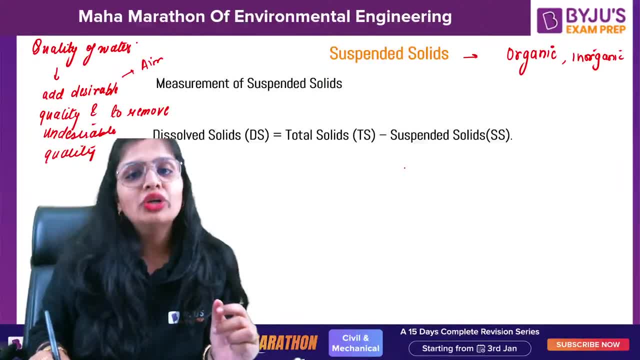 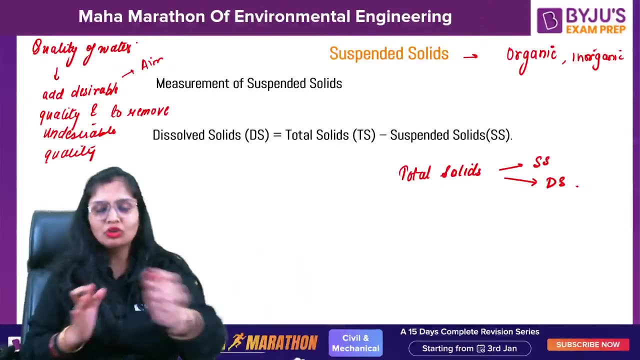 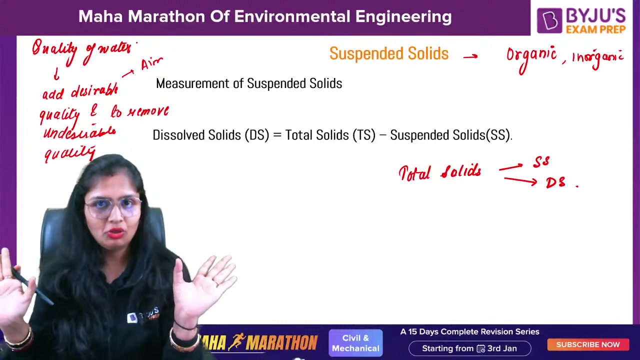 the total solids which you have. the total solids, it is suspended and dissolved solids. Now, this what this gate examination question has In gate examination question has been asked from this topic, So let's talk about it. I'll tell you the whole procedure. You have to solve the question. Okay, Now total solids. 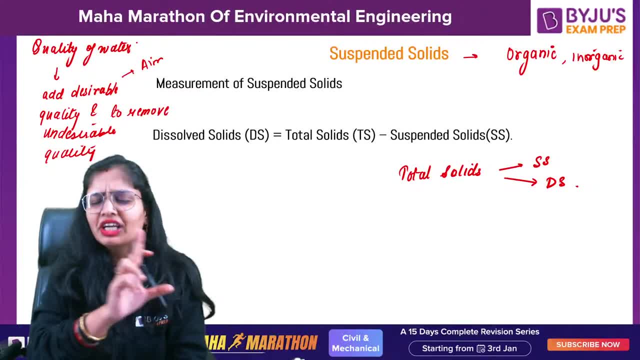 suspended solids, dissolved solids. In gate examination: never, ever. they mention what is total solids, what is suspended solids. They will tell you the procedure and they will ask you, based on your knowledge, what is total solids and what is suspended solids or what is dissolved. 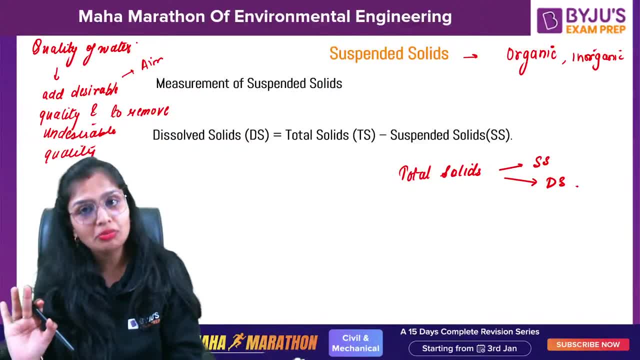 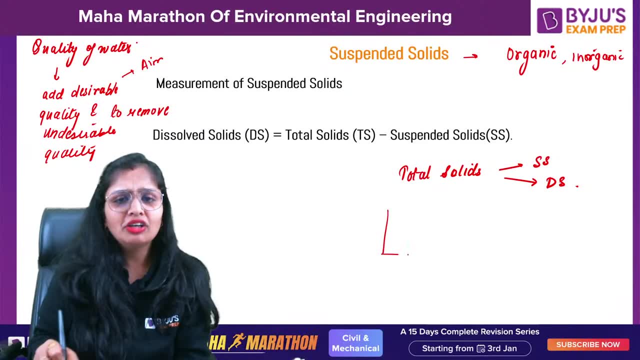 solids. So it is very, very important. So let's talk about it. So let's talk about it, In that you should know the procedure. Now, remember total solids. if you want to calculate total solids, no need of any brain in this. suspended solids will be there, dissolved. 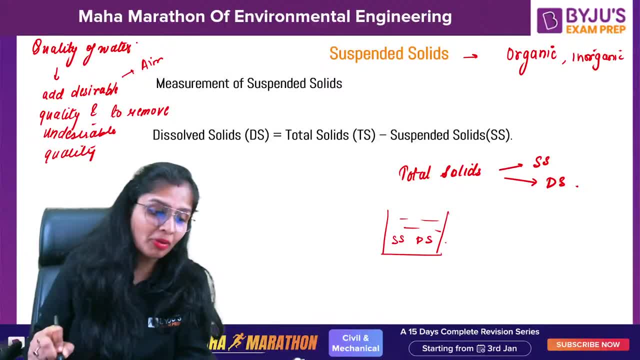 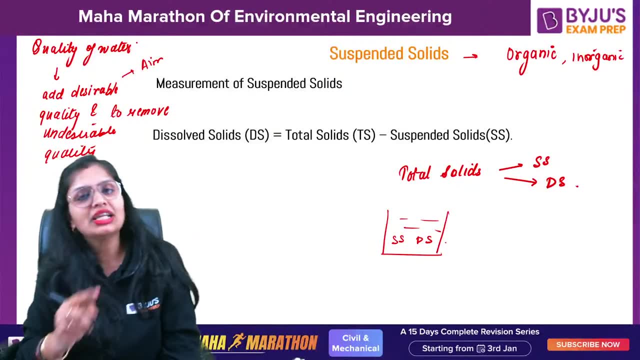 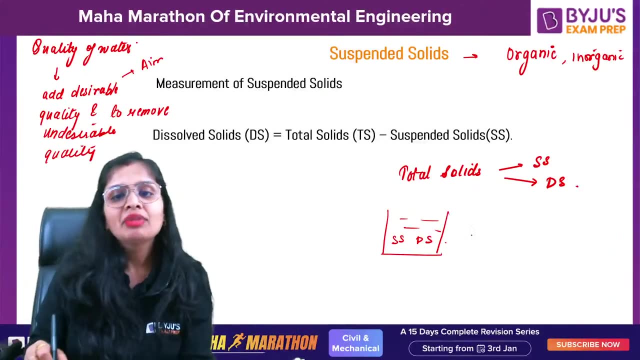 solids will be there, Settlable solids I will talk about in the case of Jalapati, in the case of wastewater sewage, because that time I'll be telling you about the hem of cone also. Okay, Right now we'll talk about suspended and dissolved, Fine, So this is 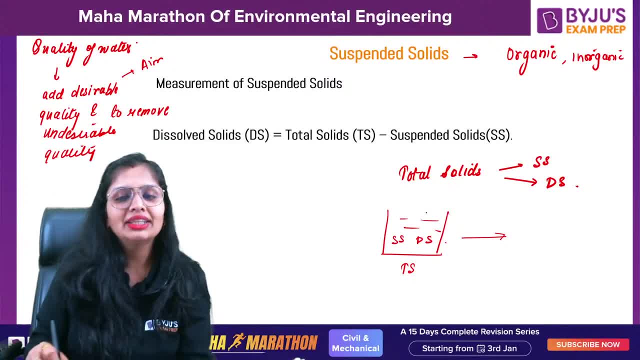 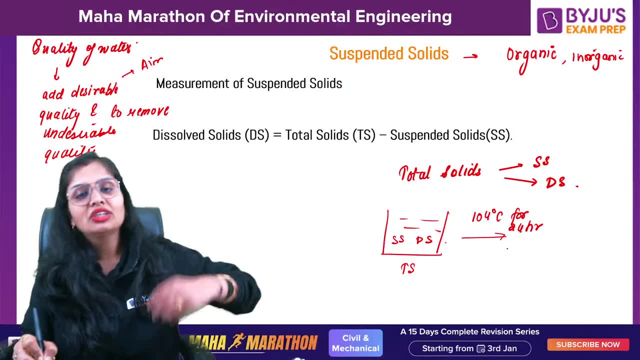 the total solids. Now let's talk about the suspended solids. So let's talk about the total solids. You will do what You will take this, heat it at 104 degree Celsius for 24 hours, directly, just measure the weight. So the technique by which you calculate the solids. 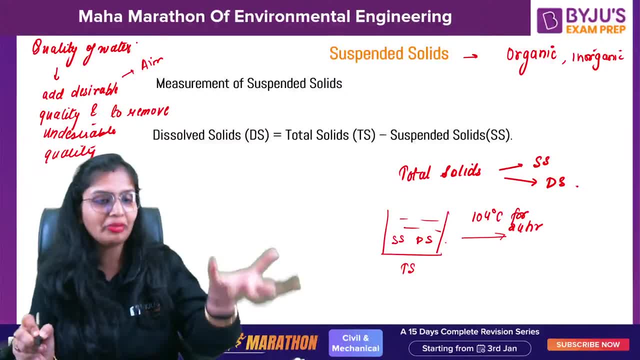 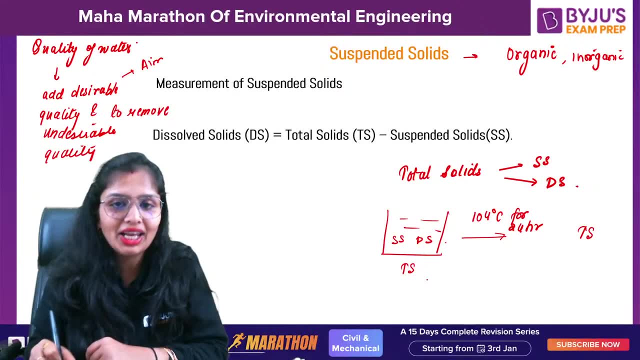 weights. and all this is gravimetric technique. Gravimetric because you are measuring the weight. Okay, So 104 degree Celsius for 24 hours. this will give you, you can calculate the weight. And let us suppose if I took 1 liter of the sample, so total solids weight will be in mg and 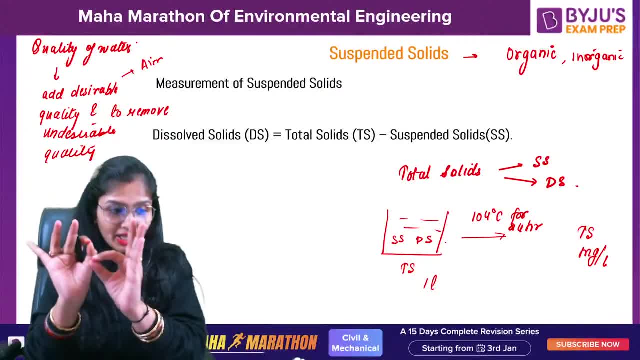 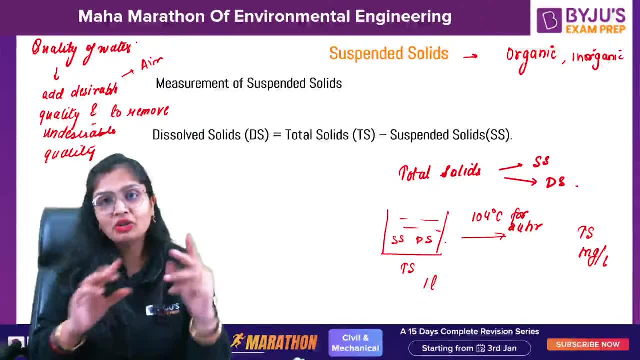 concentration will be mg per liter. Remember why I am telling you, Because in the question they will directly tell you that the sample was there. it is heated. If it is telling you, remember this is it is talking about the total solids. Now, next, what they can do is 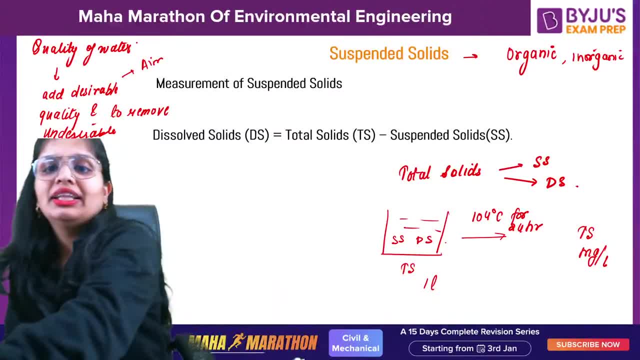 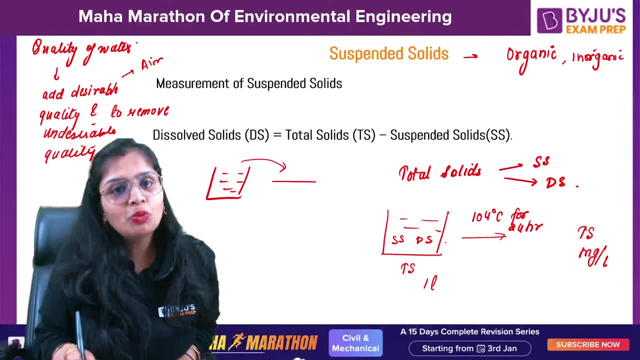 next, what they can do is, if they are telling you that the solids were there, or basically the sample was there, it is pour it through the filter paper, Okay. And then if it is pour it through the filter paper, that suspended solids will retain. 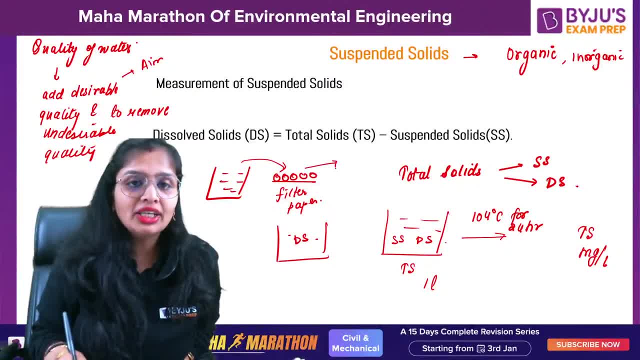 the dissolved solids will go. So these suspended solids will again be heated for 104 degree Celsius for 24 hours and then we will measure the weight. if it comes out to be x mg, So you will say the concentration of suspended solids will be x mg per liter, because the sample was 1 liter. Okay, 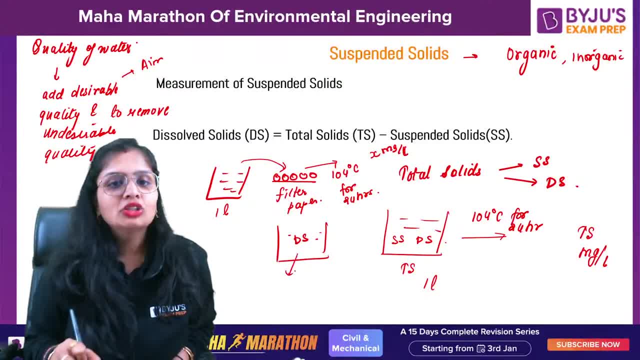 Similarly, dissolved solids have pour out from the filter paper. they will go through the filter paper. so you will measure the weight and you will say: this is, let us suppose, if y mg is there, So y mg per liter. Again, you will heat it as 104 degree Celsius for 24 hours and from here you will get dissolved solids. 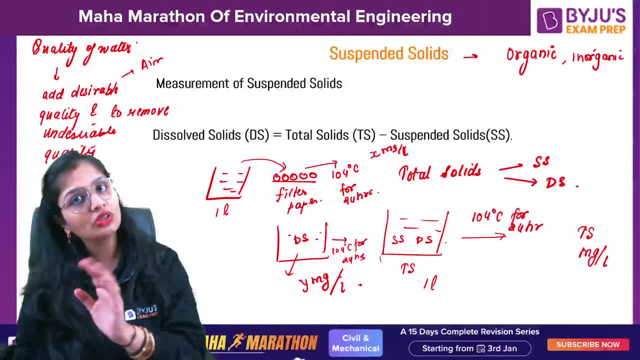 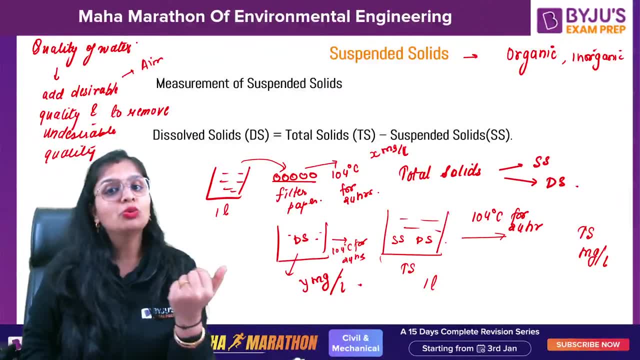 So, ma'am, how come we will know that, whether it is suspended or dissolved In the question, it will mention you. It will not mention you this is suspended or dissolved, but it will mention you the procedure, that it is poured through a filter paper or, basically, it is heated, the sample is. 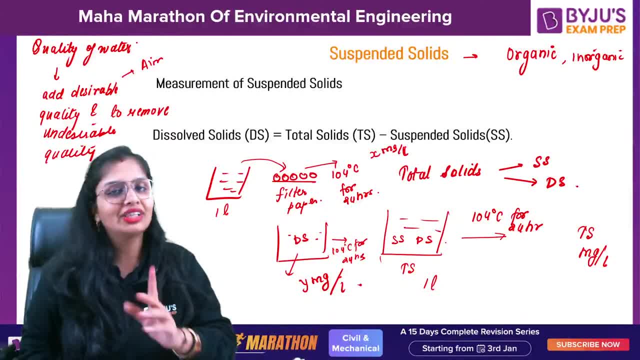 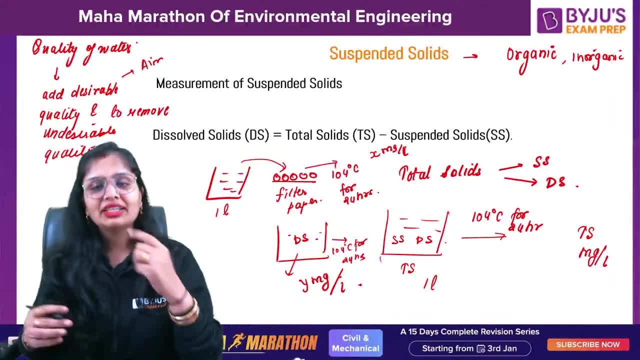 directly heated and all. So with the help of that, you will get, whether it is total solids, suspended solids or dissolved solids, Clear Now the next thing which comes is: the next thing which comes is in the suspended solids, in the suspended. 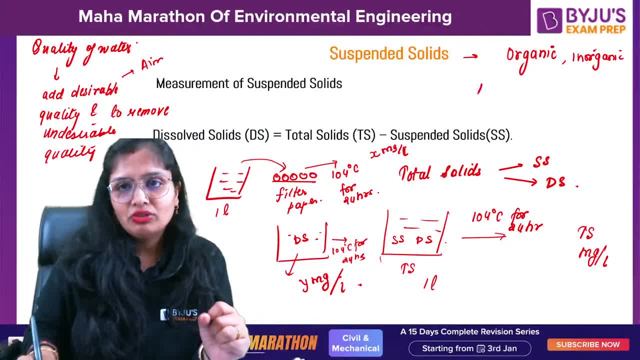 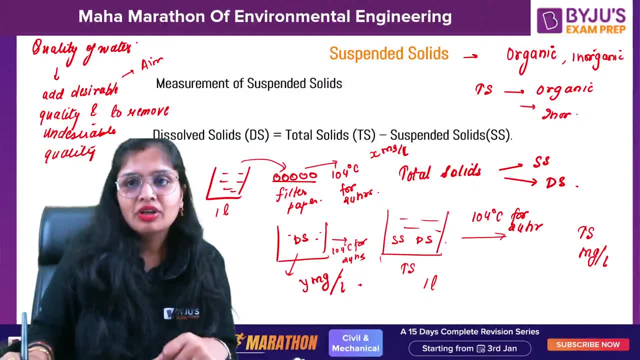 solids. there is an another category, if you know. let me tell you: total solids. there is organic solids and inorganic solids. Shall I go in the detail, Yes or no? If you want I will go, I will add an extra slide. 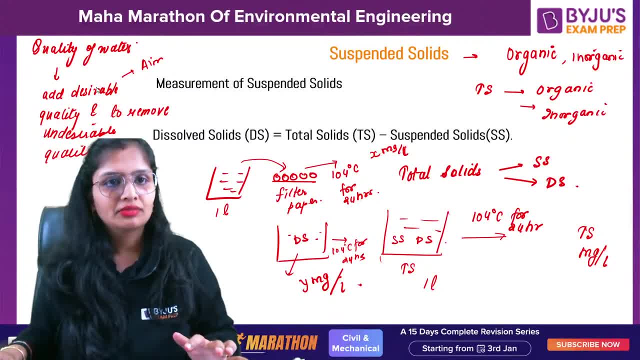 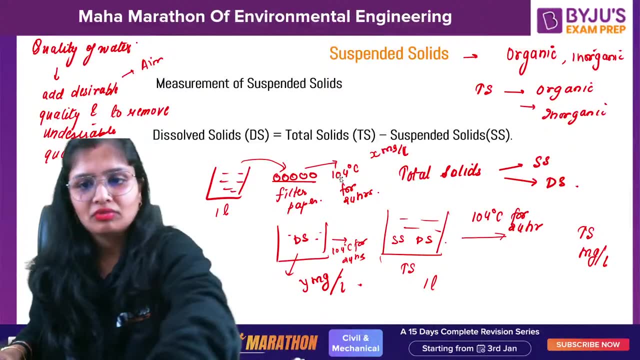 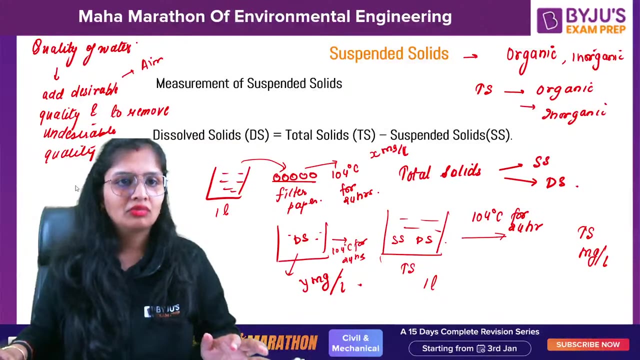 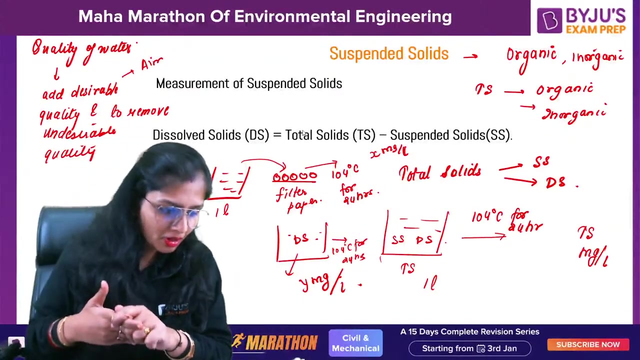 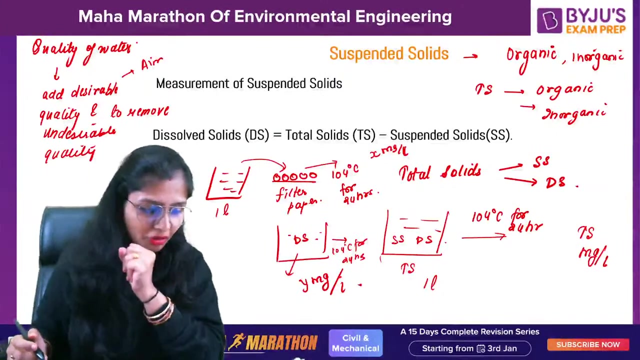 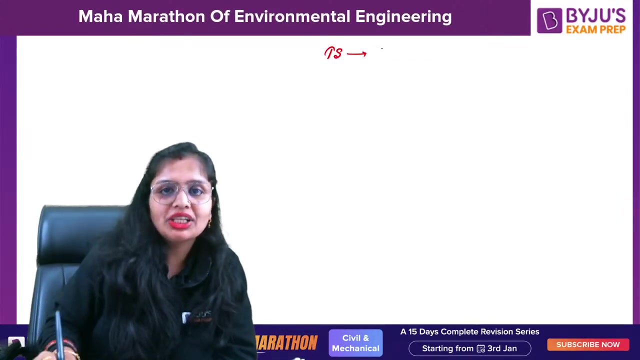 If you want I will go, Otherwise I won't. That's why I am asking you. Okay, fine, Because they can ask you and they have asked questions from it, Diksha, That's why I have to go. it actually So total solids. they have asked question actually from this in your GATE. 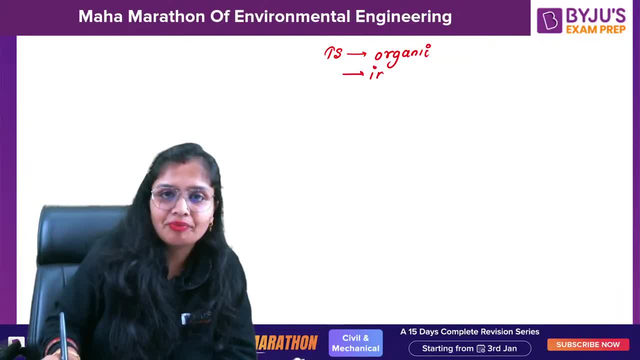 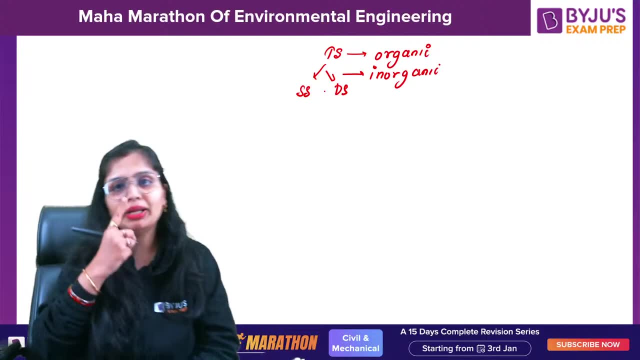 examination It is inorganic and inorganic. Okay, That means that means suspended solids can be inorganic, organic. dissolved solids can be inorganic and organic. Remember organic solids. it is not necessary in the question. The best way to complete E in one. 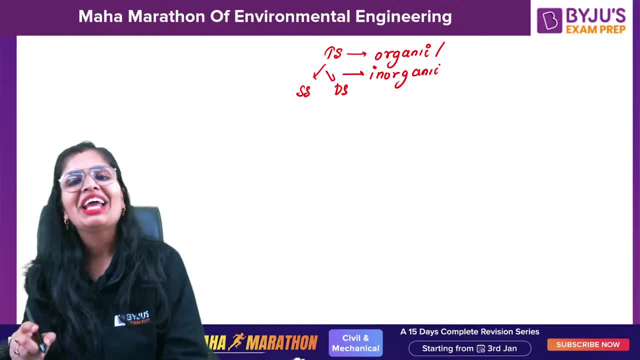 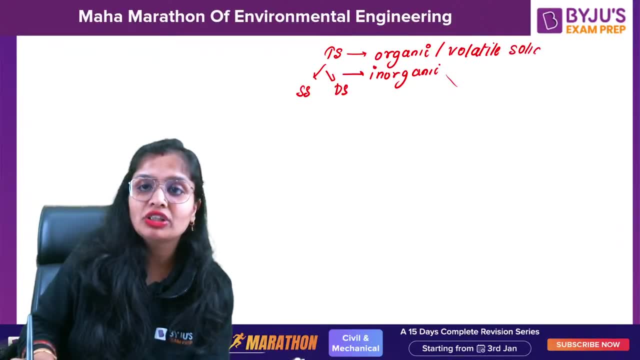 day is to follow Richa Gupta's Mahabharata. Okay, So organic solids is also known as volatile solids. Remember? no, not necessary. They will ask you what is the organic solids? Inorganic solids. they write it as fixed solids or they write it as non-volatile solids, All the name. 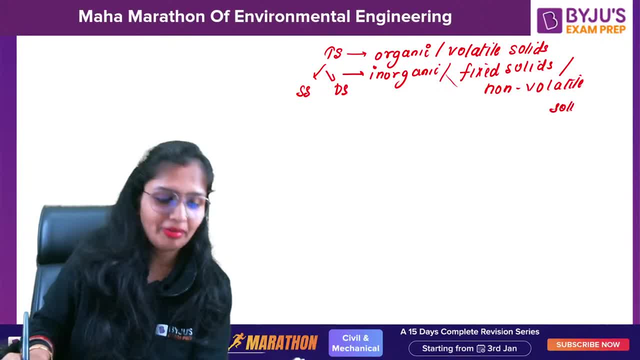 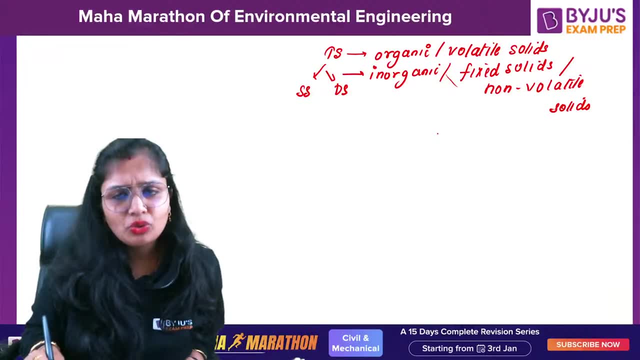 you should remember, Otherwise you will get confused in the exam. Okay, Now listen to me very carefully. Let us suppose, if total solids is there, it can be organic, means there can be carbon present in it. It can be inorganic also. So there is again. 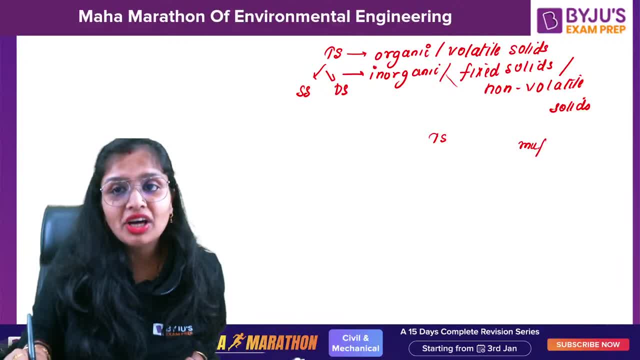 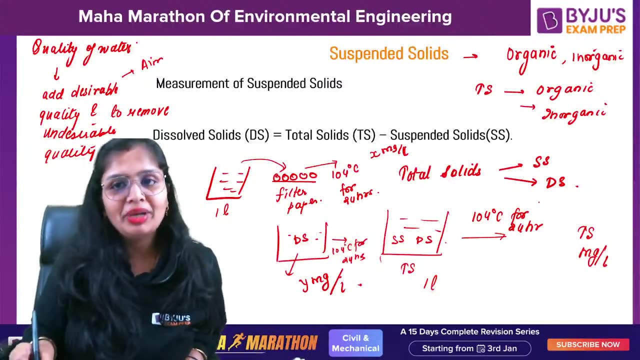 this is one marks question. There is a special furnace known as muffle furnace. Now, what is the speciality In this? you supply high heat of 600 to 650 degree Celsius. So you take the total solids. You have done what You have taken here: you have measured the total solids You will take. 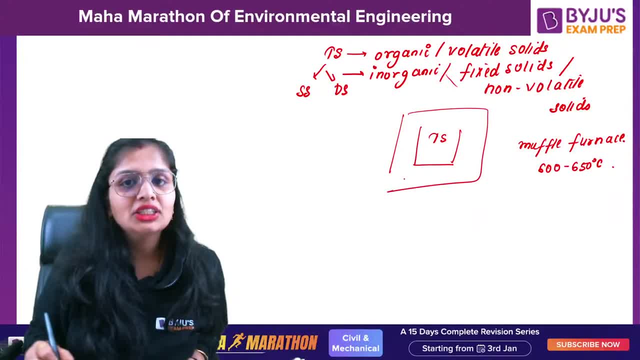 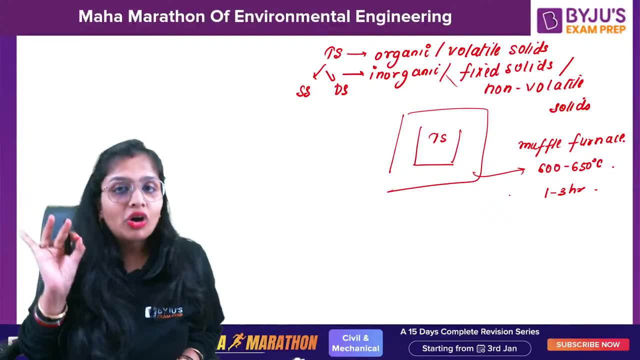 this Okay. You will place it in a muffle furnace for 600 to 650 degree Celsius temperature for 1 to 3 hours. What will happen? The organic solids has the tendency to vaporize, So they will vaporize. The things which will remain will be the non-volatile solids or the inorganic solids. 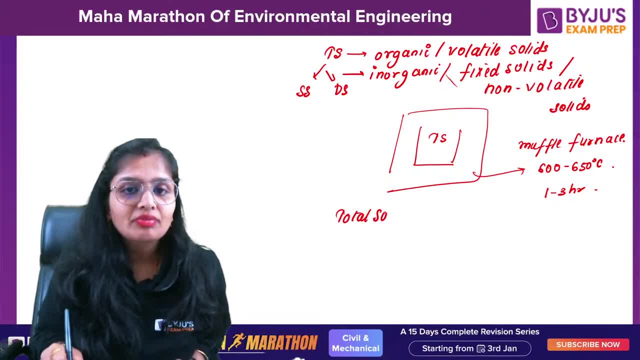 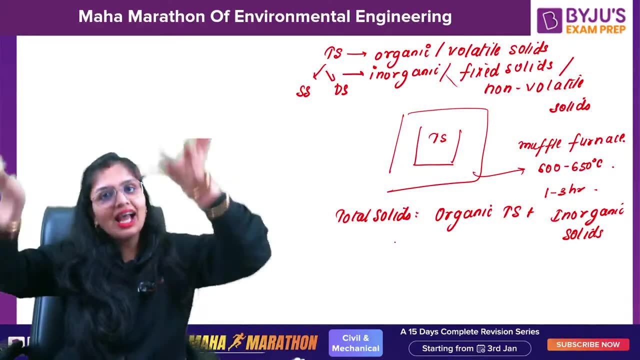 So total solids is equal to this. They can ask you Remember organic total solids plus inorganic total solids. So what will happen? Total solids value you already calculated. Organic has been what vaporized Inorganic will. 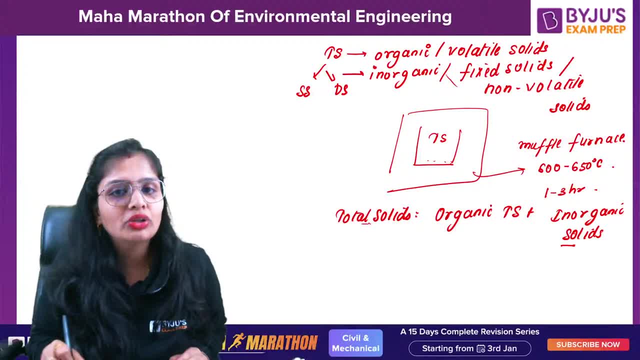 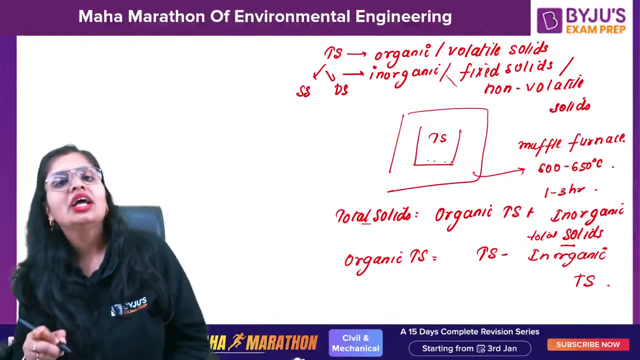 remain here. So you will measure the weight of inorganic total solids, you know. So with this you will get organic total solids. This will be total solids minus inorganic total solids. Okay, Question has asked. been in your gate examination. They write non-volatile, volatile Sometimes. 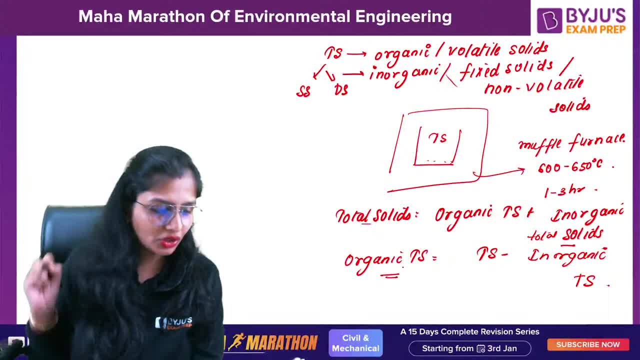 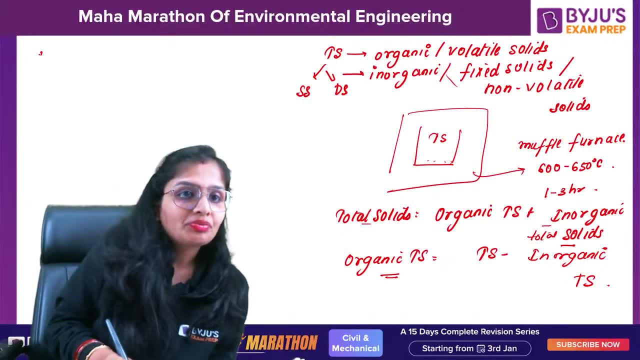 they write the fixed solids concentration. That is the reason you should know this. Okay, So total solids- organic total solids, Inorganic- already mentioned. Now, organic total solids is organic suspended solids or it can be organic dissolved solids. So what you can do is what you can do. it. you can take the suspended solids. 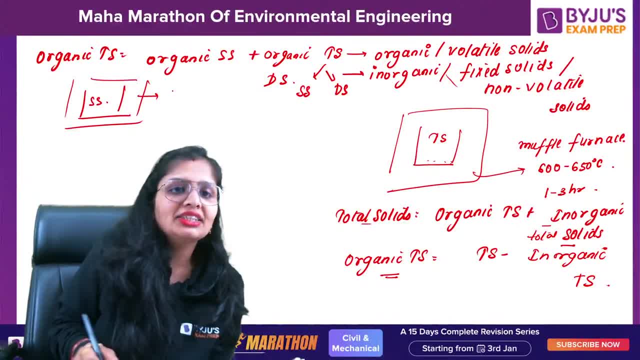 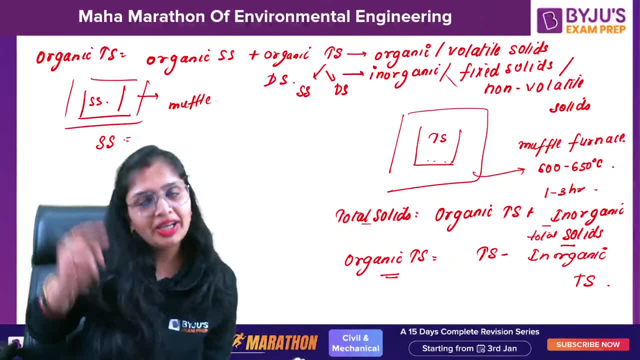 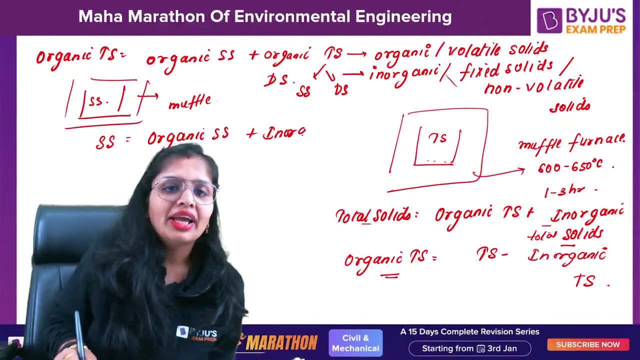 which you have measured, put it in a muffle furnace. So again, what you will get Again what you will get: Suspended solids. you already know Inorganic suspended solids will settle Similar procedure, not to repeat again and again: Inorganic solids, inorganic suspended solids will 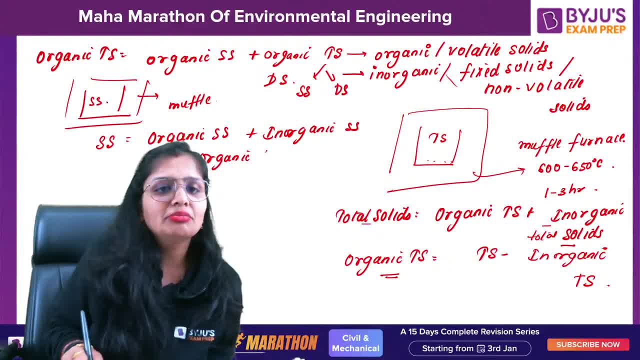 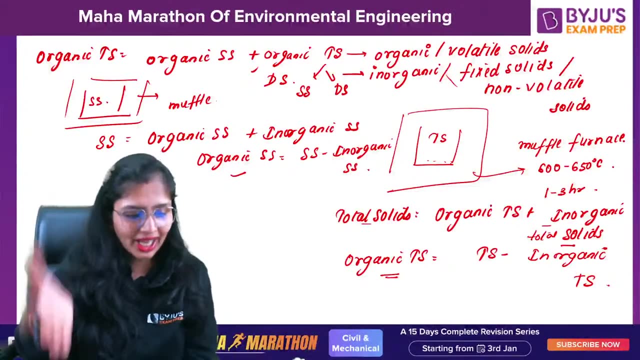 settle. You will get organic suspended solids, Simple Suspended solids, minus inorganic. So from here you will get, from here you will get organic dissolved solids. As simple as that, Okay. So in such manner you can get organic suspended solids, inorganic suspended solids, organic dissolved solids. 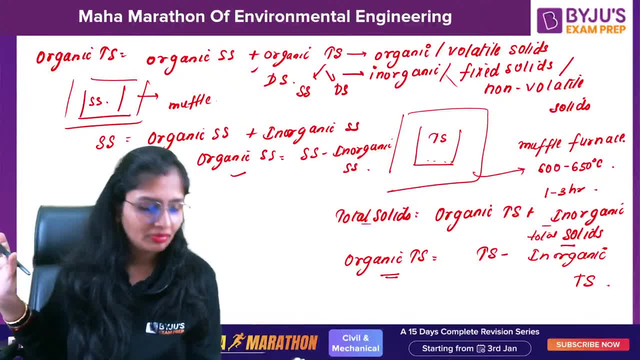 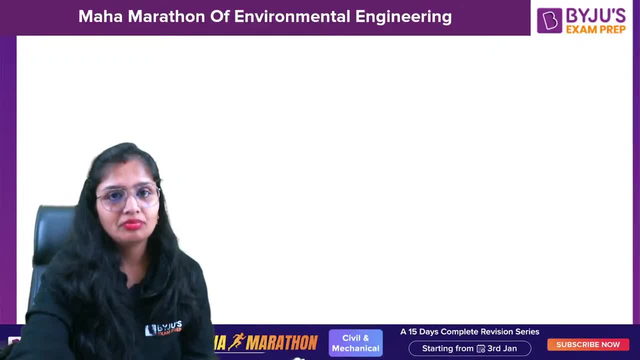 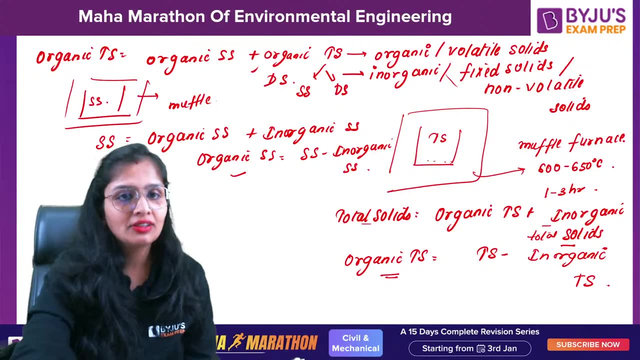 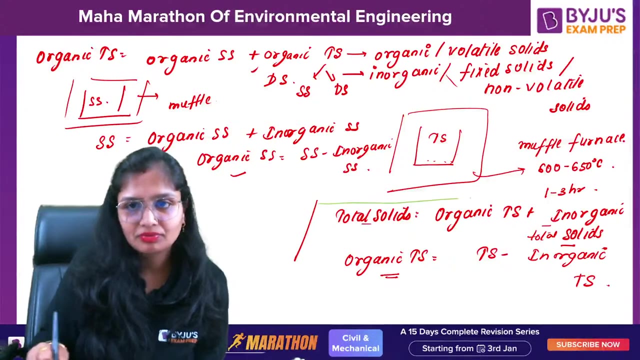 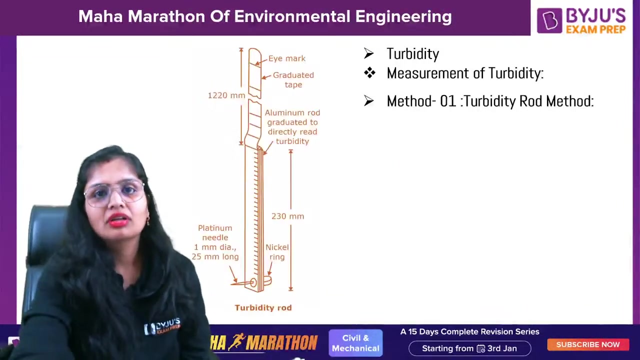 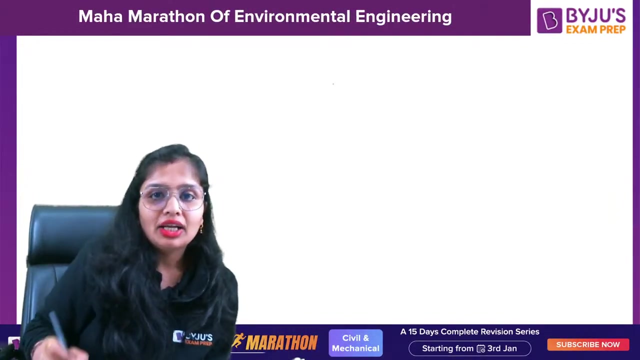 inorganic dissolved solids. Is it clear? Clear, everybody. So this is the whole procedure. So, Amy, Vishal, everybody, Gargi Girish, everybody, clear, Okay now talking about turbidity. Okay, Now let me tell you a few things. first, In the code. 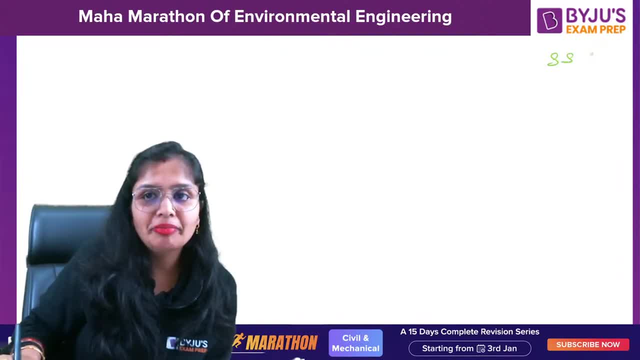 there is no limit mentioned for suspended solids. No limit mentioned for suspended solids. Limit has been mentioned for dissolved solids. okay, limit has been mentioned for dissolved solids. no limit has been mentioned for suspended solids. Firstly, secondly, if I talk about, secondly, if I talk about turbidity, turbidity. 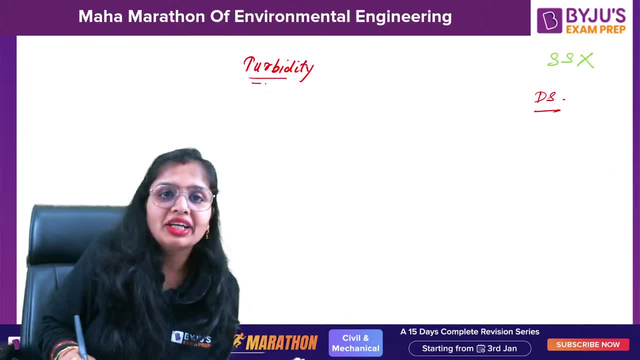 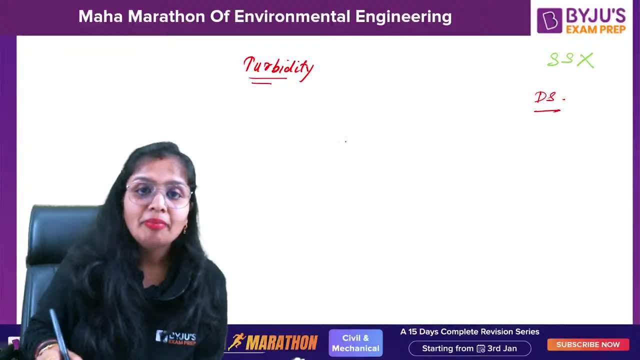 is also: you can say the more amount of suspended solids, the more amount of turbidity. But remember you cannot measure turbidity by gravimetric technique, because there are two things that you should know. I won't repeat it again, So I am telling you in detail right now. 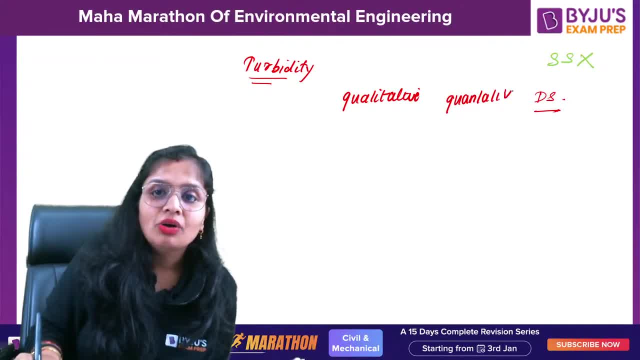 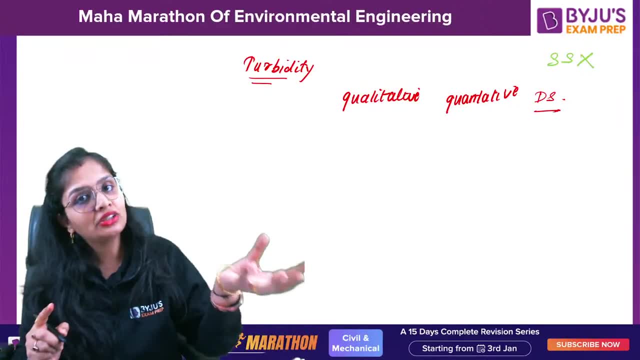 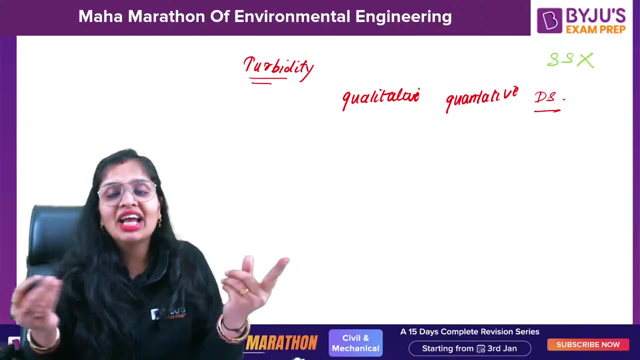 qualitative and quantitative. okay, More the suspended solids, more the turbidity. But if 10 mg per litre is the suspended solids, 10 mg per litre will be the turbidity. no, okay Amount. you cannot say quantitative analysis, you cannot do qualitative. it is true that more the suspended 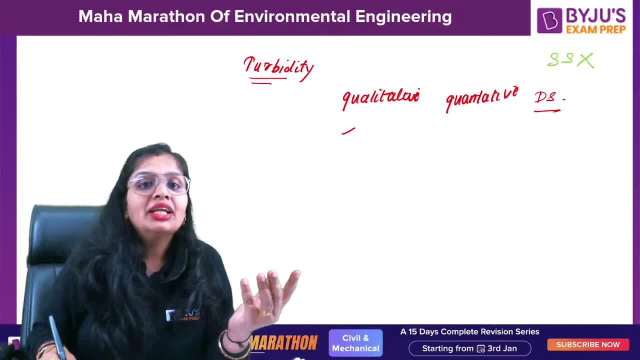 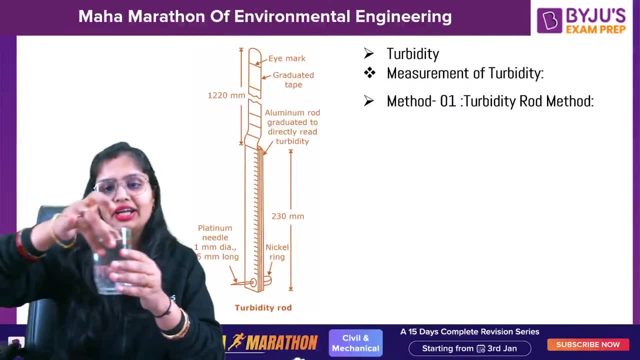 solids, more the turbidity. okay, Now, turbidity means what? Now let's understand it with the help of an experiment. Again, I have done it in sandika funda also. Okay, this is the glass. I guess you 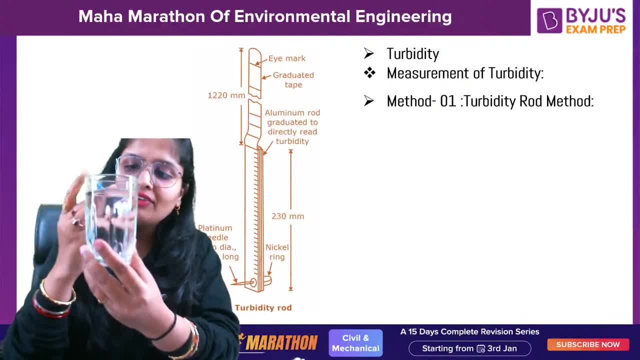 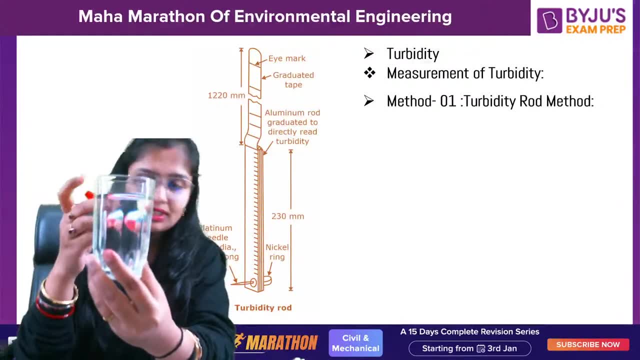 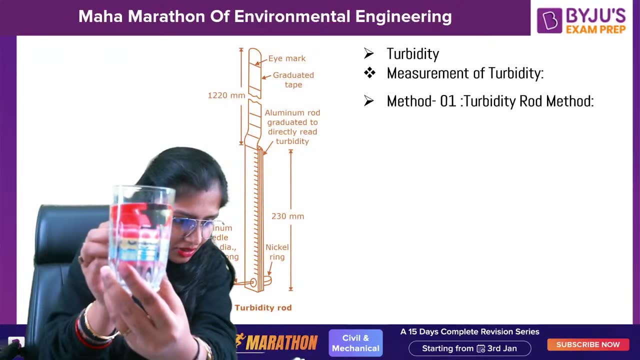 can see it. I have to check it myself. Could you read it? what is written? Okay, this is the glass. Can you see what is there behind it? I don't know in the camera which is. I think you should read it because I will be able to read. 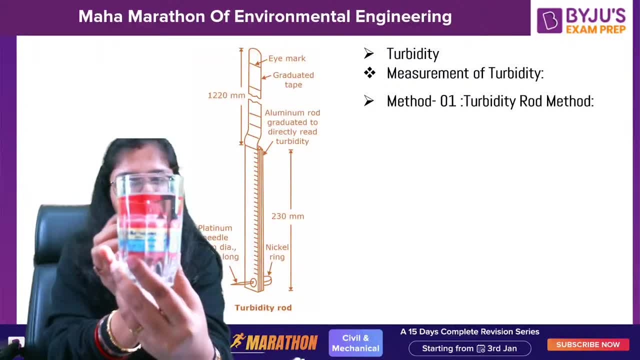 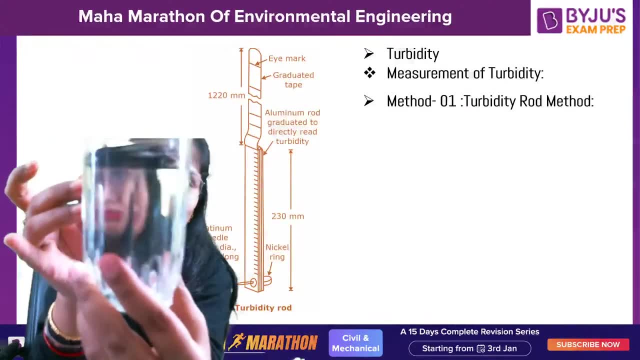 Can you see what is there behind it? I don't know in the camera which is, you guys can see it. Can you mention in the comment what is written Actually you should in this problem right now? Oh my god, what is that? 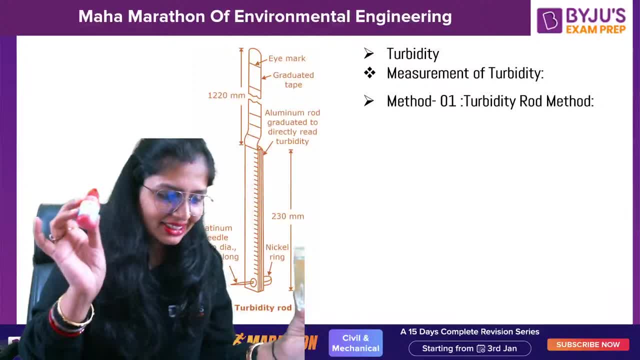 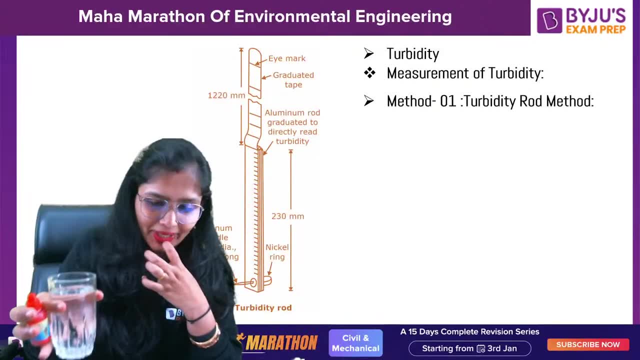 Dikh raha hai. Okay, fine, You can see it basically. basically, it's written art line, but I can see it clearly, but because of the lights you cannot right now. okay, Otherwise, we can see it clearly, but because of the lights you cannot right now. okay, Otherwise, we can see it. 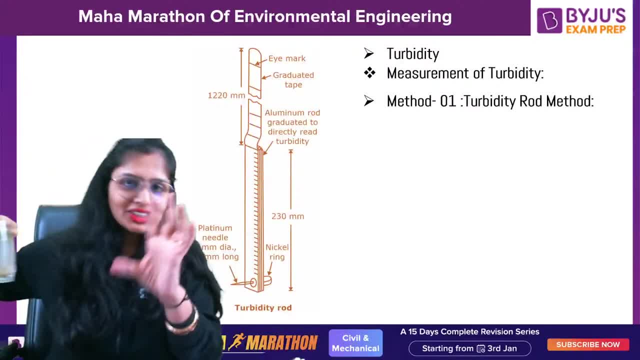 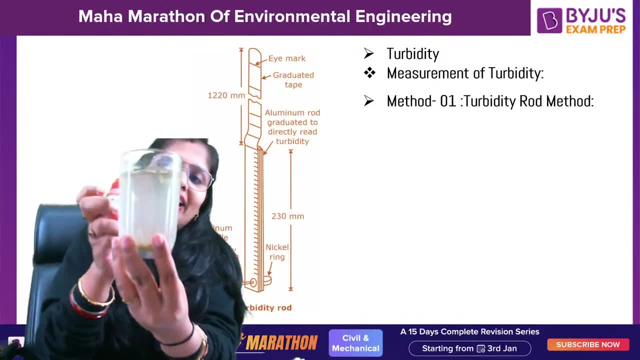 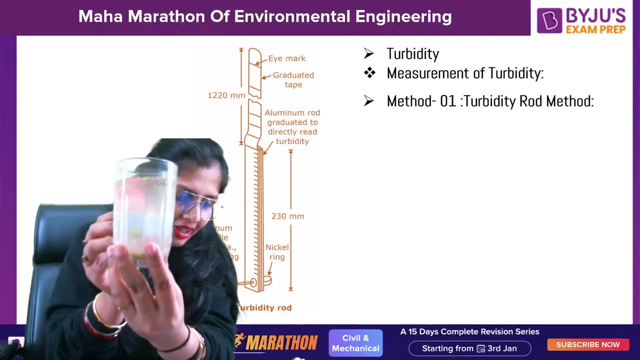 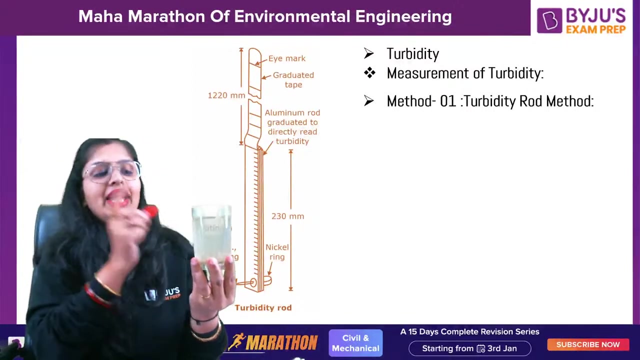 clearly Now what is happening Now? somewhat you can see, but if I am taking a sample which has suspended solids in this- and I am taking it- can you see anything? Can you see anything, Yes or no? You cannot see anything at all. This is turbidity. It is basically what is at. 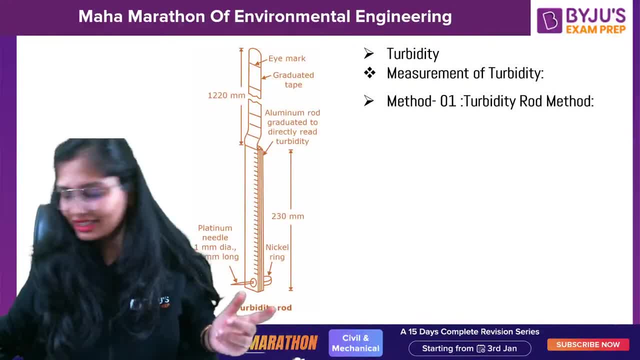 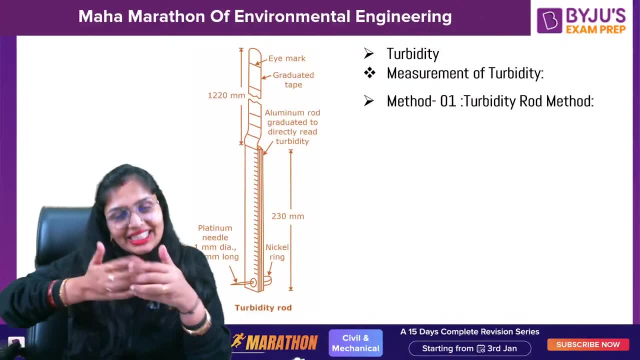 abhi nahi dikh raha. Abhi nahi dikh raha. basically, You cannot see it. So what is happening? Turbidity is the extent to which light is either scattered or reflected. So in this water at least, you were able to see. 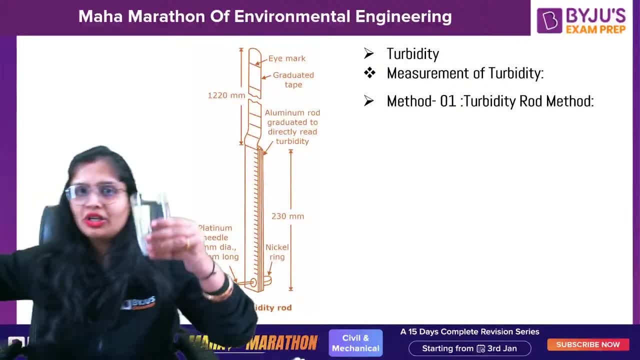 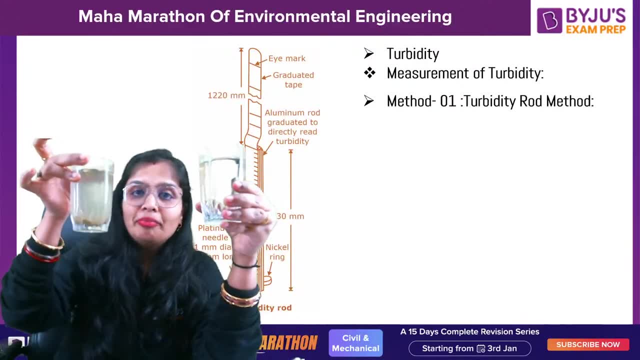 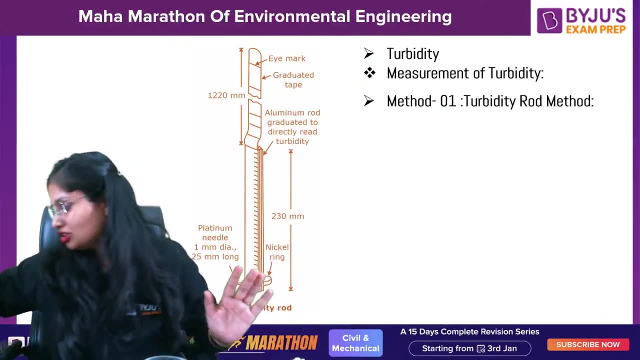 that something was written, but when I took this water, which has suspended solids in it also, then you cannot see anything. Why? Because the light was not able to reach to you. So this was turbidity, Understood with the example: Something seen before, but now nothing. 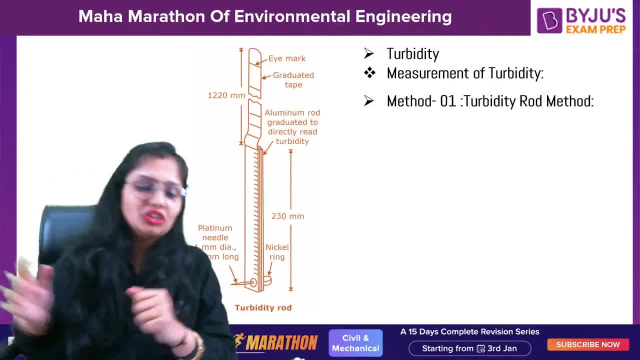 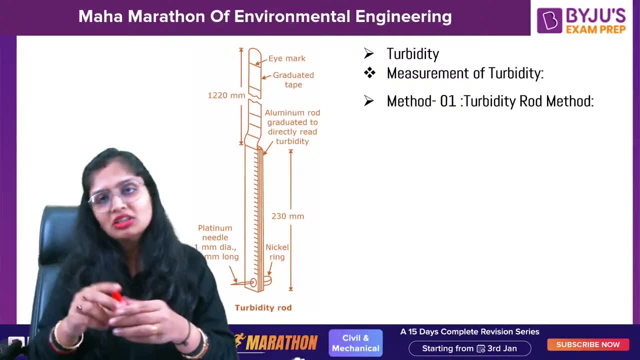 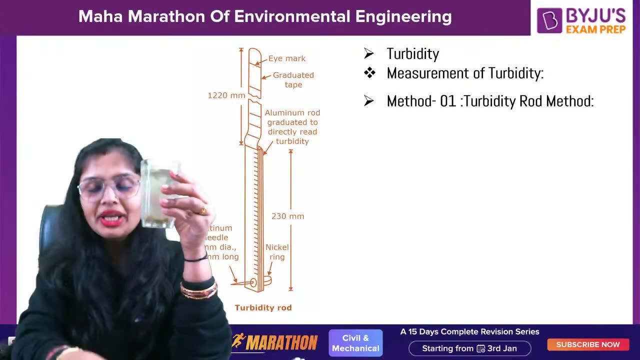 Yeah, that is what is turbidity. That is what is turbidity- Clear, Clear. I was not talking about the soil particle, That was soil particles. Turbidity was this, If you see it here, the turbidity I created Here. I created the turbidity. Okay, Anything you cannot see. 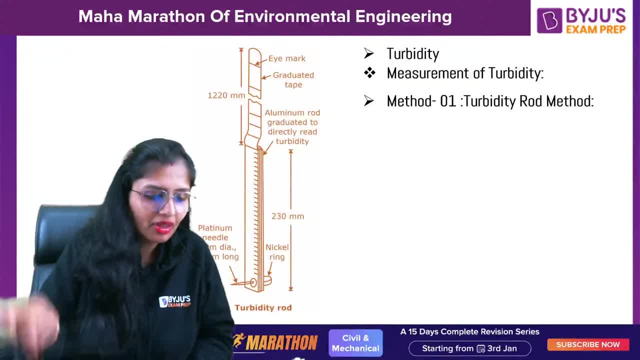 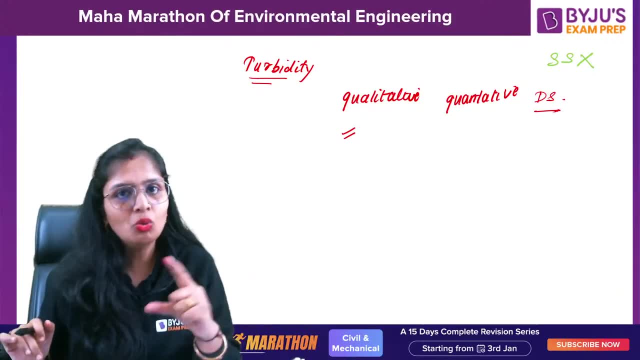 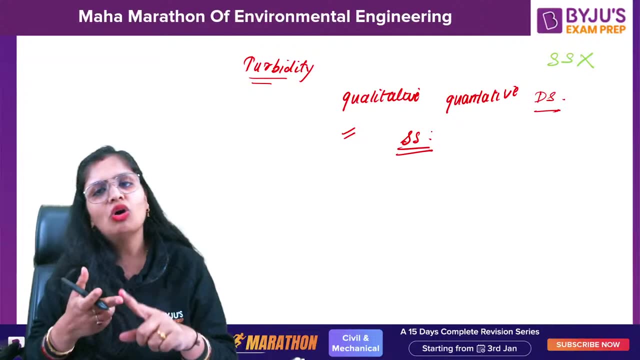 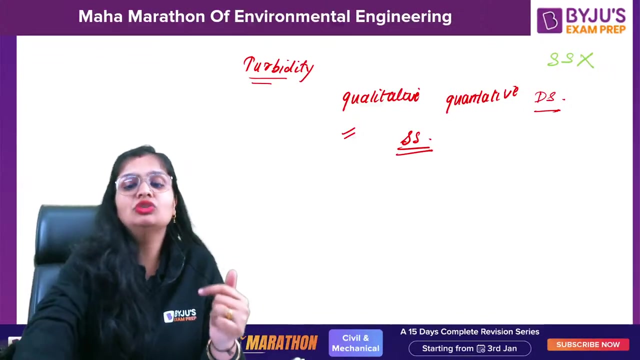 Fine, So now. now, turbidity is the extent to which light is either scattered or absorbed by the water sample. Now, turbidity, I say it is due to what It is due to suspended solids. So all the impacts, everything of suspended solids is the same, But there are few things which you need to. 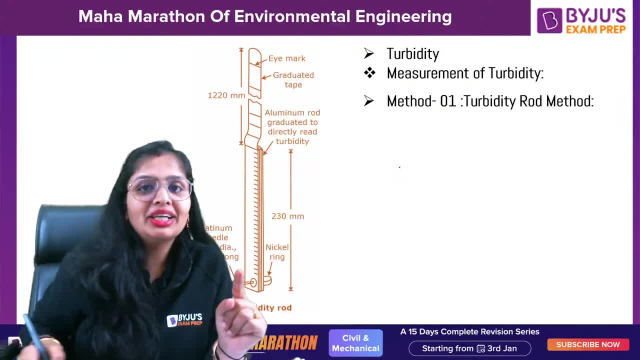 know. regarding the measurement, One thing: worst measurement is by turbidity rod. This is a field method. Again, a question for one month. Field method is only turbidity rod. Now, you can see it, here is. you can see it here is: this is a rod. Okay, There is a platinum needle. 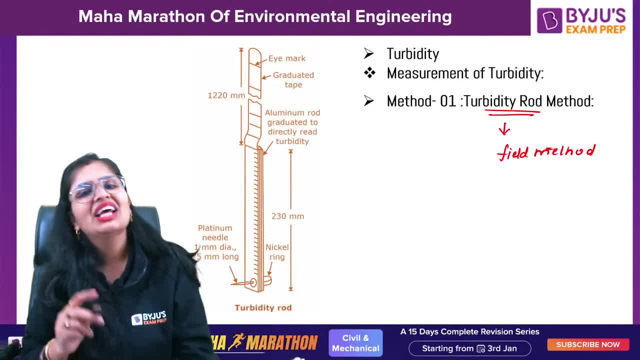 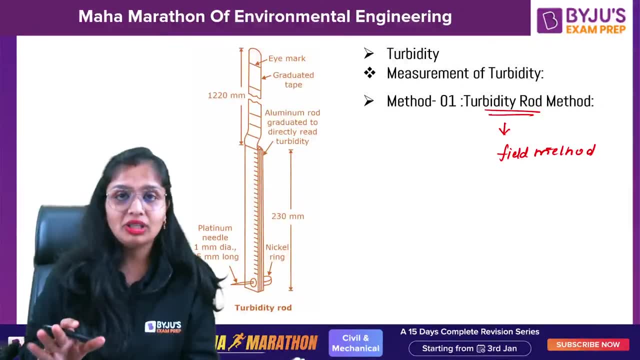 In your state level examinations. you know they ask you these basic terms: The needle which is of turbidity, rod made of platinum, aluminum, nickel, such sort of things, but not in gate Till now. if they want, they can ask you in MSQ statement wise questions. So platinum needle. 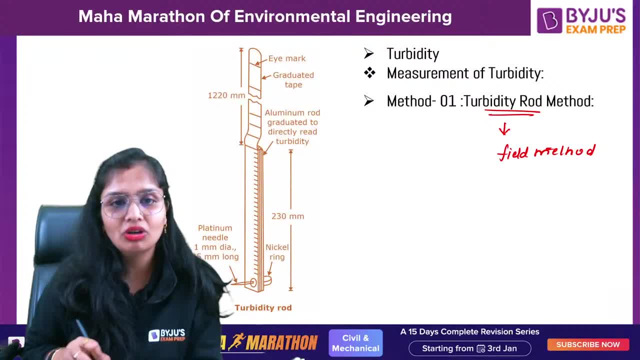 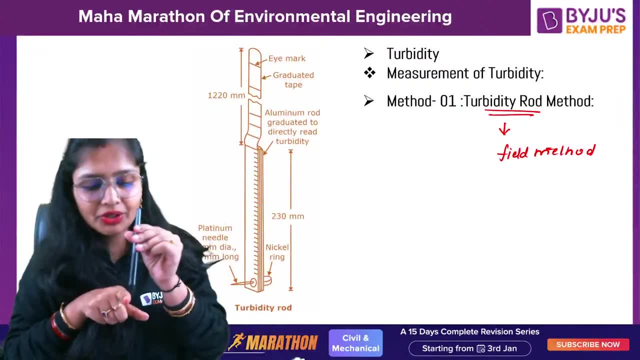 you can see it: 1 mm diode, 25. mm long and this is the nickel ring. What you will do Inside there will be a needle. You will insert it in the field water. you can see the needle. Insert it. you can see the needle, The. 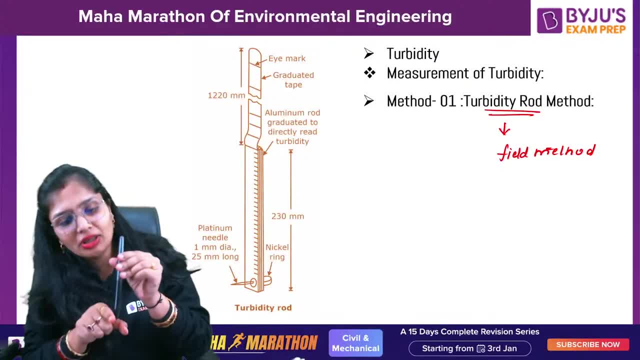 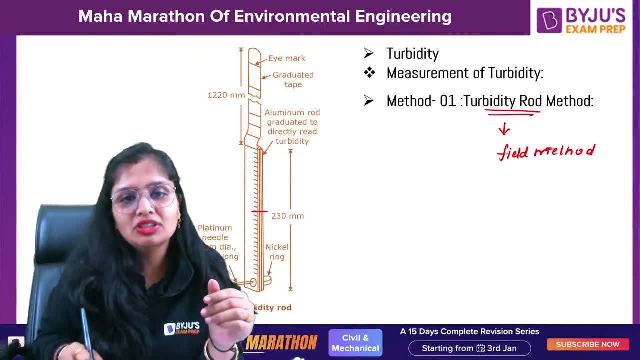 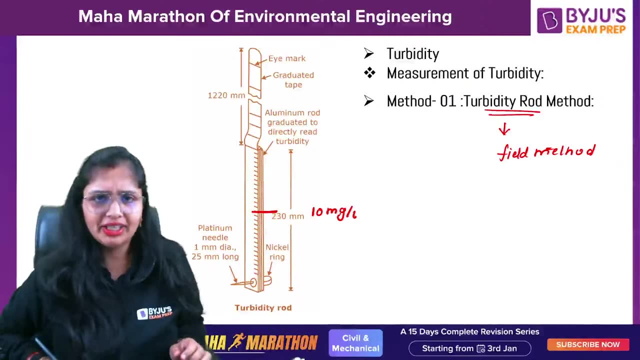 moment when you are dipping it deep and the moment when you are unable to see this needle, stop that measure. measure the reading. Okay, let us suppose this will be the reading. So here it will be 10 mg per liter. Now you will say: ma'am, we directly got the turbidity right. I will say: 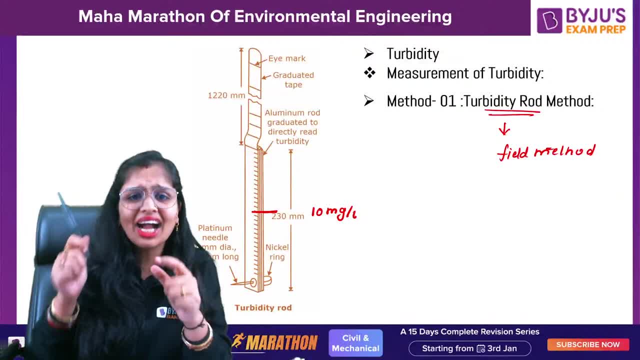 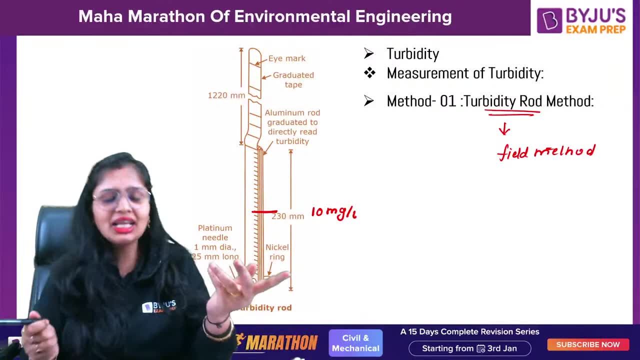 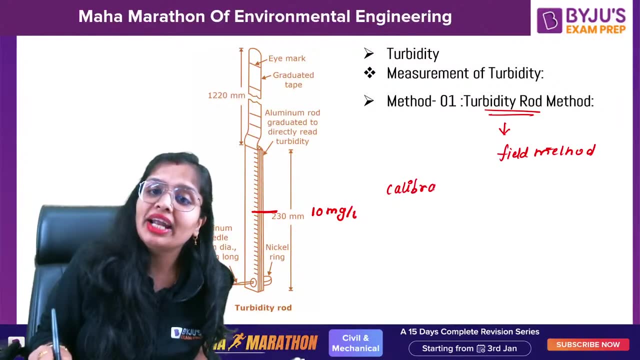 but you would say, ma'am, this rod should give me the height, but this is giving me the turbidity. How come? Means any magic, is there or what? So what is happening is? what is happening is there is a calibration done. Calibration means when you relate to unknown parameters. 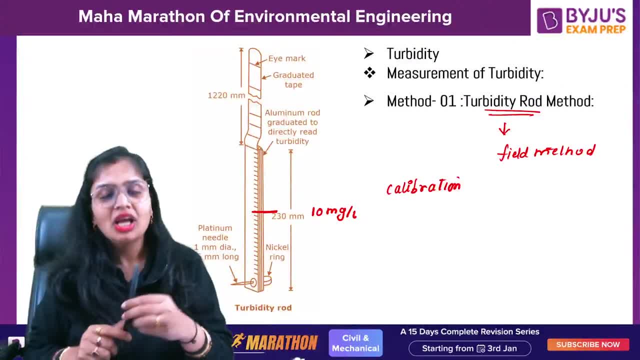 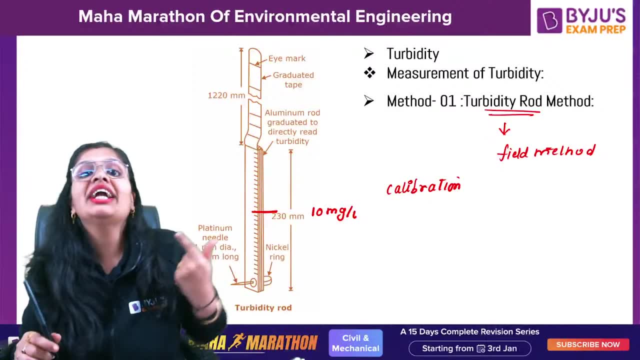 I measured the height but I got the turbidity. So, ma'am, how come you did this calibration? Initially, this was a simple rod. What I did, I myself turbidity and inserted the rod And the moment I saw: okay, for this turbidity, this one will be. 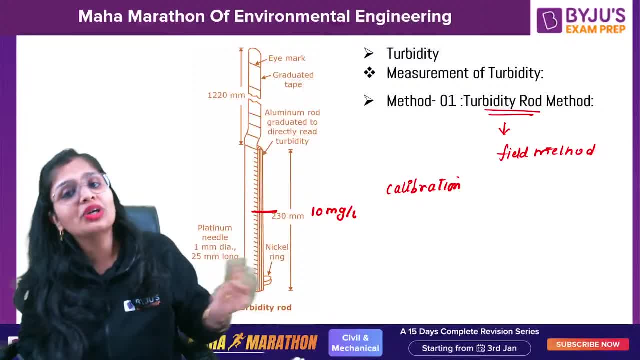 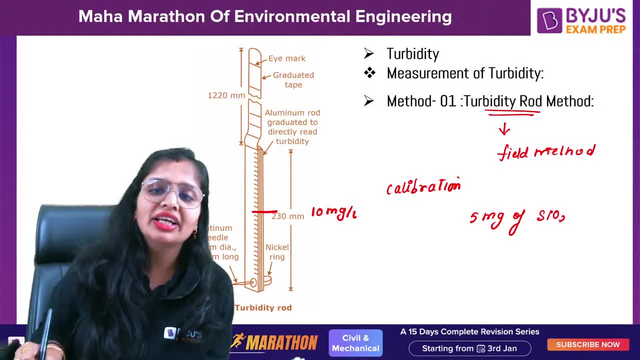 the reading for this turbidity? Second question, ma'am, how you created the turbidity? Let us suppose if I add 5 mg of silica in the form of silica dioxide in one liter of pure water or distilled water, I call it as 5-STU. STU stands for silica turbidity unit, So in this manner: 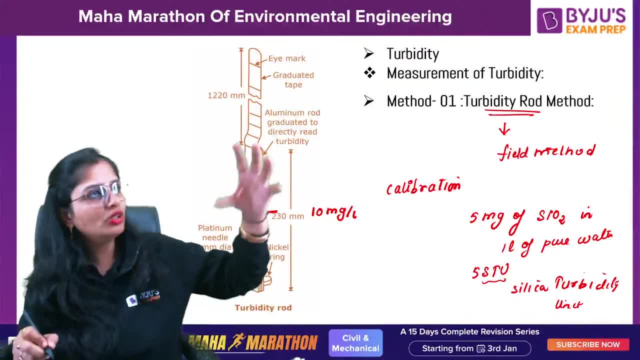 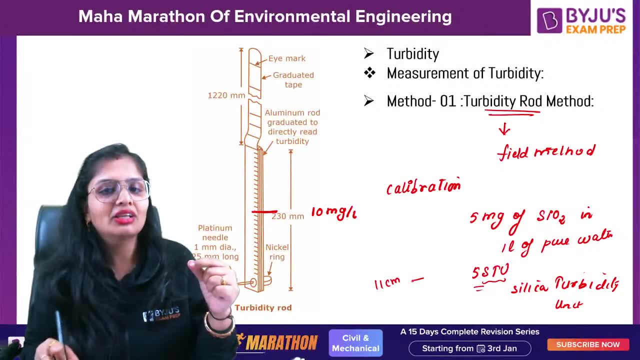 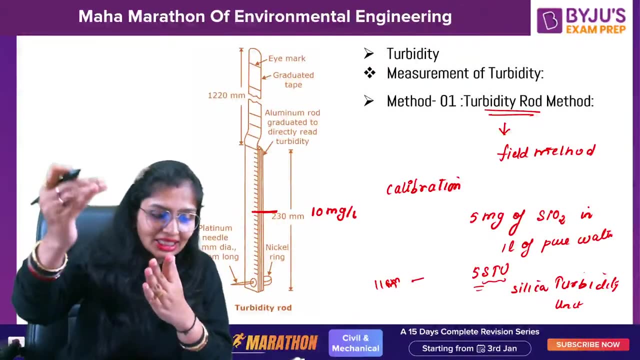 since right now also, you can see, i created the turbidity, so i put silica. i made the turbidity, let's suppose, for 5 tcu, 5 mg per liter. the depth comes out to be 11 centimeter. so when 11 mm, so when 11 mm will be the depth, the turbidity will be 5 mg per liter. so in this manner, what i did is: 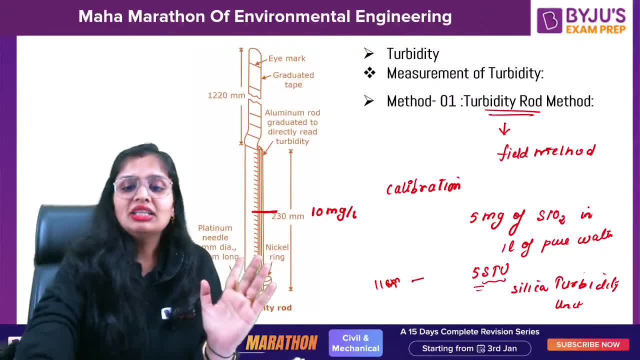 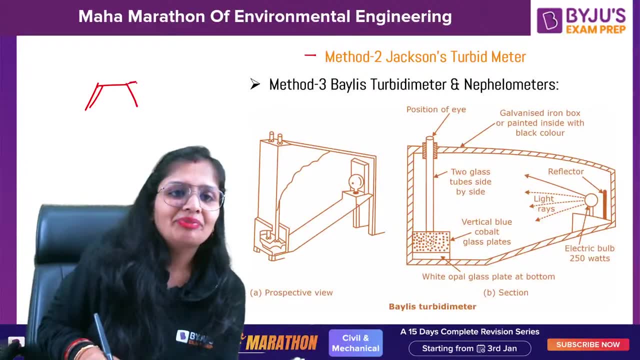 i created the turbidity similar, similar you can do by. there is another method, that is jackson's turbidity method. simple, there will be. same method is there. there will be a measuring glass will be there and all, and there will be a candle flame again. you will pour the water. you can see the 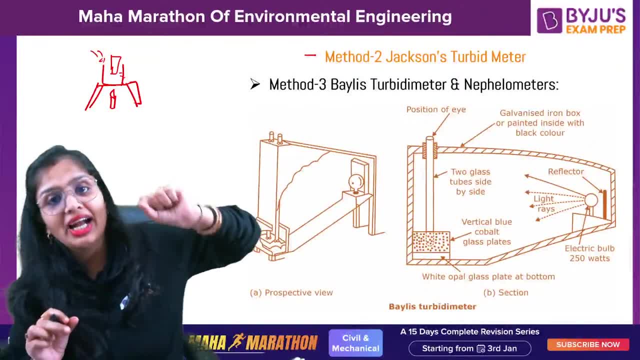 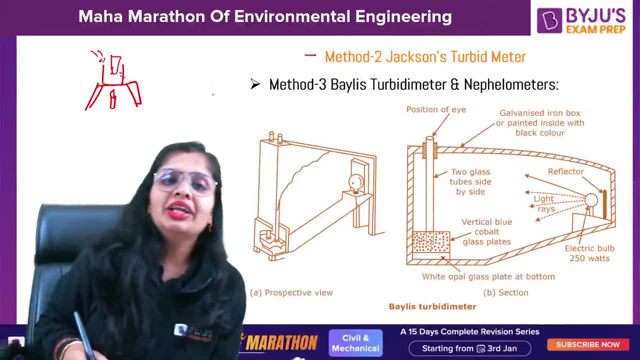 flame of the candle. you will pour the water. you will see the flame of the candle. the moment the flame of the candle you cannot see is. you will note the reading here. also, you can get the unit as jtu jackson's turbidity unit and stu silica turbidity. 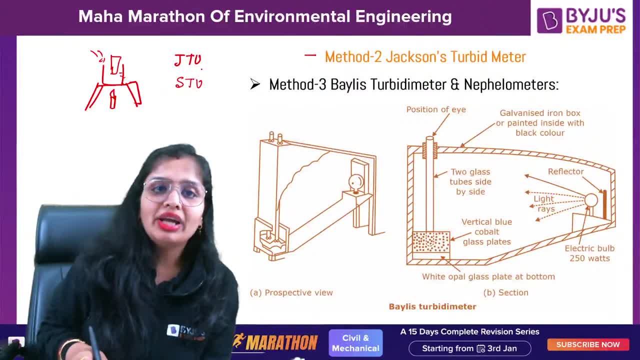 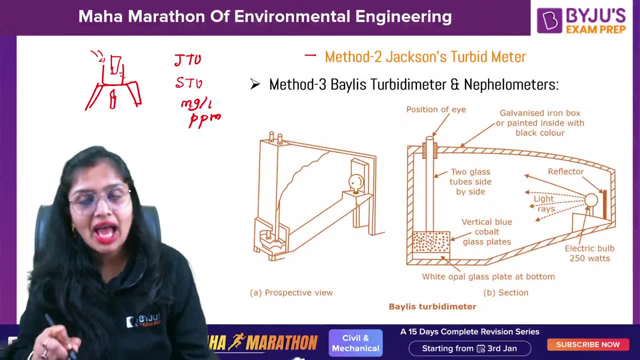 you can get the unit as jtu jackson's turbidity unit and stu silica turbidity unit. if they have written in the question stu jtu mg per liter, ppm and they'll ask you which of the following is correct, appropriate, you will write stu technically for writing purpose. 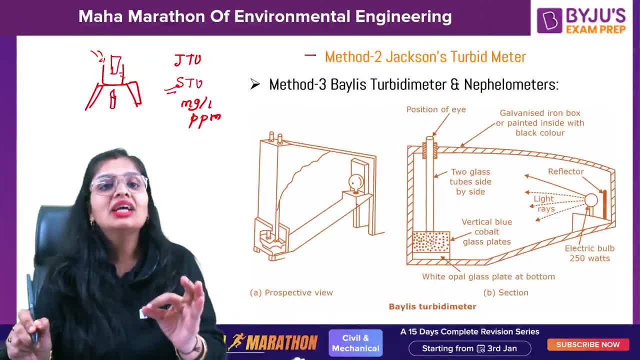 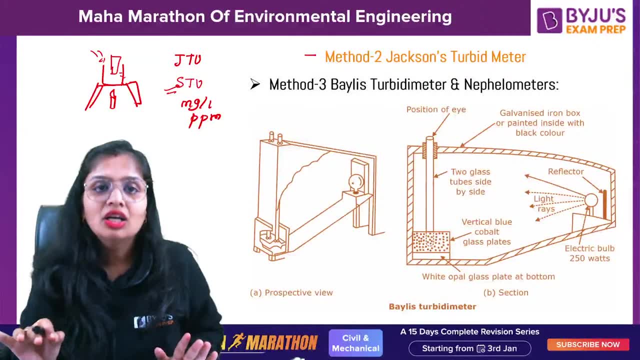 everything means same. okay, but we take stu. why? because the principle involved is of silica clear. moreover, we cannot. we don't use jackson's turbidity meter because it's not the same thing. we don't use jackson's turbidity meter because it's not the same thing. 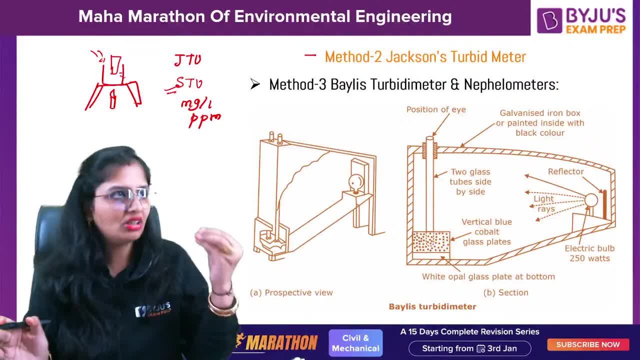 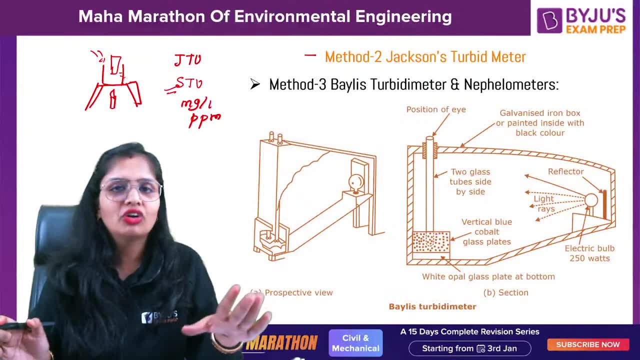 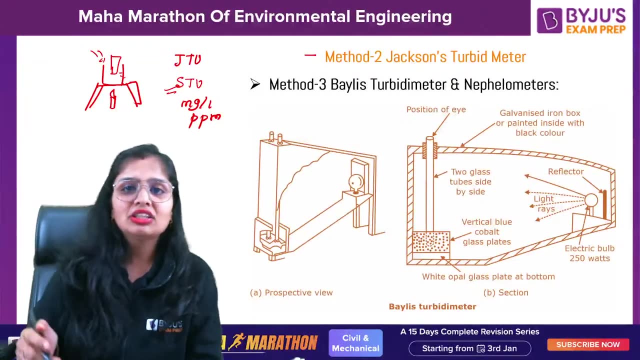 it gives turbidity more than 25 units. okay, and turbidity of about 5 units. we can receive it by naked eye only, so you can use it for large water bodies, but for drinking water we don't use jackson's turbidity meter. okay, now talking about bailey's turbidity meter. bailey's turbidity meter is based 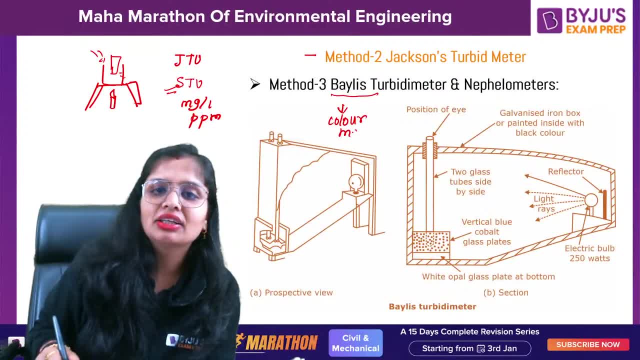 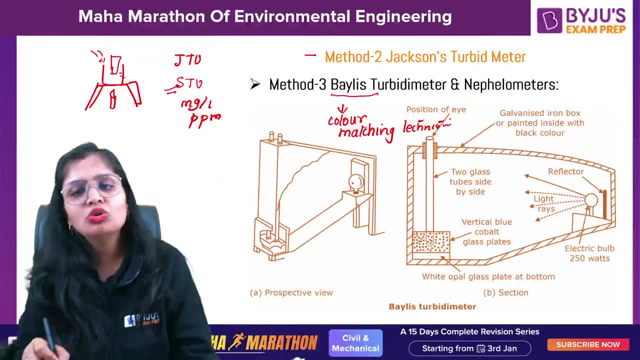 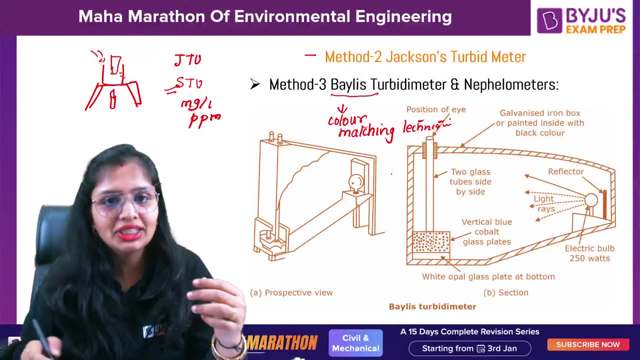 on. initially, it is based on color matching technique. color matching technique. so what do you see it here? generally, there is a blue cobalt glass plate which is attached first, and there is a two test tubes- okay, two test tubes- which you can see it here, you can see it in this prospective view also. so what you will see? what you will see. 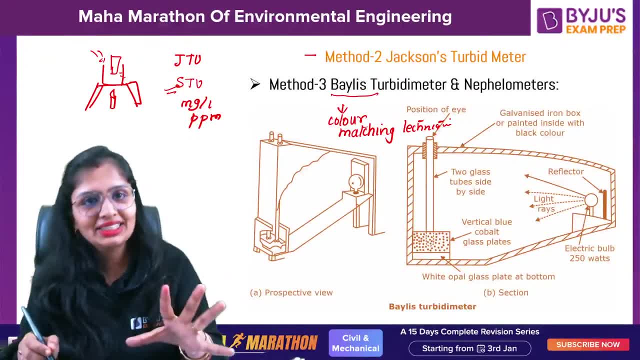 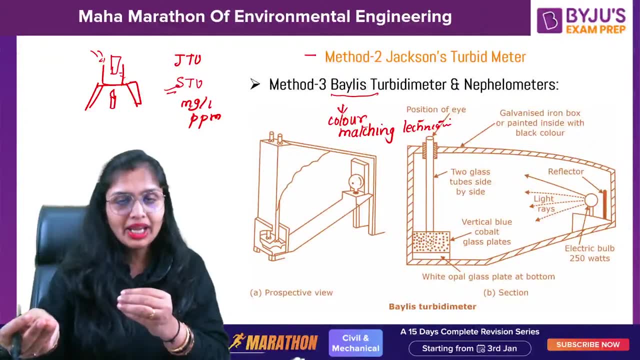 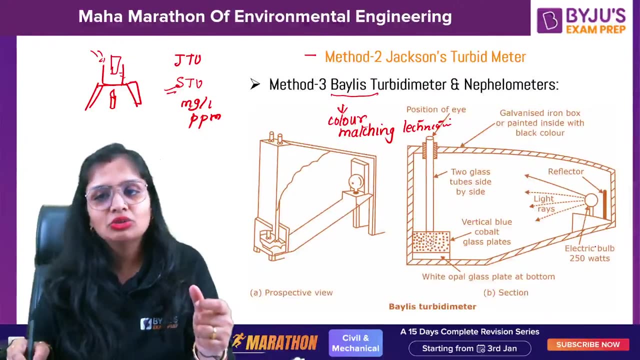 that basically, basically, there will be a test sample and there will be a standard sample. standard sample is that sample which you have prepared, okay, and test sample is that sample where you need to find turbidity. so what you did, what you opened, uh, basically switched on the electric bulb. there is blue cobalt glass plate. the light will reflect and it will reach to your 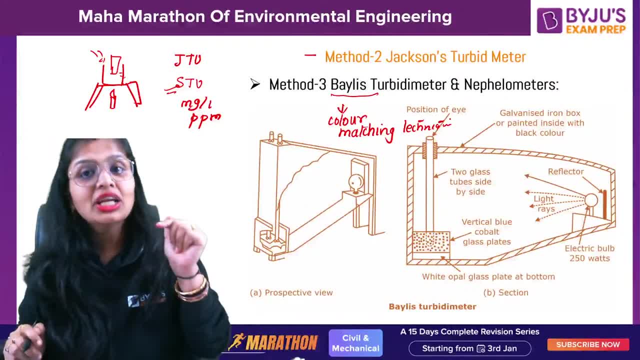 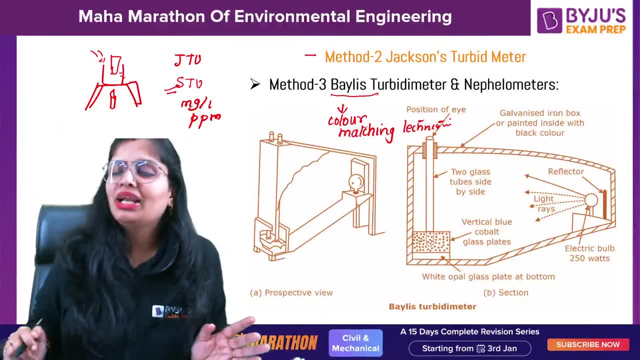 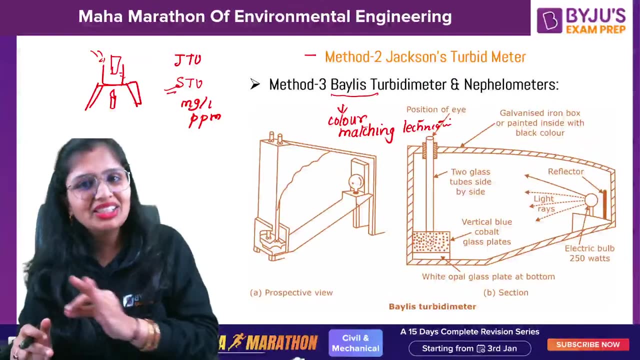 eyes. if you see in both the samples you get the same colors, same intensity of light scattered. you will say that turbidity is same of test sample as that of standard sample. if it is not what you have to do, you have to change the standard sample. but this method we generally don't. 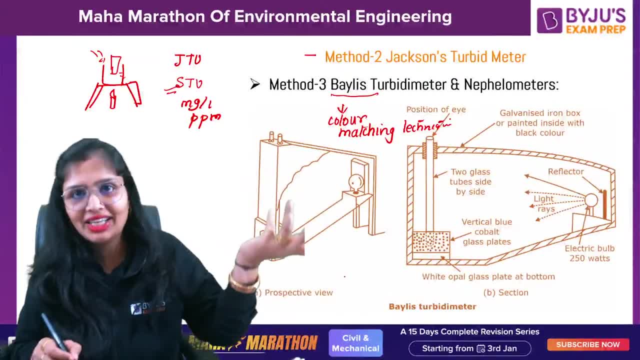 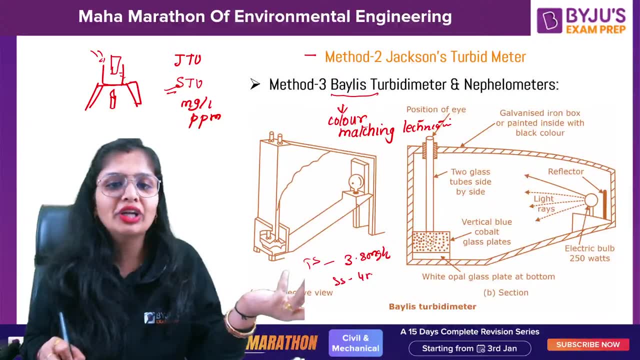 use it because you don't have that super eyes. the wish like: if it is 3.8 mdms per liter of the test sample and standard sample, it is 4 mg per liter for you. will you be able to detect it? no, for you it comes out to be the same. or if the test sample, it is 4.2 mg per liter also. 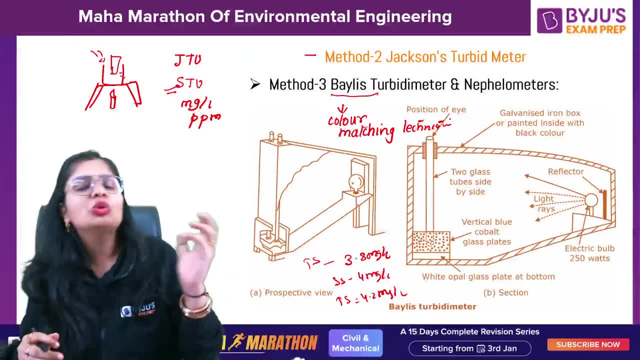 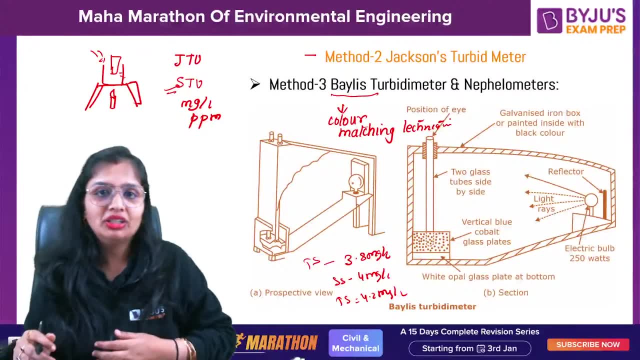 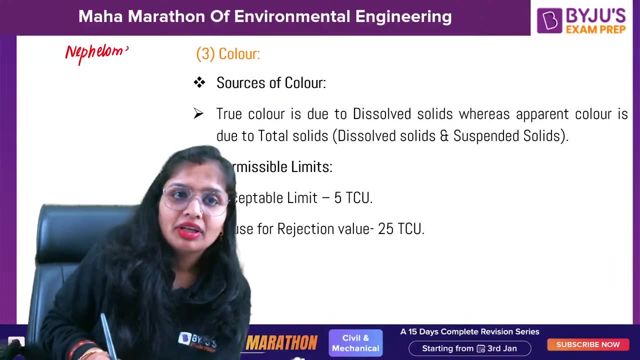 then also you will say that it is 4 mg per liter. so what happens you cannot predict accurately. so that's why we go for nephelometers, and nephelometers are based on current matching technique. nephelometers are based on- i'll write it here, spaces then, of course, 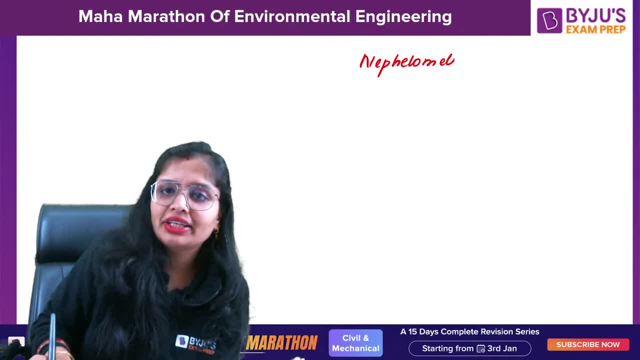 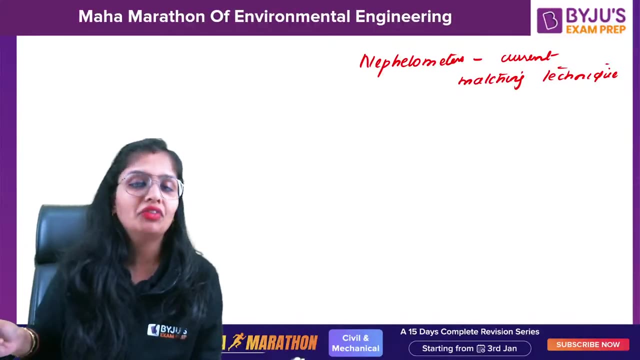 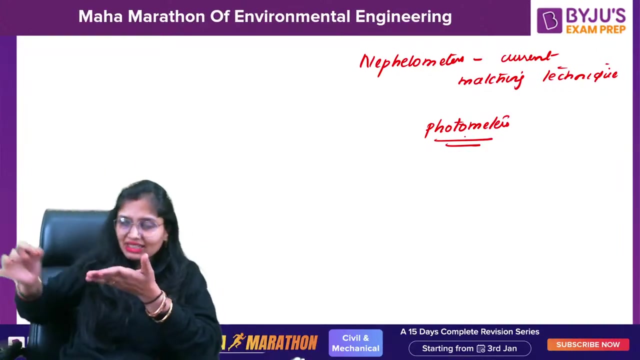 nephelometers are based on current matching technique. now, let me tell you this is very important. first of all, nowadays, if you go it in the, in the experiments and all you will see nephelometers, only photometers. photometers is a semiconductor device and as soon as light is incident on this photometer, it produces current 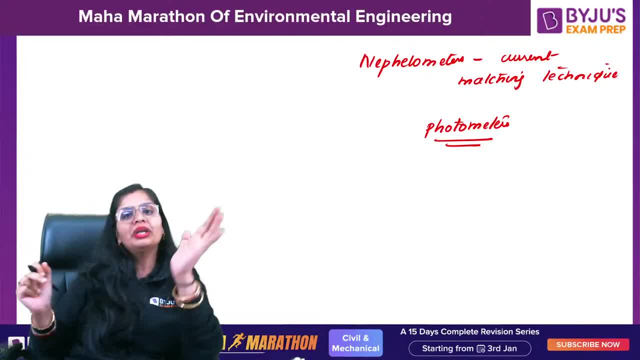 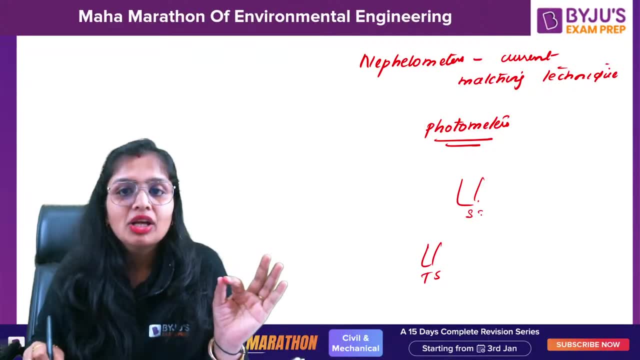 so as soon as the light is incident on it, photometers will produce the current. so now what happens? there is a test sample and there is a standard sample. so what you do? when bailey's turbidity meter was there, you place the photometer behind it and this bulb was there. 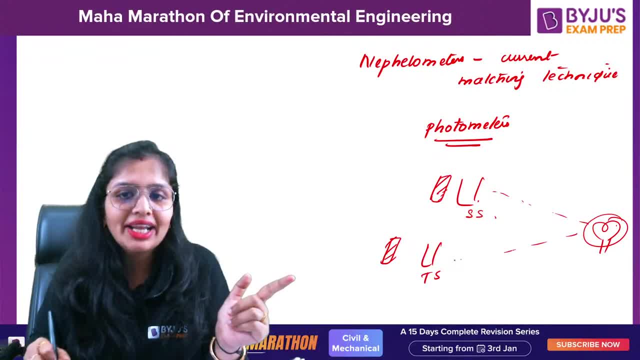 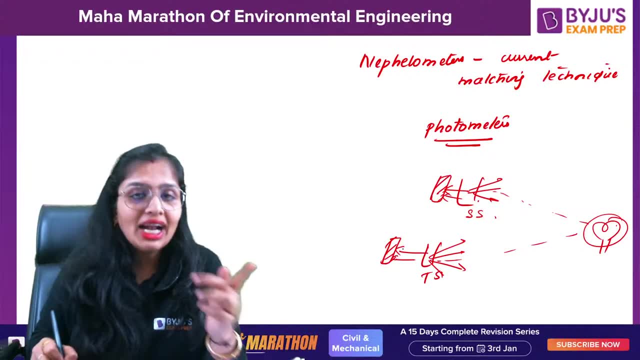 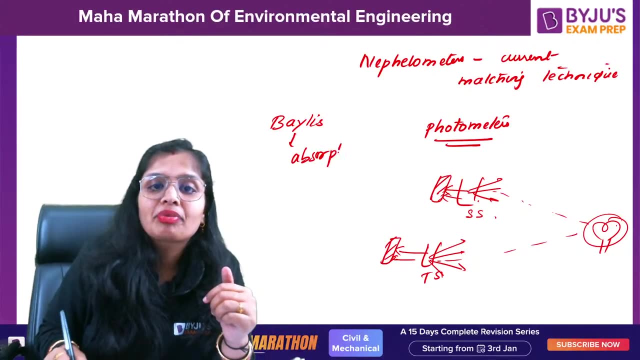 so what used to be there? when you scatter, when you just this light comes, a part of it used to get scattered and a part of part of it used to get absorbed. okay. so that's why, again a question asked. bailey's turbidity meter is based on absorption principle. similarly, nephelometers- again photometers- was there. 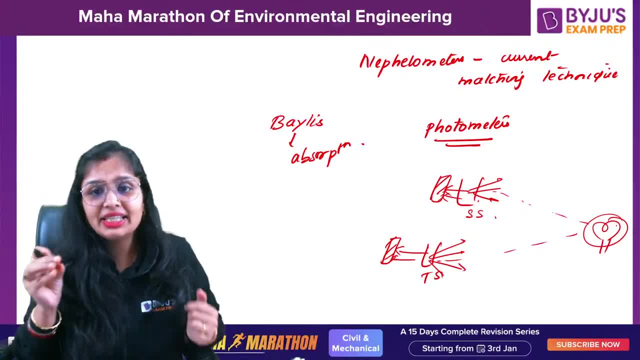 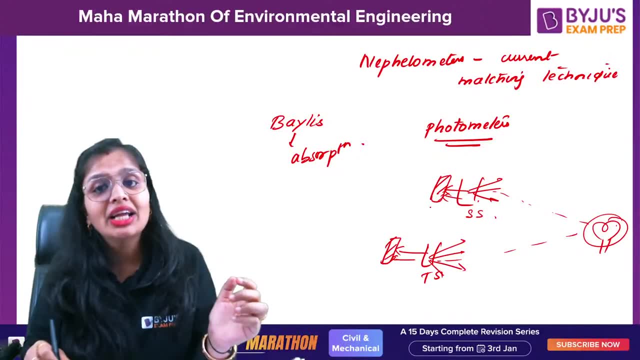 but, ma'am, how you measured the turbidity? see when the light got striked in this photometer, current was produced. if the current in standard sample and test sample is same, then whatsoever is the turbidity of standard sample. that will be the turbidity of test sample. 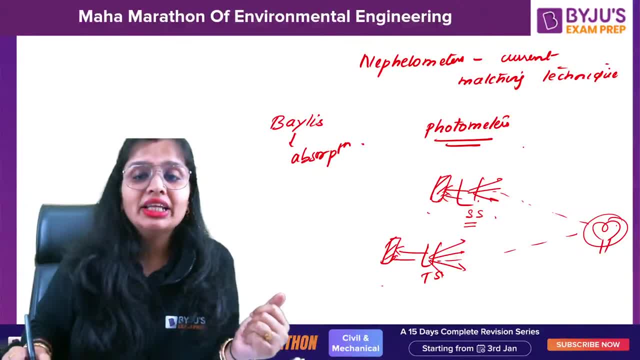 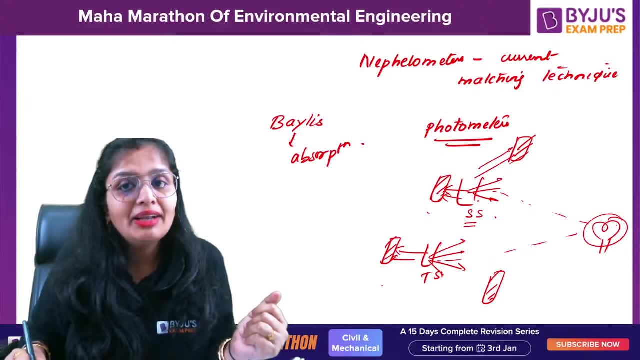 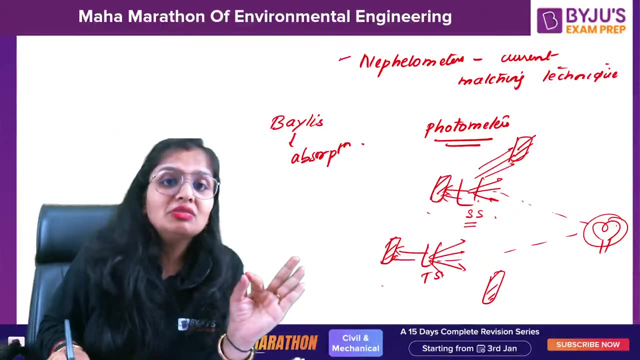 okay. secondly, if it was the case of nephelometers, you place them at 90 degrees. so what does nephelometers do? it measures the current which is incident on it at 90 degrees. so nephelometers measure these nephelometers do they measure the current which is incident on it at 90 degrees? 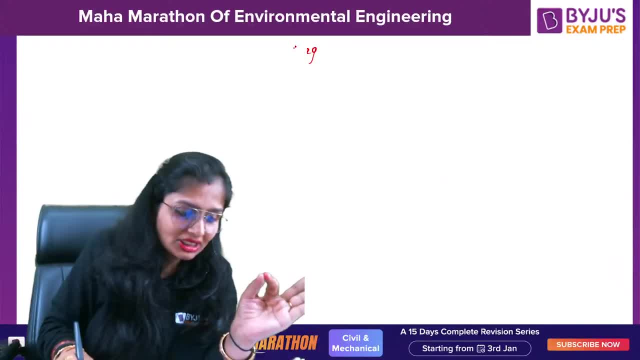 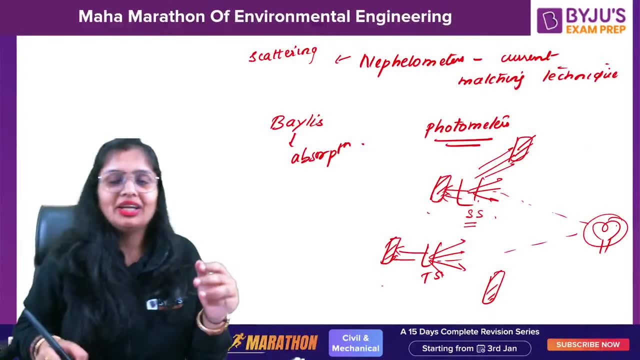 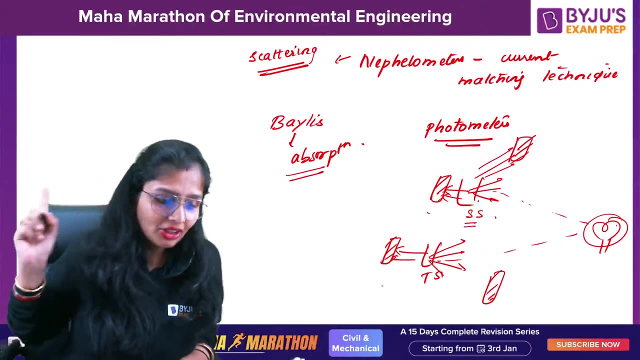 the scattered light. so nephelometers is based on scattering principle. oh my god, it has gone over. something is pressed by my. it is based on scattering principle and bailey's turbidity is based on absorption principle. now, one thing asked in your gait: examination asked in your gait. 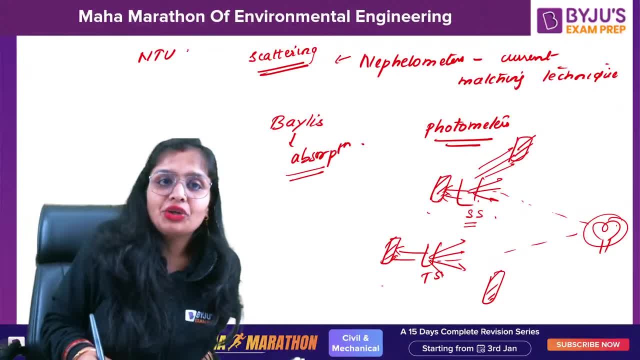 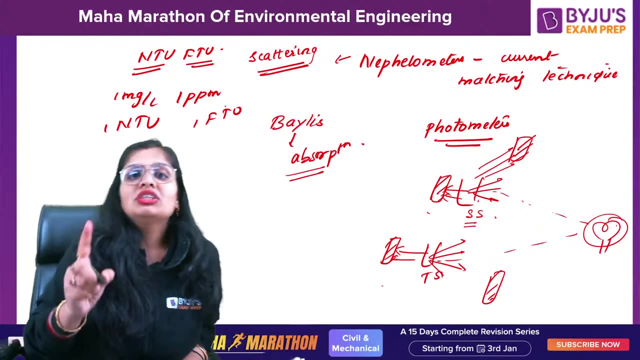 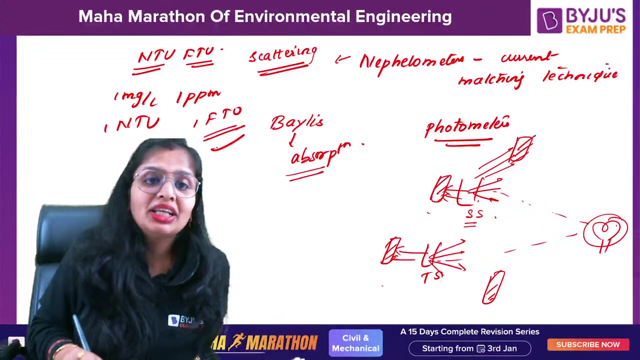 examination that is NTU and FTU. FTU's NTU means nephelometer turbidity unit, FTU means formazine turbidity unit. if they give you one mg per liter, one ppm, one NTU, one FTU- this was asked in gait, asked in your polytechnic lecturer, AE, ESE- every examination they have asked you, FTU will be the. 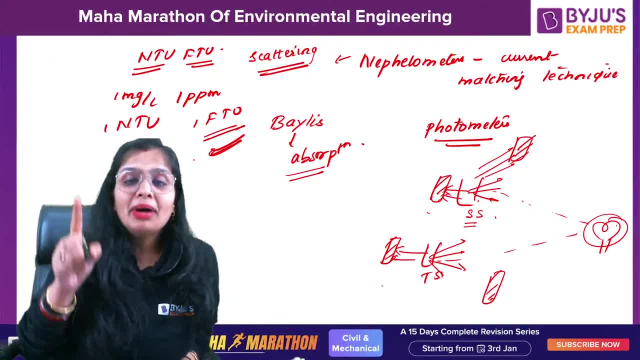 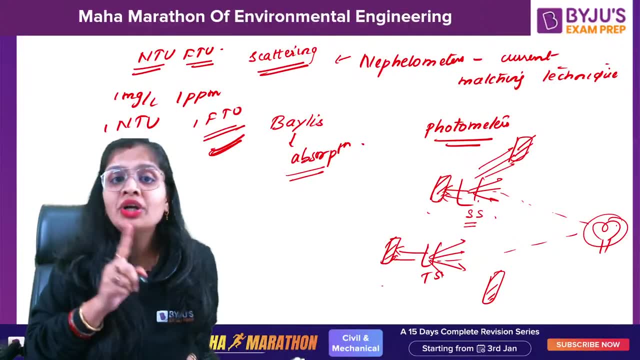 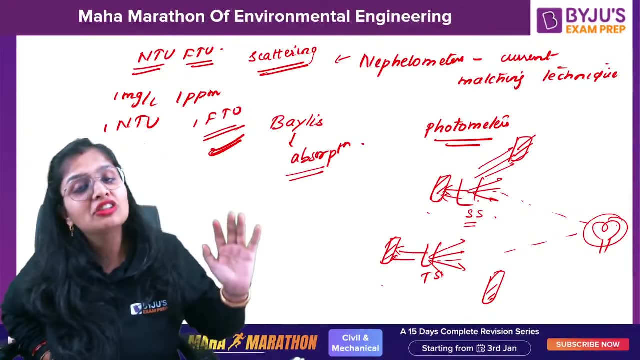 correct answer, ma'am, but all are equal. yes, beta, but when you basically make standard sample, in the case of nephelometers, you don't use silica dioxide, you use formazine, ma'am. why we used formazine? because it gives better results as compared to silica dioxide. so 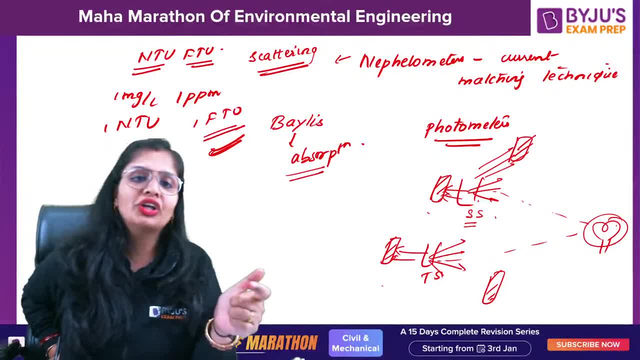 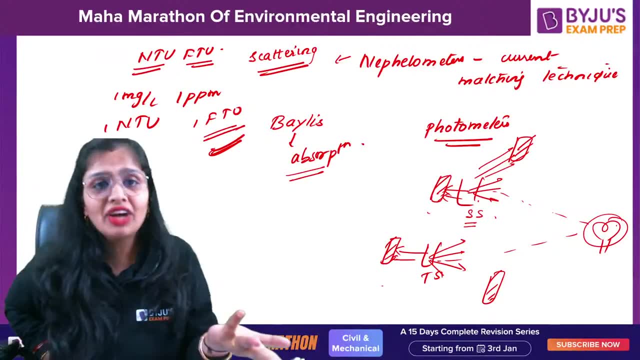 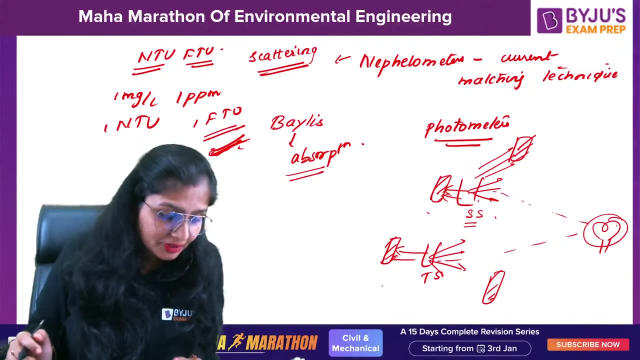 when you add one milligram of formazine in one liter of water, you will get one FTU. if you add five milligram of formazine in one liter of pure water, you will get five FTU. so FTU will be. FTU will be the correct answer. nephelometers: Prashant what I did for the case of nephelometers: I placed. 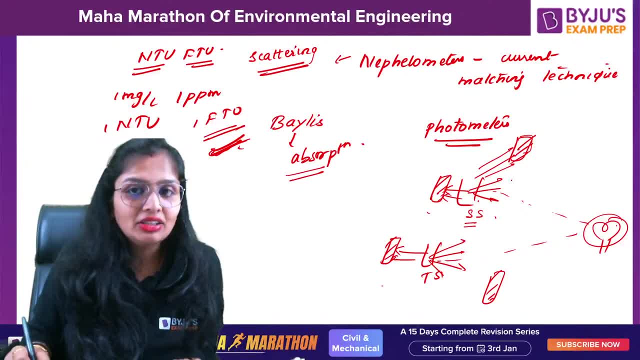 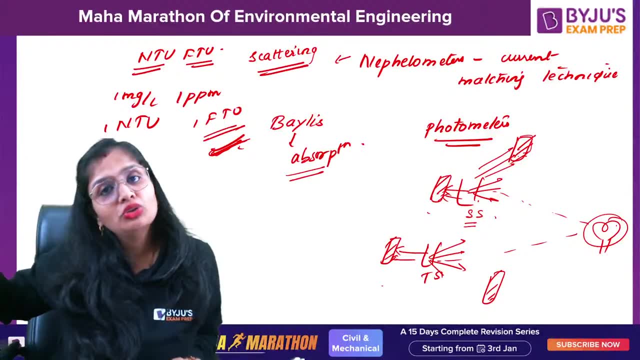 that 90 degree. so when the light came it scattered. okay, and this scattered light was incident on the photometers. so photometers current was produced due to the scattered light. so if the current in standard sample and test sample is the same, you will say that standard sample and test sample 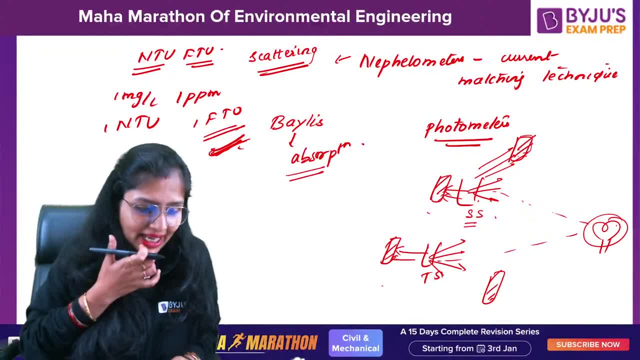 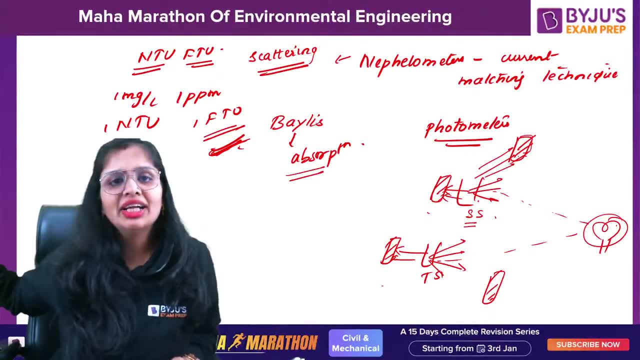 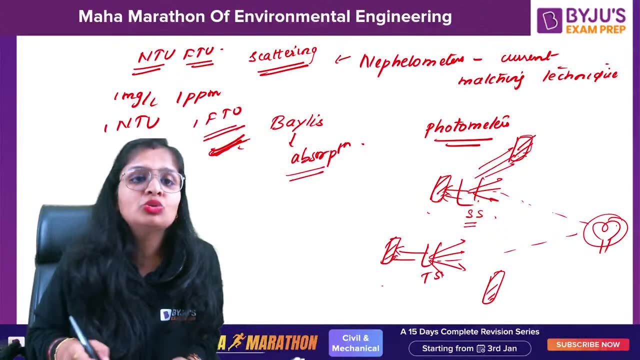 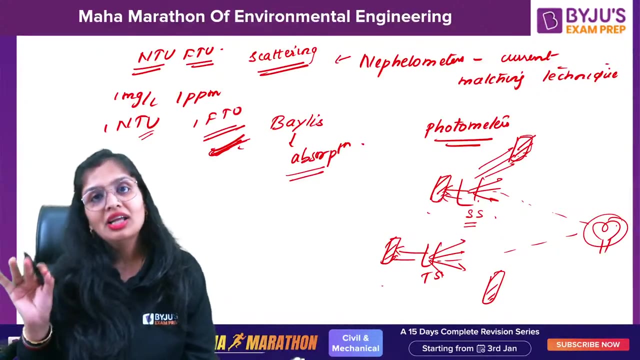 both have the same turbidity. okay, clear: STU and FTU: both are given STU. no, no, STU is different if you want to compare MJ. this was the question which was asked in gate examination. maximum students wrote NTU. why? because, as per the codal provisions, they have given NTU as the limits. but 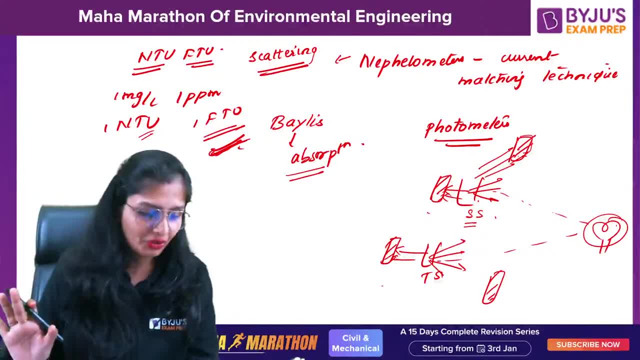 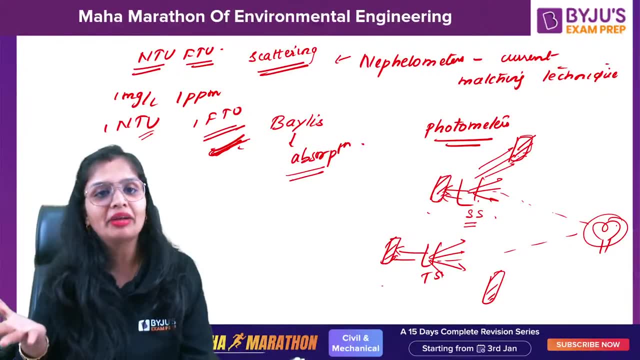 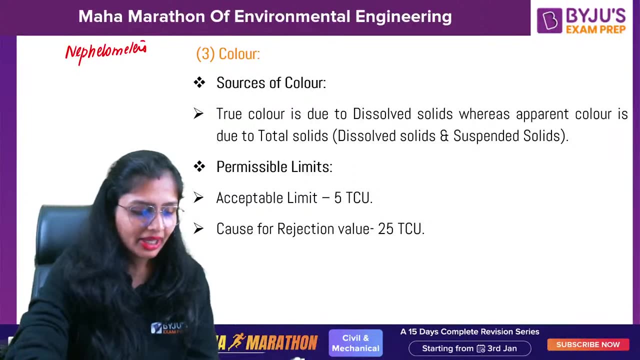 if they ask you the appropriate one, you will write FTU. okay, if STU and FTU, both are given, they can't give it. why? because for comparison you need a common parameter, right? okay, this was any doubt still here. any doubts, Prashant clear, any doubts anybody? so nephelometers, right now we use 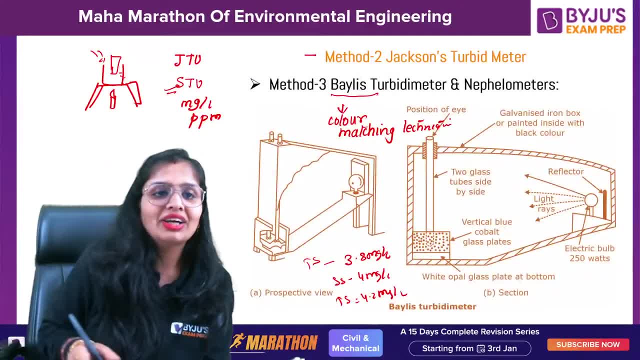 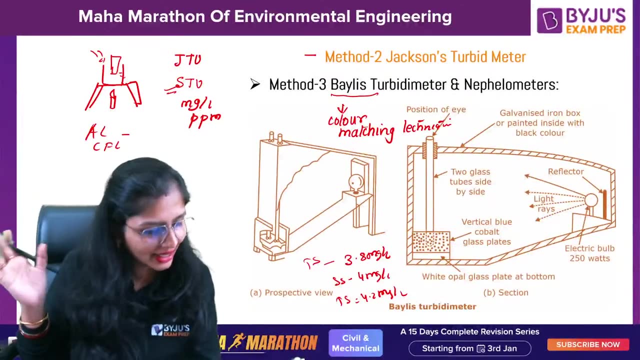 it. and if you talk about, two limits are also there in this. one is acceptable limit, another one is cause for rejection limit. why only 90 degrees? because it has been like this only for nephelometers. you can arrange it at any other degree also, which you want. yes, correct, Vishal, correct, okay, what? 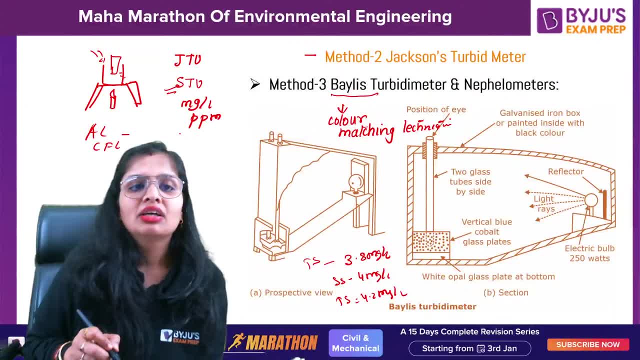 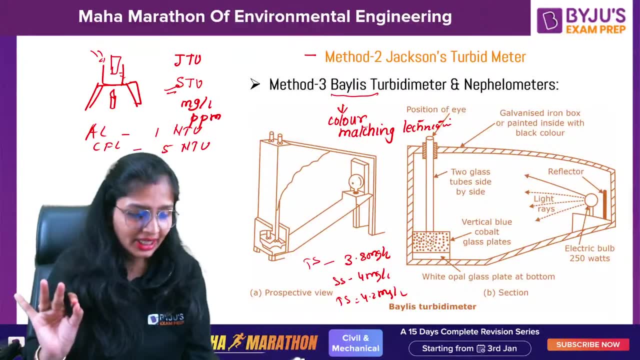 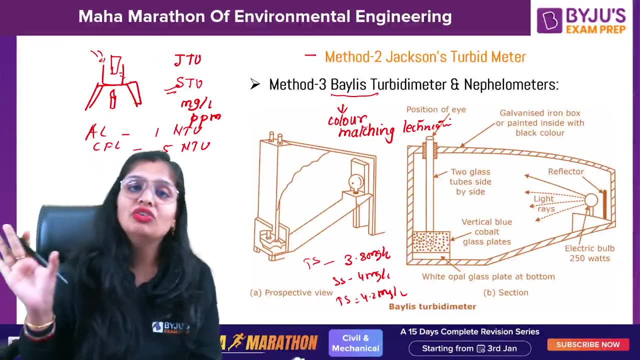 is the acceptable limit and cause for rejection limit? just tell me: 1 NTU, 5 NTU, is it remember? if it cause for rejection limit when there is no alternate source available, then we go for cause for rejection limit and it doesn't mean it should be 5 NTU. this is the wrong concept asked in. 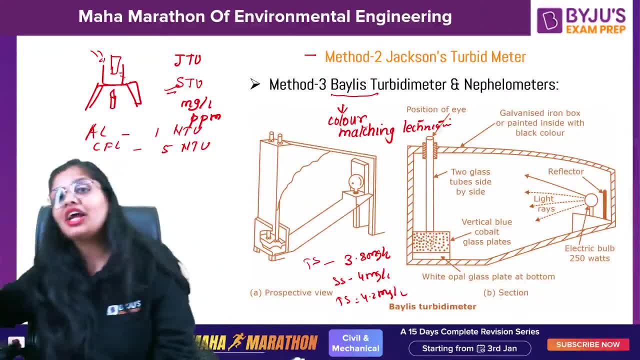 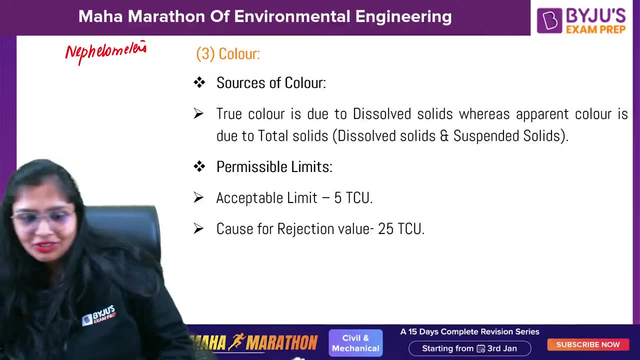 interview questions. also, it means up to 5 NTU. it can be 2, it can be 3, it can be 4, up to 5 NTU. it is talking okay, so this you should know. okay, now talking about color, color, okay, fine, so let's make. 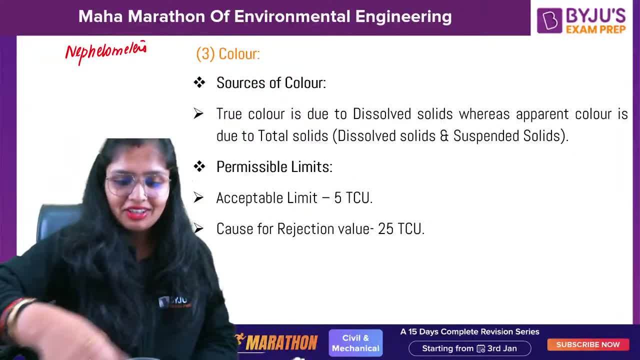 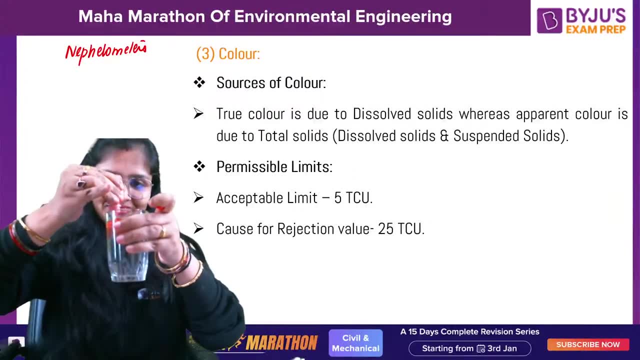 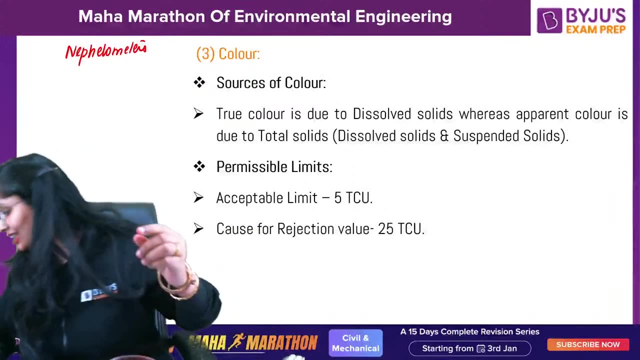 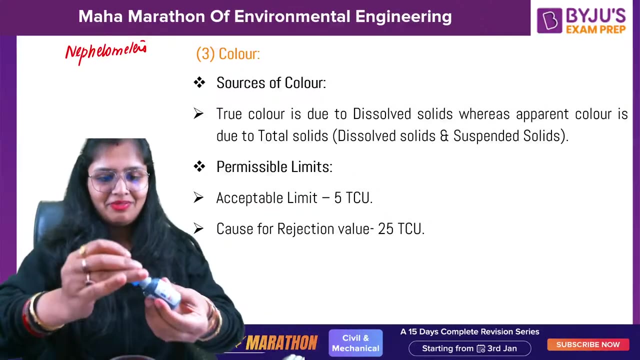 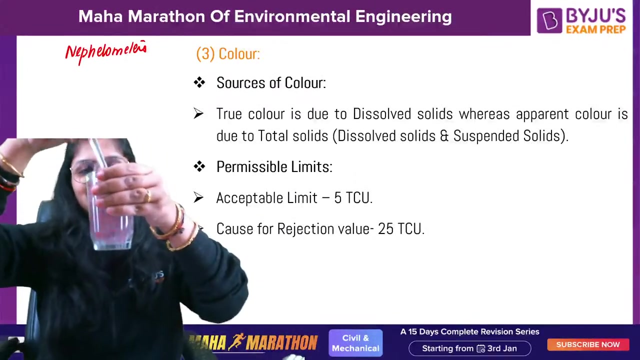 it exciting. pure water. you can see it. come on, guys. so don't see what I'm adding, don't see, close your let's make it colorful in exam. F2 is more preferable. yes, it is more preferable, because the principal involved in this is it has more density out. so, guys, this is standard. roo abzak. 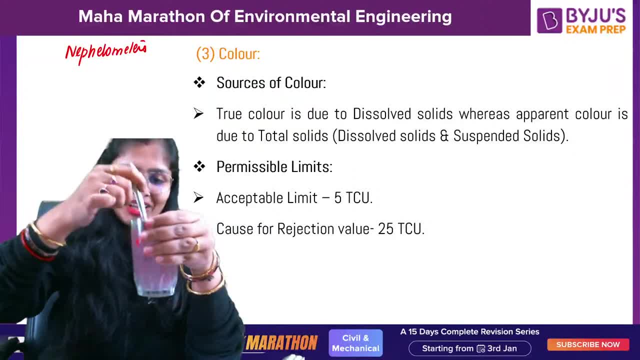 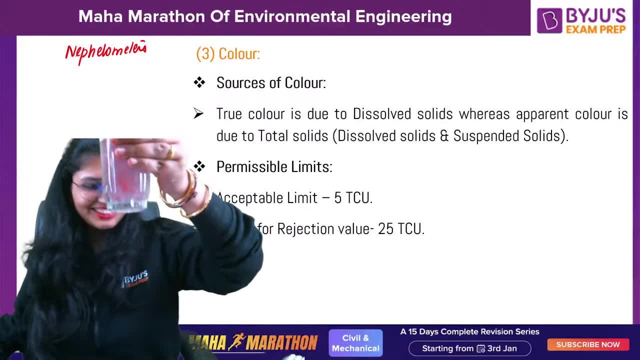 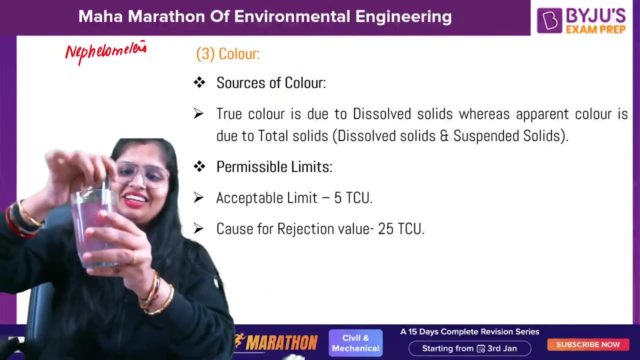 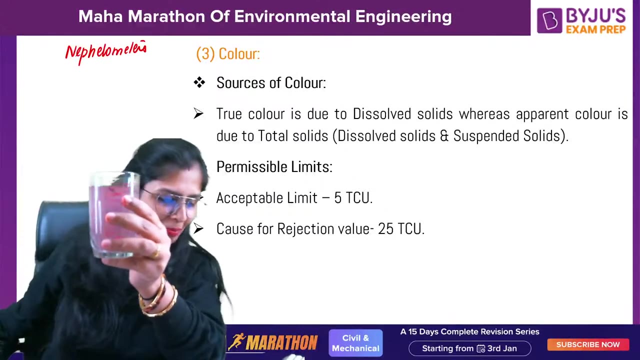 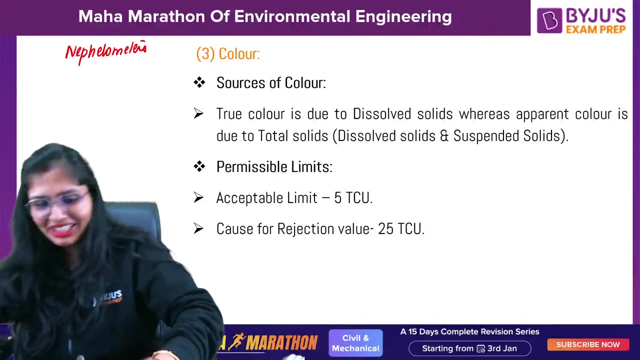 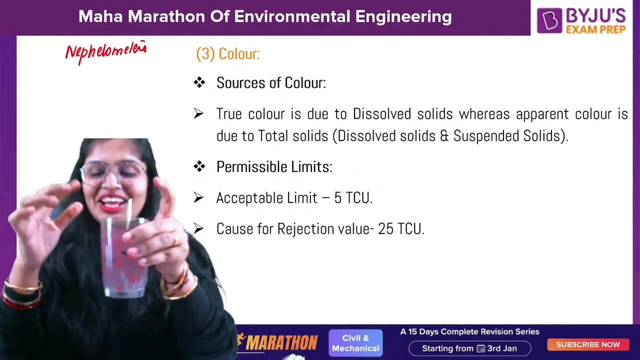 with fruit pulp and all in it. will you drink it? don't see what I have added: colorful. come on, Diksha, everybody. Girish Prashant, mango pulp and all is also there. strawberry pulp, strawberry plant. this is my equipments, which I have added. no right why if it had been yeah, mix, yeah, this is my secret recipe. Arun suspended particles. that. 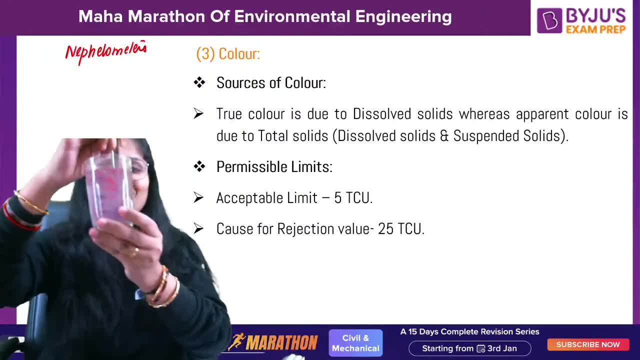 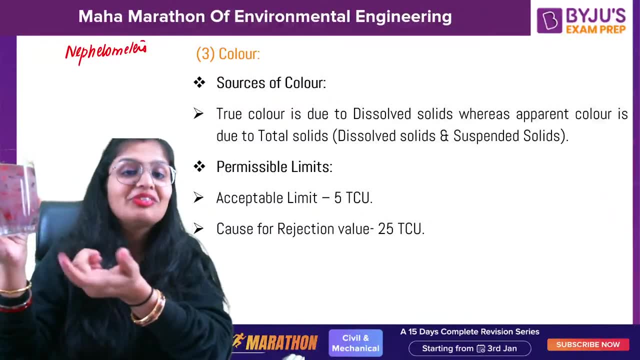 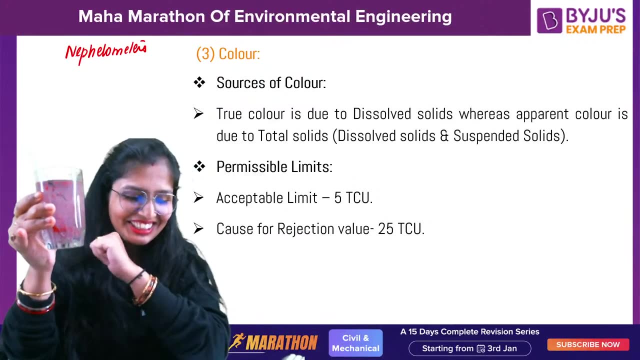 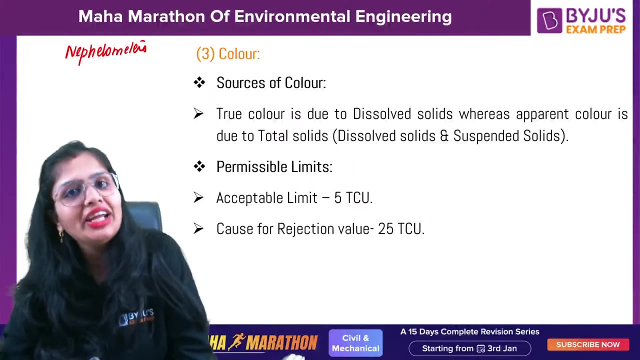 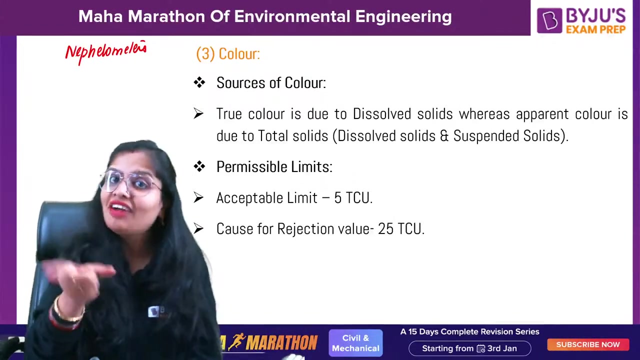 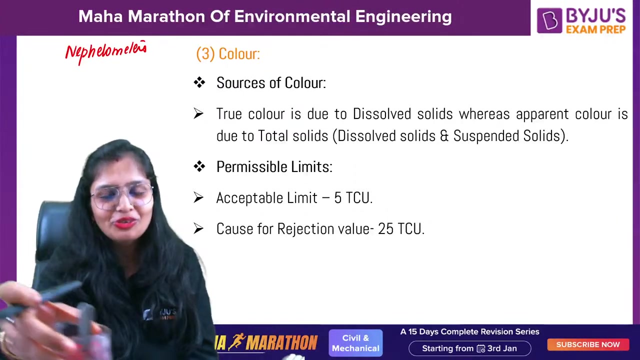 is pulp like this. that is pulp, fruit pulp. secret recipe. will you eat, drink? basically no ink juice. excuse me, so mature. all this work around the Artist's 450 Ultra rupees 2009: 28, 22, 22, 23, 44, 45, 6. 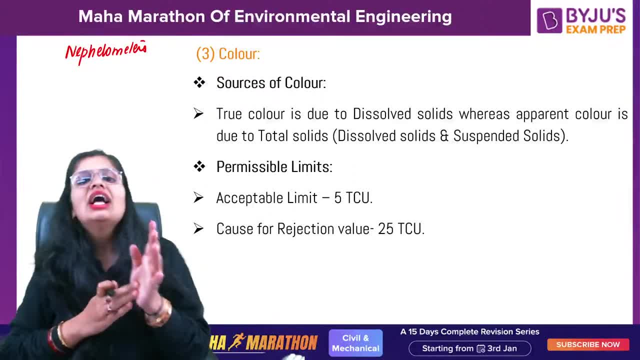 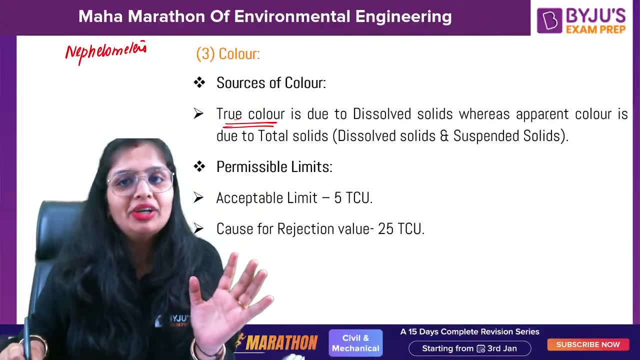 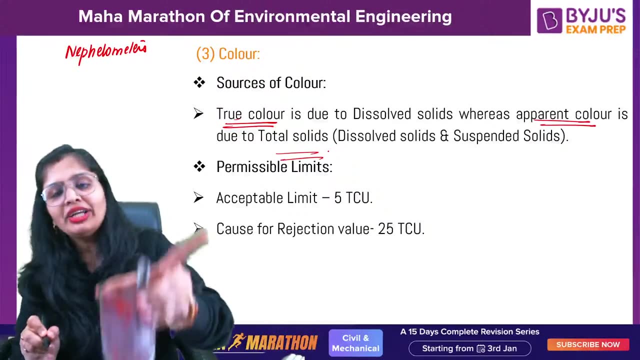 all those things. So what happens is color is basically due to dissolved solids. There are two types of color. One is true color and one is the apparent color. True color is due to dissolved solids. Well, apparent color is due to total solids. Can you tell? 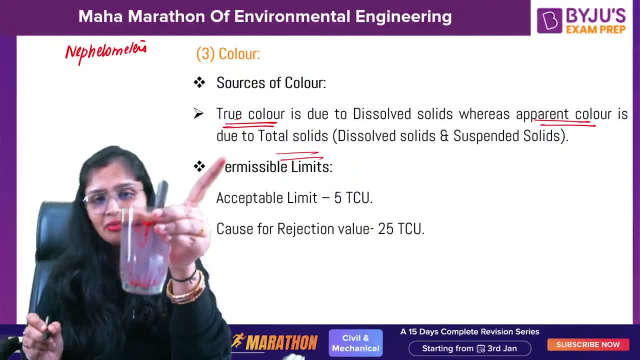 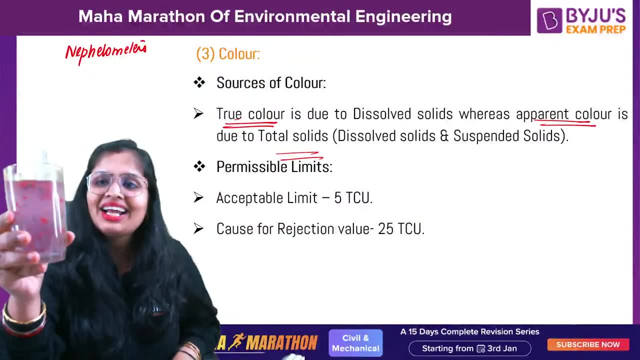 me whether it is true color or apparent color. Can you tell me whether this is true color or apparent color? True color, apparent color? You can see it and tell me fast. True color, apparent color? Apparent color? Why? Because your suspended solids are also. 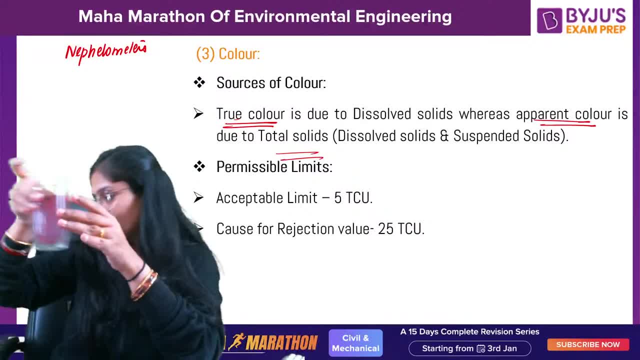 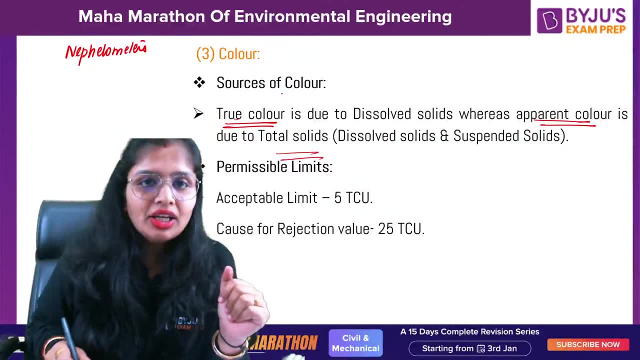 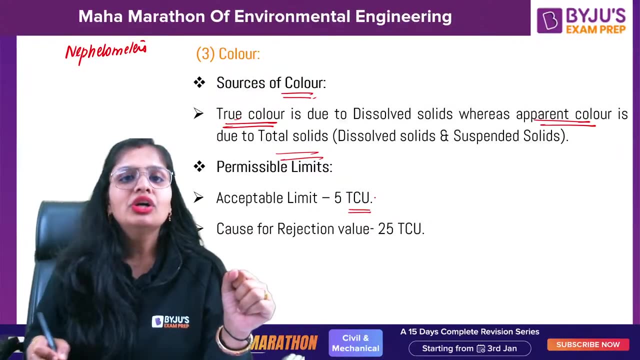 there. Okay, Suspended solids are also there. So this you should know. Now, if you talk about it basically, color we measure, we measure the unit of. it comes out to be true color unit. What you do: You take a test sample and you take a standard sample. This is not. 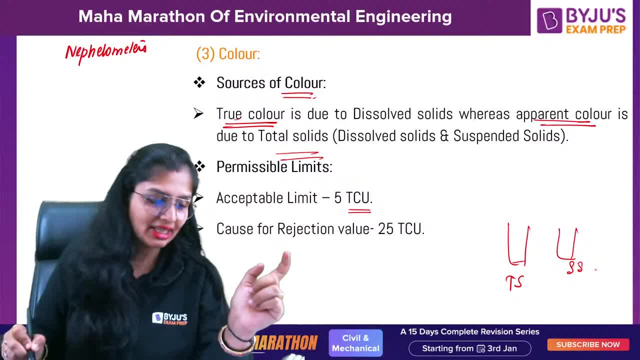 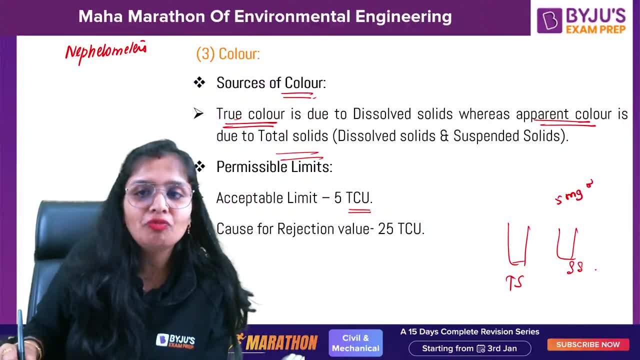 total Solids and dissolved solids. This is test sample and this is standard sample. What you do, Standard sample is one, something which you make it. If you put, let us suppose, 5 mg of platinum in the form of chloroplatinate ion Chloro, It has so strong smell now, Oh, 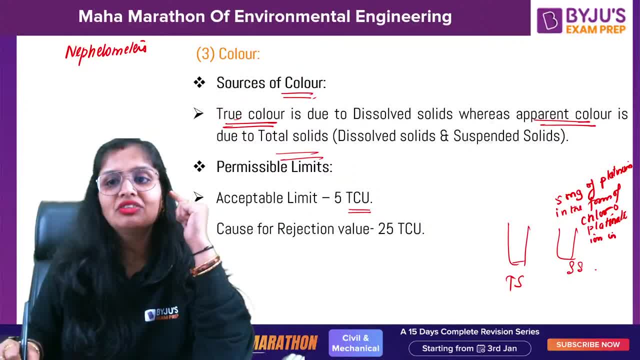 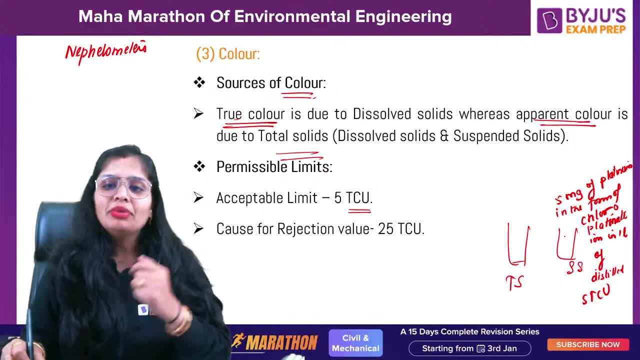 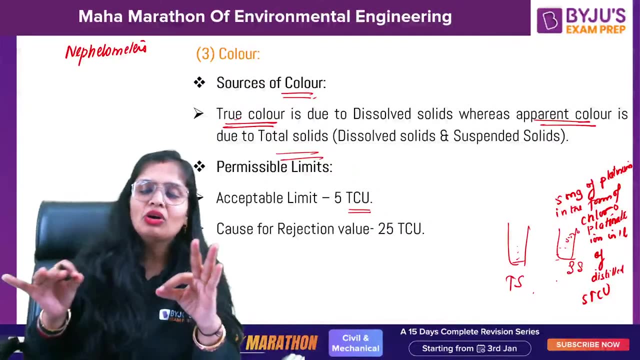 my God, This ink In one liter of distilled water. In one liter of distilled water You will call it as 5 TCU. So this sample, you made it, So you know it. If the color produced in both the sample is same, you will say test sample also has the color of 5 TCU. Generally, 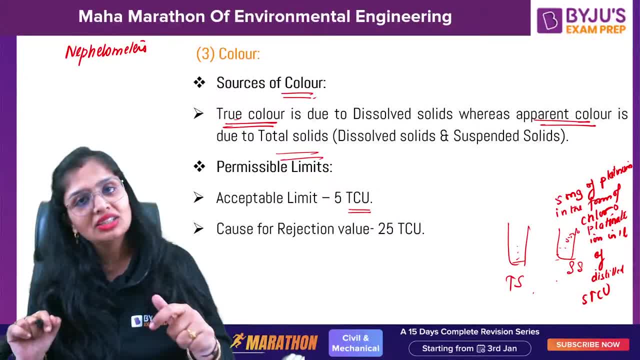 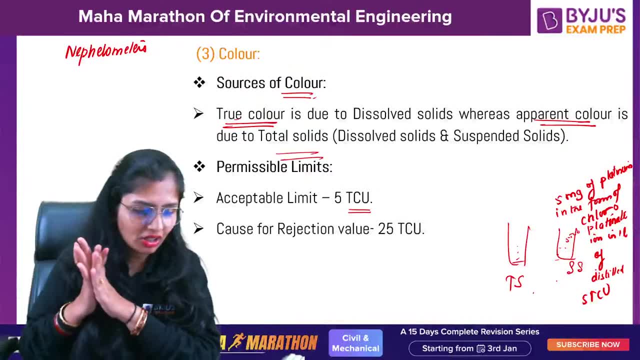 this gives only yellow color, So, but colors can be any other. So there is advanced technique, known as spectrophotometer technique, for the measurement of color. Okay, Acceptable limit is 5 TCU, Up to 5 TCU. color is 5 TCU. So you know it, So you know it, So you know. 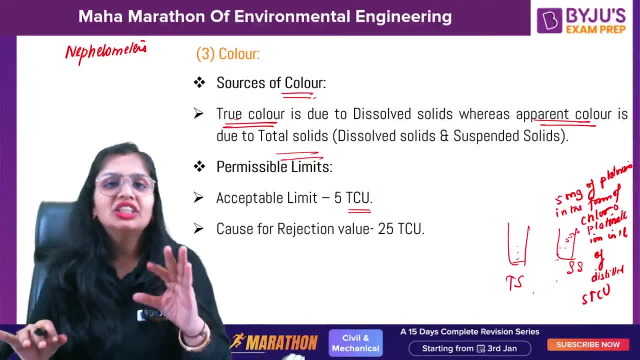 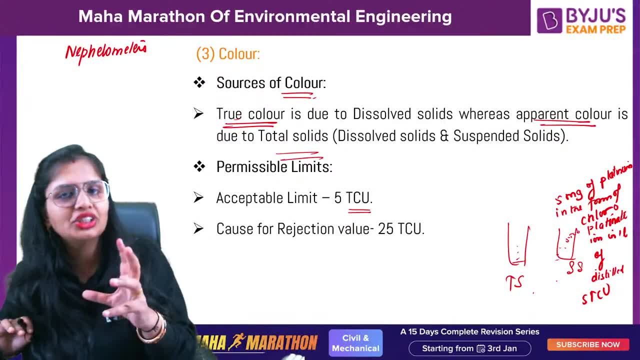 permitted cost for rejection value is 25 TCU. Generally the color and all. you can see that yellowish tincture, specifically during rainy season. You guys would have seen that yellowish tincture and all color. So that is also permissible. up to 5 TCU, Okay That. 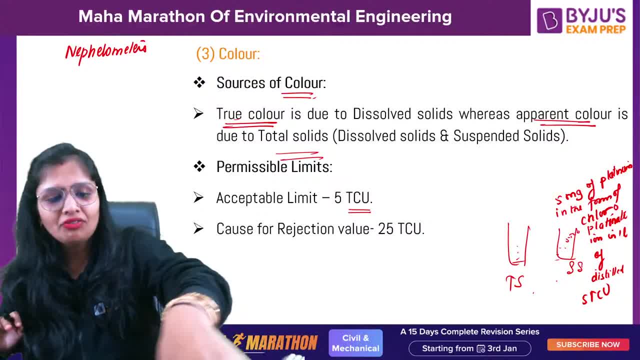 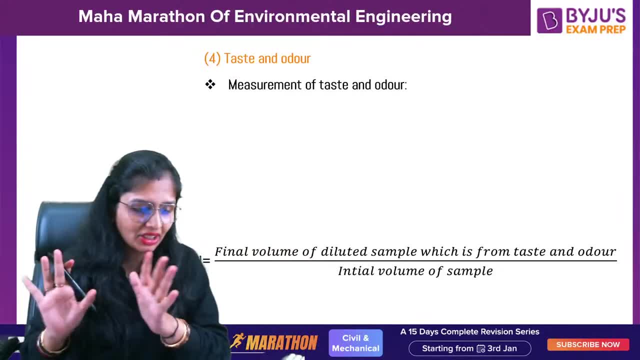 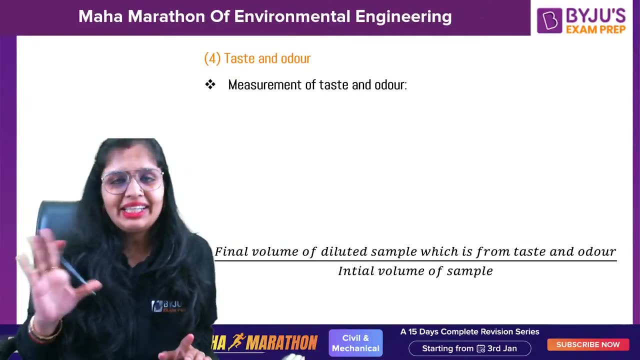 is also permissible up to 5 TCU. Now coming up further. coming up further, we have taste and odor. This again, this question has been asked in your examination regarding taste and odor. If you want to measure taste and odor, you why we take it. these two are different. 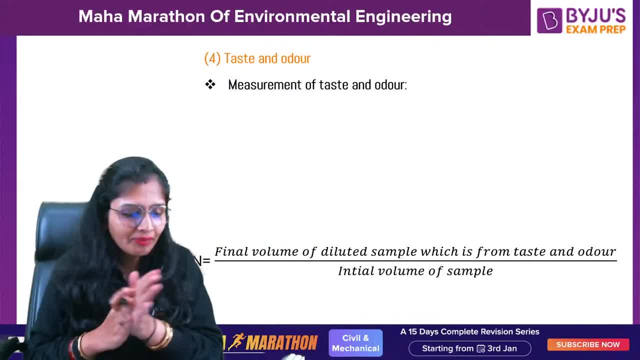 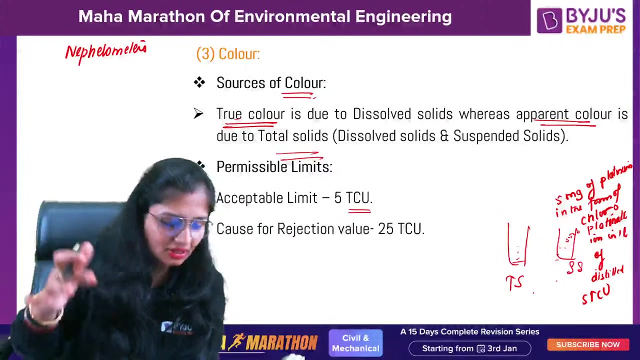 parameters. These two are different physical parameters. Okay, Is it measured by tintometers and Nestler tubes? As per 105.00.2012 I am talking, Is it? Yeah, Yes, So if you want to measure taste and odor, you can take this pressure gauge. So we don't take equal to. 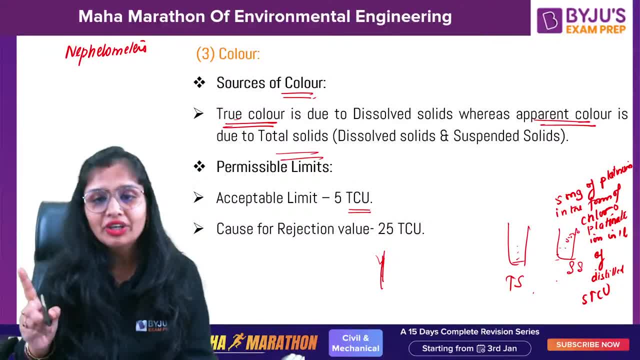 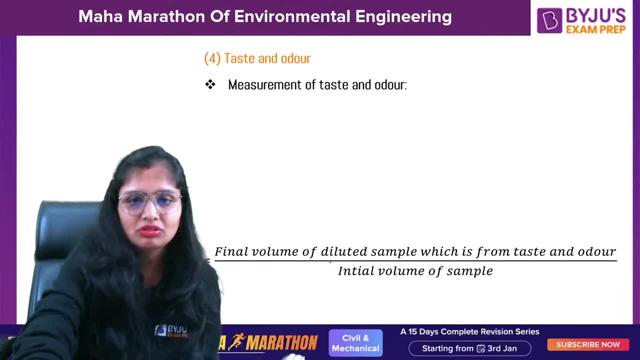 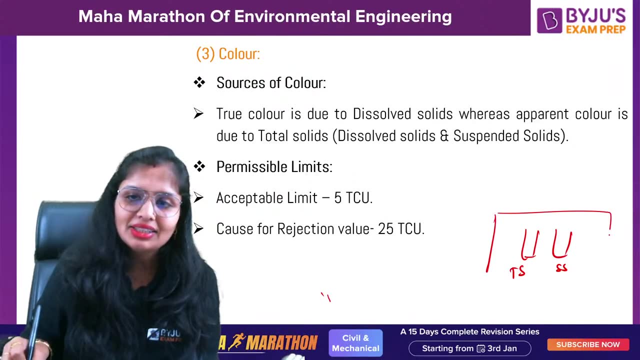 TCU equals to PPM. We don't take equal to PPM. And what else was there? Yeah, So tintometers, where it has gone, There's something, It is gone. Standard sample: the. this tubes are known as Nestler tubes and this equipment is not Centers Fest. Those are the tubes that we use. Let us take a sample. Here is the the sample. This is the sample that it is what we have. It is the sample. So here it is. This is the sample that it is called the Nestler. Now. the sample is called the Nestler tubes. Now, if you have a, it is the sample. Now you can do the tuning of the this sample. 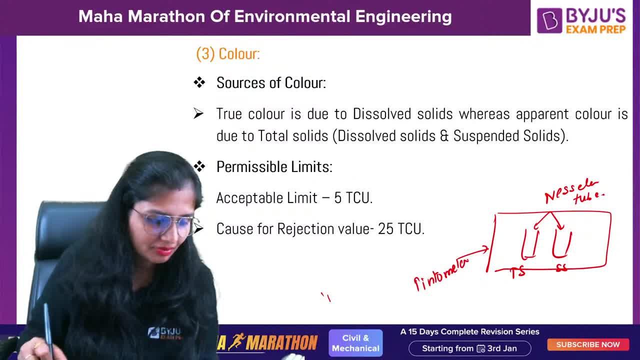 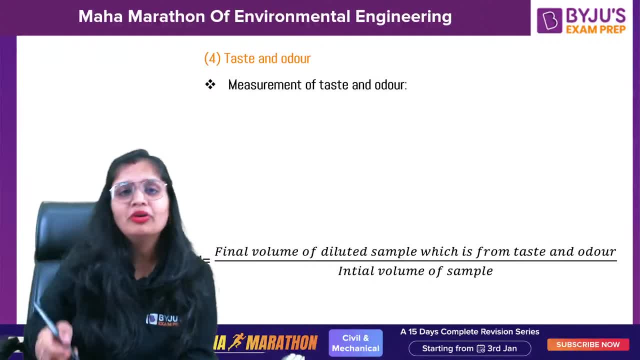 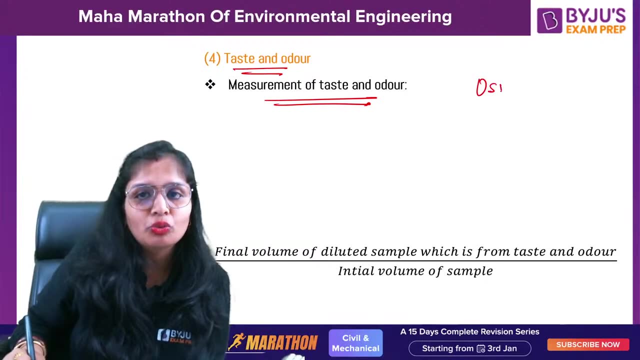 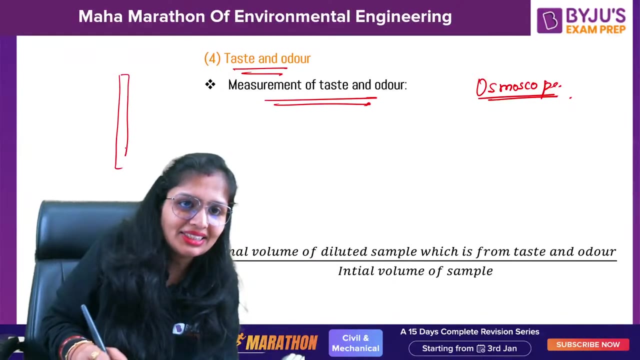 known as tintometers. Okay, Now, when you talk about taste and odor, the measurement of taste and odor, if you talk about this, is done by osmoscope. The measurement is done by osmoscope. There is an equipment like this, Okay, And there is a place to insert your. 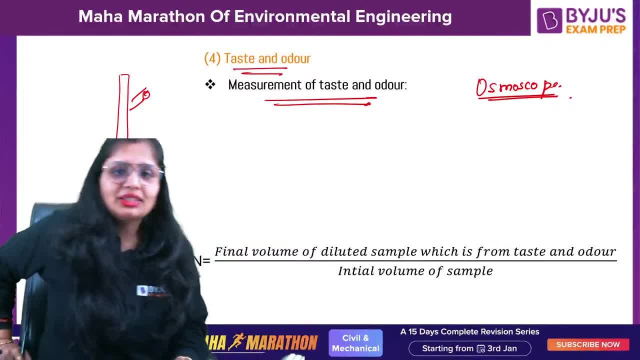 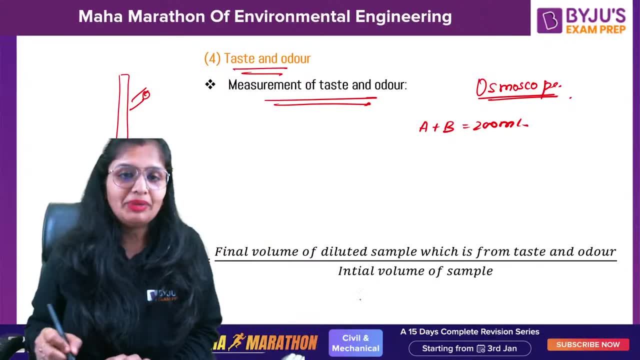 nose. Now what happens in this? What happens in this is, as per the code, A plus B is mentioned as 200 ml. Now you will say, ma'am, what is A, what is B? A is the raw water sample. 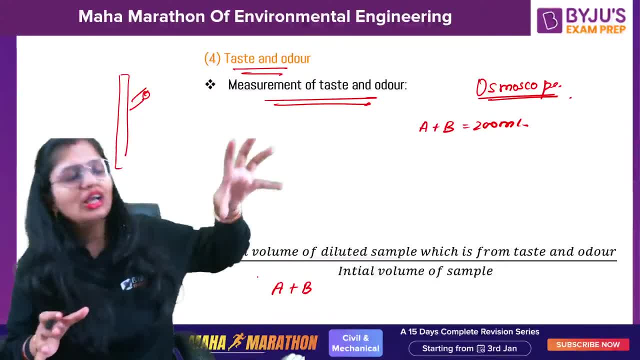 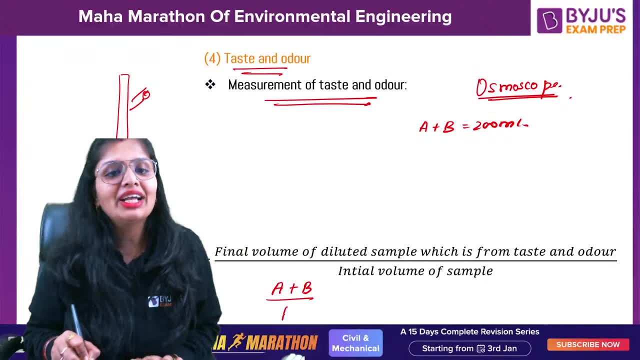 B is the sample, When, what you will do, You will add distilled water. You keep on adding, adding, adding till that time you see that no smell is there. So A plus B divided by A, this will give you threshold odor number. TUN stands for threshold odor number. 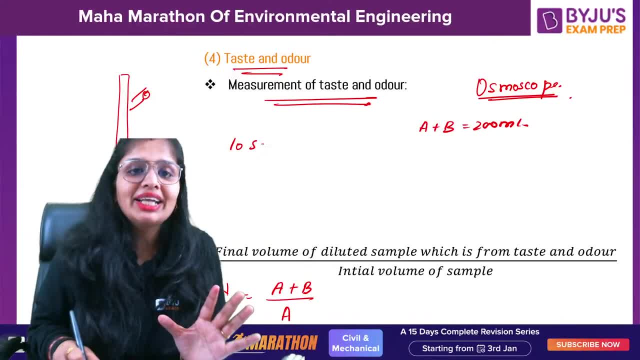 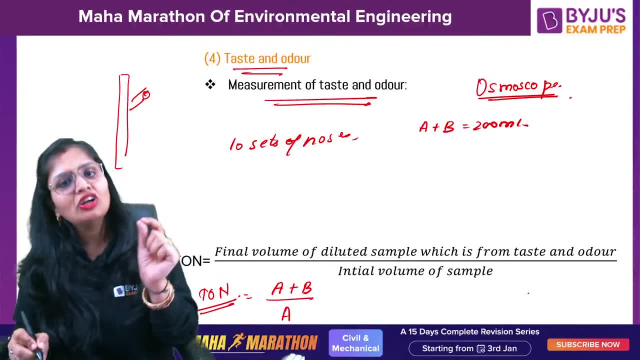 Now what happens is not. what happens is, in this case, you take 10 sets of noses. 10 sets of noses means you will take 10 people who will smell it. If anyone of the 10 people say that smell is there, you will add more water, But you have to take it in such a manner. 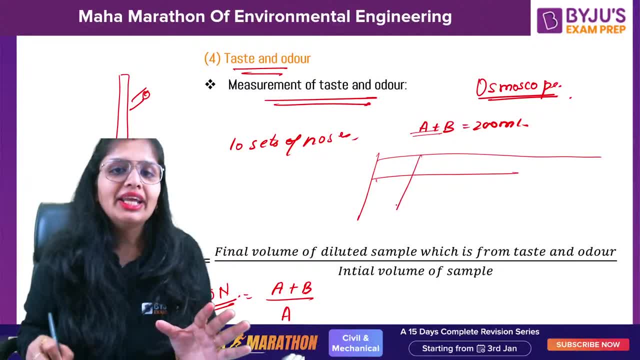 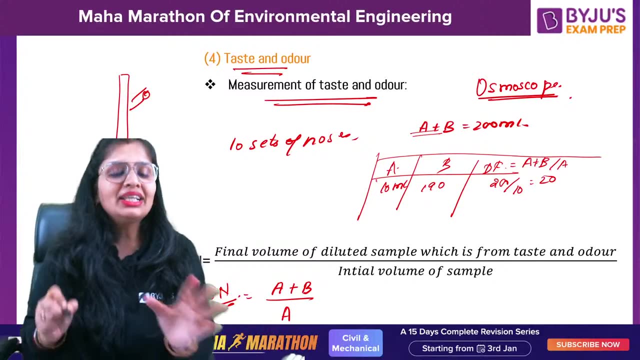 that A plus B has to be 200.. Let us suppose initially A is 10 ml, B is 190 ml, So the dilution factor which we call it comes out to be 200 by 10.. 20. Because dilution factor is A plus B by A. But still one of the person, like Ayan, said that 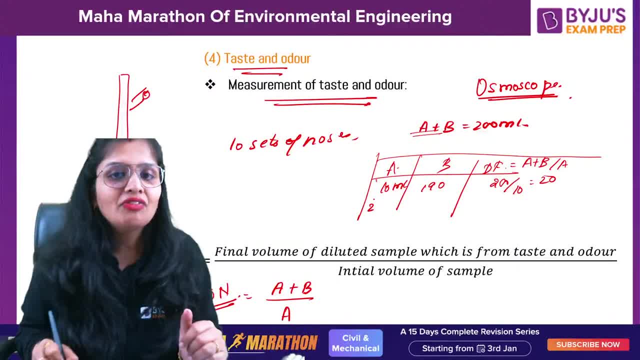 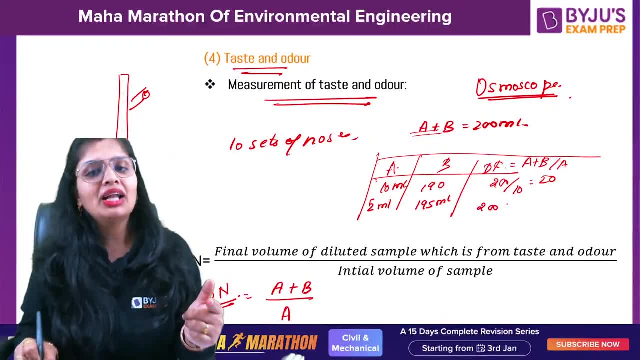 ma'am smell is still coming. So what I will take? I will take 5 ml as the raw water sample and I will take 195 ml as the water. Then I will say that 20 people again, 10 people will again. 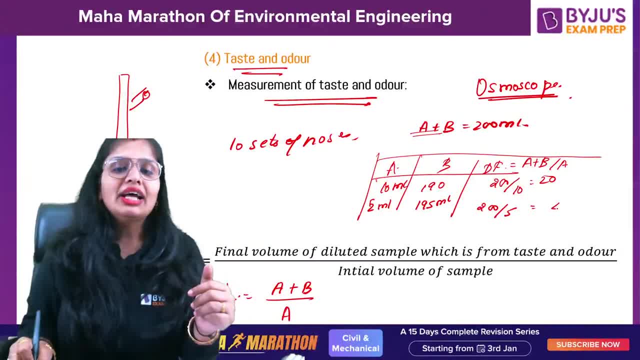 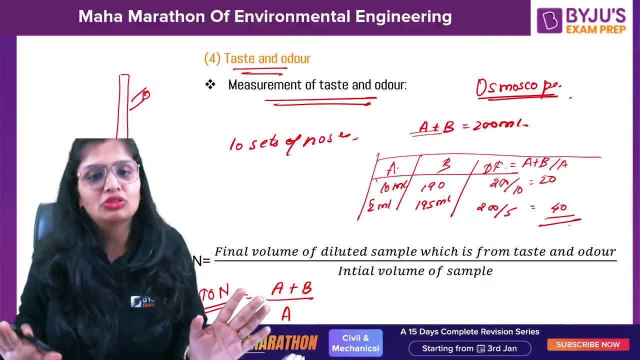 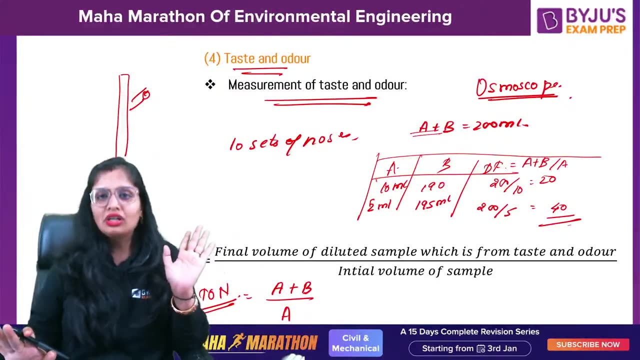 come and they will smell it. So what will happen If again nobody said that any smell is coming? So I will say 40 is the dilution factor and I will do the treatment. Okay, So osmoscope is used and 10 sets of noses are taken. for 10 sets of noses are taken. 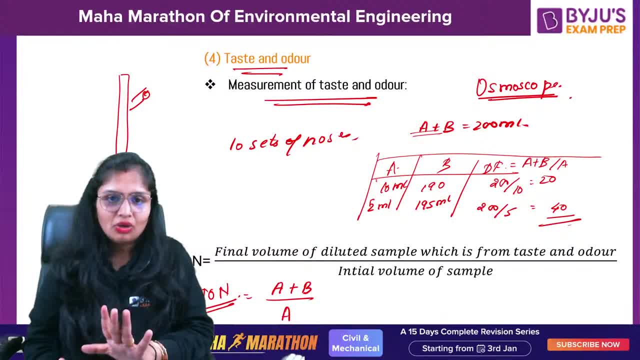 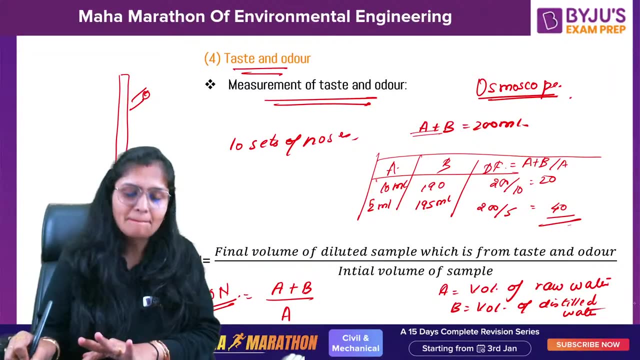 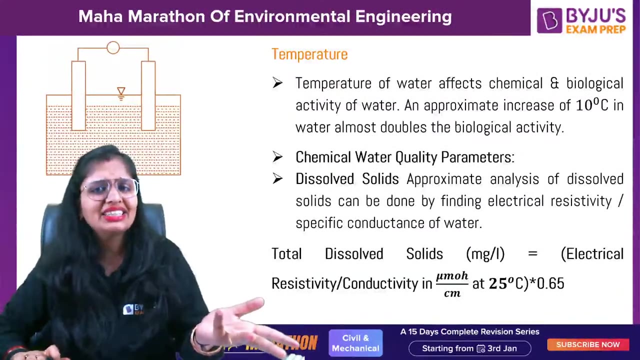 for checking it. if any smell is there, Okay, And A is the volume of raw water, B is the volume of distilled water. Clear, Okay. So that's temperature. Temperature is basically very simple. It affects taste and odor. If you talk about the limits, initially it was 1 TUN and 3 TUN cost for rejection limit. 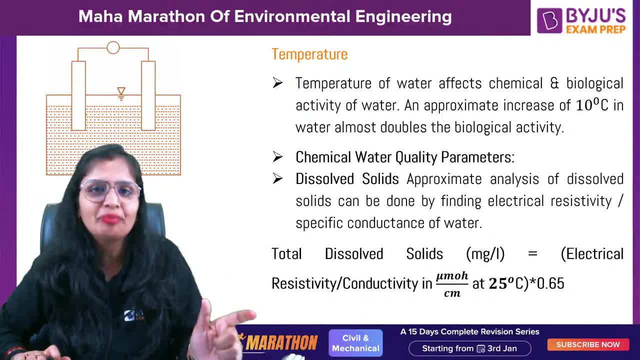 Now, if you take the code, they have written it there acceptable. Okay, That means basically they have written acceptable. or you can say they have written it there agreeable. So that one which agreeable means basically they don't allow any taste and odor in the 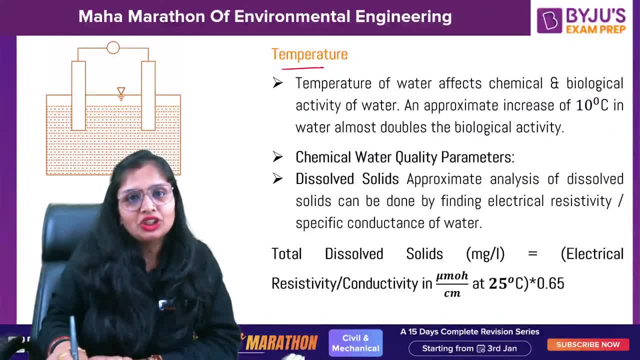 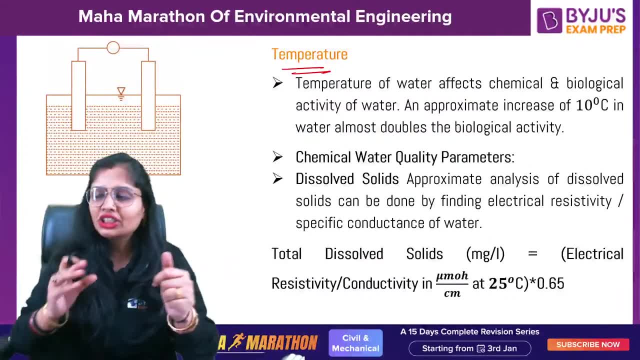 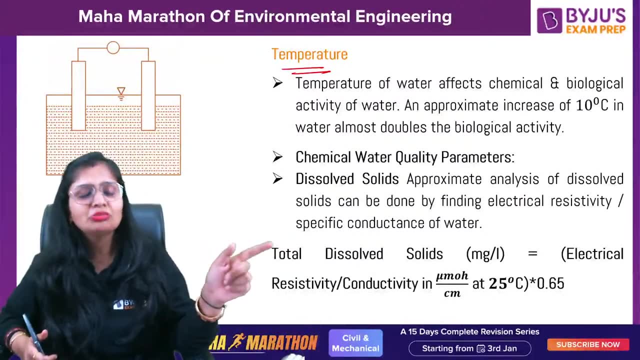 water. Okay, Now when you talk about temperature- temperature obviously you can feel it and you can see it affects the chemical and biological activity. If 10 degrees Celsius you increase the temperature, almost the biological activity will double it up. 1 TUN, 3 TUN. was there, Ashish? but if you check it now they have. 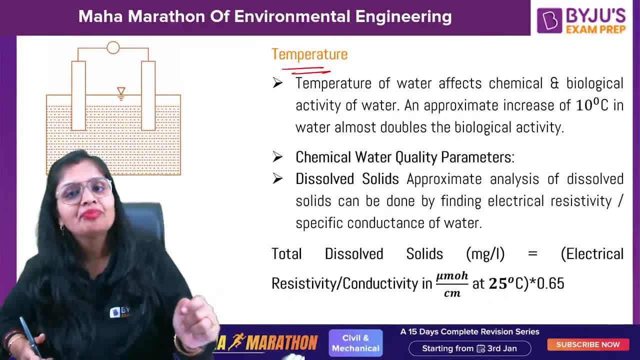 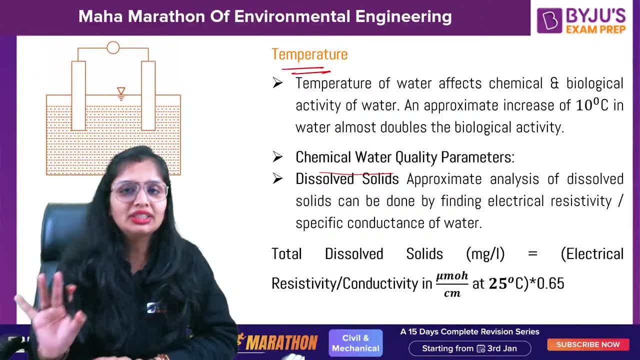 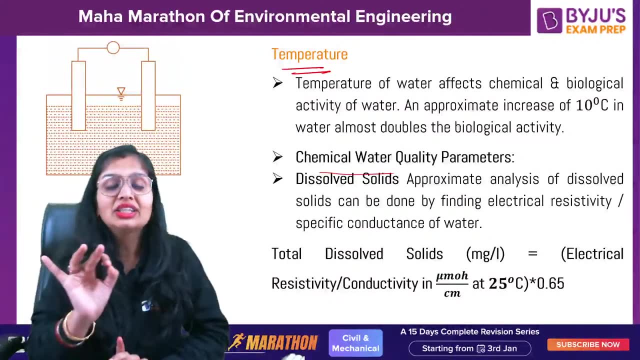 written it agreeable there, Okay, So this you have to check it out Now, talking about chemical water quality parameters, chemical dissolved solids: is there Dissolved solids already? I told you the measurement technique. You can suspend it solids. But there is one more method that is an approximate method. 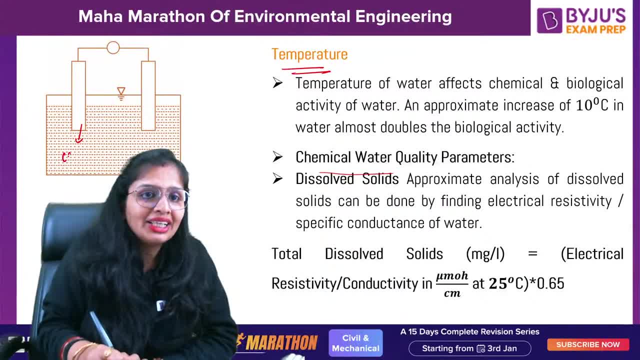 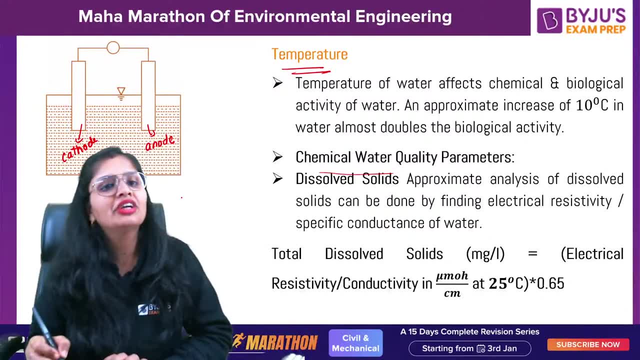 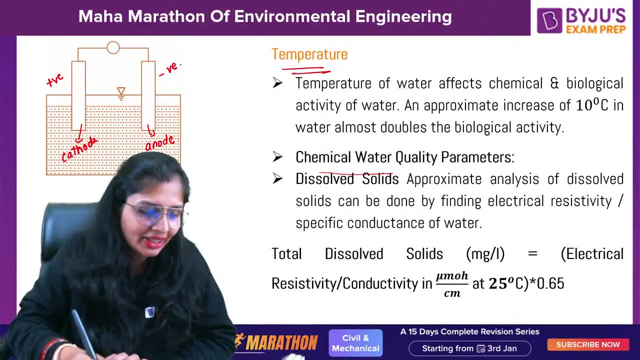 What do you do? Let us suppose you know what is cathode and anode. You know cathode and anode Guys. cathode is positive or negative, Positive electrode, Anode is negative electrode, Yes or no, And you have ions present here, Cations, positively charged ions. 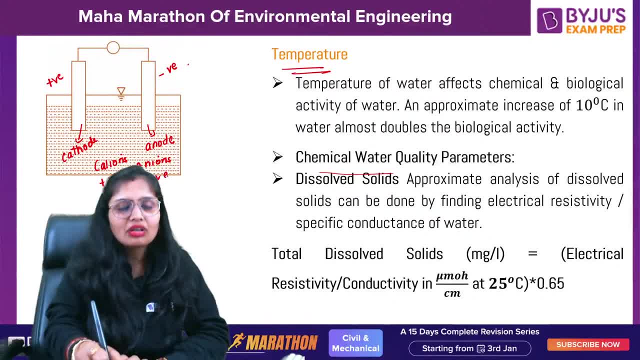 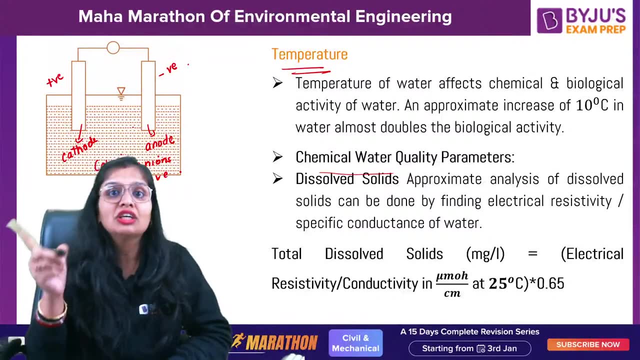 Anions, negatively charged ions. So now, what will happen? Now, what will happen? When you put this water here and when you measure the electrical conductivity, the positive opposites attract, So the positive charged ions which are present in the water. remember: 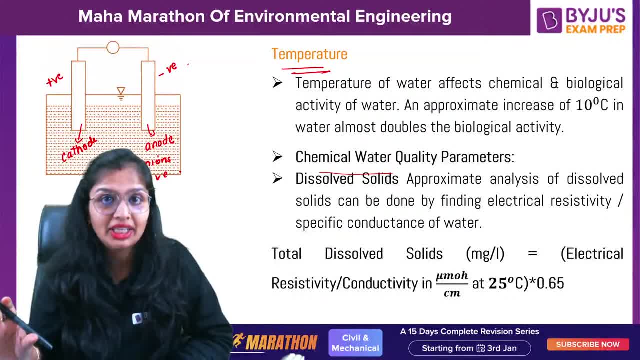 pure water is a bad conductor of electricity. But if in that water ions are there, if you take distilled water, it will not conduct electricity because it is just 2 moles of mole of oxygen Cations. positive charge will go and deposit on the anode. negatively charged. 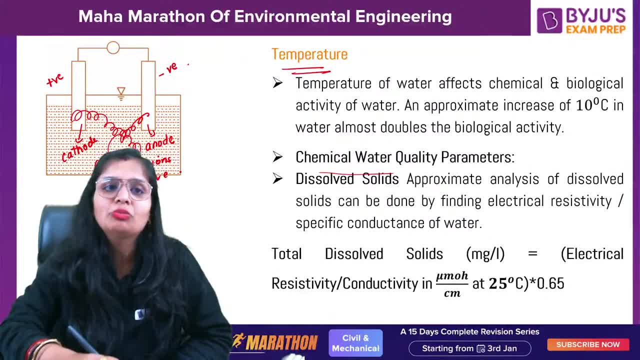 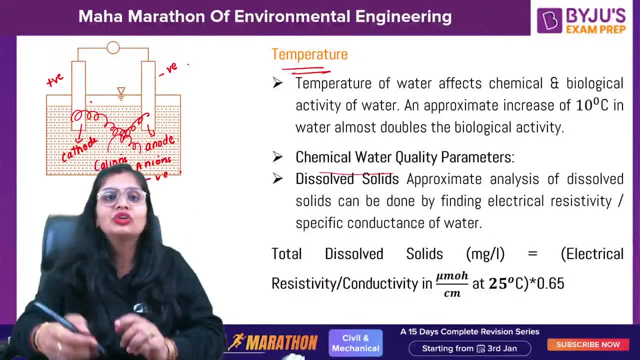 electrode. Anions will go and deposit on the positively charged electrode, that is, cathode. When they will go, the movement will be recorded, The movement will be there, due to which current will be produced. okay, Ammeter will be there, So current will be produced. You will measure. 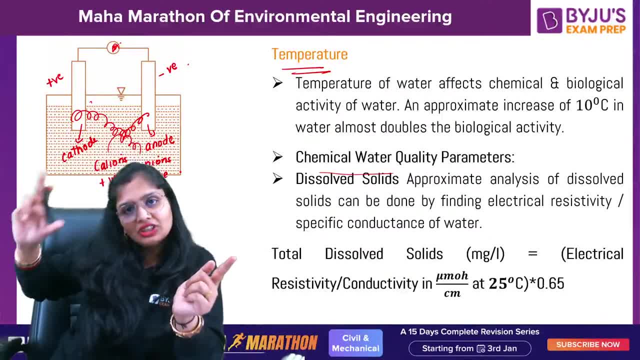 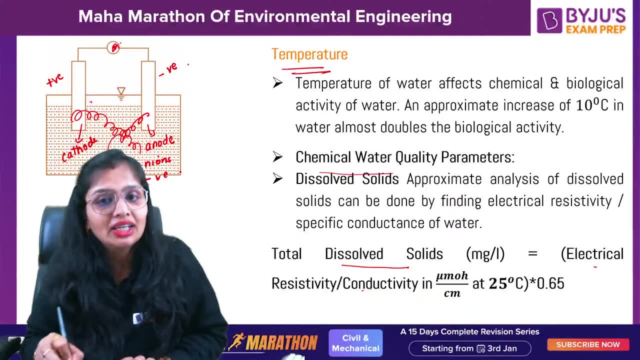 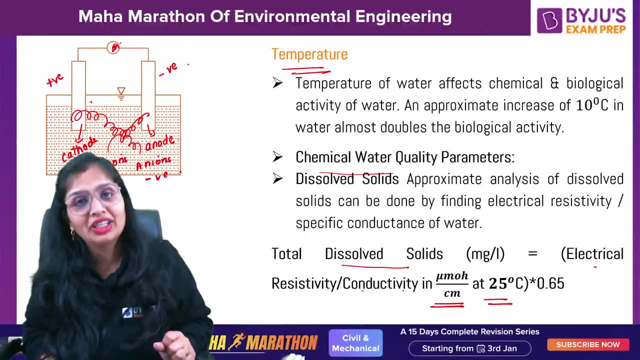 that current, okay. And that current is further calibrated to total dissolved solids. So that's the reason: total dissolved solids is equal to electrical conductivity in micromole per centimeter at 25 degree Celsius. Now why it is necessary to measure the temperature? Because the conductivity 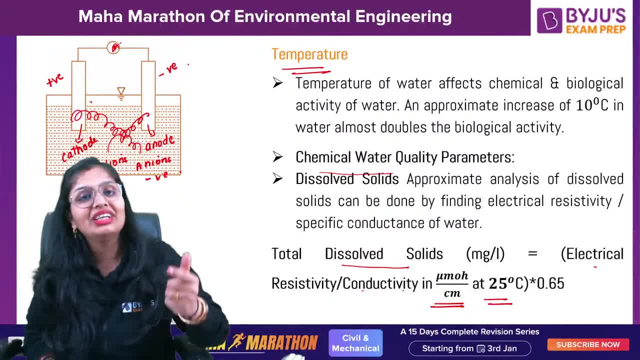 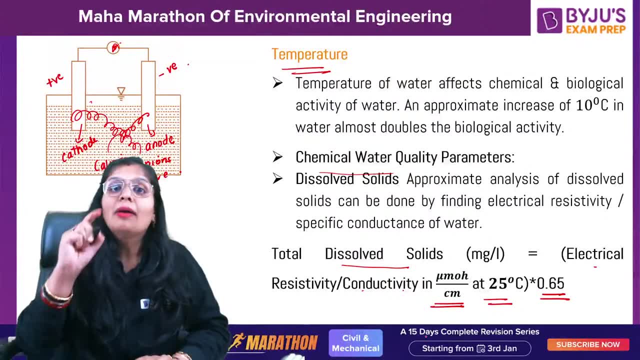 changes. Dissolved solids will remain same, but the conductivity changes as the temperature changes And that's why a factor known as 0.65 is also interesting. But this is an approximate method. Reason: Pure water is exactly pH 7.. Yes, Or you can say 2 moles. 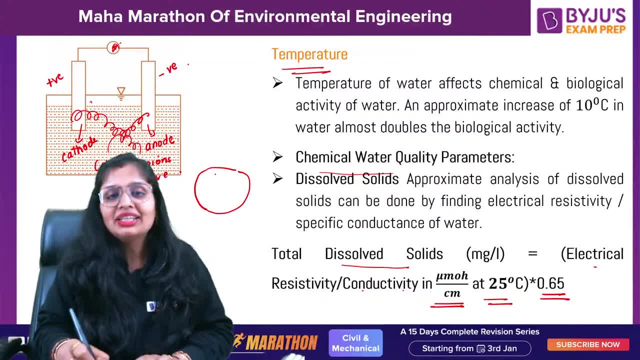 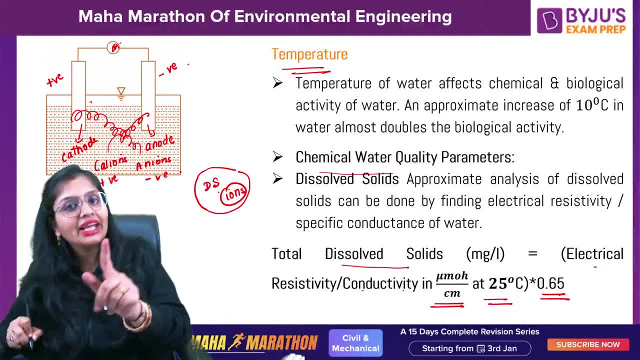 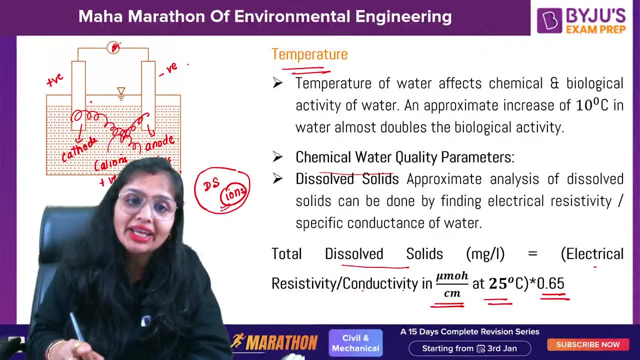 of hydrogen, 1 moles of oxygen. But it is an approximate method. Why? Because all dissolved solids are not ions. All ions are dissolved solids, but all dissolved solids are not ions And this will give me only the ions concentration technically. That's the reason this is an 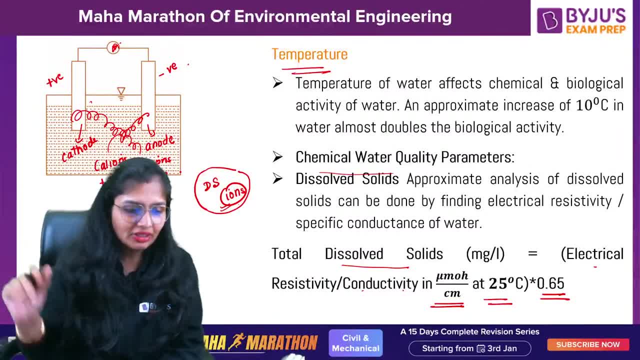 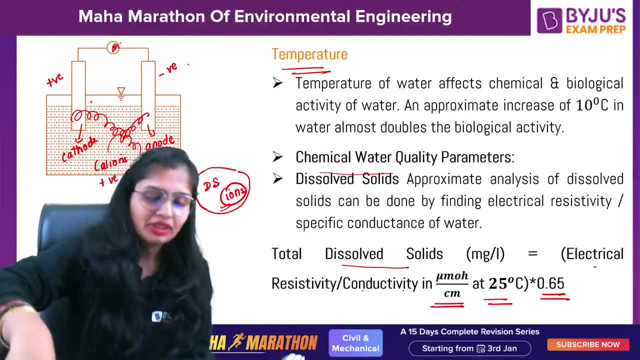 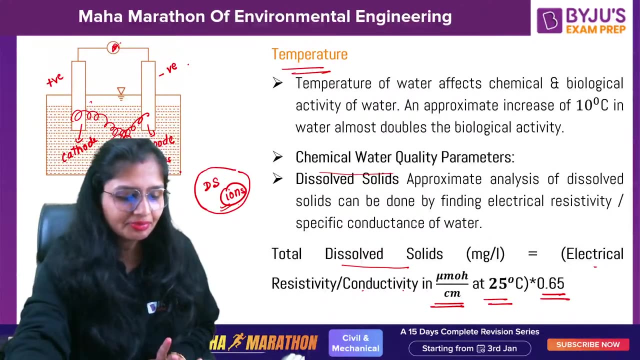 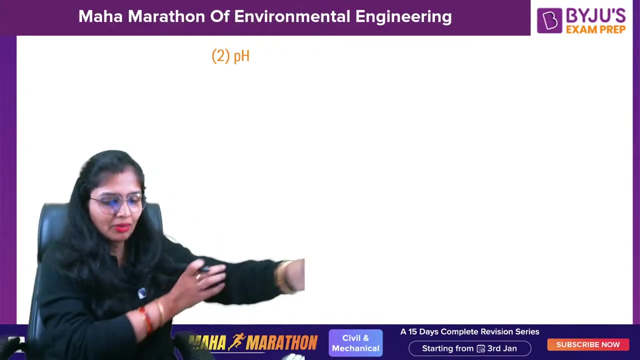 approximate method. Any doubt till here? You can measure it. Any doubt till here, guys, Faster, faster. Any doubt Shall I increase the speed? little Arun, Vishal, everybody, Okay, Fine, No doubt, Okay. So let's talk about pH. pH is the scale approximately analysis. 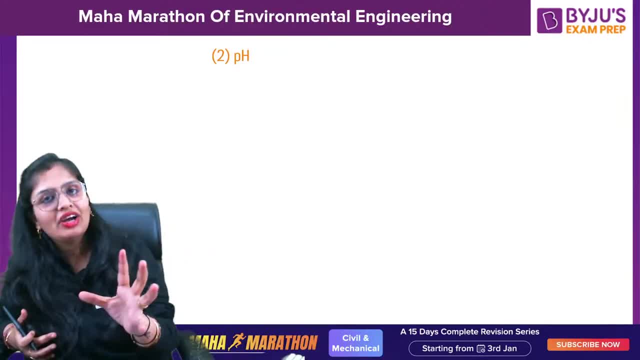 I already told you. If you want to measure the exact one, then I already told you. take the sample which is poured through the filter paper. That sample- 104 degree Celsius. you will get the exact value. This is the approximate one, But they can also measure the exact one. So let's talk about. 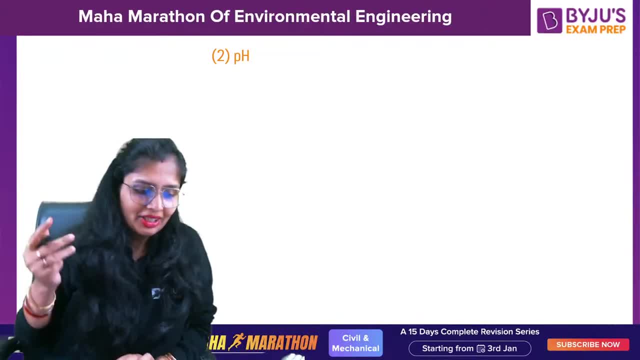 pH. I will just make sure I am giving all the nothing into parentheses, So let me just keep my example. I will be letting everyone just keep their number lists down, Got it? Let me just start the sequence here. Let me ask in context. Let's see what it is walking. 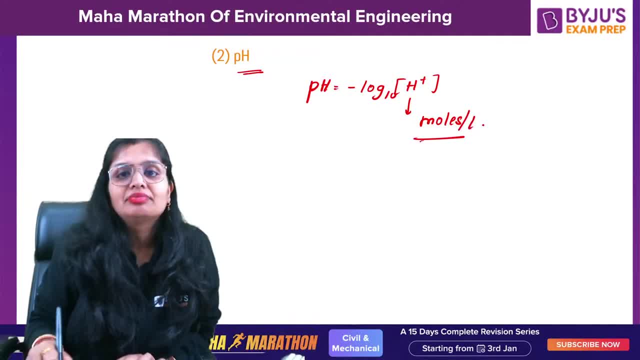 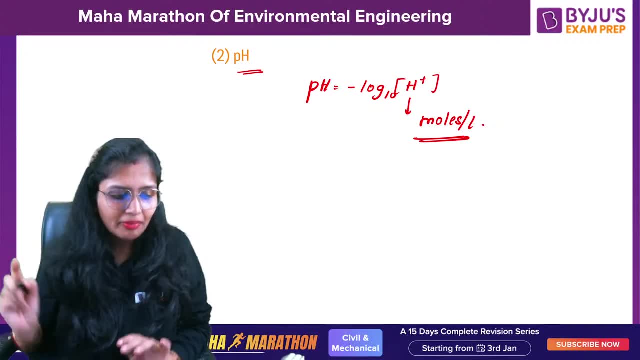 fast, regardless of where we are sitting. this particular column, This is the number 7.. Some of you feel comfortable when I use theählt에. Just keep your answer in the description. Of course, I can put the screen so that you feel comfortable. Okay, Let me ask you. that is. the reason: Speed. okay, I was asking to increase a little, if you guys permit. So pH is the scale of pH is there. So that is minus log base 10. H+. Remember this H plus is in moles per litre, Very, very important. 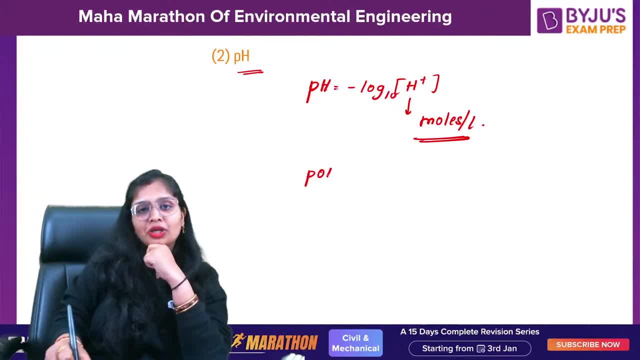 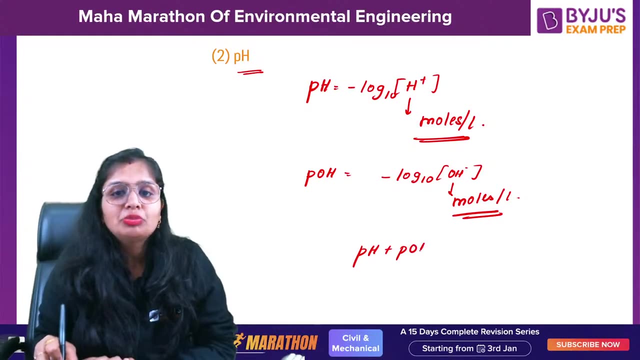 this is the pH. now talking about pOH, this is the basic formulas. is only needed in this: OH minus iron. okay, and this also- this is the only thing which you need to know- that the concentration here is in moles per liter. now, pH plus pOH is equal to 14. H plus into OH minus is 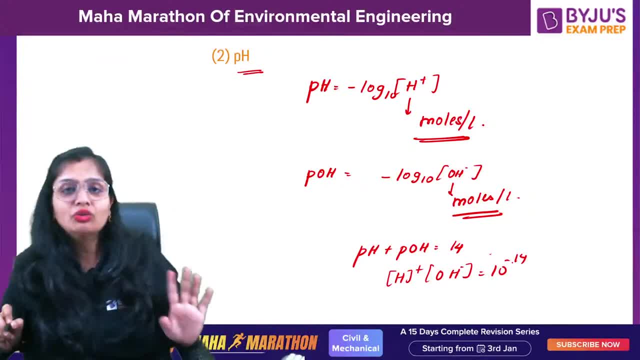 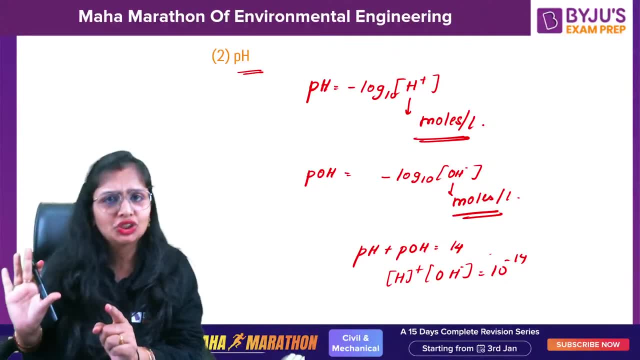 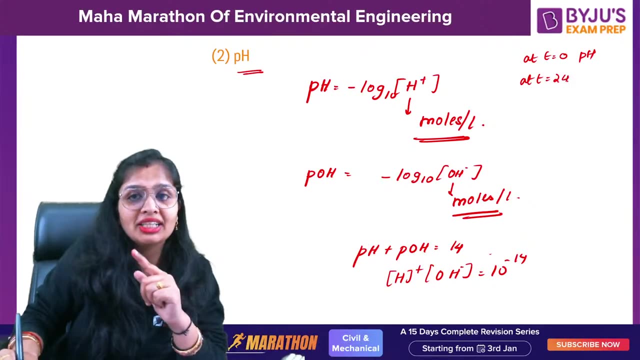 equal to 10, raised to power minus 14. now gate question was been asked. I tell you, if this say in the question there is linear variation in the pH, at t is equal to 0, let us suppose a pH was given to you at t is equal to 24. very important guys, listen to it very carefully. 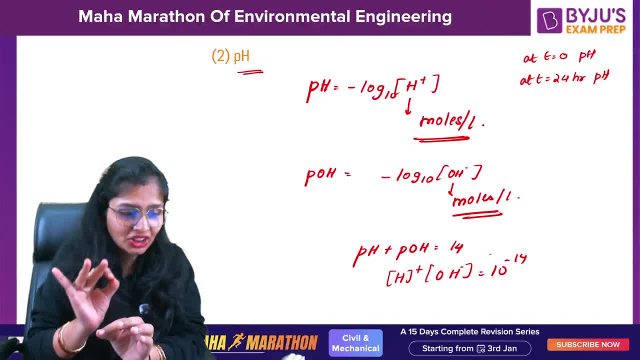 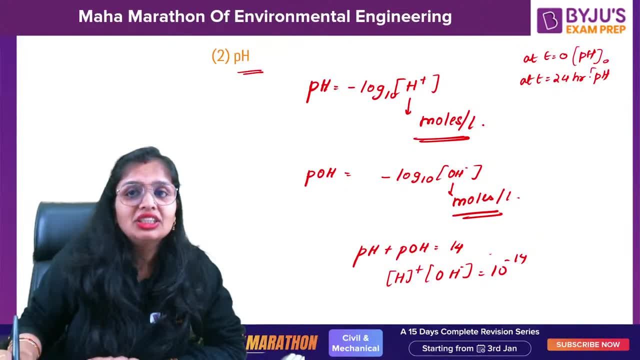 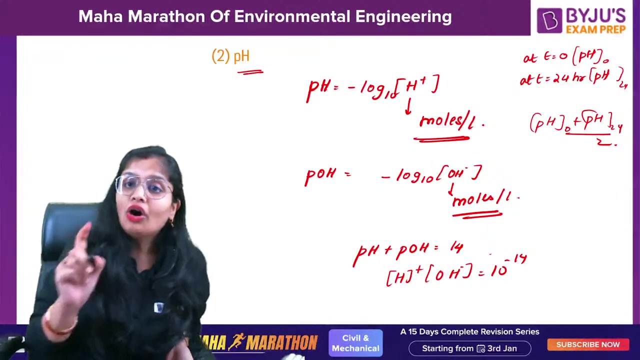 pH is given to you and it is telling you linear variation of pH is there, what you have to do? just add both of them. if it is in the question, it is written linear variation of pH is there. but if in the question it is telling you linear variation in the hydrogen ion concentration or H. 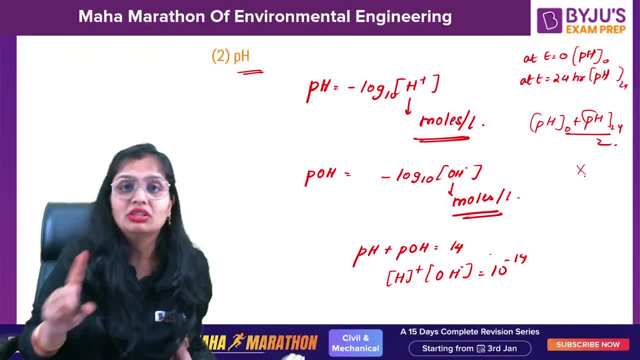 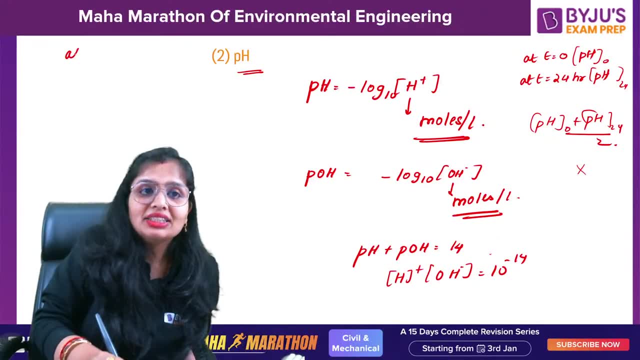 plus ion. constant concentration is there. don't go by this method. no, it will be wrong. what you have to do in that case? what you have to do in that case is first: at t is equal to 0, you have to measure H plus ion concentration. at t is equal to 24 hours, you have to measure H plus ion. 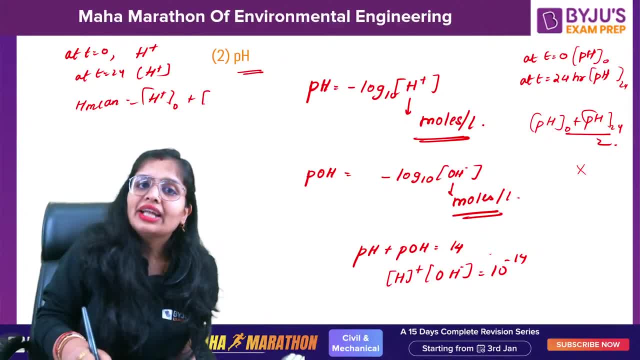 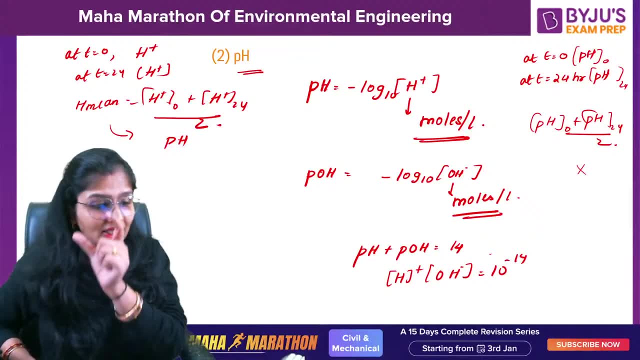 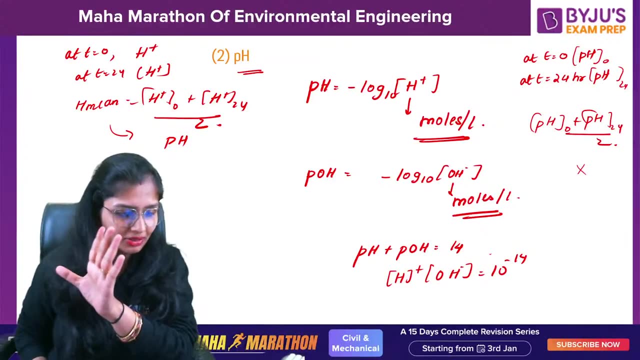 concentration at 0 and then from 0 you can come up with the temperature of H plus at 0 hours, H plus at 24 hours divided by 2, and then you will measure pH. so that's the reason. understands the wording very well. I will make you understand that very well. 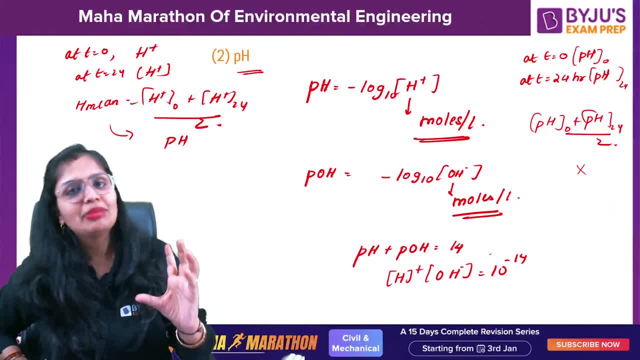 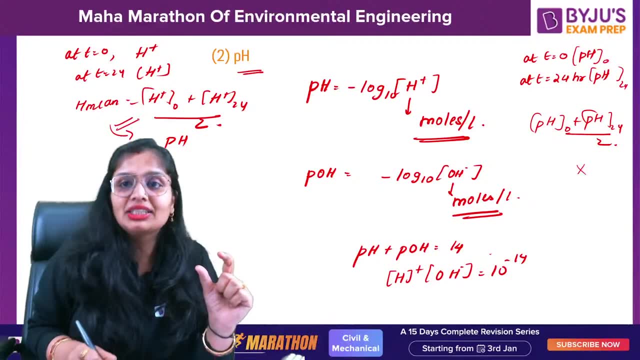 my bad, Arun, you are saying this. is this nana you have to calculate? okay, H plus is. when it is telling linear variation in H plus, go by this method. if it is telling you linear variation in pH, go by this method. okay. 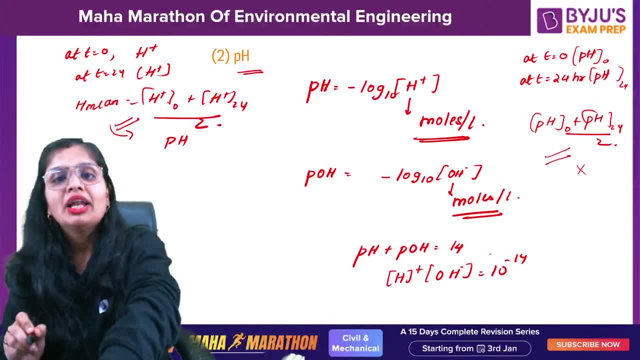 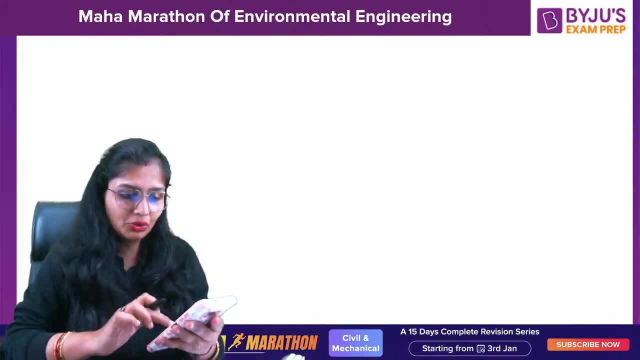 this you should know, very, very, very important. okay, now, one question is there. I will mark it for you guys. one question is there which I will mark it for you guys. you guys should do it. this is a very good question and this is of your gate question. okay, I have it. this question was: 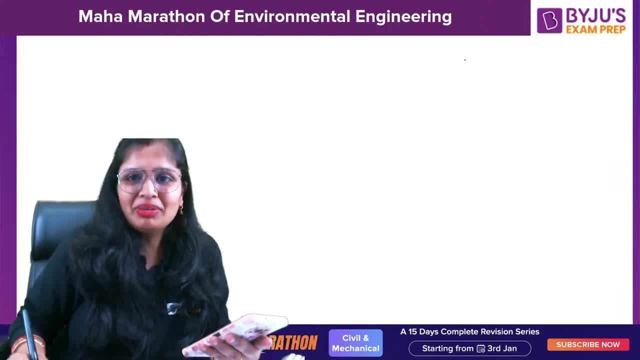 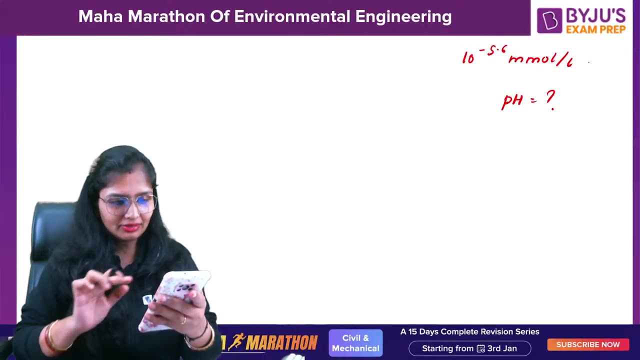 there based water sample, simple data. I will write it, you guys will have it. 2008 IISC, Bangalore. question. 5.6 millimoles per liter is there. it is asking you the pH: calculate, calculate. 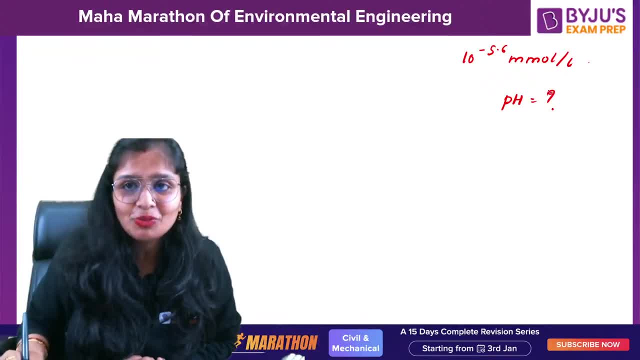 calculate my okay pH pH now in this question, guys, 10 minus 5.6, first of all, millimole is written, so you have to take it as moles per liter. so this will be 10 raised to power minus 8.6 moles per. 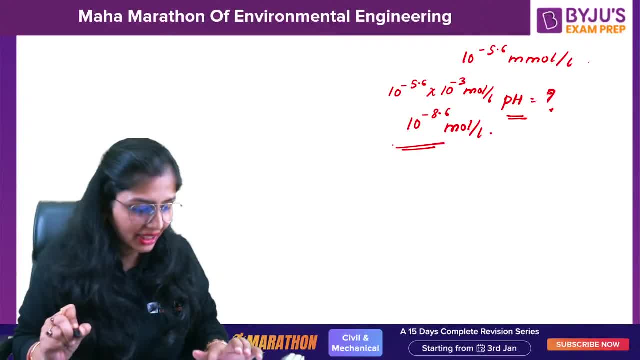 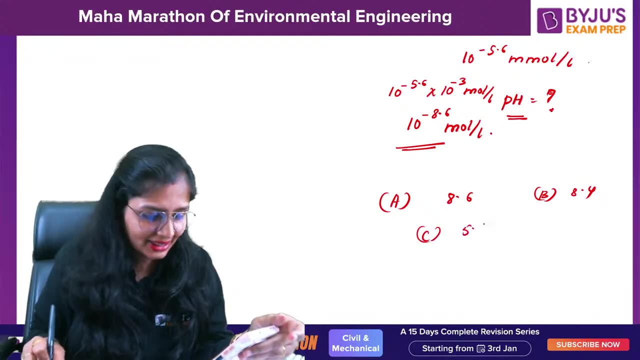 liter. this is the. this is the concentration. it is asking you pH, how you will calculate. calculate in the option it is given me. in the option it is given me 8.6, 8.4,, 5.6,, 5.4,. it is asking me pH: calculate pH. and it is given me what a water sample. this is OH minus and concentration. solve it. OH minus and concentration is given to me. 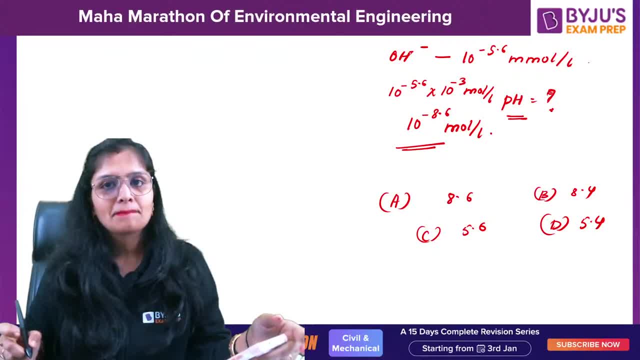 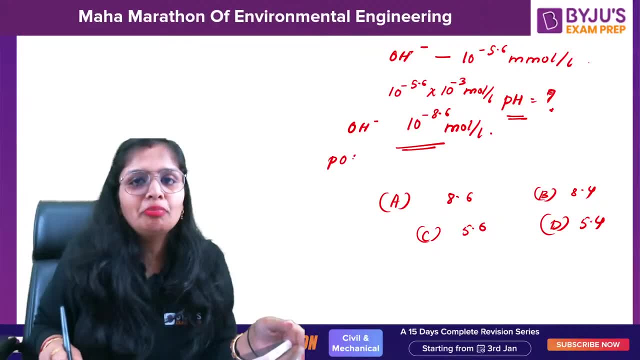 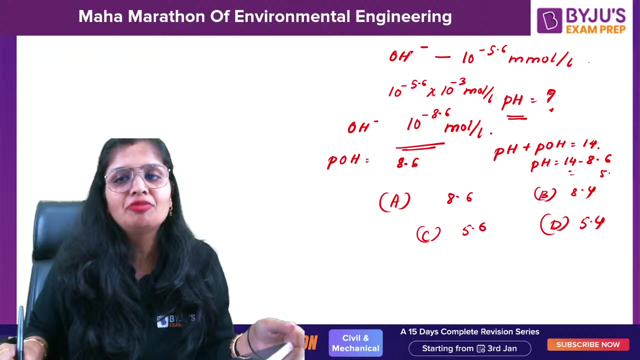 how can you do OH minus first? first you will calculate POH. that will come out to be how much 8.6, pH plus POH is equal to 14, so it will come out to be how much pH will come out to be 14 minus 8.6, it will come out to be how much 5.4, as simple one. last question: this is a very important question. 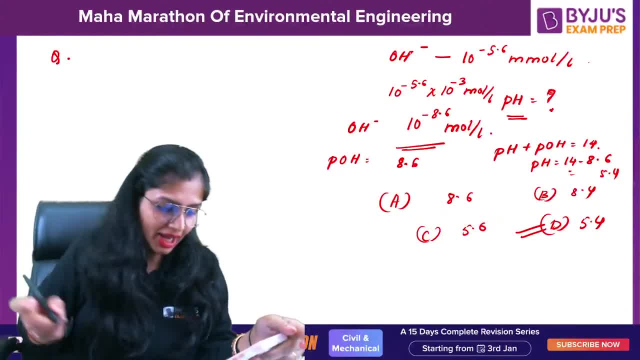 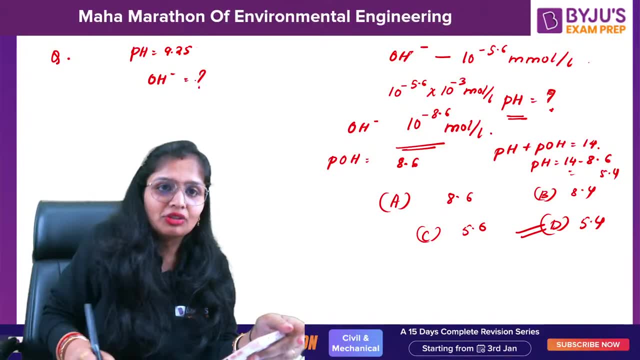 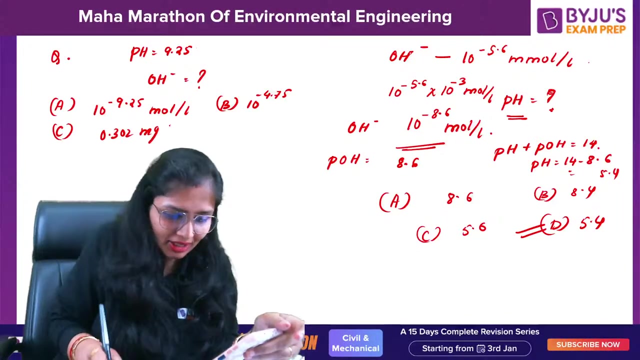 guys, when you go, just prepare this question and go. water sample pH is given to you as 9.25, and it is asking you OH minus and concentration options. I will give you. this is a good question: 10 raised to power minus 2.5, 9.25 moles per liter. B is 10 raised to power minus 4.75,, C is 0.302 mg per liter and D is 3.020 mg per liter. 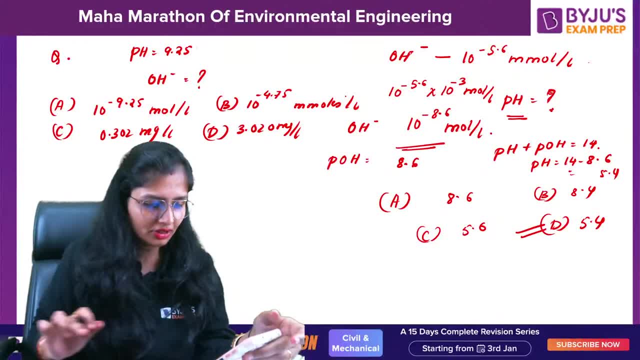 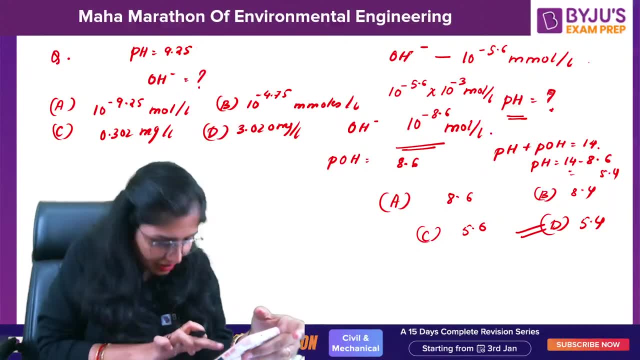 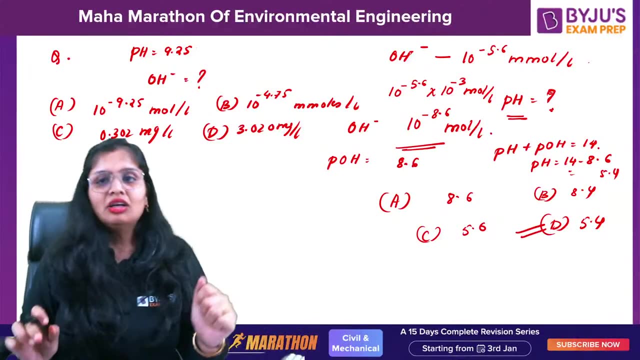 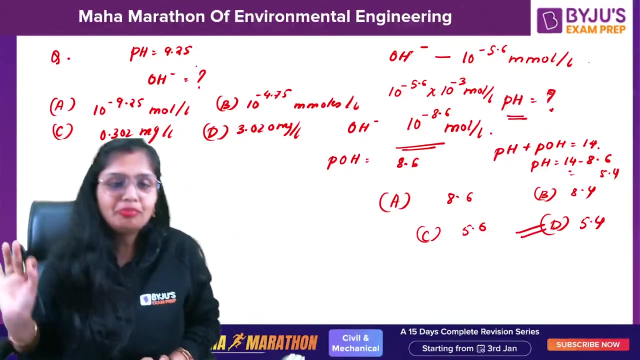 come on, guys, solve this good question, solve this. thank you so much, Prateek sir. come on guys. this you should know: pH is given to you 9.25,. pH is given to you 9.25, if you need OH minus and if you need OH minus and. 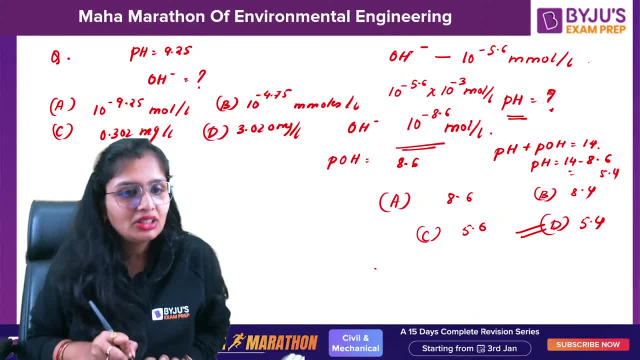 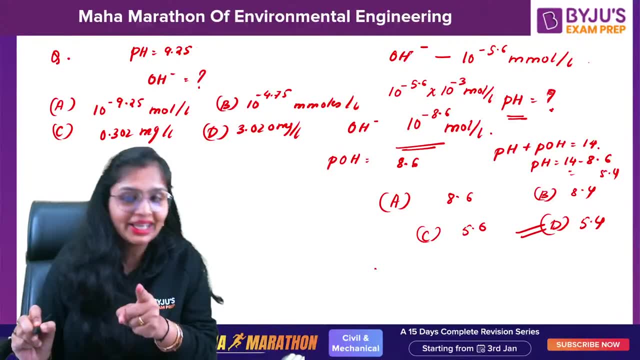 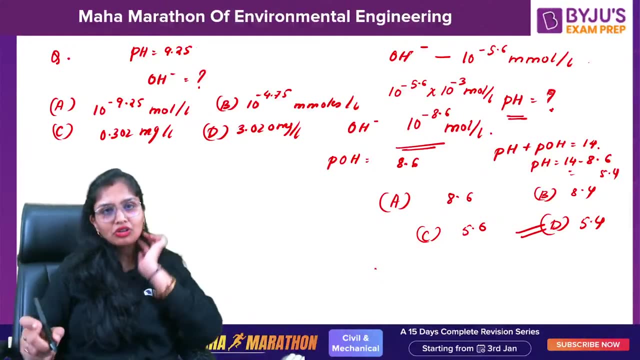 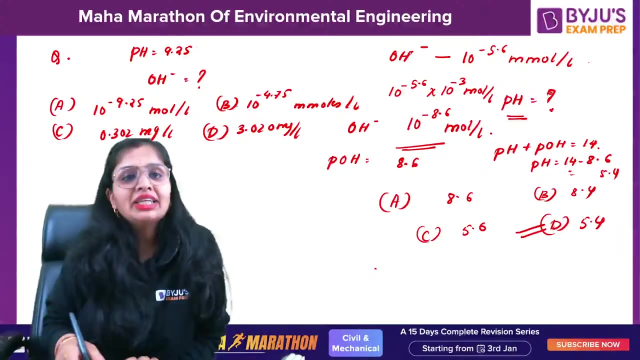 what will happen? I will take other color pen. this is an important one. this will clear your concept of molarity. no, wrong, wrong, wrong. everybody giving the wrong answer. guys, wrong answer, wrong answer, wrong, wrong, wrong. see, nobody gave the right answer. come on, guys. Arun Sagar, everybody gave me the correct answer. now see this question. 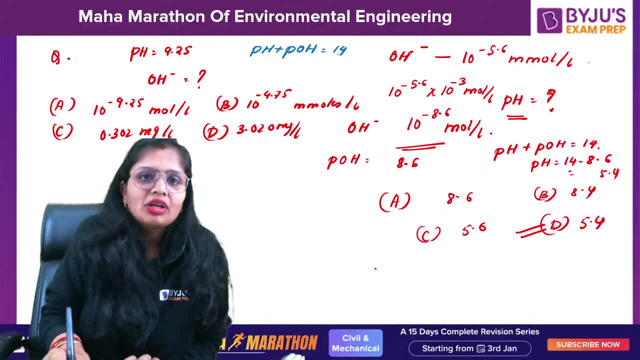 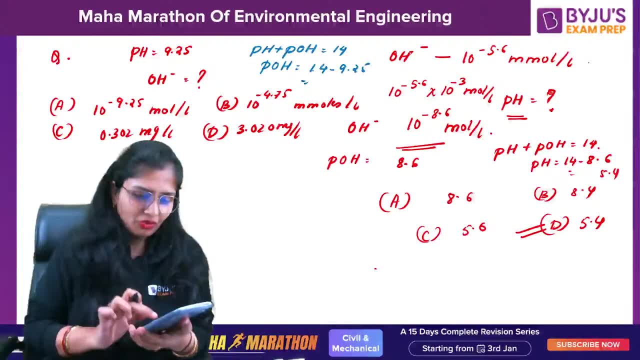 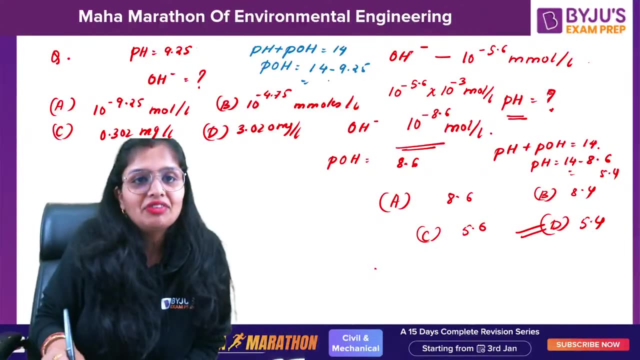 calculate POH. pH plus POH is equal to 14, so what will be POH? that will be 14 minus 9.25, how much it will come 14 minus 9.25, 4.75,. guys, if you check it out it is written mm. millimoles is written so technically. you know what it is written: 10 raised to power minus 4.75 into 10 raised to power minus 3,. 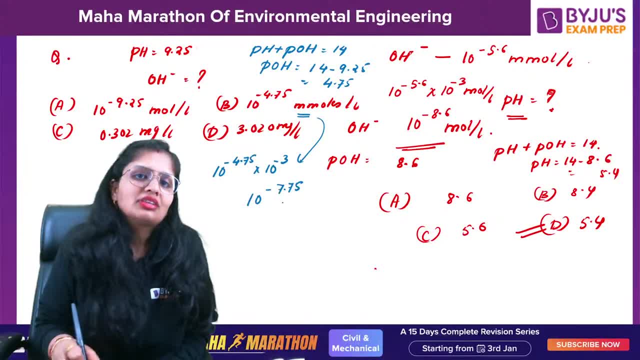 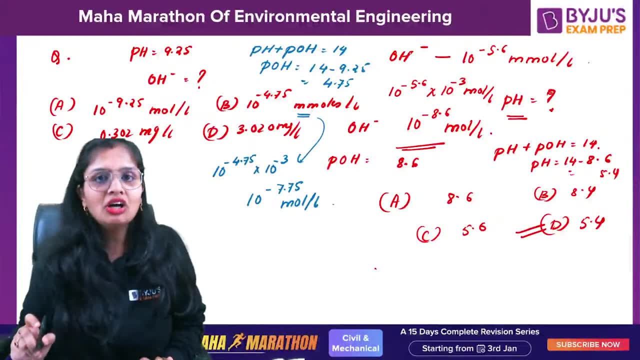 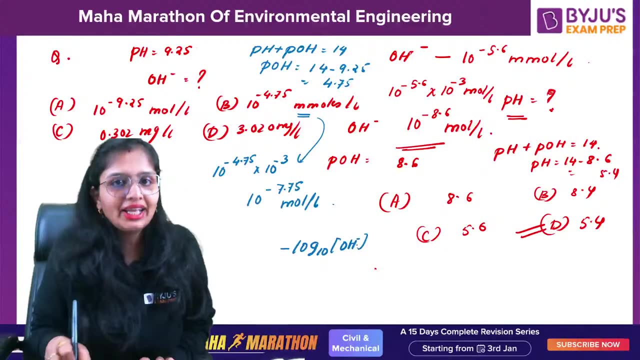 so it is written: moles per liter. this is written in the question, so is it coming? no, it is not coming. this is the POH and if you mention minus log base 10, OH minus iron, this is practice, this question before you go for the gate examination. this has already been asked. no option like this is being given in the question, so just check it out. 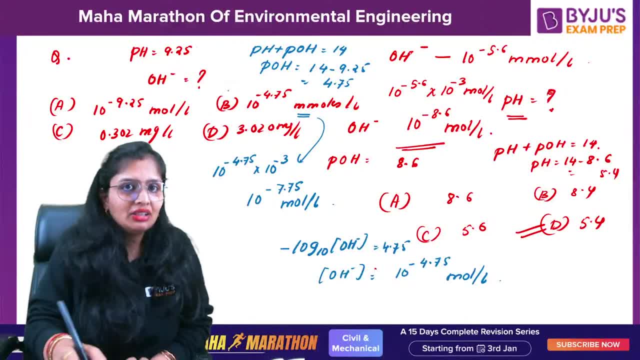 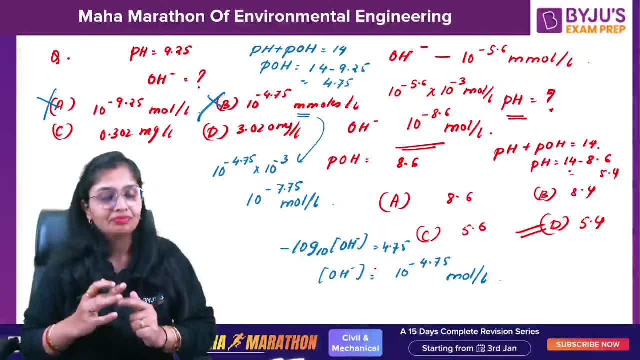 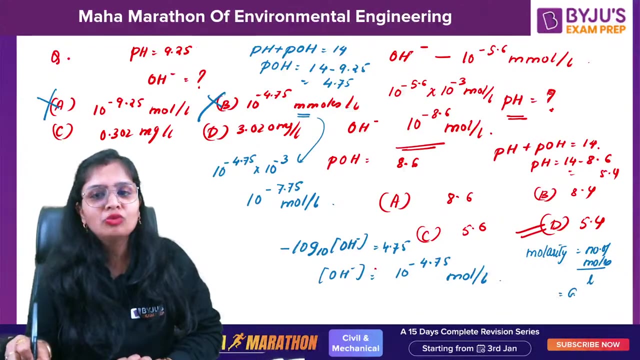 unit ray dikh raha tha millimoles per liter. toh ye bhi galat. this is wrong. this is wrong. now comes the next one. just check it out. you know that molarity. molarity means number of moles per liter. okay, so number of moles means given weight upon molecular weight. 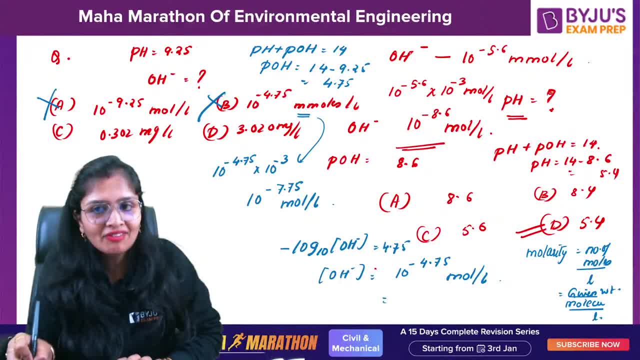 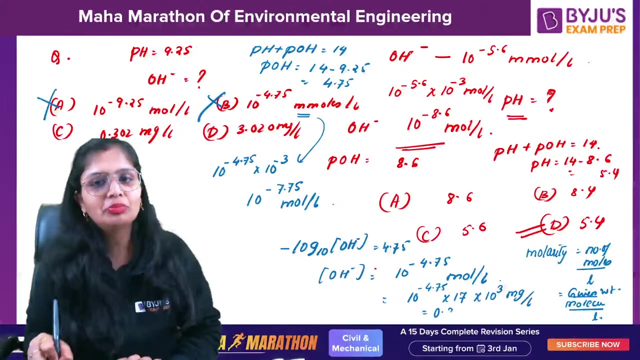 liters. so if I multiply with the molecular weight, molecular weight of OH is oxygen 16 and H plus is 17,, 17,. okay, this will come out to be in gram per liter. for getting it in milligram, I will multiply by 10, raised to power 3, what you will get. what you will get: 0.302 mg per liter. 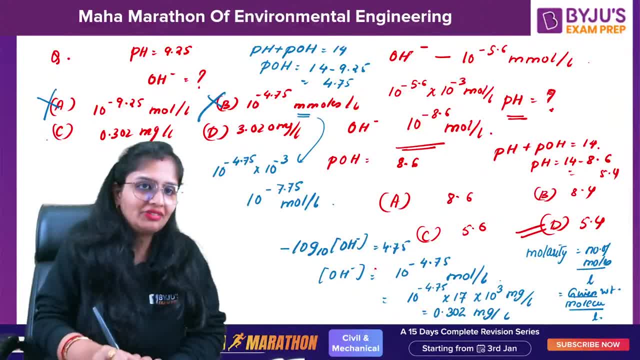 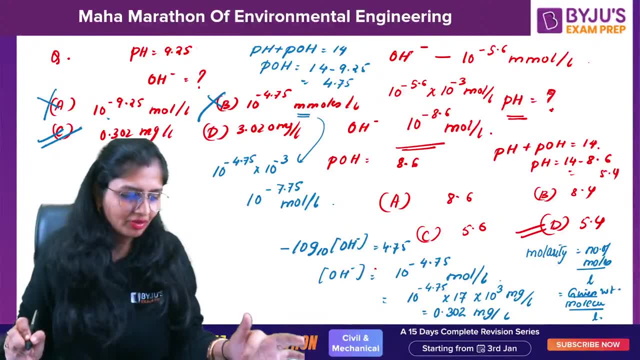 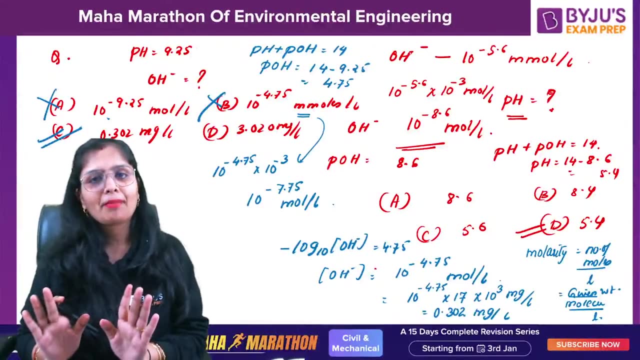 so option C will be the writer. clear those who were telling the wrong answer. Prashant MBS was telling it correct, clear. so this question, practice it and go clear. Tiksha, okay. so these are the questions regarding pH which you need to know. 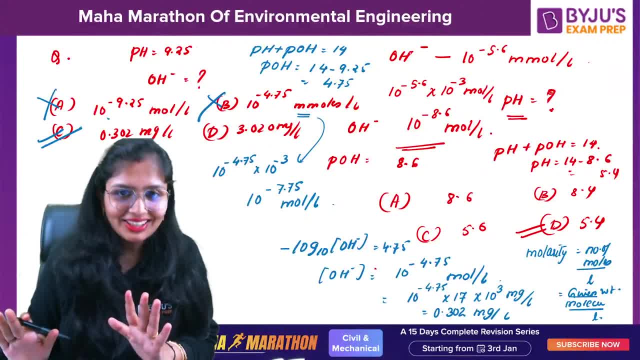 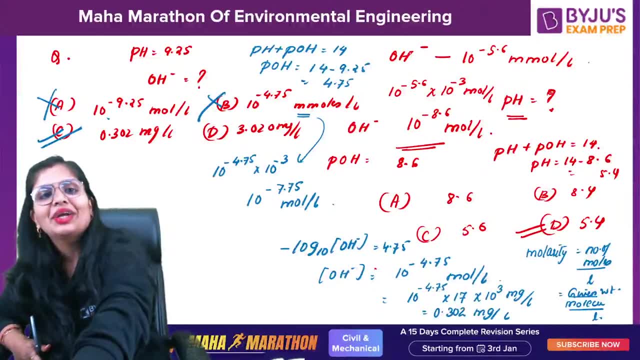 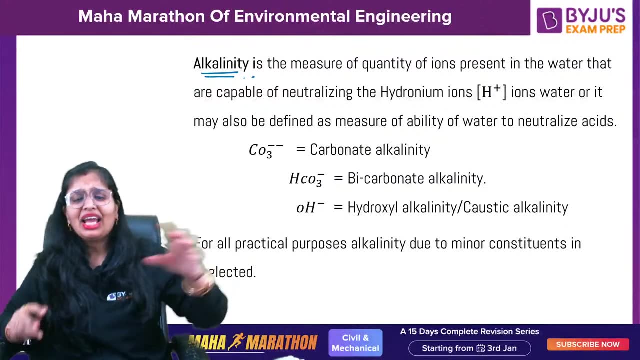 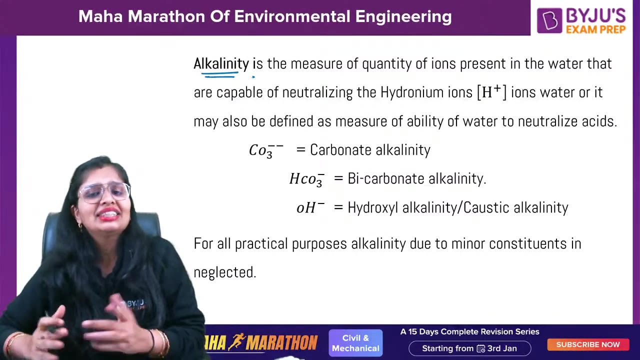 17 ko ratta mar le. 17 ko ratta mar le. okay, beware of trap. correct, correct, Ayaan. okay. so now coming to to alkanity. now, what is alkanity? alkanity is basically we say there are certain ions which are present in the water, which neutralizes the H plus ions? 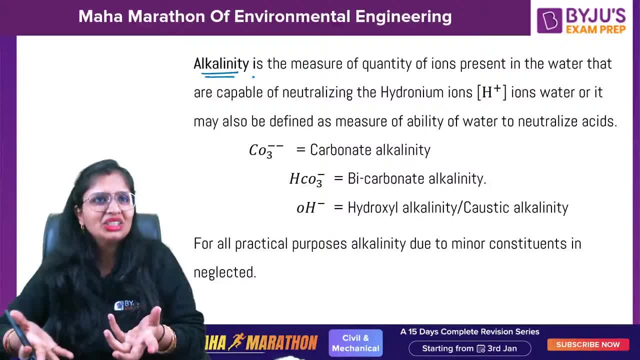 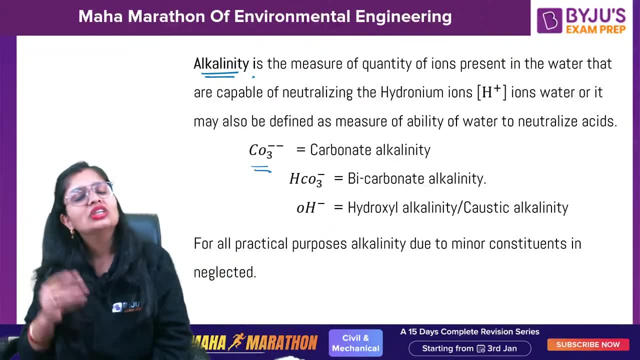 okay, or you can say: H plus ions means what? these are the acids. so in water there should be some other elements which should be present, which should neutralize acids. now, if the carbonate ions are present and it neutralizes acids, so alkanity due to carbonate ion is known as carbonate alkanity. 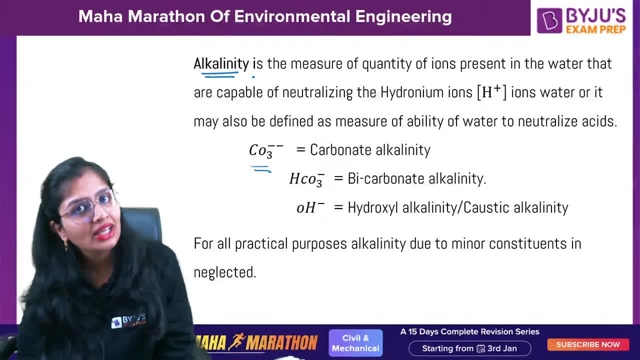 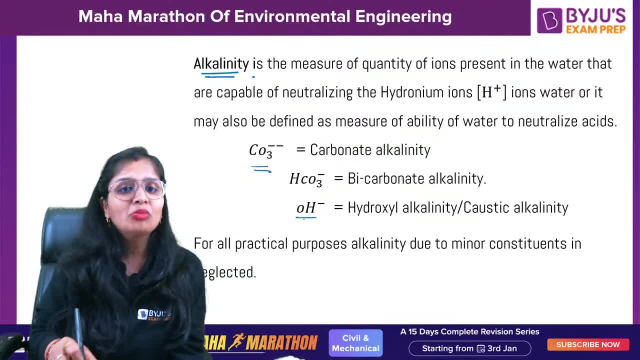 alkanity due to bicarbonate ion is known as bicarbonate alkanity. alkanity due to caustic ion is known as hydroxyl or caustic alkanity. okay, there are more alkanity also, like HPO, 4, 2 minus. 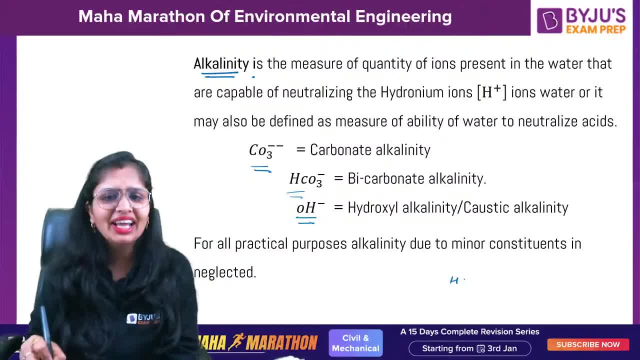 H2PO 4 minus bivourette ions, sulfide ions and number of ions are there. remember very, very important thing. I'm telling you: if in the quotient, if in the quotient, wait I'll explain you. molarity, normality, prashant pranun. 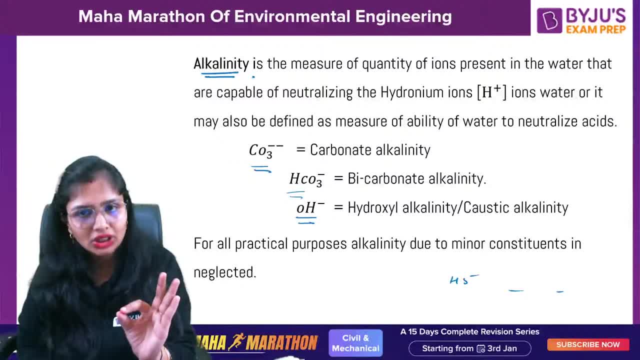 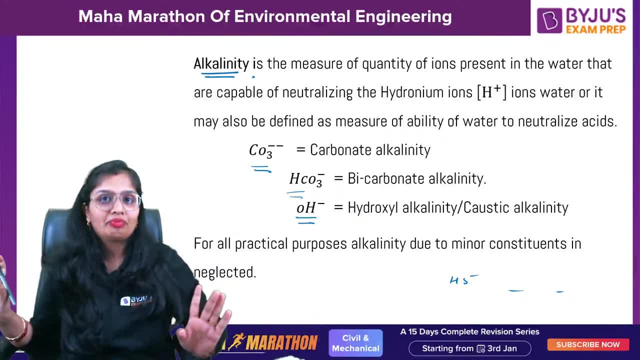 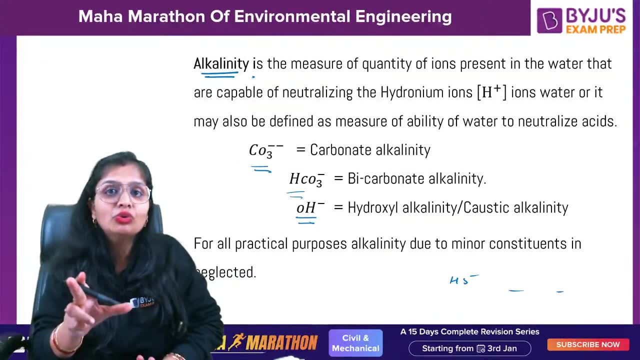 I'll explain you right after this. if in the quotient it is not telling you to take the minor alkanity, don't take it. don't take it until and unless mentioned. if they have mentioned in the quotient and they're telling you neglect the effect of it, 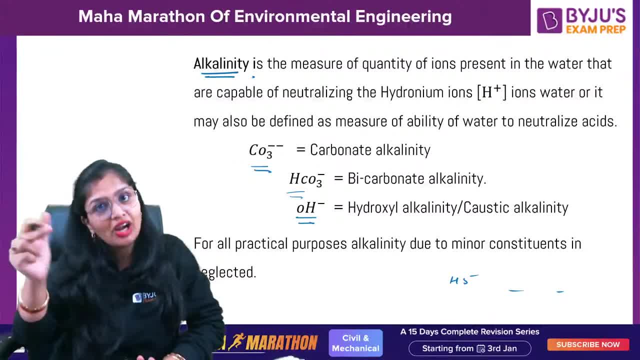 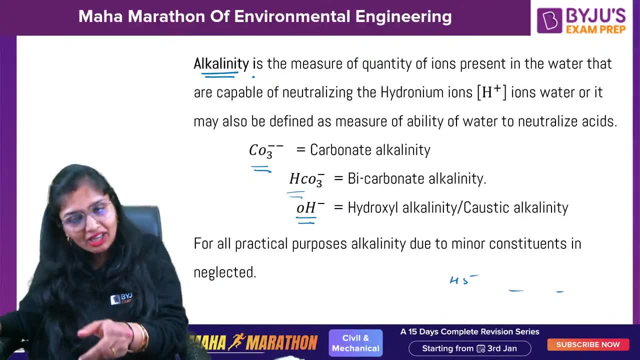 neglect it. but if they haven't mentioned anything, then you have to consider. this happened in the case of hardness. maximum students did it wrong. that's I'm telling you. if any other alkanity is mentioned, you in the quotient and it has not written anywhere, neglect the effect of it. 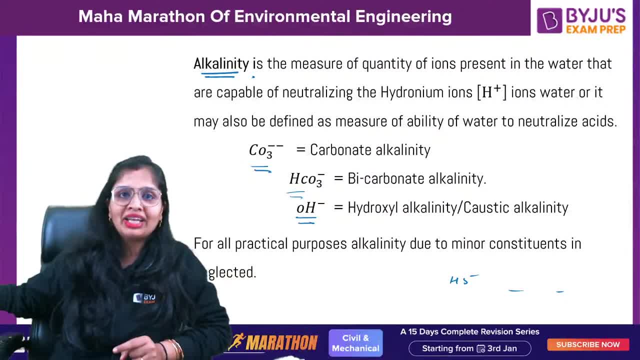 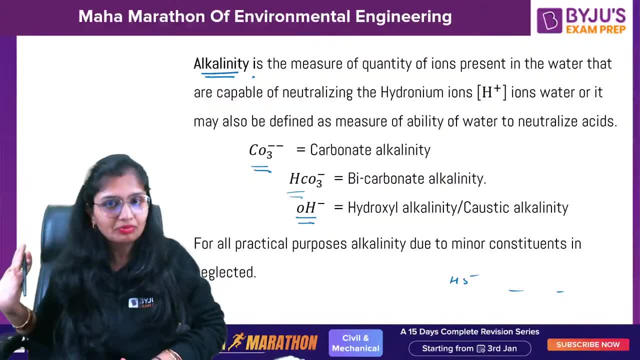 you have to consider it. don't say that, ma'am. you told it is minor alkanity. of course it is minor, but if in the quotient it is asking you to consider it, you have to consider it. okay, this now comes next. 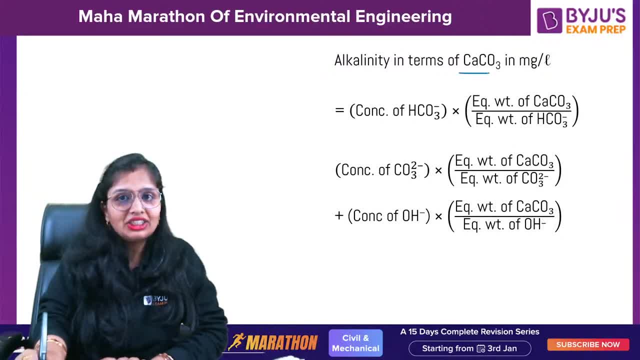 now comes next. if you want to calculate generally, it is due to bicarbonate carbonate and OH minus N. the best ways: concentration: take it in mg per litre. okay, take it in mg per litre. equivalent weight of calcium carbonate divided by the equivalent weight. 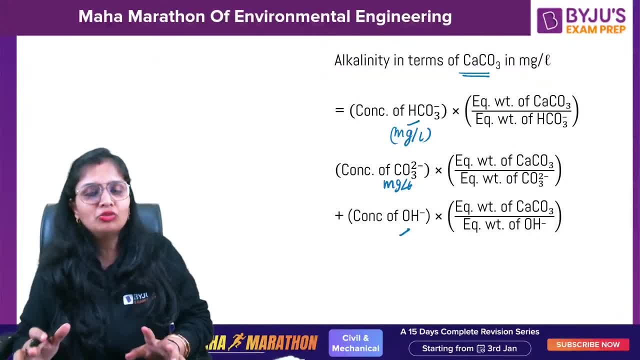 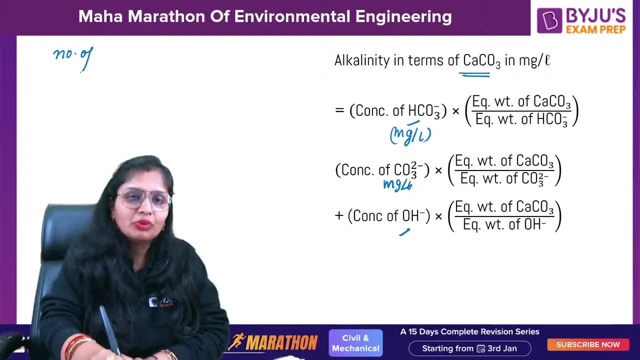 now I have to tell you few things before we move towards this. now everybody was telling me. let me tell you first of all, let me tell you number of moles quickly. number of moles, if you want to calculate. 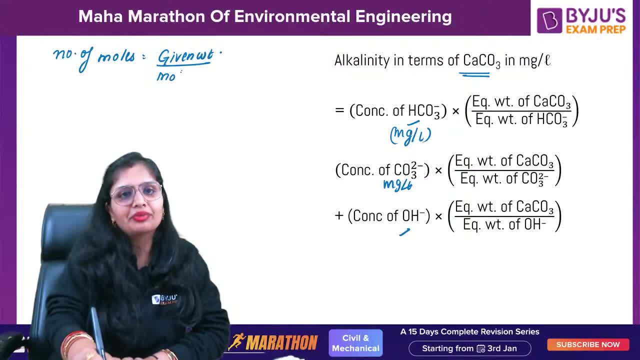 this is given weight by molecular weight, molecular weight in the quotient. they will give you the atomic weight. so generally, don't worry. now if you talk about another thing, that is, molarity, molarity generally in the quotient, you will see, they will denote it by capital M. 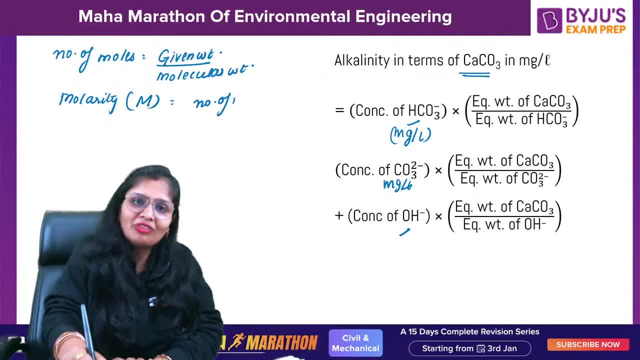 molarity is number of moles present in 1 litre of the solution. so I have done this only normality. if you talk about before that, you have to understand one thing: gram equivalence. now what is gram equivalence? that is equal to given weight by equivalent weight. 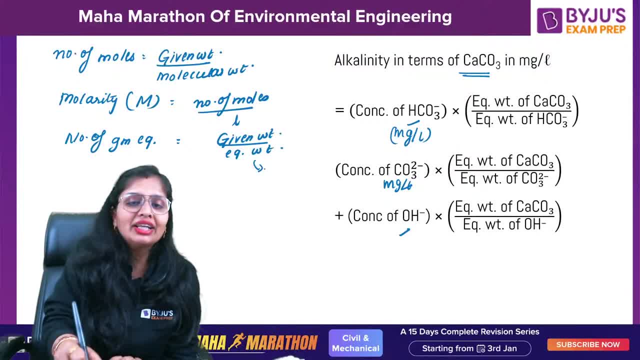 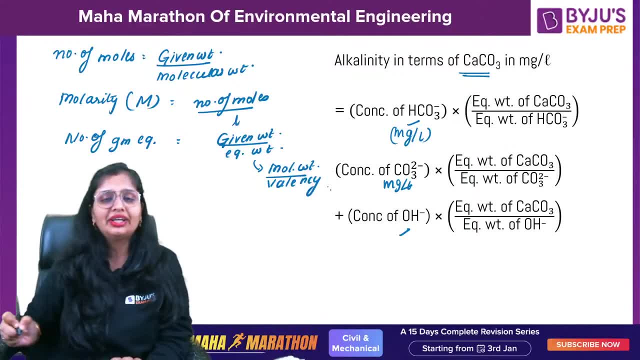 now, what is equivalent weight? equivalent weight is molecular weight by valency. you guys know this, otherwise if you don't, then I will deal it in slight detail. so equivalent weight is molecular weight by valency. valency means combining power of an element. 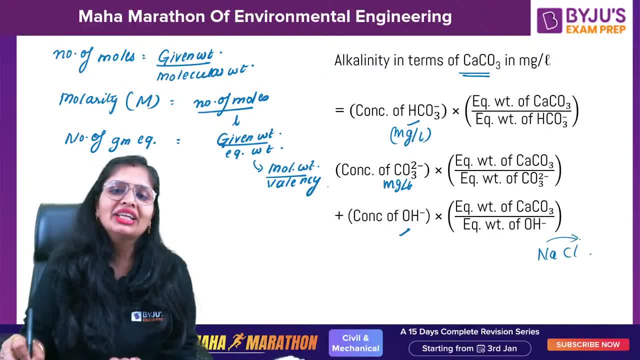 example, if sodium chloride is there, sodium will give its 1 electron to achieve the octet. chloride will take 1 electron to achieve its octet, so the valency of NaCl will come out to be 1,. similarly, remember you don't need to mung up for everything. 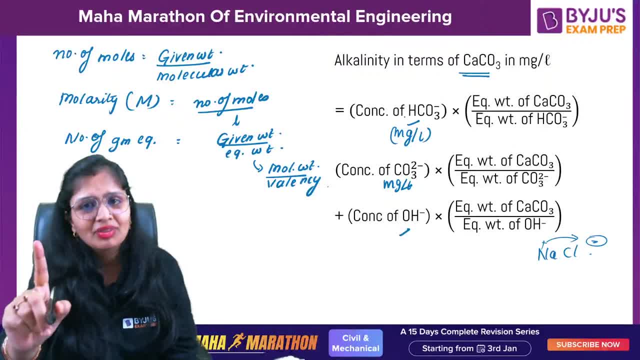 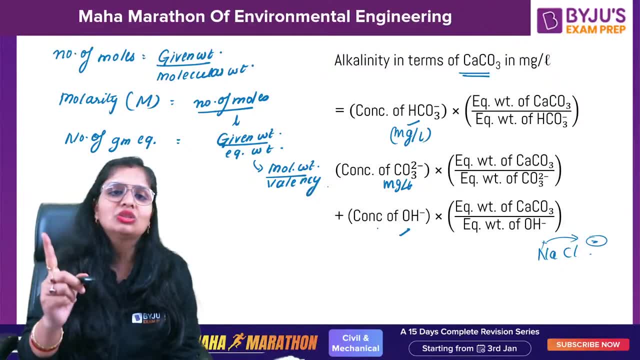 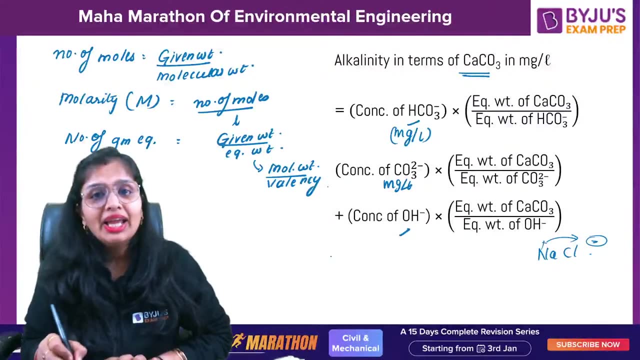 only 3, carbonate valency is 1, bicarbonate valency is 1, carbonate valency is 2, and caustic valency is 1, so you don't need to remember for every other thing. now there is one concept which you need to know. 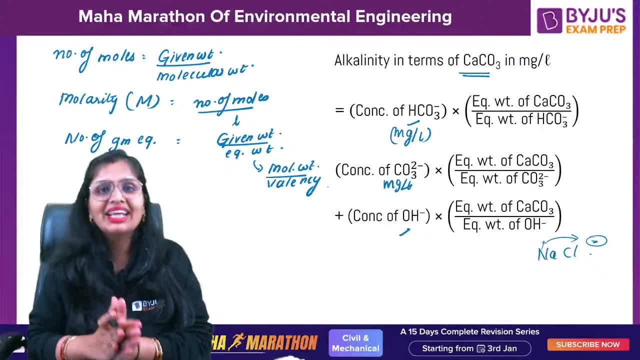 it is not possible. see, when you add 2 things, if you want to add kg and mg, or if you want to add rupees and dollars, either you have to convert dollars into rupees or rupees into dollar. so what happens is: 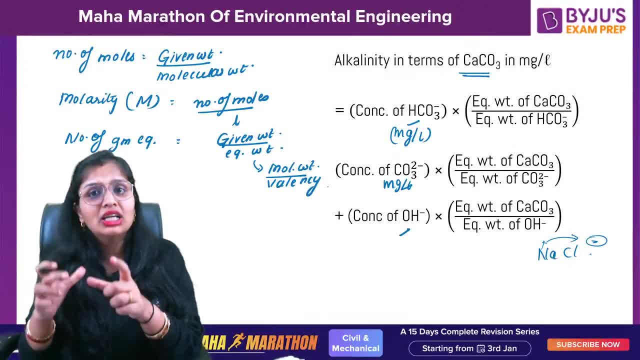 what happens is you have to make it in a common parameter. similarly, if you want to add HCO3-, CO32- OH- you cannot add it directly. so what we do? take the help of calcium carbonate. why? because there is a funda. 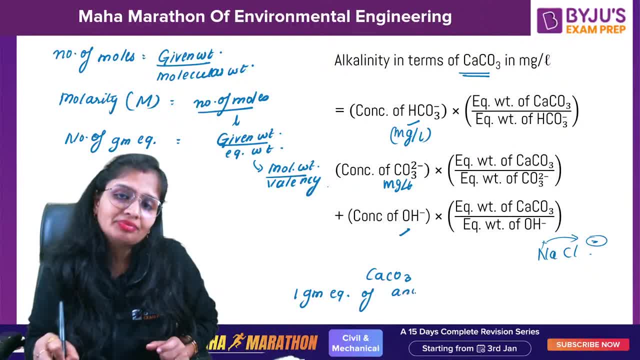 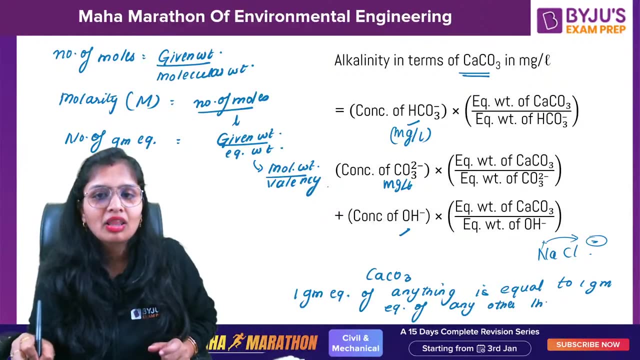 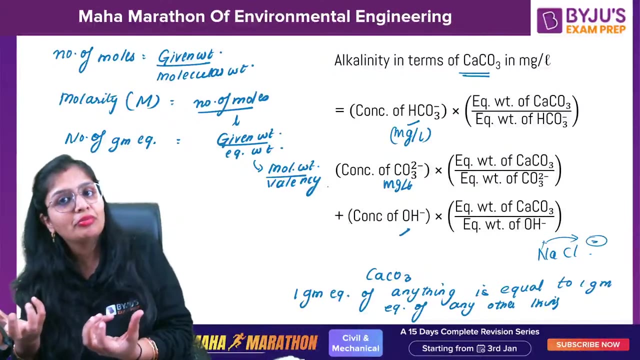 1 gram equivalent of anything is equal to 1 gram equivalent of any other thing. so how many gram equivalents of HCO3- will be there, that much gram equivalents of calcium carbonate will be there. that how many gram equivalents of CO32- will be there. 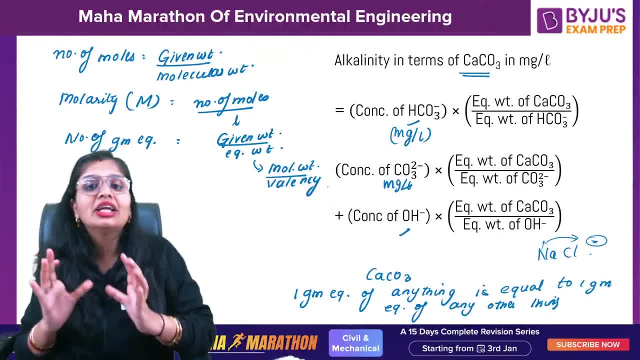 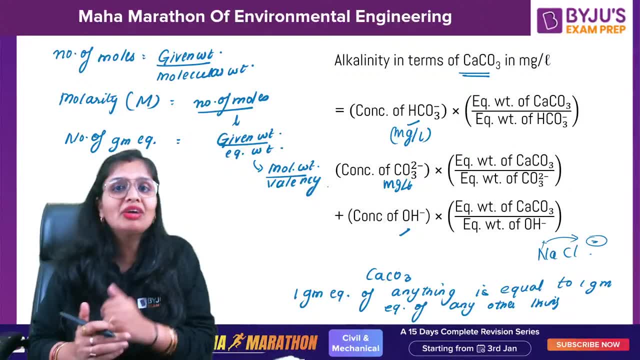 that much gram equivalents of calcium carbonate will be there. so, in this manner, what we do, we report every alkalinity in terms of calcium carbonate. now you will say, ma'am, why calcium carbonate? because its molecular weight is 100,. 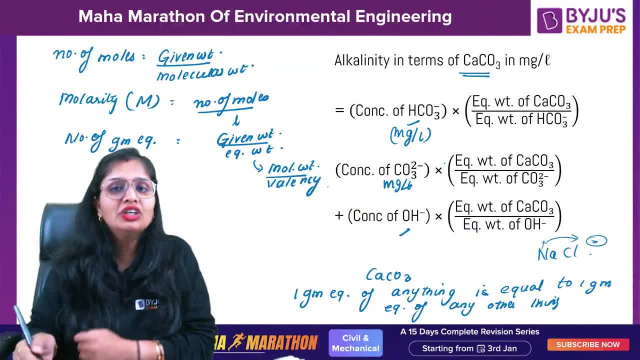 it is easy to use. that's the only logic. so first we calculated the gram equivalents, so HCO3- divided by equivalent weight, this will give me the gram equivalents of HCO3-. then I will multiply by the equivalent weight. 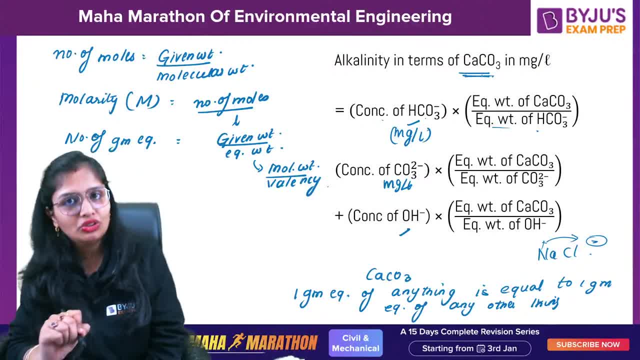 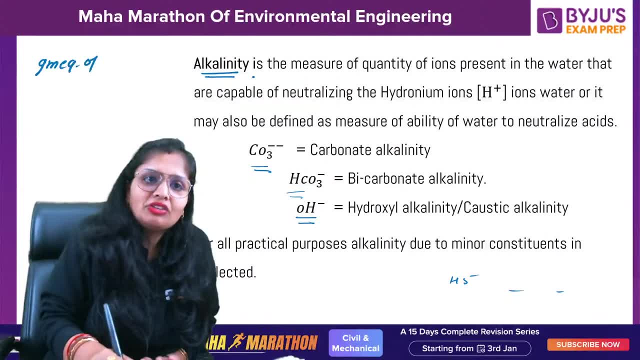 for getting the concentration of CaCO3-. that's very much simple. if you want, I can tell you gram equivalents- common sense gram equivalents of HCO3- is equal to gram equivalents of calcium carbonate. so what I did. 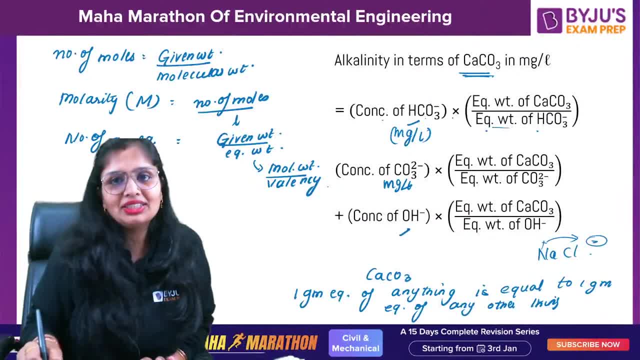 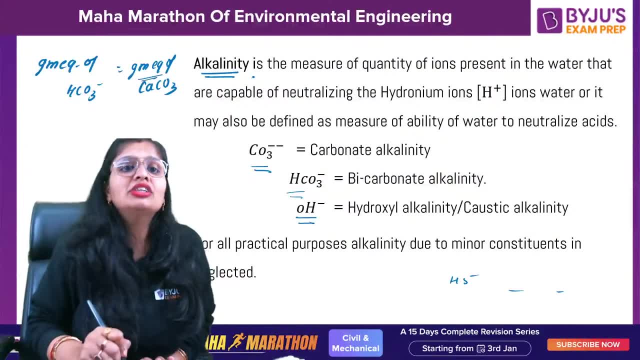 I calculated the gram equivalents. this is the gram equivalents. this divided by this, this will give me the gram equivalents. so here I don't want the gram equivalents of calcium carbonate, I want the concentration. so if I want the concentration, 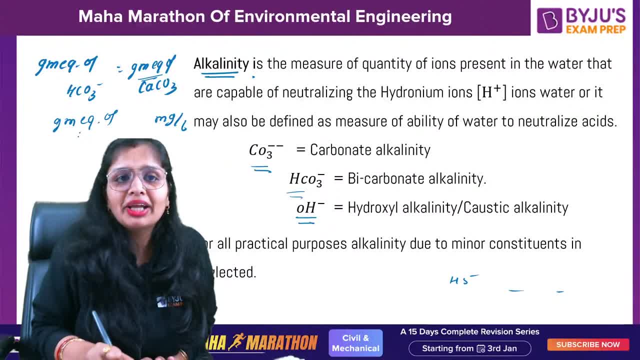 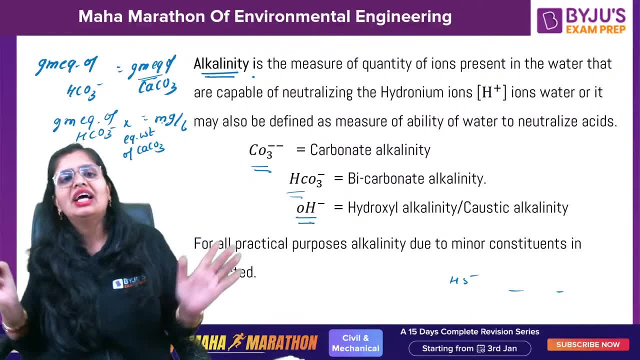 I just gram equivalents of HCO3- whatsoever I got. I multiplied with the equivalent weight of calcium carbonate for getting the concentration. that's simple as that. so how many gram equivalents was there? that much gram equivalents of calcium carbonate was there. 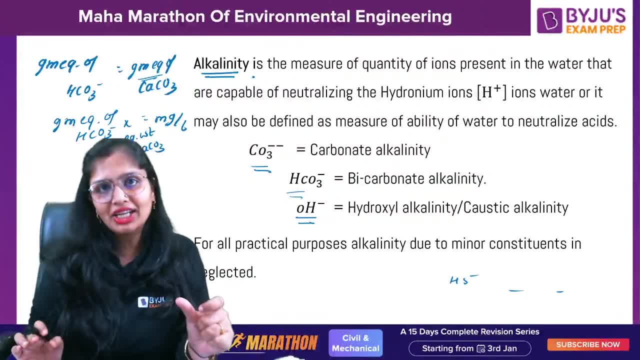 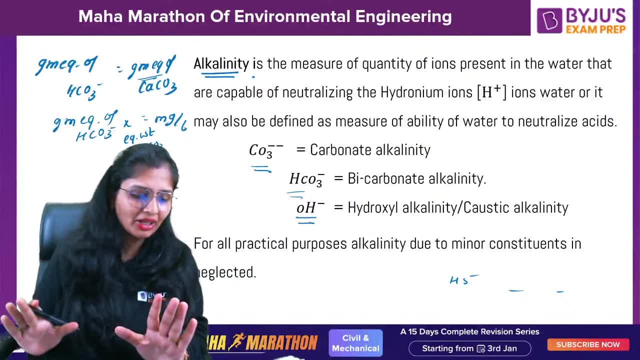 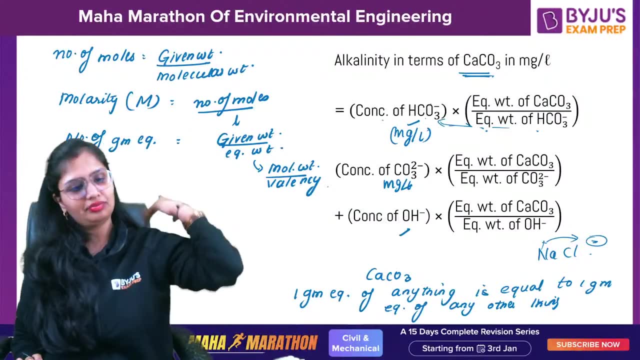 but in the portion it doesn't ask me, in gram equivalents of calcium carbonate, so I multiply with the equivalent weight of calcium carbonate. clear, understood, Prishant Barnod, understood molarity and everything. if not, tell me fast. 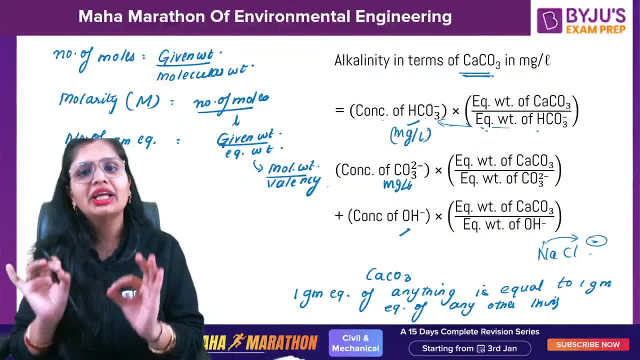 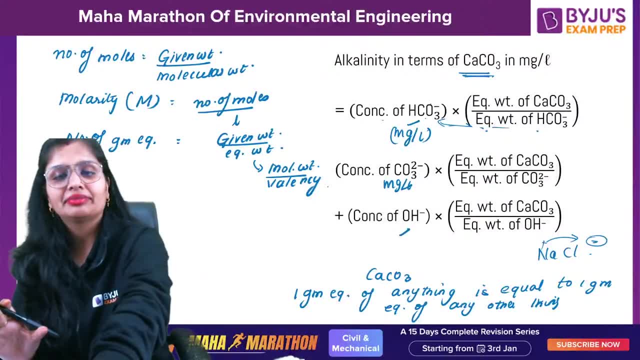 understood if, in the question, any of the alkalinity is not given. don't consider it yourself. take it as zero. take it as zero, as simple as that. okay now, acceptable limit and cause for rejection limit. if I talk about 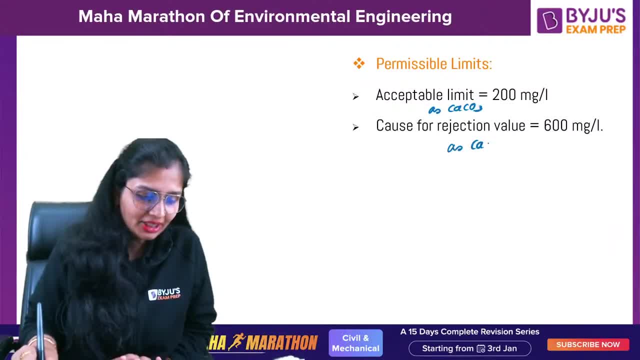 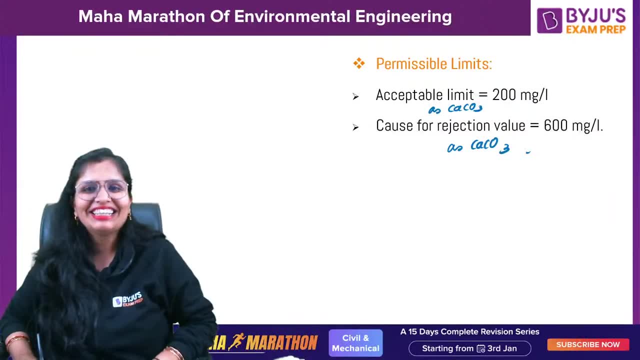 this is also as simple. this is also as calcium carbonate, as calcium carbonate. now, Arun, you hurt me, you love me. what kind of love is this, tell me? okay, just kidding. acceptable limit: up to 200 mg per liter. 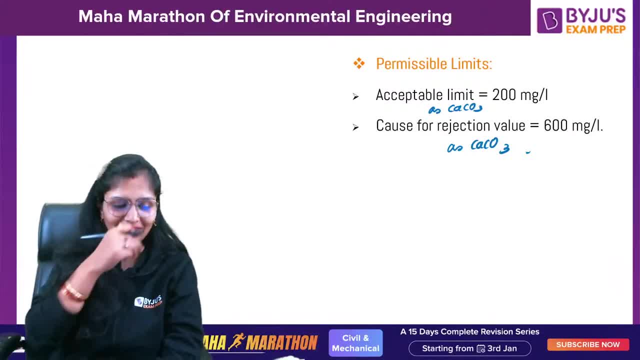 it is acceptable and cause for rejection limit when there is no alternate source available. up to 600 mg per liter is the cause for rejection. okay, showing pole. what is the pole showing? okay, so this is the cause for rejection limit. 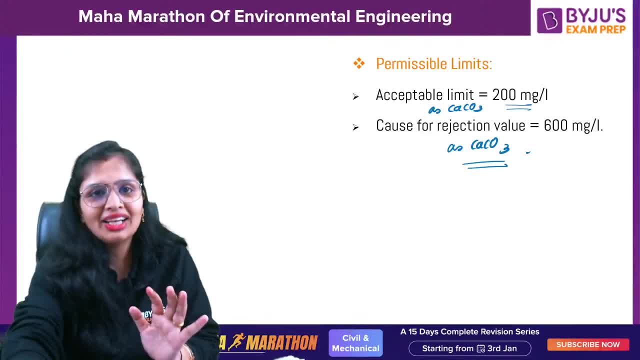 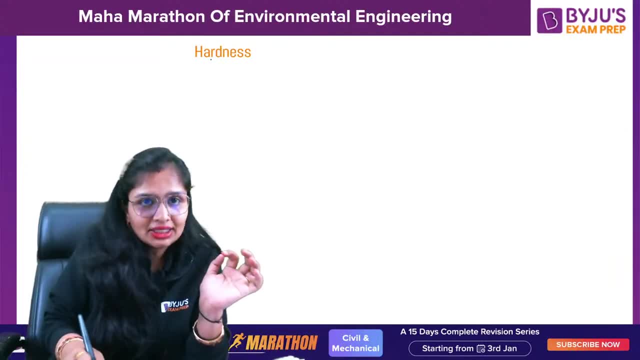 okay, so this you should know, and let me talk about hardness, then we will deal the questions. I am interested now. hardness is due to presence of multivalent cations. this is, this is so like and like. 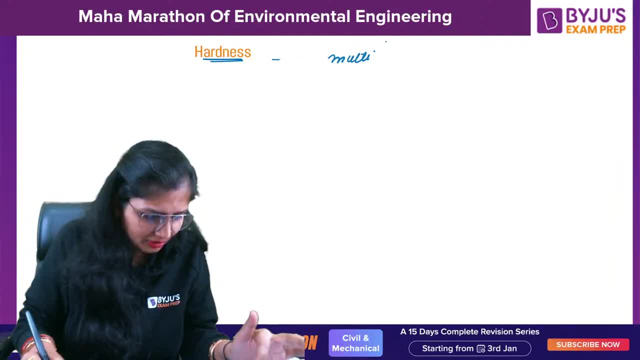 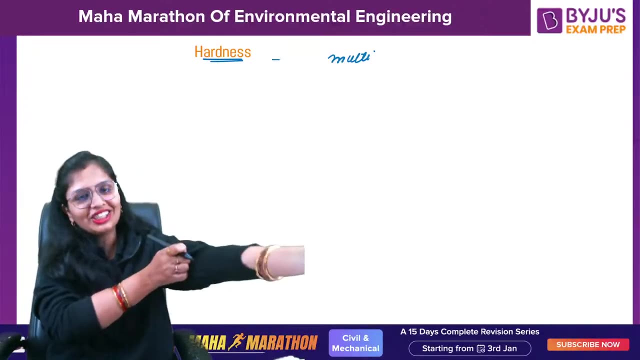 there is a play already, can you not see? ok, you have not punt your like now. now many people who have checked 70 plus and after that also have not like 90, operator are telling them: now do it. 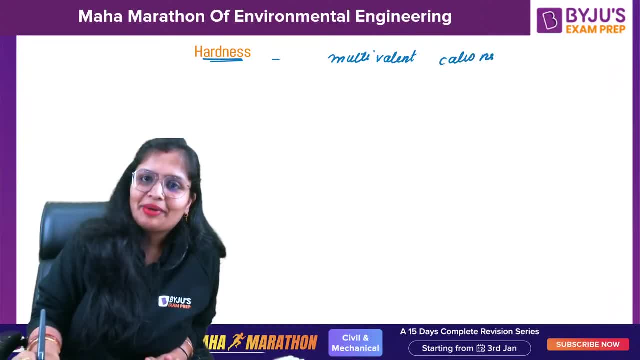 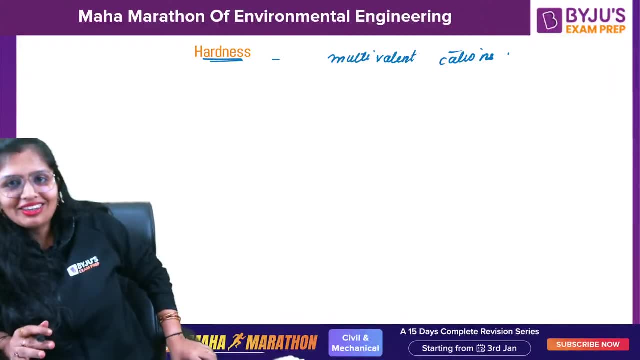 now you don't like to talk to me еще? alright, it is the case of hardness. What I am saying is coming from my side, from your side, ma'am. I am not doing anything. So you guys See, 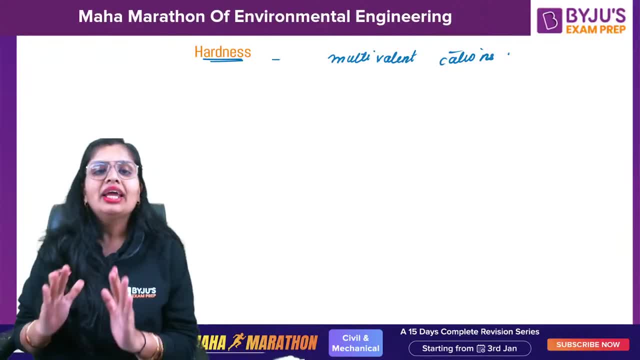 What is hardness? What is hardness That? What is hardness? That whenever We have to talk in English, If you write comments in Hindi, I will start speaking in Hindi. Hardness is whenever multivalent cations is present: Multivalent means. 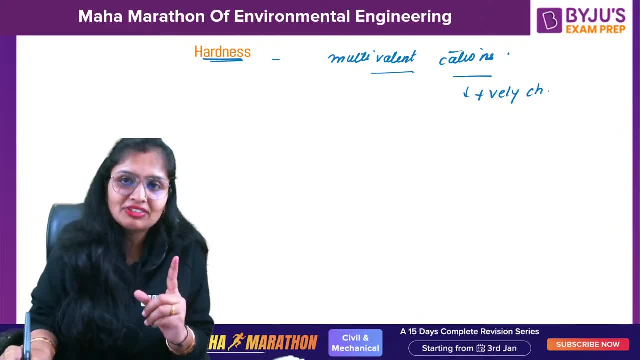 Cations means- Remember this is very important. I will tell you where you guys will make mistake- Cations means positively charged ions. Positively charged ions Multivalent means valency more than 1. So those cations which have a valency. 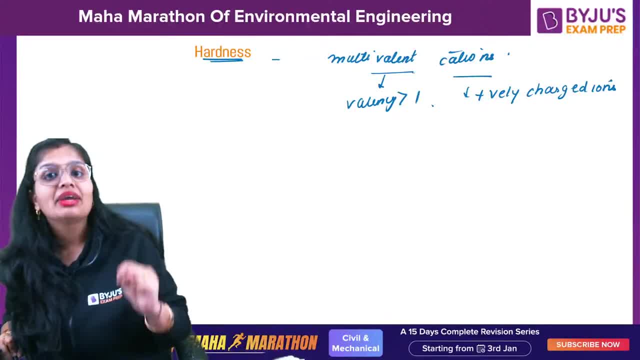 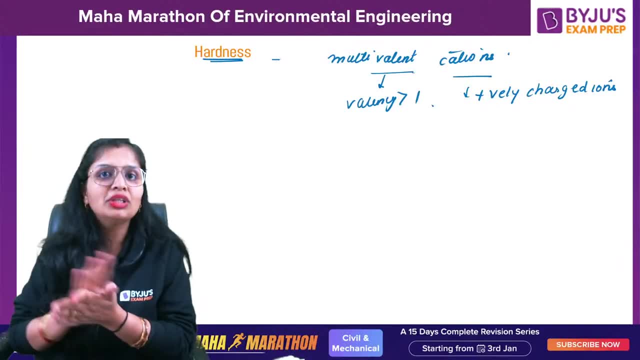 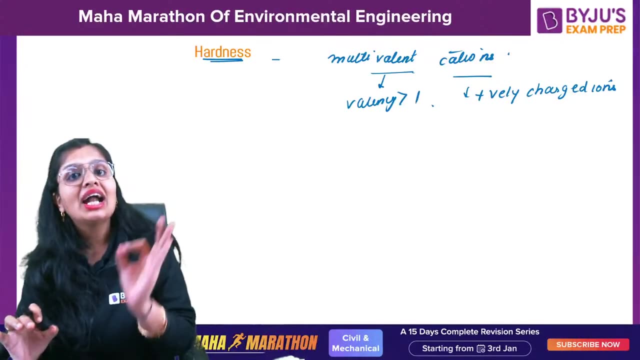 more than 1, they will impact hardness Firstly. Secondly, hardness is what Hardness is whenever you say that the water is hard And when you rub the soap, It doesn't produce foam rather than it produces precipitate. Okay, So you say hardness. 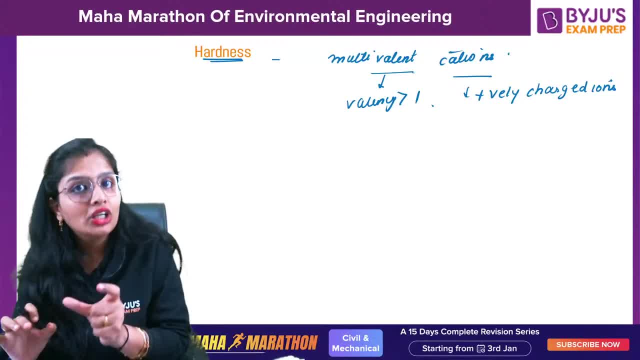 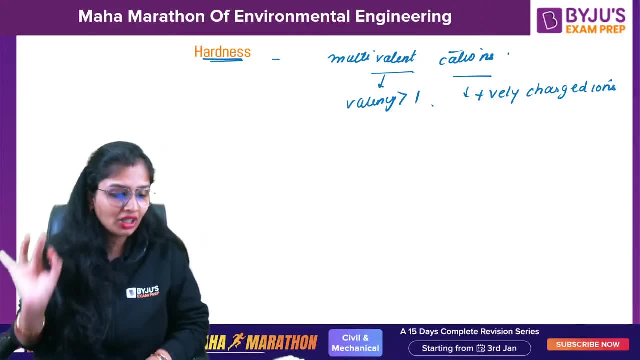 is what It destroyed: the ability of water to destroy the surfactant property of soap. This is a technical definition: Ability of water to destroy the surfactant property of soap. Surfactant property means generally, you know the water when it should be rubbed with a soap. it should. 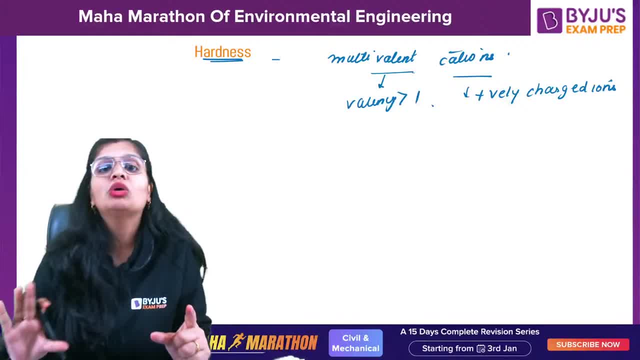 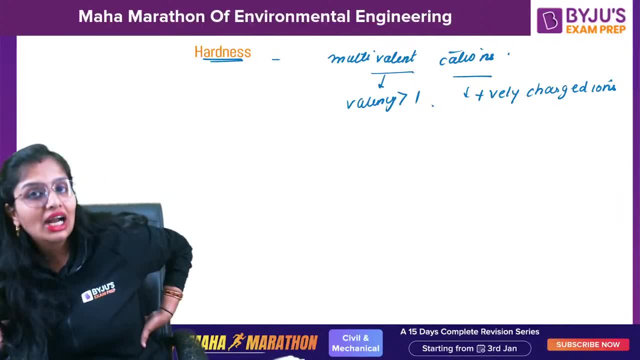 produce foam, But when it is not producing, it means that the water is hard. So, ability of water to destroy the surfactant property of soap that is known as hardness, And how hardness is caused. Hardness is caused due to the presence of multivalent. 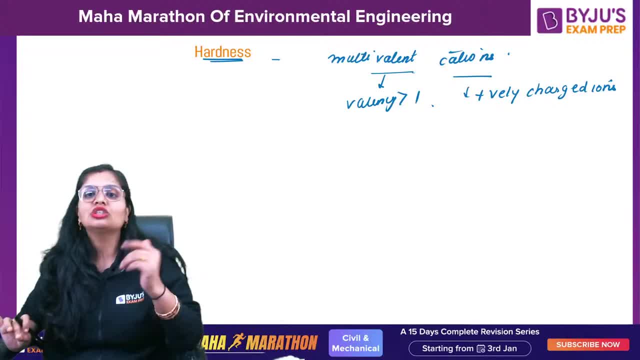 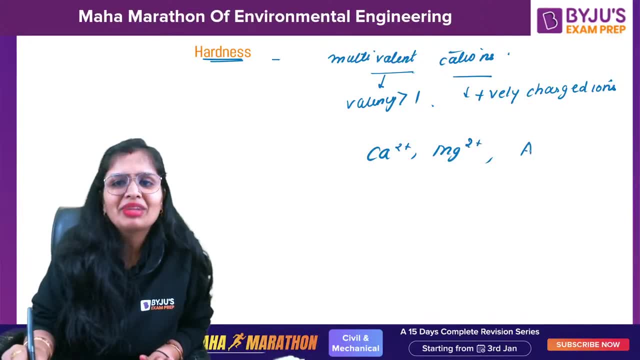 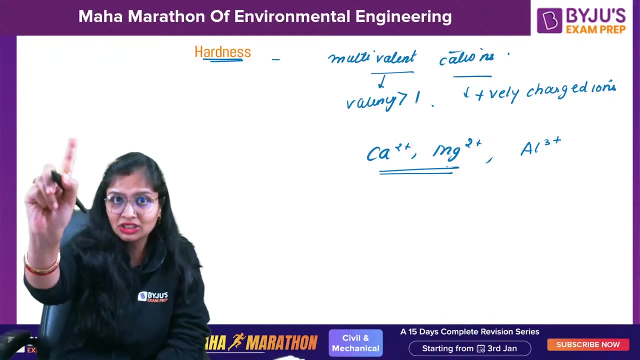 cations, Those positively charged ions whose valency is more than 1.. That means you will say: ma'am, calcium, magnesium, aluminium, etc. all will impact hardness, Yes, Everybody, But majorly basis calcium and magnesium. Again this question I. 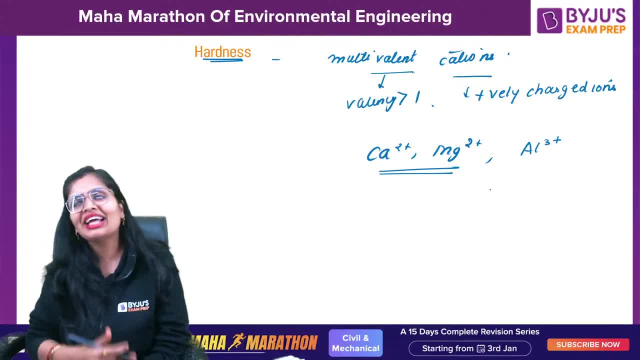 have been asked in your GATE. In the GATE question generally, every time: calcium magnesium, calcium magnesium. you will give the test series. you get calcium and magnesium only. But in that year paper aluminium was also given And maximum students didn't consider. 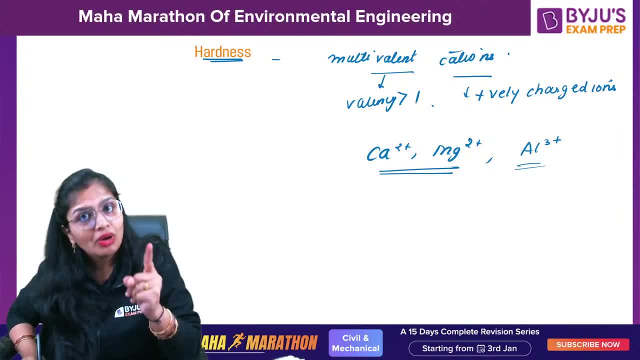 it Clear, But you have to consider it, Although you know that the concentration is negligible. But if in the question it has not mentioned neglect the effect of it, you have to consider. Okay, So that is the reason you have to consider. 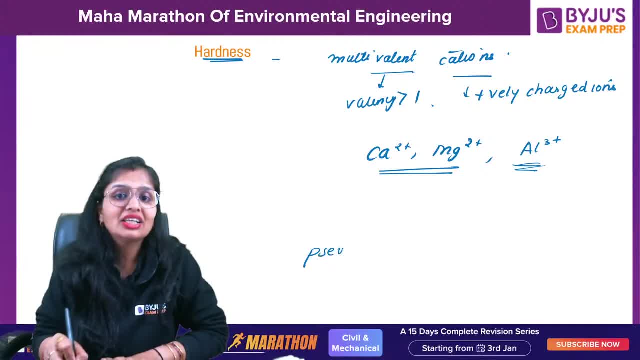 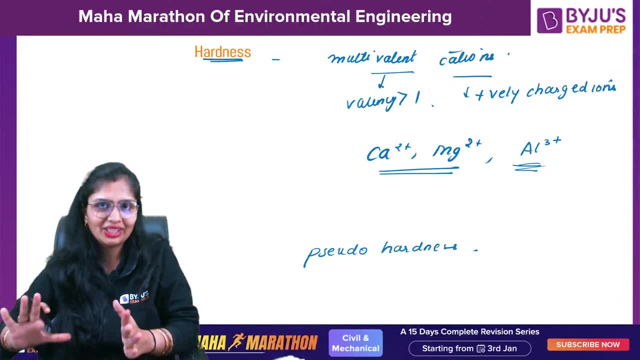 Now there is a one term: pseudo hardness. There is a term pseudo hardness Technically, let me tell you there is nothing like pseudo hardness. But what generally, in books, what is written? I will tell you The elements which does not impart hardness: they impart pseudo. 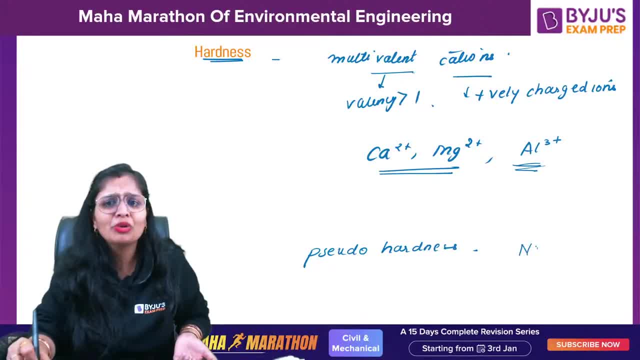 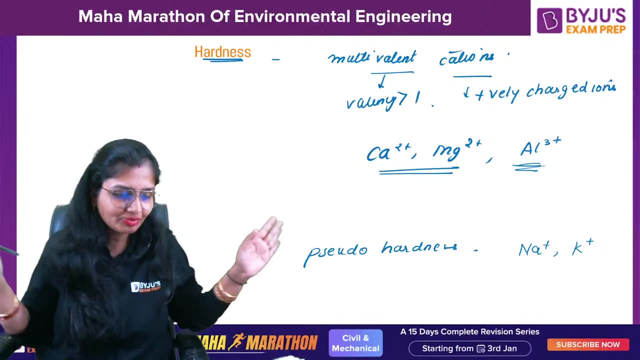 hardness. Any common sense, Like sodium, potassium, Why, Although they are cations, but they are univalent, Because they have one valency. So those elements which does not impart hardness, they impart pseudo hardness. That's it, No other logic than that. 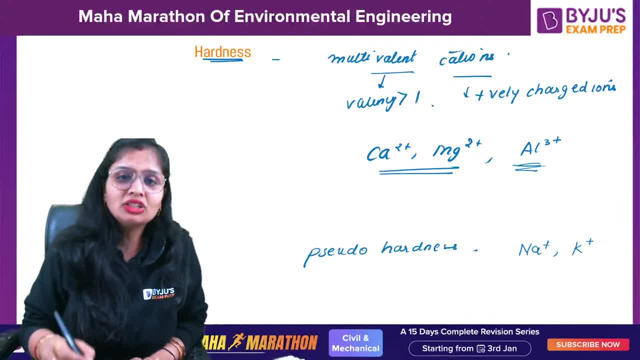 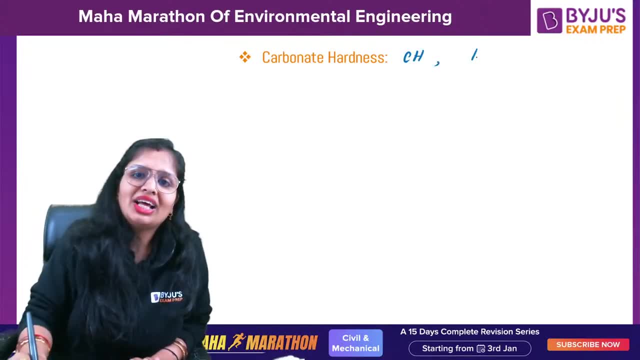 Okay, So this you should know. Now, in hardness also, we have two types. One is what? Carbonate hardness? Another one is non carbonate hardness. Carbonate hardness is known as temporary hardness. Why? Because by simple boiling or you add lime, they are being 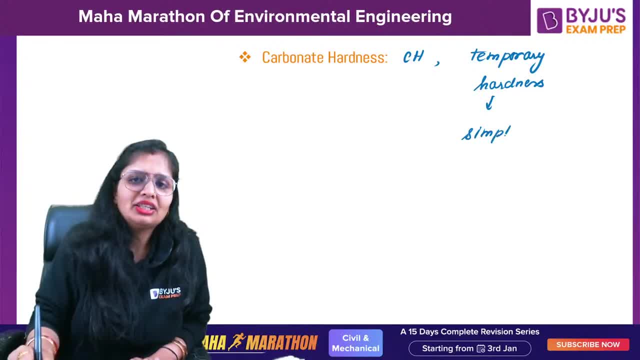 reduced. So simple boiling, no need to apply more brain. Simple boiling or by addition of lime. they are being removed. Okay, Now, if any carbonates? Now, this is the thing maximum. students get confused. I will tell you one thing and this I will explain you. 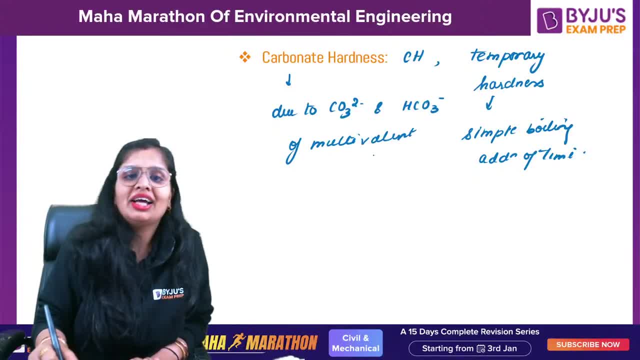 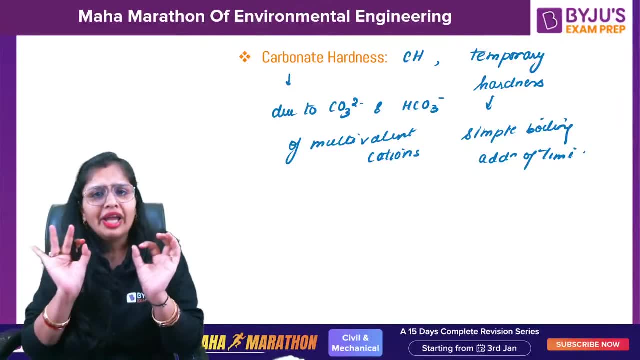 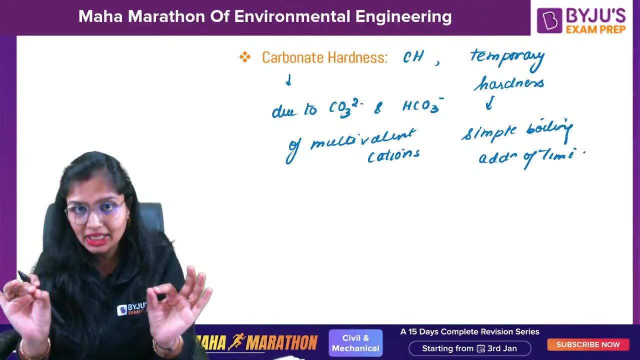 with the help of a numerical also, Because I know whenever I ask this, in offline and online, maximum students make mistakes. That's why I am stretching this out, Remember every time. this should go in your head. hardness is always and always due to multivalent cations. 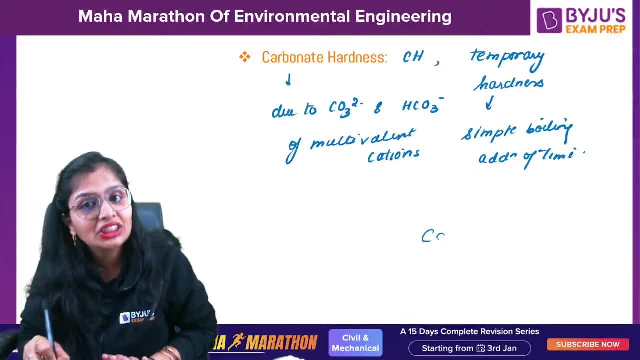 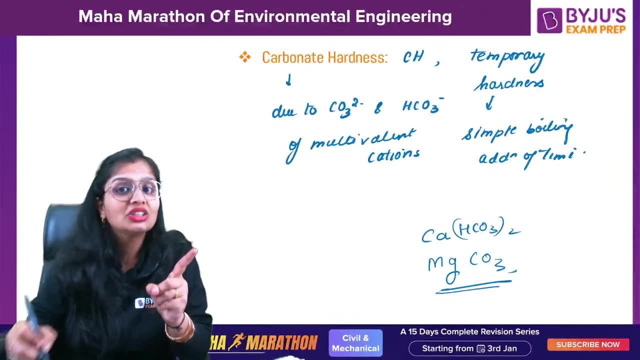 If the suffix of it Calcium and magnesium are the one which will impart hardness. But if the suffix of it is bicarbonate or carbonate, then you will call it as carbonate hardness. But that doesn't mean that hardness is due to carbonate and bicarbonate. 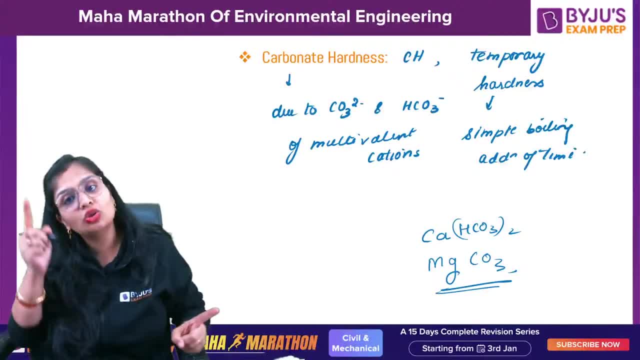 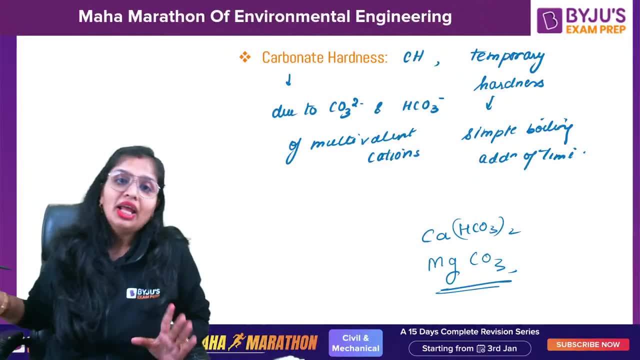 Never, never, never. Hardness is due to multivalent cations, that is, calcium and magnesium Clear. So this you should know. Now, if I talk about non-carbonate, and you can see it also, If you want, you can see it also. 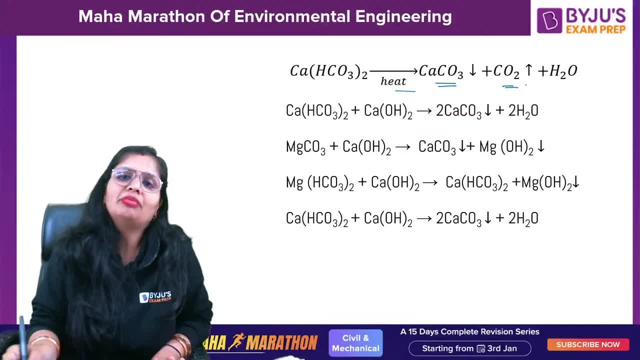 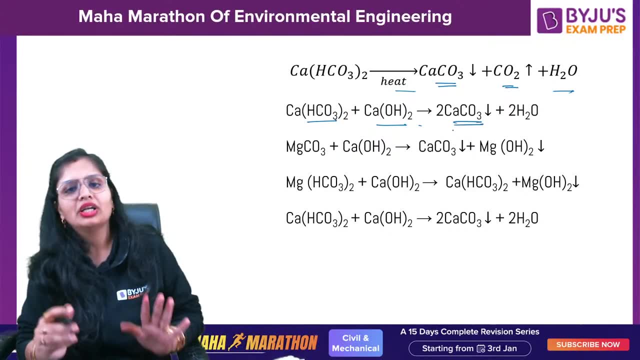 Calcium bicarbonate. heat it, you will get calcium carbonate, carbon dioxide, water, Calcium bicarbonate- you will put lime in this Calcium hydroxide, you will get calcium carbonate. So, in this manner, either add lime- Okay, we have added here, It is slaked lime- or quick lime. 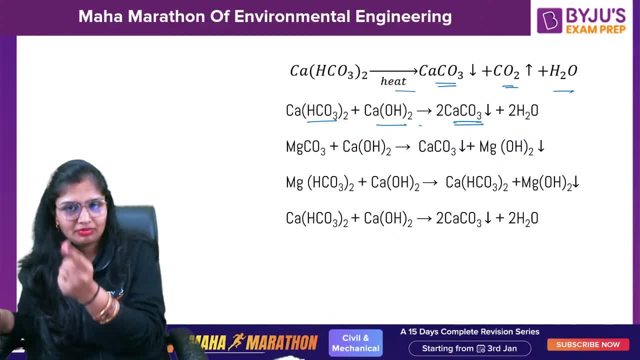 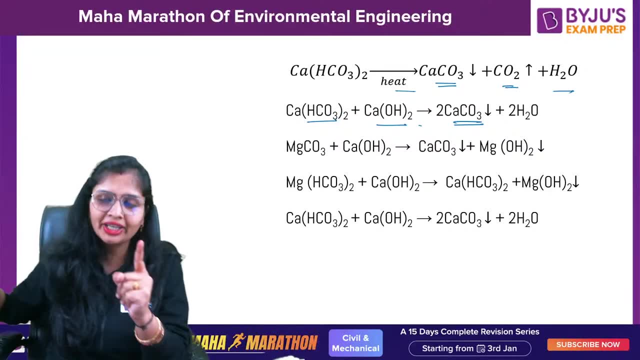 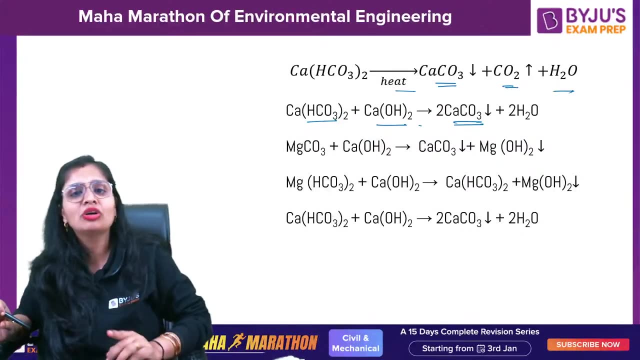 guys, Is it slaked lime or quick lime? Slaked or quick, Because in the examination they won't give you calcium hydroxide, calcium oxide. Slaked or quick- Come on faster. This is slaked lime or quick lime. Calcium hydroxide. 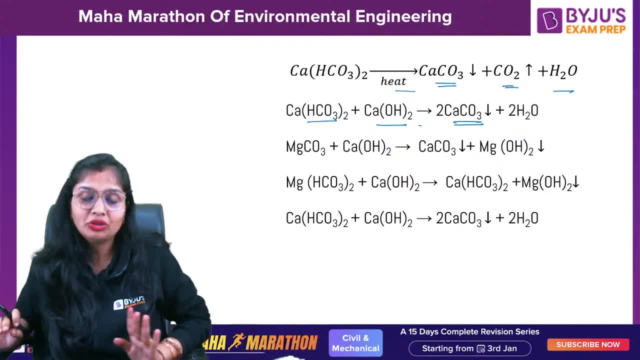 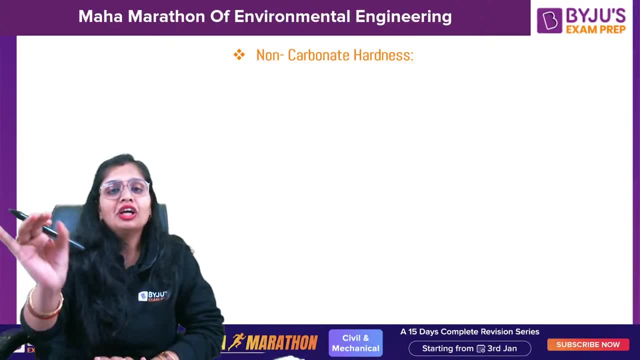 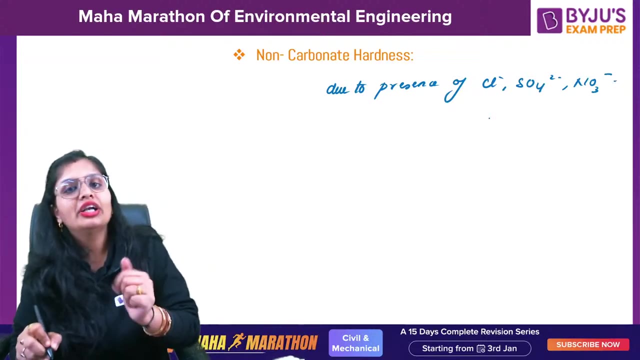 Slaked lime. So remember that They won't give you in the question calcium hydroxide and calcium oxide. Okay, Fine. So now talking about non-carbonate hardness, If chlorides, sulphates, nitrates are there, Then you will call it non-carbonate hardness. 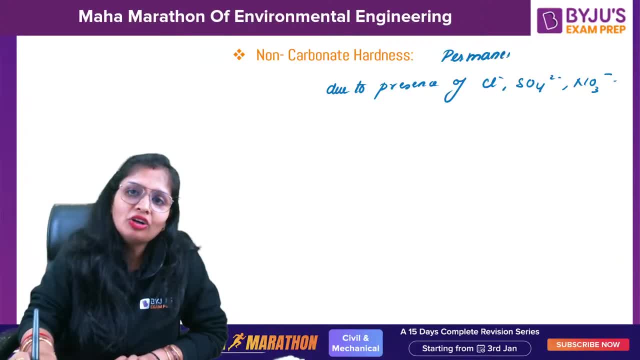 Or you call it as permanent hardness, because if you do boiling also, or you add lime also, it won't be removed. So techniques, special techniques are being used, like zeolite method, demineralization methods are being used. Now let me tell you: 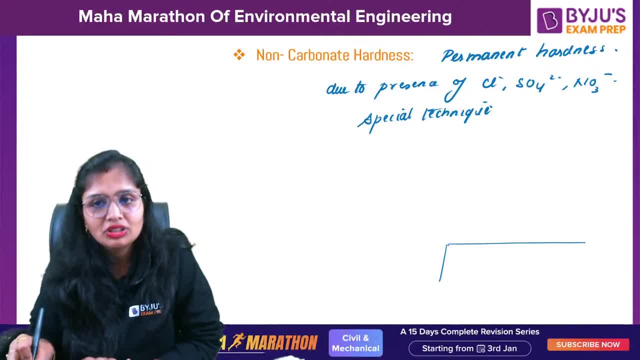 Actually why I am telling you is because in the questions- this tabular format questions are there- They write like this: Chlorides, sulphates and HCO3 minus. let us suppose They write calcium magnesium. You won't believe what students do it. Let us suppose it is written mg per litre. 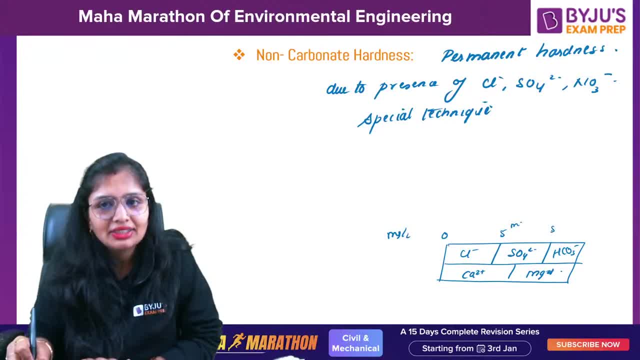 concentration is there: 0,5, and this is 8, this is 10.. People say let me tell you one thing: 0 to 5,, 5 mg per litre, okay, and this is 5 to 8, 3 mg per litre. They write: 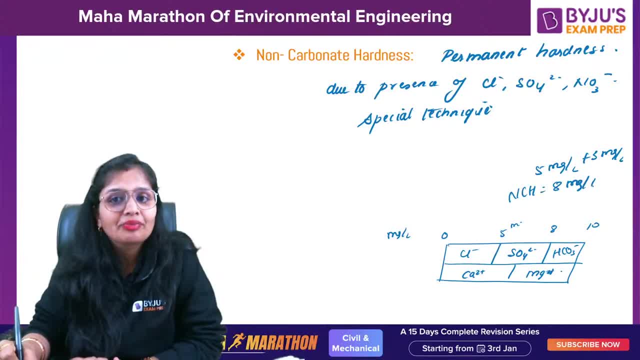 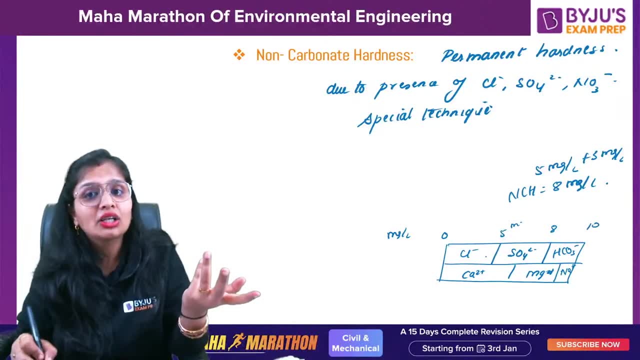 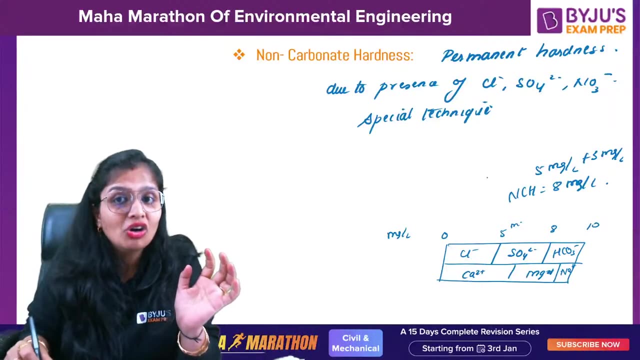 non-carbonate hardness is 8 mg per litre. Let me write sodium also here. How come you can say, how do you know, that chloride will combine only with calcium or it will combine with magnesium? It cannot combine with sodium. This is a wrong concept. 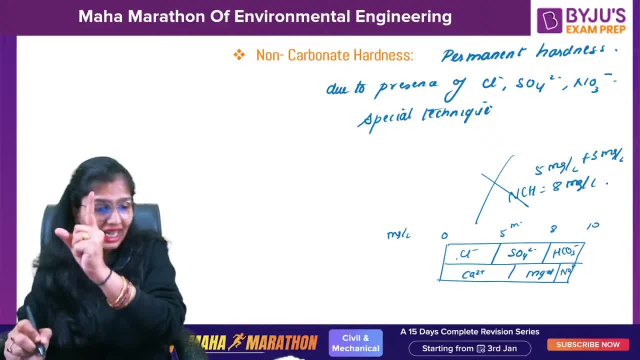 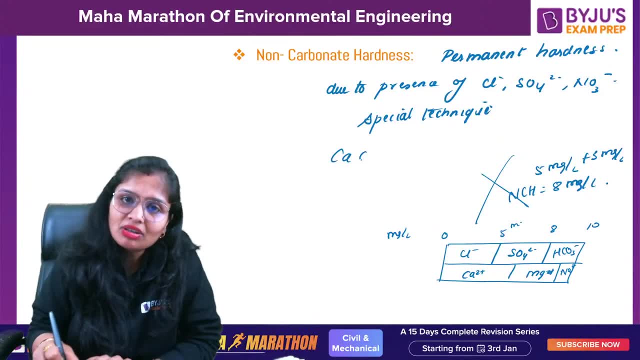 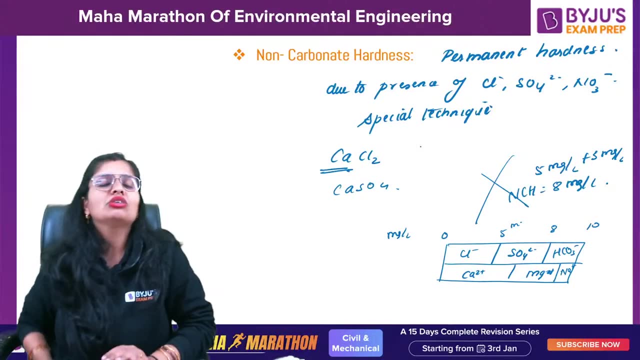 Wrong, wrong concept. Okay, that's why I am telling you here again. Okay, so chloride sulphates. again, the hardness will be due to calcium, and not only. But in the suffixes, chloride sulphates are there. then you call it as non-carbonate. 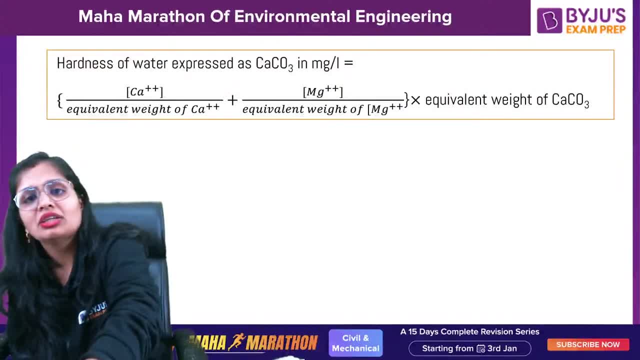 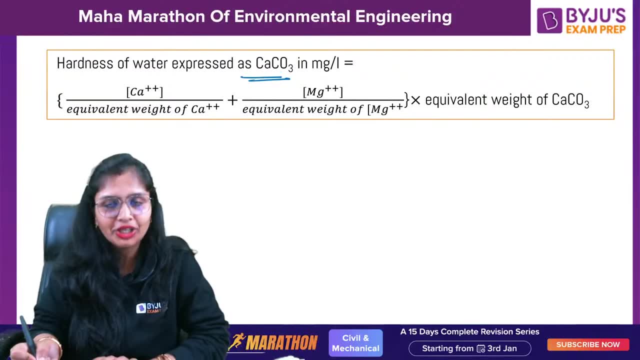 hardness, That's it, Okay. and one more thing: Hardness is also reported as calcium chloride only, sorry, as calcium carbonate only Here. also, calculate the gram equivalence of calcium. calculate the gram equivalence of magnesium. You want to get it in mg per litre. just multiply with the. 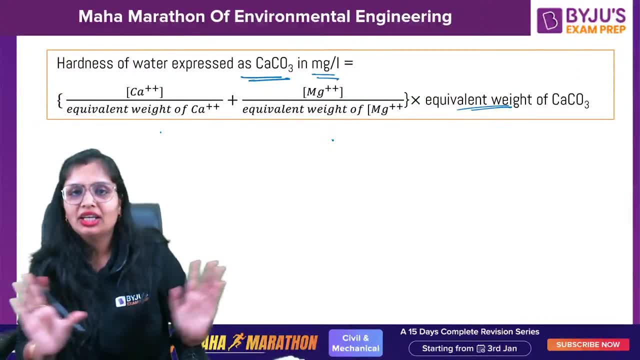 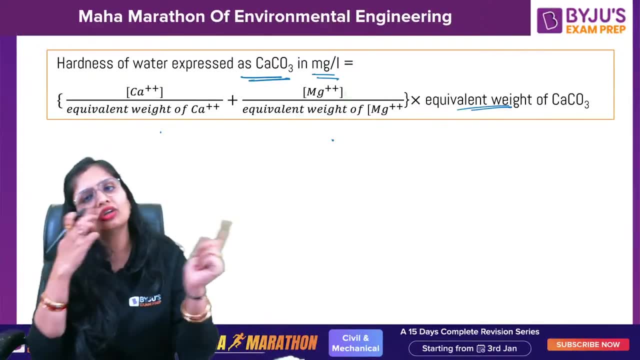 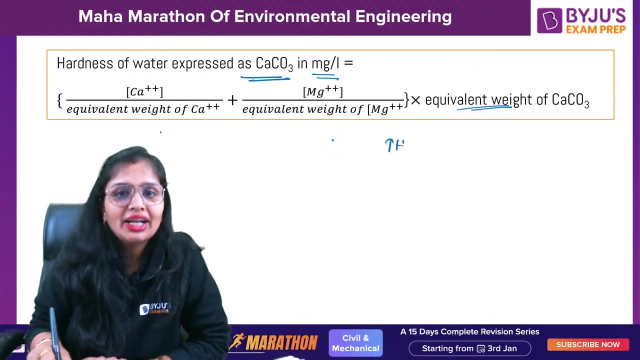 equivalent weight of calcium carbonate. As simple as that, Nothing you need to do. Limits, exactly same Limits exactly same as you get for alkalinity Here also 200 mg per litre and 600 mg per litre. Okay, lastly, you should know that, total hardness. 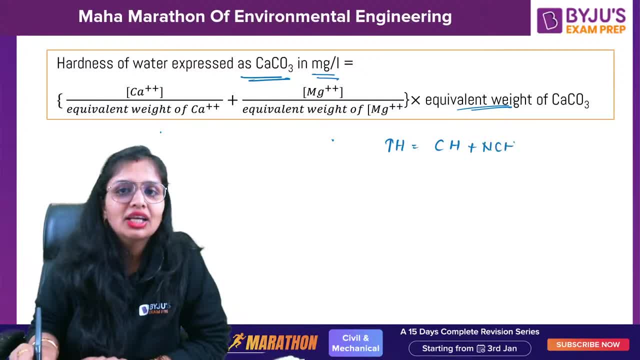 is carbonate hardness plus non-carbonate hardness, and carbonate hardness is minimum of total hardness and alkalinity. So you have to calculate total hardness and alkalinity, then you can check it out And non-carbonate hardness will become how much Total hardness minus carbonate hardness. 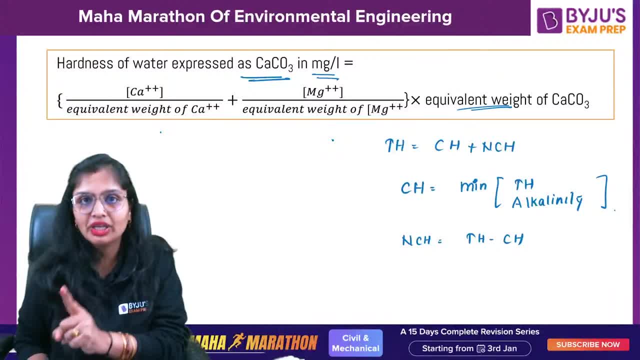 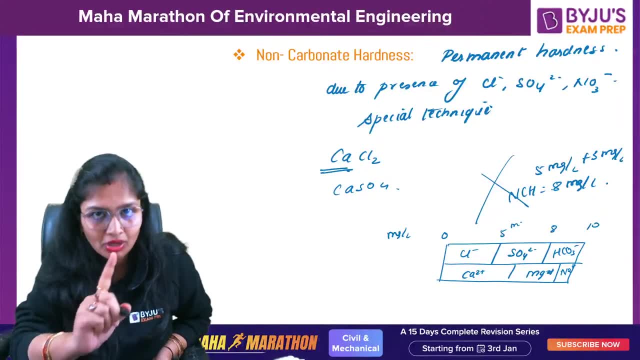 You cannot and cannot calculate non-carbonate hardness directly Like. if you think you can calculate non-carbonate hardness like this, you are wrong. Remember this. This is very important. You have to go through this procedure for calculating non-carbonate. 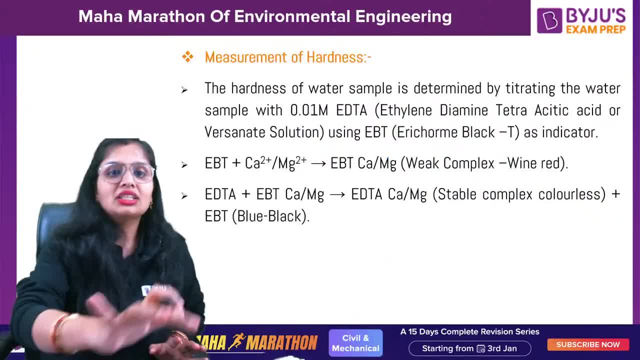 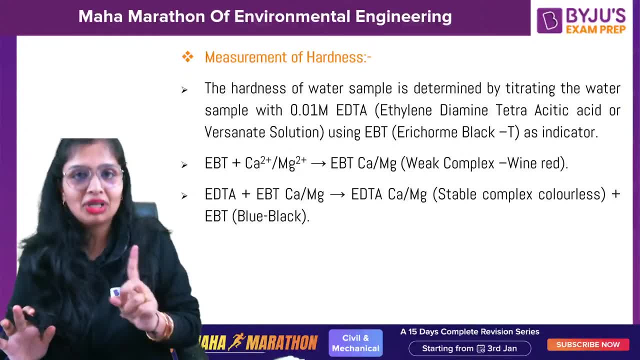 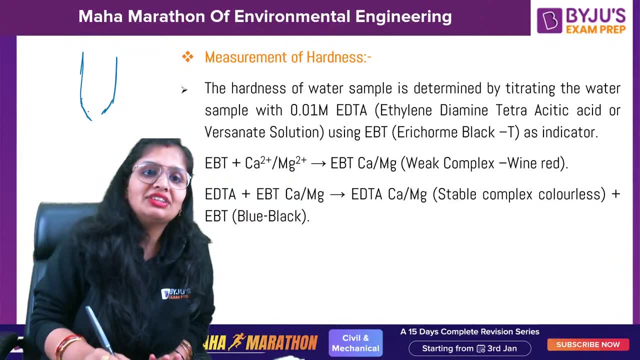 hardness, Okay. lastly, talking about measurement, because a question in GATE 2021 has been asked from this for one simple theoretical question, Let me talk about it in measurement part. This is the burette. You guys would have seen it. A burette is there, Okay. 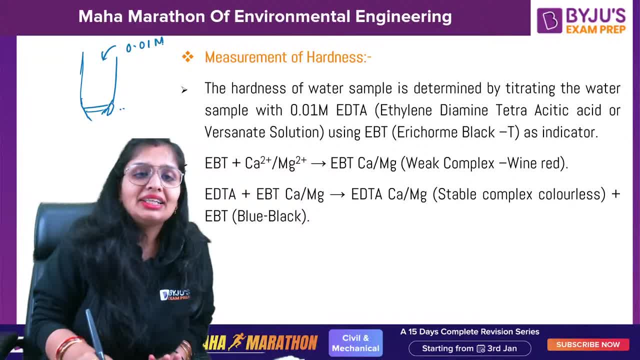 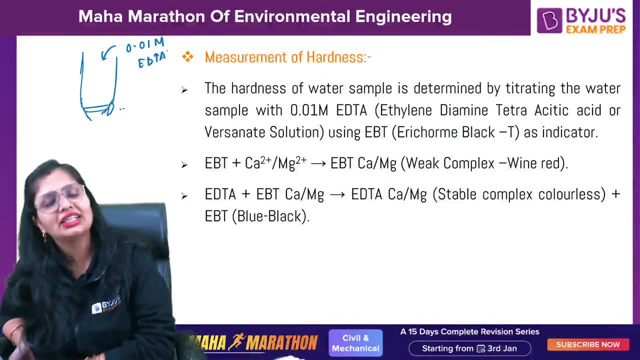 So what is happening? You are putting it a titrant. Titrant is that which reacts with the unknown parameters present in the water sample. First of all, the titrant used for the measurement of hardness is EDTA, ethylenediamine tetraacetic acid. 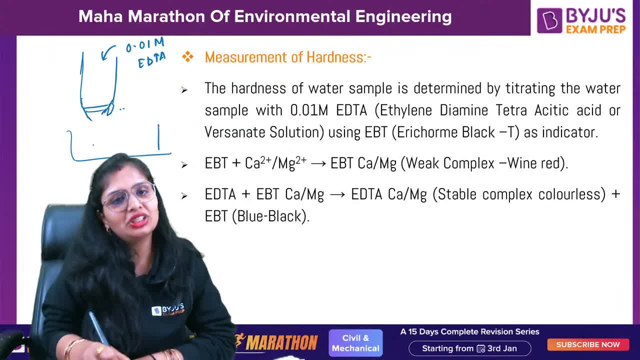 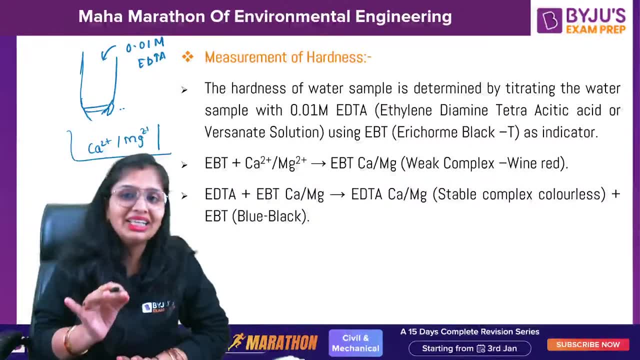 Now what you do. This is the sample. Generally, you just measure calcium and magnesium, because they are present in predominant form. Before starting the experiment, you will add EBT, that is, Eriochrome black tea. Okay, Now what will happen When you? 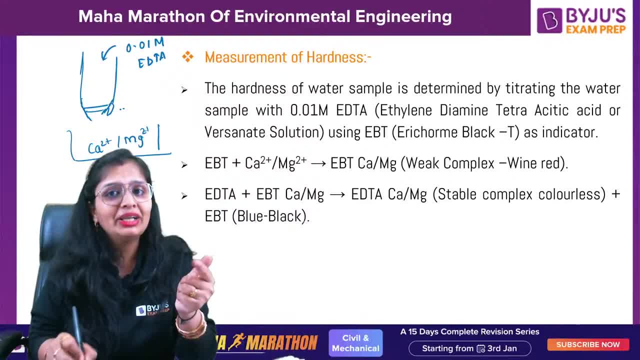 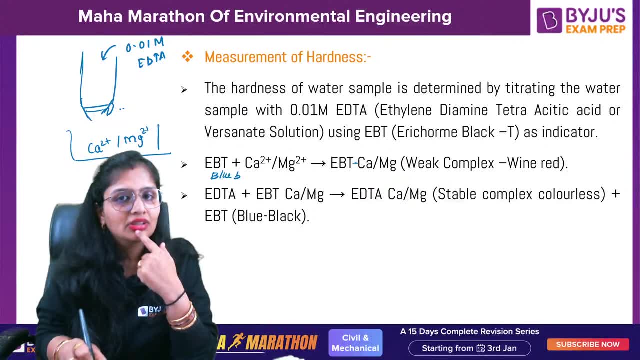 will add EBT. when you will add EBT, what will be the color of it? What will be the color of it? EBT is blue, black. What will be the color of it When you will add it? it will become wine red. Okay, Generally, you know, in. 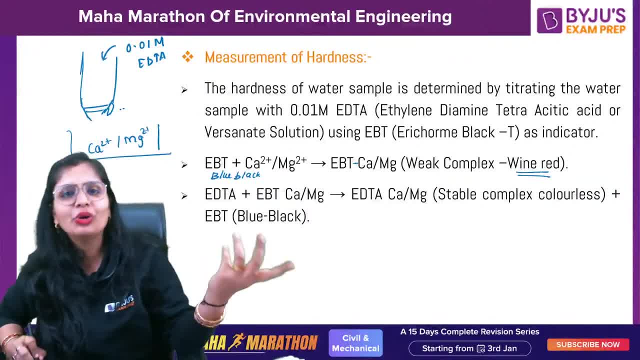 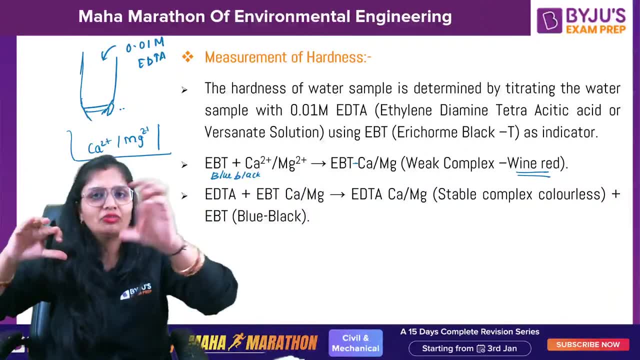 chemistry, we enhance the color greenish, pink, yellowish, orange. we say like that: Okay, Now what will happen After this? you will turn the burette on, EDTA will pour You properly mix it. Okay, The moment, the moment, what will happen? 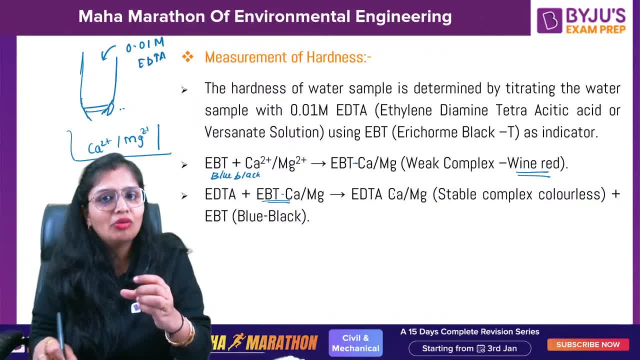 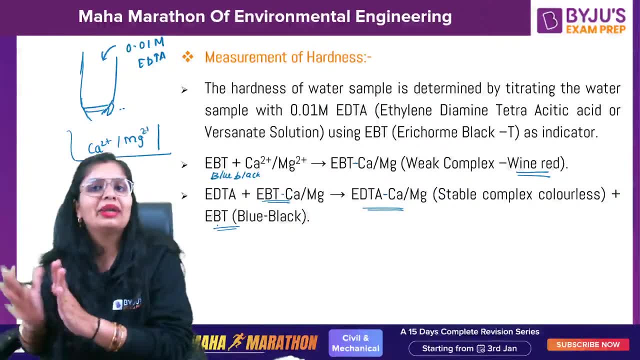 EDTA will break this complex and it will form a complex with calcium and magnesium. This will be colorless and EBT will be again there, present separately blue black. So technically the sample will become blue black. So the quotient and gate was, as the 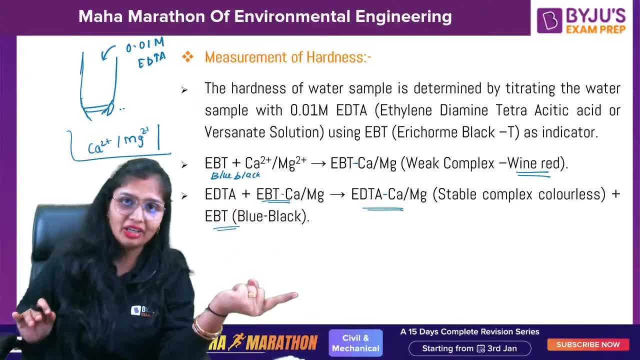 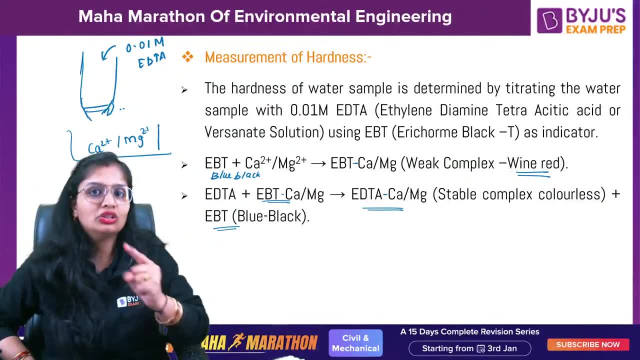 change of color. So the change of color becomes from wine red, because before the experiment the sample was wine red. After the experiment the color became blue black. So this was being asked in examination. Okay, So remember, EDTA is being used, EBT is the 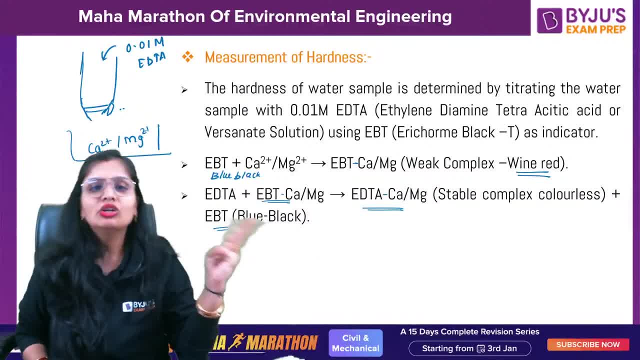 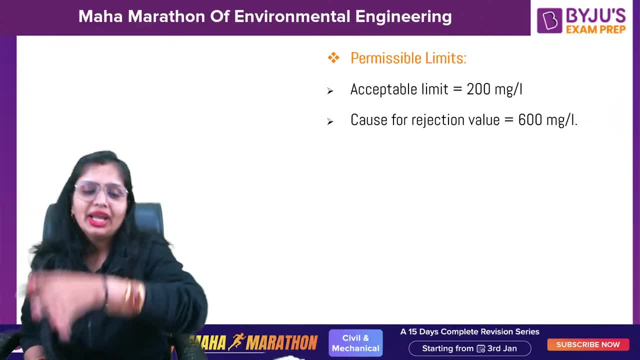 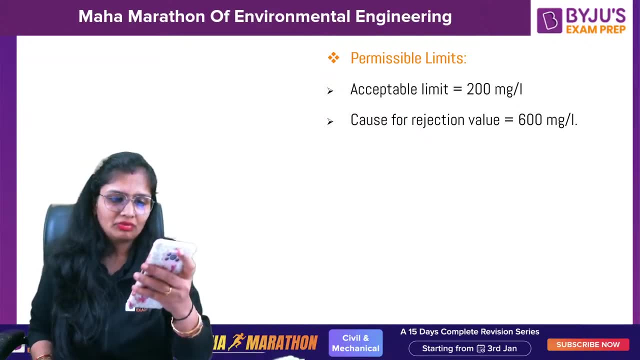 indicator which is used, Color change is from wine red to blue, black, Clear. So these three things which you should know, it Limits already. I told you. Any doubts still here? If there is no doubts, so let's be quick and solve one. 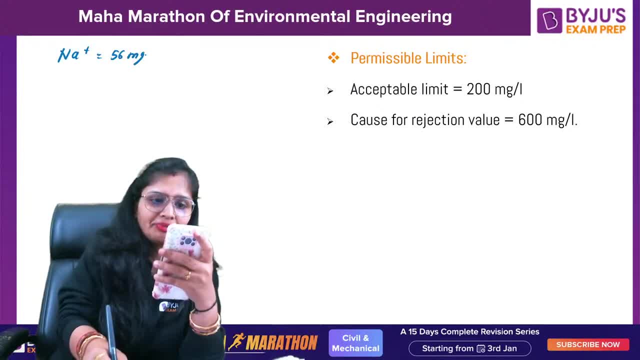 question: Sodium: 56 mg per liter, Calcium, 40 Mg2 plus 30 mg per liter. Aluminium, 3 mg per liter, HCO3 minus 190 mg per liter and Cl minus is 165 mg per liter, And it is asking you firstly to calculate total hardness. 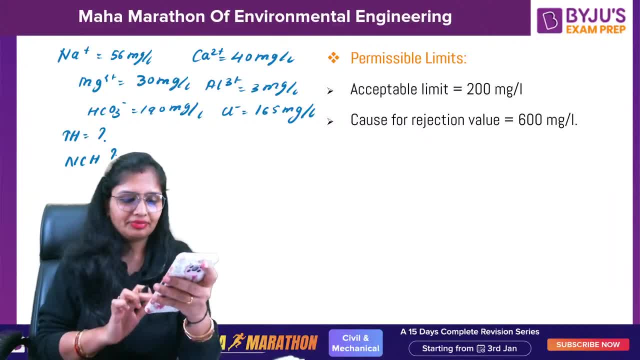 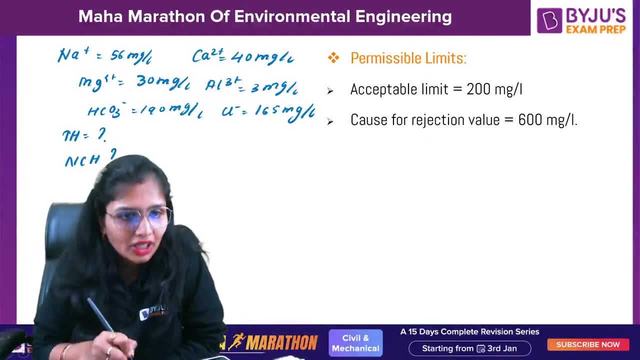 and the second is noncarbonate. Come on, guys. So all this Total hardness and noncarbonate hardness, Total hardness, that is, it is asking you to calculate: magnesium will be there, calcium will be there and aluminium Why? Because in the quotient, nowhere it is given. 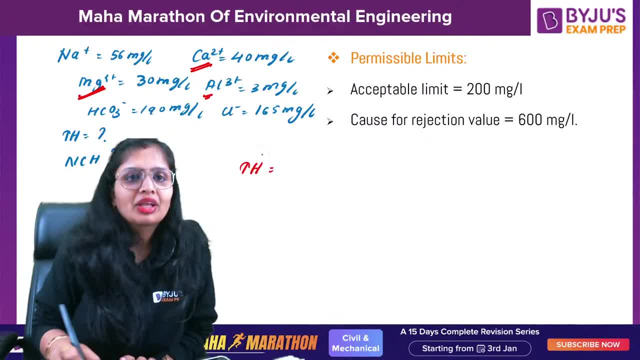 Very good. So the total hardness will be 30 mg divided by the equivalent weight. I will tell you one more thing: beta Magnesium. firstly, the weight equivalent weight is 12.. If it is written like this: 30 mg divided by 12. 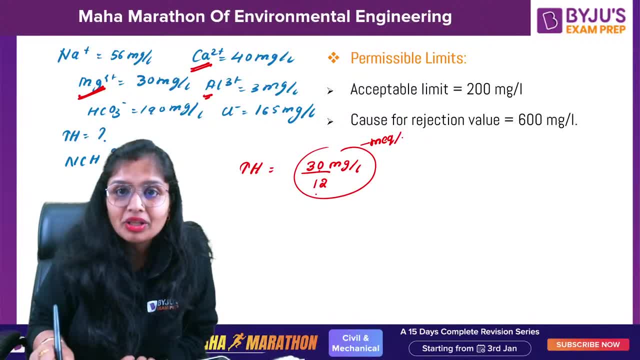 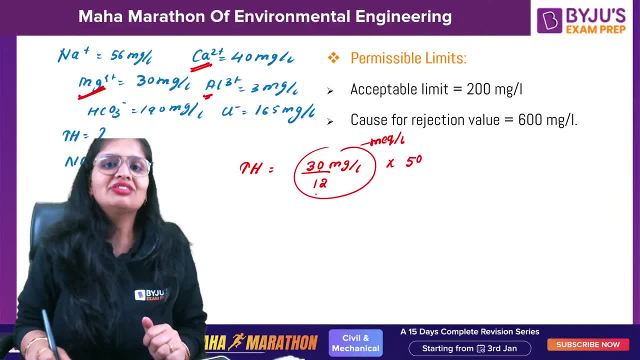 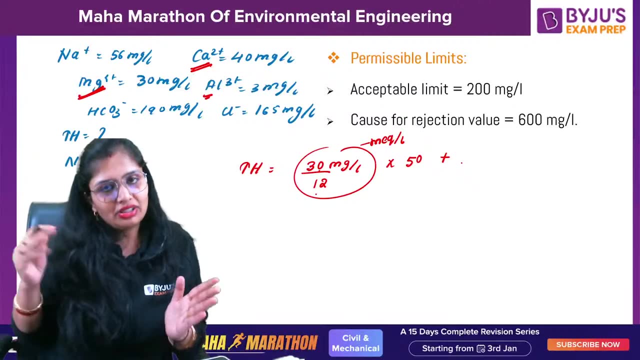 this. you call it as milli equivalents per liter, Remember this. And then you multiply with the equivalent weight of calcium carbonate. This equivalents and equivalents will get cancelled out. You get it as mg per liter. Clear Then. I have multiplied it separately, but take it. 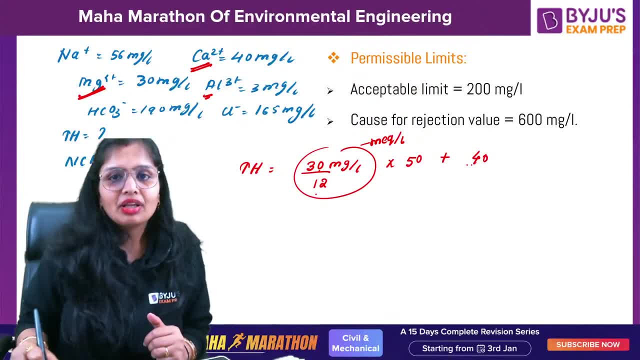 common and multiply it at the last: 40 divided by 20 is the equivalent weight of calcium: 50. 3.. Equivalent weight of aluminium is 9.. Why? Because the molecular weight is 27.. The valency is 3.. So 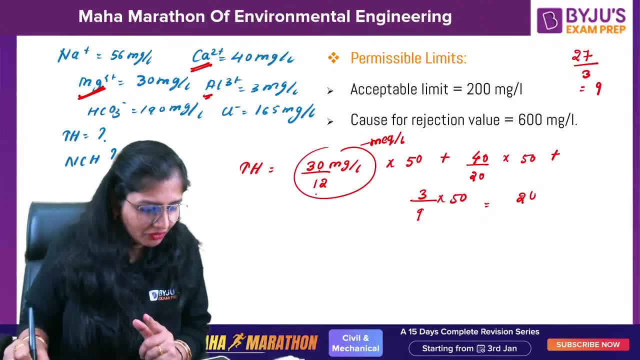 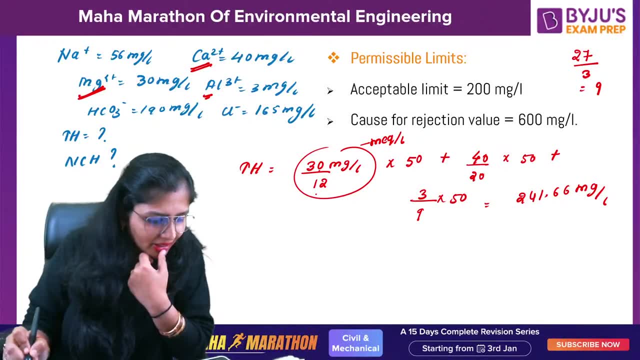 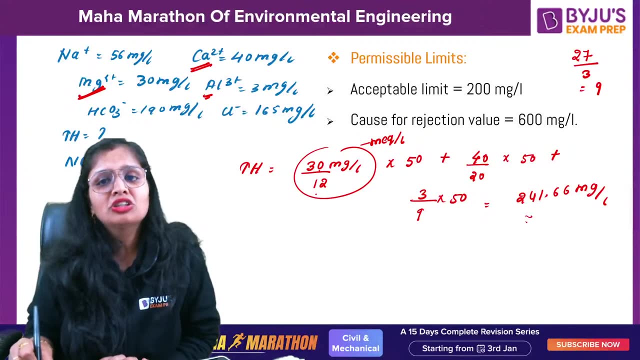 9 into 50. How much it is coming? 241.66 mg per liter. Why mistake again? Both Ankit and you are getting 241. it is getting Alekh Ankit beta, no calculation mistakes. So approximately 242 mg per liter. 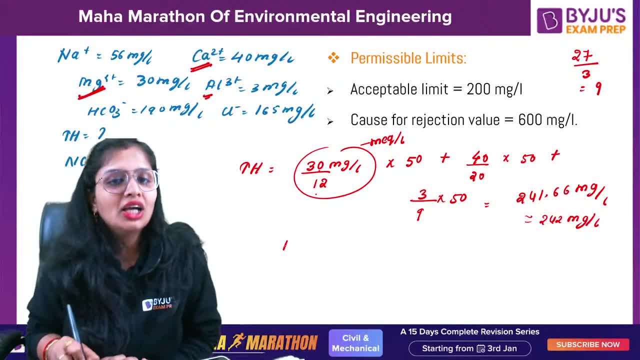 Next, it has asked you noncarbonate hardness. Noncarbonate hardness is total hardness minus carbonate hardness. Carbonate hardness you cannot calculate directly. You have to first calculate alkalinity. Alkalinity only one is given, It is CO3 minus. 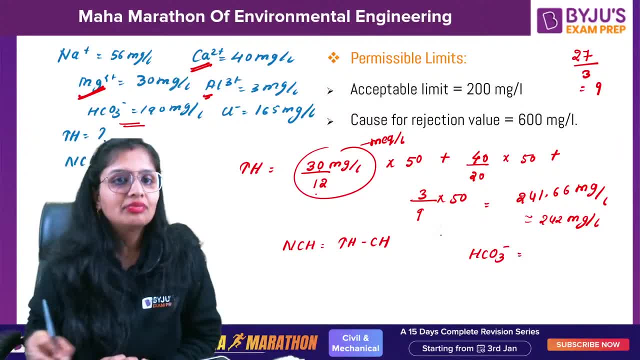 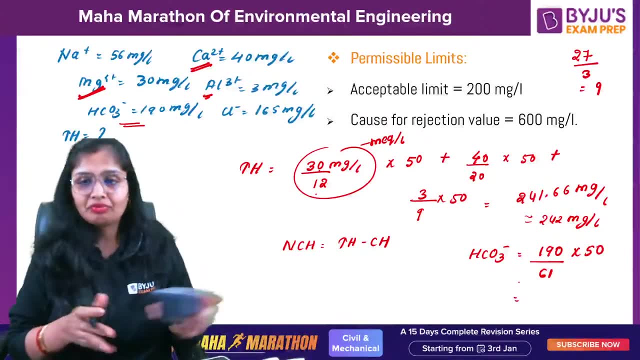 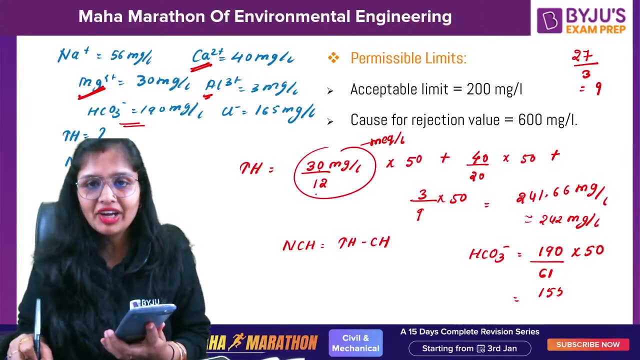 Take that It is CO3 minus 190 divided by 61 is the equivalent weight into 50.. How much it is coming? 190 into 50 divided by 61. This comes out to be 155.73 mg per liter. 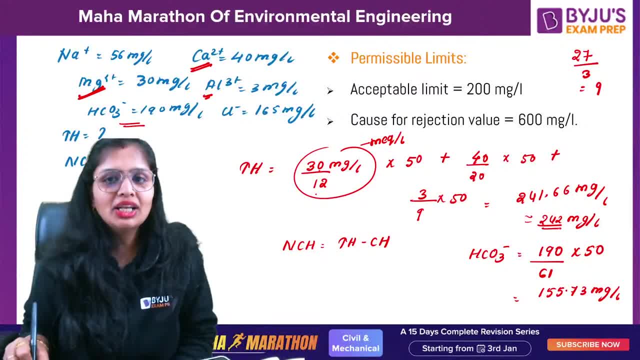 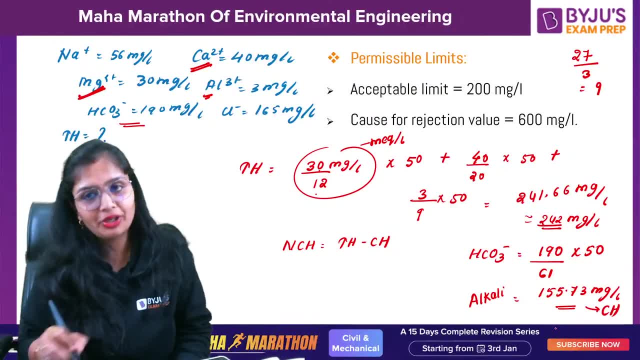 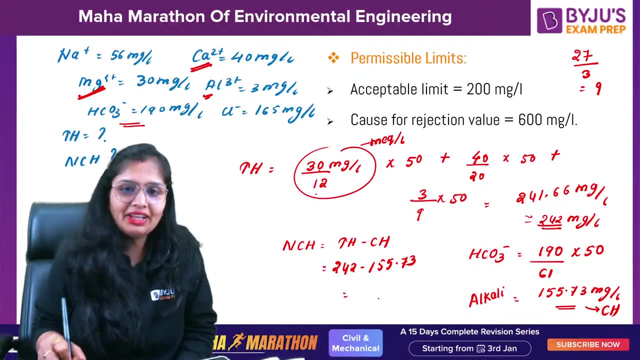 So what will be the carbonate hardness? This is total hardness. This is alkalinity. The minimum is how much? 155.73. So this will be the carbonate hardness. So total hardness is 242 and this is 155.73, 85.93. 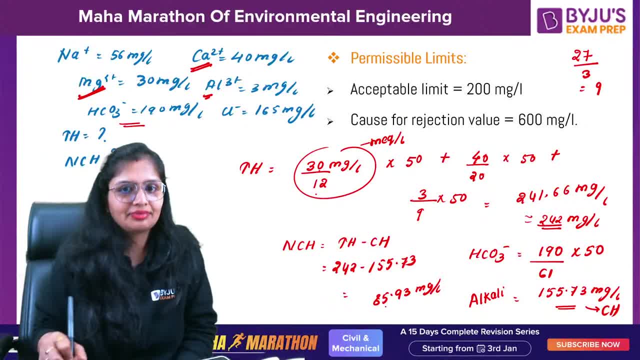 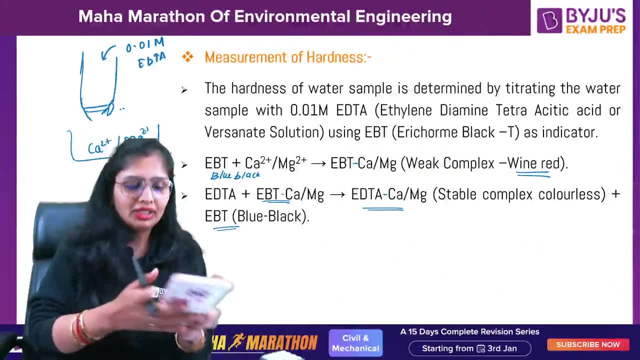 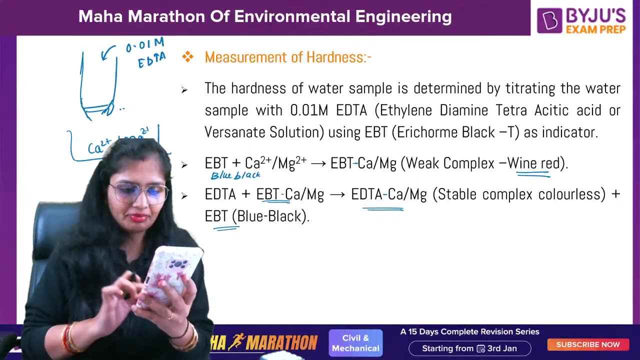 mg per liter, approximately 86.. This will be the answer. Ok, One last question of milliequivalents per liter. I will tell you That is also required. That's it. Then we will move further. Milliequivalents per liter. 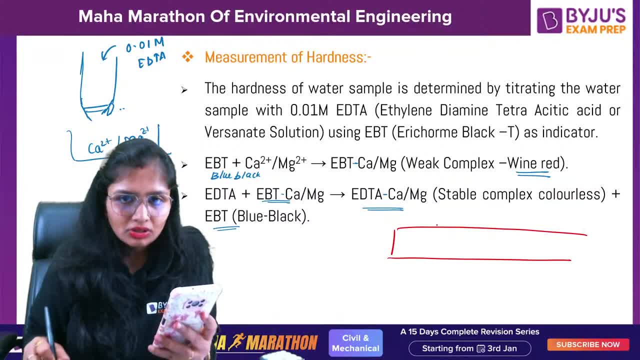 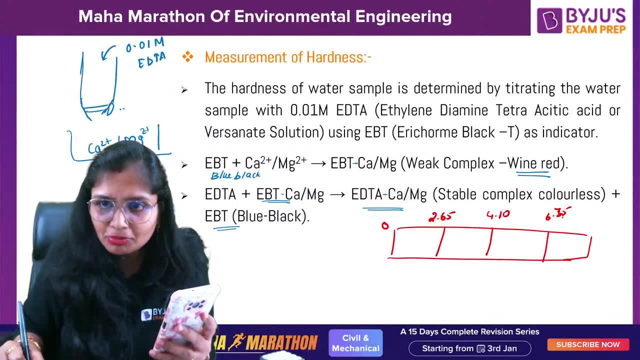 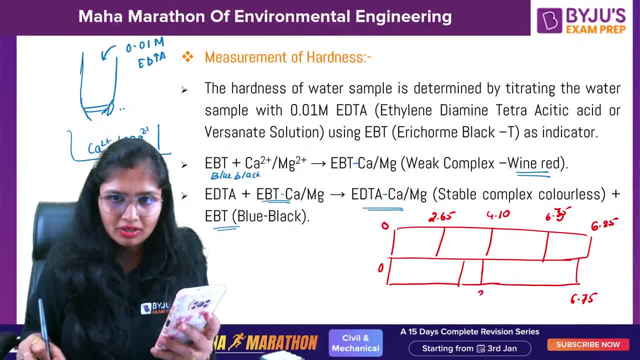 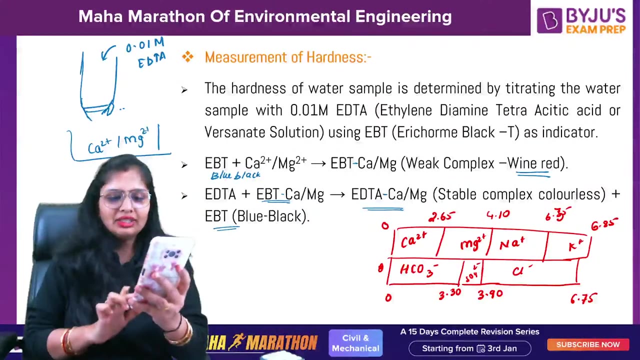 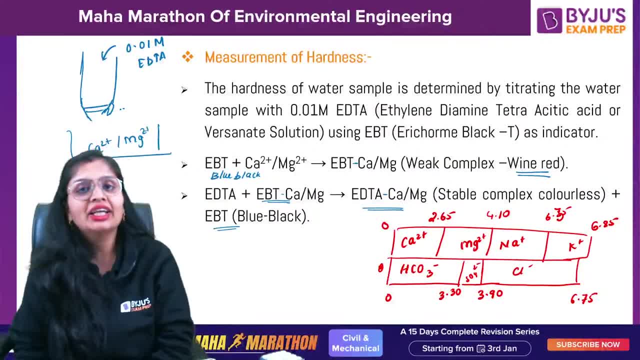 the question atomic weight as 24. just check it out, the atomic weight. if the atomic weight in the question is given you 24, okay, then you have to take is 12. if they are giving you another atomic weight and based on that, if it is coming 12.5, no issue. so just check it out here they have given 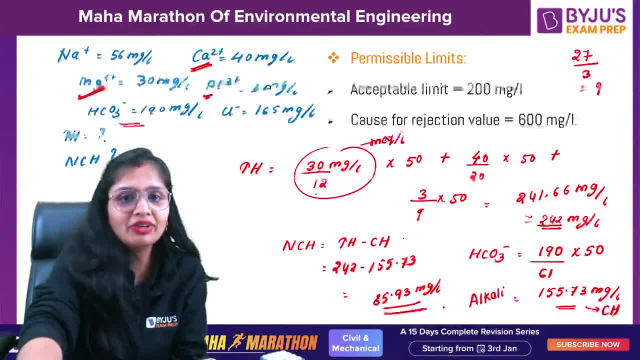 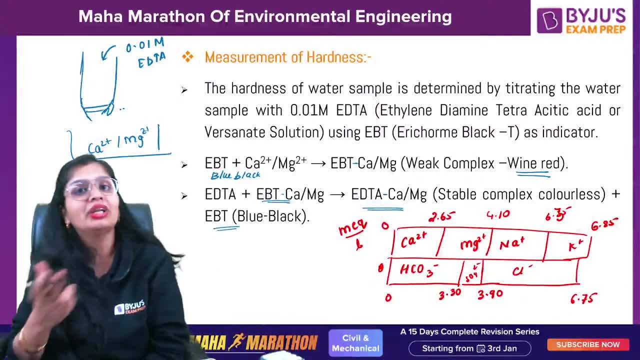 you in milli equivalents per liter. that means milli equivalents per liter is given. that means this value is directly given to you. so just check it out in the questions whether it is in mg per liter or milli equivalents per liter, since it is in milli equivalents per liter. calcium 0- 2.65. 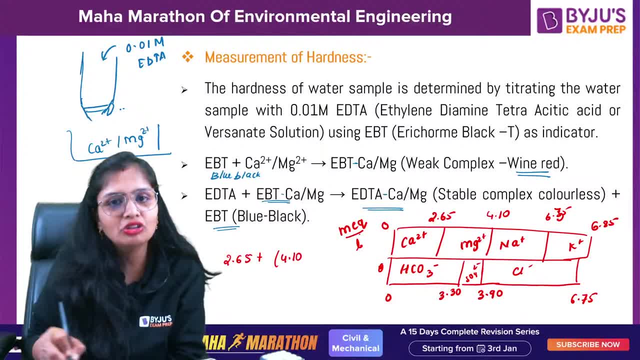 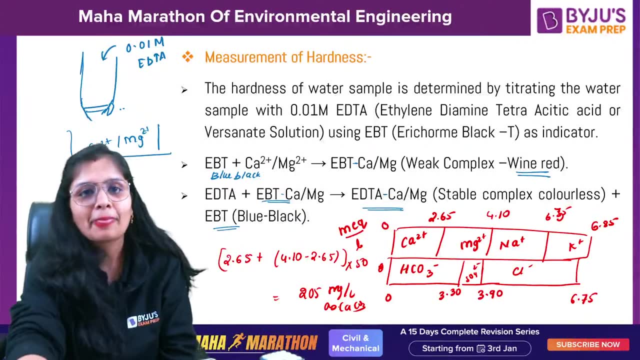 magnesium will be how much? 4.10, because here to here it is 4.10 minus 2.65. just multiply by 50, that's it how much it is coming: 205 mg per liter you. so this is the thing which you need to check it out. okay, fine, now talking about chloride content. 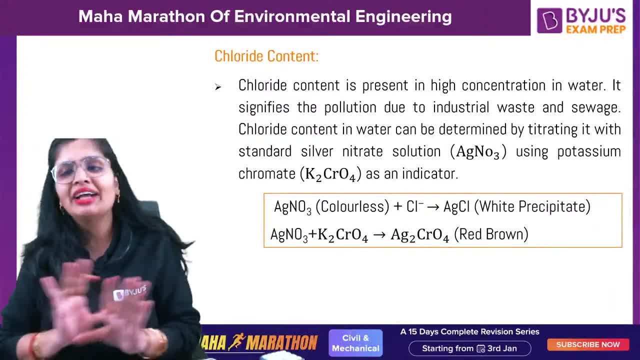 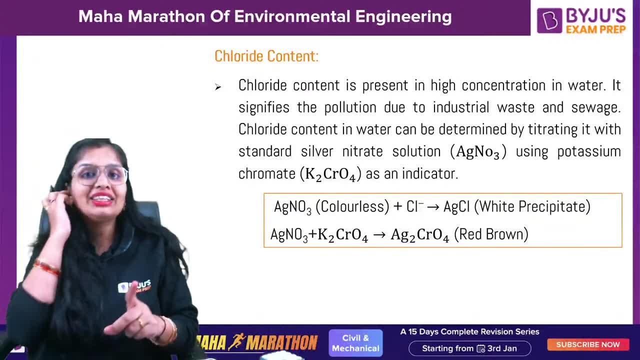 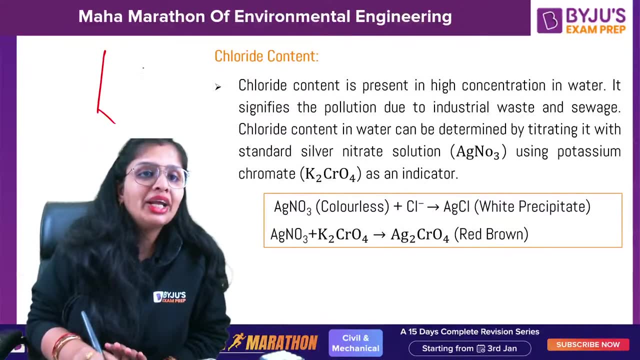 chloride content. if it is present in excess, that means that water has been polluted. either industrial waste is there or sewage is there, the technique of measurement that is known as moore's method. so you should know the indicator, the name of it. so what is happening in the burette? 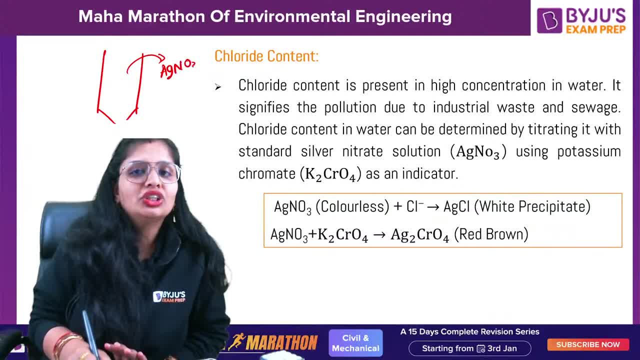 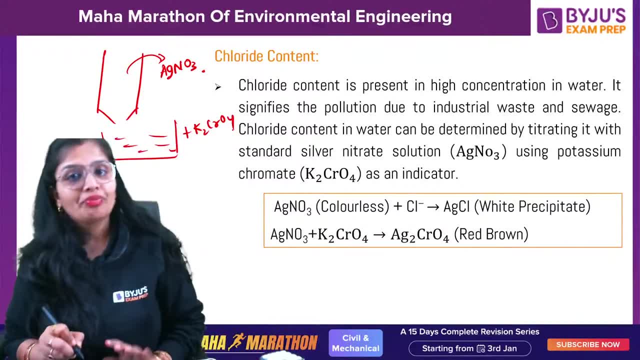 you have to take a solution that is silver nitrate solution is to be there. what you will do: you will take the sample and you will add indicator that is k2c ro4. when you will add it before that, you won't start the experiment. you will add it now. what will happen? 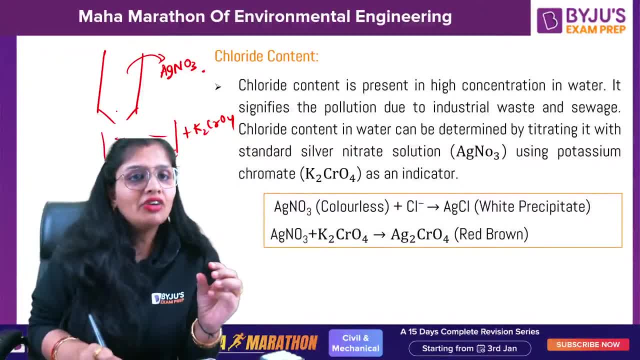 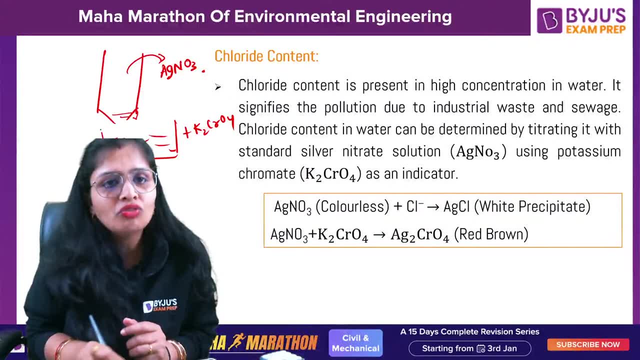 here chloride is present, so agno3 will pour, it will react and you will see, eventually this whole water will become white. this whole water will become white. that means the whole chloride is exhausted. after the whole chloride is exhausted, even a sample will become white. now what will happen? 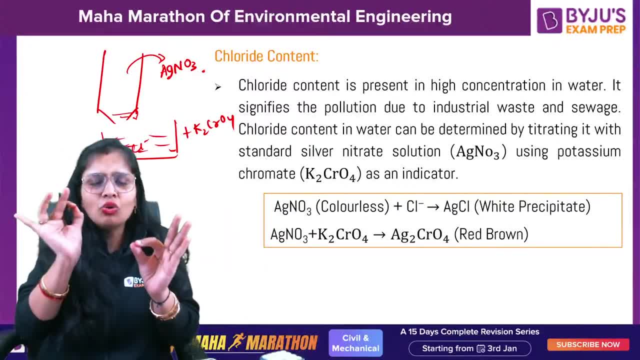 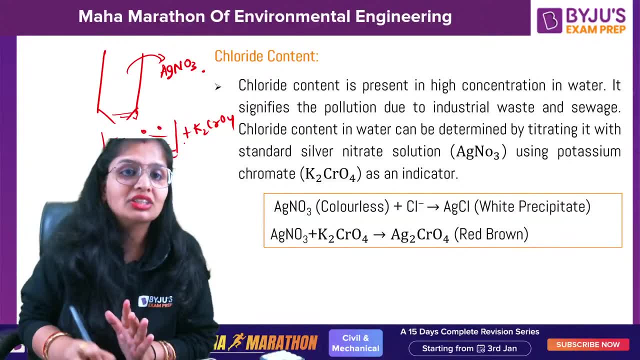 this whole water will become white and we will get away with thumbnail and live the wholecompleted jaw. point that after it is completely magnets. so once we add it, second lot, fique. the entire. the whole chloride is exhausted, exhausted. even a single drop of silver nitrate you will pour. you will see red color on this. so 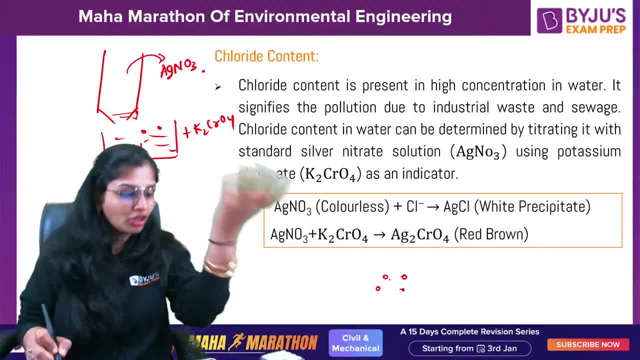 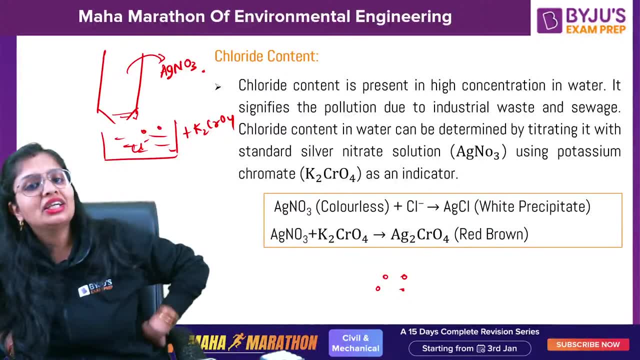 imagine this white color is there and if you pour red color, it will automatically it will be visible. okay, so now you will say, ma'am, initially also k2cr04 was present, why agno3 is reacting now, because the affinity of agno3 was more for chloride rather than for k2cr04. okay, so this? 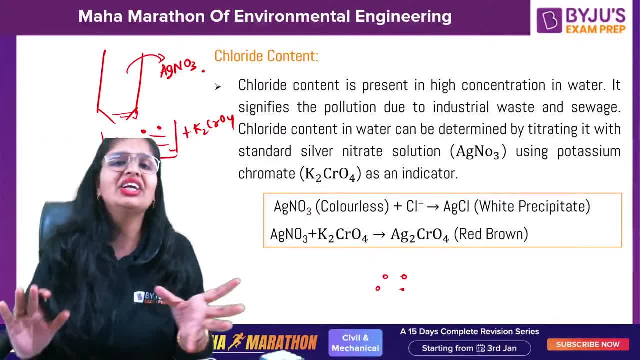 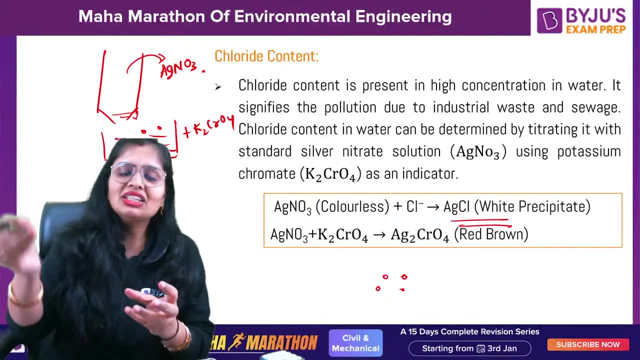 experiment. you guys would have done it in college also. this is clearly. you can see this. so this is agcl, is the white precipitate. the moment it is purely exhausted, even a single droplet, you will add. you will get red, brown color. so you will close the burette, so you will take. 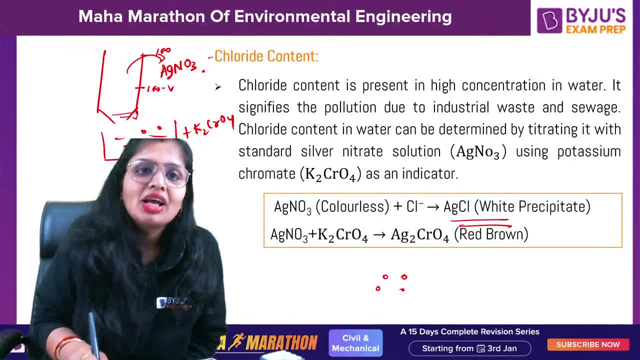 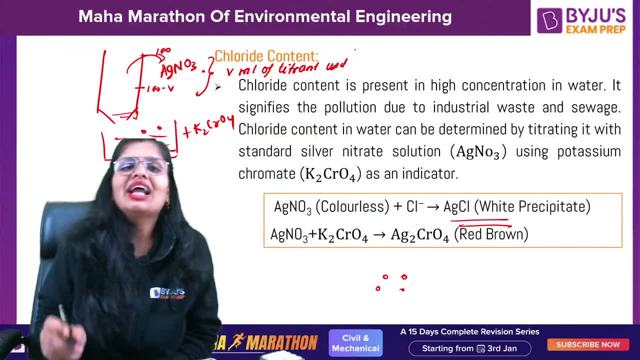 the reading if it is 100, and here this is 100 minus v. so how much is the titrant used? if vml of titrant is used, you will say how much is the gram equivalents of agno3 used. you will say how much is the gram equivalents of agno3 used. you will say how much is the gram. 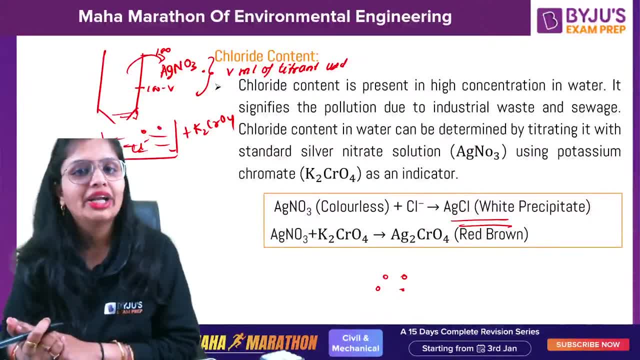 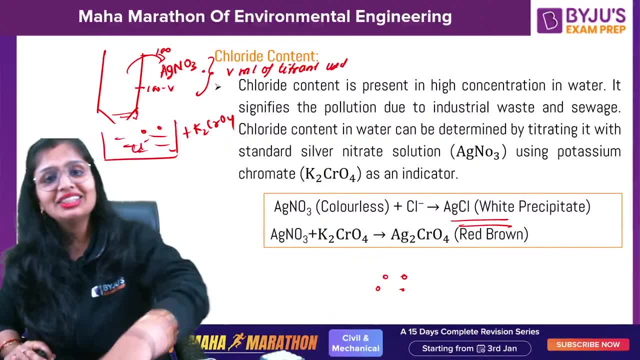 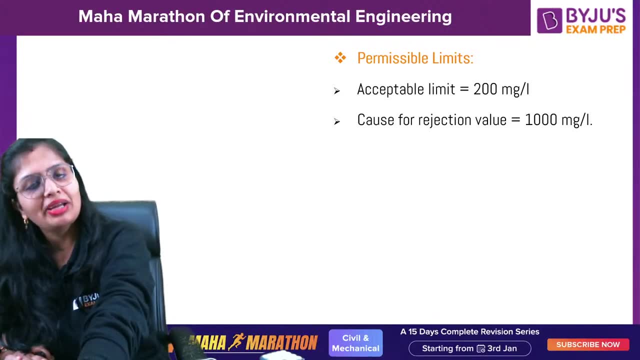 equalence of silver chloride will be present, basically, that much amount of chloride will be present. in hindi class is not working. it is working, it is working okay. so this is chloride content limits: acceptable limit: up to 200 mg per liter. cost for rejection limit: 1000 mg per liter. okay. 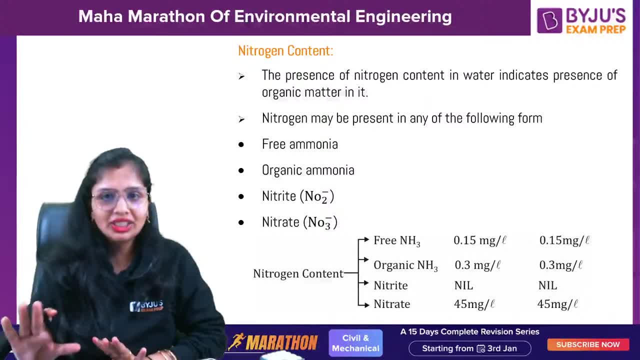 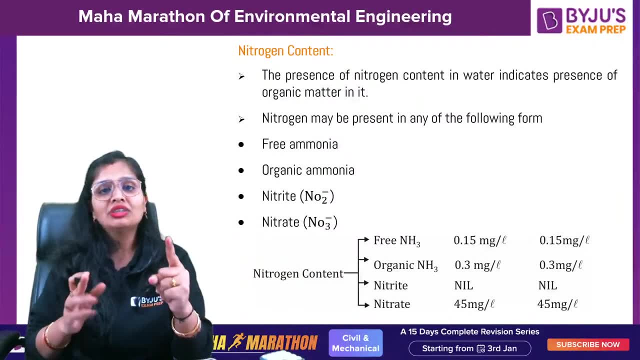 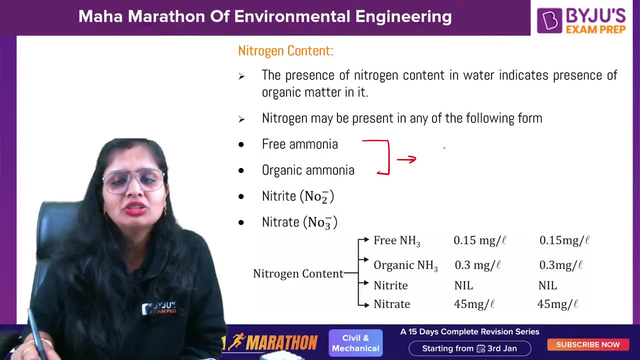 lastly, uh, again last, basically nitrogen content. is there again one basic formula. they are basic thing. they ask you: firstly, nitrogen may be in pre-ammonia, organic ammonia, nitrite nitrate. okay, the summation of pre-ammonia and organic ammonia is known as what? don't look at here. 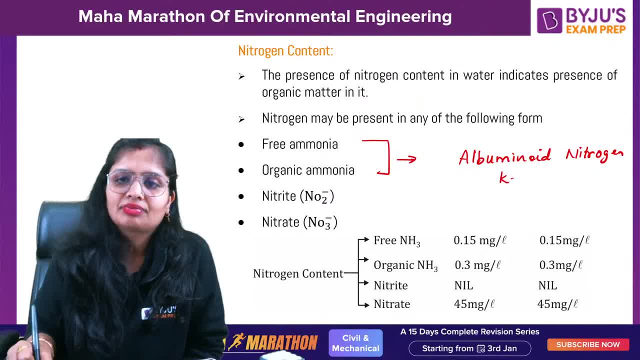 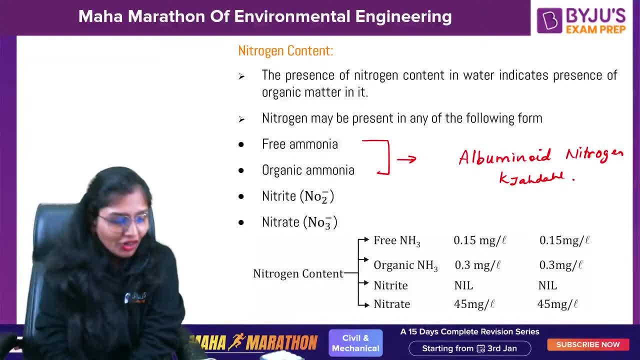 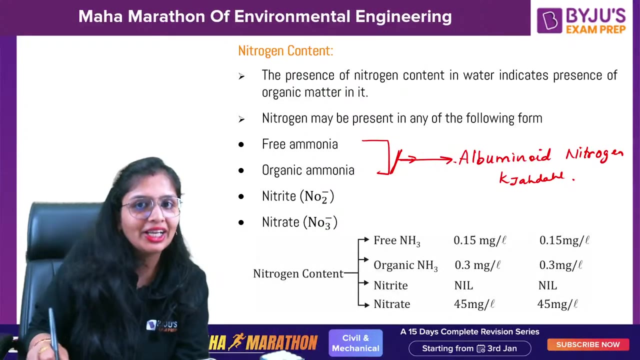 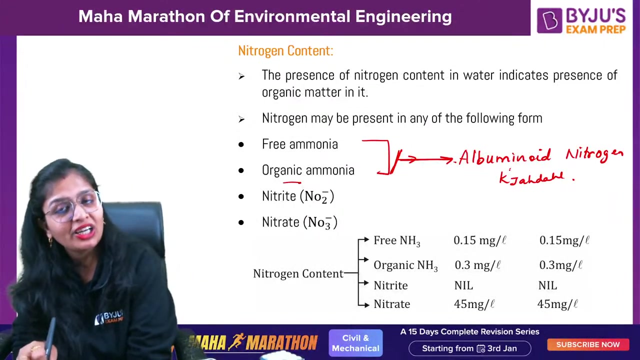 nitrogen, or this is known as no. you want anything? a cage nitrogen, okay, albuminoid nitrogen. this is wrong. you should tell me, ma'am, this year i've written wrong why. because organic ammonia is known as albuminoid nitrogen. remember this maximum students get confused. that's why i've written: organic ammonia is known as albuminoid nitrogen. but summation of: 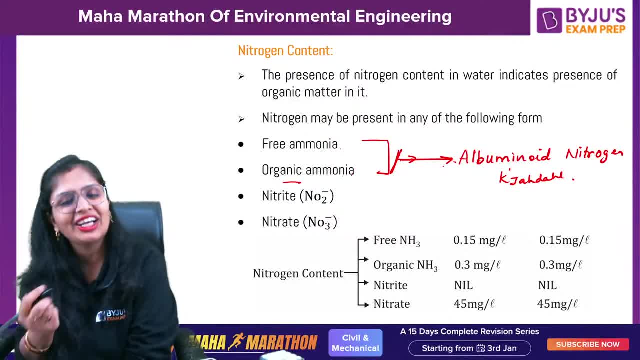 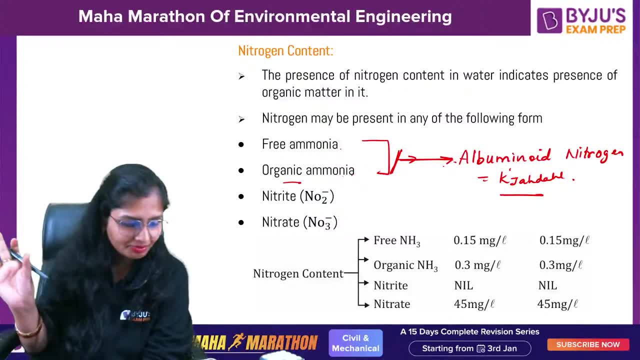 both of them, that is, pre-ammonia plus albuminoid nitrogen, or you can say organic ammonia is known as schedule on nitrogen. okay, so don't get confused. so this is the sum of both of them and the sum of those is a new specification that people are confused in this. okay, i have written the wrong. 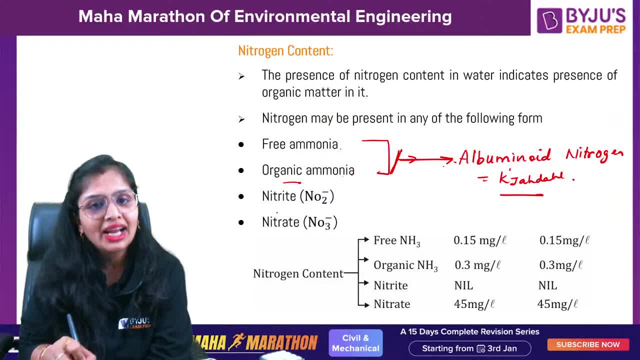 spelling also: fine nitrite nitrate pre ammonia. organic ammonia nitrite means partial decomposition, ł of organic matter is going on right. that means you cannot use that water. that's why the limit is mentioned to you. nil nitrate means oxidation is completed. but again, tell me the prominent name. 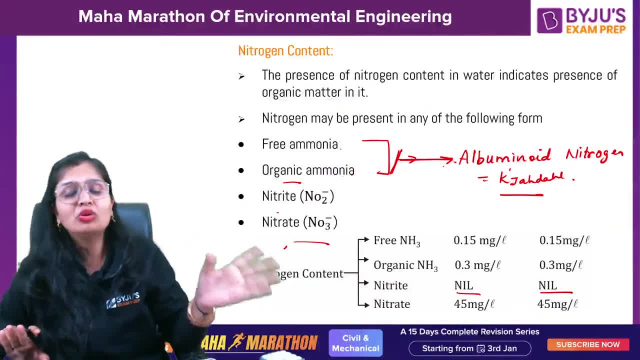 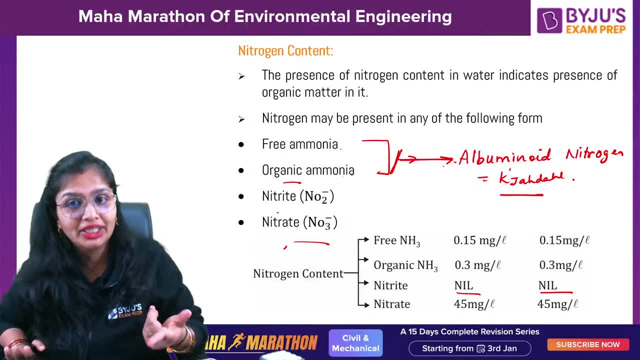 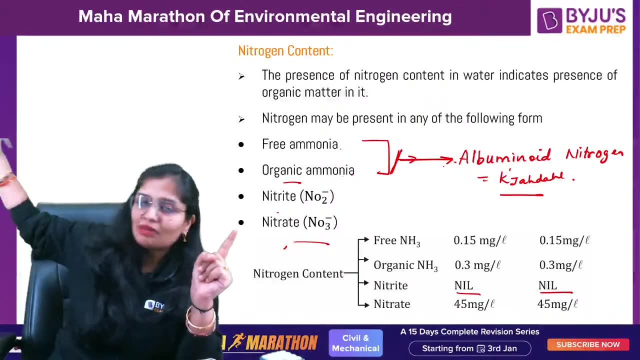 prominent name asked in all of the examination: blue baby disease, or we call it as methamoglobomania. So if the concentration exceeds by 45 mg per liter here, cause for rejection limit and acceptable limit is same. that means there is no relaxation If you live in that place. there is no alternate. 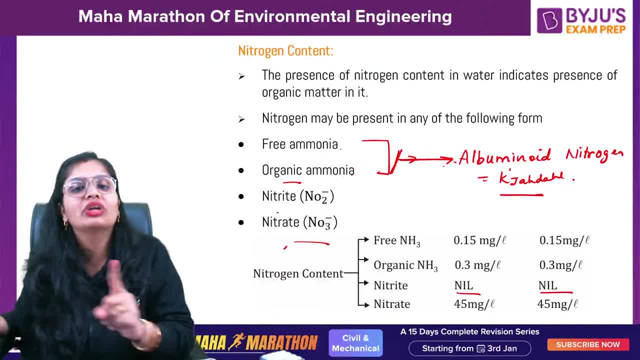 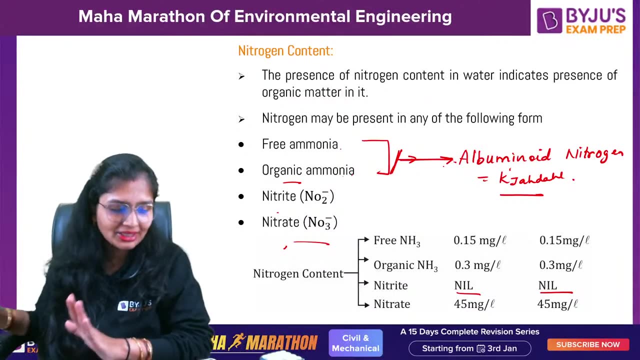 source available. then also, you have to follow this limit. it means no relaxation. So if concentration is more than 45 mg per liter, you will get those blue baby disease which will get, which will be happen to the infants, not to you guys, okay. So that is blue baby disease. Now one more thing. 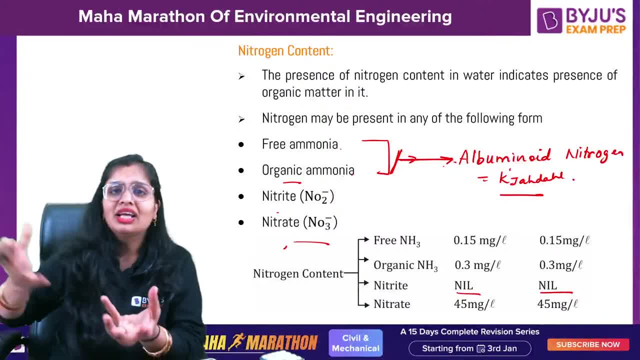 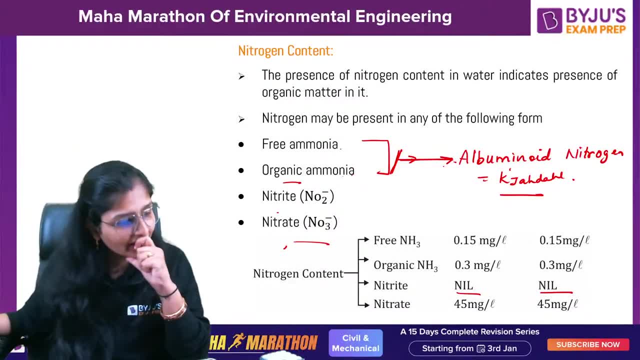 how to measure it. free ammonia: just boil the sample. NH3 will be liberated. distillation: you will get the value Organic ammonia. can anybody tell me how we'll get organic ammonia? Organic ammonia- you, neela bacha. It's like. it's like blue baby disease. the color of the blood becomes like that. okay, Next. next talking about next is 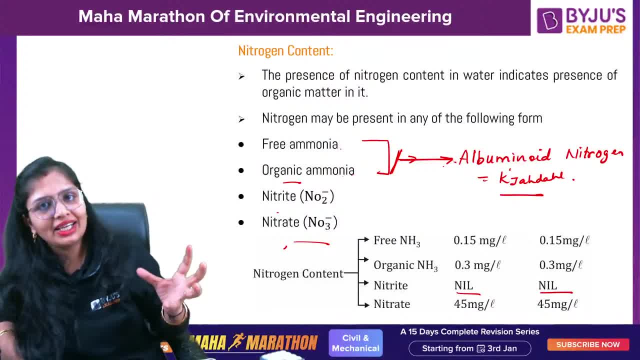 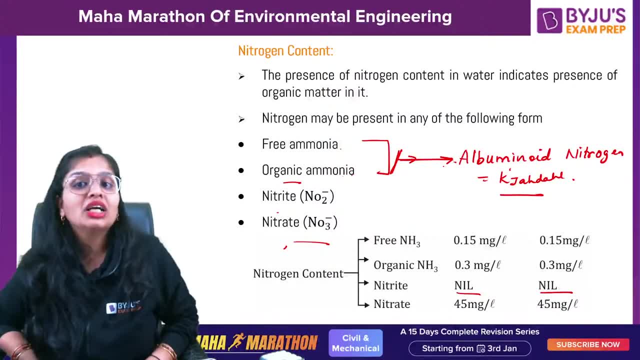 organic ammonia. already boiled sample is taken, add a oxidizing agent, again boil the sample. Why? Because organic ammonia consists of complex organic matters. If you'll heat once, it won't go. So that is the reason what you have to do: you have to heat it again by adding oxidizing. 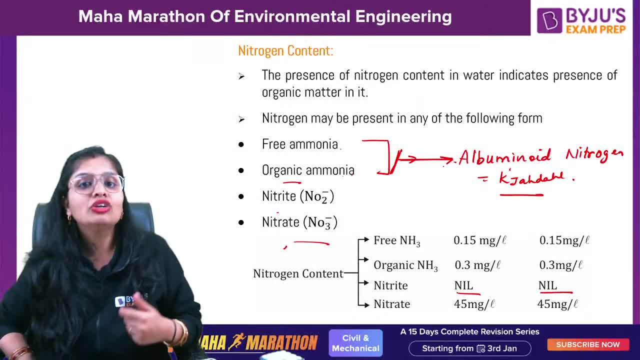 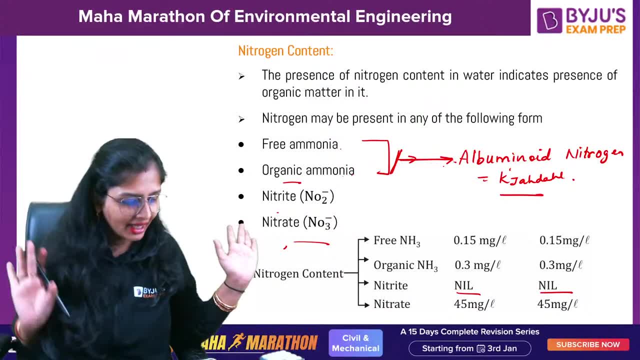 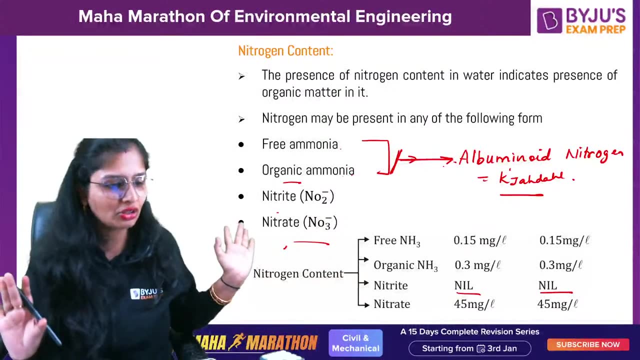 agent. So that is organic ammonia. while you talk about nitrite and nitrate, you can measure them by color matching technique. That's it and out. clear boiling plus kmino4. you cannot kmino4. you can add oxidizing agent or any other strong oxidizing agent also, can clear. 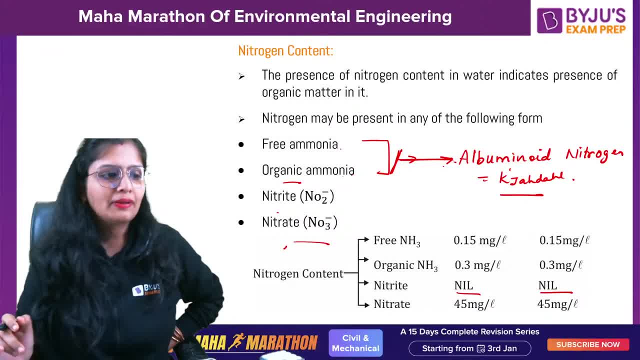 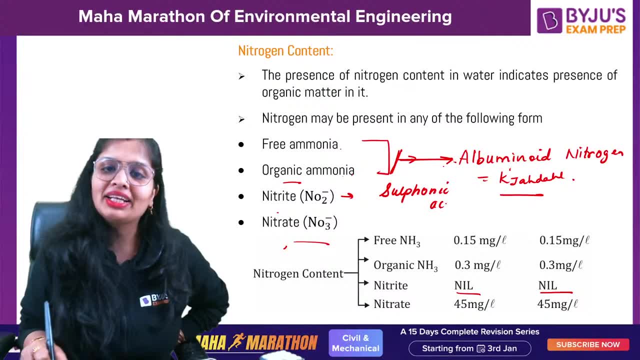 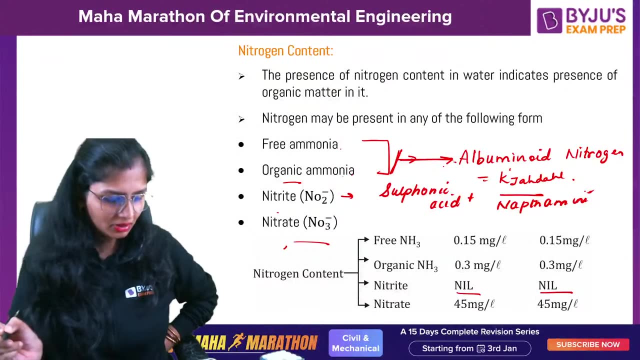 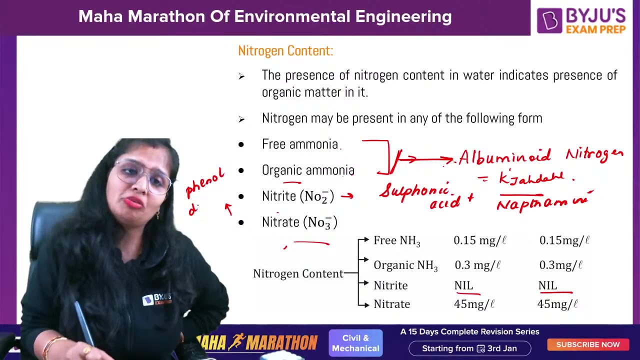 Tell me fast any doubts and if you want, I can write it for nitrite. it is sulfonic acid plus naphtha- color matching technique- plus naphthalmine. okay, clear, no nitrite. also, this is phenol disulfonic acid. they haven't asked till now, but if they will, phenol disulfonic acid plus potassium hydroxide. 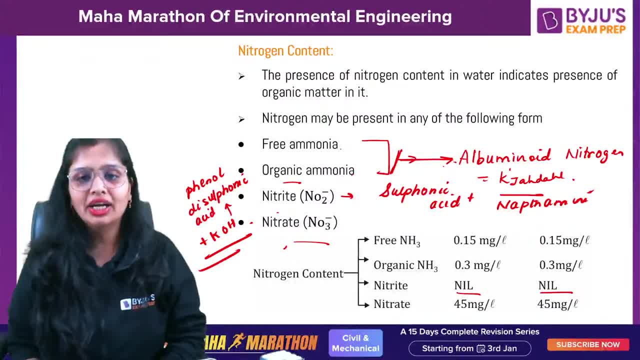 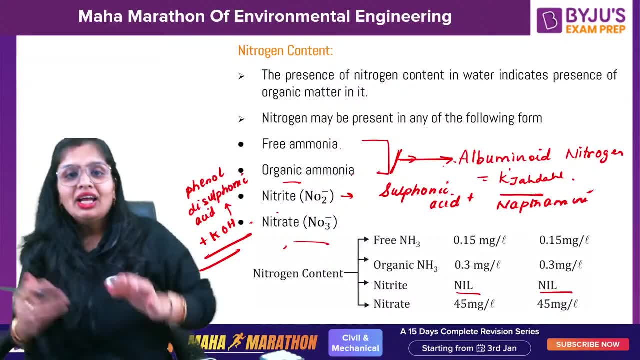 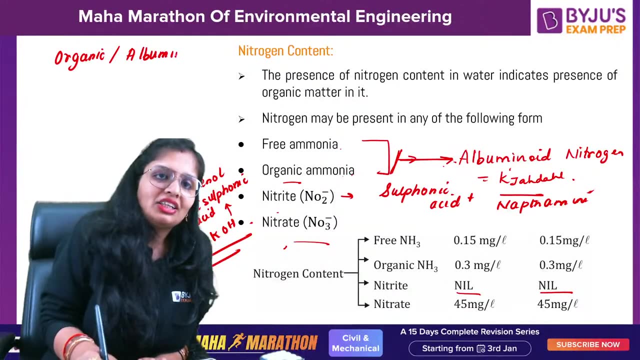 clear. so this is the nitrogen content, which you should know now. lastly, everybody knows about ma'am, albuminite and JIA. once again, organic ammonia is known as albuminite. okay, so generally students get confused. that's why I wrote it like this: and this is free. ammonia is different. 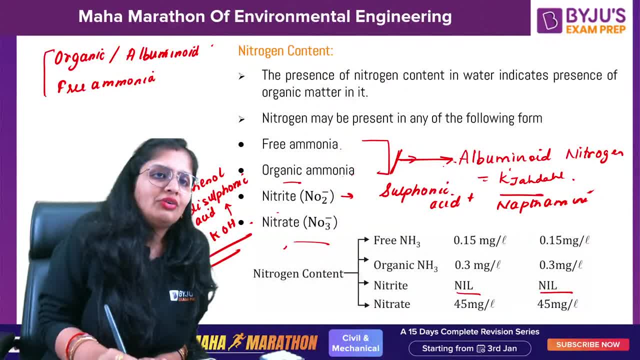 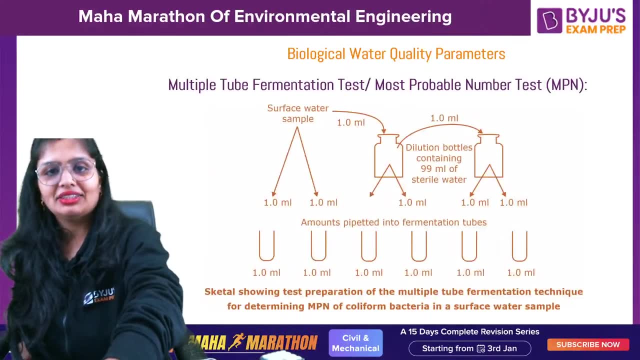 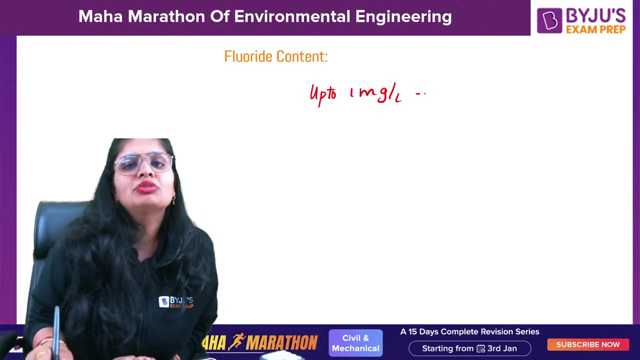 when you add both of them, you will get a K-genic nitrogen clear, Prashant clear. so now last, this is the, then we have MP and I guess yeah, so right content. so right content, up to 1 mg per liter. it is good why? because it helps to prevent from dental cavity and helps in the permanent. 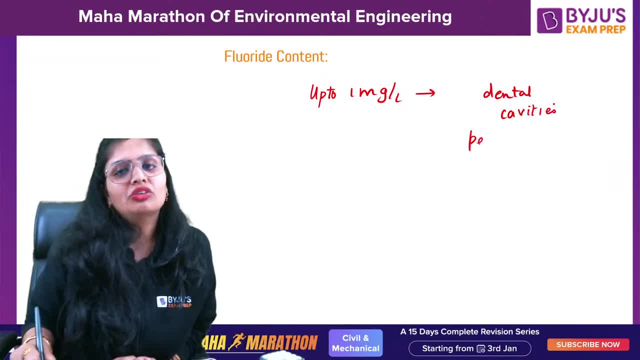 growth of teeth, permanent growth of teeth, and if you have permanent growth of teeth today, this pen is my writing is becoming bad in this permanent growth of teeth now, after 1.5 mg per liter, what will happen? decolourisation. you will see in the teeth brown precipitates are there. so decolourisation. 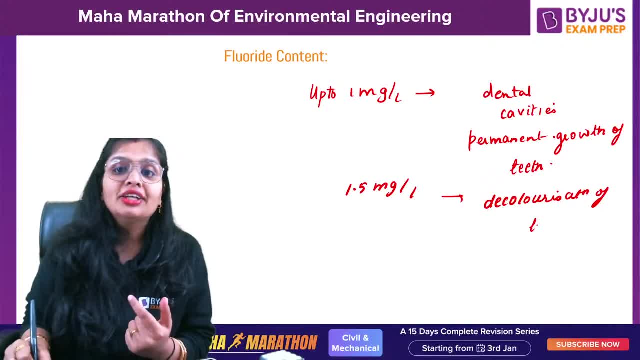 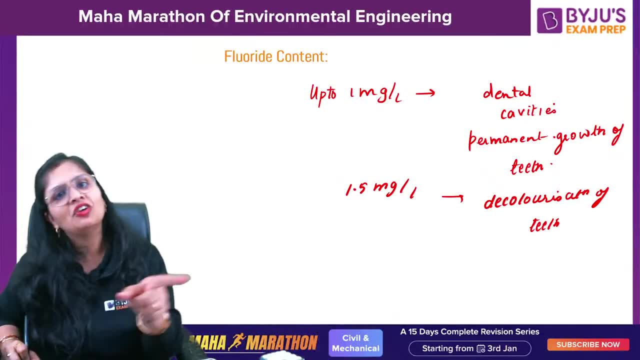 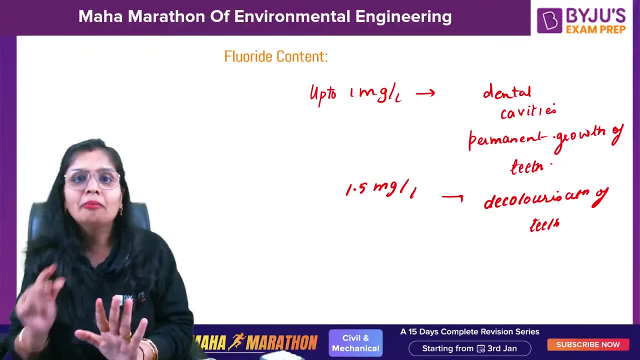 of teeth, or you call it as mottling of teeth. is there so generally, generally, this cavities thing? I already told you it's not that if you don't brush your teeth and if you eat chocolates and on and you will say that, ma'am, in my water fluoride is not there, so don't like this. but 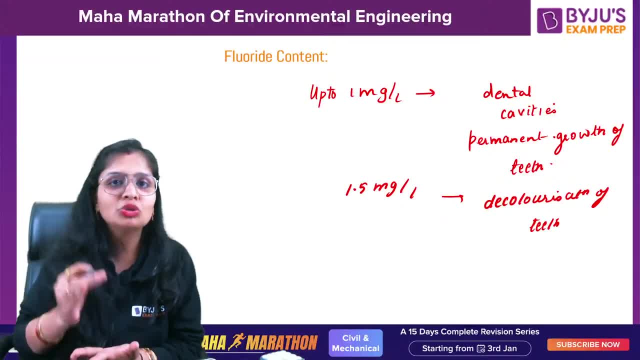 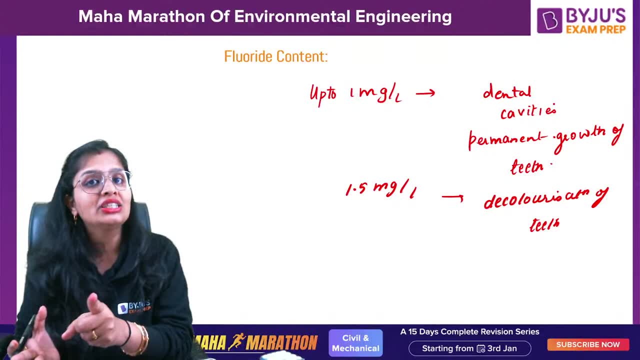 generally you will see in cities and all maximum students have the problem. maximum students or maximum people have the problem of cavities. one of the reason for this can be that in your water fluoride content is not there proper and if you can see in the toothpaste and also it's written with added 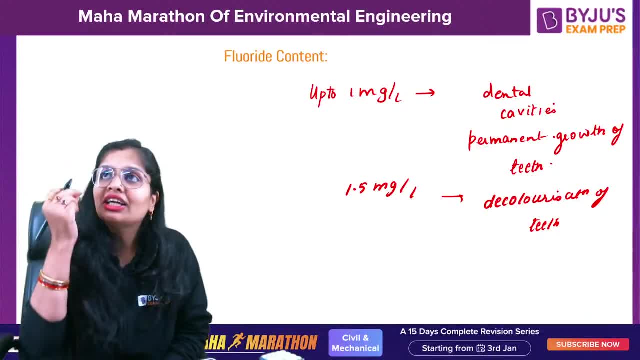 fluoride content with added fluorine, so that generally the cavities which is present on the top of the teeth- okay, not in between two teeth. I asked my dentist because I just wanted to know it. so if the cavities is present on the front of the teeth, then the cavities which is present on the 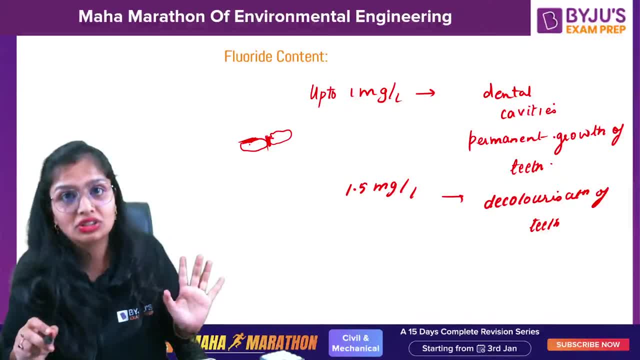 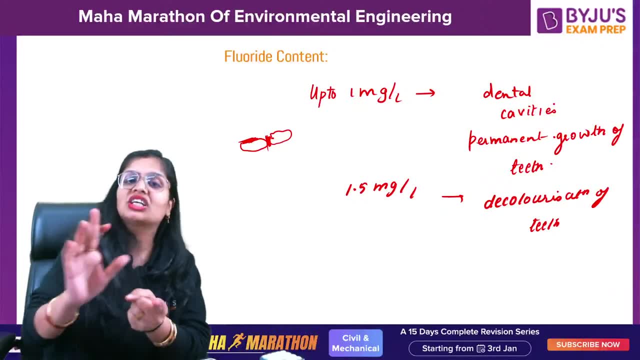 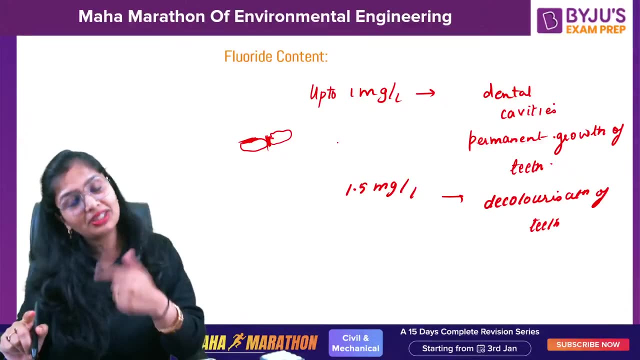 front, on the top of the teeth, that is due to fluorosis. okay. so if fluoride content, and that's why the doctor advises you to have that toothpaste which consists of fluoride, fluoride, okay. so that is the reason. if it is not there, dental cavities. if it is present in excess, like you would have seen. 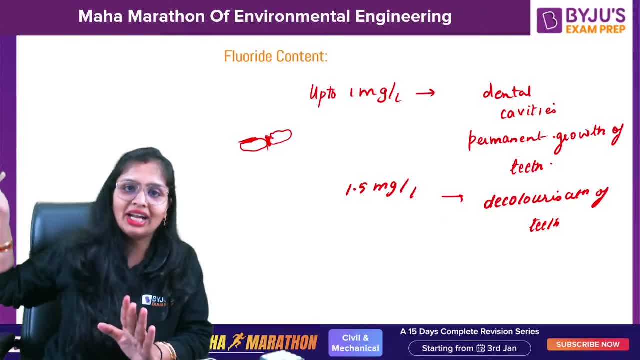 it in villages, and all because they use the underground water in that fluoride content is more that case. adult not affected by mottling of teeth? we are, we are affected, we are affected. mottling means what gala? okay, we are affected, so decolorize, but generally in cities. 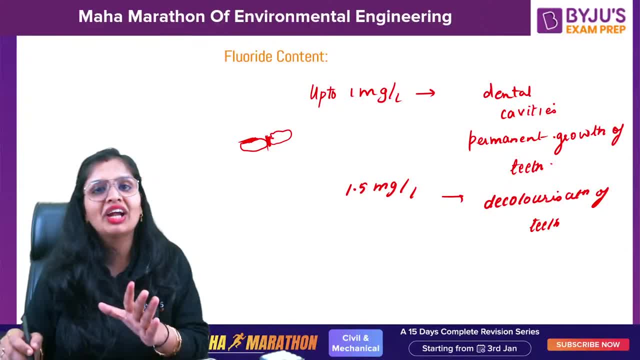 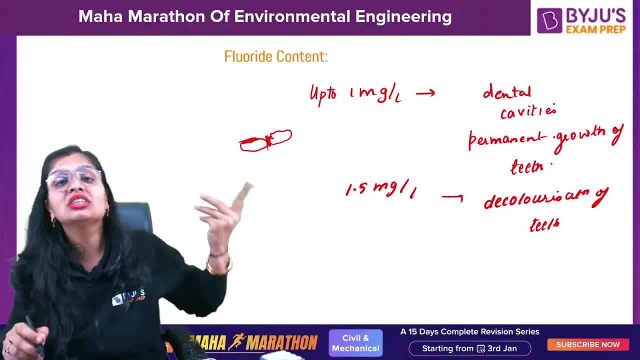 you don't find it why in sasheen cities? you don't find it because in because we take water from rivers and all, and surface water does not have excess quantity of fluoride. in maximum cases they have deficient of fluoride. generally you will find this in villages and all because there they take. 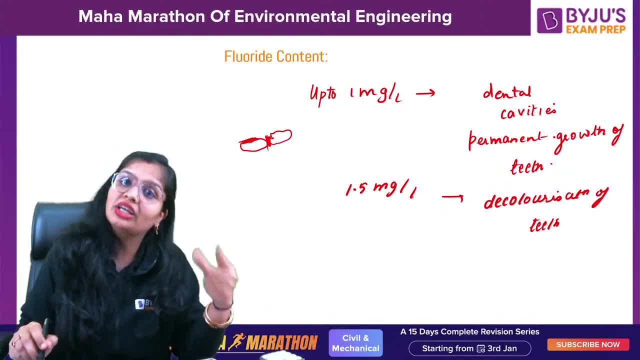 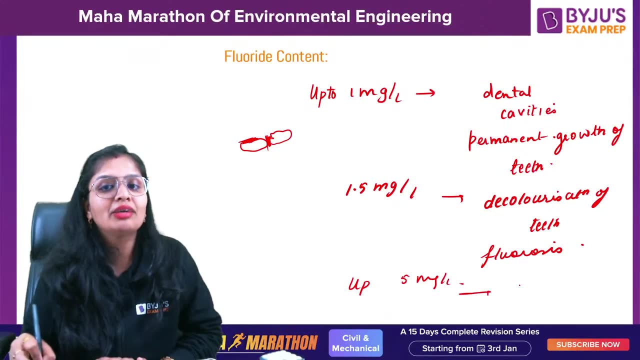 out the underground water, okay, subsurface water, so they're dissolved solids as well. so if you want to get the fluorization mottling, you go get it there, and that is known as fluorosis if more than 5 mj per liter is there. so what you will get, you will get bone fluorosis, that is known. 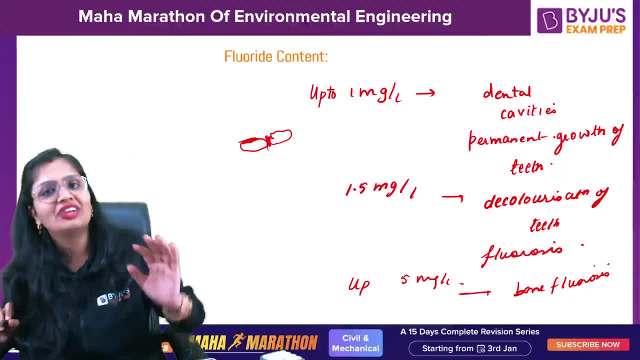 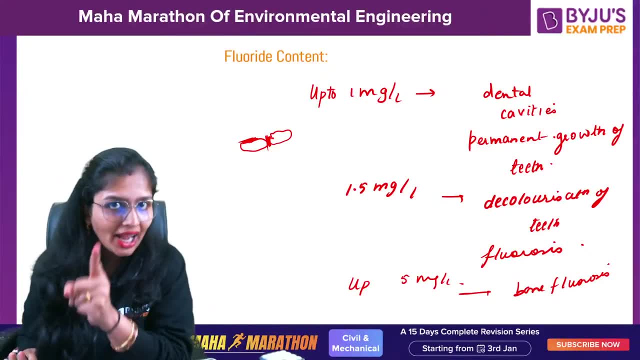 as deformation of bones. this also generally you would have seen it in villages- when the bones are not proper, they are just deformed here and there. so that is that is also risky. so i guess now you guys understood why the fluoride continue. you know the most tricky. 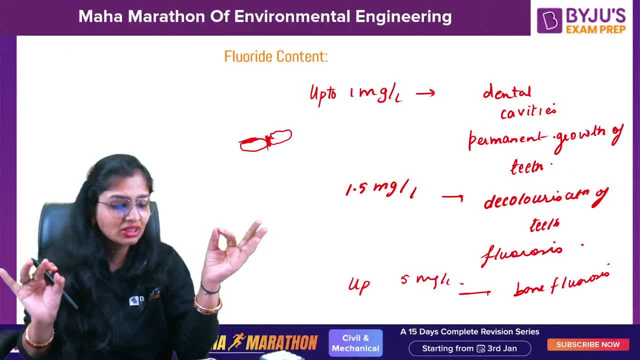 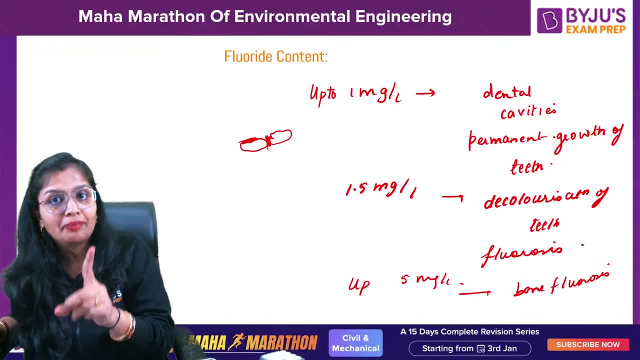 of all, the parameter nalgonda technique is used if excess of fluoride is there. it is was developed in the village. that's why, now, let me tell you one thing. that's the reason. it's not like a moral science chapter, which i'm doing, but that's the fact. generally, in villages you get more fluoride. 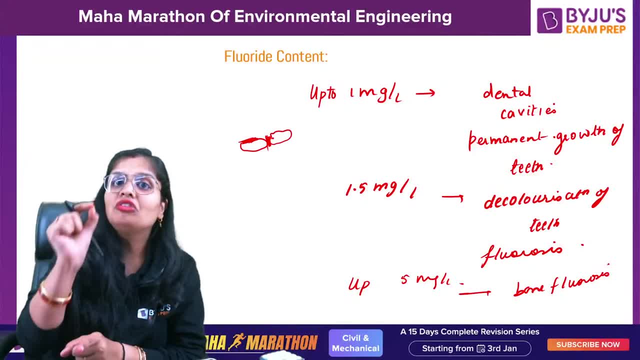 because of the subsurface water. check it out. if you are facing the problem of cavities like this on the teeth above it, the chances are that you will get more fluoride because of the subsurface water. check it out. if you are facing the problem of cavities like this on the teeth above it, the chances 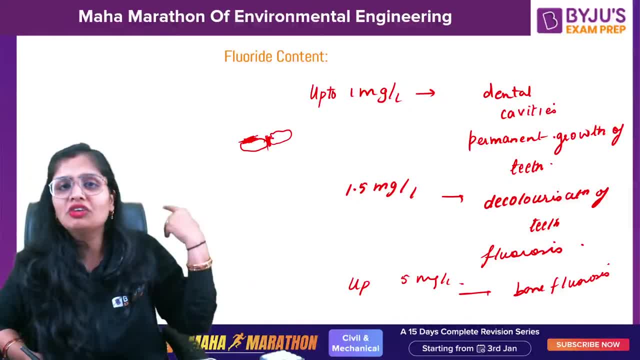 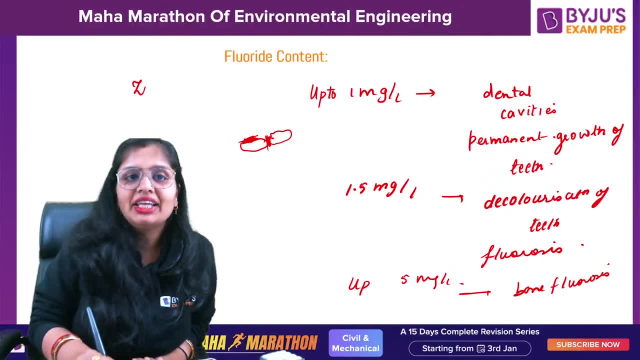 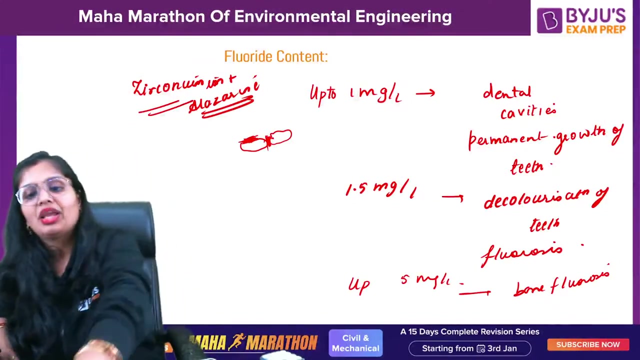 that the fluoride content in your water is less. so you can go for the fluoride toothpaste also. okay, and ma'am, how we measure? so there is a color matching technique: zirconium, iron and alazerine. this you have to use. okay, fine, oh, shall we start? biological water quality. 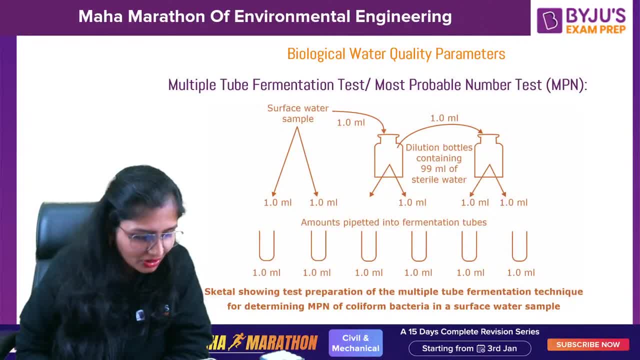 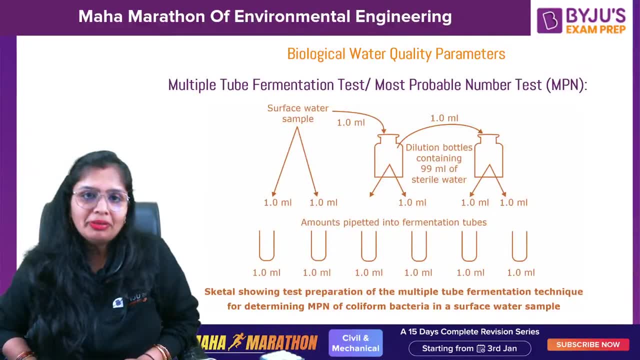 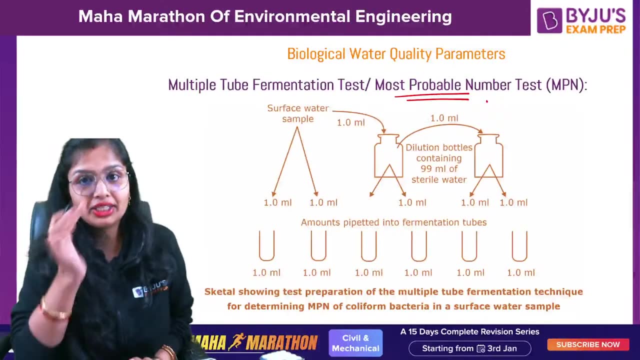 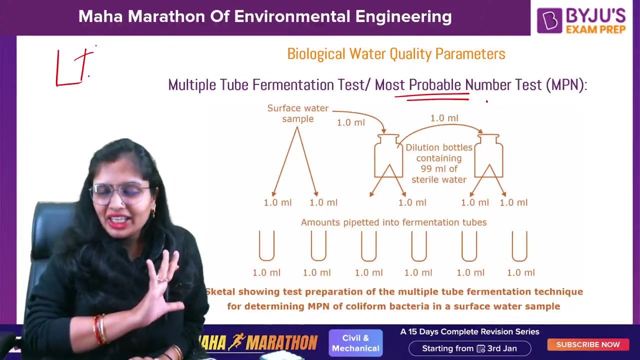 okay, so now biological water quality parameter. first we will go for mpn test, most probable test. this is very quick, i'll tell you, but very important things. what happens? there is a sample of water. this test is practically obsolete, but gate people ask questions from this test. that's why i'm telling. 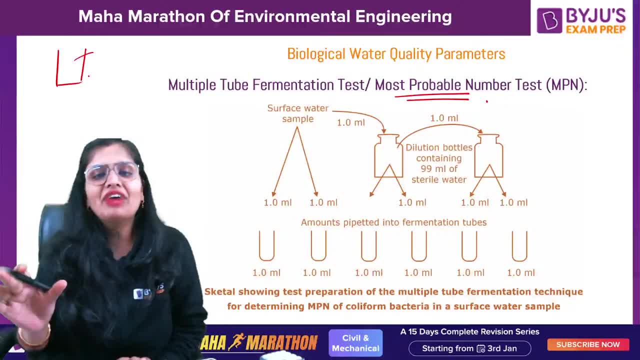 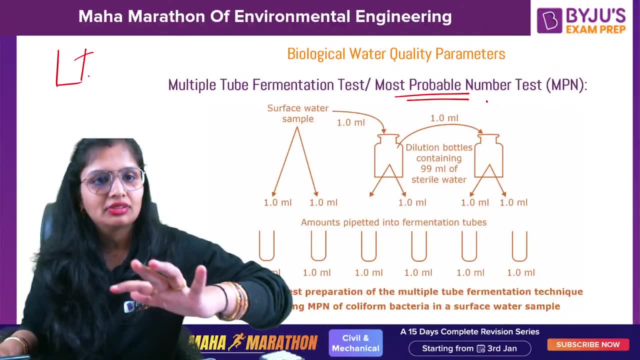 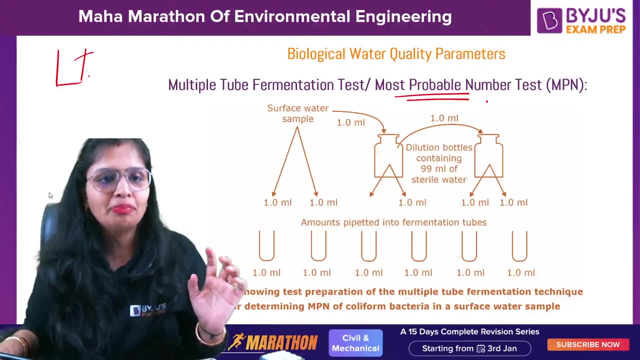 you. that's it. now what will happen? you will take five tubes. i'll take just a minute. i'll add some slides in this as- and let me tell you that, practically, if you will go and you will see, this is obsolete. this is not at all being used, but since it has been asked in the examination, we have to teach this. 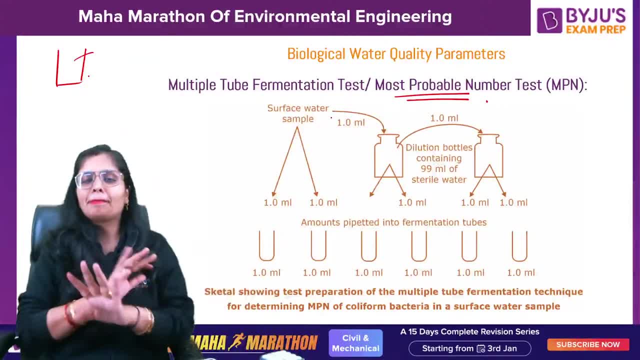 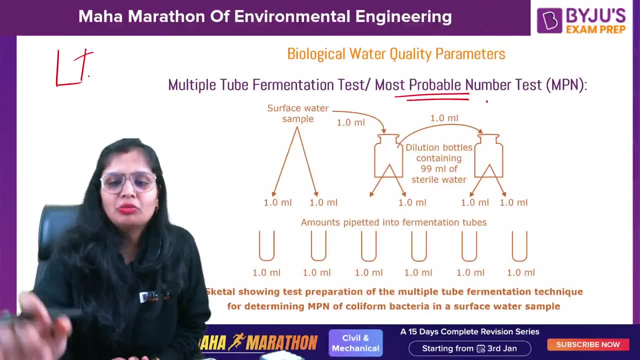 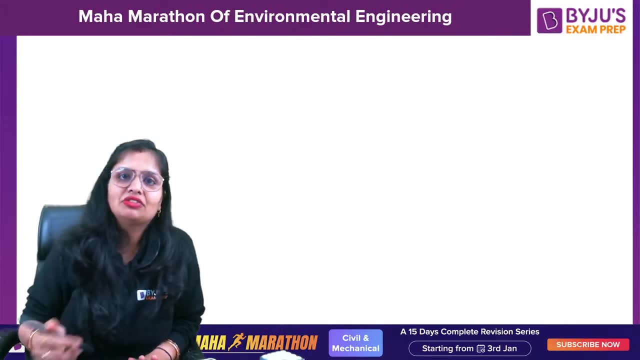 but otherwise, otherwise, otherwise, otherwise, otherwise, not useful. okay now, when you talk about mpn test- most probable test- yesterday i dealt a daily dose. so that student was asking: ma'am, deal the concept in detail. so that concept in detail takes 15 minutes at least. so now what you do? you have to take tubes, sets different, set like set one. you have to take five. 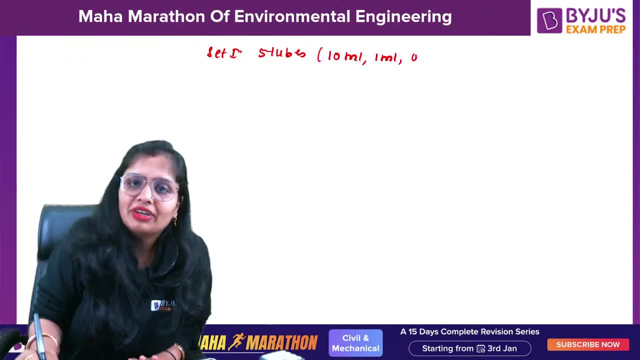 tubes of 10 ml- 1 ml- 0.1 ml. Then you have to take 5 tubes of 1 ml- 0.1 ml- 0.01 ml. Then you have to take 5 tubes of 0.1 ml- 0.01 ml- 0.001 ml. 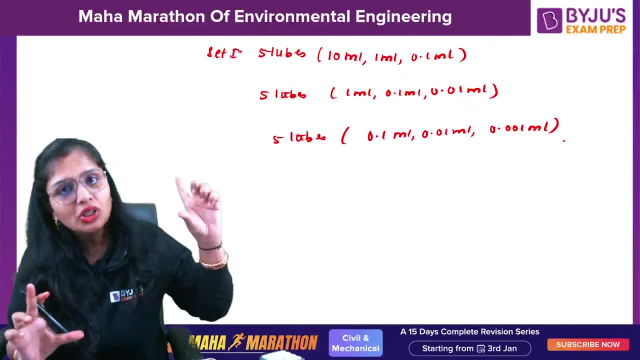 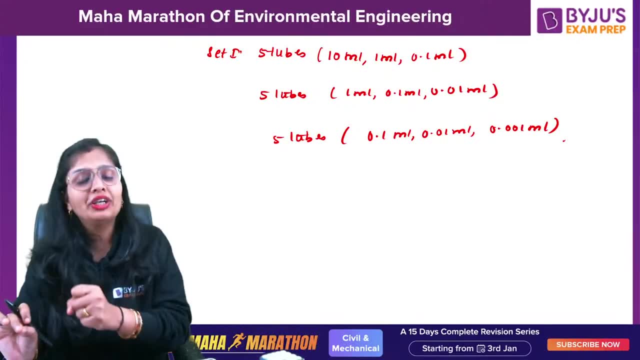 Okay, Now, actually, the total volume in every test tube is 10 ml only, But, ma'am, you have written 10, 1, 0.1. This 10, 1, 0.1 signifies 1 ml, signifies that 1 ml is the test sample. 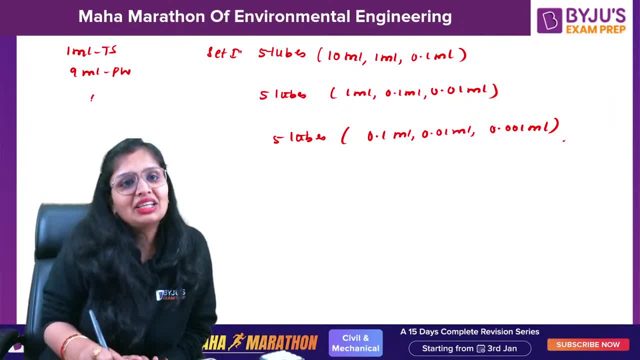 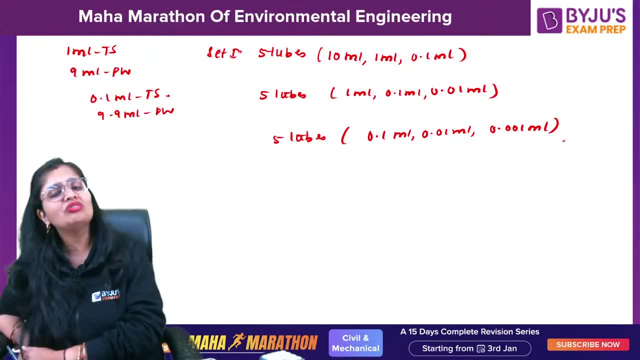 9 ml is the pure water. 0.1 ml signifies 0.1 ml is the test sample. 9.9 ml is the pure water, Ma'am, but if the same is the volume, Why you are doing it like this, Then how come I will know that in this test sample is different? 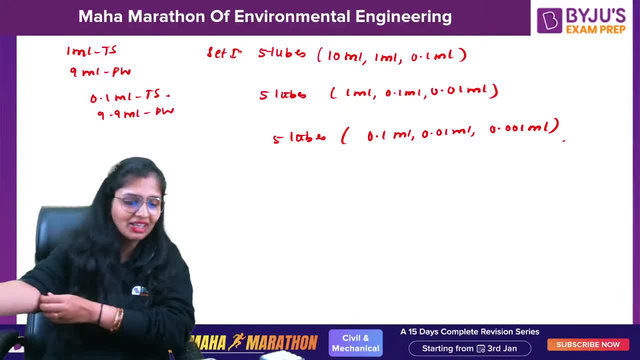 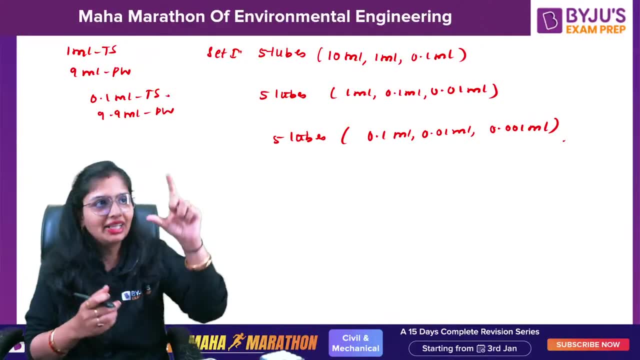 In this test sample is different. That is the reason what we have done. That is the reason what we have done. We have bifurcated for understanding, Like, whenever you give your blood sample, They take it in a test tube and they write your name. So, because everybody's blood color is same, 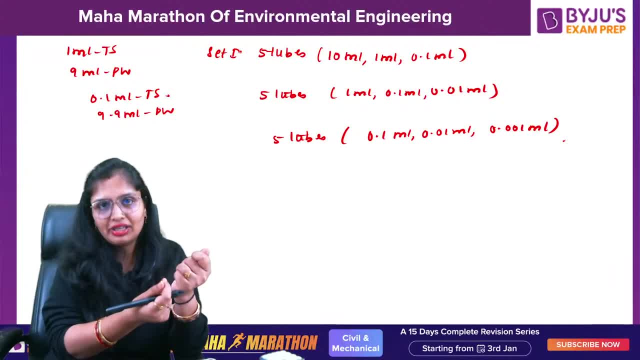 For distinguishing it, they just label it Right. Similarly, here the sample volume is same. For distinguishing it, we write 10, 1, 0.1. 1 for making it 1 ml is the test sample, 0.1 for making it understood that 0.1 ml is the test sample. 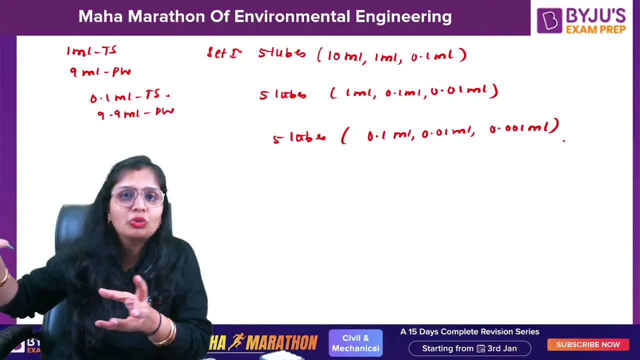 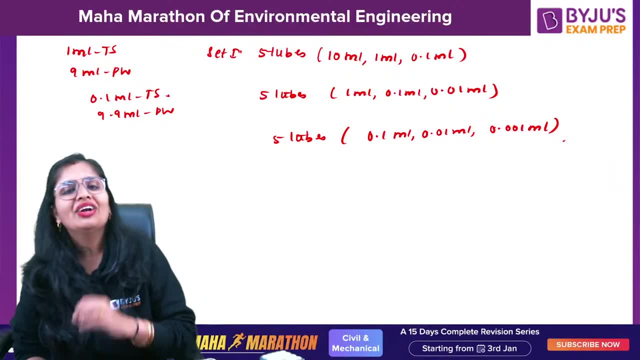 Now what you do? You add lactose growth in all of these When the gases are in the test sample, When the gases are being produced, That means in that coliforms are present. Now, technically biological water quality parameter. I need to check the pathogens. Pathogens are disease causing microorganisms. 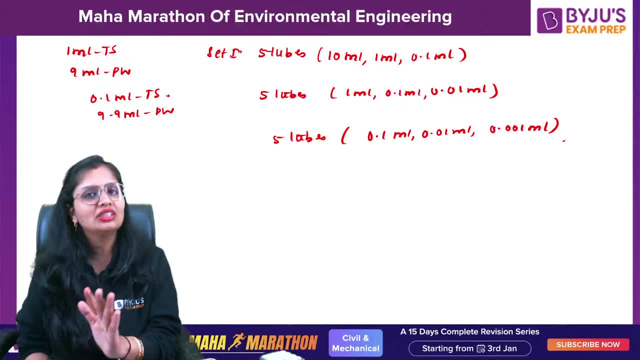 Because this water is supplied to your homes. We don't consider that you guys are water purifiers in your home. It is the prime responsibility of the government That it should supply you water Which you drink without even getting it purified. Nothing should happen to you. So now, technically, you have to check the pathogens. 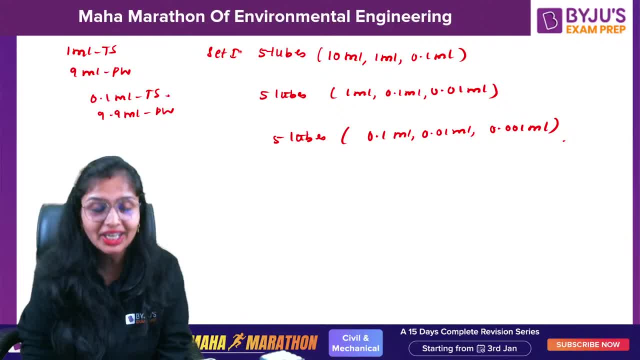 Technically we use should test pathogens, But it is expensive, It is time consuming. So rather than testing pathogens, We test, We test what We test: the coliforms. Coliforms testing is easy And it's like: whenever coliforms are there, Chances of pathogens present are there? 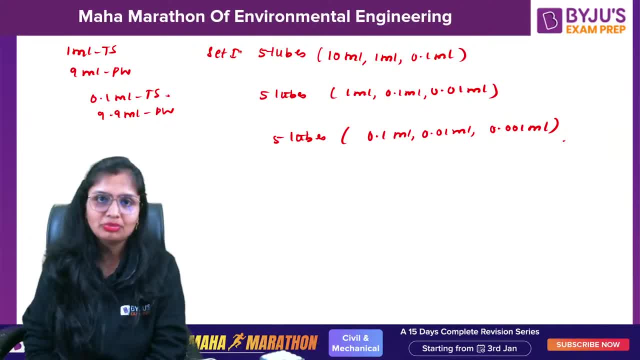 So, rather than on everyday basis, We test the coliforms. Now comes the next question: How we do it. So first we add lactose growth In all the samples, In all the test tubes, And we put it in an incubator. Incubator is like your microwave and all. 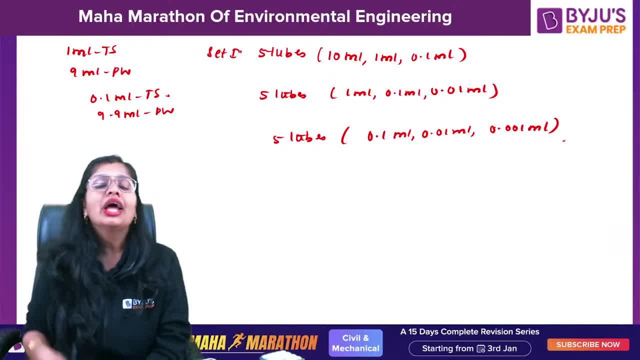 Where ambient condition and temperature is maintained. Now what happens is If gases are evolved, That means it is a positive test. Now, 5 test tubes of heat. Let us suppose here 4, Here 3, Here 2, Here 3, It is 2, Here 1. 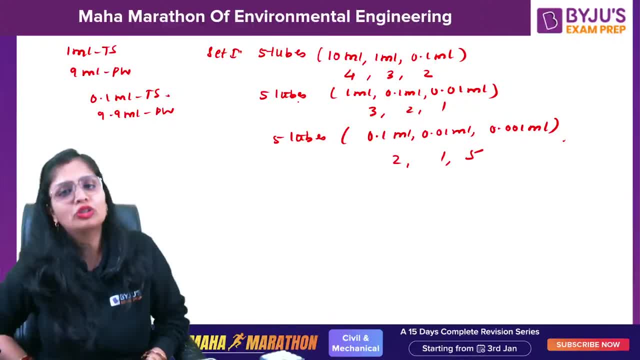 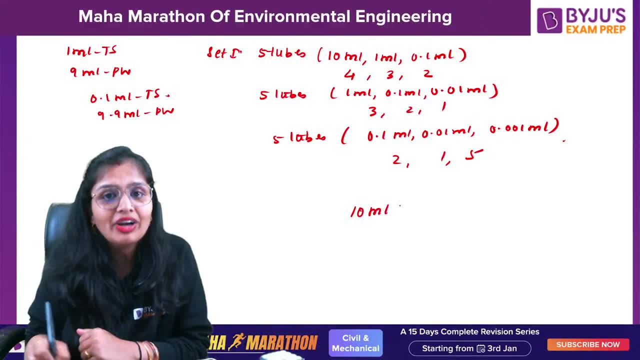 Here 2. It is 1, Here 5. These are the positive results. Now, according to the code, A table like this: The table is given to you For 10 ml, 1 ml, 0.1 ml. It is not given for any other dilution. 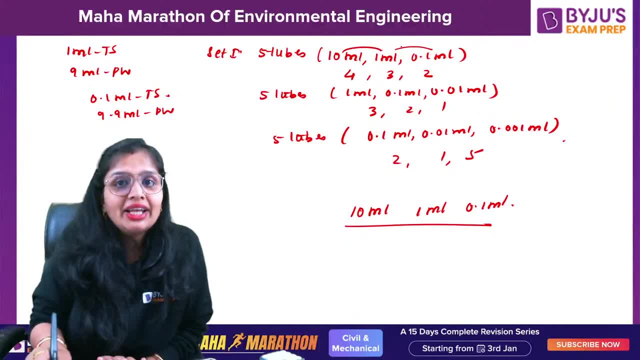 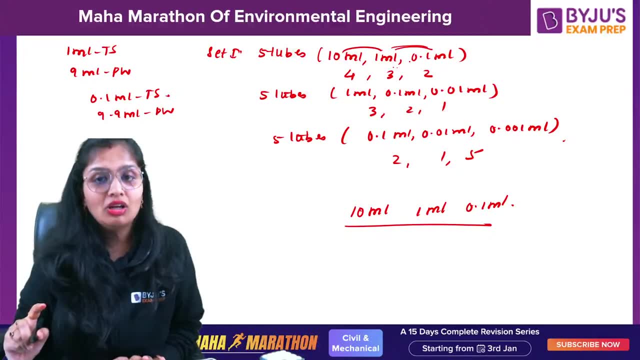 It is given, And remember, No adjacent dilution should be more than 10 times. You can see this: 10, 11.1. So it is only 10 times diluted, Firstly. Secondly, the table is given for 10- 1.1. Now I am telling you a very important thing, guys. 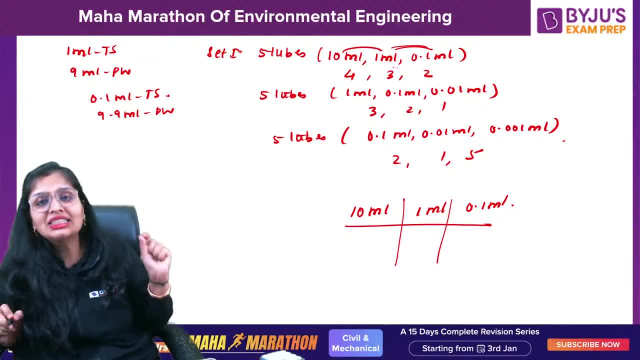 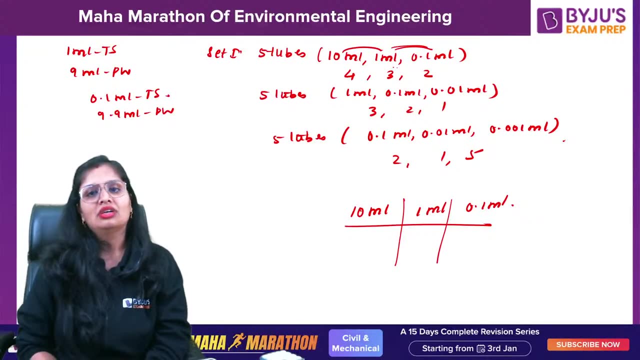 Listen to me properly. If all the samples positive test results are given, You will receive positive results. Whatever the results come, You will take that sample. You will take that sample where that dilution is maximum. Now tell me which one you will take If on all the sets you are getting positive results. 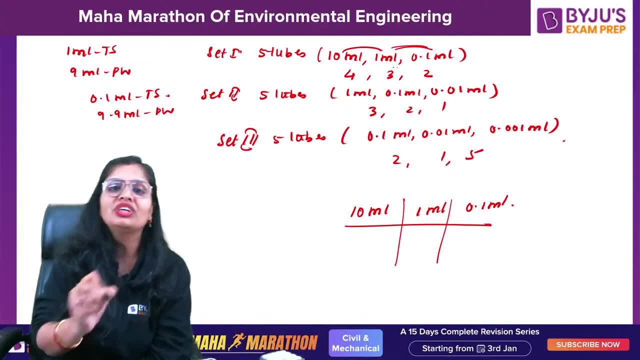 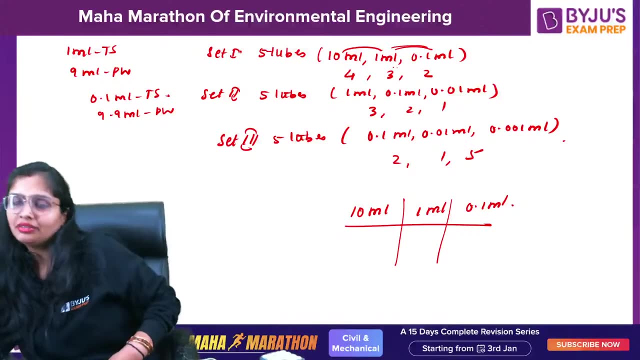 You will take the set in which dilution is maximum. Which set will you take? This is as per the code. Tell me Which one you will take. you will set Take set 1, set 2, set 3.. Which one you will take? Hurry, hurry Dilution. 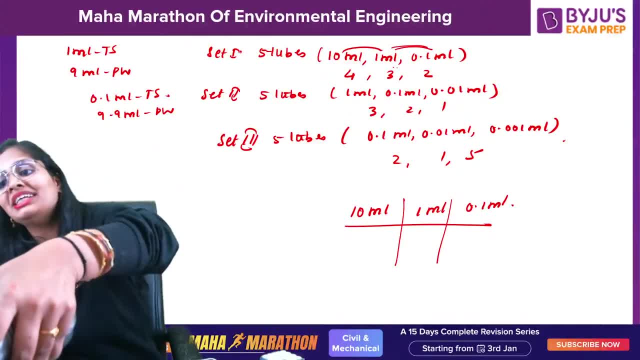 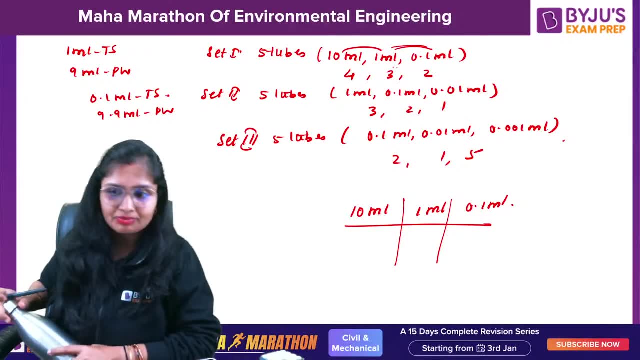 is maximum, Dilution is maximum. This means maximum amount of water is added, Dilution is maximum. So for 215, if, let us suppose, the NPN is 30,- okay, you checked it for 215.. You check example I am taking. I am not giving you the exact value, the 30, you will write. 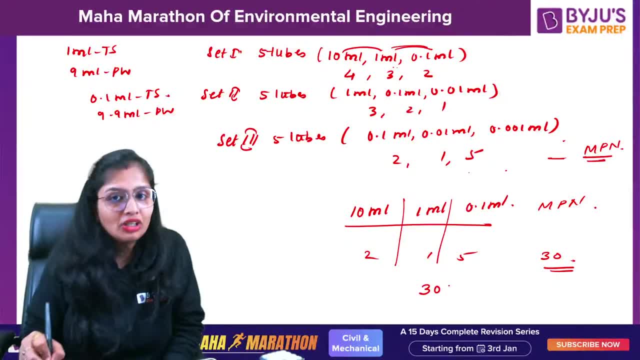 it 30. No, Why? Because NPN is maximum. So for 215,. if let us suppose the NPN is 30, this 30 is for 10, 1.1 ml. This sample is how many times diluted. This is 10, this. 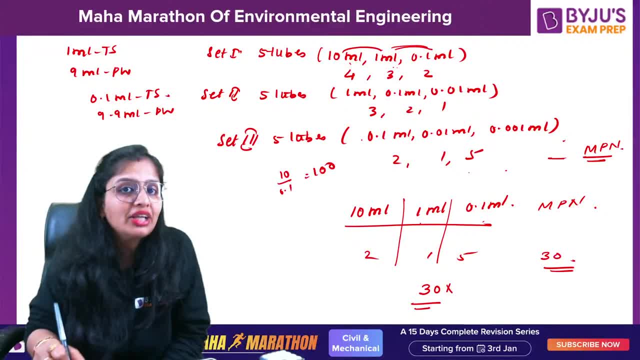 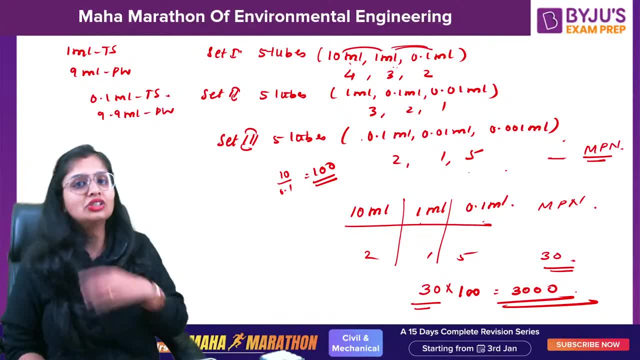 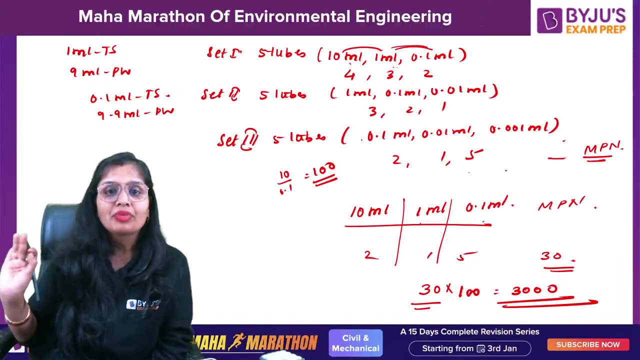 is 0.1.. How many times diluted? 100 times diluted. So the NPN you have to multiply by 100, you will get 3000.. Understood This, you should know. This, you should know Now. 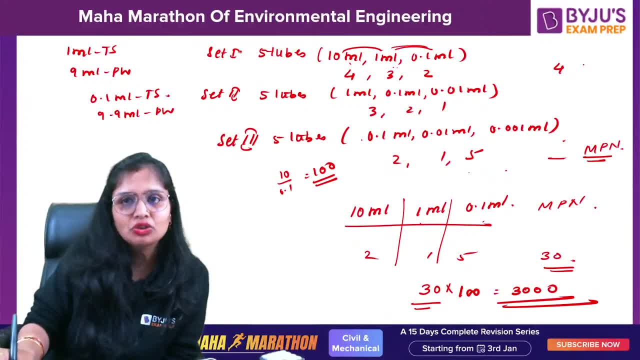 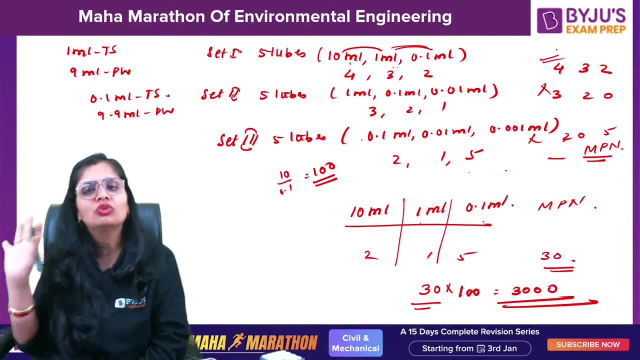 what if? if in this sample this is: let us suppose 4, 3, 2,, 3, 2, 0. So 205, then discard this 2, directly you will get for 4, 3, 2,. okay, Directly you will. 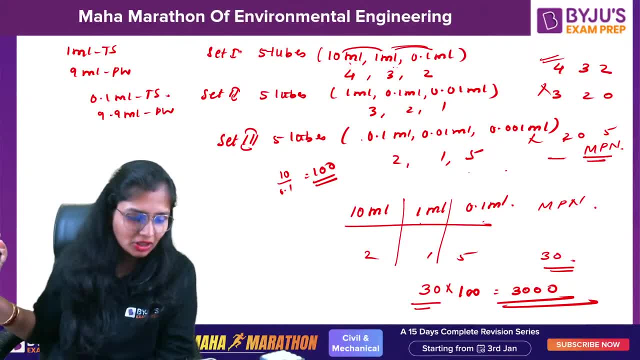 get for 4,, 3,, 2.. So in this manner you have to do it. Smallest dilution, smallest dilution we take means okay. I am saying if in all the if in all the sets we are getting. 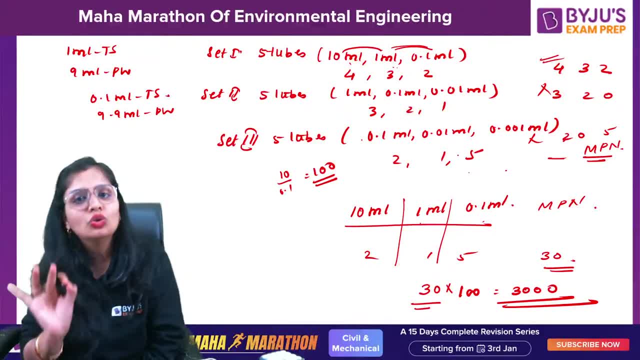 the positive results we will take those set in which the dilution is maximum. So the dilution is maximum in this one. Why dilution is maximum? Because here 0.1 ml is the test sample and 9.9 ml is the pure water, So the dilution is maximum In this case, that is. 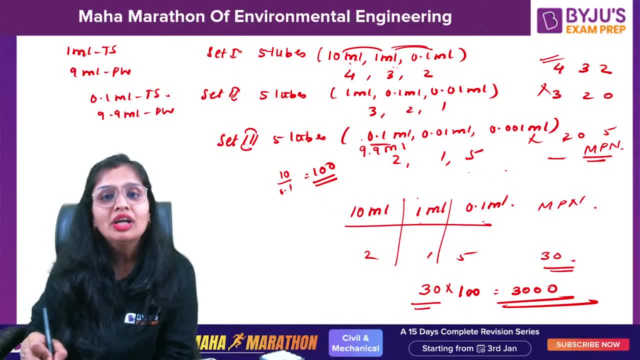 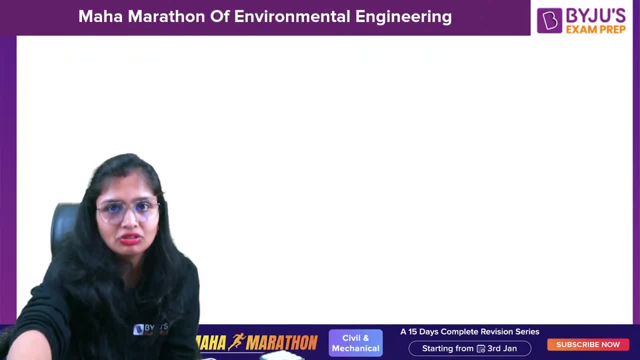 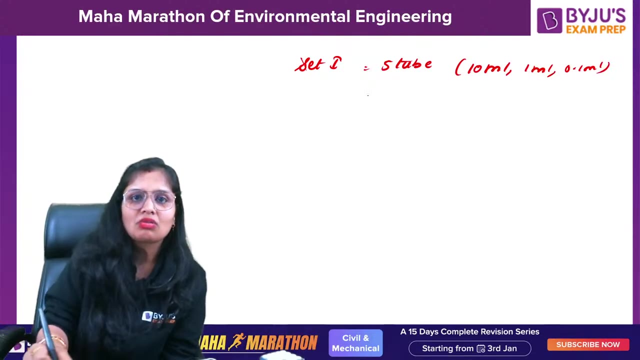 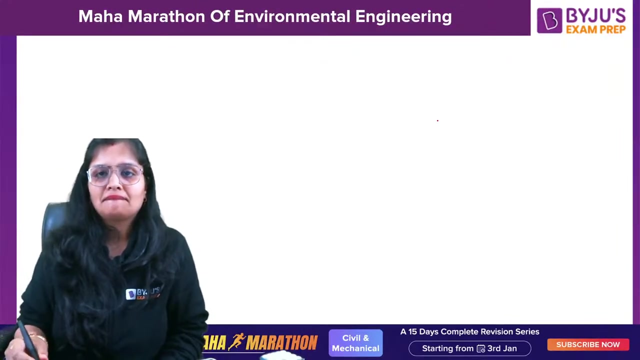 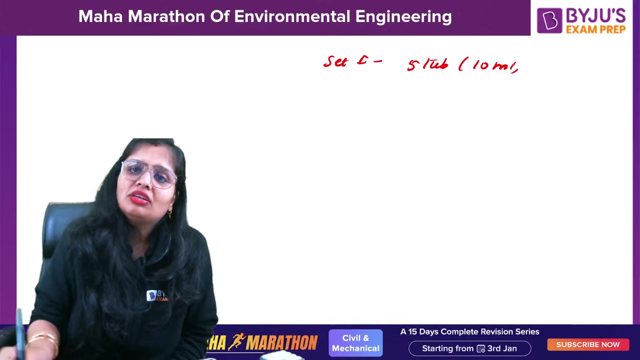 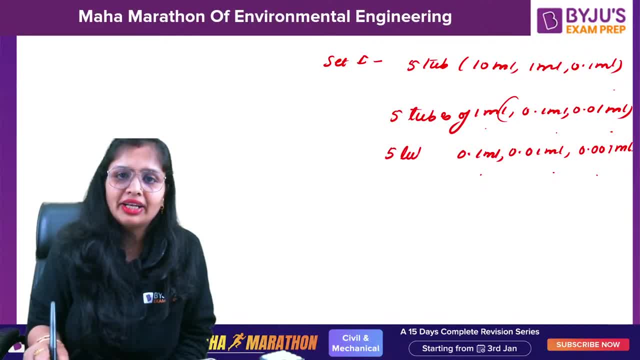 should not be. the dilution should not be more than 10 times 5 tubes. Now what I said? in all of them the result was positive. Let us suppose 421,, 210.. No 212, let us suppose, And this is 123.. So in this case we take that dilution. we 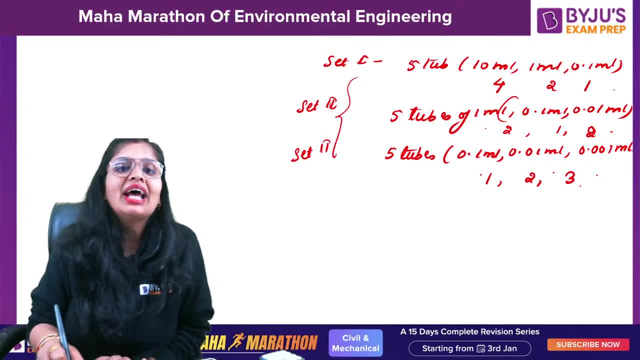 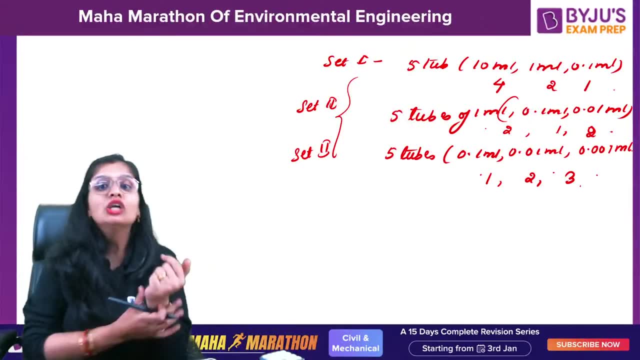 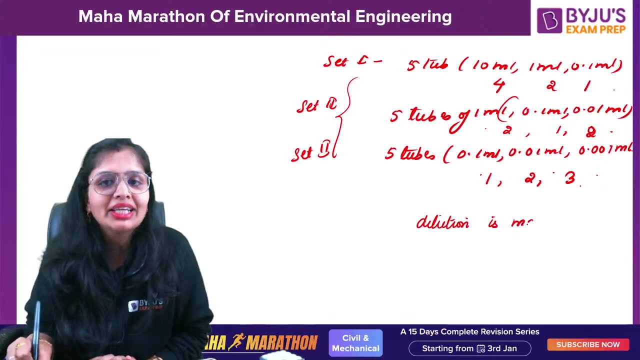 take that set in which dilution is maximum. Dilution maximum means we say that this is concentrated acid, this is diluted. Diluted means water is there. So we will take those set in which dilution is maximum. So dilution is maximum in the case of 123.. So let us 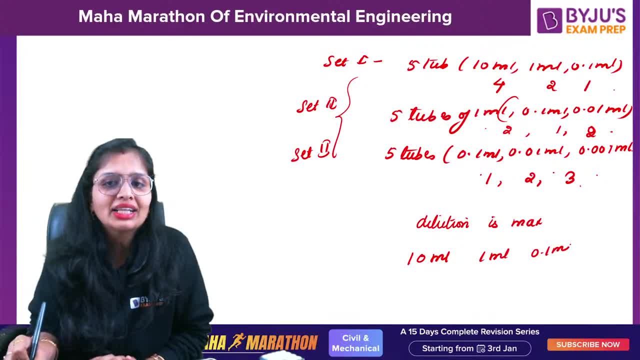 suppose. But the table which is given to you, as per the code, that is for 10, 1, 0.1.. So let us suppose the MPN comes out to be 30. But this is for 10, 1, 0.1. You want it for 0.1, 0.01, 0.001.. So you would check that. 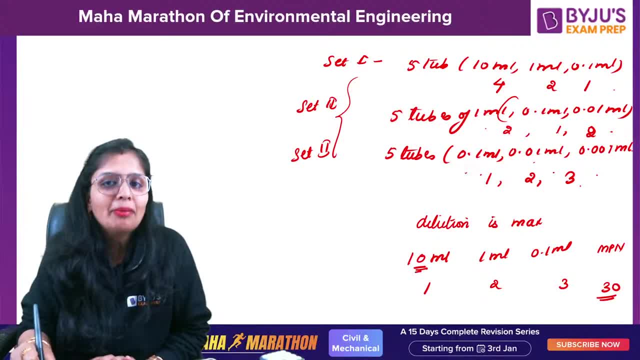 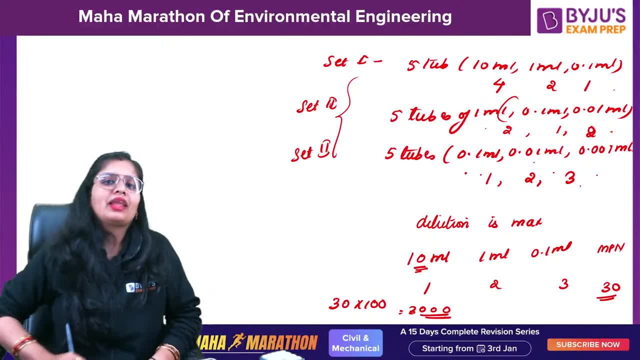 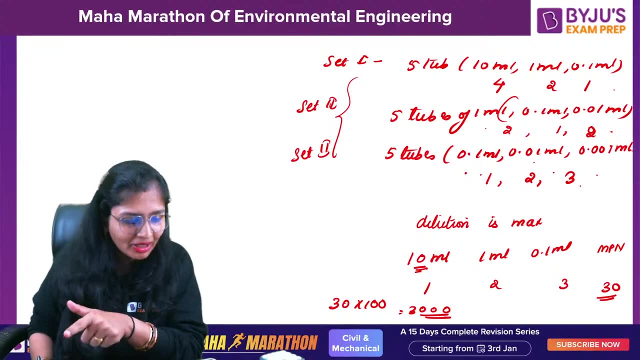 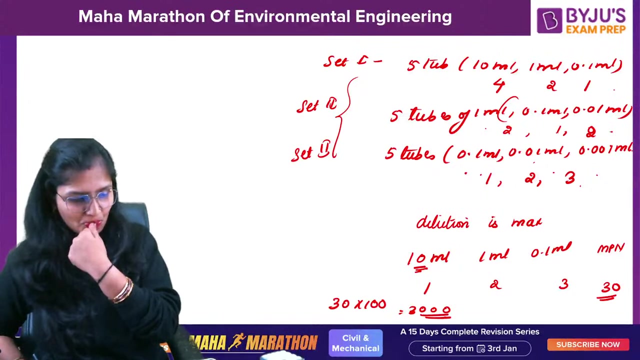 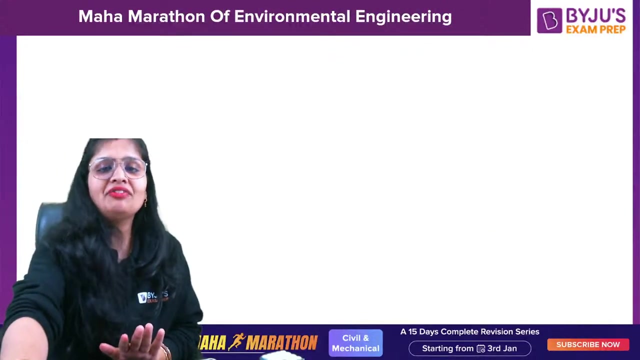 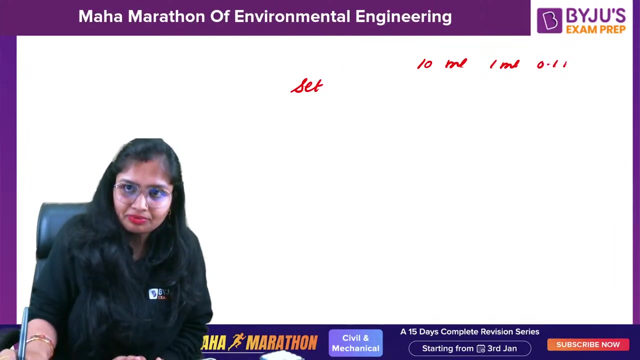 this sample as corresponding to this sample. this sample is 100 times diluted. That is the reason you multiply by 100.. Clear, Clear, everybody Dimple. you were asking me, or you were telling me, And Arun also. Okay, Now let us check it out. And if it is 0, is there Like if set 1, 1,, 0.1, 0.01.. 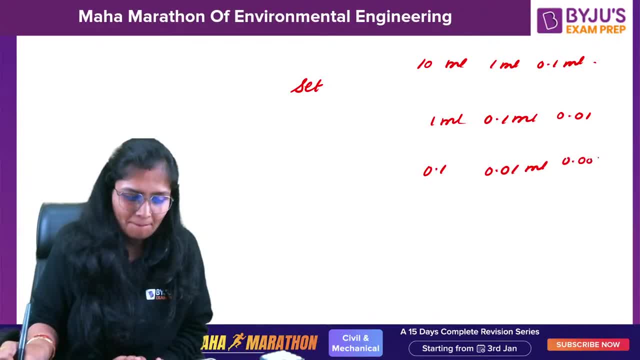 Or not. Nb questions accepted. File 2, 0.. 2… No 5, 2, 2… 2, 2, 0.. Which set you will take? 1.. 2 or 3?? Which set you will take, guys? 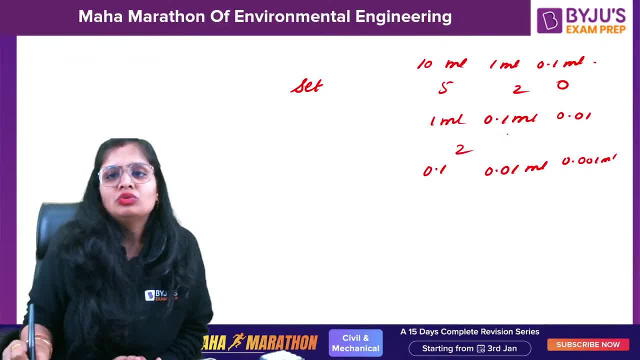 No, no, you had asked that in the start. Some smallest one in the beginning, minimum. I felt that if there is any doubt, Arun Yes, But darling, I would joke that it is 10%. it has been negro at the beginning. 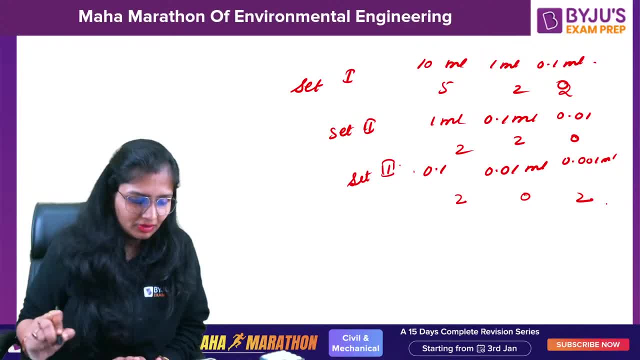 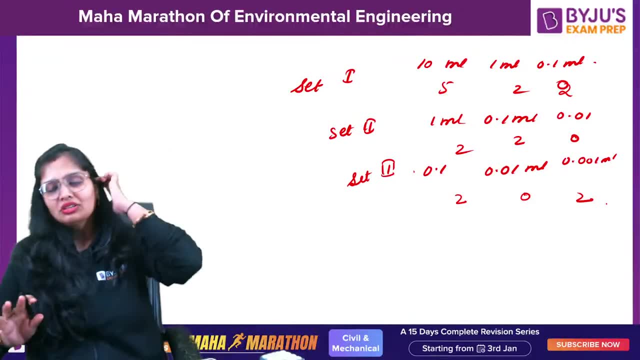 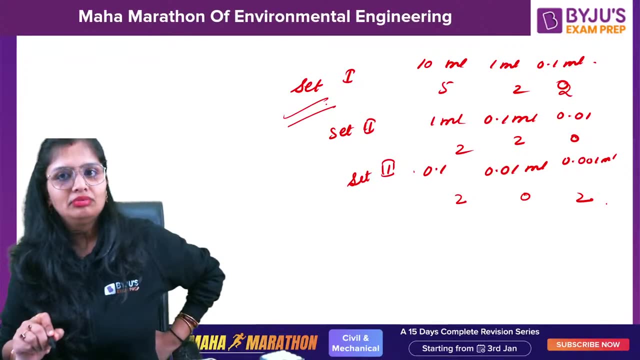 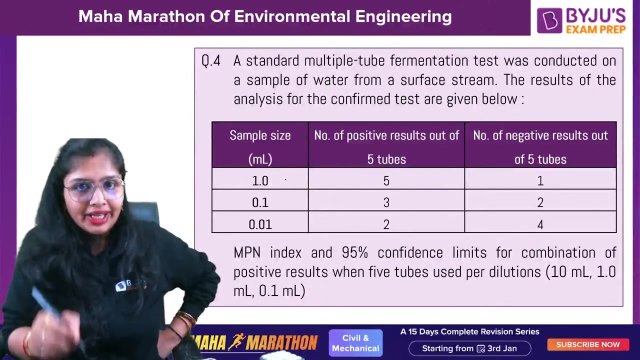 But it is X. What are your ideas? arm Is it X, X. Which set you will take, in this case Set 1.. Okay, Now let's check it out. See, in this the sample is 1.1.01.. 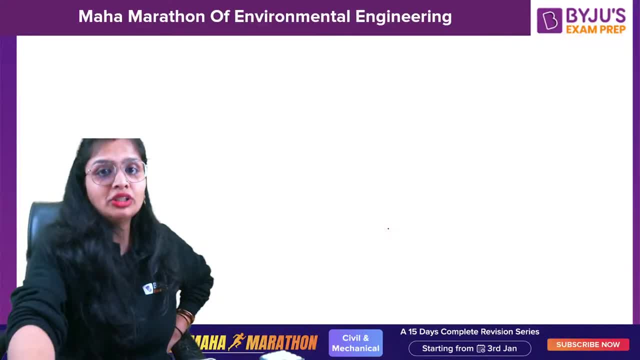 Okay, 5.3.2.. And one more thing. you guys should ask me, ma'am, if every set. shall I tell you one more thing, If, let us suppose, 5.2.0.2.0.3.0.3.2.. 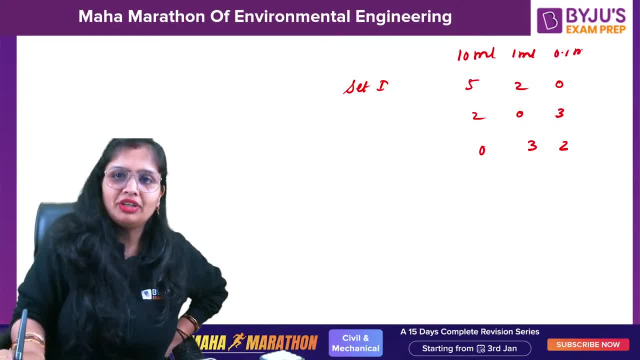 10 ml- 1 ml- 0.1 ml. And this will be 1 ml- 0.1 ml- 0.01 ml. And this is 1 ml- 0.1 ml, 0.01 ml- 0.001 ml. 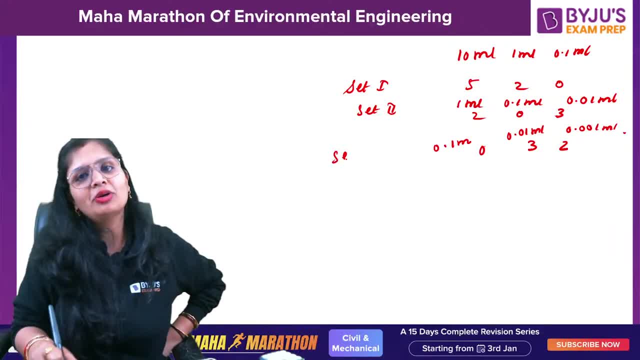 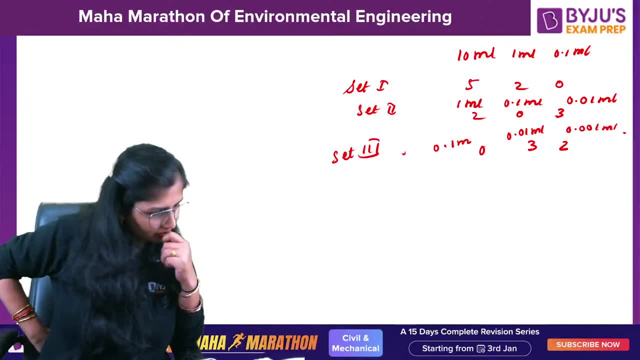 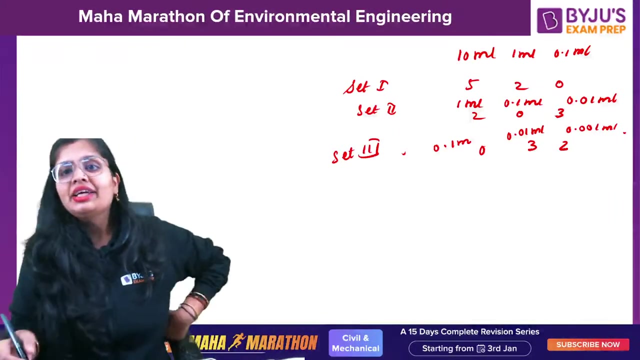 See, now we are testing Which set you will take. Come on, guys, Based on your brain, tell me which set you will take First. I want the answer. Okay, Okay, Feel First of all, you will take those set in which, if every test you are getting 0, you will take that set in which second dilution is positive. 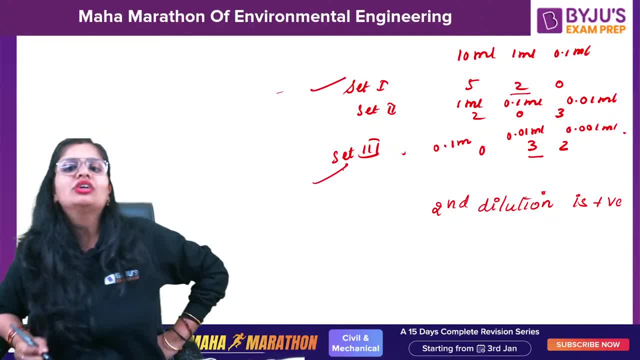 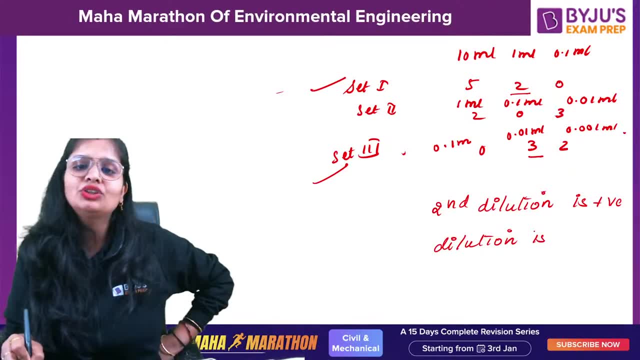 Second, dilution is positive for set 1 also and for set 3 also. So in this case, as per the chordal provision, you will take that set in which dilution is minimum. So dilution is minimum, That means less amount of water is added. 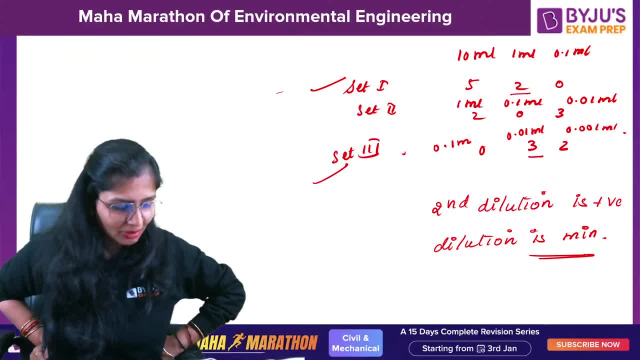 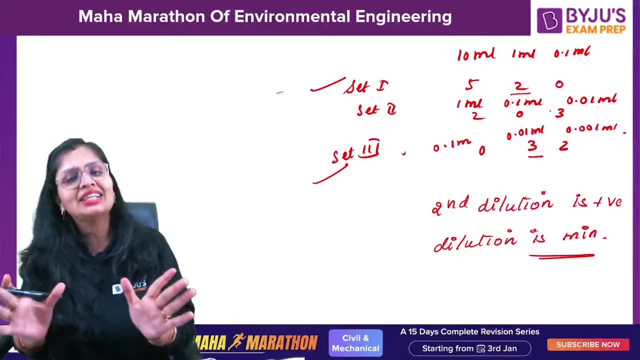 So it is added for 1 has maximum No, not based on That maximum No, no, no, That logic is wrong. Firstly, you will check if in every test 0 is there. So you will check that the second dilution should be positive. 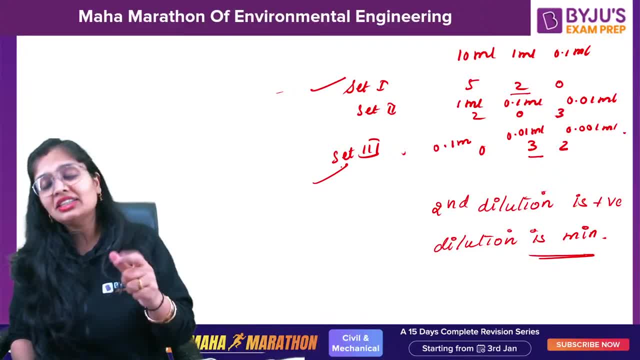 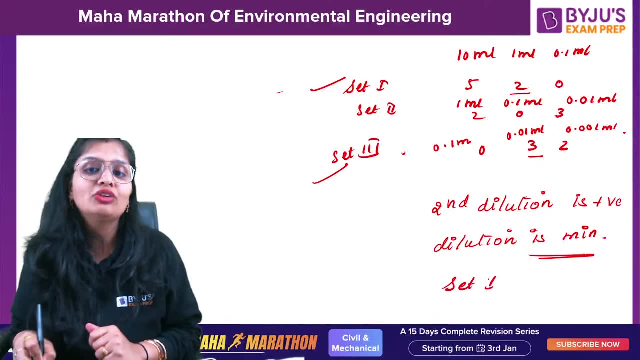 It is positive for set 1 and set 3.. After that, since 2 sets are there, you will check that in which the dilution is minimum. Dilution is minimum for set 1.. Dilution minimum means less amount of distilled water is added. 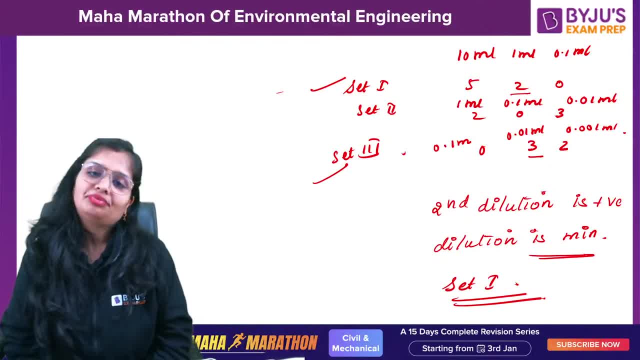 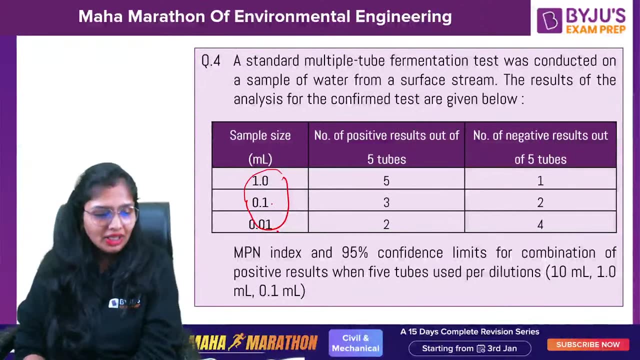 Clear. everybody Understood the concept, Understood it. Diksha Dhanush, MVS Devanshu understood everybody. Okay, Now now talking about next. Now see, in this question we are not interested with negative people and negative tubes. 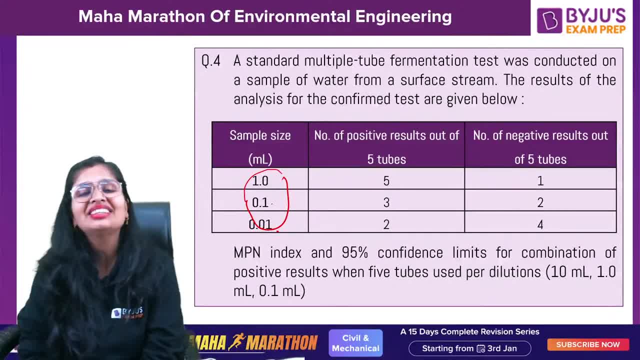 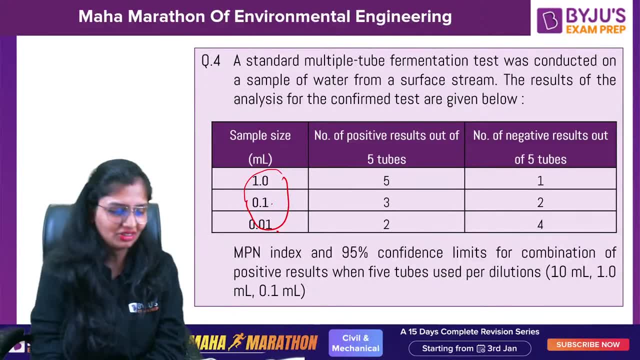 Okay, Here we go for minimum dilution: Girish. this is as per chordal provision. beta. This is not which I created it As per the chordal provision It is mentioned. Okay, So 1.1.01 test is given to you me. 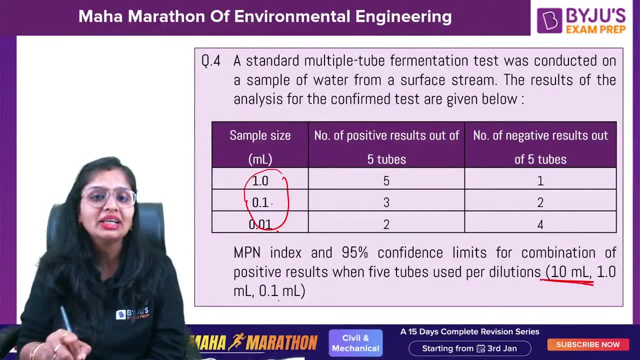 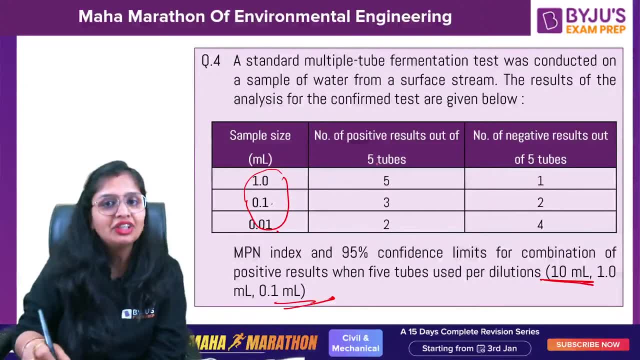 But remember always the combination MPN which you will get. you will get it for N1.1 ml, Just check it out. 5.3.2.. 5.3.2,. what is the MPN? 44.. 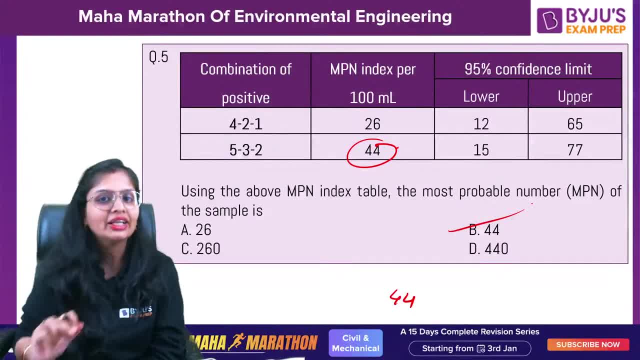 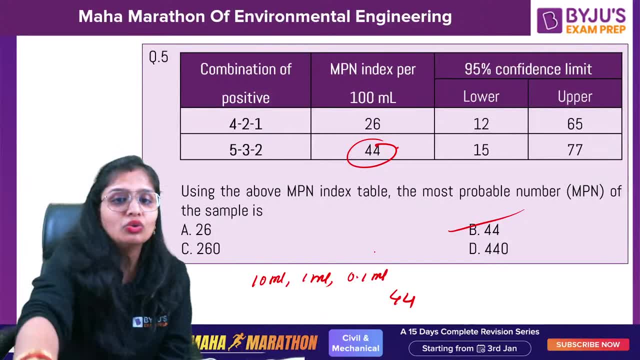 Without even seeing, you will mark B. Is B the correct option? No, Why? Because this is given for 10 ml, 1 ml, 0.1 ml. In the question it has asked me for 1 ml. 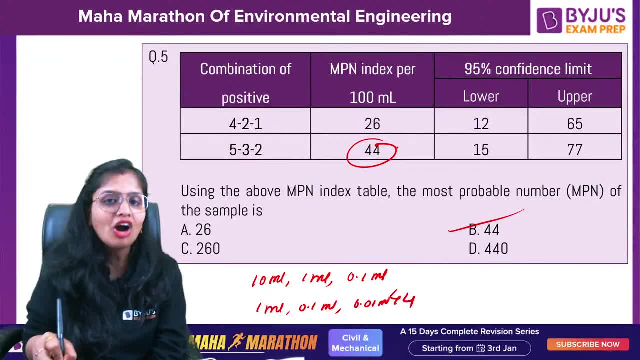 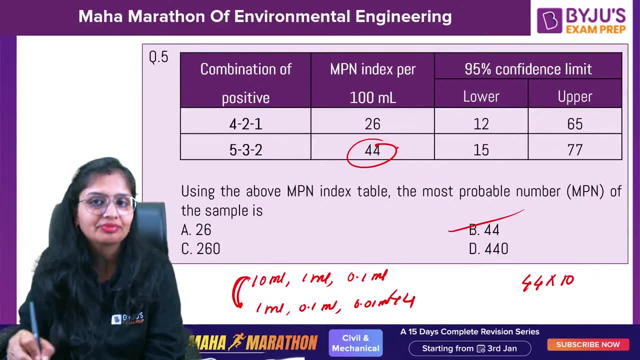 0.1 ml, 0.01 ml. How many times it is diluted? 10 times. So that is the reason: 44 multiplied by 10.. Understood everybody Who was asking, Lagom, everybody, It is clear. 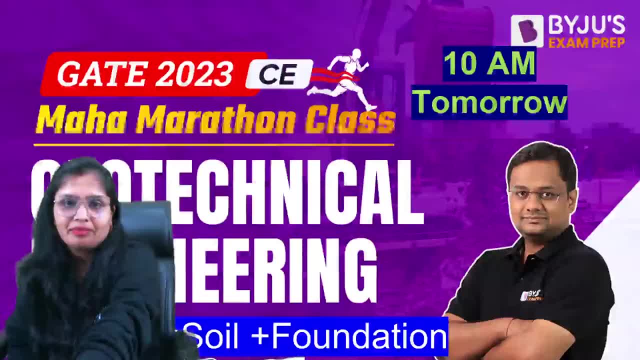 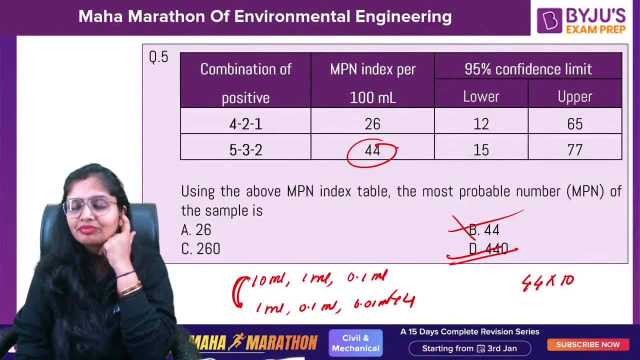 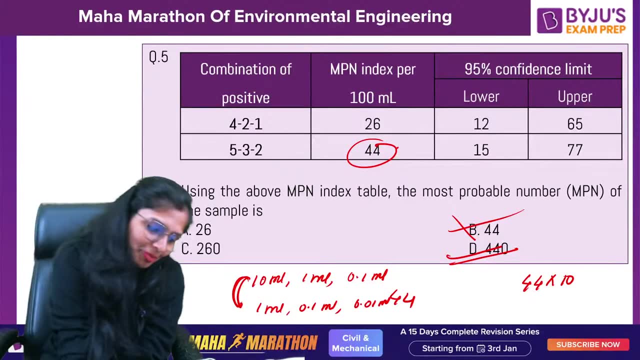 Okay, So this was your MPN. So this: With the help of this, we complete the second chapter. Any doubts is there? Tell me Any doubts. Shall we complete treatment of water. Then we will give a break. 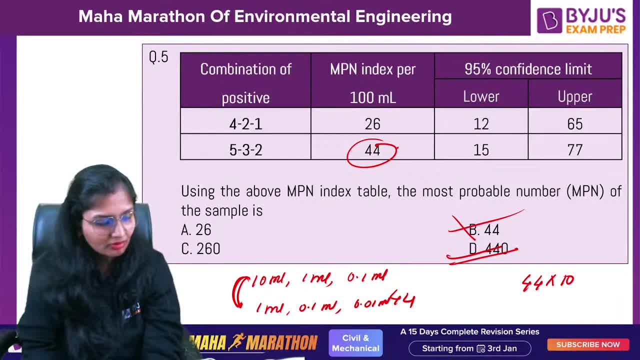 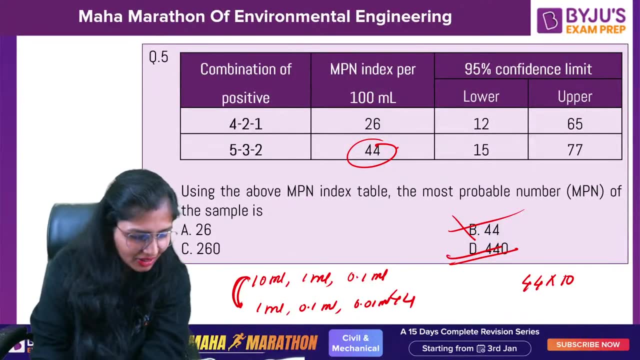 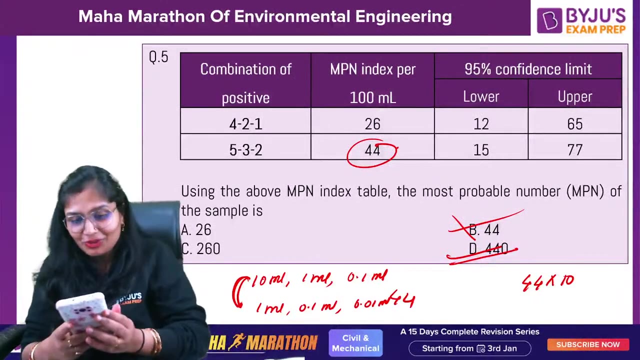 What do you say, guys? Coliform index test. Coliform index test is the reciprocal of the The smallest quantity of B coli test. 5 minutes break. Okay, Let me create Now also- I do not know how to do a poll- 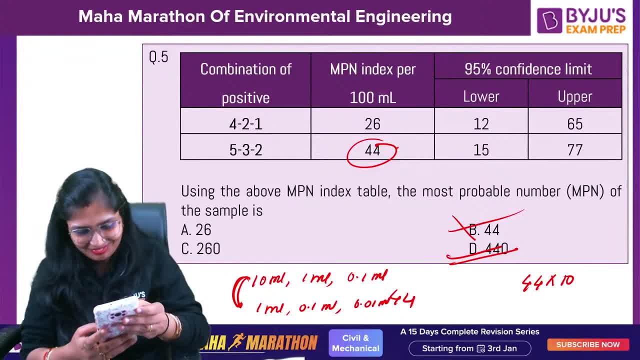 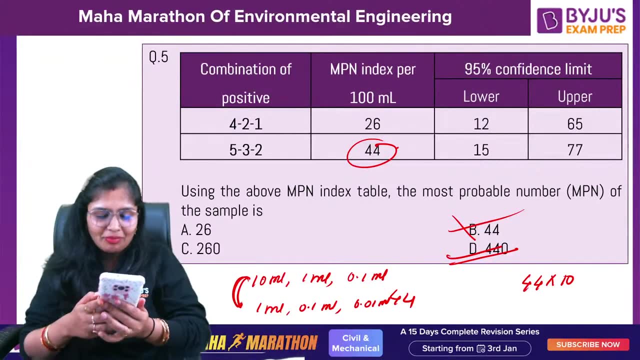 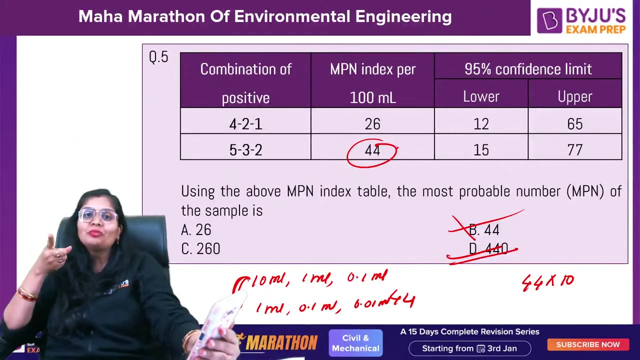 Okay, Everybody wants break TP low- Ok, Fine, I will give you only on one condition: When everybody of you will promise that nobody will go. Otherwise, what happens after break comes, some people goes, that okay, fine, I will see the recorded lecture. 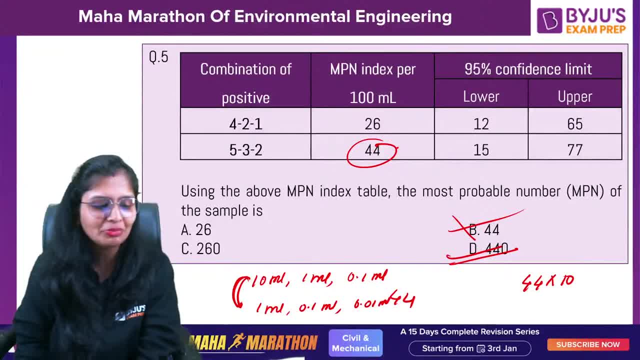 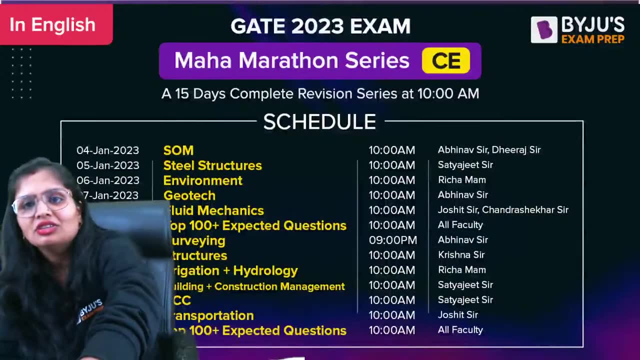 I will make sure that this lecture becomes private. Promise me, I have come now. You have come late, right, Dhanush? Promise me, Okay, fine, Then we will take a five minutes break. Fine, So five minutes break. 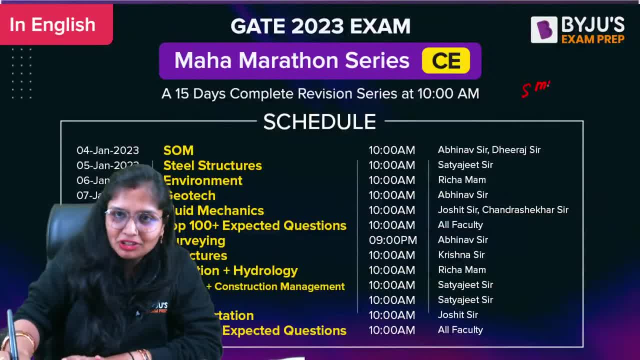 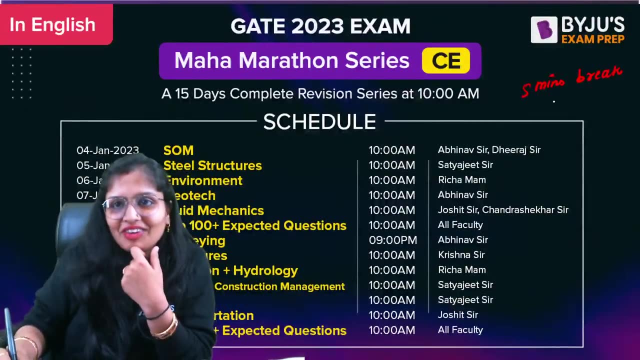 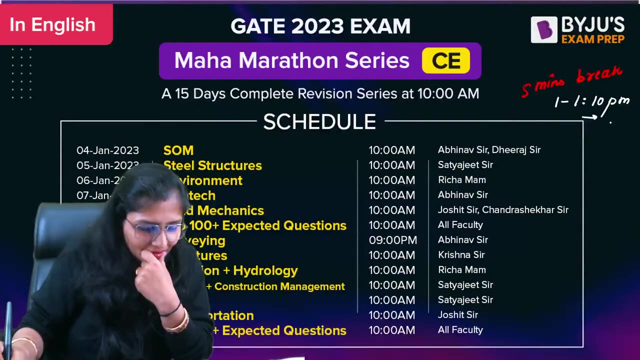 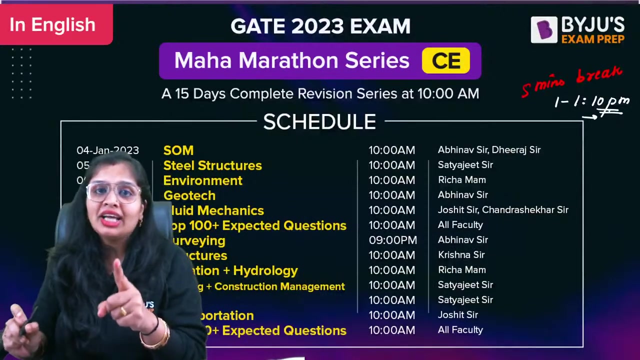 Fine, Five minutes, Five minutes break, Promise me. You guys cheat me, man. How much time is taking? now 1.10 pm. I gave you eight minutes. Give us five minutes. girish guys, come on time, because i'll be starting treatment of water and i'll be. 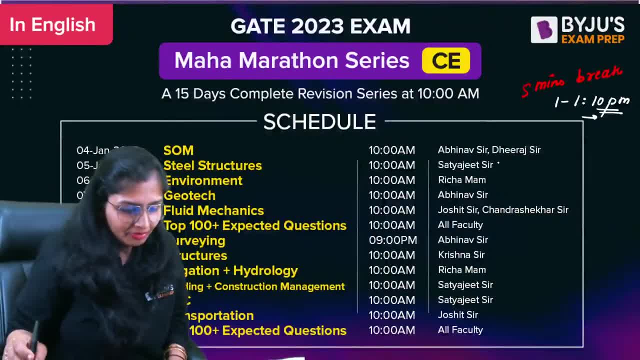 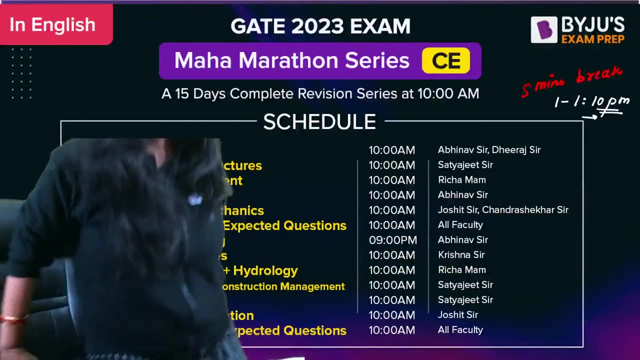 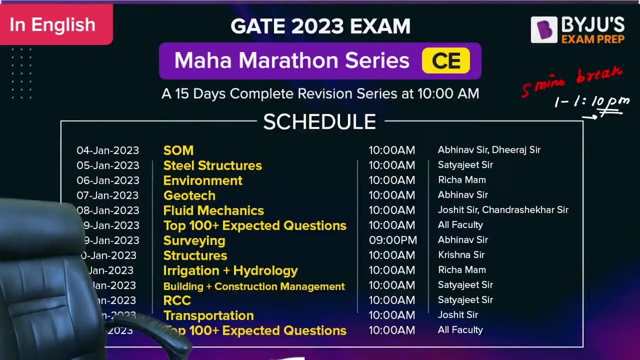 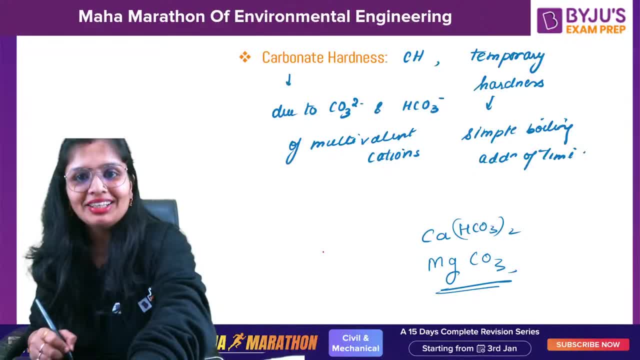 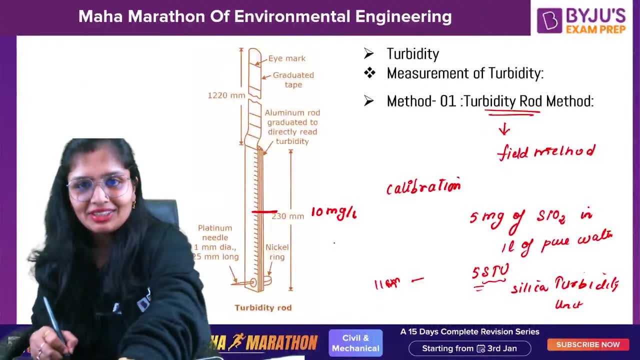 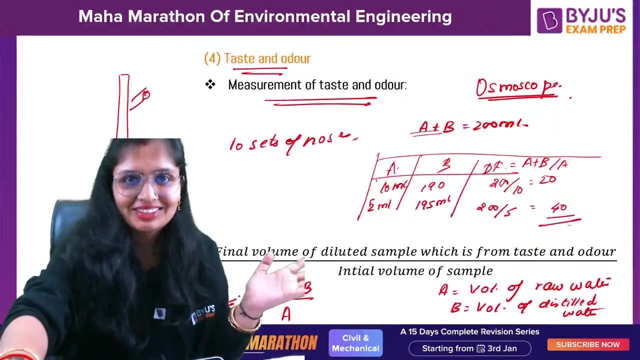 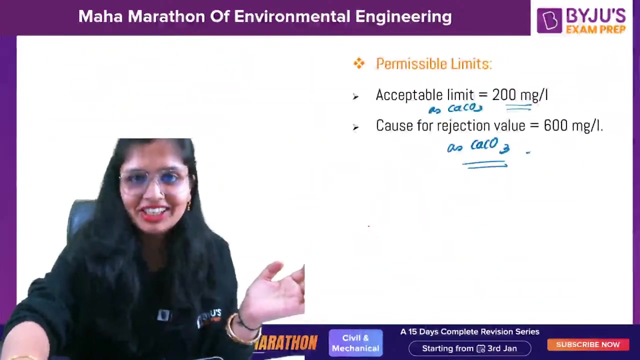 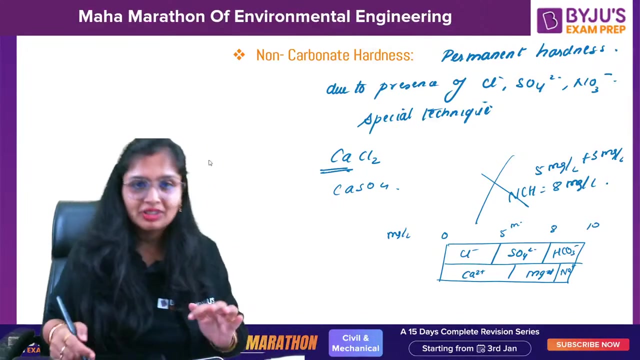 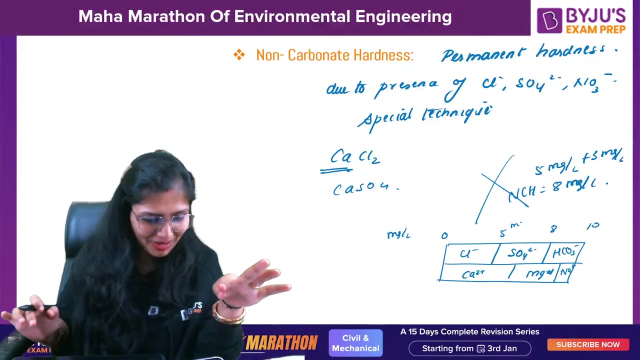 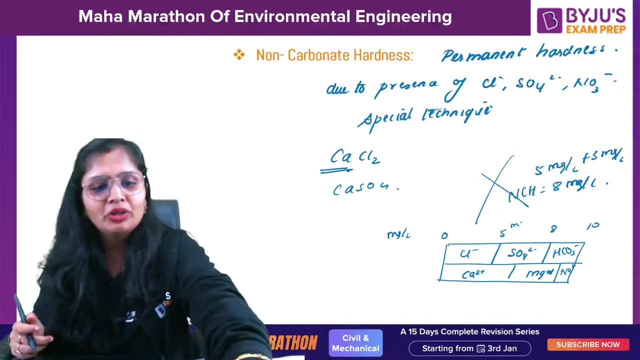 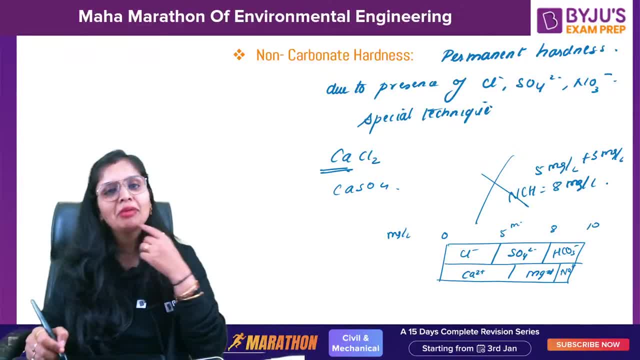 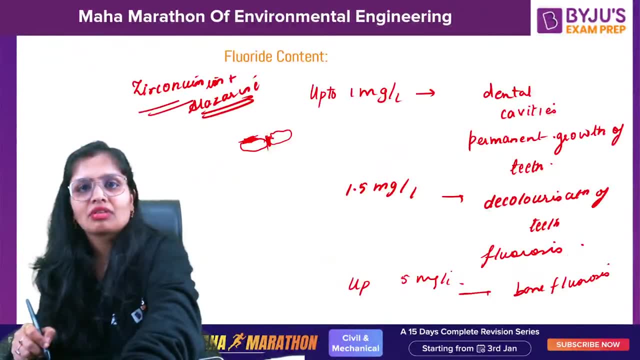 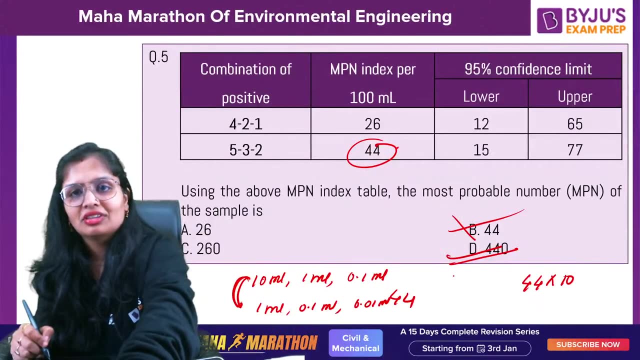 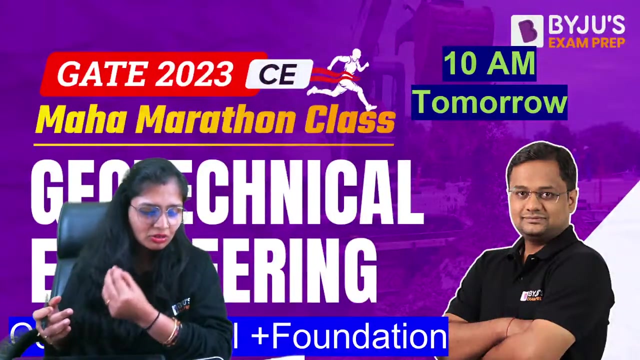 So that's why I used white PPT. Now, if you are giving me the feedback- Hydrologian irrigation- I will take it black ppt. okay, last time you guys told me white, that's why i took white, okay. so, guys, as i told you, environment blue, tell me the color so that the next ppt venture i'll 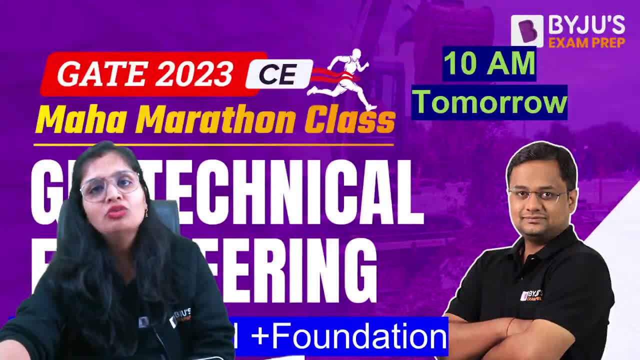 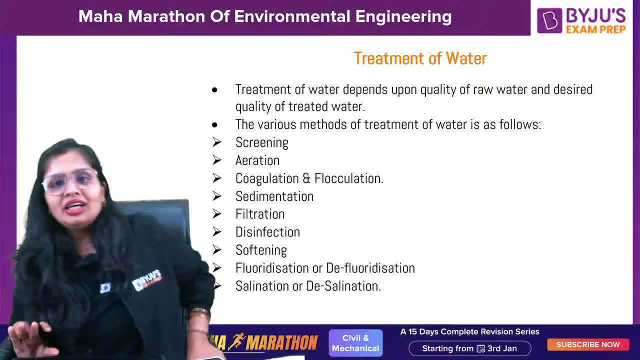 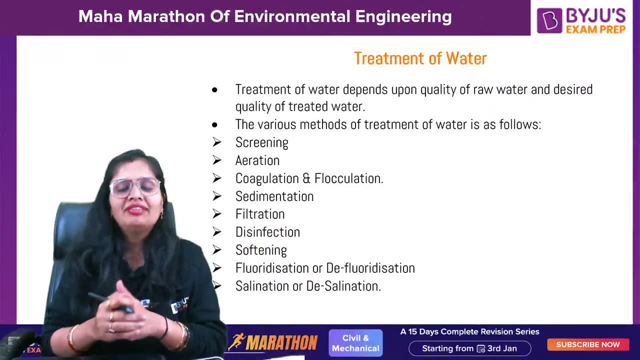 make. i'll make it in that color: maha marathon tomorrow for geotech 10 am sharp. okay, so, guys, uh, now talking about treatment of water. obviously, first we will check the quality. if, as you know, if desired quality is not there, if fluoride is not there, we will add fluoride. 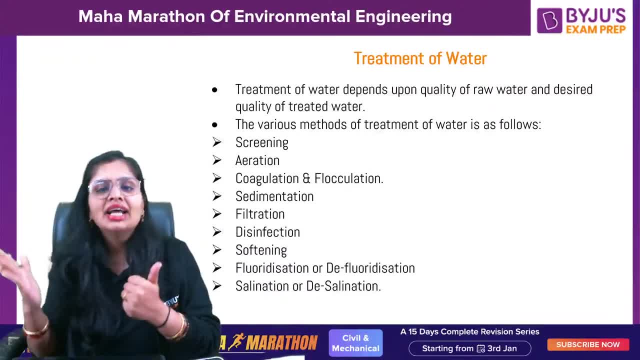 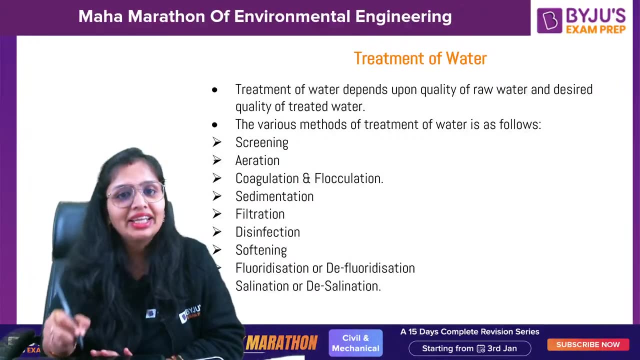 if excess quantity of fluoride is there, we will remove fluoride. similarly we'll do for other parameters also. so here if you talk about uh, here if you talk about we have various methods of treatment. we go it in a sequence also, like first screening, then aerating and then we will do. 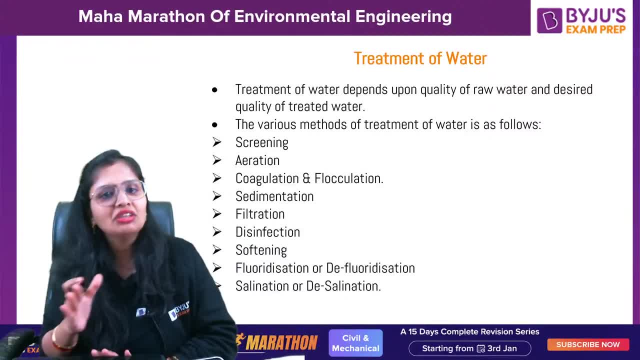 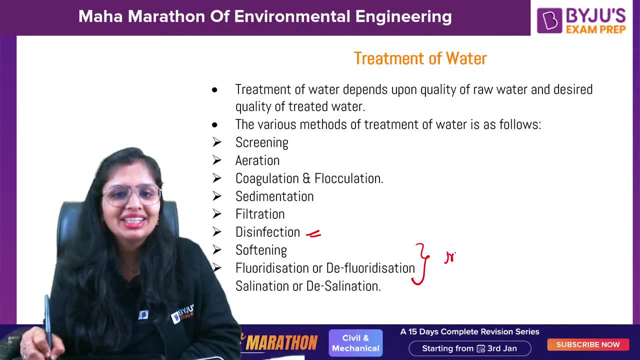 coagulation, flocculation, sedimentation, filtration, disinfection. a disinfection is the last. these are the miscellaneous treatments which is given. these are the miscellaneous treatment. if the water is hard, then only you will give softening. if the water has not fluoride- no fluoride is there then- 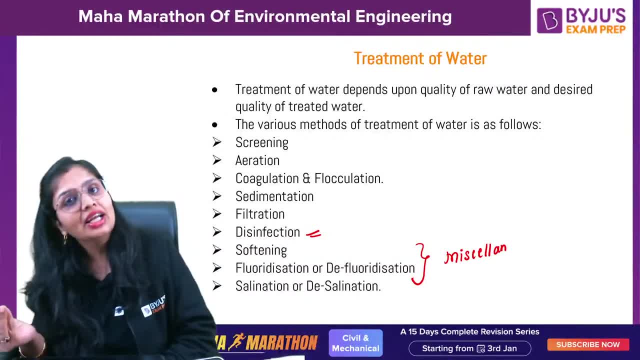 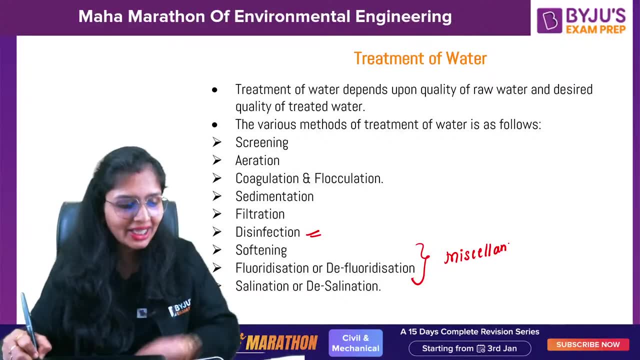 you will add fluoride. if excess is there, you will remove fluoride. similarly, if salts are there, it's okay. if excess is there, you will remove it okay. so what will happen here? miscellaneous treatment has been given. miscellaneous treatments has been given, for this required depending upon the quality. 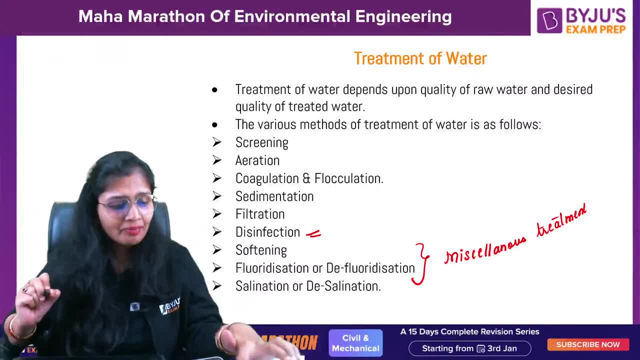 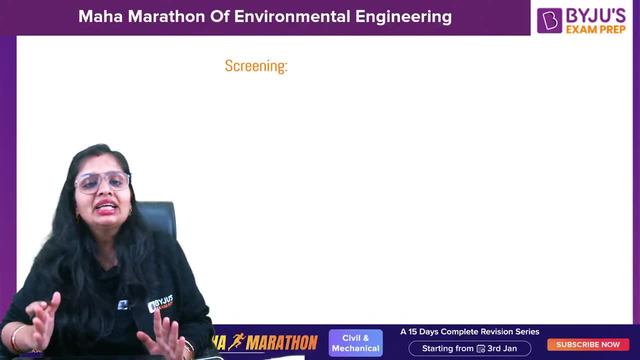 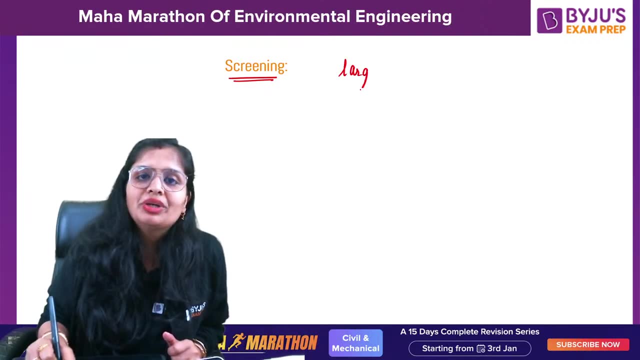 of water, depending upon the quality of water. okay, now, what happens now? what happens here talk about first is the screening, screening, screening, as you see, the screening is done for the removal of large suspended particles, or you can say large floating matter. so whatsoever, paper bags and all are there animals. 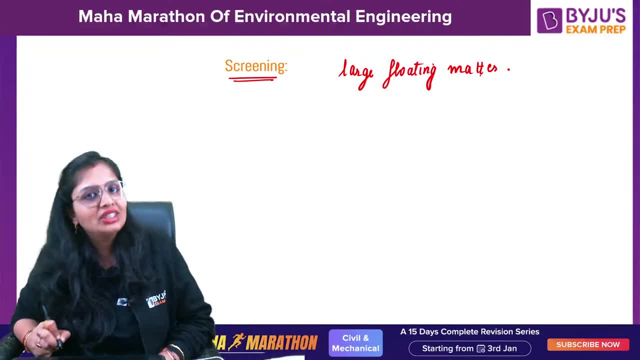 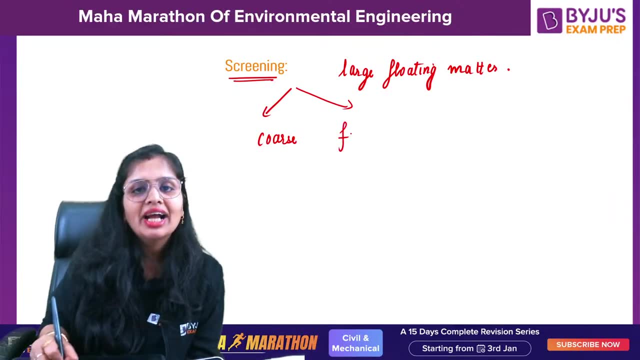 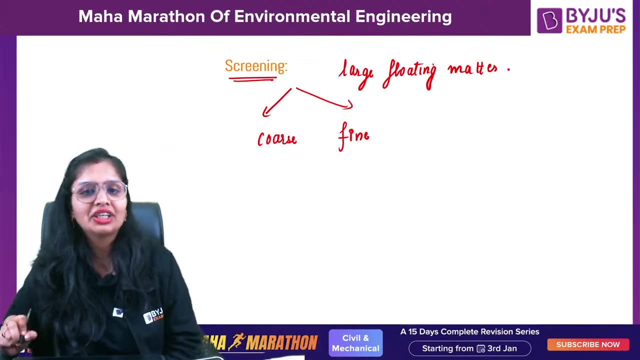 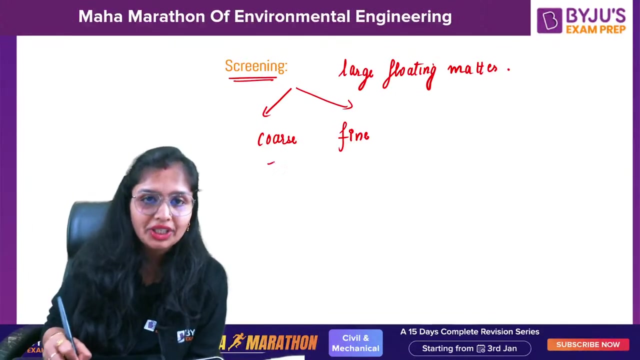 or all the things which are floating. these are being removed in screening. now, screening, we have two types of screens. you know that: coarse screens and fine screens. guys, what is the screens which he used on prominent basis? coarse screen or fine screen? coarse screen or fine screen? coarse screen or fine screen? which we use on prominent basis? we use coarse screen. now, if you. 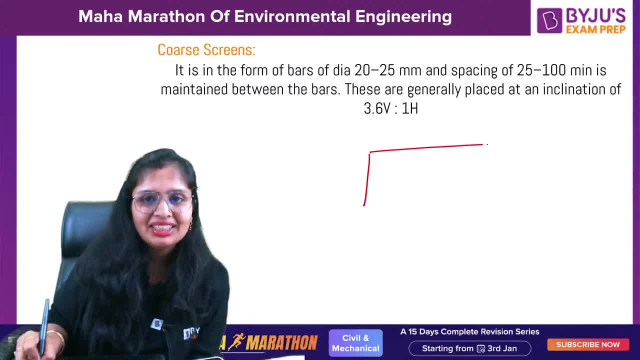 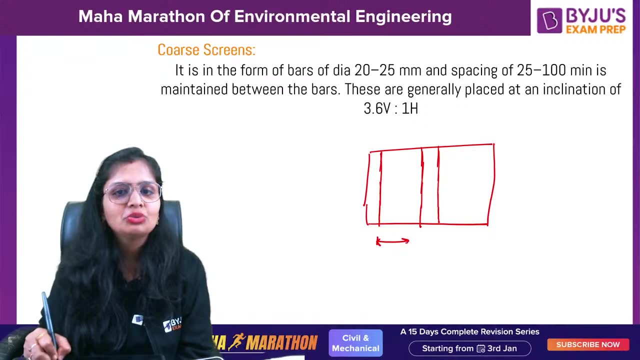 talk about it generally. they are in the form of bars, already mentioned, that i have mentioned. however, it is not used so much for your gate. it is used for your esc, for conventional designing purpose. these are the bars. the bars are 20 to 25 mm dia and the spacing between them is 25 to 100 mm. 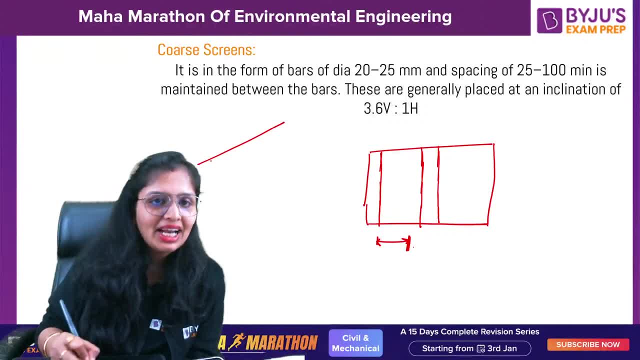 generally, they are not placed there like this. they are placed at an inclination. these a single bar. i have told you these are placed at an inclination. now you'll ask me, ma'am, why they are placed at inclination. generally, if not mentioned, we take it 45 degree. however, 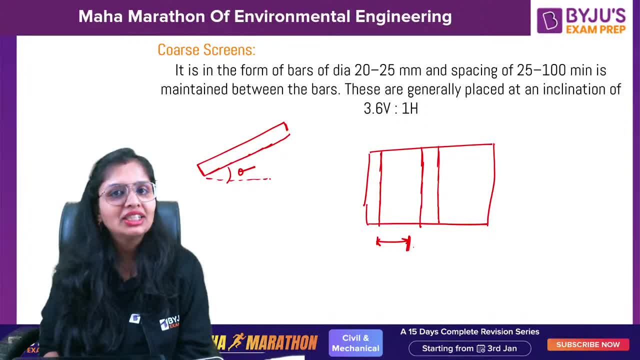 the they have given you 3.6 vertical is to one horizontal now, uh, generally we use course. everybody answered it correctly. the reason is: fine screens. obviously it is good, even it will trap the final impurities also. but the headloss is more, head loss is more, so water has to spend more amount. 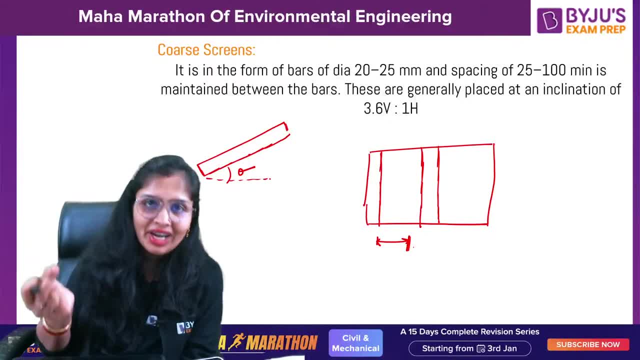 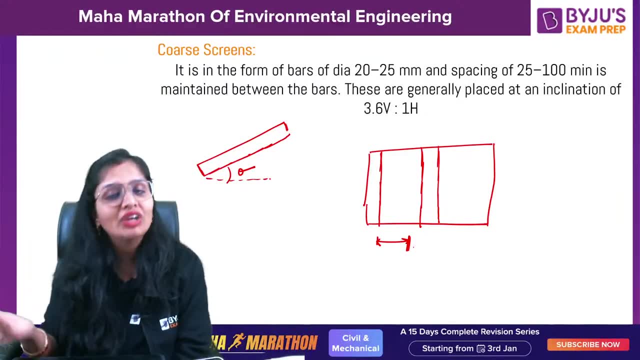 of energy to overcome the friction offered by the fine screen, firstly. secondly, what will happen? frequent clogging will take place, So frequent removal has to be done. that is the reason we go for core screen. In core screen generally, we place it at an inclination so that the amount of area 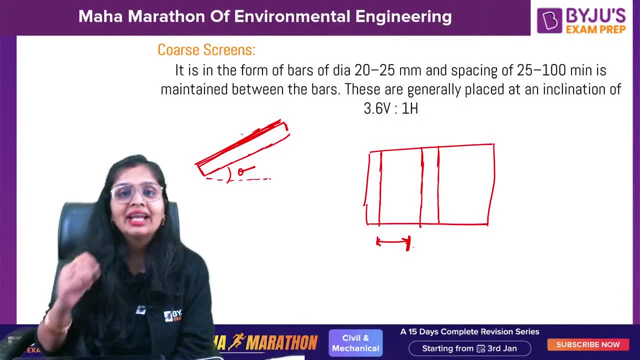 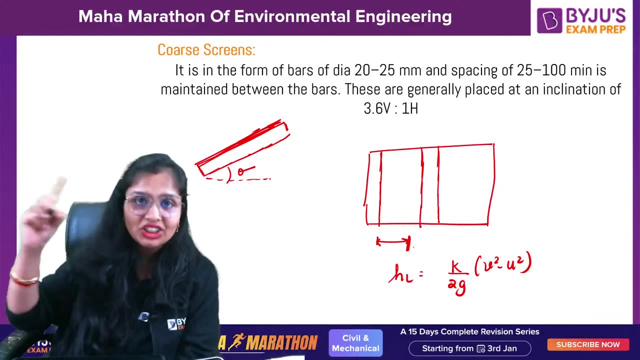 which is available is more. Then, for calculating the head loss, there is a formula: k by 2g, v square minus u square. k is constant, depends upon the material of the screen. g is acceleration due to gravity. If, by chance, in the case, they don't give you the value of k upon 2g, you take it as 0.0729.. 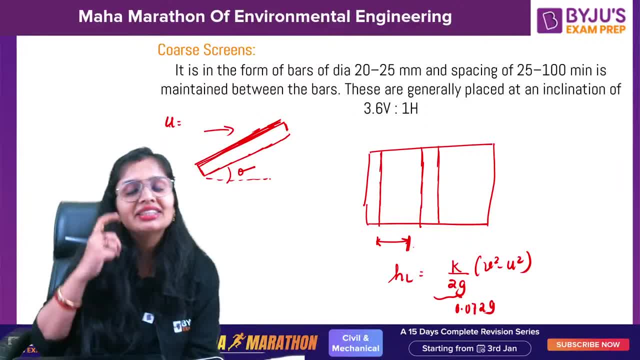 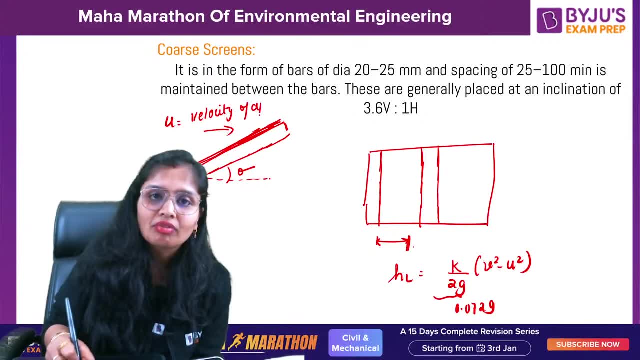 Clear Now. two velocity are there. u is generally they say use velocity above the screen, but you should know that it is velocity of approach And this is v velocity through the screen. Now can you tell me v will be more or u will be more? 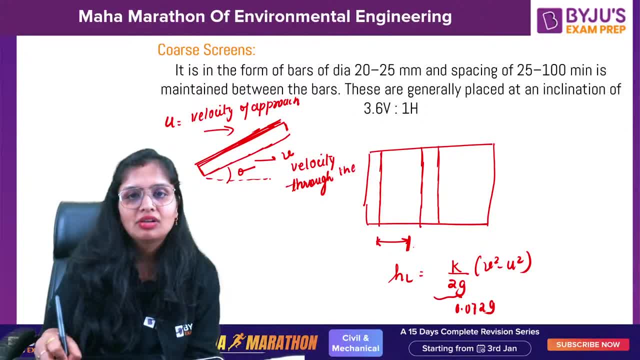 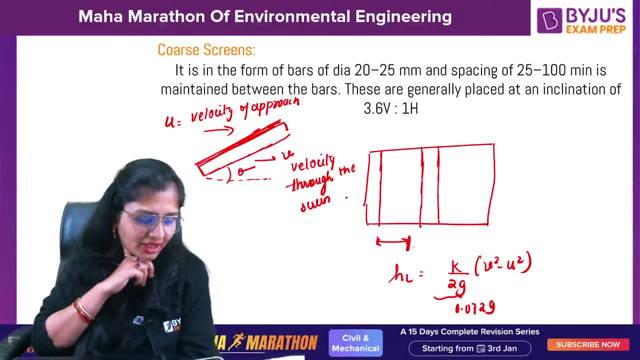 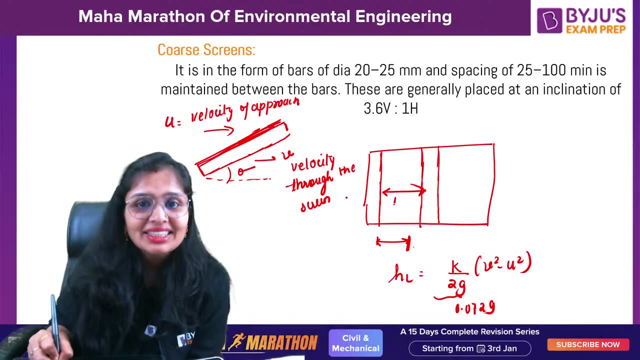 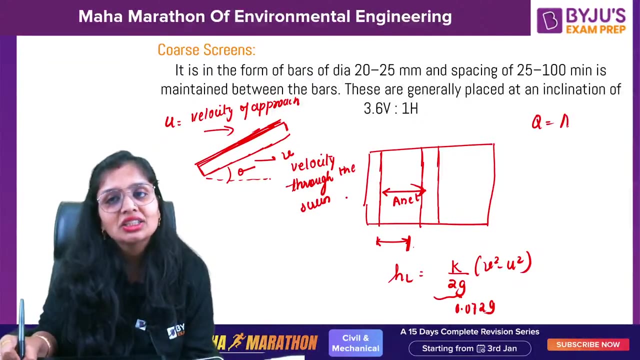 v will be more or u will be more. No, k by 2g. it is there, not k. square v will be more. Why? Because here, in between this, this area, this area will be there, this net area will be there where the water will be passing. So discharge is constant, Discharge is equal to area into velocity. 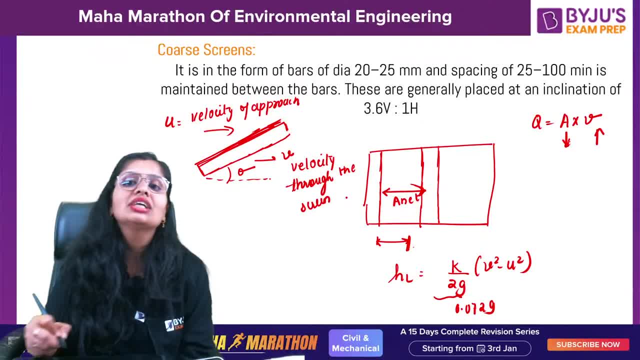 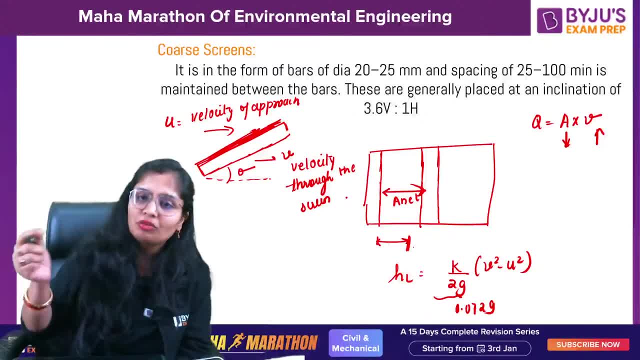 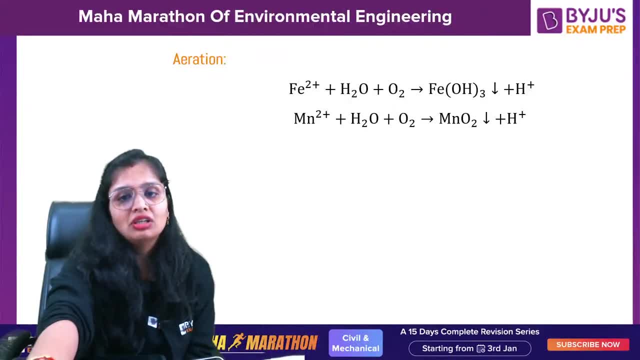 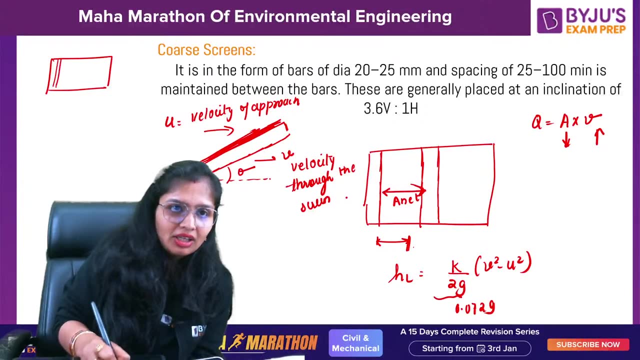 So area was more. that's why velocity of approach u was Clear. This you should know. Now, talking about further fine screens, already told you frequent calling and they are in the form of wire mesh. I will show you the diagrams also. Wait, These are like this. These are in the form of wire mesh. 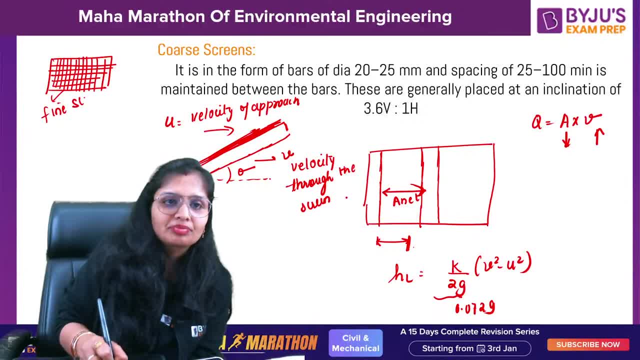 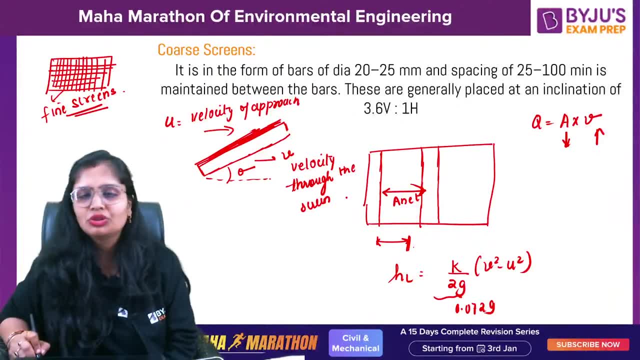 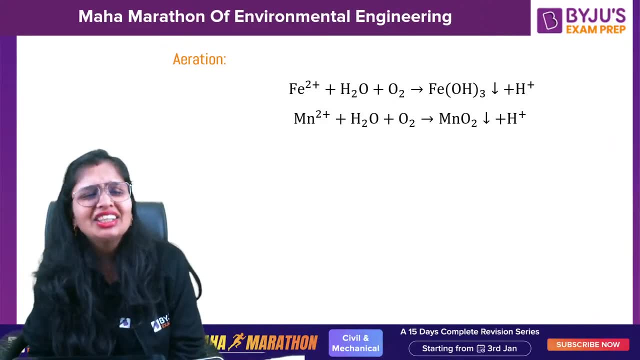 These are fine. These are fine. Okay, Generally not ask questions, but they can ask you MSU patterns and all. So you should know, or they want they can ask you in one marks. the head loss part Coming up next is the aeration. Aeration means something related to oxygen. 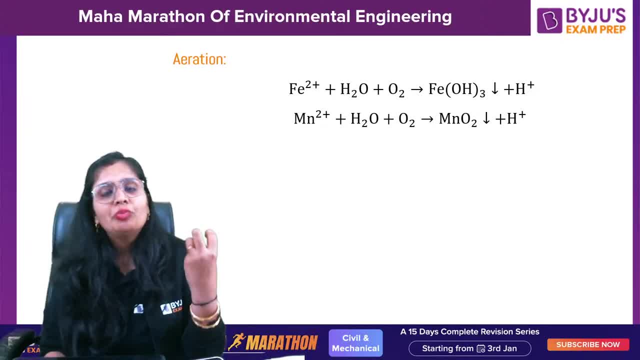 So what you do in the case of aeration, you bring the water in intimate contact with the oxygen present in the atmosphere. Okay, When you do so, the dissolved minerals, the gases, gets removed. You don't want gases like H2S. you know Nali ki Badbu, which we call it, and you would have done it in your salt analysis. 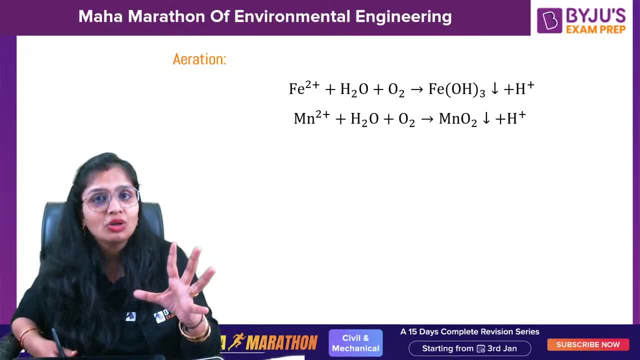 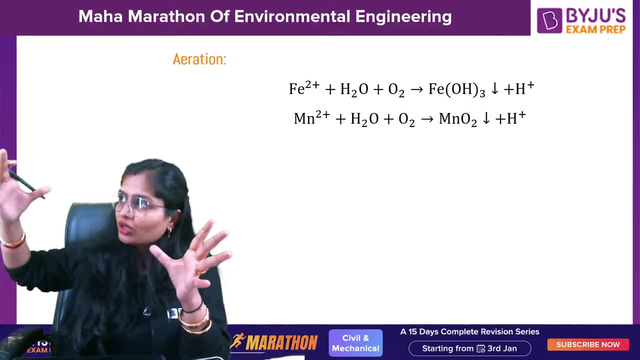 That strong smell of H2S comes out. So that smell, you don't want it. Okay, So that is the reason: you take the water and you try to bring it in contact with the oxygen which is present in atmosphere. So what will happen? 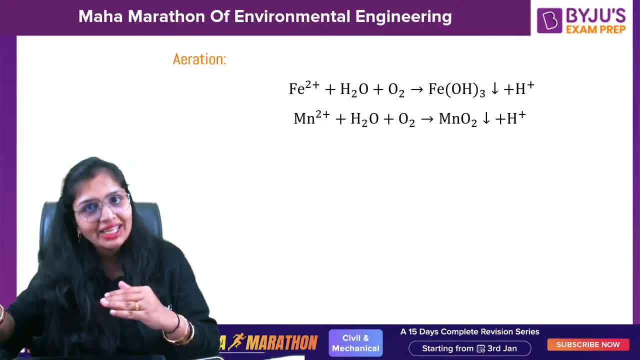 So what will happen? It converts into acid like H2S, gets converted into H2SO4.. Okay, if carbon dioxide is there, it will get converted into carbonic acid so that the impact of gases can be reduced. Now comes the next question. 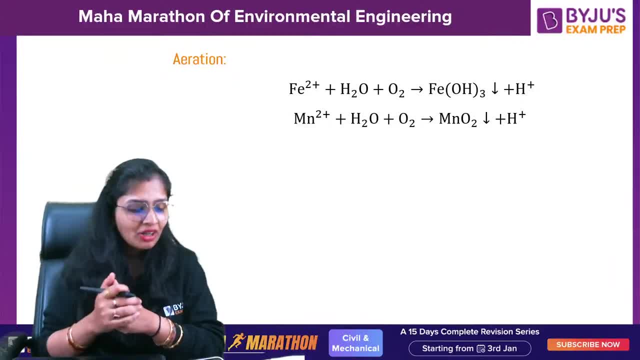 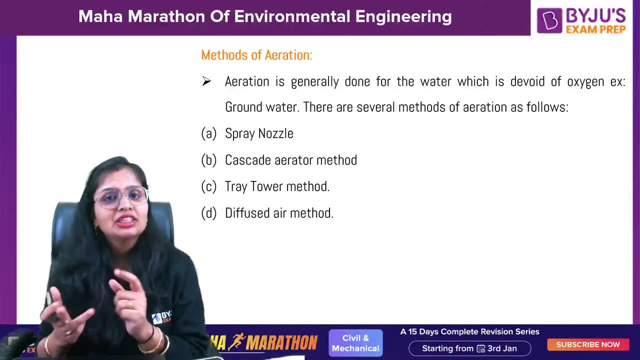 How do we do this aeration So pungent smell, or you can call it as rotten egg smell. Also you can call it Okay. Now there are various methods like spray nozzle, cascading aerator, tray tower, diffused air. 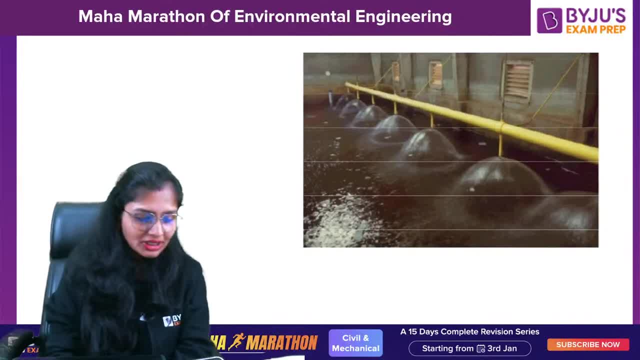 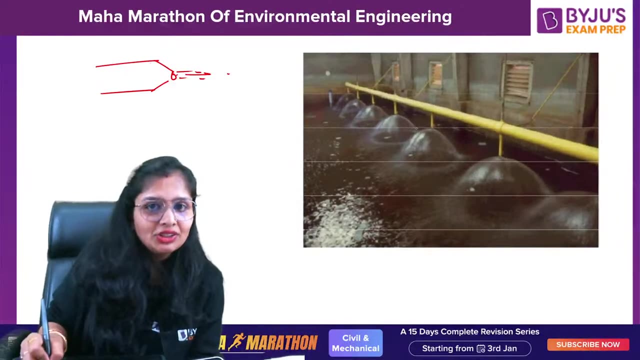 Now let me show you spray nozzles method and all, as you can see it in the diagrams, and all What will be happening Like if I show it to you. The nozzle will be there, from which water goes out. Okay, it forms into number of layers. actually, as you can see here, the number of layers are there. 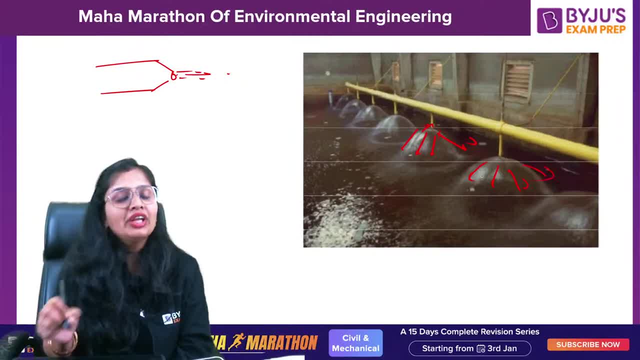 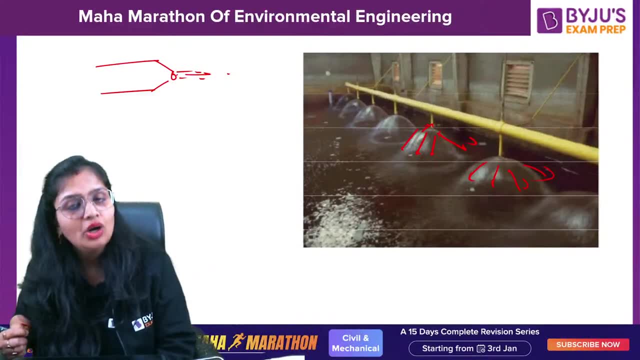 You can see number of layers. So when there are number of layers, the opportunity of oxygen to come into the air- So when there are number of layers, the opportunity of oxygen to come into the air You can contact with the water increases. Okay, so this is a good method. 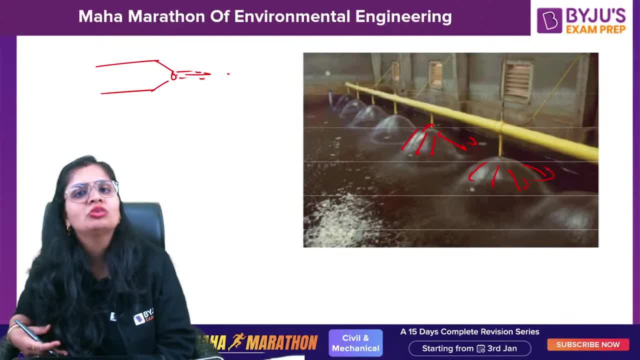 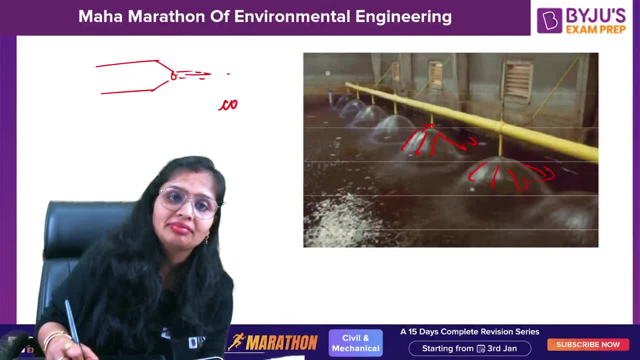 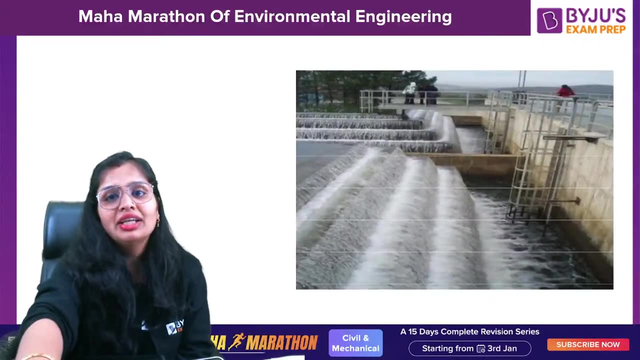 It has greater efficiency- 98 99% efficiency for removal of carbon dioxide, H2S gas- but still we don't use it. Why? because it is costly, So we don't use it now. Next comes the other one Is: this is now. this is what cascading aerator method. 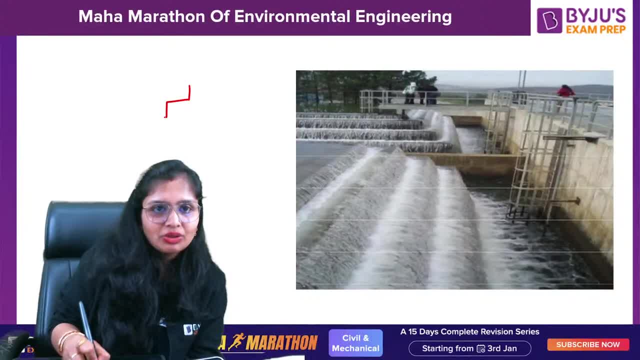 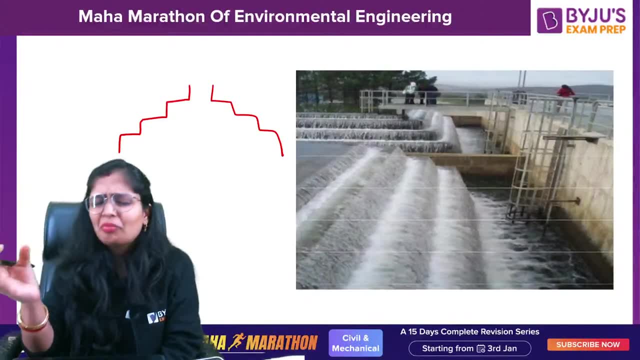 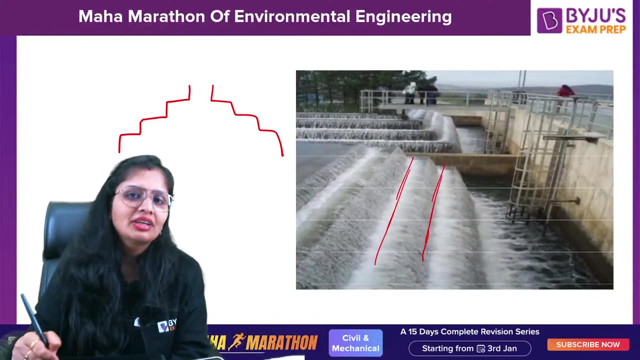 You can see this here. You can see this. concrete steps like this. you know, right, these concrete steps: three to three point. five concrete steps. this is very simple, no need to apply any easy for operation, no brain to apply. you can see this here. steps are there. steps are there, right, you can see these? steps are there. three to three point. 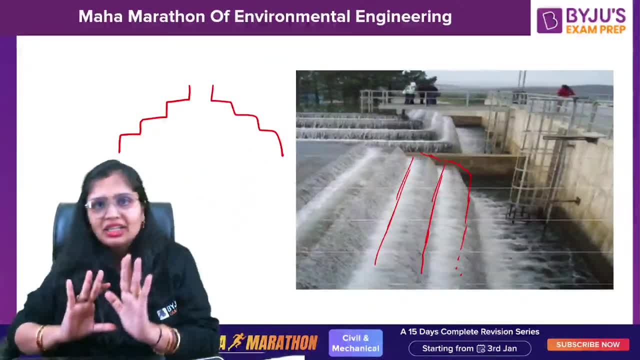 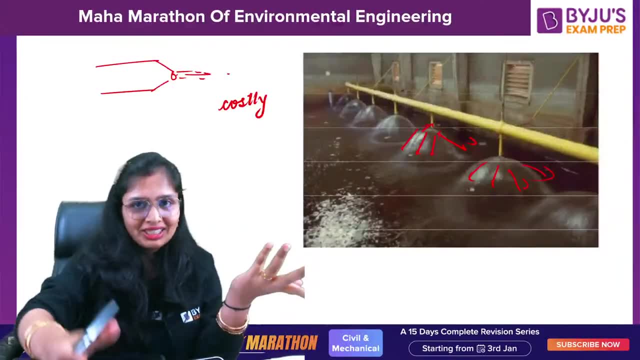 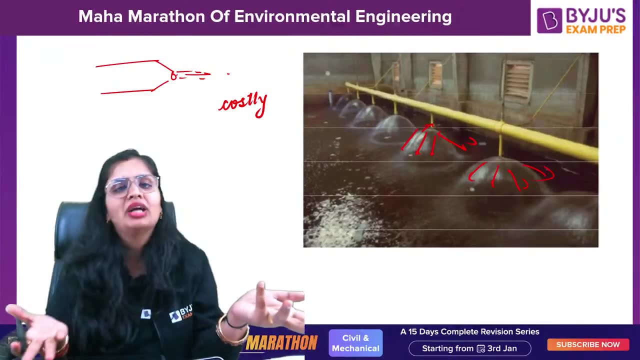 five steps are there. thus, bring it. what will happen? it does not have a higher efficiency. that spray nozzle, that is one. this that is obviously. it is required. you have what pressure? you said pressure is required, and pressure is required. that means what you have to install other equipments and it becomes costly as well. okay, now coming next, as i told you, casket aerator. 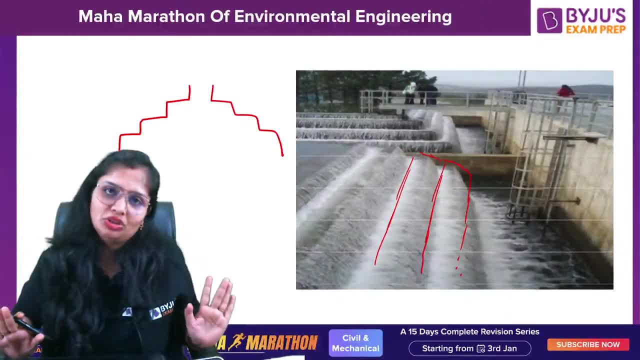 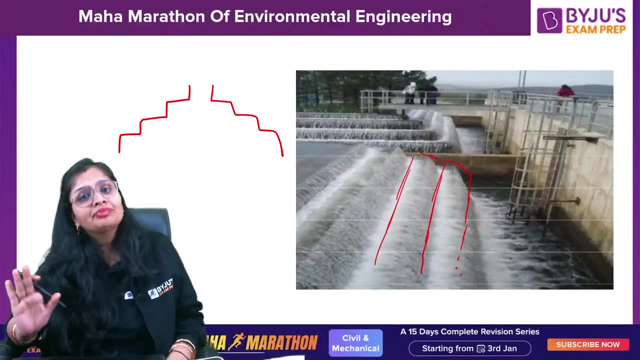 you ask, ma'am, which is the one which is used? this is the one which is used. so if you go, if you visit your treatment units and all you will see this casket aerator which is being used. so now what you do it here? three to three point five steps. 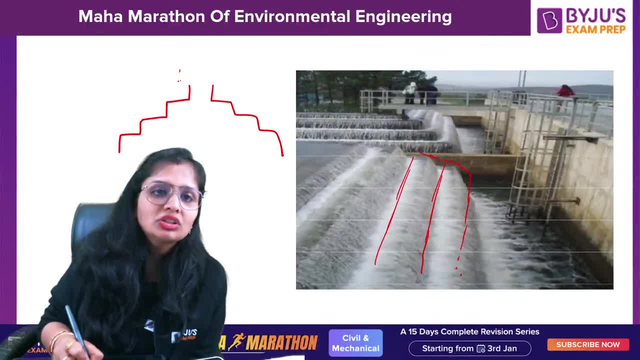 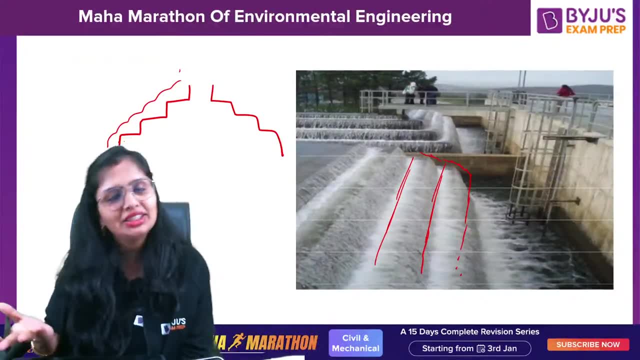 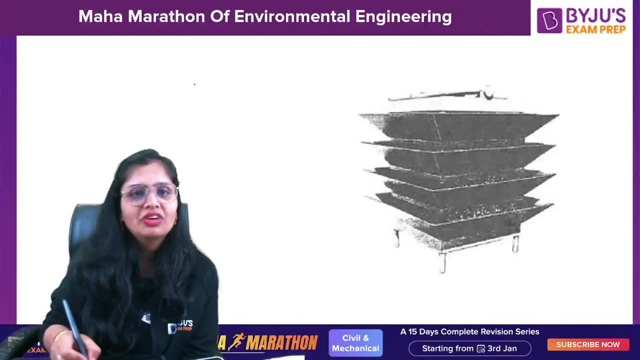 are there three to three point five steps are there. water goes into this, flows into steps and it comes in contact with the oxygen which is present in the atmosphere. simple, easy to operate. we use this. after this we have tray towers method. this is diffuser. we have tray towers, multiple number of trays like this tray of different sizes, then this: 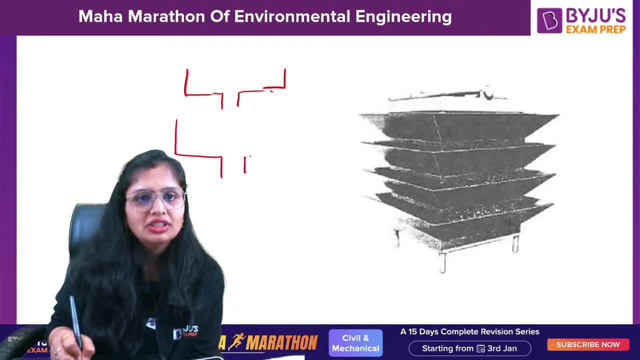 tray, then this tray is there, then again a tray is there, so multiple number of trays are there, so of various sizes, sizes. so from here also, water moves into number of layers and the oxygen comes in contact with it. so there are n number of methods, but the one which we use. it is cascade aerator method, simple to 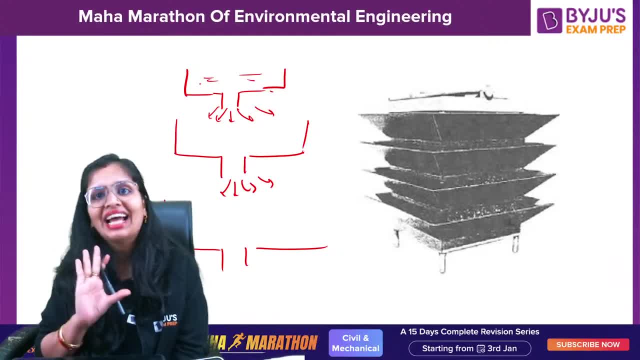 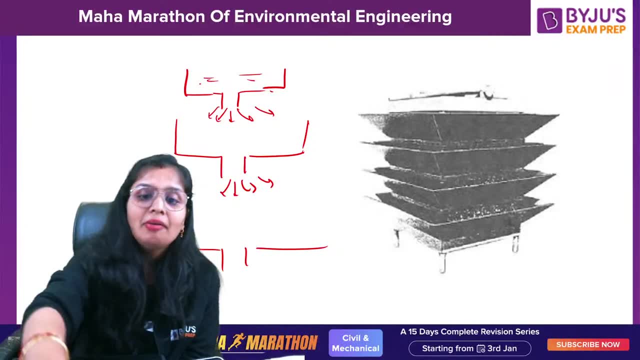 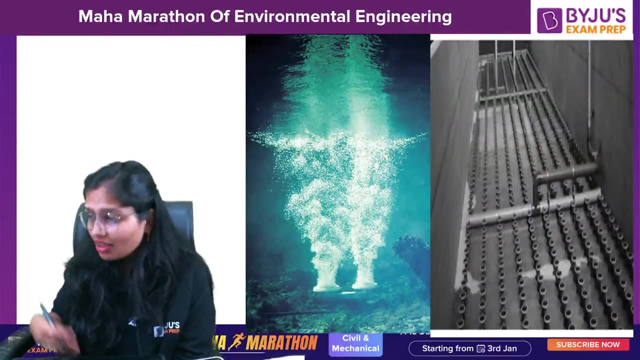 construct it okay. next, these three were natural. that means you were using the atmospheric oxygen for treating the raw water. but this diffused air method, what you do, just like you would have guys would have seen it: aquarium and all what you see it there from the bottom, the gases comes out, the 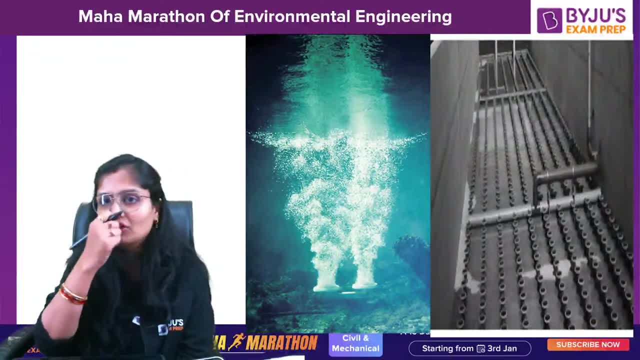 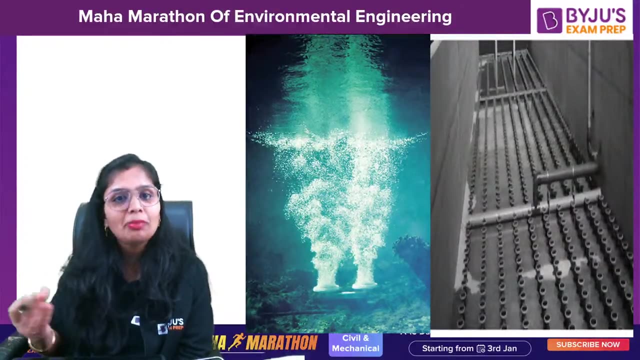 oxygen comes out. okay, so here also, in dissolved oxygen method also, what will be basically happening is a diffused air method also. what is happening here? you, here, you are artificially here. the atmospheric oxygen is not being used. okay, so the oxygen is supplied from the bottom, but 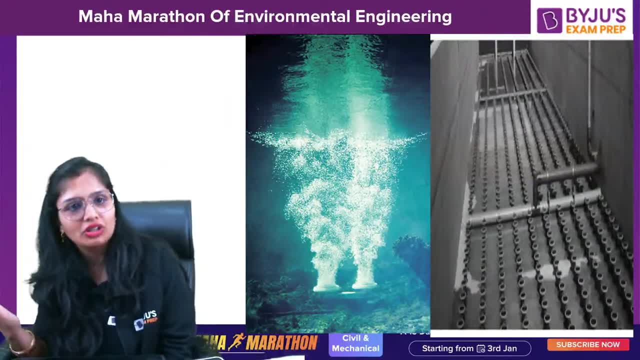 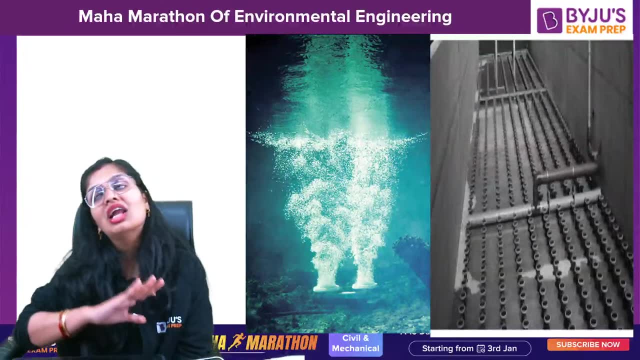 practically we have to need million liters of water. so it is not possible that we can satisfy that much demand of oxygen. so we don't use it on a large. you can use it for a certain community, but you don't use it for a wider population. okay, so this is the 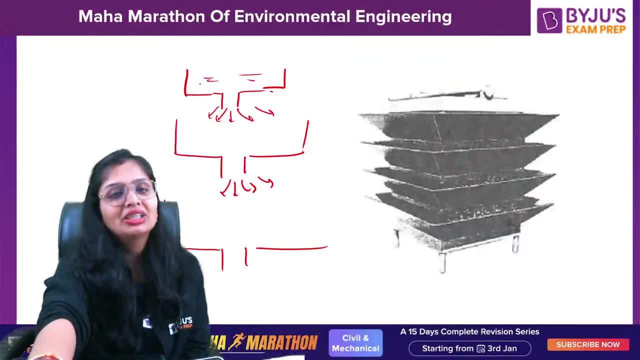 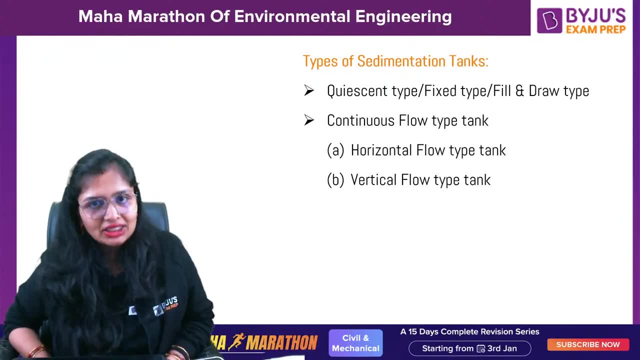 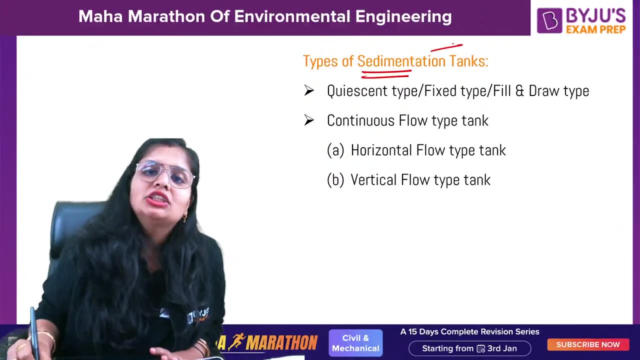 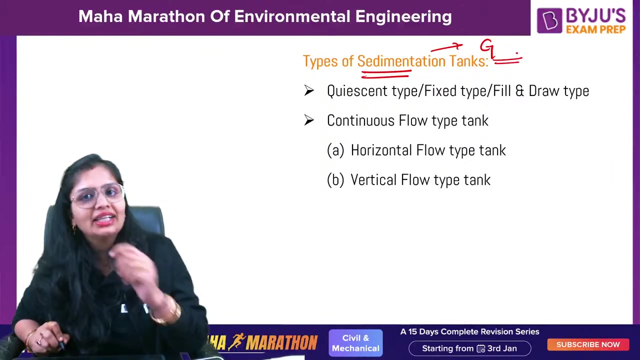 thing which you should know out of this: we use cascade aerator, but the best out of this is the spray nozzle. okay, now coming to the sedimentation tanks, if you talk about sedimentation, the whole hero of this sedimentation is specific. gravity is the hero of this chapter. now, first, if we talk about the sedimentation tank, there are two types. 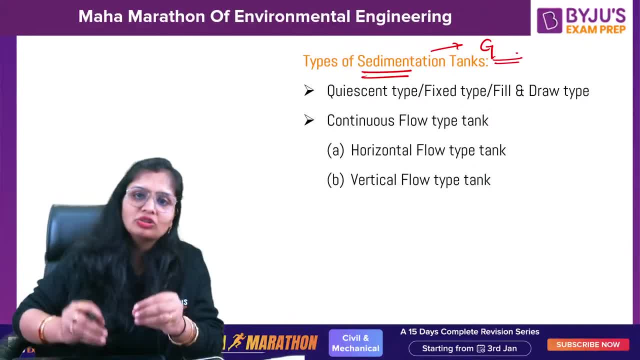 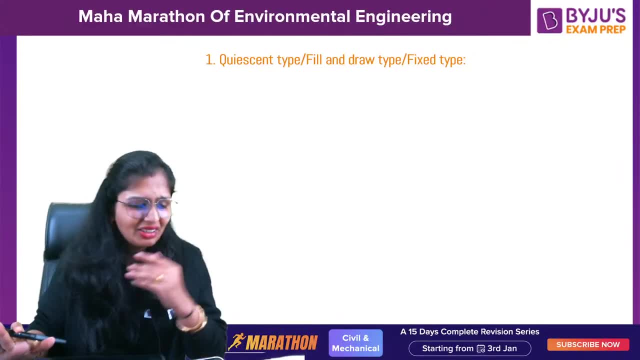 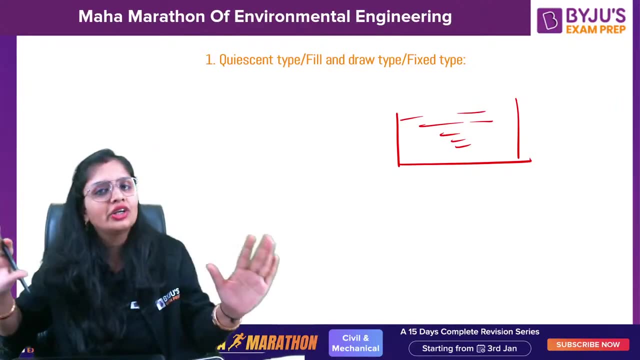 of it broader sense question time. you call it fixed type also and you call it fill and draw type also. second is continuous flow type. now let me talk about question type time. nothing to apply brings what is that? what you bring? the water you make that turbulence, zero water is not at. 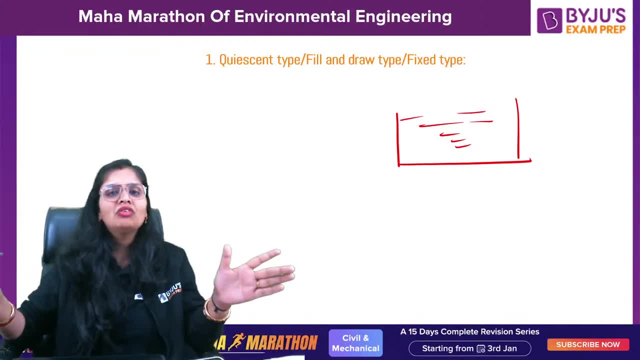 all flowing water. is that fresh? that will happen. you keep the water for 24 hours long, for which means you will not bring any more water. water is less than 1 million liters with素 water. You keep the water for 24 hours, Whatsoever. suspended solids are there? suspended solids are there? 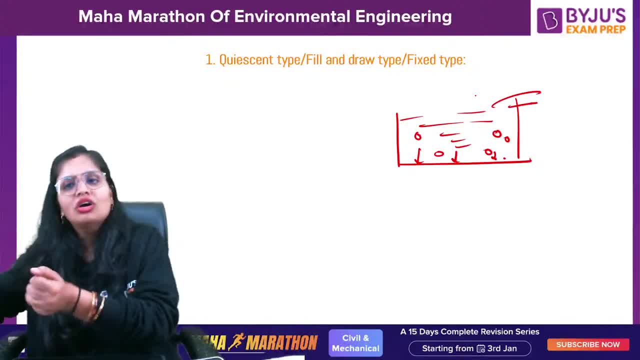 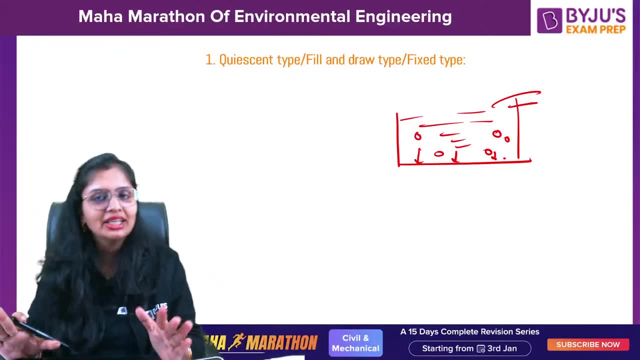 They will settle. You will take the water, Fill, draw, Fixed, no turbulence, nothing is there. So fill and draw. type tank. question: type tank. this is there, Okay. Next, if you talk about generally, how many tanks are basically used, 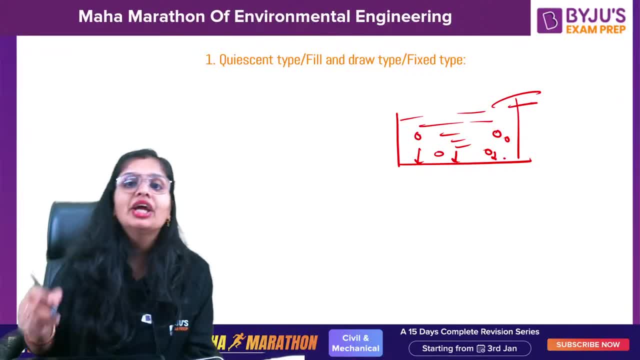 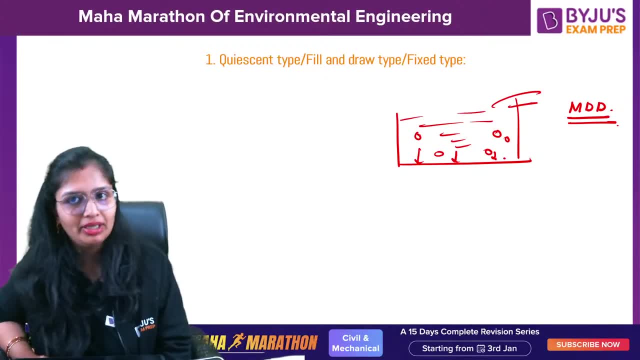 Three. Two are operational. One is kept as standby. You design it for maximum daily demand. You design the tank for maximum daily demand. Okay, There is nothing more we need to understand about it. Detention time is 24 hours. You keep it as your manual cleaning is applied, because here the suspended solids settled out. 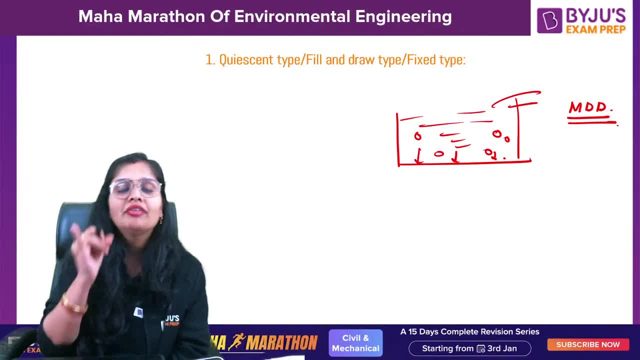 When you talked about screening, large floating matter was removed. When you talked about aeration, dissolved solids and gases are removed. When you talk about sedimentation, suspended solids are removed. Okay, Now coming next, We have continuous flow type tank. 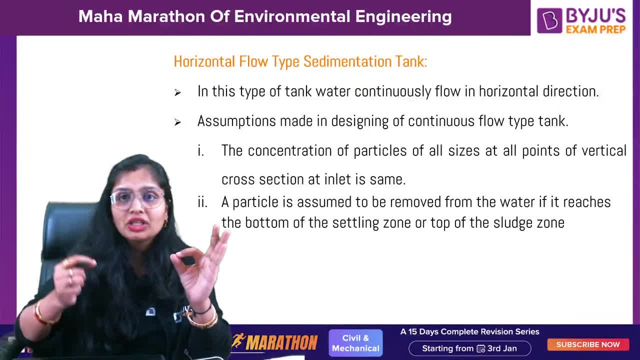 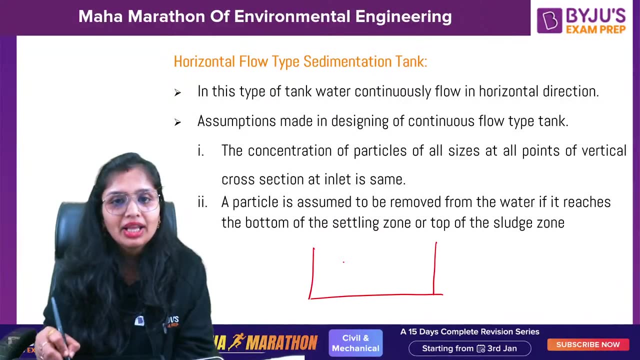 Remember, continuous flow type tank means water is flowing. Water is flowing, The turbulence is not zero. Now, when you talk about horizontal flow type tank, you should know very important thing: This is the settling zone, This is the sludge. 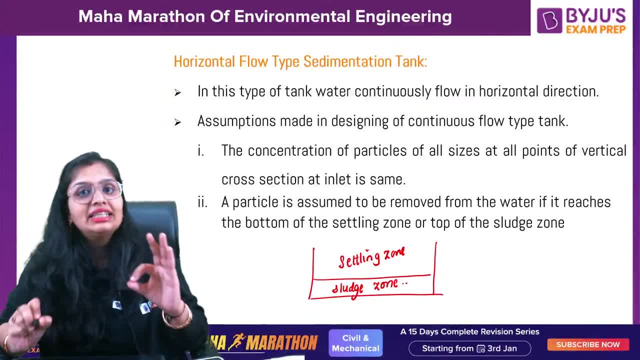 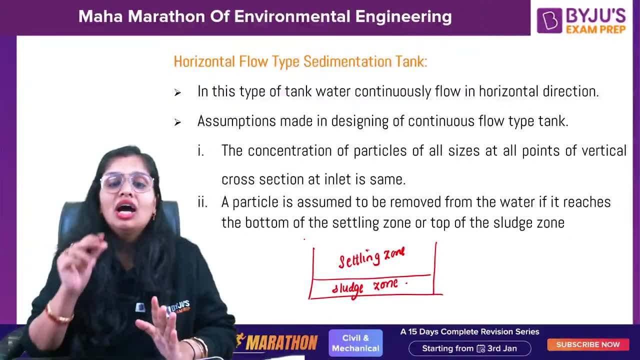 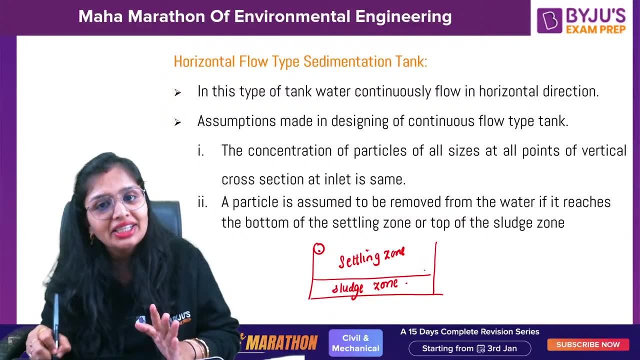 Now what happens? These are the assumptions. Assumptions might not be true, but assumptions are taken to simplify our calculations. A particle is assumed to be removed. So if a particle is present here and it reaches the bottom of the sludge zone, if it reaches here, it's not required to reach it here. 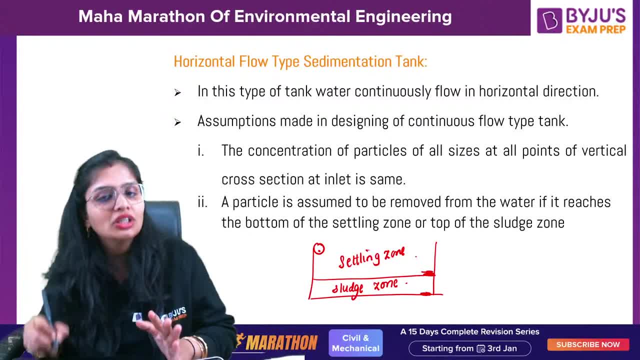 So if it reaches the bottom of the settling zone or the top of the sludge zone, it gets removed. Okay, It's not See. this is the bottom of settling zone and this is the top of the sludge zone. If it reaches here, it is removed. 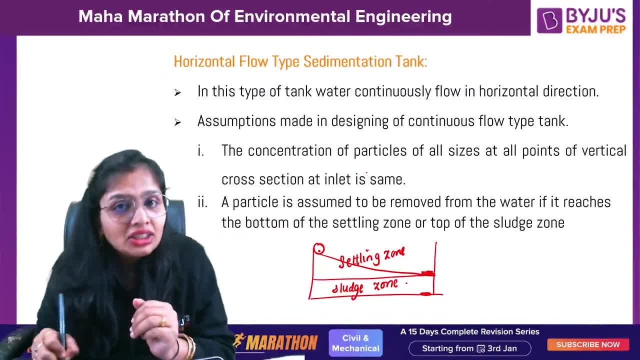 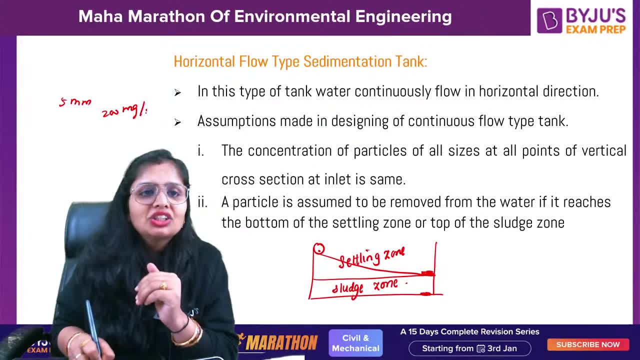 That's it. Next, the concentration of particles of all sizes. Let us suppose 5 mm particle is present. 200 mg per litre is the concentration of 5 mm particle. So it is saying, and let us suppose it is imaginary: 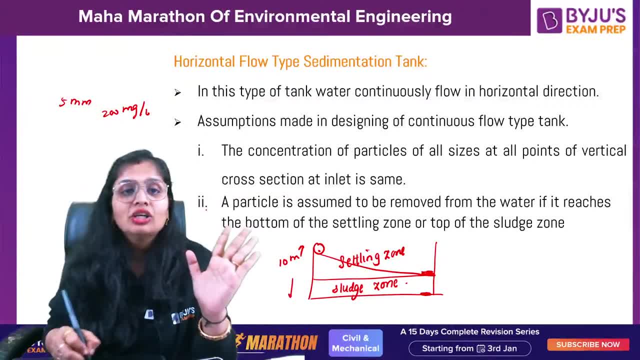 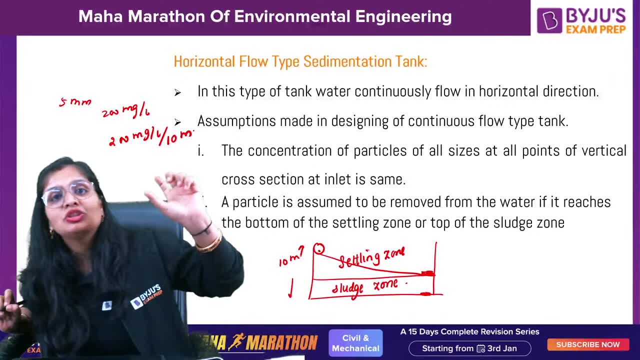 The depth of the tank is 10 meters, Imaginary, I am telling you So you mean to say that 200 mg per litre of particle, Per meter 20 mg particle is present, which you also know, that it's practically not necessary. 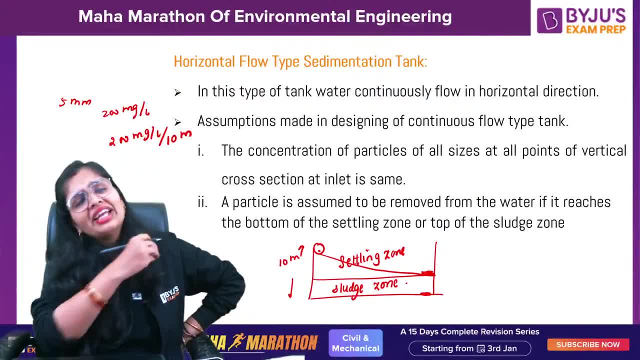 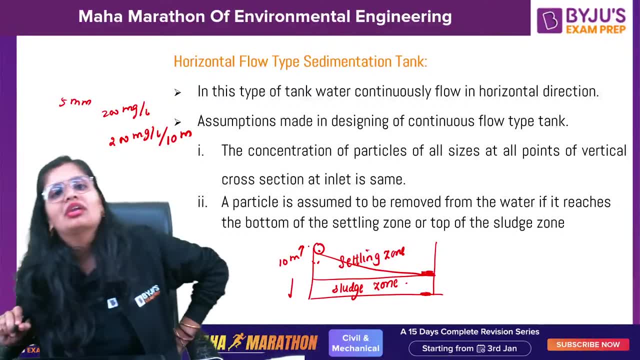 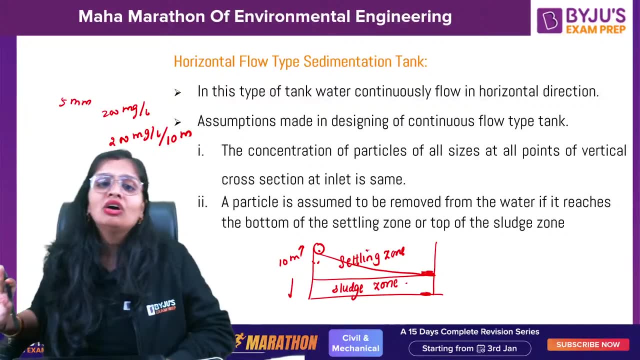 But this is the assumption that the concentration of any size of particle which is present along the vertical cross section at the inlet is same At the inlet is same. This is the assumptions you have taken. Okay, Now, based on that, you know two things you should know. 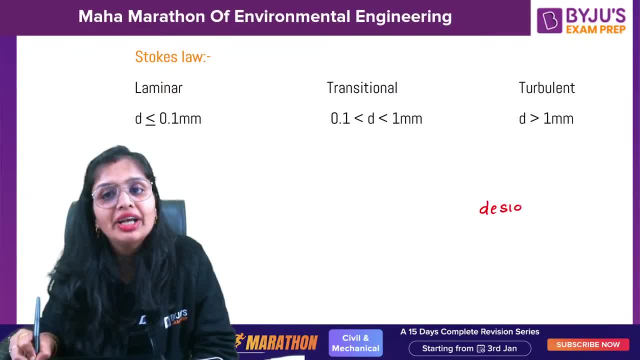 One is the design Size of particle, or you call it as concerned size of particle. Design size or concerned size of particle is that particle for which you design the tank so that your desired efficiency is maintained. So you call it as design size of particle or you call it as concerned size of particle. 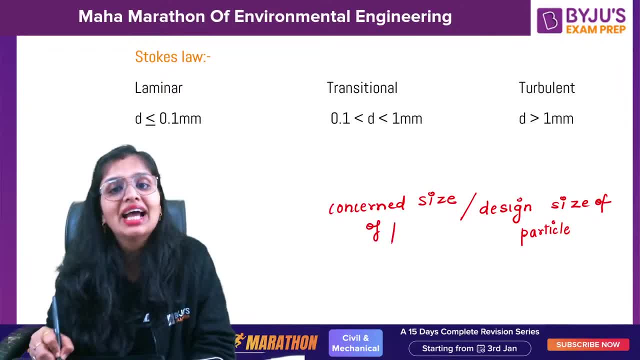 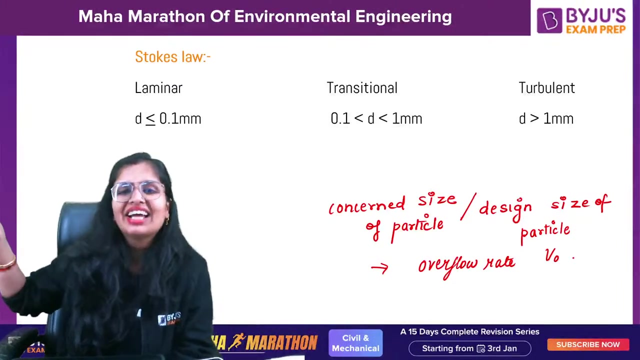 This is that particle- I am repeating it again- for which the tank is being designed. The velocity corresponding See this velocity is Exclusively for design. size of particle is known as overflow rate And you denote it by V, And for velocity of any other size of the particle you can go by laminar flow, stokes flow. 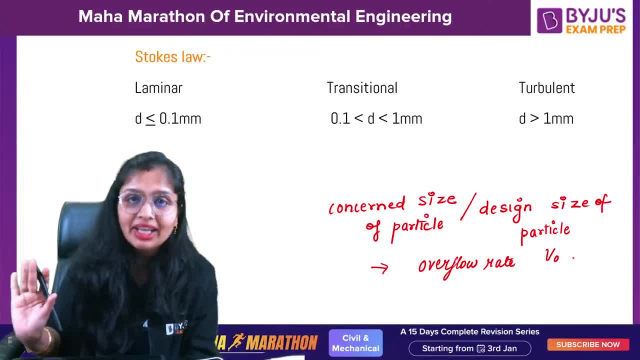 You can go, you will get the velocity Settling velocity. Why? Because the suspended solids are present in the tank and you want them to settle. If you want them to settle, You won't make the turbulence zero, but you will slow it down the velocity. 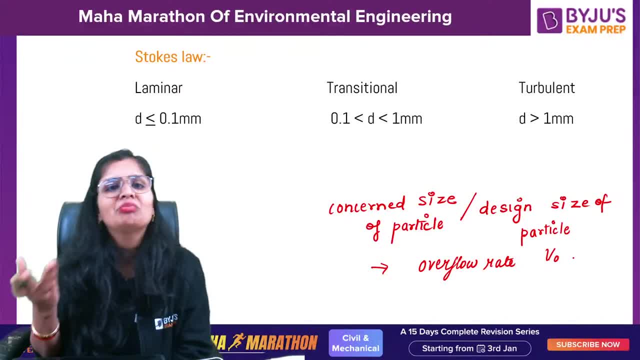 Now the die of the particle can be anything. It can be 5 mm, 0.1 mm, 0.15 mm, anything. So we have divided into laminar transitional turbulence. Now a frequently asked question: Settling velocity here. 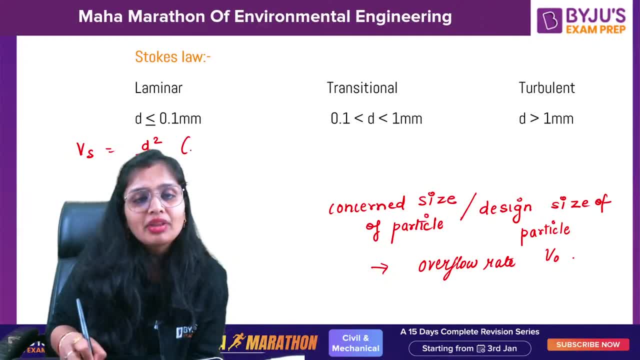 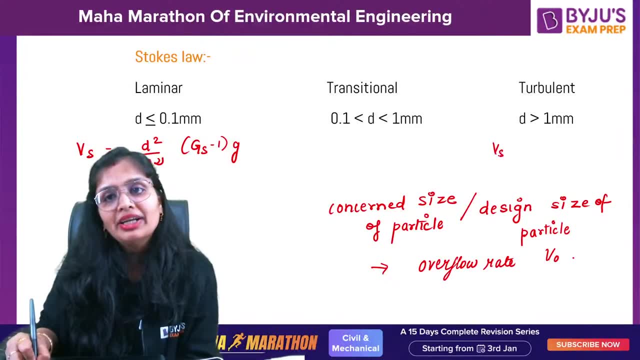 It will be D square upon 18 nu Gs minus 1 into g. Nu is the kinematic viscosity. If I talk about turbulent, It is 1.3.. It is 1.8 root over gd Gs minus 1.. 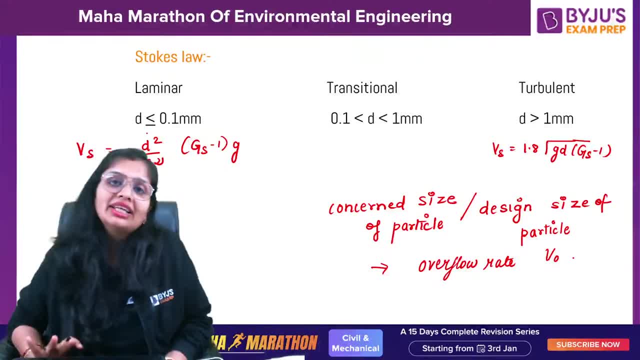 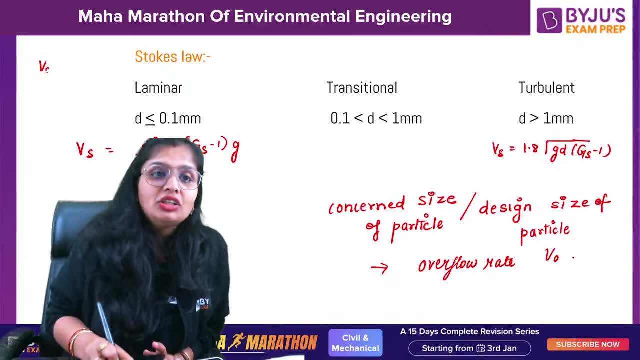 Now there is one more formula. Let us suppose in the examination They ask you: Consider the effect of temperature. Consider the effect of temperature. So for laminar There is again an empirical formula. You guys need to know D square 3t plus 70 by 100.. 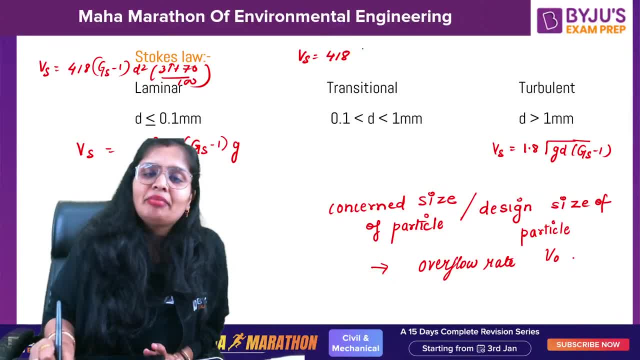 Same formula is there for transitional: Exactly same, But only one change. So D square: this time it is D, That's it Okay. And Vs: settling velocity: you will get it in mm. per second Dia: you will get it in mm. 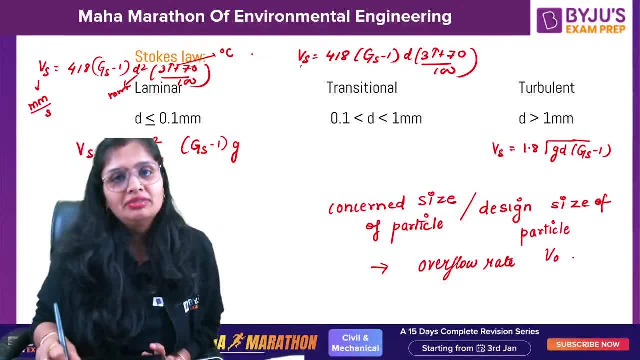 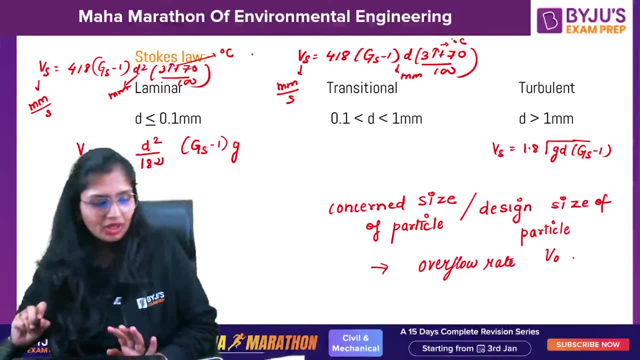 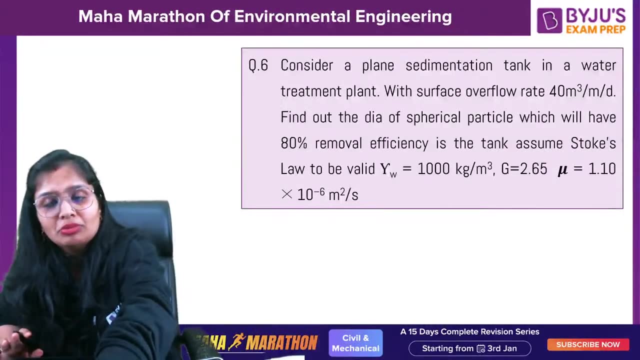 And temperature. you will get it in degree Celsius. Similarly here. This you have to make sure. Okay, So this is regarding the sedimentation tank. Now comes the question Before you. we move to the question Part: Percentage removal efficiency. 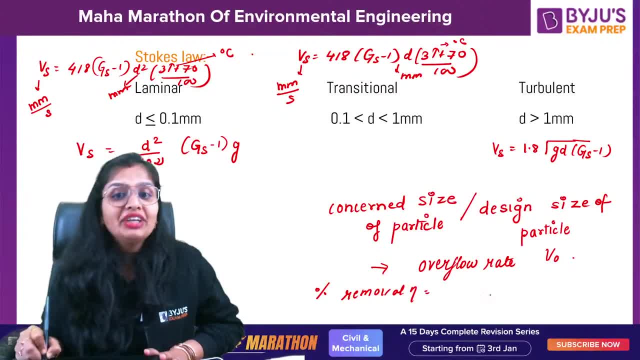 Remember Percentage removal efficiency. See, we design it for V0.. But there might be some particles Which have a velocity more than that of the concerned size And which have the velocity less than that of the concerned size. So that's why Vs into 5.. 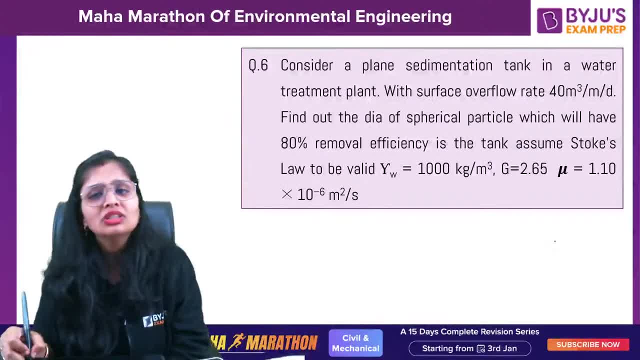 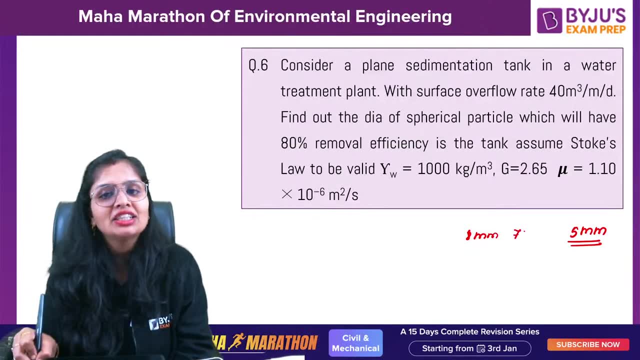 Now you guys will answer. Suppose. Suppose I design for a 5 mm size of particles And 8 mm, 7 mm size of particle is present. What will be the efficiency? 100%, 50%. This is my design size of particle. 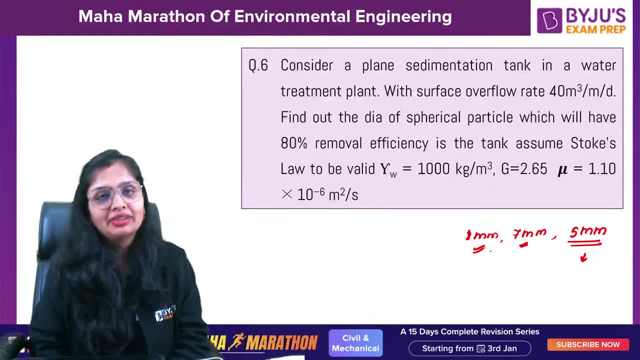 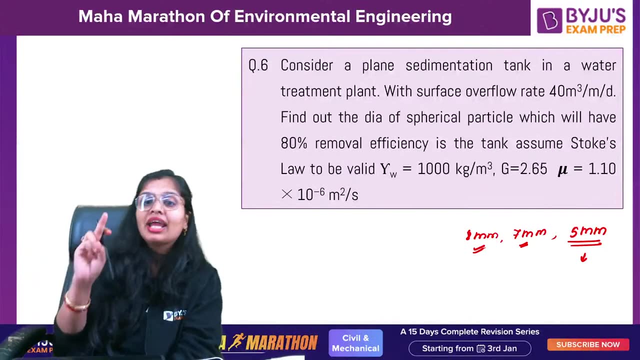 And in the water 8 mm and 7 mm particles are there 100%. Very good Why? Because any size of the particle or any velocity- Remember Any size of the particle or any velocity more than the settling velocity of the concerned size of particle. 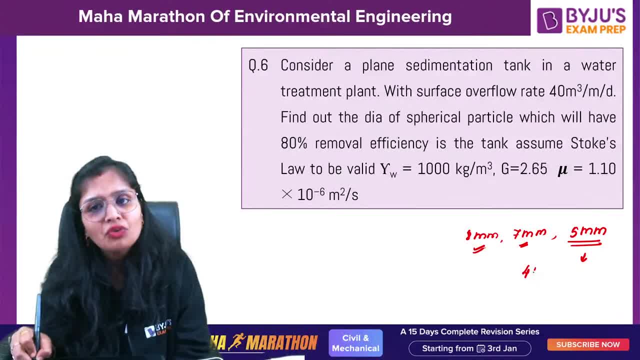 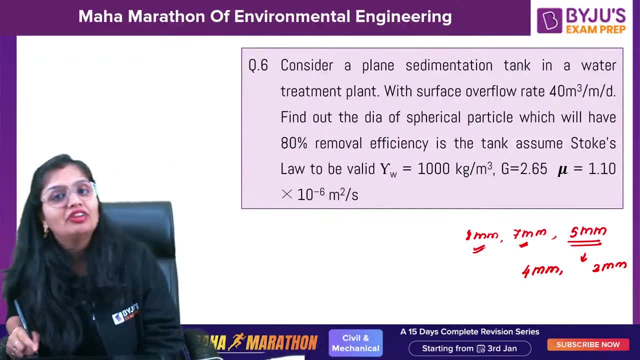 100% efficient Will 4 mm, 3 mm? They will also be removed. Remember, This can be asked in statement. wise, But not completely. They will be partially removed. Okay, This you should know. Now Talk about this. 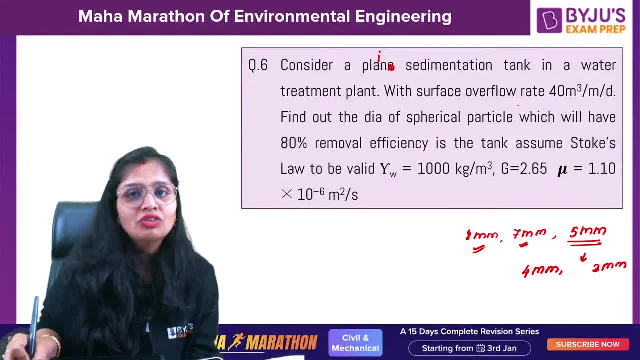 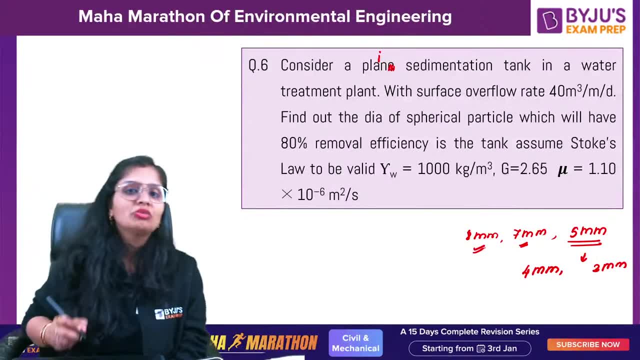 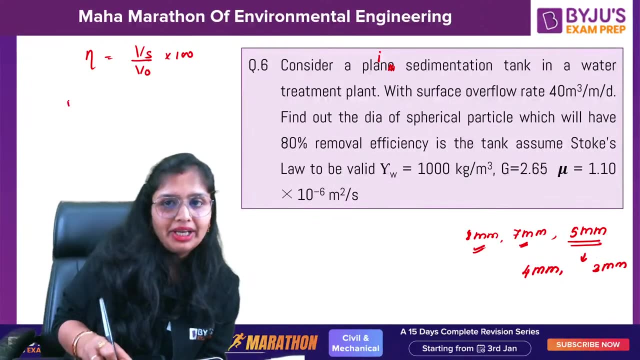 Consider a plain sedimentation tank. Surface overflow rate is given to you. It is asking you to calculate the dia Of that particle, which has 80% removal efficiency Vs by V0 into 100.. So 80% is given to me. 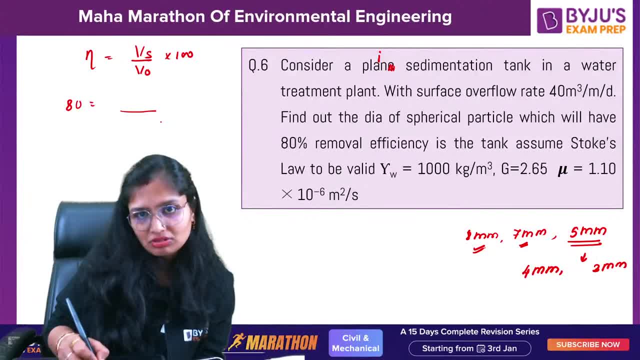 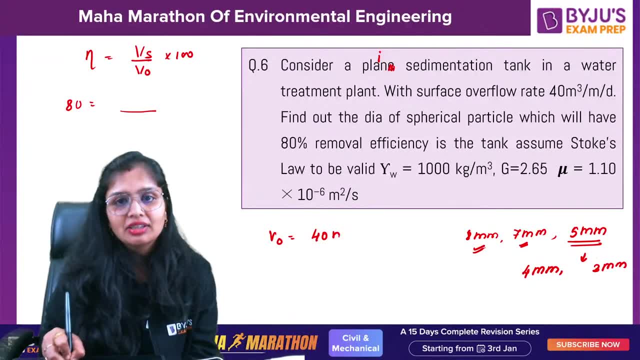 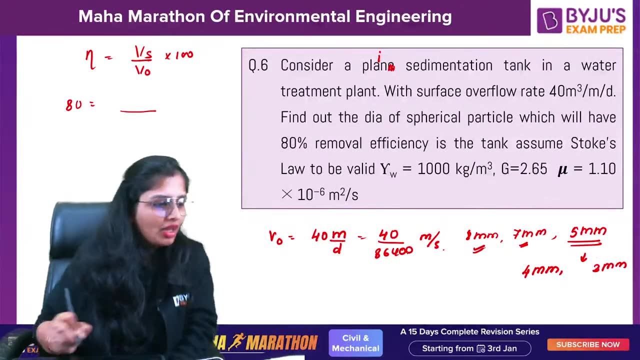 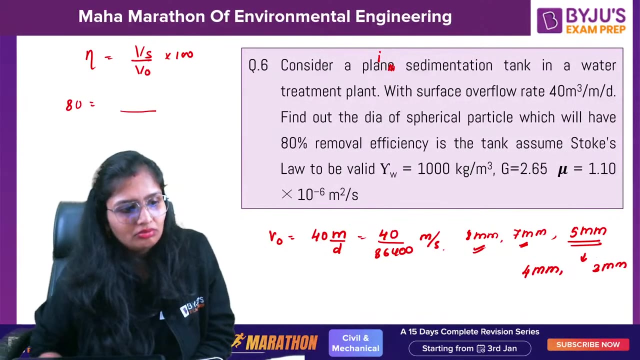 Velocity overflow rate. Let us calculate it in meters per day. Convert it into meters per second. first, V0 converted into meters per second. This is meter per day Vt divided by 864, 00.. Converted, How much it is coming? 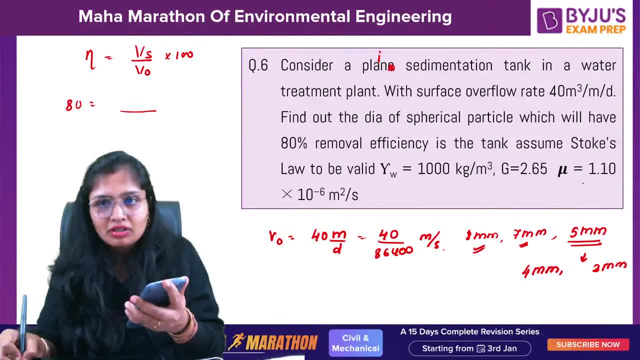 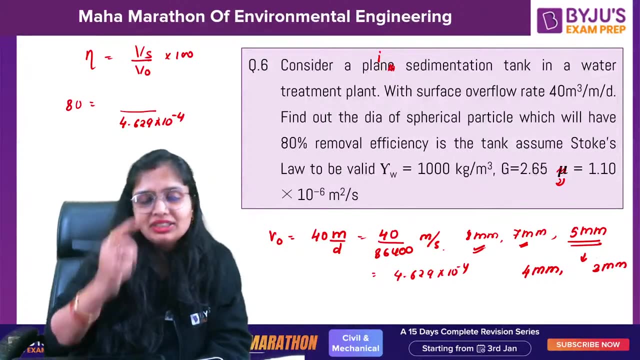 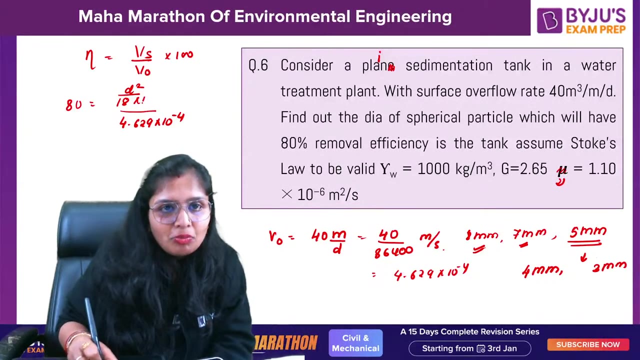 J. This is kinematic because it is given meter's square per second, no 629 into 10 raised to power minus 4.. This much it is coming: 4.629 into 10 raised to power minus 4.. Now settling velocity d square by 80 nu laminar- We are assuming it laminar- 1.10 into 10 raised. 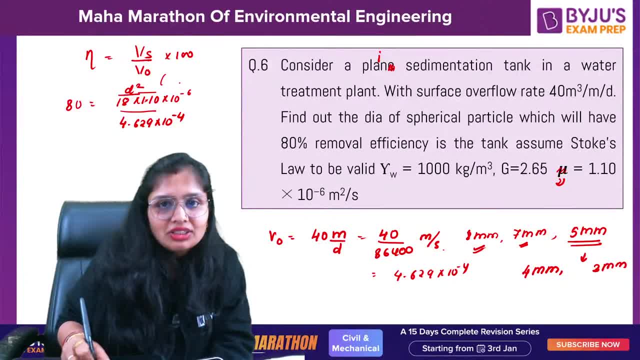 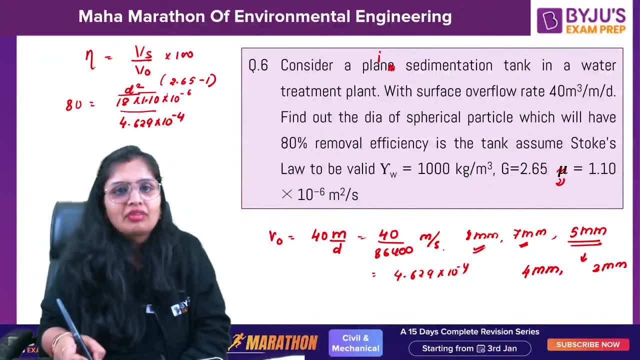 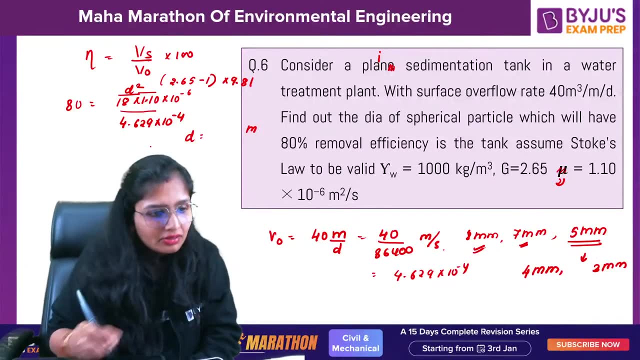 to power minus 6.. gs minus 1.. gs is 2.65 minus 1.. How much it is coming Into 9.8.. See first tell me the answer in meter. You are telling for this. Ashish, Ashish, I have. 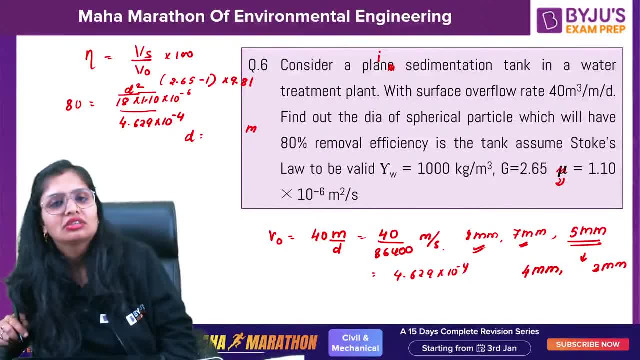 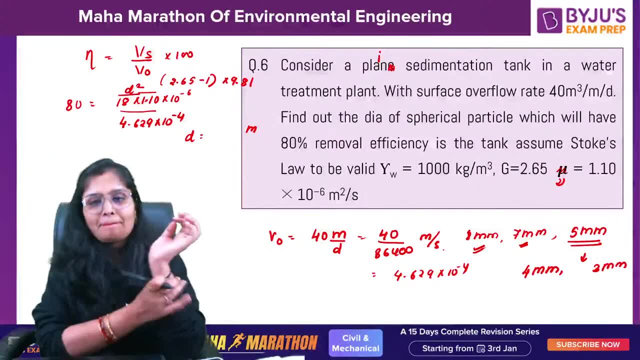 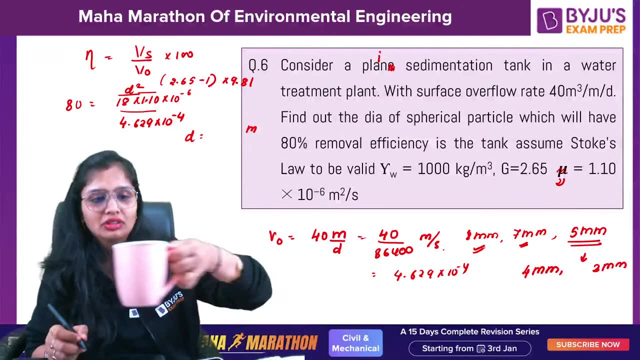 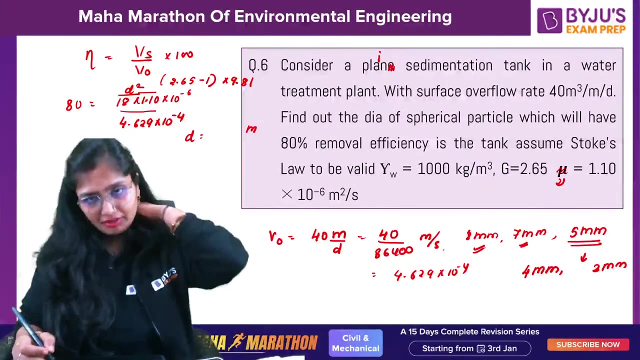 corrected it. It was 15 TCU. I corrected it. I guess you were not there, so I am telling you How much it is there. Come on, guys, solve this and tell me Fast, fast. Tell me in meters. We will convert it into micrometers. 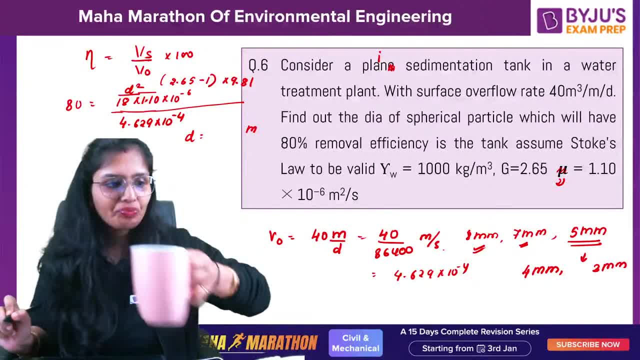 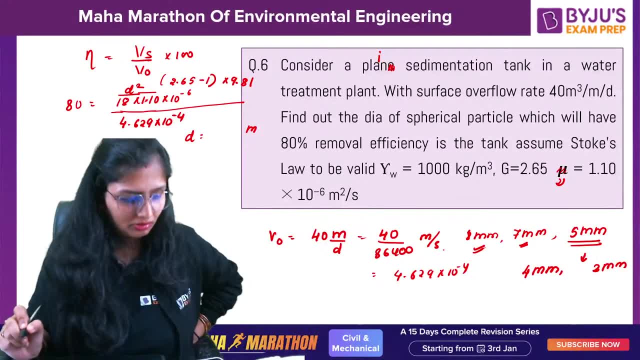 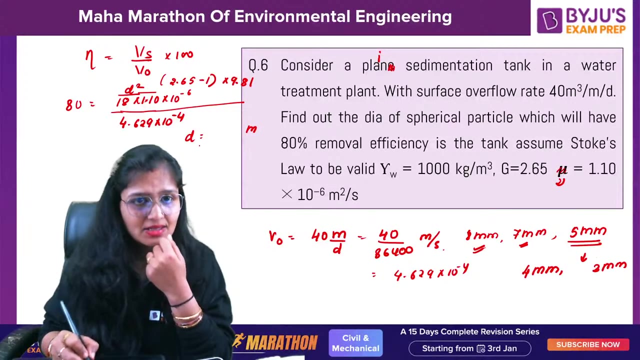 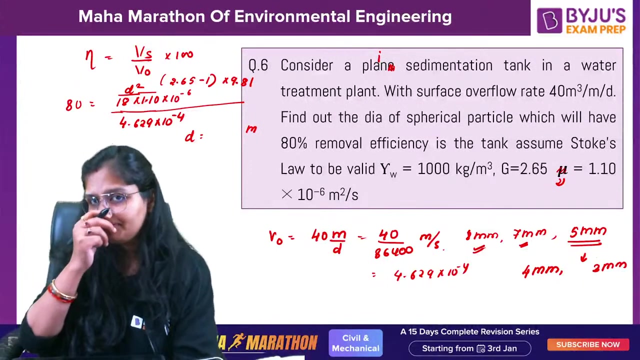 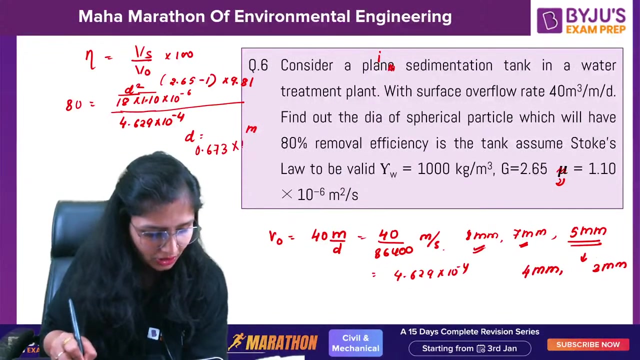 How much it is coming, Is it? I have taken this as nu. Fine, Okay, it is coming like this: 0.673 into 10, raised to power minus 6.. No, no, no, no, no, Deepak, it is wrong. 1, 2,, 3, 4.. This is wrong. Just one of the other. 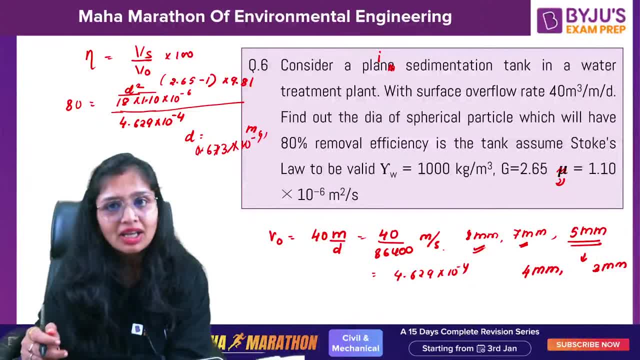 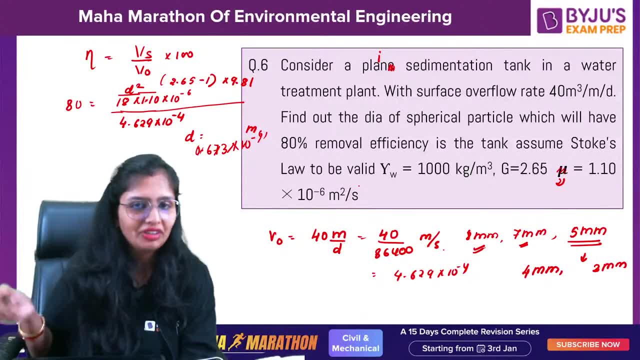 person also calculate mvs. Okay, fine. Actually they should have written it here: newton. second per meter square. This much kinematic viscosity we do not get. but fine, We have written meter square per second. 0.673. Deepak is correct, So mvs is wrong, Fine you. 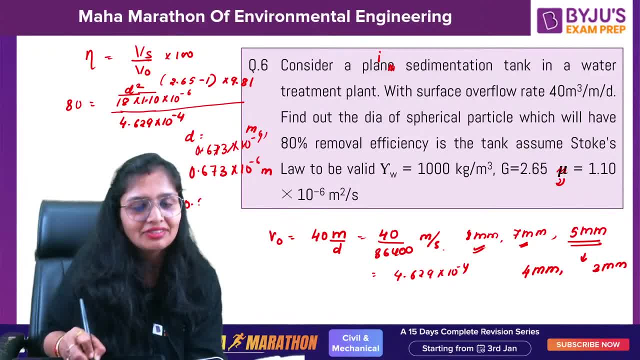 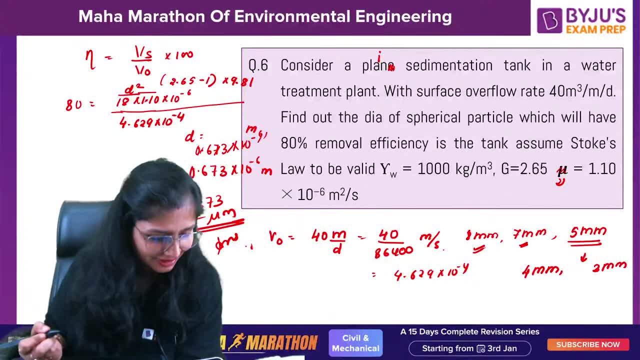 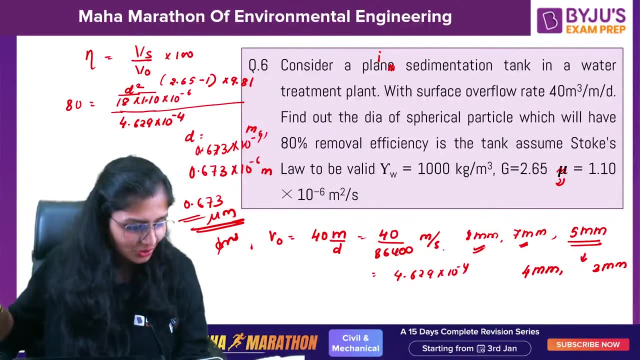 guys can calculate this. This is 0.673 micrometers. Okay, fine, mvs is correct: 8.48 guys calculate this logic. I have told you: Okay, you guys can calculate this. 2, 3 people have got the. 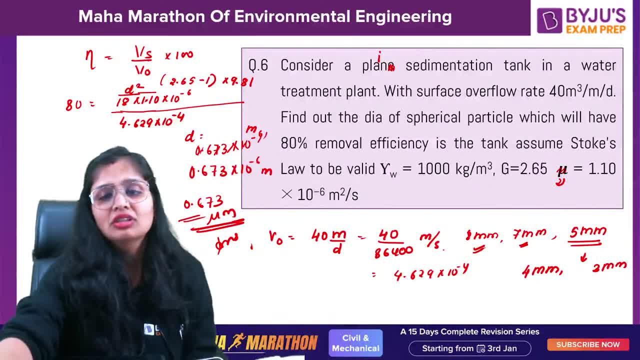 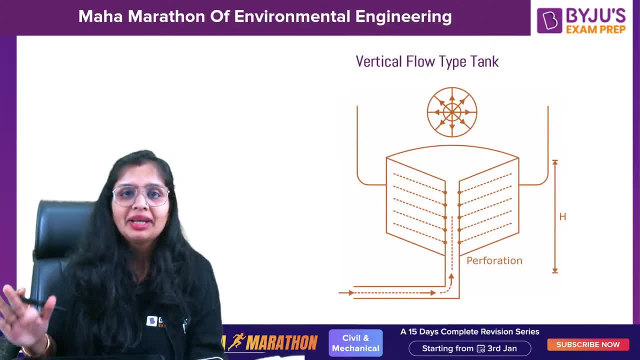 same answer. so I am taking that Arun, just take it one more time. It is correct, This is correct. I have taken this one as nu. I have taken this one as 2.73 micrometers And take it once again better, okay, fine, so now talking about vertical flow type: tank vertical flow type. 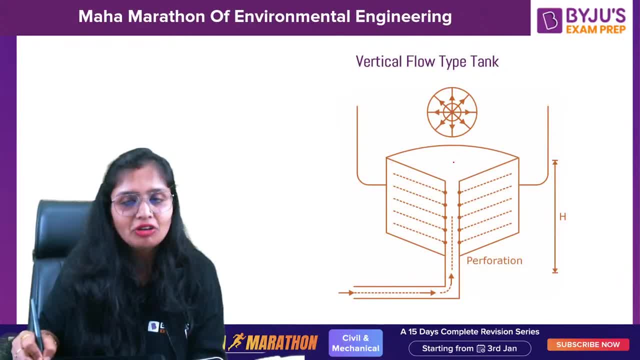 tank, what you see as you move. actually you see it from here. you see that the water moves only in two directions, but the water moves in all the directions. so now, what is happening here? what is happening here? the water moves. as the water moves away, the velocity decreases first, 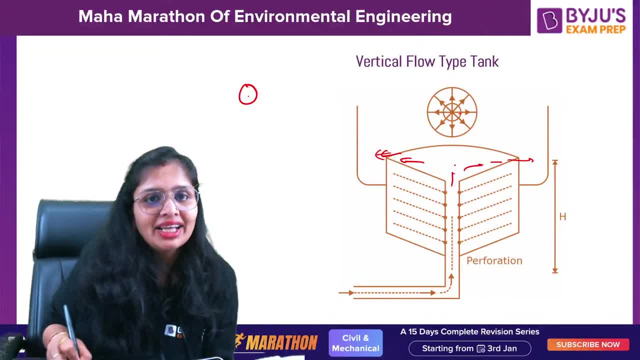 of all. moreover, here, if the particle is there, it has two velocity: one is settling velocity and other one is the flow velocity. so, if you take the resultant of it, this is the parabolic in nature. remember- this is an important statement, wise questions when you talk about horizontal flow. 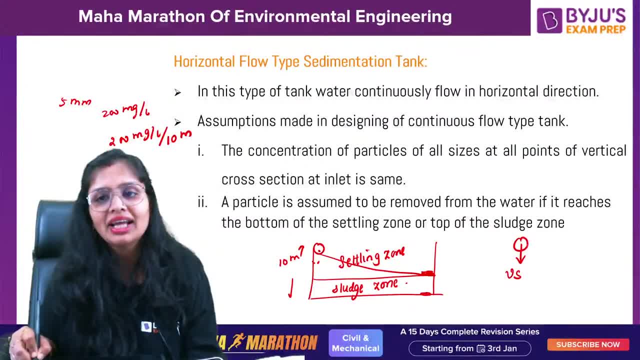 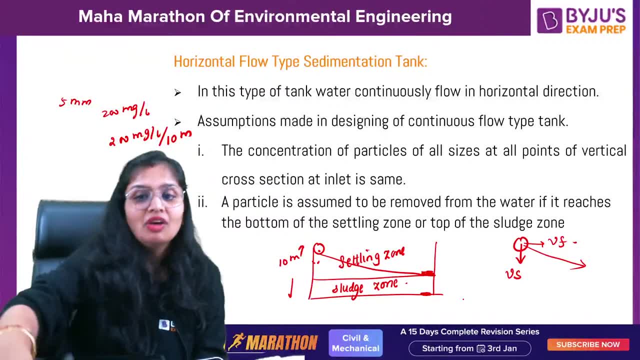 type tank. if this is the, this is the settling velocity and this is the flow velocity. so the resultant will be linear, okay, straight path will be followed, while in the case of vertical flow tight tank, parabolic path is followed. Firstly, and here you should also know, one thing, you should also know: 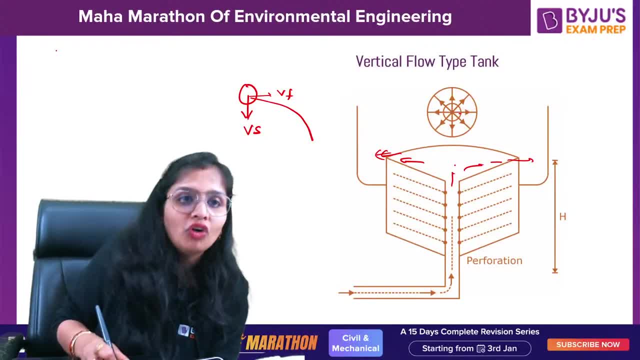 one thing: that here, if you want to calculate the volume, there is a formula: d square 0.785h plus 0.011d. So d is the diameter, h is the height. So with the help of this you will get. 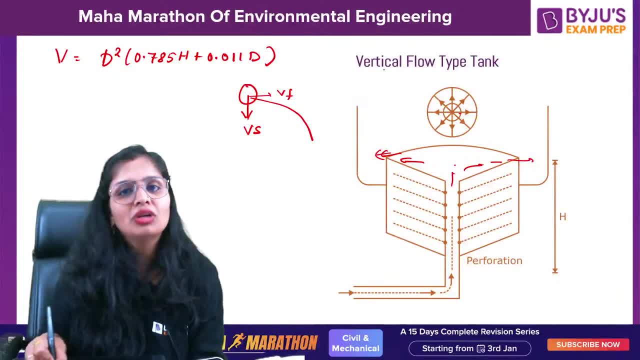 the volume, you will get the volume. So this is the formula for vertical flow type time. Now in examination, sometimes they ask you simple questions, like they will: discharge is equal to area into velocity, So they will give you the discharge, they will give you the area, they will. 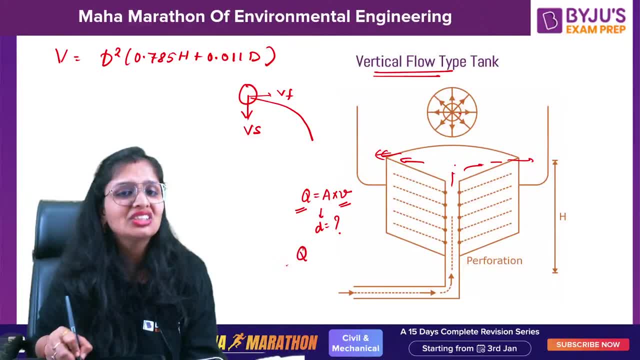 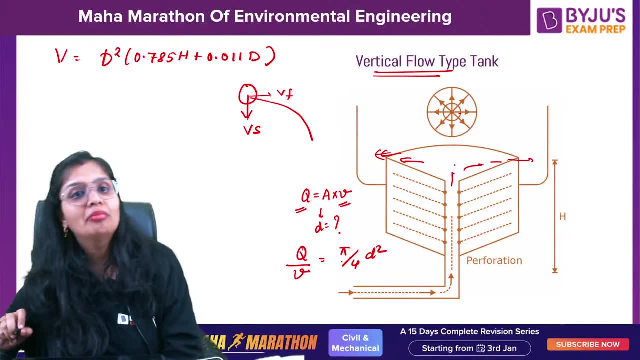 ask you the dia. So if they ask us out of quotient discharge divided by velocity, this will be pi by 4 d square. So in that case you can go by this method. But if, specifically, it is telling you to use the empirical method, you can go by this method. So in that case you can go by this. 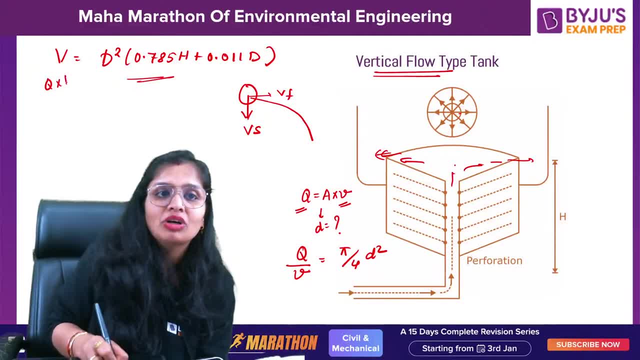 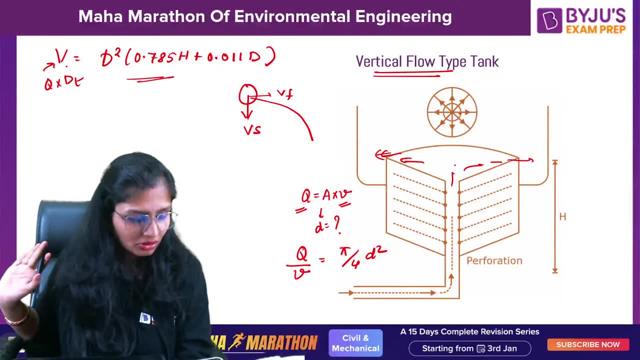 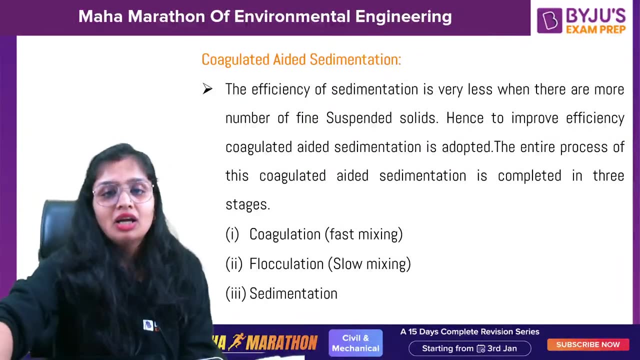 formula. It has given you discharge retention time and all. So first you will calculate the volume and with the help of that you can get the dia. Okay, So anybody else haven't checked the answer. So this is for vertical flow type time. Okay, Okay, Any doubts still here? Any doubts? 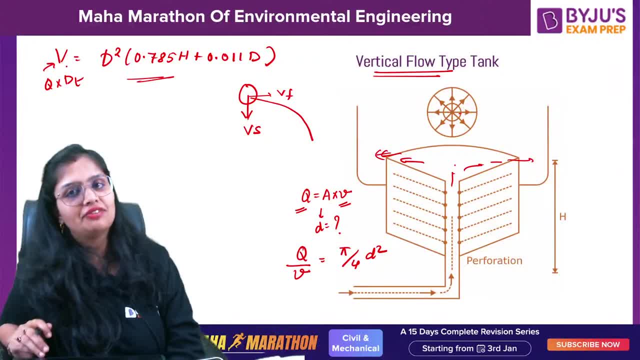 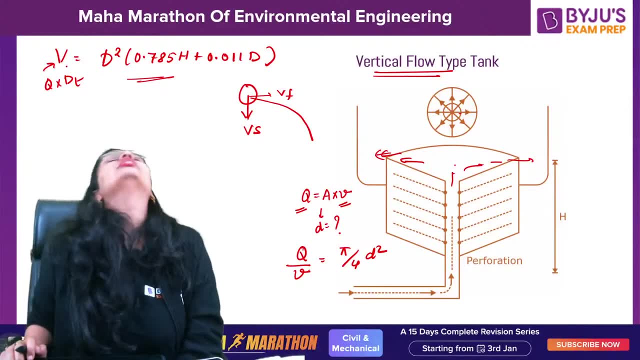 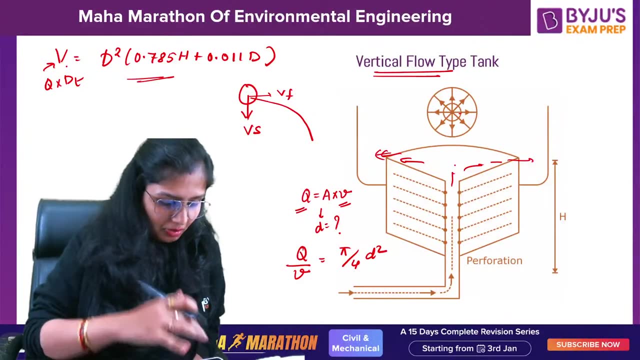 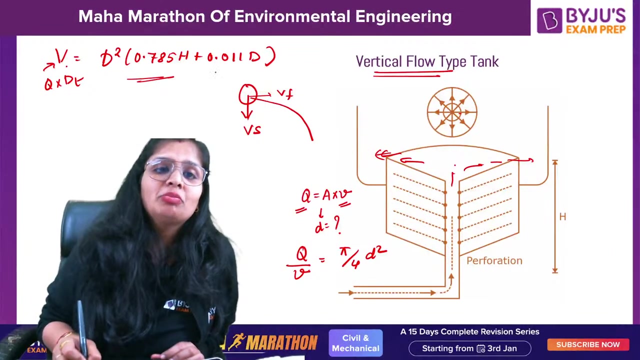 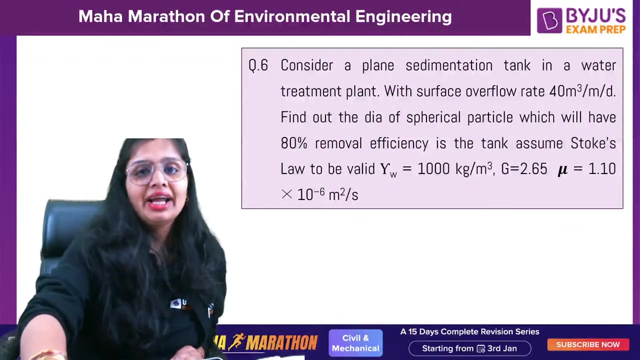 still here? Ask to me fast, Fastly, fastly, fastly, No doubts. Formula once, ma'am, Ma'am, previous quotient, please show. Okay, fine, Formula is: v is equal to d square 0.785 h plus 0.011 d. d is the diameter and h is the height. h is the height. 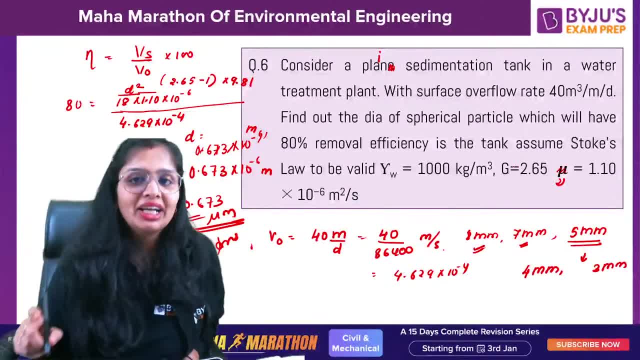 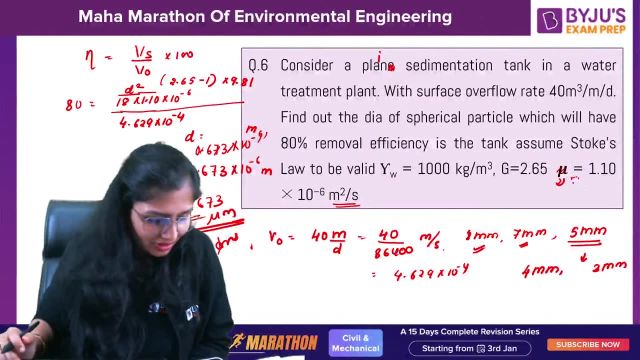 Okay. Next, this quotient. they have made a mistake. They should have written in: this should be: if it is kinematic Viscosity, it should be dynamic, But based on the unit it comes out to be kinematic, Some sort of magic is happening. I am not touching and the slide is going. Okay, Fine Now. 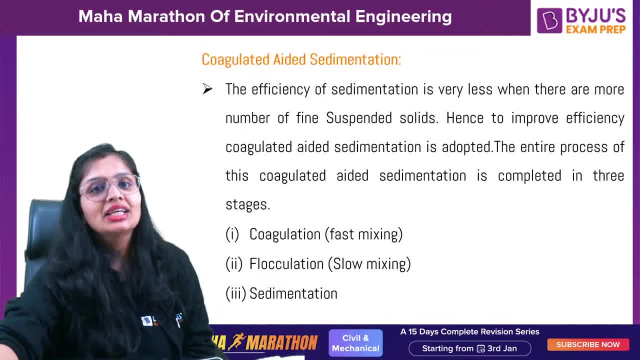 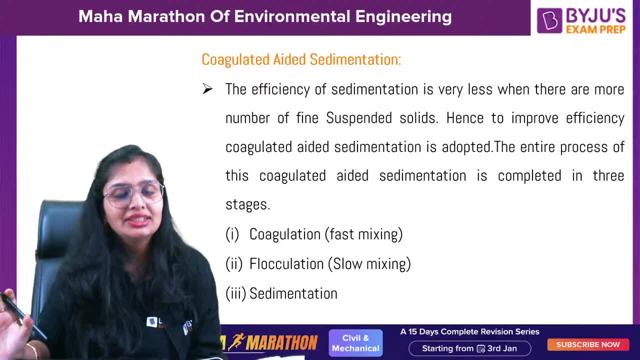 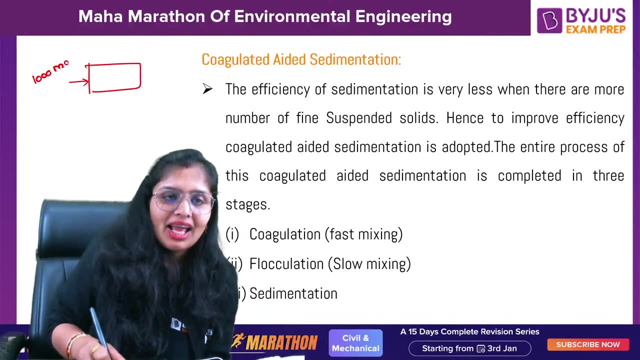 talking about next? talking about next is coagulation, aided sedimentation. Some student was having doubt also. You can understand this. See, let us suppose if the solid switch was coming is 1000 mg per litre and the solids after plain sedimentation, which goes, was 600 mg per litre. 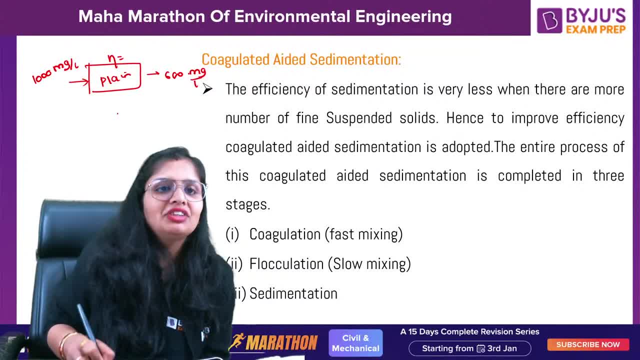 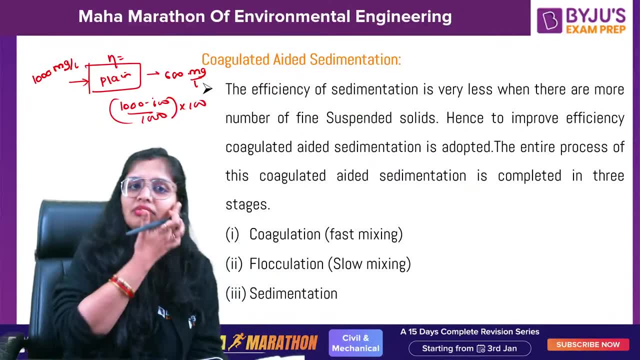 What is the efficiency of the sedimentation tank? What is the efficiency? 100 minus 6,000, minus 600, divided by 1000 into 100.. It comes out to be how much? How much is the efficiency? 400.. 40%. 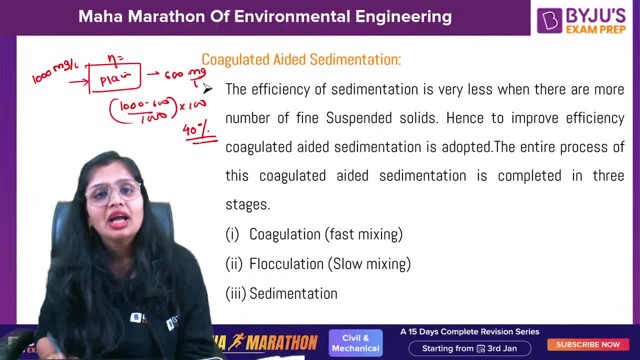 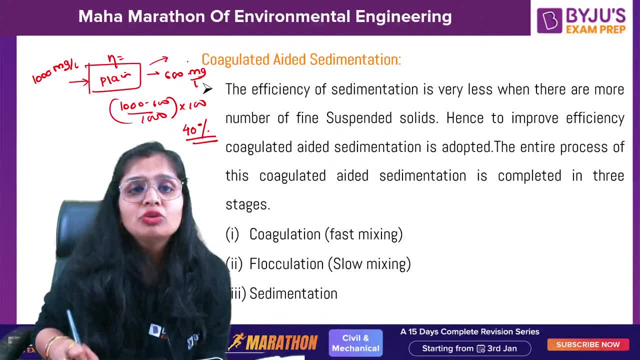 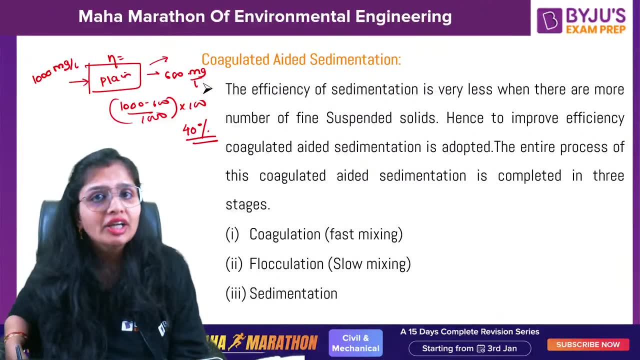 is the efficiency. But actually I need a tank with the efficiency of, let us suppose, 80% or 90% or 95%, because I want even the finer solids should be removed. That doesn't happen. plain sedimentation In that case. 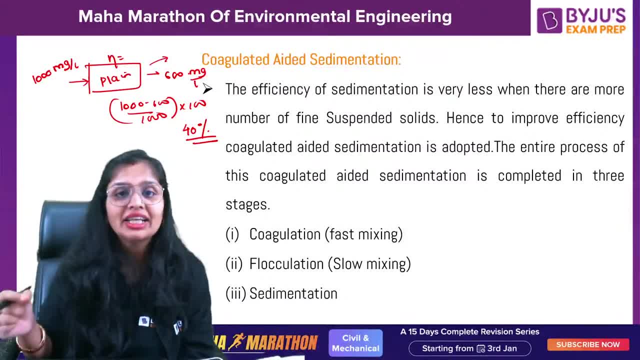 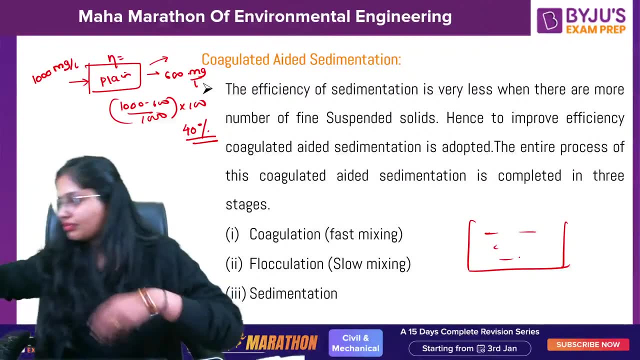 you have to go for coagulants. you have to add certain chemicals. Now these chemicals are known as coagulants. What do this chemical do When you add them? See, particles are not settling. if you see this, these particles are not settling. 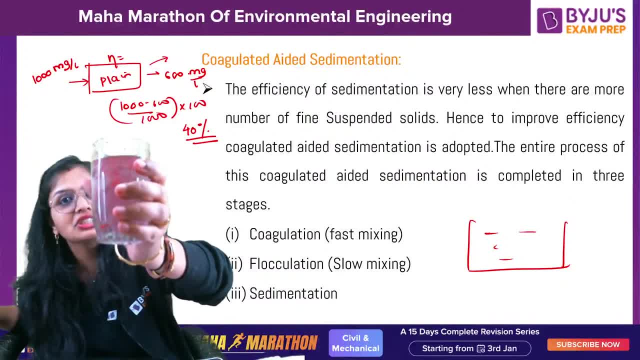 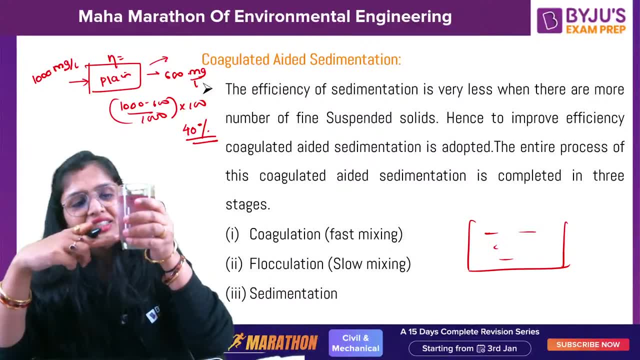 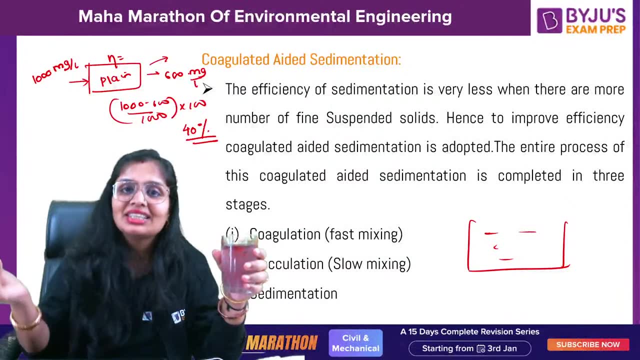 why? because they are stable. because they are stable, they will settle. if I add a chemical in this, if I add a chemical in this, so that the stabilization will be what the destabilization will be take place, the stabilization will be destroyed, the destabilization of the particle will take place. so for the 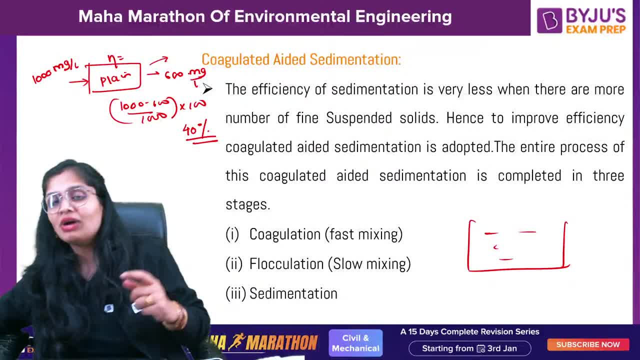 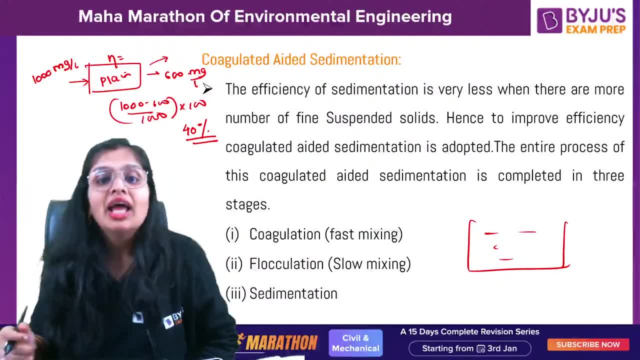 destabilization of these suspended particles. I need to add chemical. I need to remove the finer impurities. also, I need to add chemical, which is known as coagulants. now, firstly, you can add coagulant in powdered form. you can add it in solution form. generally we add it in solution form. now, when you add any, 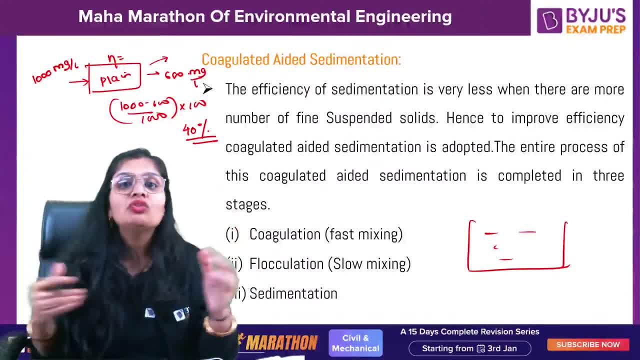 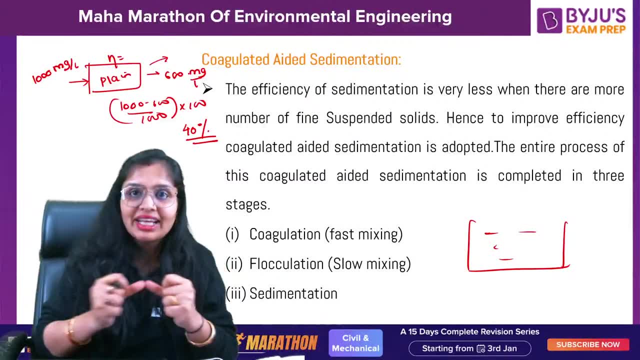 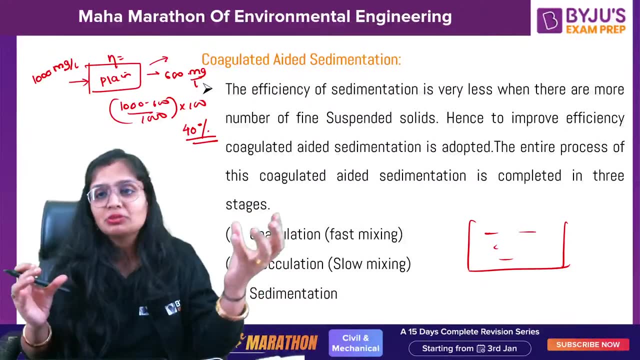 coagulant. you want that it should evenly spread. so you do fast mixing. okay, fast mixing is introduced so that first the particles get destabilized, after that you pass it through mixing right, so that the destabilized particles- small, small particles, which are now not at all stable- they combine with each other. 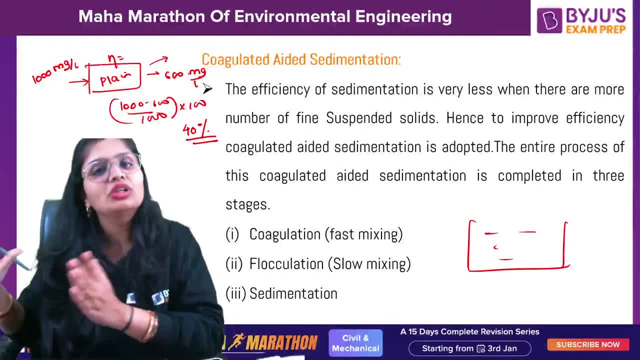 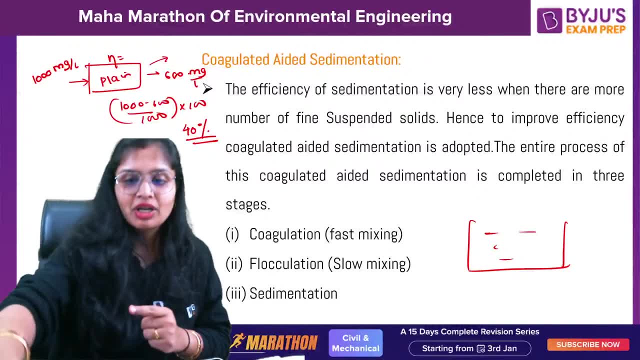 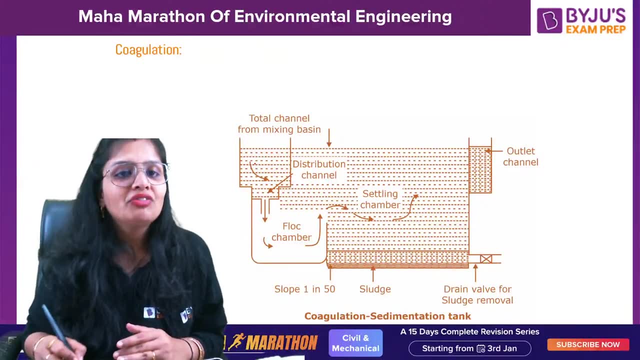 become bigger in size and eventually they go into the sedimentation tank and settle. so it's coagulation, it is sedimentation, coagulation, flocculation, then sedimentation. now this is the thing. you can add three different chambers for this or what you can do it. you can first mix it, then make it in the, take it to the flocculation. 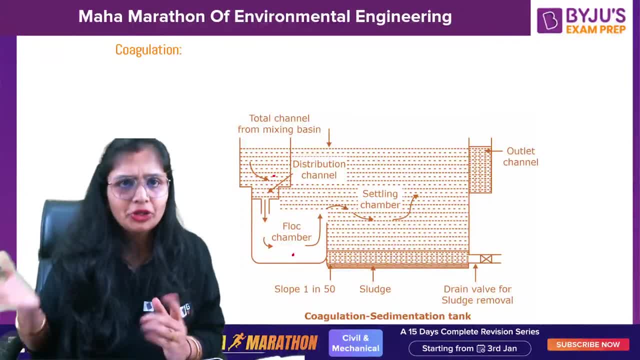 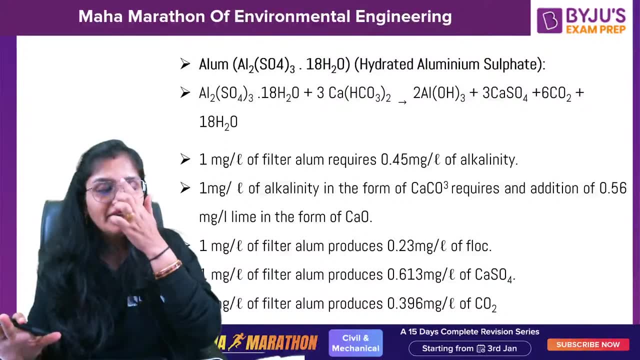 chamber and then take it into the settling chamber. that depends upon you. okay, now what happens here? there are different types of coagulants which are added. one coagulant which is very much important, on which questions has been asked, is alum AL2SO43.18H2O, that is, hydrated aluminum solvent. 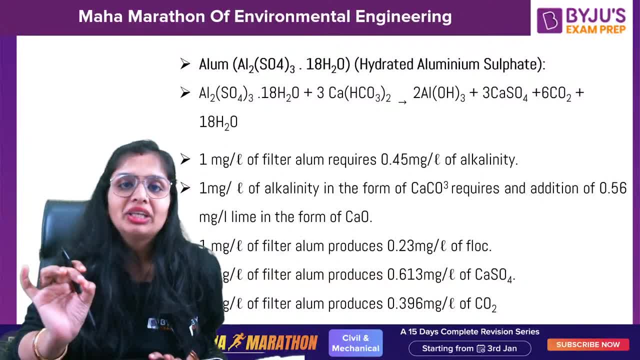 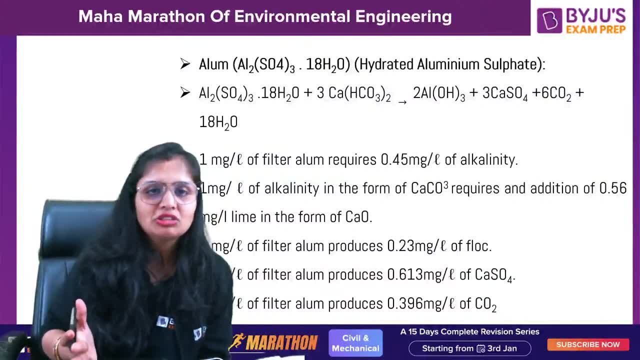 AL2SO43.18H2O, that is hydrated aluminum solvent. AL2SO43.18H2O, that is hydrated aluminum solvent thing Generally. I tell you to remember this so that you can solve any questions. If you want to go by gram equivalence method, you can go by that method. also, See the weight of this Al2SO4. 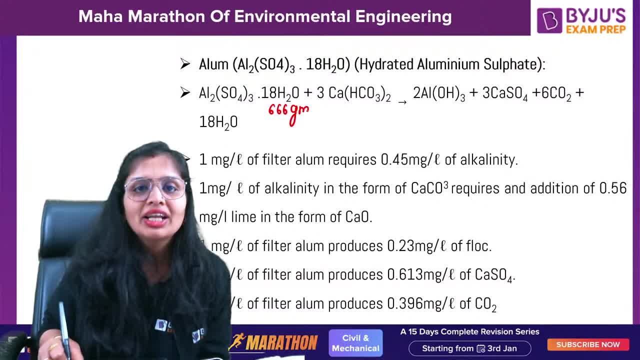 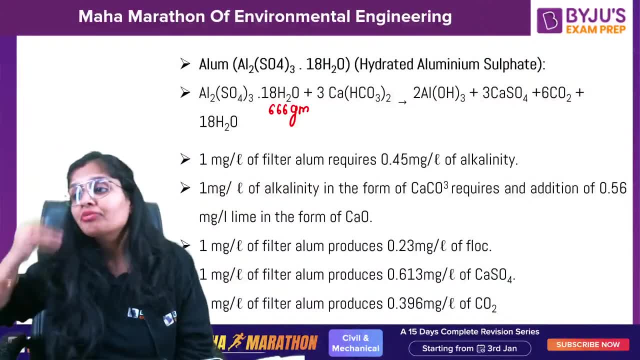 thrice dot. 18H2O is 666 grams. What I tell you is: alum will function only if you give bicarbonate alkanate Now. if it is not present, it won't function. So if you want alum to function, 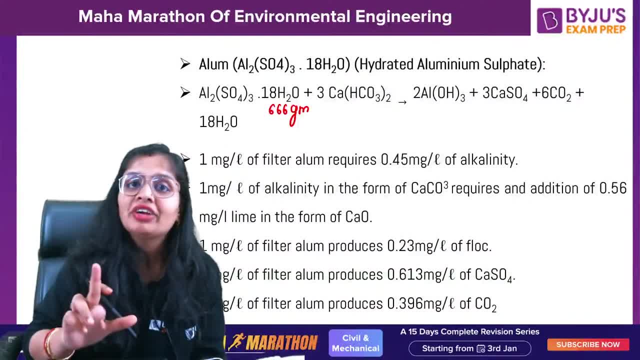 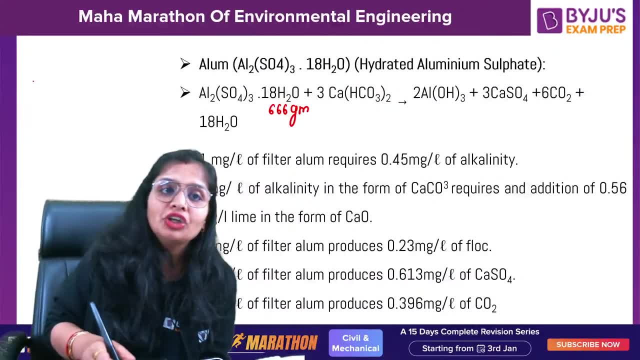 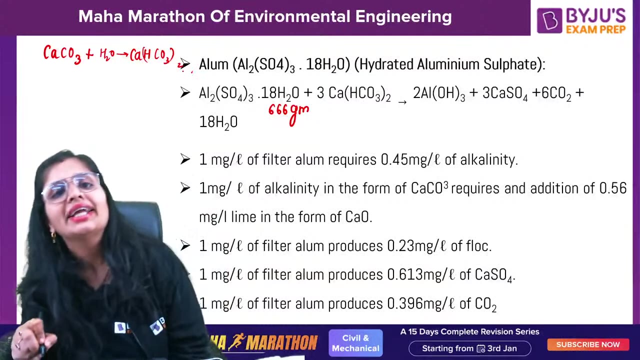 you need to give it bicarbonate, alkanate. If you are not giving it, it will not at all function. Firstly now, if calcium bicarbonate is not present, what you will do? You will add calcium carbonate. plus how you will get Water or carbon dioxide? Tell me For getting calcium bicarbonate. 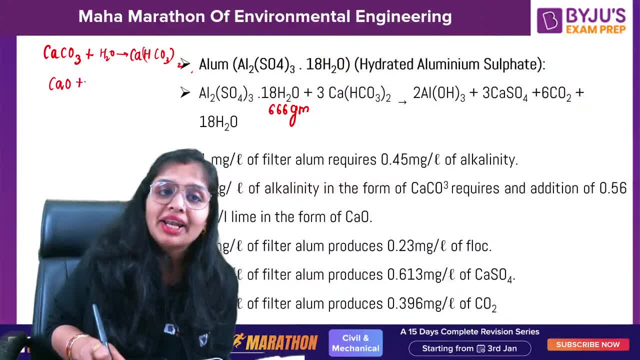 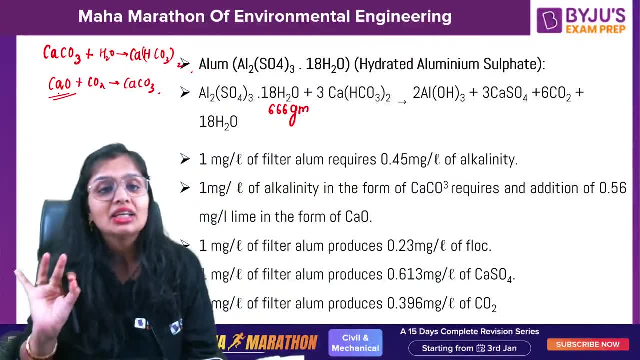 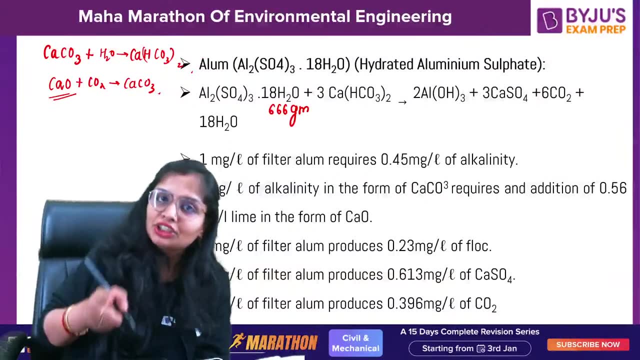 Calcium carbonate will also be not available to you directly, Then you need to add what You need: to add: calcium oxide. So this is the question which is asked on prominent basis: Calcium bicarbonate will be formed when you add calcium carbonate. 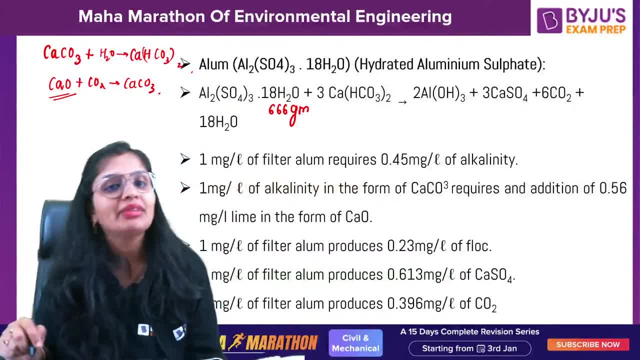 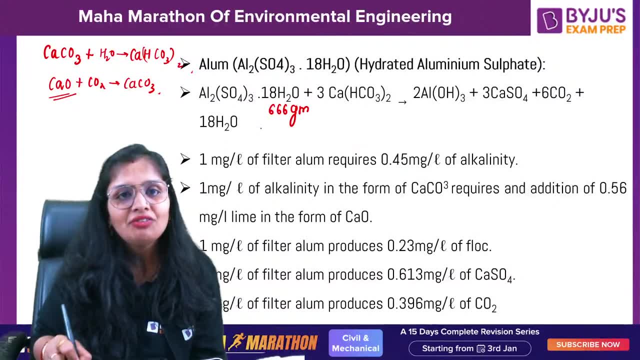 Calcium carbonate will be formed when you add quicklime. that is calcium oxide. So generally, it is very simple to understand that. what happens if 666 grams requires 3 into 8 grams? This is firstly, this is calcium bicarbonate, and calcium bicarbonate will come. 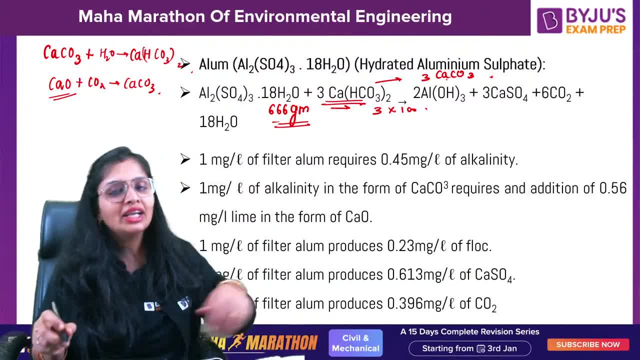 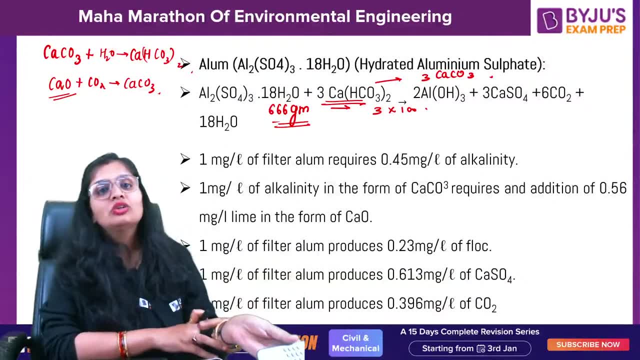 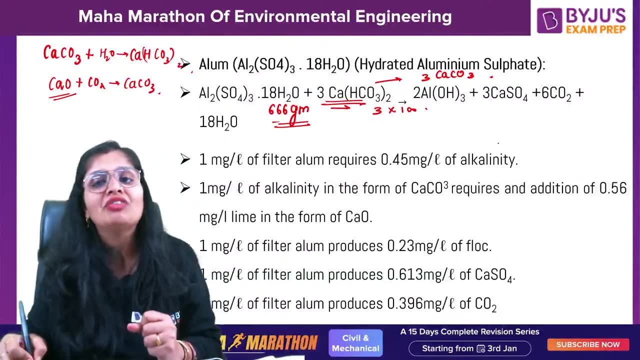 when you add 3 into calcium carbonate. So 300 divided by 666, you will do 0.45, it will come. So if you need, if you want 1 mg of filter alum to function, you need to give 0.45 mg of. 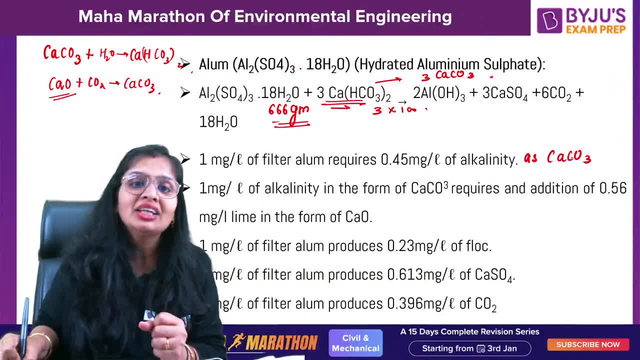 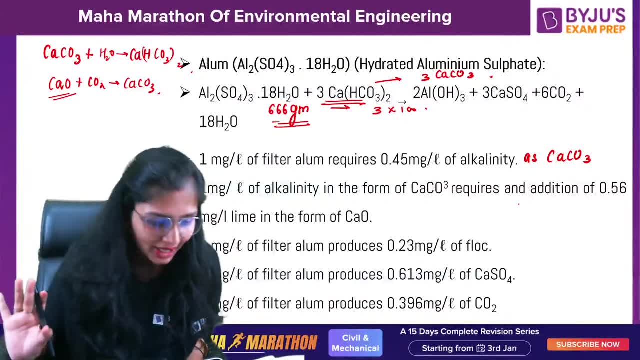 alkanate as calcium carbonate. So either you can have waste your time doing the manual calculation or you can remember this. This will be easy for you to understand. That depends upon you. That's entirely your call. You can do it and you will get the answer. 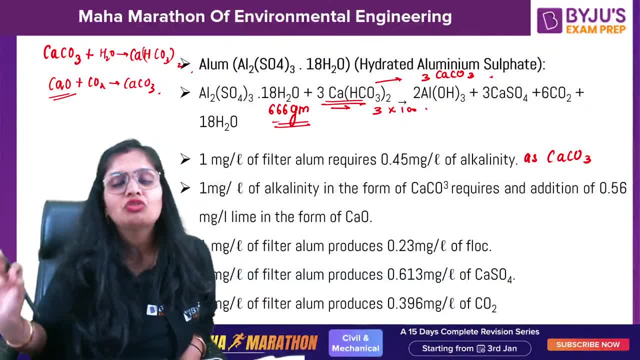 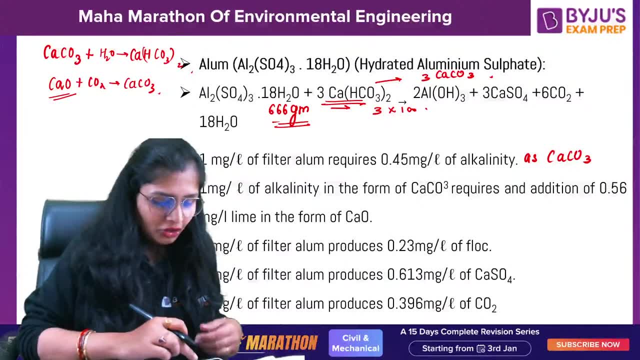 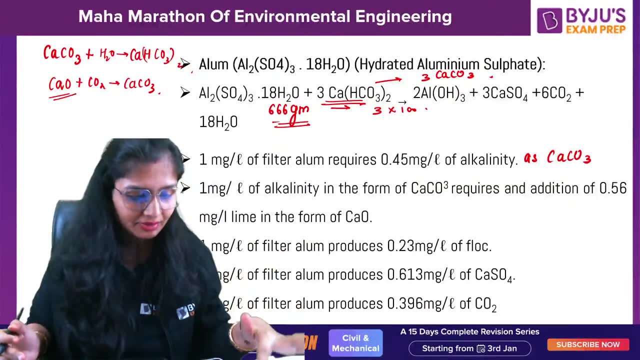 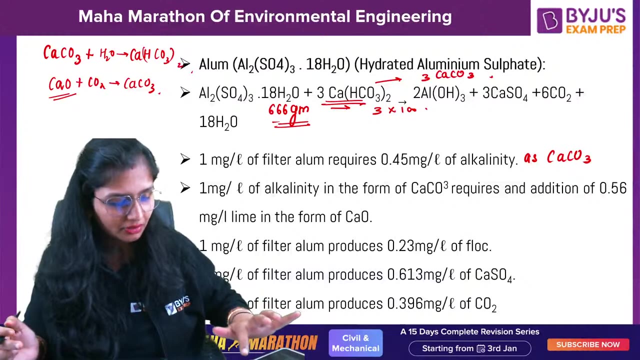 Okay, But remember, alum will not at all function if you won't provide the algorithm. Till here it is clear. You want to do question on this. You want to do question on this or you have practiced already. Tell me fast: You want to do question on this or we will move further. 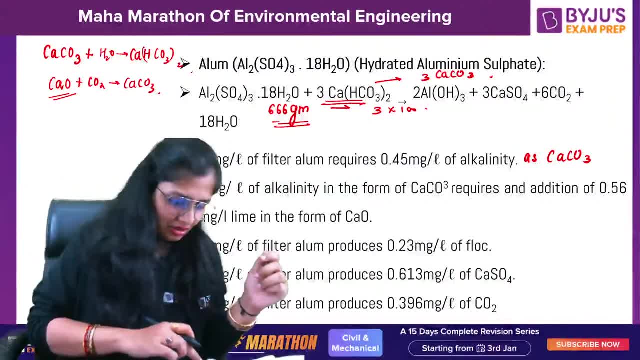 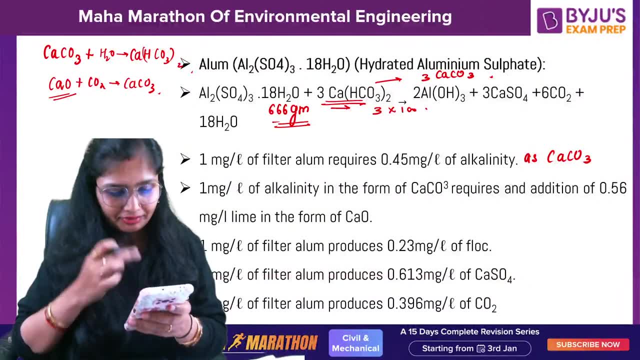 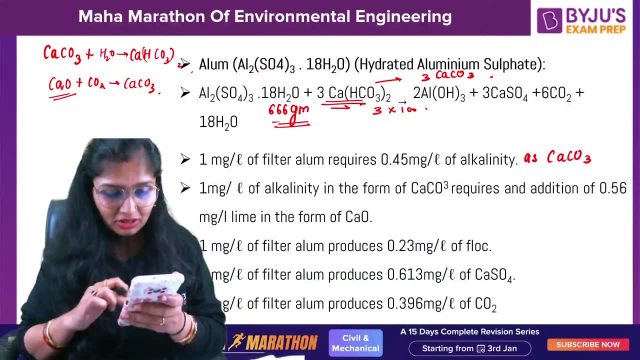 Question. Okay, So simple question. is there Fine That gate question which is asked, and you will understand that this is very important. You will understand that this is very important. You will understand that this is very simple. Based on this, you can solve any question. 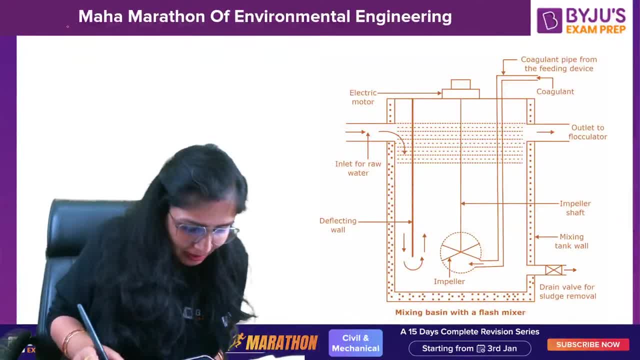 Simple question is there? What you have to do? Simple, simple: 10 MLD of water is to be treated. 10 MLD of water is to be treated. Alum dosage is given to you as 20 MG per liter. 20 MG per liter, it is given to you And water already has alkalinity. 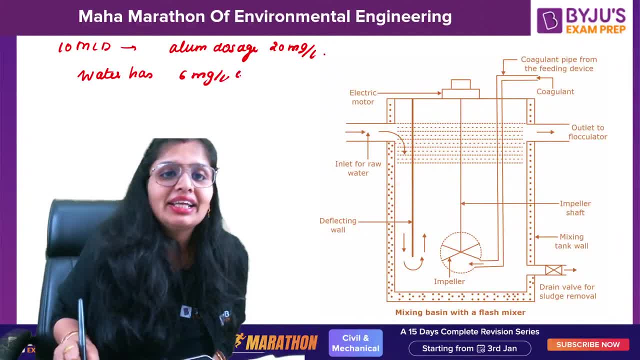 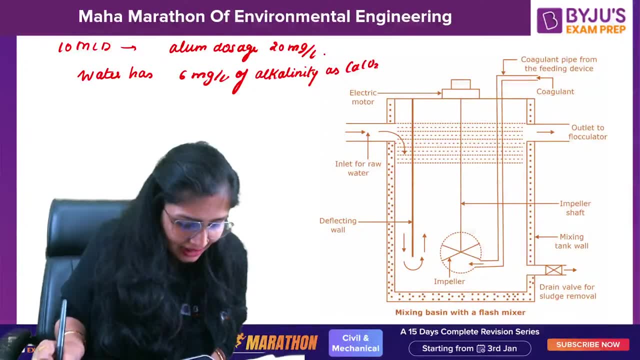 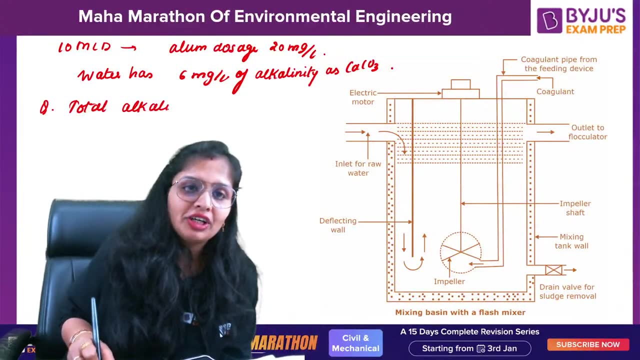 Water has 6 MG per liter of alkalinity as calcium carbonate. It has this much alkalinity as calcium carbonate. Now what it is asking you in the question: Total alkalinity requirement. Come on, guys, Solve this. Arun Devanshu, I want everybody to answer it. Total alkalinity requirement. 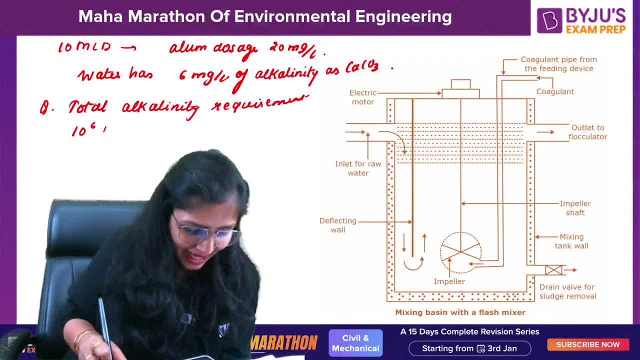 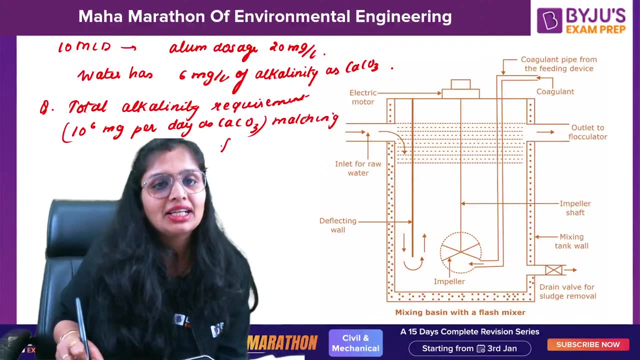 Okay, How much? 10 raised to power: 6 MG per day as calcium carbonate. Total alkalinity: it is asking Total means it is not bothered about how much is there and at all. It is asking the total alkalinity as calcium carbonate. Come on guys, A option is 120.. However. 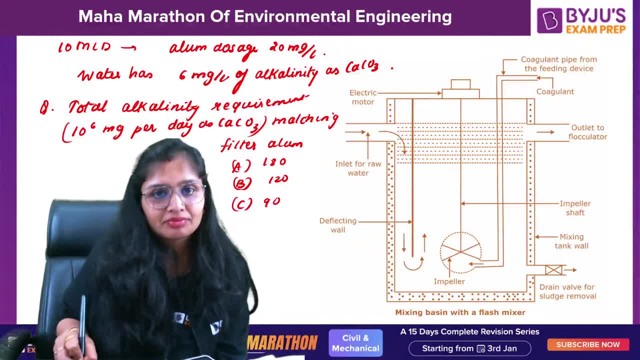 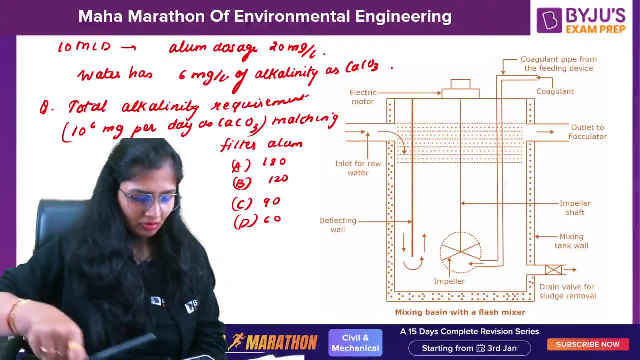 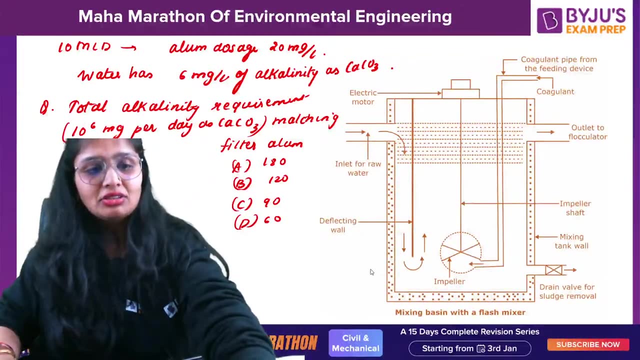 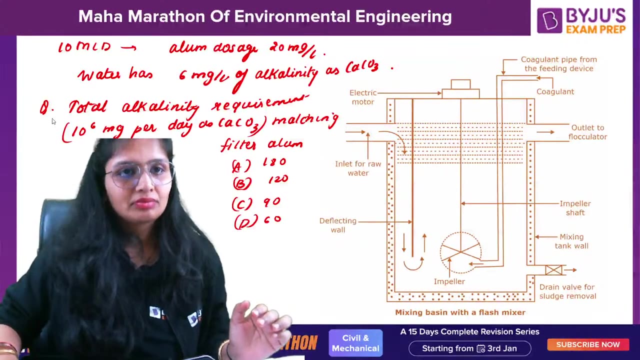 I shouldn't give you, but fine, I am giving it. Come on, mate, I will repeat it at the last beta. it's not possible now to go there. Not possible. I have to clearly repeat. I have to clearly repeat all the questions. 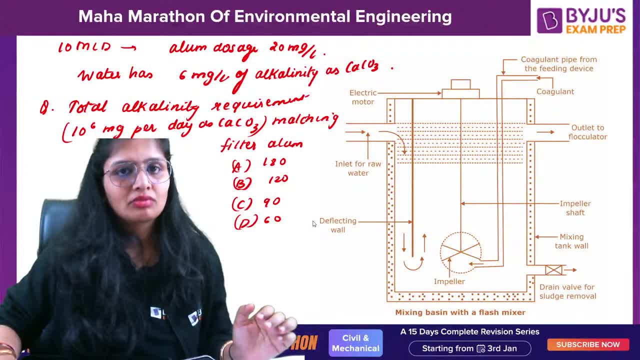 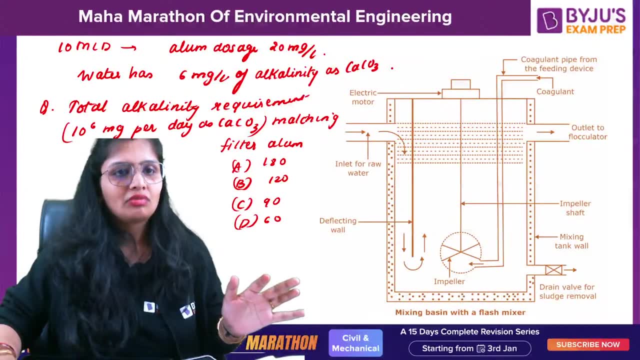 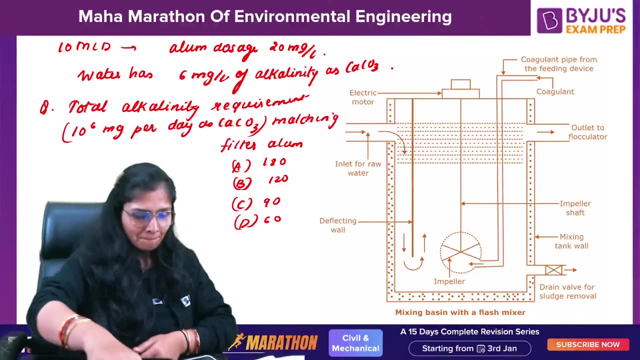 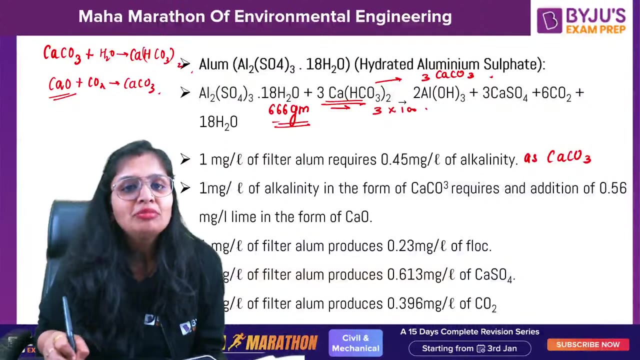 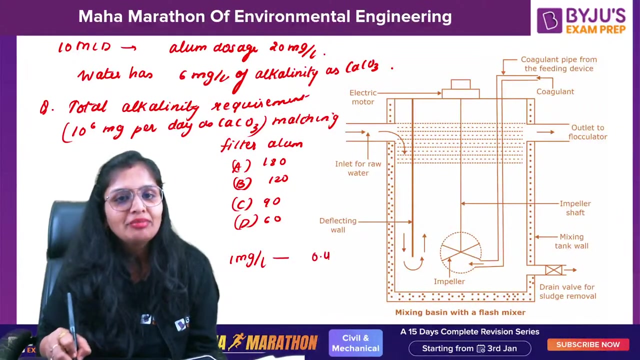 The other questions will be answered. question one, question two. question one, question one. got that okay, let's check it out. see, very simple. if you know this, 1 mg of filter alum requires 0.45 mg of alkalinity. 1 mg per liter requires 0.45 mg per liter of alkalinity. so, so, so, so so. 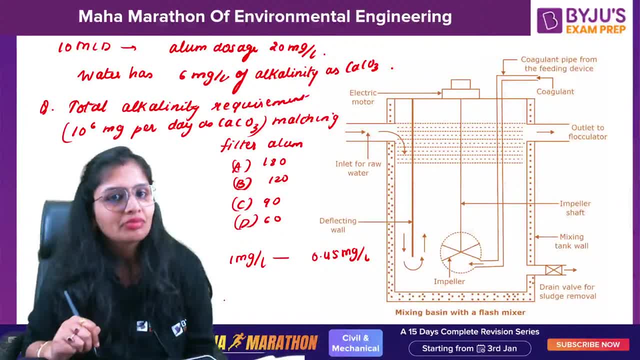 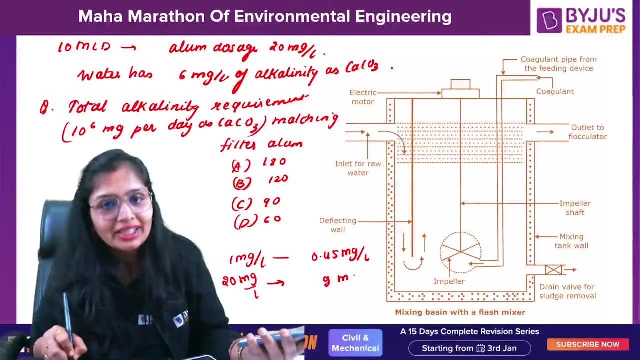 so 20 mg will require how much? in this manner you did it, 20 mg per liter will require how much of alkalinity? 20 into 0.45 it is coming 9, 9 mg per liter of alkalinity. so if 1 liter of alkalinity 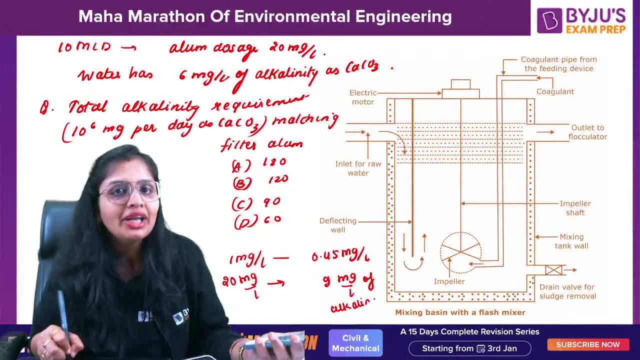 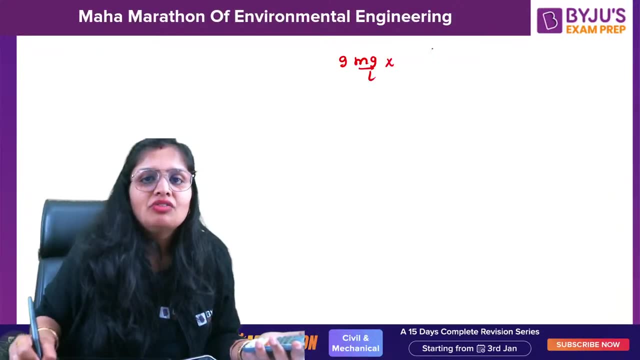 9 mg per liter of alkalinity is required, so for. so for how much liters it is there? 10 ml t, how much it will be required? so how come it is coming 120, so 9 mg per liter is required, so for 10 into. 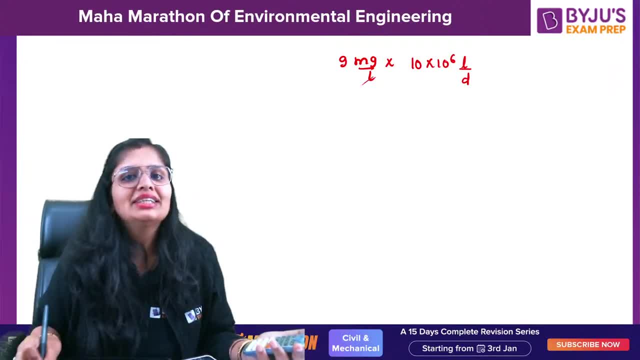 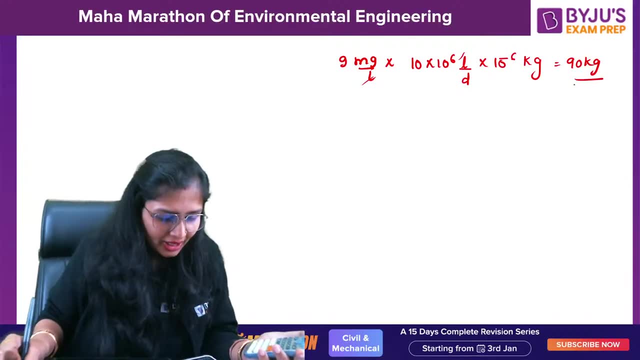 10 raised to power, 6 liters per day. how much it will be required: see liters, and liters will get cancelled. mg converted into kg, it will be like this: so it is 90 kg. got it? Devanshwar who was telling me no, no, some other guy was, Prashant was telling me for understanding. 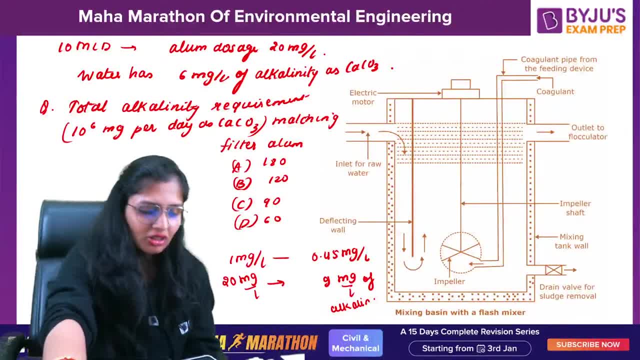 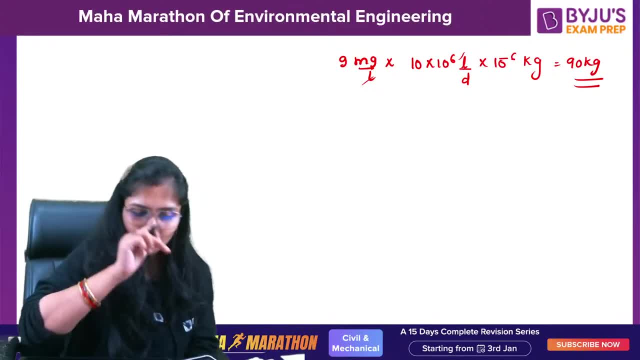 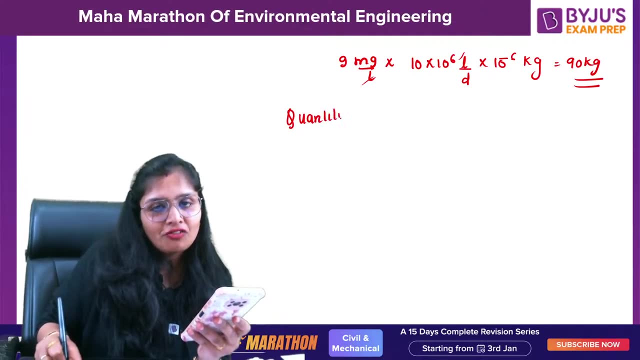 this very carefully understood. so if you know this, things becomes very easy. now, one more question which was asked in this topic, one: oh, Swapnil, you are there now. you answered my god, I thought you are not there today. okay, quantity of quick lime required now. see, this is the second question. 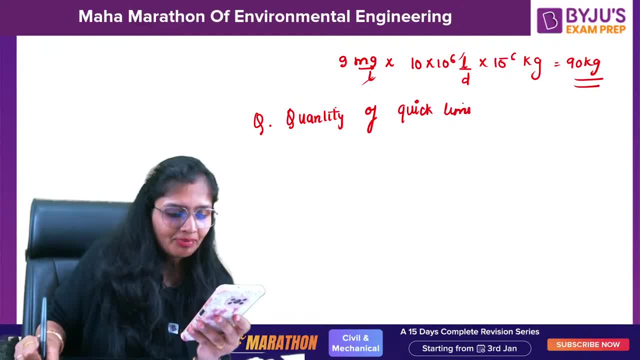 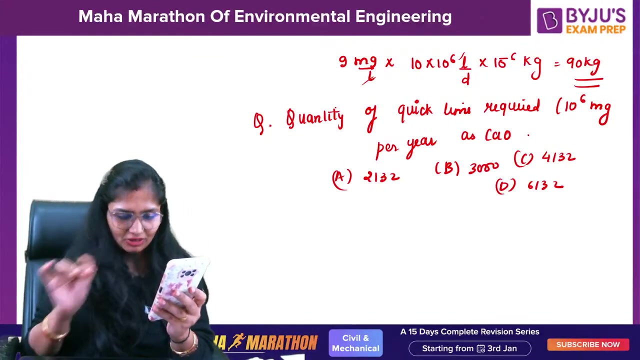 quantity of quick lime required. now, see, this is the second question: quantity of quick lime required. quantity of quick lime required. this is 10 days to power, 6 mg per year as calcium oxide to 1032 3000 for went through to India's respond from. so this is very simple. we have seen you out. the table is: 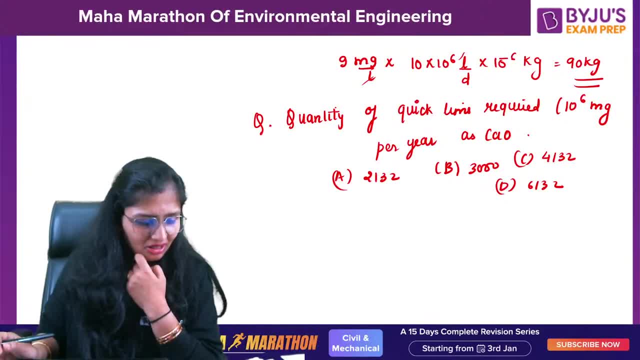 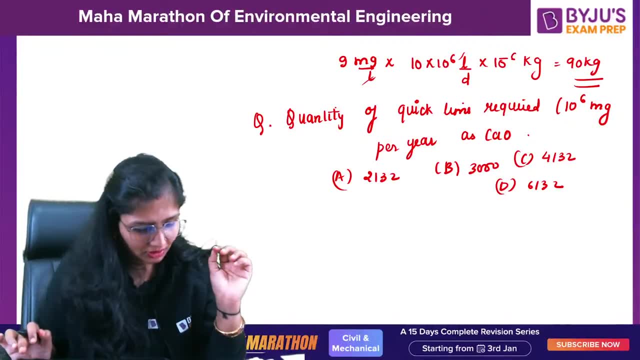 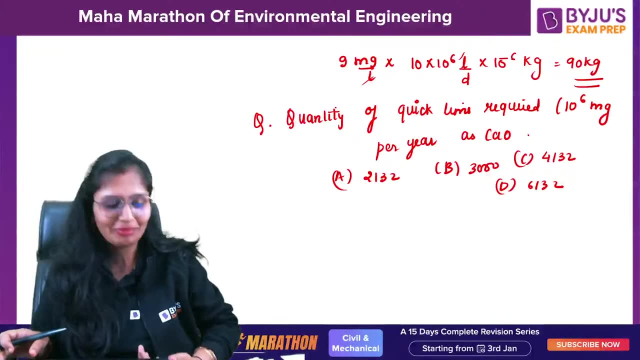 not learned by you which table you are talking about? beta? i'll check it out. melendra, i'll check it out, but good risk equation. you're saying no, actually you were not answering now. so up until morning i know you wished me, but after that you were not answering. 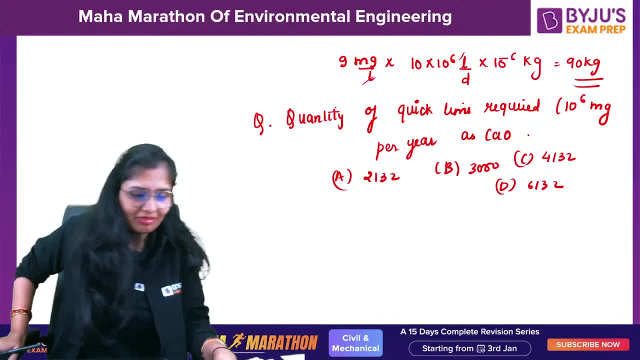 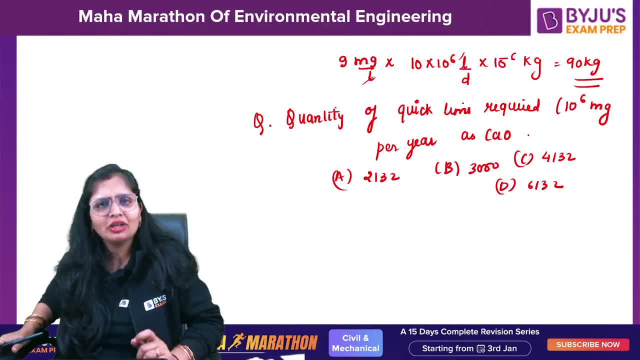 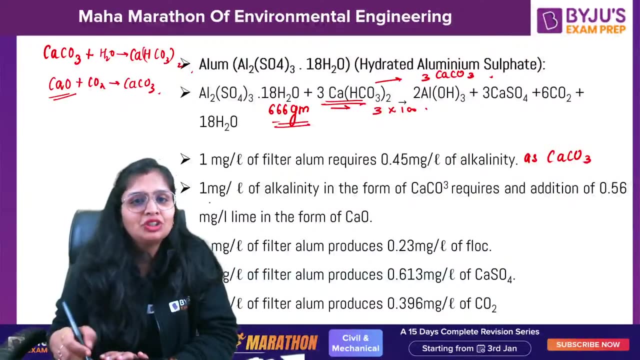 million. tell me that table, i'll see you which table. peak factor demand table: i already told you 1.8, 2.7. that table i told you now which peak factor table you want now see again. 1 mg per liter of alkalinity requires 0.456 mg per. 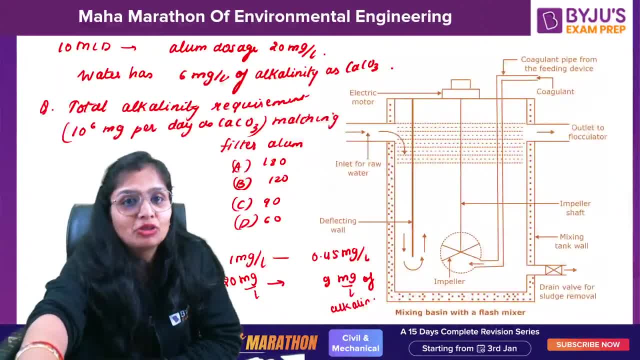 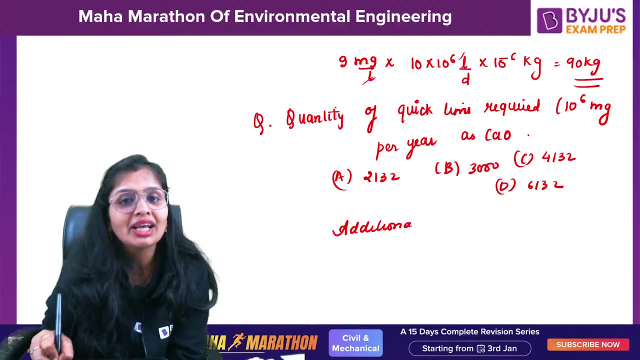 liter of lime in the form of calcium oxide. now see, you require 1 liter. 9 mg of alkalinity in the solution, already 6 mg. is there additional alkalinity? how much you require additional? you require 9 minus 6. that means for only 3 mg per liter of alkalinity as calcium carbonate you need. 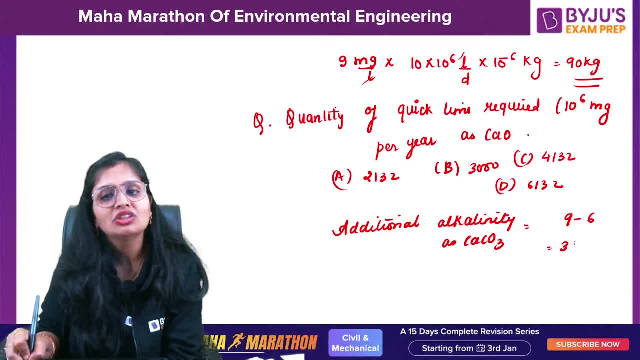 to add calcium dioxide. so this is 3 mg per liter. now for 1 mg per liter of alkalinity as calcium carbonate. you require- already mentioned is- just check it out guys- 0.56. so you require 0.56 mg per liter of calcium oxide. so for 3 mg per liter as calcium carbonate. how much calcium oxide is required: 0.56 into 3, 1.68 mg per liter of calcium oxide. so if for 1 liter, 1.68 mg of calcium oxide is required, for 10 into 10, raised to power, 6 liters, how much will be required? and it is needed for per year. 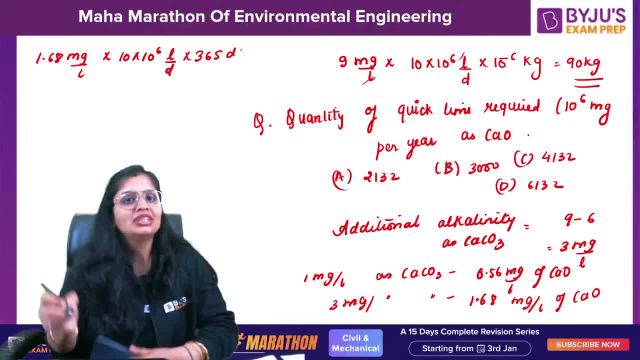 so per year is 365 days. how much it is coming 6132 into 10 raised to power, 6 milligrams. and it is already given. 10 raised to power 6 is gone, only 613. so see, quotient becomes so simple if you know the following bullet points. 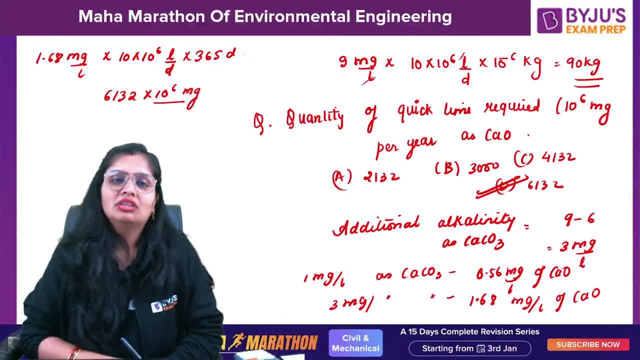 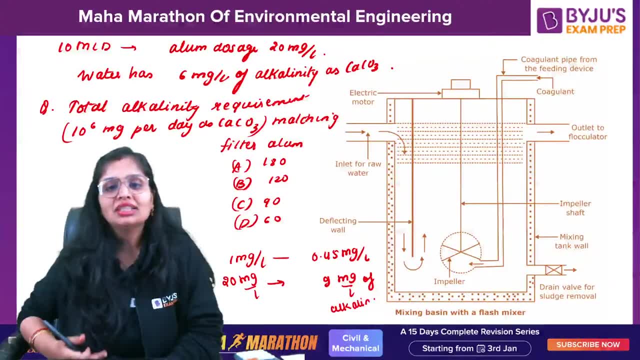 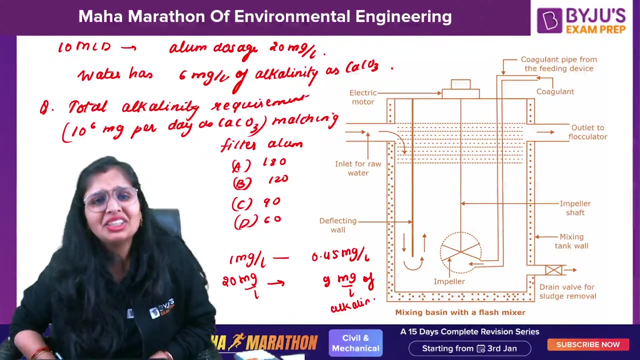 hope that are to as simple as that clear so such questions can be asked. so already told here. now coming to the next one, that is when you are mixing. see, mixing you can do it. no talking about. i asked about small meeting peak factor demand that population 1 up to two lacked up to. 50 000 000 to two lakhs greater than 2 lakhs. that population 1 up to 2 lakhs larger than 2 lakhs. as you can do in the same, you can do that more like in the same way than 1. 들어. 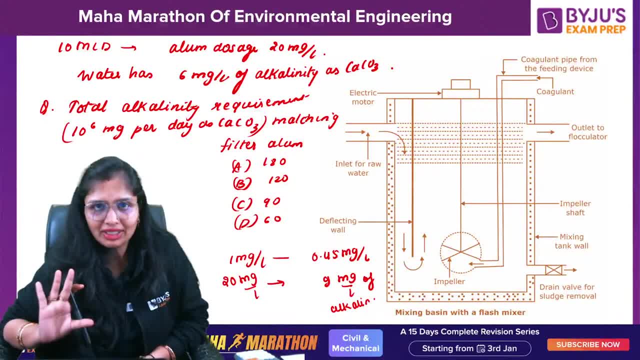 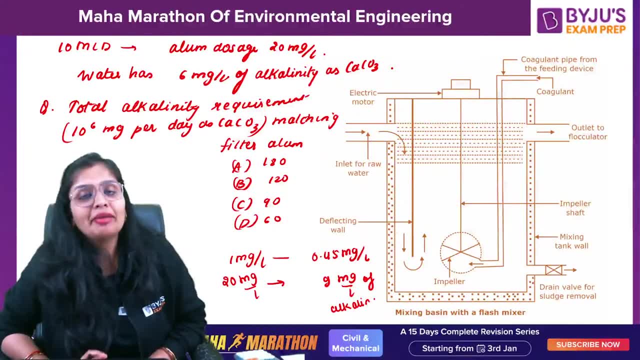 greater than two lakhs, that one you're talking about. i'll provide you at the last. okay, now, when you talk about coagulation, you want that the chemical should mix. so what you can do, you can, uh, basically do what you can provide baffle walls. when you provide baffle walls, what will? 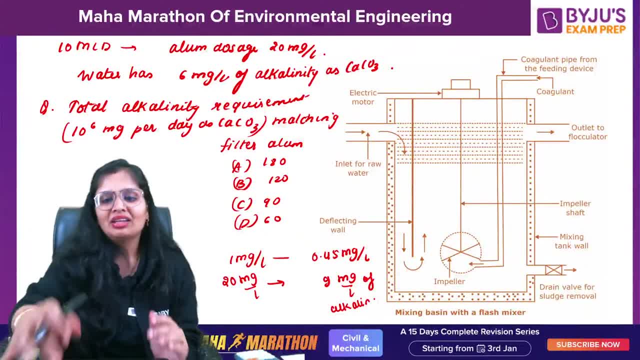 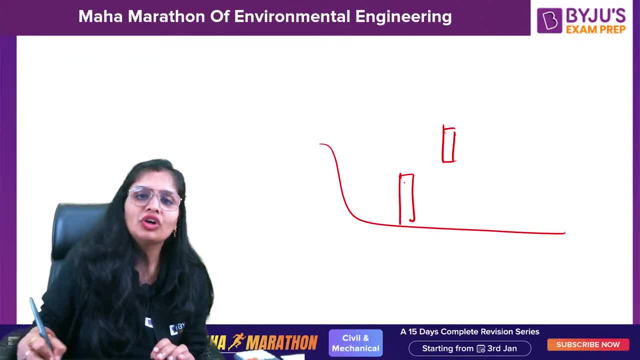 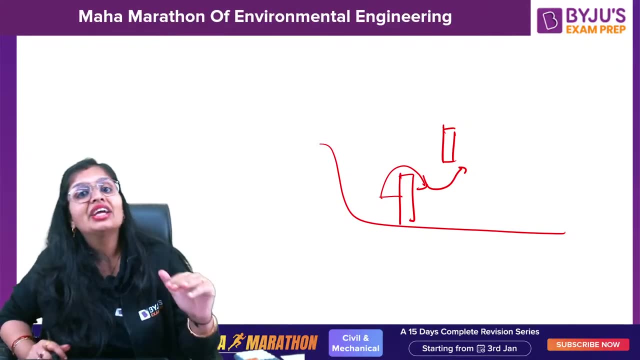 happen is the mixing will take place. okay, like, i'll provide a baffle wall and show you like here you have baffle walls, you have various baffle walls, so water will go, splash it here, go like this, splash it here, and so on. now, what happens here? now what happens here? here you don't get. 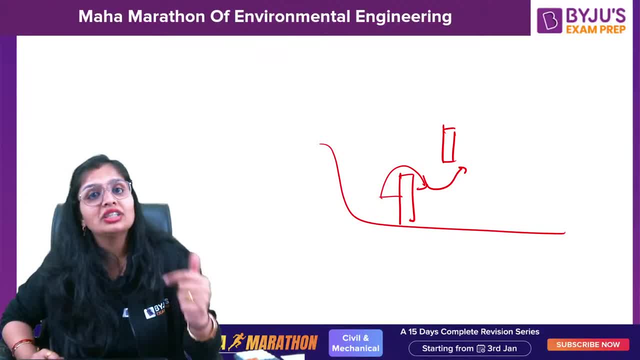 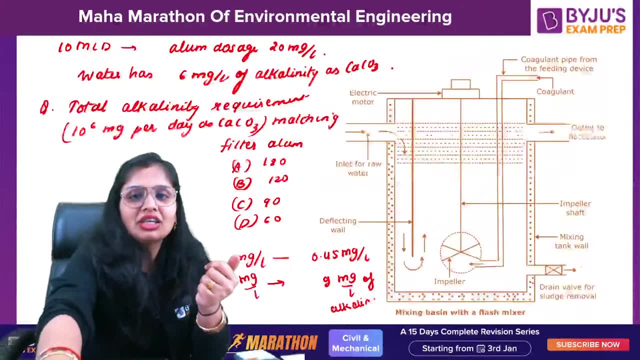 the desired efficiency. or you can say, mixing of coagulants does not take place 100 percent. that is the reason we go for flash mixer. what will happen here? paddles are there. you can see it here- impeller. and then these paddles are there. what will happen? you will feed the coagulant and 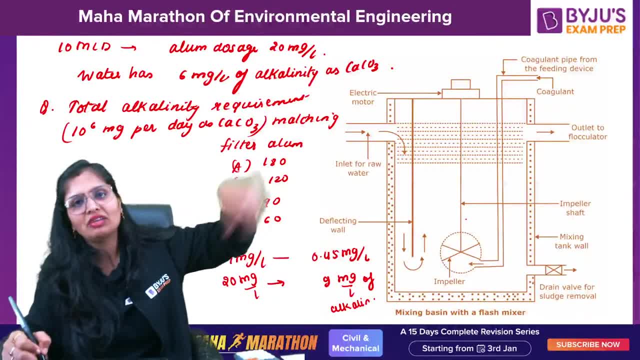 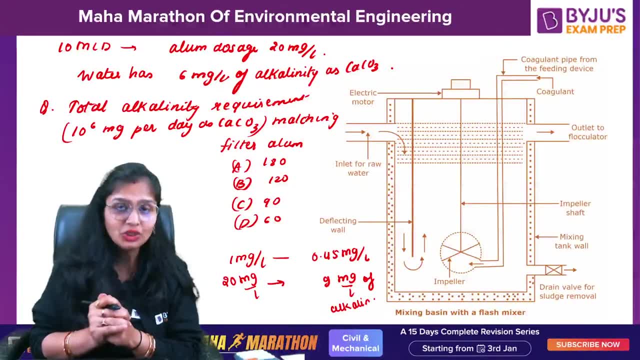 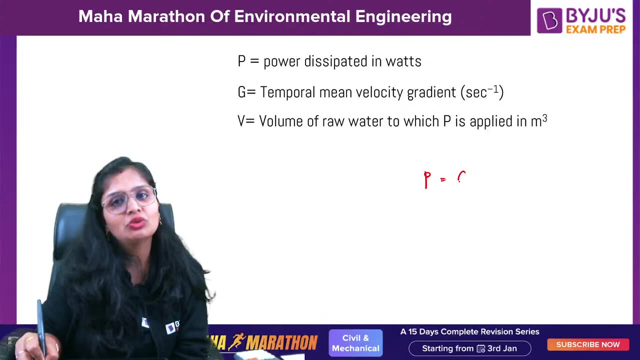 what will be happening is: motor is there, so it will rotate. the paddle will rotate fastly so that the rapid mixing of the chemical can take place. but for this you need to supply power. so how much power is to be supplied? that is given by the formula. p is equal to g squared mu- v. remember many students. 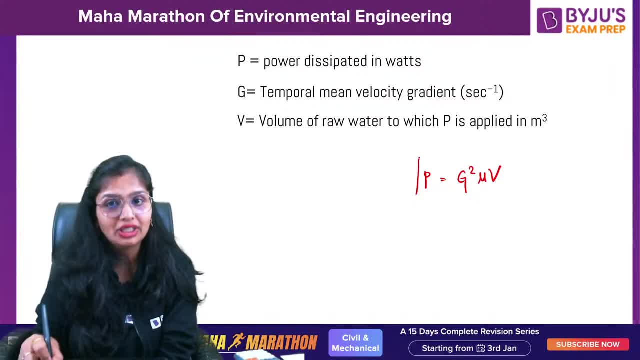 get confused: v is the volume here, it is not the velocity. first now, what is g? g is the temporal mean velocity gradient. okay, g is the. if this particle is there, there is another particle and both have the distance x. both the difference in the distance is x. it has the velocity v1. it. 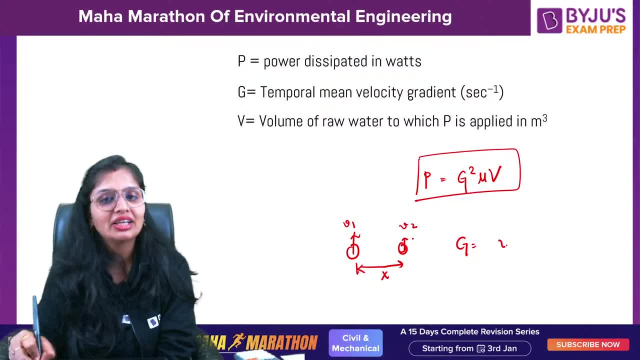 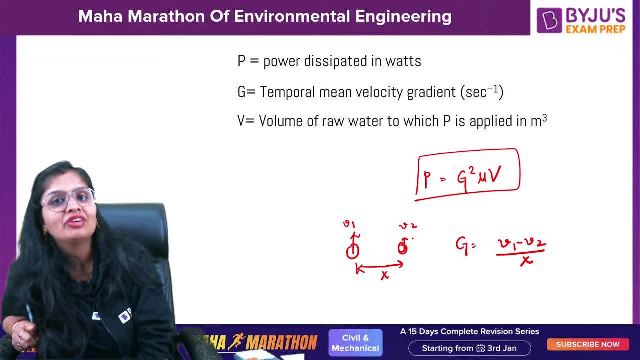 has the velocity v2. so temporal mean velocity is the relative velocity between the two divided by the distance between them. so this will give me the temporal mean velocity gradient. technically, this term g specifies me how much individual velocity is there. so this is the temporal mean velocity gradient. 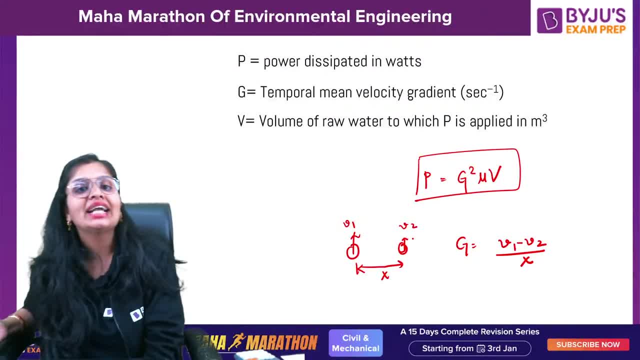 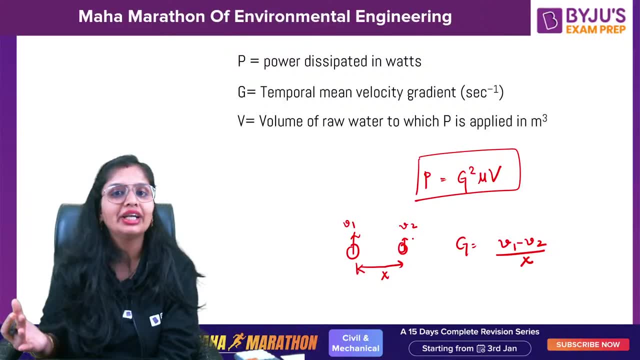 intensity of mixing is taking place. okay, that is specified by g, that is temporal mean velocity gradient. so you can use this formula for calculating what. even you can derive it. but derivation is not at all important. based on dimensional analysis, the formula comes. so p is equal to g squared mu v. this is the formula, simple. nothing else is required for this. 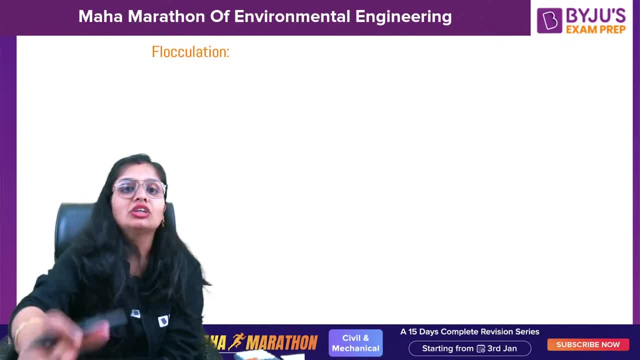 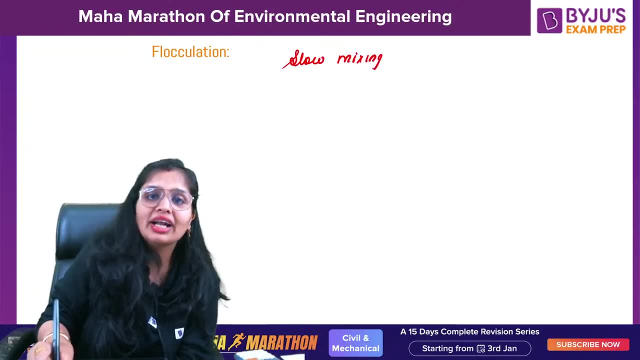 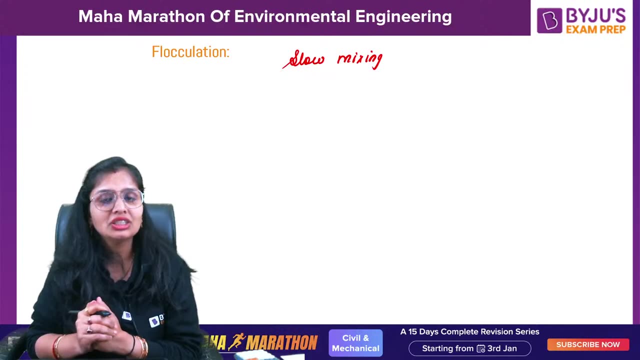 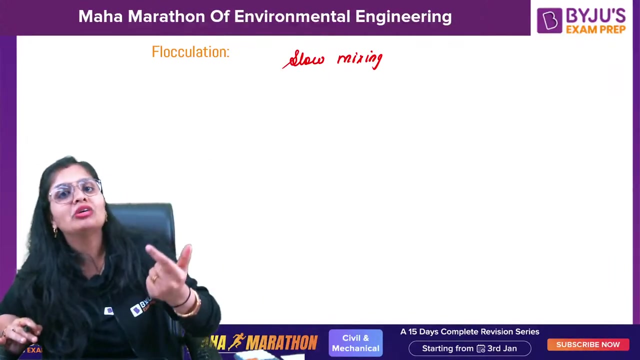 okay, now talking about flocculation. flocculation is slow mixing, slowly, gently, you are mixing so that what happens? so that all the destabilized particles comes in contact with each other. now for this, for this, if i talk about here also, same mixer is there, but the rpm, the rotation per minute, is reduced. why? because, even if you say ma'am, why flocculation? 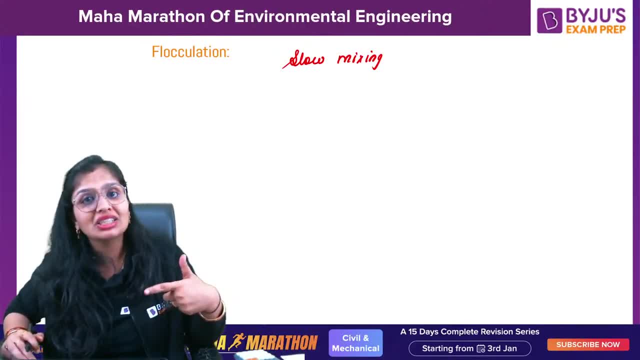 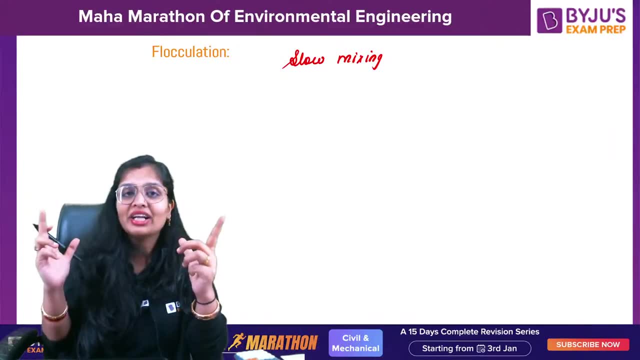 you don't provide fast mixing. if i provide fast mixing, then the destabilized particles will not come in contact with each other. so this is the formula for this. so this is the formula for this. that is the reason, because my funda is: i want that those destabilized particles should come in. 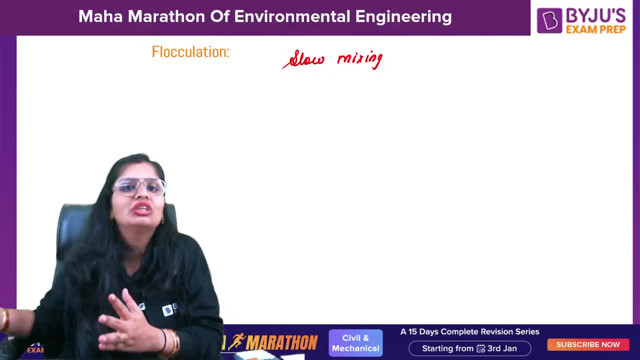 contact with each other, grow bigger in size and eventually settle. but if they don't come in contact because you're doing fast mixing, then there will be no use of flocculation. okay, so that is the reason. that is the reason. in flocculation we go for slow mixing and uh. 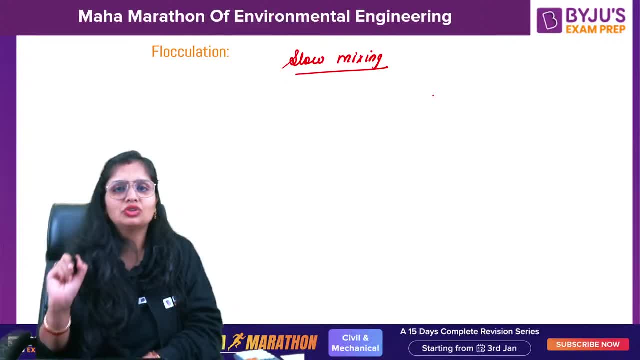 there was- huh, this was the thing which you should know- any doubts. also, this is a short poll for coverage. you should go for that drop down at the end of the then just come back if you want to see how fast inside it can go, and little bit more. 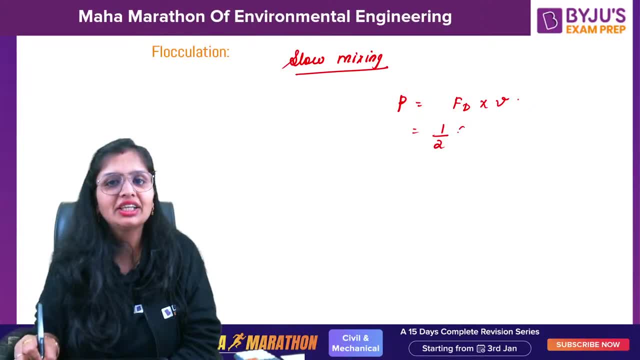 okaproxy several times. this is the formula for it, because we are just curious about all the formulas for this, this formula, mind you, the formula isoning form. and one more formula for power. power is this formula. you remember? there is one formula, half C, D, row W, a, we are. 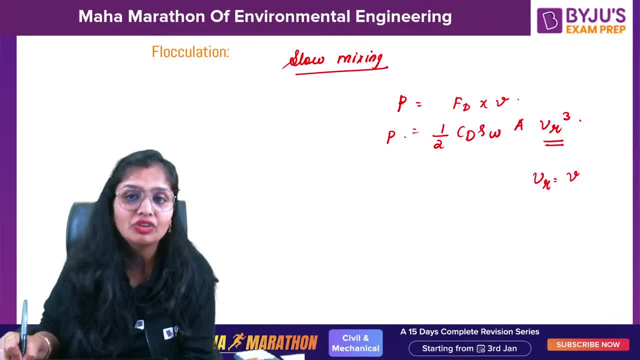 this. this will become. we are. keep you women. this formula, guys. this is the formula for velocity of pedal minus velocity of water. Technically they take velocity of water as zero. So in books you find it. they write it as like half cd. rho w a v p. 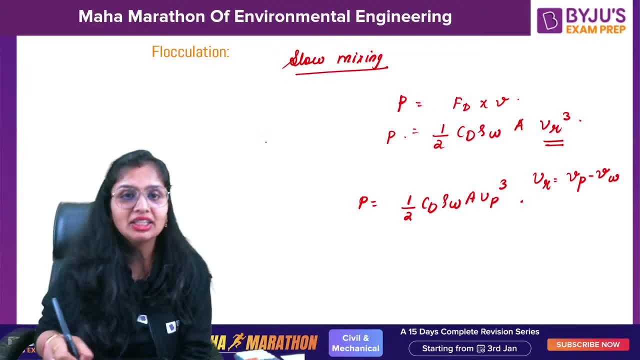 Okay, a is the total area of pedal. Let us suppose if the width and length of pedal is given, you have to multiply with the number of pedals to get the total area of pedal. Okay, So this is the thing which you should know. If they ask you, you should be able to answer. 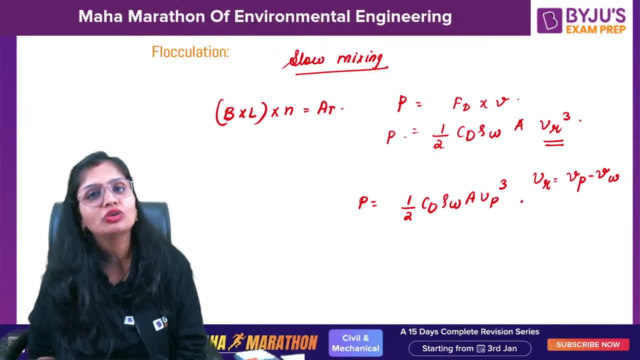 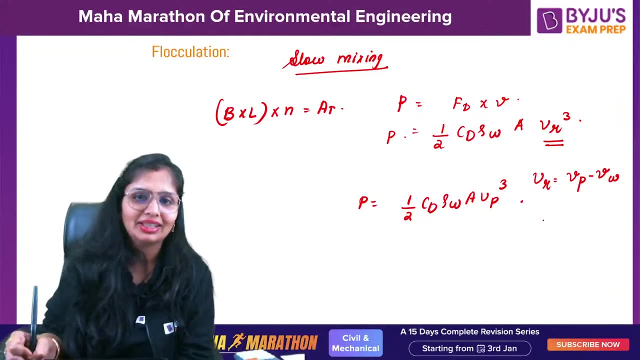 As simple as that. Okay, And power, you already know g square, mu, v In place of volume. they can give you discharge into detention time. You can do. It is given in triangle lift. It is given in environment also. Formula is of drag force, but it is given in this also, Okay So, 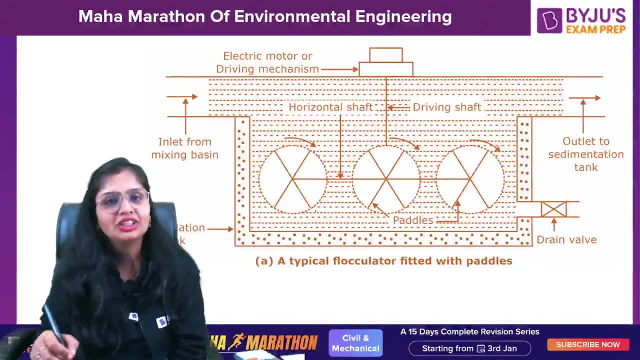 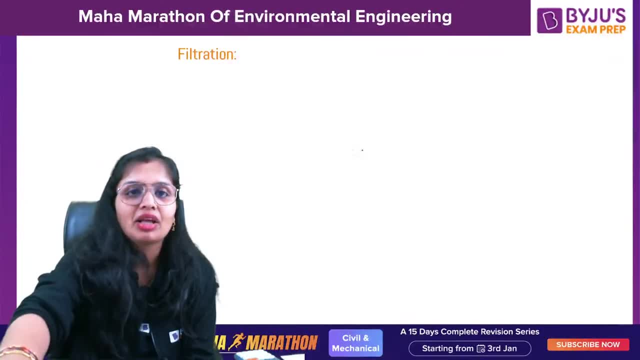 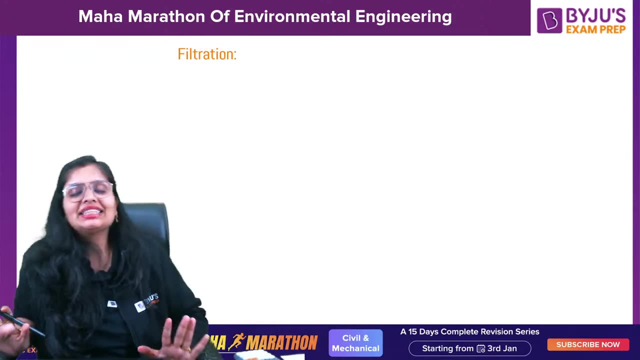 you should know. Okay, So this is the flocculation. You can see same like that, but pedals are here, also there, but slow mixing is induced. That is it Now talking about filtration. Filtration is in itself a complete treatment unit. Why? Because it will remove fine suspended 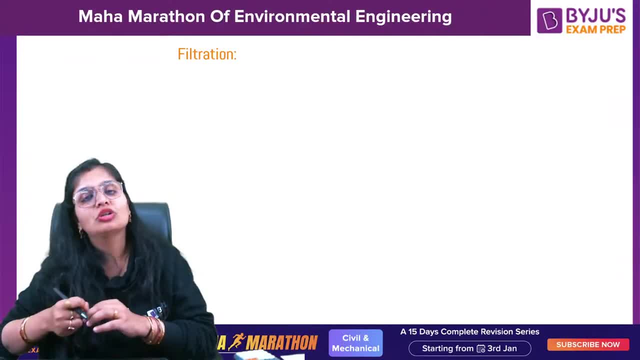 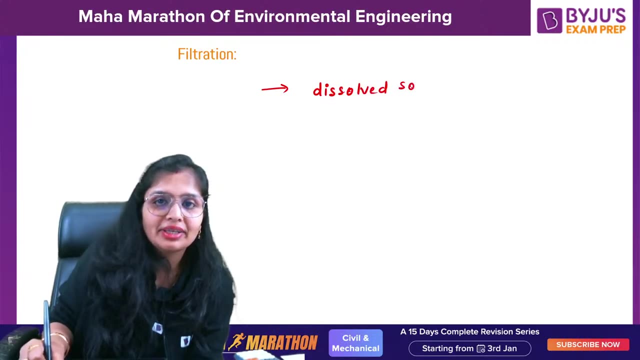 solids also. It will remove microorganisms also. It will remove any sort of foreign impurities also. It will remove dissolved solids also. So it removes everything. It removes dissolved solids. It removes dissolved solids are there? Then you have what. 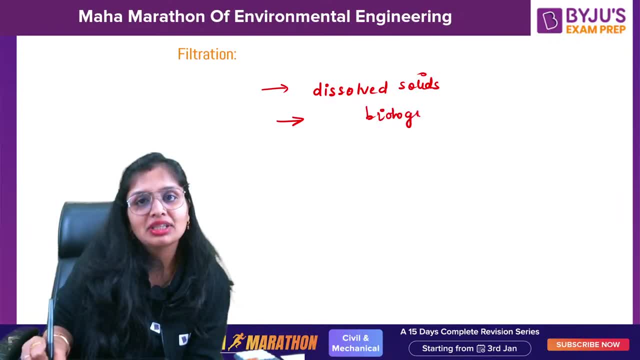 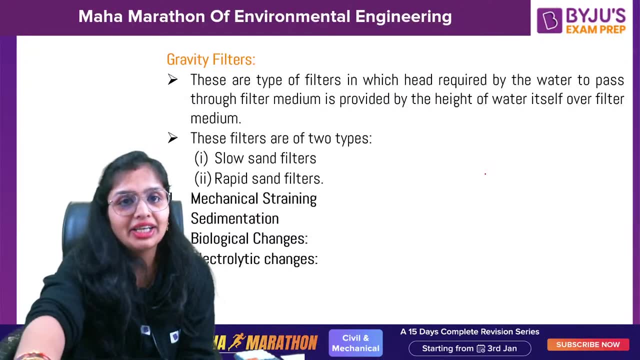 Biological or you can say any microorganisms are there, It will be removed. That also can be removed. Now, when you talk about filtration, we do the process of filtration by the units known as filter. Now, filters, we have generally two types: One is gravity filters, another one is pressure filter. 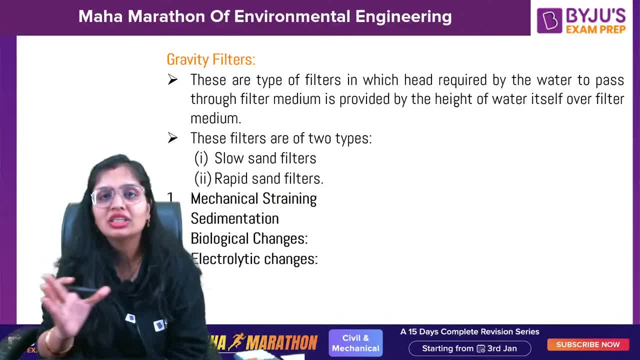 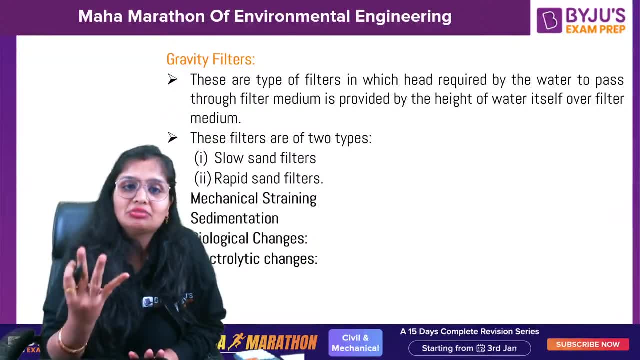 Gravity filters. we have again two types: slow sand filters, rapid sand filters. Now, first we will understand how this filtration will take place. There are four mechanisms: mechanical straining, sedimentation, biological changes, electrolytic changes In mechanical straining. what happens? 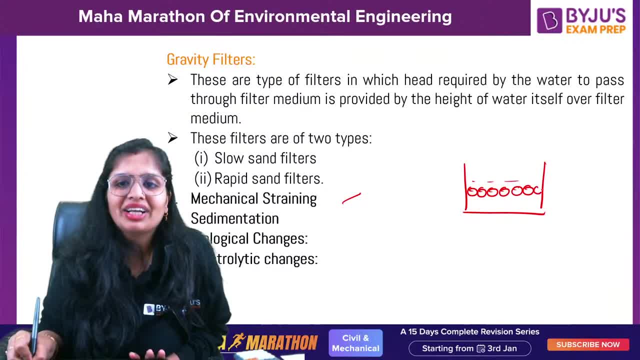 This filter bed is there. You can take sand, you can take anthracite, you can take geotextile- anything you can want, you can take it. I am making the size of the particle bigger so that you can see this. Now, when the water comes in this mechanical straining. 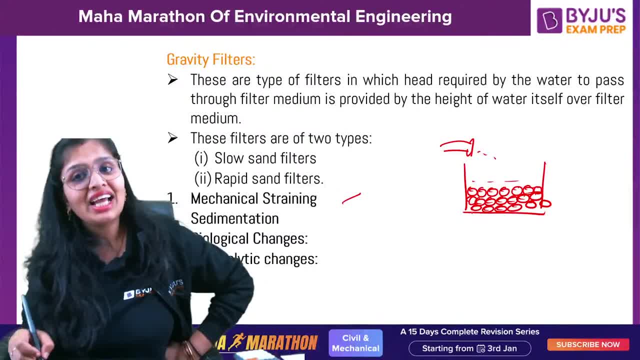 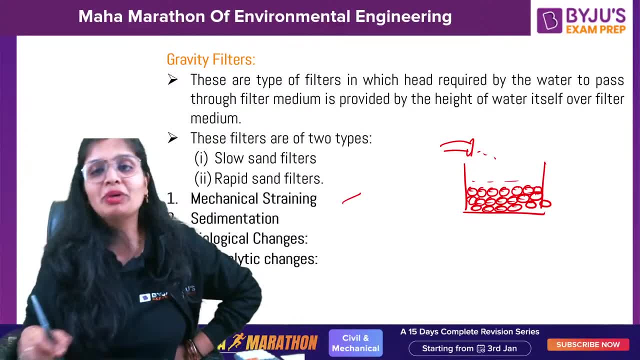 what you will see, the particles which have a size greater than the size of the sand particles. they will not be able to pass through it. They won't be able to pass through it and they will retain here Eventually even the size of the particle which is smaller than the size of the sand particles. 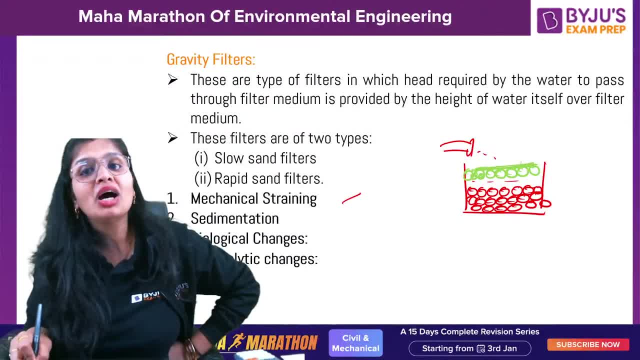 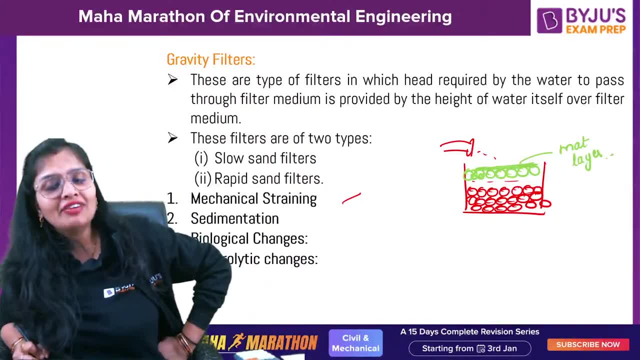 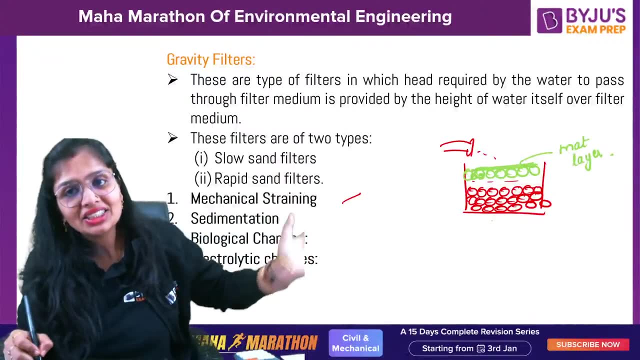 will also be retained at the top and they will form a layer which is known as mad layer. Now what will happen The moment they get deposited on the tower? what you can do? You can strain it out. You can mechanically strain these impurities out. 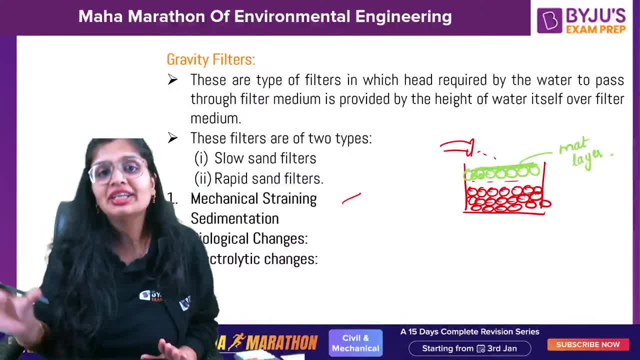 So the manner in which these suspended solids are removed, the process is known as mechanical straining. Okay, Now, next we talk about sedimentation. When you go by the process, sedimentation generally- this is happening in the filtration chamber, So generally I will take it as red color only. 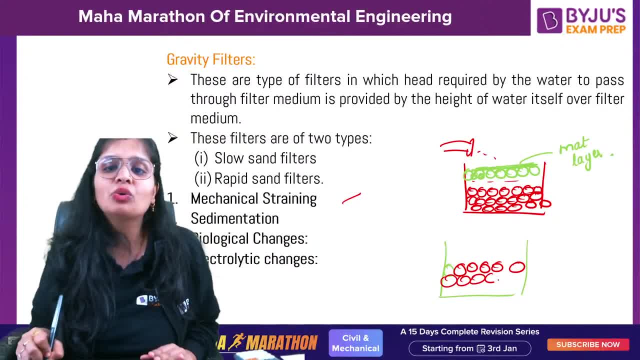 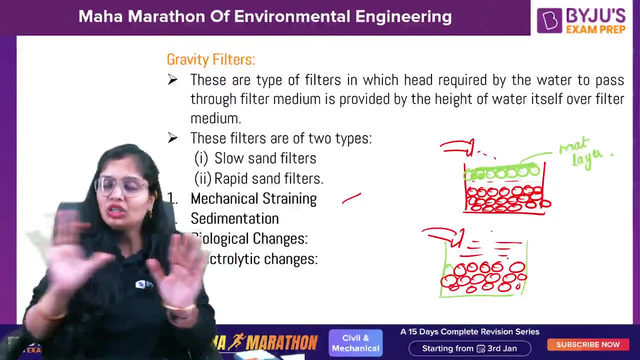 So these are the sand particles. It behaves like a quiescent type tank because the filter is not at all moving. You are bringing The water here, the water is accommodated, So the water is at rest, Specific gravity will come into action. 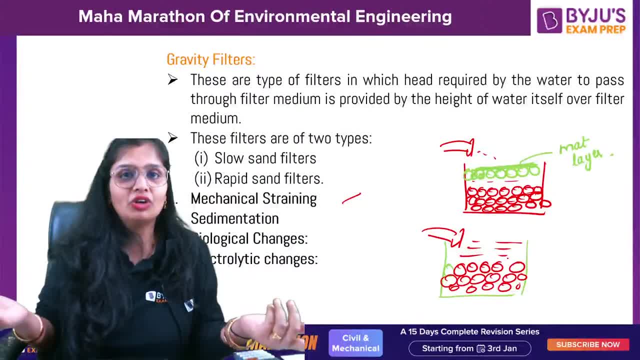 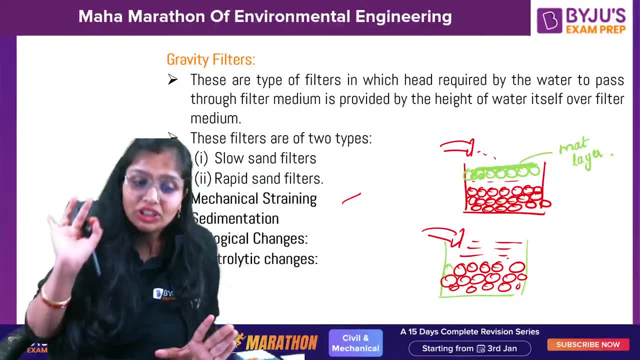 Those particles which have a density more than the water, it will get settled So it behaves like quiescent type tank. Now biological changes. Biological changes gives you higher efficiency, but it takes time. It is not a one day that it will happen. It takes time. 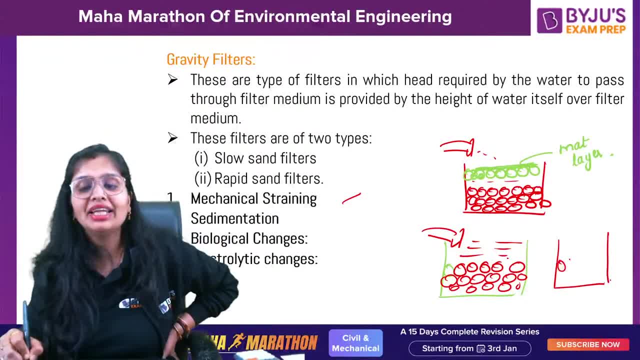 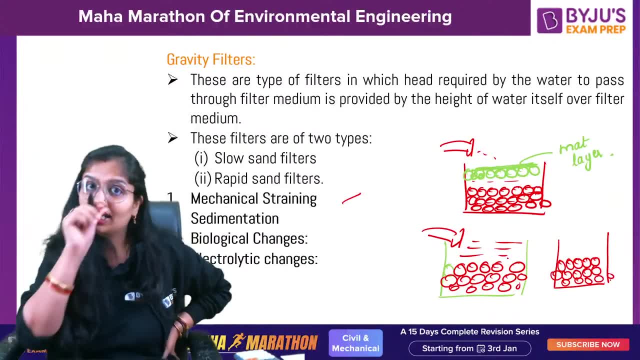 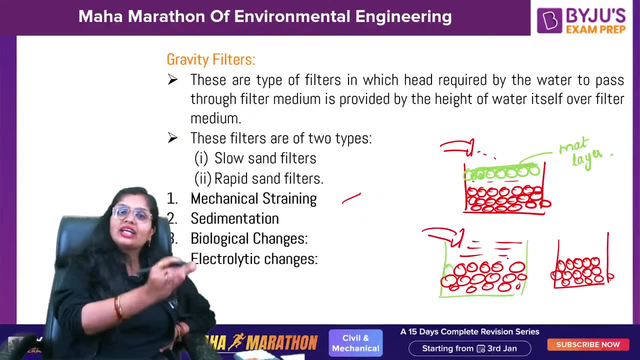 So what happens in biological changes? initially, Initially, when the water comes, It has microorganisms in it, It has organic matter in it. Technically, the microorganisms are there and they are not completely removed. The organic matter is partly decomposed. Right now, the organic matter is still. 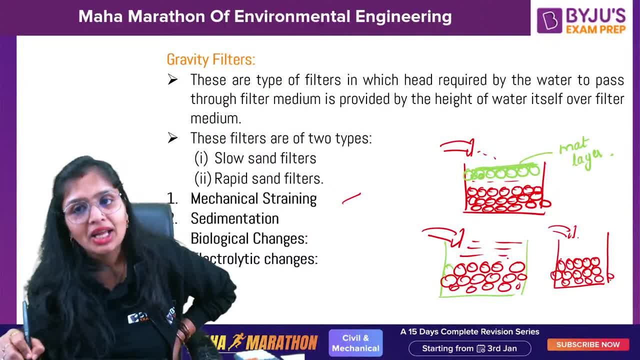 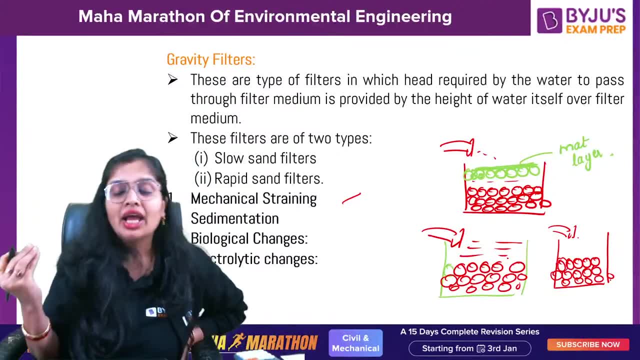 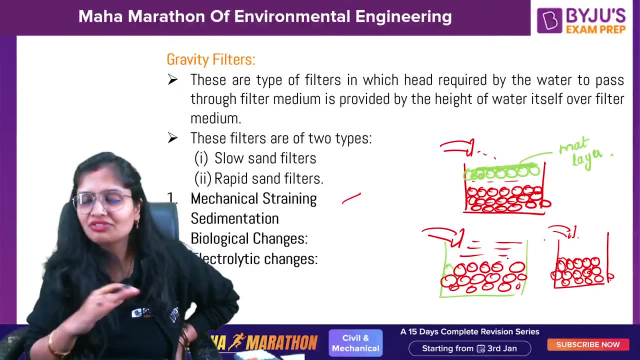 So what will happen is, when you pour this water, the microorganisms decompose the organic matter and they form a sticky deposit. Now, here, algae will also be coming into action. Now, algae will be there. This tank, this filtration tank, is open to the atmosphere. 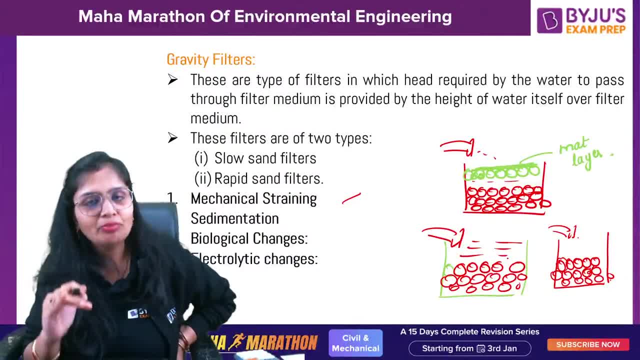 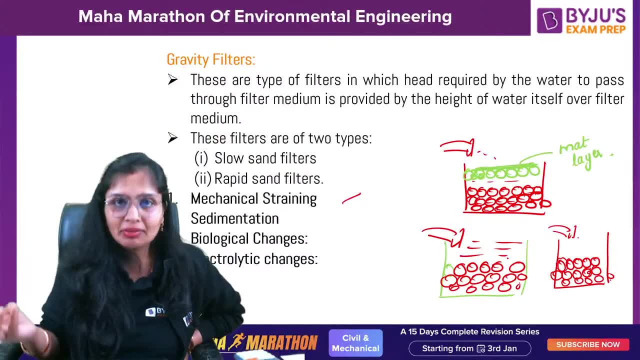 So what will happen? Algae will get sunlight with the help of sunlight. What will happen? And if you'll ask me how algae will grow? because in this water, organic matter is there and the general formula for organic matter is Ca, Hb, Oc, Nd, Ac, Pf. 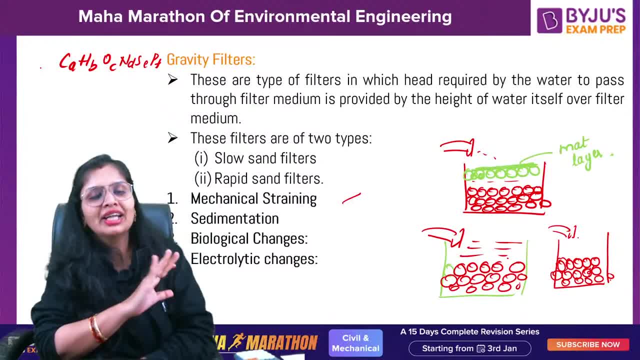 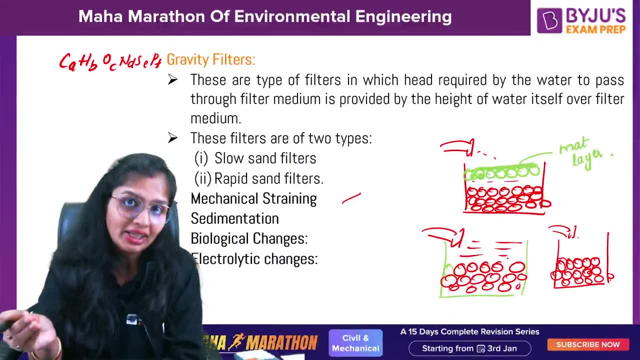 A, moles of carbon, B, moles of hydrogen, and so on. It's not necessary that every element has to be there, but this is the general formula. These carbon Hydrogen is the nutrient for algae. If such conditions are there, algae generation will take place. 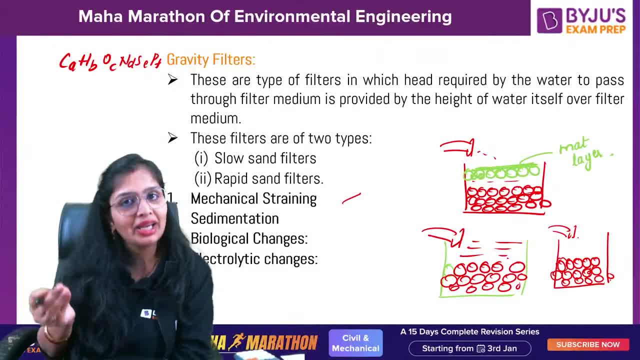 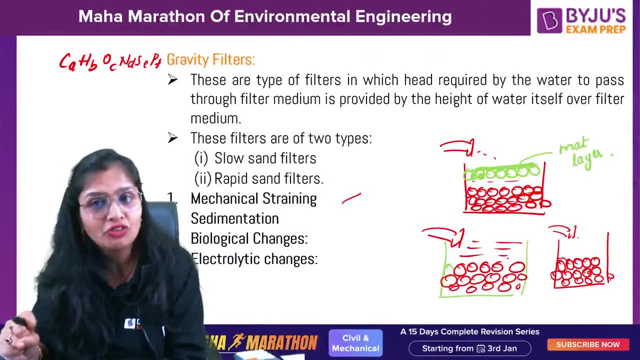 Algae on the action of photosynthesis will prepare it food. It will liberate oxygen. That oxygen will be used by microorganisms for decomposition of organic matter. Over the time, what will be happening? Microorganisms will be decomposing the organic matter and the layer will be formed which is known as smut stick layer. 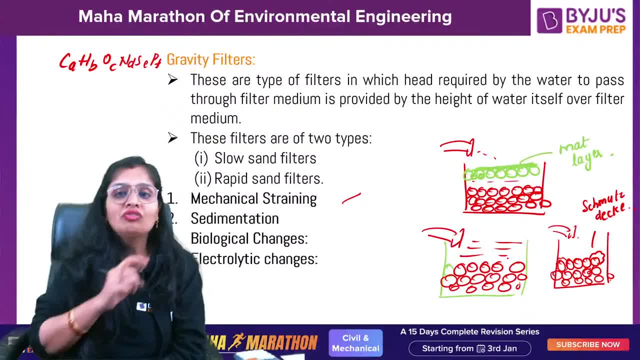 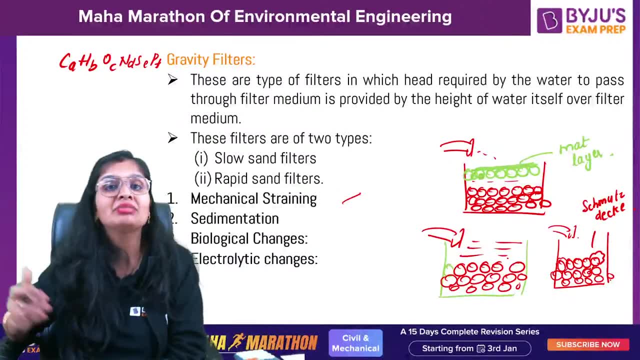 Now what will be happening? Decomposition is happening over the time. Microorganisms have rapid reproduction rate means they multiply themselves exponentially through cell division: 2 to 4,, 4 to 8 and so on. So what will happen? The microorganisms will increase. 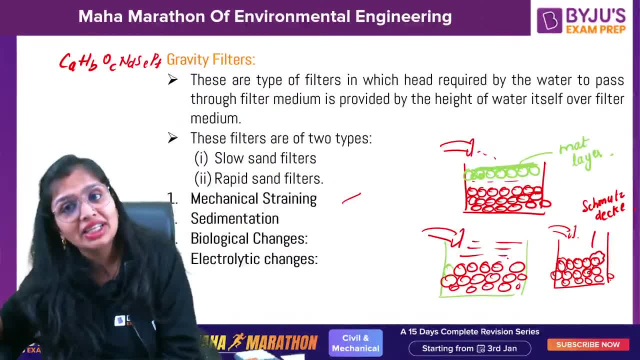 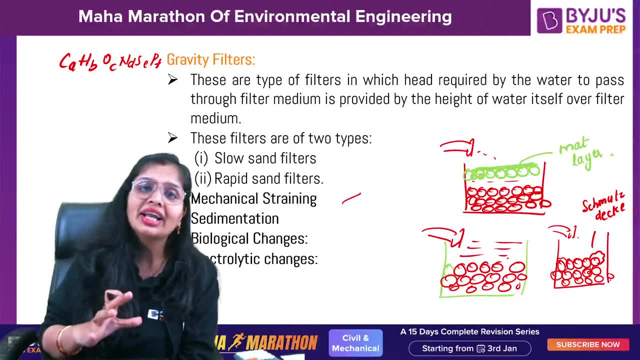 The organic matter remains the same. Those microorganisms which are getting food? Okay. those who are not getting food? They will go endogenous respiration. That means they will kill themselves on their own, Okay. So what will happen? The microorganisms will increase. 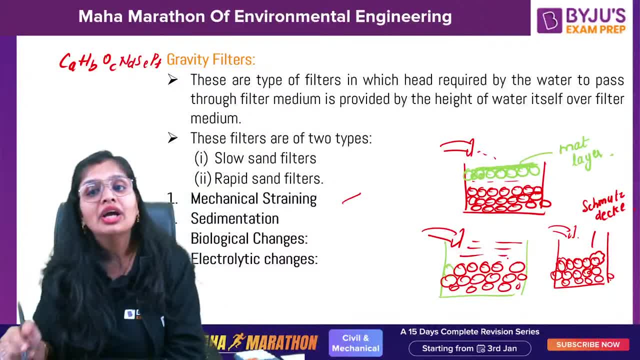 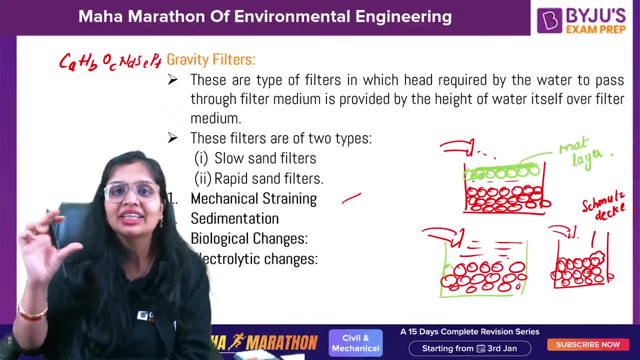 The organic matter remains the same, They will kill themselves on their own. Okay, So what you will see here here, in this layer, there will be what large smut stick layer will be there, The thickness of this layer will go on increasing and the water which will come out. 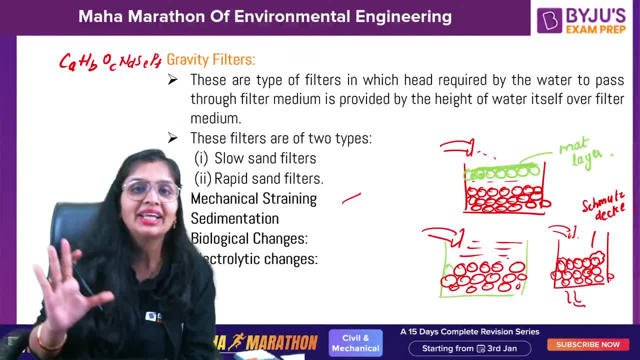 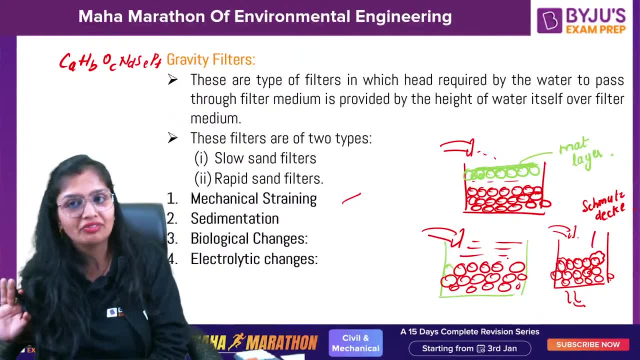 It will have- almost, if you go for slow sand filter- 98 to 99% of bacterial removal efficiency. you will get Okay If you are using slow sand filters. So, because of the development of smut stick layer, Let me tell you: 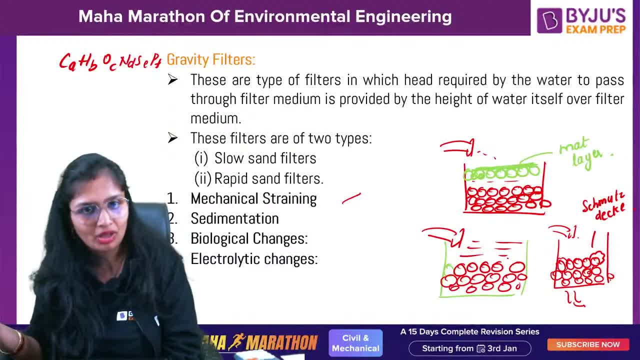 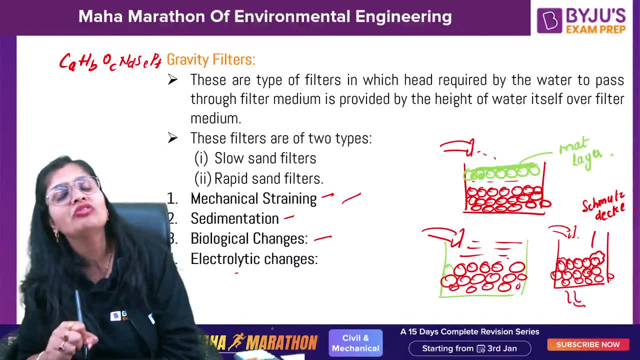 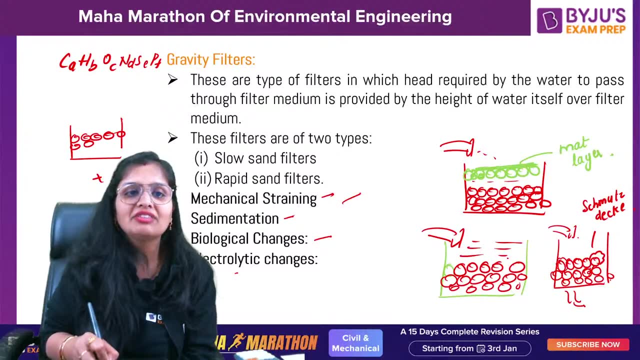 It is developed like in an hour and all. It takes time, Okay, Last. So here you remove pathogens, Here you remove suspended solids. Now, how to remove dissolved solids? What happens? These beds are charged. Okay, They might be having positive charge, negative charge. 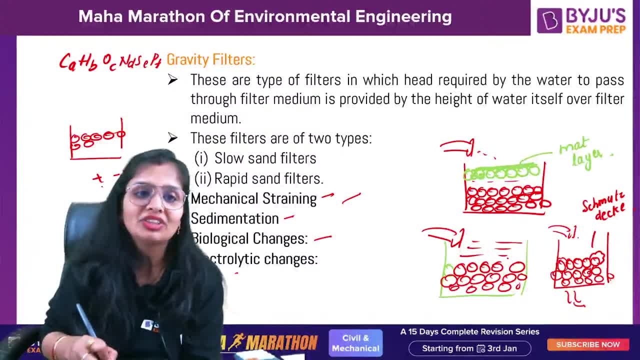 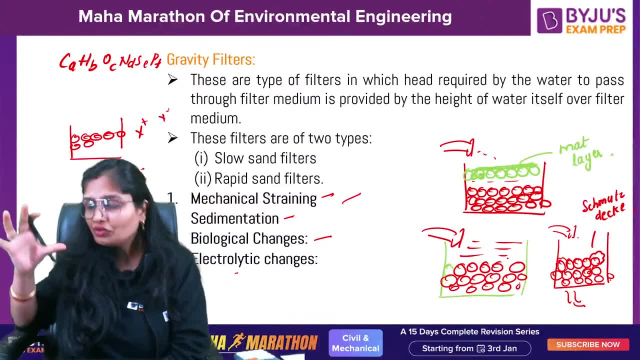 The dissolved solids which are coming. They might let us suppose if this is A and this is B- The dissolved solids which are coming- They also have charge, Positive charge and negative charge. So when the water which has dissolved solids and solids and in ionic form is there, 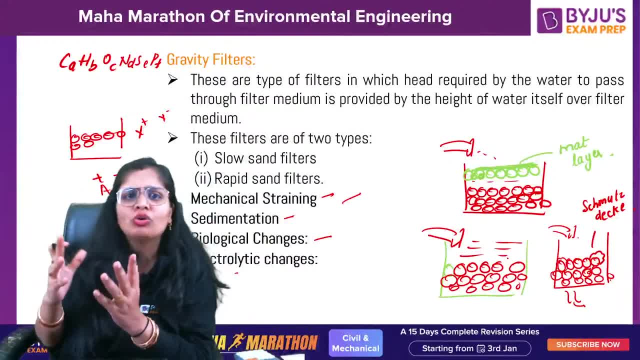 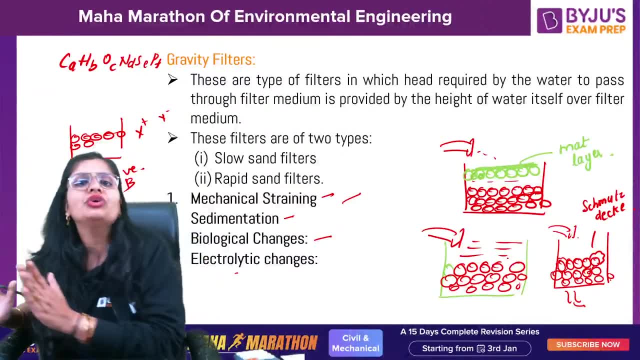 They pass through this filter bed. You do not know They react with each other. How much they react you would never come to know. But at the end, whatsoever water you get, you will see that the dissolved solids amount is very less Okay. 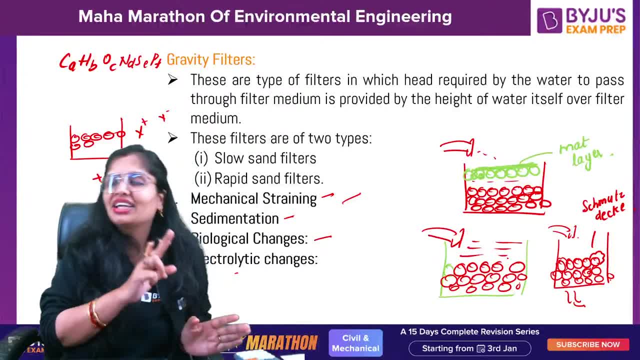 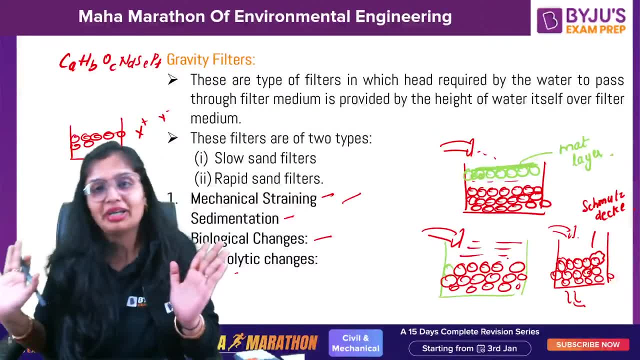 So, based on electrolytic changes, and if you think, first mechanical straining will take place, then sedimentation, No, All the things are taking place simultaneously. Okay, All the things are taking place simultaneously. So this is the theory of filtration which I told you. 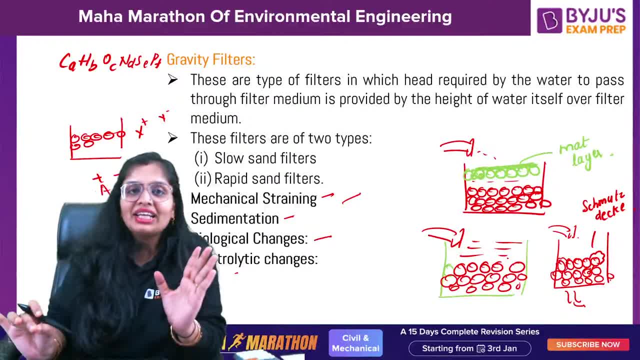 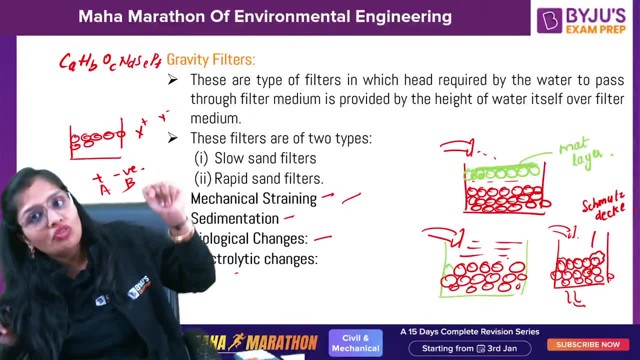 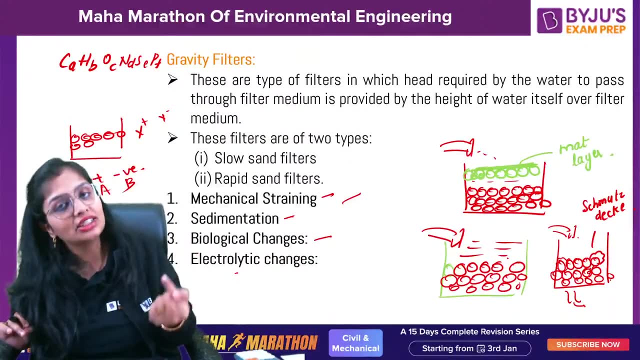 Gravity filters is important. Gravity name is given because see whenever water will pass through the sand, it will offer resistance. So to overcome the resistance whatsoever, energy is required that is provided by the water itself. So that is the reason it is known as gravity filters. 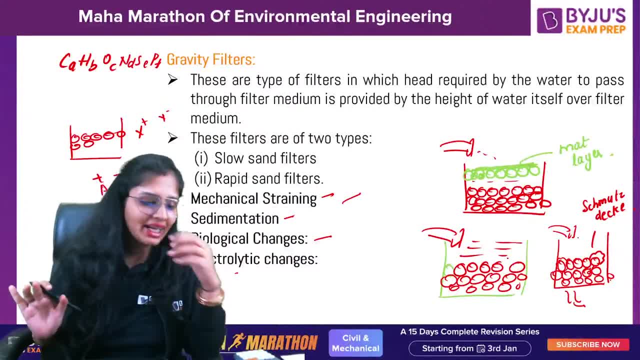 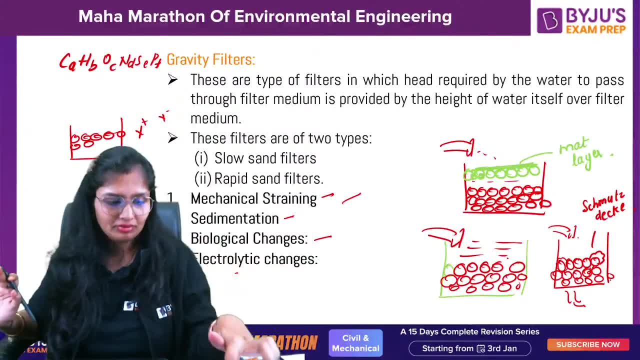 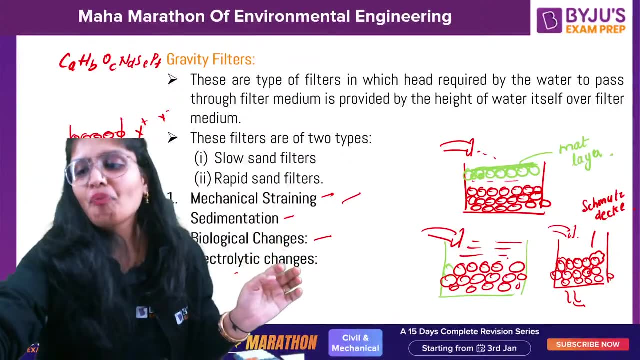 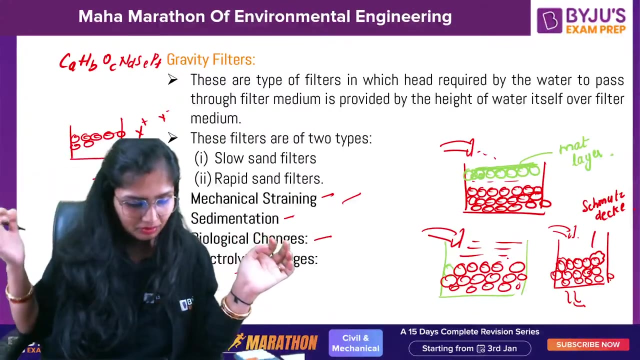 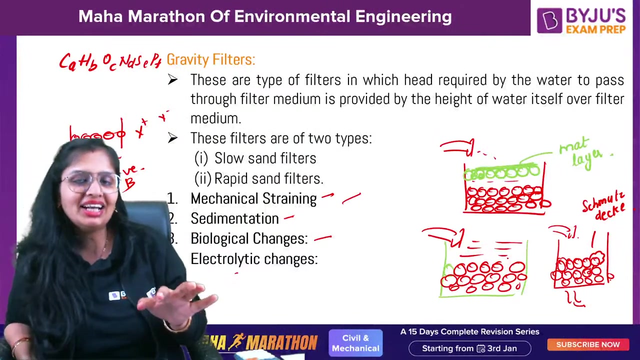 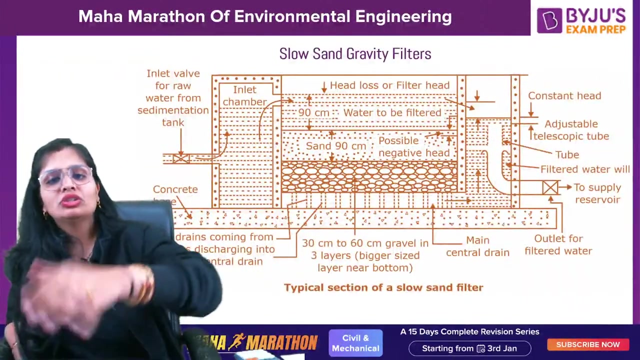 Any doubt till here, Guys, any doubt you have till here? let me know fast Any doubts you have have. Generally for idle it takes weeks, But for rapid sand filter we can't wait for that much amount of time. Okay, Now talking about the slow sand gravity filters. let's be quick. 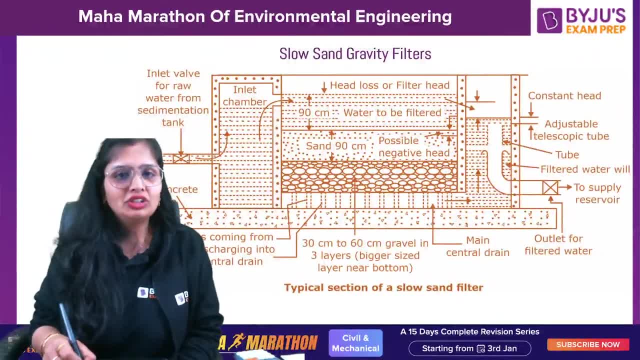 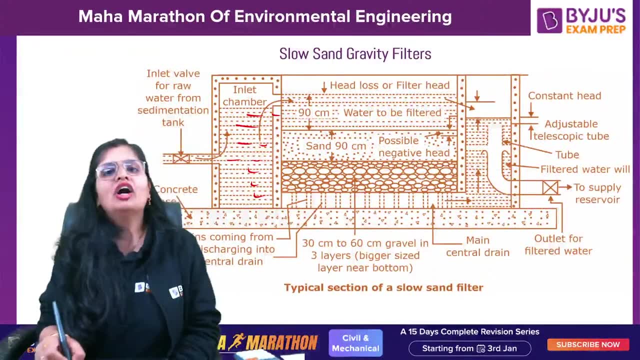 This is very simple. This is an inlet chamber which we have provided. This is an inlet chamber where water is accommodated. Now, what you will do is- I'll take a blue color. Now, how much is the depth of the water? Remember how much is the depth of water? How much is the depth of sand? 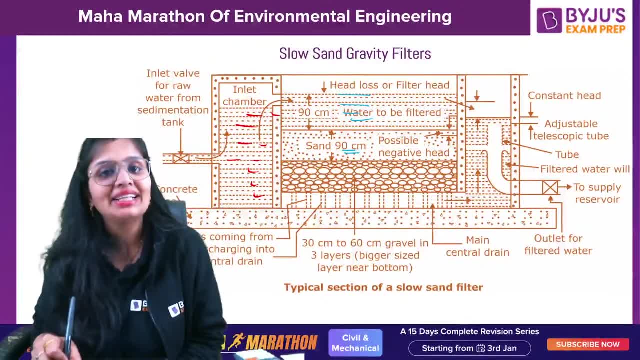 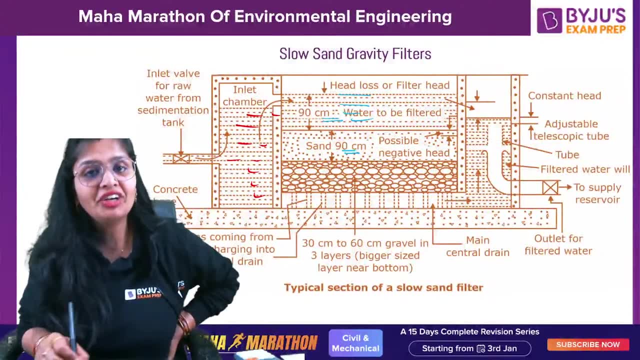 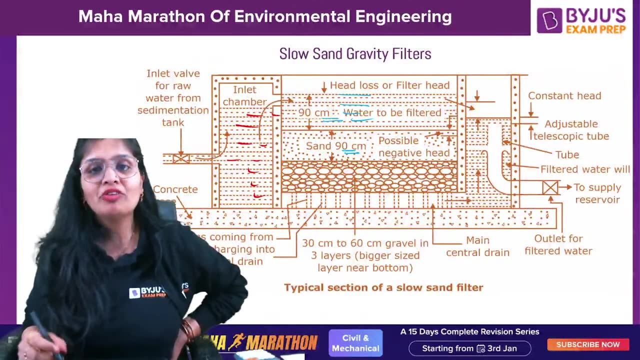 That much depth of water should be there Always. Here the sand depth is 90 centimeter. Here the water depth is also 90 centimeter. Finer quality of sand is provided at 15 to 30 centimeter of the sand out of 90 centimeter is a finer quality. Okay, Next gravel is provided to support. 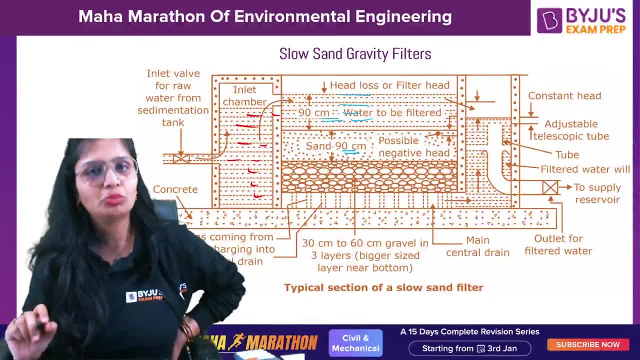 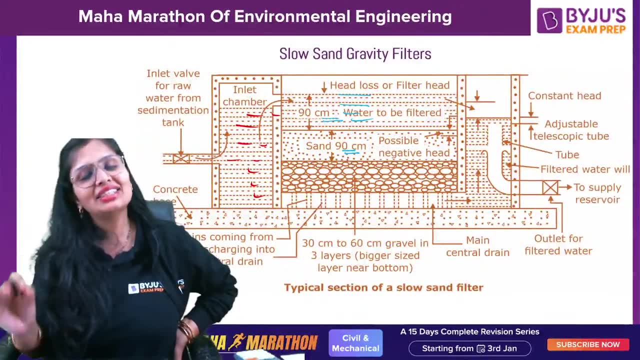 the sand. It has no other function. It has function is only to support the sand. Now what will happen here When the water will get poured? obviously, the resistance will be offered. That resistance will be uncounted by the water itself. Same mechanical straining, sedimentation, all will. 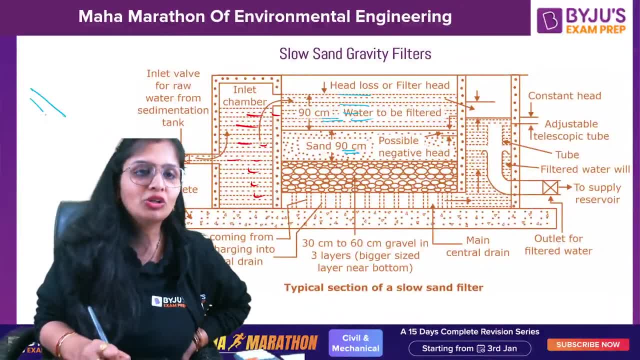 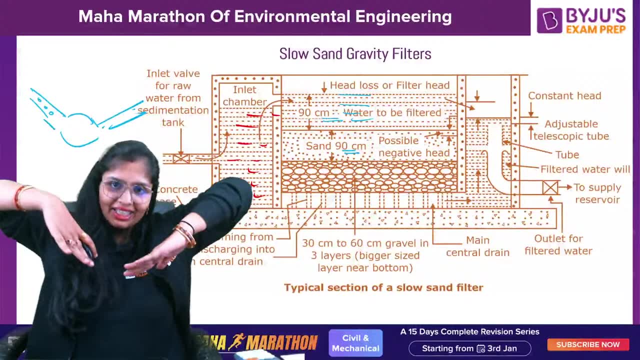 take place. After that. there are lateral drains. These are the small. small lateral drains are there and this water goes into the bigger one that is main drain. So on both the sides. technically it is like this, because you are seeing a section of it, you can't see it. So these are the number of under drains. 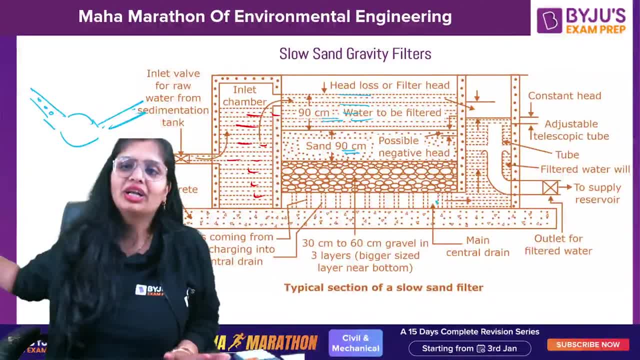 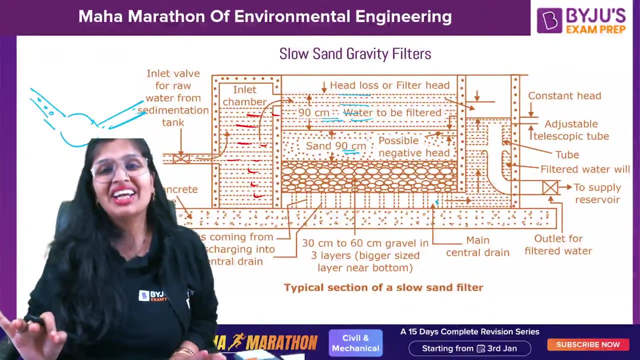 lateral drains. From here, water goes into the main drains, where you can take it to filter it, disinfect it or directly supply it. Okay, This low sand filter. the major drawback is it requires water. That's why it's not possible to use it. Moreover, the rate of filtration is also very slow. 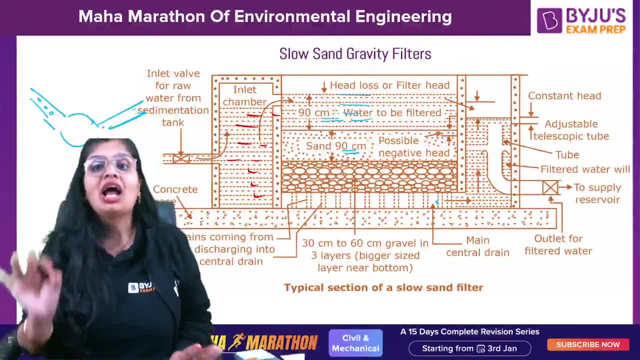 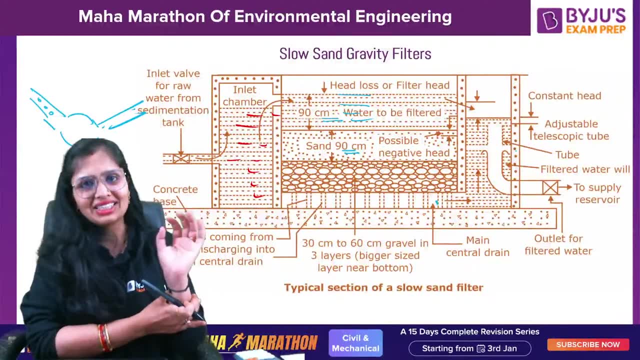 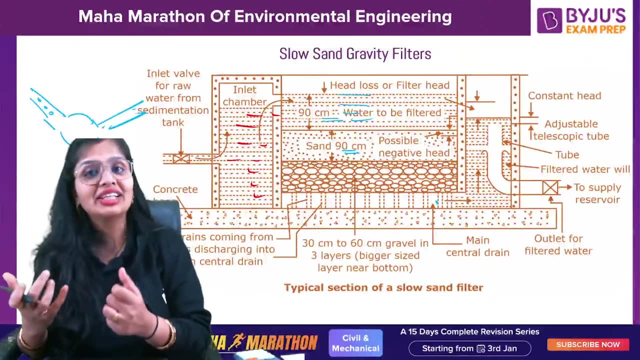 So that is the reason you cannot use it for urban population. You can ask me what is the function of this adjustable telescopic tube? See, initially the head loss is very less, Even 10 to 15 centimeter. Eventually the head loss increases. If the head loss will increase, it will affect the discharge. 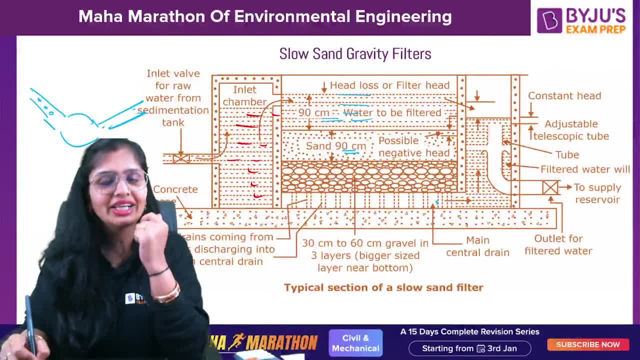 So this tube, you can adjust it in such a manner, You can see it, so that you get a constant amount of water. So you can adjust it in such a manner, You can see it, so that you get a constant amount of water. 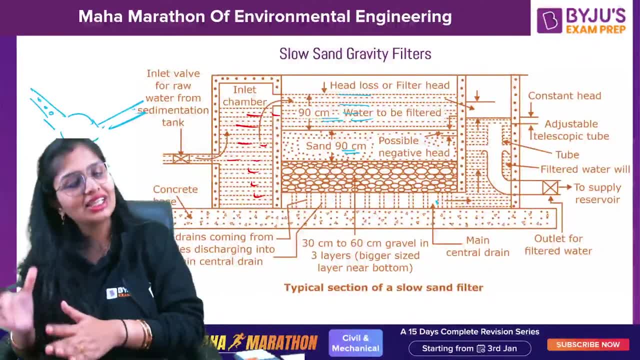 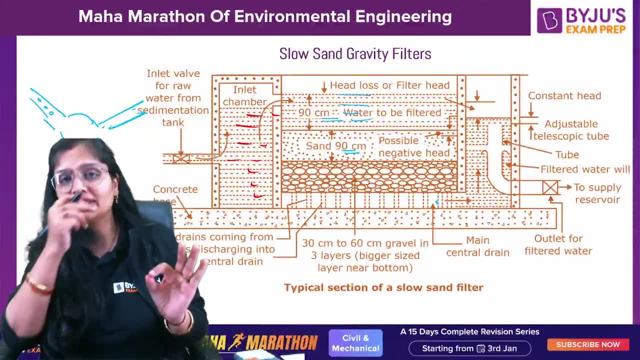 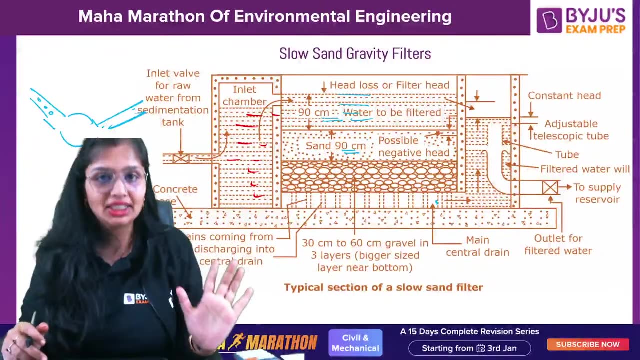 So, for getting the constant amount of discharge, irrespective of the head loss, you have this adjustable telescopic tube. Okay, The moment you see that the head loss is 0.7 to 0.8 times the depth of the sand, you need to clean this. Okay, Generally in 1 to 3 months you clean. 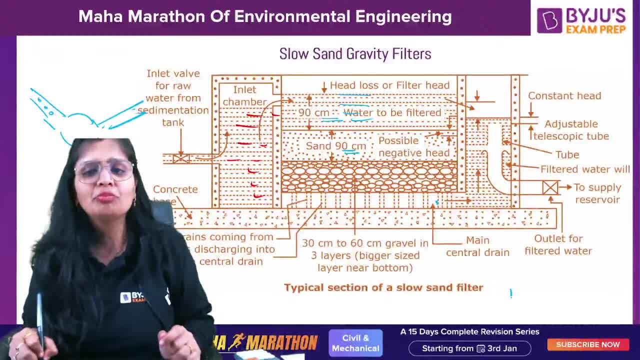 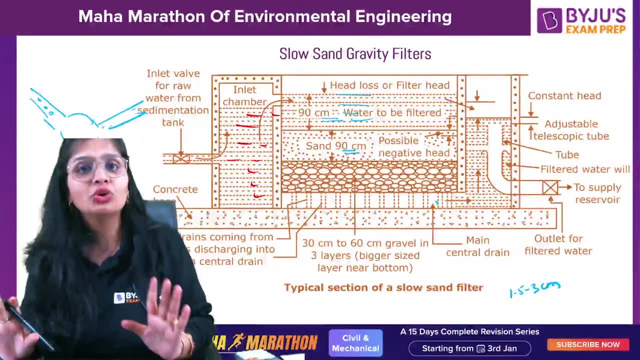 it. What is cleaning? Nothing to be done. Remove 1.5 to 3 centimeter of the top layer. That's it. Remove that. Your filter is clean, But you don't use it for 1 to 2 days, Why? Because you give time for the development of. 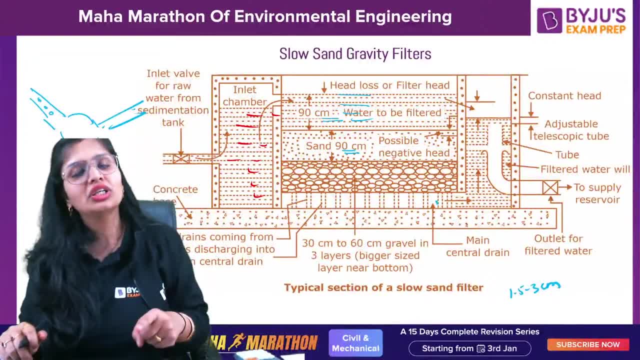 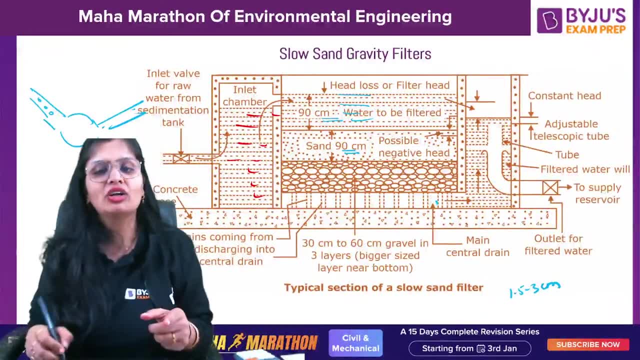 smart stack layer to be formed. Okay, So you don't use it. You give time for the smart stack layer to be formed initially and you clean it 1 or 3 months after that, when the head loss becomes 0.7 to 0.8. 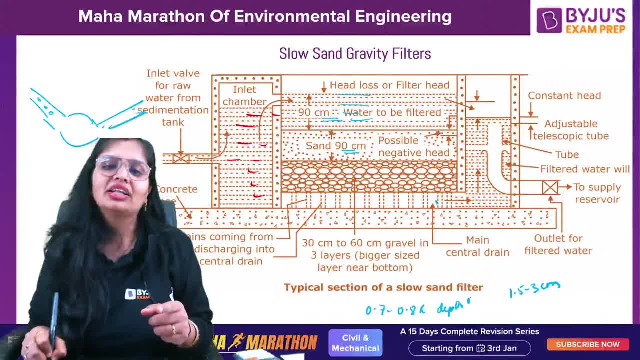 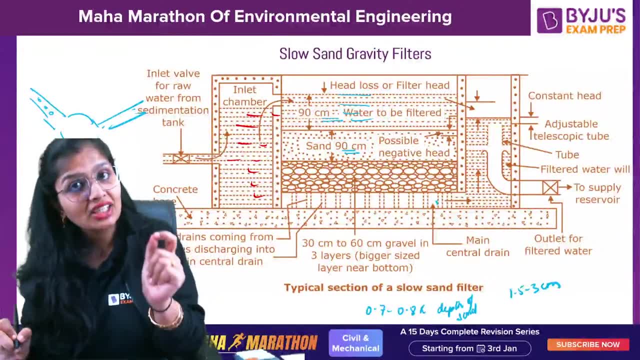 times the depth of the filter media. That is the depth of sand. Then you clean it. Just remove 1.5 to 3 centimeter of the top layer of sand, Ma'am. why that? Because that was a finer sand, So the 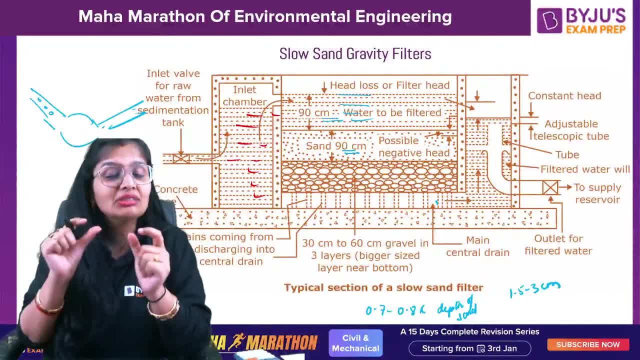 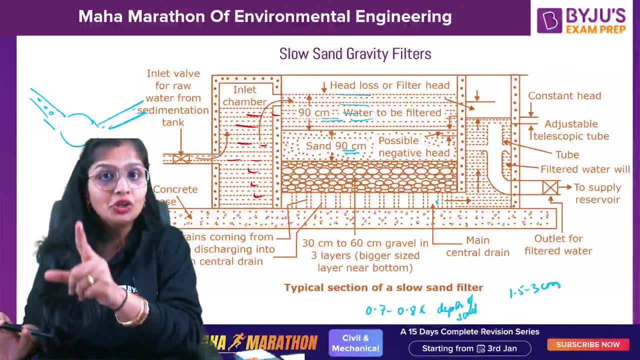 impurities is even finer than that. So the maximum amount of impurities are trapped only on the top 1.5 to 3 centimeter layer. So that's why remove that. But you won't put extra sand. No, you don't. 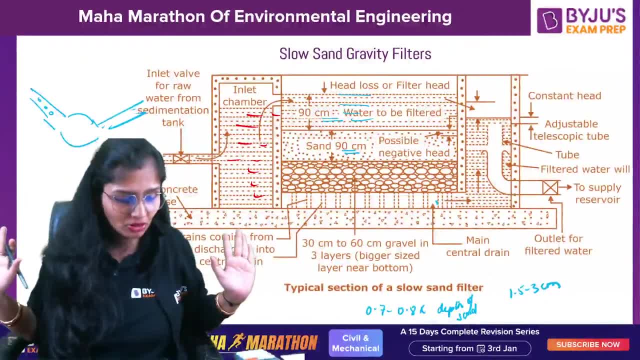 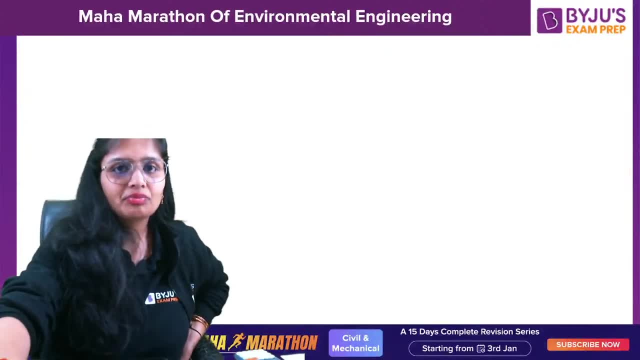 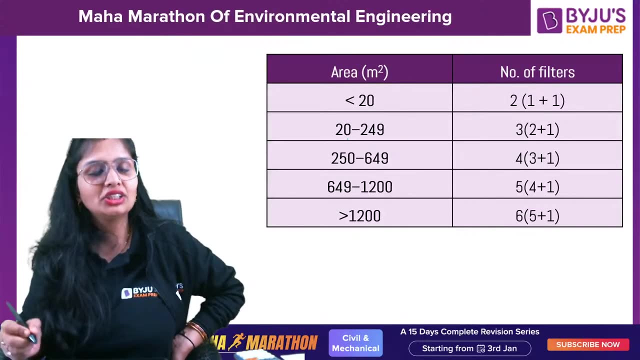 do that. Only you just remove it. This is the process of slow sand gravity filter Cleaning. I told you no Cleaning. I told you right now, Okay, Now this is conventional. If they say don't mention the number of filters, this is for conventional If the area is 20 to 20 meters. 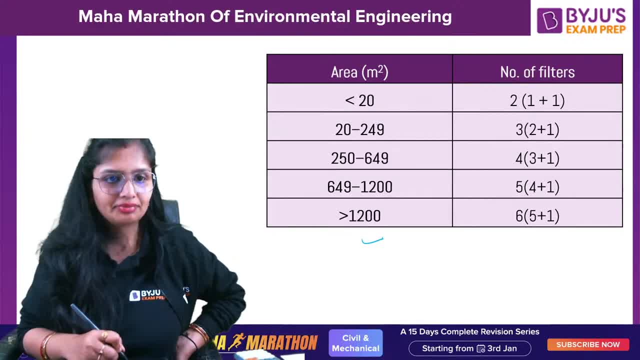 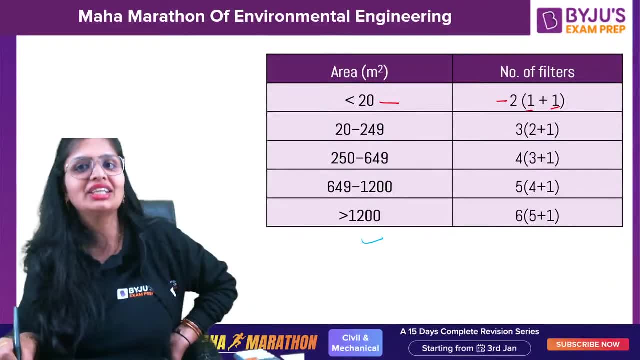 if it is less than 20 meters square, 2 is required. Generally, 1 plus 1 means 1 is operational, 1 is standby. 20 to 249 meters square of area 3, 2 operational, 1 standby. Standby is always. 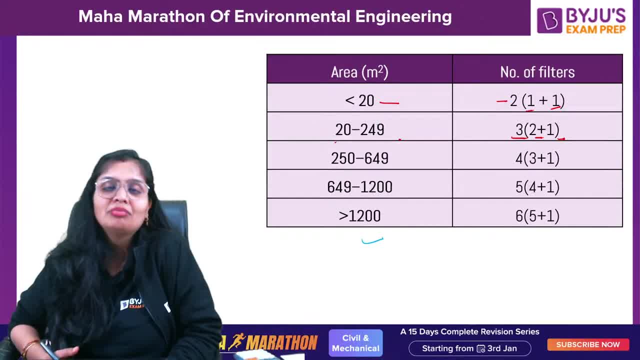 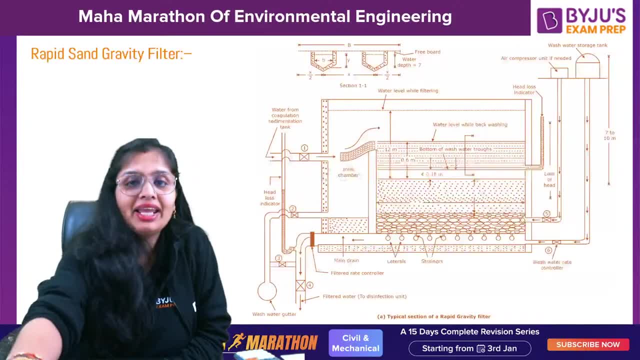 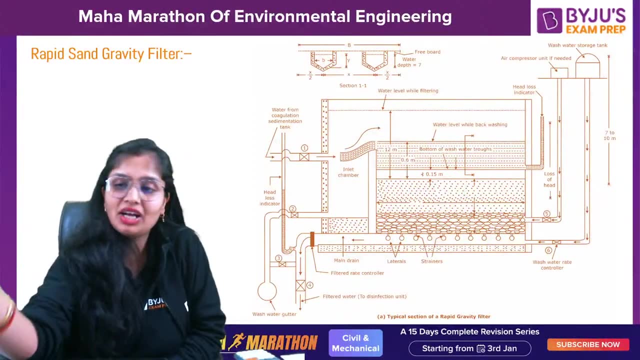 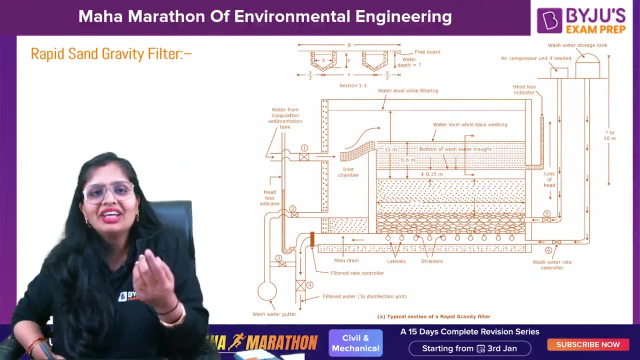 needed so that in case of any operational man functioning anything it happens. So there should be extra filter units. Okay, Any doubts till here? Any doubts till here? Fast, Then we have rapid send and disinfection. That's it, guys. Quickly. Any doubts? 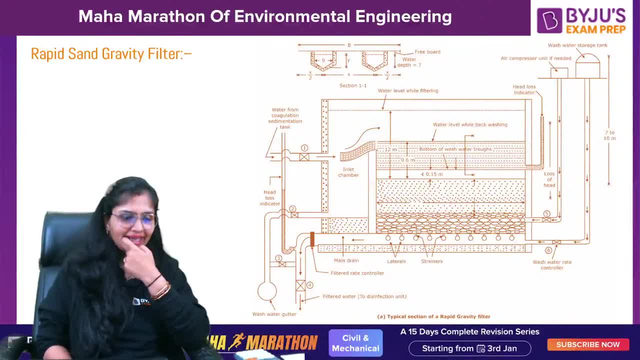 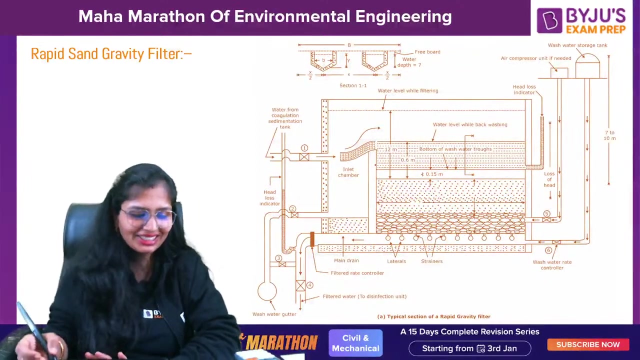 Any doubts? My head gets stuck. Okay, Now, you guys are not hungry. na, Are you guys hungry? No, right, Okay, Fine, So rapid sand filter. if I talk about Rapid sand filter, Girish is hungry. 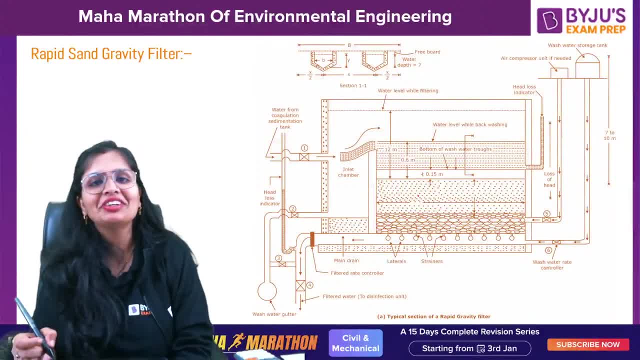 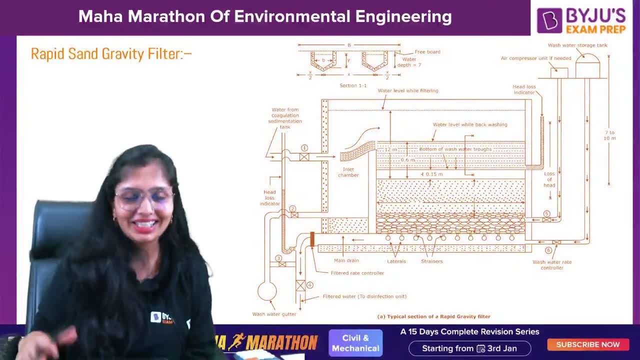 Then you have to be hungry till we complete. I want that distribution we should complete so that when we come to the wastewater characteristics we will come after half an hour. we come with a fresh mood, But let's see how much we will be able to do it. 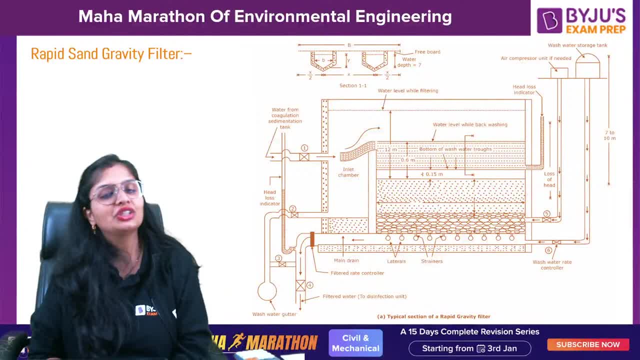 Okay, So this is the schematic diagram which you can see a section of it. Simple, You can see here the walls are being provided Simple. One more thing: In the case of slow sand, filter water comes from raw water or the plain sedimented water. Why we don't use coagulation needed? 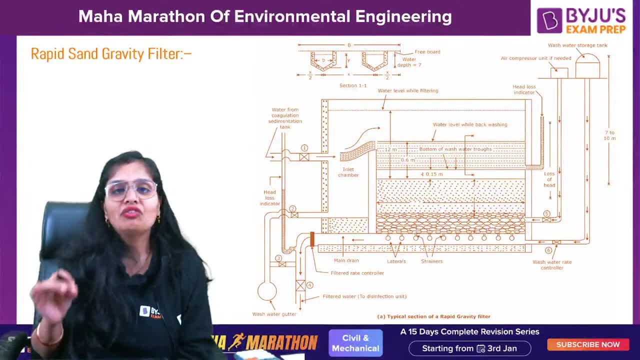 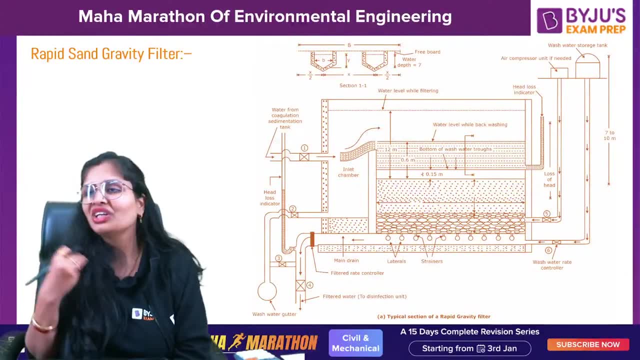 sedimentated water. Otherwise the voids of the filter pores will get clogged. That's the reason we don't use it. But for rapid, You can use any water you want. Okay, Generally we use coagulated sedimented water. Now what is? 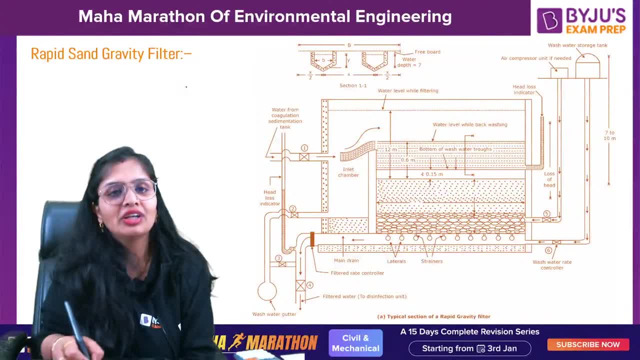 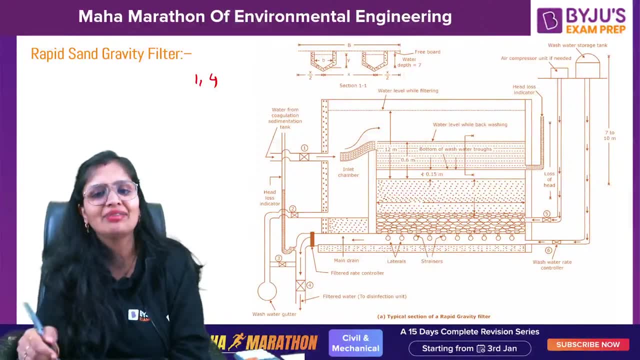 happening. From wall one, the water will go. Okay, Wall one is open. Wall four is open. It will go again. Same amount of water is to be maintained as the depth of the sand. Everything is same with water four. It will go to the disinfection unit. Everything was going, going, going, going going. 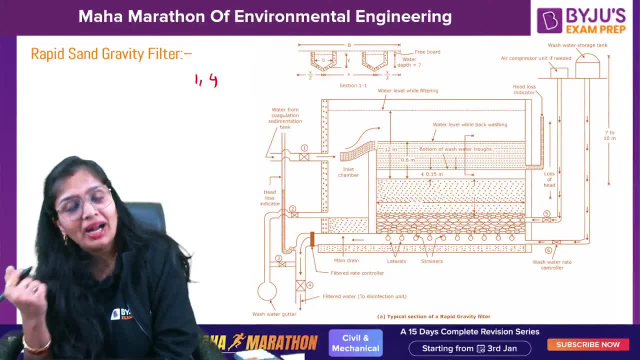 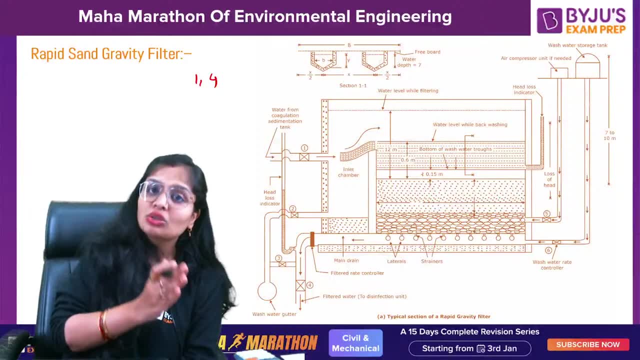 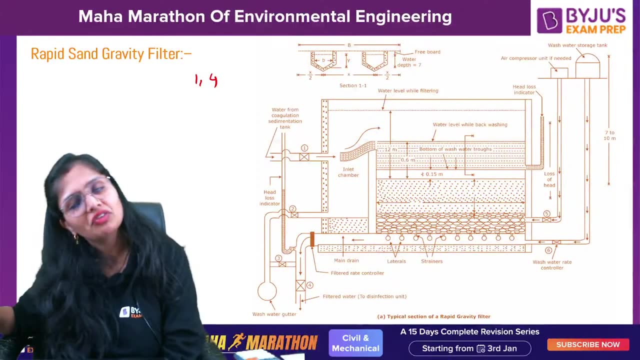 Here, the size of the particles of sand or the uniformity Coefficient is poorer as compared to the slow sand filter, Ma'am. then why we are using it? Because we will go for disinfection After this. we are not giving you the water to drink, We will go for. 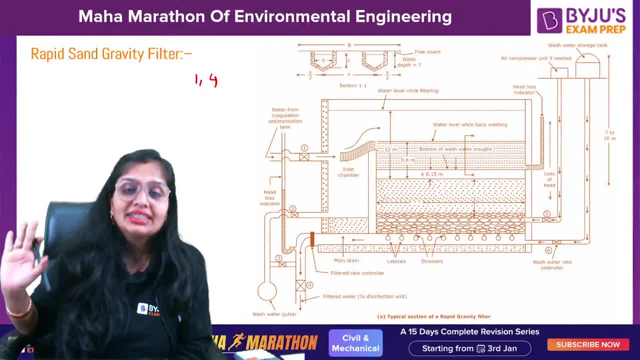 disinfection. So no matters if it happens. Secondly, if you talk about. Secondly, if you talk about What you will see it here, What you will see it here: Mechanical staining, sedimentation, biological changes, electromagnetic action, all will be taking place Eventually. here you will get. 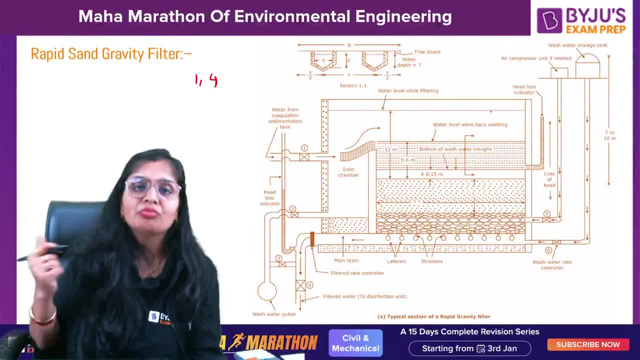 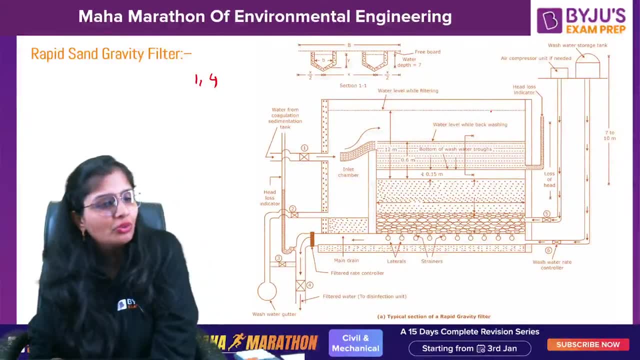 that You have to Clean the filter more often. More often means one to two days, 24 to 48 hours. You have to clean the filters. When you will be cleaning the filter, what you have to do is you have to close one and 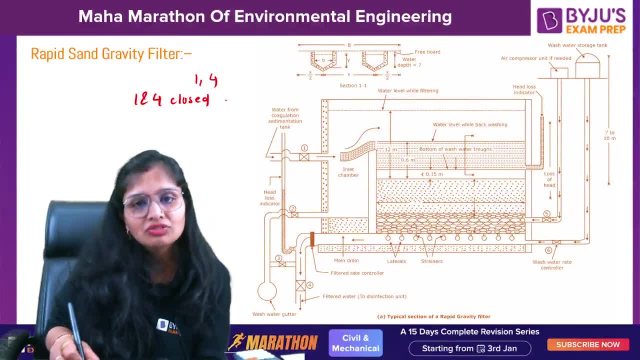 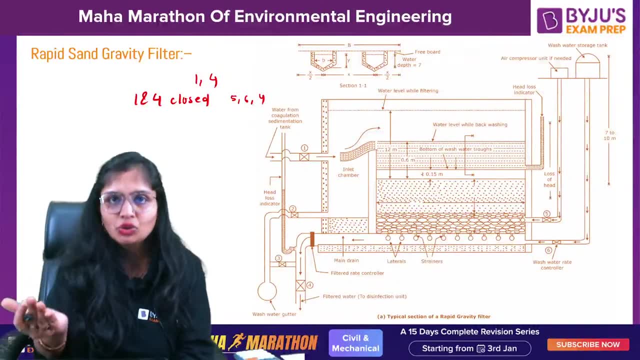 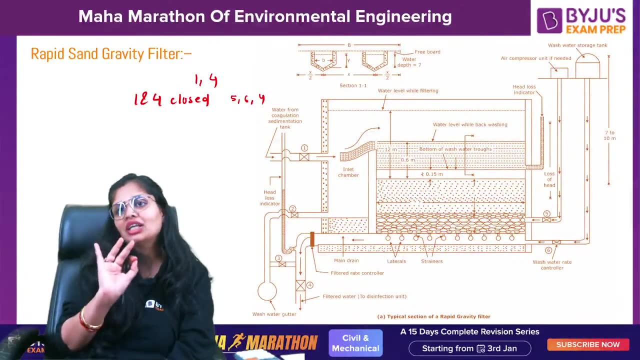 four. This wall will be closed and what are the walls will be opening is five, six and four. So now what happens? Whenever you will do the cleaning, you do it with the clear water, That is, but obviously you do it with the clear water. So what is happening is when you do it with the clear 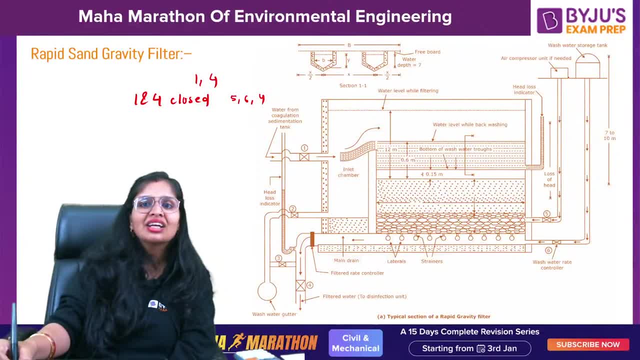 water, a certain amount of filtered water is stored and then air compressor is provided. When, in some places where you cannot maintain the storage tank, you need to supply with air compressor unit. Okay, so it's not everywhere, it is mandatory. in those conditions, you have to supply air compressor. 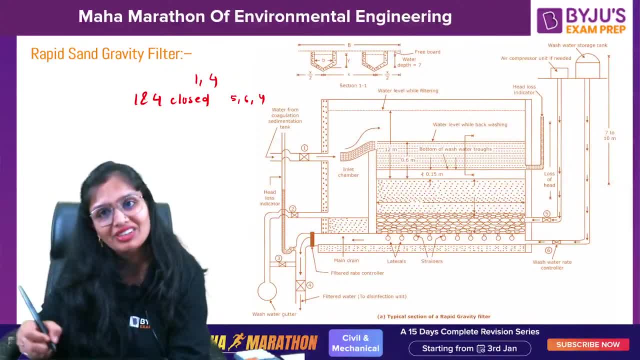 what will happen From here? you will bring the water- okay- back. right now it was going from top to bottom. Now, for cleaning, the water will go from bottom to top, along with compressed air. so what it will do? it will expand the filter bed. it will expand the. 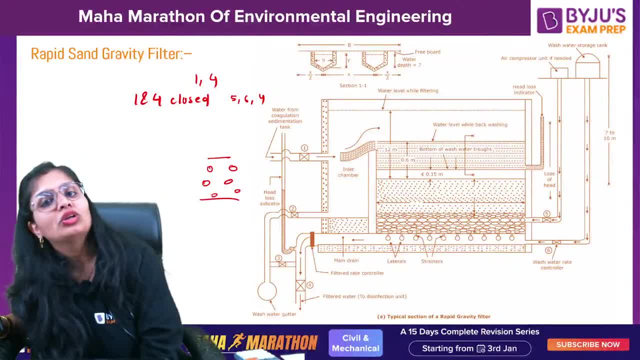 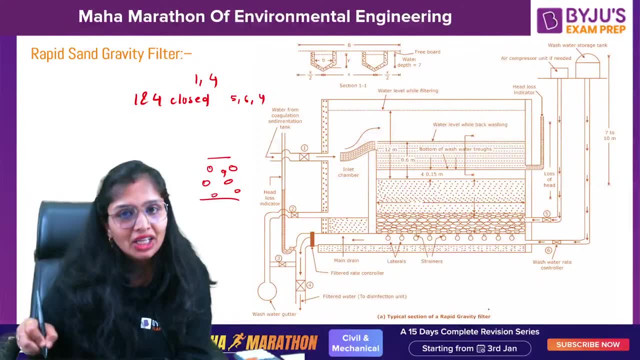 filter bed. but the filter bed should not expand more than 50 percent. okay, so now, when the filter bed particles will expand, the impurities will be set free. the water is being passed through it. these impurities, these are the wash water troughs. these are collected over here, from here it goes. 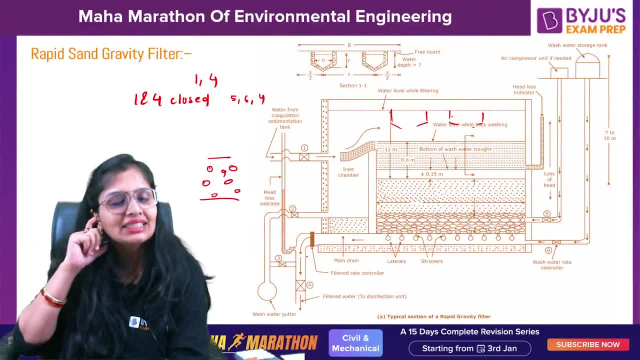 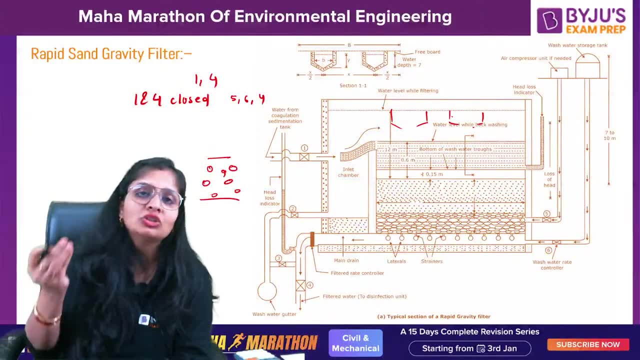 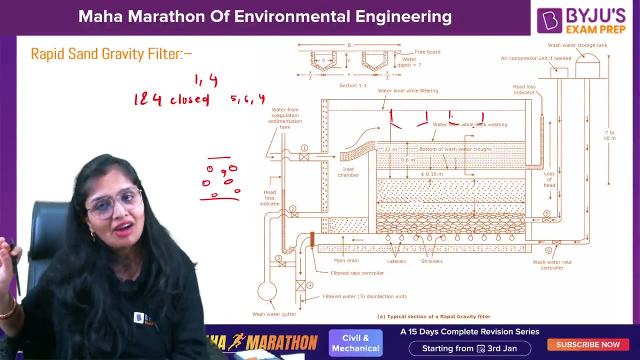 into the wash water, cut. okay, as simple as that. it goes in this manner: okay, so now you are doing back washing. you are doing back washing so that the impurities which are entrapped, they can be removed. that's it, simple as that. now, over the time after, it takes around 30 minutes time if in the 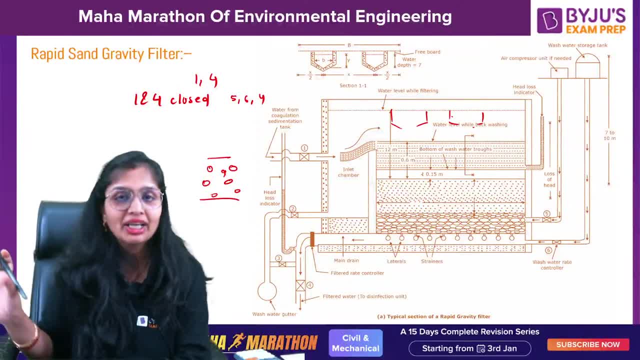 question. it is not getting you telling me anything about back washing, don't take it. but if it is telling you, deliberately, you have to take it. okay, this whole process requires 30 minutes of time, okay? so now you are doing back washing. so now you are doing back washing. so now you are doing. 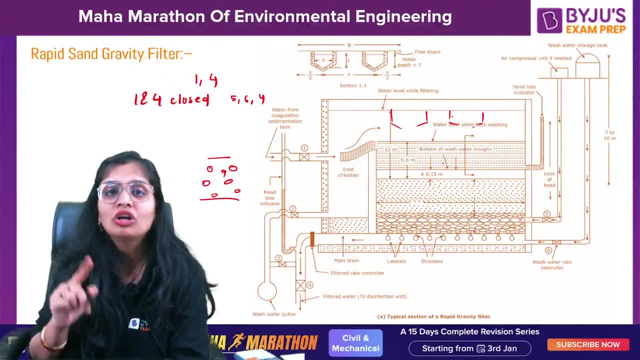 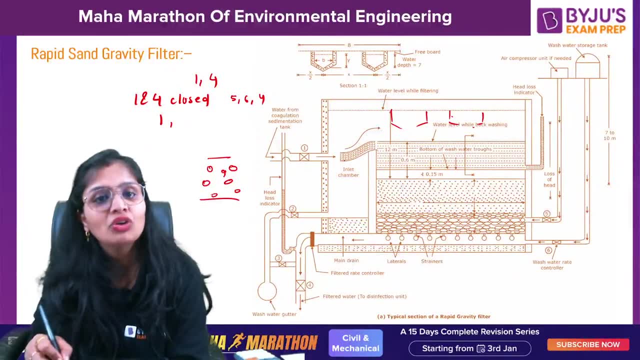 eventually, after this back washing is done, you do not use the water because certain impurities can still be present. so you will open wall number one, but this time you will open what. you will open wall number, which wall? the water will come, but this time it will go what it will go through wall. 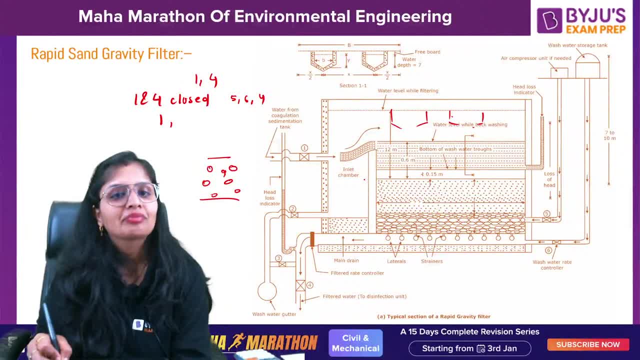 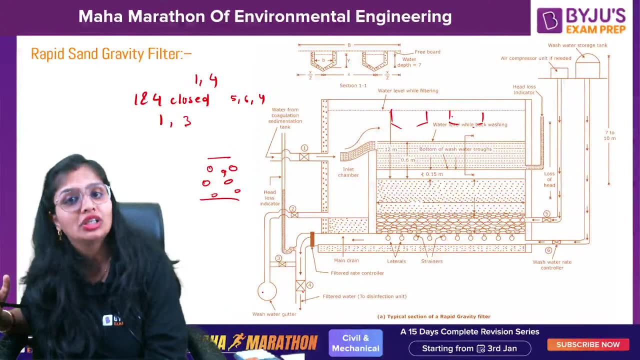 number three. wall number three: it will go into the wash water cutter so you won't take it to the disinfection unit. it will pass through the lateral rains and all, but this time it will not go through here. it will go to wash water gutter. it will go to the wash water gutter. okay, so make. 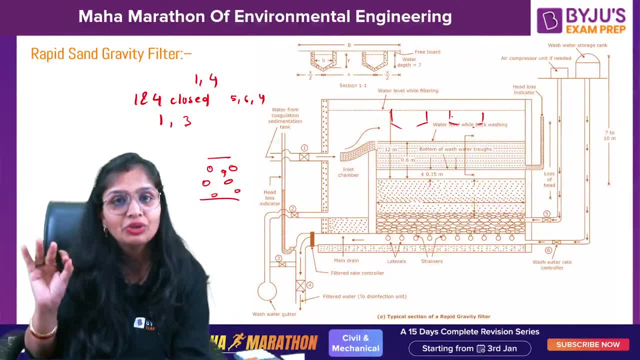 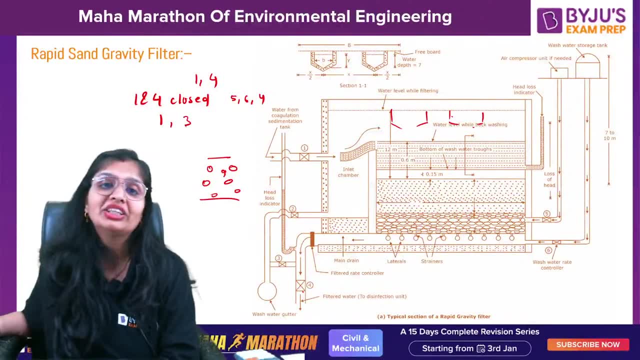 sure, make sure this whole time and during this process, when you passed it, you gave the time. who was asking me to see here? we don't give much amount of time for the formation of smudged deck layer, so that is the reason the efficiency is not much as compared to that of slow sand filters and 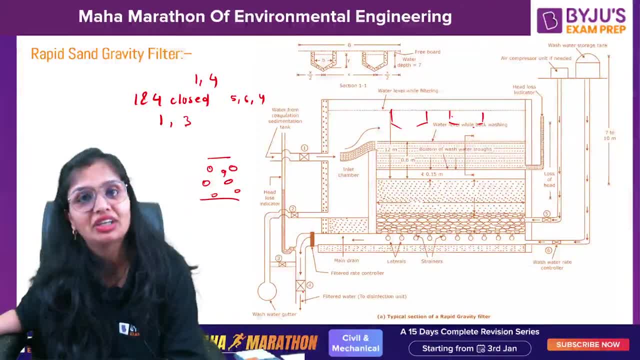 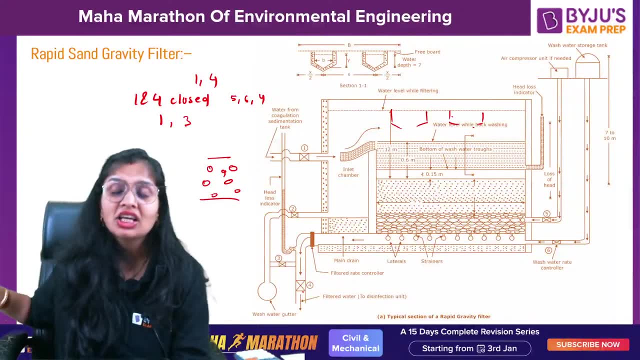 that is the reason it is to do disinfection after rapid sand filter. however, the rate of filtration is 3000 to 6000 liter per hour per meter square, so it is 15 to 30 times more as compared to slow sand gravity filters and that 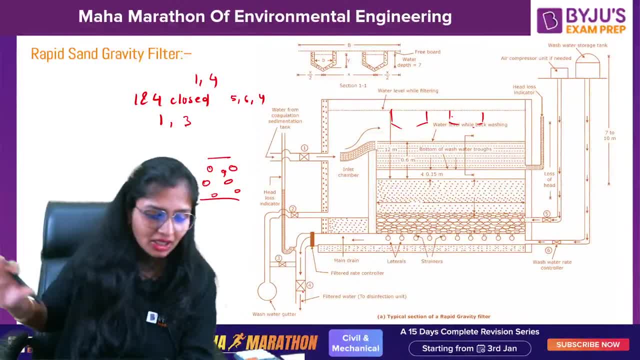 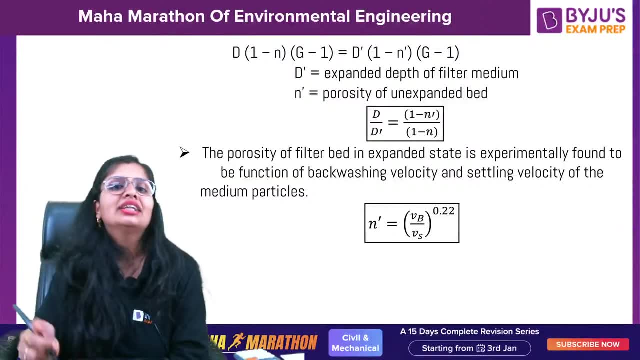 is the reason we use RSF clear. this is the whole procedure which you need to follow. last, if, when you are expanding it, this is the formula, the head loss which happens. this is a formula D: 1 minus n, G minus 1. in some books, instead of D they write L. so this is the depth of the filter. media n is the 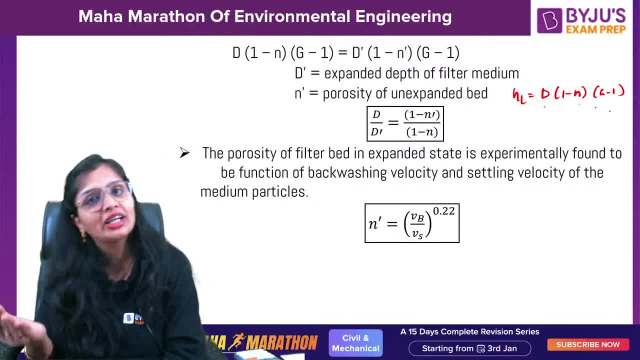 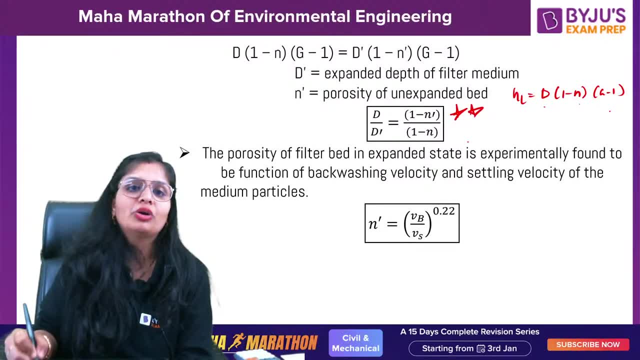 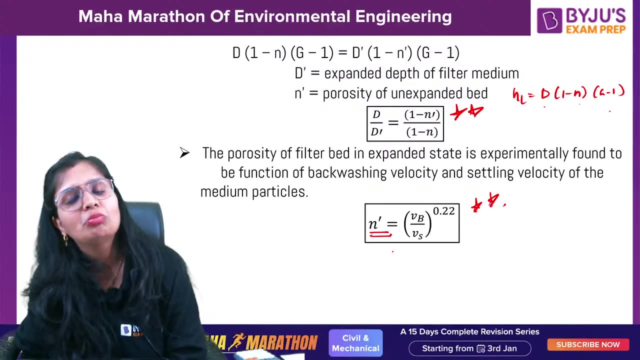 porosity, G is the specific gravity. if you expand it also, the head loss remains to be the same. so this is the formula and this, this is very important, this one is important and this one is important. so the expanded porosity, it will come out to be VB VS to the power: 0.22. this is the expanded 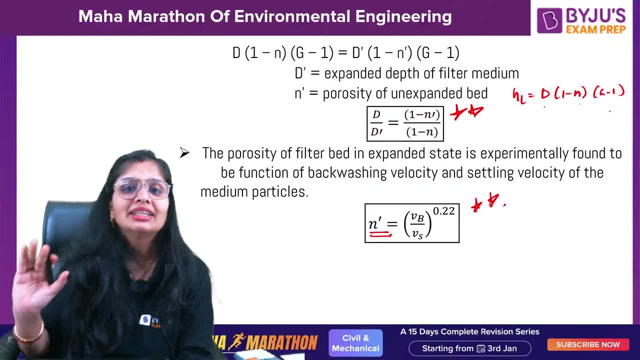 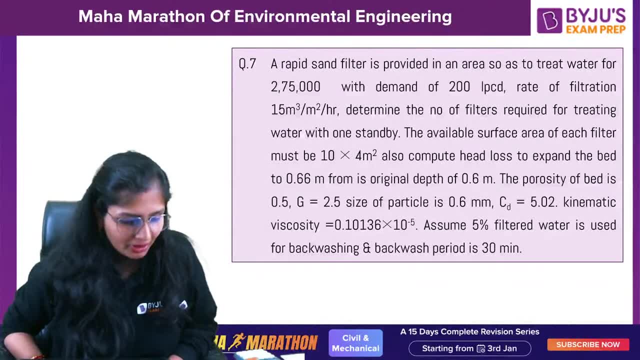 porosity, which you will get. okay, Now guys, solve this question. Why do you put on headphones? why do I sound so bad? Why are you putting on headphones? or hear such a normal sound? will my ears go bad? Okay, solve the question. 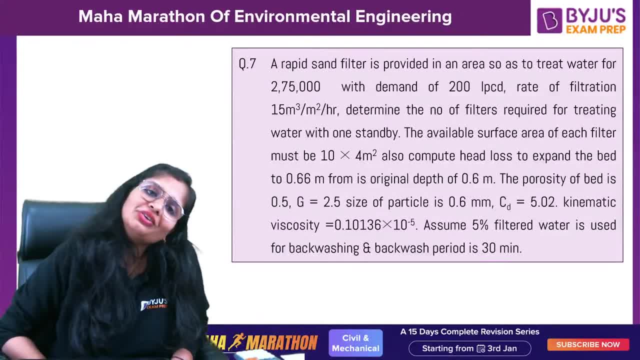 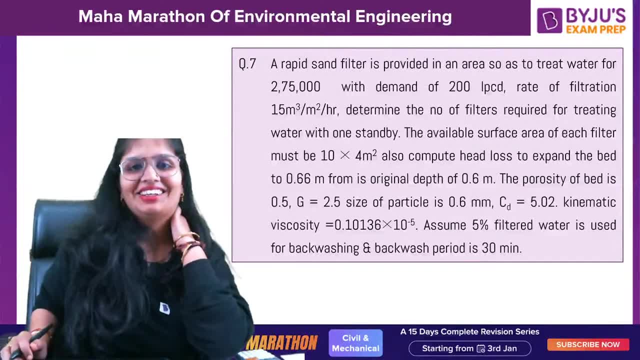 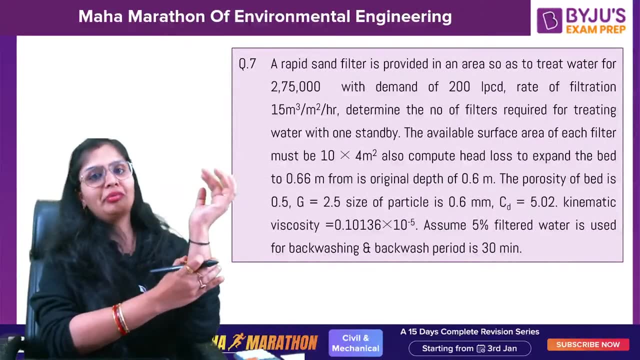 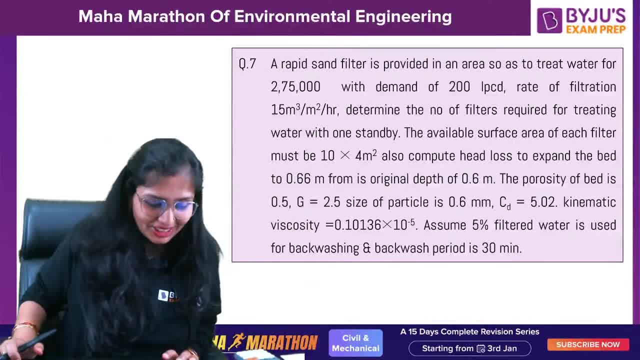 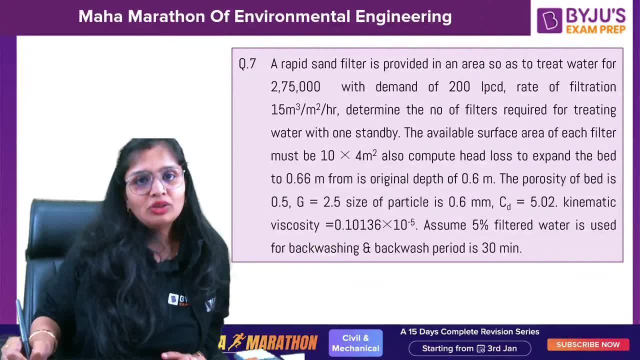 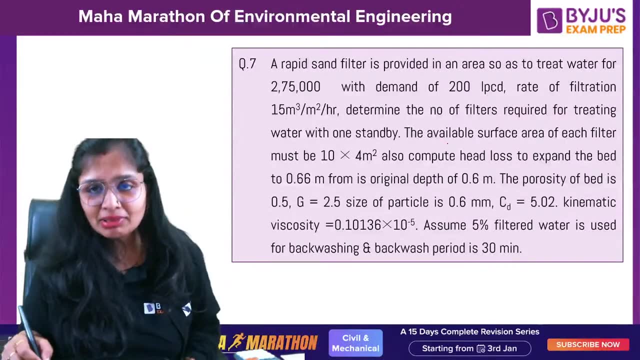 Yes, Hello, Mr Shravan, Let's solve this question. Rapid sand filter is given for 2,75,000 people. We have to treat water for 200 LPCD. Come on, guys, I agree to design for maximum daily demand. It is not written here, I will write it. 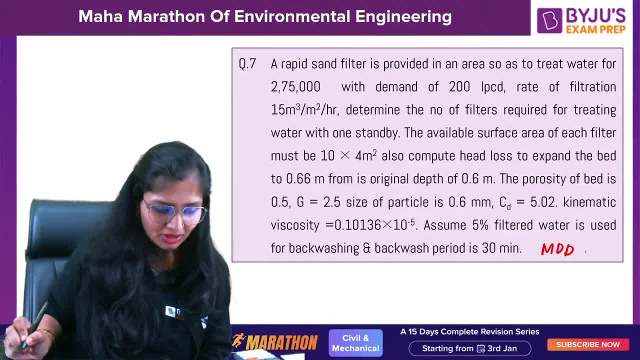 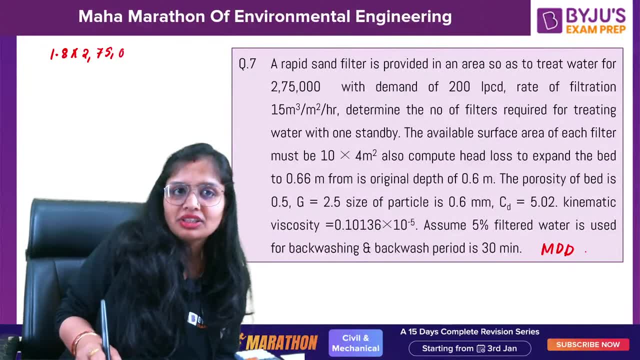 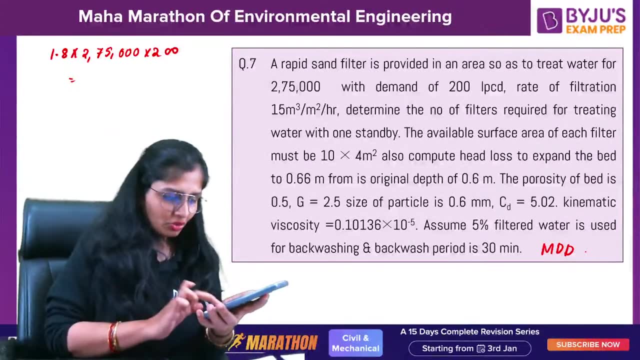 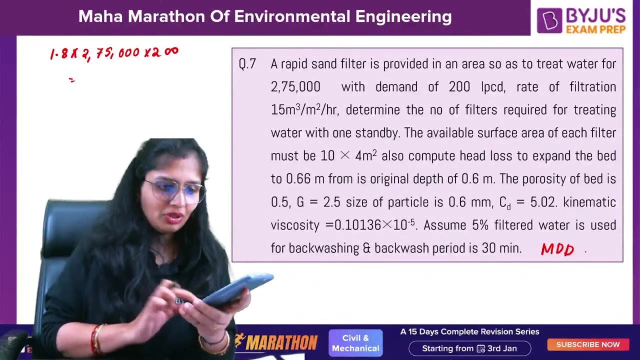 For maximum daily demand. Let's go. I am in the library. 1.8 times 2,75,200 LPCD. How much it is coming? Wait a little, Arun, I will give till 3 o'clock 200. This comes out to be 99 MLT. 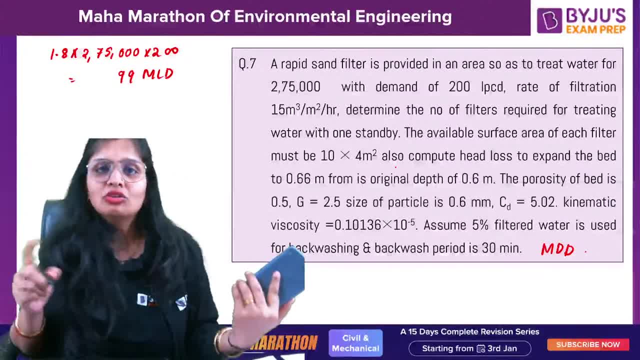 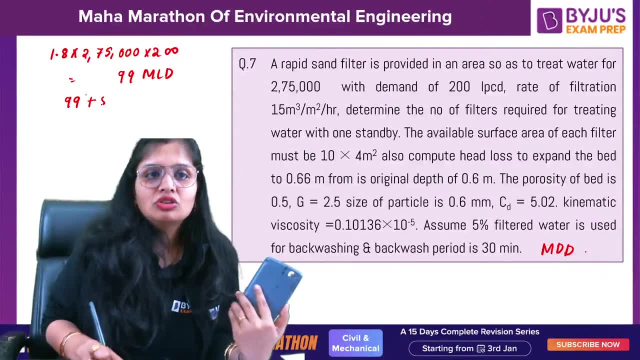 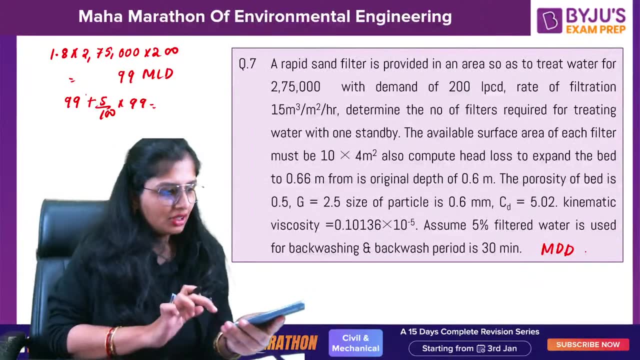 But 5% more water is required. So if you want to clean it, You will clean it. with what? Clear water? only filtered water. So 5% of it is required. So this will become 99 into 1.05. This will come out to be how much. 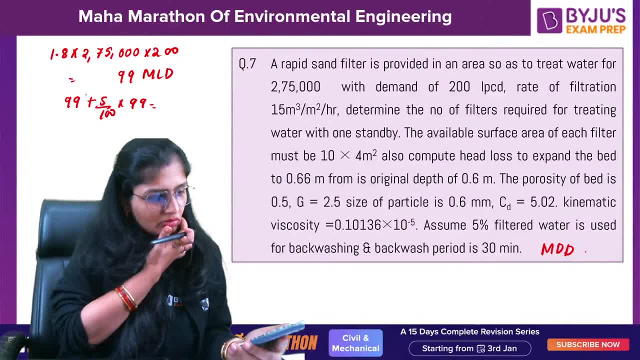 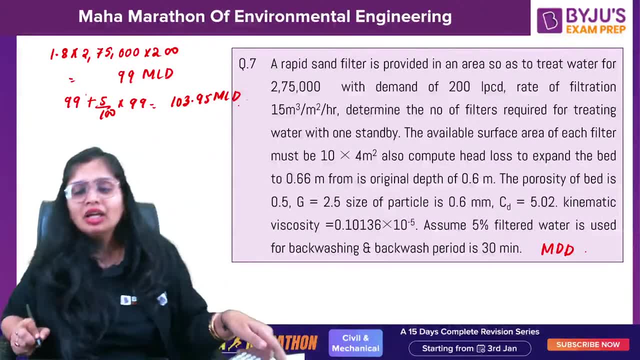 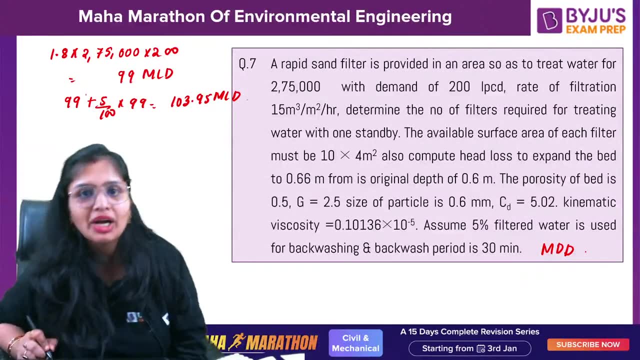 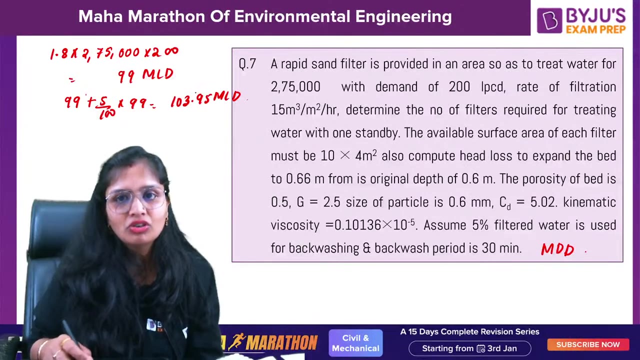 This will come out to be 103.95 MLT. Now, what it is telling me in the question? What it is telling me? It is asking me to calculate the number of filters required For treating water with one stand by. So, first of all, First of all, this much amount of water is required. 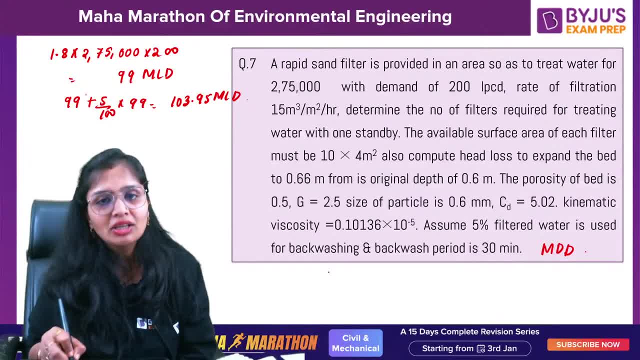 And rate of filtration is also given to you. So the total number of 103.95 into 10, raised to power 6 L. But the filter is operating for how many hours? 23.5 hours. Why? Because 30 minutes it was being what. 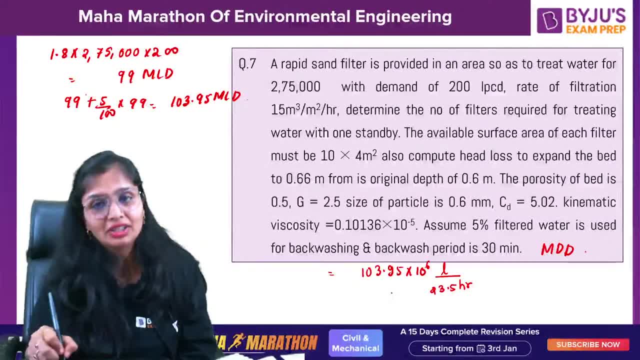 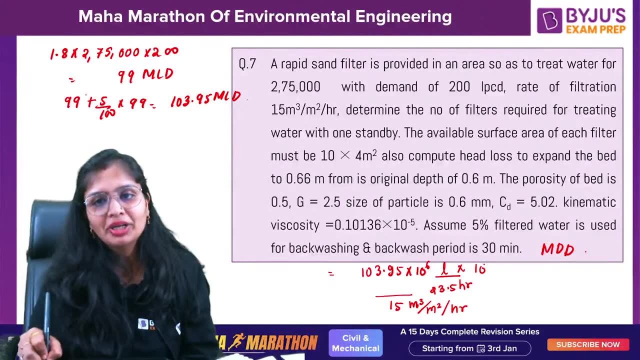 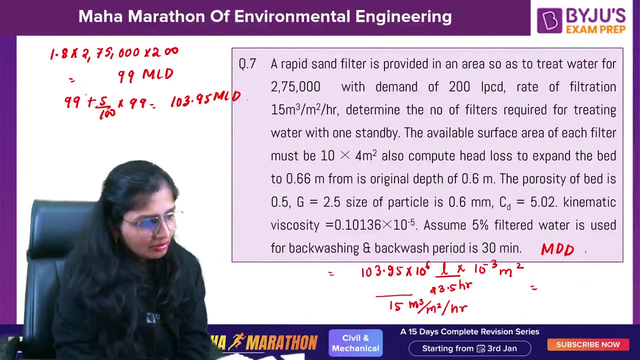 Clean, So that time water was not being filtered. And what is the rate of filtration? 15 meter cube per meter square per hour. So from here, convert liters into meter cube, You will get the total area of the filters. How much is the total area coming? 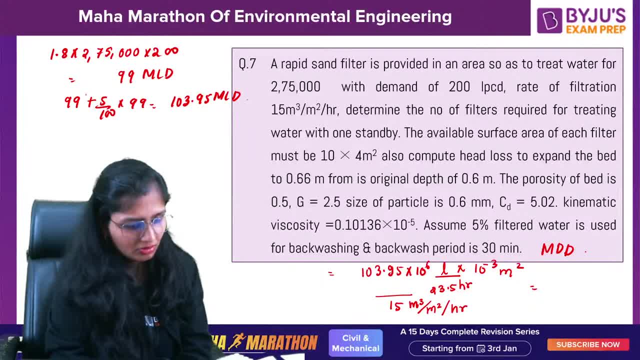 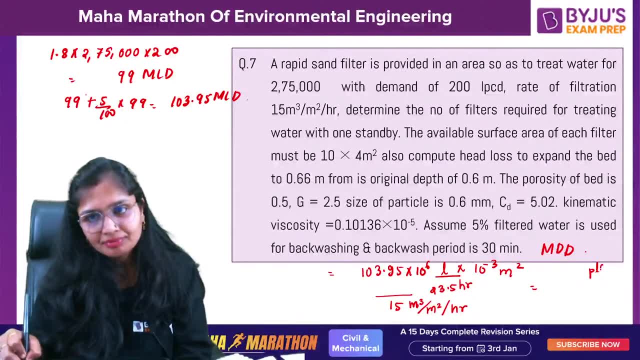 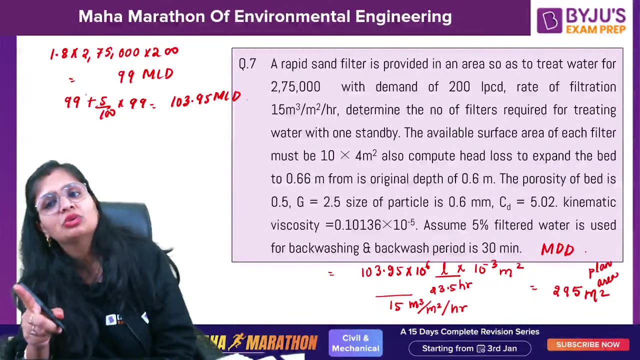 Total area? I am asking Total planned area. Is it coming 295 meter square? Just check it out. So if one area surface area of one filter is 40 meter square And the planned area is 295, So how many number of filters will be there? 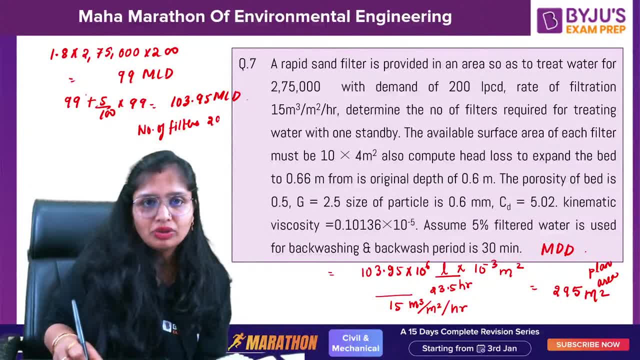 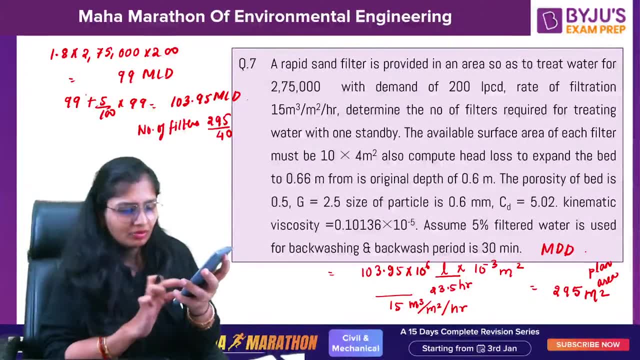 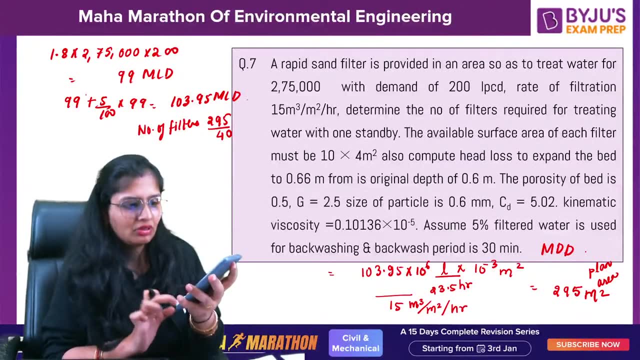 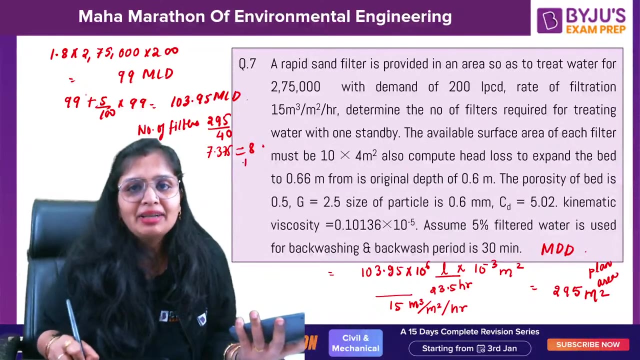 295, divided by 40, It comes out to be 7.375. So we will take it as 8. So the total number of filters will be 8 plus 1, Because 1 will be as stand by. So 9 filters are there, What it is asking. 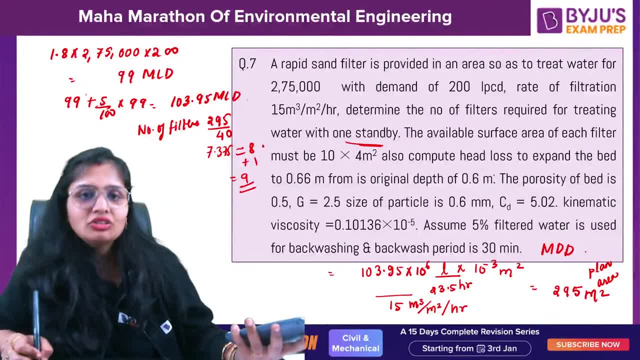 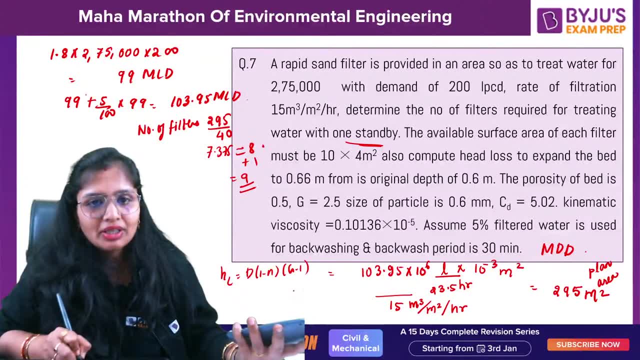 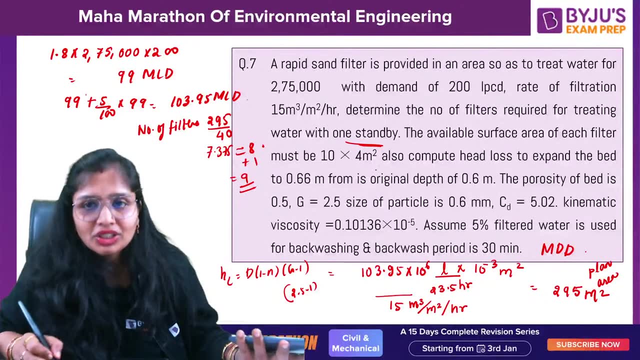 What it is asking you: Calculate the head loss. So it is asking you to calculate the head loss also. Head loss is d: 1 minus n, g minus 1, So 2.5 minus 1. To expand the bed to 0.66 meters from its original 0.6 meters. 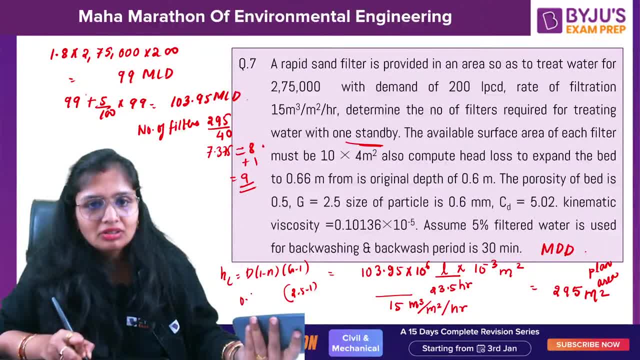 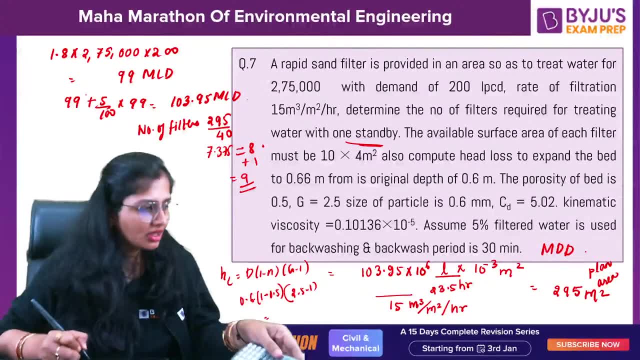 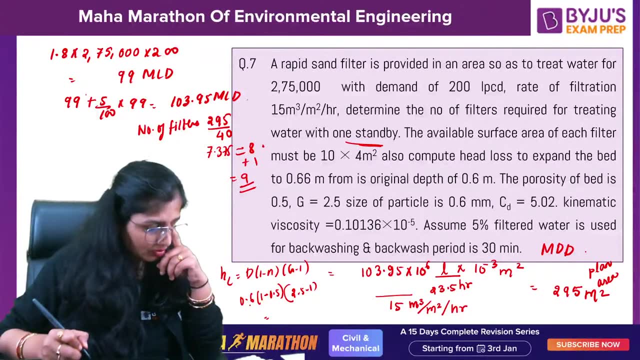 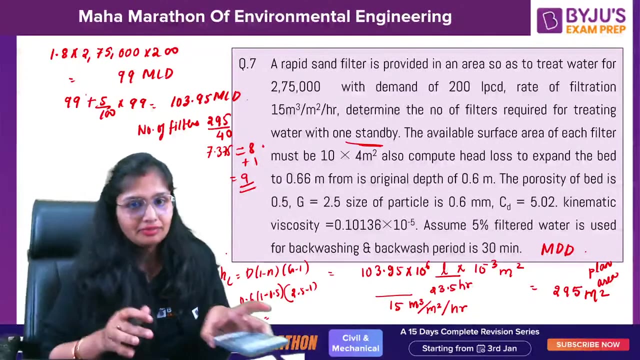 Porosity is mentioned. very simple, Nothing to do. Simply calculate the head loss. Nothing to do: Head loss which is required to expand the bed It is given. Simply, you can do it. 295 Previous answer. you are given. This one is coming out to be 0.45 meters. 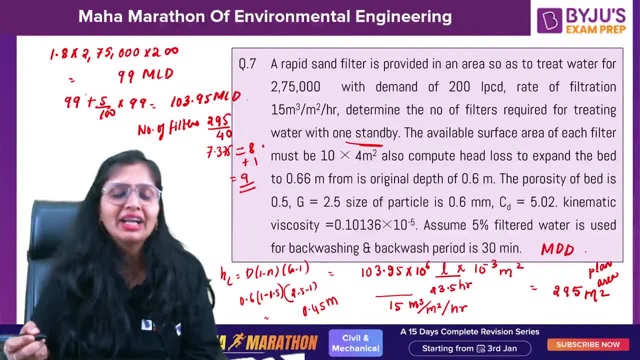 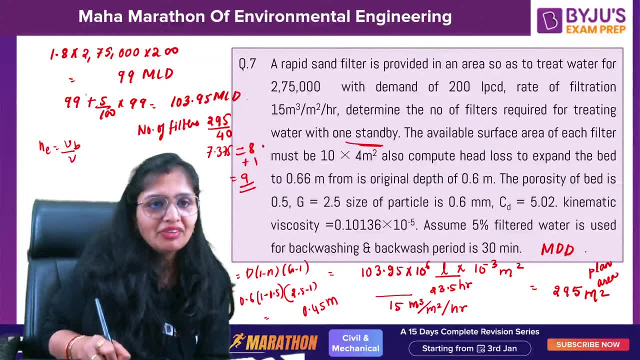 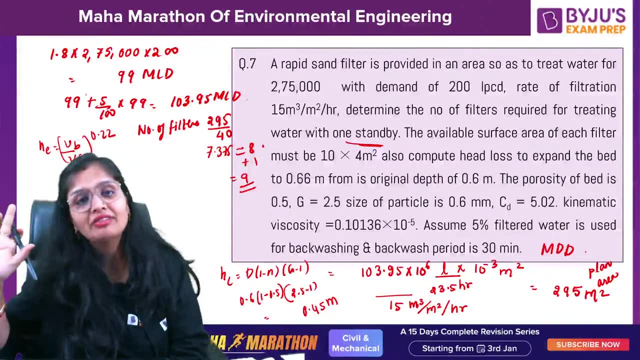 In this question it can ask you some things like expanded porosity. So if it ask you expanded porosity, You can calculate that also. Ne is equal to Vb by Vs to the power 0.22. Remember settling velocity. Remember settling velocity in the case of rapid sand filter is transitional in nature. 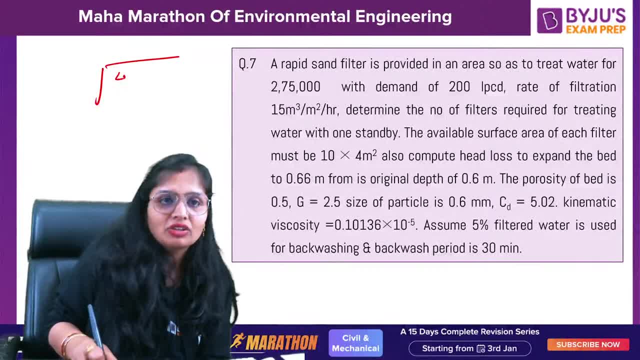 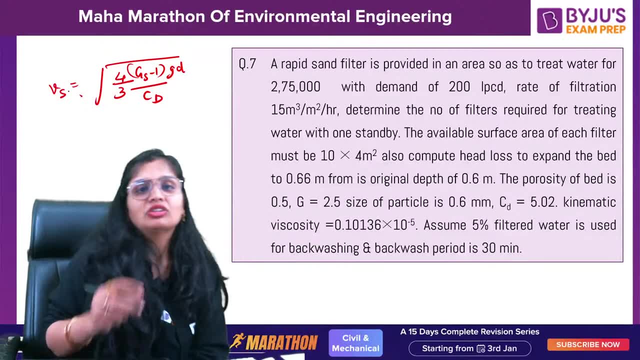 So the formula which you get it here for settling velocity is 4 by 3 Gs minus 1 Gd upon Cd. This is the formula of settling velocity which you use Here. the flow is not at all laminar, It is transitional in nature. Ok, 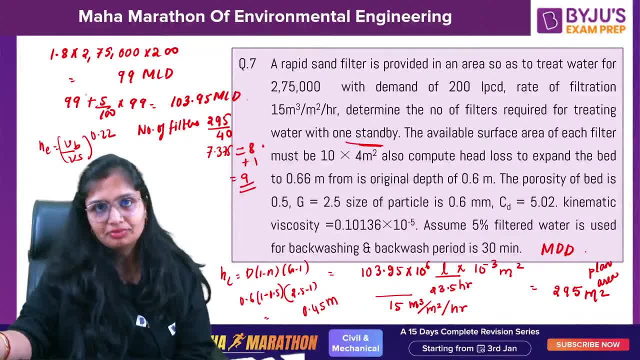 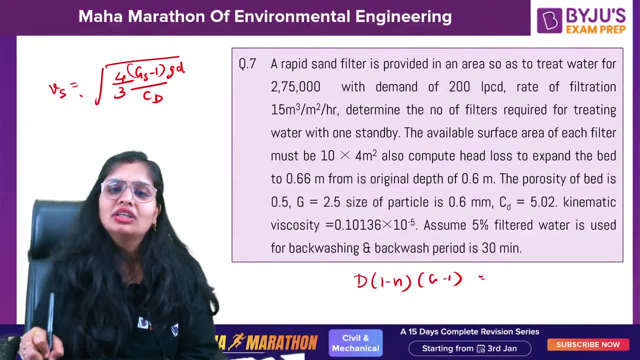 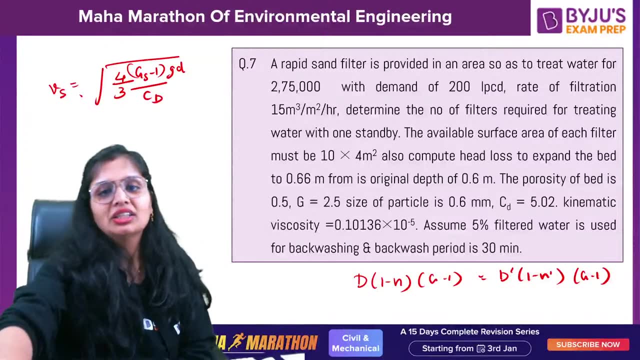 So if it is asked, you can go by that And expanded porosity you will go by this formula: D1 minus N, G minus 1. D dash 1 minus N, dash G minus 1. So I told you two things, but if they will ask you any other thing, you should be able to solve. 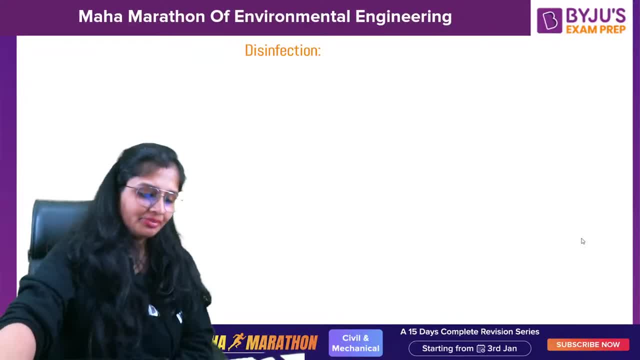 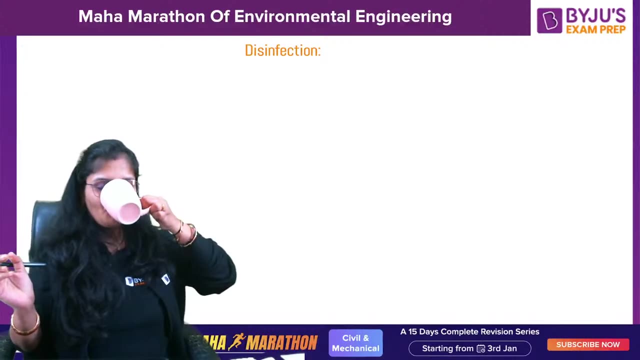 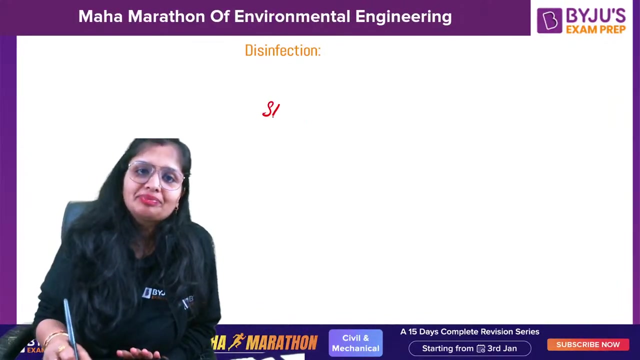 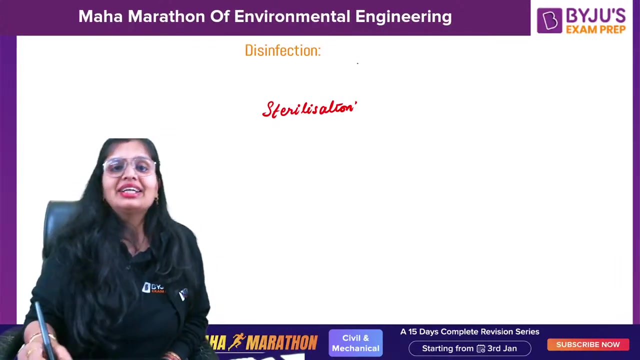 Clear. This whole concept is clear. Tell me fast, Now we have reached to the last topic, Disinfection. Ok, Now, technically there are two things. One is disinfection and the other one is sterilization. The process of killing disease, causing microorganisms, that is, pathogens, It is known as disinfection. 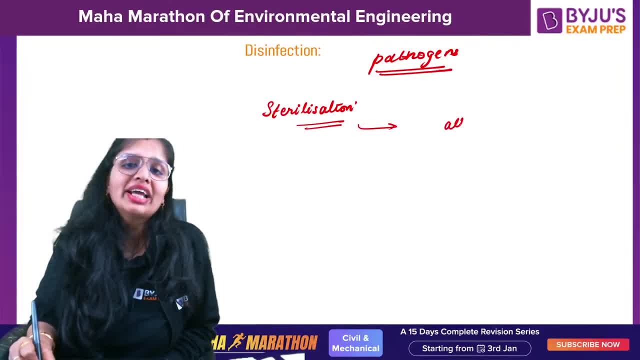 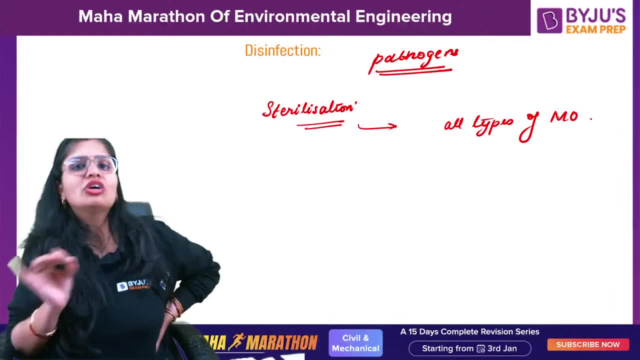 Sterilization is the process of killing disease causing microorganisms, that is, pathogens. it is known as disinfection. Sterilization is the process of killing all types of microorganisms. All types of microorganisms is killed based on sterilization, And disease causing microorganisms are killed based on disinfection. 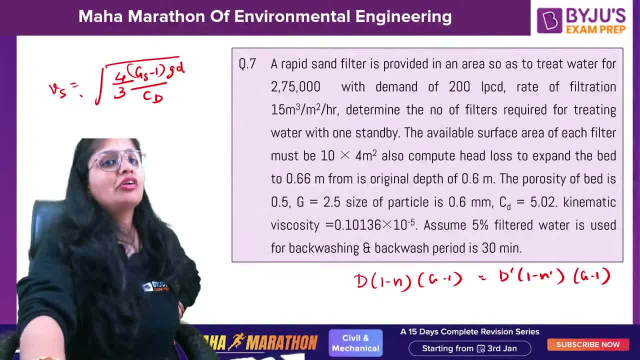 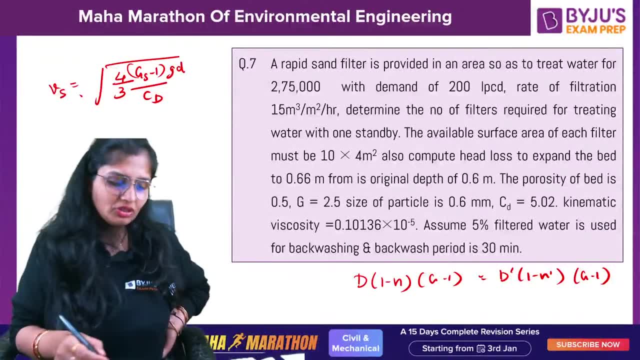 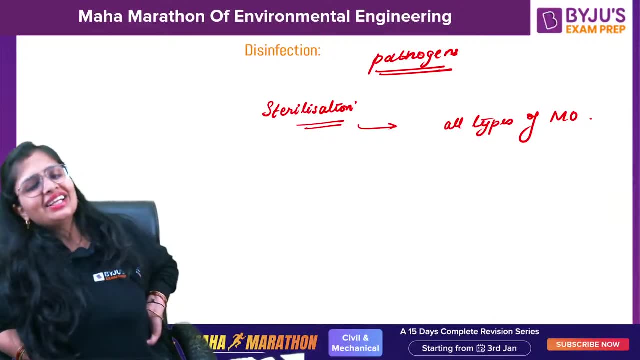 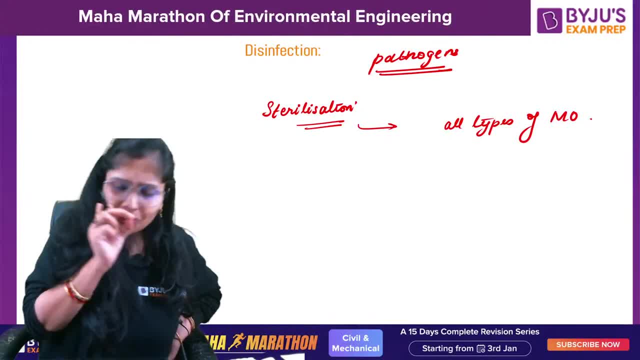 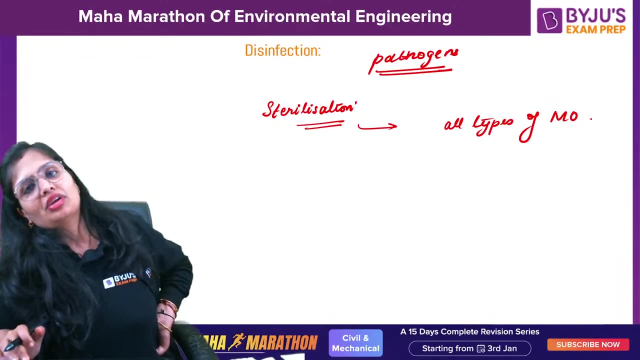 Ok, you are disease causing, I will kill you. You are disease causing, I will kill you. Is it possible that we apply any chemical and it will only kill disease causing microorganisms? Is it possible? CDS coefficient of drag: We have formula 24RE plus 3RE by half. 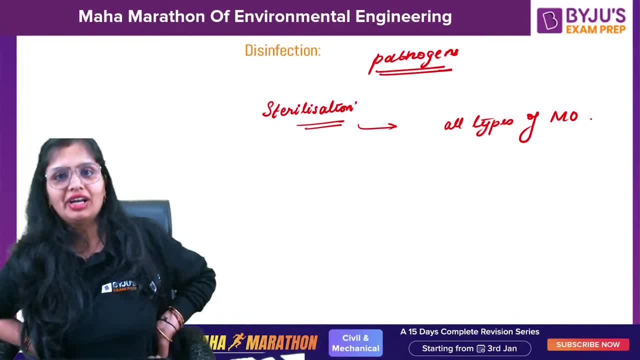 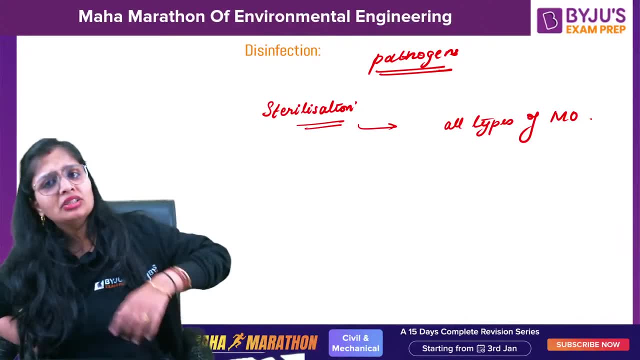 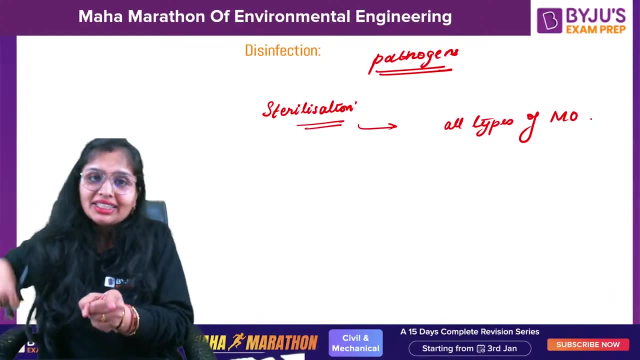 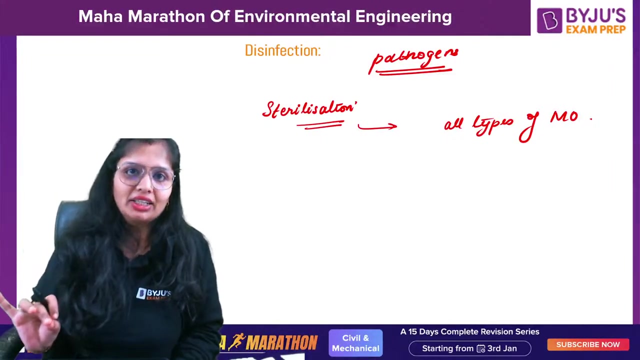 That formula: CDS coefficient of drag. CDS coefficient of drag- Is it possible, guys? No, So technically, what happens? all types of microorganisms are killed. So in the process of sterilization, disinfection happens. It's not possible that we can check it out. what is the disease causing microorganisms? and we will kill that. 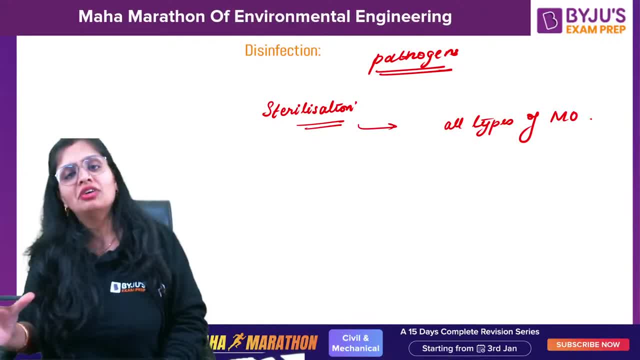 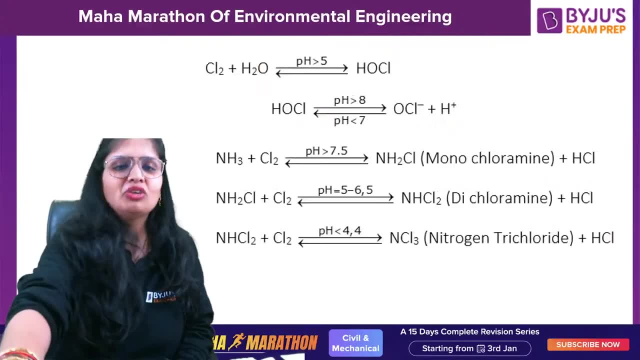 No, it doesn't happen like this. In the process of sterilization, disinfection happens. Now there are various types of things. you can add ozone, you can add KMnO4 and types of things are there, but we go for chlorine. Why? Because you need two things. 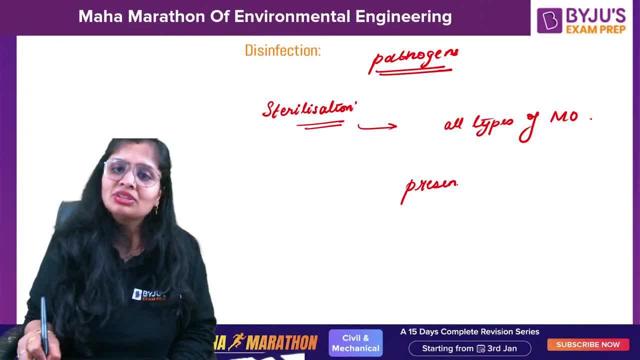 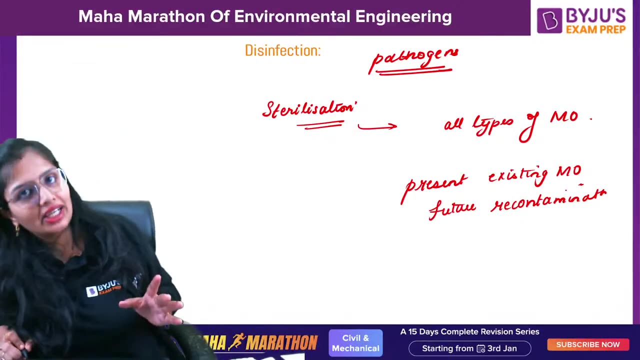 It should kill the present existing microorganisms And it should take care of future recontamination. So if you do boiling, first of all it requires lots of fuel. It does not safeguard against future recontamination. UV rays also it does not safeguard against future recontamination. 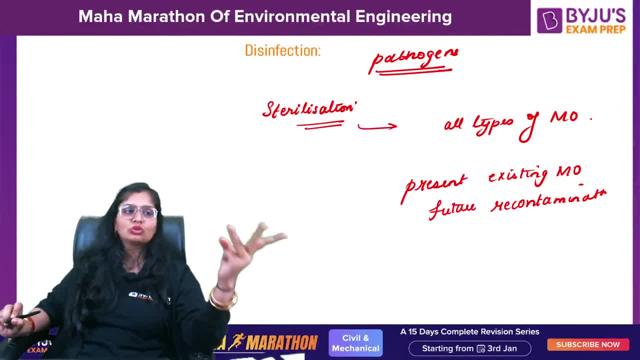 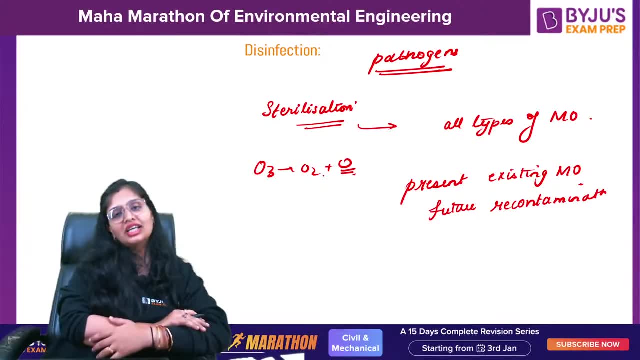 UV rays. also, it does not safeguard against future recontamination Ozone Ozone. you know Ozone is O2 plus O. This nascent oxygen is a strong oxidizing agent. It kills the existing microorganisms. It is costly. in Chandigarh and all you use this, but on prominent basis you don't use it. 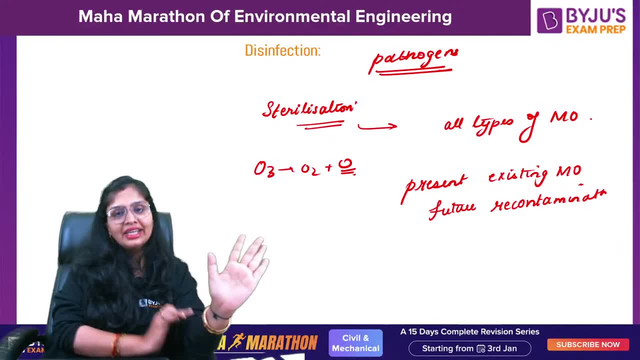 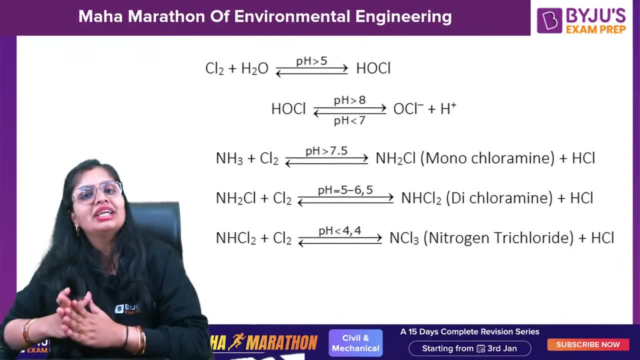 Okay, So basically we go for Cl2, that is, chlorine. Now this chlorine will function only when the pH is greater, When the pH is greater than 5. If it is less than 5, it will remain as it is, as molecular chlorine. So if you want it to function, you have to provide the pH of water more than 5. 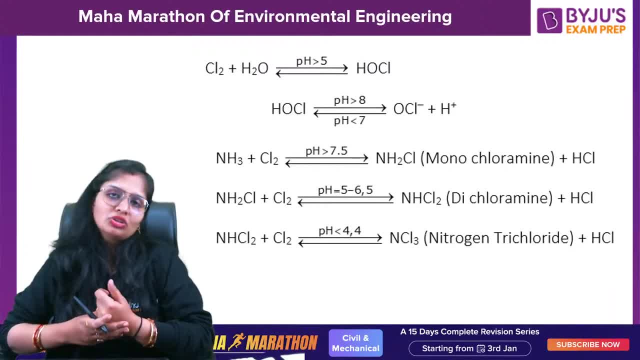 And you know also, the pH which is permitted as per the codal provision is 7 to 8.5. That means in that pH chlorine will function. So it will form hypochlorous acid And hypochlorous acid, when the pH is greater than 8, it will form hypochlorite ion. 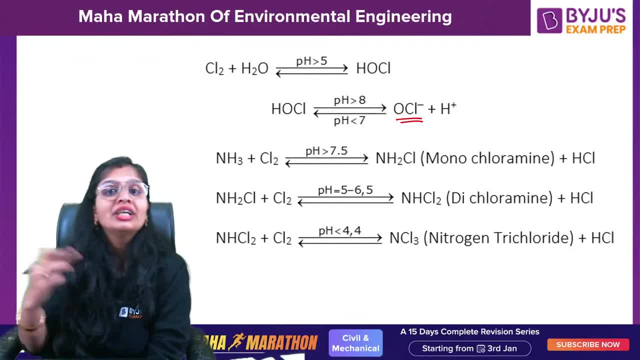 And hypochlorous acid. when the pH is greater than 8, it will form hypochlorite ion. Hypochlorous acid is 80 times more destructive than the hypochlorite ion, So that means it quickly reacts. Now, if you want the present existing microorganisms to be killed, 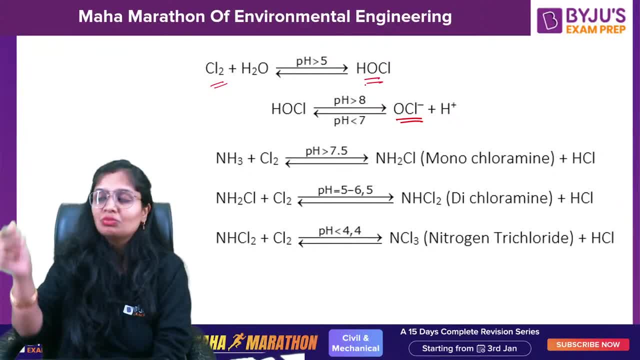 Then we go for chlorine, in that HOCl is responsible for present killing of the bacteria Or the any microorganisms For future recontamination. if you want Silver and oil also, we don't use it. We don't go for silver, copper and oil Because sometimes it becomes toxic. 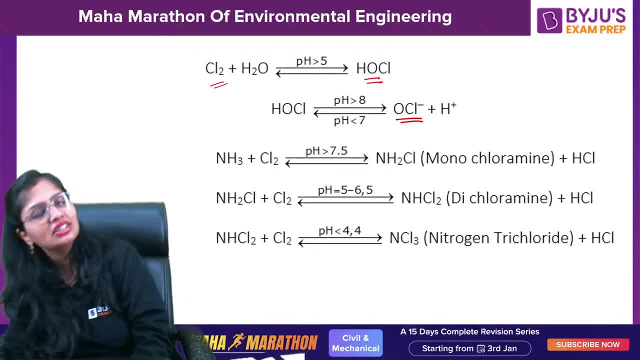 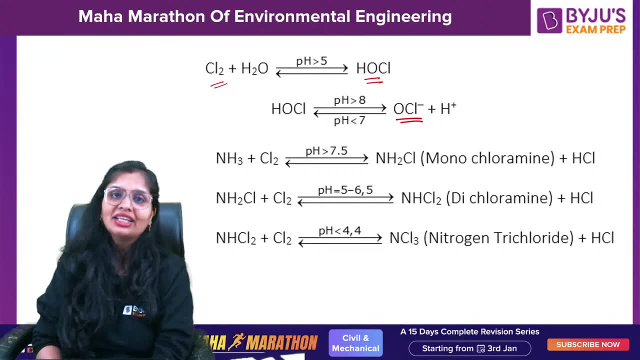 We don't go for acids and alkali, Because if you want acids to be used, the pH should be less than 3. If you want the alkalis to be used, the pH is greater than 11. So technically that is not the pH permissible by the government. 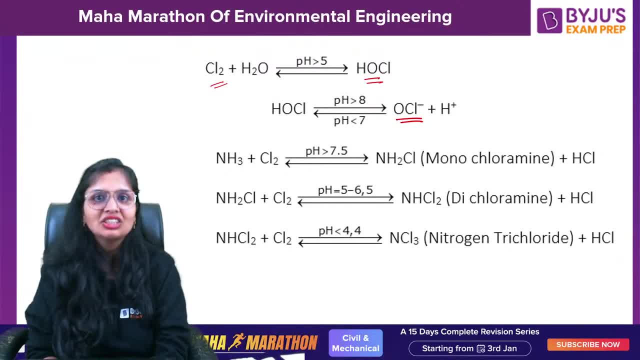 And remember, disinfection is the last treatment After this you cannot do anything After this water is supplied to the homes. So the last treatment, so you have to make sure of the, You have to make sure of the pH and oil. also Now for preventing against future recontamination. 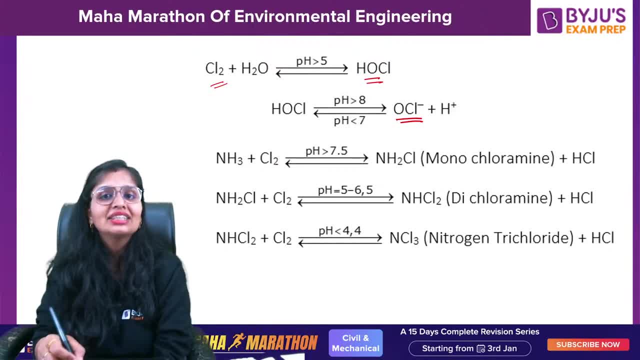 There is ammonia which is present, NH3. It reacts and forms chloroamines. So it reacts, it forms monochloroamine. Again it reacts with chlorine and forms dichloroamine. This is- pH is very important. Reversible reaction. you know the sign right, It is reversible reaction. 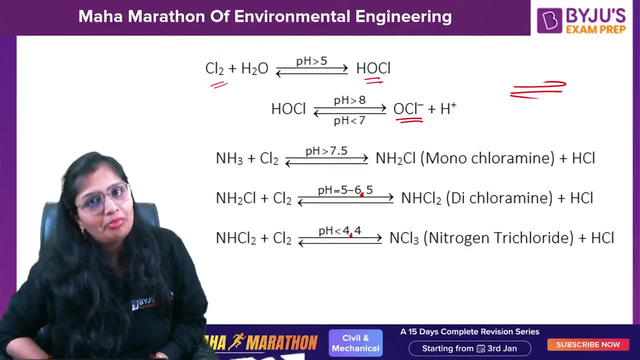 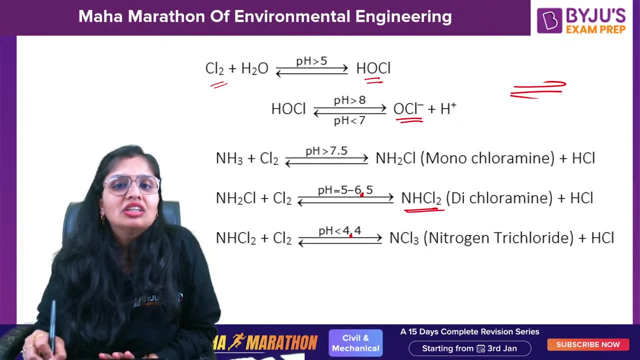 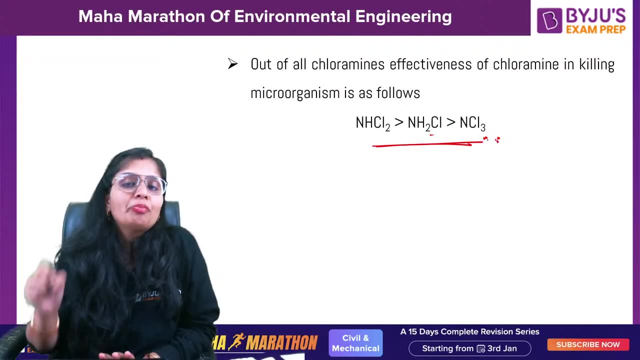 So it will move forward or backward. It will depend upon the temperature and pH. Okay, Next, coming further, If you ask me the effectiveness, The topmost is dichloroamines, Then monochloroamines, Then trichloroamines. So this is responsible for preventing the water from future recontamination. 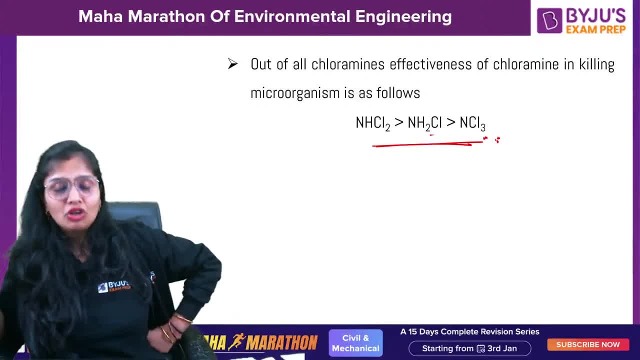 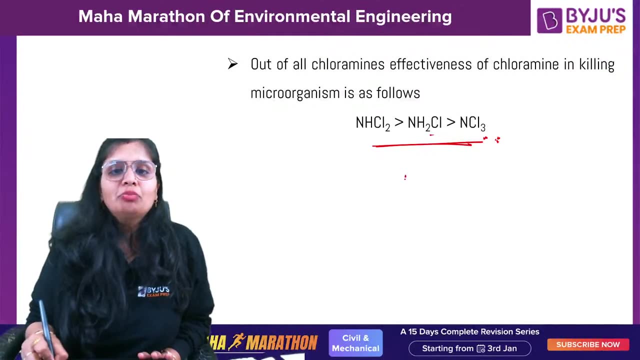 Because others were not given. Other types of treatment units were not giving you this effectiveness. Okay, They were not giving you this property of future recontamination saving. That's why we go for chlorine Now, Before we do this, There is a formula which is, Since you know it properly: 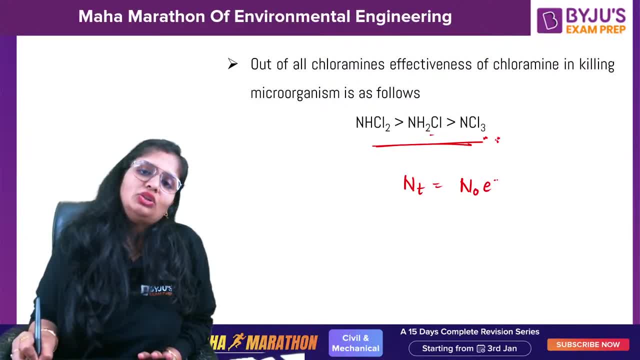 That is Fixed law. e to the power minus kT. N number of times questions in GATE have been asked in this topic. So whenever they ask you percentage removal, percentage scaling, That is N0 minus Nt, Is it? Or Nt minus N0 Into 100? 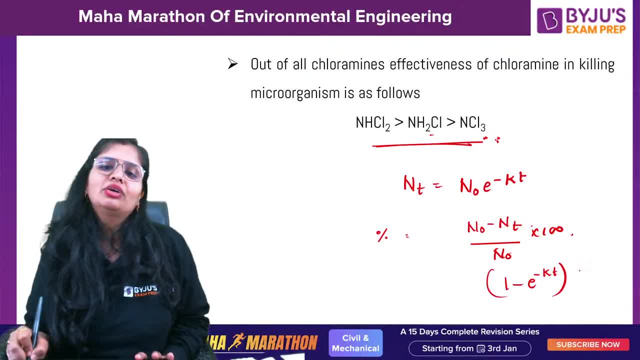 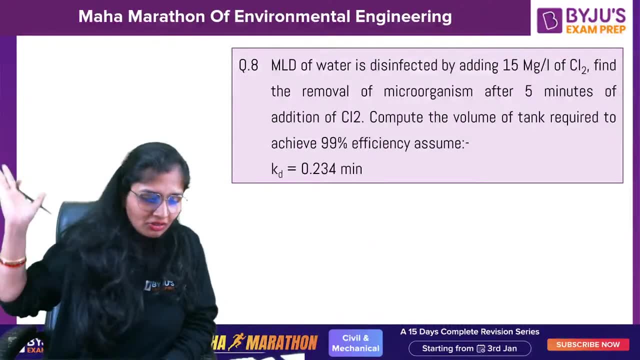 So how much it becomes? 1 minus e to the power, minus kT into 100. This is the percentage efficiency which you get. Okay, So now solve this question. This is very simple question. It has asked you to calculate the volume, Two things it has asked you. 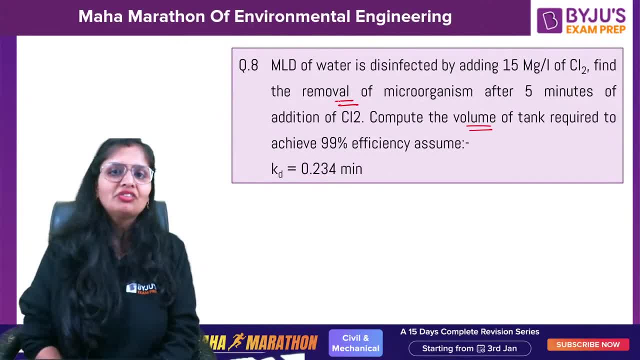 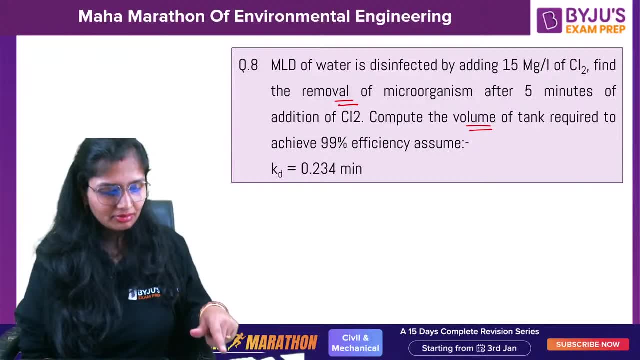 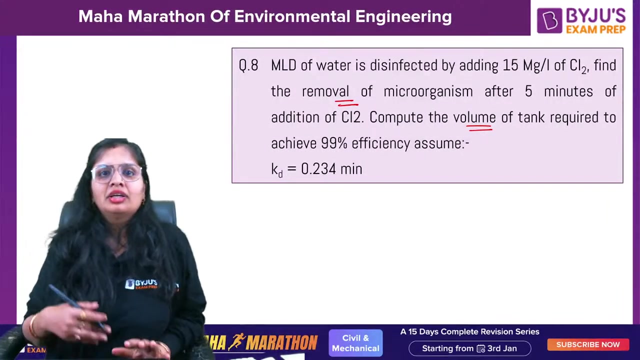 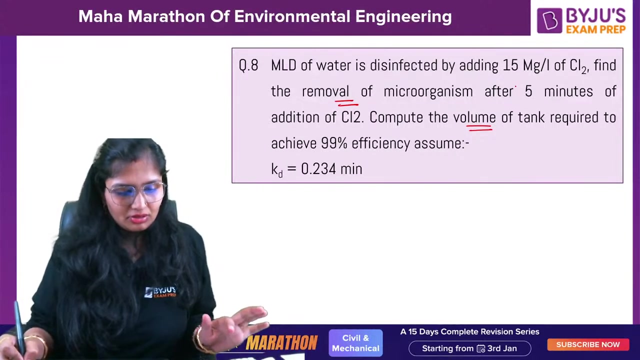 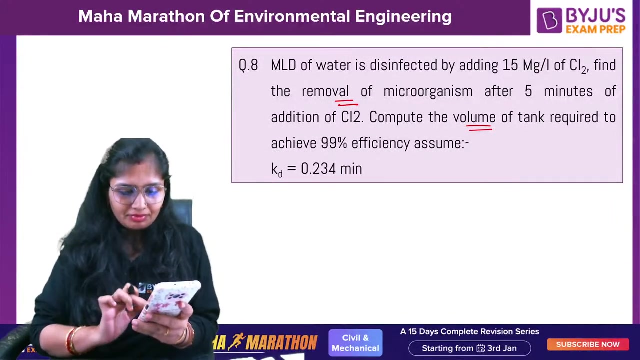 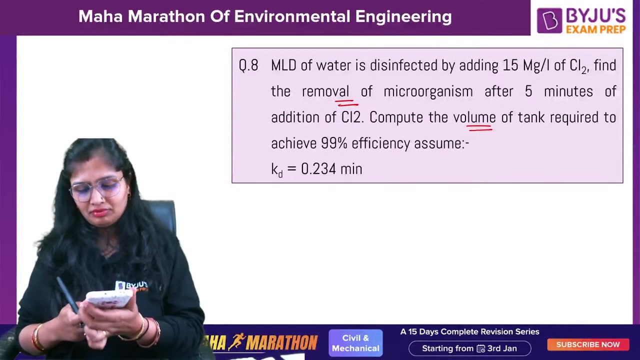 First, it has asked you find the removal of microorganisms after 5 minutes And it has asked you the volume of time. Come on guys, Come on guys fast. Come on guys, fast, Fast. Did anyone get the answer? I am very good at this. I am very good at this. 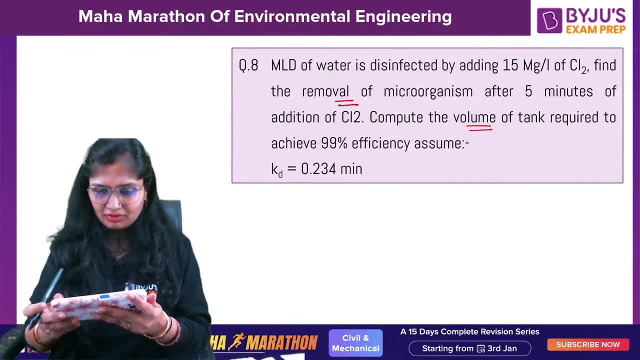 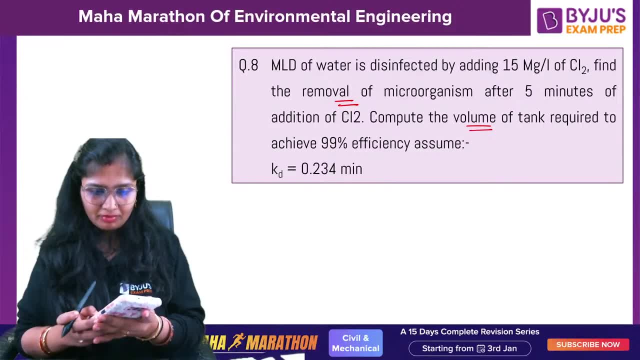 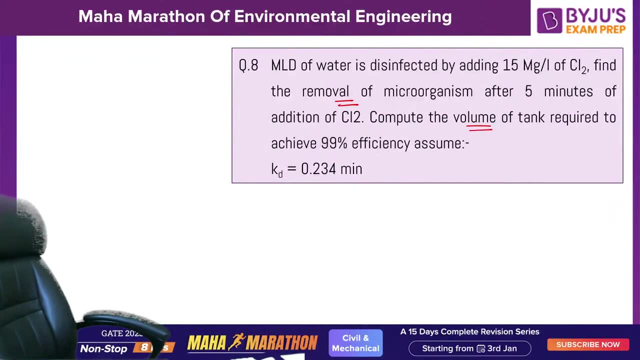 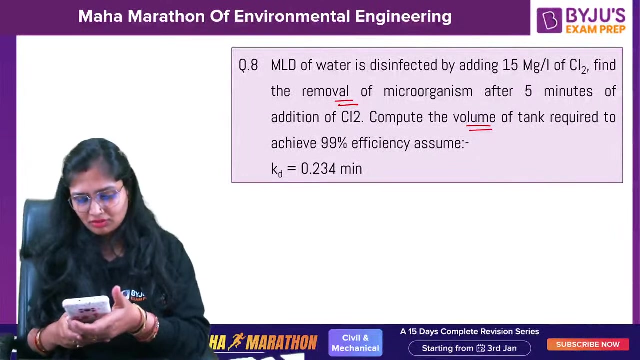 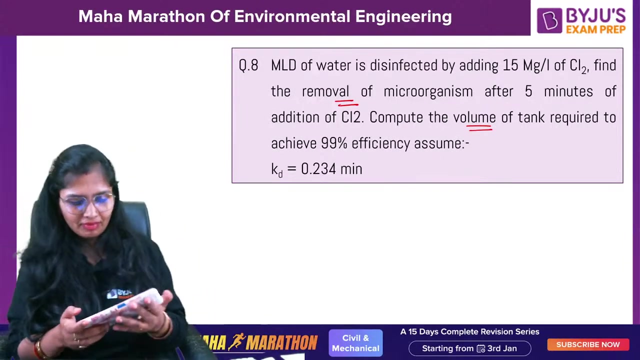 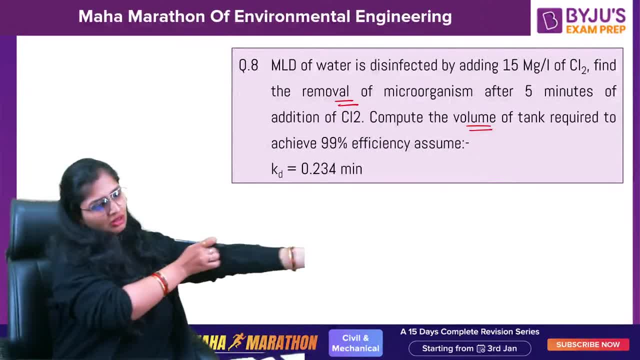 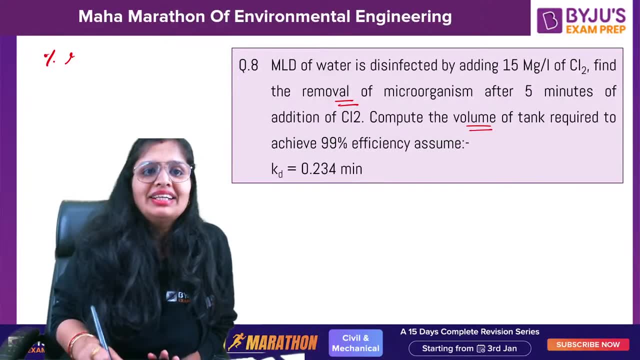 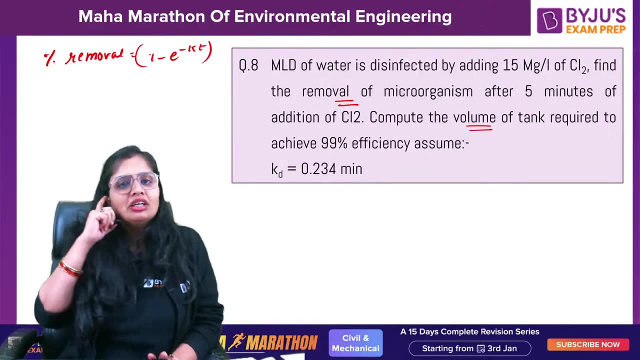 You guys are waiting for me to solve. See, Nobody answered till now. What is this Percentage removal? Already I told you 1 minus e to the power minus kt. So what is happening here? What is happening here? 8 MLD is given. 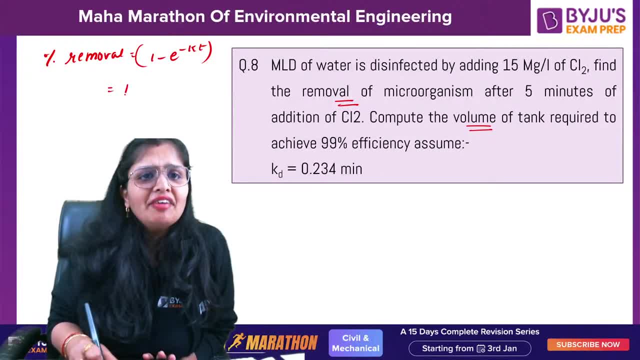 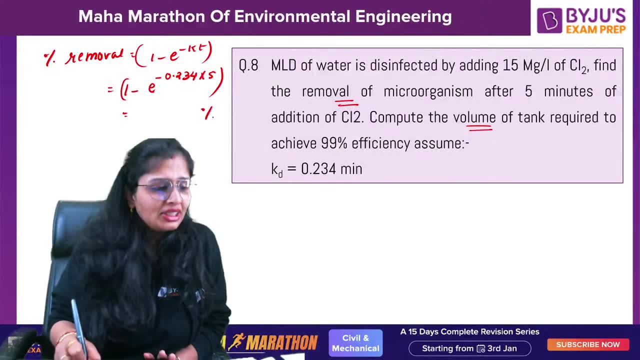 Find the removal of microorganisms. after 5 minutes, Everything is given to you What to do in this question. I don't understand 5 minutes, So tell how much it is coming 10.34.. How it can come 10.34?. 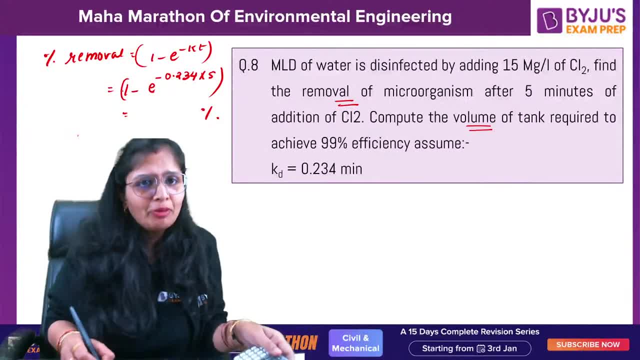 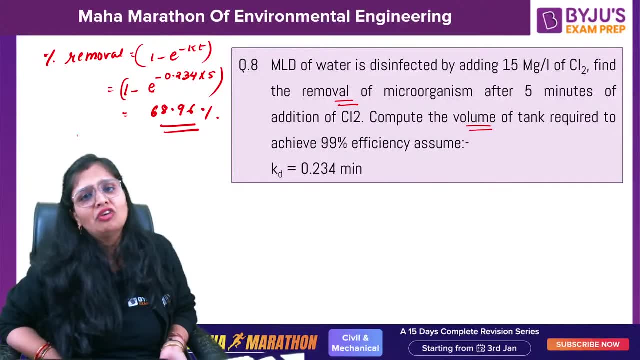 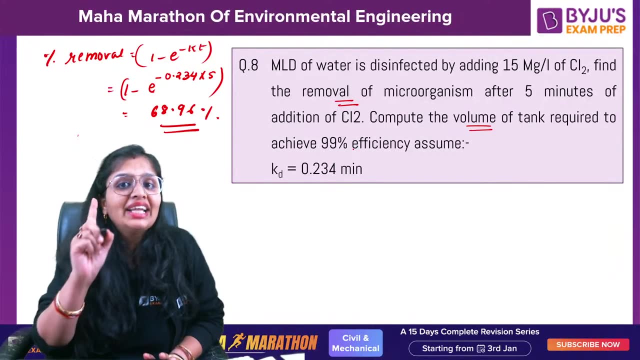 Simple: 1 minus This will come out to be 68.96 beta. It is as simple as that. This is the percentage removal efficiency. Simple, Just apply the formula. Next, in this question, it has asked you to compute the volume of the tank required to achieve 99% of the efficiency. 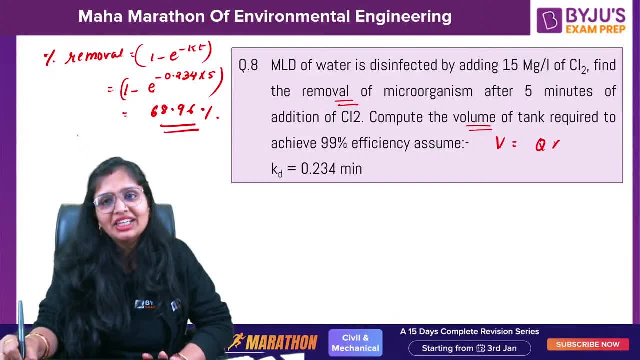 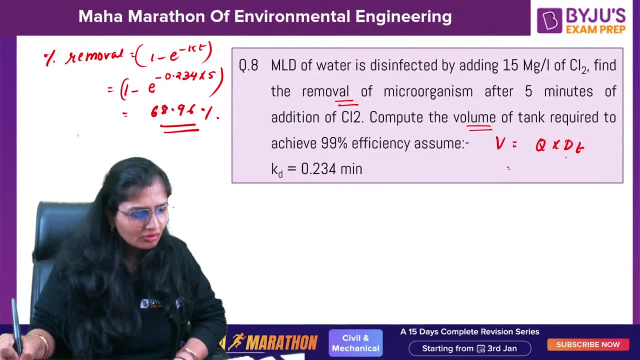 If it is asking you volume, that means discharge into detention tank. Discharge is given to you in the question is 8 MLD. What you are telling me In this question, discharge is not mentioned, or what? Take it 10 MLD. 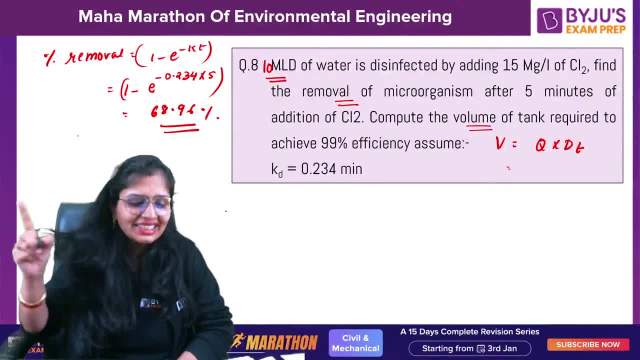 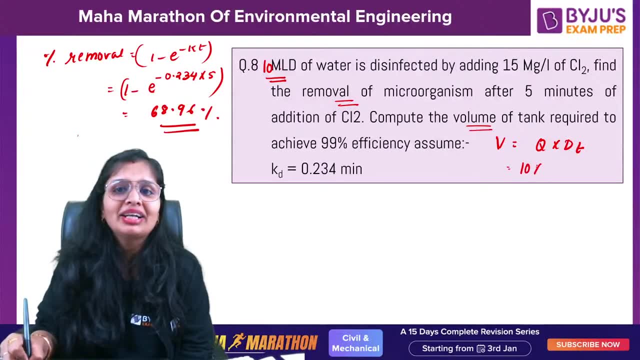 10 MLD- 0.689. it has asked in terms of percentage, So it becomes 68.9.. Now talking about discharge. Discharge is 10 MLD, that is 10 into 10 e to the power, 6 liters per day. 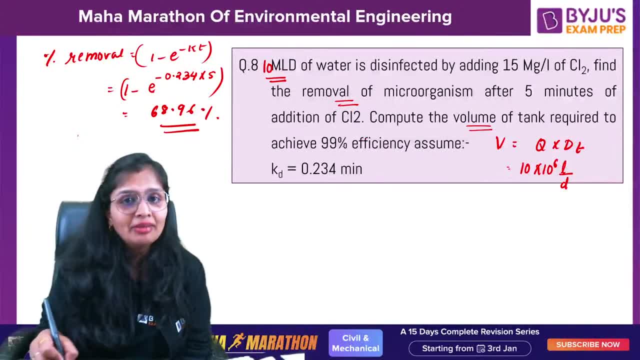 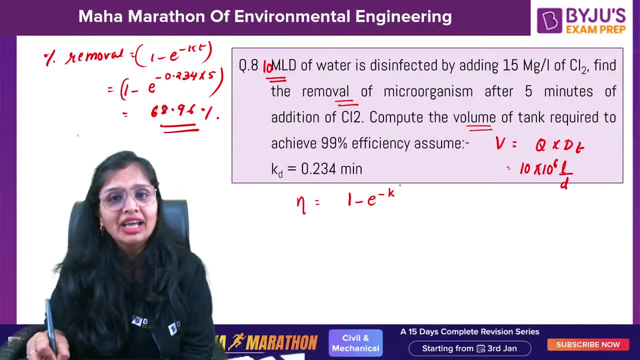 You need only detention time. Time you can calculate Because efficiency is given to you in the question. this time See any type. this way, question can be asked, Reverse question can be asked. So the efficiency is 99%. You can write 0.99.. 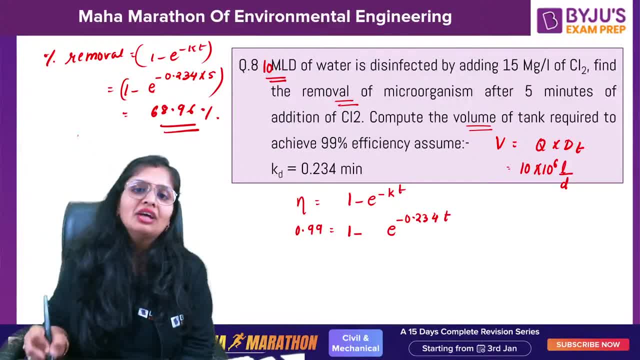 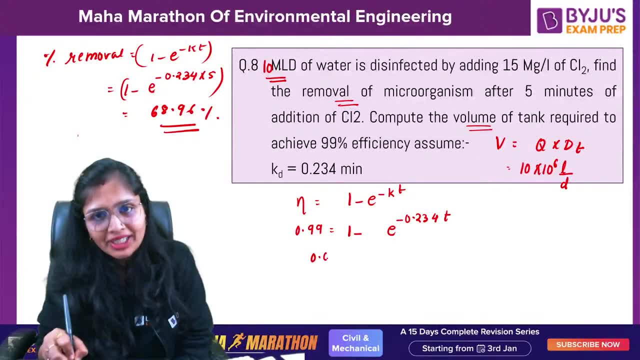 Okay, This is given to us 0.234 into t, Since if anything is there in the power, you have to go by what you have to go by log. So 1 minus 0.99 is 0.01 e to the power minus 0.234 t. 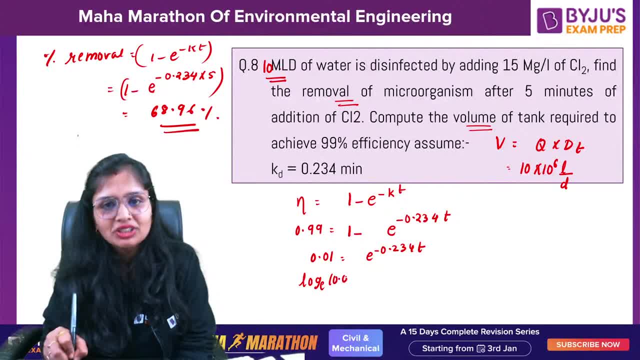 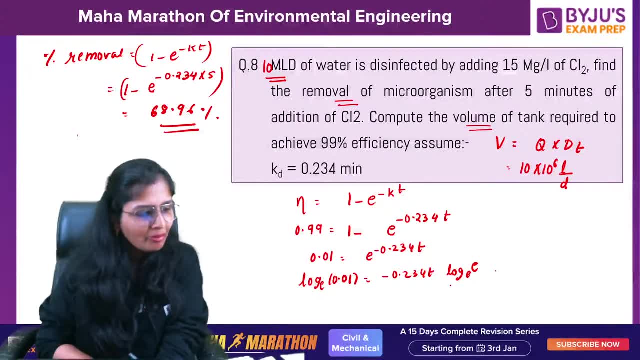 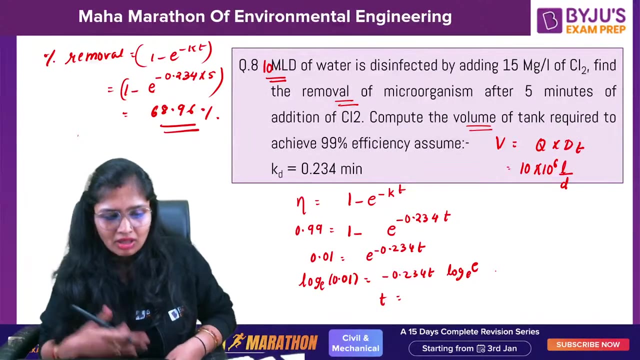 So take log on both sides: Log basis 0.. 0.01 minus 0.240. log e basis: How much it is coming Time comes out to be how much 50. you are telling What answer? you are telling 50?. 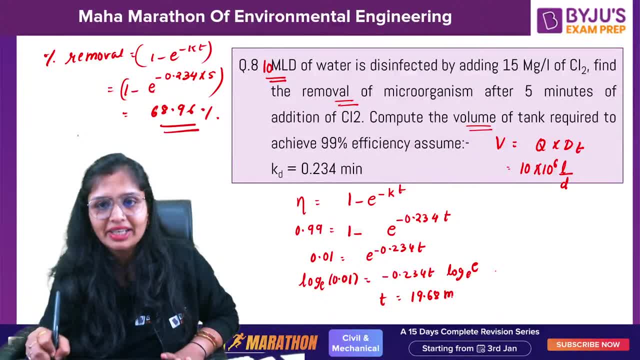 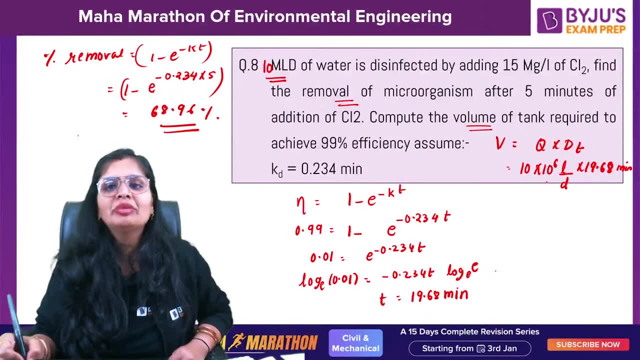 Very good, Sabrita. 19.68 minutes Correct, So 19.68 minutes, 19.68.. So convert days into minutes: One day is equal to 24 hours, One hour is equal to 60 minutes And convert liters into meter cube: 10 raised to power minus 3 meters. 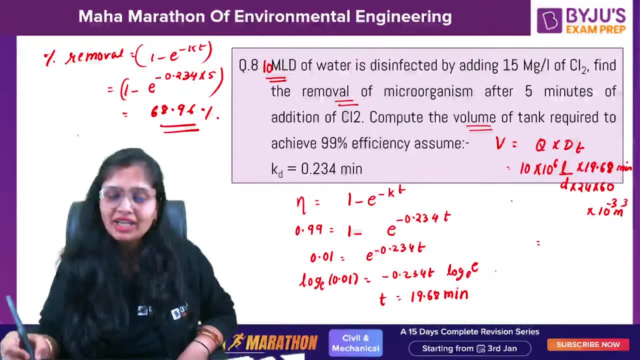 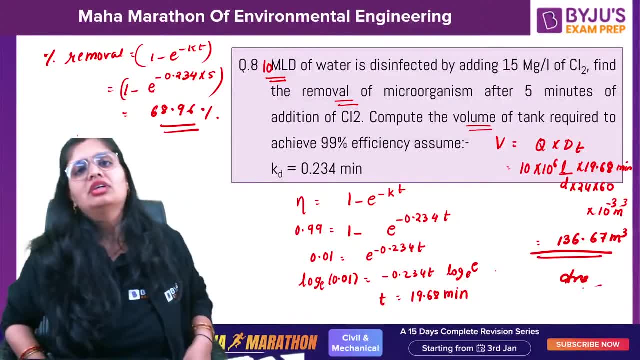 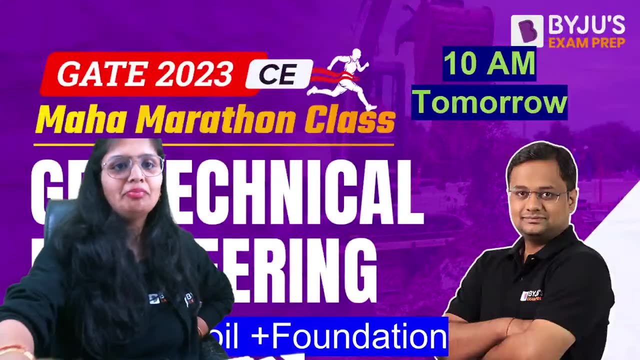 You will get the answer 136. Correct, Very good, Devanshu, 67 meters. So this will be the volume, Simple. So such sort of questions are being asked, Okay. So with this We complete geotech marathon already told you. 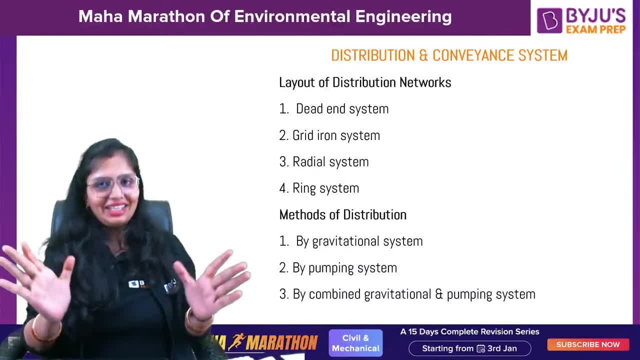 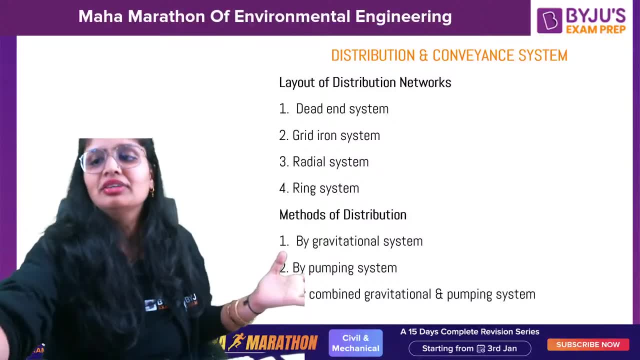 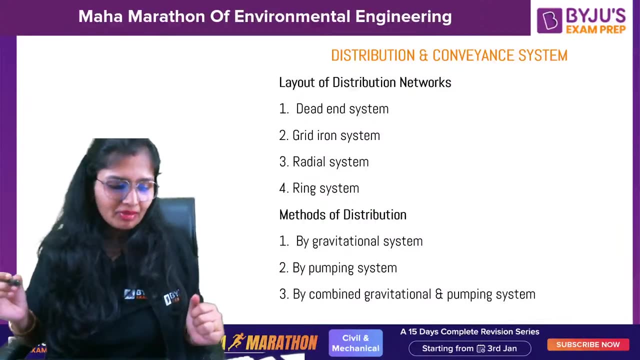 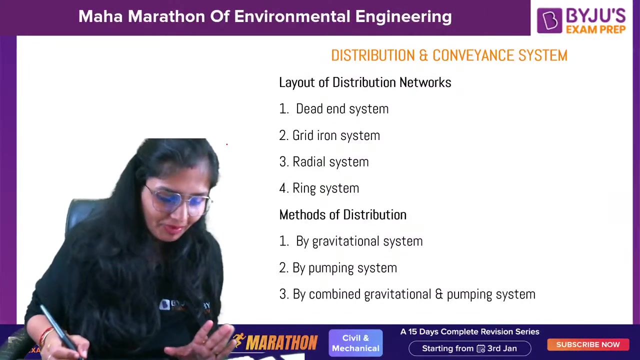 With this we complete our treatment. Shall I do distribution, and then we take a break. It will take hardly 20 minutes Shall we do it. Arun, Girish, everybody Pratiksha, Okay, Fine. So now, lastly, in this raw water part, we have distribution and conveyance system. 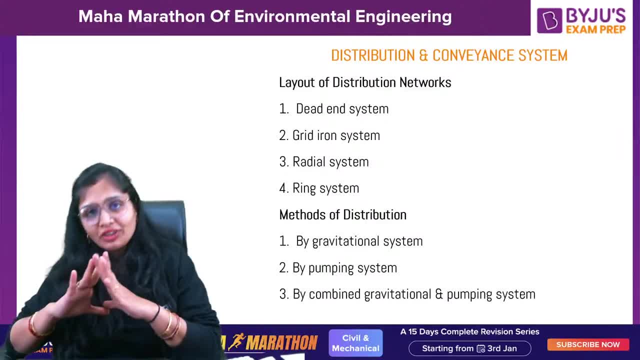 Distribution and conveyance system. So generally, when you lay out the distribution networks you have dead end grid, iron, radial and ring system. Whenever you take any distribution system, you make sure that you don't with laying of pipes and all are there. So generally it should be economical. 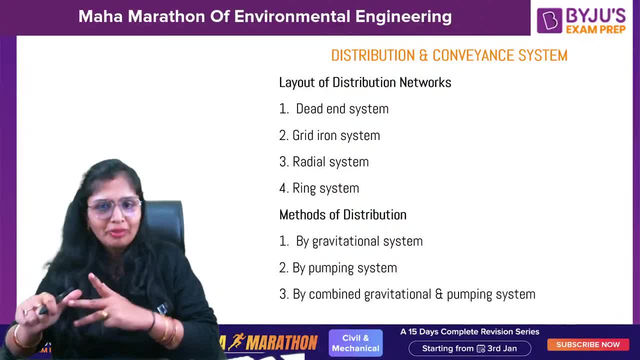 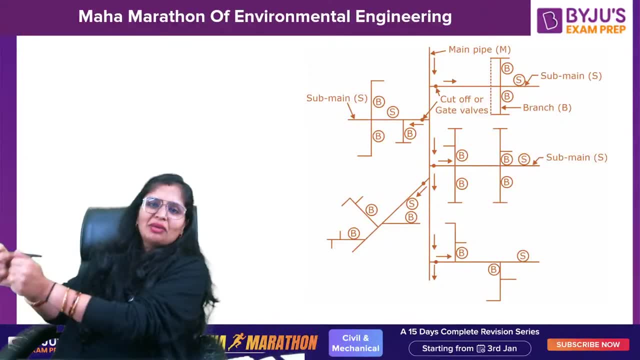 Laying should be cheaper. All these conditions, you have to make sure. So now this is first the dead end system. Dead end, no logic, nothing. You made your house connect the pipe. You made your house connect the pipe, That's it. 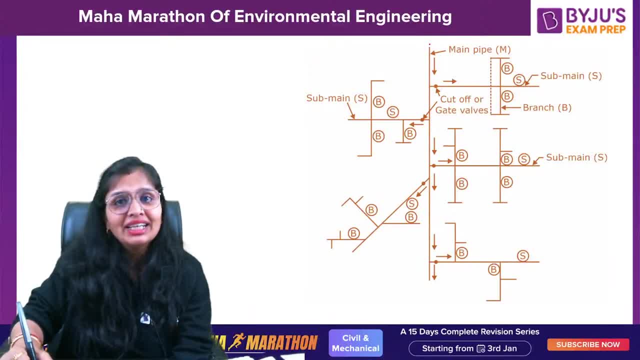 No brain is applied, Okay, So you can see it here. There is a main pipe, Okay, And these are the sub main pipes which is there. These sub main pipes are there. From the sub main pipes you can see there are branch pipes which are there. 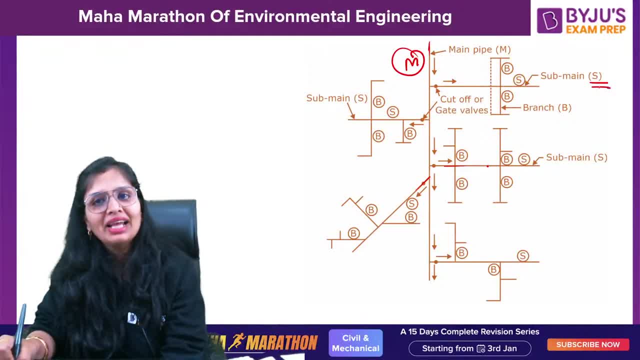 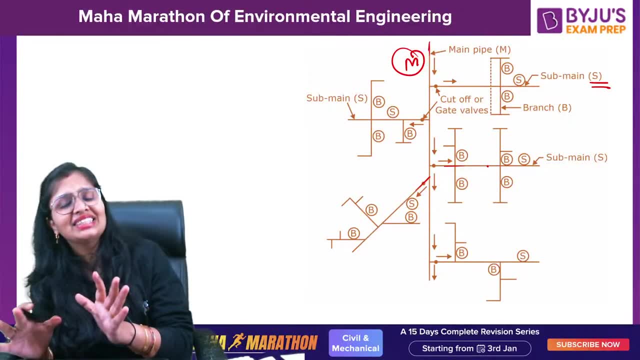 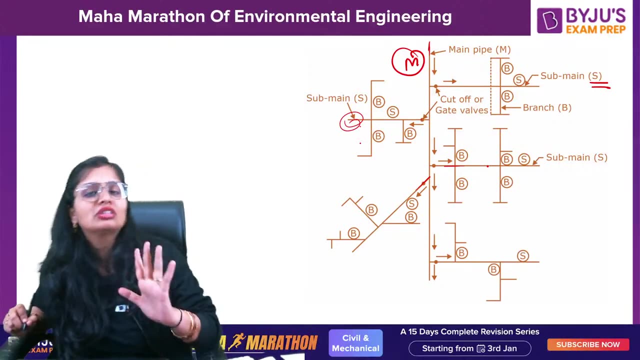 So this is main pipe M, Then sub main pipe S, Then branch pipe B. So what is happening here is What is happening here is. by any reason, if this pipeline goes for maintenance work or failure, this portion of people will not receive water. 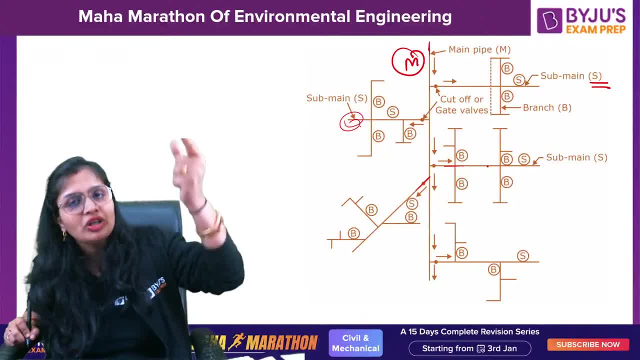 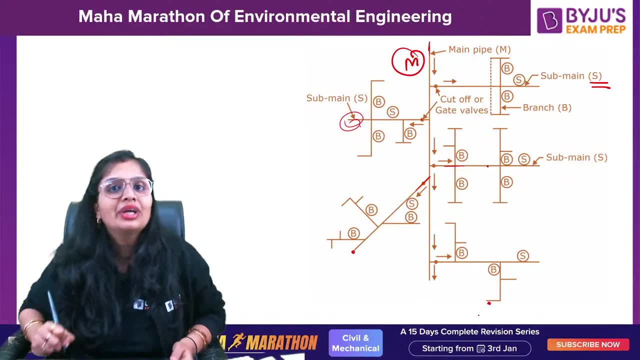 If outbreak of fire is there, you have only one route, so you cannot divert the flow of water also, Moreover, these are dead ends. These are dead ends, Okay, So stagnation of water can also take place. There is no free circulation of water. 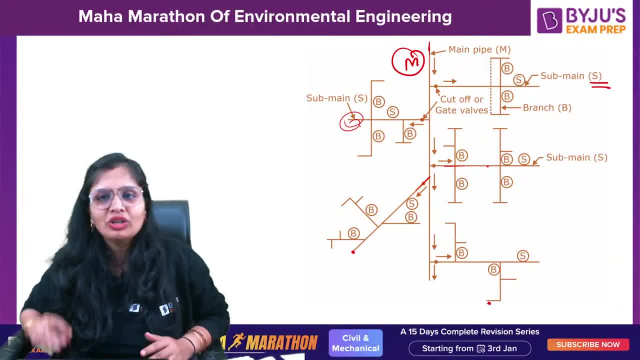 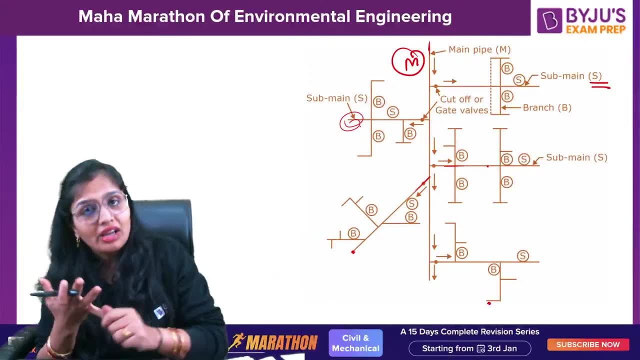 So there are n number of drawbacks which you get it. Yeah, Circulation of water is there. Single, No brain to be applied. Nothing regarding head loss, Just fix it, That's it. But emergency cases, outbreak of fire, nothing it can maintain. 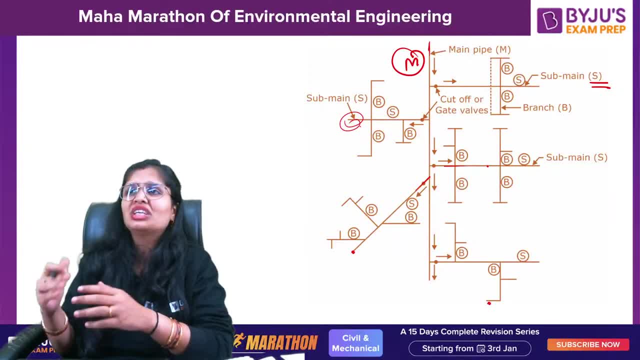 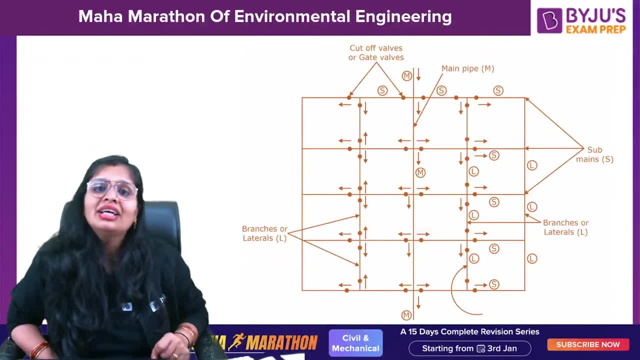 And that is the reason. dead end system is for old cities, Those cities which were not properly planned There. you will see these systems. Now you tell me which is this system. This is grid iron system. Generally, you will see it in development. 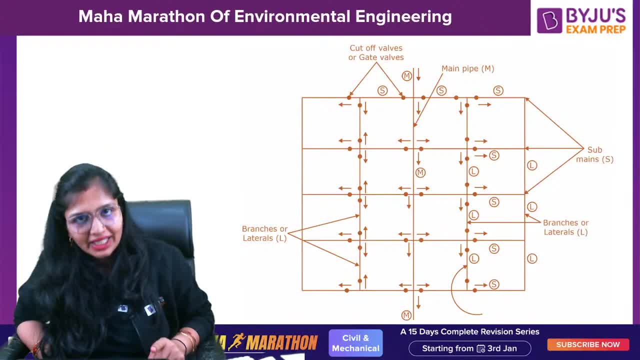 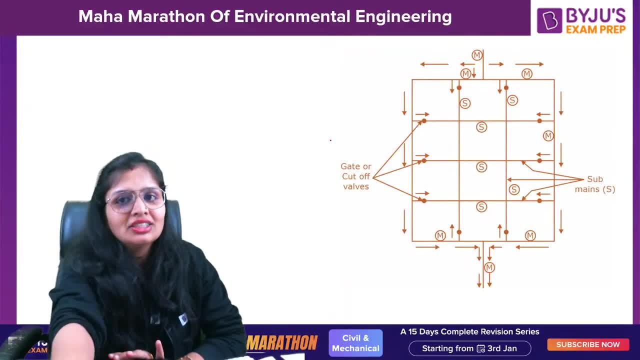 You know, Chandigarh is the first planned city. So in those planned cities and all you see this types of things, There will be a main wall. This is cut off wall or this is one, The grid iron system. Which one is there? 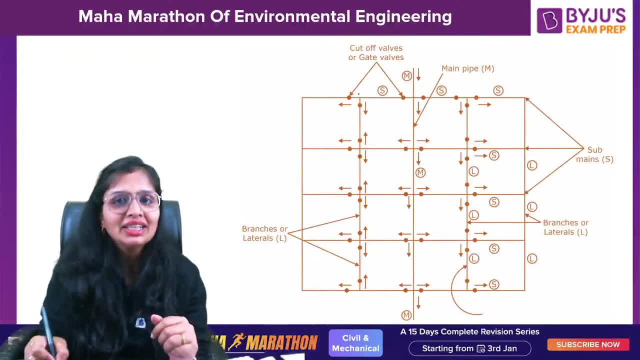 This one is there. Okay, Now, what happens here? These are cut off walls. I will tell you about the walls Right now. I will tell you this: gate walls are used to regulate the flow of water. Okay, So now what will happen here? 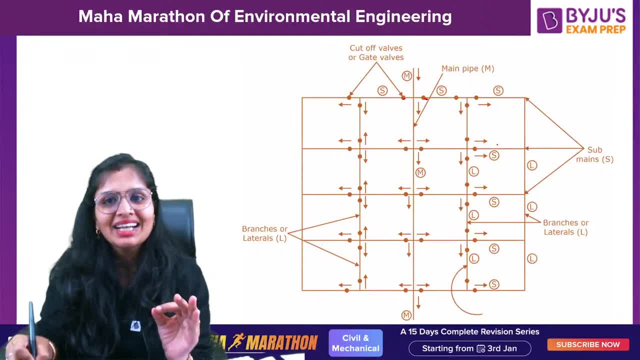 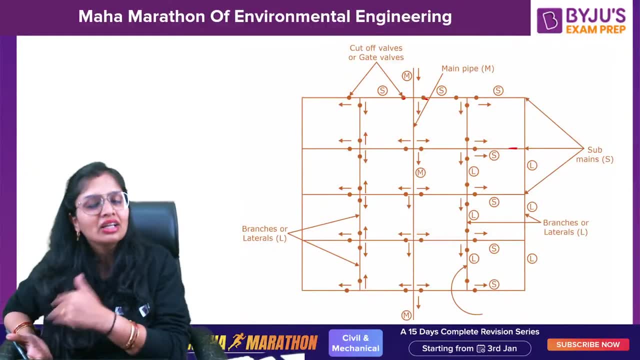 Now what will happen here? Here You can see that if any case the water does not come in this position, You can divert the flow from any other positions. Okay, Laterals are there. You can adjust it in that manners. If fire outbreak is happening, you can divert the flow in that position. So all several drawbacks was there in the dead end system. It is eliminated in grid iron system and ring system. Okay So ring system, you go for. You go for grid iron system, And in both of the cases All the drawbacks are there. 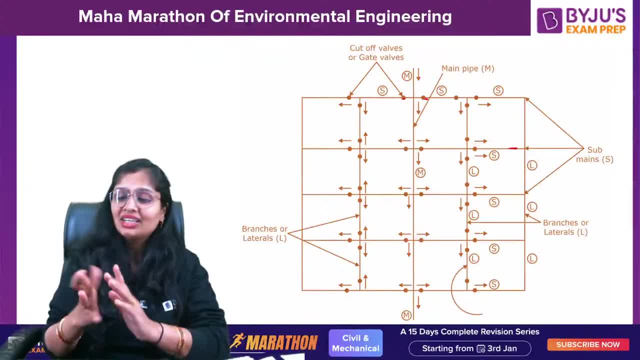 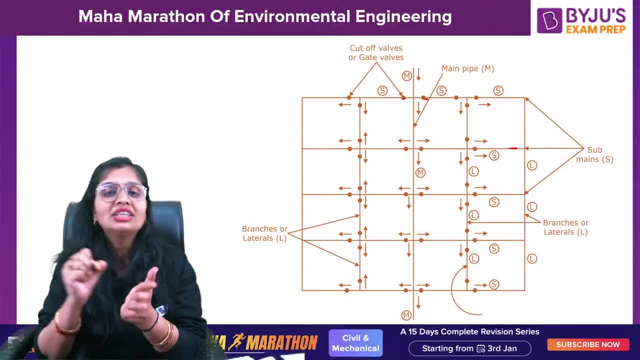 All the drawbacks of dead iron system was eliminated, But this process is costly. You need to calculate how much head loss will be there at each and every positions. All these things you need to do it. Moreover, if you see that large number of radial roads, 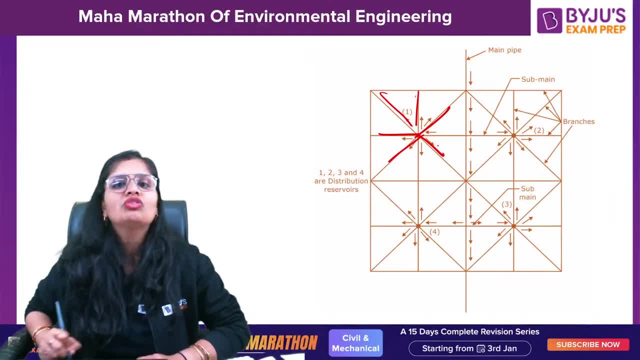 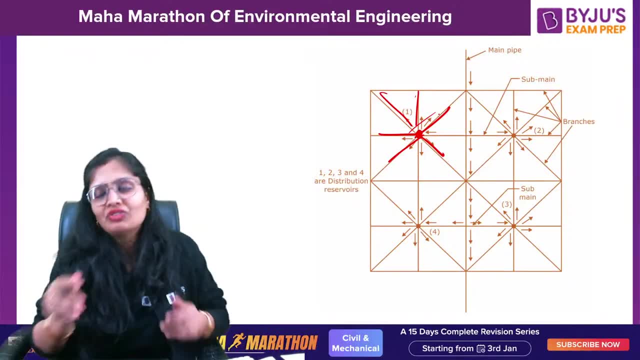 You can see, These number of radial roads are there. So what you can do, You can install a service reservoir here So that the water can be provided to all these, Because wherever roads are there, Their sides houses are there, They will be supplying it. 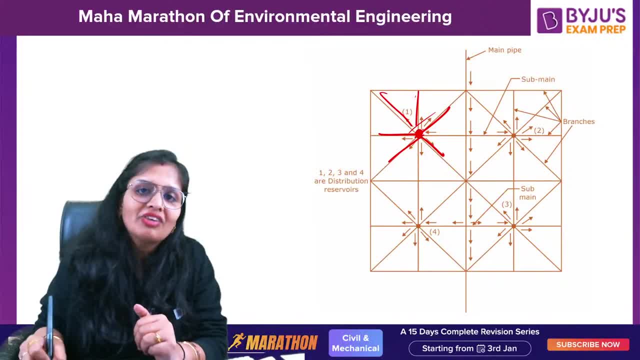 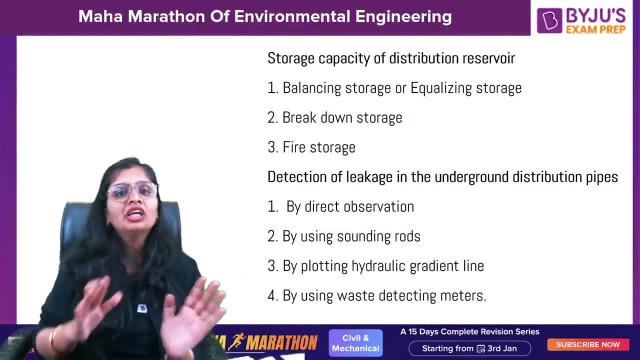 So you install a distribution reservoir at the intersection. As simple as that. That's it. Now talking about the storage capacity, See, three things are there: Balancing storage, Breakdown storage, Fire storage, Fire storage: already told you Breakdown storage in case of failure of pumps. Emergency cases, Generally 25% of the total storage capacity, Or 1.5 to 2 times Of the average hourly supply. See generally what happens in case of failure of pumps and all. also You get the water from the service reservoir. 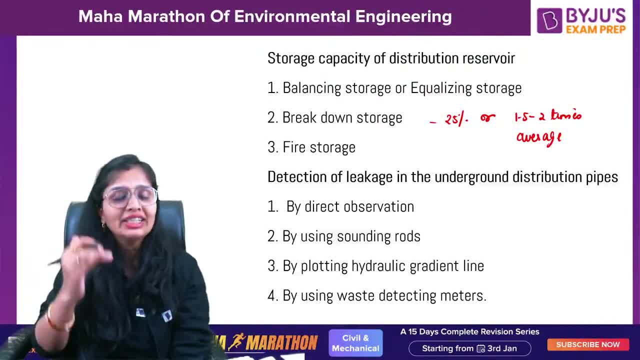 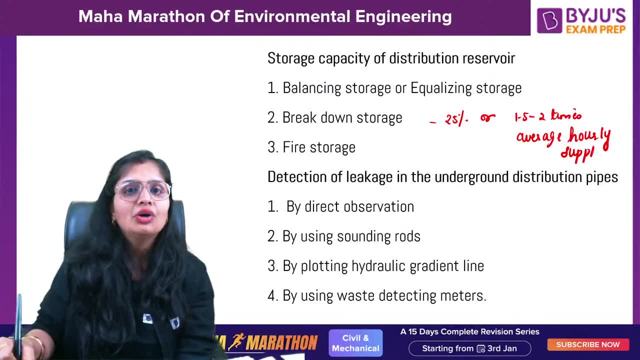 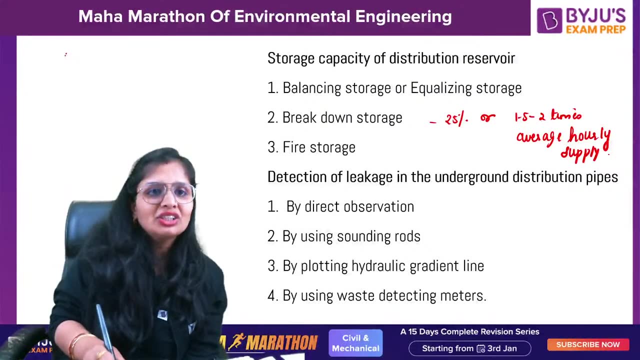 Because, for safety purpose, for all these conditions, Certain amount of water is stored in the reservoir. Okay, Now let me talk about balancing storage or equalizing storage. Balancing storage or equalizing storage is: Let us suppose The supply is constant. 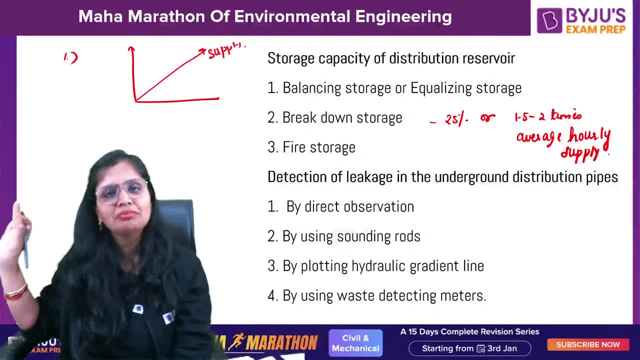 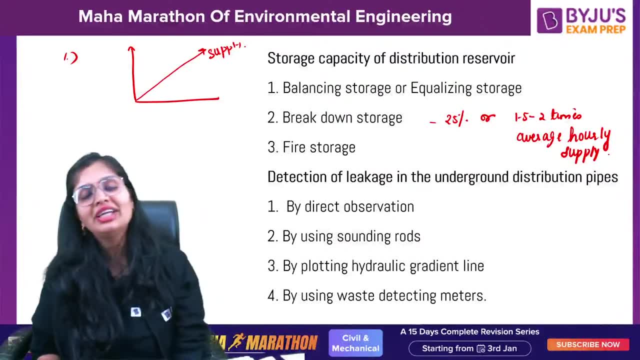 Supply does not vary. It comes at a simple rate. It will come that. let us suppose 10L per minute water is to come. It will come in that rate. But Like Arun said, He took a bath with 8L of water. 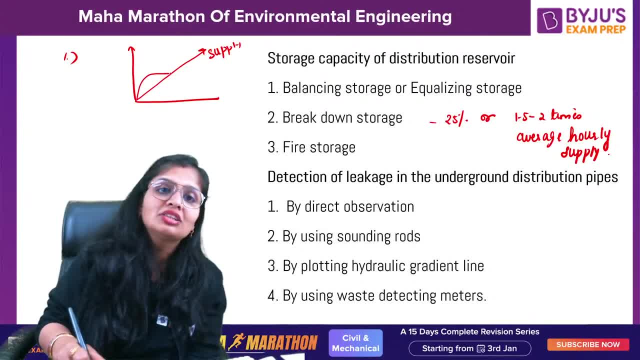 So his demand was more. Some doesn't have To take up water, So their demand is less. So the demand fluctuates. So in this case, Balancing storage tells you The storage in the service reservoir should be there. Okay. 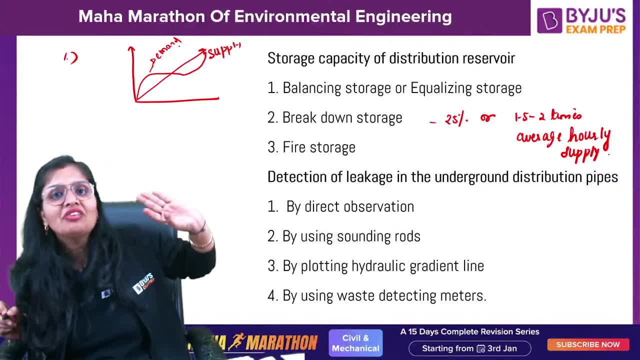 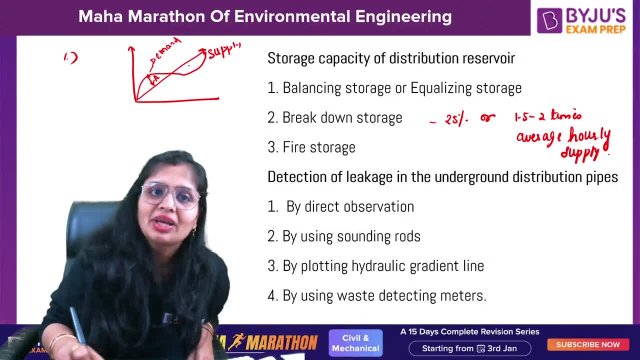 reservoir should be such that it should balance the variable demand by maintaining the constant supply. So here you see, demand is more, supply is less. Here supply is more, demand is less. So you take a mod of it, mod A plus B, That means maximum depletion plus maximum accumulation. 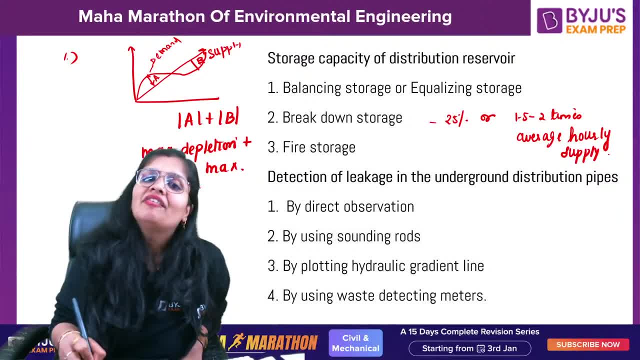 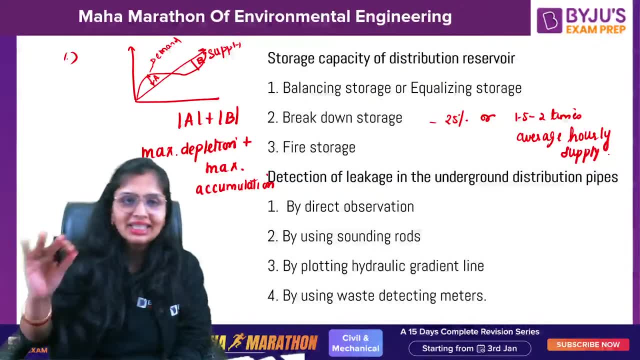 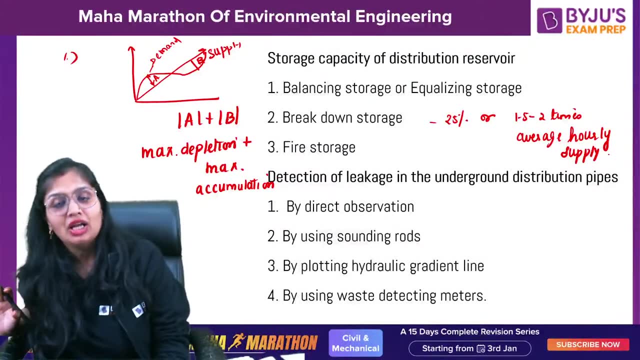 Accumulation will happen when supply will be more. depletion will happen when demand is more. Okay, So this: you have to balance the variable demand against the constant supply of water. Now, these names you should know after this, Whenever you want to detect leaks and all. 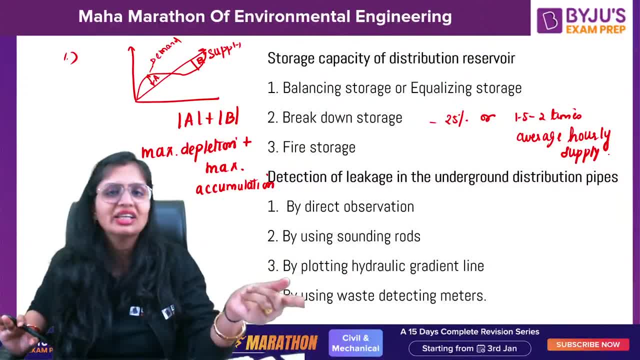 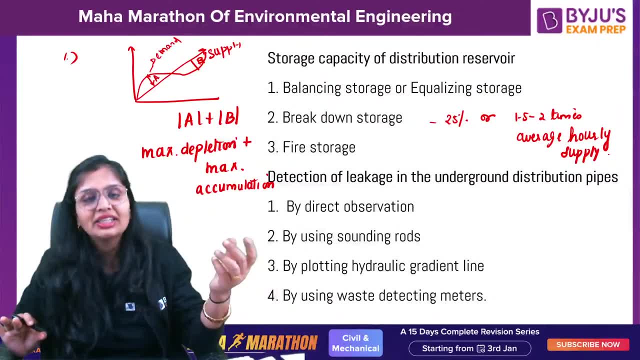 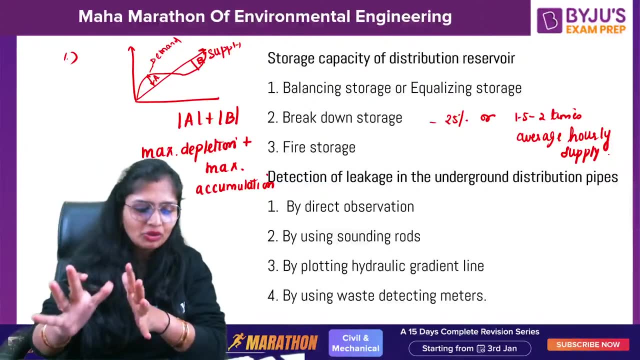 if you see a sand is there and you see wetness is there, you can clearly say that yeah, here leakage of pipe has happened. Or there are ways, detecting meters, and all are there. Sounding rods are there which will tell you that if sounds comes, that means the leakage is taking place. So these names you should know. 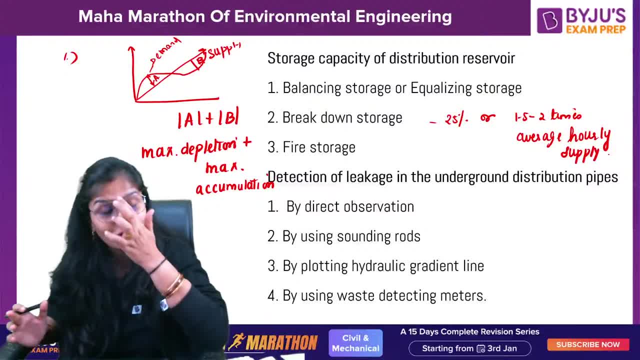 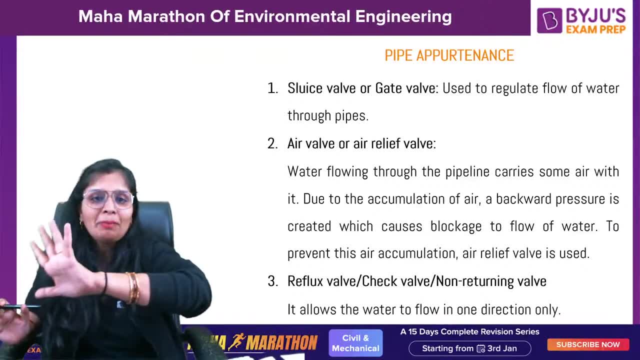 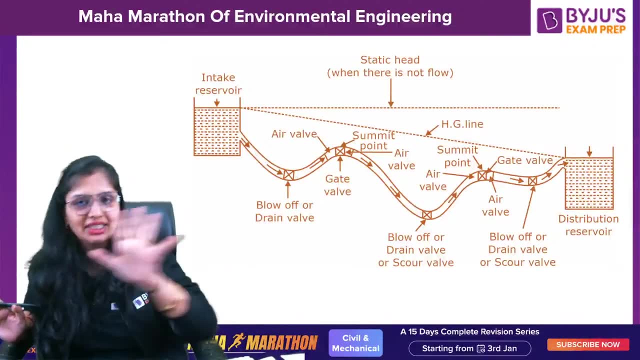 in case they ask you, Very cold weather and that Then do you bath with eight buckets of water. hats off Arun. Okay, So these are the pipe apprentices. Maximum four, five apprentices are there, which you need to remember, which is very much important. That's it. That's it First. 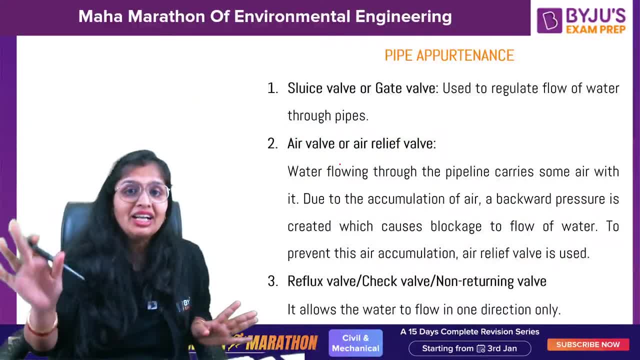 is gate valve. See, very, very important. I'll tell you, Remember the alternative names of it. They can ask you in: one marks portion, Don't lose it, This is cut shot. They can ask you in match the fault and they can ask you in any way: Squeeze valve, gate valve or you call it as cut off. 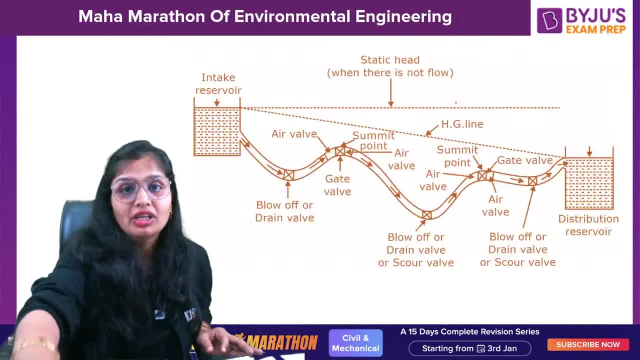 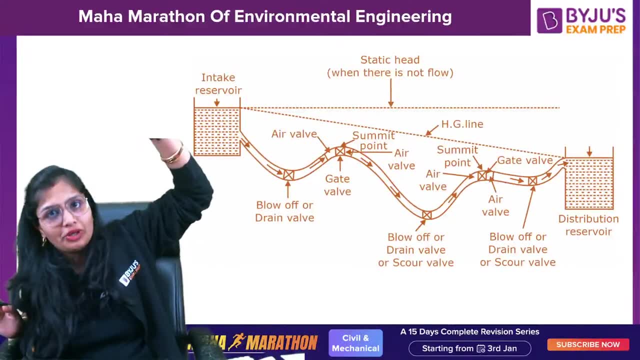 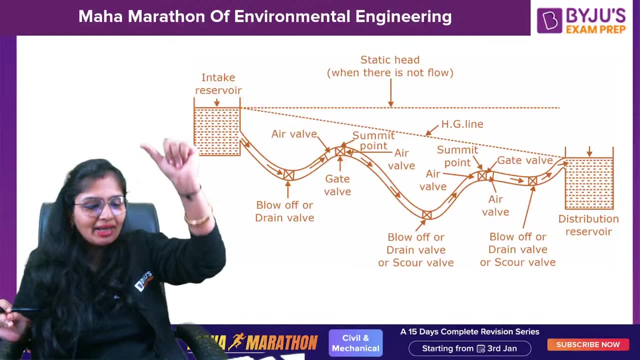 The function of it is to regulate the flow of water. These are manually operated. Secondly, these are placed on the summit point, That is, the crest point. Okay, The topmost point. Now, why they are placed at the topmost point? Because the pressure at that position is very late. 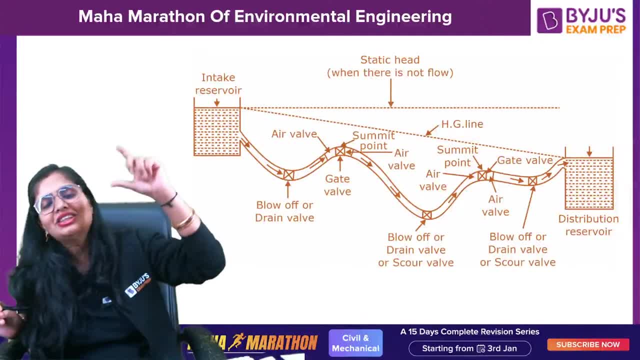 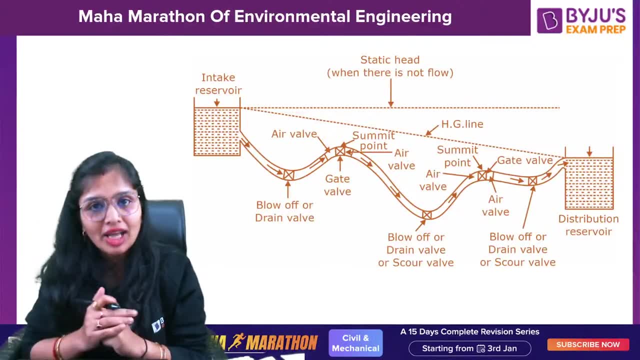 Prem. how could I know? The pressure at top point is less? Moreover, whenever the proper regulation is not happening, whatever water hammer effects happens, this gate valve prevents the pipe from it. Next is air valve. Now, two things are there. Air valve is for the air valve. Air valve is for the air valve. 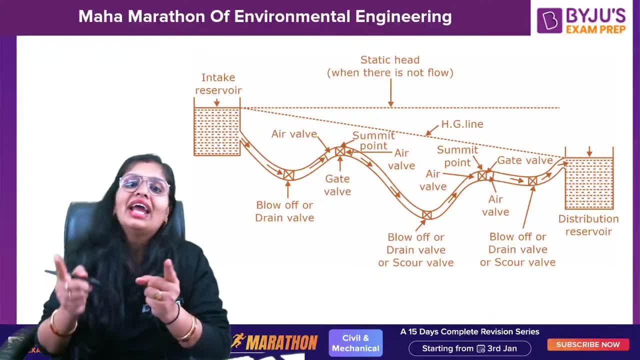 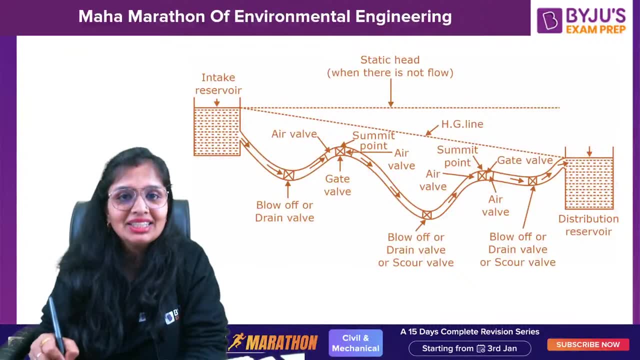 It is placed on both the sides of the gate valve. Air relief valve is there and air inlet valve is there. Both valves are there. So can you tell me this is air inlet valve or air relief valve? Air inlet valve is there or air relief valve is there? 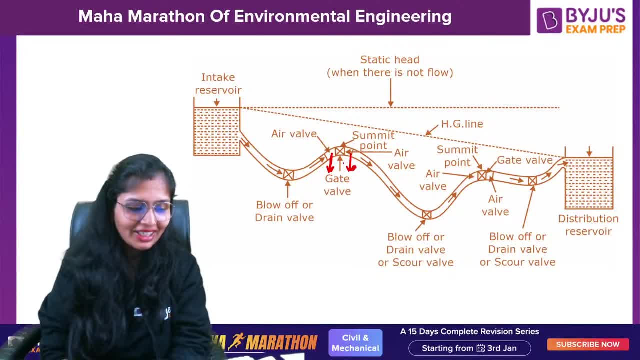 Good afternoon, Abhinav sir. Abhinav sir is also there. Yes, sir, Lecture is tomorrow at 10 am. Geotechnical lecture. Air inlet valve or air relief valve. Guys, we have two valves right. 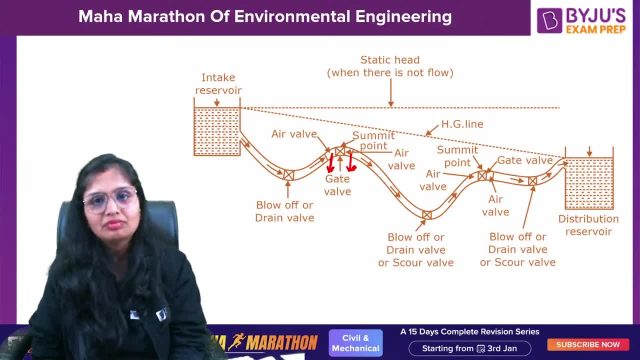 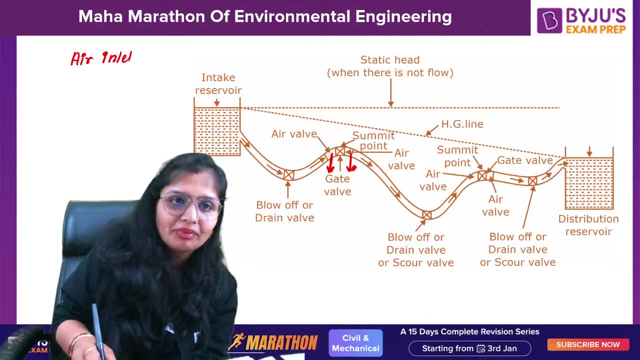 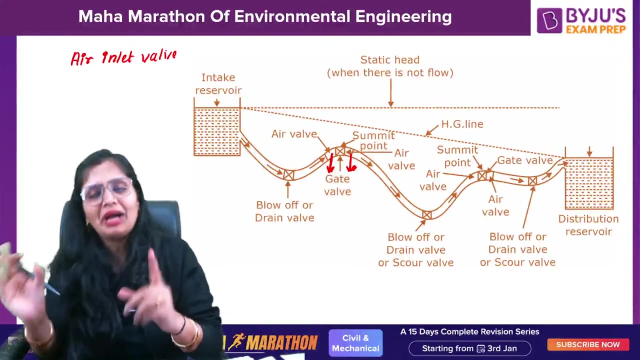 Air inlet valve or air relief valve. Inlet or relief. Guys, fast, fast, I'll tell you first the difference between the two, so that you can tell me the correct one. See, now we design the water for the pressure of pipe. Okay, For the pressure of pipe. 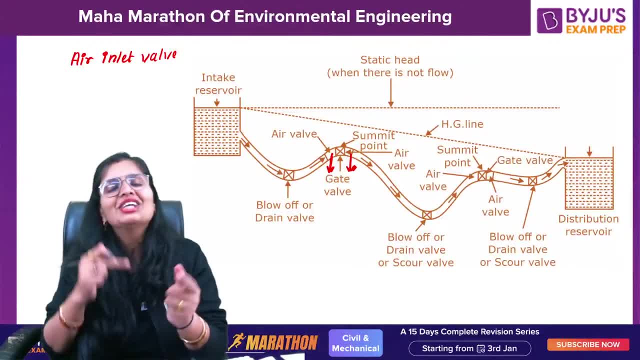 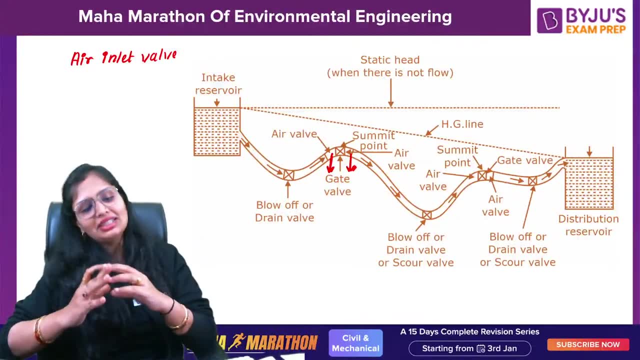 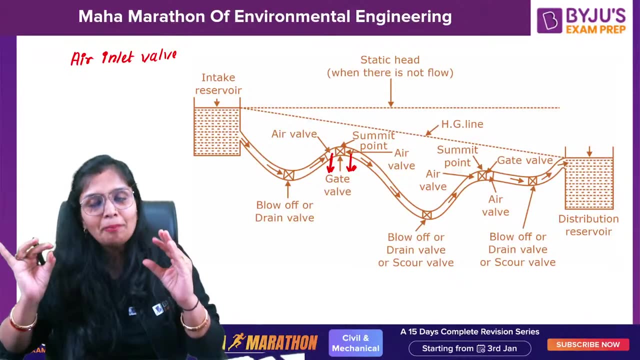 basically, we design the pipe for the pressure of water. I said the opposite. So we design the pipe for the pressure of water. We never design it for air. So now, what happens? Now, what happens is by any reason. by any reason, if you see that the water or the pressure inside the pipe falls below. 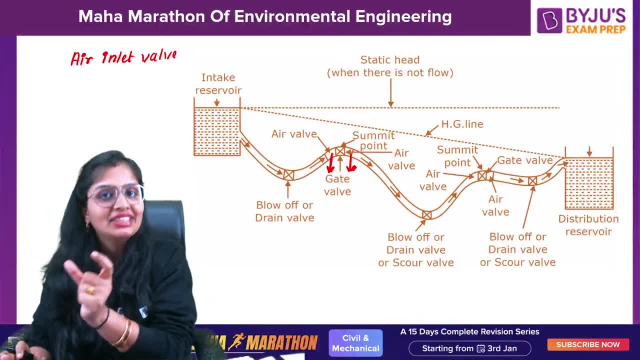 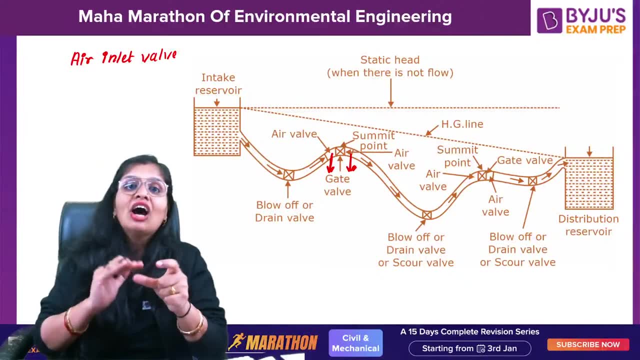 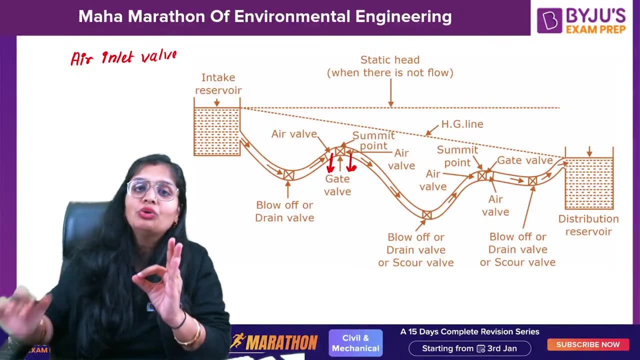 a certain predetermined value for which you have designed it. So if the pressure in the pipe falls below a certain predetermined pressure, then or you can say a negative pressure is created. So, in case a negative pressure is created, what do you need to do? You have to bring the 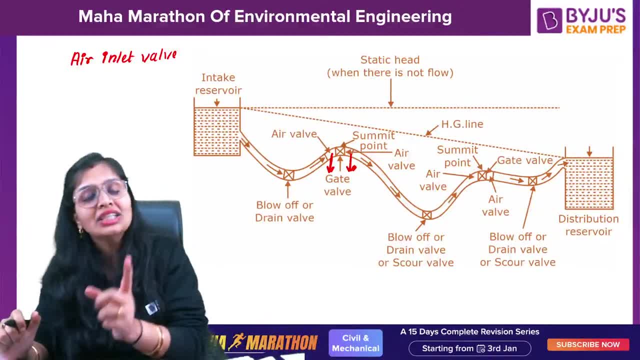 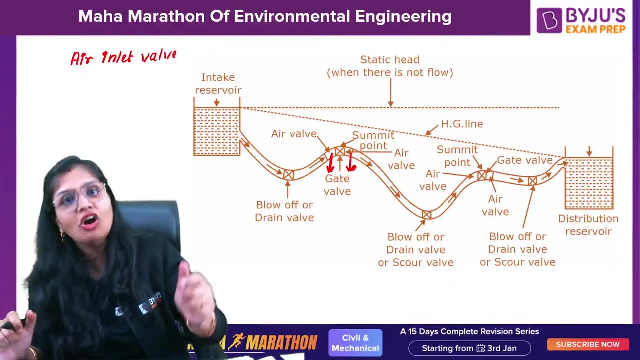 the atmospheric air pressure into the pipe so that that negative pressure can be compensated. Okay, If it is not done, then crushing failure will take place. Now, coming to air relief valve, If pressure of air in the pipe is more than the predetermined value of the pressure, 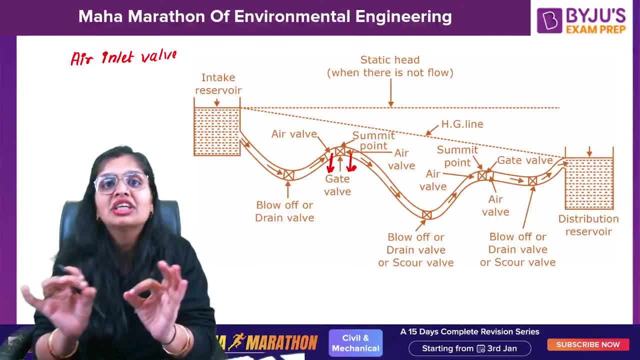 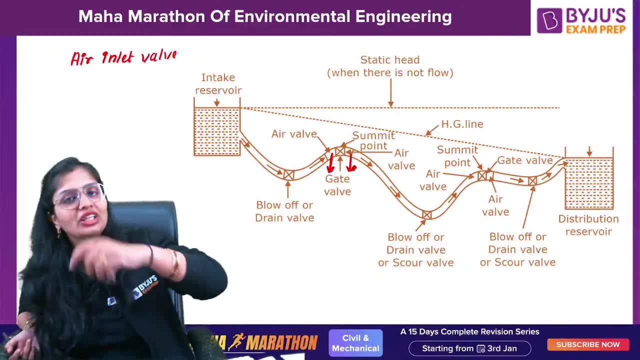 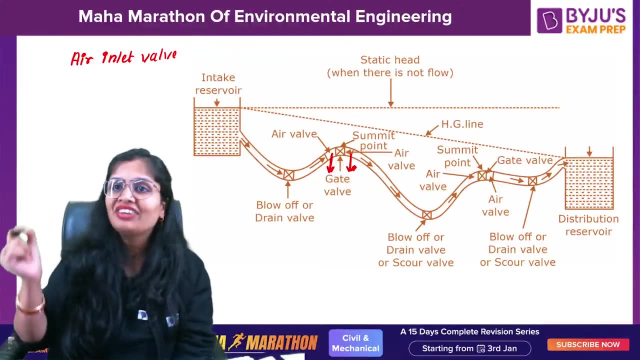 and if you don't remove that pressure, bursting of pipe can take place. And that is the reason you need to provide air relieve valve. Relieve valve is for the release of pressure, air inlet valve for bringing the air into the pipe, Because if negative pressure is there, vacuum will be there. 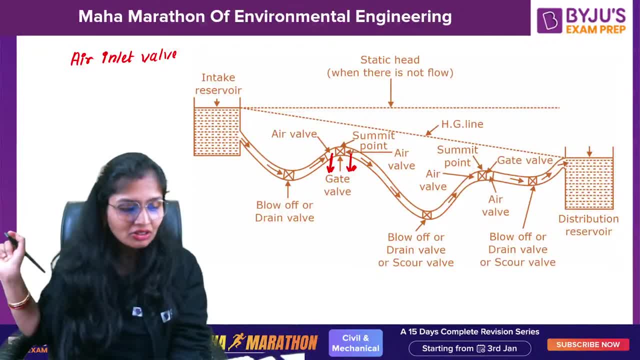 vacuum will be there, crushing failures can take place. Clear, So this you should know. Okay, okay, Now coming to last question: power down pressure due to larger amount of pressure winds. Now what happens? So this is the first question. So first question is: where can I garbage water? Okay, Okā. 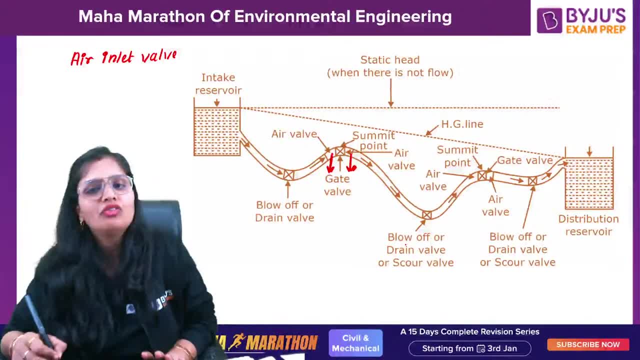 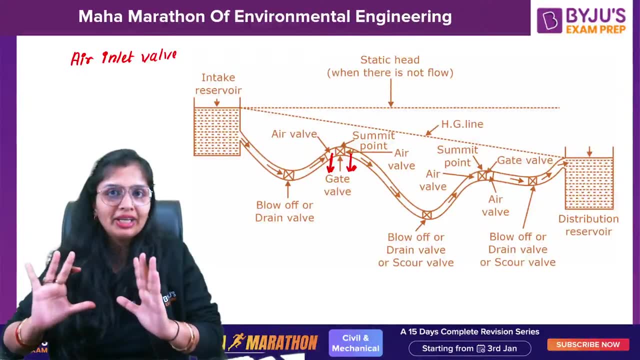 last one is tool. second last one is cover wall, blow off wall or drain wall. what happens in this case is this: air valve and air inlet valve is mechanically operated, or you can say: they are automatically operated. okay, you don't have to measure it each time. they know how to adjust it. 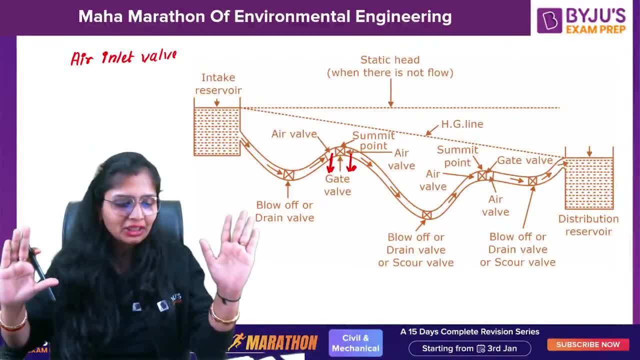 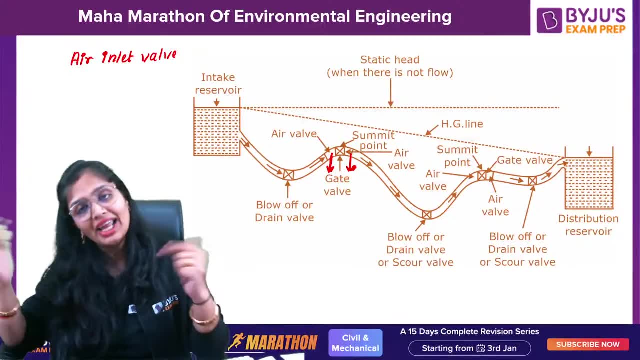 how to bring the air, how to remove it. it's what negative gauge pressure, negative gauge pressure, is for the case of when air inlet it happens. for compensating that negative pressure, air has to enter, otherwise crushing failure will take place. now, blow off on drain. well, this is manually. 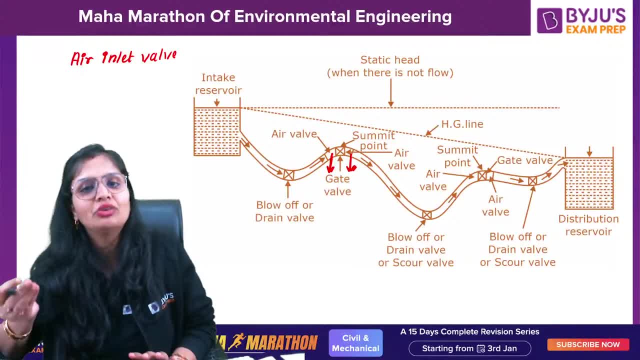 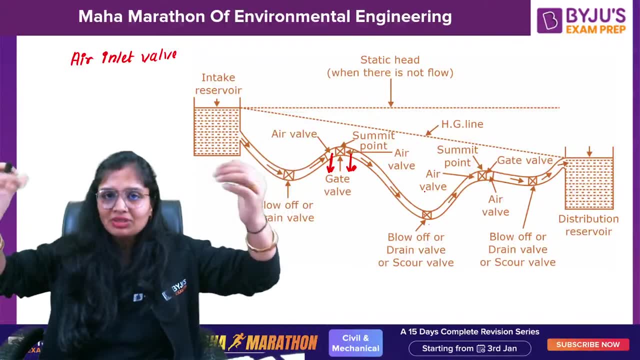 operated whenever the suspended solids have deposited and you need to clean, clean that you will stop the valve so that you will open this valve so that the water comes and it carries suspended solids with itself. okay, so this blow off wall, drain wall or scour wall- all the names. 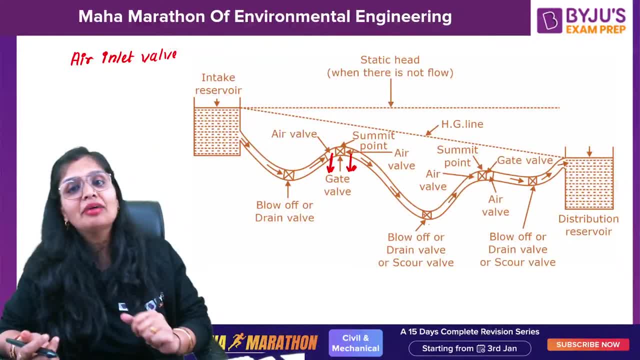 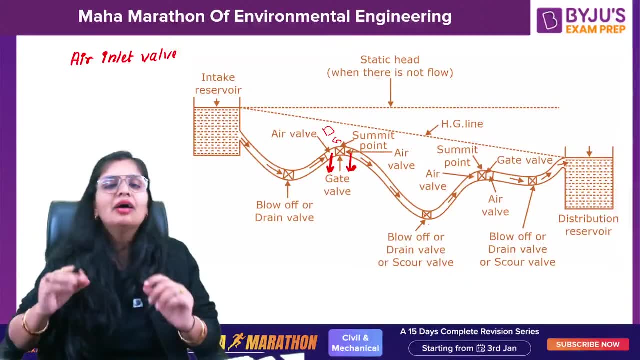 you should know synonyms. they are okay. last coming is pressure pressure wall. these are also placed on the air inlet valve. so these are also placed on the air inlet valve. so these are also placed on the summit points. here they are placed. pressure wall. pressure wall is the pressure of water. 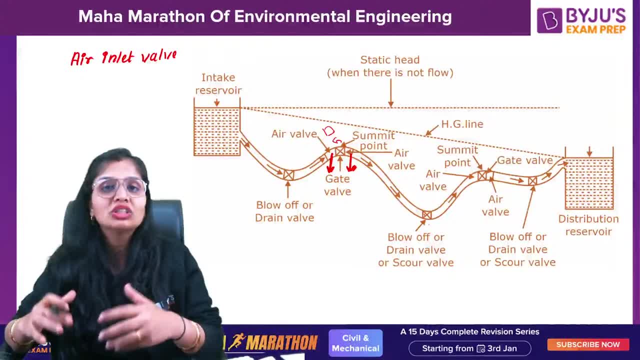 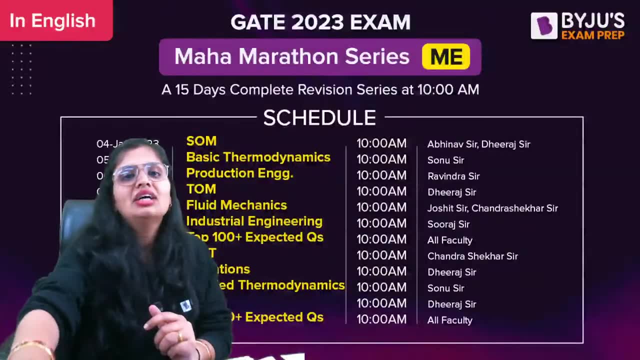 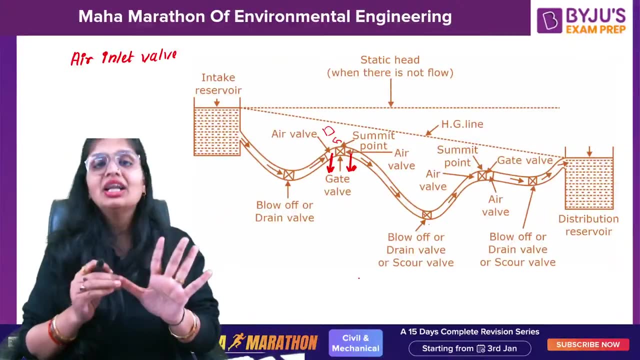 falls above a certain, or basically it goes above a certain predetermined value. so that is the reason for relieving the pressure of water. you need it. so that is the pressure relief wall. it's not mentioned it here. so this is the pressure relief five walls, which are very much important. and let 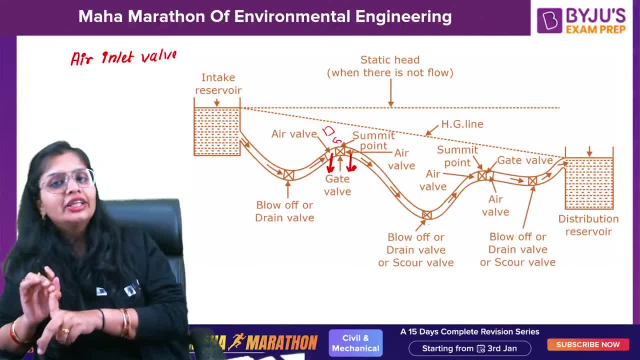 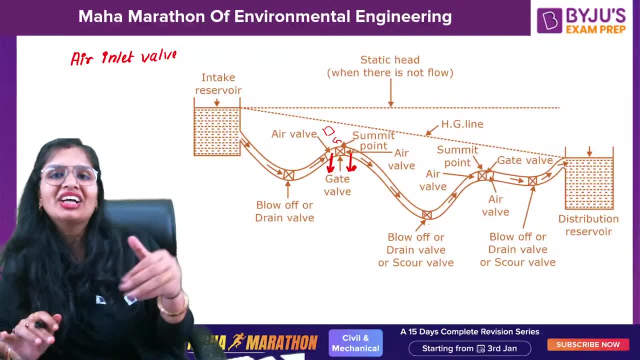 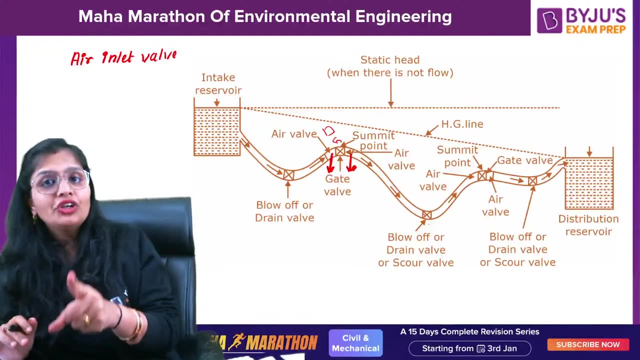 me tell you butterfly valve and globe valve. they also have the same function of regulation of water, but the only difference is: but the only difference is their functioning is different, but the thing is same. okay, and one more valve is there, check valve, or you call it as non-returning. 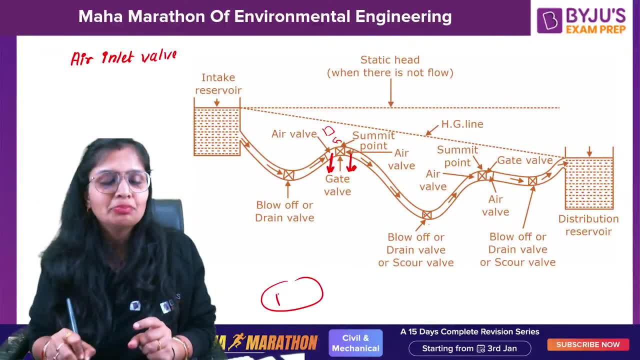 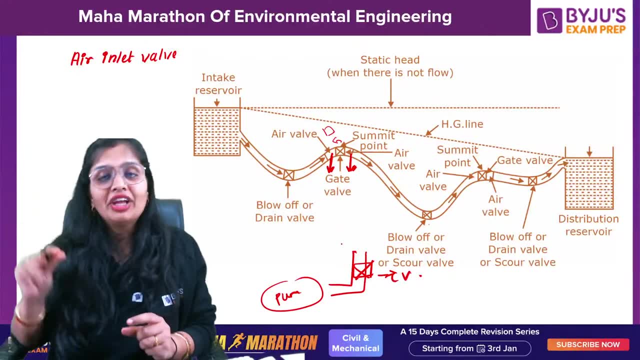 valve, check valve, non-returning valve is. let us suppose there is pump is there and here you are supplying water. so these valves are installed in these places so that when you stop the pump, the backflow water in the pump does not take place. so check valve. 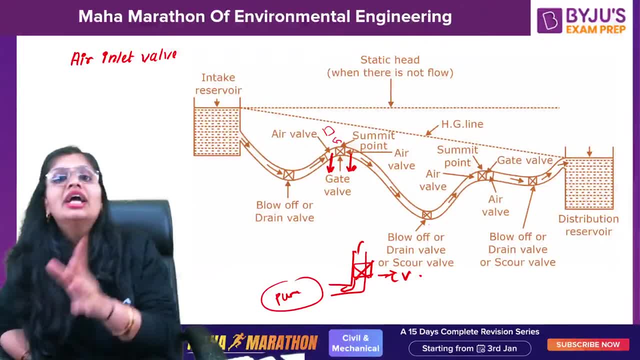 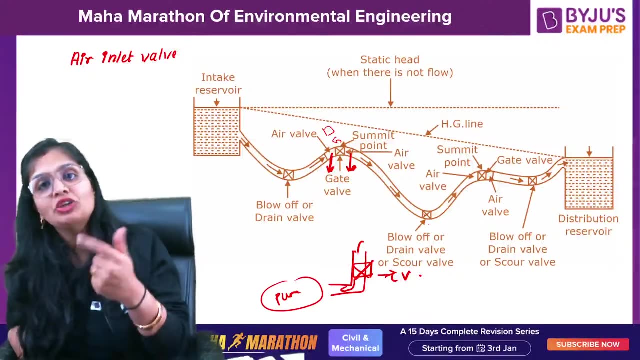 non-returning valve to allow the flow in, unidirectional gate valve for regulating the flow of water, air inlet and air relief valve. i already told you pressure valve. if the pressure is more than pressure of water, is more than a certain predetermined value, then you provide. 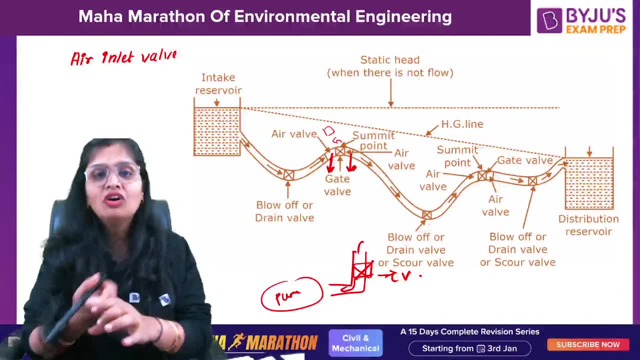 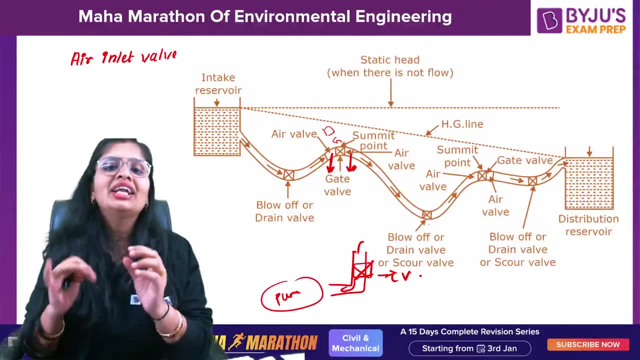 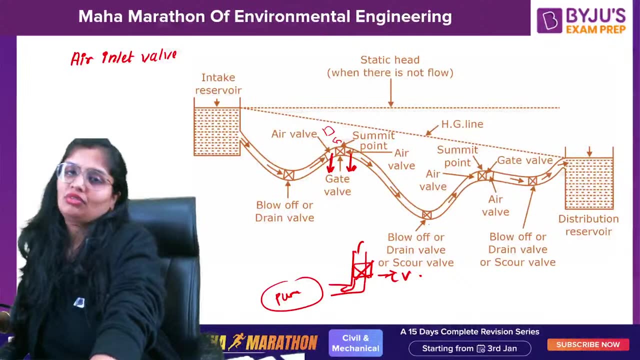 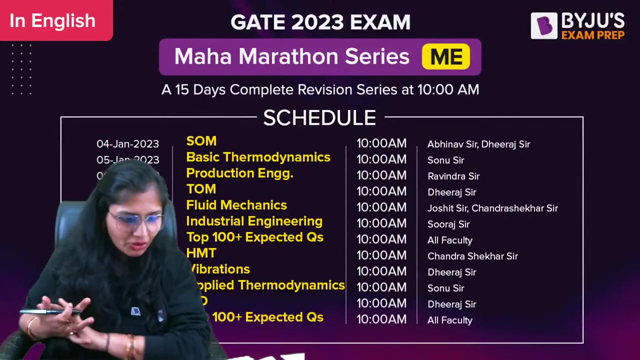 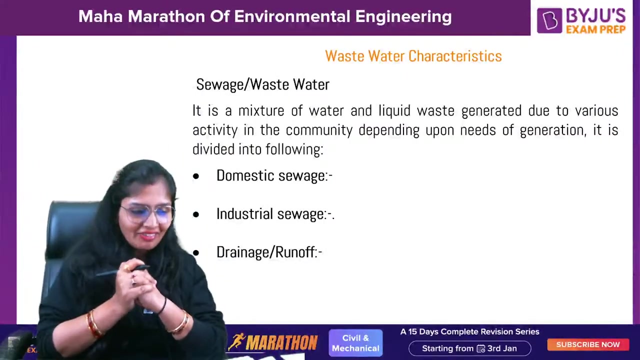 pressure relief: clear pressure relief valve, air inlet valve, air relief valve. these are automatically operated, while a blow-off valve is manually operated. clear, understood this much. so this is the schedule which already told you: control water and marathon class of sir tomorrow. so test water. shall we continue or you require a break? 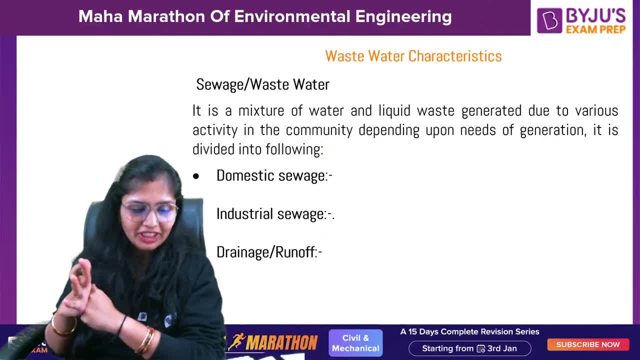 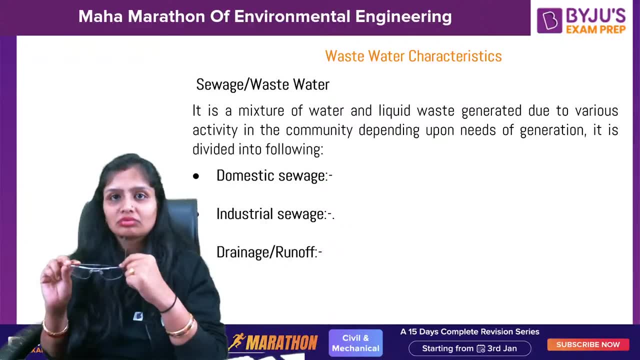 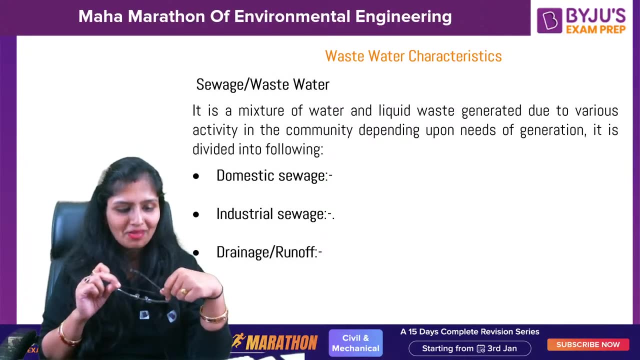 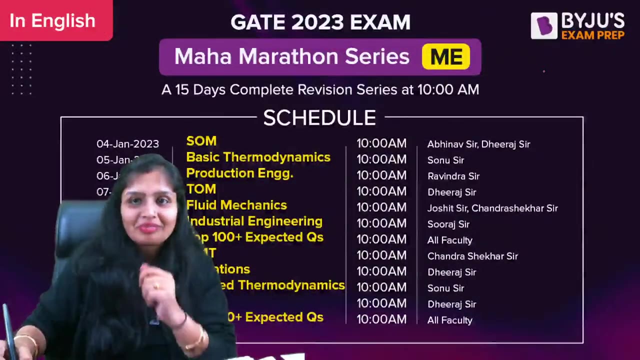 tiksha prem arun break or shall we continue? ok, First promise me, then you will 윽, and after that I will tell you. tell me back how many times delete set is called. kill me first once again. First promise me. tell me fast. how can varun eat in the library then? 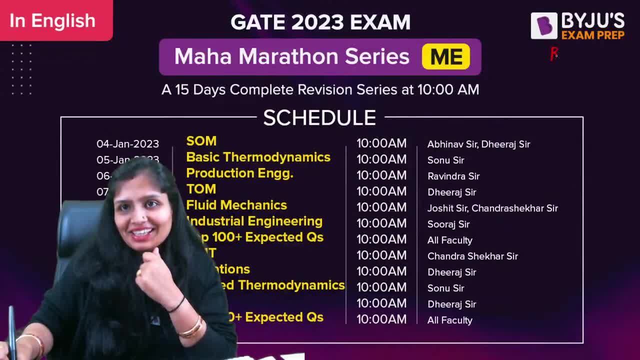 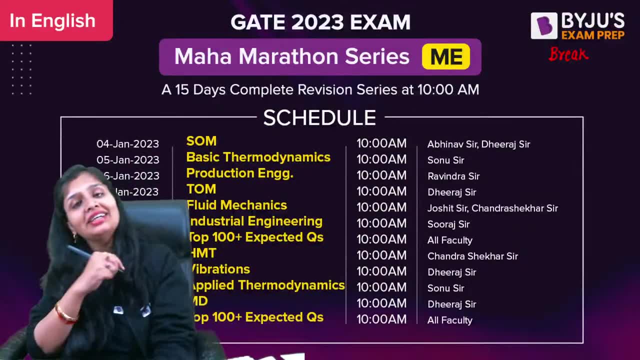 ok, you will not eat food, ok, fine break, ok, ok, ok, ok, k break. how much time? first promise me, then you will come, otherwise, si 10, next one, ok, ok, ok, ok, how much time please? injury, please, johnny, can I have time? sir, once again the students get reduced when you take the break, promise me and tell me the time first, promise and 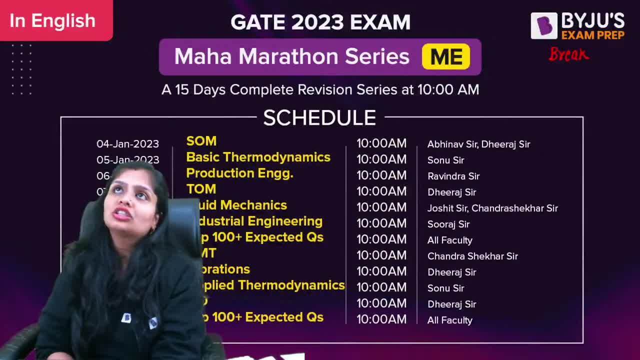 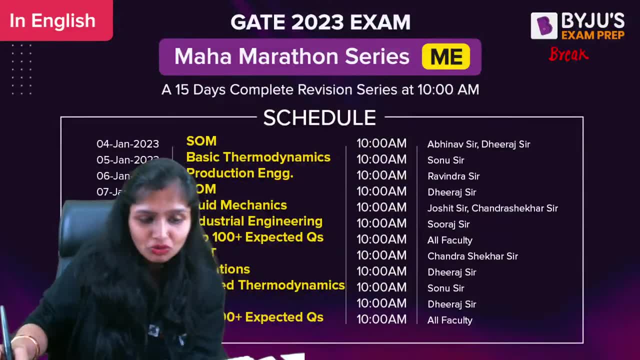 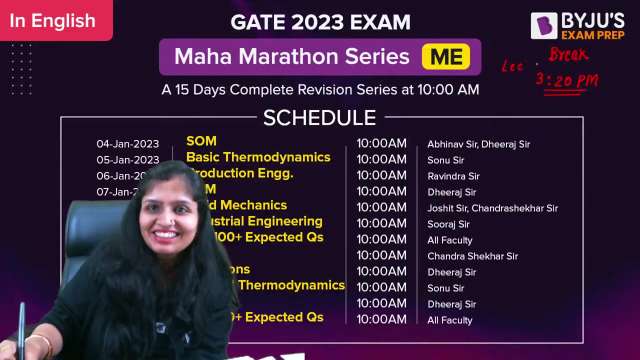 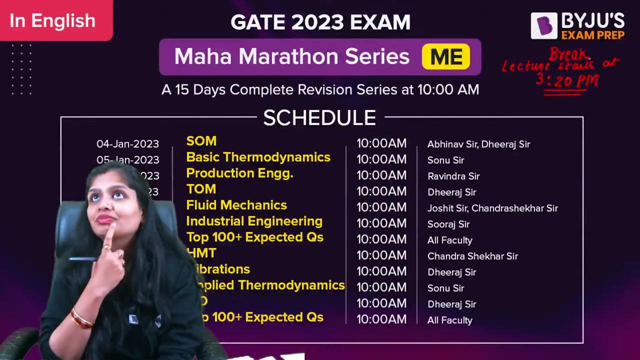 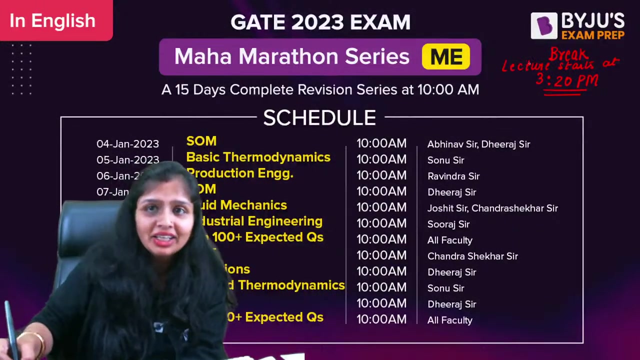 tell me the time when you'll be back, because wastewater disposal, everything is remaining. how much 30 minutes? it's 2, 40, no, no, don't say that. 3.30, 2.50, how much 3.30? come on 3.30. 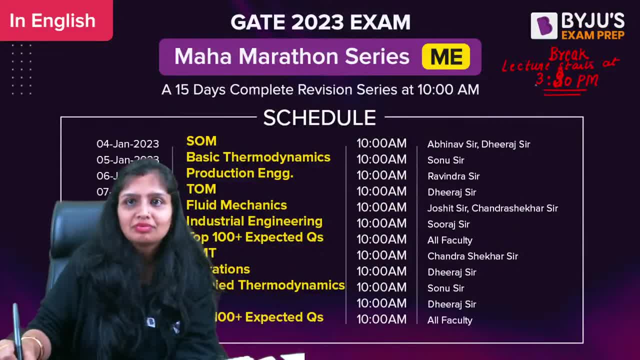 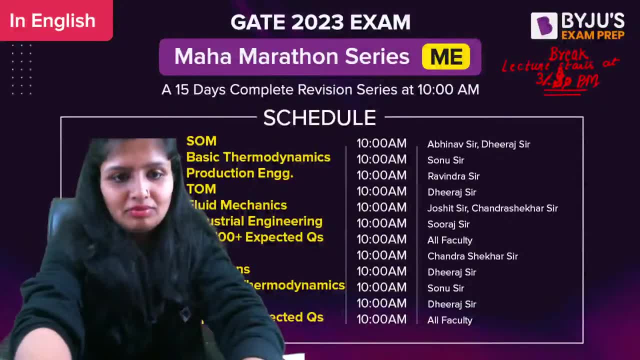 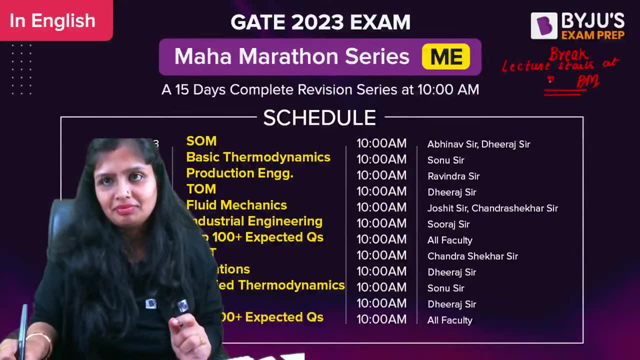 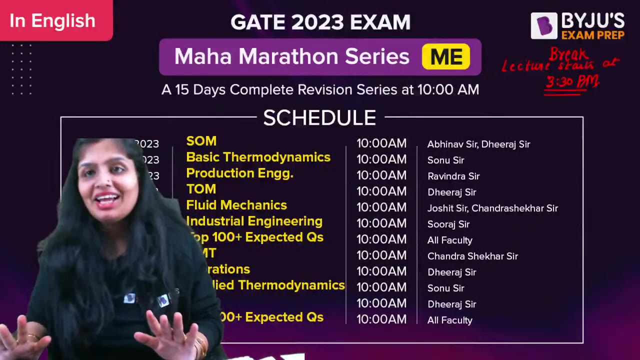 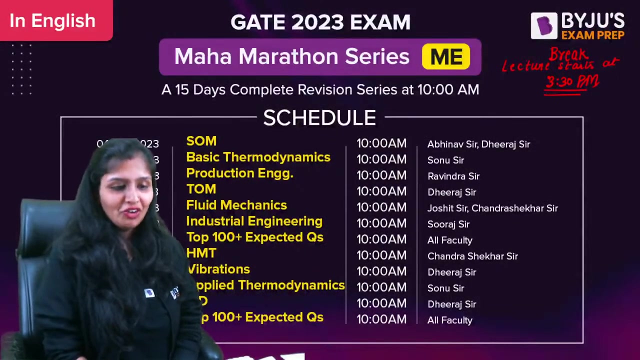 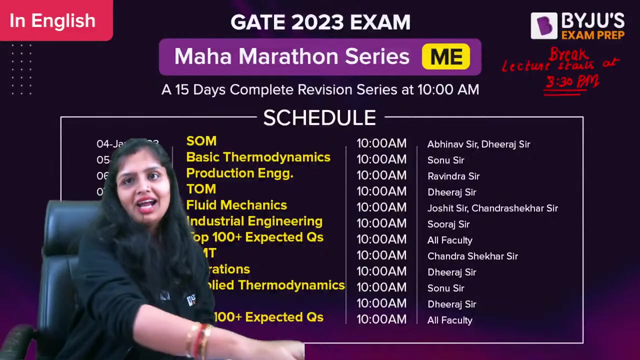 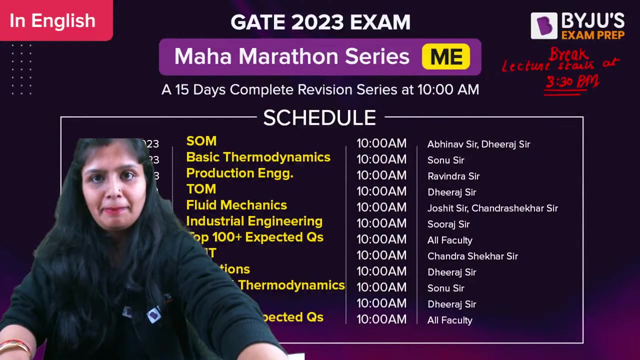 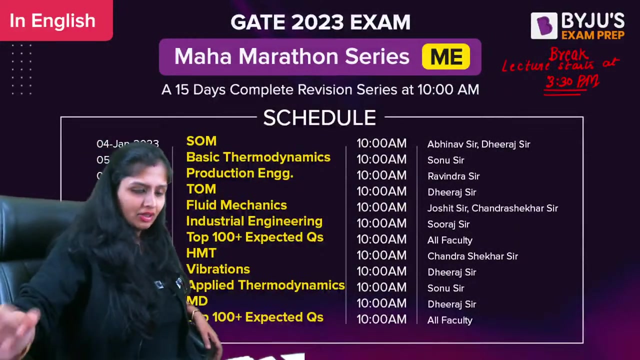 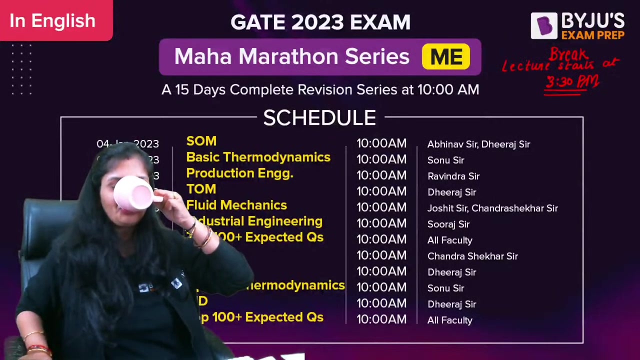 you guys promised me, so we'll meet, and now after this we'll complete whole wastewater. so, if you want, take a power nap, also of 10-15 minutes. hello, Navneet, okay, so we'll meet at 3.30 pm. fine guys, you, you. 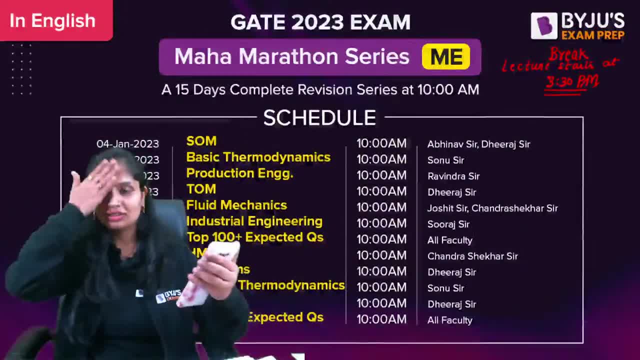 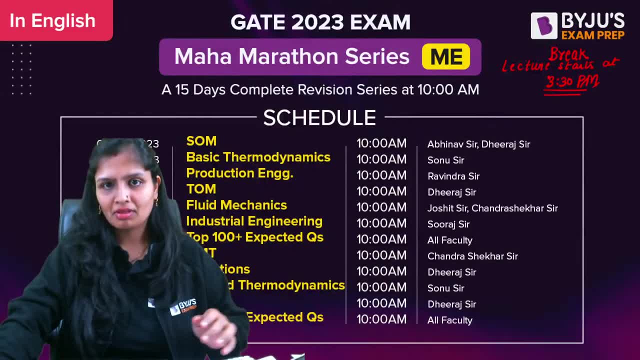 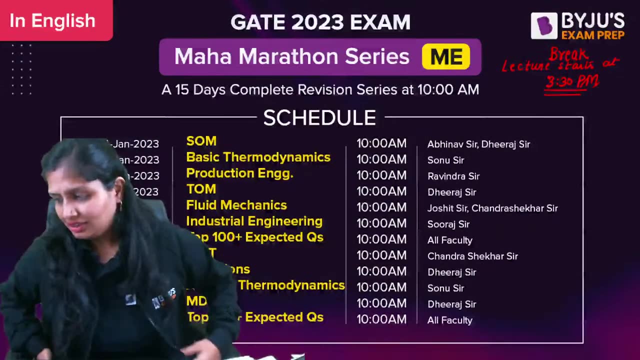 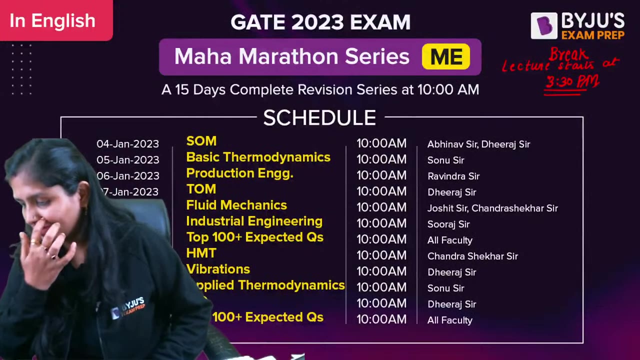 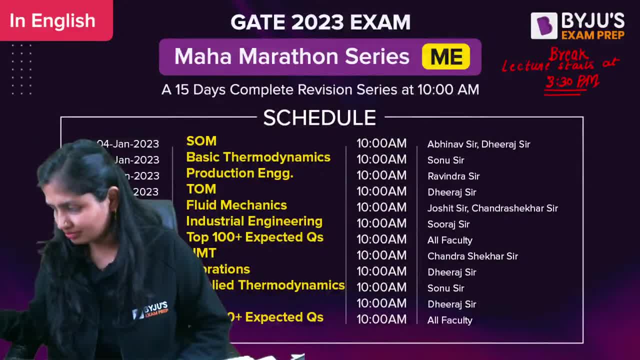 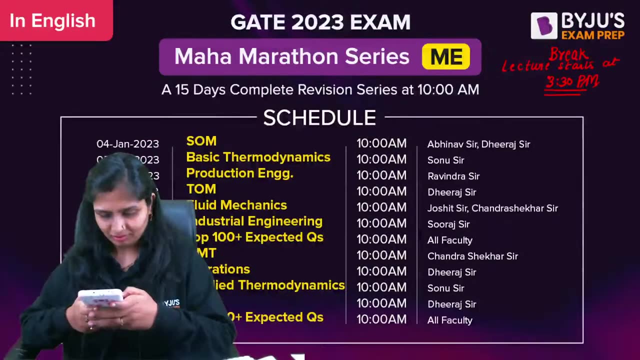 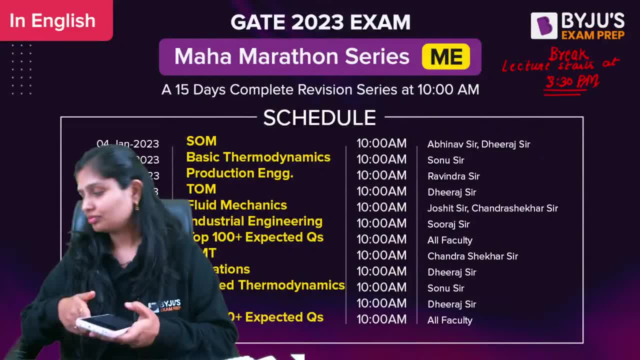 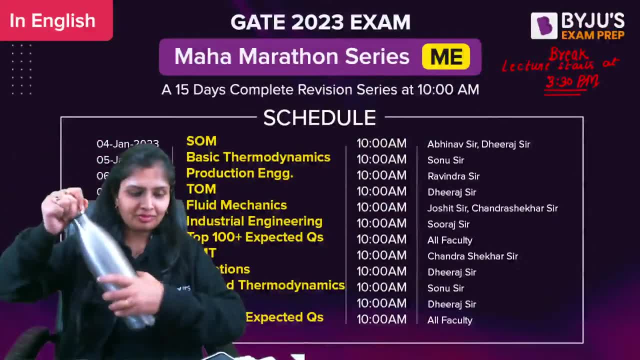 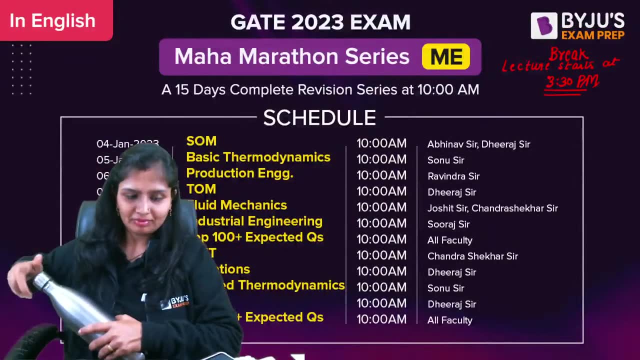 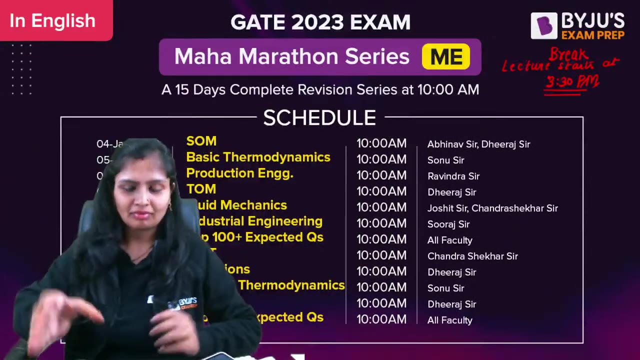 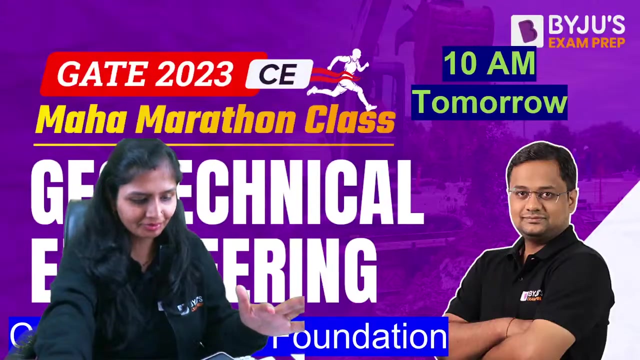 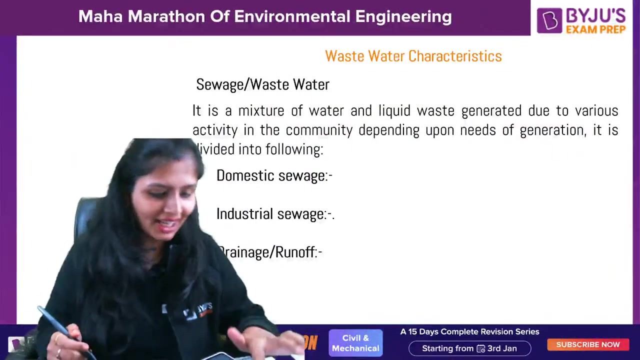 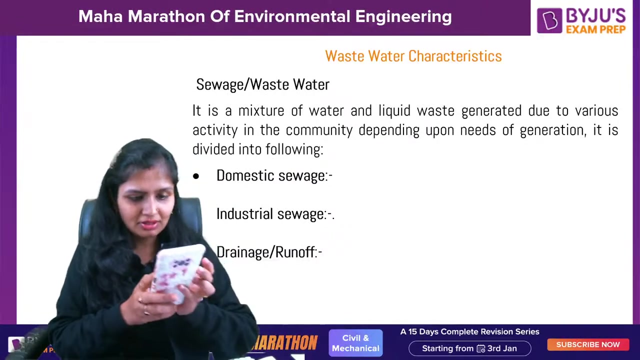 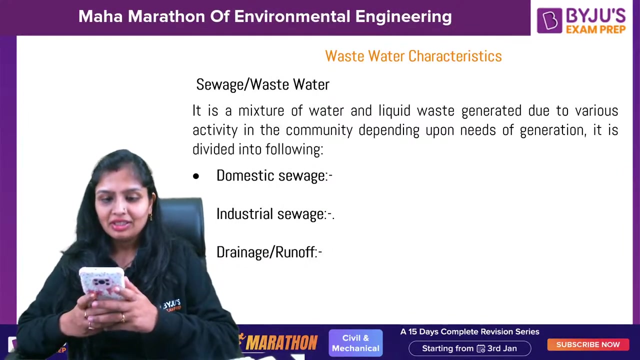 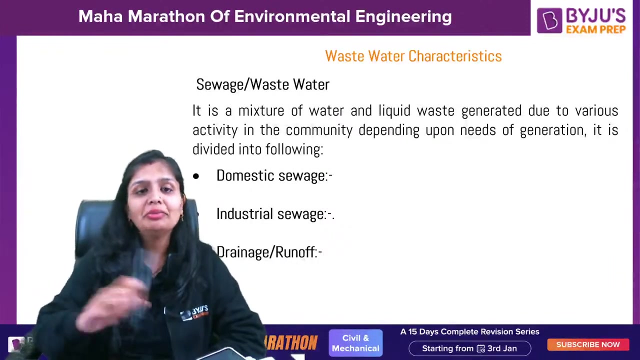 you, how you, you, can you, I, I, a I here to Good evening everyone. so geotech marathon right after this tomorrow shall we start Pete plus ma'am. ok, fine, fast, fast, fast. Ok, hello, shears, Swapnil back, fine, ok, then we will be talking about ways to order. 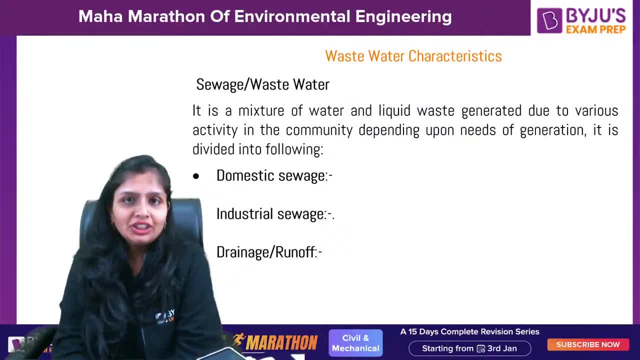 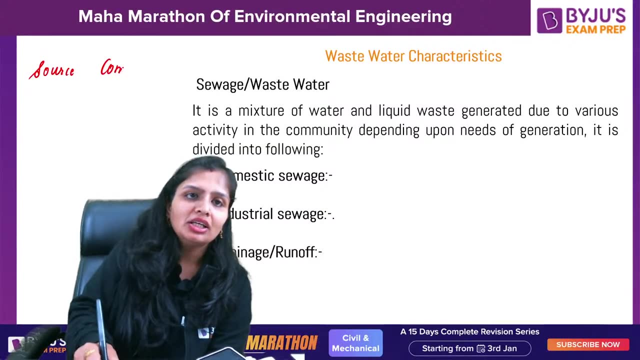 characters. So initially till now, we did regarding the raw water engineering. now we will be talking about waste water engineering. When you talk about waste water engineering right now- before that you were talking- source to the community. this was known as this was the whole process, was known as raw water. 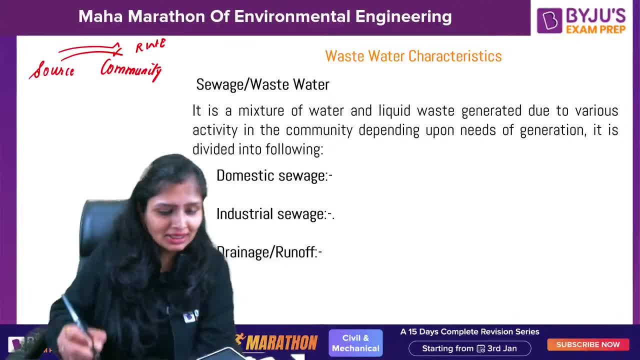 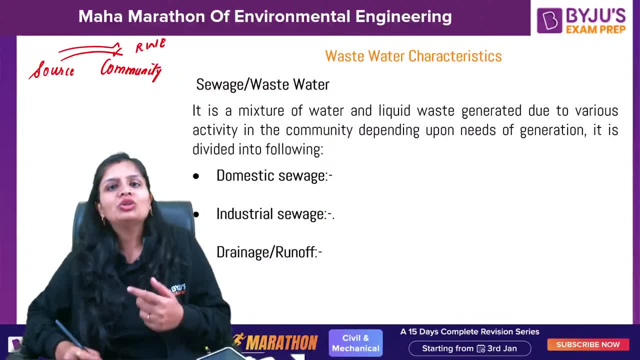 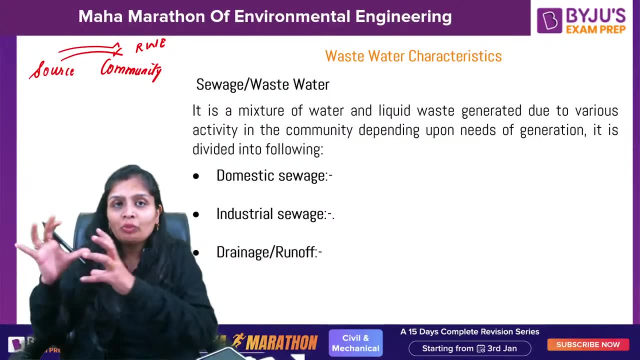 engineering RWE. Now what happens? What happens? The waste, the water which was supplied to your homes. eventually you will use it for drinking, cooking, washing and all those things, so that water will convert into waste water, So that waste water from the community, after being treated when it is discharged to the 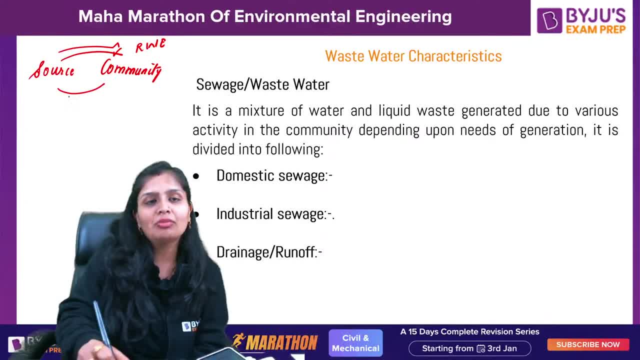 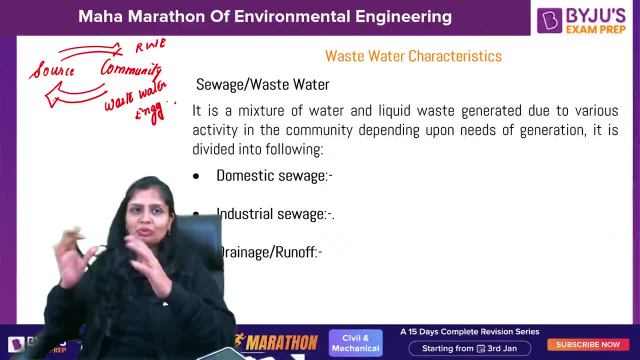 source. this whole engineering now we will be talking about will be the waste water engineering, So this engineering will be now waste water engineering. Ok, so that is waste water engineering we will be talking about Now. technically, there is a slight difference between sewage and waste water, but on a basis, 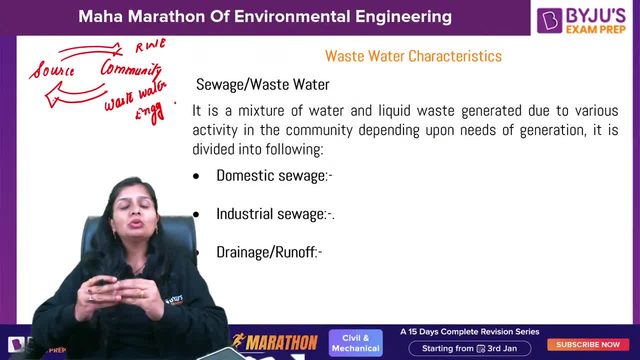 we take it as same Now what we understand by the word sewage. When you talk about sewage, it is: generally it consists of 99.9 percent of water and 0.1 percent of solids. So when you talk about sewage, it is a mixture of water and liquid waste. 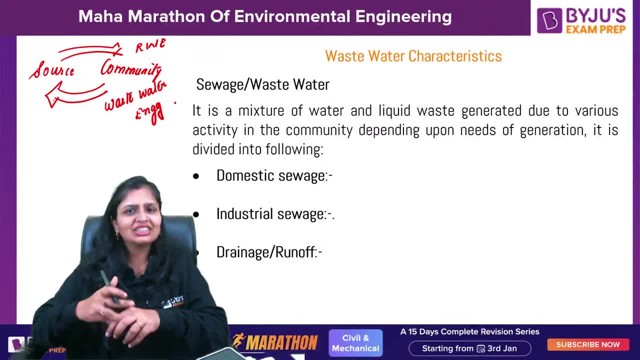 So when you talk about sewage, it is a mixture of water and liquid waste. Now we are then talking about what is waste water engineering? ok, so the first thing is: and liquid waste which is generated upon different activities. okay, if it is generated due to domestic. 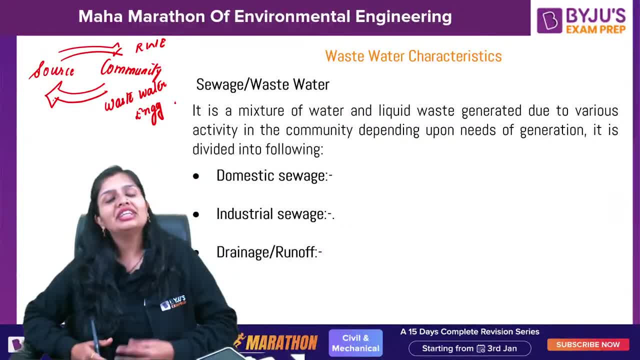 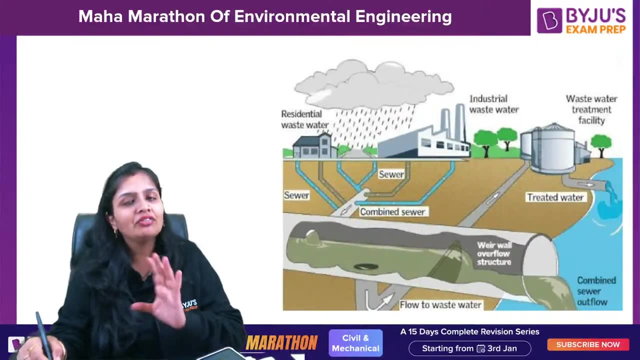 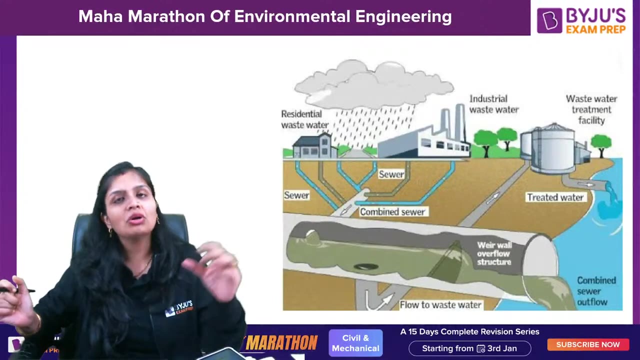 activities, you will call it as domestic sewage. if it is generated due to industrial activities, you will call this as industrial sewage. now, if it is generated, because what happens? if you see this diagram? what happens? rainfall occurs. okay, rainfall occurs, so certain amount of water infiltrate, certain amount of water go into the ditches, some amount of water goes into the rivers. 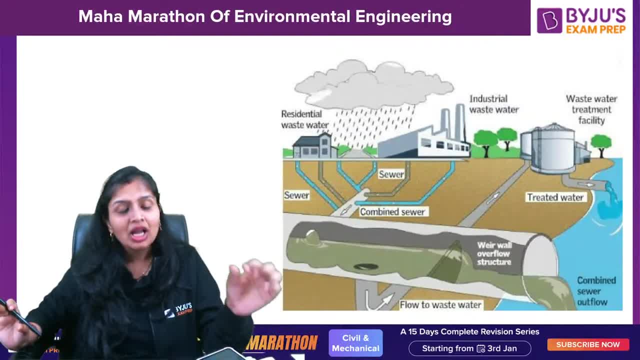 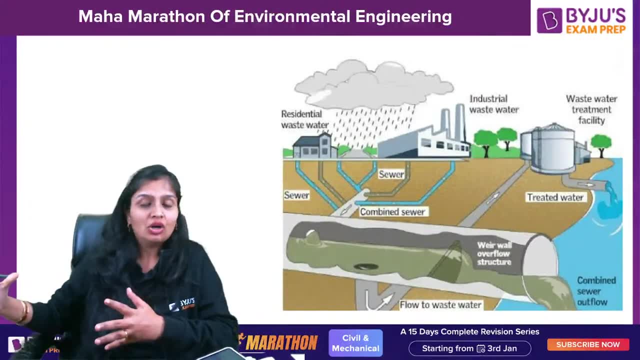 some amount of water gets stuck in the trees and all. so, after all this water, the amount of water which get drains- okay, and which you can see it okay, that water is known as runoff. so that amount of water which drains from the streets, and all after all the losses, has been satisfied, that is. 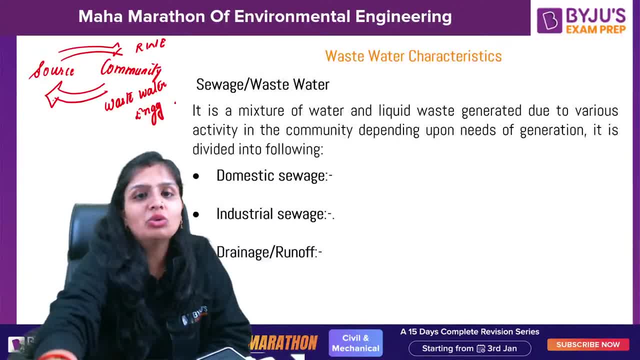 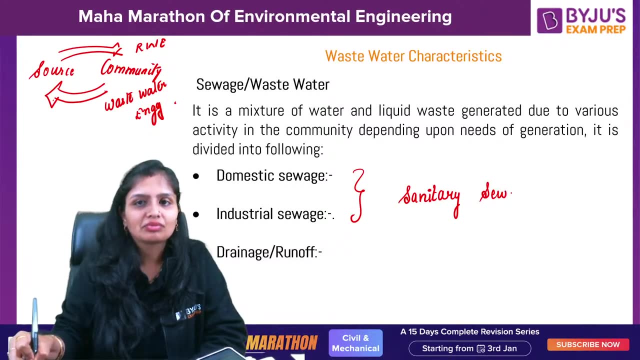 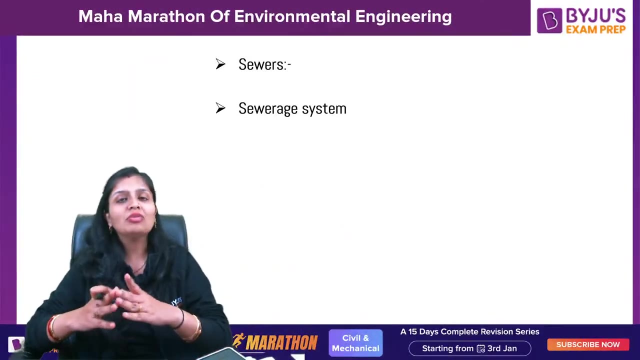 known as runoff or you call it as drainage. so that is what, drainage or runoff? technically they say that domestic sewage plus industrial sewage is known as sanitary sewage. sanitary sewage now coming up further. now coming up further, talking about sewers. some people call it a sewers, sewers, sewers, whatsoever pronunciation, i just call it. 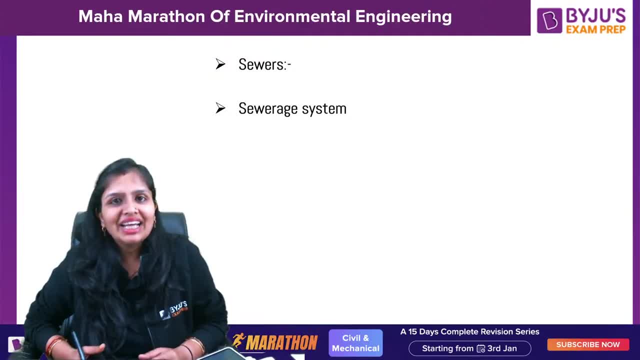 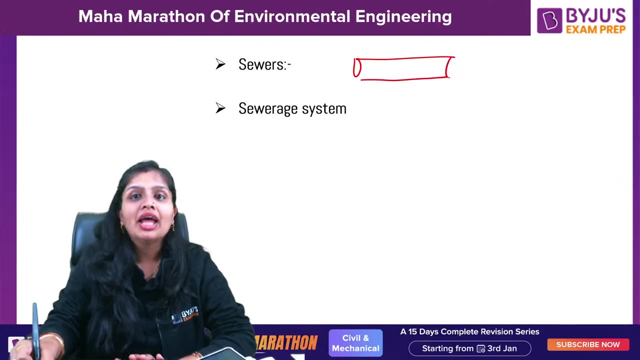 as sewers. now, sewers are nothing. they are pipe, or technically, in a fashionable manner, you call it as conduit, conduit, whatsoever you want to say. so these sewers are generally pipes or conduits which carry the sewage from one place to another place. now, sewage system, the whole system of 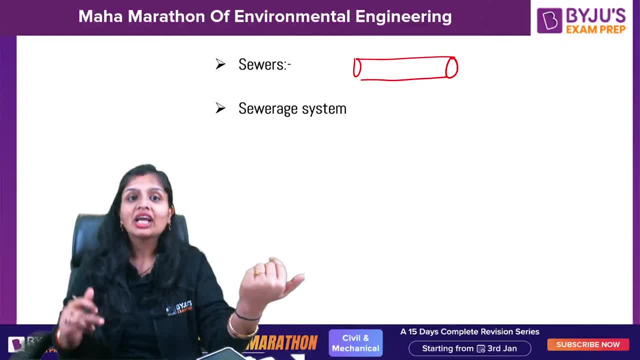 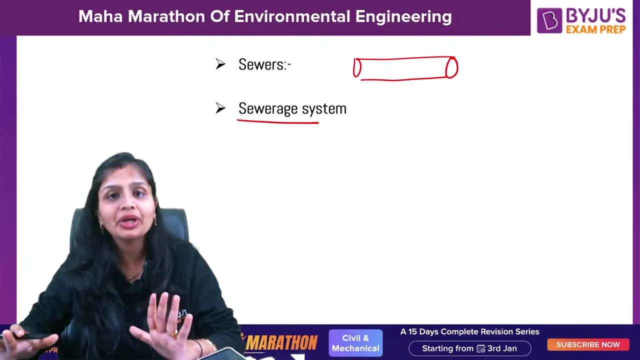 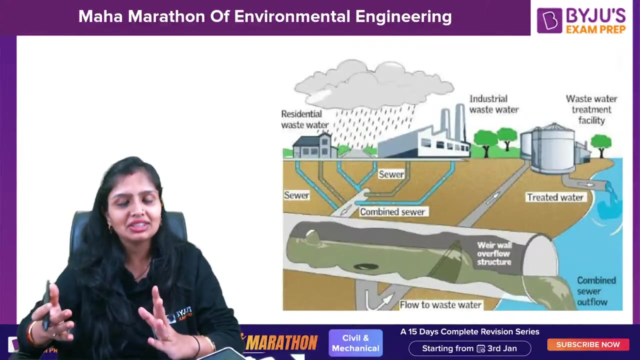 collecting, treating and disposing it. this whole system is known as what sewage system. so the whole process of collecting it, treating it and then discharging it to the reverse, and all everywhere, that is known as the sewage system. okay, now. now the question comes when you talk about it, when you talk about the various types of sewage system. before that, let's talk about the. 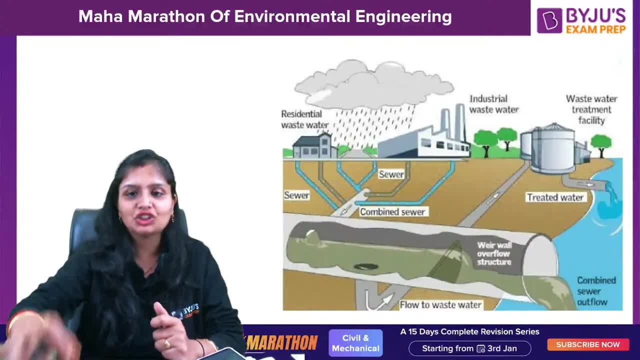 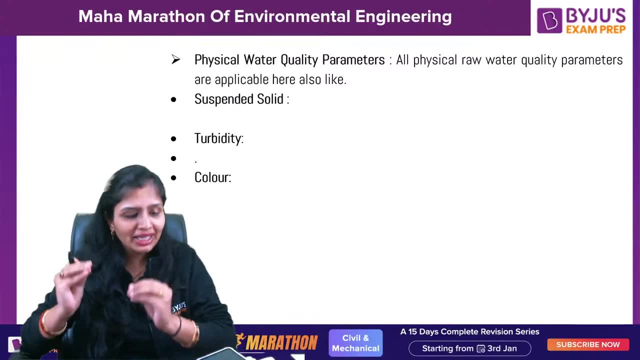 physical parameters of this sewage. when you talk about the physical water quality parameter, the measurement of solids which is present in the sewers, so the measurement of solids which is present in the sewers is known as sewers, so the SEI is said to be transparent kinds of SE. 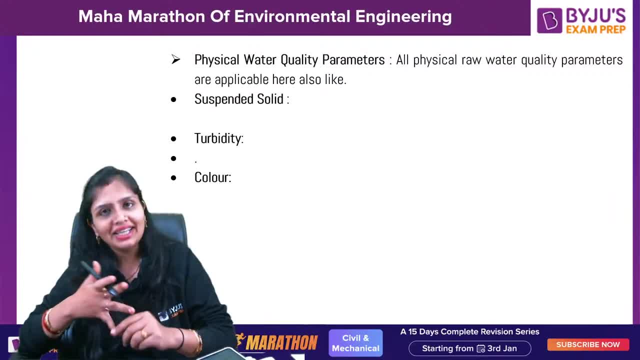 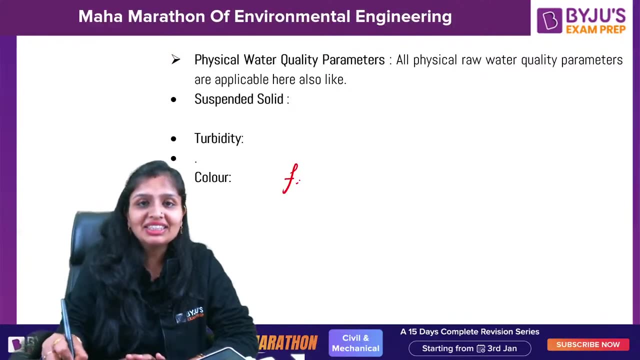 like pretend. we say all watchlow, 처리RALE chameray なきゃいけない. okay, so what's over test and all which you have studied in the raw water, exactly it is the same turbidity sing. talking about color, this has been asked- the fresh sewage, if the sewage is fresh. 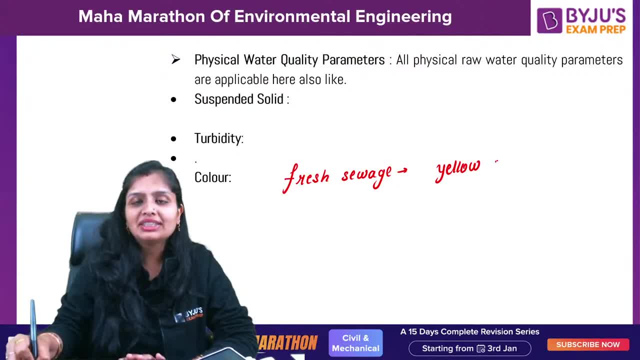 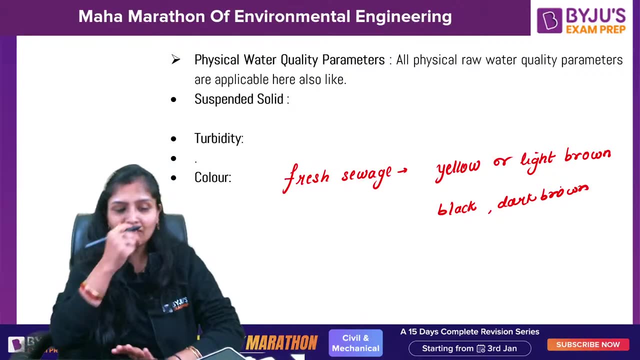 if, When there is a bigger size of the sewers which are watchedlow, turns yellow, it is yellow or you can say light brown. So over the time the sewage color becomes black, or you can say gray or you can say dark brown. So when the color of it becomes black or it becomes dark brown, it becomes septic and acidic. 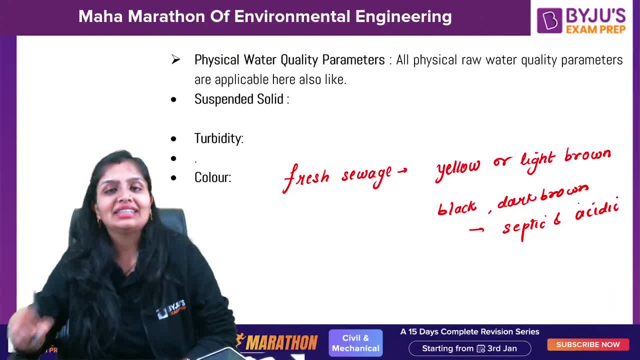 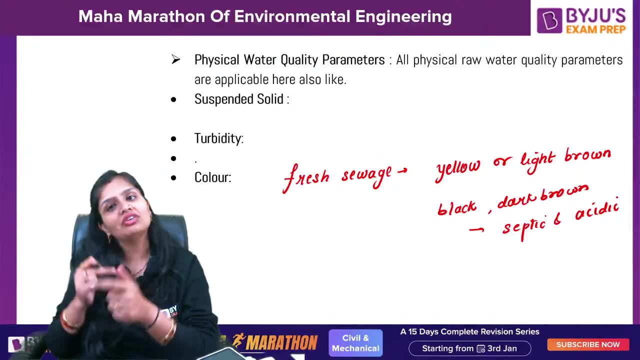 The sewage becomes septic and acidic- Clear. So initially, if it is yellow or light brown in color, it is fresh sewage, Afterwards when it starts to become black or dark brown. so basically it has become septic and now it is acidic. 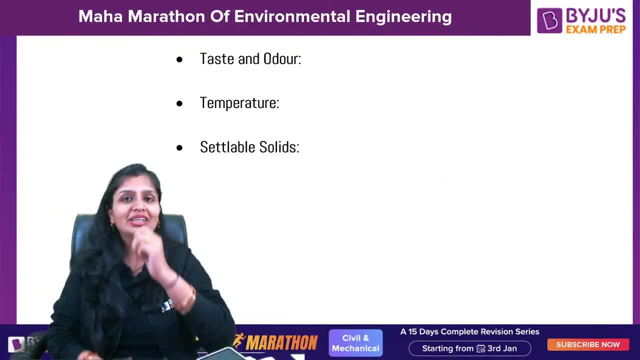 Clear. So this you should know. they can ask you in one month: Taste and odor. So I guess you can say: yeah, Initially that odor. when it is there, it is odorless. When it is generated sewage, it is odorless. 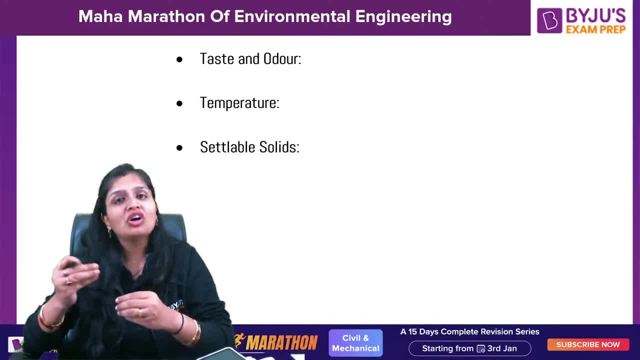 Over the time you will see that, because of the oxygen being exhausted, H2S gets liberated, Vibration and all will take place. So it becomes a pungent smell, or you can call it as a rotten egg smell. Temperature again: with every 10 degree Celsius rise in temperature, the biological activity will double. 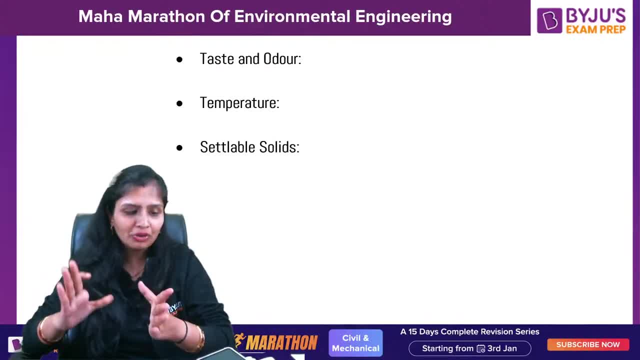 So all these are the physical parameters? Yeah, black, dark, brown, gray, Correct, So all these are the physical parameters. Now, if you talk about solids, here we have four categories. I will tell you. All the things will get enhanced. 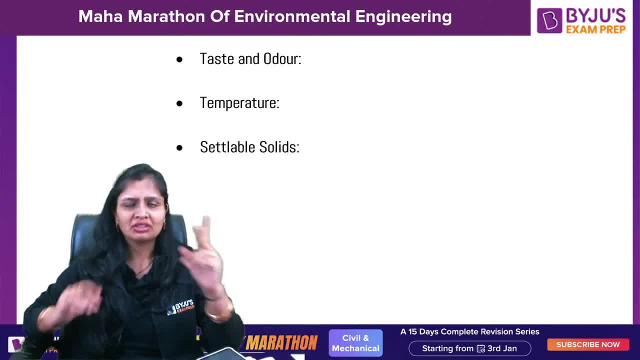 How There, you started in raw water two times. Two types of screens, Excuse me, Two types of screens: Medium, sorry- fine screens, coarse screens, Wastewater. you will study medium, fine, coarse In raw water. you studied one sedimentation time. 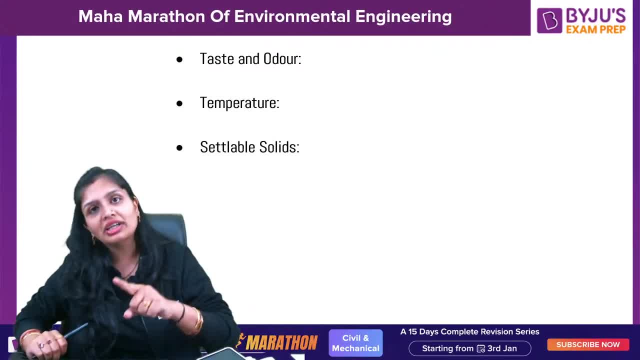 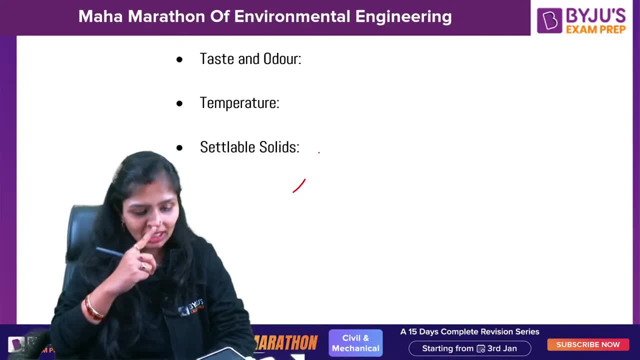 In wastewater there will be two sedimentation times In solids portion in raw water. you studied only three types. Here you will study settleable solids. What are the other types of solids, guys? What are the other types of solids? 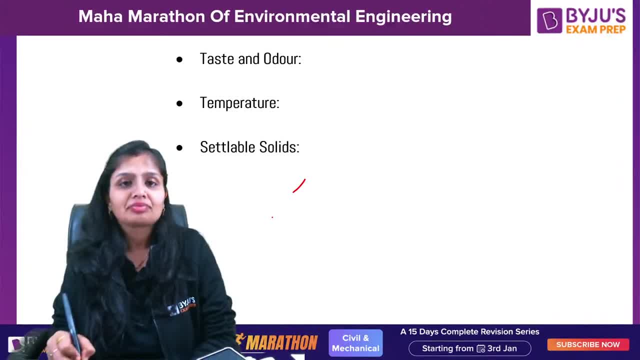 Settlable, and three already. I told you fast, Settlable solids. three more Suspended solids, Colloidal solids, Dissolved solids, Now dissolved solids. Now let me tell you- I didn't tell you that time regarding settlable solids, and I told you, I will tell you in wastewater part. 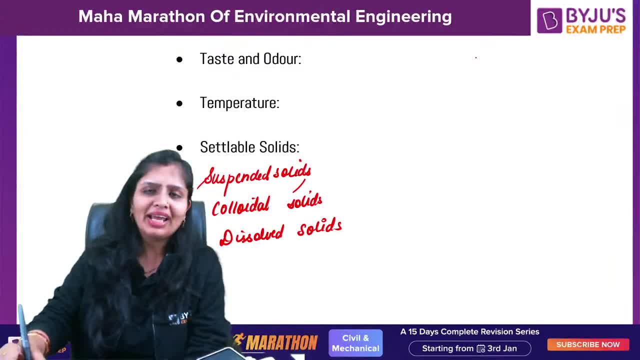 If you want to measure settlable solids, no need to apply any brain. There is a hemofcone- This is sort of cone is there And here calibrations are being matched. So here calibrations are being matched. 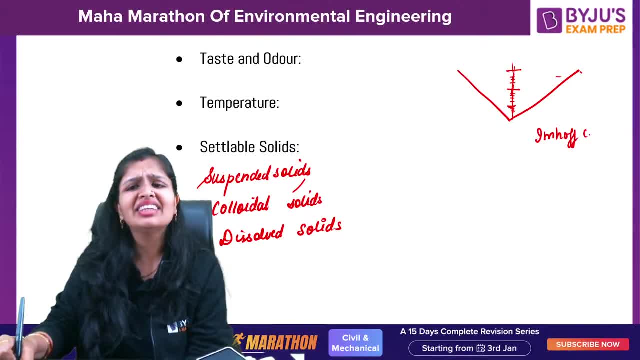 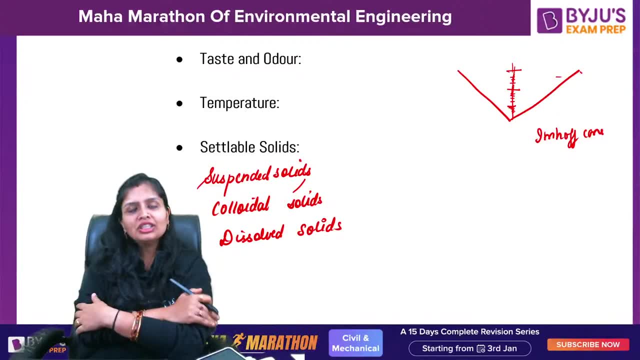 Like this. So this is a hemofcone, Nothing to do. Don't apply your brain. Take the sewage sample, Put it in this hemofcone, Let and you just wait for two hours. What will happen? Whatsoever. solids are there which have the tendency of settling. they will settle in this hemofcone. 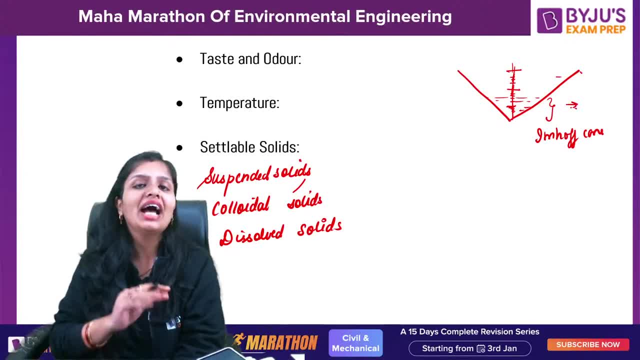 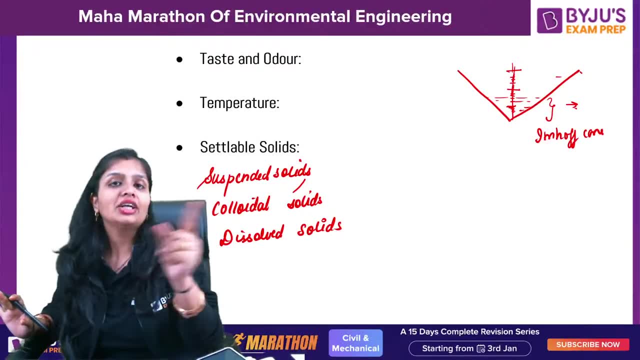 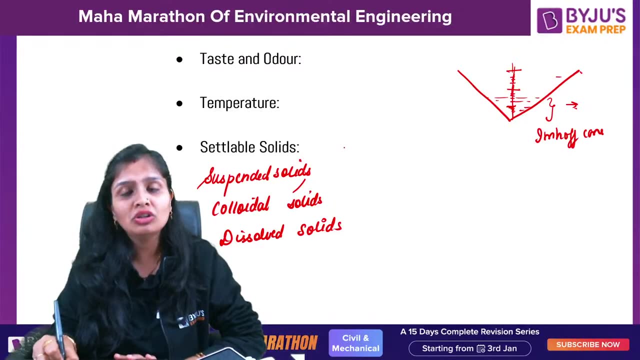 They will settle in this hemofcone and you will measure it Directly. you will come to know the concentration. Why? Because here also you have done calibration, You have related to unknown parameters. That's it Clear, everybody. And if you want to know the dimension, this is 10.. 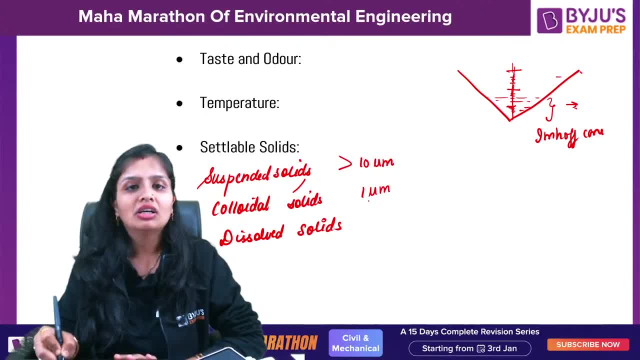 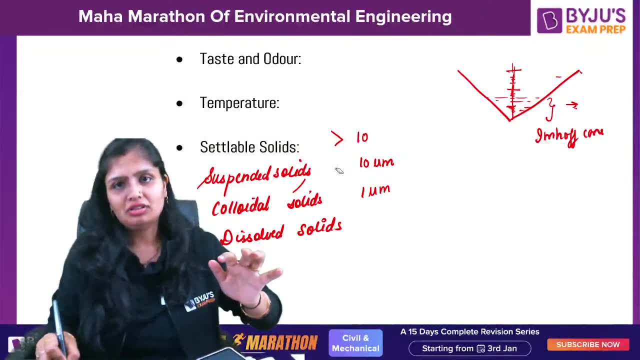 This is 1 micrometer. This is 1 micrometer. This is 10.. This is 10.. Just a minute. This is 1 micrometer. This is 1 to 10 raised to power minus 3.. And this is 10 raised to power minus 3.. 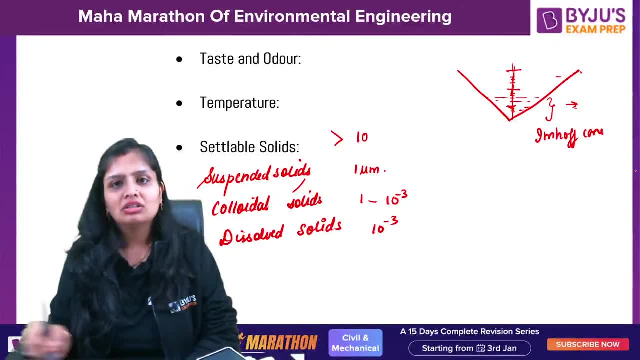 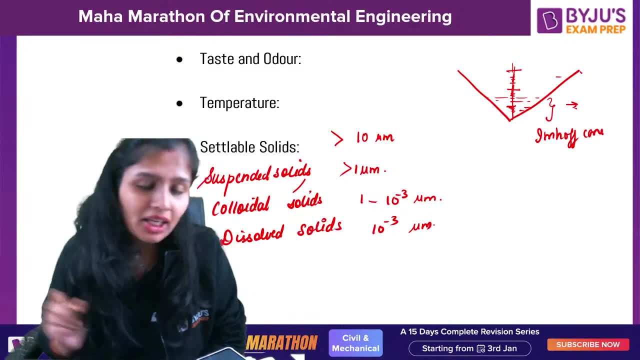 So in case, if they ask you, you should know this. So everything is in micrometer, greater than micrometer. This is also micrometer Clear, So this you should know. This is regarding the dissolved solids, suspended solids. 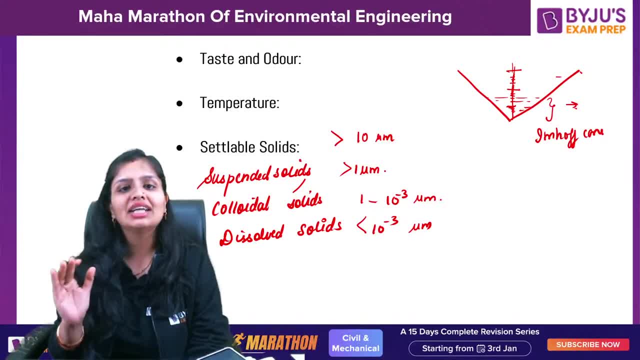 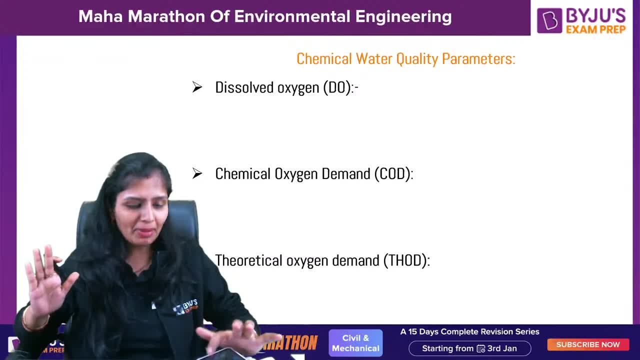 If ever they ask you to match the following, and all you should know this- These are the types of solids which they can ask. Fine, Now coming further regarding the chemical water quality parameter, Talking about the chemical dissolved hemofcone. Okay, 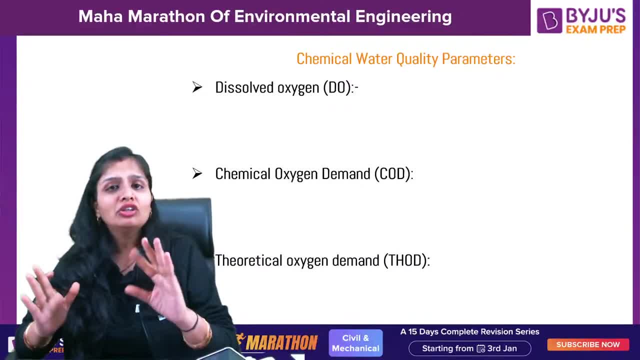 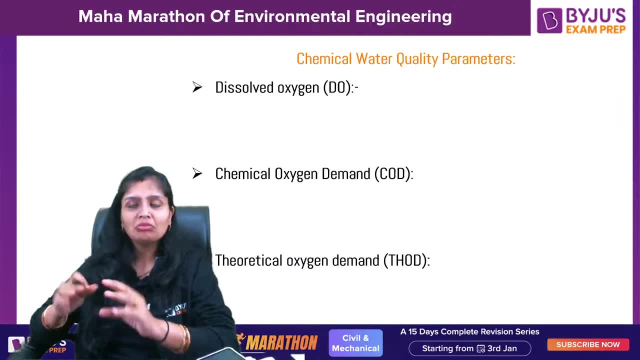 Now understand this very carefully. When you talked about dissolved oxygen, you know, you have memorized it or you have studied a number of times- that the minimum oxygen required for the survival of fishes is 4 mg per liter. Leave that Right now. I will tell you one thing. 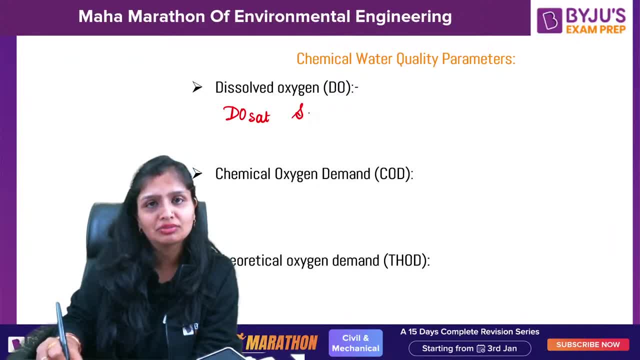 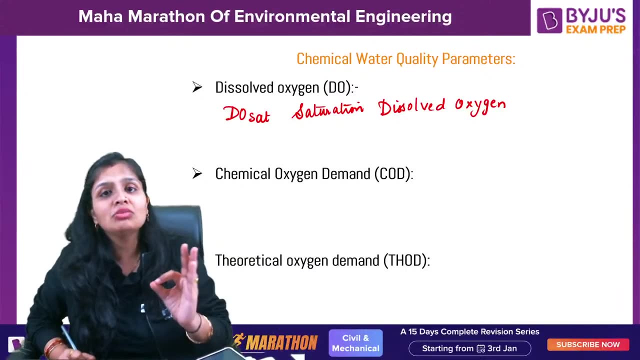 DO saturated, which you call it as saturation dissolved oxygen. Now listen to it very carefully. Saturation dissolved oxygen: maximum quantity of oxygen that is practically dissolved in water at a given temperature. That means at 20 degrees Celsius. if I say that DO saturated is 9.2 mg per liter, that means that means that anything can happen. maximum at 20 degrees Celsius. 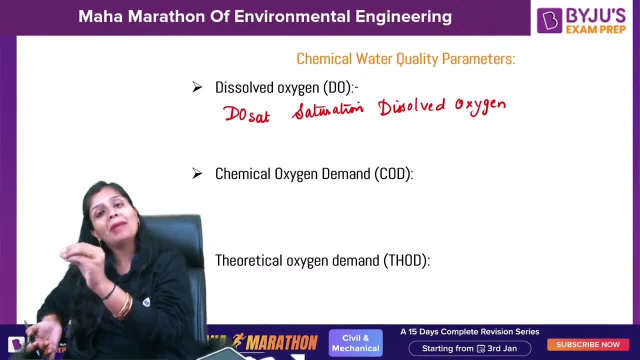 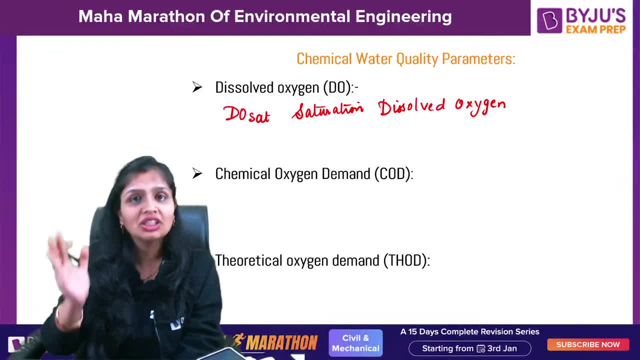 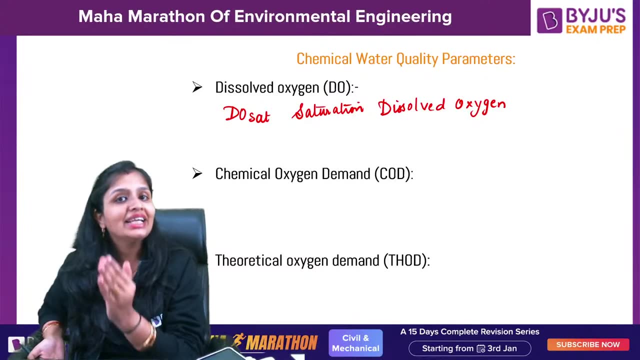 So that is the maximum quantity of oxygen that is present in water at a particular temperature is known as DO saturated. Yes, it is temperature dependent. If you change the temperature, the dissolved oxygen changes With the increase in temperature. the solubility of dissolved oxygen. 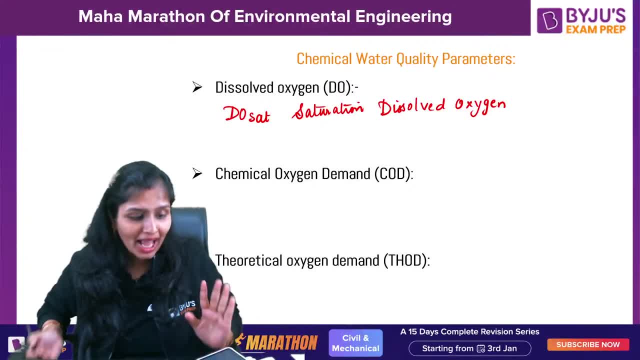 So the amount of dissolved oxygen decreases, as per Henry's law. As per Henry's law, Okay. So increasing the temperature, increasing the temperature DO saturated decreases. Now, how will I come to know that organic matter is present? Now tell me. 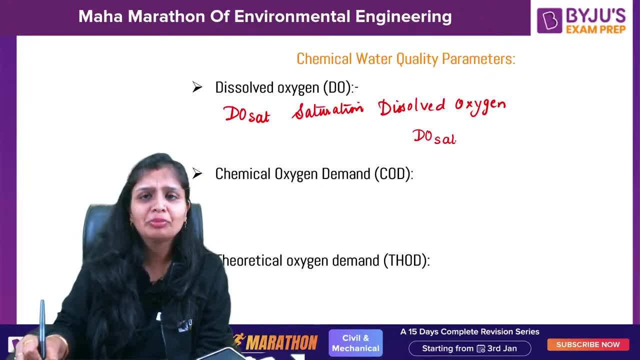 In water. DO, saturated should be there. Okay, There should be the oxygen present, But at any time the oxygen present is D. Okay, This is the oxygen which is present. Okay, So if I subtract DO, let me talk dissolved oxygen. 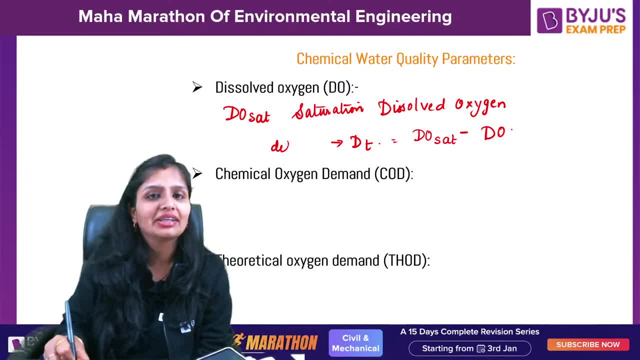 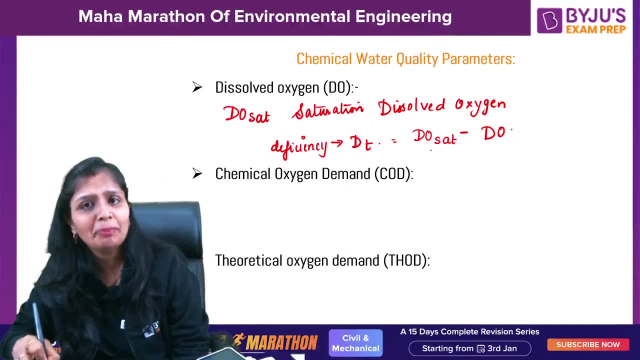 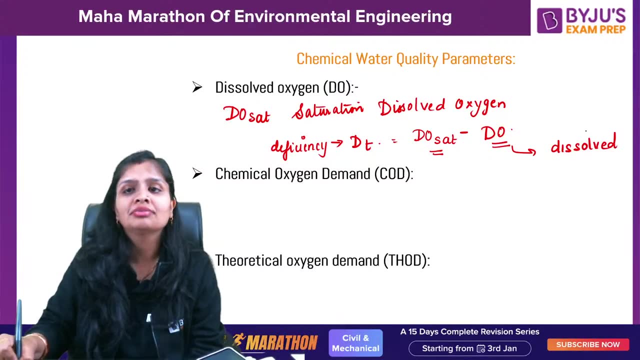 This will tell me that deficiency, how much deficiency is there? How much deficiency of oxygen is there? If deficiency of oxygen comes out, this should be present And this is the current dissolved oxygen which is present. Dissolved oxygen, present at any time. 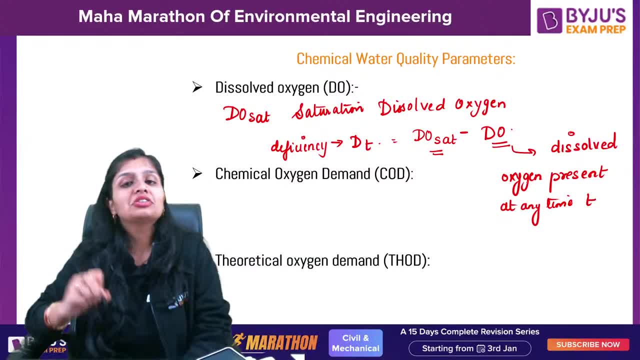 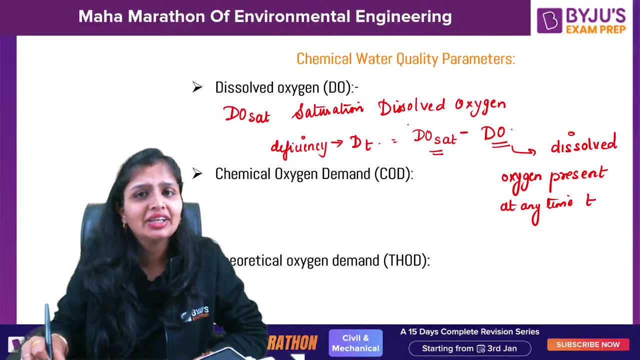 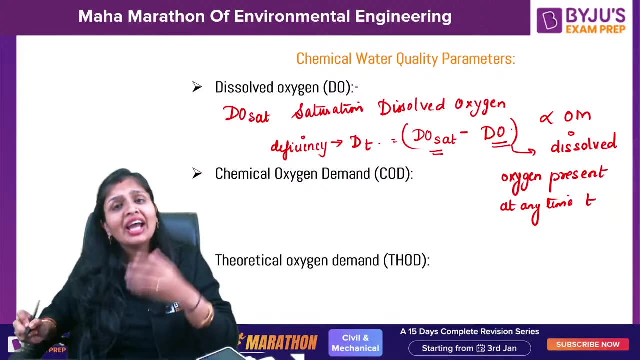 So when you will subtract this, you will come to know the deficiency. If there is deficiency, deficiency is directly related to organic matter. More the deficiency, more the organic matter. Why, ma'am? Why? Why the oxygen is deficient. 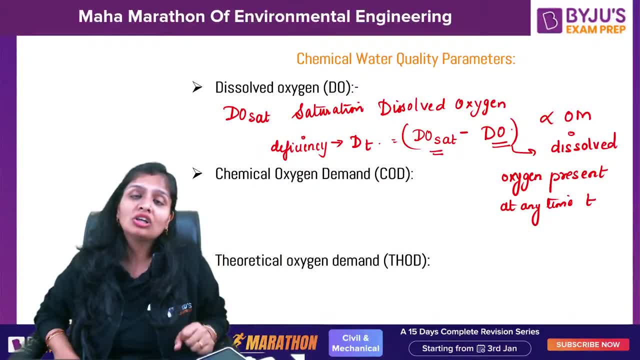 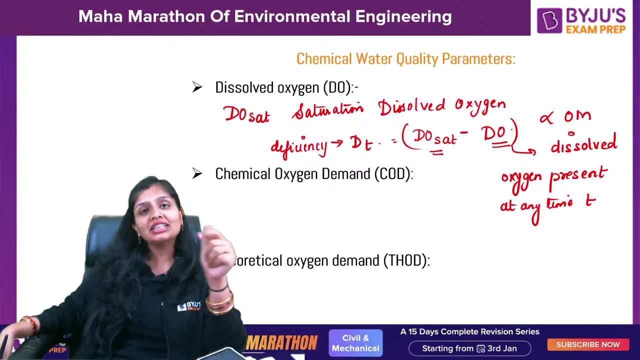 Because microorganisms is using that oxygen. Why microorganisms is using? Because it want to carry out the decomposition of organic matter, To be precise, To be precise, biodegradable organic matter. So more the deficiency, more is the concentration of organic matter. 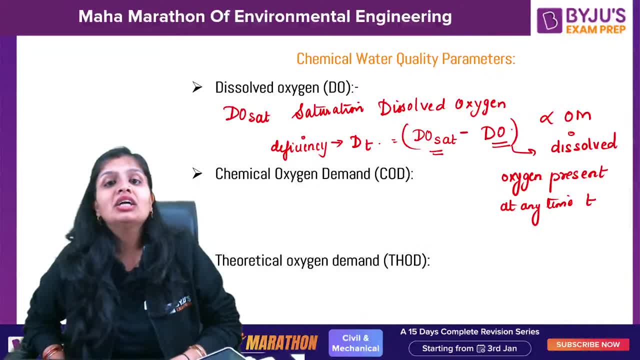 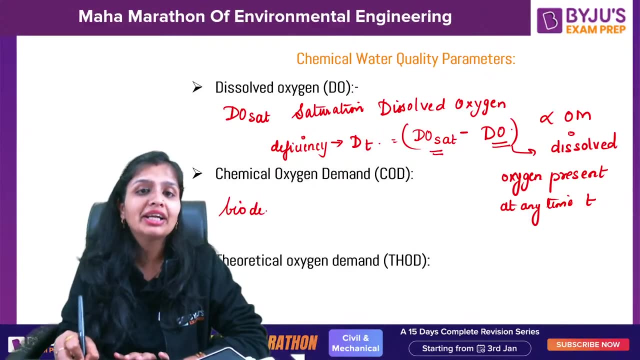 Now coming up next. Coming up next: Chemical oxygen demand. Chemical oxygen demand is the total quantity of oxygen required, Total quantity of oxygen required for the decomposition of biodegradable as well as non-biodegradable organic matter. Now let me tell you something. 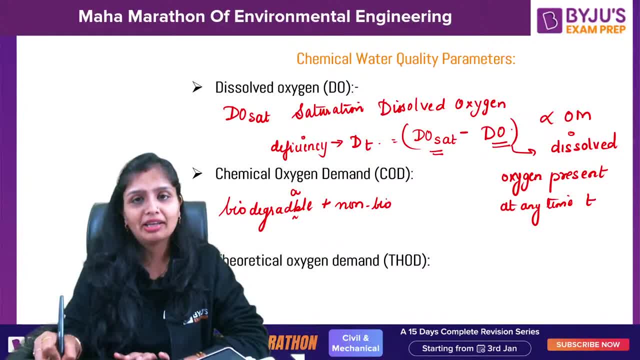 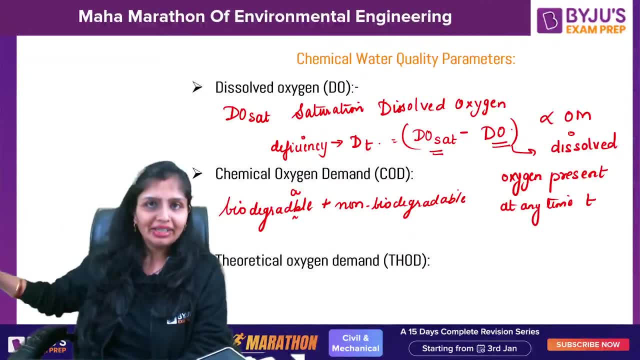 Let me tell you some things which are truth. non-biodegradable organic matter. First of all, this is just a demand which we are calculating In practical. when you go in the treatment plant, you don't apply chemicals. Why? Because when you are applying chemicals, you are spending money on that. 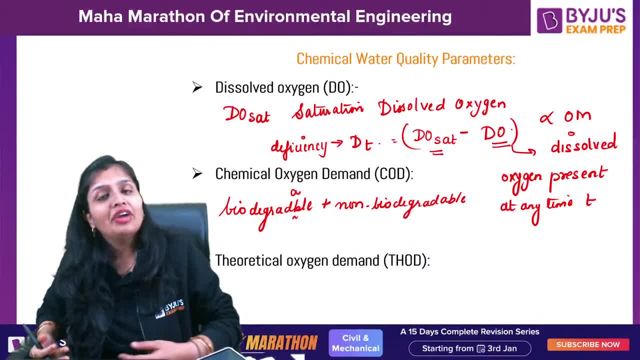 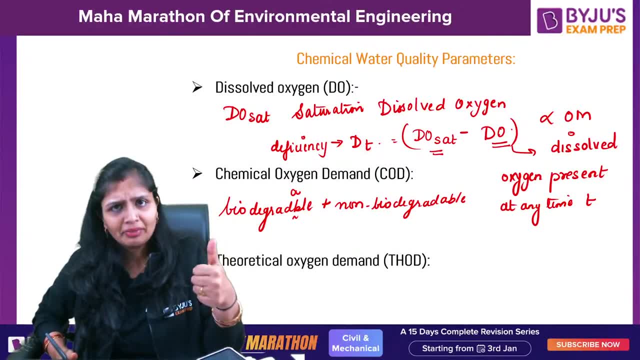 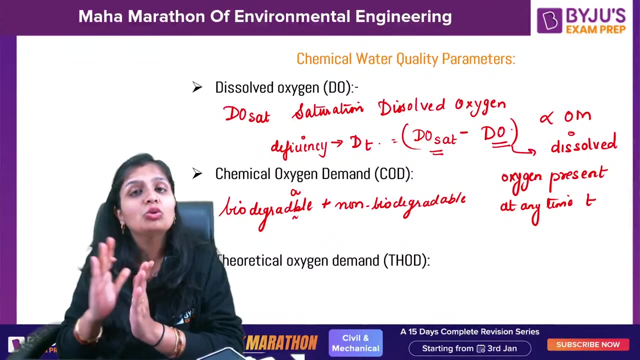 But you can say the advantage is when you leave it for the microorganisms for carrying out the decomposition of organic matter. Firstly, it is time taking Okay. Secondly is basically you have to maintain ambient conditions and all That's okay. But when you use chemical biodegradable organic matter as well as non-biodegradable organic matter, both will be decomposed. 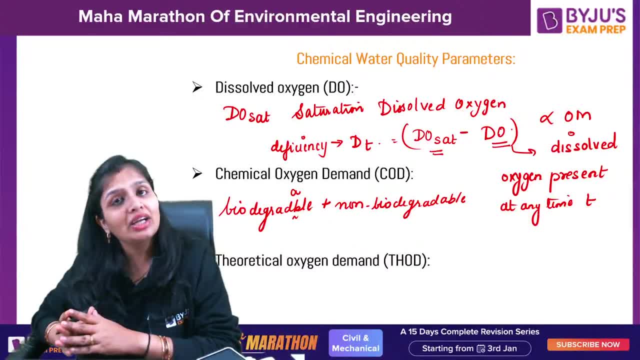 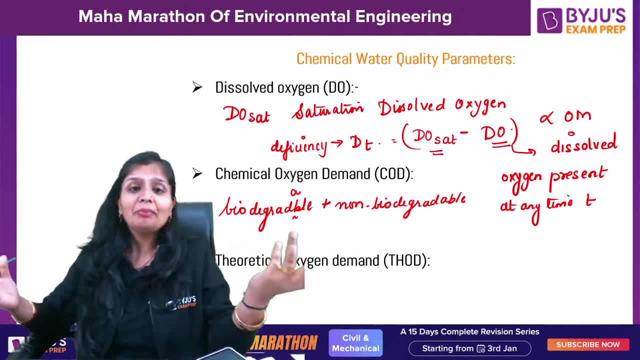 But if you go by the microorganisms, generally, they carry out the decomposition of only biodegradable organic matter. So, ma'am, if so much are the benefits of COD, why we are using not COD, Why we don't, Why we don't use chemicals? 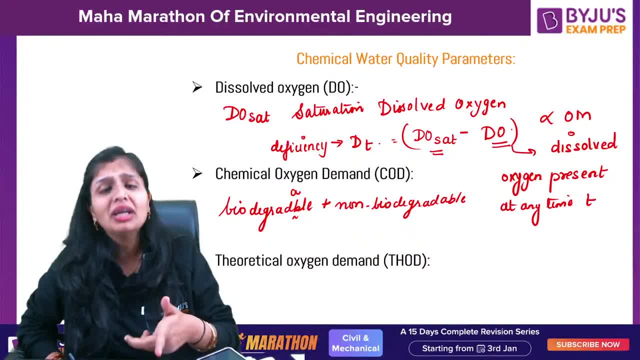 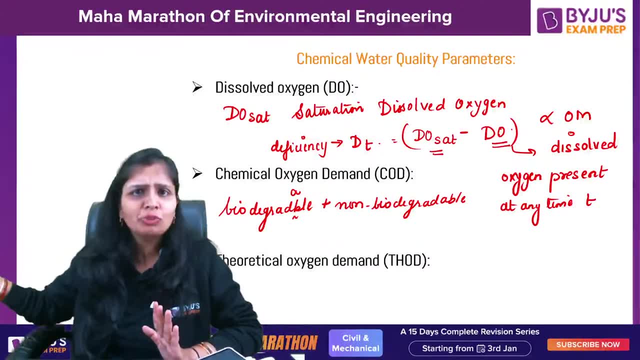 Because beta, it requires money. Moreover, this water, we are not going to drink it Ultimately. after treatment also, you will be disposing the water, So it's not that you will add chemical. the water will become fit and you will drink it. 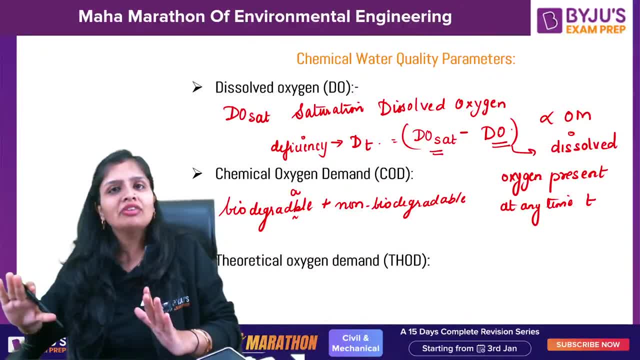 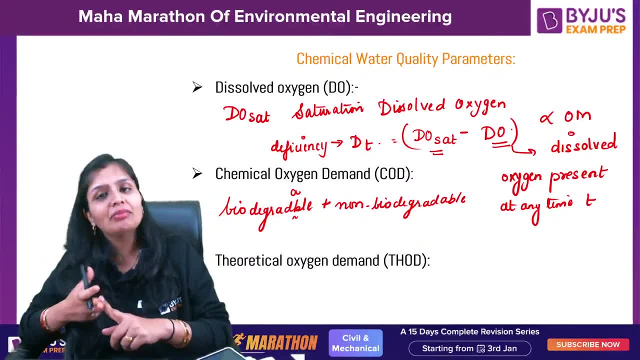 It's not going to happen like that. Okay, So ultimately, what will be happening? you will be disposing it, So that is the reason what you have to do. So chemical oxygen demand biodegradable as well as non-biodegradable organic matter. 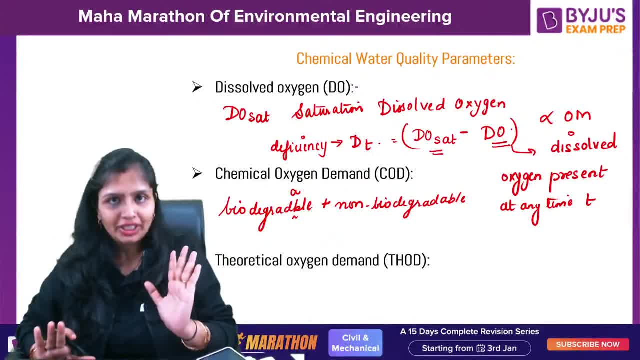 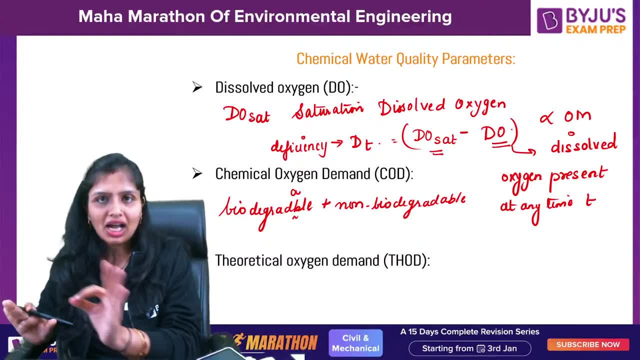 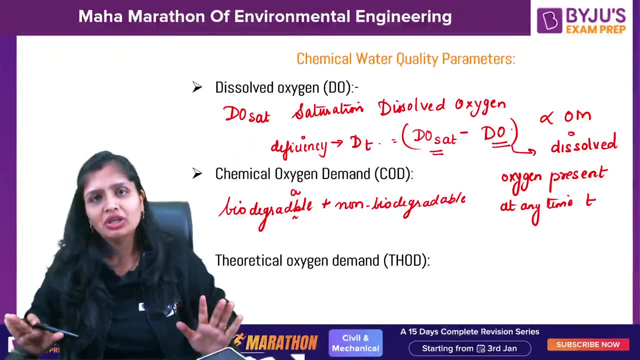 How much oxygen is required, that you will check it out. Okay, Now guys, tell me, do you want that I should tell you? it's not asked, but if you say, I'll write it for you guys, Do you want the test to be also told to you, that dichromate demand test? 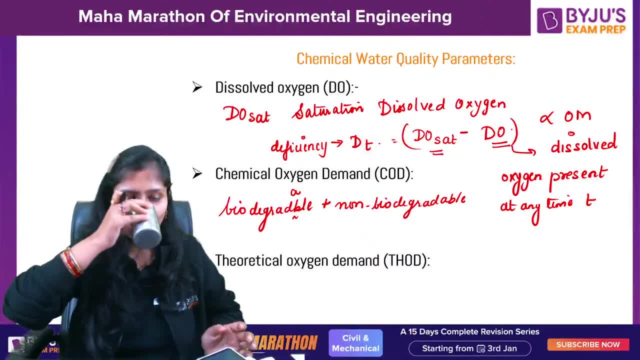 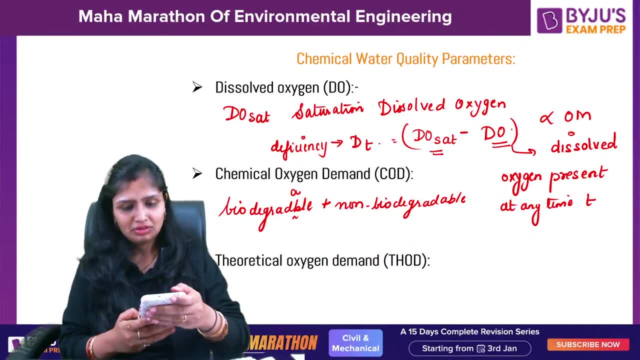 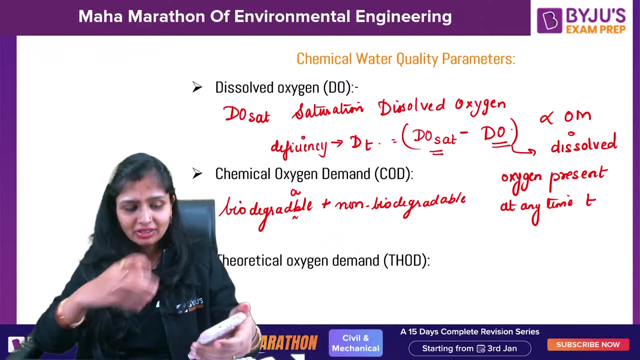 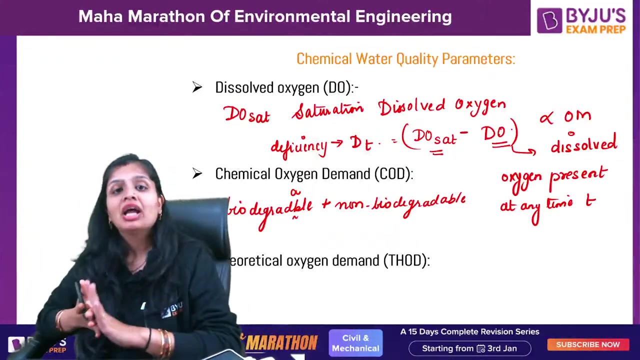 If you will say: I'll do it Fast, Yes or no, No, Not needed, Okay fine. So basically not needed, Okay fine. One thing I'll tell you. Okay, one thing I'll tell you. 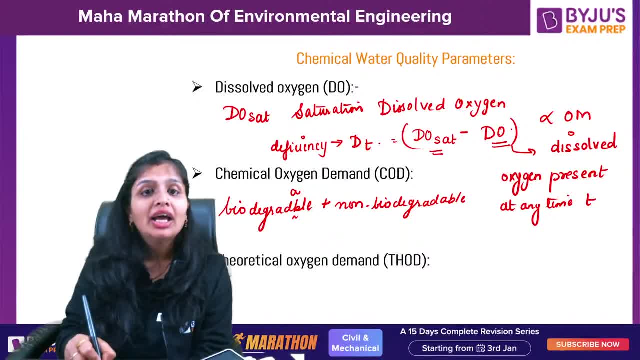 If they can ask you in MSQ questions, Take: Technically chemical oxygen demand is known as dichromate demand test. This you should know. Okay, Here you use K2CR2O7.. So it is known as dichromate demand test. 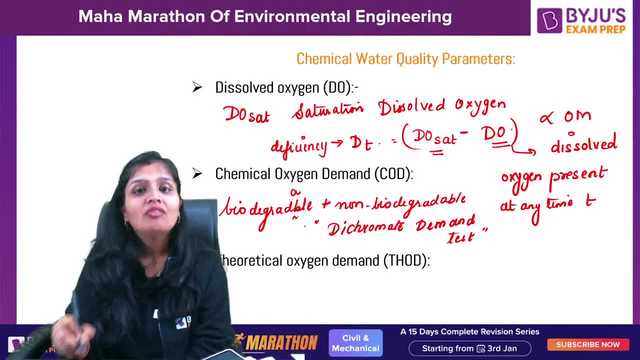 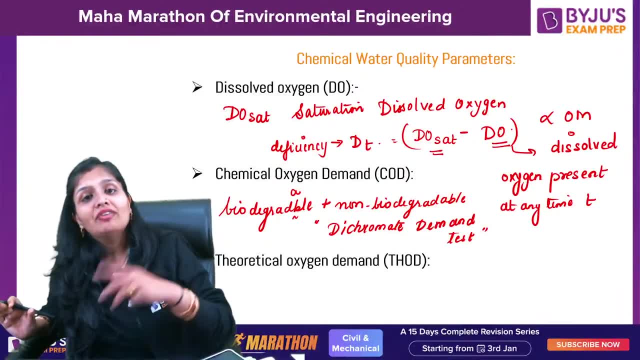 Firstly. Secondly, what happens? What happens? These are statement wise. I'm telling you the important things. Secondly, what happens? What I said, the amount of oxygen required for the decomposition of biodegradable as well as non-biodegradable. 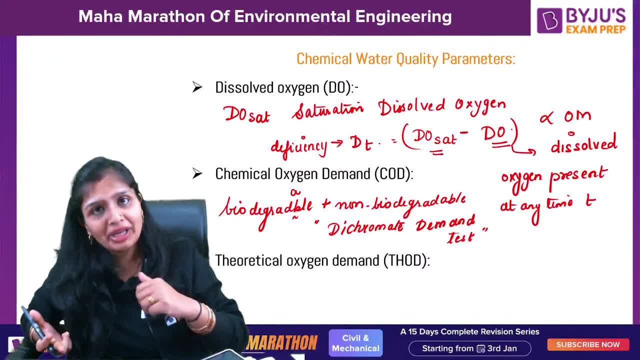 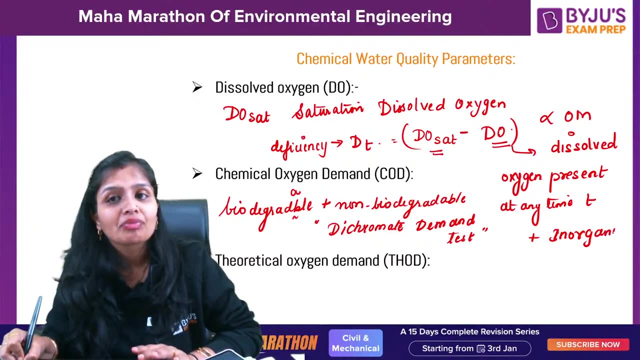 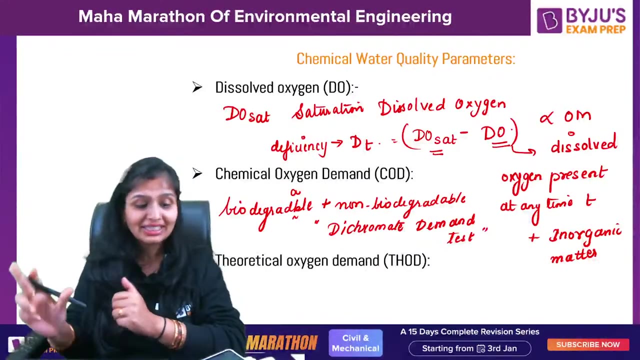 Biodegradable organic matter. but when you add dichromate K2CR2O7, when you add it it not only decomposes biodegradable and non-biodegradable, it also decomposes in organic matter. So that is the reason we say in normal COD test, COD test, but beta it is not a COD test. 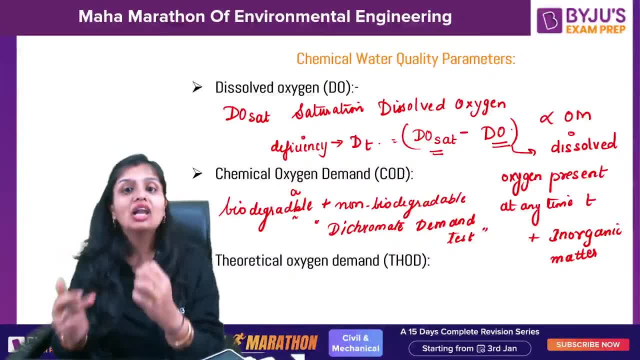 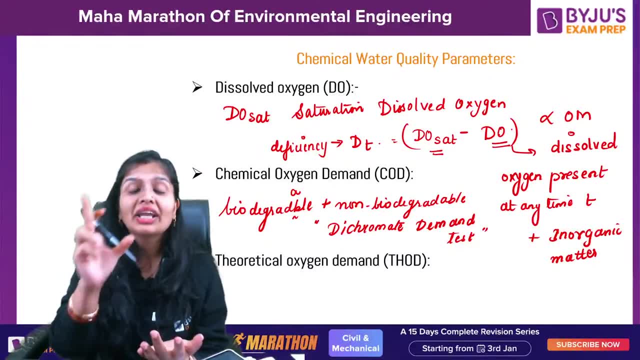 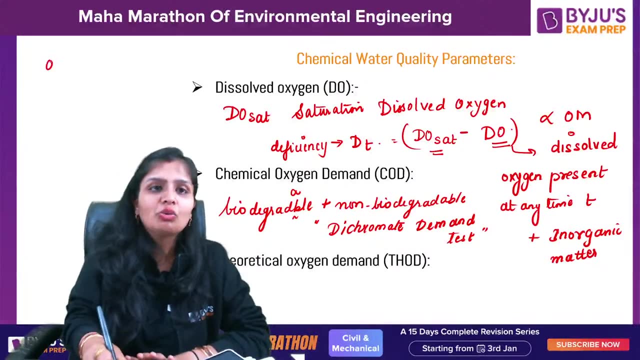 It is a dichromate demand test because along with organic matter So inorganic matter is being decomposed, but organic matter is not completely decomposed. So don't get confused. We say COD is oxygen required for the decomposition of total organic matter. 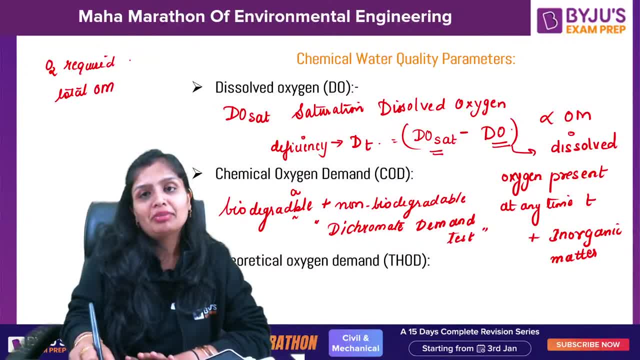 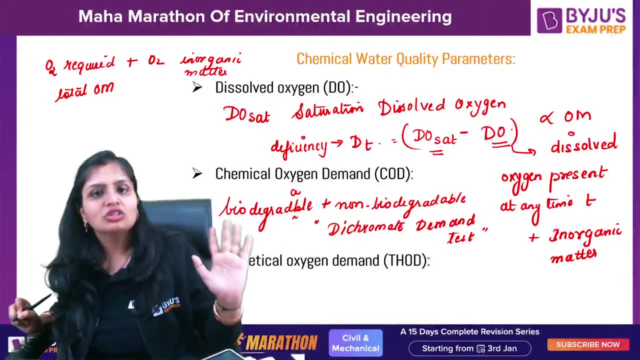 That means biodegradable and non-biodegradable, plus oxygen required for inorganic matter. Then I also told you that organic matter is not completely oxidized Or not completely decomposed. So that is the reason it is known as dichromate demand test. 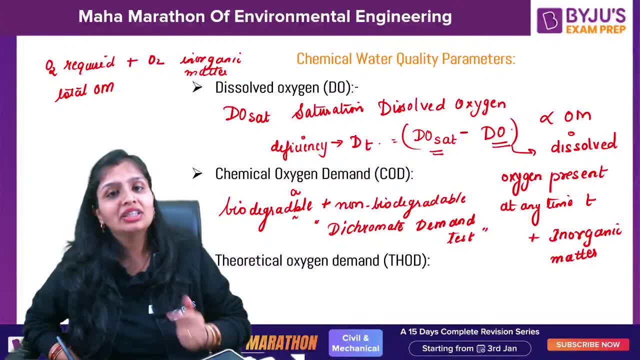 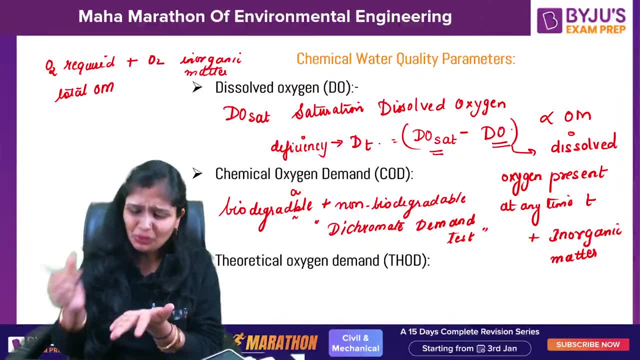 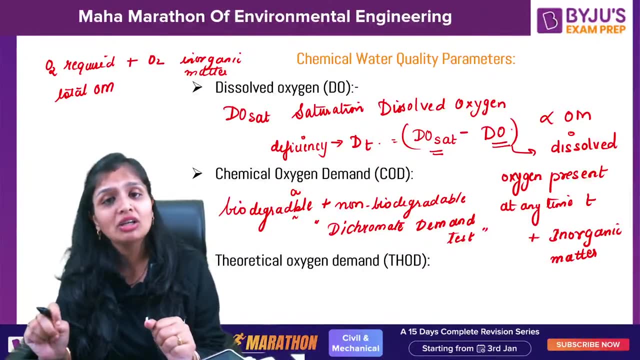 Okay, Now coming further. the next test is theoretical oxygen demand test. Now what happens? This is theoretical in nature. I am doing it in pen and paper. Nothing practical, no experiments, nothing. So when you go by theoretical oxygen test, if you know the type of organic matter, 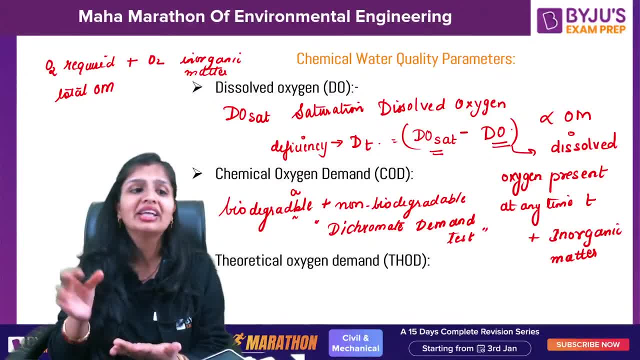 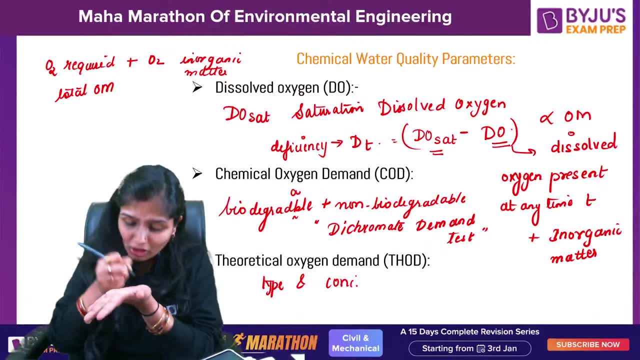 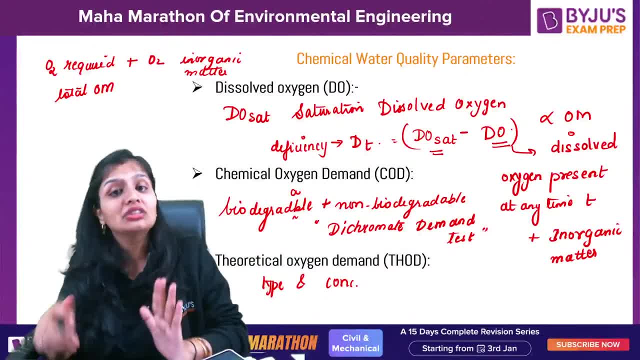 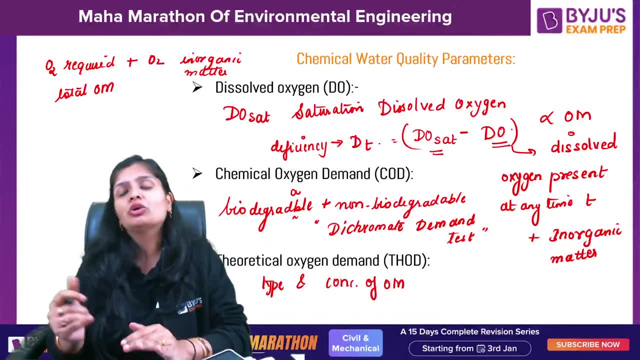 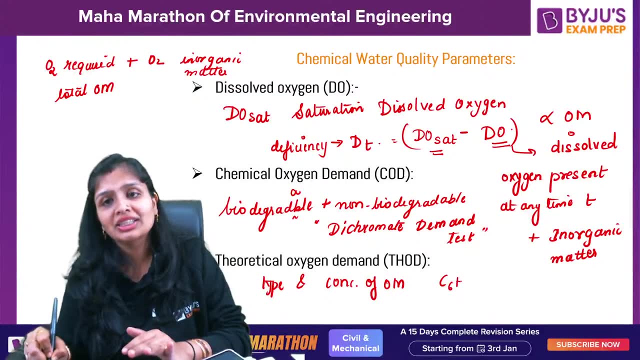 organic matter has taken place, which in practical has not. So if you know the type and concentration of organic matter, how much demand of oxygen is required. that is known as theoretical oxygen demand. Now I will tell you here only this question, this type of question, has been asked. 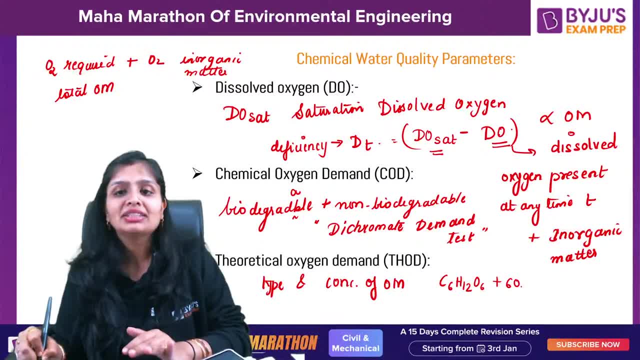 in your gate. So C6H12O6 plus 6O2, this will give you 6CO2 plus 6H2O. So let us suppose we say if 180 grams of glucose requires 6 into 32 grams of oxygen, So in the question it will give you. 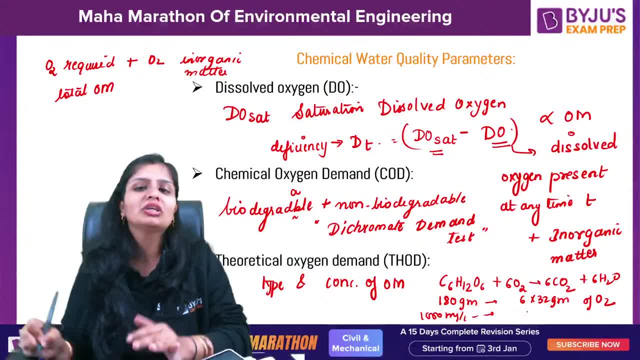 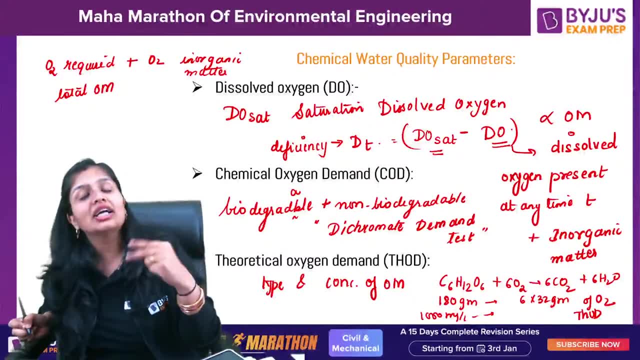 let us suppose 1000 mg per liter of glucose will require how much oxygen. So that will be termed as theoretical oxygen. So that will be termed as theoretical oxygen. So that will be termed as You know. the type of organic matter, it is glucose, The concentration also, you know. 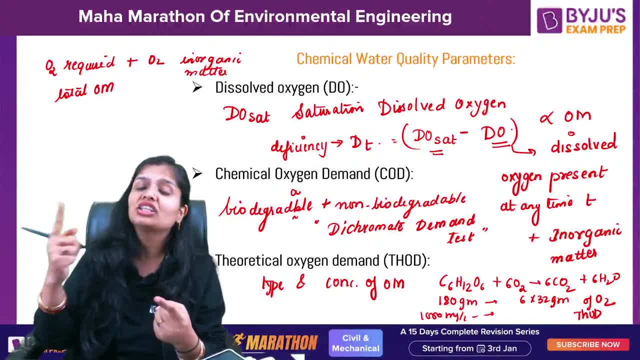 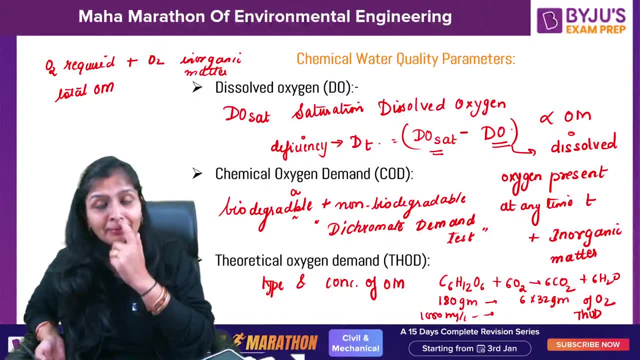 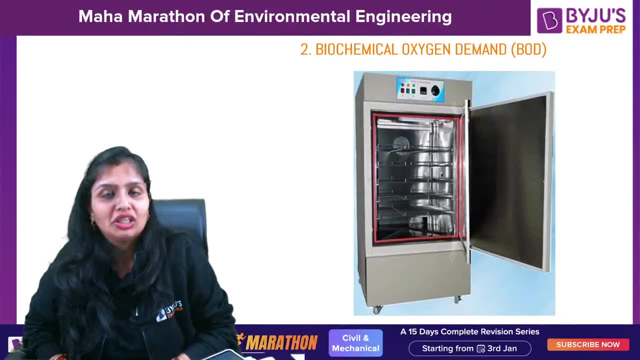 1000 mg per liter. So if the type and concentration is known, you can calculate theoretical oxygen. Simple, Very, very simple. Okay, Now coming further. now coming further to the very important, that is, biochemical oxygen demand, which you call it as BOT. BOT is the amount of oxygen. 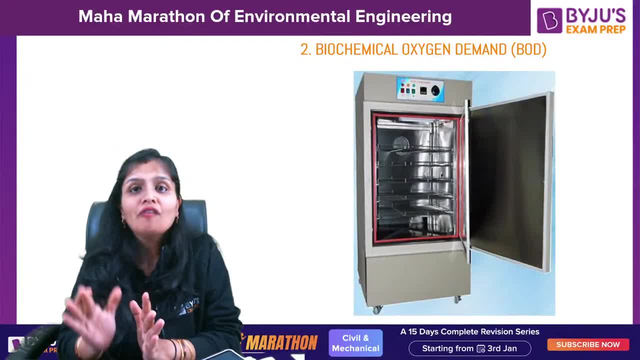 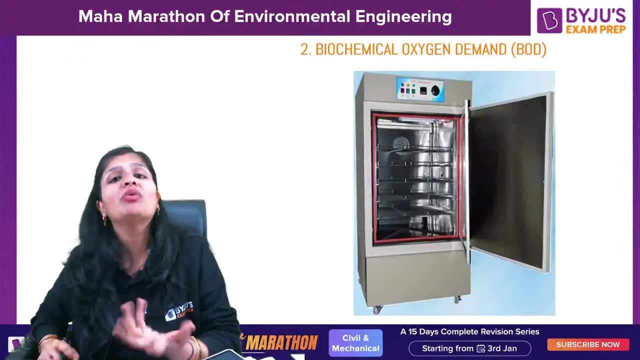 required to produce oxygen. So BOT is the amount of oxygen required to produce oxygen. So BOT is the amount of oxygen required for the decomposition of biodegradable organic matter. Remember the amount of oxygen required. to be precise, who requires oxygen? Aerobic microorganisms. 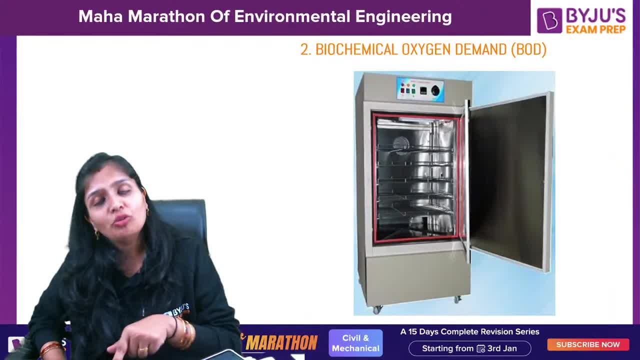 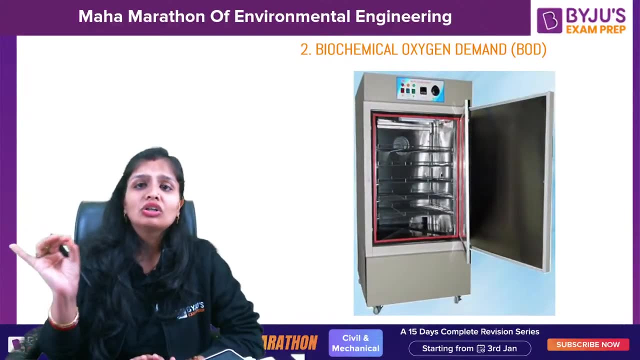 So the amount of oxygen required by aerobic microorganisms for the decomposition of biodegradable organic matter is known as biochemical oxygen demand. In short, we call it as BOT. Now if you want this oxygen demand to be calculated, you need three things. If you want BOT, you need organic. 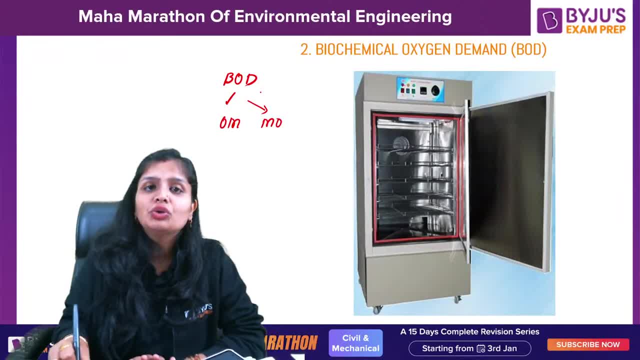 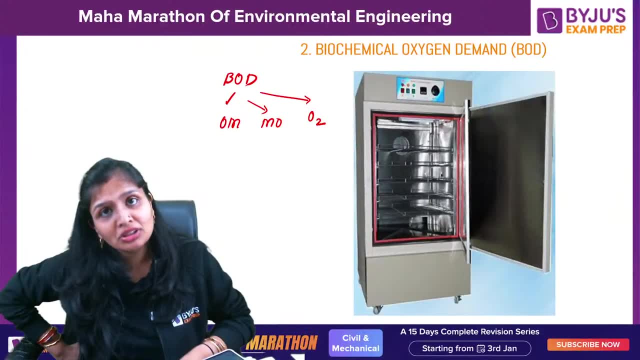 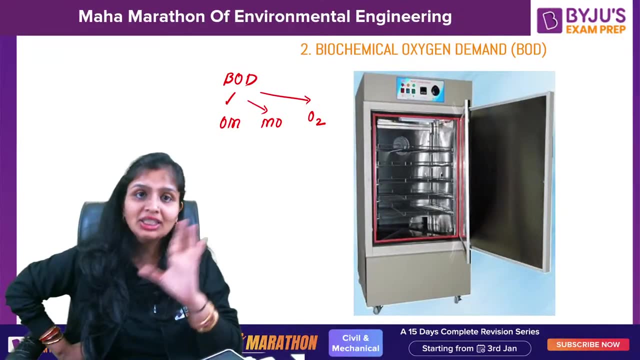 matter. you need microorganisms, you need oxygen Ma'am. if oxygen is not present, you will add oxygen Ma'am. if microorganisms is not present, you will bring microorganisms from other plant and you will add. Okay, So this, you have to do it Now. coming further, three cases are there. Generally, 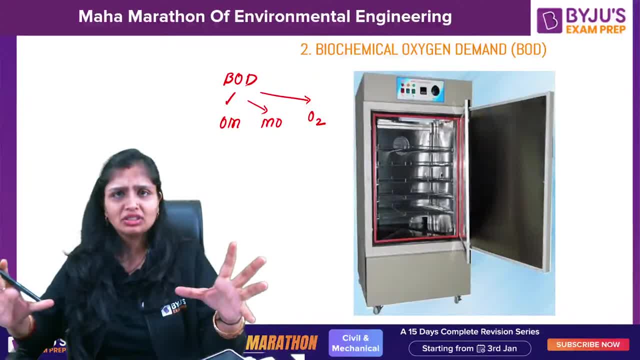 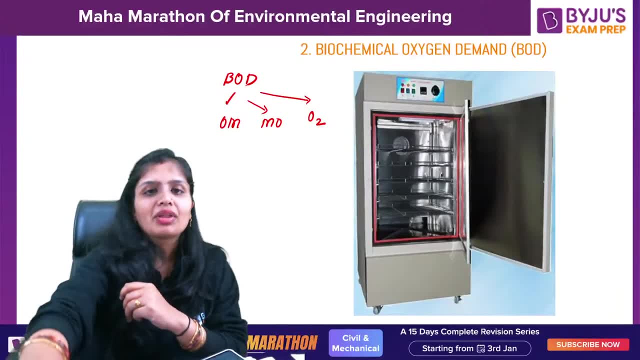 the third case is not asked. So basically we'll do two cases. If you want, we'll do the third case also, but most prominent, one case is asked out of these three cases. Okay Now, first case is: let us suppose case one is: 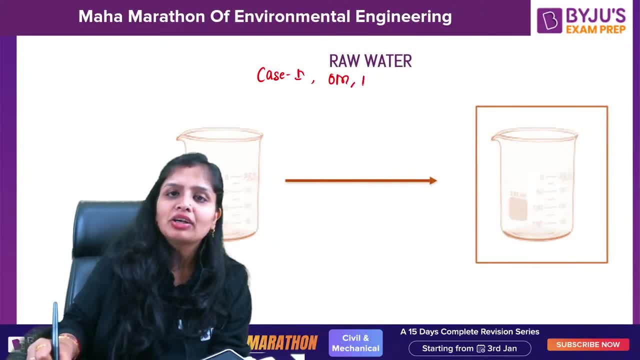 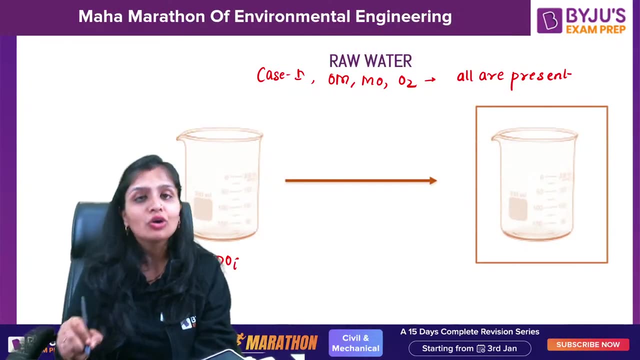 when organic matter is there, microorganisms is there and oxygen, all are present. So what you will do is you will take the sample, you will measure the initial dissolved oxygen. Ma'am, how do we measure? There is a test known as Winkler's method. Okay, Generally, firstly, 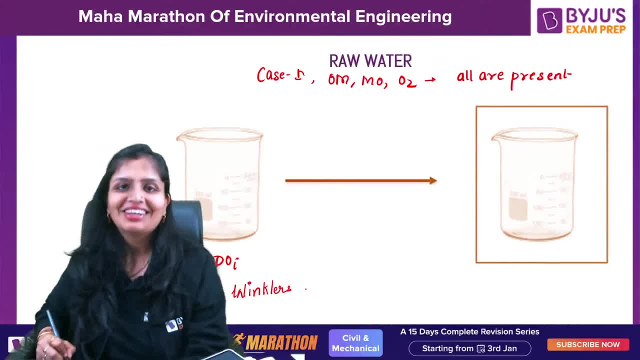 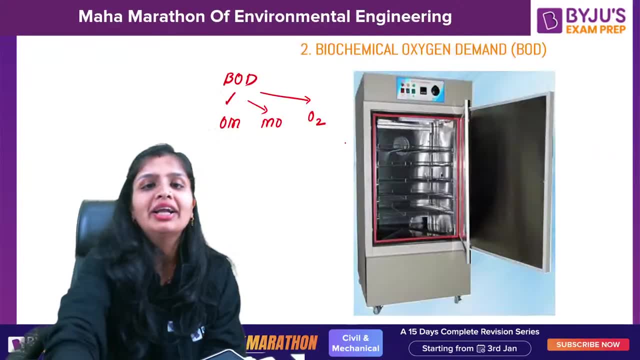 I for a remembering purpose. I used to remember like Wrinkler's, So it's Winkler's method. So you can measure the dissolved oxygen initial by Winkler's method. You will put it in this incubator. 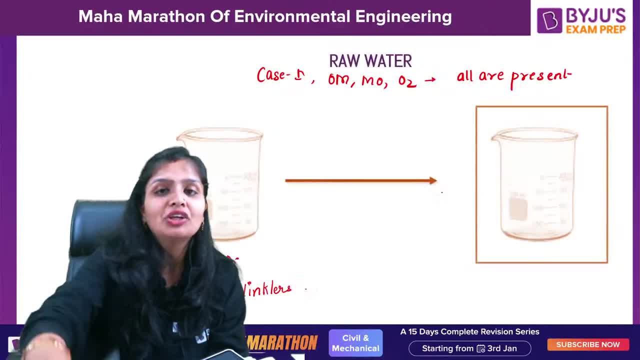 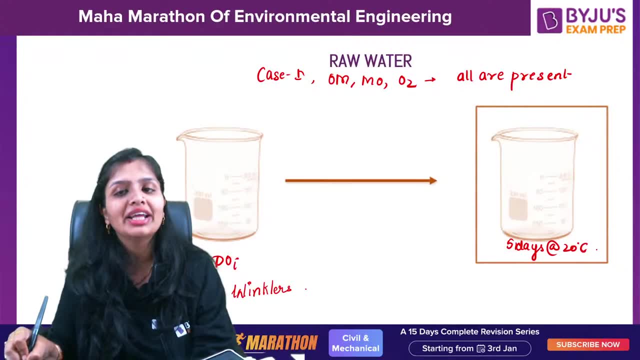 You can see this incubator. right, You will put it in this incubator for five days, 20 degrees Celsius, And after five days you will take it out. You will take it out and you will put it in this incubator and you will check. after five days you will check it out. the dissolved oxygen: final. 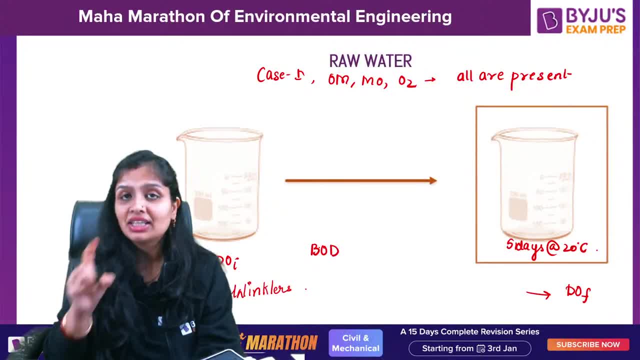 So you will say, since you incubated for five days, I told you here you are totally dependent on microorganisms. For microorganisms, temperature and days are very, very important. So BOD for five days at 20 degrees Celsius is DO initial, minus DO final. In this case, microorganisms was there. 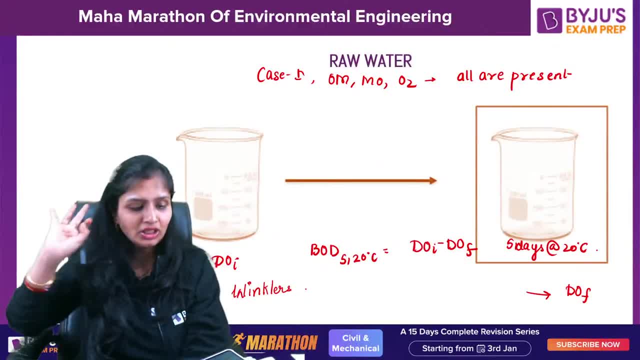 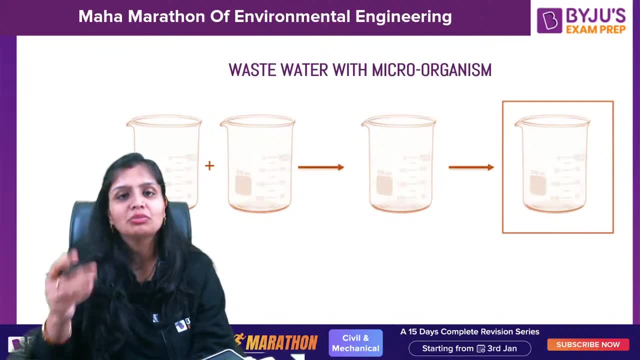 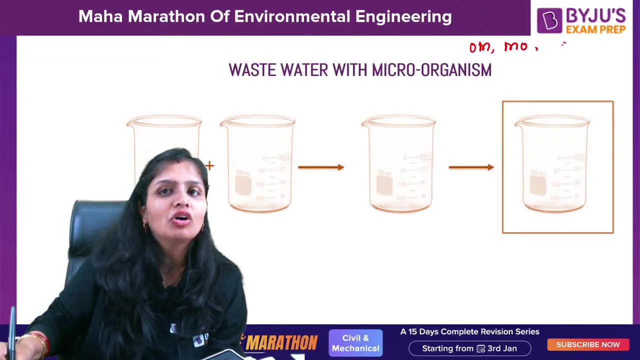 organic matter was there. So you will take it out and you will check it out. the dissolved oxygen, final. So this was the case, first case. Now let us suppose what is happening: Organic matter is there, microorganisms is there, but oxygen is absent. Now how you will do. Now, how you will. 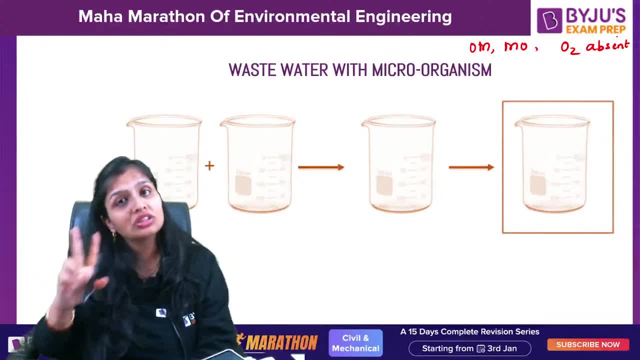 come that oxygen is absent or, second, the oxygen is not present in sufficient quantity. In the same way, you will take it out and you will check it out: the dissolved oxygen final. So you will take it out and you will check it out. the dissolved oxygen final. So, in the same case. 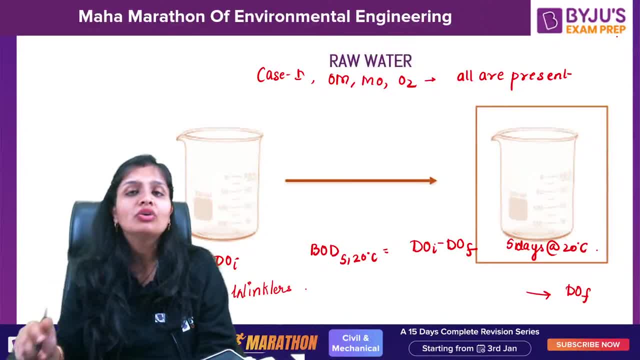 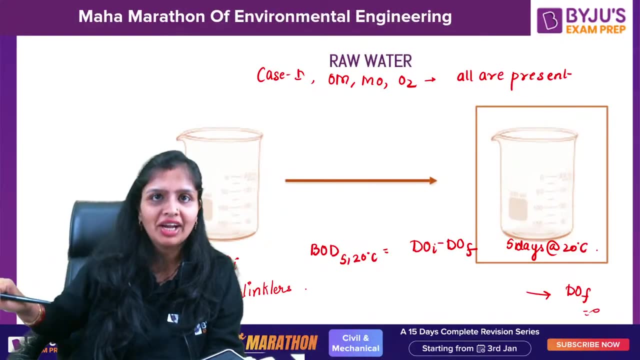 let us suppose you conducted that test and you found that dissolved oxygen final comes out to be zero. In this case, you cannot do that. This experiment will become wrong, Why? Because you took the sample out after five days and you found that the dissolved oxygen final is zero. 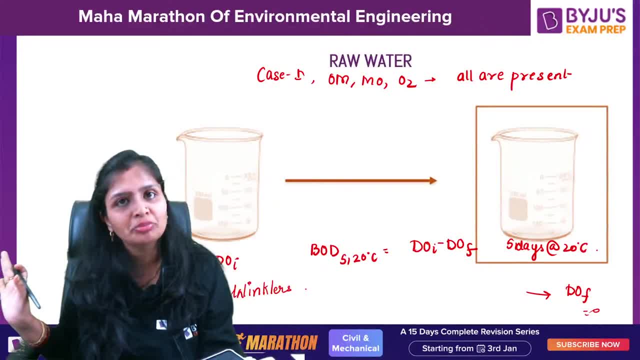 But it might happen that on the second day the entire oxygen was being used. On the very first day the entire oxygen is used. But you are telling the wrong thing. You are putting it as five days BOD, but it might be possible that the BOD would have been of different. 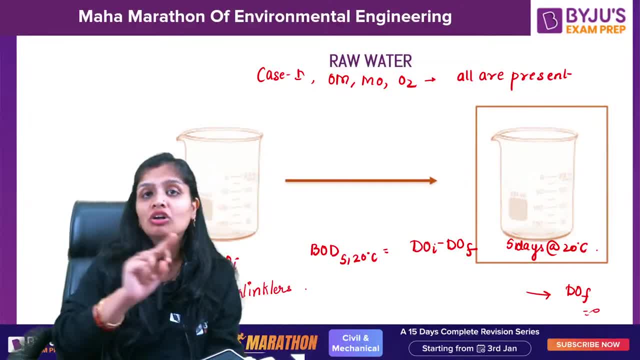 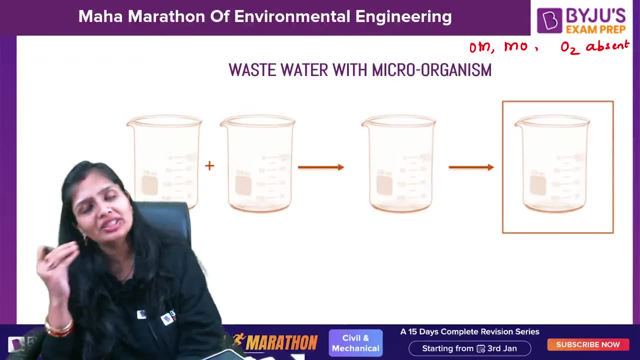 day. So that is the reason when you get dissolved oxygen final as zero. this pattern question has been asked in your gate. You do not consider that reading. That reading is wrong, That reading is eliminated. So, ma'am, if such condition happens, if O2 is absent or is not present in sufficient, 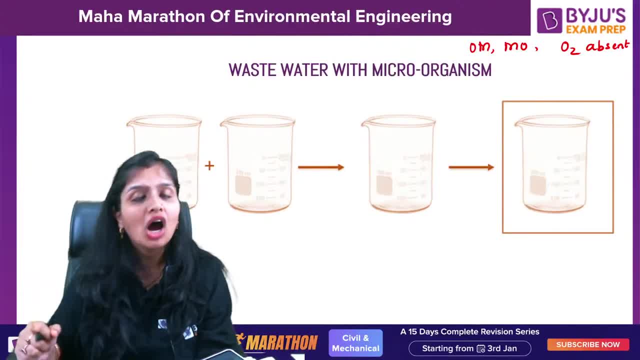 quantity, then you need to add O2.. How you will add, You will take the sample out and you will take a distilled water which is fully saturated with oxygen. Fully saturated means if it is at 20 degree Celsius, the oxygen which should be present is 9.2 mg per liter. It should not contain any. 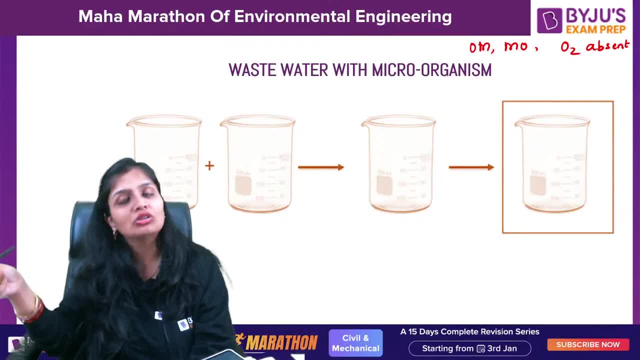 organic matter. Why, If organic matter will be there, so in that also microorganisms will be there, In that also oxygen will be used, So it should be distilled water. It should not have O2.. These are used. Okay, Okay, Harish, They will do it. That's true Whenever you study theory, whenever you do. 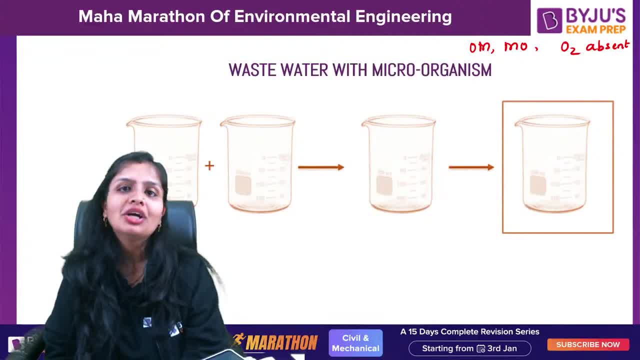 practical. there is lots of difference. As I also told you, when you do it here, you do it by geometric mean method of population forecasting. When you go there, you will do arithmetic mean method Already. they know. My students already know. I don't think that they need your advice. 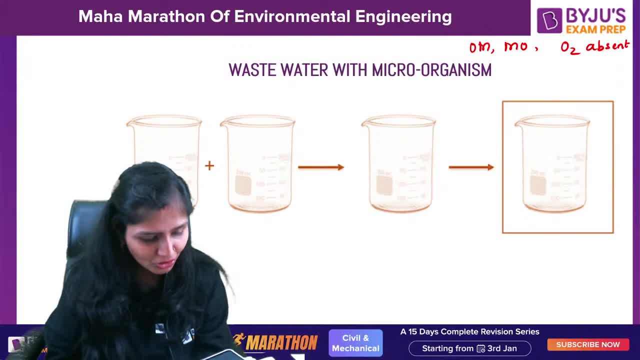 for this purpose. Yes, she is BOD. 5 is removed oxygen or remaining 5.. They always. I get confused. That point also. I will take it out. Okay So, Harish, thanks, but no thanks. Okay, So when you talk about waste water, as I 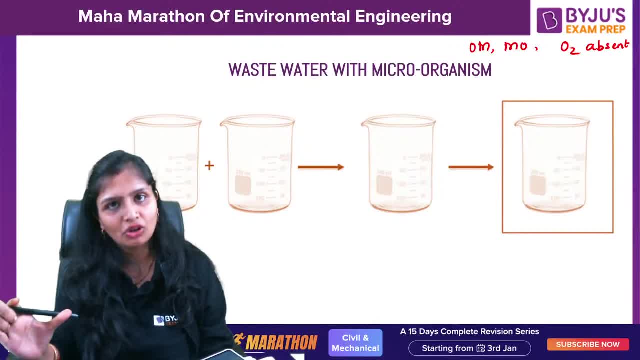 told you. you take that water which is fully saturated with oxygen, Okay, And there shouldn't be any organic matter and microorganisms present. Now, if this is the volume of the sewage, okay, it will have some dissolved oxygen and this will be the volume of water. It will be having some dissolved oxygen. This is dissolved oxygen. 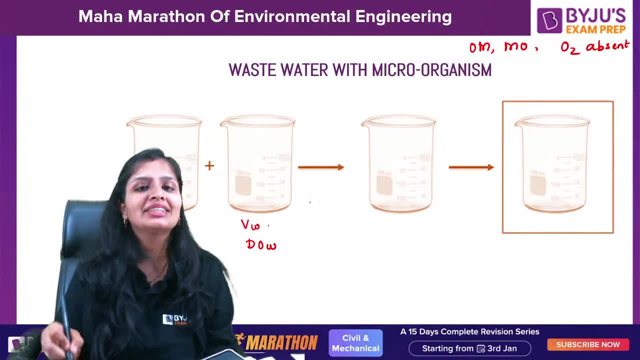 of sewage. This is the dissolved oxygen of water. You will mix them. So now the du mix will become how much you can discharge. also, You can add it or you can add it the volume here: Volume of sewage into dissolved oxygen of sewage. volume of water: dissolved oxygen of water divided by volume of. 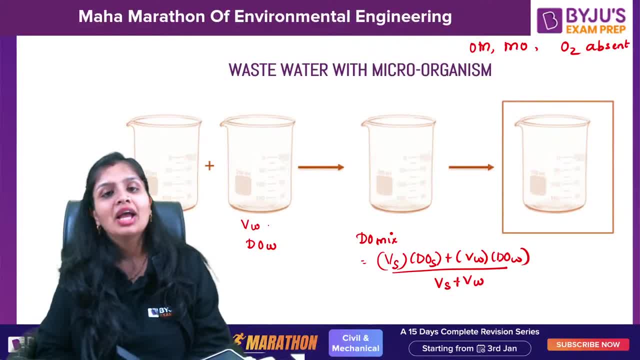 sewage plus volume of water. Okay, So you will get du mix, which is initial. Now you will put it in the incubator. After 5 days, when you take out the sample, you will get the du final mix. So when you calculate, 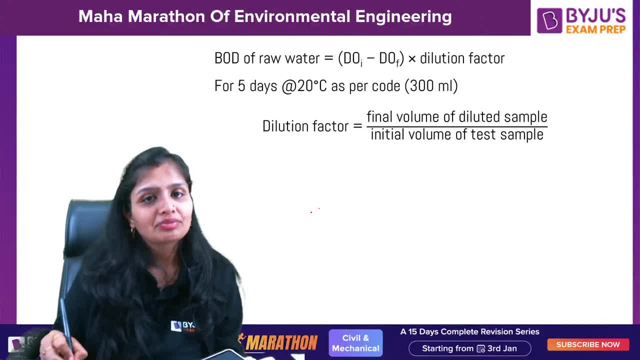 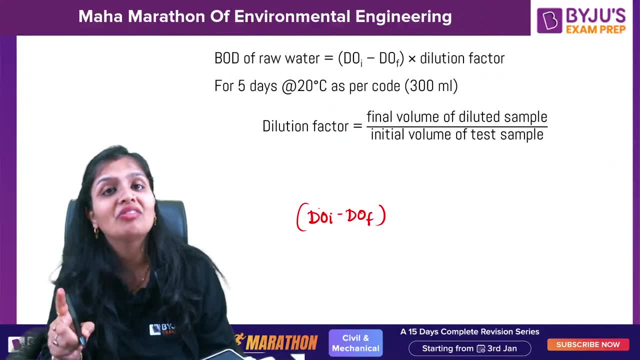 the BOD BOD is du initial mix minus du final mix. This is not the BOD of the test sample. Why? Because you added water in this. For removing water, what do you have to do? You have to multiply by the. basically, for getting the BOD of the test sample: not removing for. 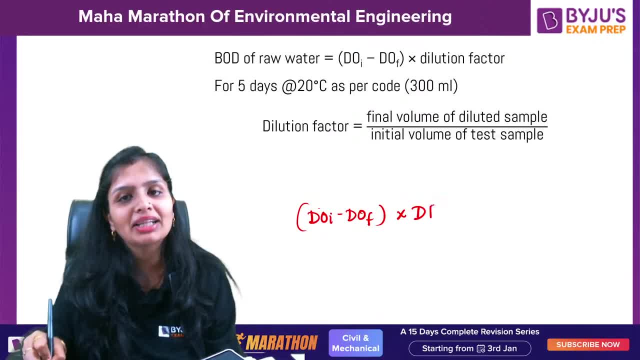 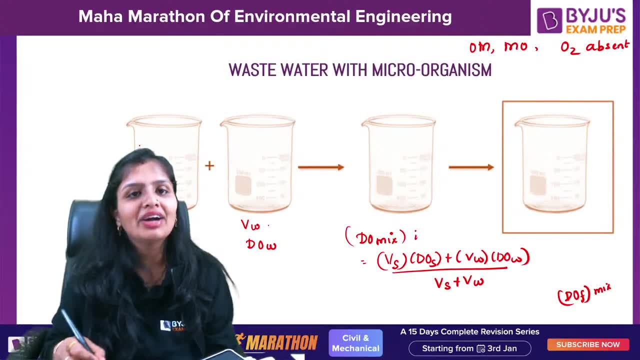 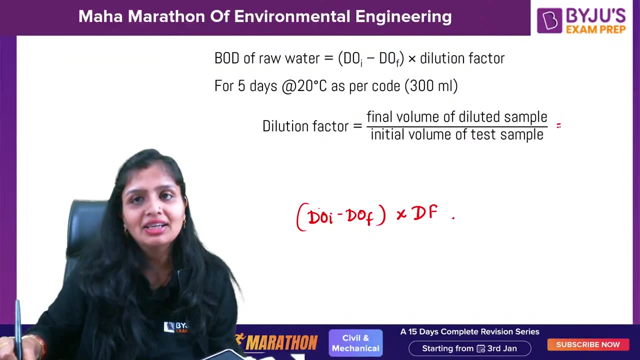 getting the BOD of the test sample, you need to multiply by the dilution factor. And what is dilution factor? Final volume of the diluted sample divided by the initial volume of the test sample. Okay, So how much water you added? Like, if I want to say, I will say final. 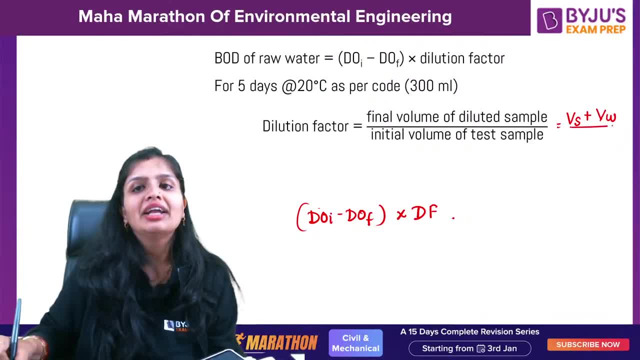 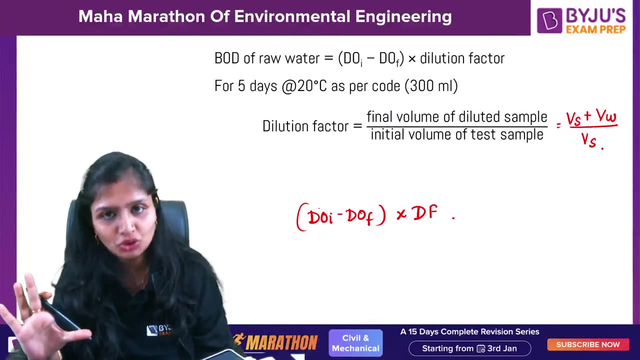 volume is the volume of sewage plus volume of water divided by the volume of sewage. This is the dilution factor, As per the code, the BOD bottles which you take it. that is 300 ml. 300 ml is the size of the BOD bottles which you take it. Okay, So if you incubate, 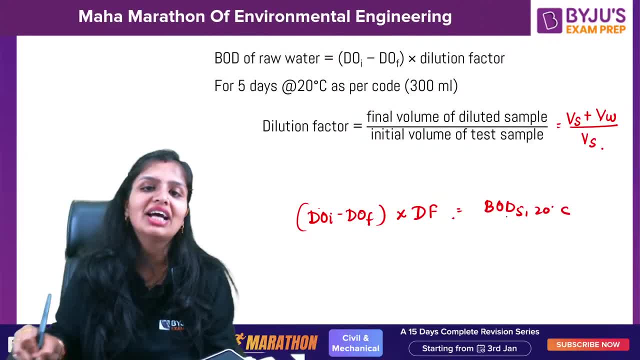 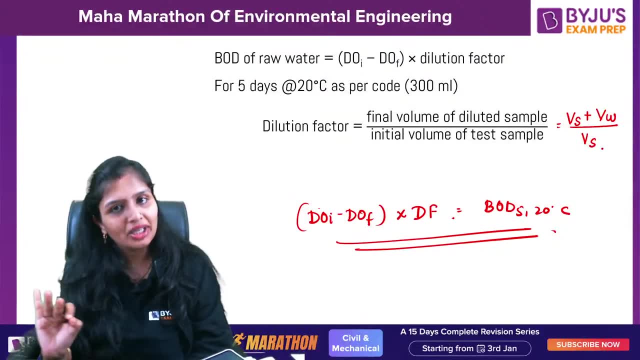 it for 5 days. the BOD which you will get is for 5 days at 20 degree Celsius. this will be the BOD. So generally till now in gate examination, whichever questions have been asked, they go by this formula. That's it. 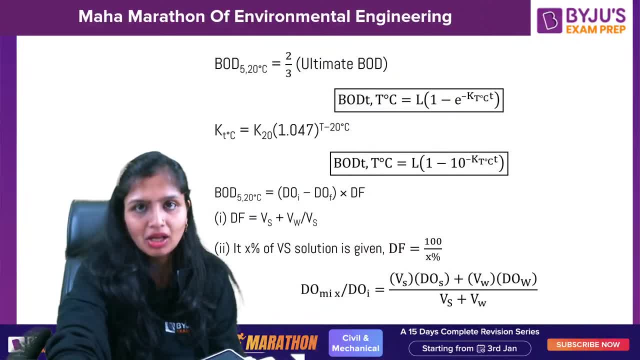 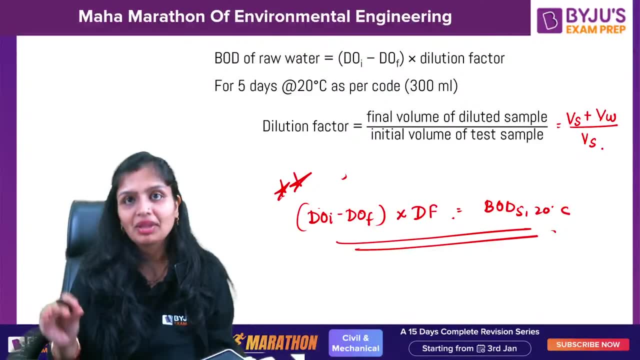 Till now, the scenario has not changed. Okay, Now, as already told you, now she has. was asking- now let's go further- Why we take 5 days BOD, Generally 5 days BOD, if you. 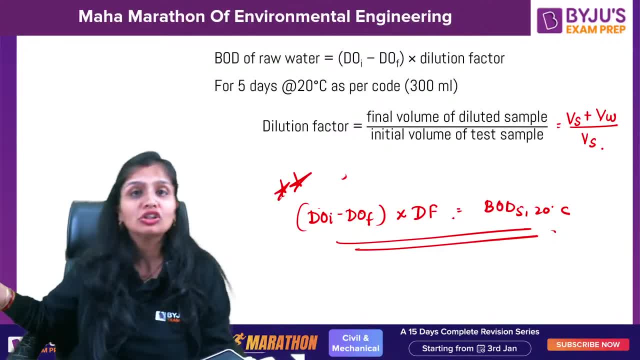 want to take that ma'am. I want to know when complete decomposition of organic matter will happen. Not even a single organic matter is there, So that will take. that will take large time. Large time means infinite, So that decomposition will take infinite amount of time, Okay, Firstly. Secondly, we 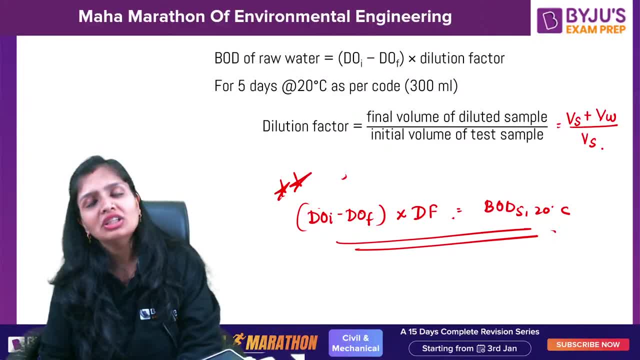 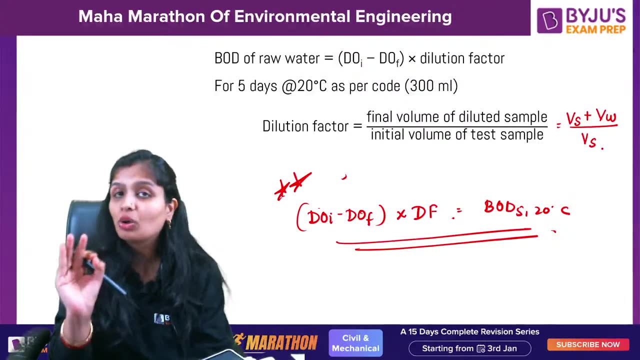 go for 5 days, 20 degree Celsius, because here, 2 by 3, or you can say 66.67% of the decomposition of organic matter has taken place. There is a term known as ultimate BOD. Ultimate BOD is the amount of oxygen required by aerobic microorganisms for the decomposition of two. 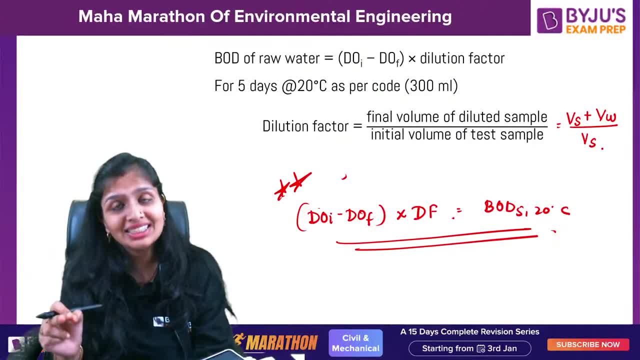 biodegradable organic matter. So for this it requires infinite time. However, ultimate BOD is independent of temperature. It remains same. Okay, It won't change whether you make it 20 degree Celsius, 30 degree Celsius, But there was a curve, you remember, and it was. 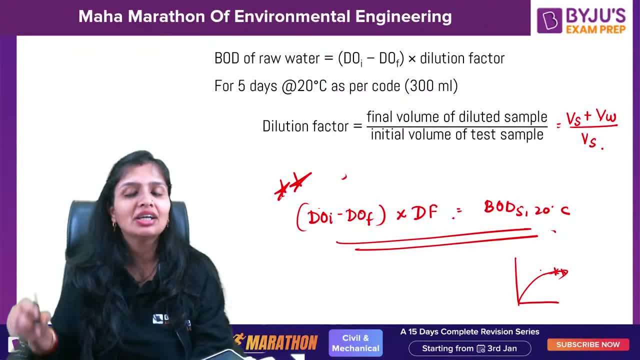 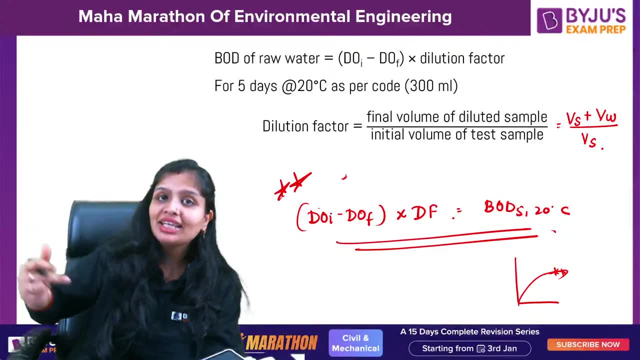 like this curve which is there and it used to tell you that this curve, when you increase the temperature, where it will shift, it will shift to the left. Why? Because when you increase the temperature, it will shift to the left. Why? Because when you increase the temperature, 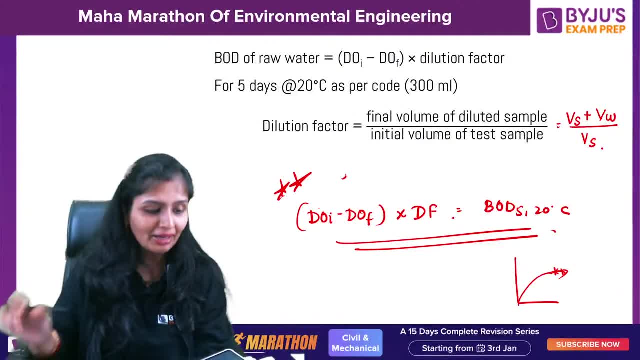 it will shift to the left. Why? Because, when you increase the temperature, it will shift to the right. Why? Because you increase the temperature, it will shift to the left. Why You increase the temperature, it will shift to the left. Why is that You don't increase? 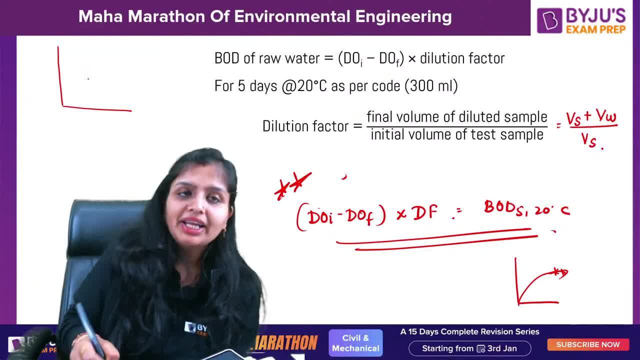 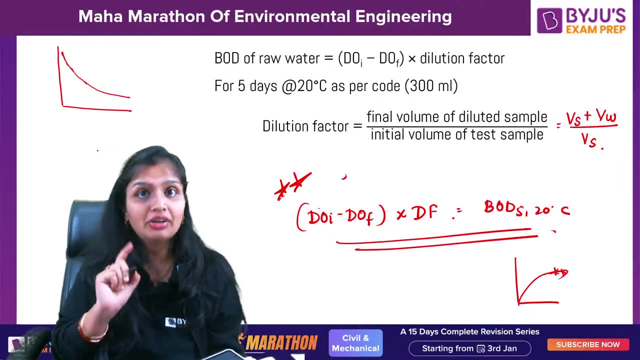 the temperature, It shifts to the right enough time. So that's why you require 50 times per day. so you pesos more, Okay, And so what more you do, Then once a year and 15 years it will increase. 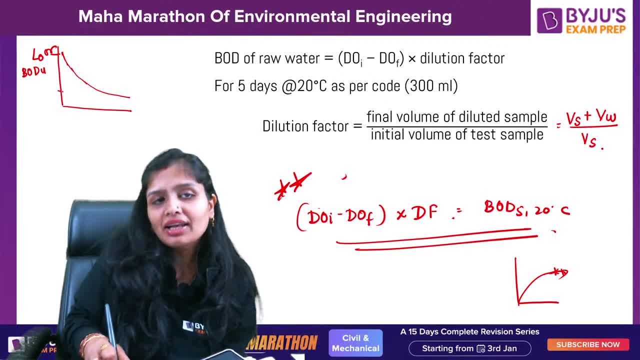 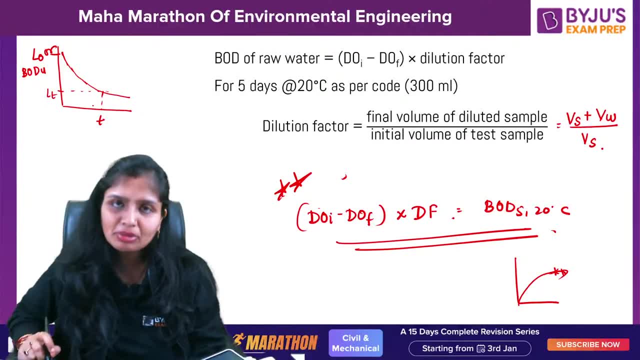 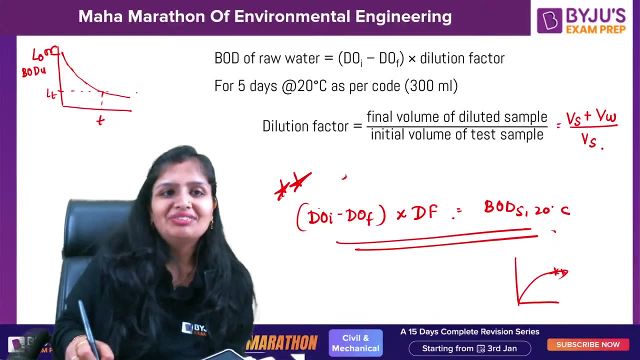 ultimate that depends upon. I want to calculate the value of BOD at any time t. Now you guys get confused in maximum cases, whether it is asking about BOD consumed or it is asking BOD remaining By this graph. you know that. let us suppose at any time t I am talking. 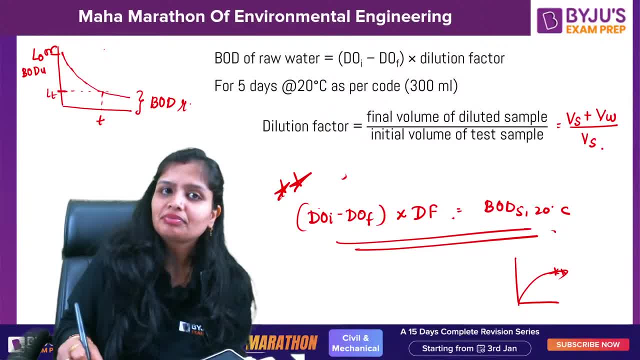 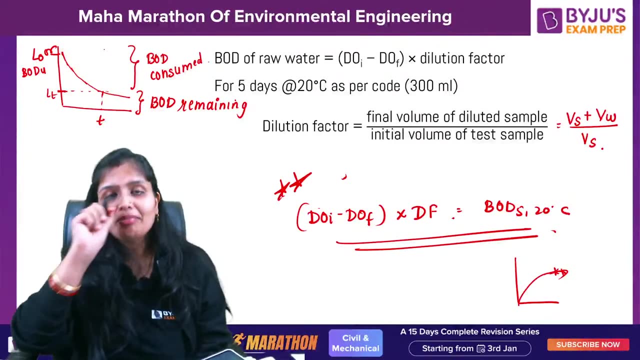 about. So this is the BOD which is remaining and this is the BOD which is consumed: L0 minus L, This is the consumed BOD. Now, when maximum students, when you are getting confused, let us talk about it. Yes, I agree two, three points. let us discuss first In the portion: sometimes 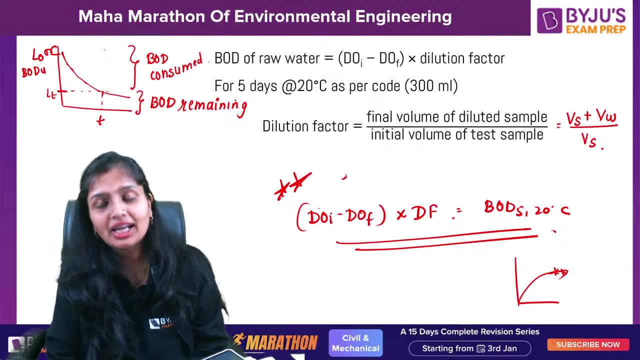 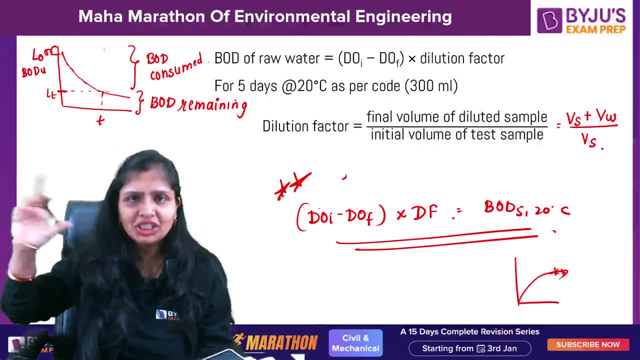 they write it as BOD remaining, which is easy to understand, But sometimes they do not mention So generally if they say BOD 10 km downstream, Yes, you are getting confused now: BOD at 10 km downstream. So that time it is talking about the remaining. 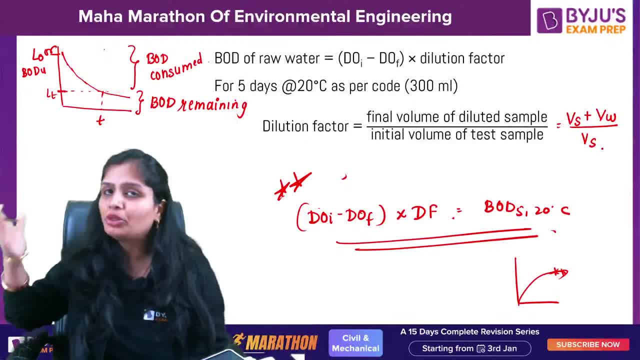 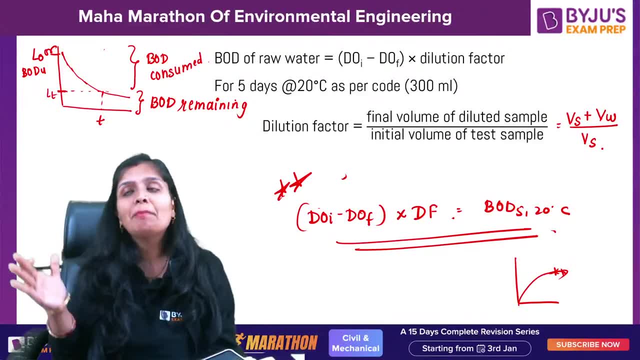 BOD That out at 10 km downstream. what is the BOD which is there? Present, Present means remaining. Now, if you see the past year's papers where the sentence was not clear, that time it is not mentioned Anything. we go for BOD consumed. But if it is telling BOD remaining, or it is telling 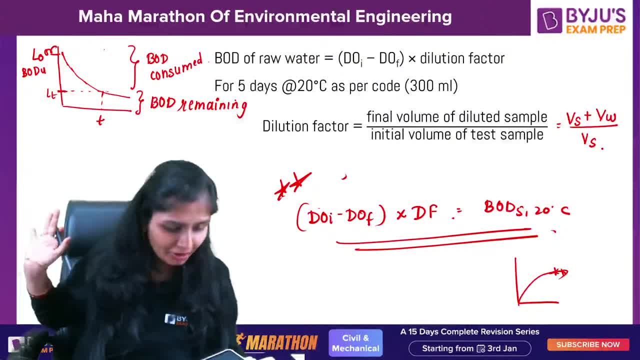 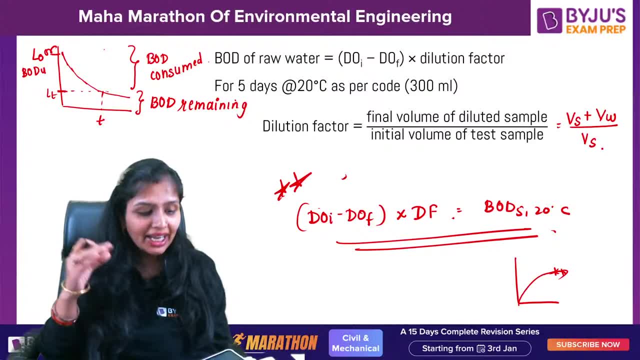 at 10 km downstream. what is the value? then you go for BOD. remaining Clear, What does the BOD 5 day test measures? It will measure how much oxygen is required by whom- by microorganisms. Why do microorganisms require oxygen? because they want to carry out the decomposition of 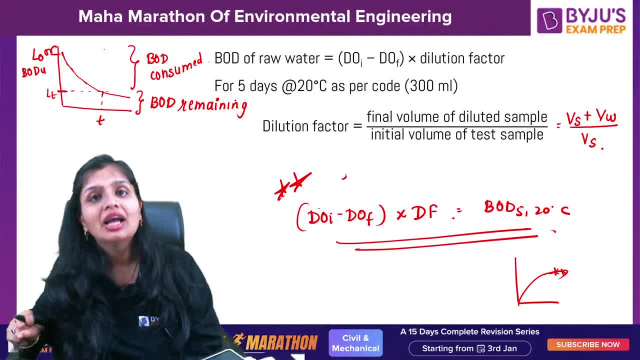 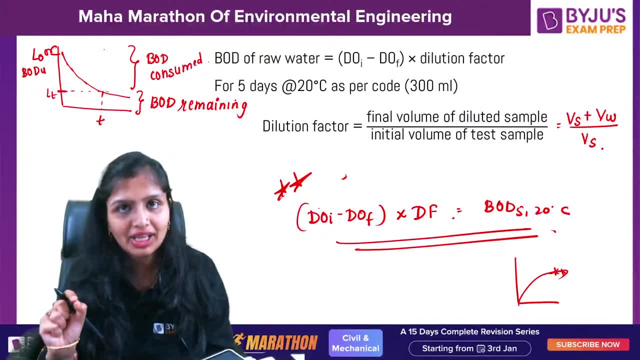 biodegradable organic matter. Okay, Because in practical, your sewage, my house sewage, everybody's sewage- is treated by microorganisms. We don't go for chemical treatment, we go for biological treatment. Okay, So we want to see Ma'am, but why you want to calculate the oxygen? because if we 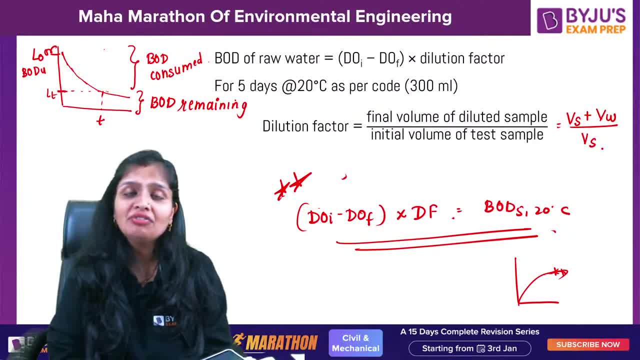 go for now. I will be telling you after this treatment method. So if you go for ASP- activated sludge process and all there- you will be the one who will be supplying oxygen. So that is the reason you are testing the oxygen. So that is the reason you are testing the oxygen. 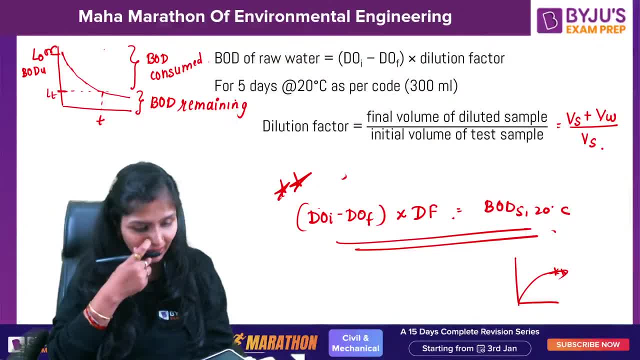 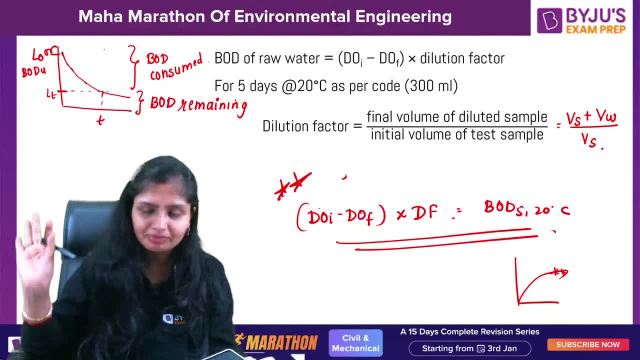 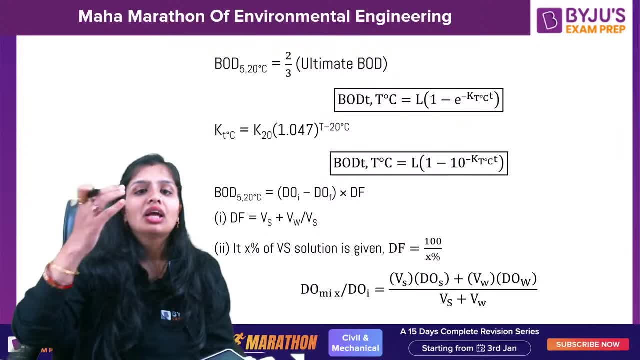 BOD ultimate is in breathing in the independent of temperature Correct. Yes, yes, pushed. Okay. Now BOD 5 days is 2 by 3. as I already told you, there are 2 formulas. One is 1 minus e, K to the k into T, and this is K d t K and K d t, Third formula. So this is 2 by 3 and 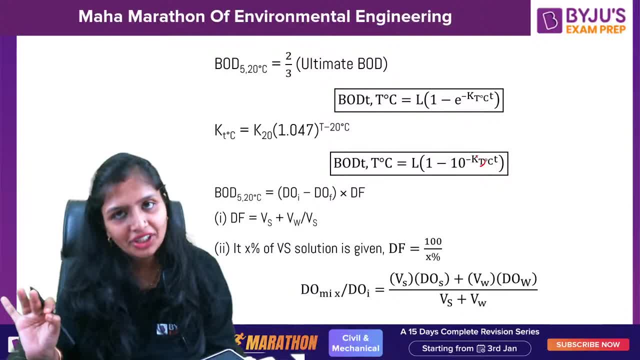 1 is 1 minus e, K into n, into t, and this is K? dt. K and K? dt are equal to 2 by 3 and the k and kd are deoxygenation rate constant. one is base e, one is base 10. let me tell you one thing. 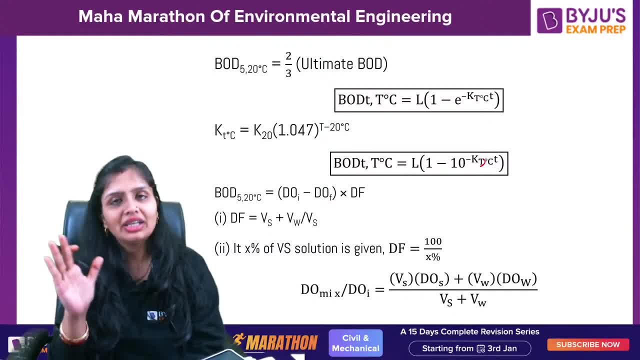 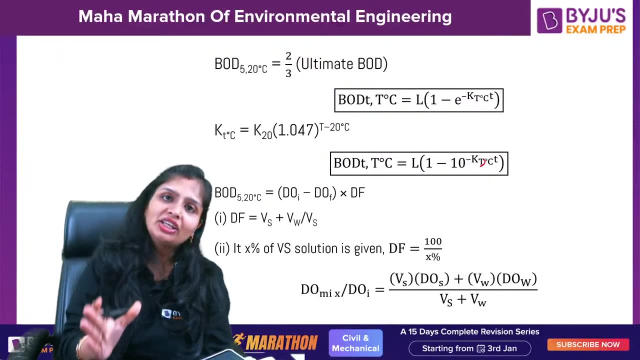 before. if you see before five years papers, in many cases they don't use to mention whether the value of k is base 10 or base 3. but since you are preparing now and since you are attempting for this time, you don't have to worry, they will give you in the question that deoxygenation rate. 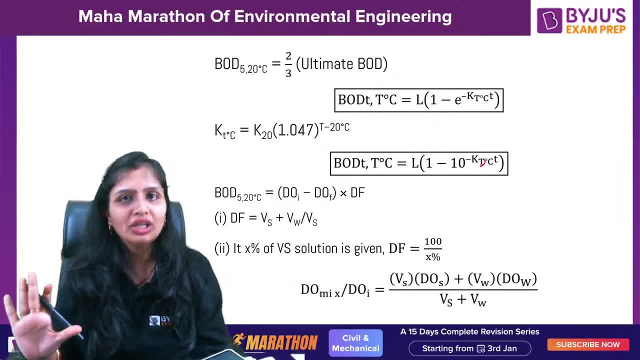 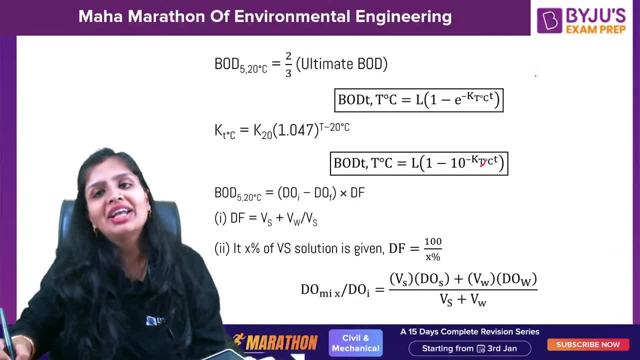 constant is base 10 or whether it is base e, so you don't have to worry. okay, if you see the past 90s paper there, it used to be happen. but i'll tell you a hack. also, when it is 0.23, 0.22, generally, it 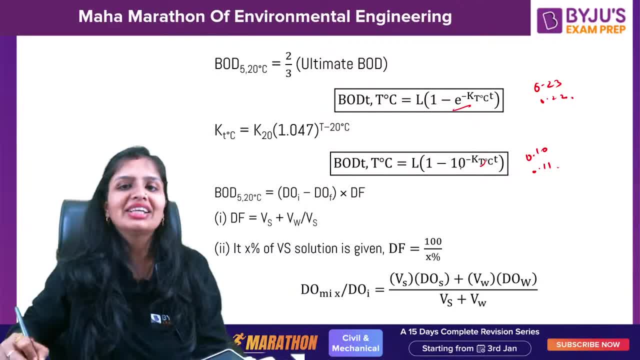 is base e. when it is 0.10, 0.11, then it is base 10, but you don't remember this because generally they will give you the deoxygenation rate constant base e or base 10. okay, now dilution factor i. 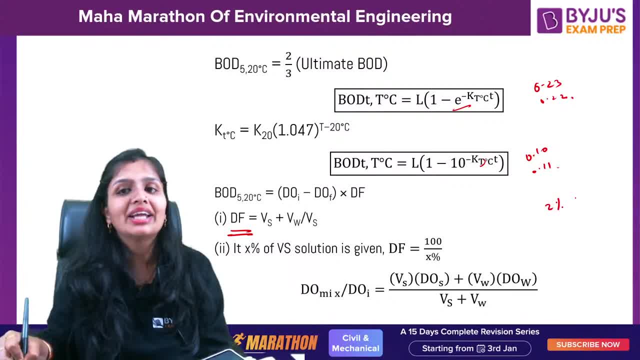 already told you. sometimes they say that 2% dilution is done. this is very important. so if they write 2% dilution, okay, that means that means what. that means what? let us suppose if 2 ml will be the test sample and 98 ml will be the distilled water, okay, so this is the meaning of it, so don't need to do it, see. 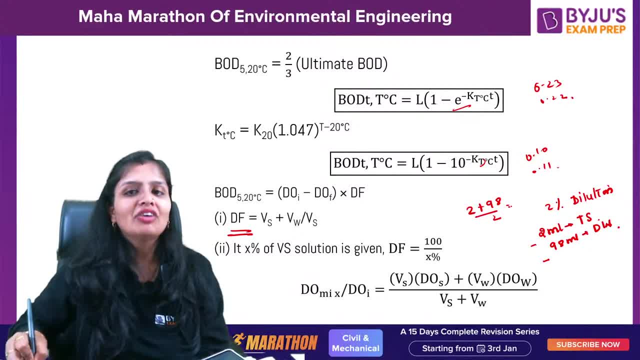 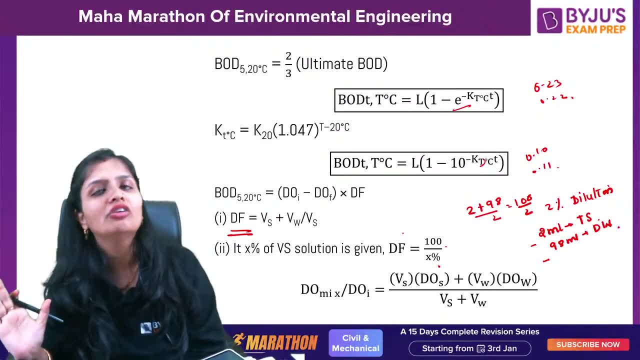 if you do 2 plus 98 by 2. so ultimately what will happen? 100 by 2? it will come, so directly they are going to give you the deoxygenation rate constant. so this is the meaning of it. so don't give a stupid form of it. it is ingredient here. so if you know that it will come, it will. 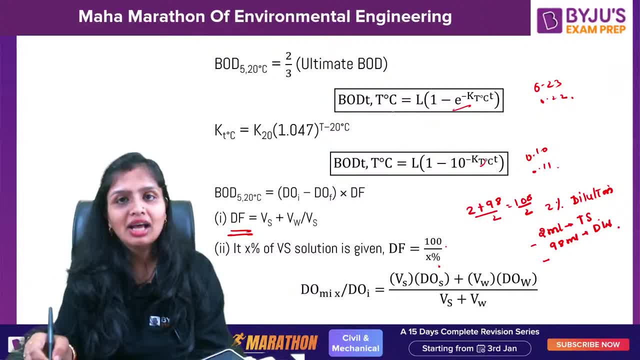 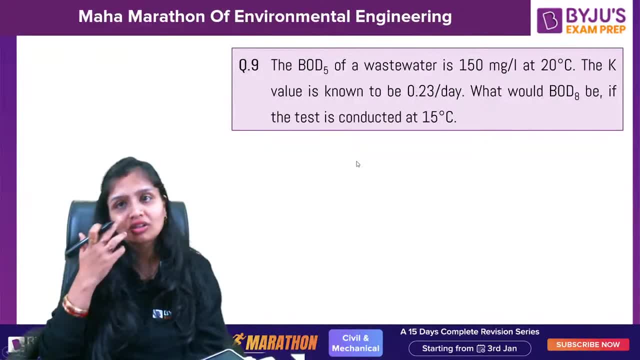 give a dysohyuk value like that, and at the stage of dilution it will come 1 by 90. so then it will be 1.23 will be the credit, and you'll get the value of delusion factor from 0.23 to 0.339. that's it. okay. now these are test samples. that's why i have written 100. 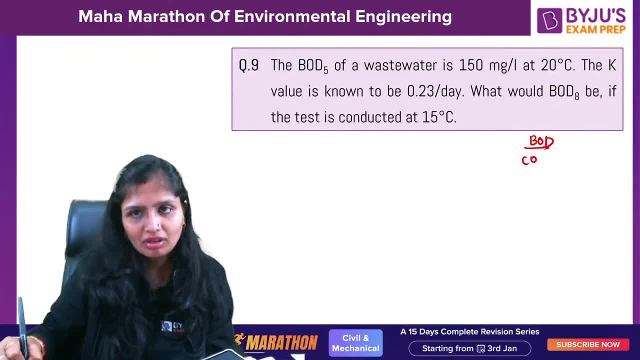 BOD COD is zero. so BOD, here it is biodegradable plus non-biodegradable zero. so it will become zero. when, when biodegradable becomes zero, then also it will become zero. so wastewater is free from organic matter. no, you cannot say that. why? why? BTEC trader? 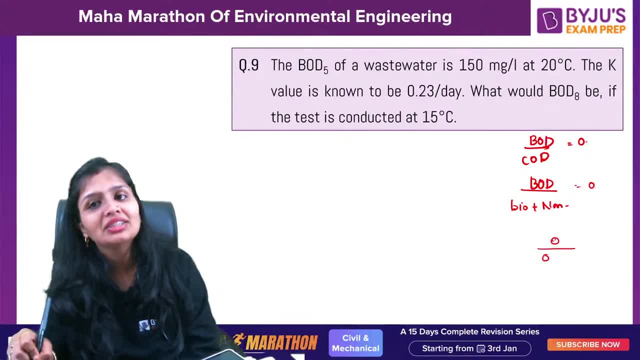 because it might be possible that the numerator is zero. okay, so you are saying like this: but it might be possible that some amount of non-biodegradable organic matter is present, so you can say that biodegradable organic matter is zero. you cannot say that total. 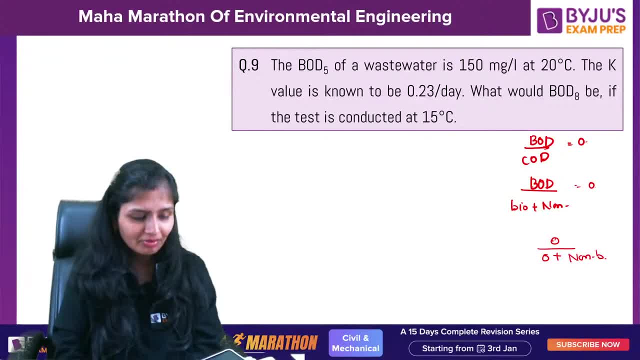 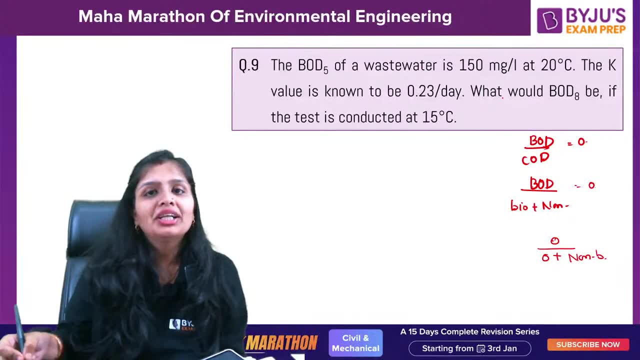 organic matter will not be there. clear, correct, correct. push now, guys. five days BOD is given to you. it is asking you: eight days BOD, but a different temperature. this is not a different temperature. this is not a different temperature. this is not a simple question, because I want to tell you one thing, but I want you should solve this. 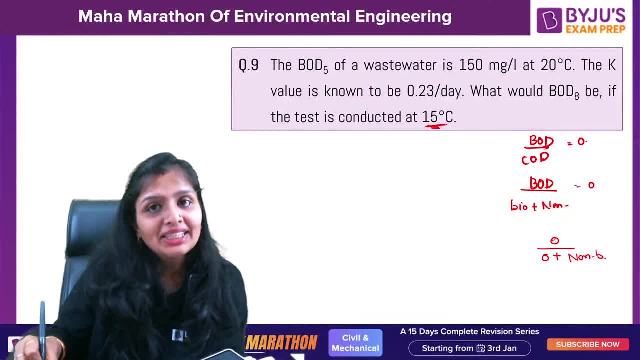 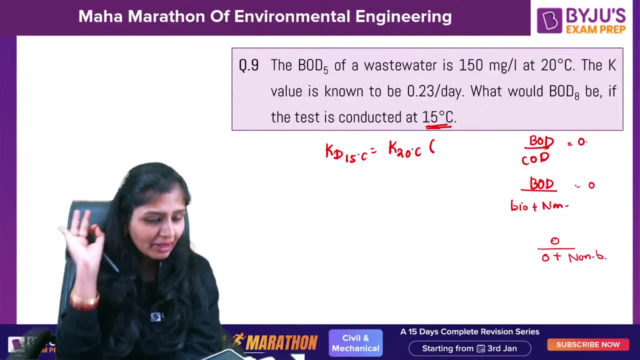 see, temperature is 15 degree Celsius. you will need to calculate the deoxygenation rate constant. but you know what? here you will not apply 1.047. when the temperature is less than 20 degrees Celsius, then the temperature is less than ma'am, is it correct? so it will be 1.056 less. you will go theta. 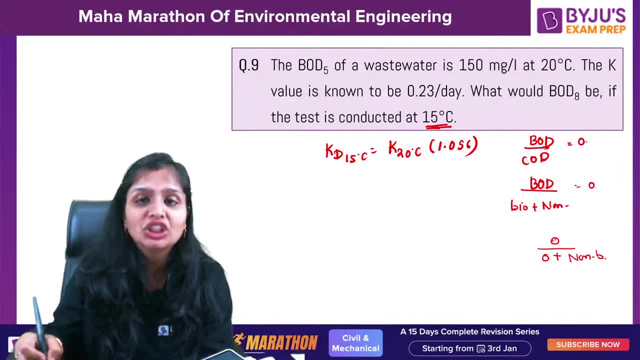 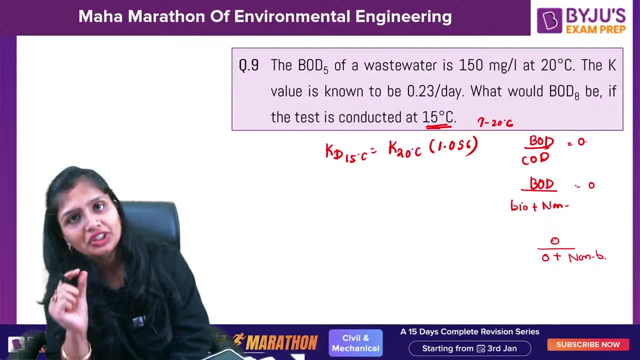 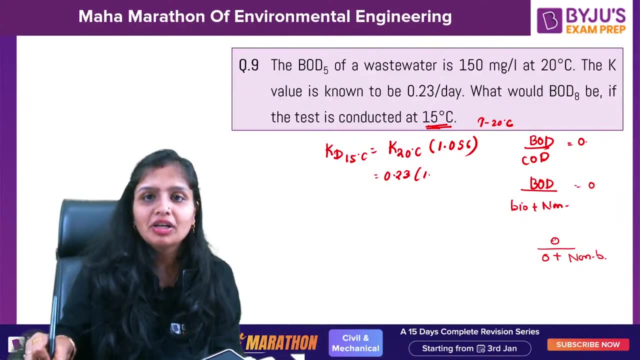 you can call it as here: T. this is a temperature coefficient P minus 20. this you will apply temperature coefficient value 1.056 when the temperature is less than 20 degree Celsius. so 0.23, 1.056, 15 minus 20. come on, guys, tell me so now. BOD eight days will be BOD ultimate. 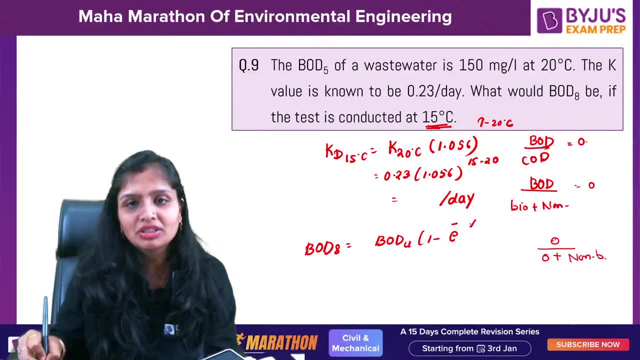 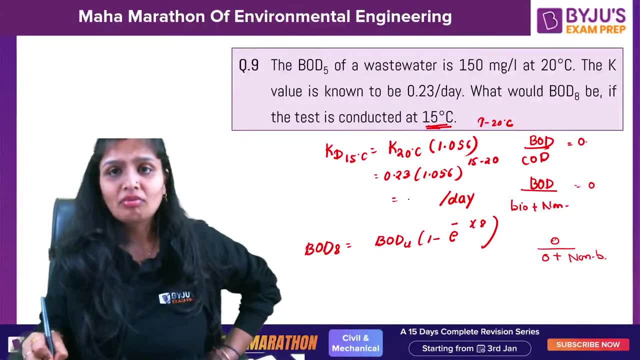 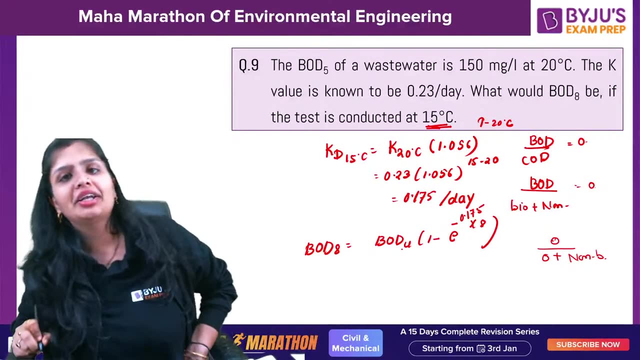 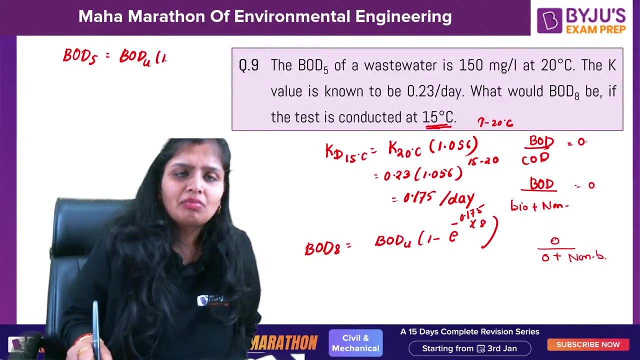 one minus e to the power minus, how much is the value coming? how much is the value coming? 0.175? but the problem is, I don't know BOD ultimate, so calculate it. no issue. foreign 150 Arun. you calculate BOD ultimate. push for you. calculate BOD ultimately it will be needed only fine. 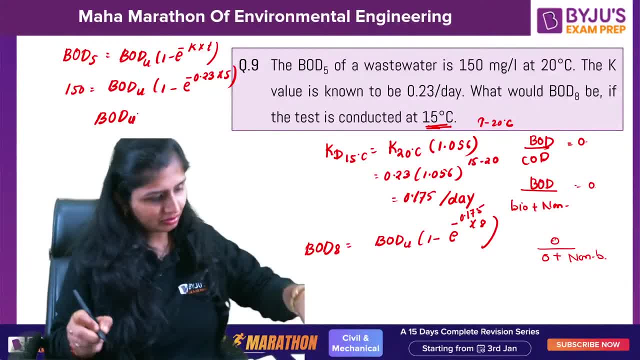 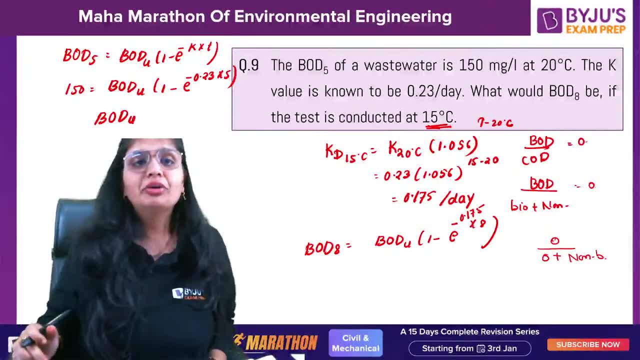 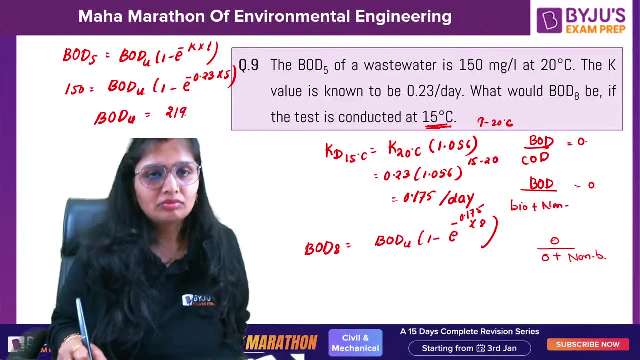 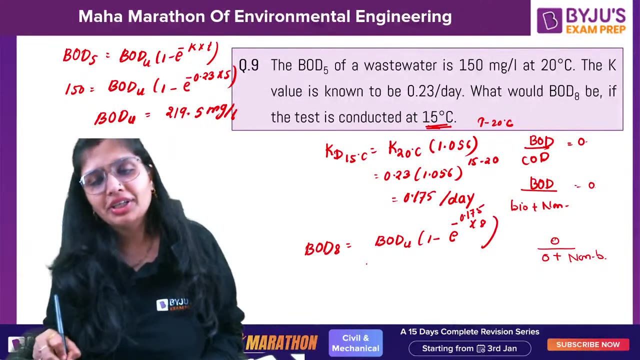 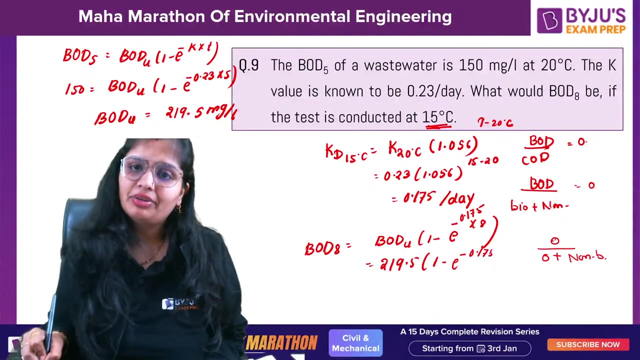 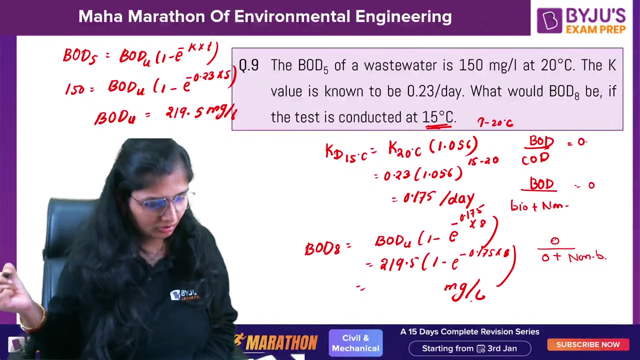 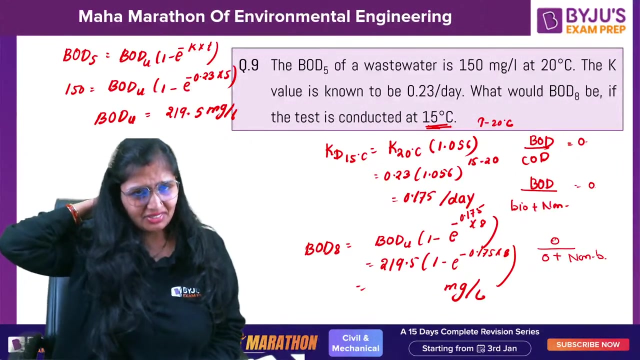 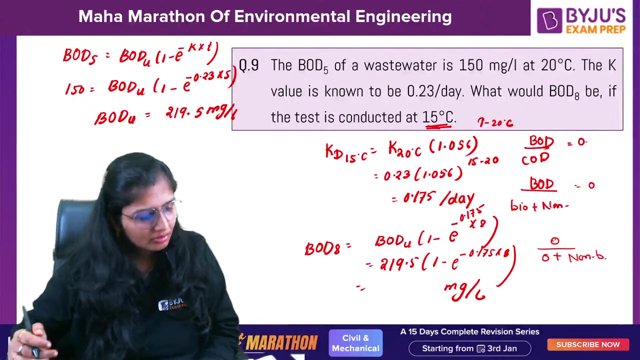 calculate BOD ultimate. first calculate BOD ultimate: 219.5- correct substituted here 219.5- 1 minus 0.175 into it. BOD at eight days: 165.5. this this 11.5. you one minus 9.5. 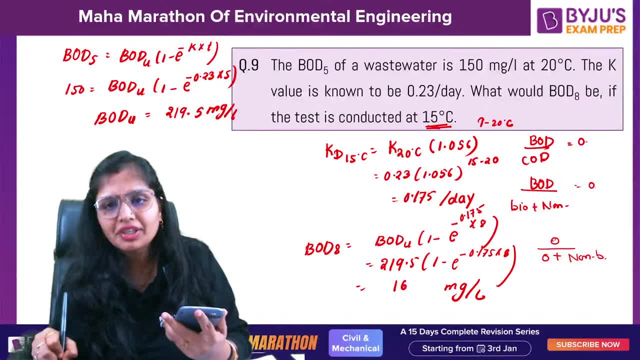 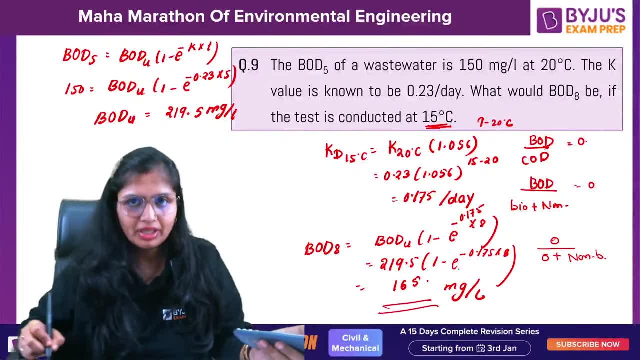 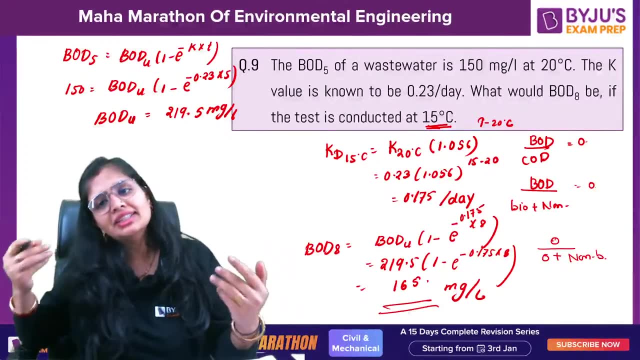 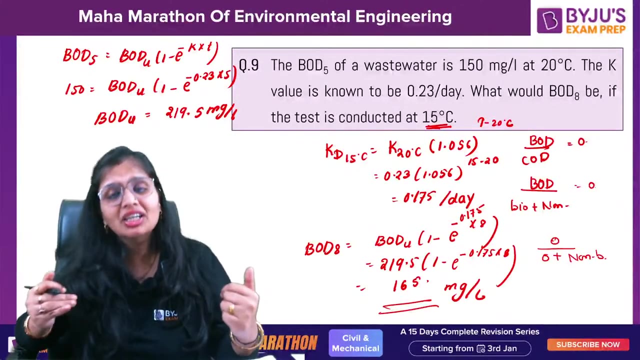 165 mg per litre. fine, fine, ok, see, if nothing is mentioned. now, shears, you were getting confused. if nothing is mentioned, it is asking you BOD, 8 days. just tell the BOD consume. but I agree that many cases it just tells you like that, it becomes difficult. 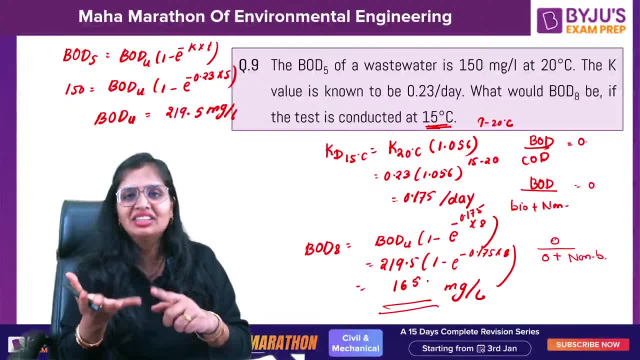 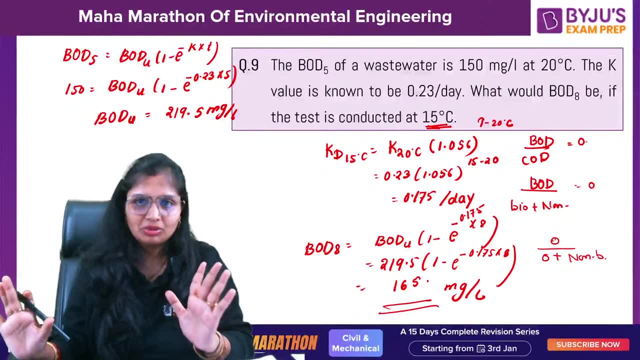 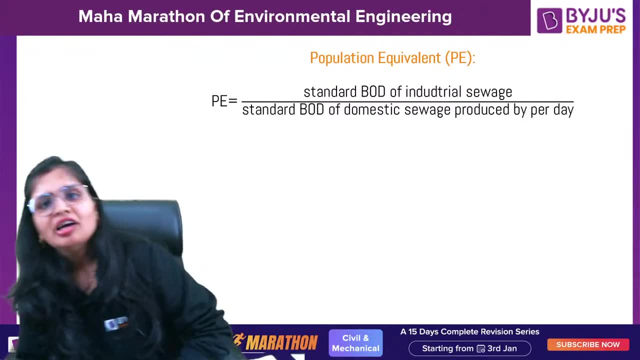 to understand whether it is asking you BC. whenever it direct, exerted and remaining, it becomes easy to understand. but when it is telling you, like this, so better go for BOD consume, ok, fine, now talking about here shears, you are there? population equivalent if I am talking. 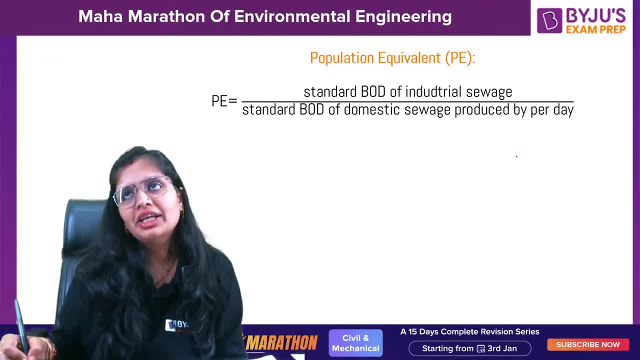 about see if, let us suppose in your home, in your city, 1 crore amount is spent for treating the sewage. ok, and let us suppose 10 rupees for a month. I am talking about 1 crore and 10 rupees is required per person. and in your home, 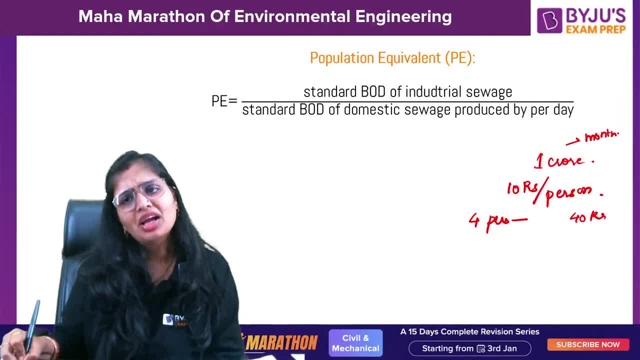 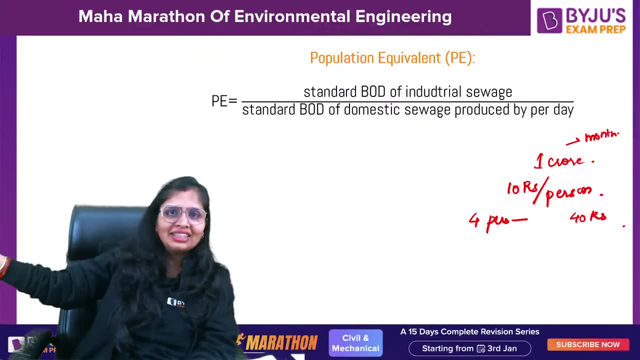 4 persons are there. how much they have to give- 40 rupees- but how you will collect it from the industrial people. obviously their sewage is also getting treated and why we will pay for their sewage. obviously, when it comes to pay for somebody else, until and unless he or she is your girlfriend or 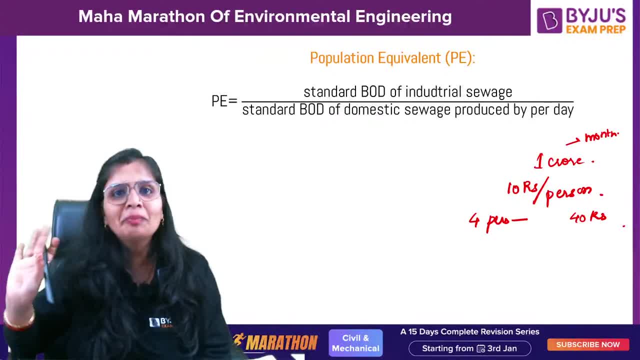 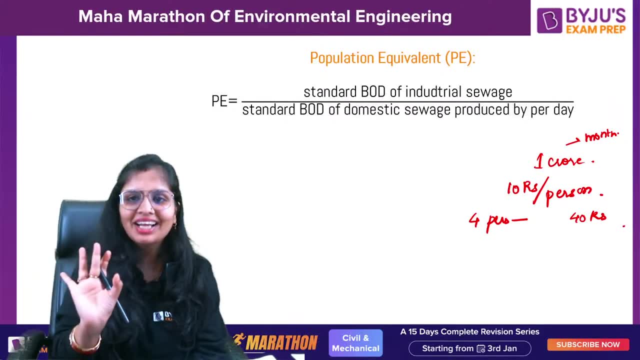 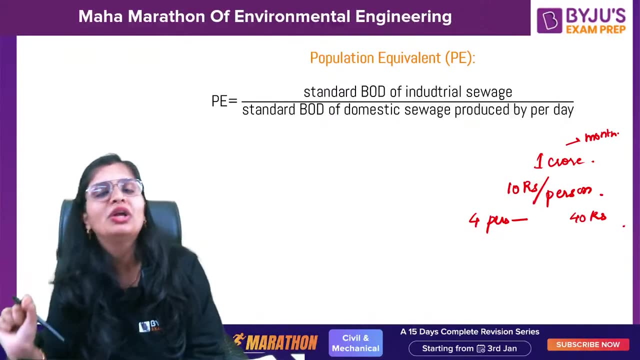 boyfriend, you won't pay. yes or no, you won't pay a single penny. I know that it happens to everybody, yes or no, Tiksha Prishan, it happens right. so why the hell? you will pay for those industries for treating their sewage. so that is the reason this term population. 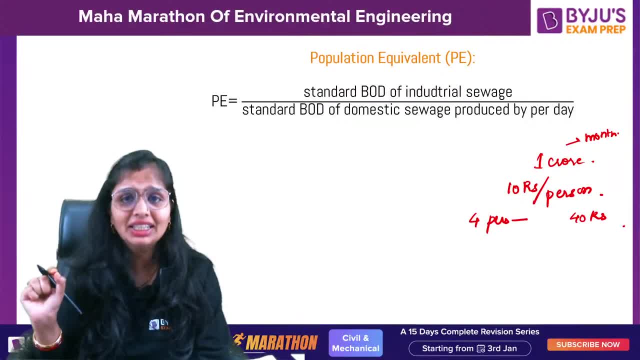 equivalent came into picture. now you will see that this sewage which is generated from these industries, from these industries, how much equivalent to how many percentage people they are generating the waste. If that industry is generating sewage equal to 2,000 people, how much money you will collect it from them? For 1 person, 10 rupees, and they are. 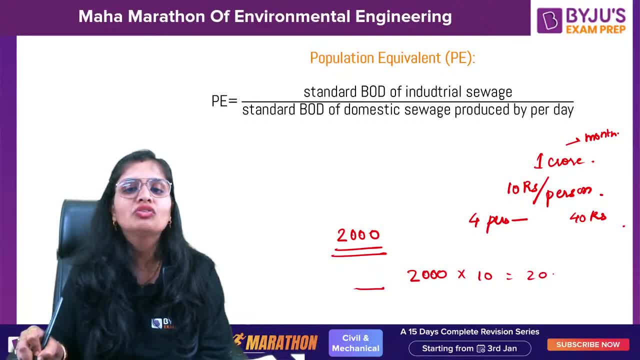 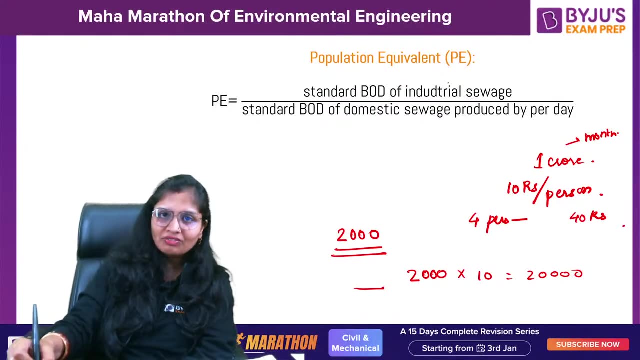 generating sewage equivalent to 2,000 persons. So you will take 20,000 rupees from them. So how you will calculate it? This? I gave you an example How you will calculate it. You will calculate by population equivalent. that is standard BOD of the industrial sewage. 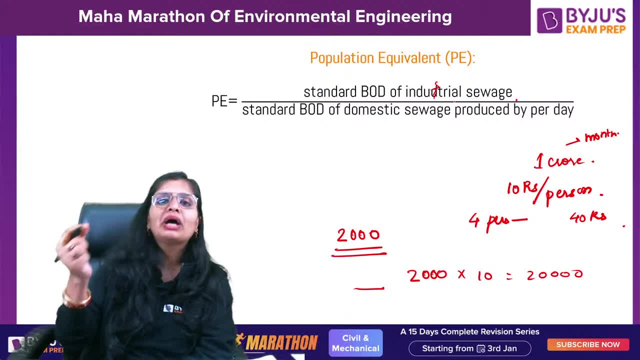 divided by BOD produced by per person per day. If it is not given to you in the quotient, it is 80 grams per capita per day. This is the BOD which is produced by per person per day. But if in the quotient it is giving you to take 75 grams, take that. I told you the standard BOD. 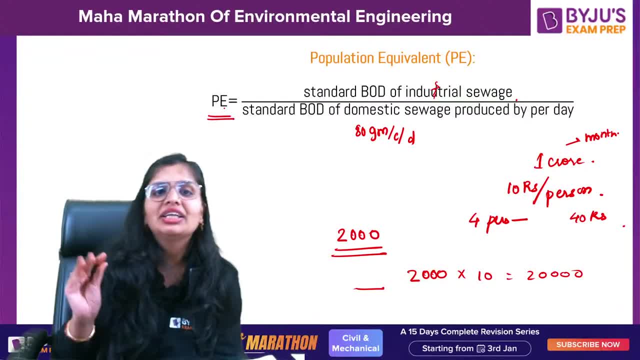 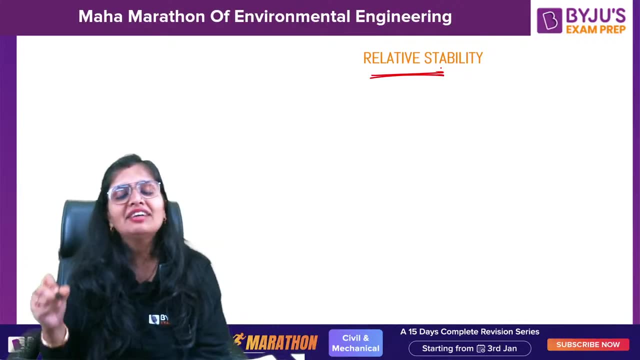 rate. So, with the help of this, you will calculate population equivalent. This is used for the industries, and all so that the charges can be taken out from them. Okay, As simple as that. Next, coming to relative stability. Okay, Relative stability Now. in your opinion? 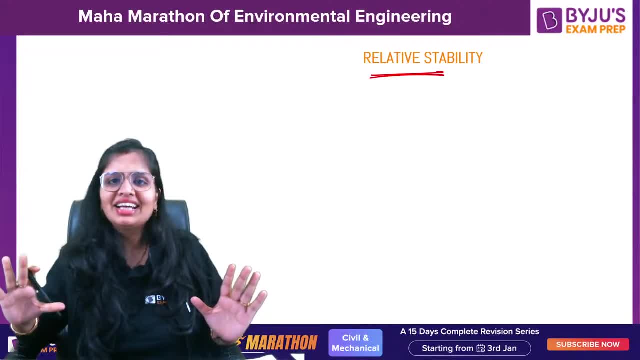 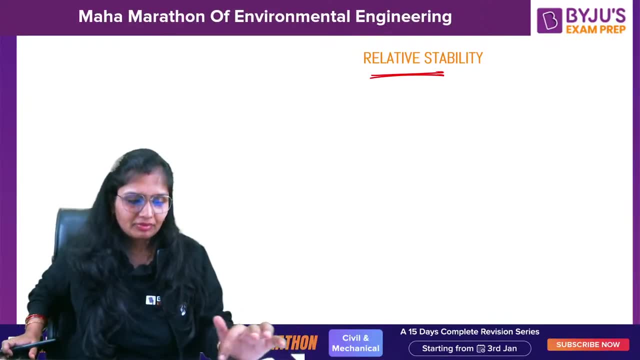 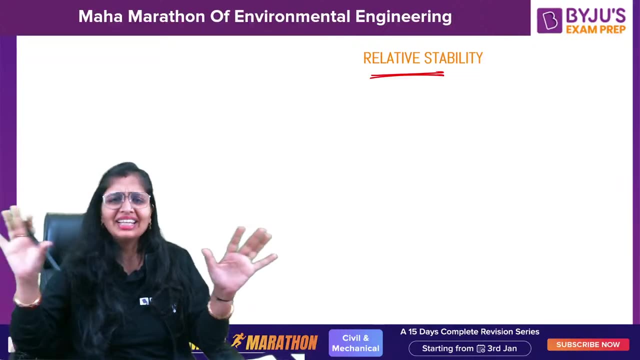 what do you mean by stability? Just tell me In your life, if I say that stability comes, what do you mean by stability? What do you mean by stability? Get a government job, get a good job, anything which is stable. Okay Here if I talk relative. 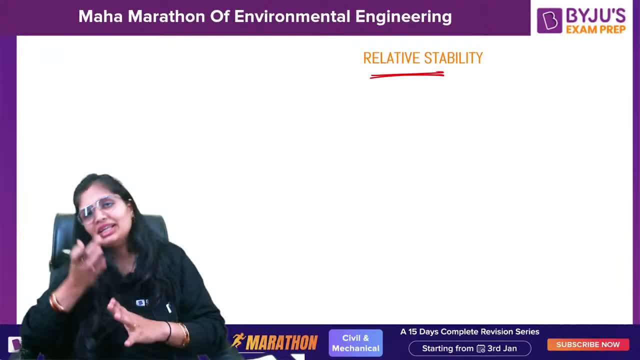 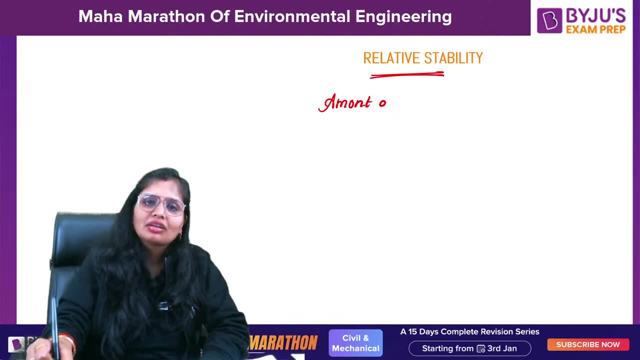 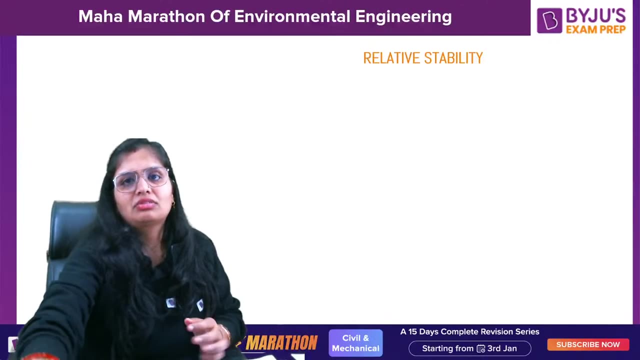 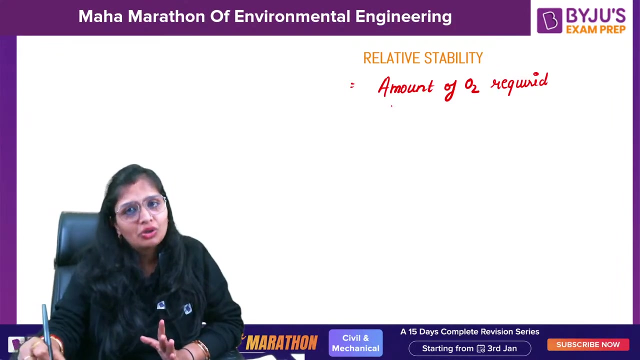 stability. if I talk about here stability means amount of oxygen required. amount of oxygen required. The spelling see what I have written: Relative stability. Amount of oxygen required In which form? Any type. It can be molecular, bonded oxygen, It can be normal oxygen. Amount of oxygen required. Okay, Be it molecular oxygen or molecular. 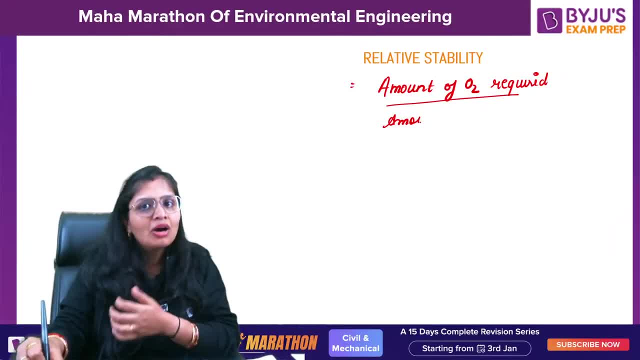 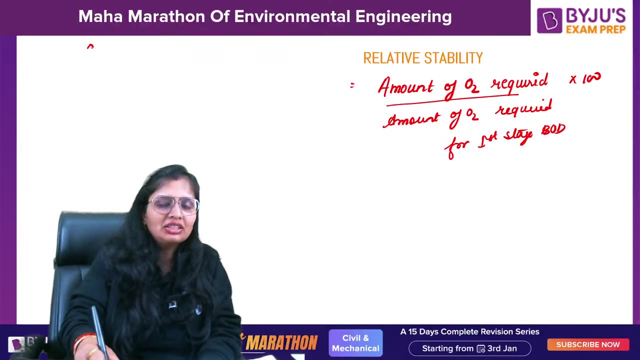 bonded oxygen, dissolved oxygen, divided by amount of oxygen required for first stage BOD. Remember, now let me tell you first stage BOD and second stage BOD are small things. I'll tell you which is required. See, this is first stage BOD: the amount of oxygen required for the 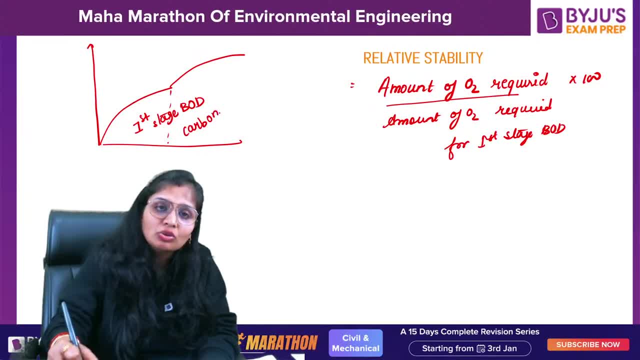 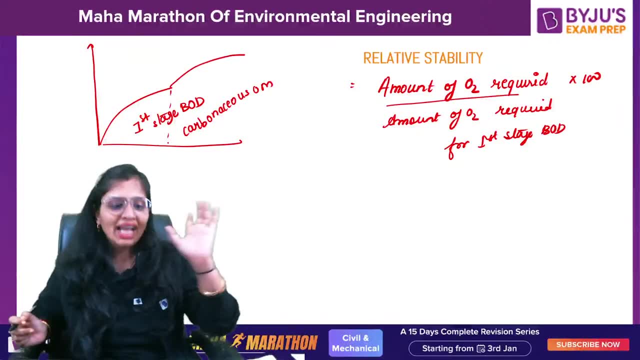 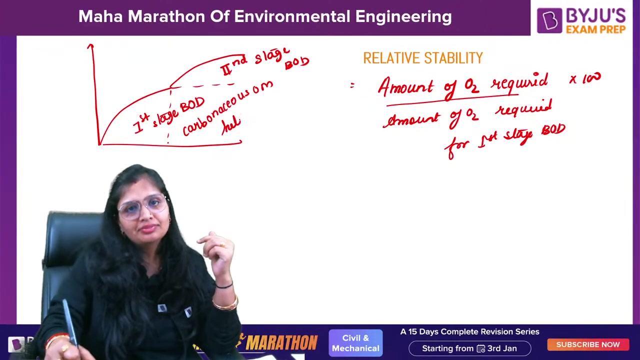 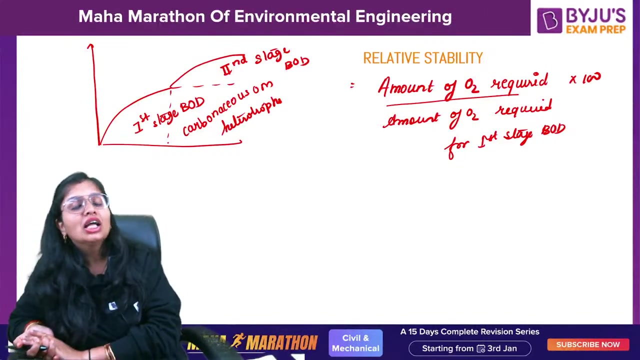 decomposition of carbonaceous organic matter. This question can be asked in your statement, not this one. I'll tell you the question: First stage BOD: who attacks it? Autodrops or heterodrops? and second stage BOD- you call it as nitrogenous BOD- the amount of oxygen required for the 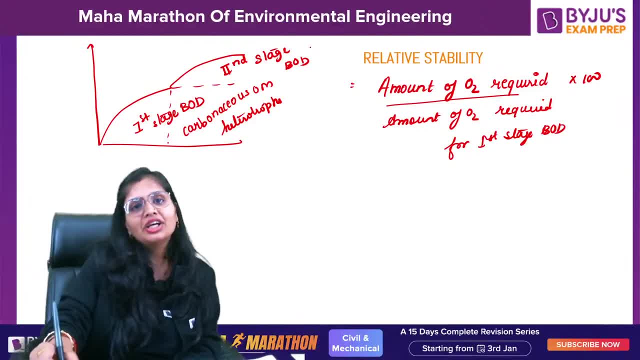 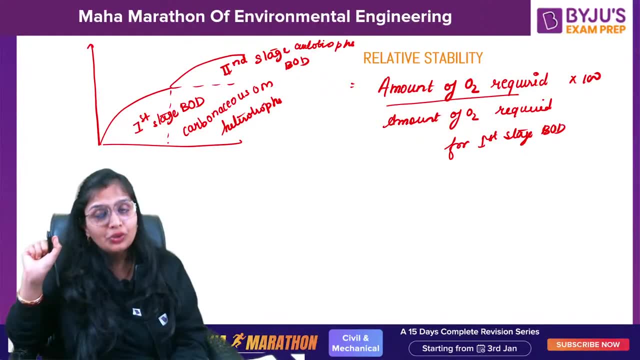 decomposition of nitrogenous organic matter. and here you have what Autodrops? Here you have autodrops, heterotrophs. Heterotrophs utilizes organic carbon. Autotrophs utilizes inorganic carbon. like in carbon dioxide, this carbon is there, that is inorganic. So how much time this autotrophs? 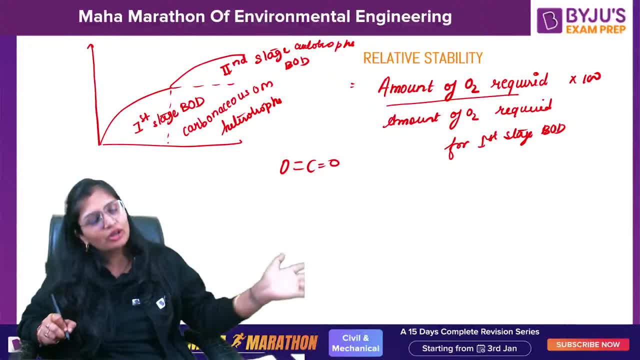 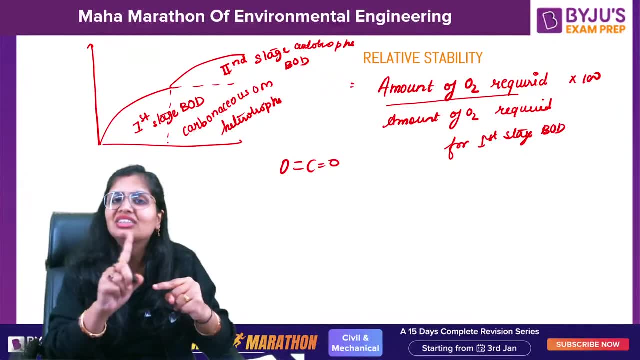 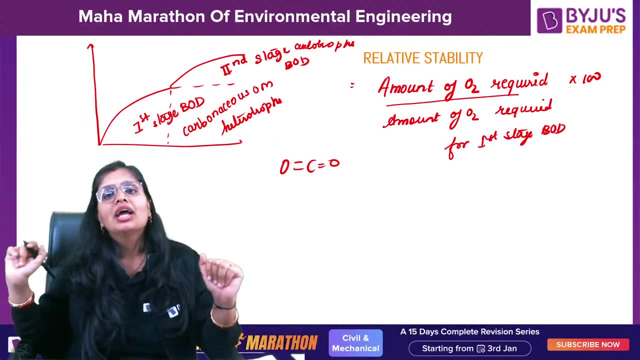 will take to utilize the carbon. in that time, heterotrophs will finish its function and go So in treatment unit. remember our primary focus: we never design it for nitrogenous treatment, never. we only go for carbonaceous treatment. Okay now relative stability. there is a formula for it. 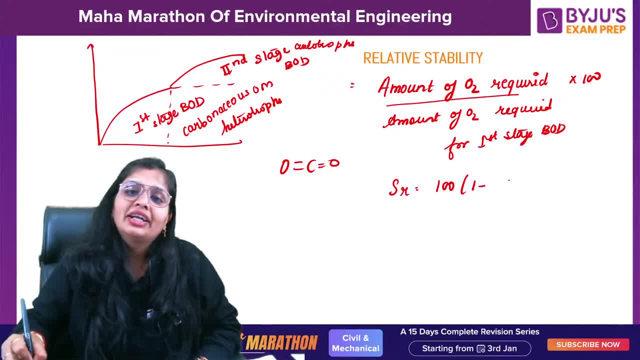 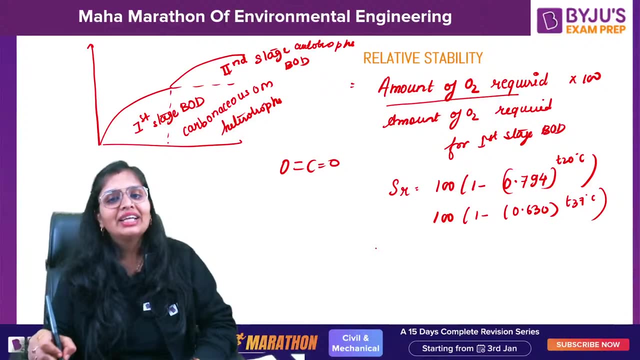 two formulas. are there 100? I will write it down. you tell me whether it is correct or not. T 20 degrees Celsius, and this is 100, 1 minus 0.630. T 37 degrees Celsius. Now: T 20 degrees Celsius and 37 degrees Celsius. 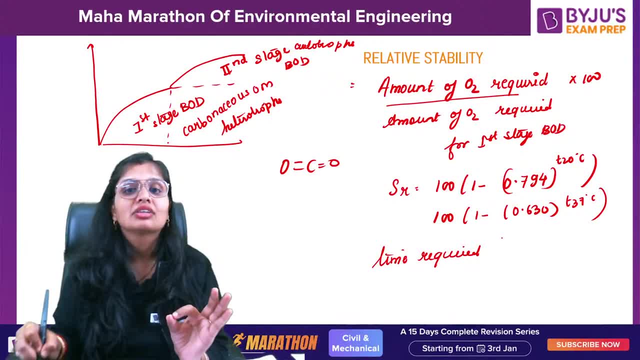 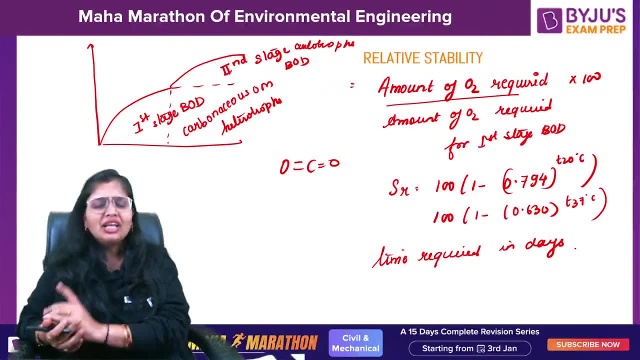 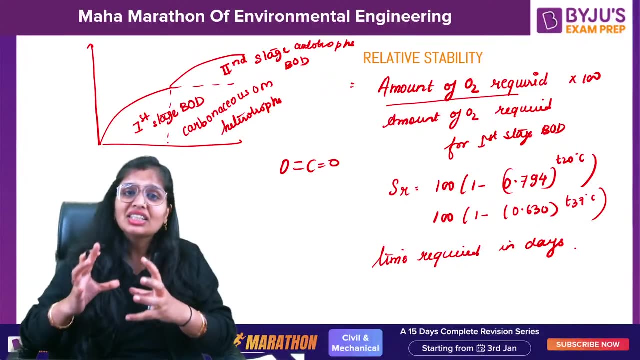 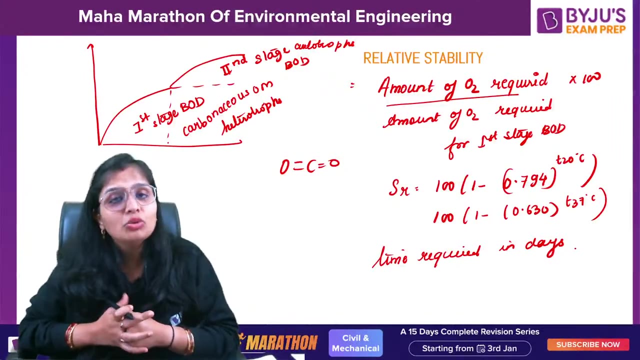 At time, required in days, for the decolorization of methylene blue colored solution. Now, why this methylene blue colored solution will decolorize? because there are certain enzymes which are present, Okay, which will lead to the decolorization of methylene blue colored solution. 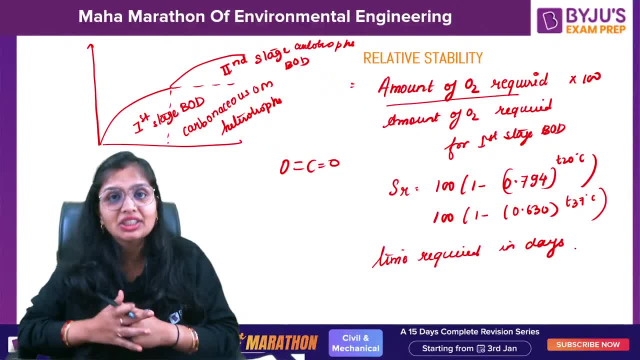 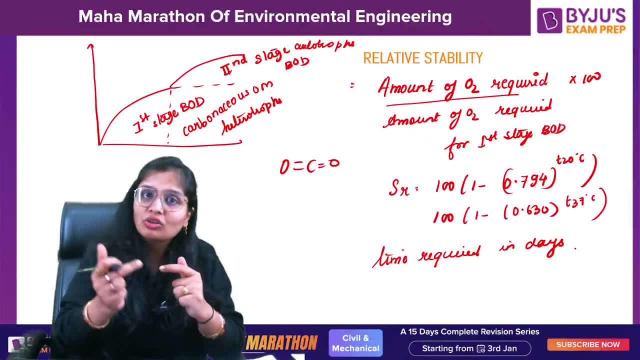 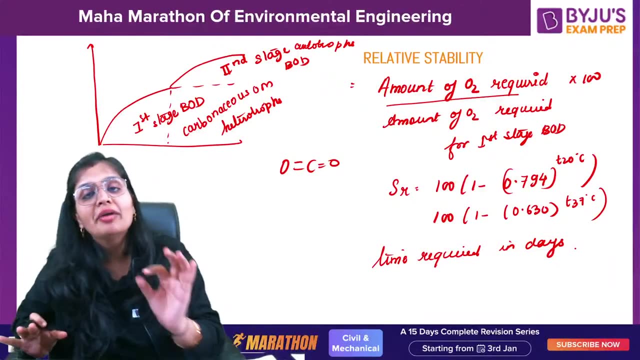 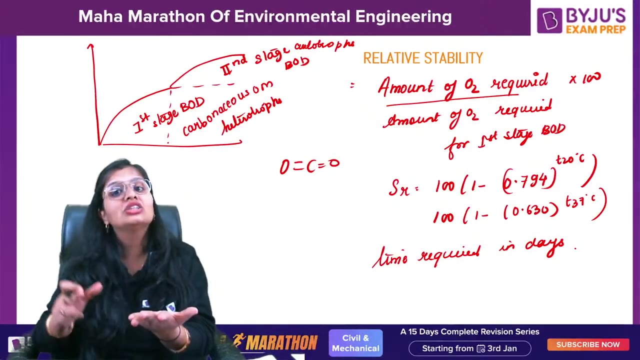 Why this? enzymes will do the decolorization? Because when oxygen is there no issue, but as the oxygen gets exhausted, anaerobic conditions prevail and there will be certain enzymes which will carry out the decolorization of methylene blue colored solution. Sooner the anaerobic condition develops, sooner the enzymes will come into action. 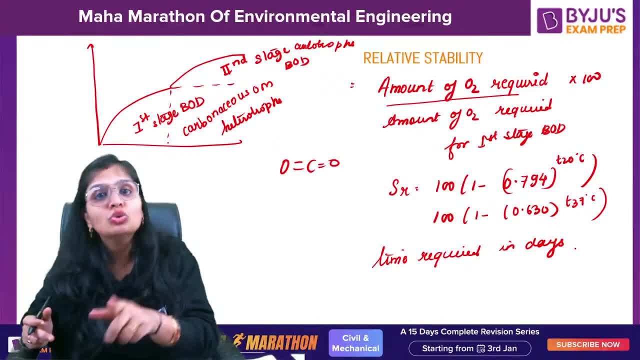 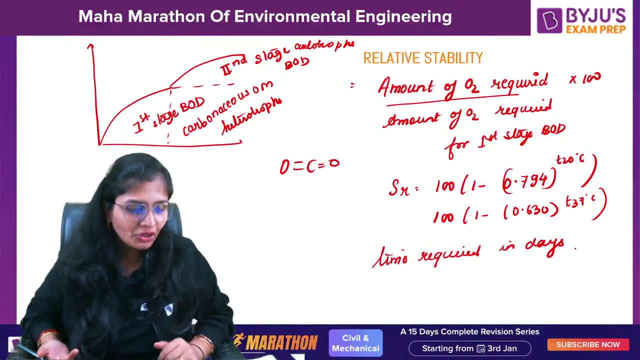 sooner the decolorization will take place, So sooner will be the unstability which will come into action. If the time is given to the decolorization of methylene blue colored solution in less than 4 days, what you call it time- is directly related to stability. you can say: 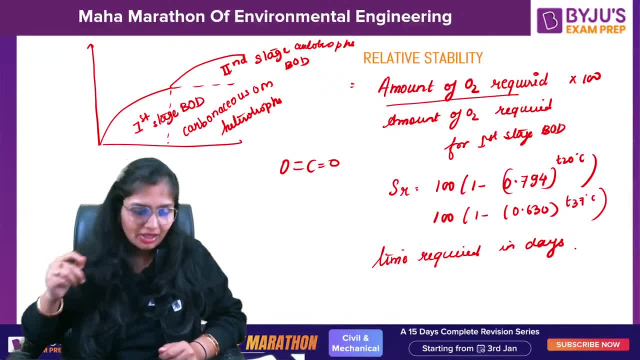 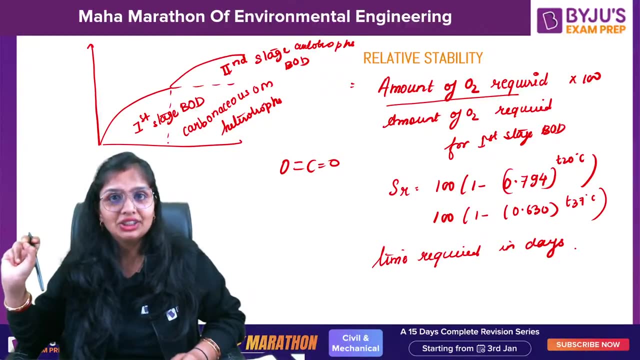 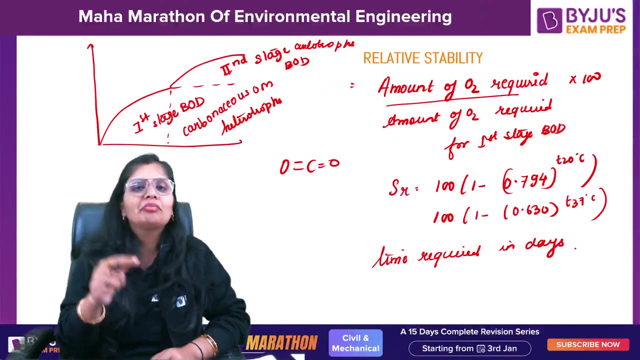 that you can say that. you can say that. why use KD, K 20, 1.05 or 4: 6 if time is less than 4 days? the sample is declared unstable because Ashish the temperature was less than 20 degrees Celsius. In fact, I was saying that we will use it when the temperature is 20 degree Celsius greater. 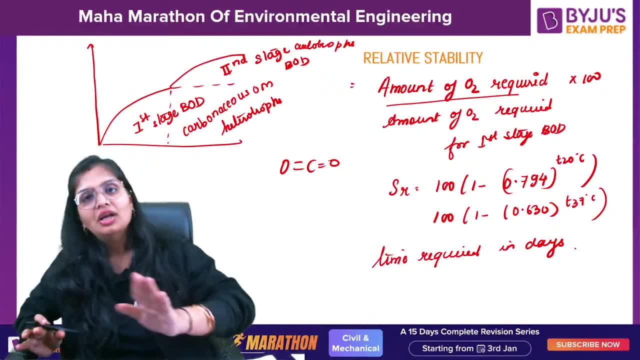 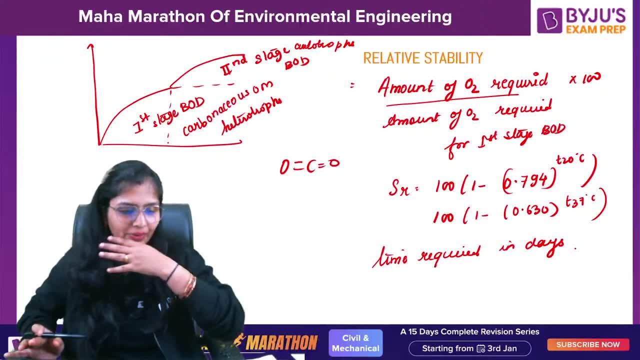 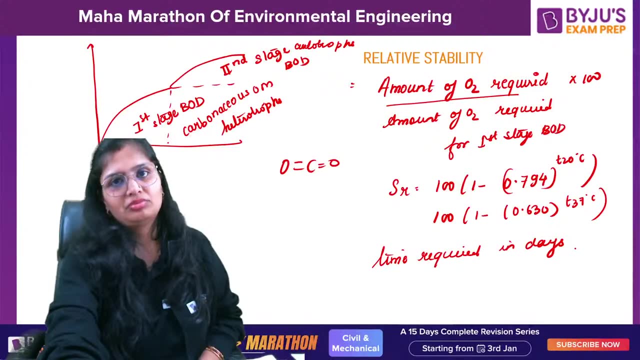 than 20 degree Celsius. since here the temperature is 15 degree Celsius, we use that. I told you also, Bitta, okay. okay, fine, This completes your wastewater characteristics. any doubt? Arun Girish, anybody? Devanshu, Dinesh Swapnil, anybody? any doubts? 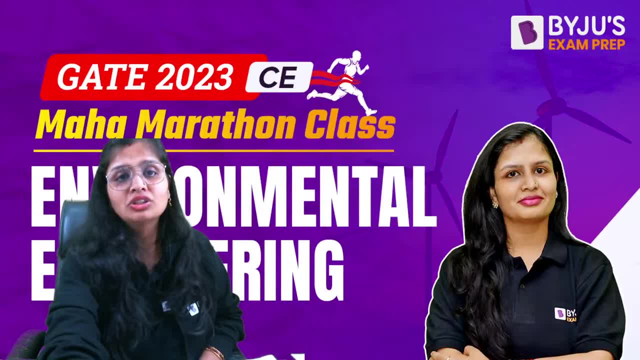 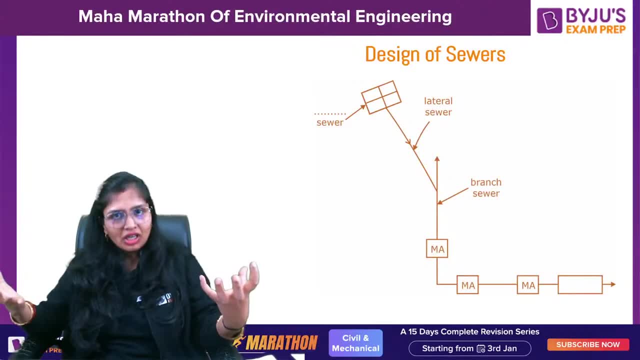 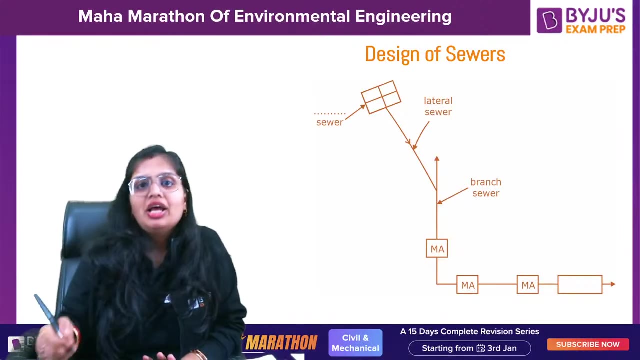 Any doubts? Okay, em fine. so first you studied the behavior. now we will be talking about the designing of sewers. okay, sewers are those pipes from which we carry the sewage from one to another. ask me, kishayala, ask me. so what happens? remember you are an engineer whatsoever- sewer designing. 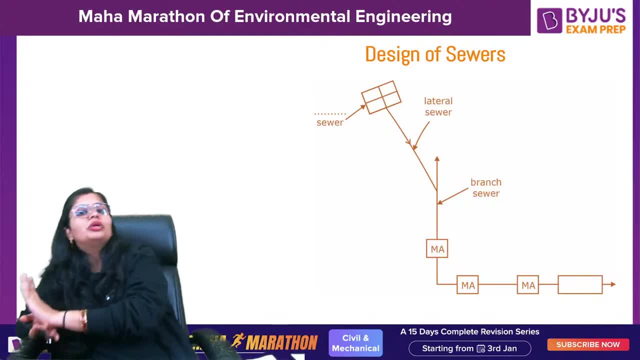 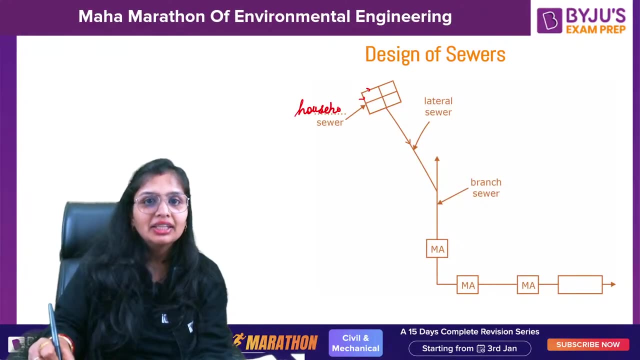 is done for your homes, you are the one who will be doing it. you are the one who will be doing all the connections. government will not do it for you. yeah, but the moment, these are the household sewers, okay, these are the household sewers. these sewers, water will go from all the households. it. 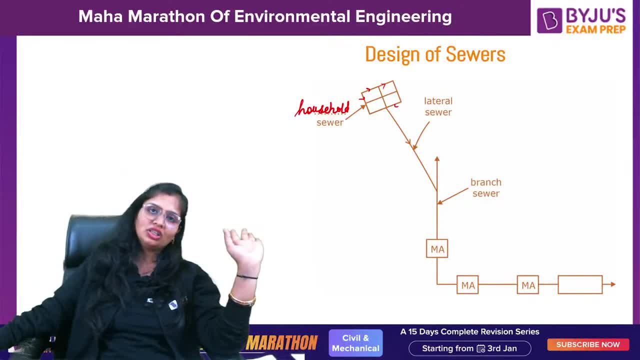 will go into the lateral sewers. this is the responsibility of the government. but your home sewers, it is the responsibility of you. government is not responsible for that. so all the household sewers gets collected to lateral sewers- lateral sewers. you have branch sewers, ma, which you are seeing. this is the manhole. 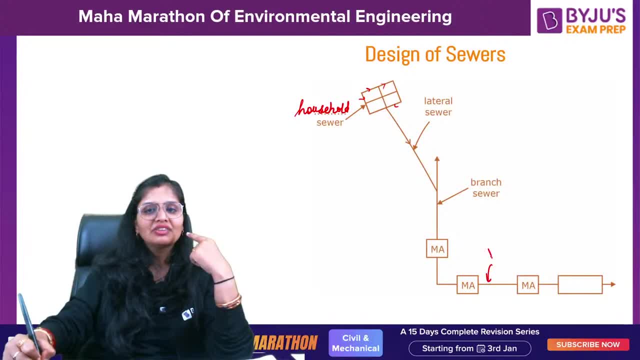 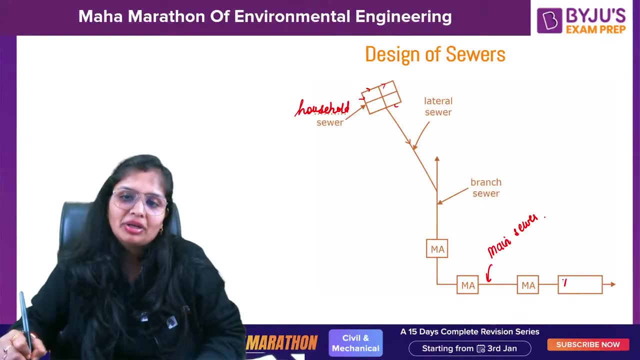 okay, from here many number of branch sewers, it will go into the main sewers. from main sewers, from main sewers, it will go. this is the treatment plant. so from main sewers, the sewers which goes into the treatment plant and from treatment plant 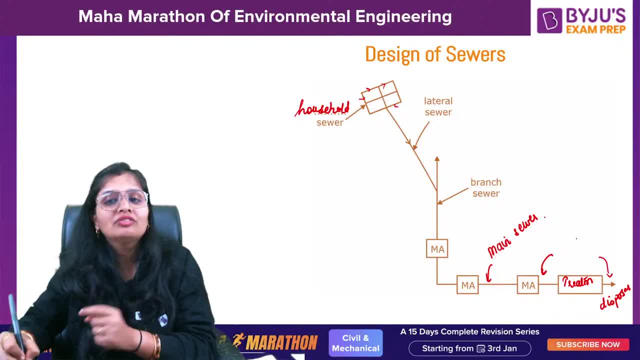 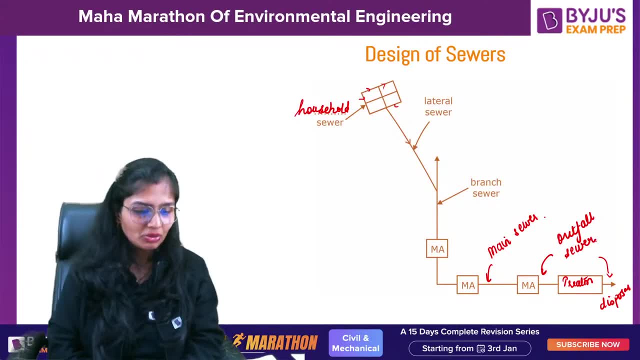 the sewers which goes into the disposal. both of the sewers is known as outfall sewers, both of them is known as outfall deworms. why we design only for carbonaceous and not for nitrogen? because, firstly, nitrogenous, for taking the decomposition of nitrogenous it takes time. 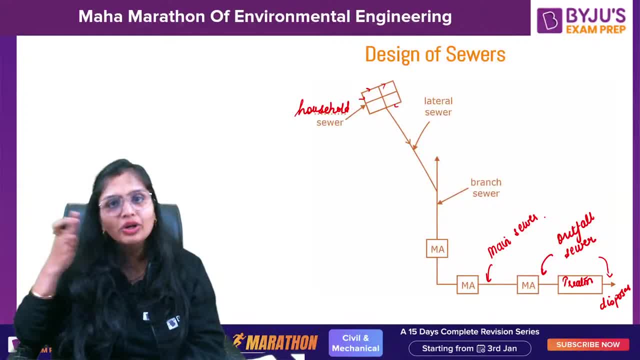 and it takes time. for the decomposition of nitrogenous, it takes time. secondly, moreover, you will dispose it okay. so when you dispose it, after this, we will study that chapter. so when you will dispose it, eventually, by dilution and by other techniques, eventually the organic matter will be removed and after that, that water, let us. you are disposing it in reverse. 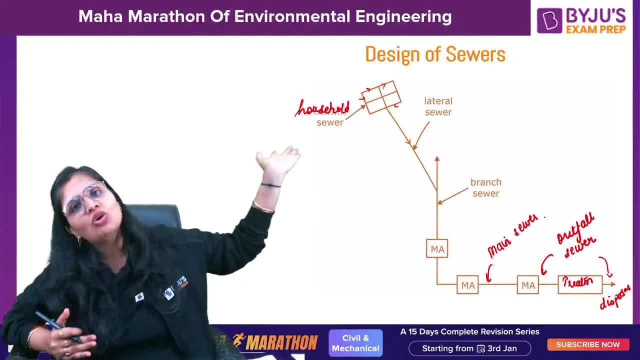 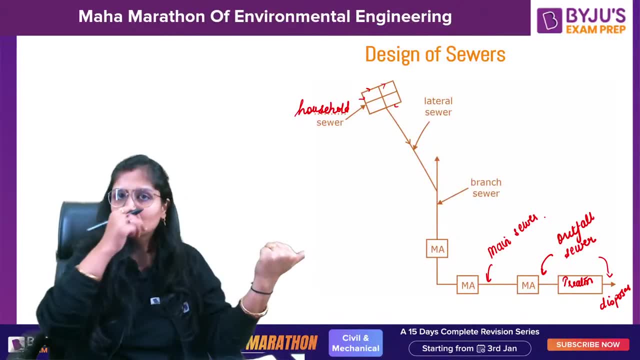 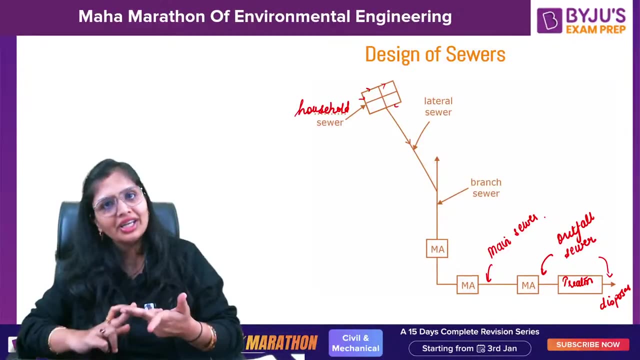 you will take the water from river and exactly the whole procedure which we dealt in the first half. again, you will be doing the treatment, but that time it will be raw water treatment, so nitrogenous BOD. it takes time, so that's not our concern. secondly, moreover, we are not drinking. 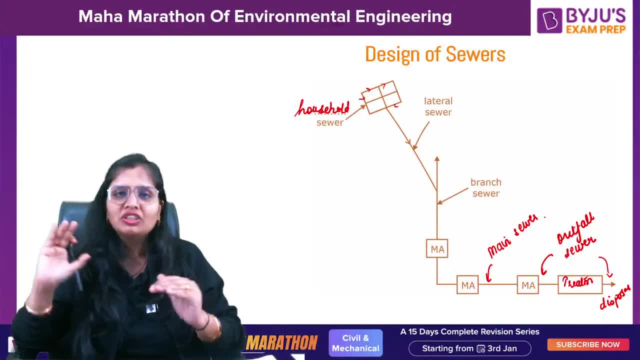 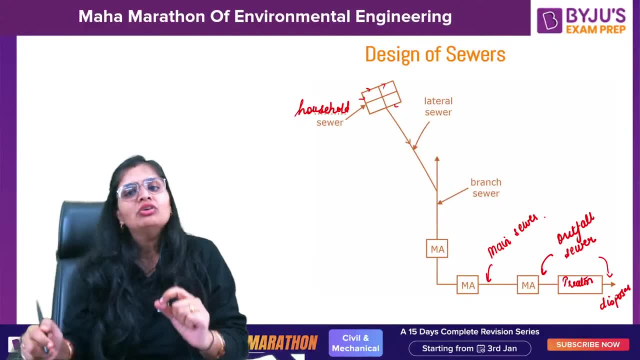 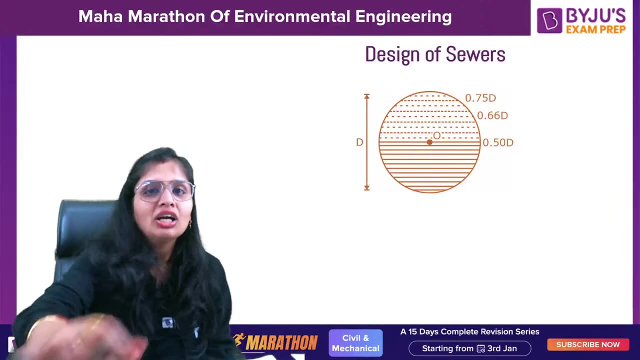 that water. we are just disposing it, so self-purification will take. okay, now coming next. coming next. we told you from main sewer to treatment unit, treatment unit to disposal. both the sewers are known as outfall sewer. now coming next, how we design the sewers. sewers are never. 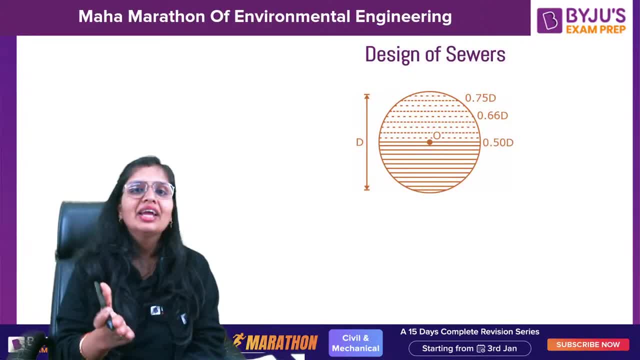 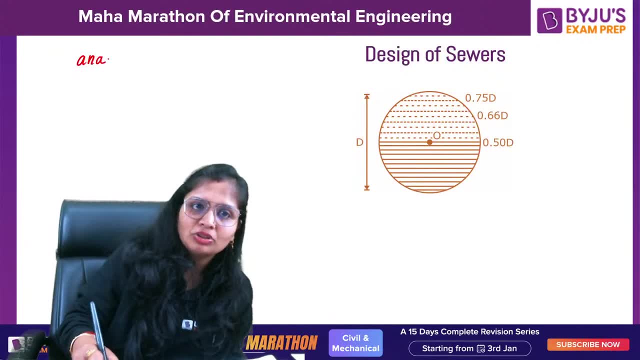 designed for full flow condition. you guys know that why? because anaerobic decomposition takes place. can you tell me what are the things which are generated during anaerobic decomposition? what are the end products? acids, alcohols, gases, gases like methane. let me tell you, methane is known for its high explosive. 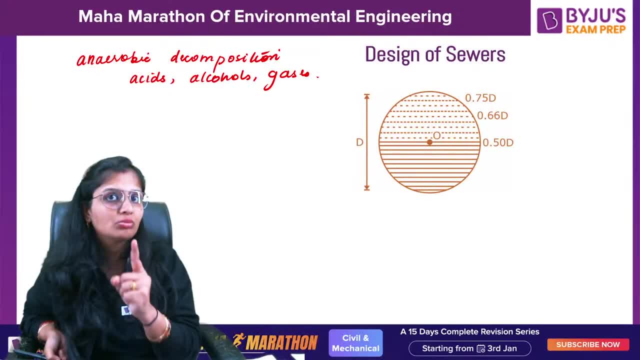 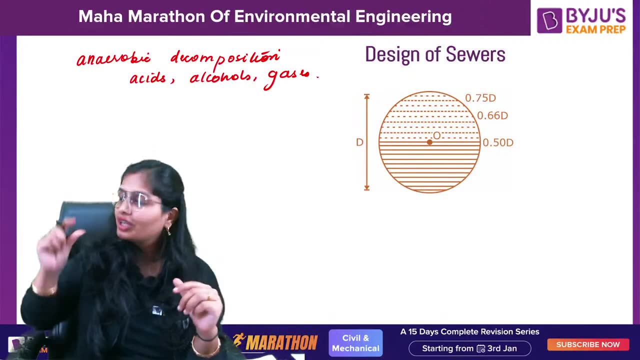 tendency. so that is the reason. that is the reason what you do, you never fill it up to the top. ISS is there, but majority concert concentration is one. we gave time for the accumulation of methane, that Tib Domoded NW is the natural biotic food infant, but we gave time for the accumulation of 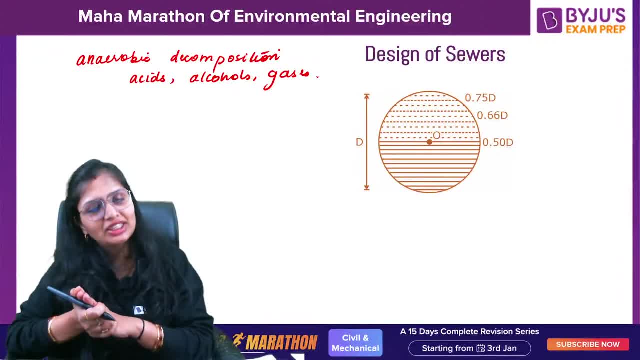 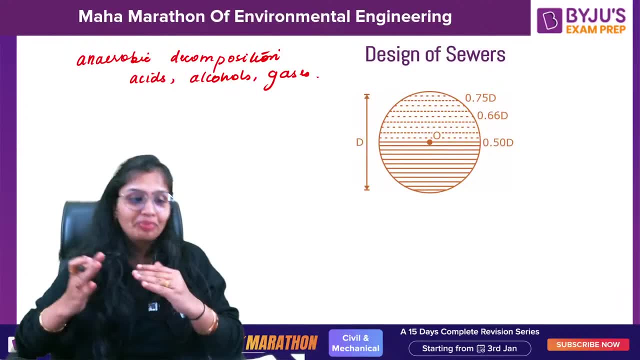 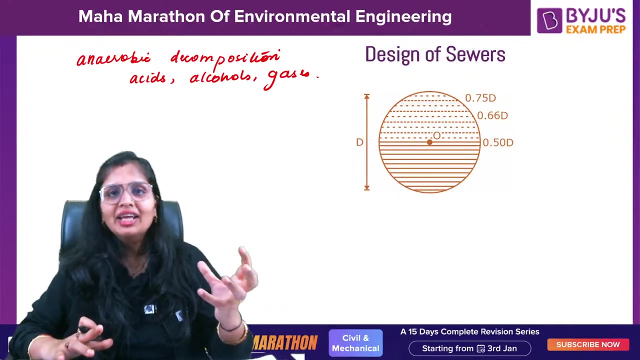 weapon as low concentration, as reasonably too high concentration. you do not have it. the the next things which comes into picture. the next thing which comes into picture is: you don't fill it full. next next is: generally we prefer circular sewer, why, if you go, you can roll this, basically, when you are sewers, or you can take the manholes, you will see they are. 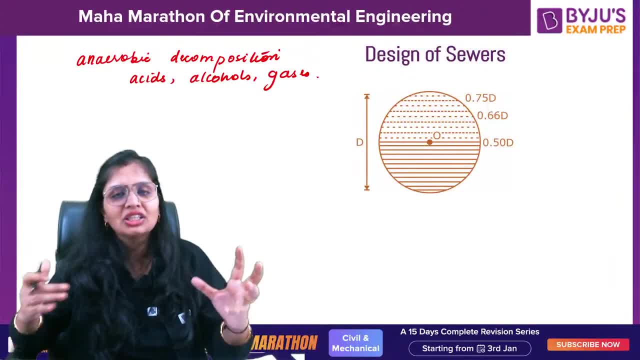 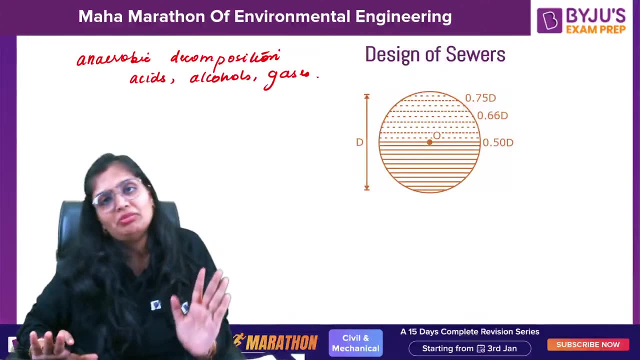 circular in nature. sewers are also circulation. the circular because the fluctuation in discharge, the fluctuation in velocity. i told you the meaning of fluctuation. how many times maximum value is more than the average, or average value is more than the minimum. so the fluctuation comes. 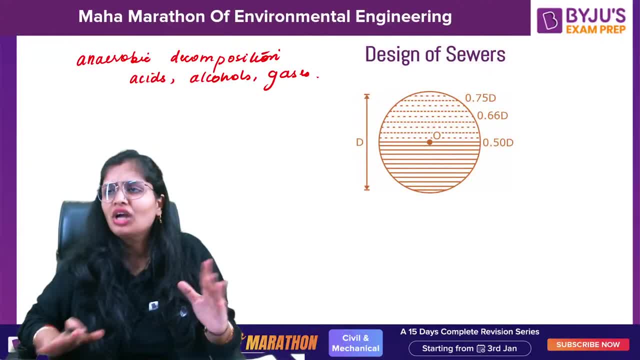 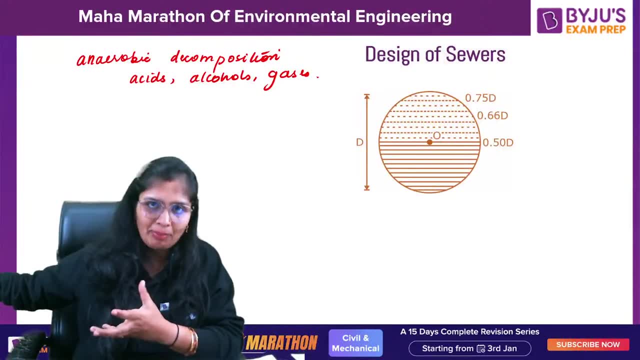 out to be minimum for circular sewers. so you have n number of sewers, okay, but we prefer circular sewers. so generally you would have seen the concrete sewers, pipelines, which is late, that is, of tata, everywhere it is going on nowadays so they are generally circular only. okay. now 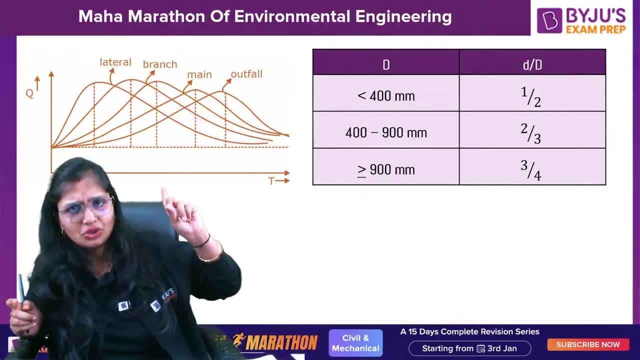 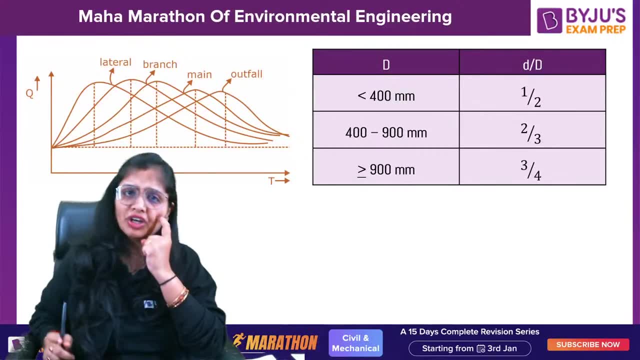 come to the next thing which comes into picture. the next thing which comes into picture is the next thing. okay, one question. i'll ask one question. i'll ask the time where your demand is maximum for water. the same time, the value of discharge will be maximum for lateral sewers. yes, 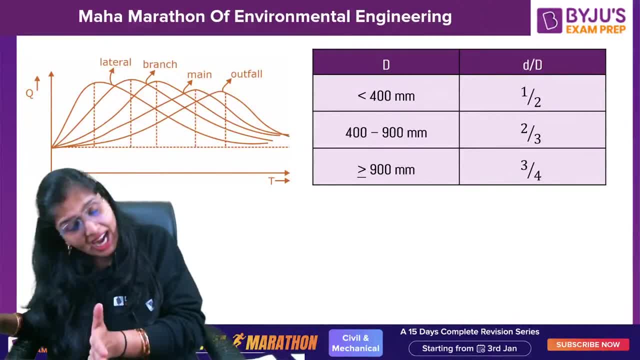 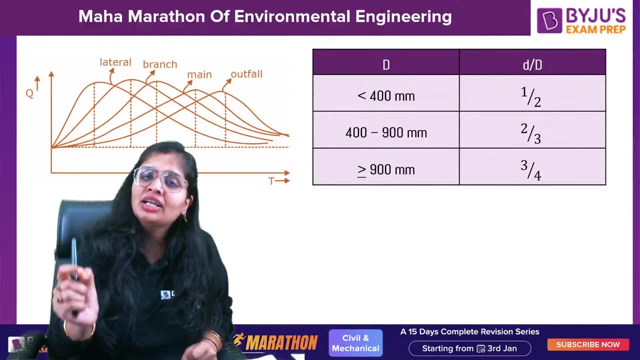 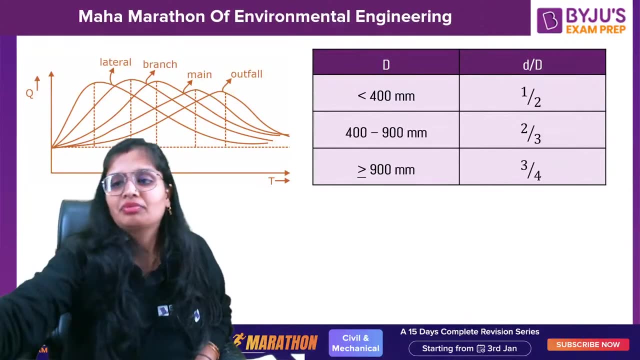 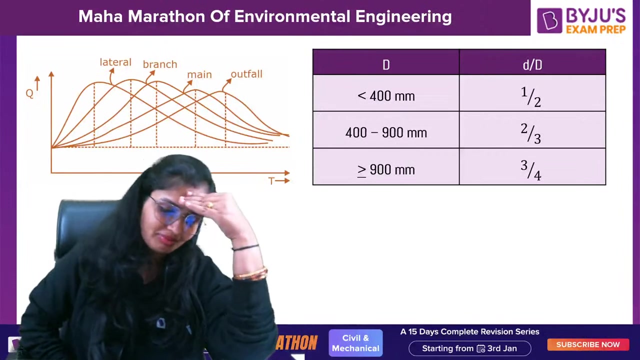 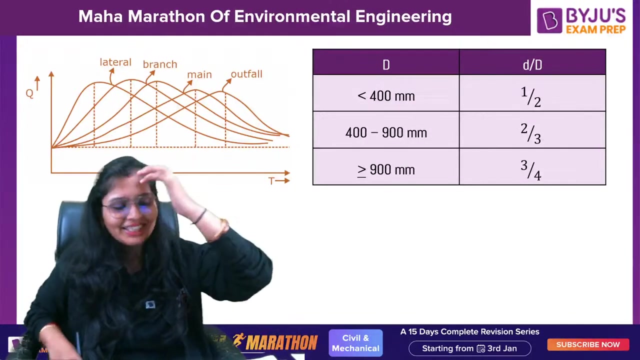 or no. i'll repeat again the time at which your demand for water is maximum. that same point. will the demand or will the amount of discharge in lateral sewers be maximum, yes or no? i expected that answer. no, no, no. just let example now in front of you, i'm drinking water, drinking. 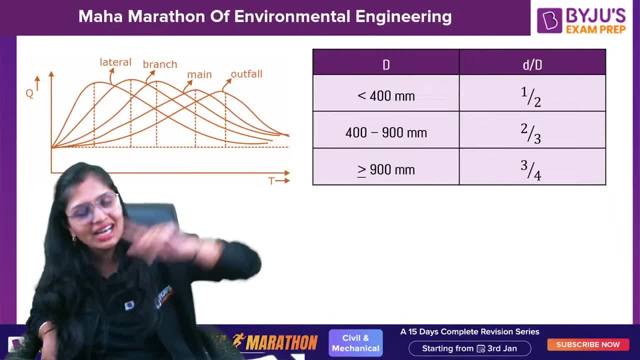 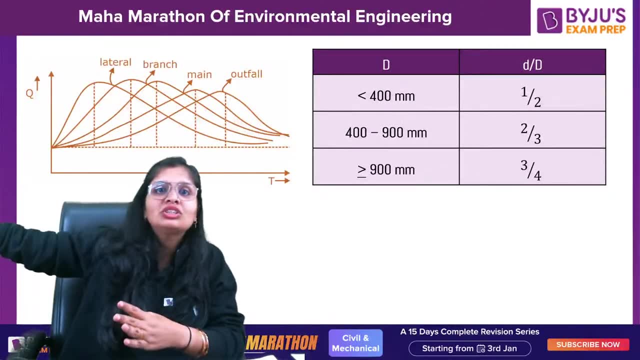 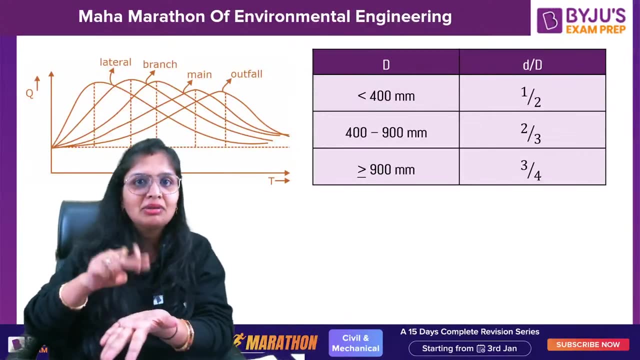 water. my demand is increasing, but right now i'm going to the washroom, or what? when i'll go to the washroom, urination then it will convert into sewage and after that it will go into the sewer. so remember that time when your water demand is maximum, that time lateral sewer discharge is. 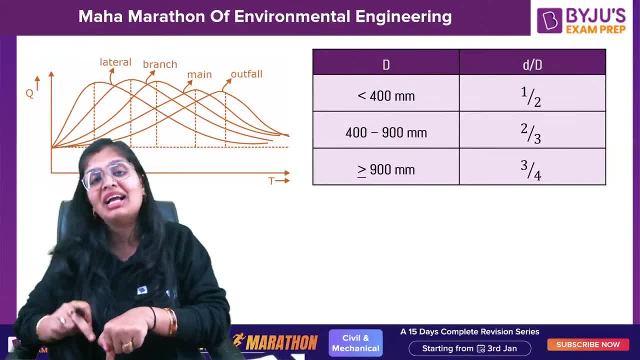 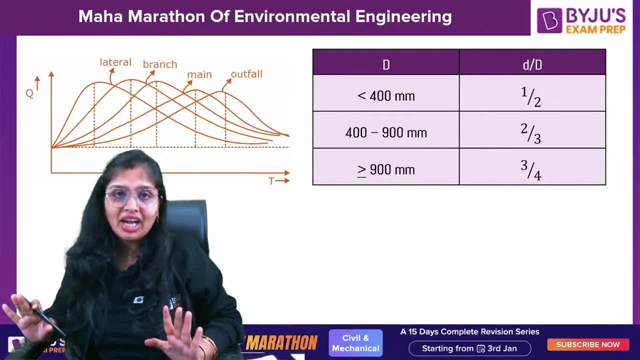 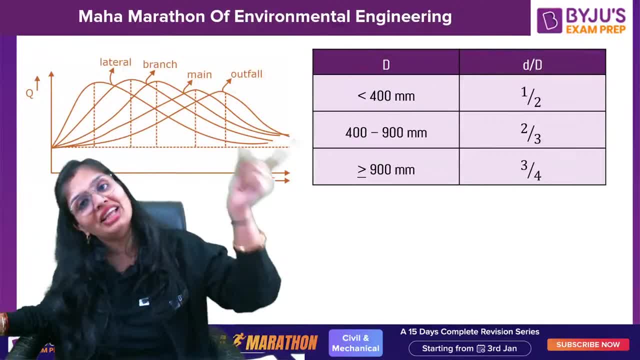 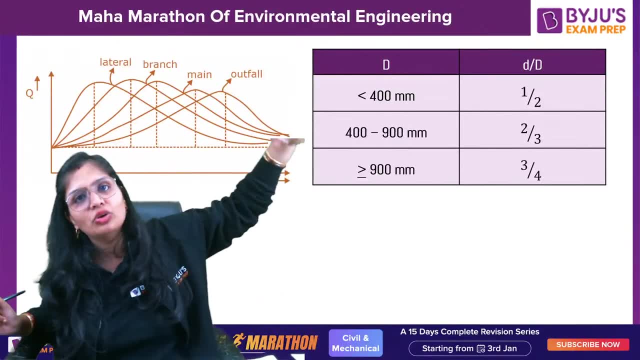 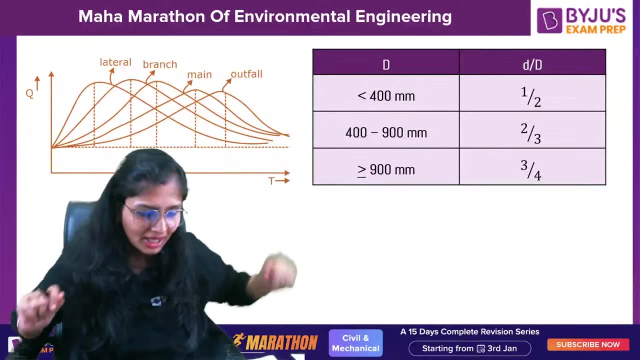 tell me arun, he took a bath with eight buckets of water. so that eight buckets of water he bathed that will go through the trap, it will go to the sewage. so at that moment the demand was maximum. but for laterals sewers the discharge is not maximum, clear. but we consider 80 percent of what 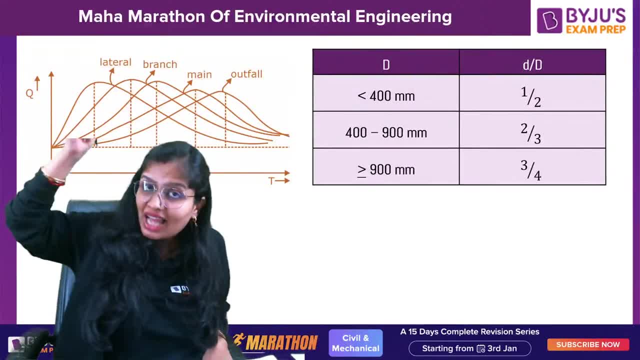 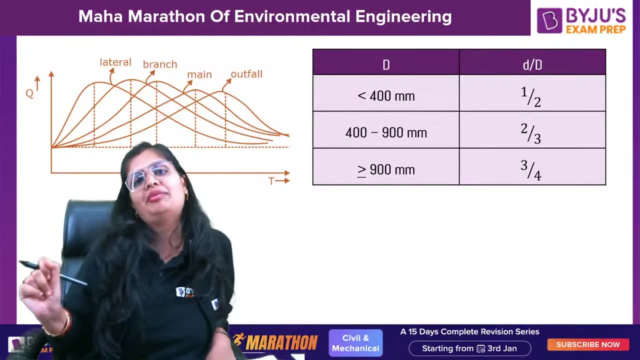 we get as supplies converted to sewage. i'm asking about that instant of time, girish, you are telling me the theoretical way of designing better. i'm telling you at that instant of time: okay, i'm telling that time. i'm talking about the time i'm not talking. 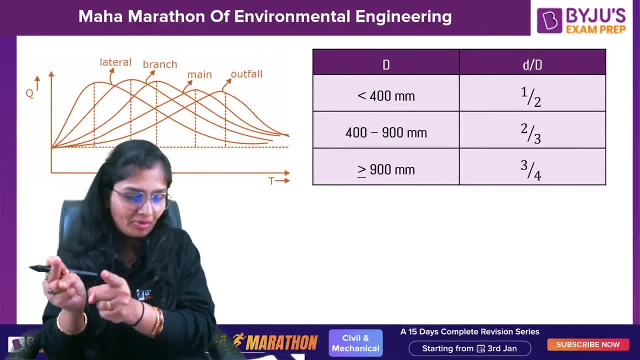 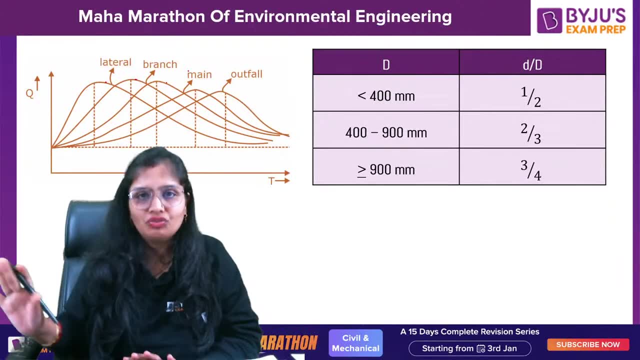 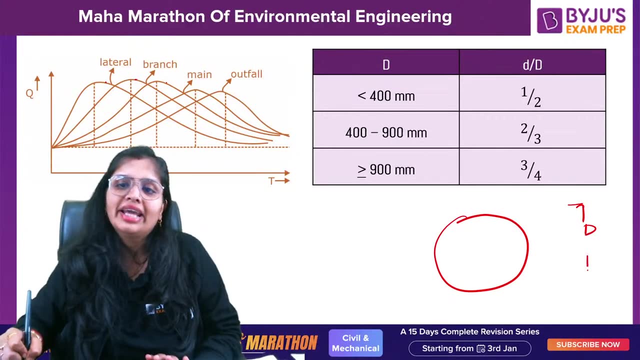 about the quantity. you are telling me the quantity and i'm talking about the time. okay, understood. so so lateral then branch, it will take time, then main then outfall, so it's not one time, it will happen next. as i already told you, this is the whole depth. 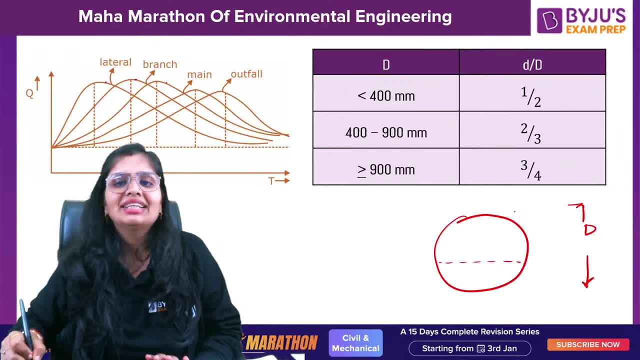 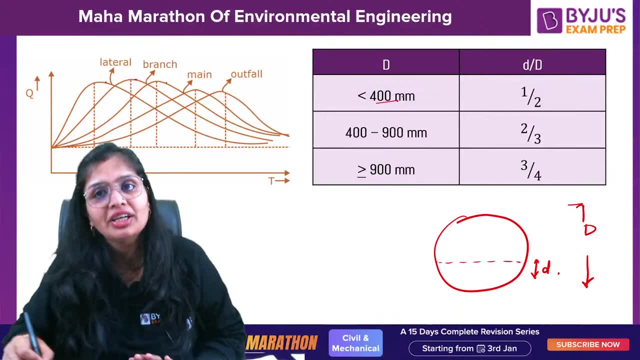 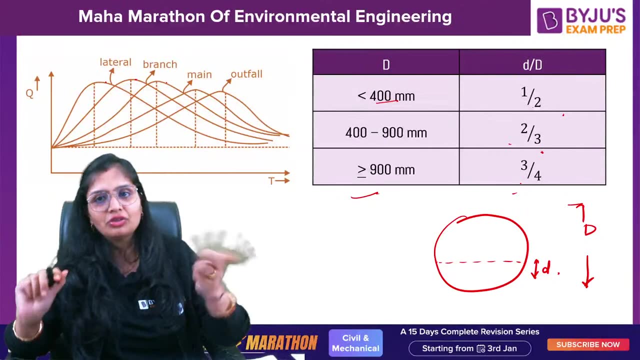 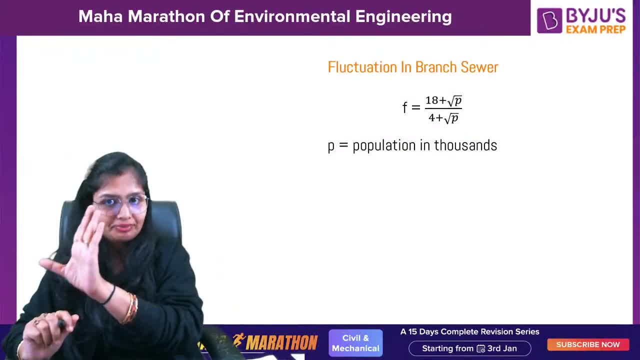 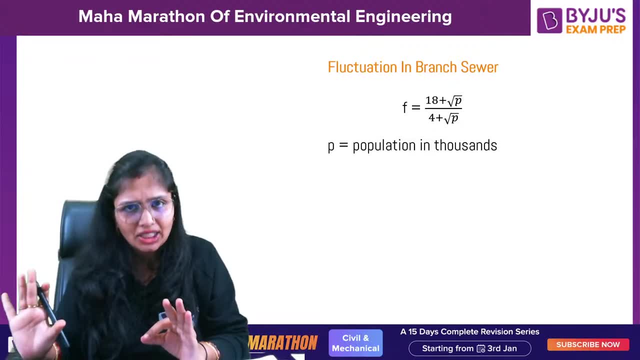 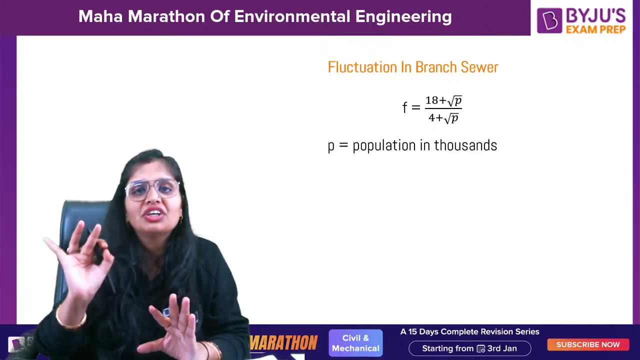 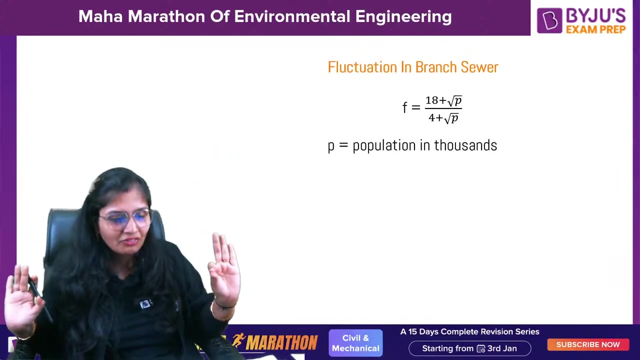 mind when you do the calculations. now remember one thing: they can ask you in one month if in the question, if this is for esc, conventional. but remember this: if never, ever, they have mentioned which type of sewer you have to design it for, design it for branch, if this is basically for esc, 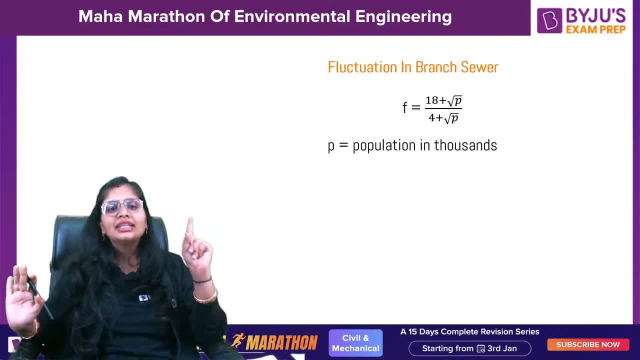 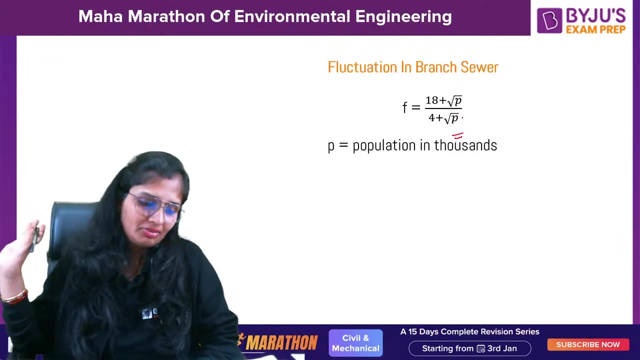 conventional. but you should know that if they are not telling you that, whether it is fluctuation is for lateral sewer branching with main sewer. you did design it for branch okay and the fluctuation is 18 plus root p upon 4 plus root p p is the population in thousand. as simple as okay. so now 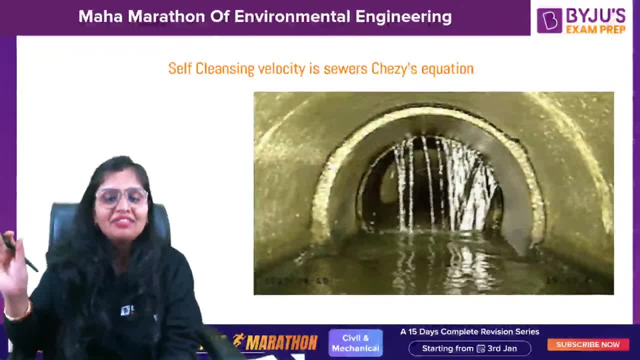 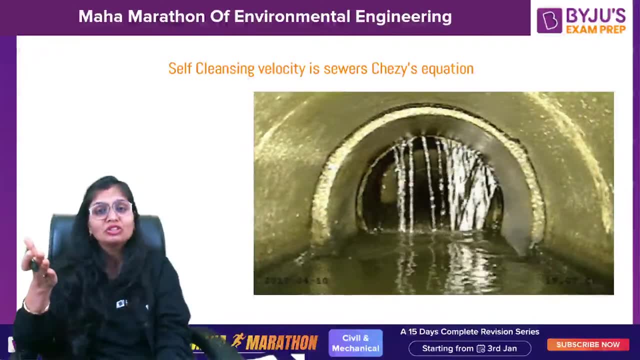 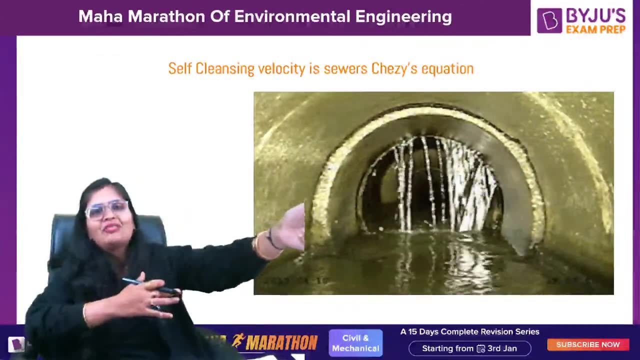 now now self-cleansing velocity. you can see the sewer now. i guess you can see. you would have seen it in hollywood and bollywood movies also- sewers and all hero goes there, removes his shirt, then lifts the pipe for doing the what you call for stealing: some jewelry, diamond jewelry and all so. 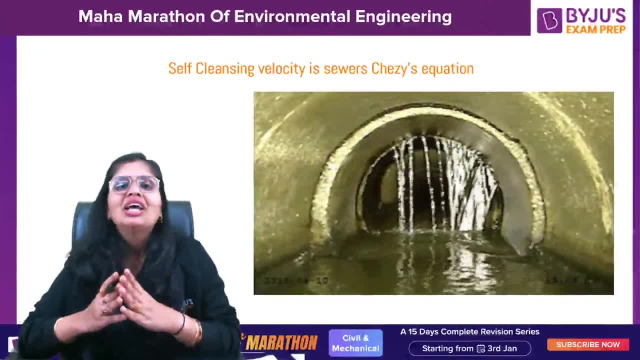 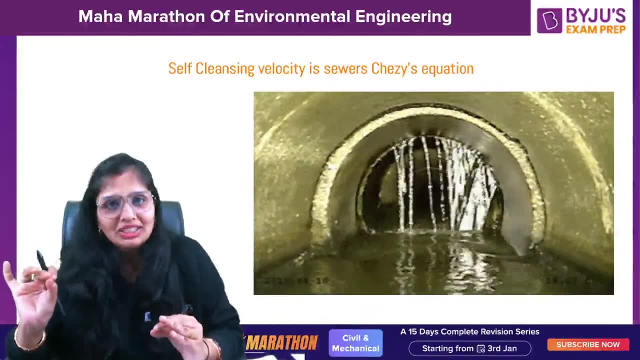 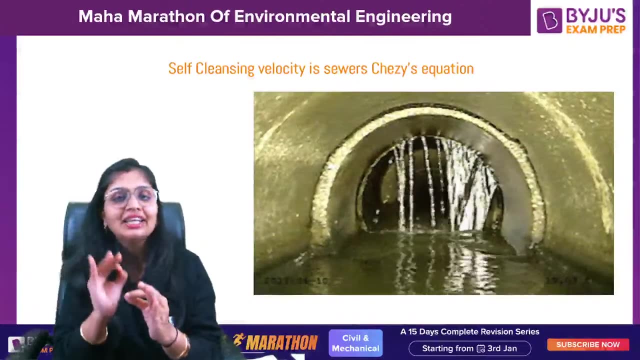 you guys would have seen the interior of sewers and all, so now let us talk about the self-cleansing velocity of sewers generally. when you talk about sewers, that is an open channel flow. i already told you, open channel flow does not mean it has to be open. it needs to have a free surface and it should be. 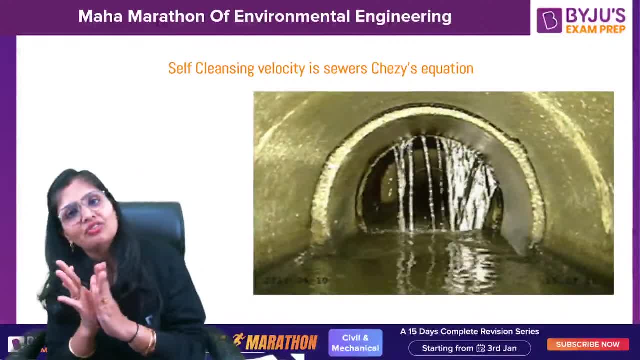 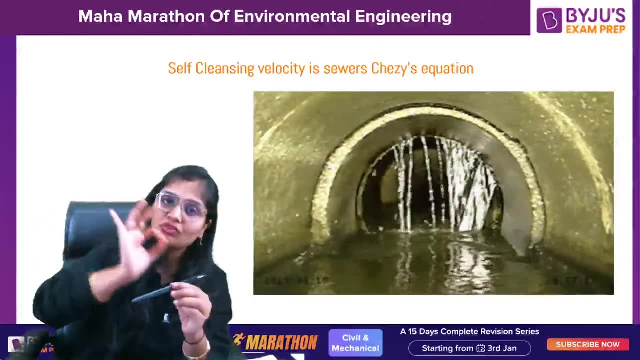 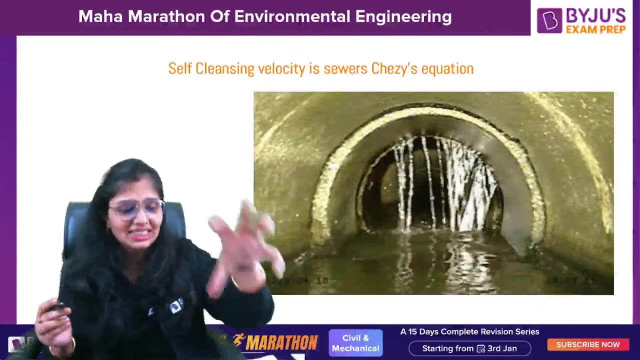 flowing flow of water takes place under the action of gravity, so that's why sewers are placed at a certain inclination- one, two degrees also sufficient, okay- so that water will flow under its own weight. here the water is the waste water. what we do when we design the 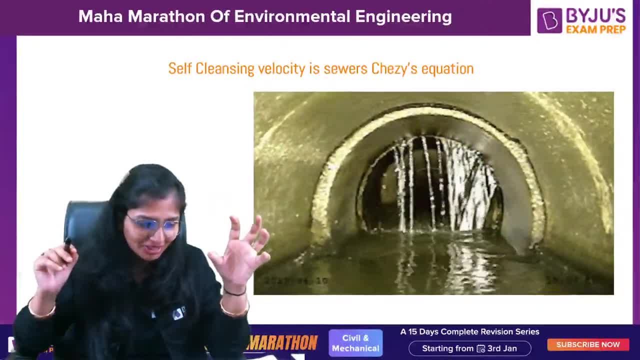 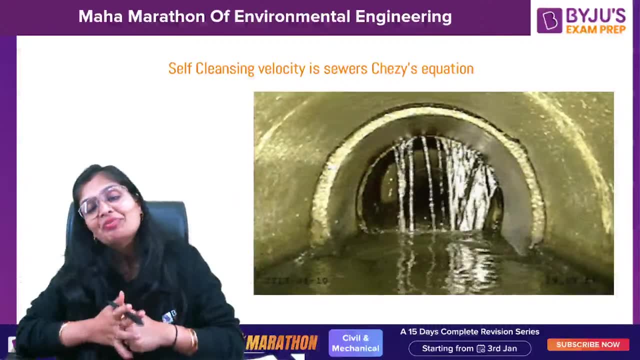 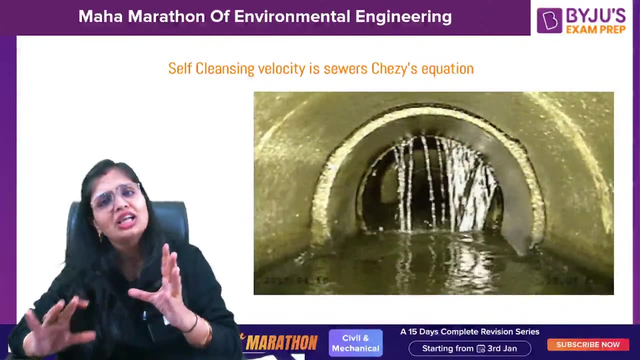 sewers we have to maintain spider-man, mission impossible, teenage mutant, ninja turtles- oh my god, now i have to see these movies. okay, so self-cleansing velocity. when you design the sewers, you have to make sure that a certain velocity should be maintained so that whatsoever solids. 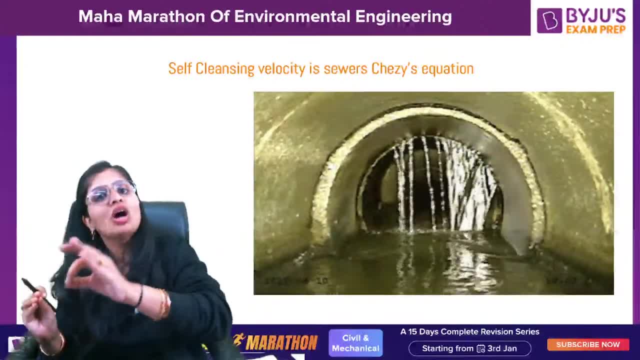 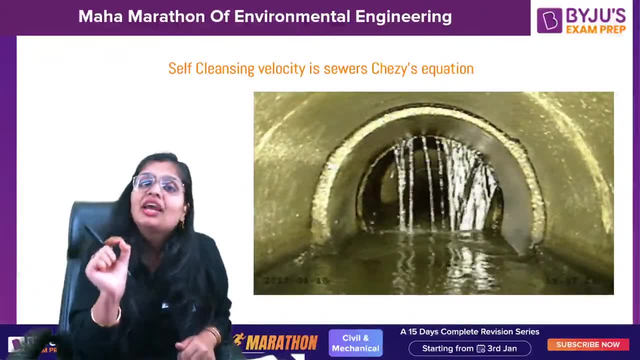 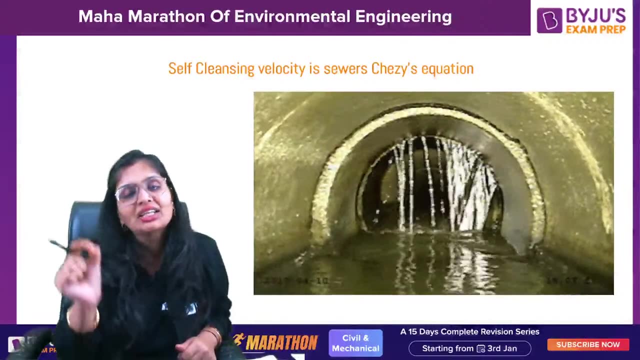 have already settled, they are removed, and no amount of solid should settle. so that's why we have to design the sewers, so self-cleansing velocity is the minimum velocity. okay, whenever you design the sewers, self-cleansing velocity is the minimum velocity so that the suspended solids does not. 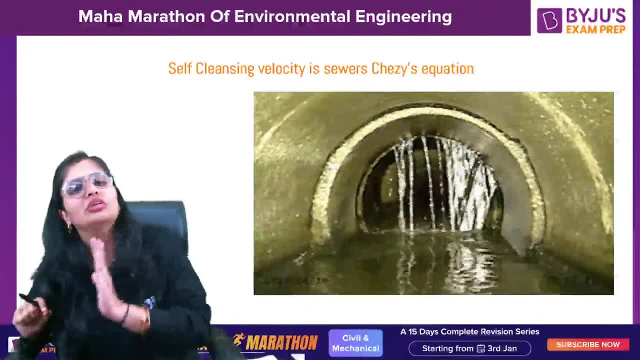 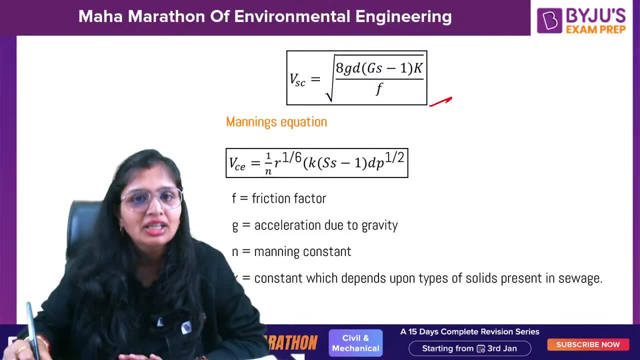 settle, and those solids who have settled, they should be removed. okay, now there are two formulas for this. this is by chesi's method, this is by manning's equation. so these are the formulas for self-cleansing velocity. okay, now we have to design the sewers so that whatsoever solids have already settled. 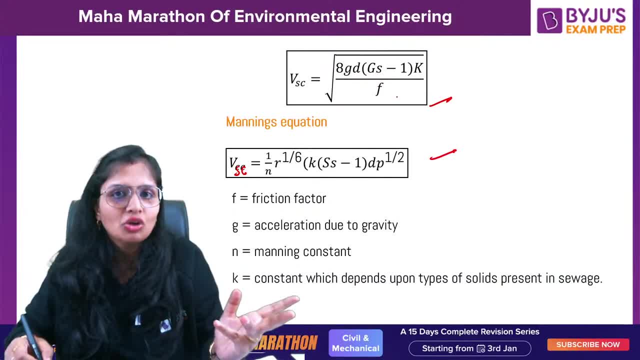 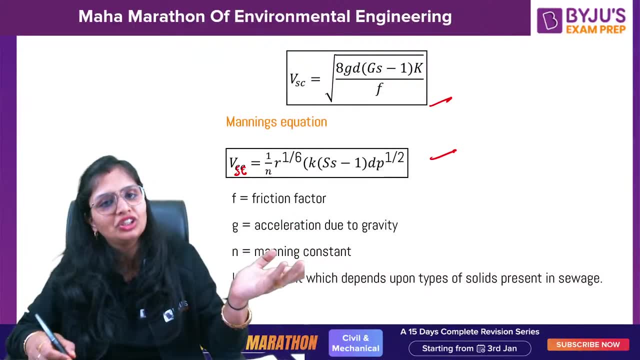 as root root over 8 g by f is chesi's constant. okay, so this is one formula, this is manning's formula. they, if they will mention the value of n, manning's roughness coefficient, you go by manning's equation. okay, you can write it as ss, as a specific gravity, or you can write it as gs, that's up to you okay. 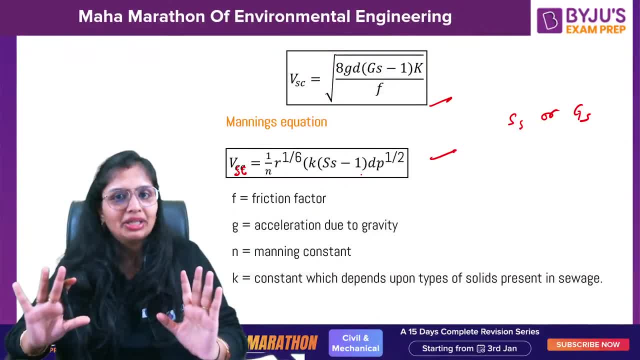 dp is the size of the particle which is present. okay, so this is the. this is the formula which you should know if you want to calculate self-cleansing velocity. okay, so this is the formula which you should know if you want to calculate self-cleansing velocity in sewers. now, now comes the next question. 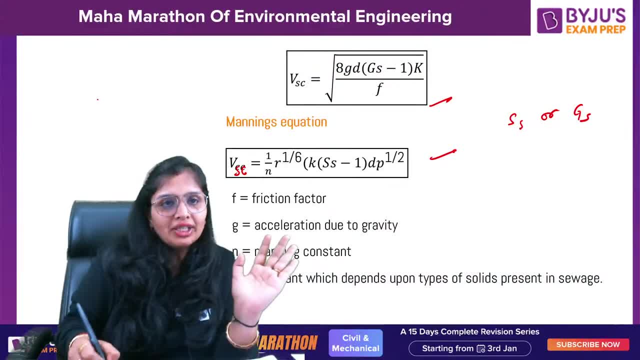 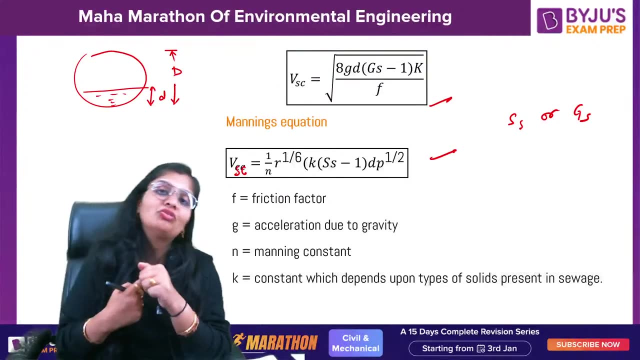 that if the water is flowing here, the water is flowing at full depth and the water is flowing at partial depth. okay, so if you want to know the area for this depth of water, the perimeter for this depth of water, the hydraulic radius, how you will go. so if this is the center, you know this. 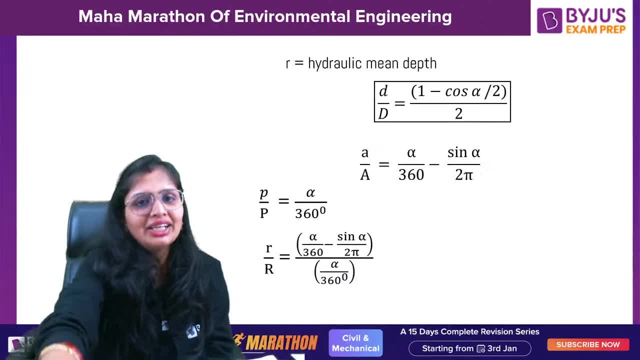 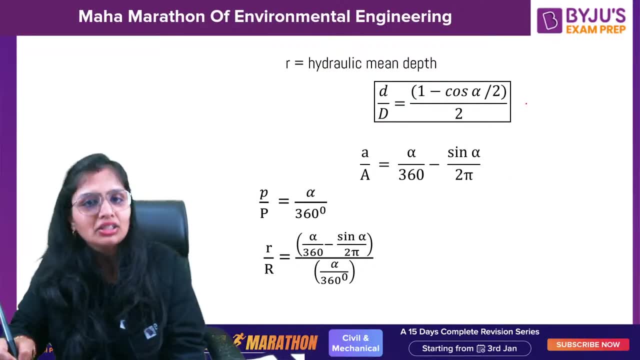 alpha. so all the equations, i don't think i need to derive it. so, d by d, the depth of water divided by the complete depth, that is, 1 by 2, 1 minus cos, alpha by 2. similarly, area, perimeter, hydraulic radius, you can calculate each of them. okay, even if you want, you can calculate velocity also. v by: 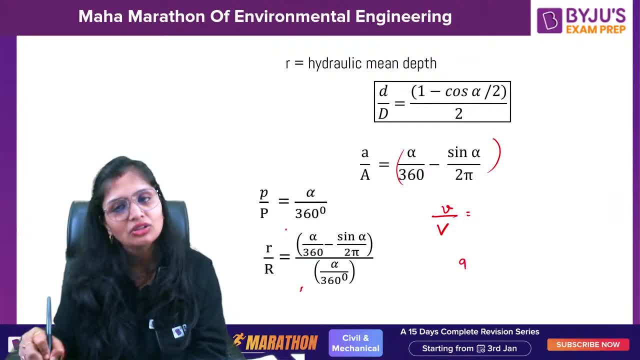 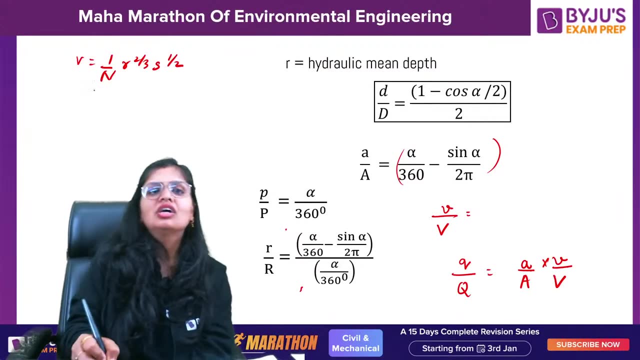 capital v. okay, you can calculate discharge also, small q by capital q, which will be equal to small a by capital a, into small v by capital v. and if you go by manning's equation you know velocity is 1 by l r to the power, 2 by 3 s to the power, half. so sewer is same, only the depth is changing. so 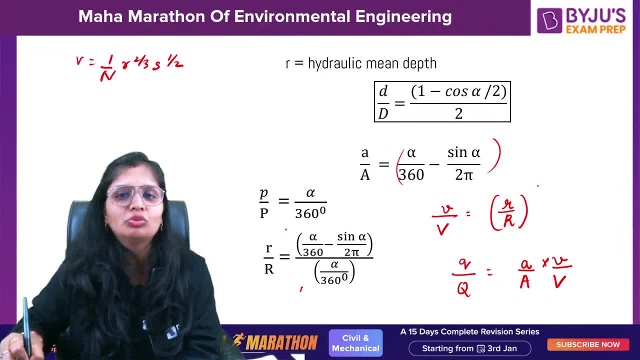 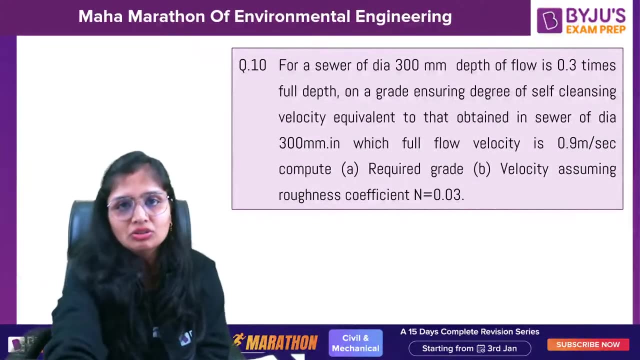 what you can do: small r by capital r to the power, 2 by 3. so exactly same thing is there, but the power is 2 by 3, okay, so this you should know, this you should know. okay, now let's solve this question. no, for this question to solve, i have to teach you this. wait a minute, huh. 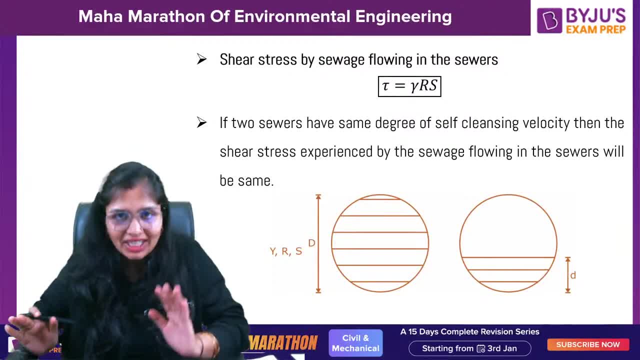 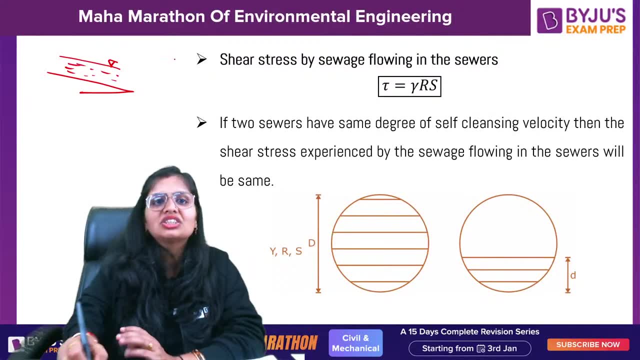 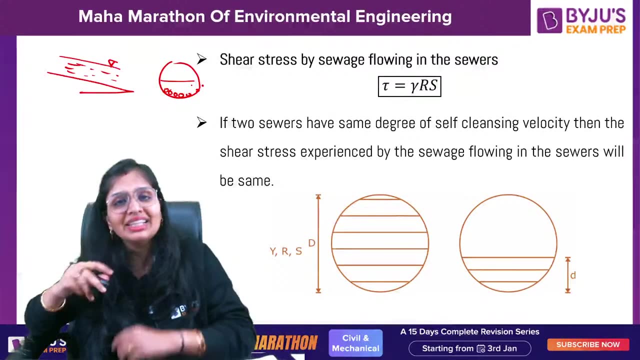 now the shear stress when the sewage is flowing. see, the sewage flows under the action of gravity. so when the sewage is flowing, there will be a shear stress which will be exerted. if you, this is the longitudinal section, this the solids are also. so what is happening? shear stress will be. 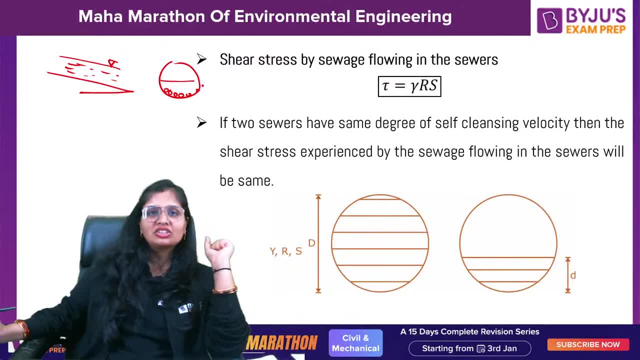 exerted. okay, so the value of shear stress not going through the derivation, it is gamma, rs. gamma is the unit weight of sewers, r is the hydraulic radius, s is the slope. now, if i say that this is one sewer which is flowing at any depth, capital d, this is another sewers flowing. 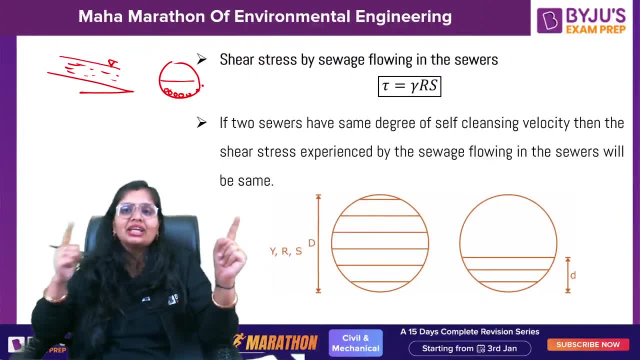 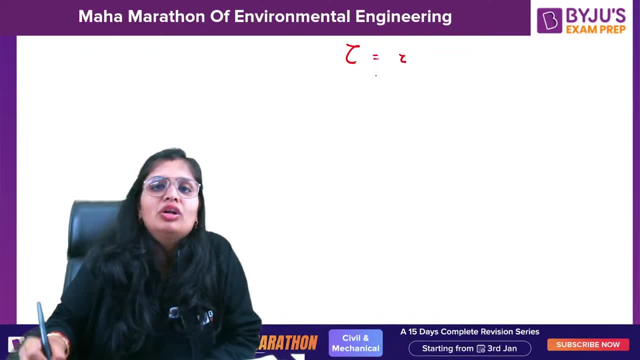 at depth, small d. if both the sewers have same degree of self-cleansing velocity, then the shear stress by them is same. this is capital. this is small gamma rs. this is, let us suppose, unit weight. this is gamma rs. if i assume c, the unit weight of sewage is slightly more than the unit weight of water. 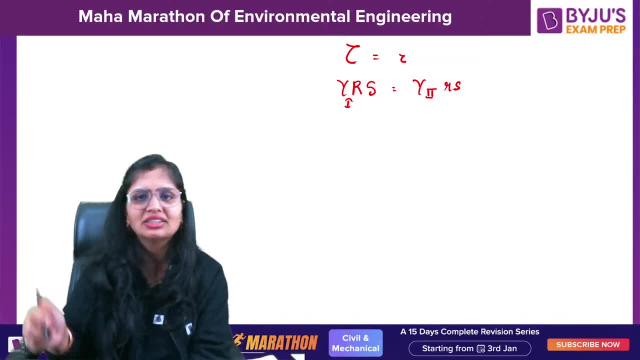 if it is, one is for, then there is 1.02 like that is there. so this will come out to me: if i take it, then my save r capital s r small s. so this will become r by capital, small r. this will become small s by capital. 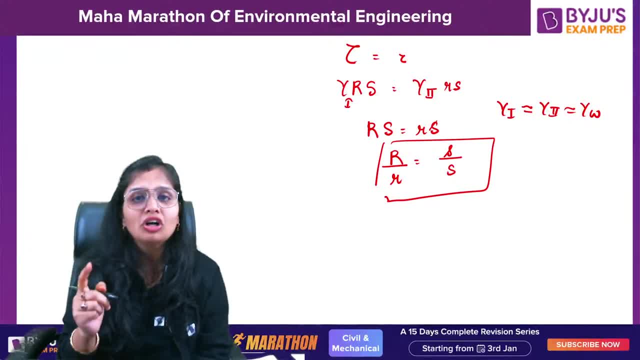 okay, this will happen. if you talk about the velocity, velocity will become how much? 1 by n? and this will be capital: n by small, n. r to the power 2 by 3, s to the power 1 by 2.. Now, firstly, it is not. 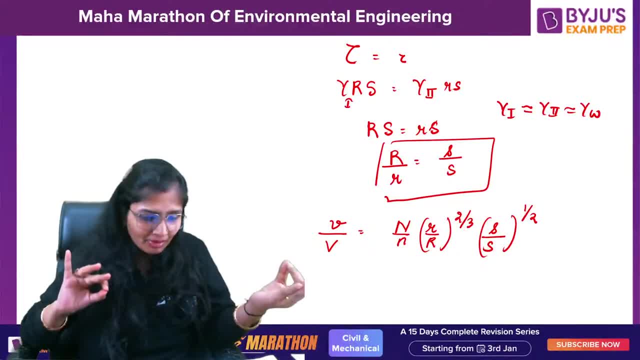 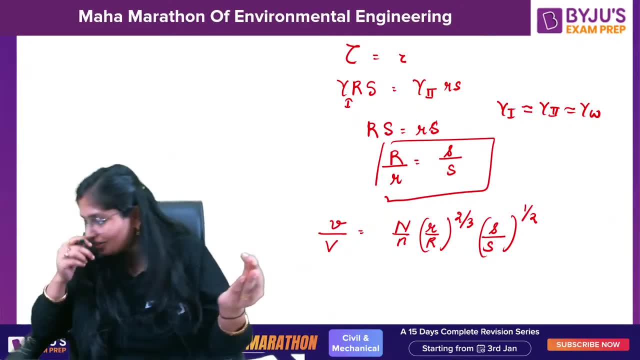 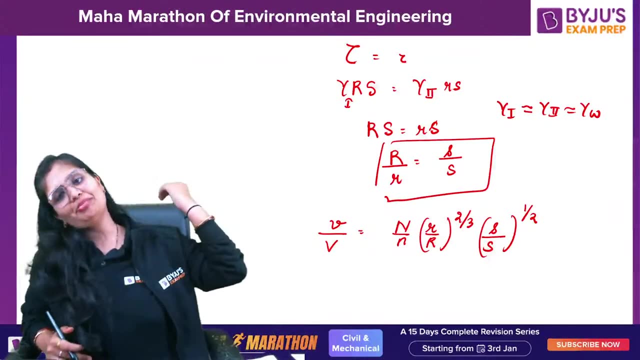 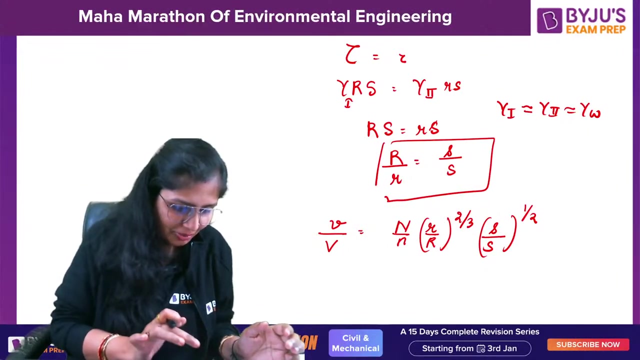 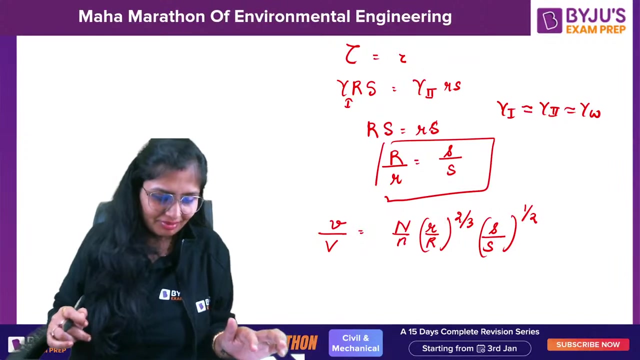 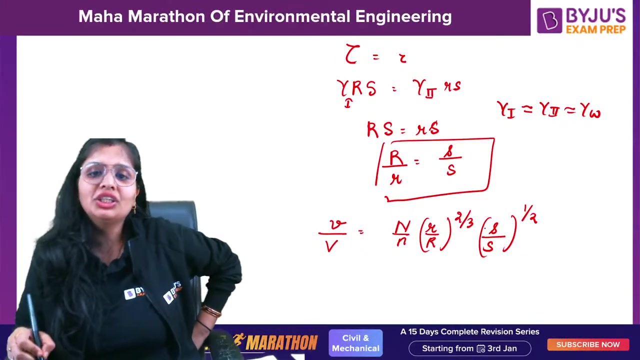 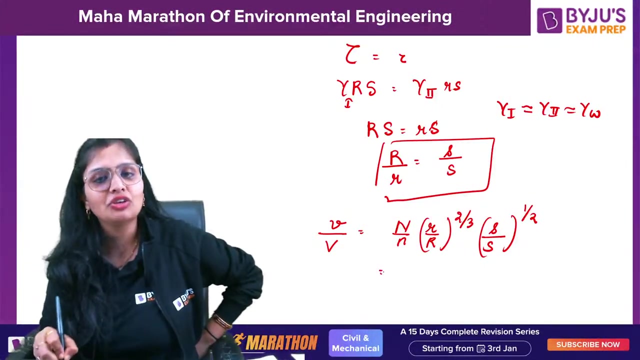 necessary that Manning's roughness coefficient is same. Now if in the question it is telling you: the Manning's roughness coefficient is same, it is same, Manning's roughness coefficient is same, then n and n will become same In. 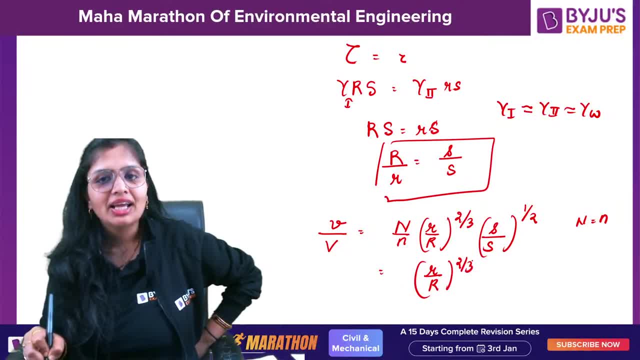 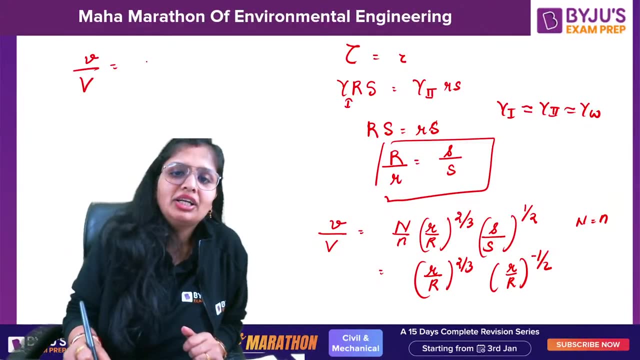 that case you will get r by r, 2 by 3 and in this place small s by capital S. you can write small r by capital R, minus half, My minus half, because r by r is there. so I just reversed it, so I wrote this. So the very important formula, very, very important, if 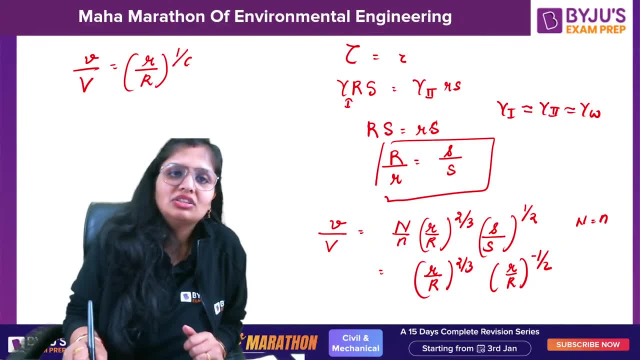 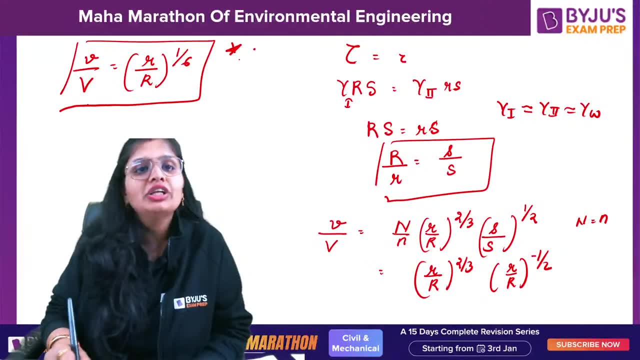 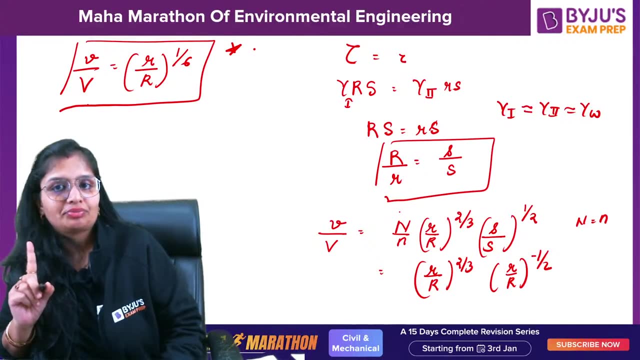 Manning's roughness coefficient is same for both the sievers. this is 1 by n, Clear, Very important. This you will use in this condition. If Manning's roughness coefficient is there, then that value will also come into action. Okay, This is used. 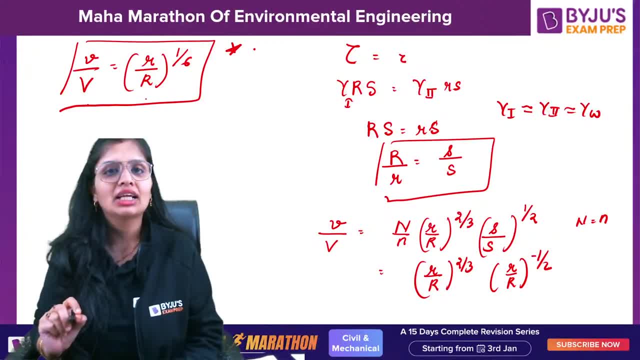 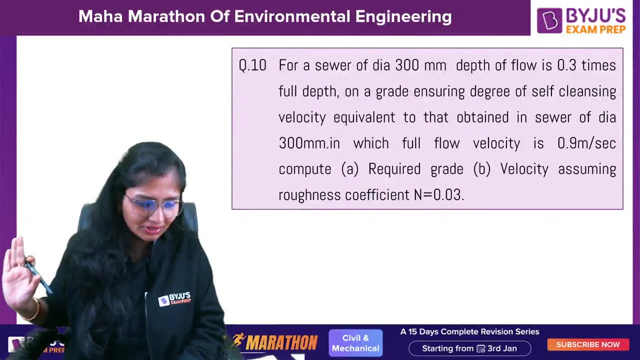 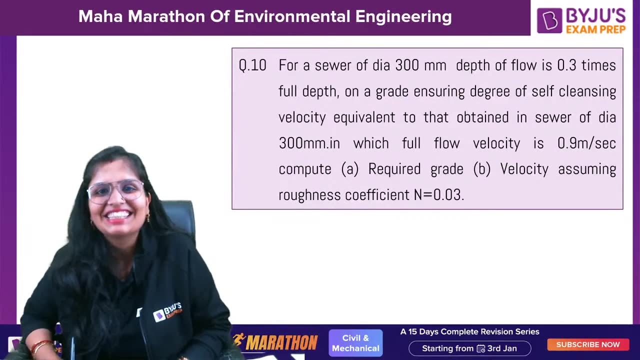 when both the sievers have same degree of self-cleansing, same degree of self-cleansing capacity velocity. Now, solve this question. This is a good question. Okay, Vishal, what a punch. Okay, Guys, solve this question. 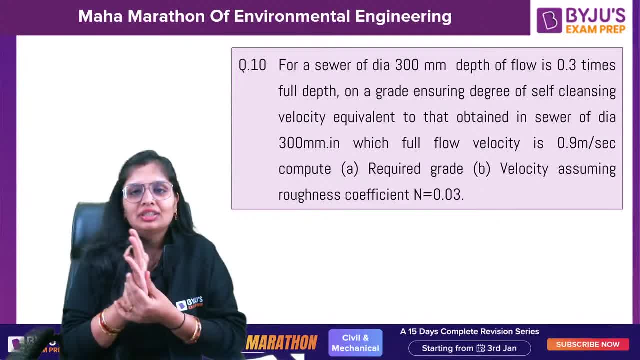 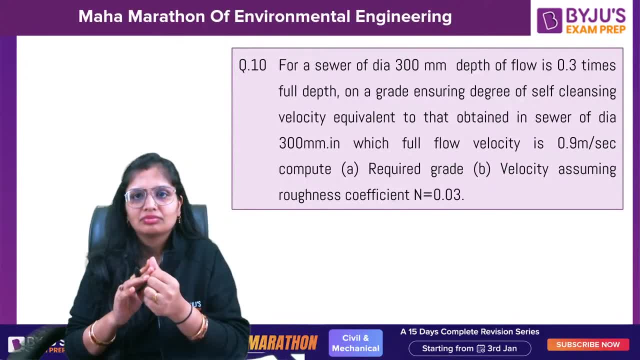 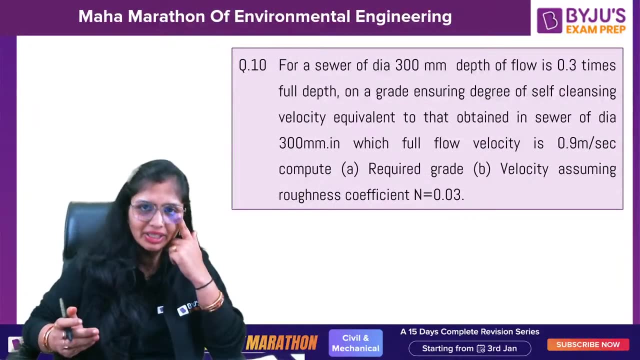 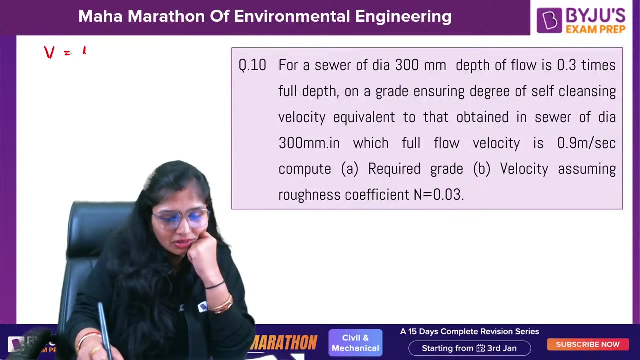 Come on. First you have to calculate slope. Slope is very easy. You can calculate right: R to the power 2 by 3, S to the power half, So 1 by n, 0.03.. R is d by 4.. The dia is given. 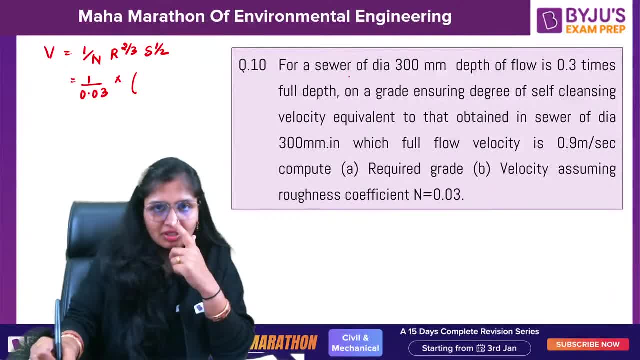 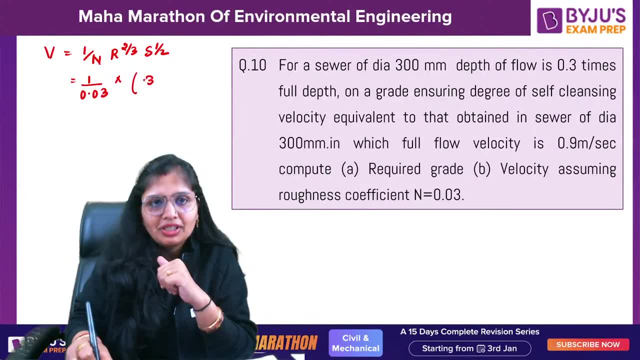 to you in the question right, 3.. Here it is asking me for full depth. I am taking, If it is asking me, 0.3, 4, 2 by 3. Slope, slope, slope. I need to calculate. 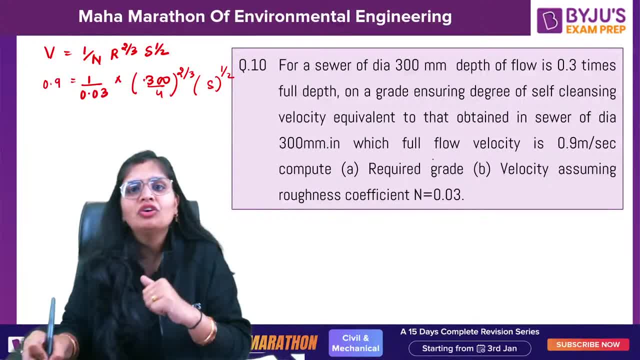 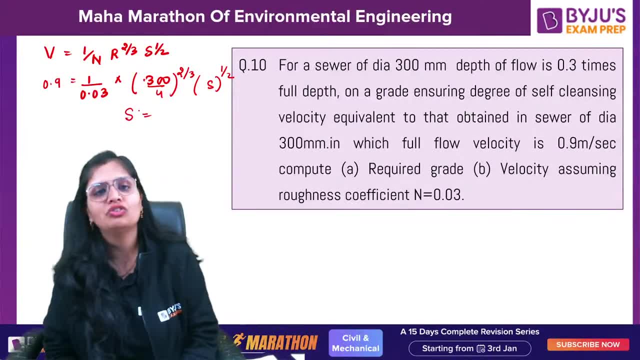 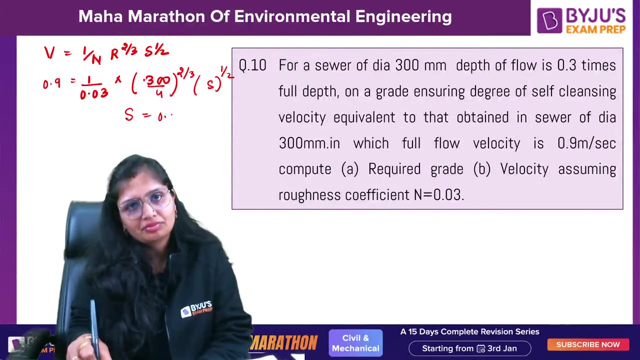 Velocity: it is 0.9 meter. Full flow velocity: it is telling me 0.9 meter per second. So I am calculating slope corresponding to full flow velocity. How much it is coming. Second part is interesting. Come on, guys, How much it is coming. Just check it out. Is this coming? 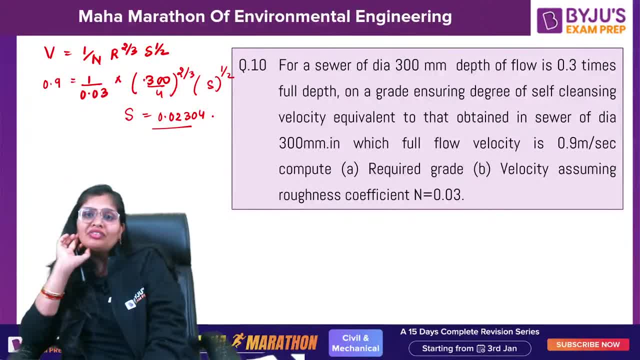 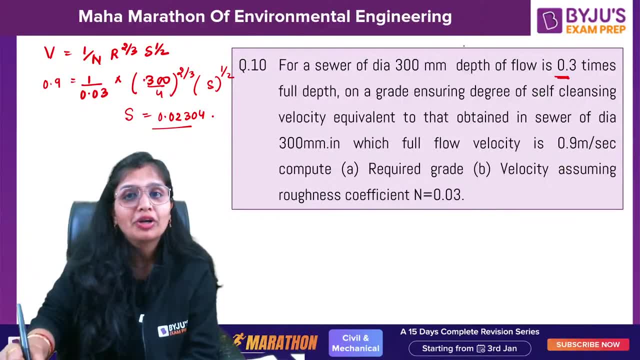 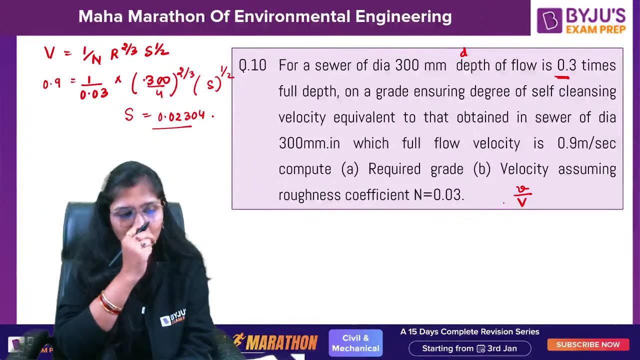 No. Now, second part is velocity. assuming velocity, it is asking you. That means it is asking you velocity corresponding to velocity corresponding to small d, That is, it is asking you small v. How you will calculate it. How you will calculate it, You know. right now I need 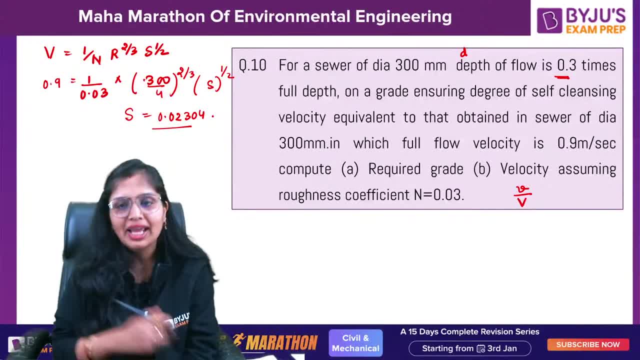 to calculate small v. How will I calculate it? Come on guys, Capital V is given to me in the question- 0.9 meter per second- And it is asking me- you see, it is written: depth of flow is 0.3 times the full depth. So it is asking me velocity corresponding. 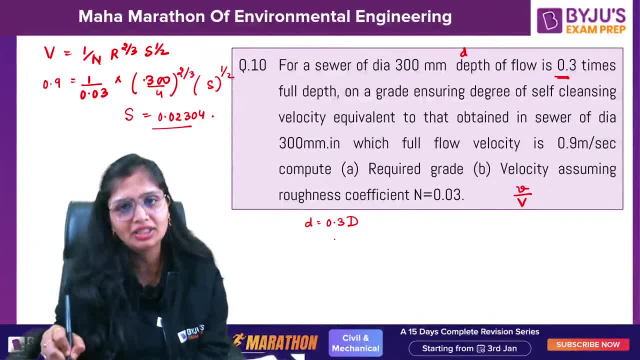 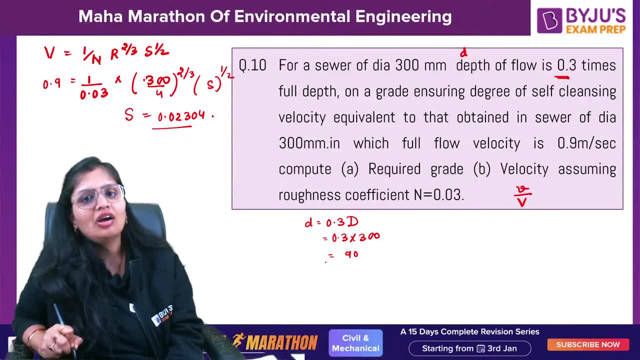 to 100 mm depth of flow. No, this is not 100. This will be 0.3 into 300. So this will be how much? 90 mm depth of flow. So how you will calculate it. Now, anybody want to give? 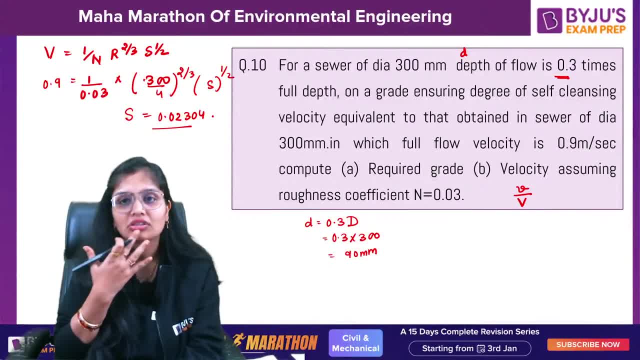 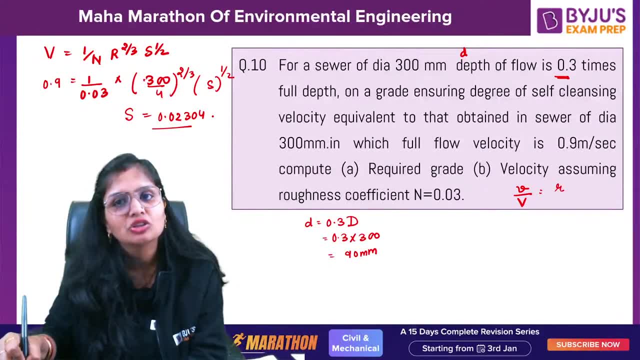 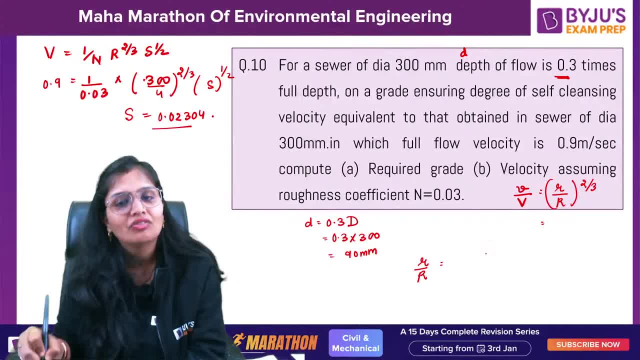 And I told you small r by capital R was alpha by 360 minus sin alpha by 2 pi divided by alpha by 360.. But now we don't know alpha. You can calculate it Why? Because I know small d by capital D is half 1 minus 0.5. 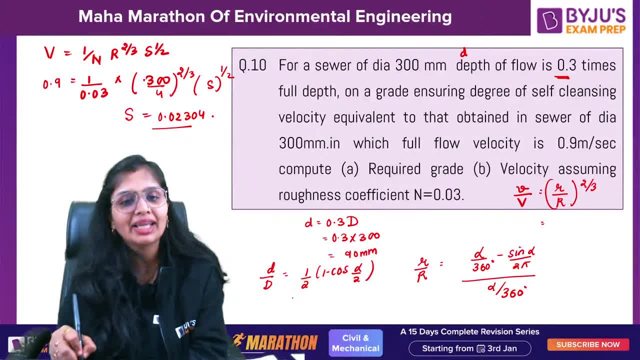 cos alpha by 2. And small d by capital D. I know it is 0.3. Come on guys, Arun, Tiksha, everybody calculate alpha now. So this was the question: All the 2, 3 formulas, they. 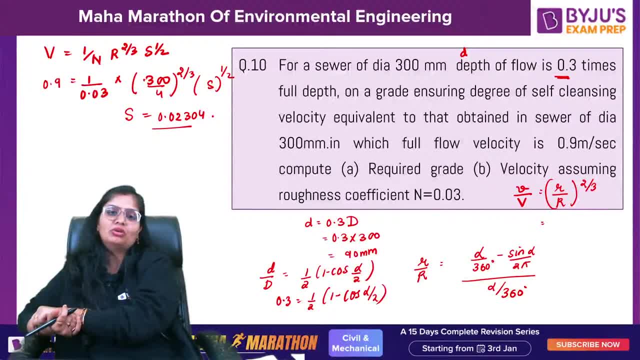 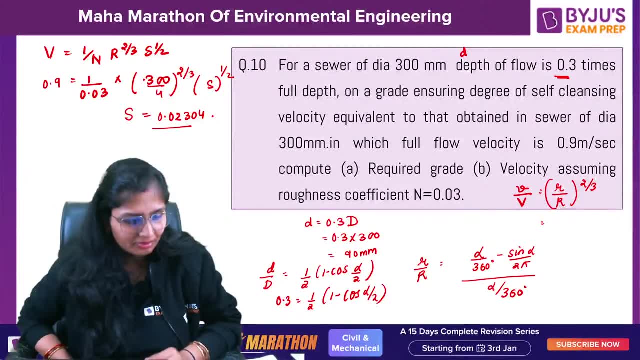 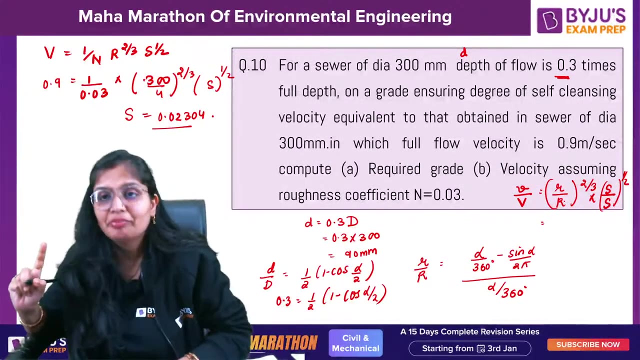 have added, summed up, and they gave you this problem. Come on, solve it. Very good, We will use it, because we will use it s to the power. this will be also there, But but we take everybody, since in the question the slope is same. they are not changing the. 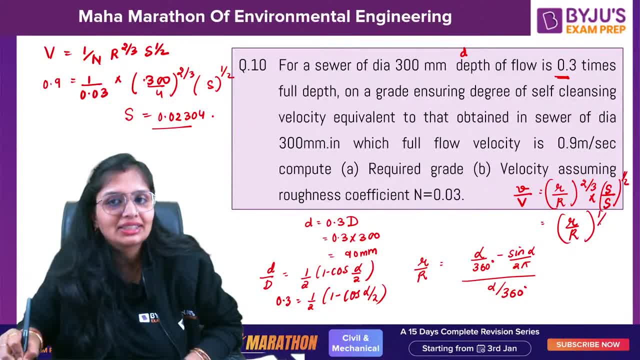 slope. So we will do it r to the power 1 by 6. Because it is talking about the same siever only, they are changing the depth, Or if they have taken different, different sievers also, but they have maintained the slope to be safe. Come on, calculate alpha. 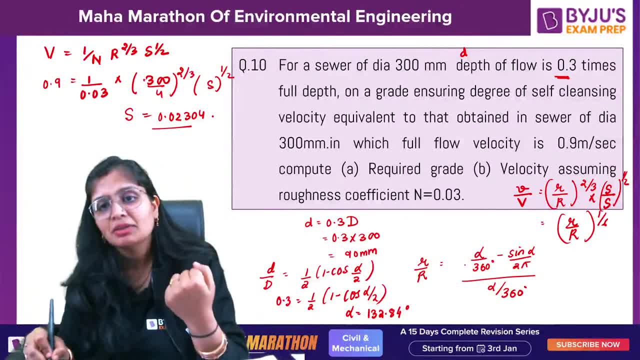 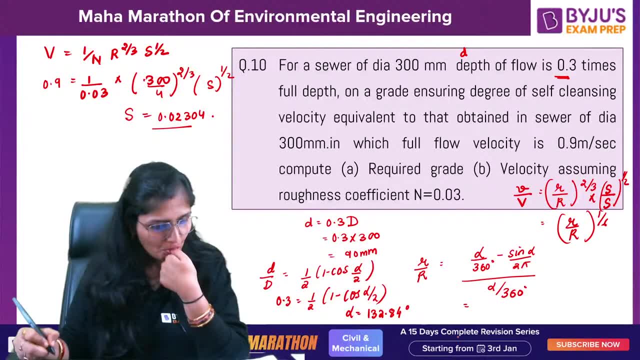 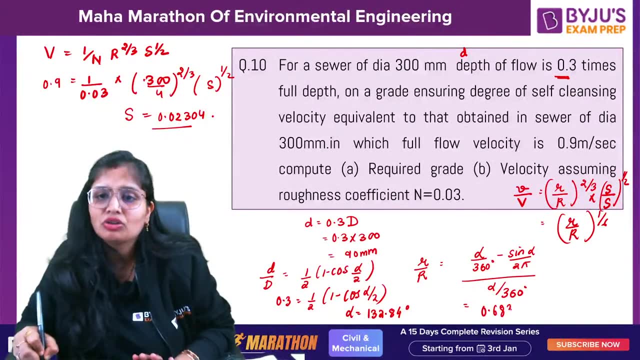 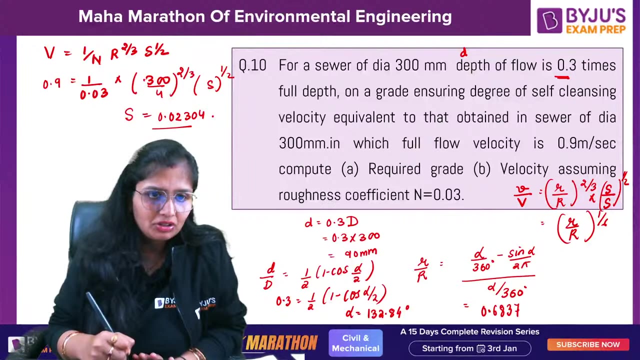 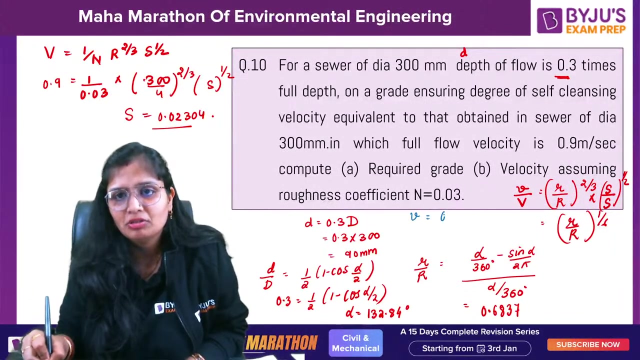 Substitute it here, Good, Substitute it here and calculate the value of r. It will come out to be 0.6837.. You guys can check it out Calculations. you should check it out. So small v will be 0.6837 to the power 1 by 6.. 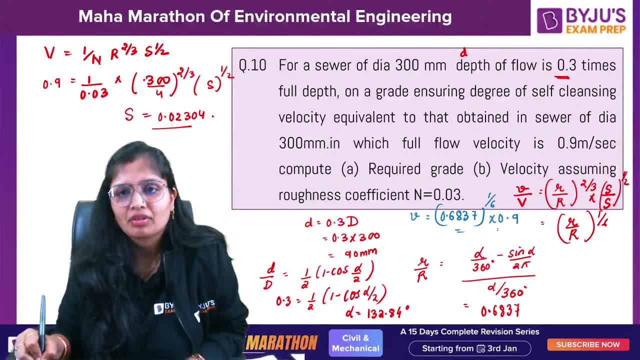 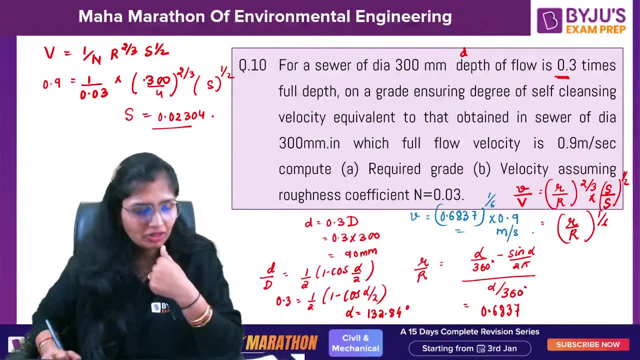 And then if we take smaller v, it will be 0.627.. Now, this isЯll change the value of the siever here. So you are cute if you see here. then these are the values, So you. 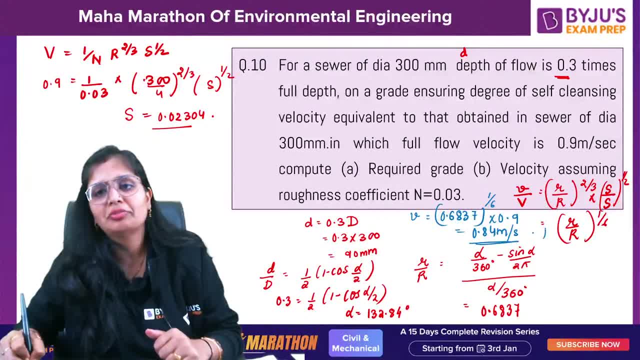 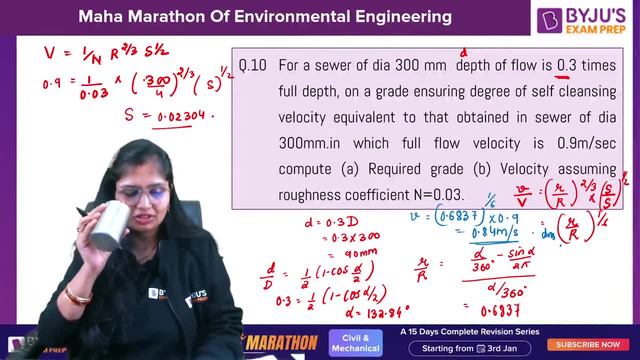 can see that the this is actual value of the siever here, So that the point is 0.627.. And then here this is A1 plus Jacobi V, V. Now you will have the sum of A1s and A2s. 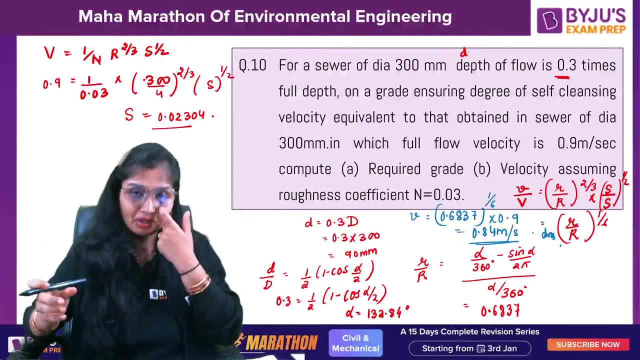 This is the function of a vector. So the function of vector is a vector. So I am going to write the vector here. So I will put here: I have written vector. Okay, So I am going to write the vector. So I am adding a value of vector. I am taking a vector here, I am putting there. 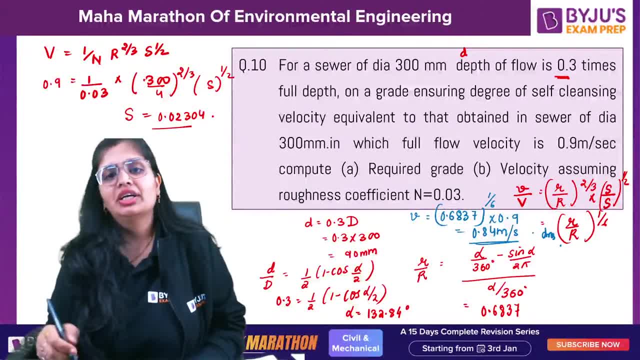 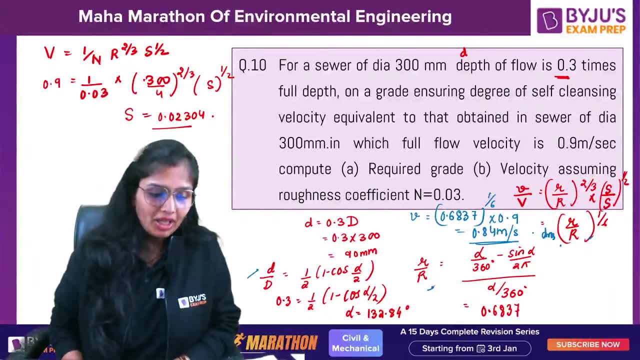 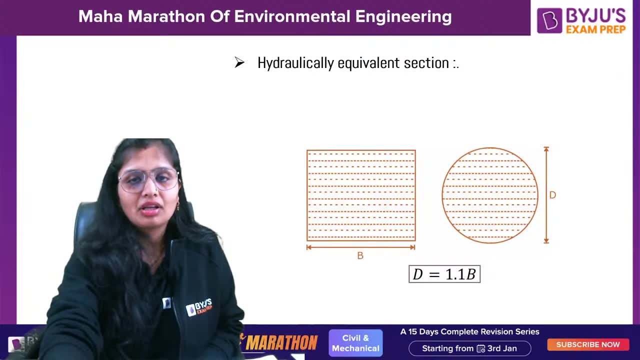 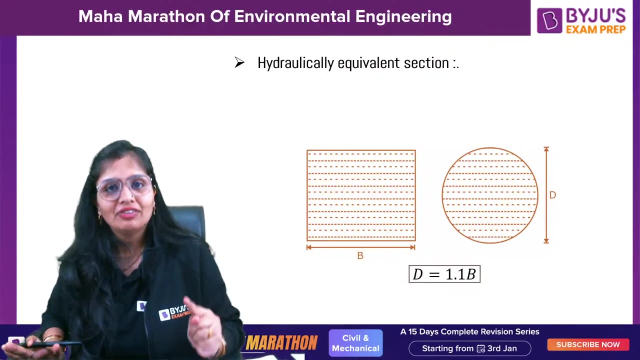 Okay, So this will be the velocity. So see this formula, this formula, this formula, three formulas are used for getting the value of velocity. So such sort of questions they can ask you. Okay, Now coming further. Hydraulic equivalent, section Two. sewers are said to be hydraulic equivalent if they carry the same discharge. 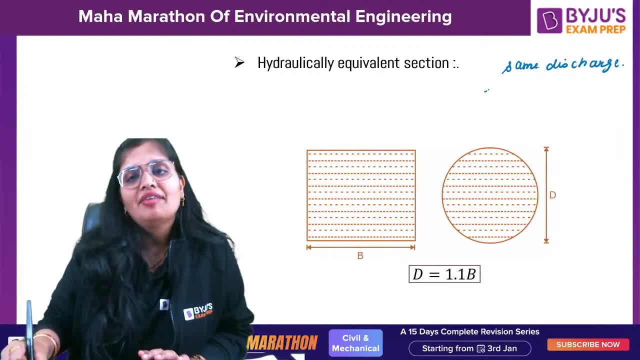 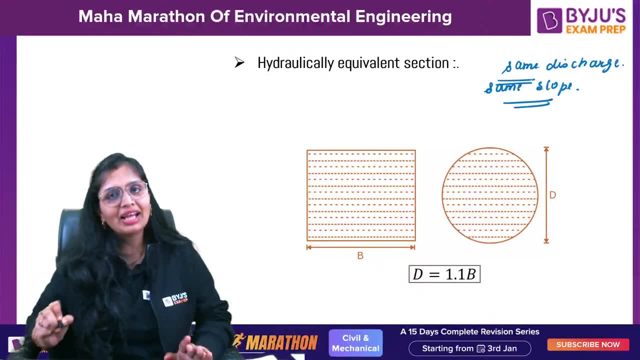 And they are having and they're running on same slope, Okay, So that discharge is same and the slope is same. Then you call it as then, hydraulic equivalent section. So if this section is there, this is square and this is circle. So what you can do 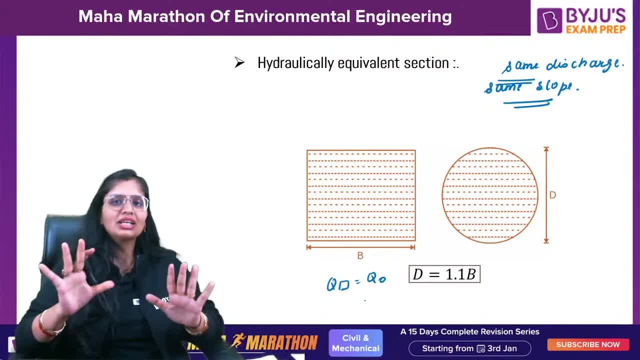 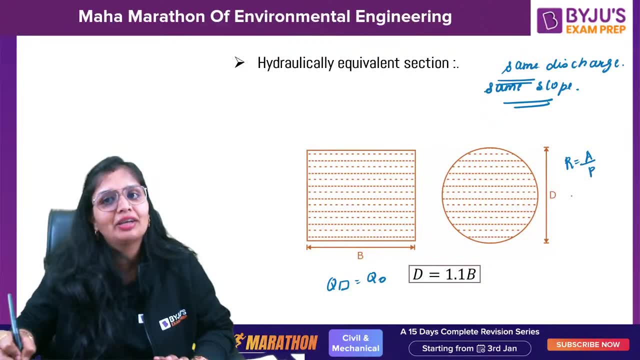 The discharge is same. You will cancel the slope And right now I'm assuming it that they are running on full depth. If they're running on full depth, So for this hydraulic radius is wetted area by wetted perimeter, So this will be D by 4.. Okay, 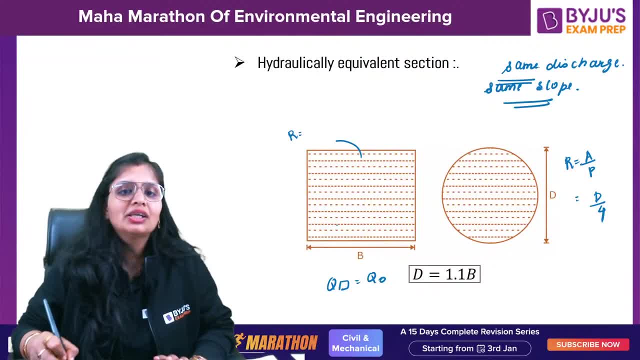 And for this hydraulic radius will come out to be how much A wetted area by wetted perimeter, So B into this. This will come out to be B. square Perimeter will be 4B, So this will be B by 4.. 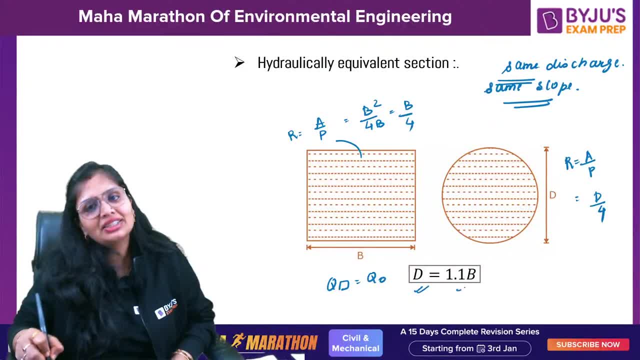 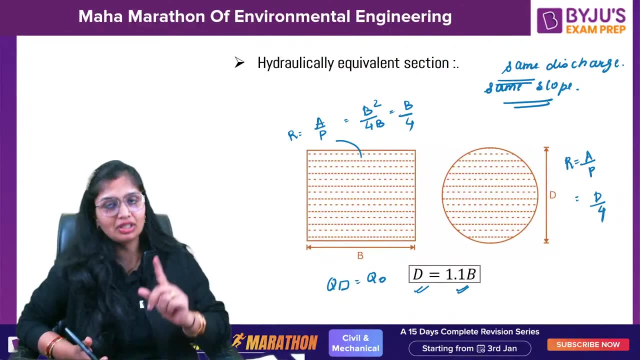 So on solving it, you will see that diameter is equal to 1.1 times of the side of the square. Okay, So they can ask you Sometimes these things. So you should know that. Okay. Now one thing more I'll say. This is very important. 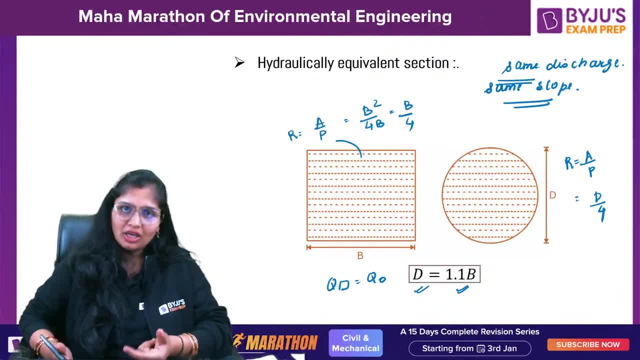 Generally, we prefer circular sievers, But why? Because the fluctuation in velocity and discharge comes out to be less, But all the benefits you will get only when the depth is more than 0.5 times the diameter or the total depth. 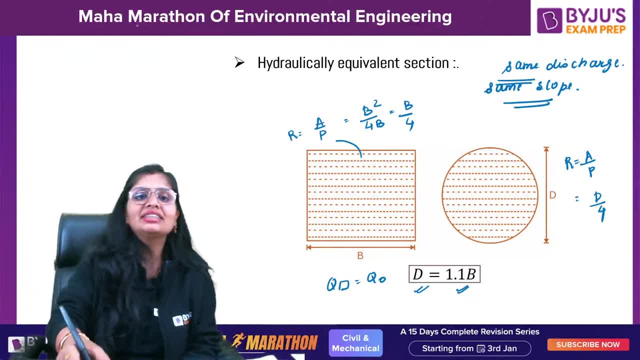 If it is less, you won't get the benefits. That's the reason Then we go for X-shaped siever, So I'm drawing it by free hand. Generally you guys have seen sievers like this. So the upper siever, this is D. 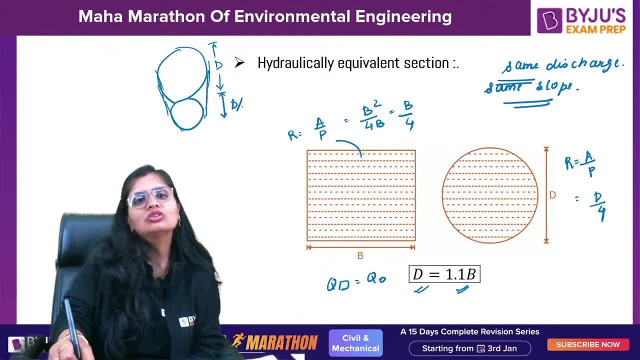 So this will become D by 2.. Okay, So generally, the upper siever is used for the rainy season And this is used under normal condition. Why? Because, beta, if you are designing a combined siever, Okay, Combined siever. 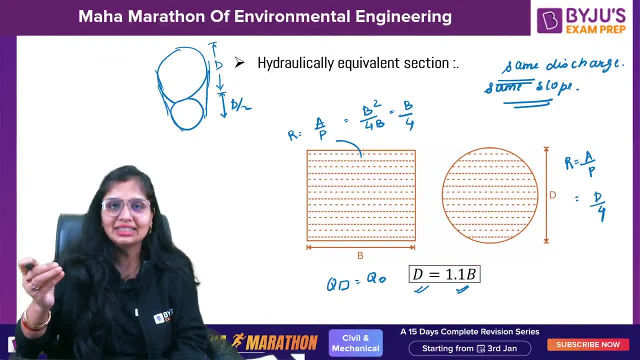 I'll tell you right now: Combined siever. So in that, In that case, in that case, what you will see? rainwater and then sanitary sievers both get mixed, Okay, So in that case, self-cleansing velocity is maintained. 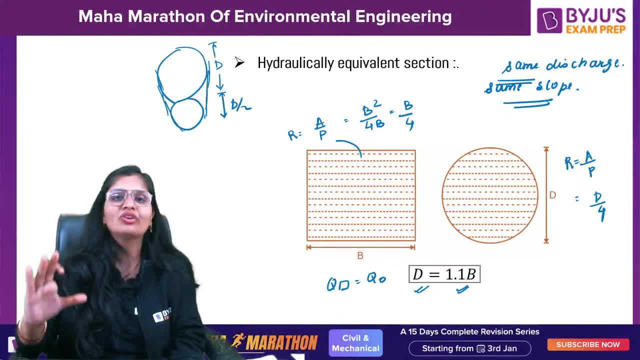 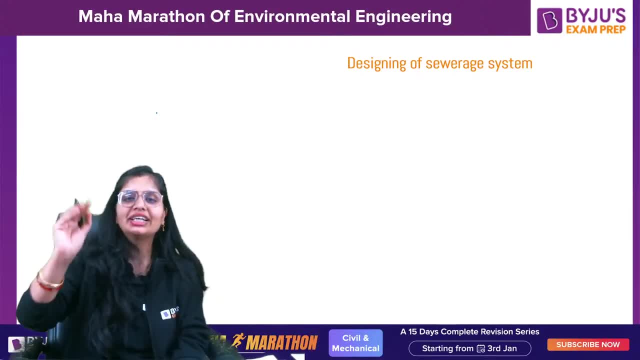 But when the rainfall is not taking place, self-cleansing velocity will not be maintained. That's the reason. In that case, you will go for this. Okay, Now, what Girish was telling? let's talk about the design. 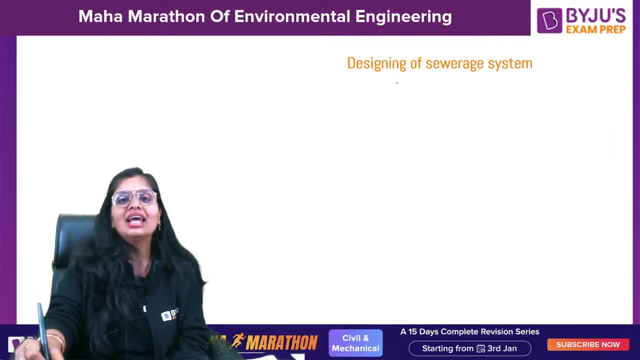 Designing, as he already told us. let us suppose if X is the population, The per person is water demand and P is the population. So the total water demand comes out to be P into X. Already told you, 80%. generally, 70 to 80% of the water supply is taken as converted into wastewater. 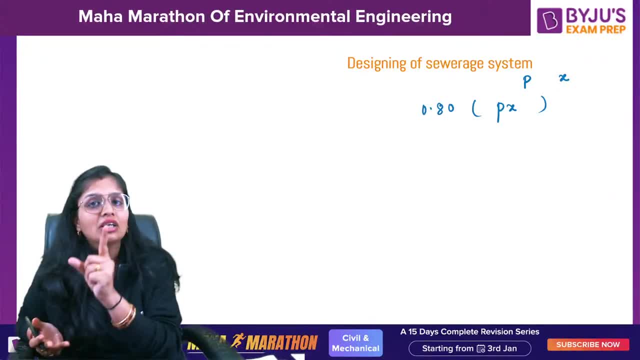 Two things Very important. First thing: read it in the question carefully, Whether it is written water supply or whether it is written as wastewater. Okay, If they are writing raw water, You have to multiply by 0.80.. If they are not mentioning raw water, or if they are mentioning raw water, you have to take it 0.80.. 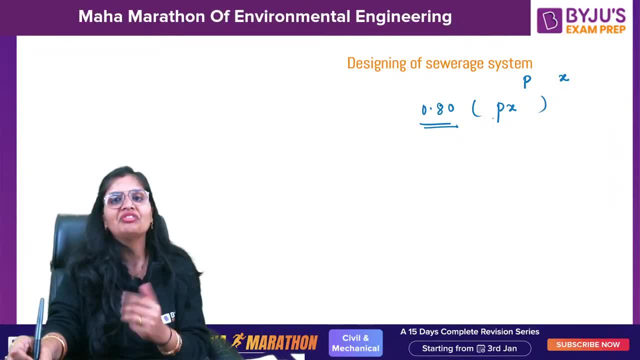 So remember, if not mentioning or basically they have written the wastewater supply just P into X, If they are mentioning, it is the raw water, multiply by 0.80 P into X. They'll mention 70% converted, 80% converted. they mentioned 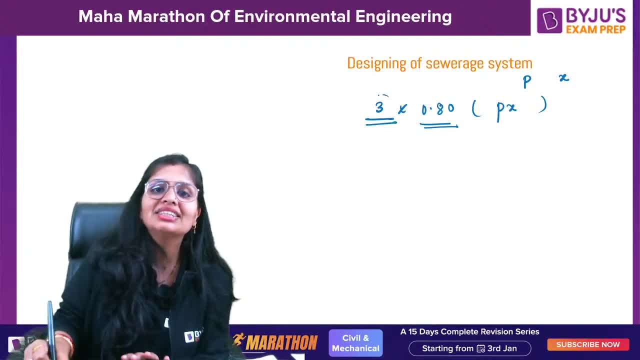 And you will multiply by 3.. 3 is the Fluctuation in branching. Okay, So you multiply, because you design it for peak value, So you multiply by 3.. Now coming further, coming further here. rainwater is also there, because when you design combined sewerage system, there are three sewerage system. 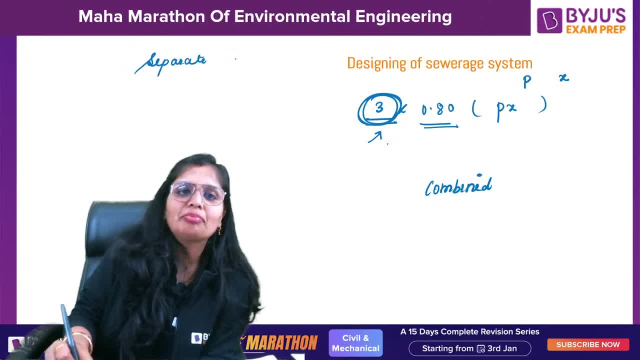 One is separate In separate sewerage system. what happens If this is a ground level? you know already. all pipes are laid below it. This is the water, This is the pipe, This is the pipe for drainage, This is the pipe for sanitary sewage. 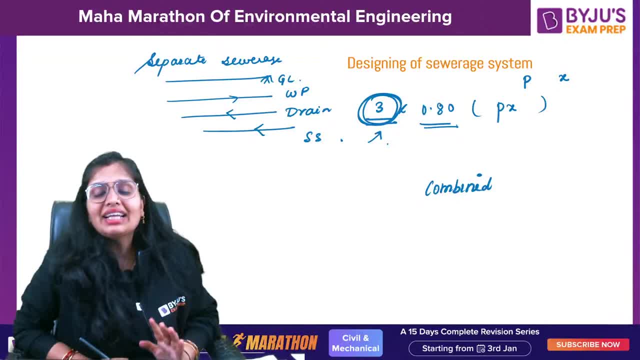 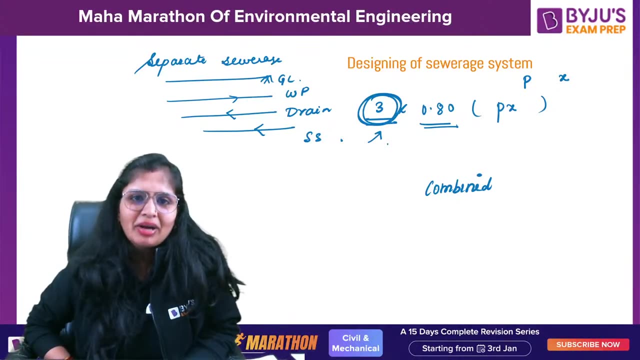 So generally, you will see. generally you will see what that in this condition, laying of pipes is costlier. in congested roads You cannot apply. However, the treatment is reduced because drainage water, the water from the rainfall and all that contains inorganic particles. they won't contain organic matter. 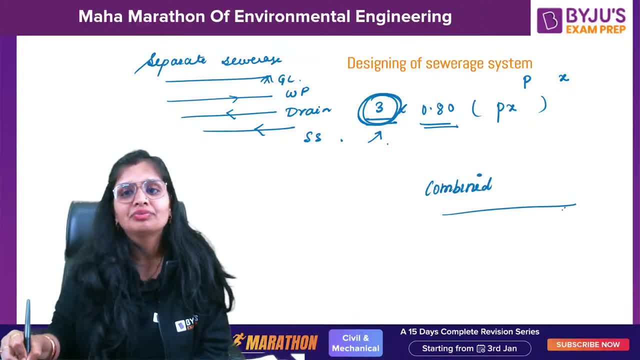 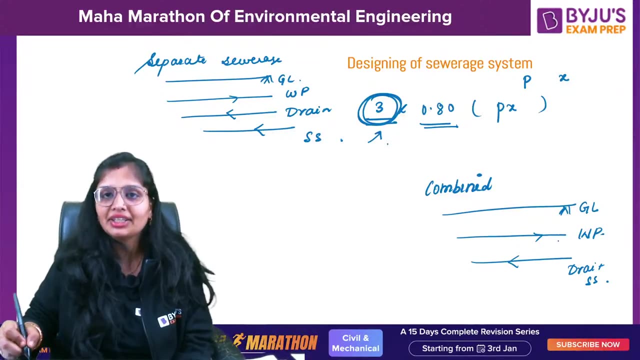 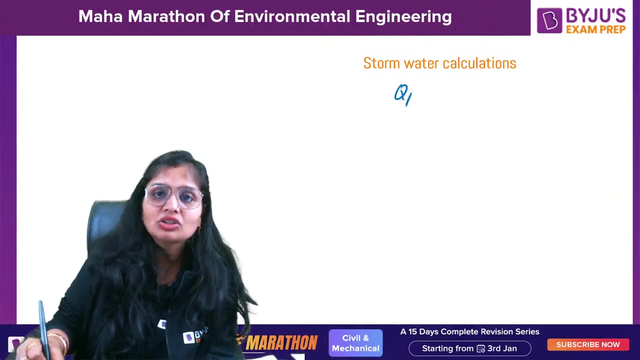 So drainage cost is reduced in combined What you do. So you are, we are at gulf again. you have only one by both for drainage community, Okay. So in these conditions, conditions and all, you make sure that you multiply by the phlactor 3, okay. 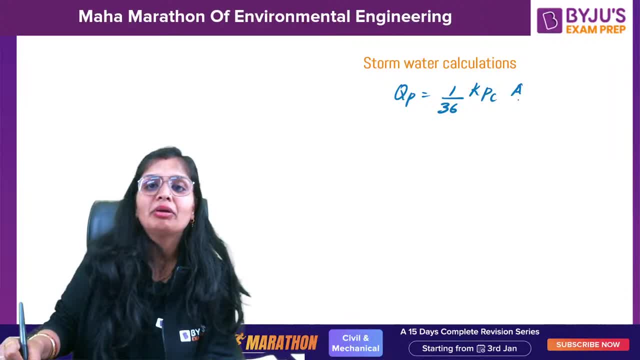 But this is the water only for sanitary sewage. 36 k PCA. Remember, this is in hectares or kilometers square, This is the rainfall intensity in centimeter per hour and this is in hectares. This is the catchment area in hectares. This formula you should know, Okay, and you will get the discharge in meter cube per second. 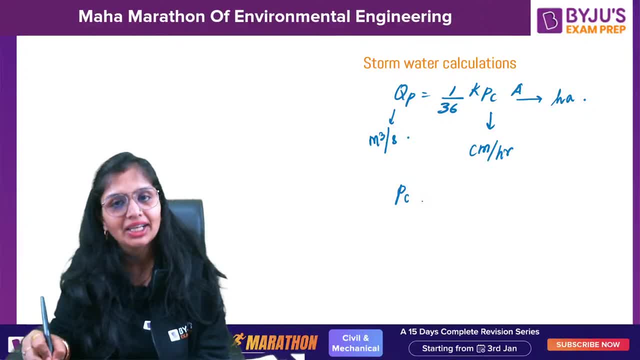 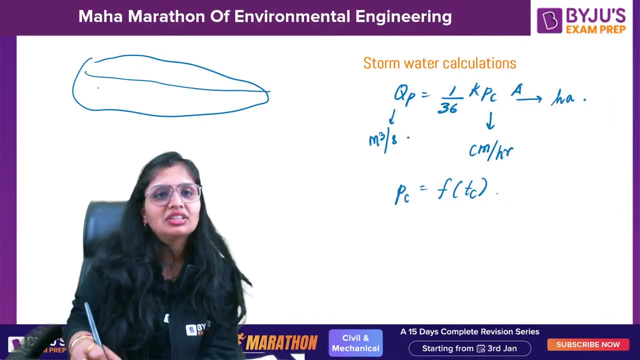 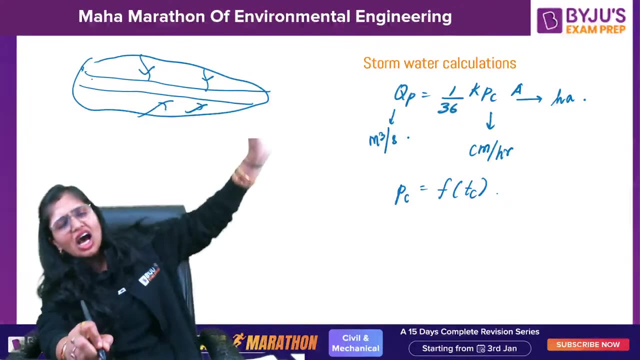 Now critical rainfall intensity will be given to you directly. otherwise it is the function of time of concentration. Now, what is time of concentration? I tell you, if this is the main streams and the water comes from here, water comes from here. So the time taken by the last water molecule droplets, 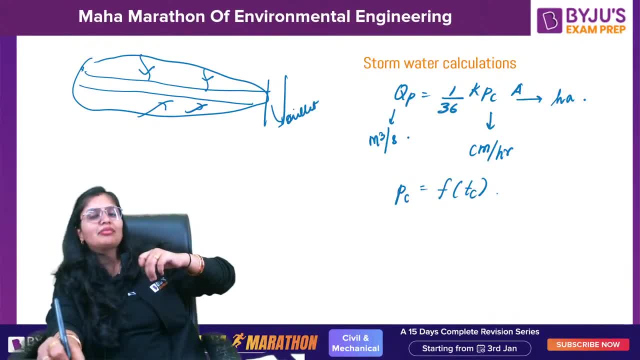 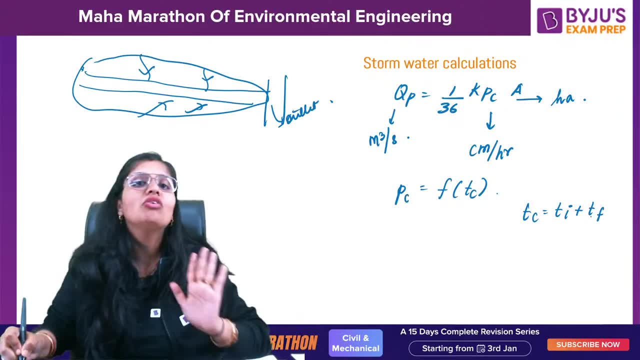 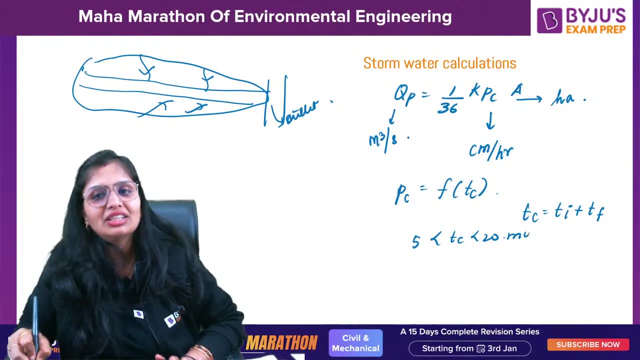 to reach to the outlet. that is known as time of concentration. That is known as time of concentration and that is equal to the time of inlet plus time of flow. Okay, when it is time of concentration is 5 to 20.. Five minutes in this range, 75 tc plus 10.. When the time of concentration is greater than 20, 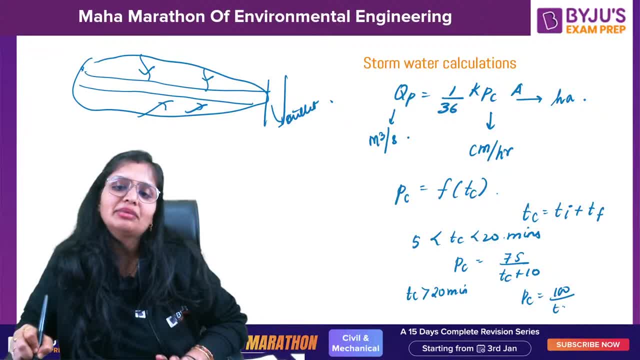 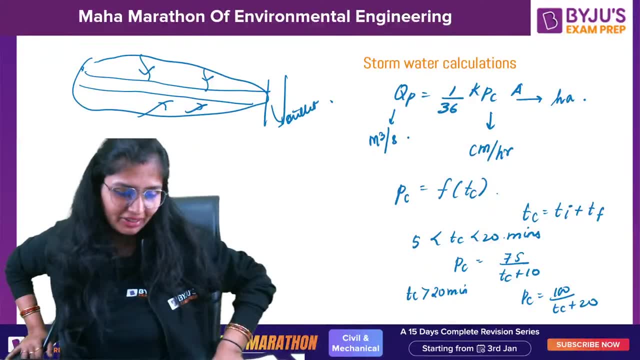 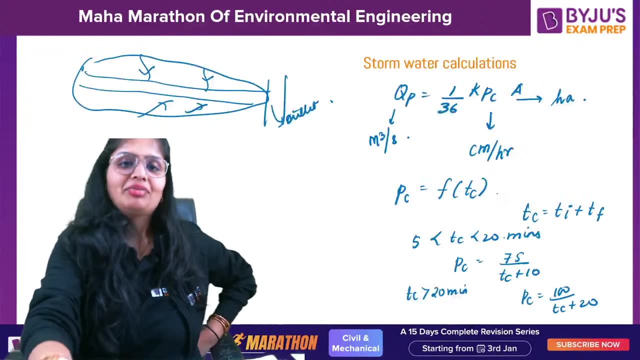 minutes. the critical rainfall intensity is 100 tc plus 20.. So this is the formula Correct, BTech trader, Correct. Okay, so this is the formula which you should know. Now coming next: Okay, fine, This completes your design of sewers. Any doubts, guys? So no logic is there. Whenever you want to, 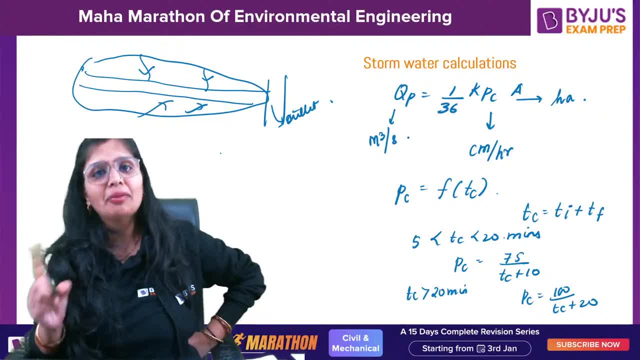 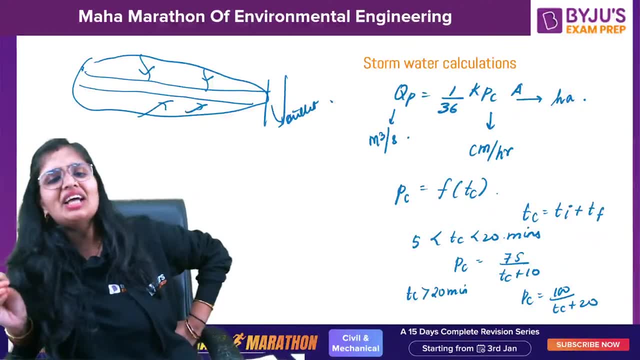 add. simple questions are being asked. If they ask you to design a combined sewer, what you will do? You will add sanitary sewage discharge and you will add this discharge. That's it. Just apply the formula. Yeah, One question which they have asked you, which you should know, which you should. 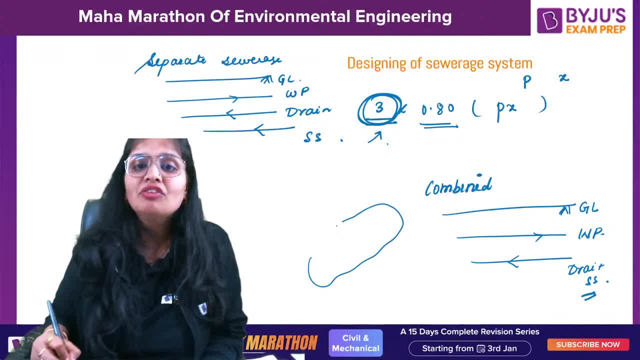 know is very important. Sometimes the value of K is not same, Like this: A1 is the same value of K. K1 area K1 is different. K1 is runoff coefficient. K3 area, A3 area K3 is different. A4 area, K4 is. 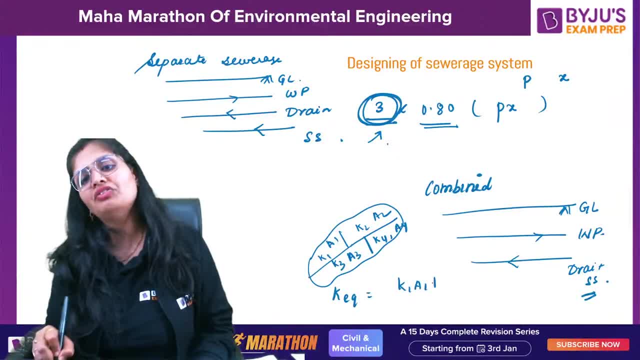 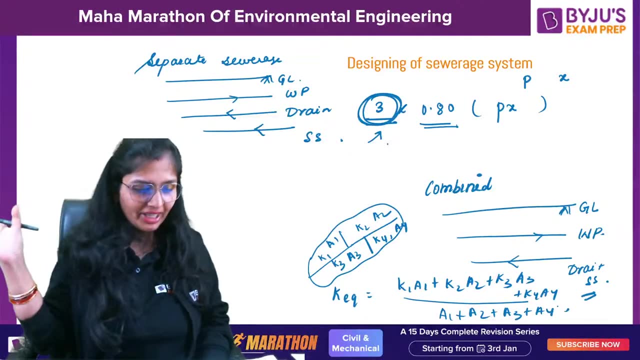 different. In this case you have to calculate equivalent runoff coefficient: K1, A1, K2, A2, K3, A3.. A question has been asked in gate examination. Till now I assume that you might have done PYQs two to three times Weighted average, Correct? 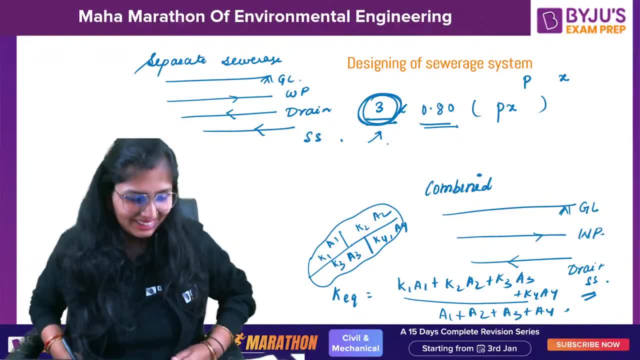 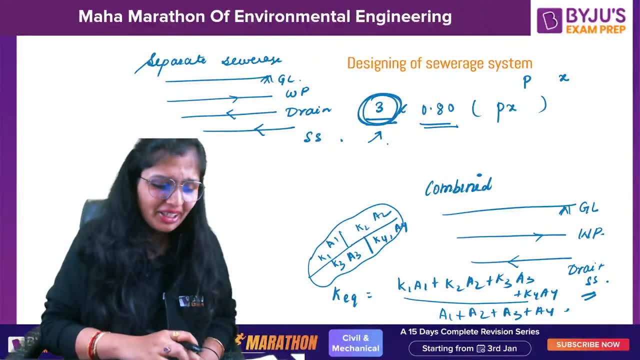 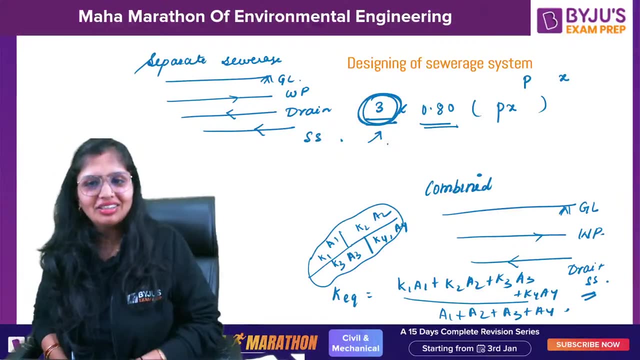 Well, 2.0, I am correct, Designing. Designing is EAC's beta. Why should I tell its numerical now? That is the part of designing. If I tell it now, then it will not come in gate, Do I have? 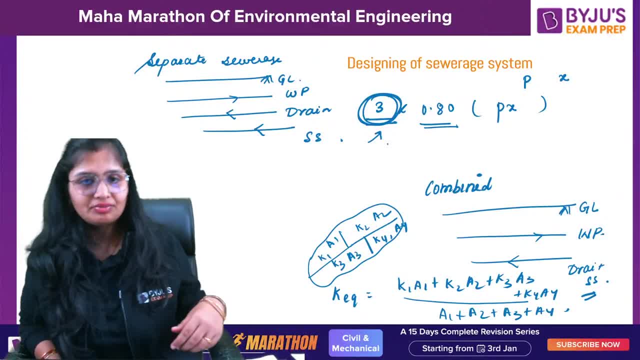 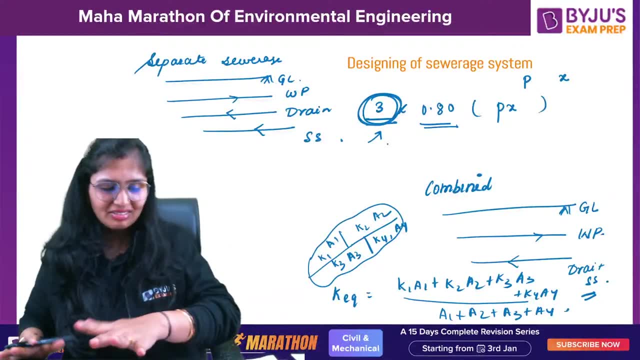 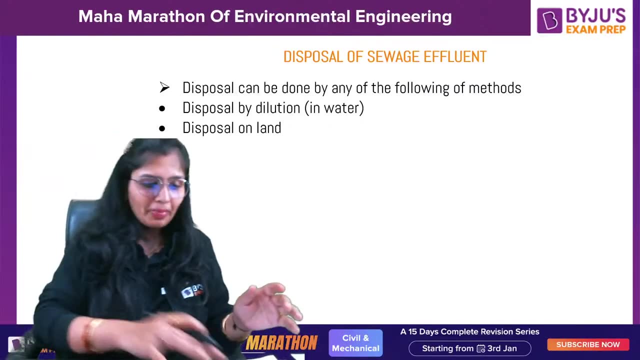 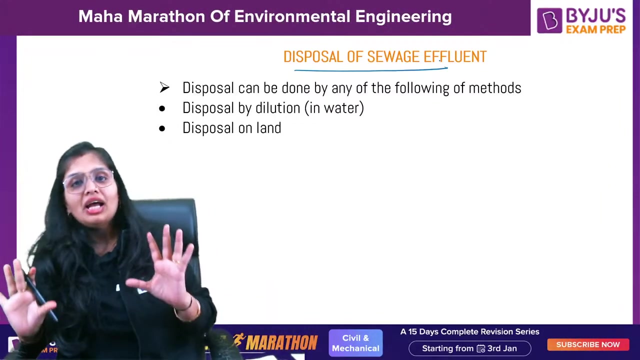 to tell Guys, everybody, Do I have to tell Simple formula based. it is there. That is not asked here. Designing is for EAC, conventional, Okay Now. Now Talking about disposal of sewage effluent, Now Why we are starting disposal before the treatment of sewages. The reason is: 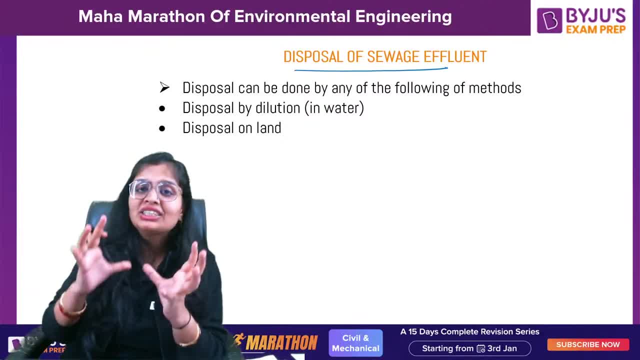 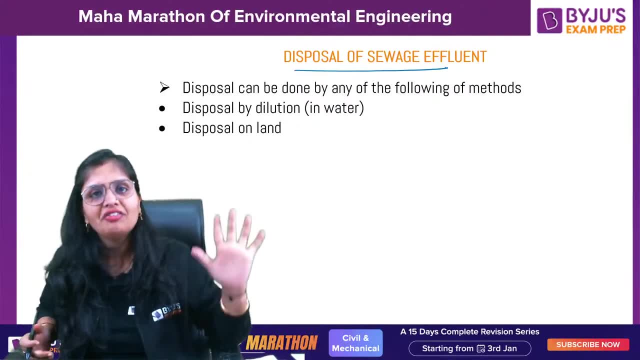 the reason is because how much treatment is to be given, that depends upon disposal. Example: Government has specified for different States, for different union territories. it has been specified: if you are disposing on rivers, what should be the five days BOD. If you are disposing on seas, what should be the 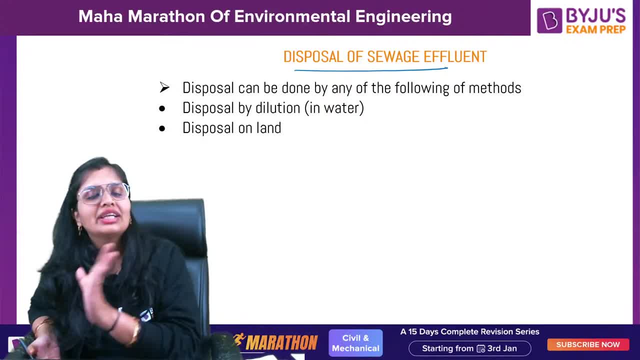 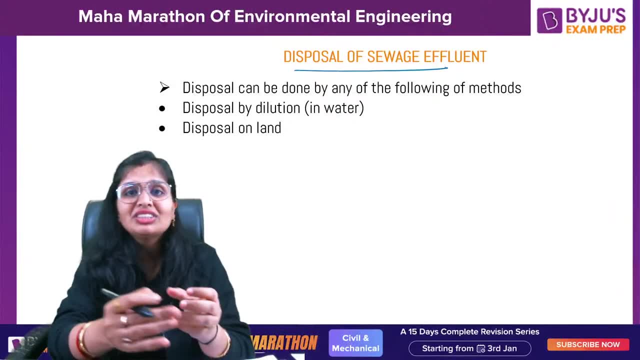 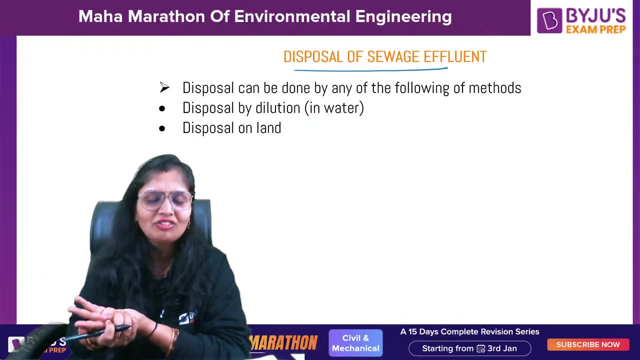 BOD and so on. So disposing when you do it, disposal can be done by two methods: Disposal by dilution, or you dispose it on land. Dilution means when you say the acid is diluted, You might have done it H2SO4. Everybody might have got burnt and all. 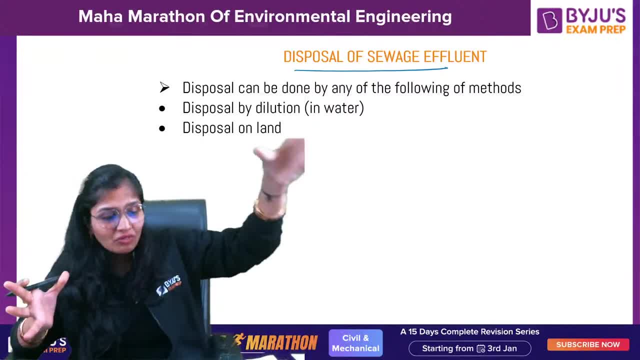 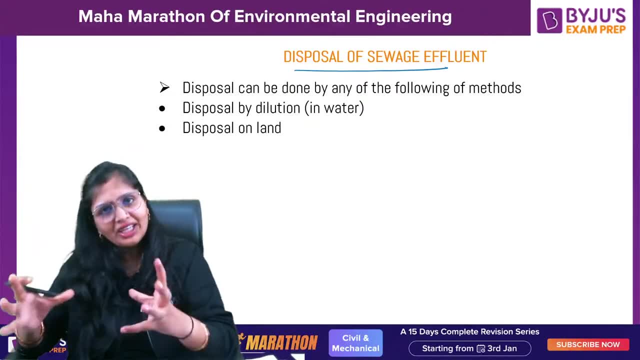 Okay, So what happens? that was concentrated. and if you add water in that? what will happen? if you add water in that, it becomes diluted. Similarly, when you throw the sewage in a place, in that water body which has large volume of water. So what is called? that is known. 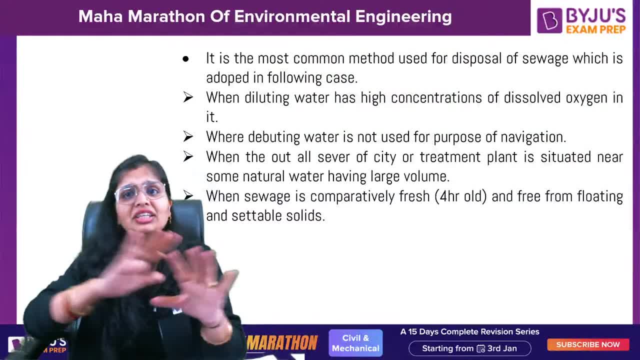 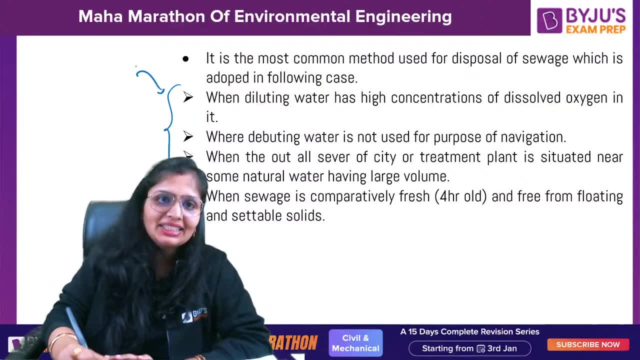 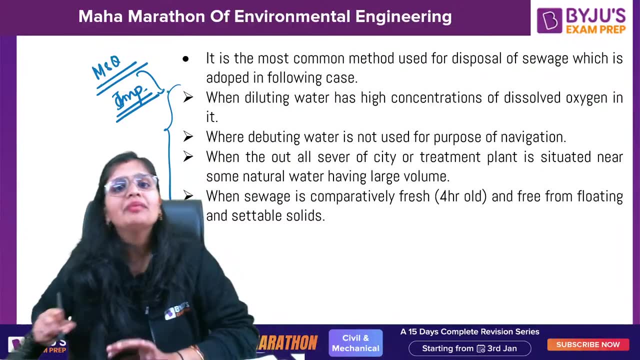 as disposal by dilution. Now, everything is mentioned to you Whenever. these are the important points. This I have written for you In the case it comes in a case. it comes in a case, It comes in an MSQ question, So this you should know. important, Okay, When you are throwing. 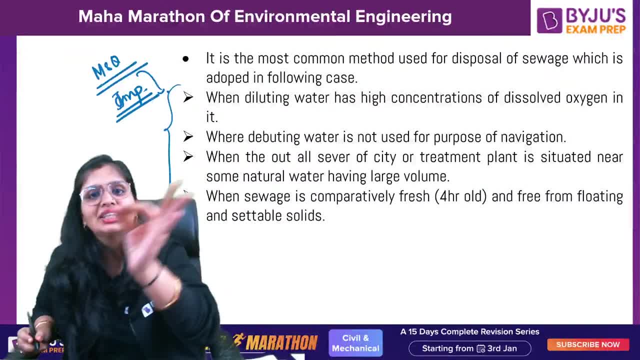 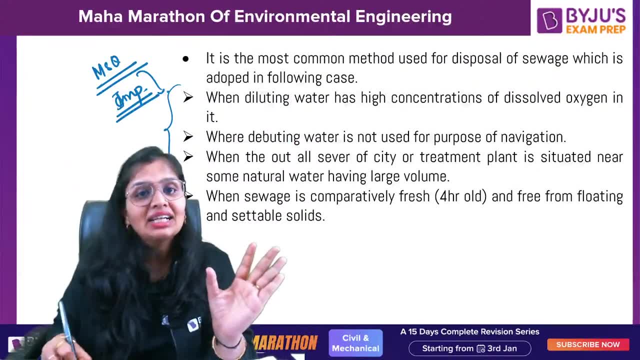 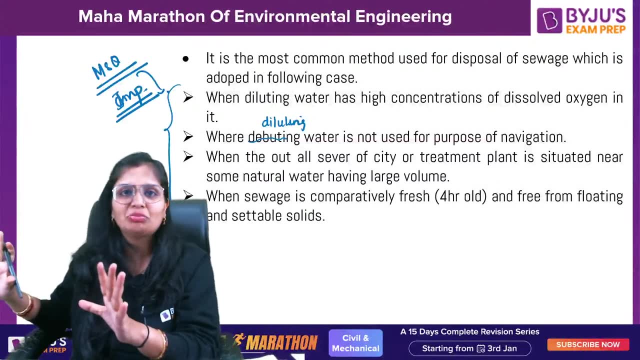 the sewage. When you are throwing the sewage, what will happen? make sure that it has high concentration of dissolved oxygen. Okay, And the diluted that water? where the diluting water, where you are disposing it? it should not be used for navigation purpose, Otherwise it does not look good. 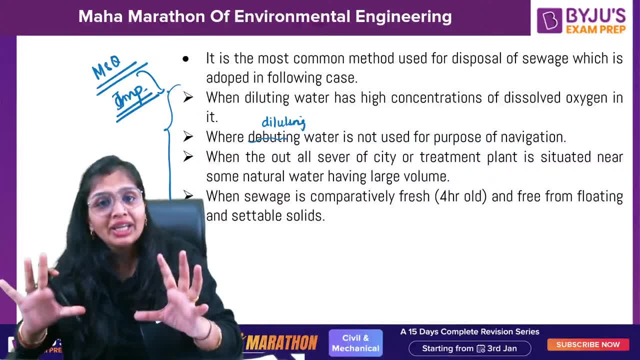 So you should note that. you should also keep in mind. You should keep in mind that you should not use sewage to dilute- Absolutely. it is displeasing, Okay, And when you are throwing it, the sewage should be comparatively fresh. It should not have stale smell and all So. 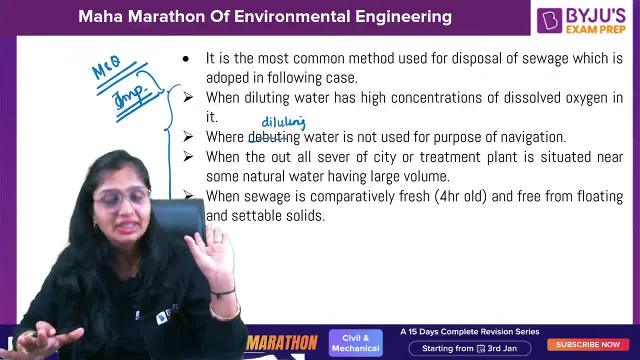 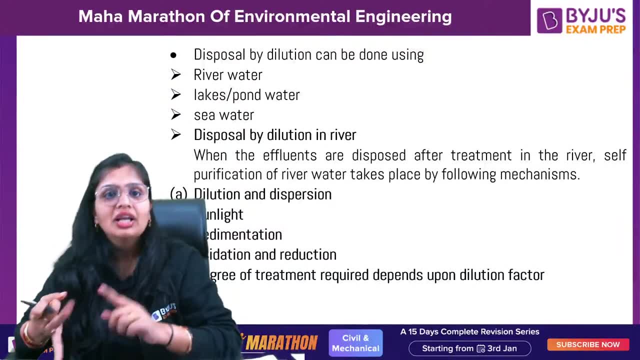 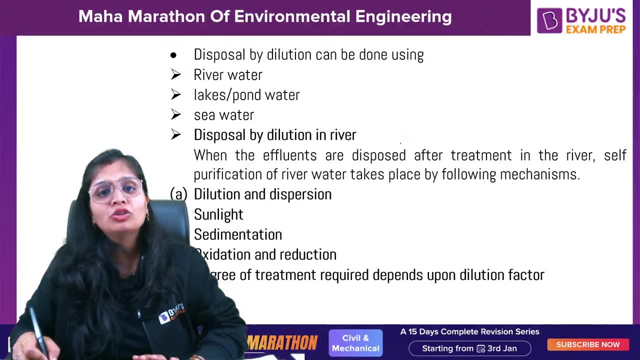 these are the things which you should keep in mind when you are disposing the sewage by dilution. Now comes disposal by dilution. You can do it in reverse lakes, sea water, Now, when you do it, When you do it, disposal by dilution in reverse, Giri, Girib, Jo Bhi. 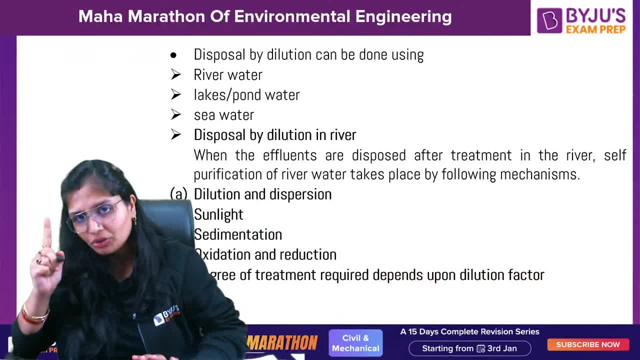 app last time. I am telling you if you are going to do this, first of all, I will block you out and I will make sure by the YouTube authorities that you never, ever be able to download YouTube again. I will just track your IP address right now if you have come. 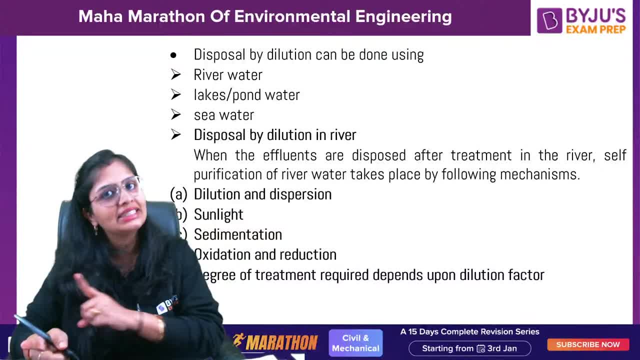 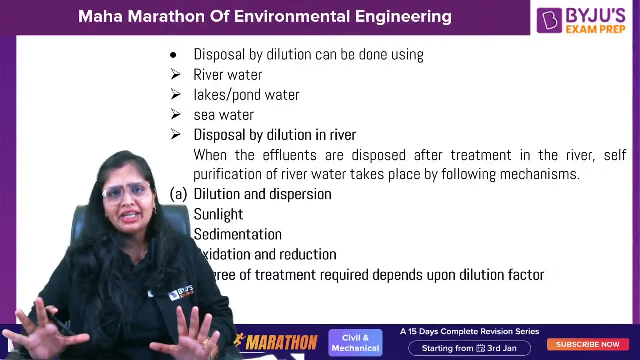 to study, then study, and if you don't want to study, then no one has called you in this channel. don't disturb the other people. this is the last and final warning. if you don't want to study, come on guys. so when you are disposing it, when you dispose by, 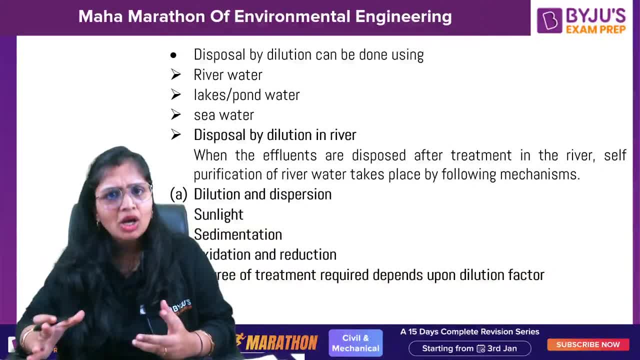 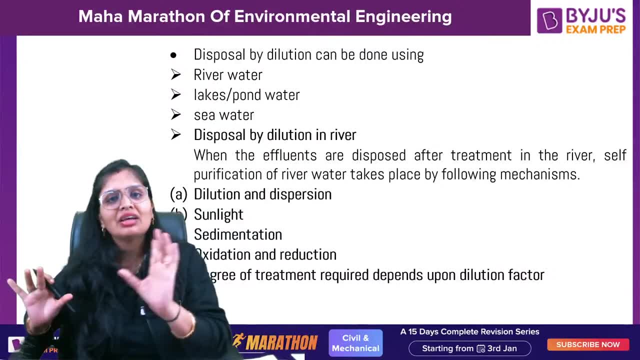 dilution method. that means you are adding water in it. okay, so disposal by dilution is: do what? disposal by dilution when you do it? this is basically for river water. generally, we use it. what happens here? the water purifies itself on its own. that is this self purification. 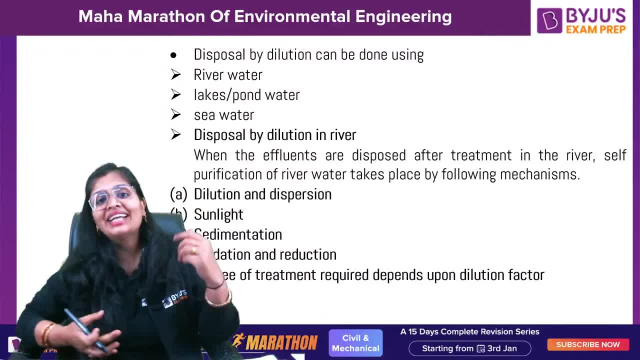 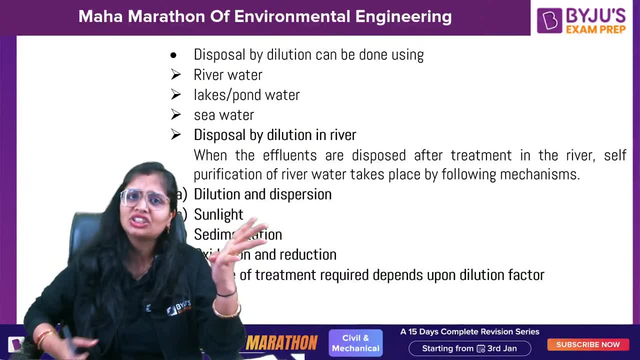 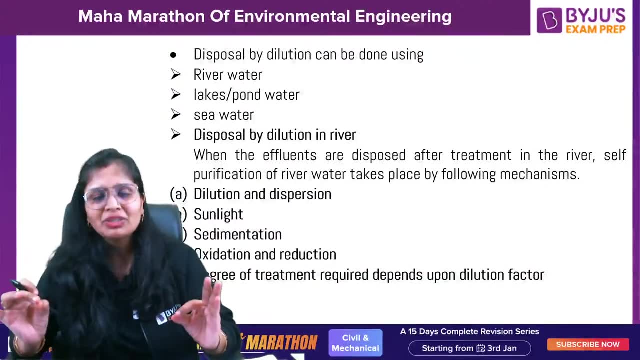 ability of the rivers. so basically it takes place by 4 methods generally: dilution and dispersion, sunlight sedimentation, oxidation and reduction. you can take it in a single or you can separate it and take it out. now what happens? dilution and dispersion are: 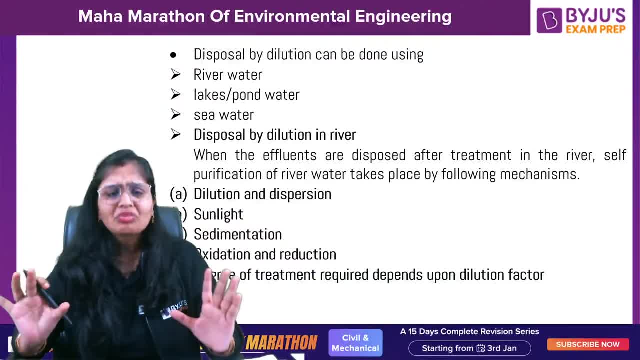 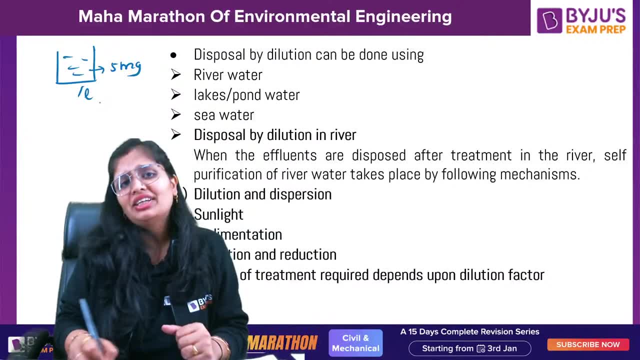 technically, not the method of treatment, what you do technically. when this: if, let us suppose 5 mg of suspended solids was present in 1 liters, you added 9 mg of suspended solids of water, now that 5 mg is present in 10 liters, so here the concentration was 5 mg. 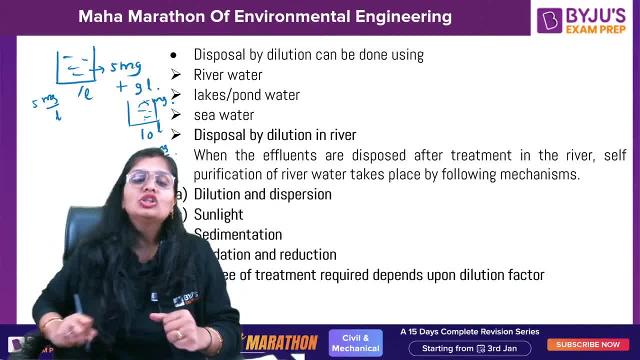 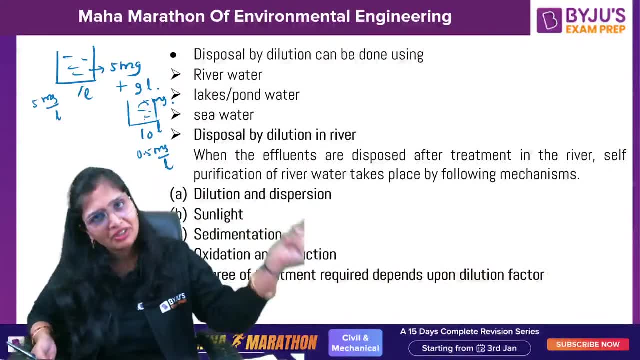 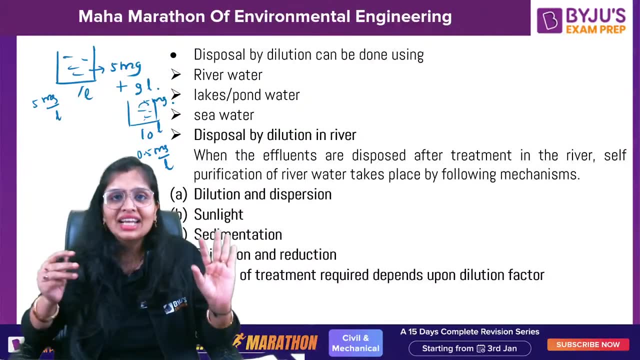 per liter. here the concentration is 0.5 mg per liter. so what is happening? what is happening here? the concentration is reduced. that's it, the suspended solids. previously also it was 5 mg, now also it is 5 mg. so that is dilution. sunlight, when sunlight comes, you. 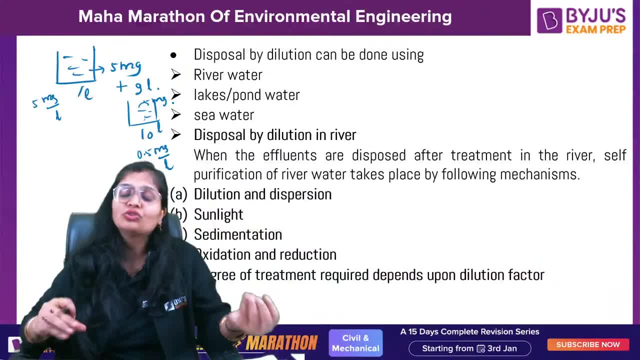 know, algae will prepare its food. when algae prepare its food, oxygen will prepare its food. oxygen is liberated. that oxygen is used by microorganisms for carrying out the decomposition. so in that manner, organic matter, who were asking the nitrogenous and all they will. 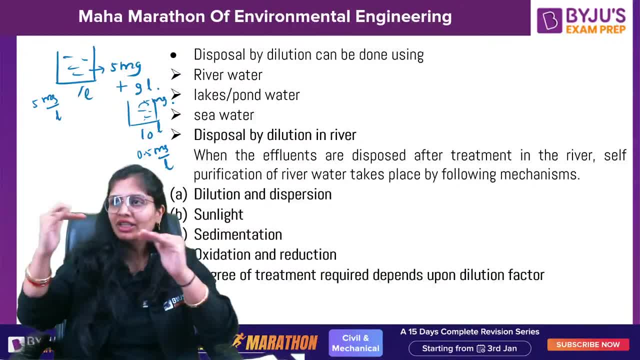 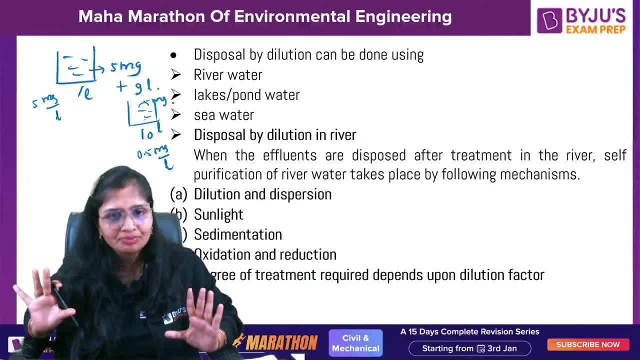 be getting removed now. sedimentation water is flowing. the turbulence is not 0, but it is flowing, so whatsoever. particles which have a higher weight, they will settle down. oxidation and reduction, chemical processes: these 3 are the physical forces. 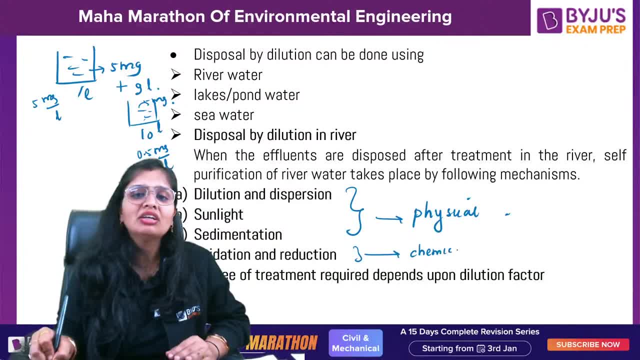 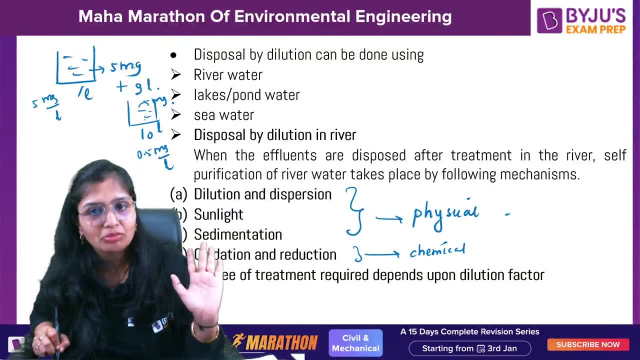 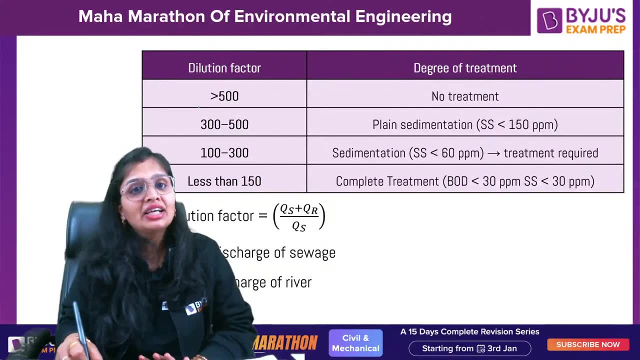 and this oxidation and reduction is the chemical forces with the help which what is happening, the biodegradable or any organic matter is getting removed. Now, degree of treatment depends upon dilution factor. let me tell you one thing, important dilution factor: if it is greater than 500, no treatment. 300 to 5 treatment do plane. 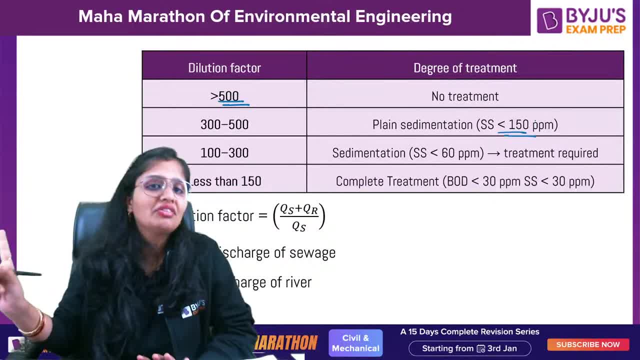 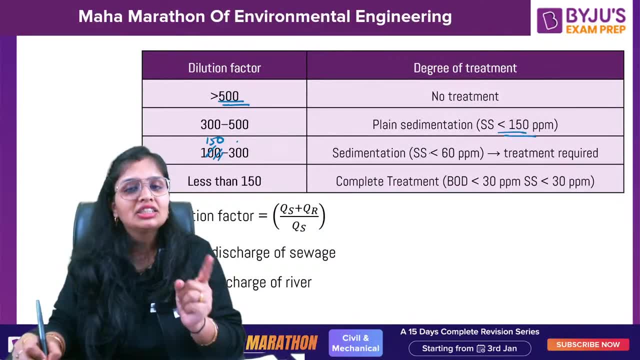 sedimentation. make sure that the suspended solids is less than 150 bpm, then about 150 to 300.. Let's see. okay, sediment suspended solid should be less than 60 ppm and treatment is required. if the dilution factor is less than 150 ppm. you need to do complete treatment such that 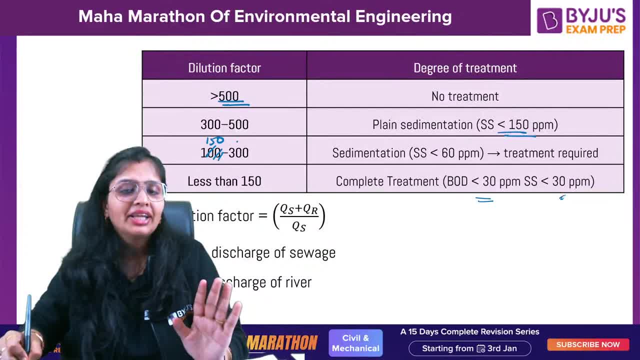 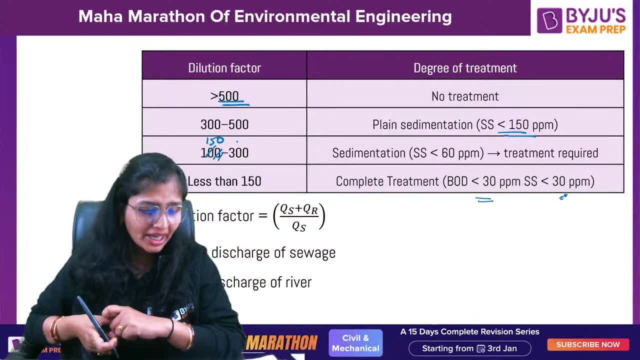 the BOD is less than 30 ppm. this is wrong. can you tell me what is the correct one? this, this data written is wrong. the date: ma'am, if depth of river is more, how sunlight will reach to algae first of all? yeah, a BTEC trader, some algae. algae are not rooted plants, so 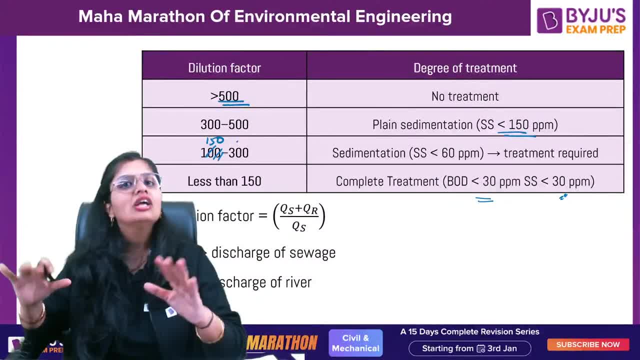 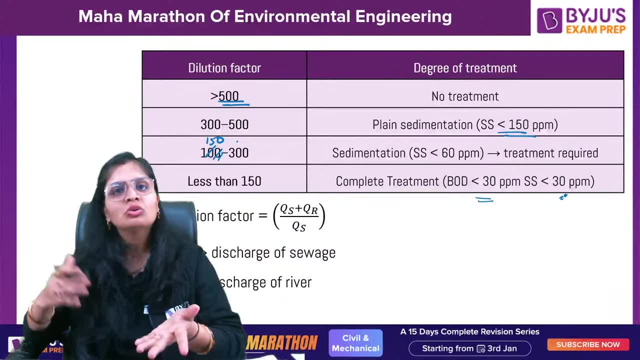 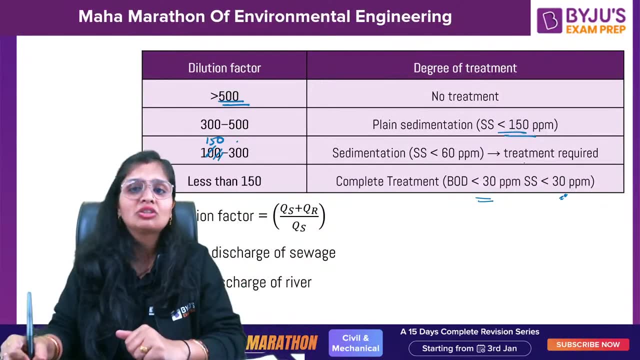 they are present on the beds also. they are present deep inside, so that portion, till where sunlight is able to receive by the algae, they'll prepare the food. those who are not, basically the sunlight cannot penetrate, they won't be able to do it. okay, as simple as that. this is wrong, can? 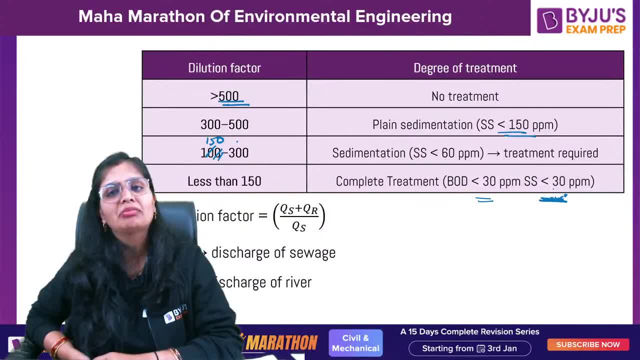 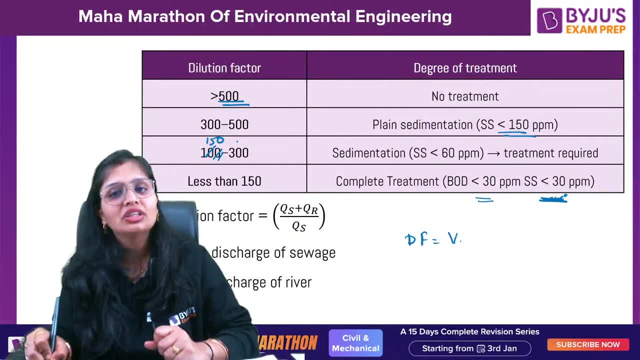 anybody tell me one of this is 20 ppm. which one is 20 ppm? guys tell me fast, okay. next, one more thing which I'll tell you: dilution factor. you will say, ma'am, you told us dilution factor is volume of sewage plus volume of water divided by volume of sewage. right now you are. 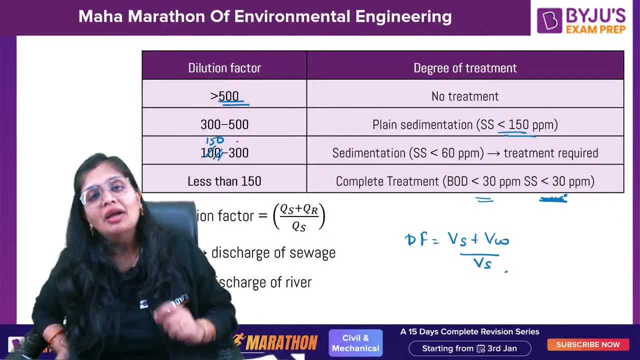 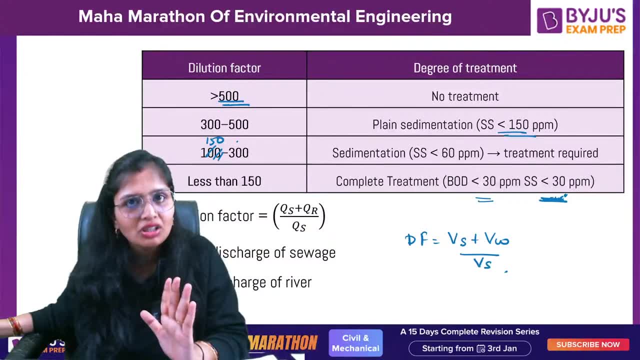 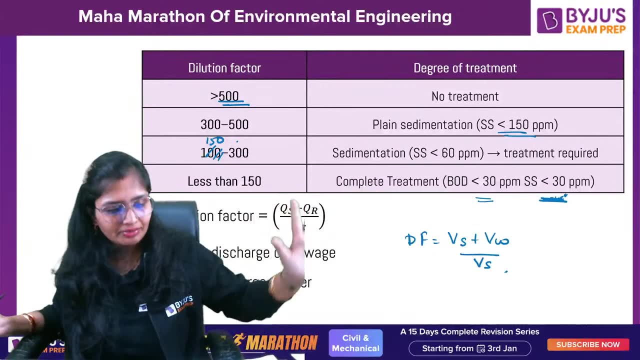 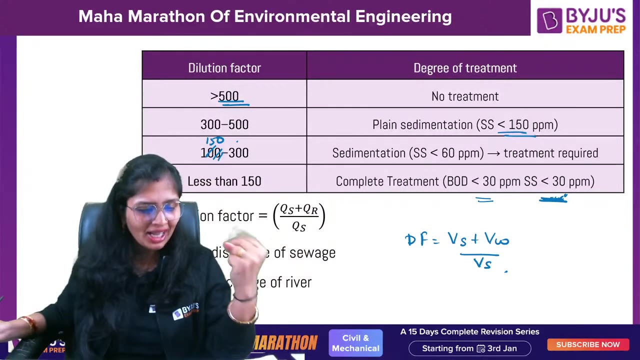 writing. discharge of sewage, discharge of river. why? because practically beta. it is not possible to measure the volume of river. can you measure the volume of river? so in that case you measure volume per unit time. okay, any doubts till here? very good, two people answered differently: suspended solids 30, BOD 20 and tixier told: suspended. 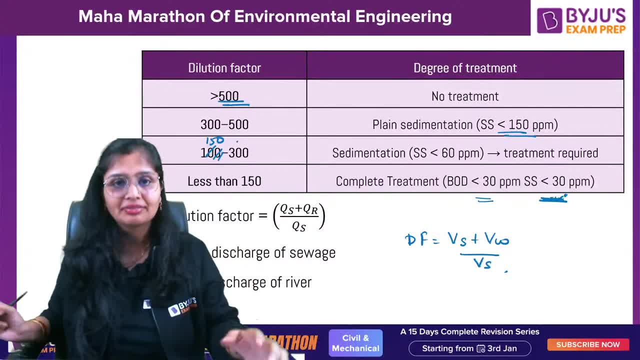 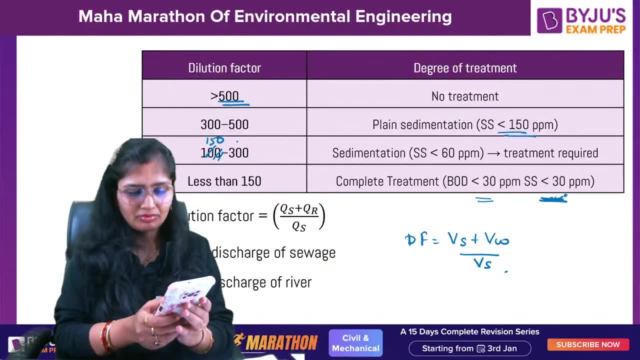 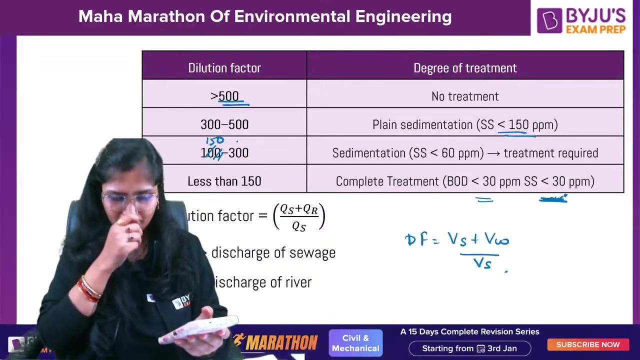 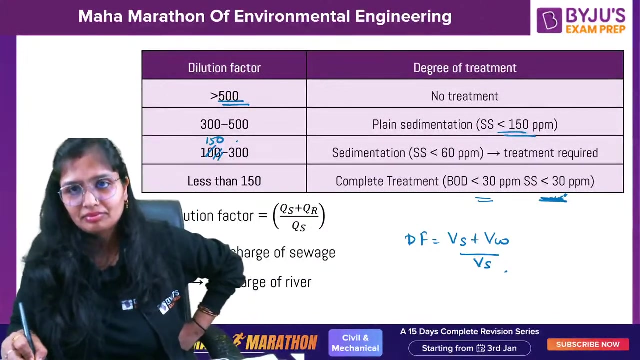 solids 20. which one is correct? come on, Girish Arun, everybody fast. okay, Just carry on. Thanks, Shri, I know it very well. if I think of such part, I feel I'll go for Idli. so it creates the original. so will you make me look healthy? 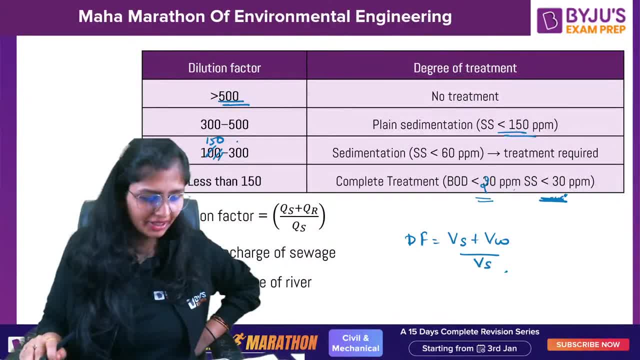 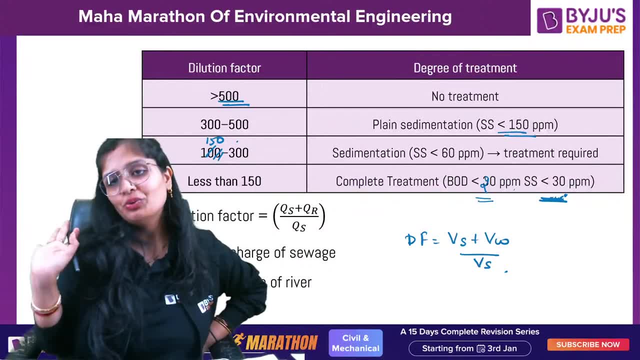 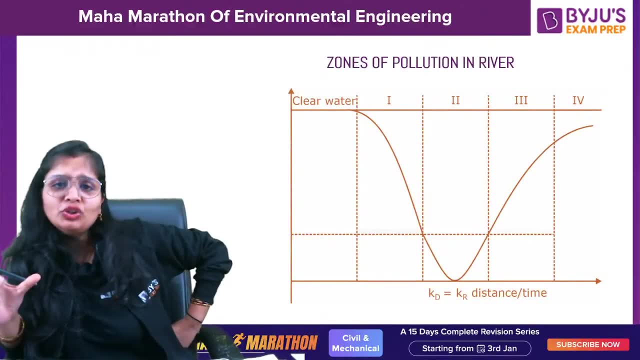 let's go. let me take ahtaking. please, two more. he is really, think me, you know, male. yes, not, yes, do not get so your basic spend also right, absolutely, Let's do it quickly. Zones of pollution: We have four zones: Zone of degradation, active decomposition. zone of recovery. zone of clear water. 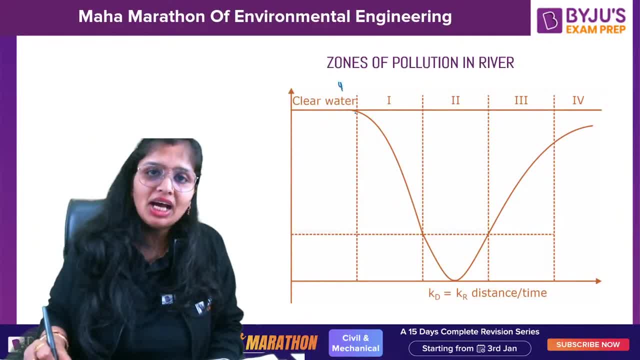 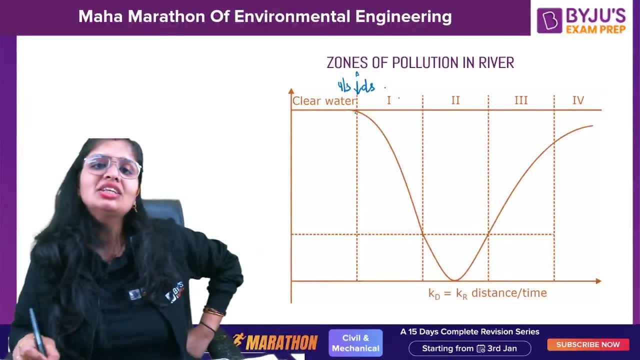 Initially the water was clear. The moment you see, this is the upstream, This is the downstream side. So here you will do what when you dispose the sewage, what you will see it: This is the zone of degradation. What you will see it in the zone of degradation, Initially fishes and algae. will there? Some amount of algae will die here. 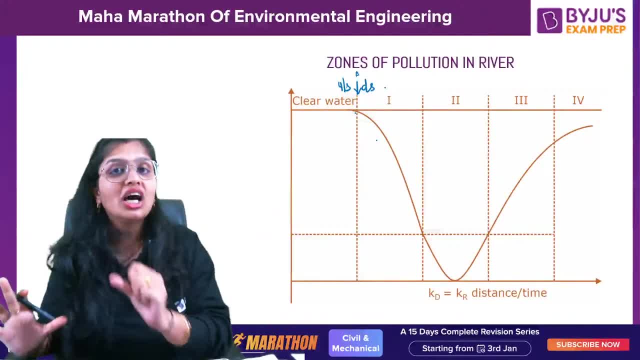 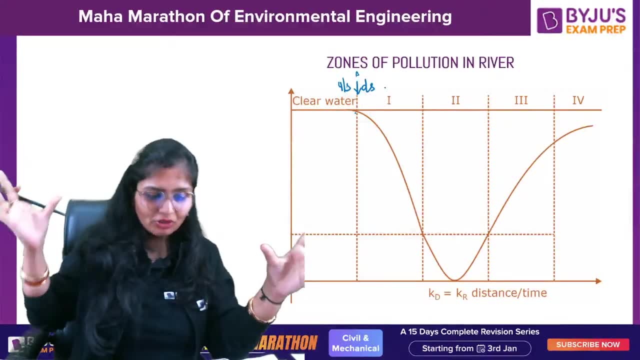 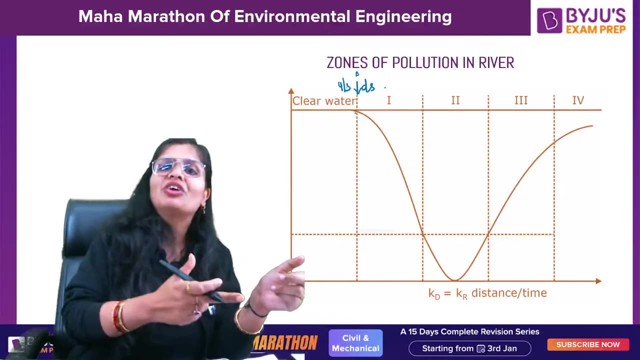 OK. Now when you throw the sewage, it has a large amount of organic matter. So when you will throw this, organic matter is there, By default, microorganisms will be there. You know that song. So wherever organic matter will go, microorganisms will follow it. 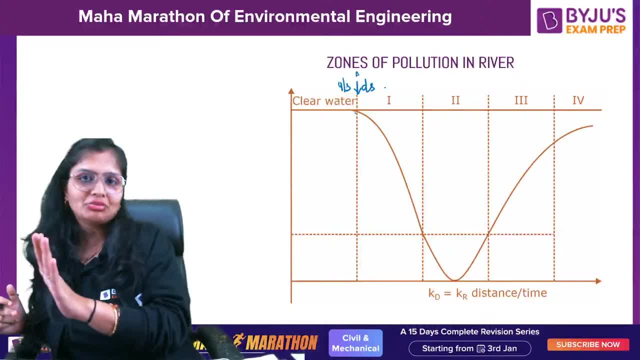 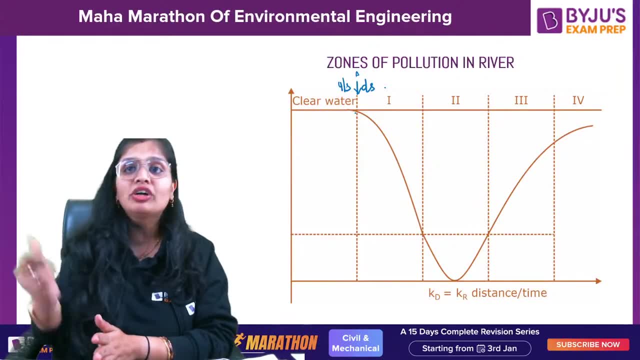 So wherever organic matter will go, their microorganisms will go. So what is happening is what is happening is here, The moment you throw it, eventually microorganisms will start to Utilize the dissolved oxygen of the river. So the dissolved oxygen value decreases, decreases. 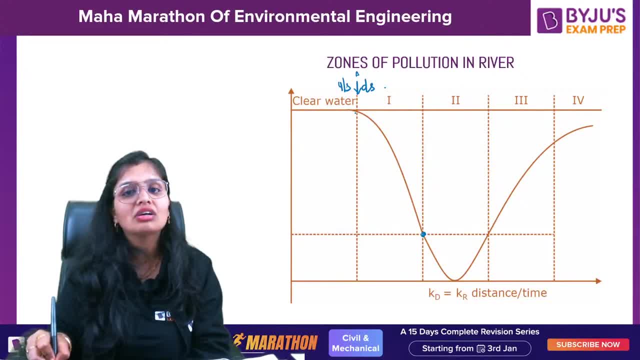 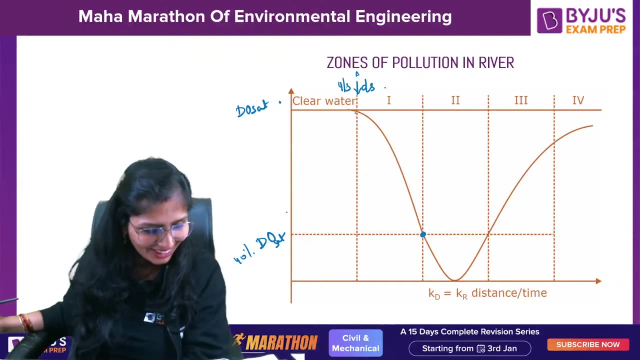 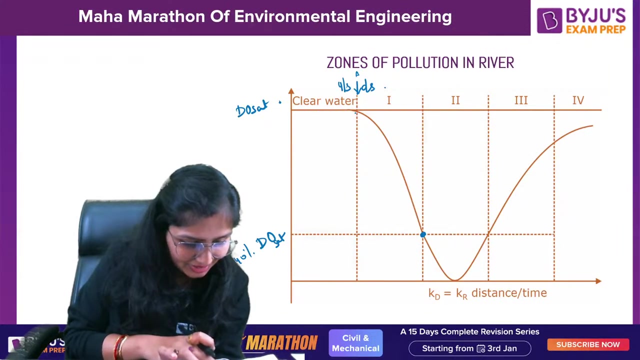 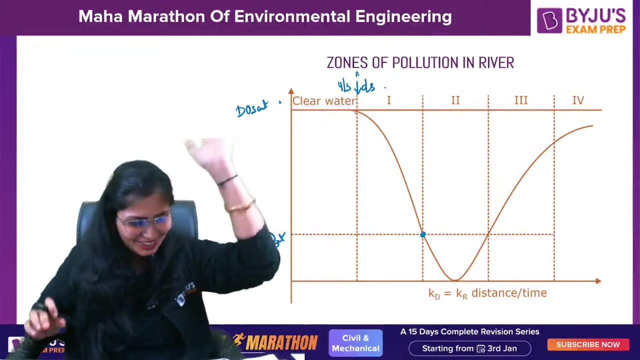 And during this process the zone of Degradation ends. when this was deosaturated, This becomes Deo 40 percent of deosaturated. So this will add When we gonna Deo To the home. That is also correct. 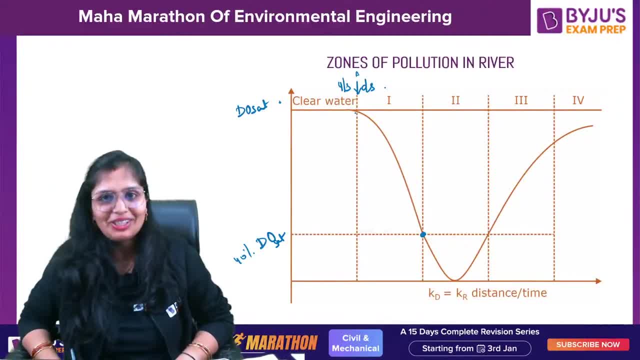 So wherever is organic matter, there, ever microorganisms will come. OK, Now talking about zone of active decomposition. This is also known as by the name of the zone of heavy pollution. What will happen? The deo level may even fall to zero. 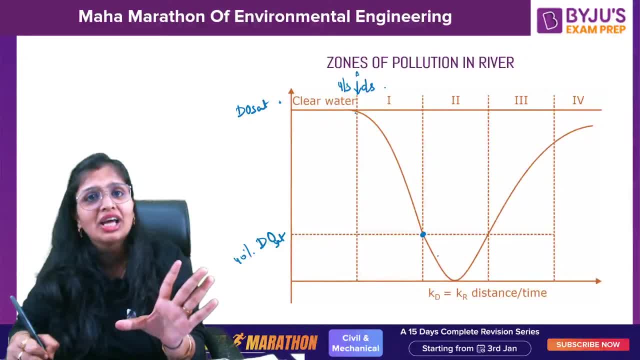 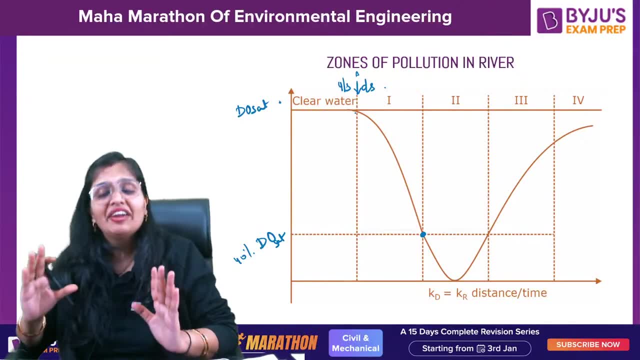 Dark and turbid water Fishes will also die. OK, Eventually, every maximum amount of fishes will die. the water will become dark. Eventually, slowly and slowly, this will lift Again. this is this zone ends 40% of DO saturated. Okay, this will lead to the zone. 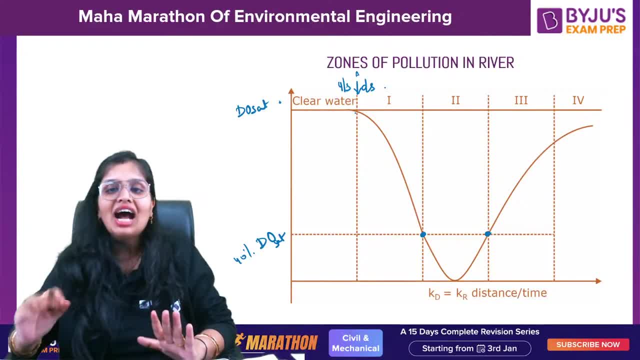 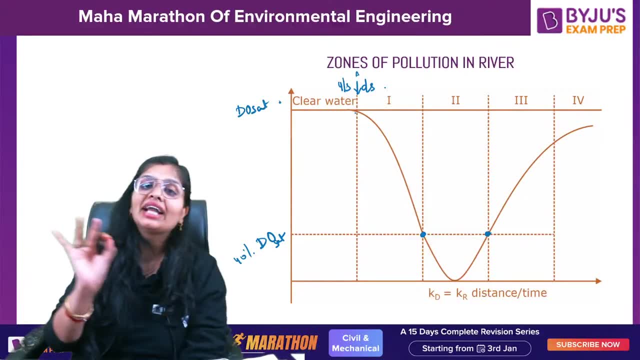 of zone of active decomposition After that zone of recovery. now maximum decomposition has taken place. Now the water is becoming clearer. But remember, at no point in zone of recovery the DO level becomes equal to DO saturated. it will be less than DO saturated. And on the fourth, 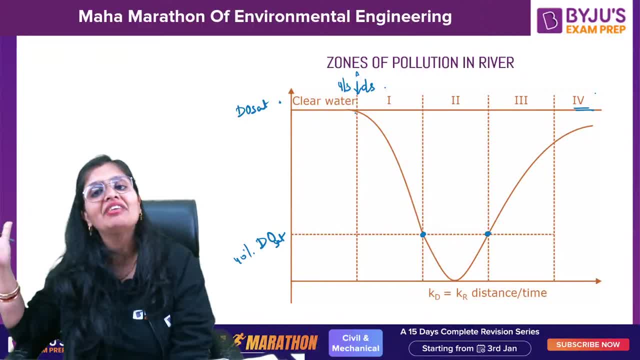 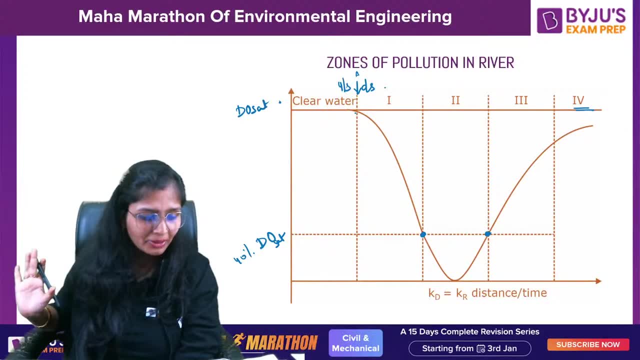 zone, zone of clear water, fishes, algae, all will be alive and it will reach to DO saturated. So this is the whole thing. An aerobic respiration will happen. Of course it will happen. So generally you guys would have ever seen in the river, certain place you get the black portion. 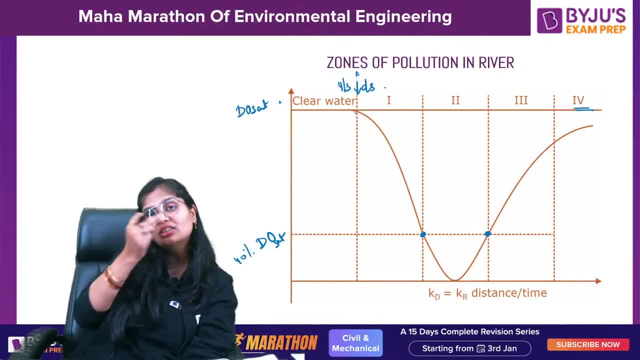 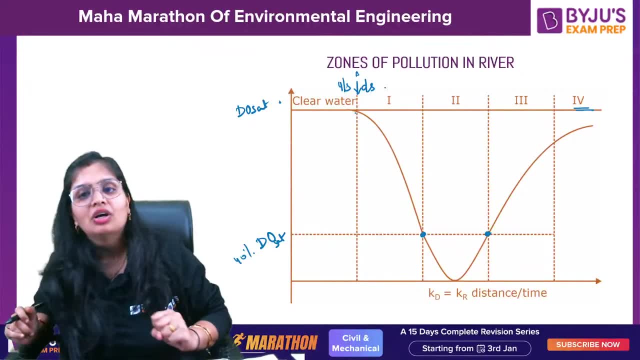 you just see it Generally, you would have noticed. So that is the zone of active decomposition. It becomes like black and turbid. That is zone of active decomposition. Okay, Now this is mentioned for you for the theory purpose. You guys can check it. 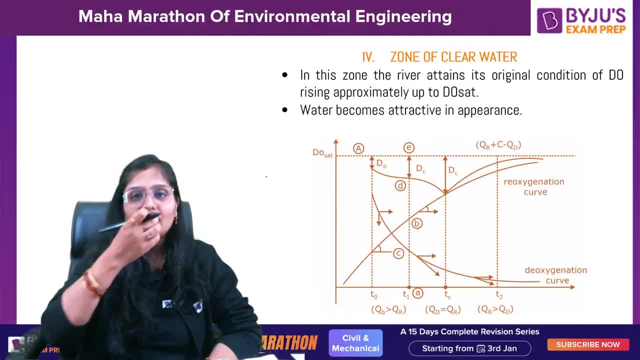 out. This is for your theory purpose. Okay, Now, like you told me, Now, at sites of river in the between also. you see it, Vamsi? Yeah, Now what happens? Like I told you? you see it, Vamsi, You. 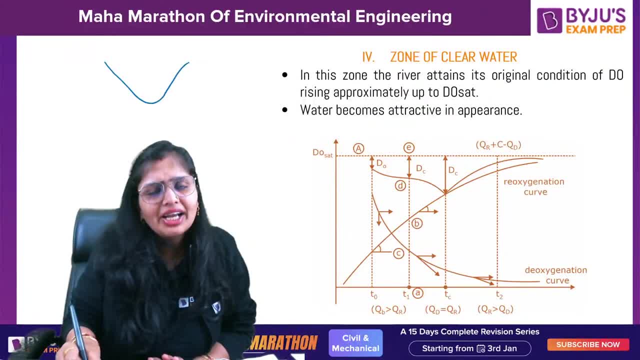 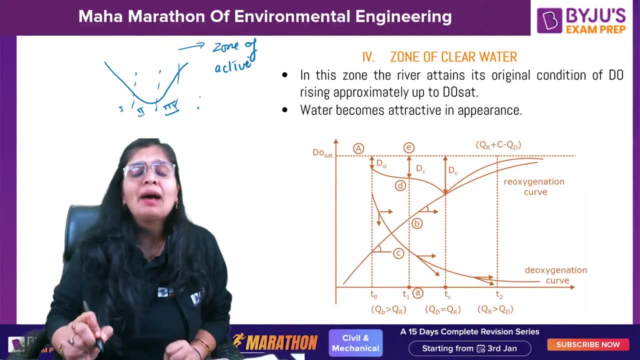 do you? In this portion it becomes like this. It writes: So technically it is divided into three zones. how, that zone of active decomposition in itself divided into three zones? How? firstly, second, third, What happens is? what happens is, you know, KR and KD. two things are there. KR is rate. 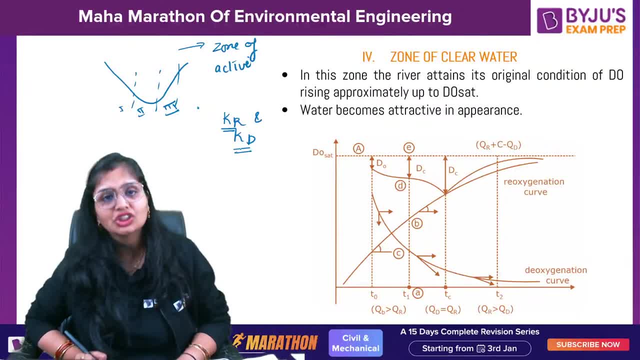 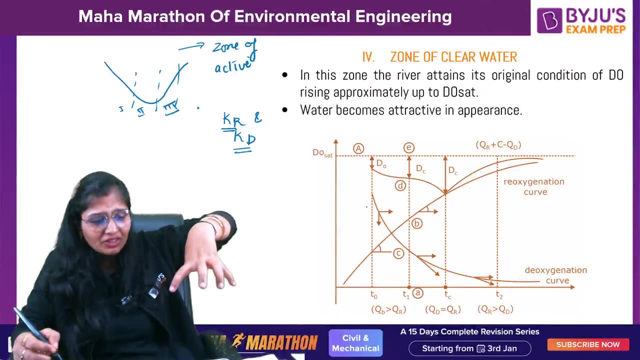 of re oxygenation, KD is rate of deoxygenation. What happens is, When you talk about the oxygenation, kr, rate of reoxygenation, both are going at some point. reoxygenation is more, at some point, deoxygenation is more. you know initially, when you dump the sewage, what you will see, what you will. 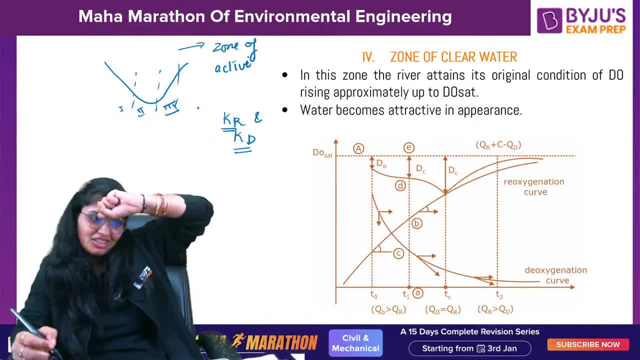 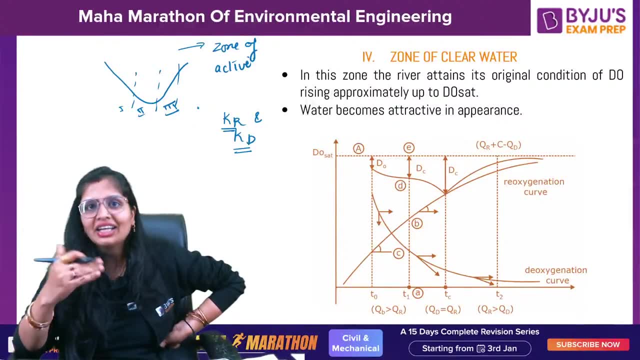 see, ma'am, ganga kabhi ganda nahi hota. yeh sach hai kya then? if it doesn't have, then why do we have ganga plan and all for see, ganda nahi hota. par ganda hum karte hai theke, vo toh nahi hota river. 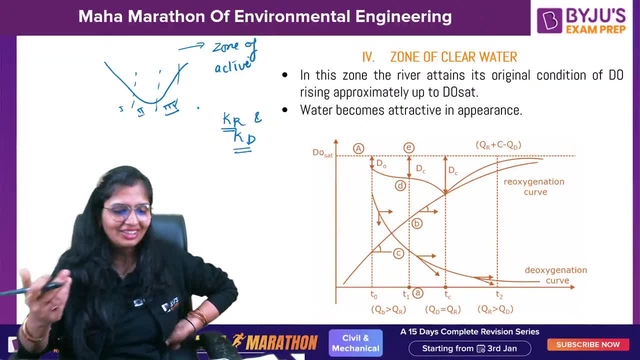 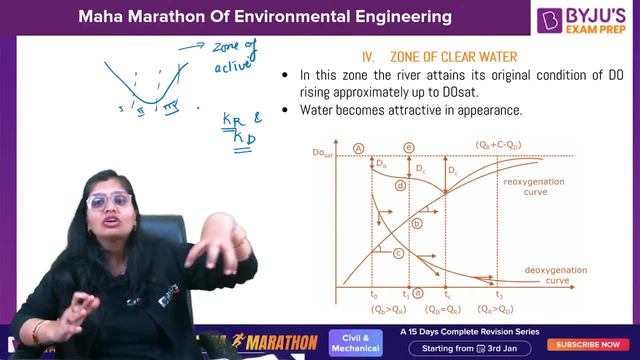 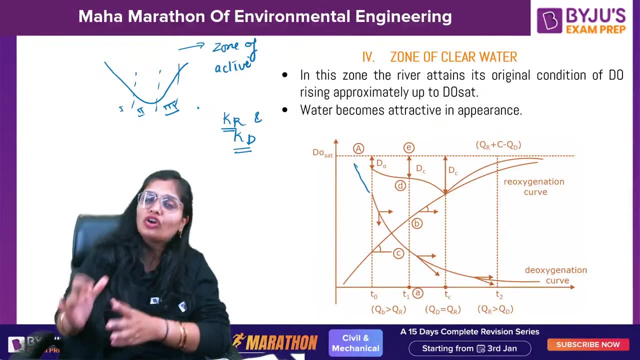 kabhi khudse ganda hoti ho, toh hum karte hai. nah. ok now, initially, when you dump the sewage, deoxygenation rate constant is more. so you can see the deoxygenation curve is more eventually, over the time when maximum demand of oxygen is satisfied by the microorganisms. 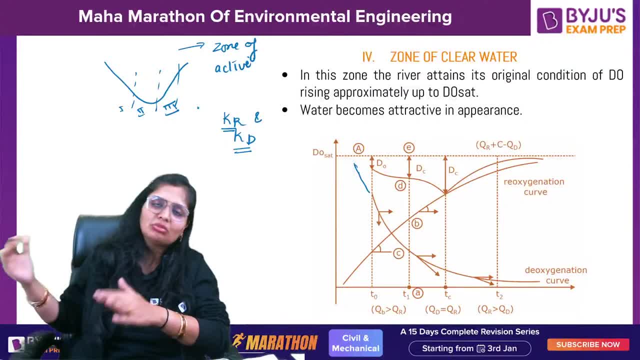 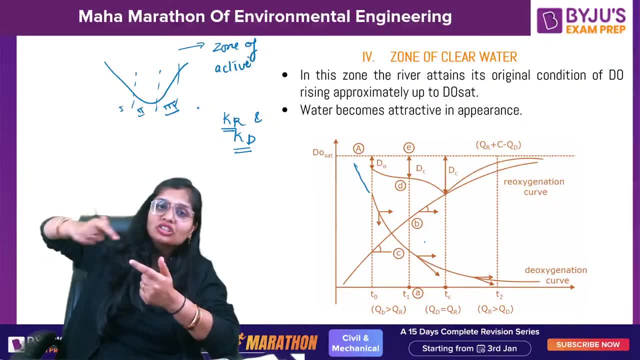 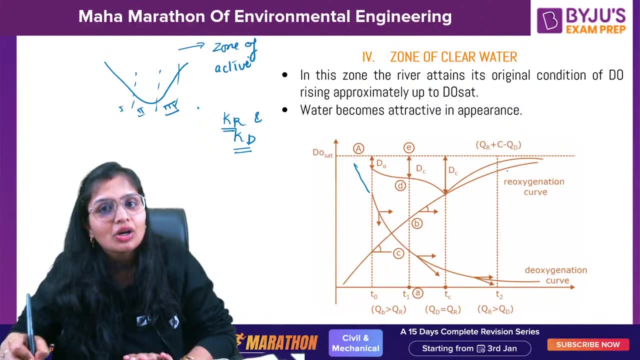 ok, they have been. they have utilized the oxygen. maximum decomposition of organic matter has taken place. this deoxygenation reduces and the rate at maximum decomposition of organic matter has taken place and the rate at which the deoxygenation of which the oxygen enters into the water. it is saved, but the rate is increasing. Okay, so when? 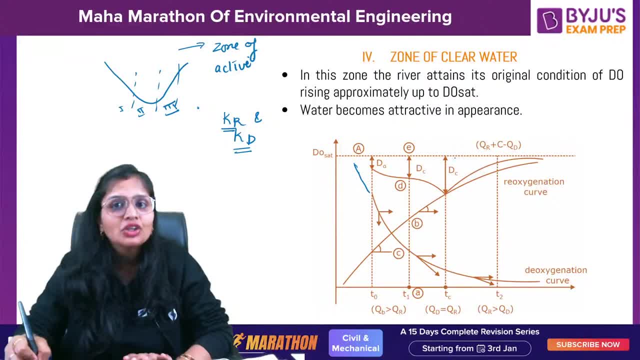 you take the summation of it, you will see here, you will see it here. this will come out to be DC. This DC is critical DO deficit and the time is critical time. Okay, now, at any time now, this is a very special formula which you guys need to know because in gate examination also they have. 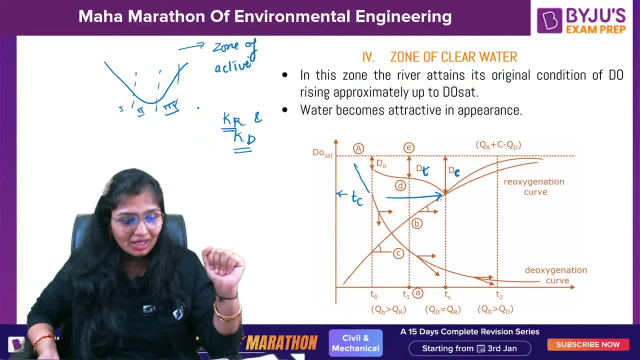 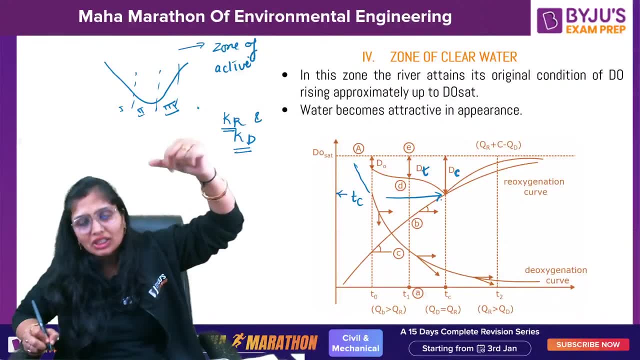 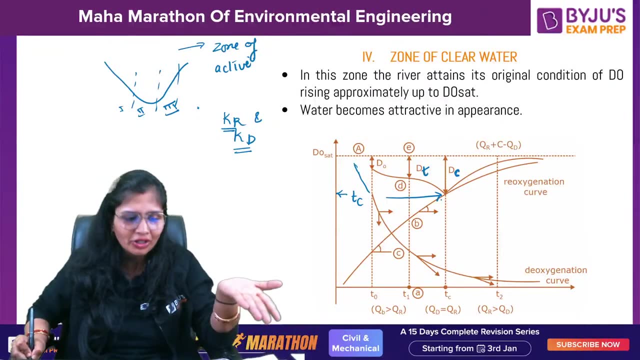 asked you. Okay, now DO is the initial DO deficit. When you dump the sewage, there will be certain deficit in the dissolved oxygen. Why? Because organic matter is there. If organic matter is there, who said na Kishal said tum jahan, main wahan. So when organic matter is there, 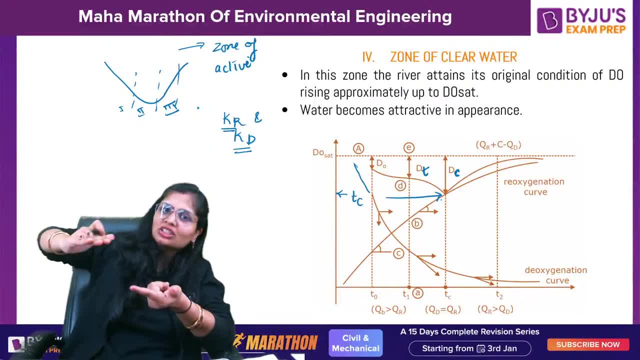 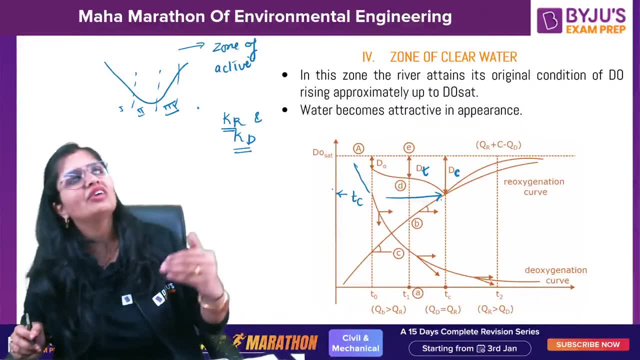 microorganisms will come. If microorganisms will come, oxygen will reduce. If oxygen will reduce, deficiency will come. Okay, so now I want to calculate. let us suppose I want to calculate the deficiency of dissolved oxygen after 5 days, after 10 days. So you have a formula. 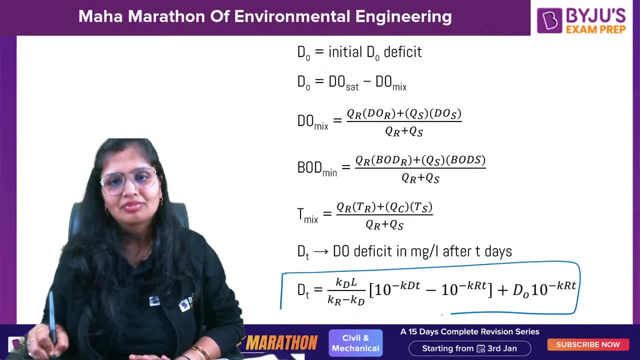 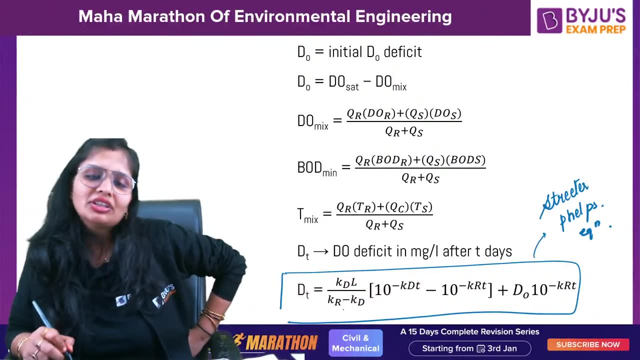 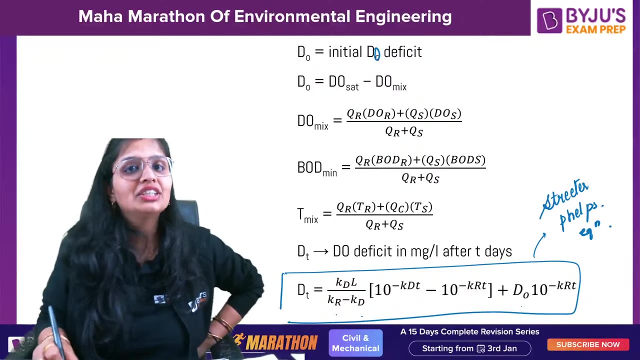 your favorite formula: Streeter-Pelf's equation. This is the formula Streeter-Pelf's equation. formula is there. Kd Kr is the deoxygenation reoxygenation rate constant. deoxygenation rate constant d naught is initial DO deficient, which is equal to DO saturated minus. 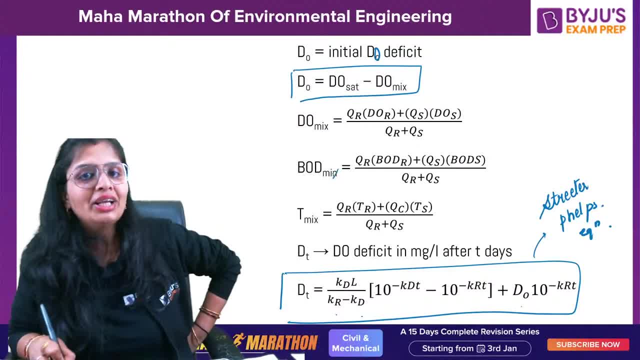 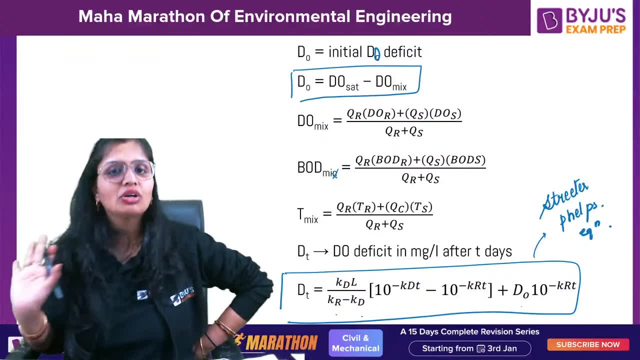 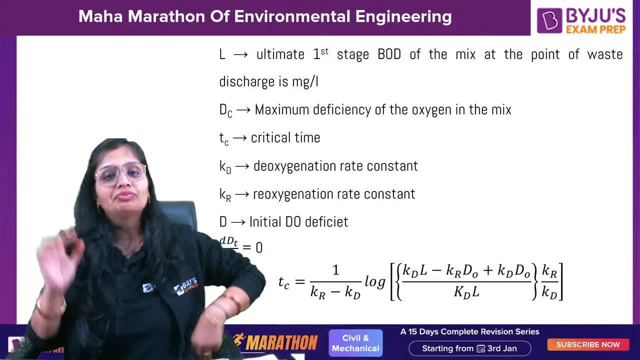 DO mix. okay, and DO mix is the DO of river discharge, of river discharge of seaway, dissolved oxygen of seaway. don't worry, I will do a portion also with it. so this is the formula. you have to remember it. I can't do it solve three, four portions. you will get it out now. next is the. 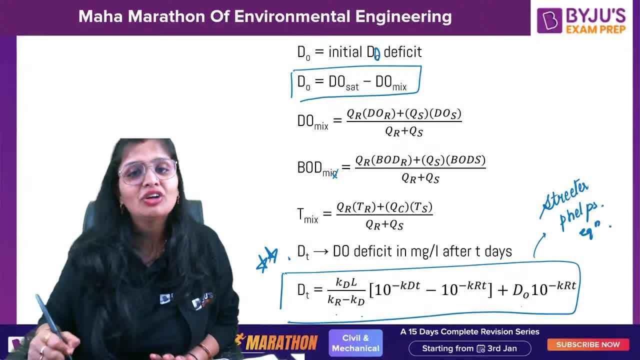 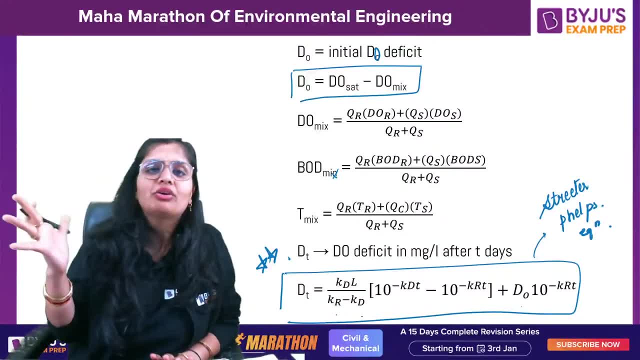 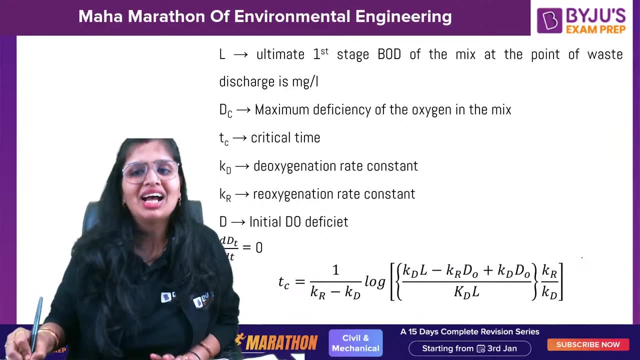 critical time. and remember: L here is not the length. many students get confused. L is the ultimate first stage BOD. as I told you, we are not bothered about nitrogenous BOD, we are bothered about the first stage BOD. okay, now TC. this is a difficult formula. I will advise you not to. 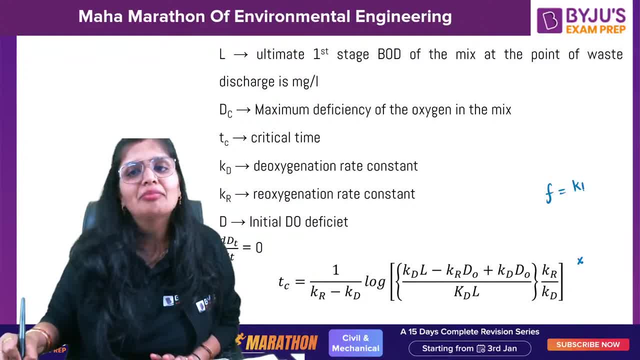 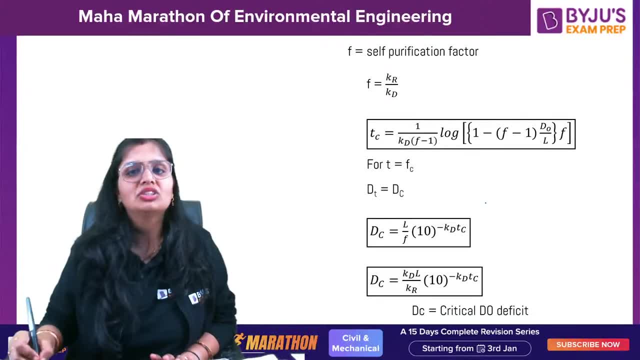 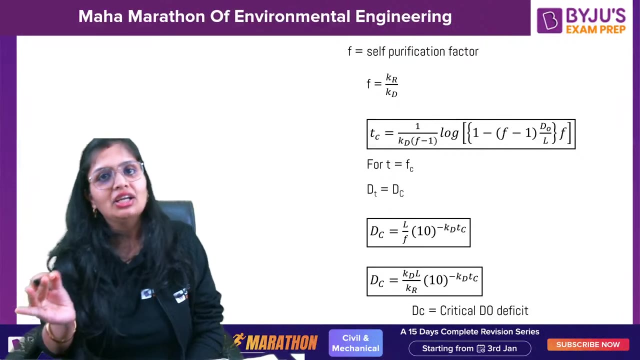 remember this okay. F is equal to KR by KD. this is a purification constant, self-purification constant. don't remember this formula. instead, remember this formula. okay, try to remember this formula now. when the time becomes equals to critical time, the deficiency becomes equal to critical DO deficiency. or you can say critical DO- deficient. so this is: 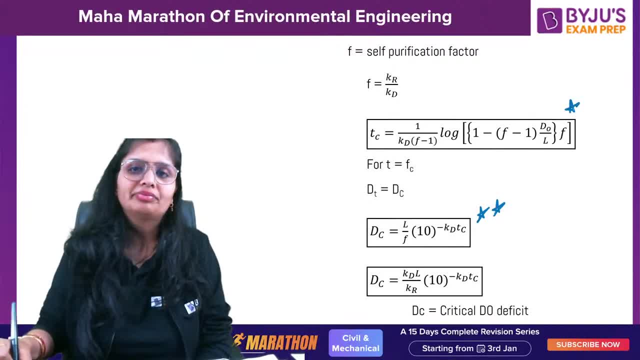 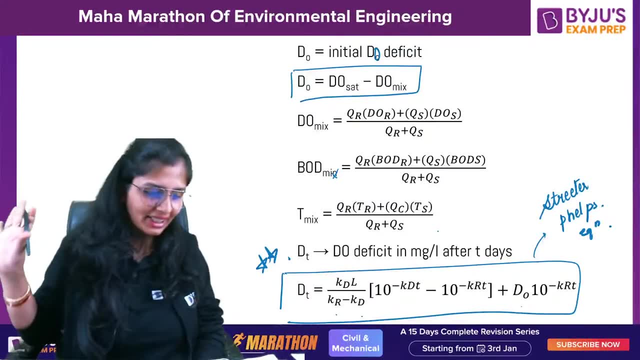 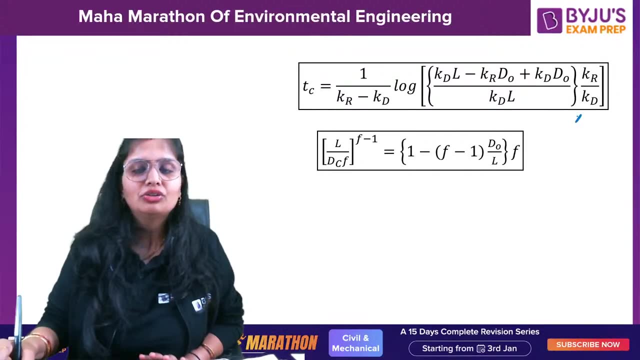 the formula. remember this formula, this formula. okay, so one, two and this is the three, three formulas you have to remember. that's it in this disposal of seaway gelatin. okay, thank you, Sagnik. now, as I already told you not to remember this, remember why? because in some 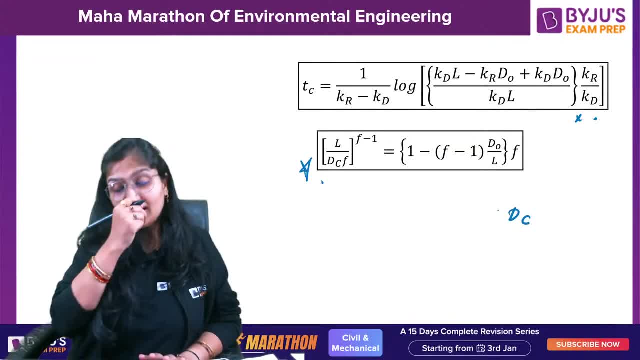 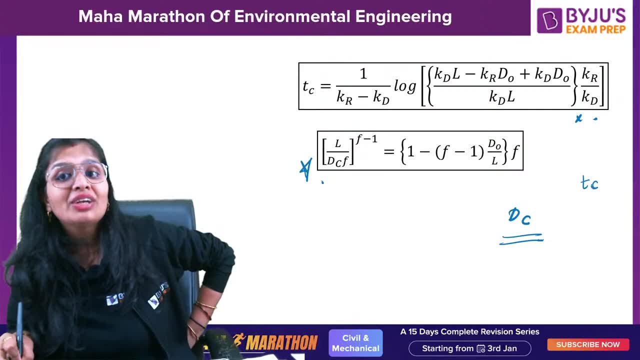 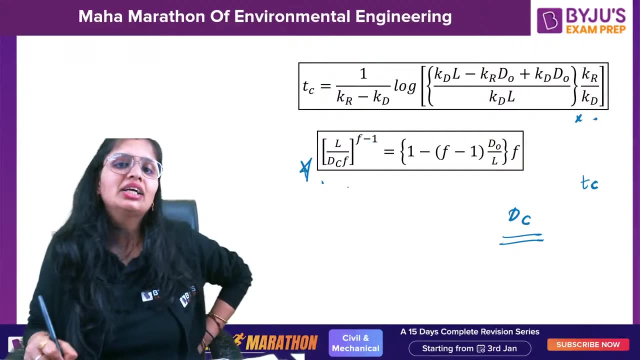 conditions. they will ask you critical DO deficient? understand this very important. some case they will ask you critical DO deficient and you don't need to calculate critical time. that is a wastage, so don't calculate using this formula. okay, you can directly get the critical DO deficient by this. 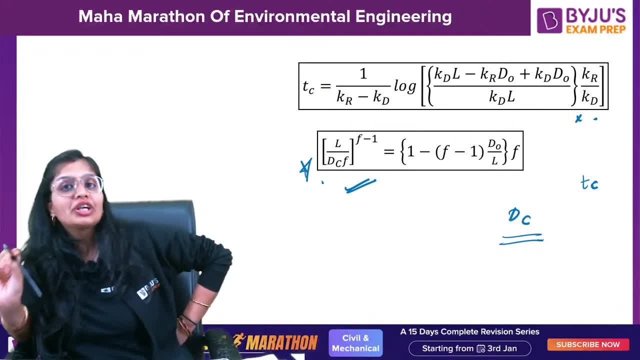 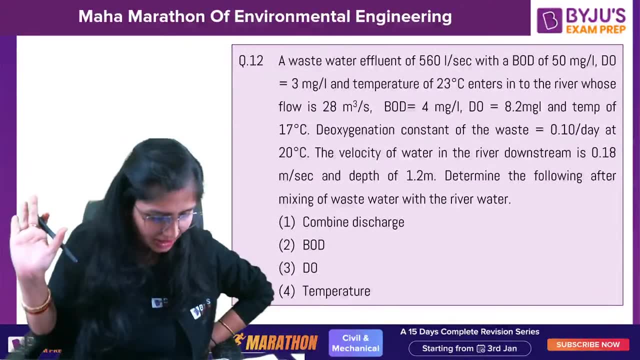 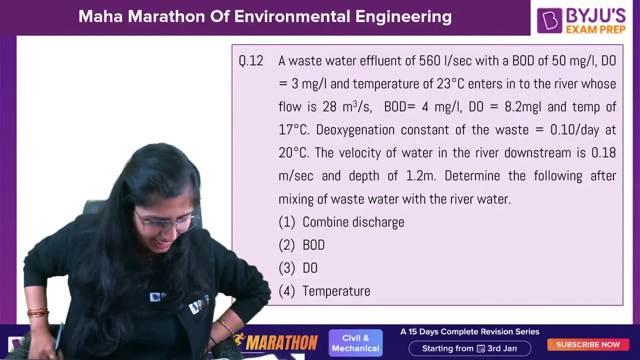 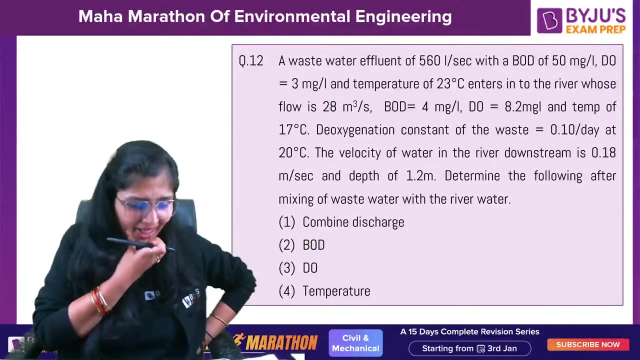 so which formula to use? that will depend upon what is given in the question. fine, now solve this question, guys. two questions are given. solve it fastly. one question only happen at night. do happen more in night than in day time. henry law do is stand on of. do its in constant 9.2 mg per liter at 20C. 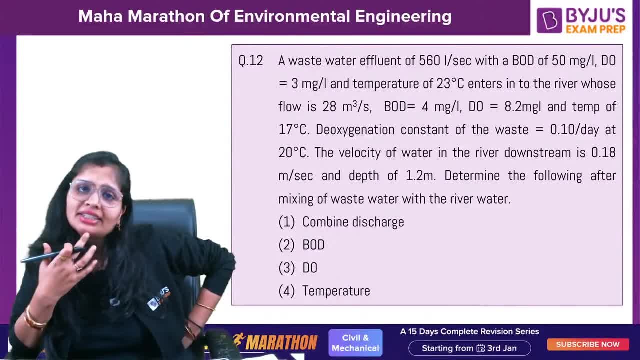 subscribe to our channel, rob, and see you in next video here with very tasty. that would be Saying this question for any with any question from now. As the temperature increases, DO will reduce, So night time and day time depends on it. If the temperature is low at night time, then DO will also increase. 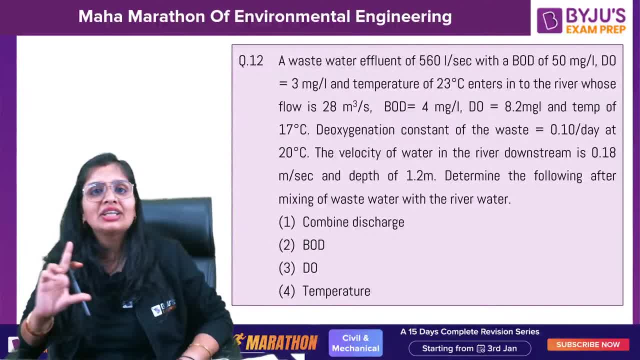 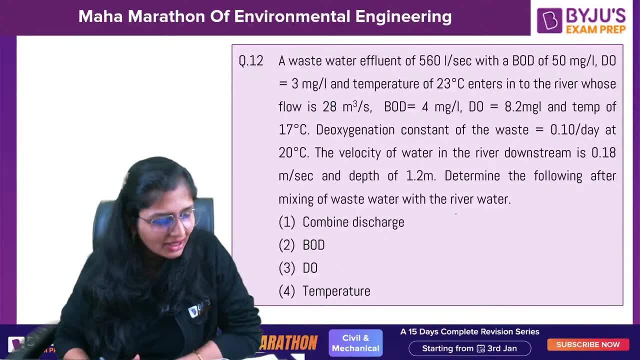 Okay, But DO can never be more than that particular temperature. Come on, guys, this is a very simple question, Combined discharge and all you guys can solve it Fastly, fastly. Now do these questions fastly, because the second question will take time. 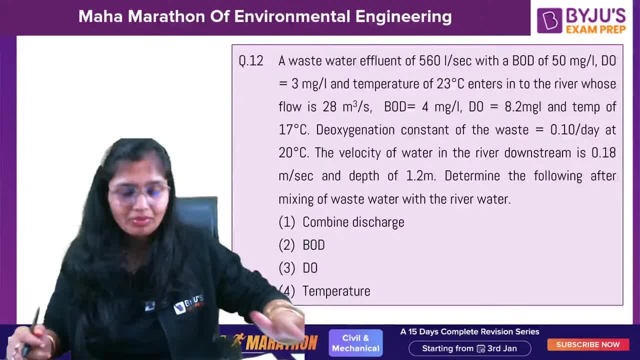 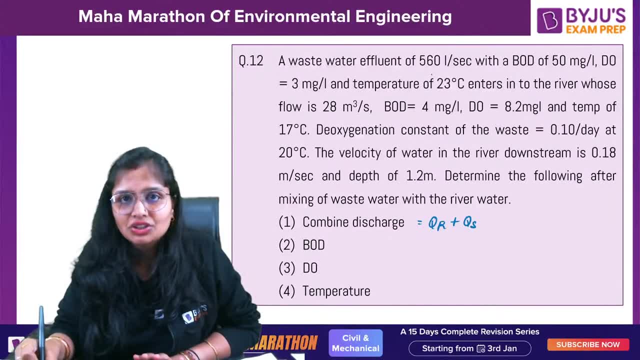 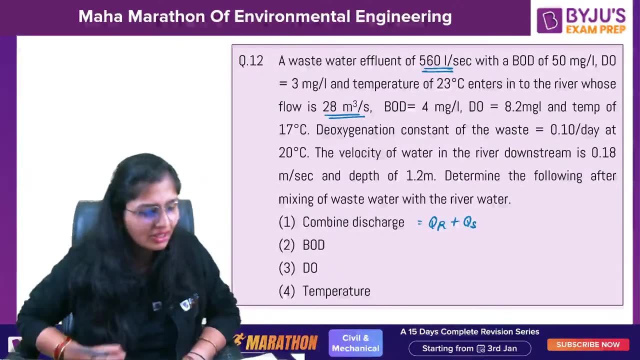 Is it 5 o'clock? I thought it will be chapter by 5 o'clock. Okay, fine, Combined discharge QR plus QS Discharge: waste water 560.. Where is the discharge? 28 meter cube per second. Convert it. 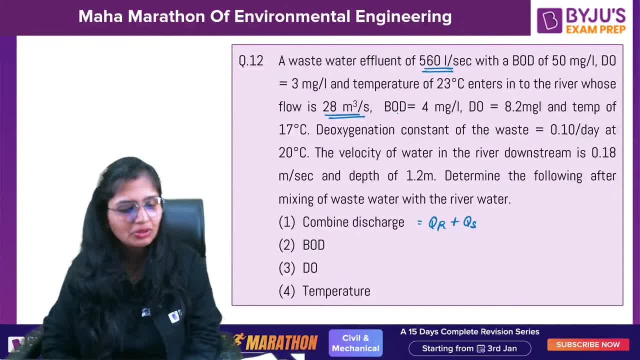 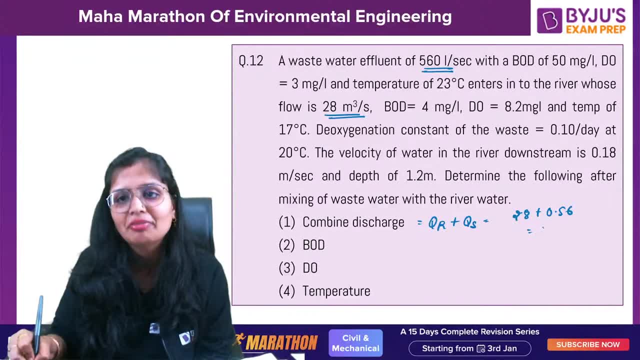 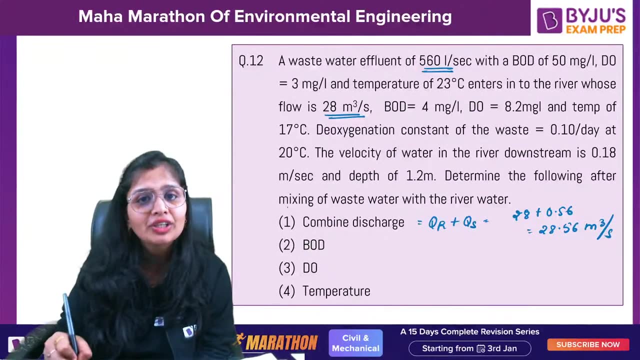 Convert 28 meter cube per second into liters per second, Or if 560 converted discharge is 28.. This I will write 0.56. It will become 28.. 0.56 meter cube per second. DOD See, they determine the flowing water after mixing of waste water with the river water. 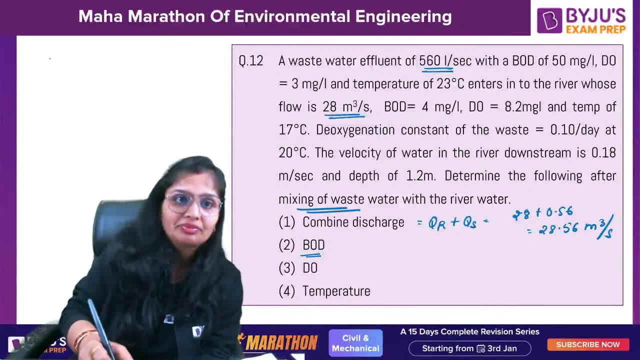 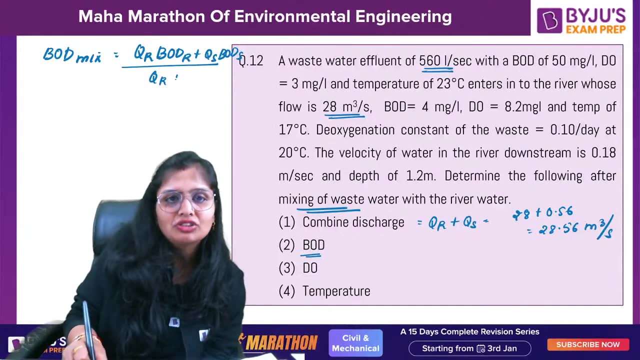 Technically they are writing DOD, but this is DOD mix, So this is DOD mix, Okay. Discharge of river: DOD of river. Discharge of sewage: DOD of sewage. Discharge of river plus discharge of sewage. 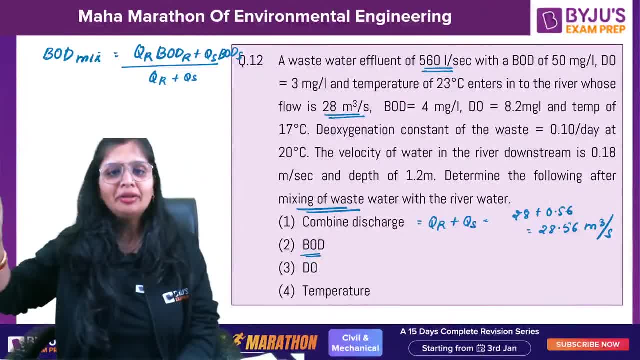 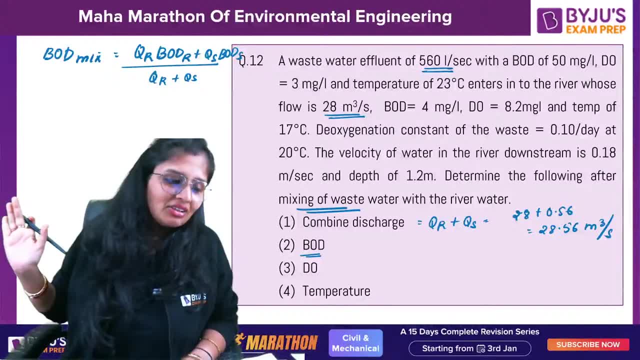 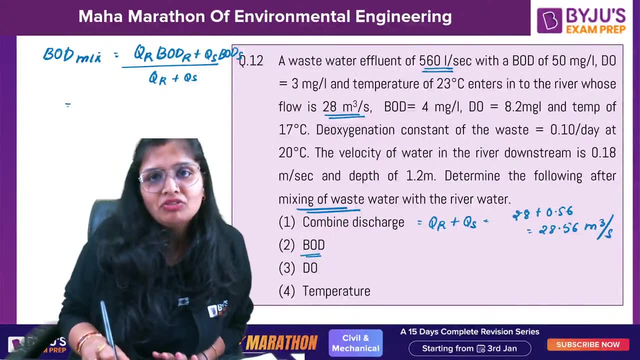 Come on, I will tell you: Vamsi, Girish Calculate DOD mix, Kishalya and BTech Trader calculate DO mix. And who was there other? Sagnik. and all calculate temperature. So, guys, tell me what are the things fastly, so that we can do it fast. 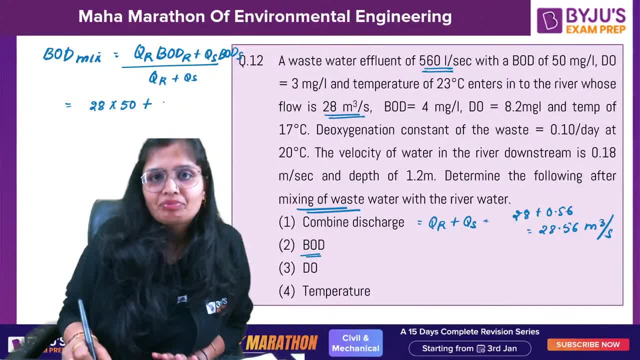 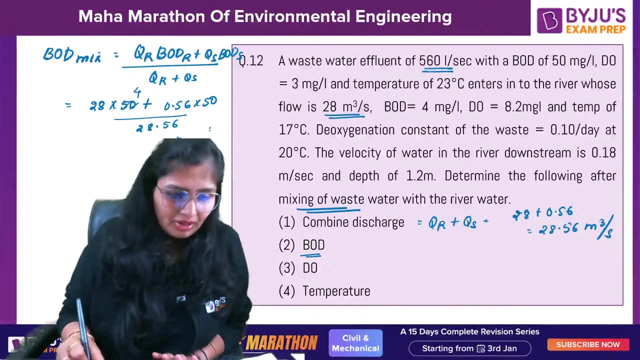 28.. DOD is 50 mg per liter. DOD is 4 for this one: 4. 0.56.. DOD is 50. 28.56.. This is only life. I think I should make it private. 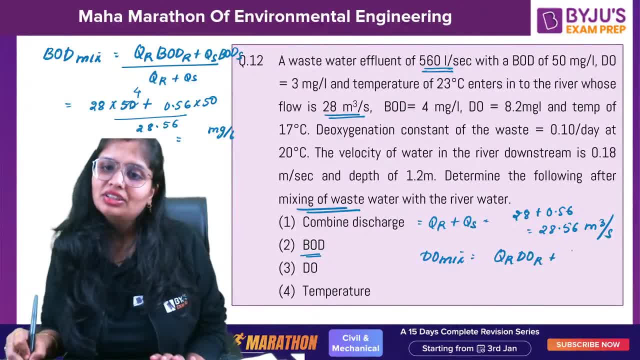 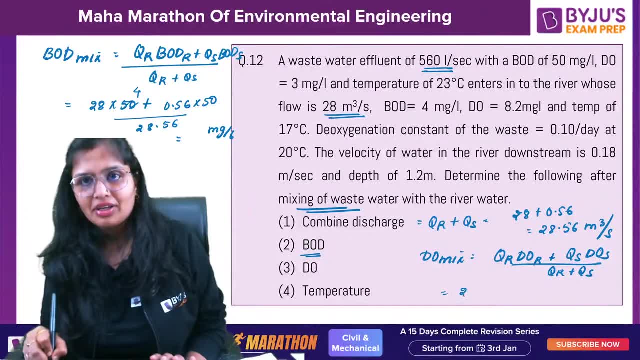 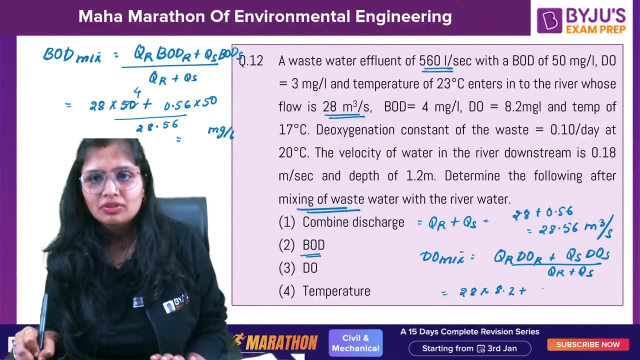 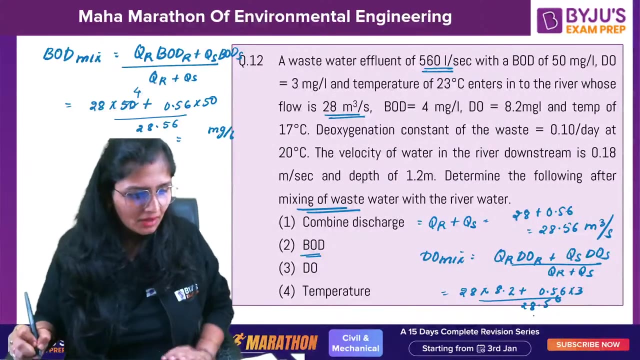 Discharge of river: DOD of river. Discharge of sewage. DOD of sewage. Discharge of river plus discharge of sewage 28.. DOD 8.2.. 4.9 is what DOD mix. 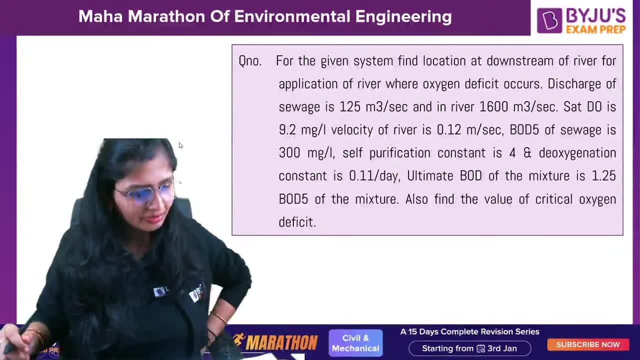 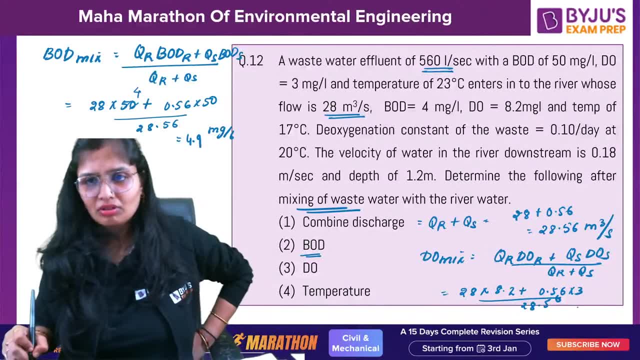 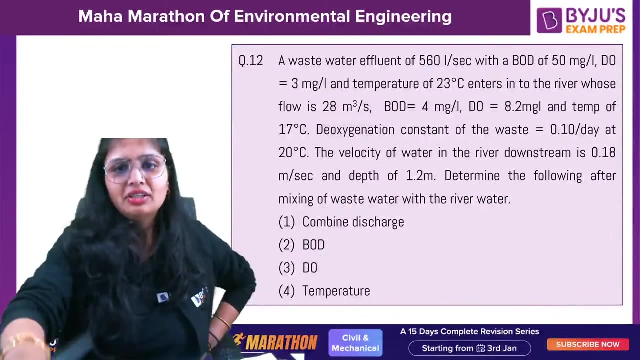 4.9 mg per liter. What is DO mix? What is DO mix? 4.9 mg per liter. 4.9 mg per liter. 4.9 mg per liter. What is DO mix? Temperature mix. I will write it here: 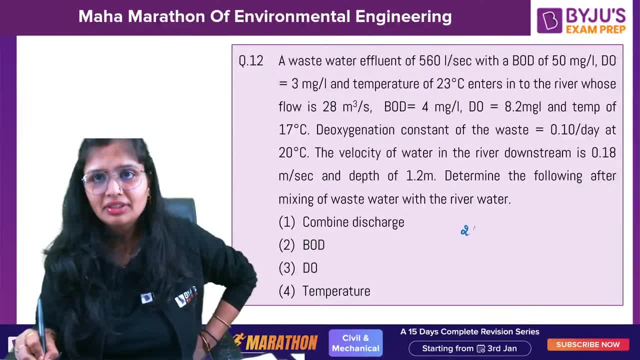 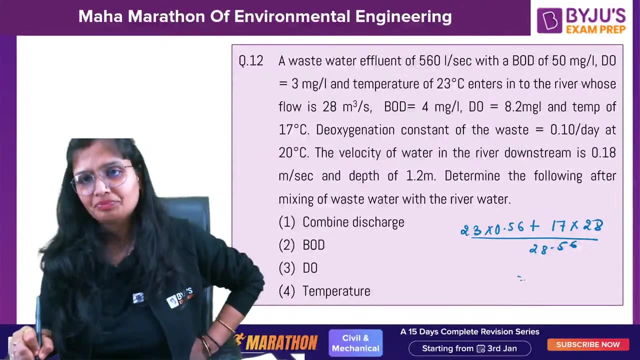 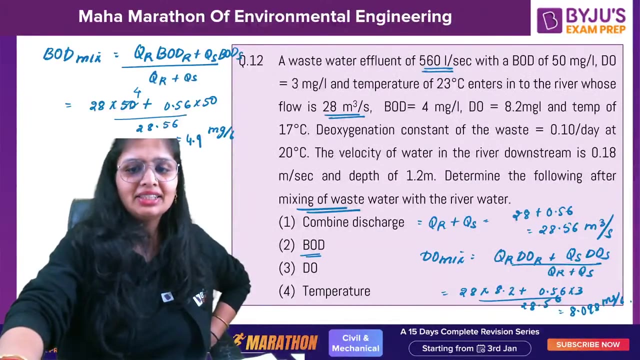 Temperature: this is 23.56 and this is the temperature. 17 and it is 28 and this is 28.56.. How much is the temperature? 17.12.. Clear 8.098, that is, 8.108.. 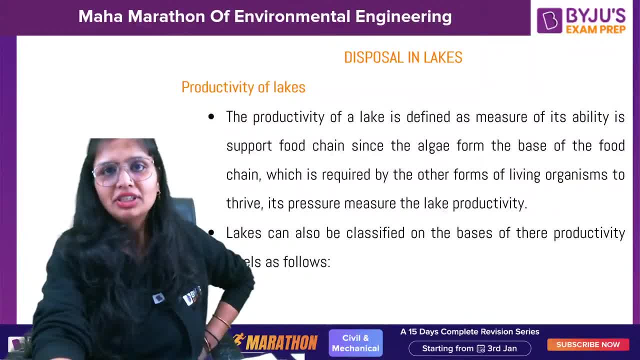 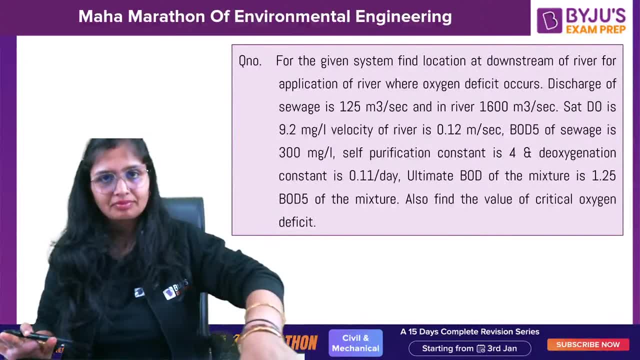 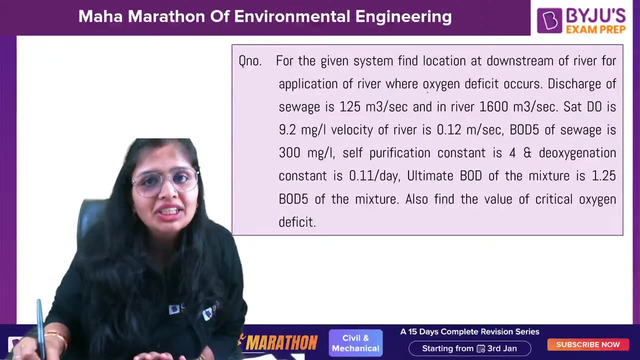 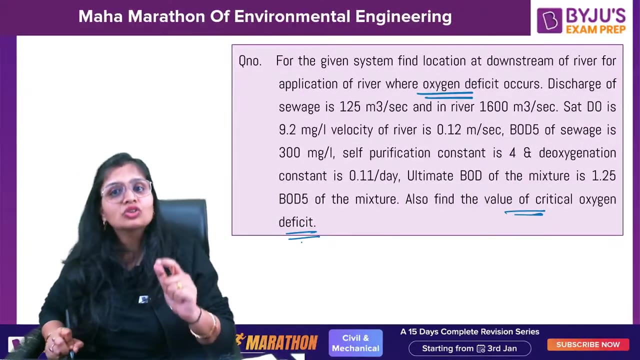 Okay, this is the second question. then we will move towards 3.. Disposal in lakes is also left. Fine, deal this. It is asking you find location at downstream where oxygen deficit occurs and also find first the location it is asking you and also find the value of critical oxygen deficit. 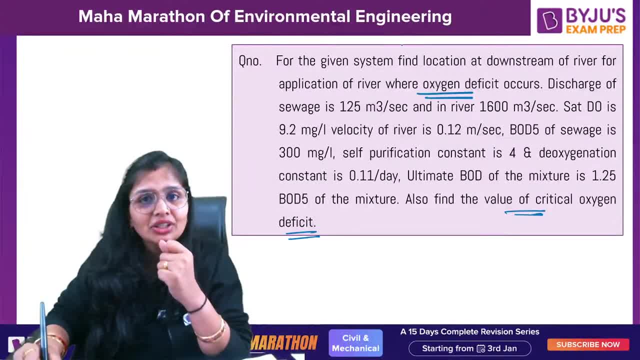 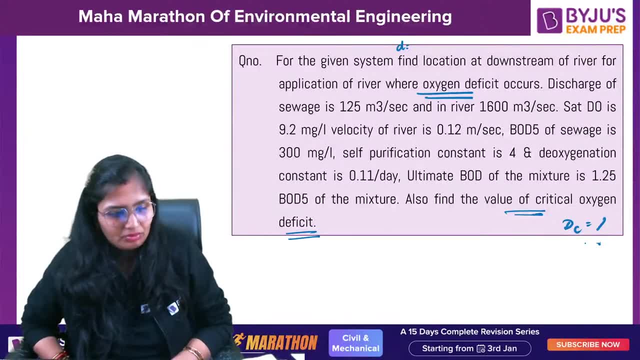 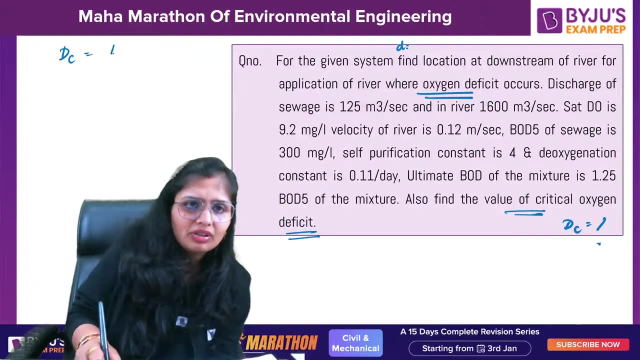 That means location. it is asking you, that means it is asking you the distance and it is asking you the value of critical oxygen deficit. Come on, guys, how we will do, How you will do it See if it is asking you. L by F, 10 raised to power minus KD, Tc. 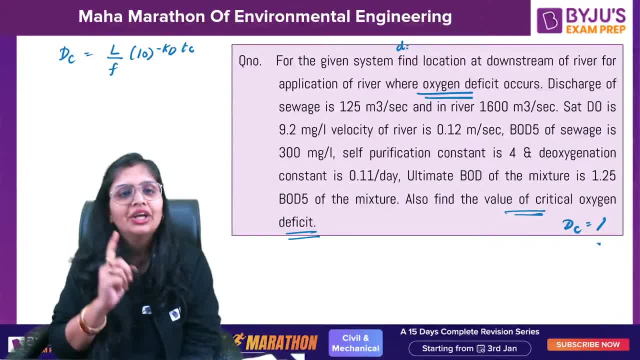 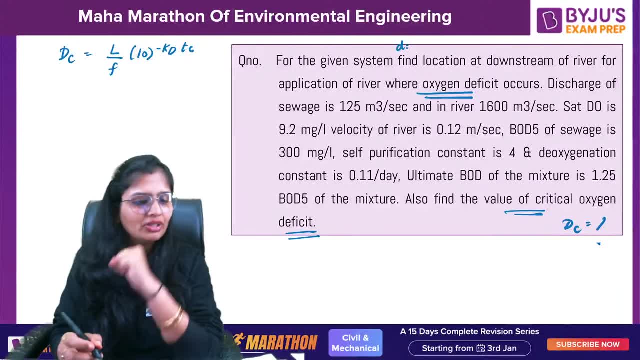 That means KD is given to you in the question. yes, You need to calculate L. F is given to you. yes, F is given to you as 4.. You need to calculate L and you need to calculate critical time. Now, how you will calculate critical time. 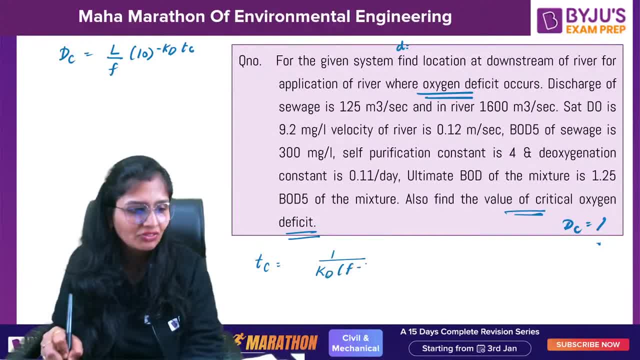 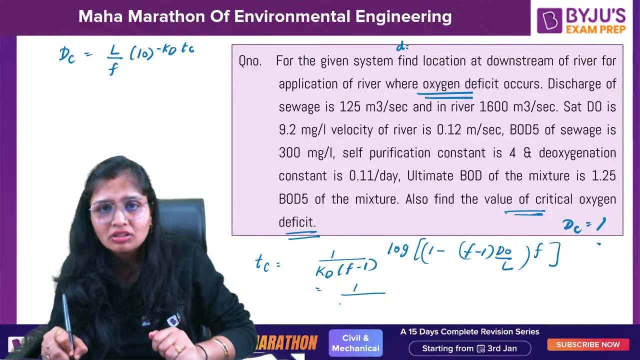 Come on guys, 1 upon KD, F minus 1, be faster log. 1 minus F minus 1 DO naught L F. So come on, substitute it Tiksha Swapnal, everybody solve it. KD is how much: 0.11, 4 minus 1 log base 10. 1 minus 4 minus 1 DO naught. 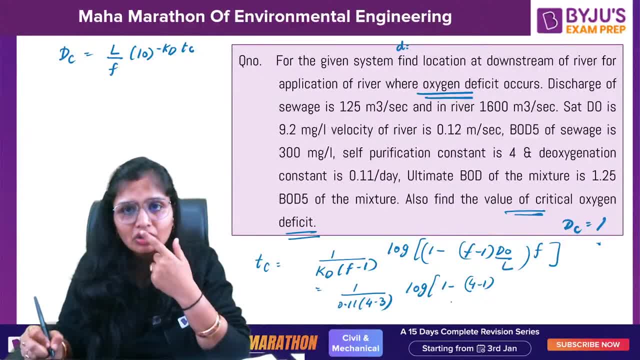 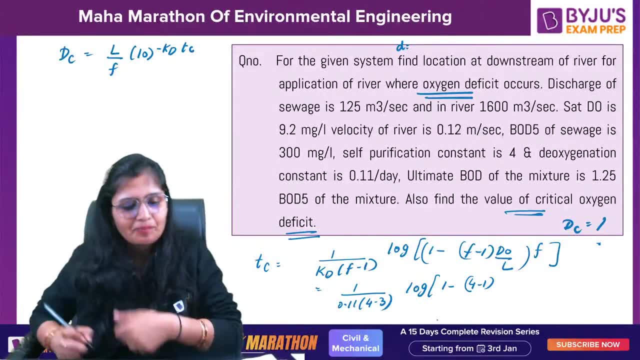 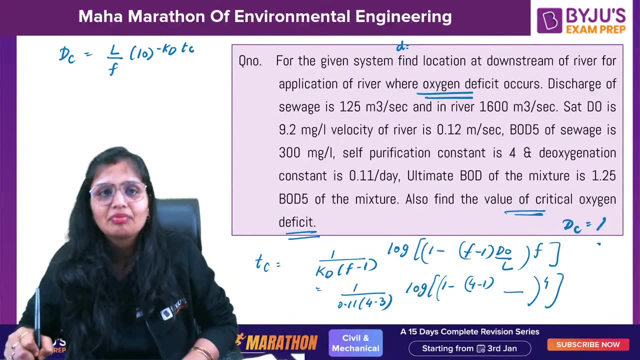 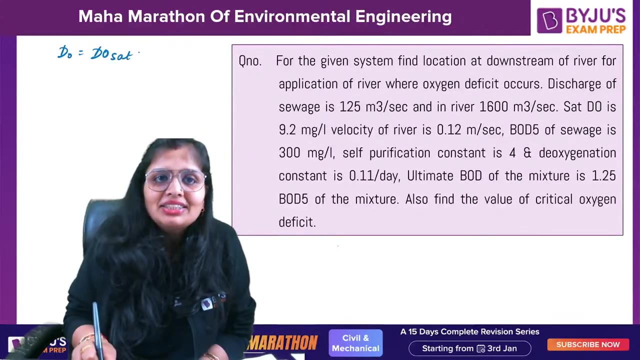 DO naught is given to me in the question, No, not given to me in the question, directly Not given to me. Calculate DO naught also. Calculate L also, Everything we have to calculate. Lendy question. Okay, DO naught is equal to DO saturated minus DO mix. 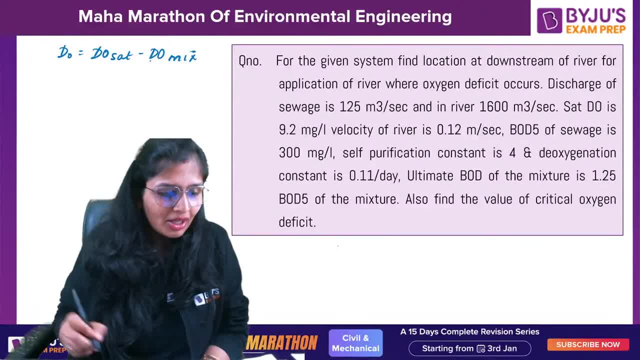 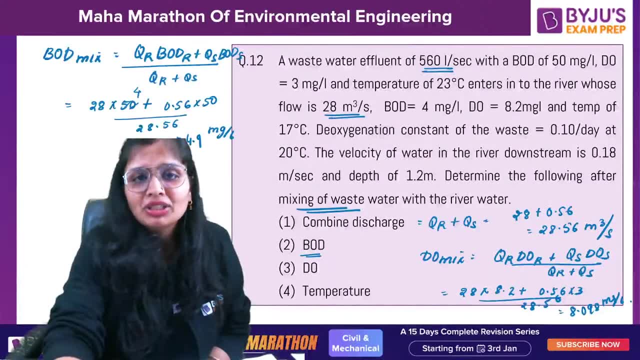 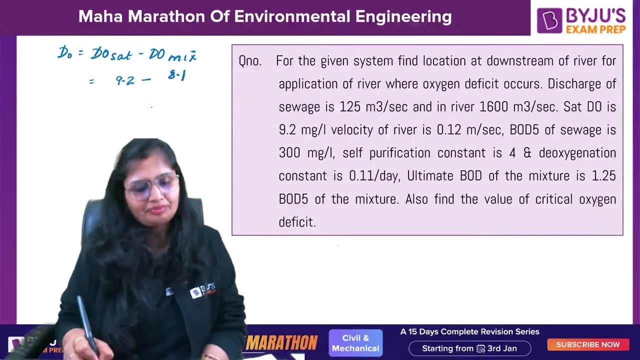 DO saturated. one question, entire thing will be clear. Okay, Okay, DO saturated is how much? How much 9.2 mg per litre DO mix? already calculated how much? it was: 8.01,. how much it is coming. 8.098, 8.1,. how much is that? 9.02 mg per litre. 9.04 mg per litre. Do you mix? already calculated how much it was. it is gone: 8.098, 8.1.. 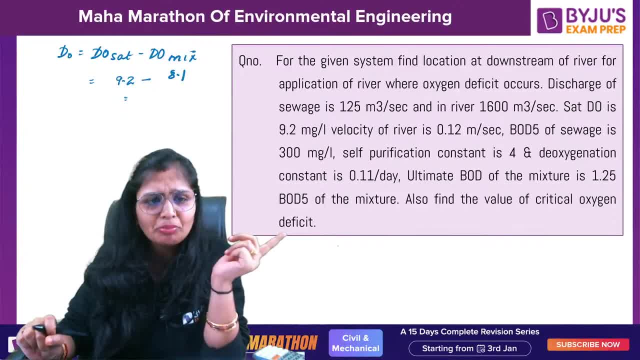 How much it is coming? Do you mix already calculated how much it was? How much it is going? 8.098, 8.1.. quotient was for the previous quotient. This is different quotient. That's not what I was thinking. 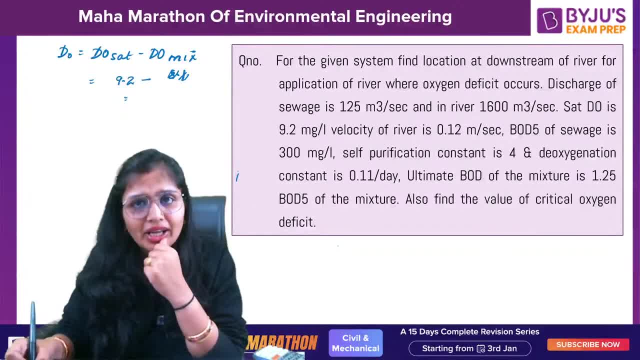 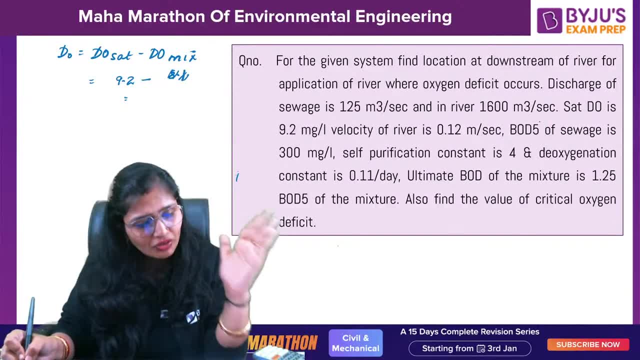 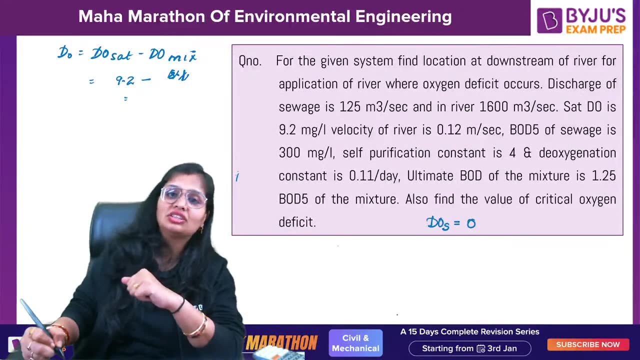 That is for different quotient. Here I have to calculate: See in the quotient. nowhere it is given it has taken oxygen deficit is occurring. Since nowhere it has mentioned, I will take sewage is heavily polluted. I will take dissolved oxygen of sewage as 0 and in the quotient it is. 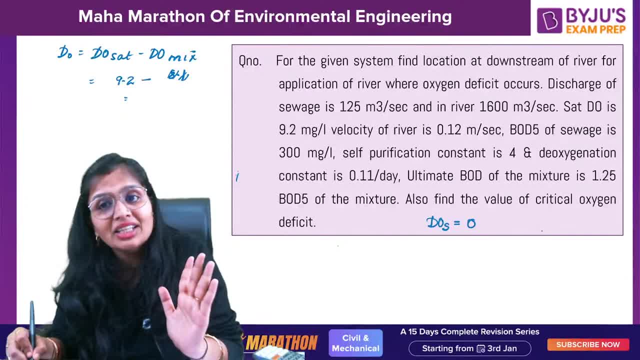 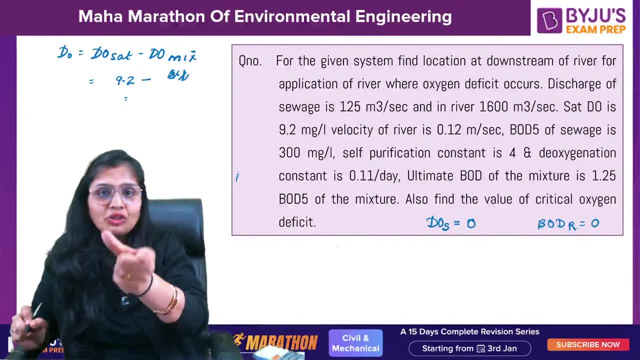 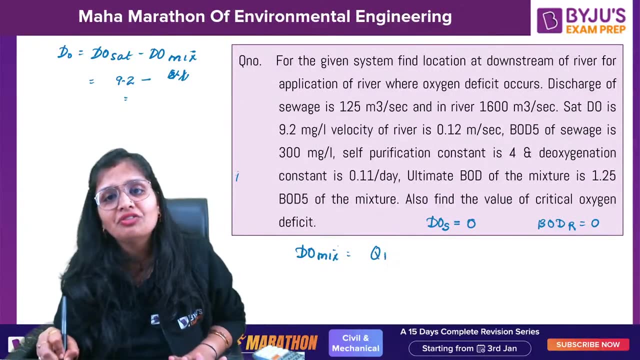 given, DO of river is 9.2.. That means there is no oxygen demand in river, So BOD of river is 0.. Remember this. So they won't tell you directly, You have to read between the lines. Now calculate DO mix. Come on Discharge of river into DO of river. Why? Because discharge of sewage is 0.. 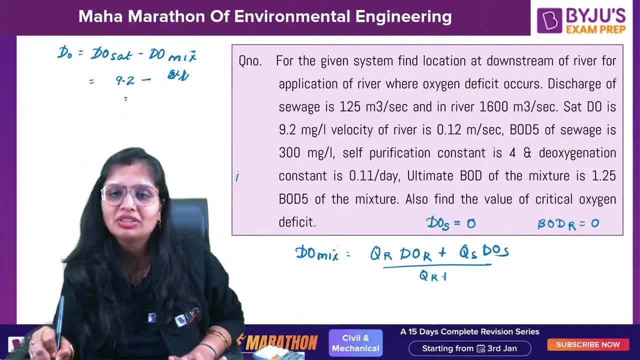 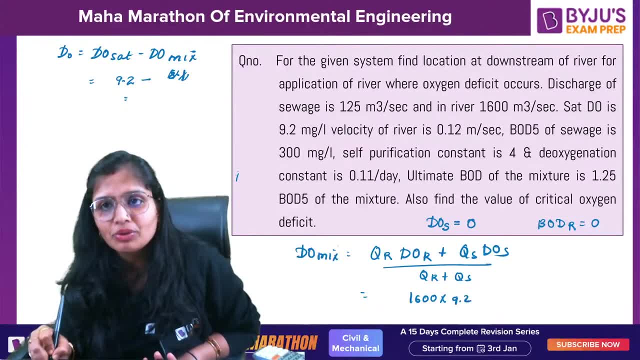 So no need, but fine, I will write it here. Discharge of river plus discharge of sewage. Come on, guys, What is the discharge of river? 1600 DO of river is how much 9.2.. 1600 plus 125.. How much it comes out to be. 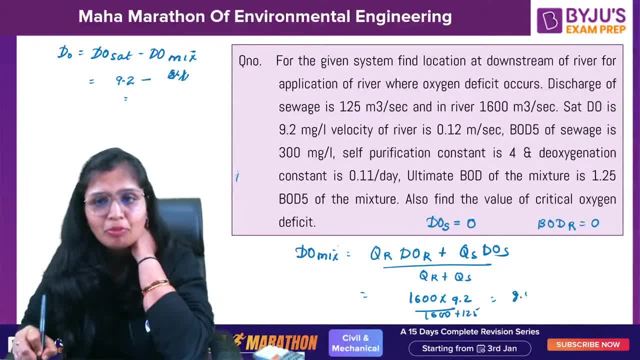 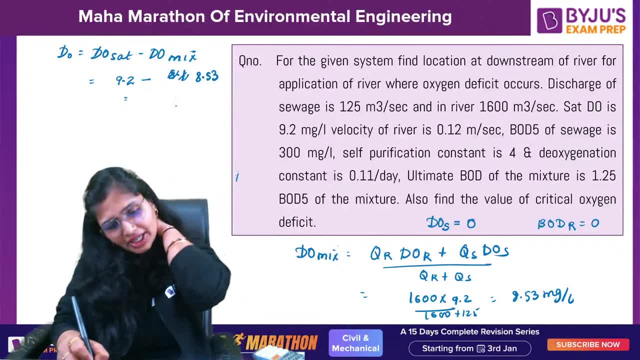 This is 0, by the way. This will come out to be how much: 8.53 mg per litre. So substitute it here: 8.53 mg per litre. It will come out to be how much: 0.67 mg per litre. Just check the calculations. 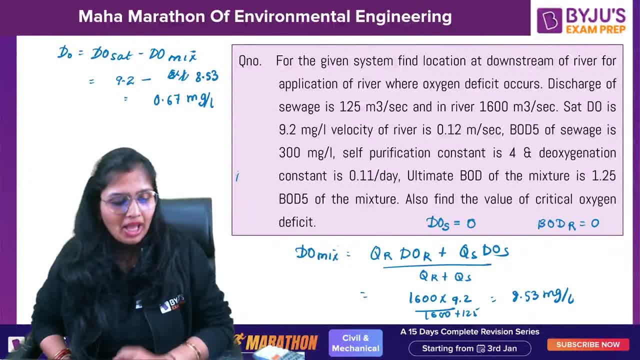 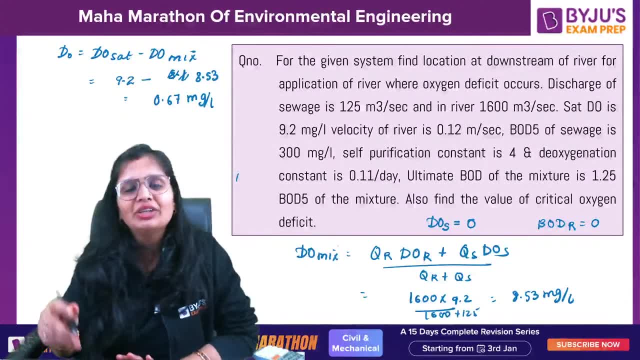 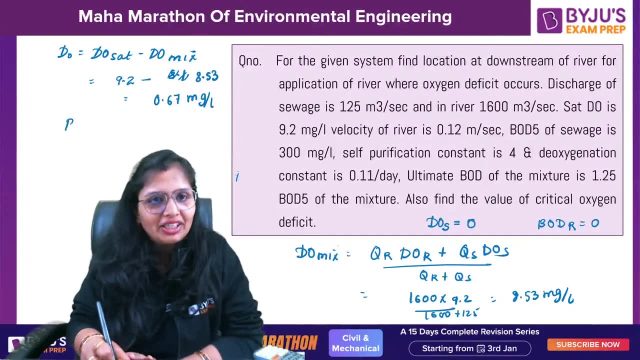 So this is the initial DO deficit, What you need. You need the value of, you need the value of BO, North, Okay And ultimate, or basically you call it BOD U or you call it L, So ultimate BOD is 125 percent, or they have generally written. 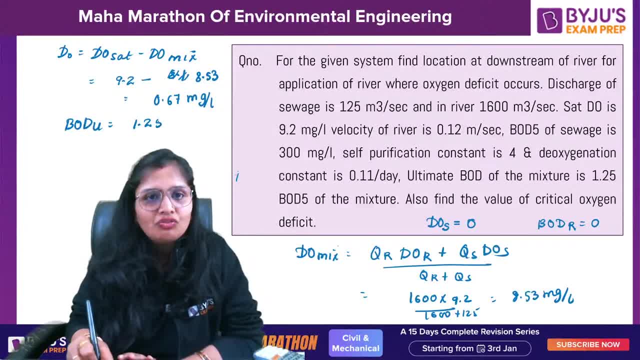 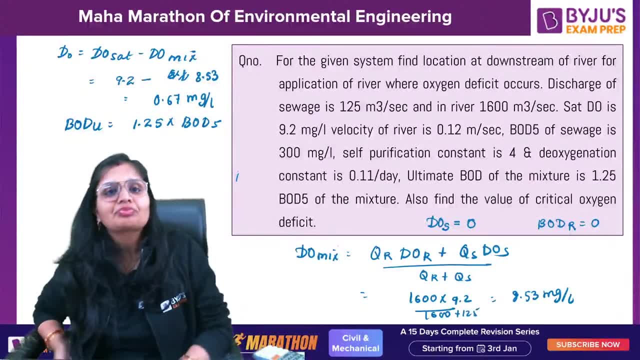 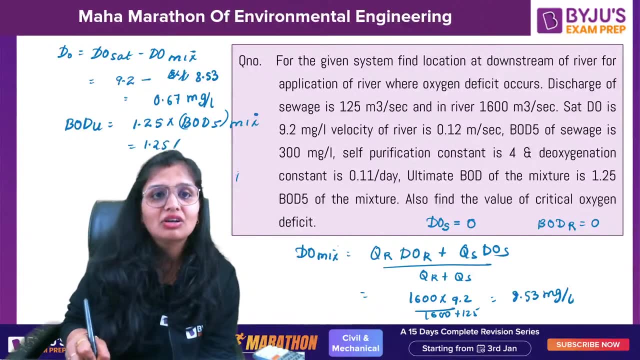 it here. BOD ultimate is 1.25 is the BOD 5 of the mix. So now you have to calculate 5 days BOD. also Calculate BOD of the mix. Come on, Come on, guys, Long things You have to do it, You won't get it easily. So, BOD mix: How to calculate? 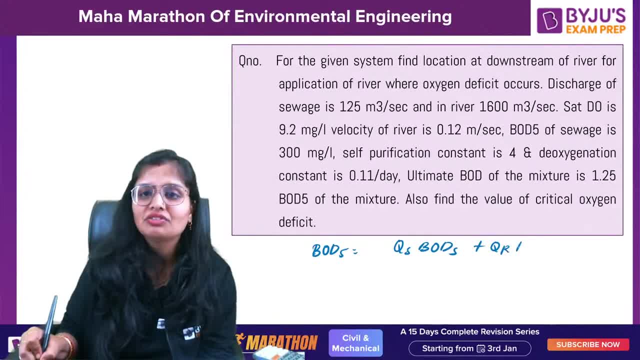 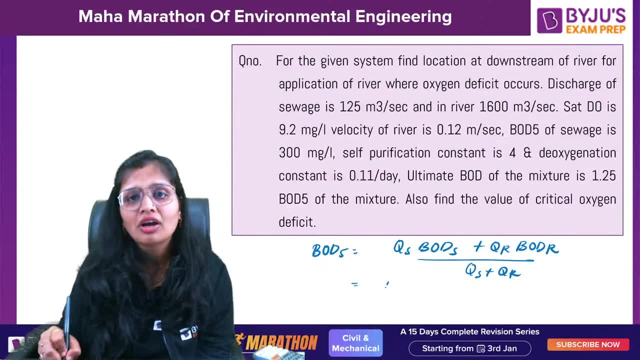 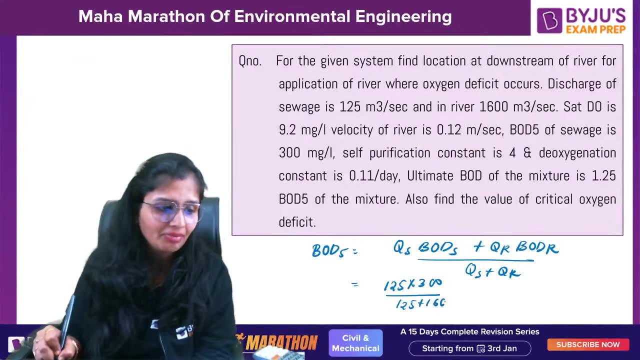 Discharge BOD of discharge river. BOD of river. Now, in this case this will become 0.. So this is gone. 125 into BOD of sewage is 300.. 125 plus 1600.. How much it is coming. 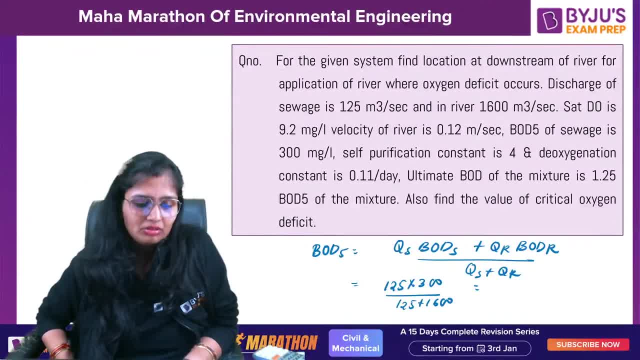 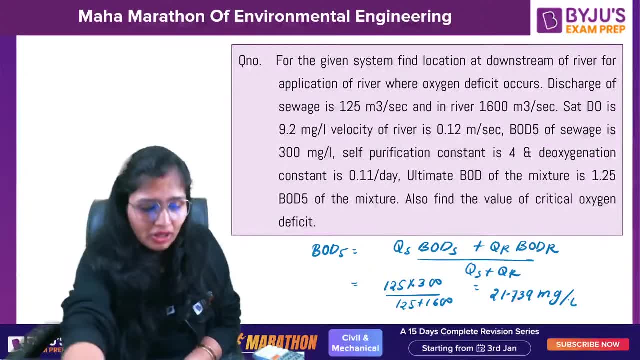 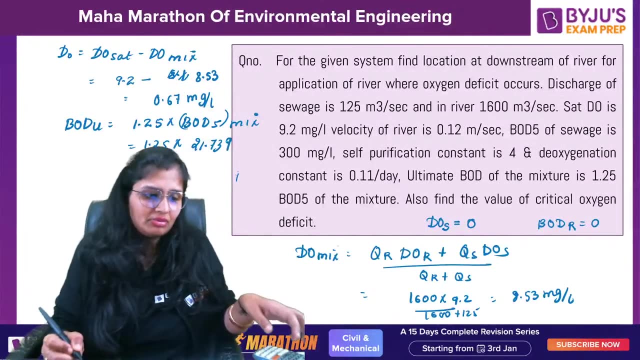 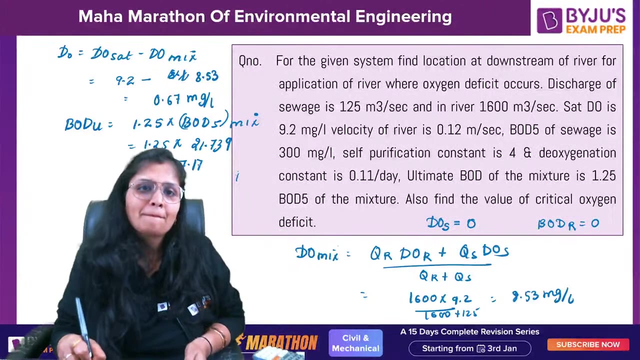 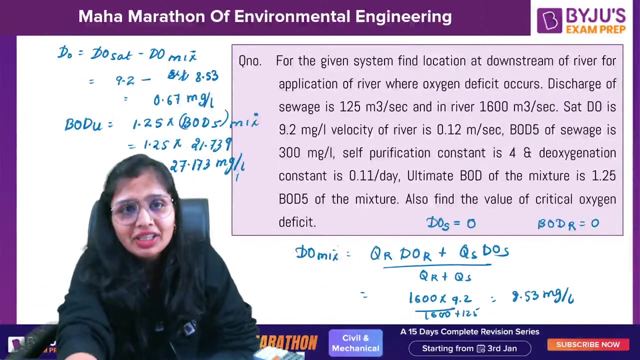 1.25.. This is the 5 days BOD. Just check it out once: 21.739.. So 21.739.. 73974.. And how much it is coming 1.25 into this Calculated. so many things Now substitute it here. How much is DO North? 0.67.. 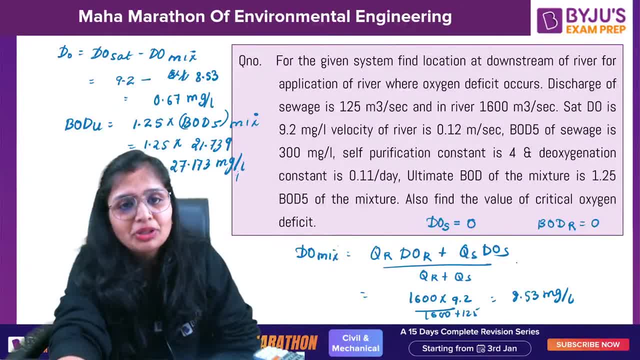 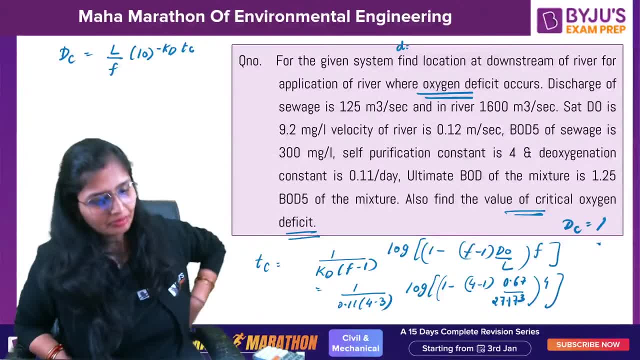 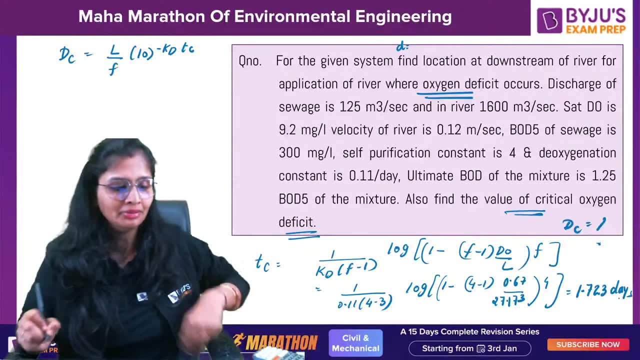 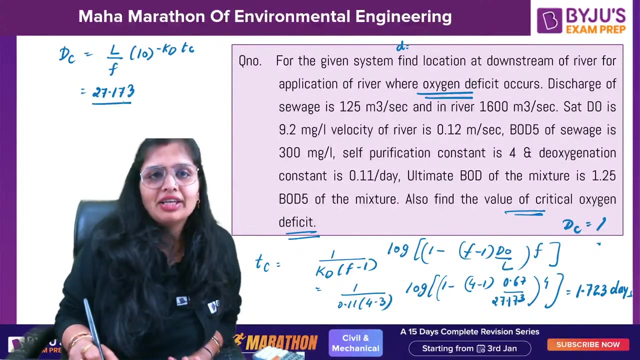 And how much is BOD ultimate 27.173.. 27.173 guys solve it, So all of it, you will get the critical time as 1.723 days. So 27.173 f value is 410 raised to power, minusvic 80.. 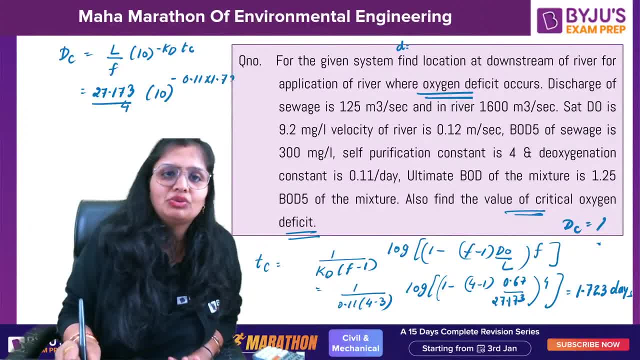 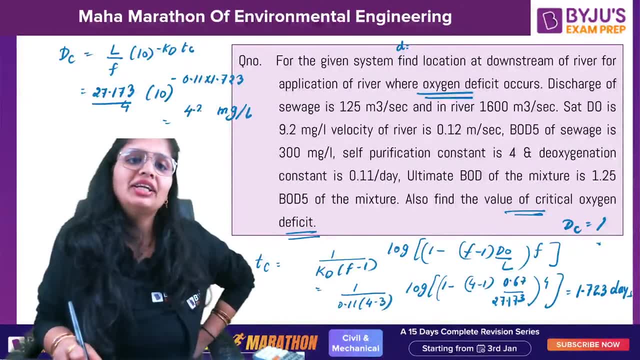 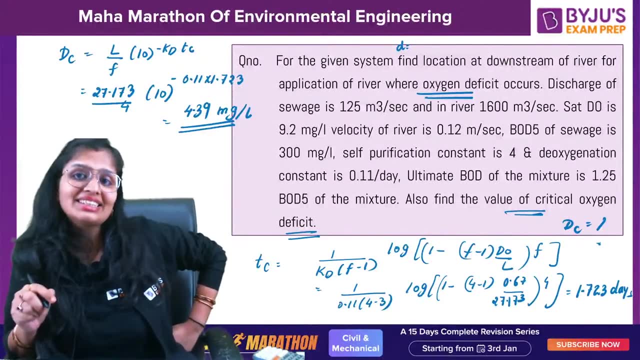 80 is booked. So from here you will get the critical DO deficit in MG per liter. How much you are getting? 4.39.. So one thing you got. It is asking you the location. Location means the distance. 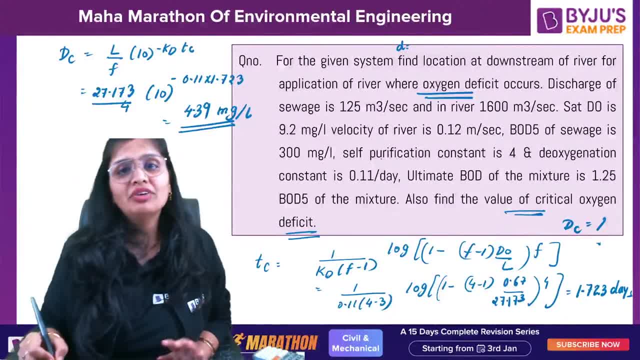 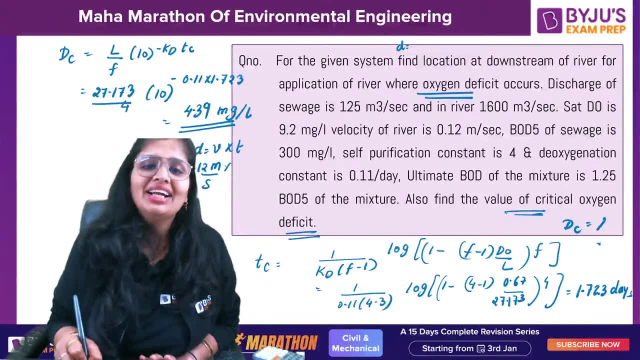 Distance is what Velocity into time. So the velocity of river is given to you, Velocity into time. Velocity is 0.12 meters per second. Time is given to you as 1.723 days, So one day, 864.00 seconds. 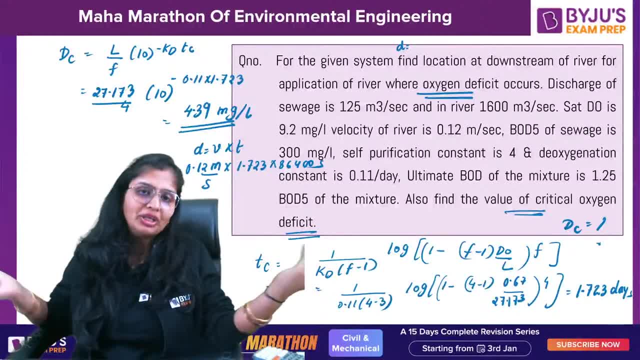 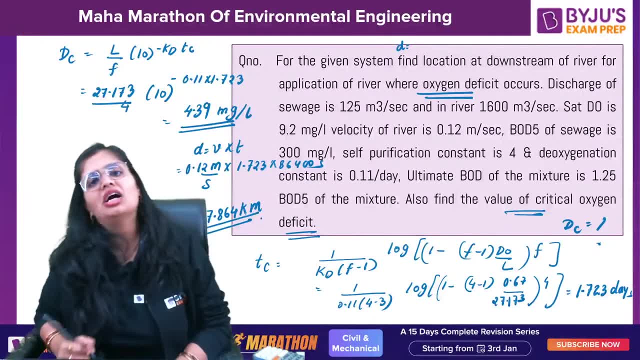 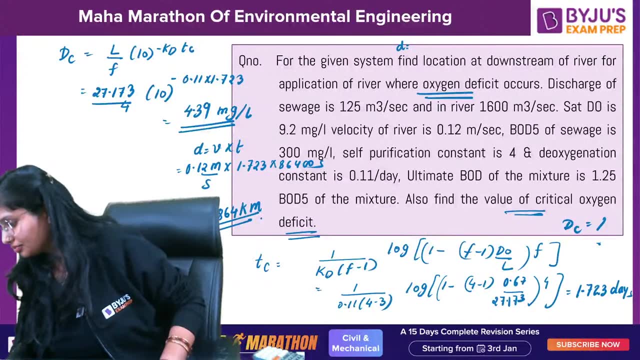 Okay, Divide by 1000.. You will get the answer in kilometers. So it will come out to be 17.864 kilometers. This will be done Clear. Understood the whole question. Understood the whole question. Everybody fast. 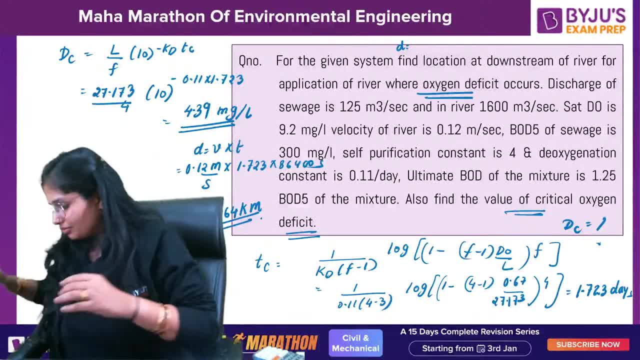 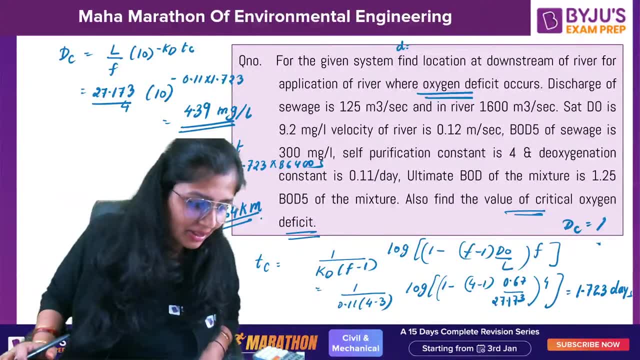 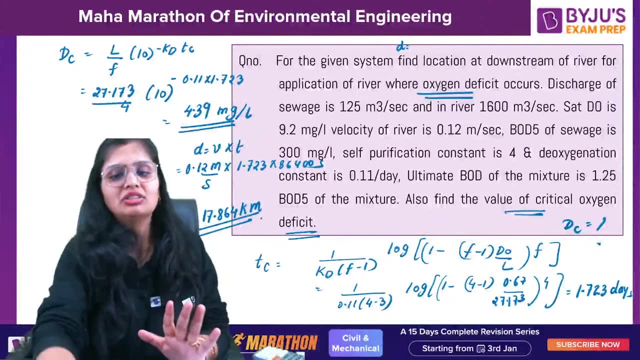 So this was the big question. at max They can ask you. ma'am, It is not expected in this much detail. Yes, Kirish. So instead of making every question part by part, I have taken a bigger question for explaining all the questions. 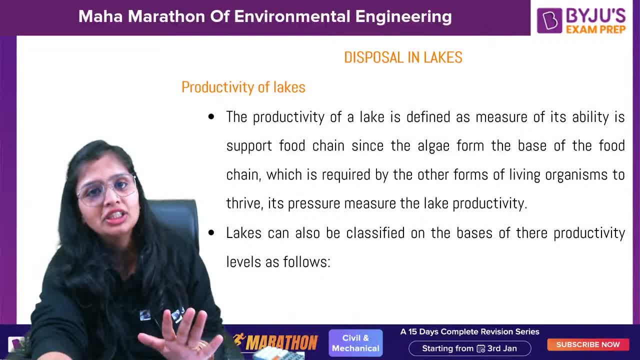 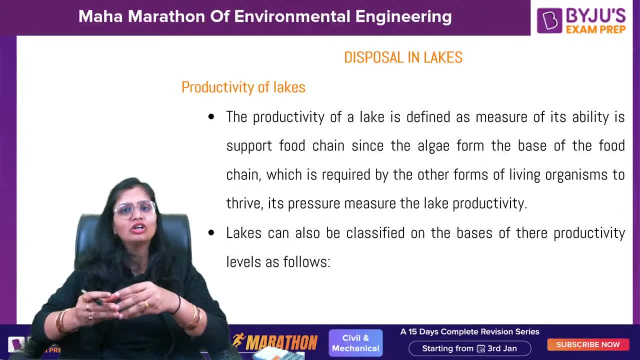 Okay, Now talking about disposal in NAICS Generally, we say we have many things to study, Many things we are studying Productivity. when you talk about The, productivity means able to support food chain. Food chain means what, What is happening. 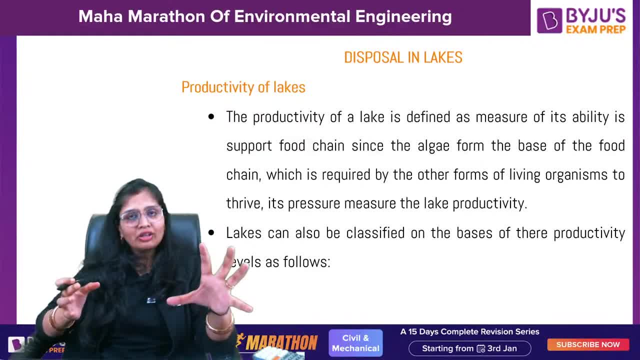 What is happening? Generally, microorganisms uses oxygen. That oxygen is given by algae. Algae gives that oxygen while preparing this food, While preparing its own food. Okay, So microorganisms attacks on the organic matter, On its decomposition. Aerobic decomposition microorganisms liberates carbonates, nitrates, sulfates. 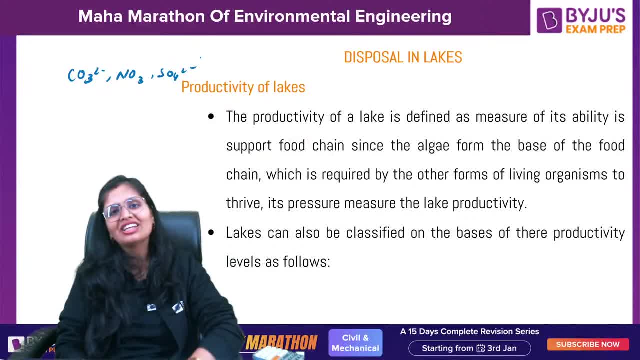 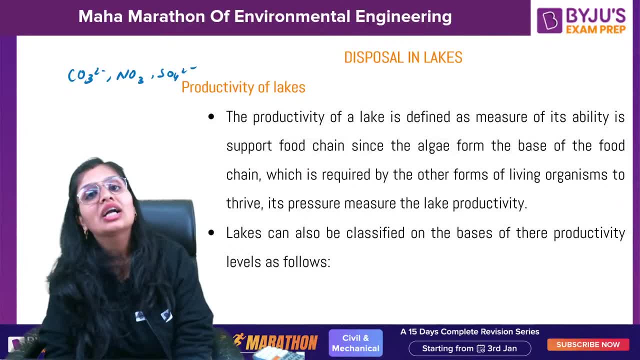 Okay, These are being used by algae as well as by the fishes and all. So this whole chain is basically the productivity. So more the concentration of algae, more is the productivity. So, based on that, you have four types of lakes. 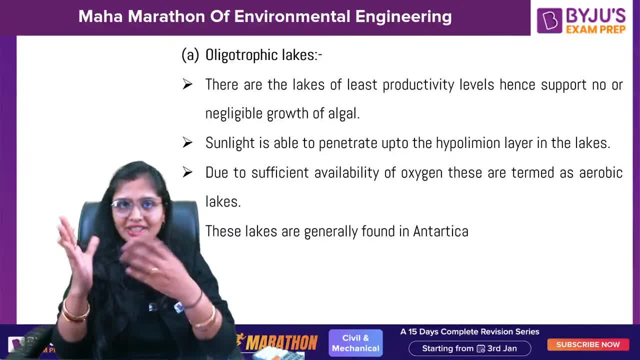 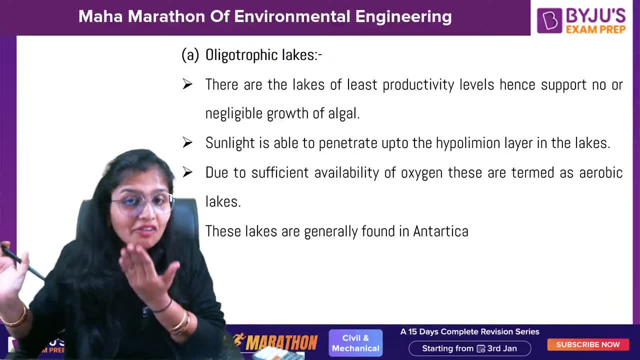 One is oligotropic: level least productivity. That means you see it in foreign and all Generally you see it that the lake is so pure, crystal clear. If you look you can see your face also. Okay, So this is the case of oligotropic. 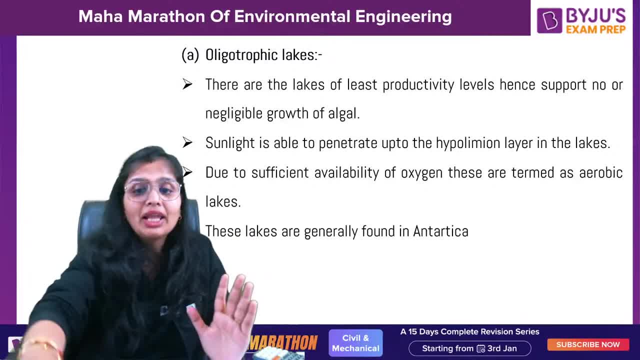 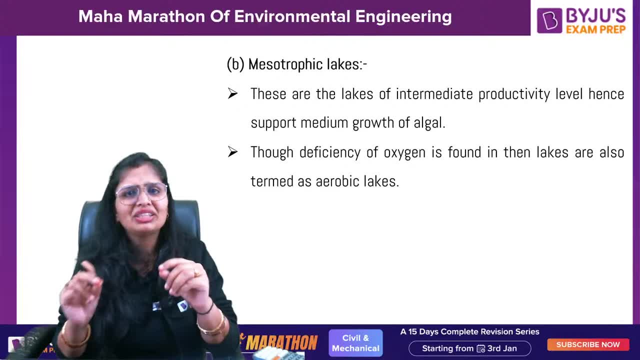 Okay, This is the case of oligotropic, Now mesotropic algae will be there, Okay. Deficiency of oxygen will be there. Algae will be there, But intermediate level will be there. Huge quantity will not be there, Okay. 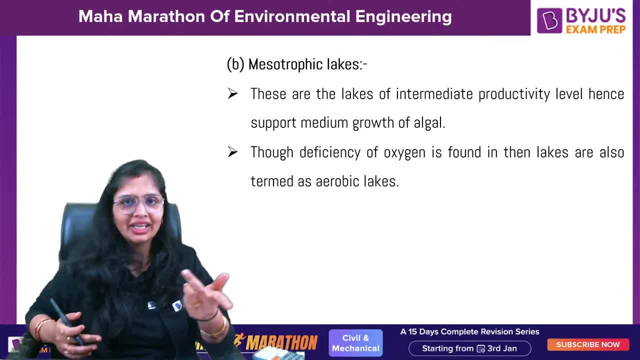 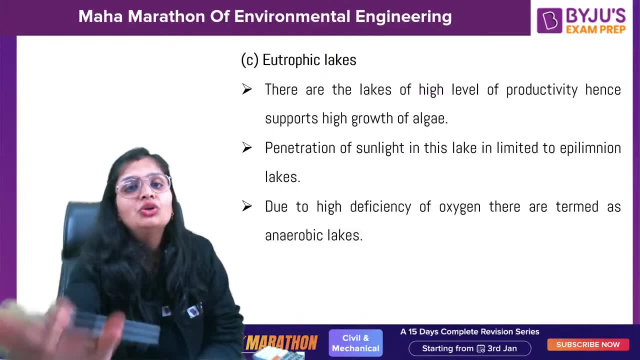 First time it is in confusion. Okay, You see this question again. I had been a little fast because I thought you know that, Then you will understand why I am saying: Okay Now. eutrophic lake, high level of productivity, high growth of algae is there. 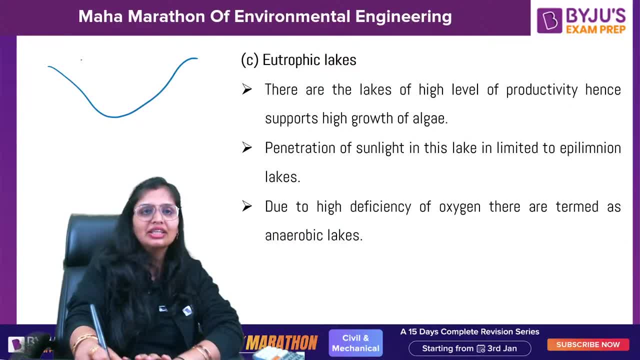 Okay, Generally when you see the lake, actually there is one layer epilimnion. This is metacline or thermolimnion, you call it, and then you have hypolimnion. See, if the lake is pure, water can penetrate, sunlight can penetrate up to hypolimnion. 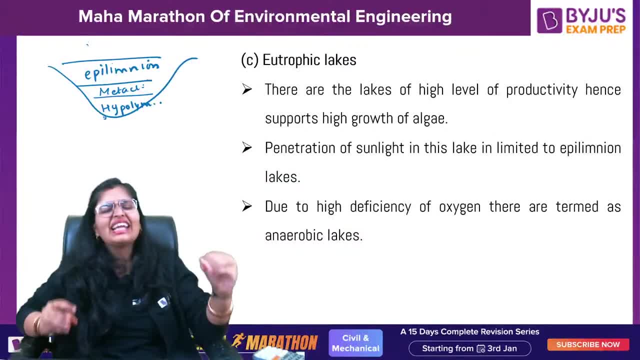 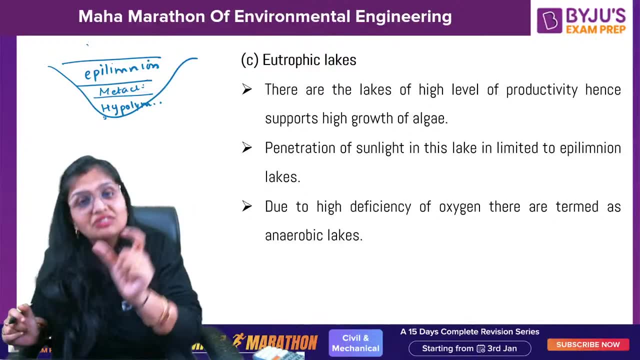 That is for the case of oligotropic. But if the lake has algae and all? So what will happen? The sunlight cannot penetrate. Algae interferes with the penetration of sunlight. So what will happen? In this case, the sunlight is limited only to epilimnion. 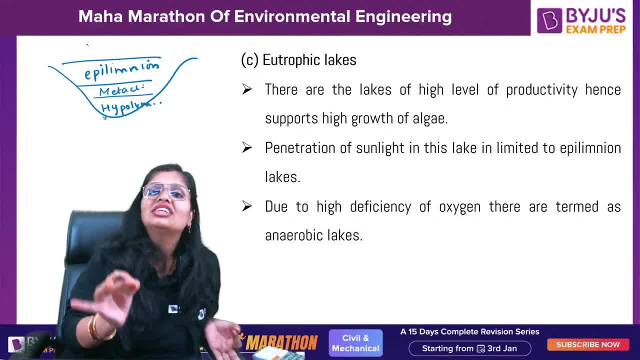 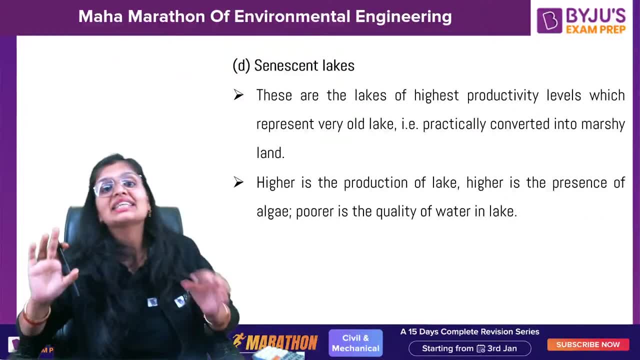 Okay, And since oxygen deficiency is there, you call this eutrophic lakes as anaerobic lakes. These all can be asked in MSQ. That's why you should know Next, senescent lakes, Lakes of highest productivity, Why? 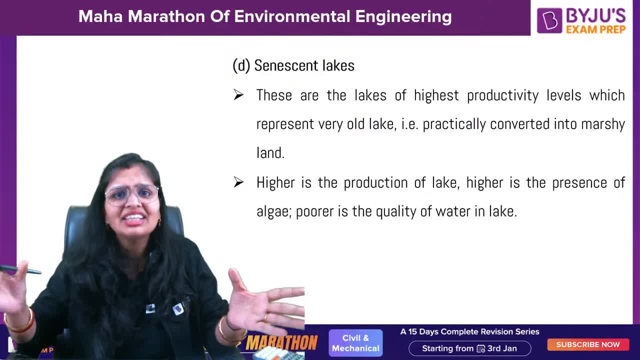 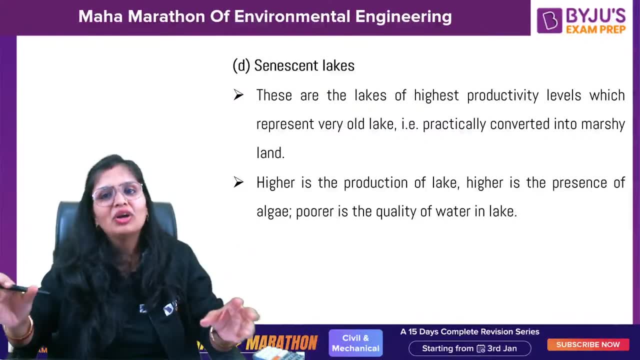 Because now they have converted into marshy land. You guys have seen it in movies and all Dal dal. You stand there and you try to sink down. So that are the senescent lakes, Because maximum algae is there and you cannot use that water. 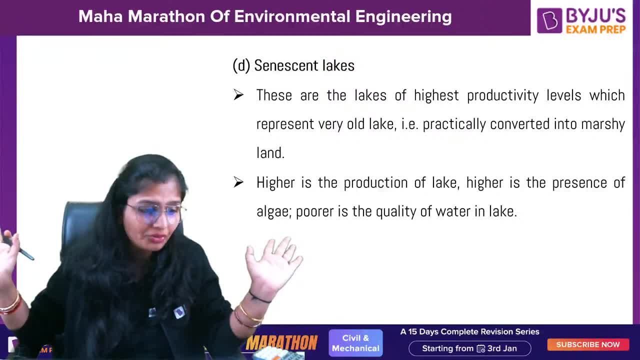 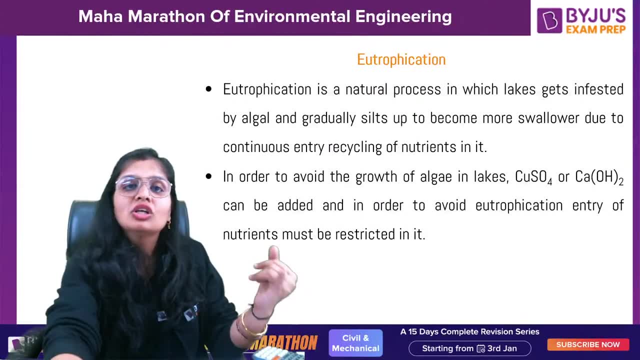 So higher the presence of algae, poorer is the quality of water. Okay, So these four lakes, if they ask you, you should know They will ask you arrange the following four options they will be giving you. Highest productivity is for senescent. 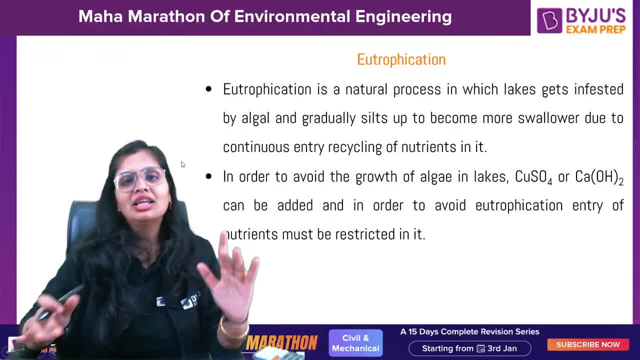 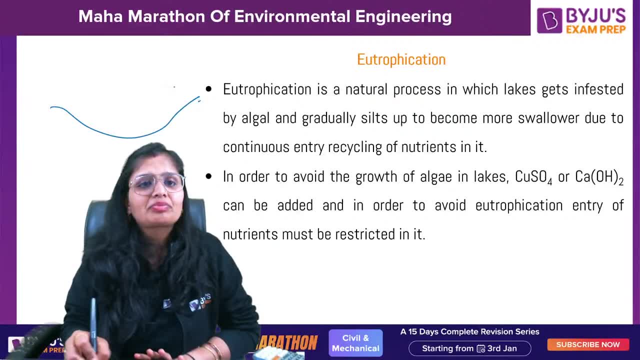 Lowest is for oligotropic. Okay, Last, second last, that is eutrophication. Eutrophication. already you know what is happening in a generally, the washing powder and oil which you use. The prime cause of eutrophication is phosphorus. 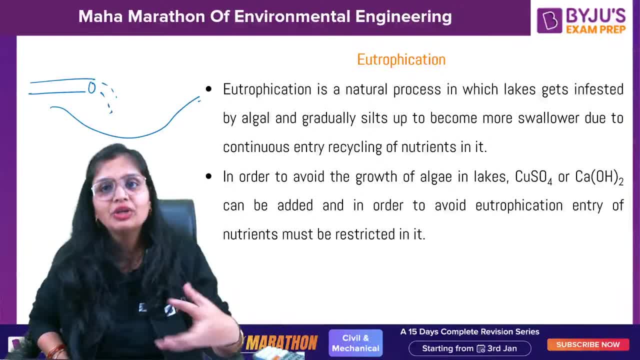 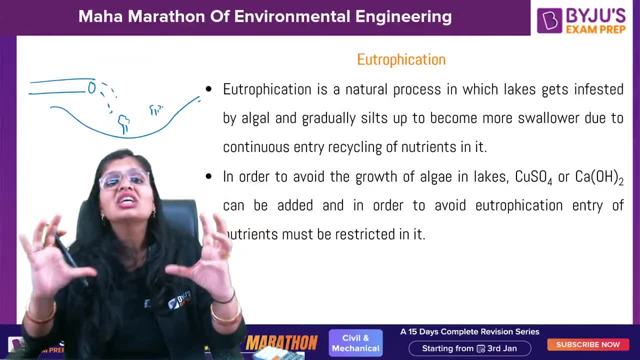 What will happen When you provide nutrients? when you provide nutrients to algae, it will grow And, moreover, if algae grows over it, the depth of water becomes shallower and shallower. Why? Because the deposition of algae is taking place. 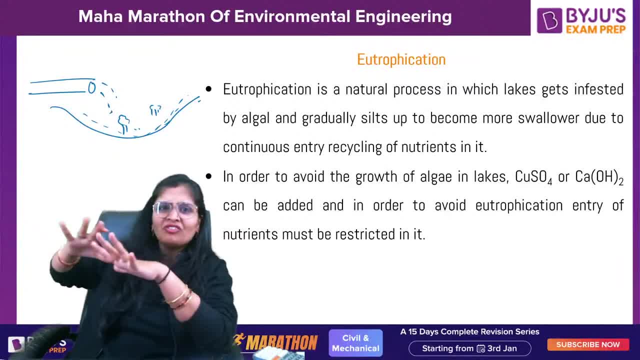 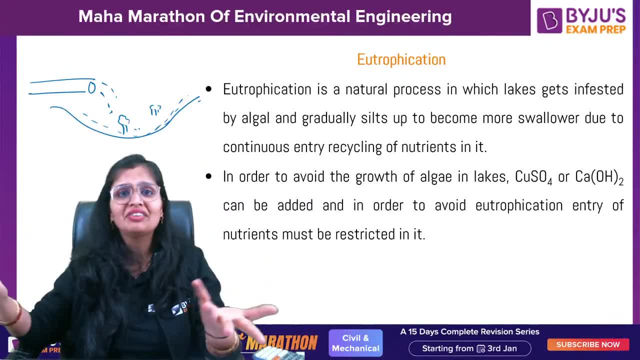 So if you see all those green type of, we say kai in Hindi. You know that Kai we say in Hindi. So there, Pura kai, jam jata, we say, Because now that lake cannot be used. Why? 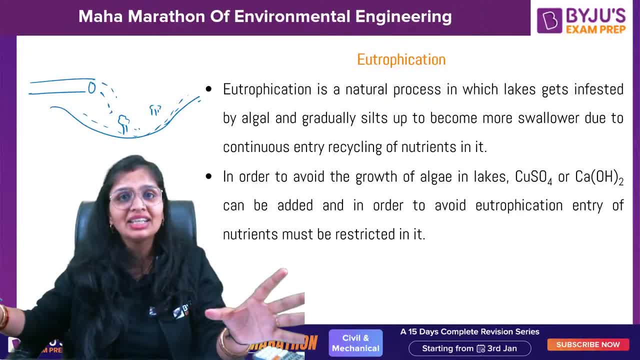 Because enough quantity of algae is present, The depth has become shallower, Okay, Specifically, the prime cause for eutrophication is phosphorus, Okay, Okay, So you guessed it. in agricultural fertilizers You get it. in the case of nitrogen, phosphorus, sulfurs. 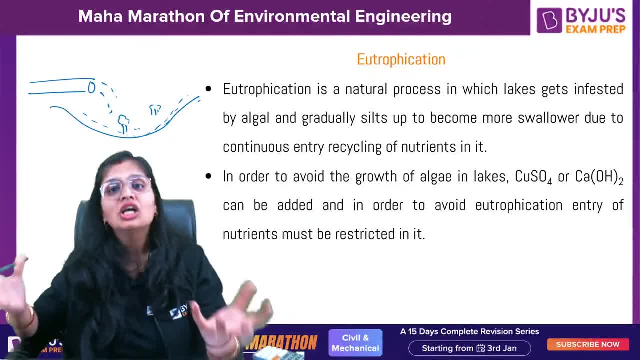 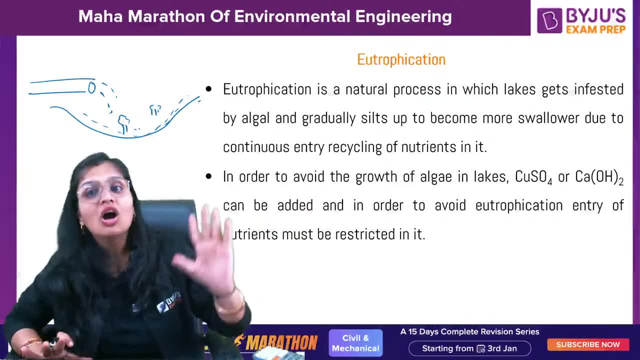 Generally phosphorus, which comes from the washing powder and detergent. So if you want to that stop. Do not add that water in which phosphorus and oil is there. Do not allow that water in lakes. Or add copper sulfate. add calcium hydroxide. 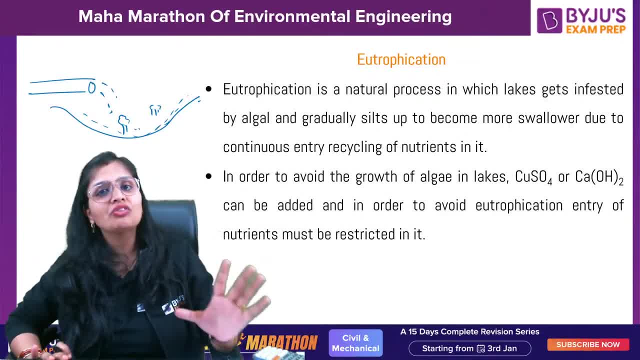 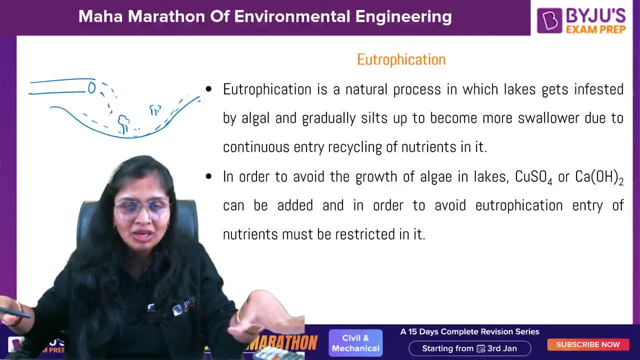 This prevents the growth of algae. Otherwise eutrophication. when excess quantity of nutrients are there, that land is full of algae, It is full of that green algal bloom comes into picture and that lake. you cannot use it for any water supply purpose or recreational purpose at all. 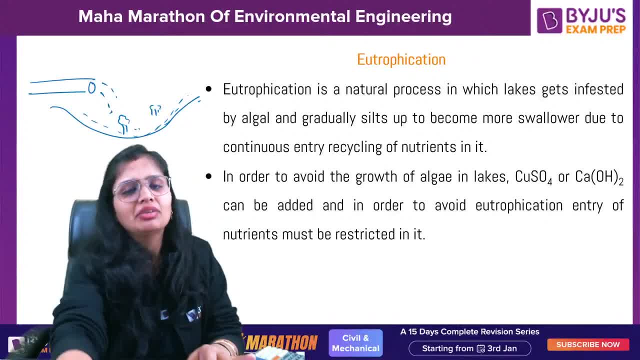 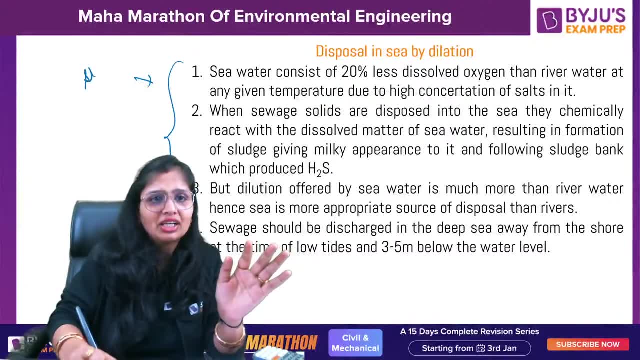 Okay, So this is it. Green, and sometimes brown, Generally green, Darkish brown, it happens. Okay, This sea statement wise, they can, if they want, they can ask you, So that's why I've written it for you. 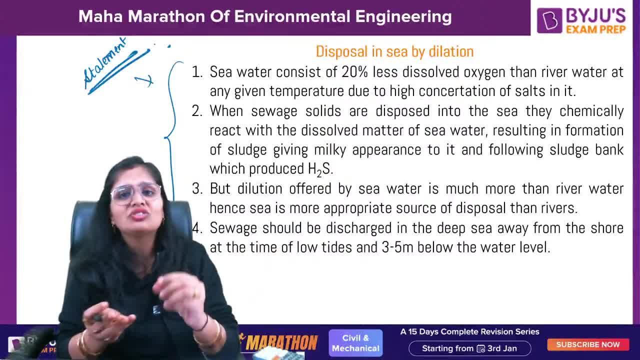 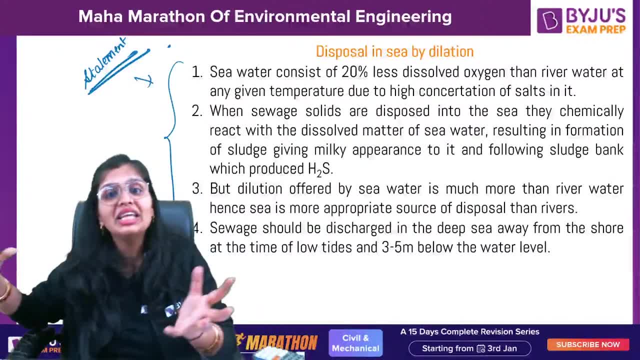 Statement wise, if they can ask you. You know sea water consists of salts, Okay. So, generally, we don't prefer salt, We prefer it. Moreover, if you throw it, it can come back. So you have to go deep. 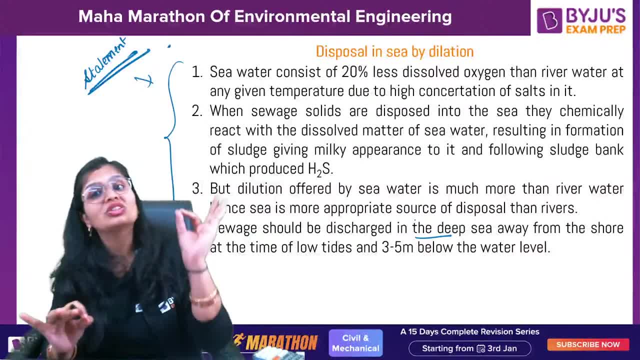 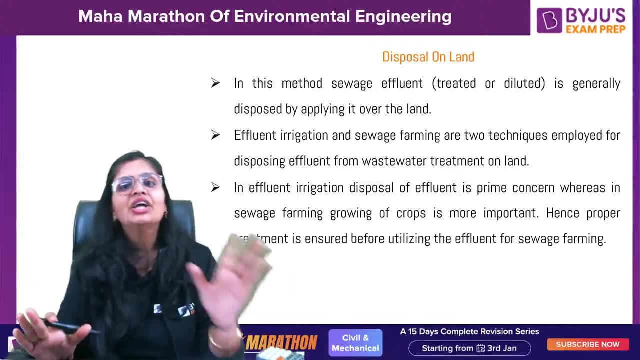 Like deep sea, you have to go it, You have to dispose it in low tide. So generally nowadays you don't dispose it into seas. No, it is not permitted Land. You know that there is a farming which is done, which is known as sewage farming. 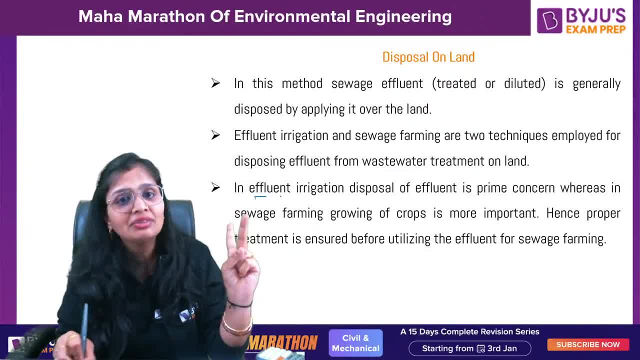 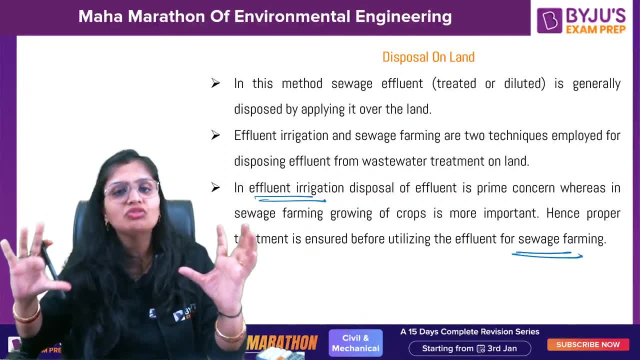 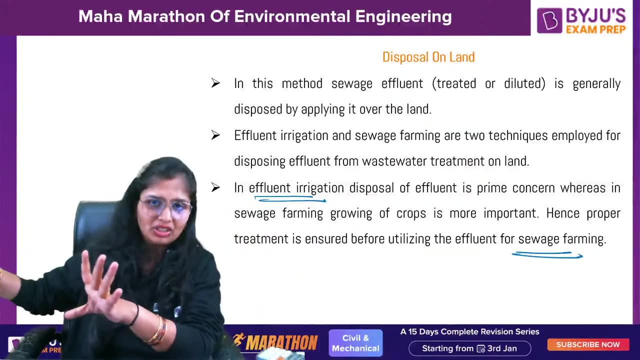 Two types of thing is there. You can go for effluent irrigation. You can go for sewage farming- Okay, Sewage farming, You are more important funders that you want to grow The crops- Okay. And when you talk about the effluent irrigation, you just want to dispose it. 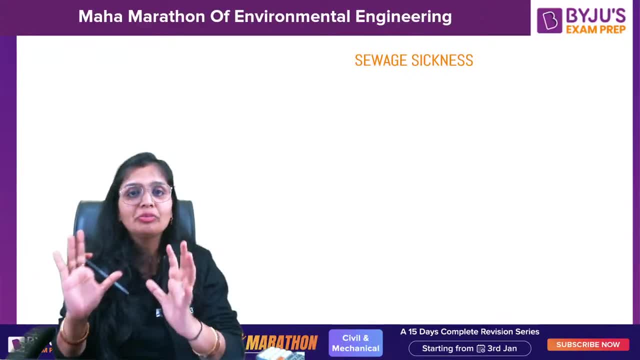 Okay, But when you are disposing it you have to make sure that there shouldn't be a condition of sewage sickness. What is sewage sickness, ma'am? What happens when you dispose the sewage? and here any filter media, any type of media, is present. 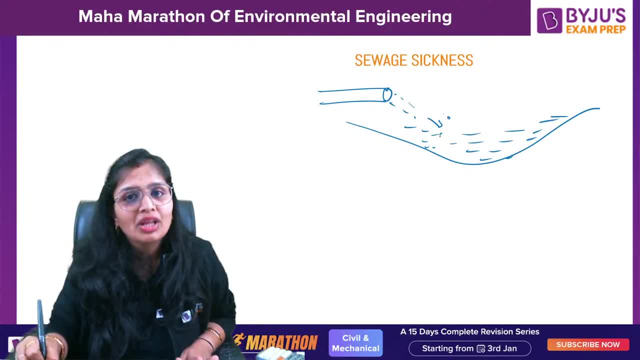 What will happen? Eventually, the sewage will have solids also, So this will clog the voids of the Filter media or any media which is material, which is present. So what will happen? The sewage has clogged the voids. 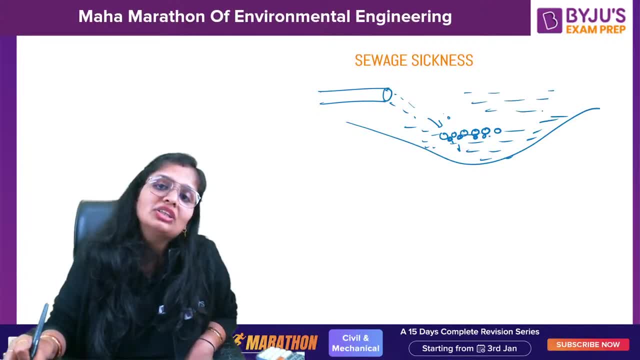 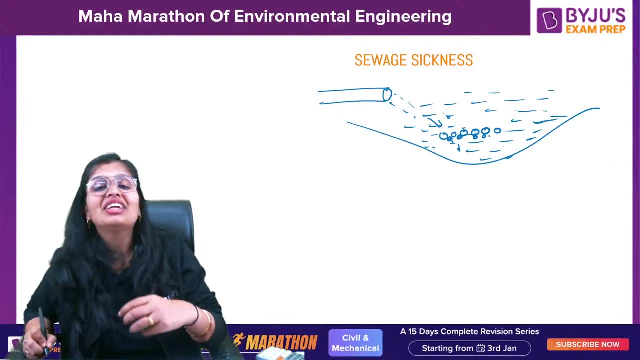 So now the sewage will not able to penetrate and it will able to stand here. So what will happen? The sewage is not able to penetrate downwards direction, It will create. it will create, you can say, unsanitary condition: H2S gas will be there. 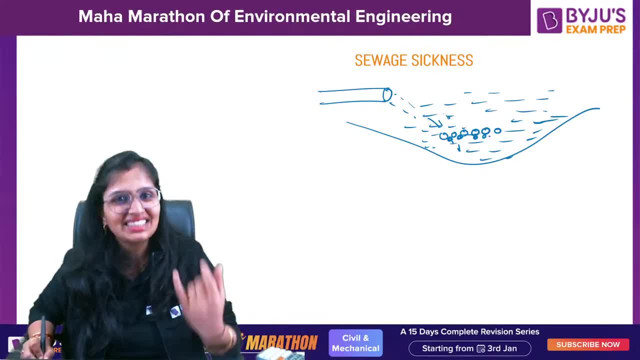 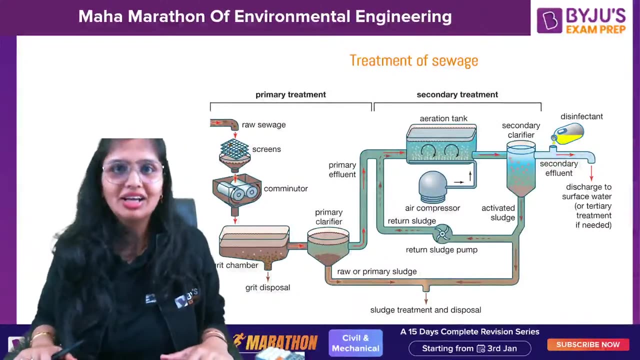 So it will create unsanitary condition or you can say it will be aesthetically displeasing at inside. So that position it is very, very difficult to stand also. So this is what is: sewage sickness Clear. Okay, so now this is the third last chapter: treatment of sewage. 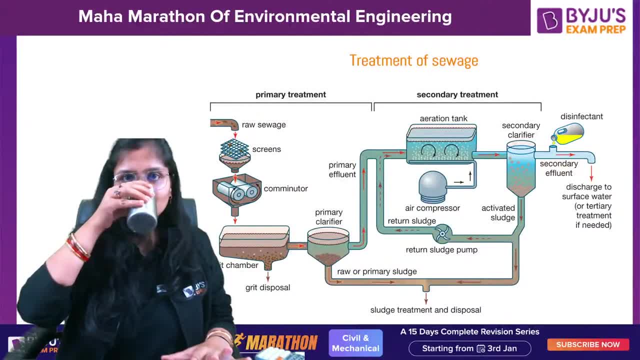 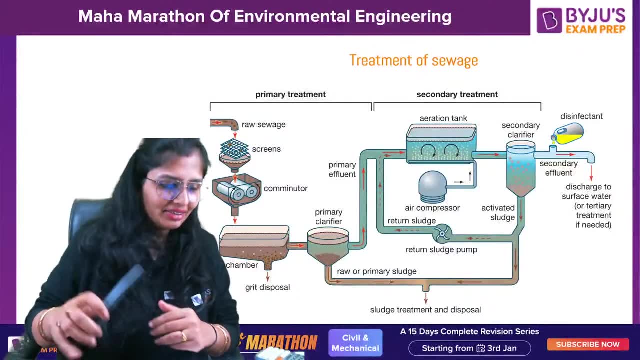 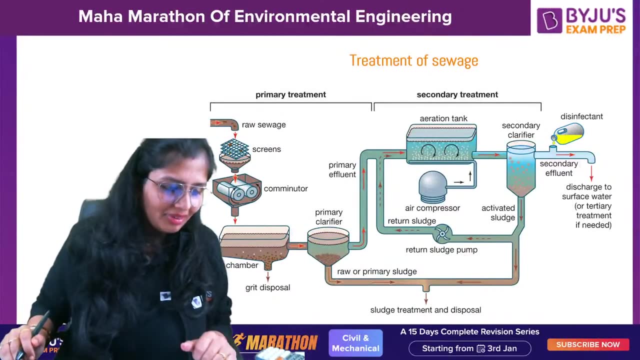 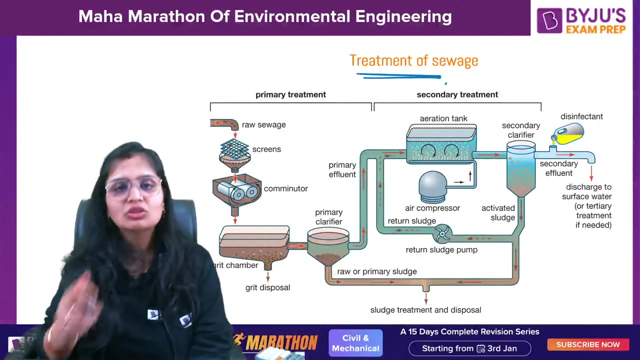 Ready, everybody Ready, After this? only air pollution and solid waste management. Okay, Okay, Fine. So let's talk about sewage treatment plant. sewage treatment plant. What is happening? What is happening? The raw sewage is there First. it is passed through the screens. 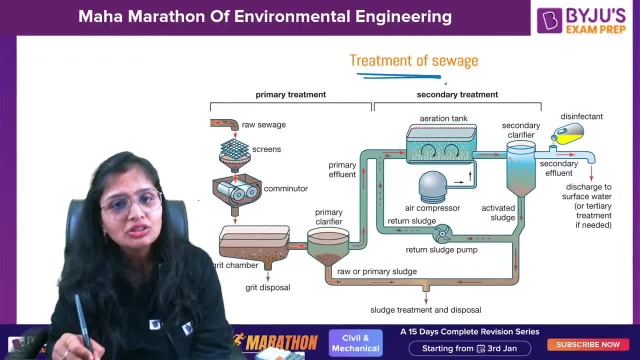 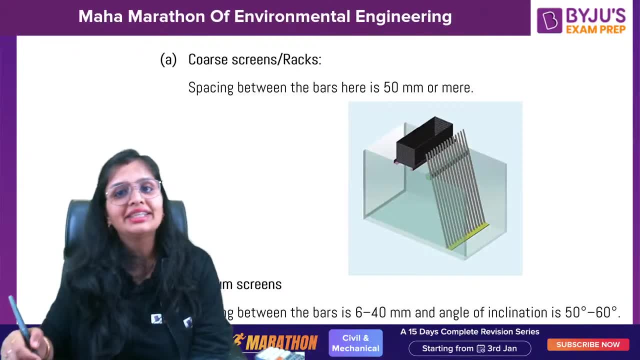 Screens remove large floating matters and all. Then it is passed through commutators, macerators. Now let's go one by one. Screening, already told you, removes large floating matter. Now see, these are the diagrams, If you haven't seen. 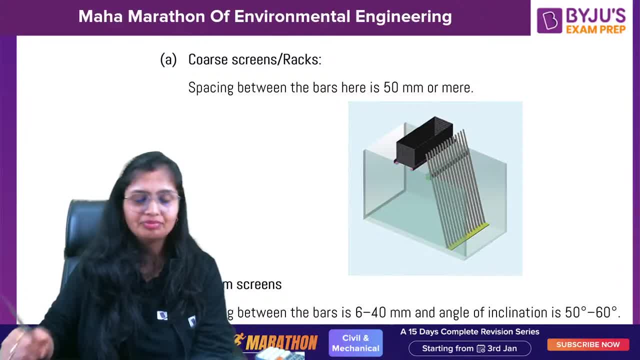 I told you that they are generally arranged in inclined manner. You guys can see it. Spacing is 50 mm more inclination. generally we keep it in the range of 30 to 60 degree Medium screens. This was not there in the case of raw water. 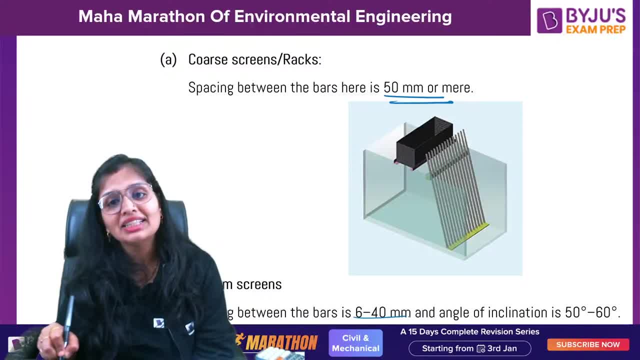 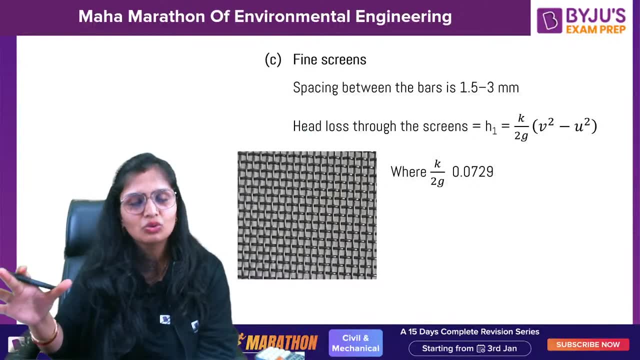 This is there for the case of waste water. So in that spacing is 6 to 40 mm, angle of inclination is 50 degree to 60 degree. Fine screens more finer than this- This is somewhat coarse medium screens- and that spacing is 1.5 to 3 mm. 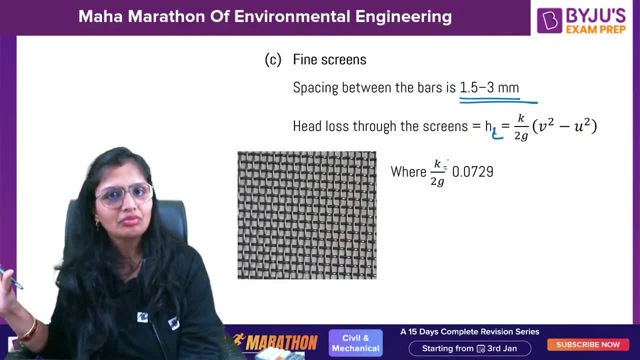 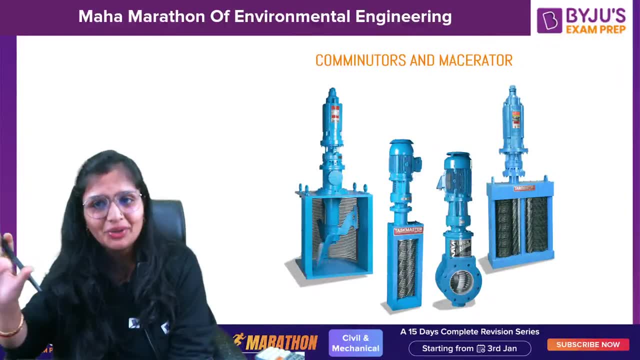 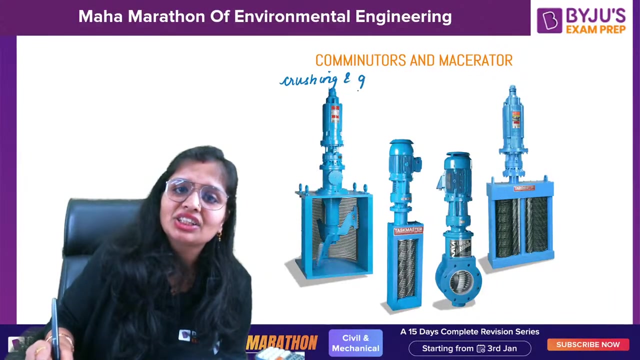 And the formula already told you. Okay, This already we have discussed. Now, coming to the next is commutators and macerators. Let me tell you, in actual, they does not perform the treatment function, They just reduce the size. Commutators is based on crushing and grinding action. 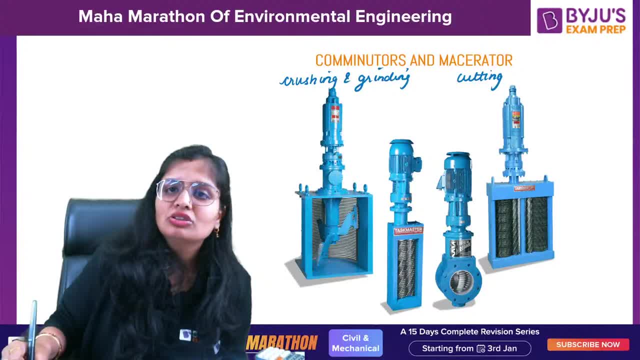 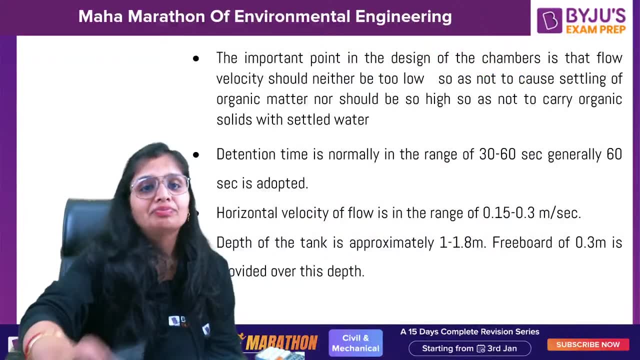 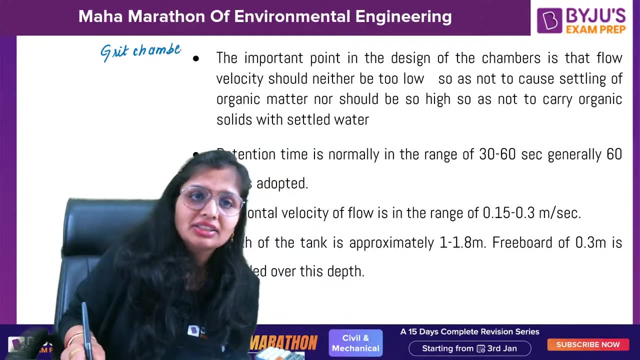 Macerators is based on cutting and tearing action, So it just reduces the size. that's it. Its function is to reduce the size. Now talking about grid chamber, The function of grid chamber. from here the thing starts. The function of grid chamber is removal of inorganic suspended solids. 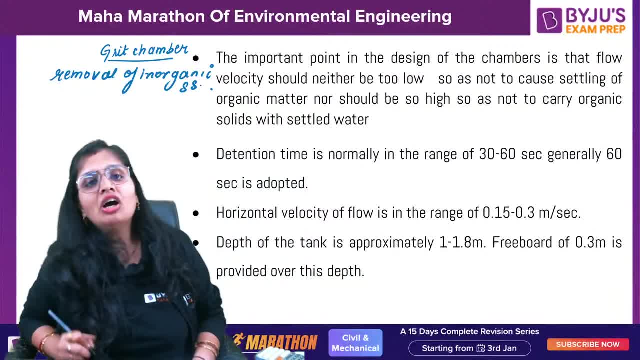 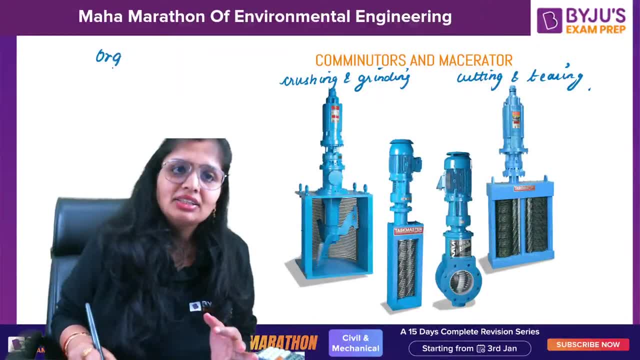 Inorganic suspended solids. Now, what happens? Now, what happens is Here we have four types of solids, basically: organic, suspended and dissolved. organic suspended and dissolved, inorganic suspended and dissolved. So, first thing, which first thing first which comes is, firstly, we removed large suspended 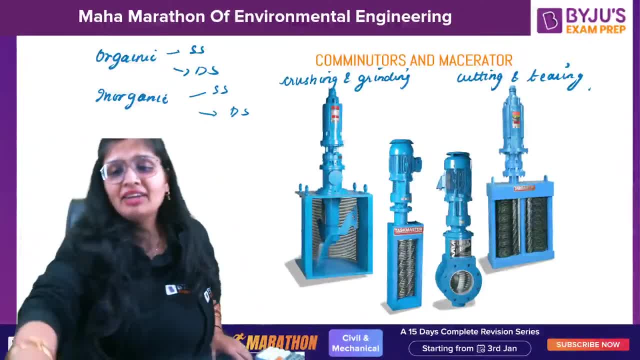 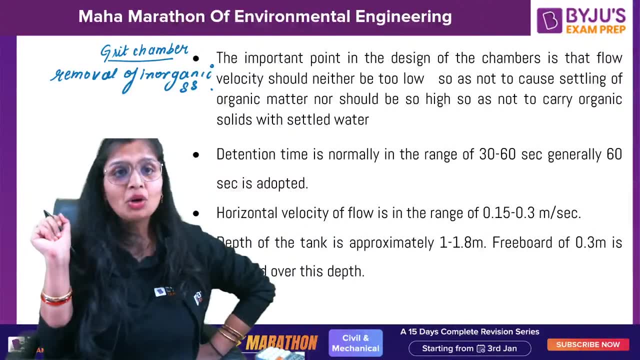 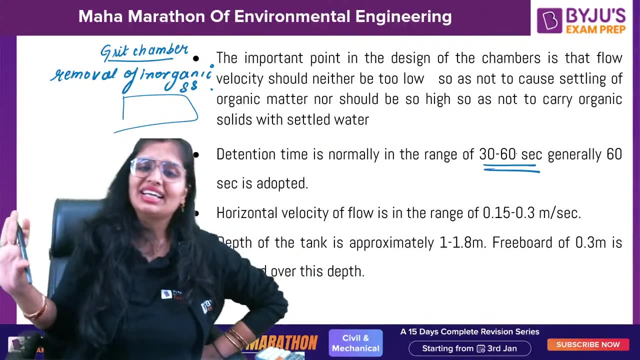 solids, floating matter in the case of screens. Then what happens when we go for grid chamber? we did the removal of inorganic suspended solids, Okay. Now, when this is a chamber, just like your sedimentation time, the thing is you keep it only for 30 to 60 seconds, that is about one minute. the velocity of flow is 0.13 to 0.3 meter per second. 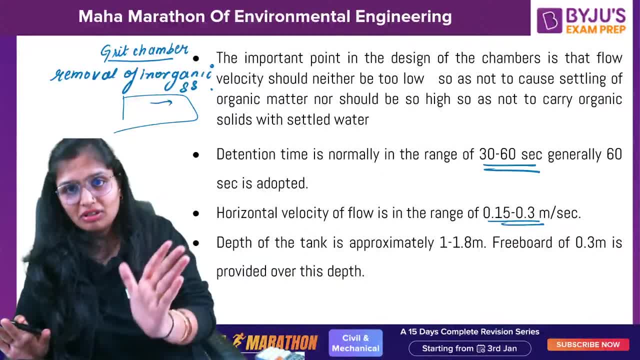 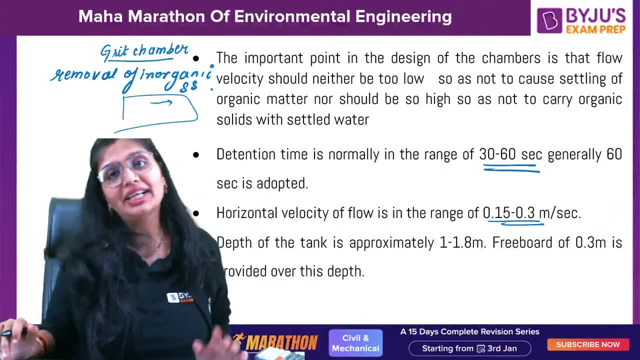 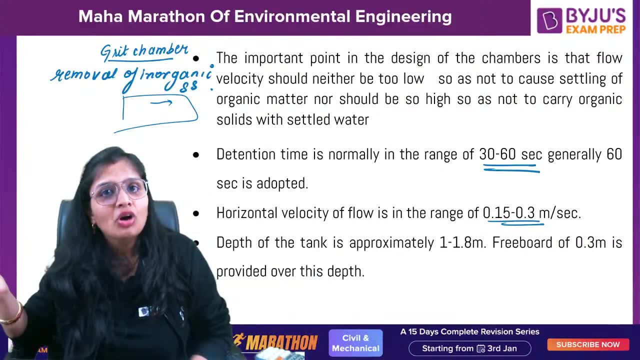 Now I will tell you in hindi. when you design the grid chamber, firstly, make sure that the length, everything is properly designed, the velocity is maintained. Why? Because if you provide more velocity, those who want to settle, they also go. Or if you provide less velocity, the organic solids will also settle out. 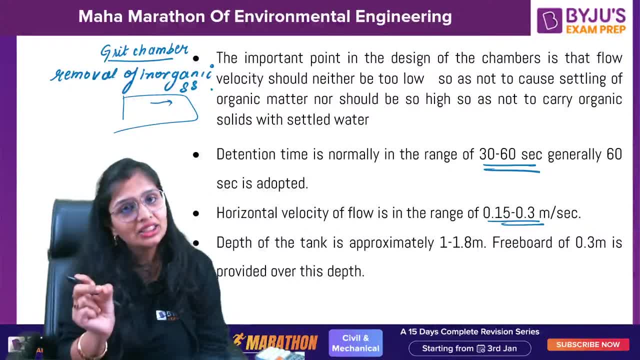 Now I will tell you in English also: If you have provided a lesser velocity, even organic suspended solids will settle. And remember: that is too much dangerous. You know why? Because we are not going to treat the impurities of grid chamber, We are just going to dispose it. 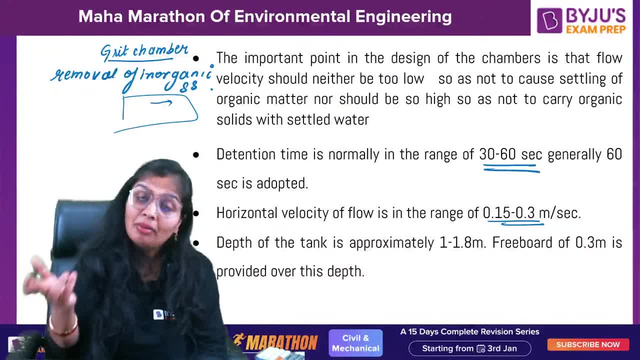 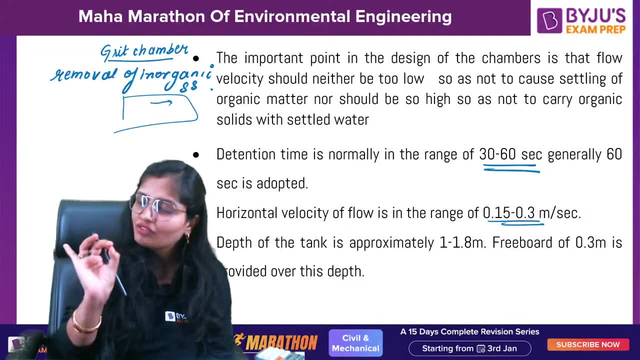 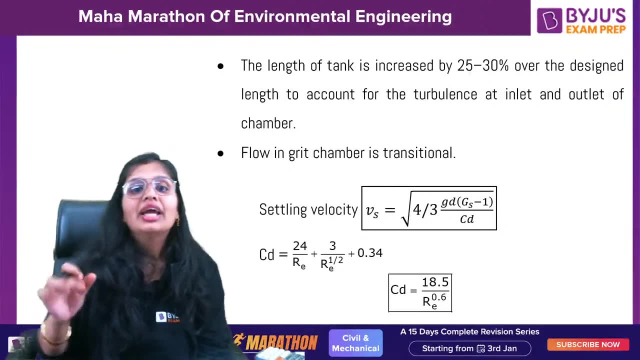 In organic sand filled particles, there is nothing to treat. But if organic gets also settled, that is a problem. Okay, So that is the reason. Here you have to maintain the velocity in such a manner that only inorganic suspended solids get settled. Now here the velocity, the flow here is transitional in nature. 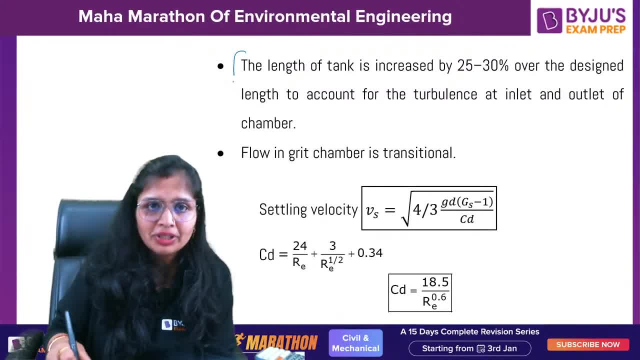 And whenever you design it. this is for designing purpose, but you should know it. The length whatsoever you design it, it should be increased to 1.25 to 1.30, because when you enter, the water enters and when the water goes out from the chamber, turbulence is there. 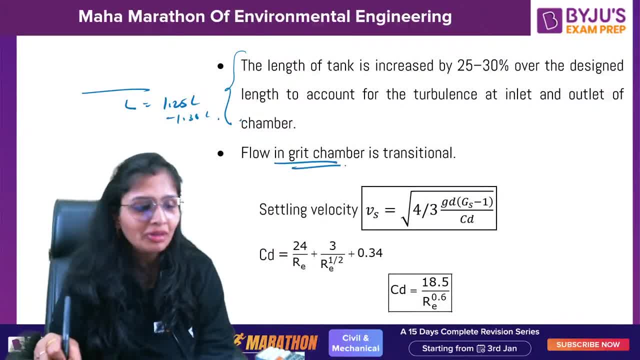 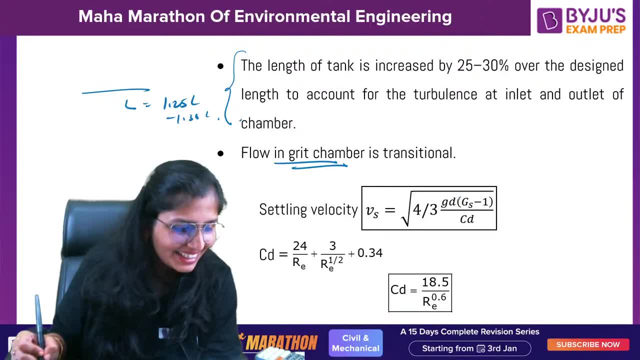 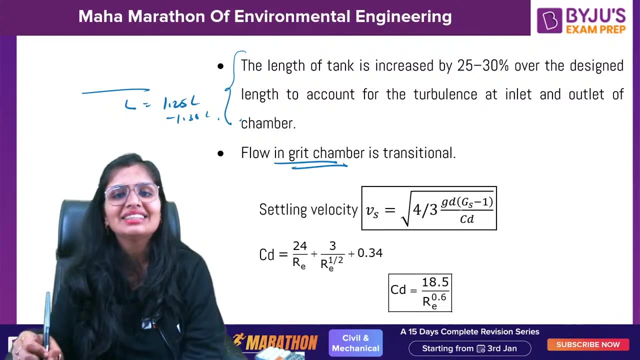 Okay, Flow in grid chamber. this is transitional in nature. Like Vamsi, you are not able to understand anything. let me know beta Settling velocity. this is the formula for the settling velocity of grid chamber. Who was asking me, Swapnil, or anybody asked me what is Ct. 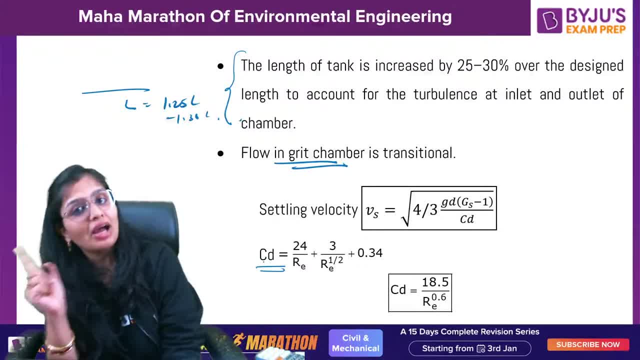 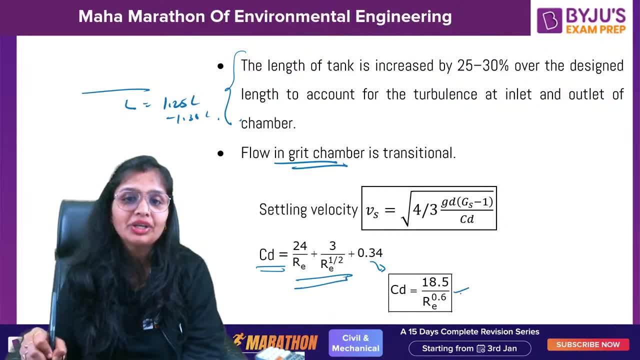 Ct is the coefficient of drag. Remember, in the case of rapid sand filter also, I told you that the flow is transitional. This is the formula And in the shortcut manner you can use this formula also: Re is Reynolds number, which is rho, Vd by mu. 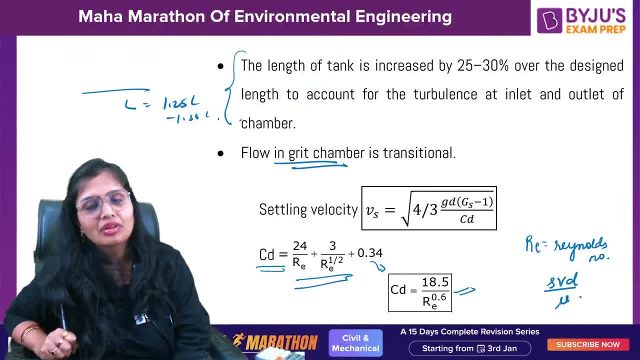 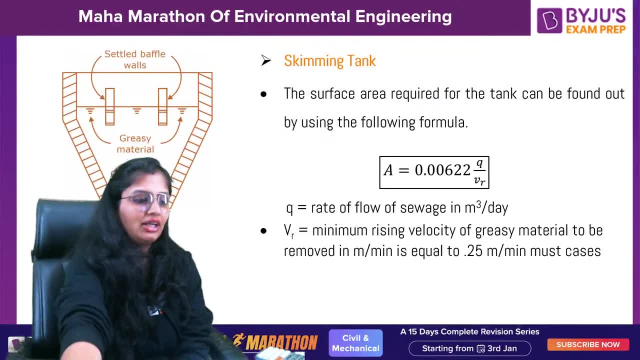 Okay, Okay. So this is the formula. Now coming next, skimming time. You were, you asked me, or what Vamsi? Okay, Okay, Now you understand what is Cd. Now you understood what is Cd. Okay, Now skimming time. 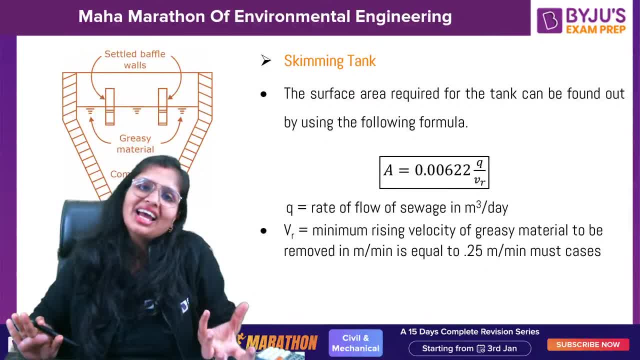 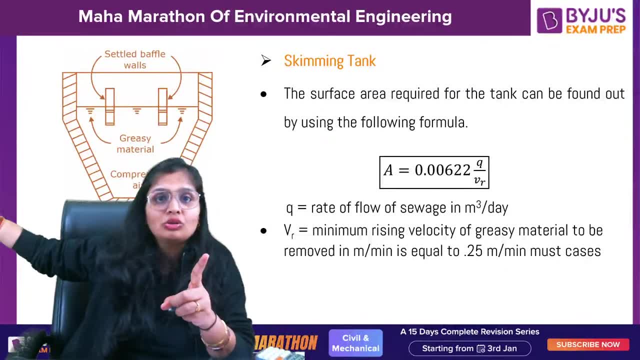 Whenever, oil and grease particles from the motor garages, restaurants, if they are there and you don't treat it, What will happen is if you go that water to trickling filter and all they will interfere with the treatment operation. That is the reason: remove it first. 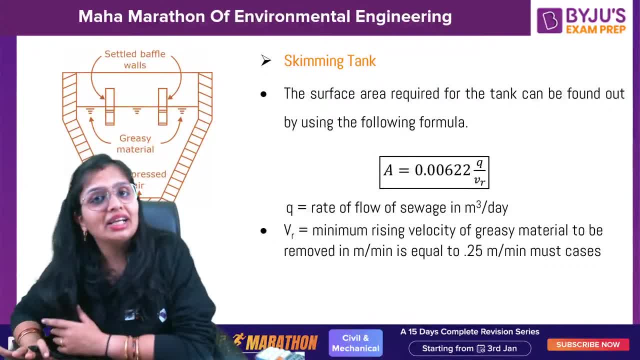 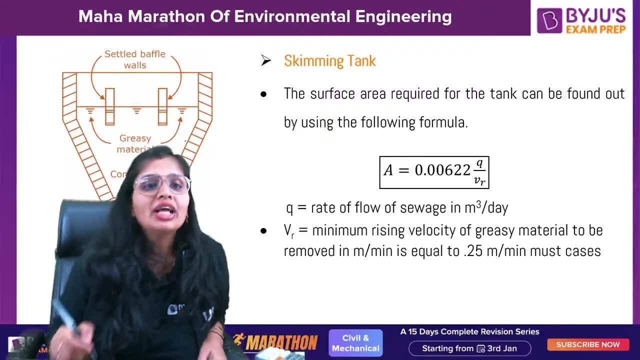 Why? Because if oil and grease particle are there, it will inhibit the growth of the water. Okay, It will inhibit the growth of microorganisms, So treatment will not be complete. Okay, So what happens is oil and grease particles are there. You supply compressed air from the water. 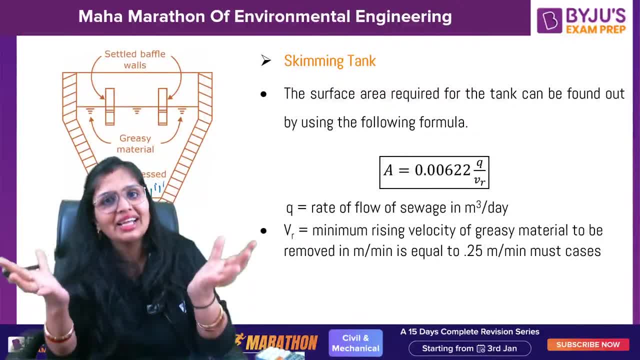 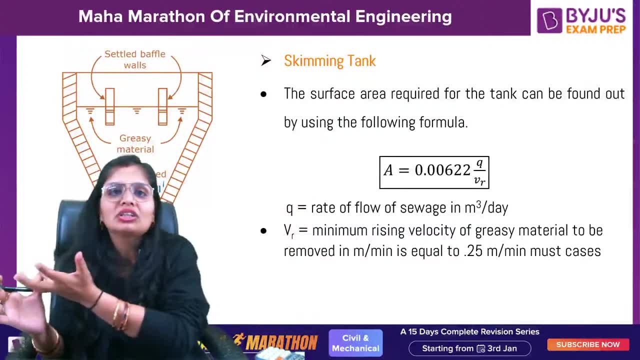 So oil and grease particles will be lifted up and, like from the milk, you remove the what you call skimmed milk, You skim up the milk on the top. So in that manner, only what you do, You skim up the oil and greasy particles. 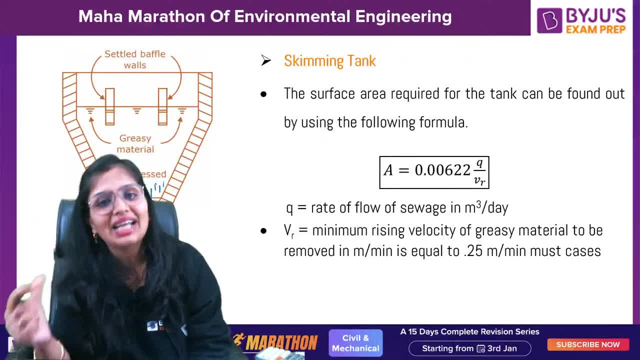 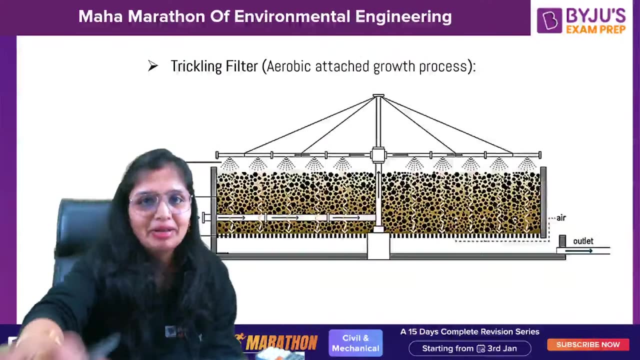 That's why it's name is skimming time, and how much area to be there. that is being given by this formula. This is the empirical in nature, Q is the rate of flow and VR is the minimum rising velocity. Okay, So this is the skimming tank. 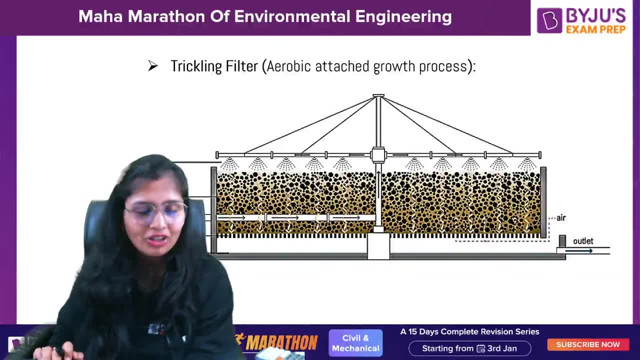 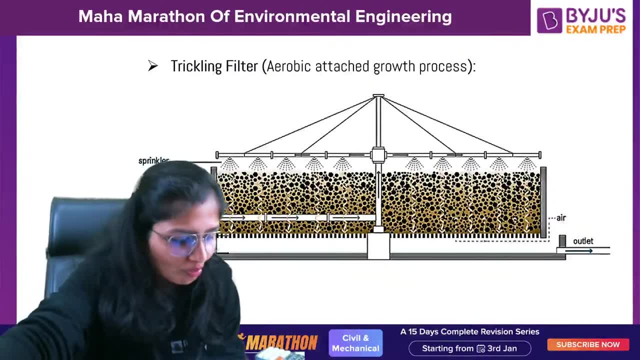 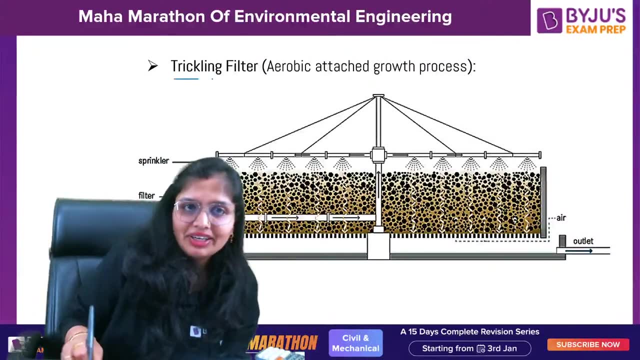 Everybody needs a break, or what? Well, let's do it. Okay, Okay, Okay, Okay, Okay, Okay. Tell me Yes or no, Otherwise we will start trickling filter. Okay, Let's do, Tell me. 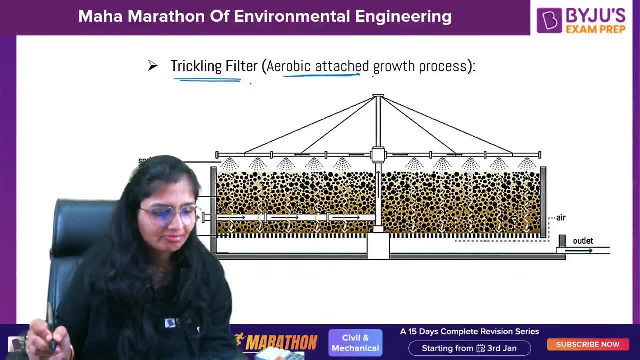 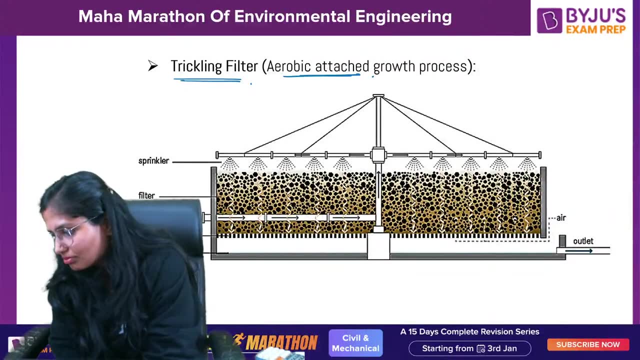 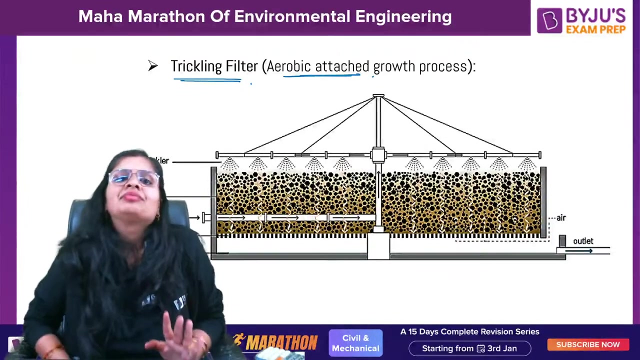 Yes or no, First vom says about now Everybody Tell me you need a break or what, raising ourψ trickling filter ke baad. okay, fine, fine, let us complete. trickling filter prashant. okay, trickling filter is based on aerobic attached growth process. aerobic means microorganisms will. 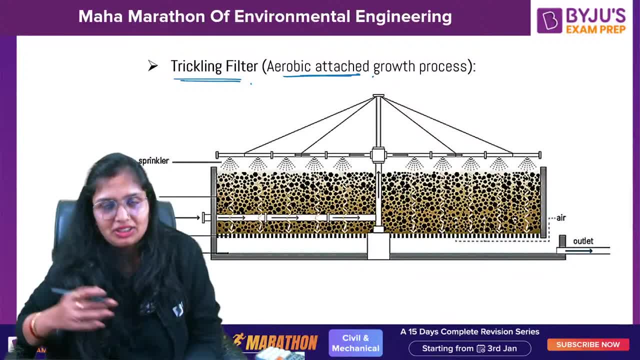 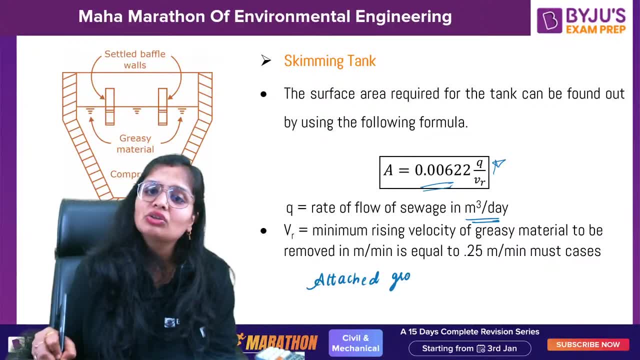 utilize oxygen, aerobic microorganisms will be functional. now there are two things: one is attached growth process and the other one is suspended growth process. attached growth process: you give the medium for the microorganisms. okay, you give a medium for the attachment of microorganisms. since you have given a medium, this is attached growth process, suspended growth. 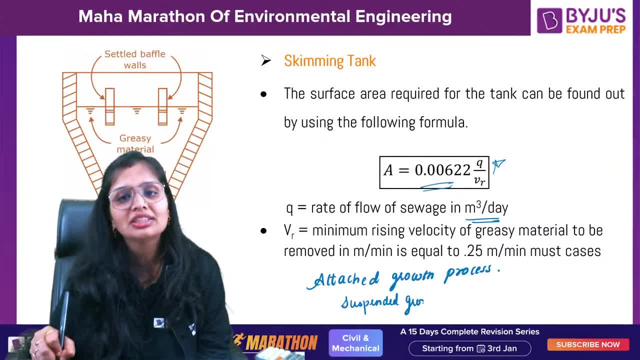 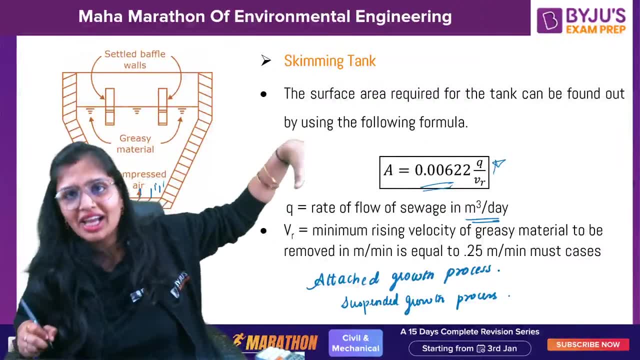 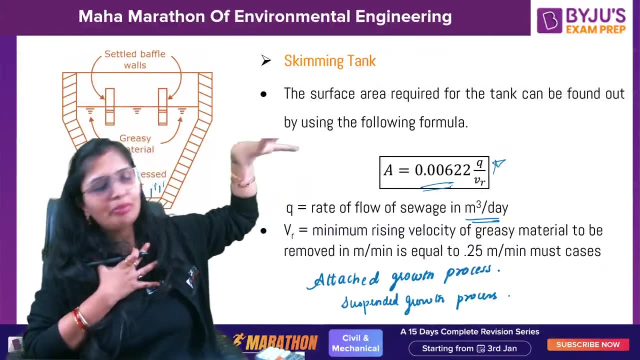 process is organic matter and microorganisms. both are in suspension. like you might have gone to the party, there is a waiter with a starter and you are there. let us suppose the starter is paneer pakoda and you are there. you are a microorganisms and that paneer pakoda. 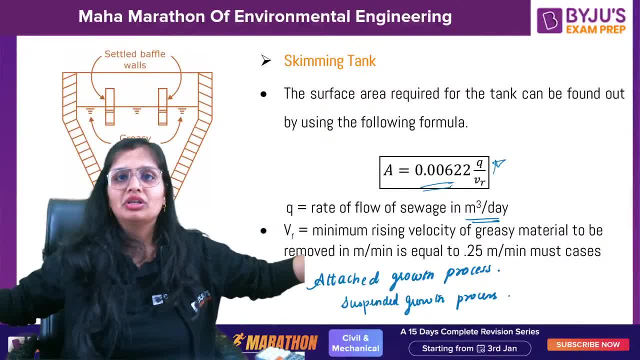 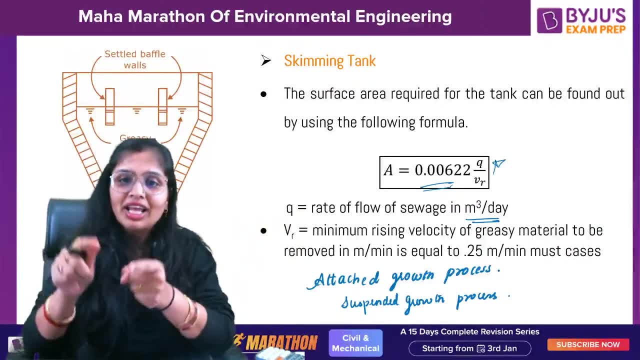 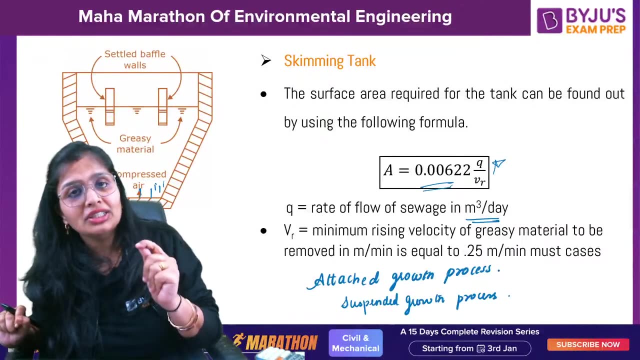 is an organic matter, the party is the waste water. so you are also moving means microorganisms is moving. paneer pakoda is also moving. that means organic matter is moving. that is suspended growth process. if i talk about attached growth process in attached growth process, what is? 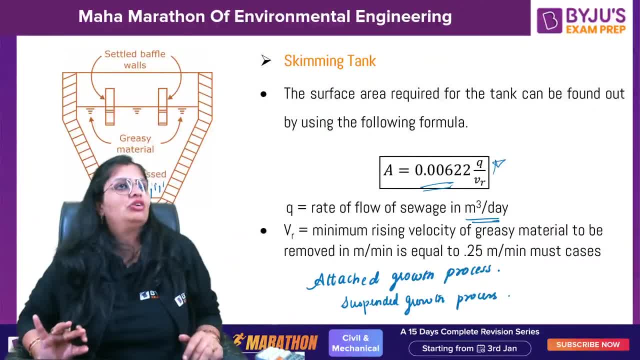 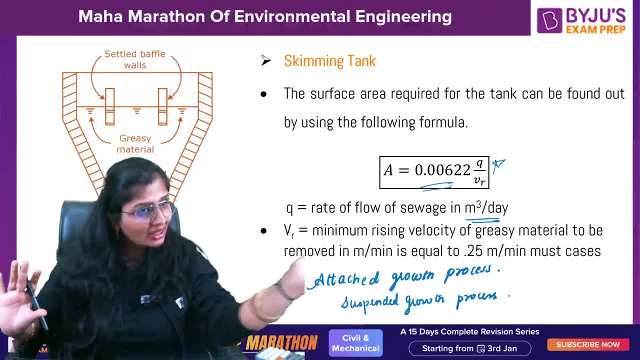 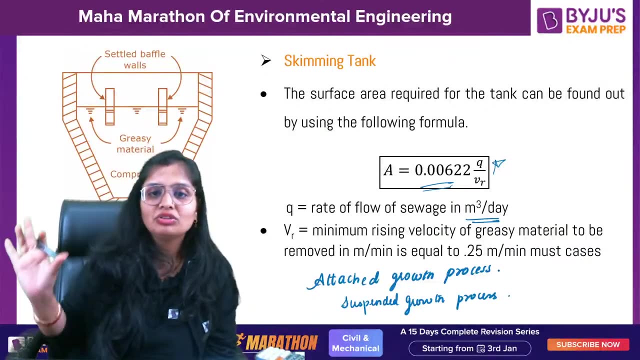 happening. you went to the restaurant. you are the microorganisms. you are basically. you are the microorganisms. you are sitting, a medium is provided to you and the organic matter will come to you. so that is attached growth process. now i guess you guys won't get confused in attached growth and 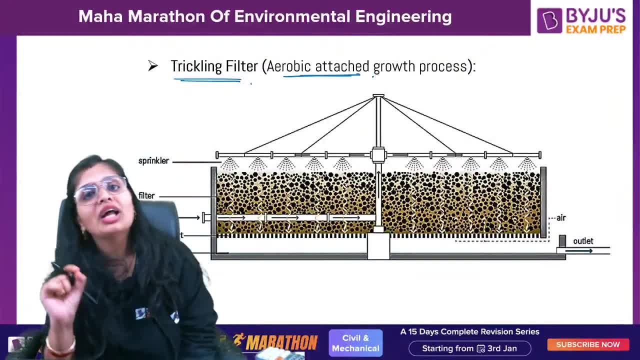 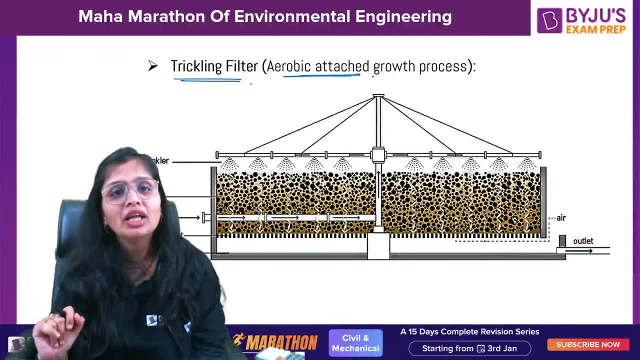 suspended growth process. so when i talk about attached growth process here, i give a medium for trickling filter. okay, now, now what will happen here? these are the filter media. make sure they are clean. they have a high compressive strength, they don't go wear and tear. okay, their durability should be high. these all things you. 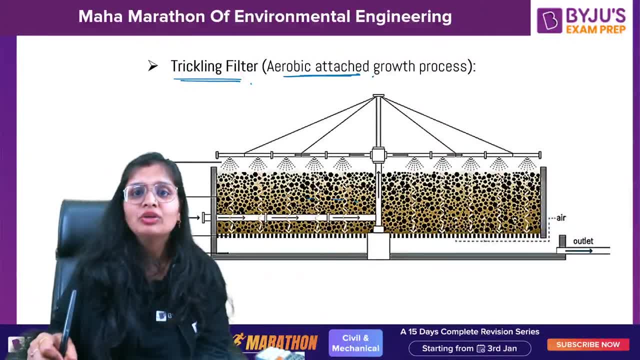 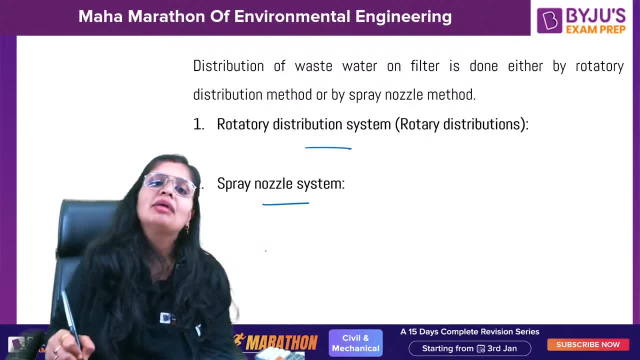 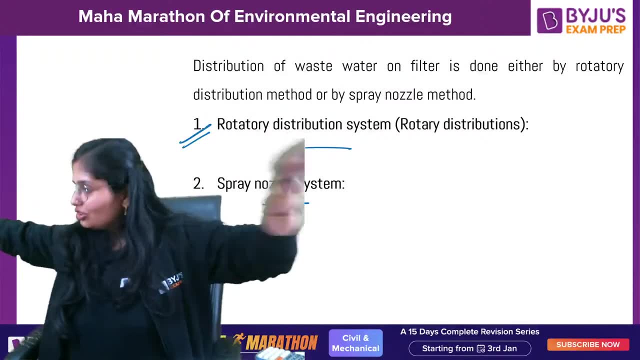 should know now when this method? generally, when you discharge the sewage, there are two methods. one is spray nozzle, another one is rotary distribution. ma'am, what we prefer. we prefer rotary distribution. if i am the basic truss here and here, so here is there. so it is rotating like. 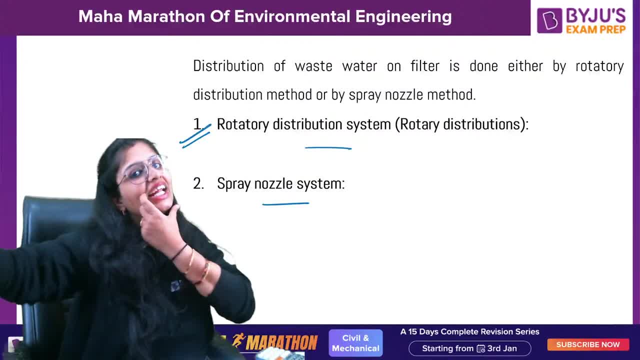 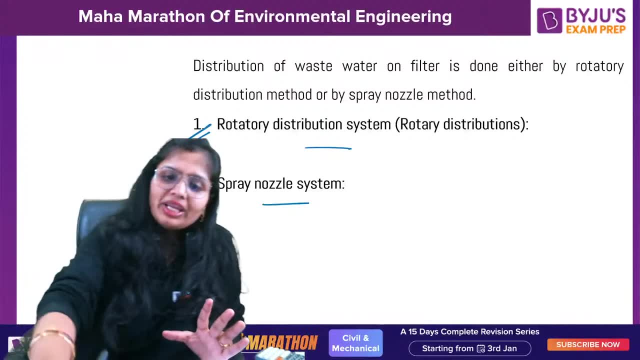 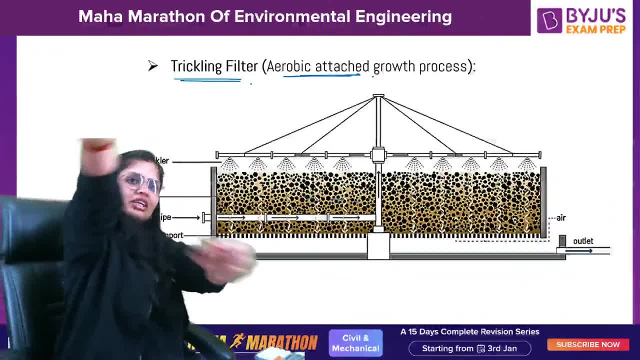 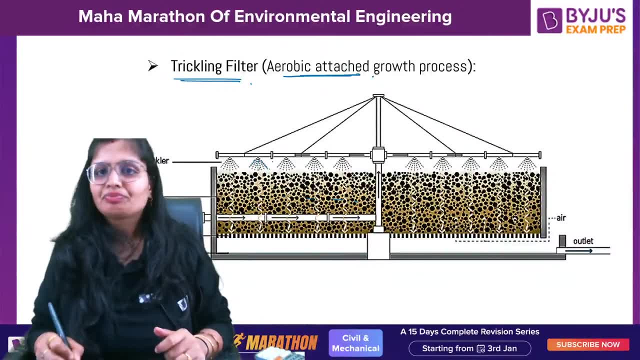 opt for it. okay, see, i am the truss here. holes are there, so it's moving. it's moving like this, okay, so what will happen? this feed pipe is there and it is discharged, it is open to the atmosphere. now, what will happen? now, what will happen? 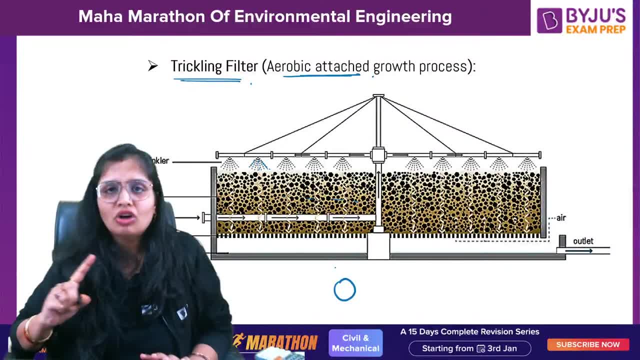 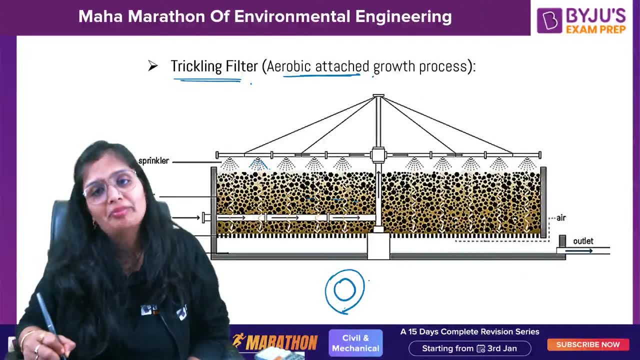 take one particle. so initially it is not an operation. first you give time for the biomass layer to be formed. you give time for the biomass layer to be formed. the moment, the biomass layer, biomass layer, is that layer. okay, firstly you give time for the biomass layer to be formed. 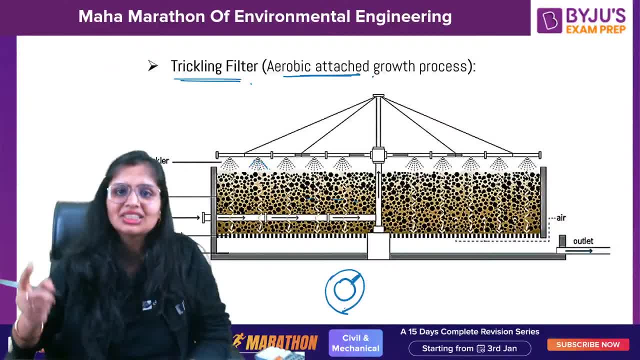 biomass layer, how it is formed. what it is biomass layer? what happens? initially the water was coming, okay, the waste water was trickling through the filter media. so they consist of sticky deposits of organic matter. so they get sticked to this filter media so a certain amount of biomass layer is stick. the filter is ready for operation now. initially, 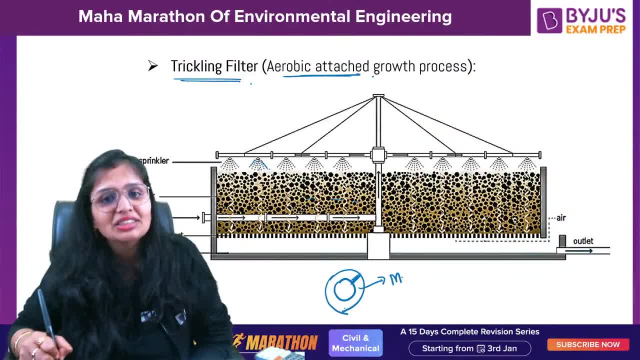 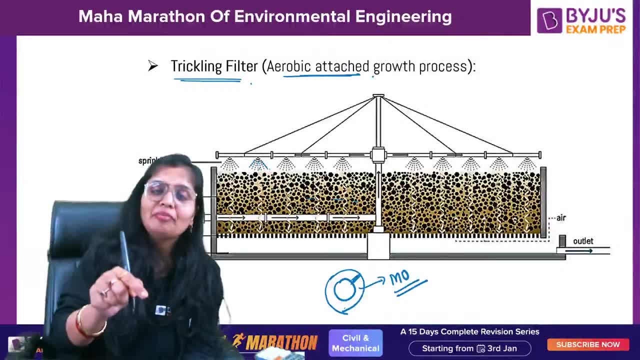 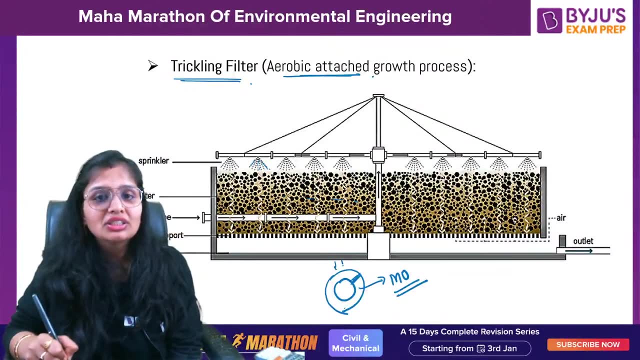 biomass layer means what biomass layer means: it has microorganisms. so whenever i say biomass layer, it means microorganisms is there. here you have provided a medium for the attachment of biomass. Next, coming further, when the wastewater trickles through this. in this wastewater, organic matter is there. 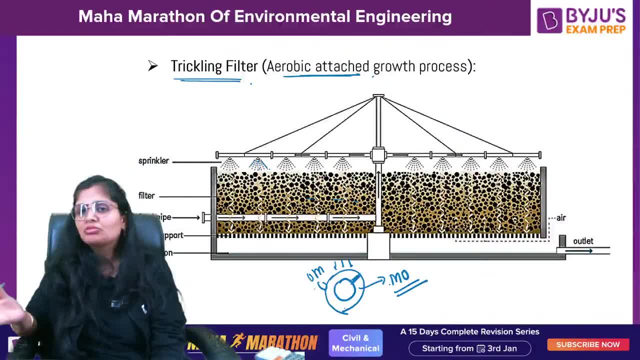 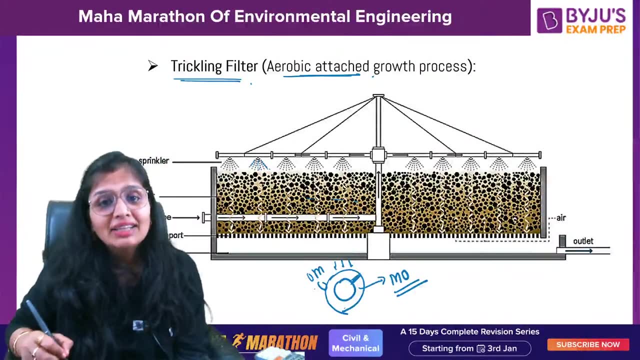 So organic matter will come in contact with microorganisms. Microorganisms, in the presence of oxygen, will carry out the decomposition of biodegradable organic matter. Now, the thing which comes out to be next, Now, the next thing which comes out to be is that in this process, when organic matter is decomposed, it also lies here. 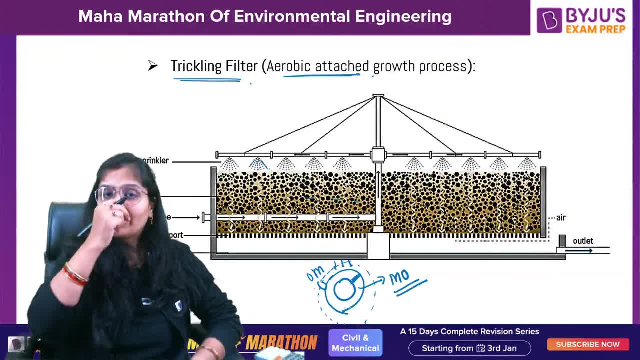 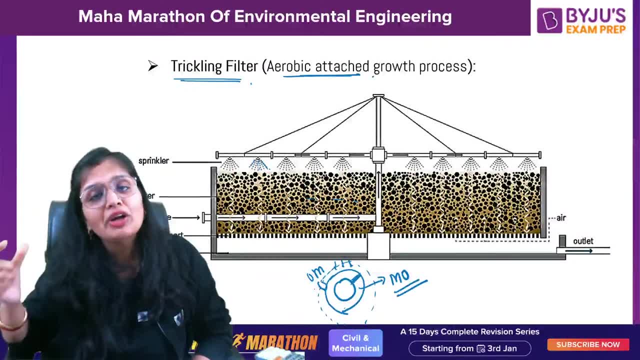 So the thickness increases. Now the microorganisms will rapidly go cell division 2 to 4, 4 to 8, and so on and so on. So the thickness of biomass layer goes on increasing The thickness. this is the particle filter, media particle- and the thickness increases. 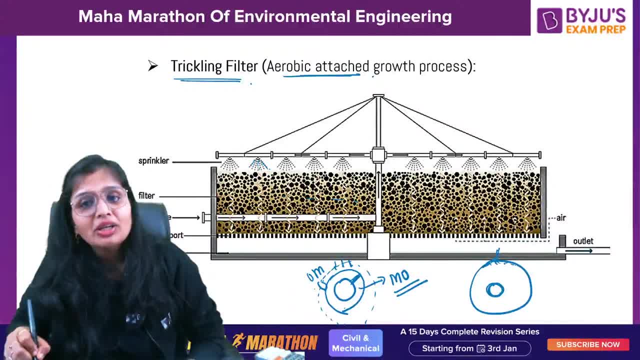 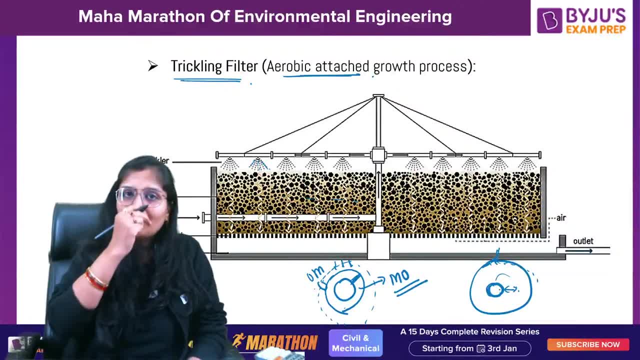 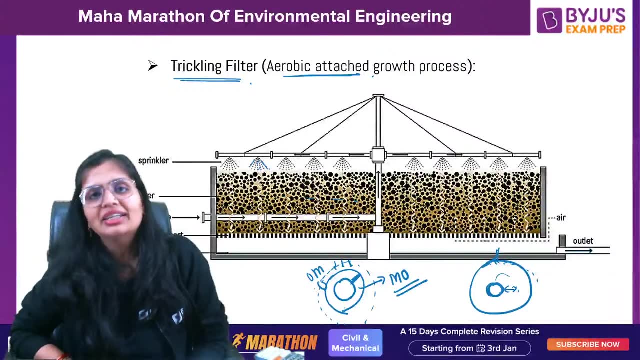 If the thickness increases, oxygen is limited only to the upper part and it is not able to penetrate to this portion. So the place where it is not able to penetrate, their anaerobic decomposition will take place, And the place where you can see oxygen is able to penetrate, their aerobic decomposition will take place. 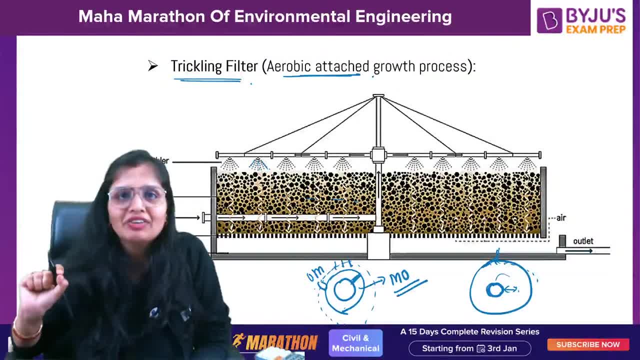 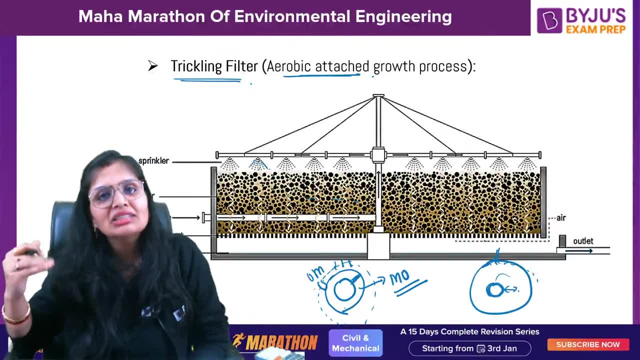 Generally, the whole thickness of biomass layer varies from 0.1 mm to 2 mm. The oxygen penetration is 0.1 mm to 0.3 mm. Okay, so maximum part of it will go anaerobic decomposition. Now the dead cell mass, those microorganisms which will not get food. they will die. 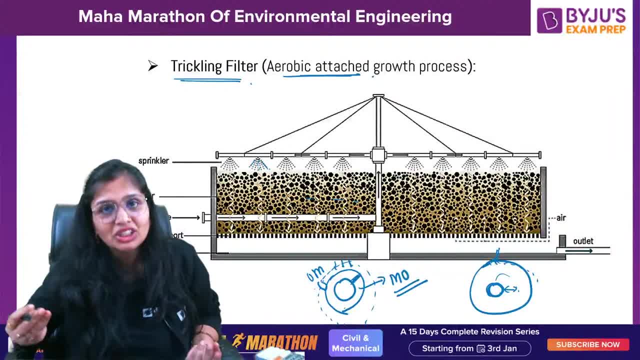 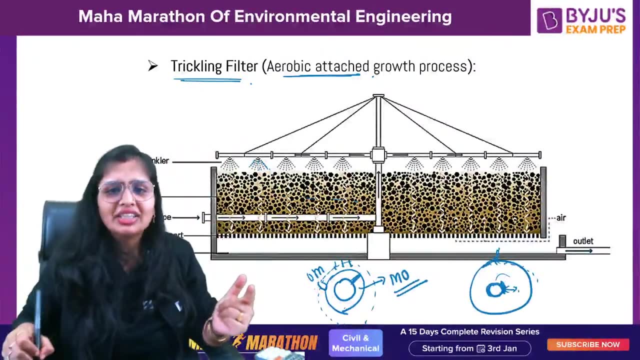 When they will die. that means they will undergo endogenous respiration And the dead cell mass are not sticky in nature. So what will happen here? the stickiness is gone, Okay, so the detachment takes place. So when the water comes now, heavy turbulence is created and this biomass layer wears off. 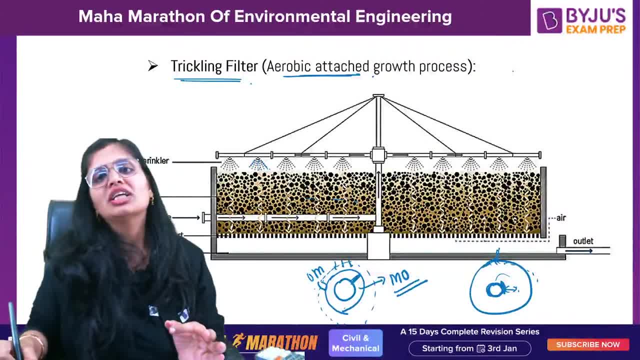 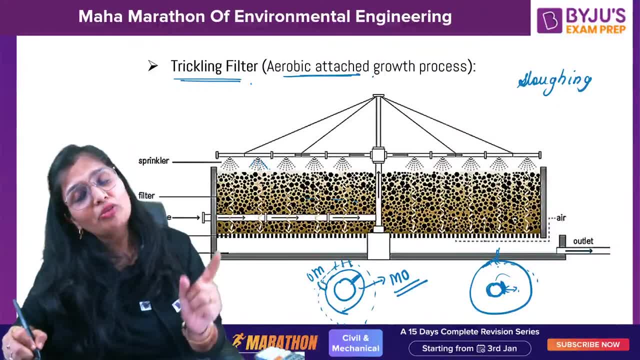 It is taken off And the process is known as slogging. So, ma'am, there are n number of filter media particles. Thus biomass layer is removed For all the particles At a single time. no better, It is a continuous process. 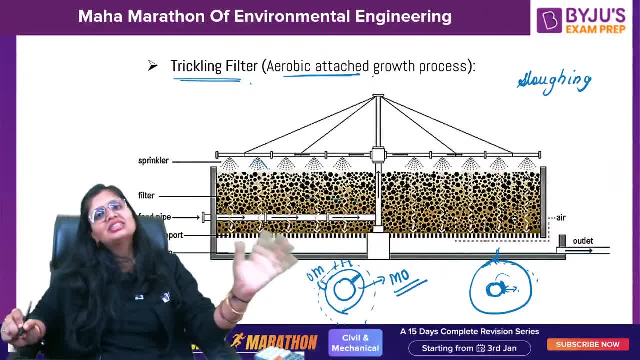 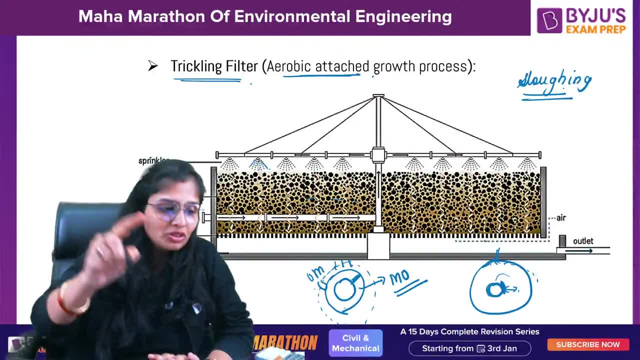 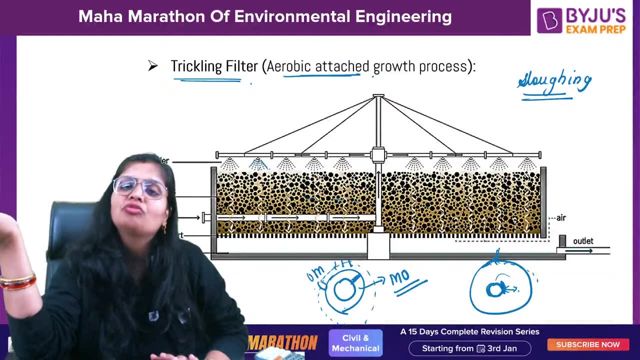 In some media particles layer was formed, In some it is removed. So it is a continuous process which goes on. Okay, so this is known as slogging. This process is known as slogging Understood. First, you gave time for the attachment of microorganisms. 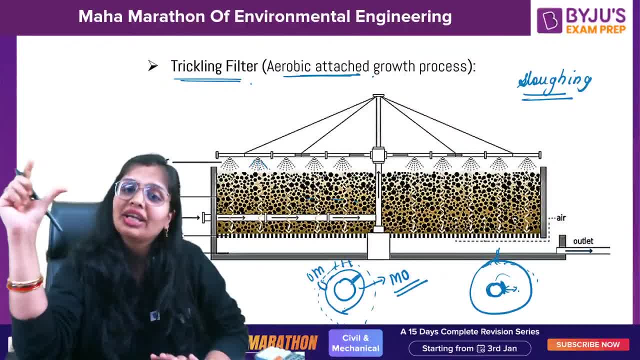 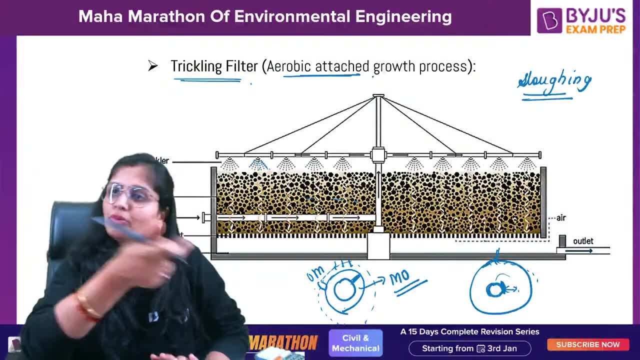 Then you operated the filter, Then the thickness goes on increasing Those microorganisms which does not got food, they go into endogenous respiration. Water came turbulence, they wear off And this biomass layer will get settled in the secondary sedimentation. 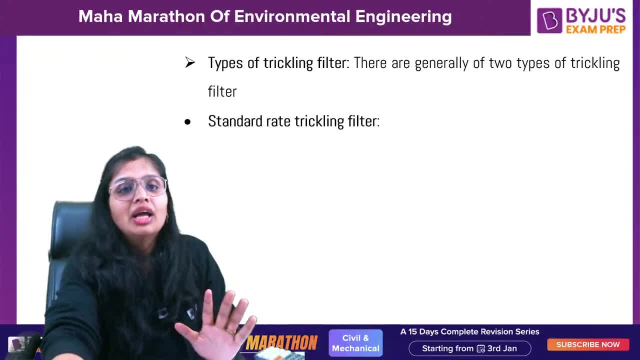 Okay Now. now we have two types of trickling filter. First is standard rate trickling filter. Standard rate trickling filter. Now, if you talk about standard rate trickling filter here, you can say the recirculation is not there. 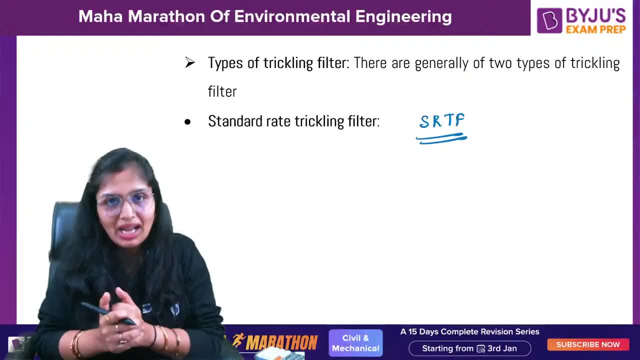 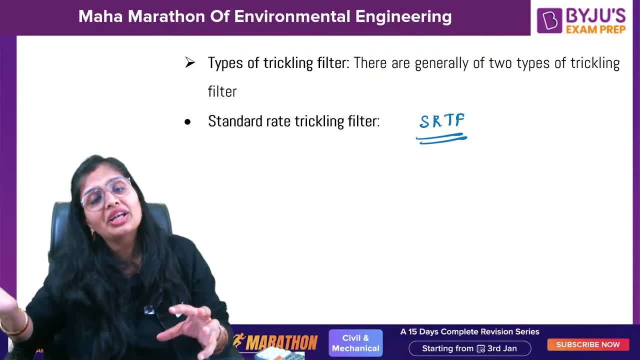 You do not recirculate the sewage back. In case you want to recirculate the sewage back In case of high, or you can say the percentage rate of removal, it takes more time to do the removal of organic matter. While you can see this also, 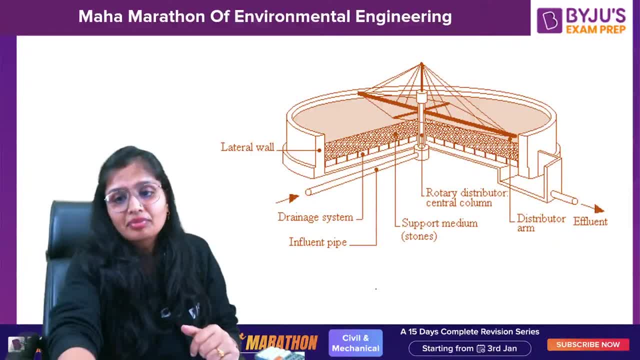 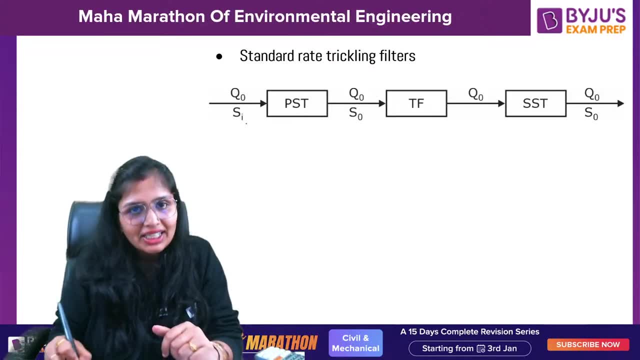 This is how the trickling filter works. Okay, Where it is high rate trickling filter, This is standard rate trickling filter. That is primary sedimentation tank. This is BOD Influent BOD to PST Influent BOD to trickling filter. 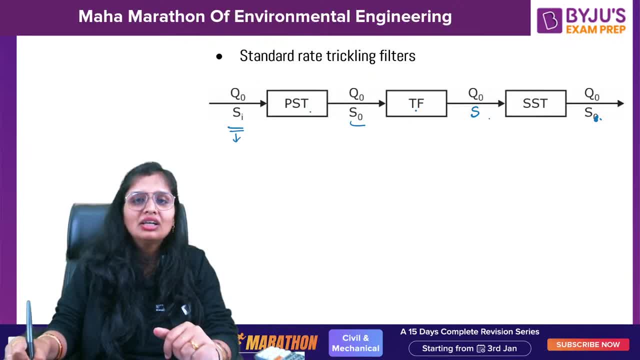 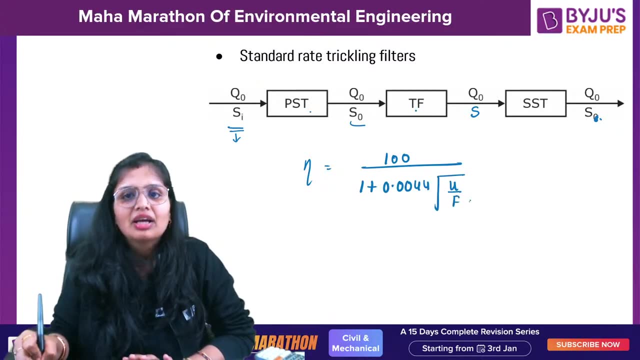 And this is the BOD From the trickling filter. So here you are not doing any recirculation. So the efficiency of it is calculated by the formula 1 plus 0.0044 U by F. Okay, 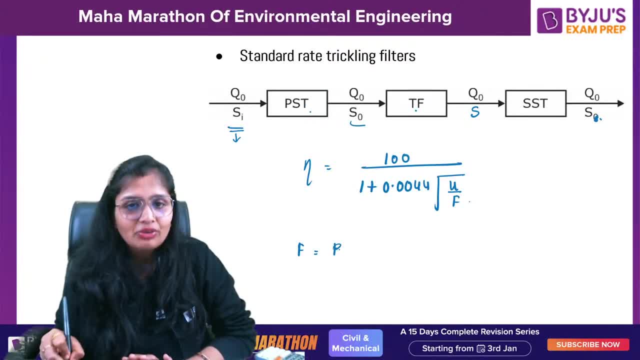 Now F. here is F. let me tell you: F is recirculation factor. Okay, And that is 1 plus R upon 1 plus 0.0044 U by F. Okay, And that is 1 plus R upon 1 plus 0.0044 U by F. 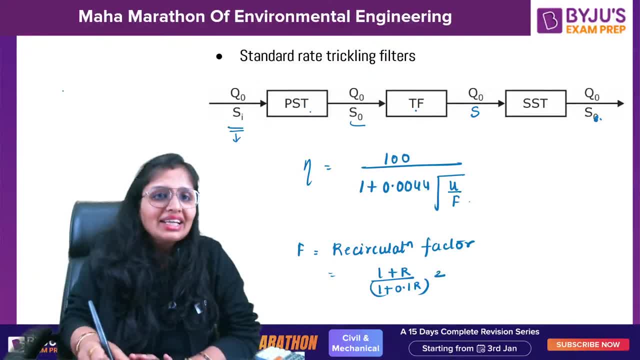 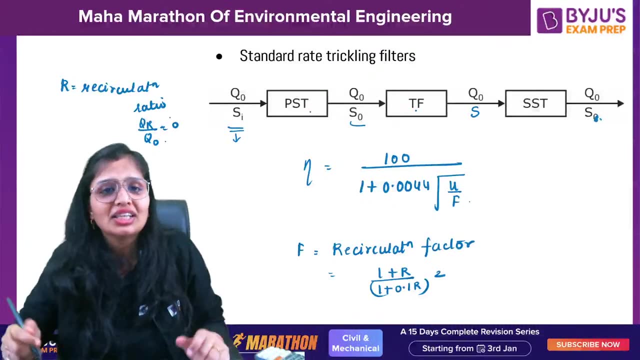 Is 0.1 R whole square And R is recirculation ratio, Which is QR by Q naught, which is equal to 0 in the case of standard rate, Because no recirculation is done. If this is 0, F will become 1.. 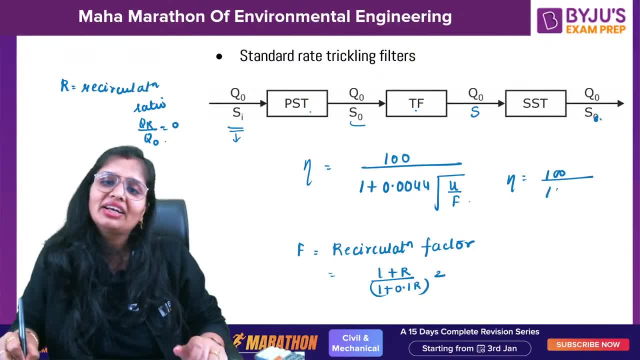 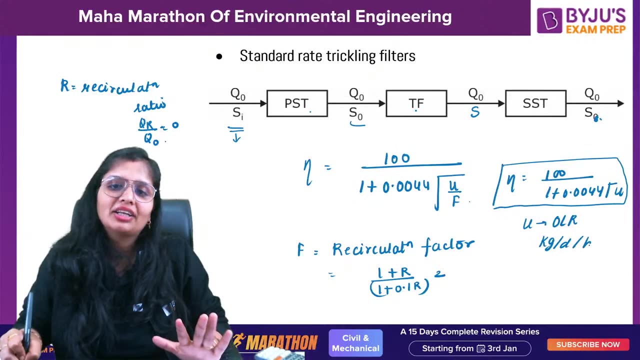 So that's why the formula for standard rate trickling filter comes out to be this. Now what is U? In different books different thing is written. So I will tell you: U is organic loading rate in kg per day per hectare meter. Now, kg per day, kg per. 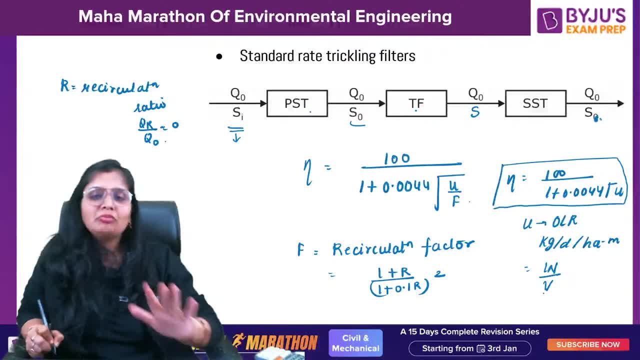 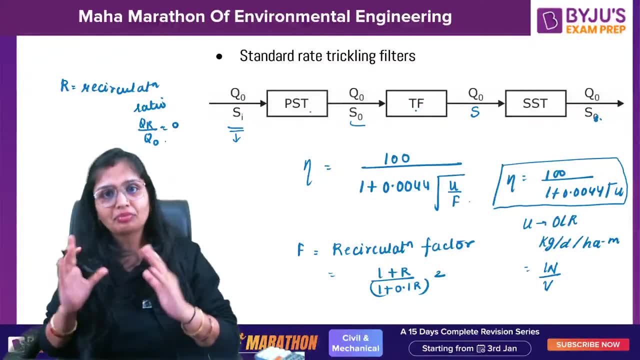 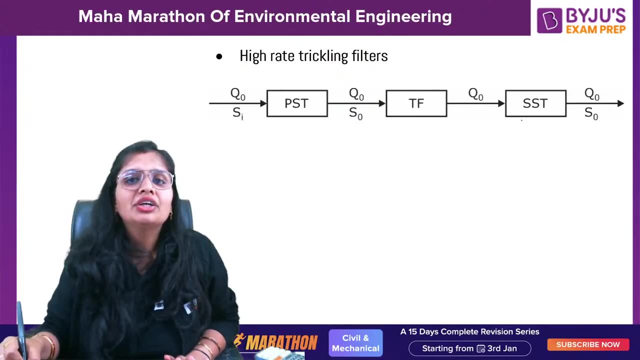 day is the weight and volume is hectare meter. So in some books instead of U they write W by V. Okay, So you can go by any manner whatsoever you want Now standard rate trickling filter, no recirculation. Go for high rate trickling filter. Here you do the recirculation. 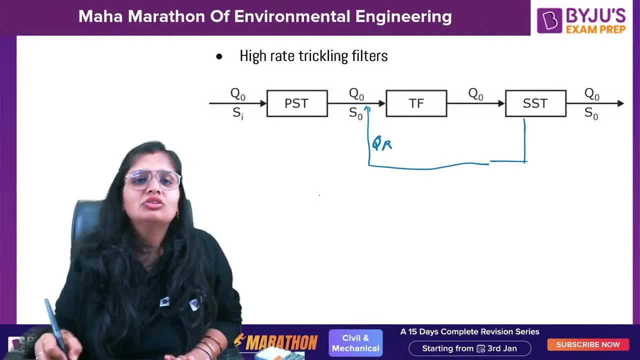 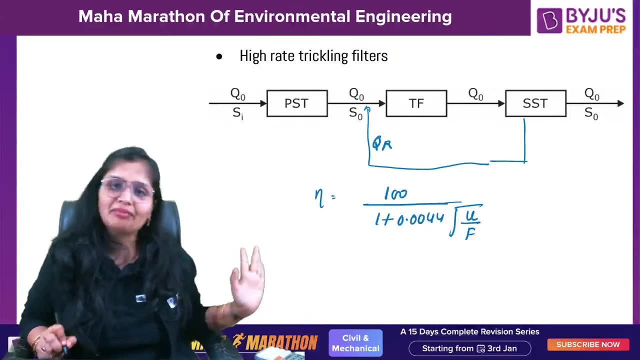 See which is recirculated QR. So exact same formula, but here F will not be 1.. F will not be 1.. There will be a value of F and the formula for F and all remains to be same. This since you are doing recirculation once. 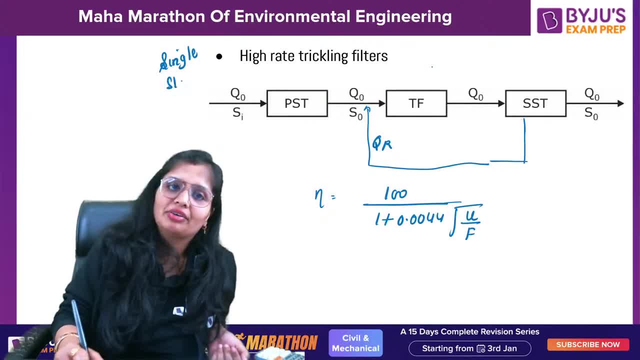 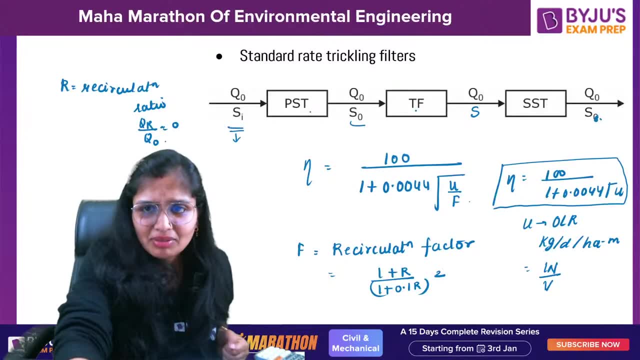 so you call it as single state high rate trickling filter. If efficiency F kaha gaya ma'am, Efficiency F kaha gaya ma'am Efficiency F kaha gaya ma'am Samji nahi, main sa nahi. 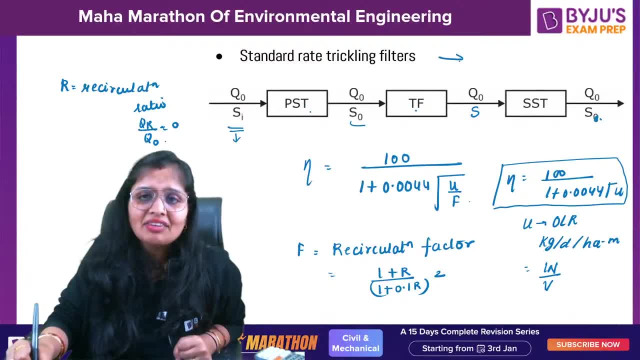 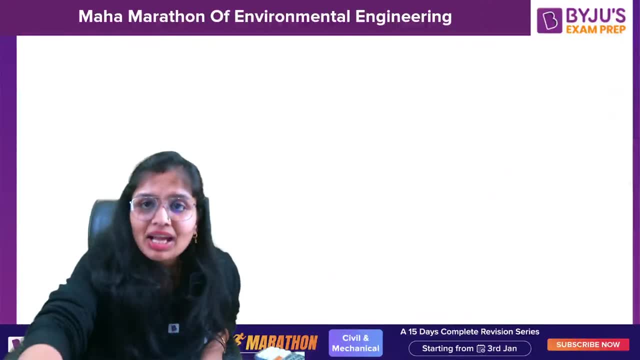 F 1 hai na F 1 hai. Standard rate trickling filter F is 1.. Okay, That's why F is not there. Okay, For high rate trickling filter, F is not 1.. So that's why F is not there. 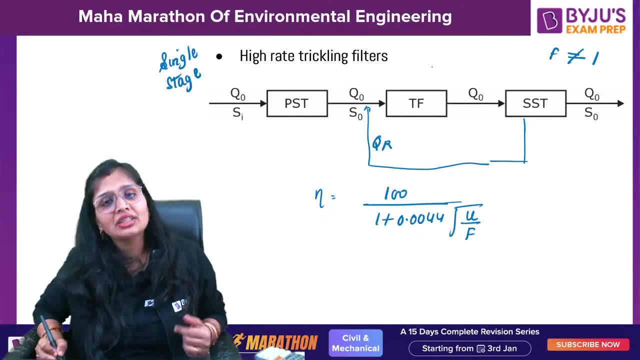 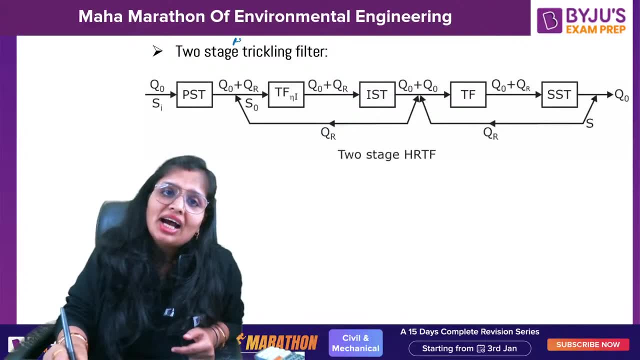 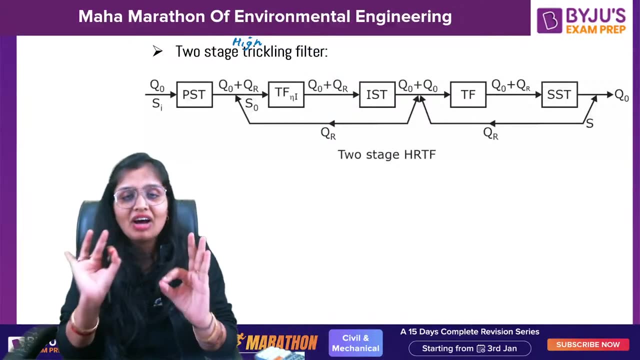 So that's why F is written here. This is since you are doing it recirculation once. this is single state. If you do recirculation twice, it becomes 2 stage high rate trickling filter. Now till now in gate examination: never, ever, they have asked the question. Thank. 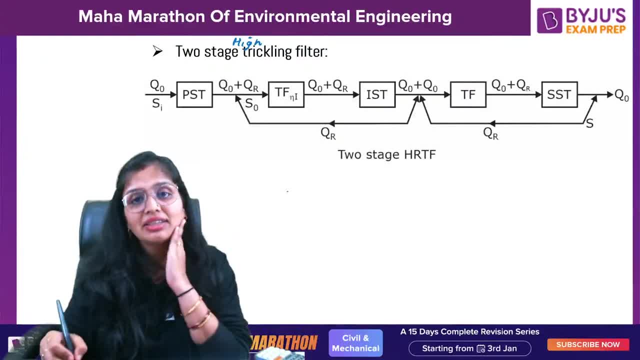 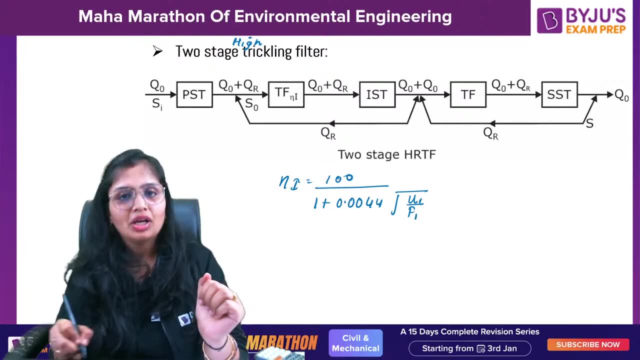 you Prashant for 2 stage. but if they can, so let me tell you Efficiency of first stage. this is U1, this is F1.. Okay, Now what is U1?? You can write it as W1 by V1.. W1 is how. 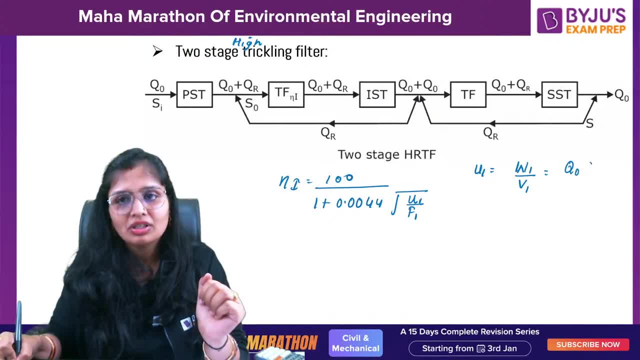 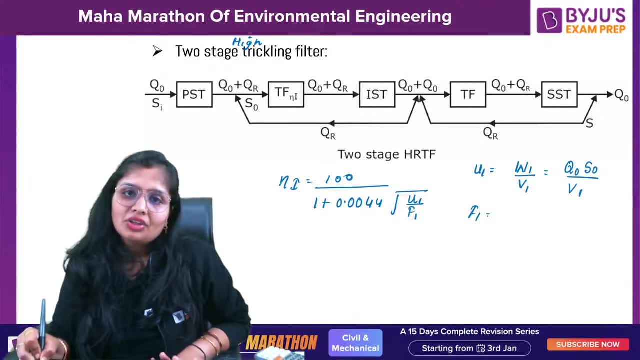 much amount is entering Q naught into S naught. That is the BOD which is entering. This is V1.. Okay, QR, this recirculation can be same and they can be different also. So F1, this is R1.. So 1 plus R1, R1 can be same, can be different. So from here you. 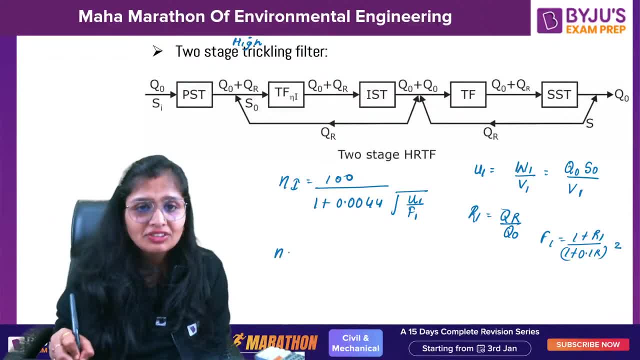 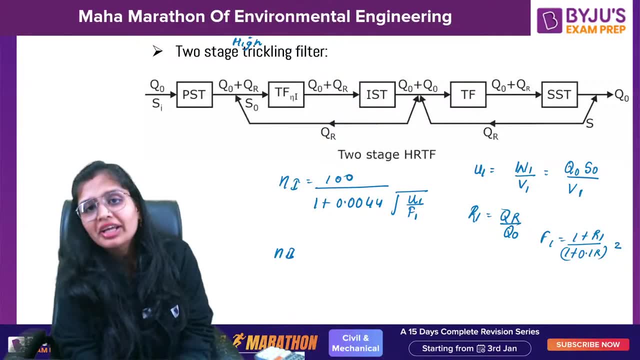 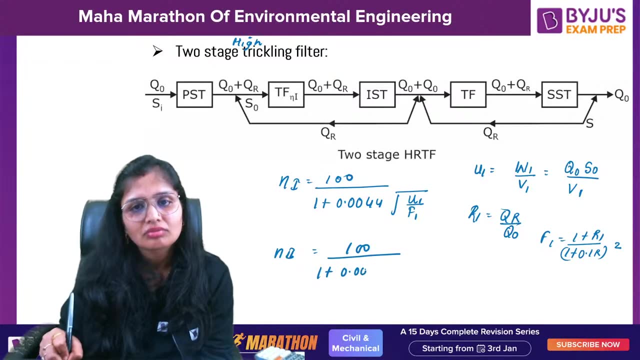 will get it. Okay Now the efficiency of second stage: Anybody. How you will calculate efficiency of second stage Anybody? One more thing will be there, 1 minus 2 things. Firstly, U2 will be W2 by V2.. Volume of the. 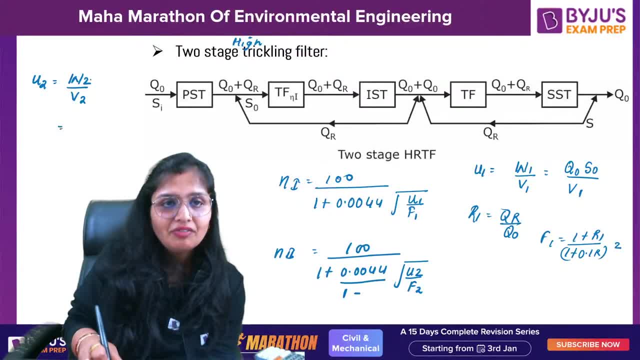 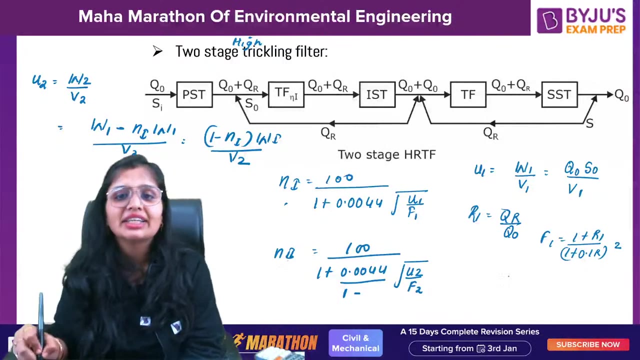 trickling filter can be different. also can be same. also V2 will be. how much W1 was there? the efficiency of first V2.. This is actually 1 minus W1 by V2.. Okay, And this is first stage, this is second stage. 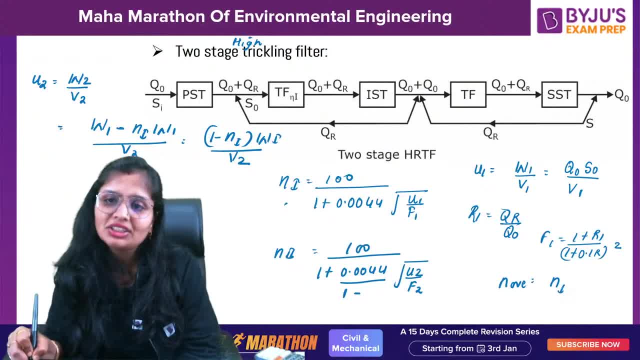 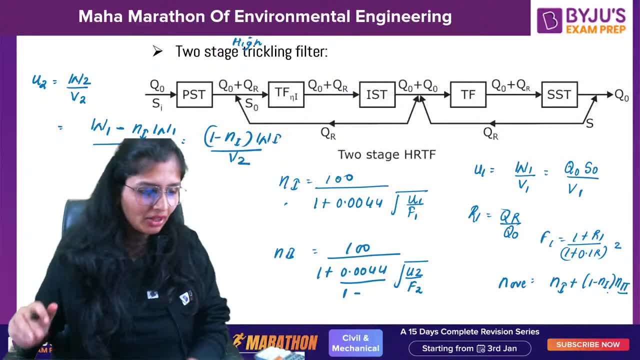 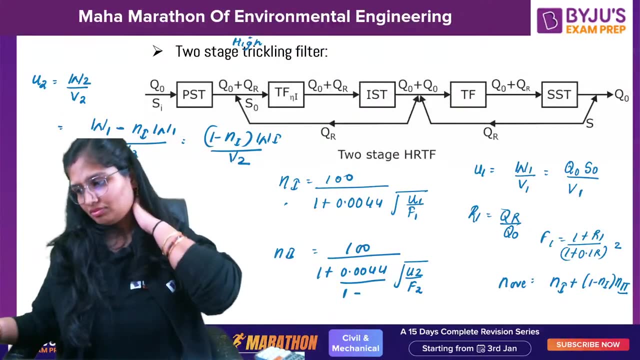 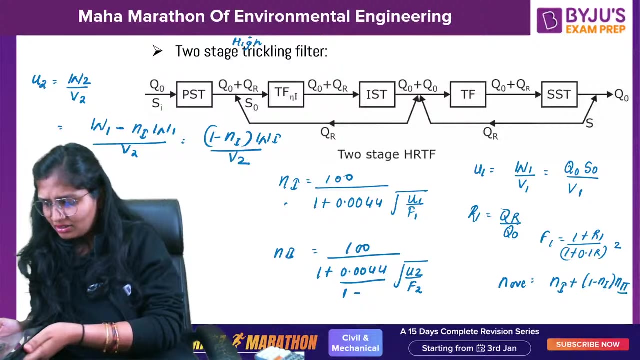 Overall efficiency will come out to be: how much efficiency is of first stage, how much efficiency is of second stage? Any doubt, Any doubts anybody has? Yes, Yes, Yes, Yes, Yes, No doubt. BOD exit generally. we don't go by that. No, we don't. This is left 1 minus. 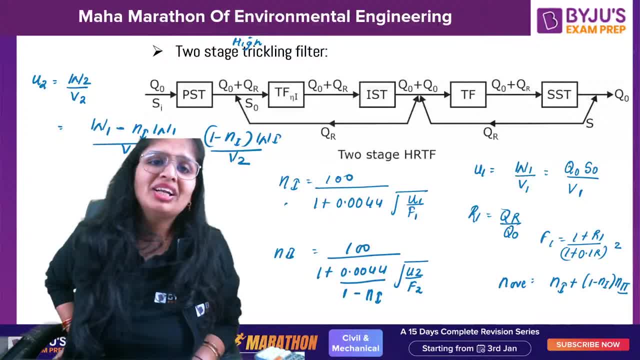 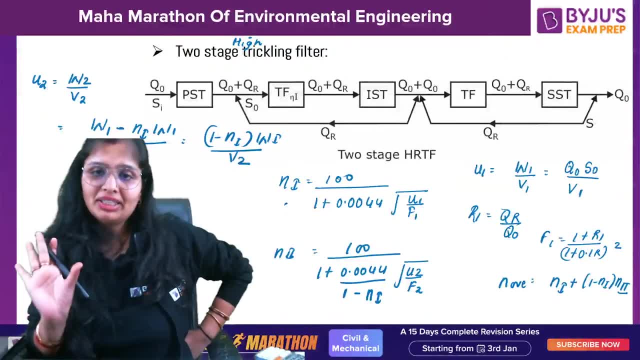 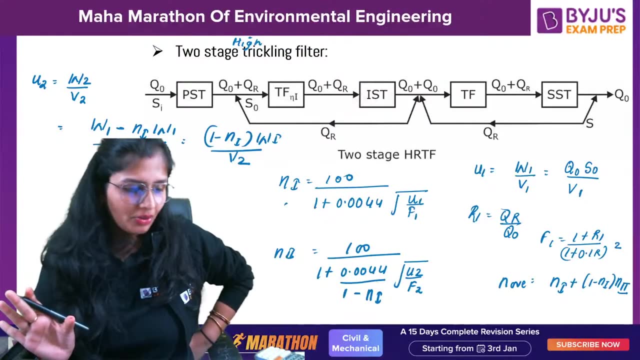 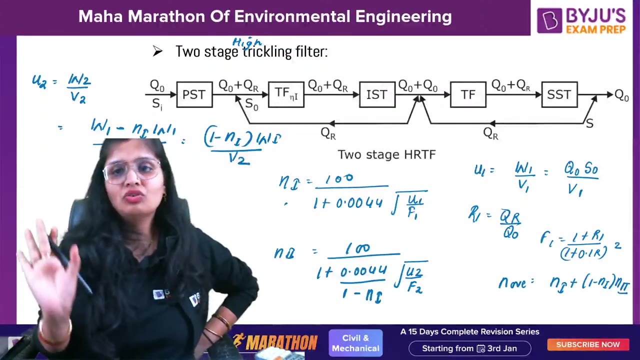 theta. That formula is used when you get the value- what you are telling me- BOD in minus, BOD out. I know this is difficult to learn, but this is the formula, which is that's what I am telling, okay, here. so this is the overall efficiency formula. this is the first. 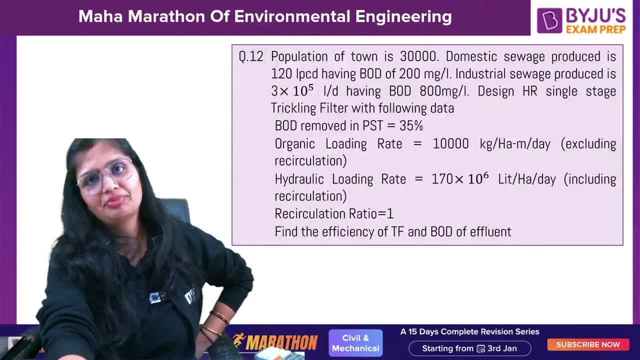 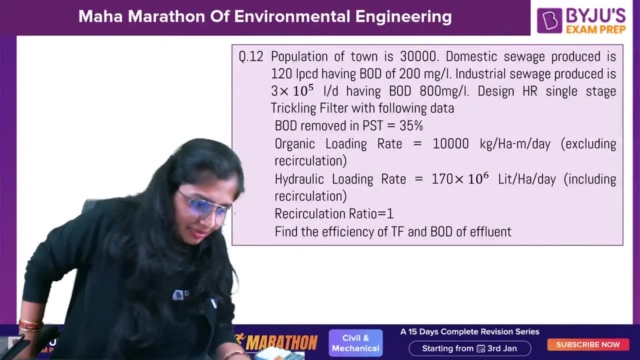 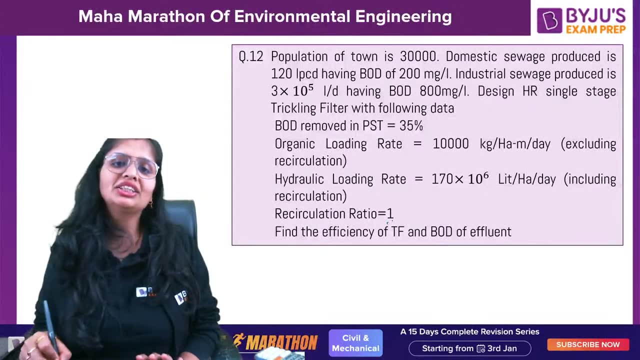 stage, second stage: till now, never, ever asked in your gate examination. come on, guys, this is the question. let's do it fast. thank you, Tekhsha. come on, guys, solve this. we have to calculate the efficiency. recirculation ratio is one that means it is a high rate trickling filter. one thing which I'll give you advice. 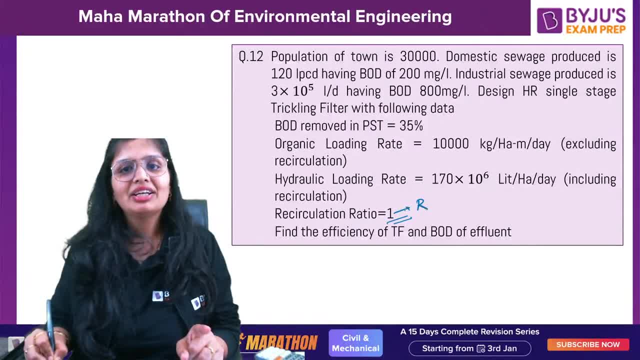 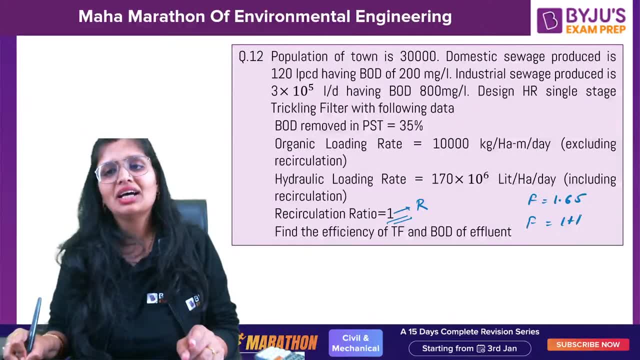 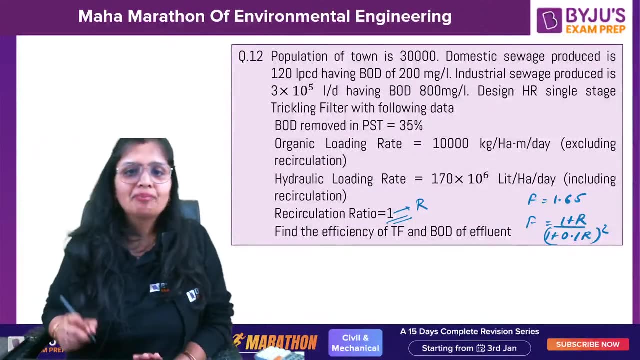 since you have to do it in virtual calculator. when recirculation ratio is 1, F is equal to 1.65. remember this. otherwise you can calculate also: 1 plus R upon 1 plus 0.1 R, whole square, you calculate, you will get 1.65. okay, now it. 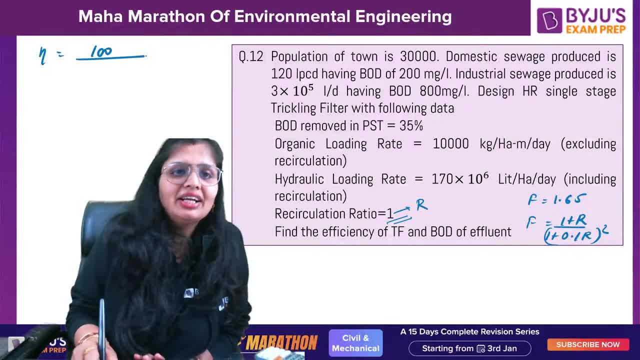 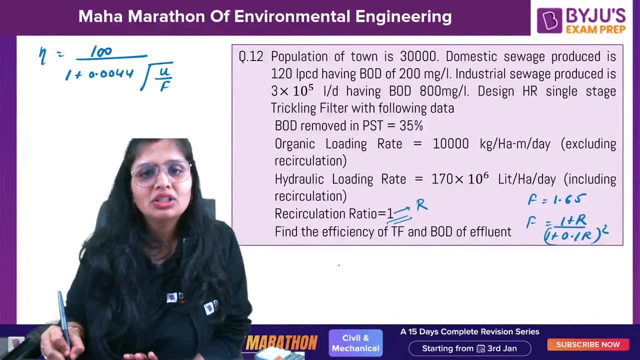 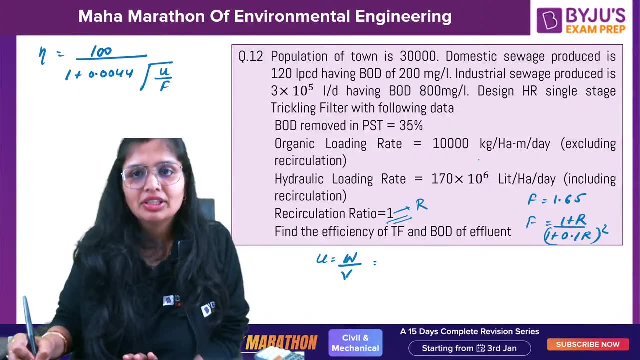 is asking me: efficiency. efficiency is hundred one plus point, double zero, double four, U by F, F, I know U, I want to know U. is the organic loading rate W by V volume? not at all given to me directly. is it given? yes, just check it out. two, three, four kg per. 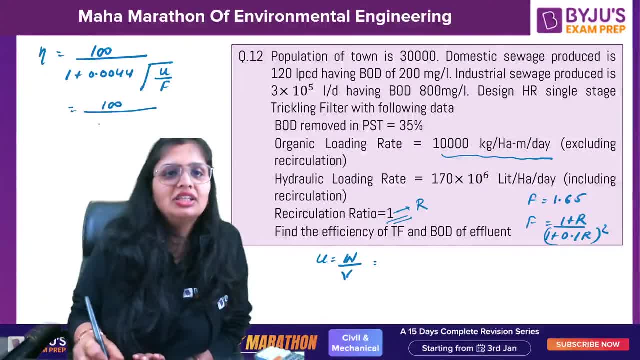 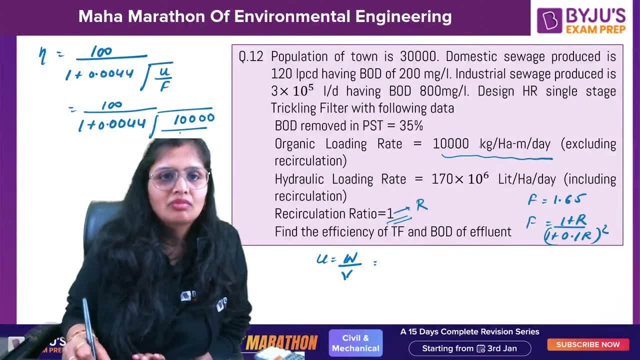 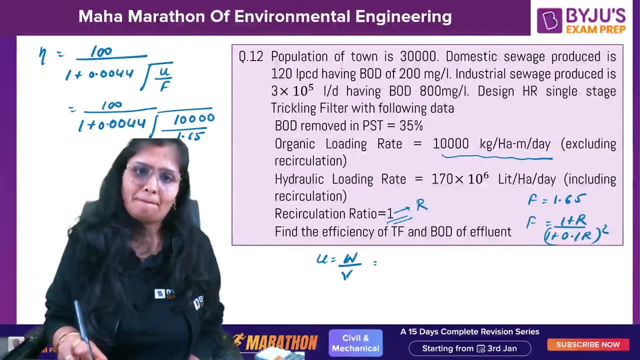 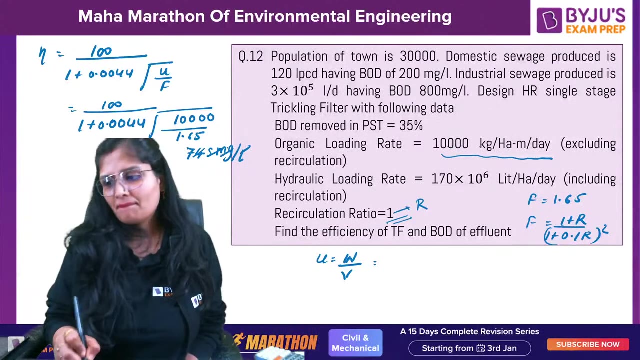 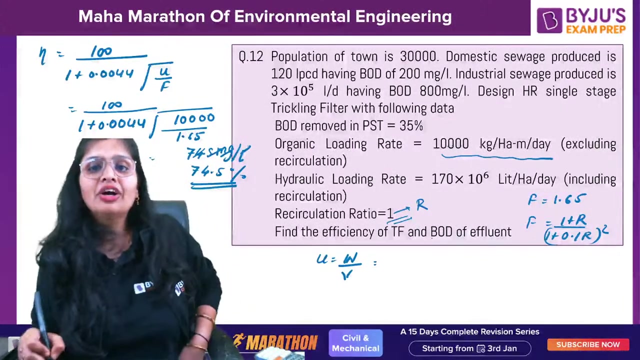 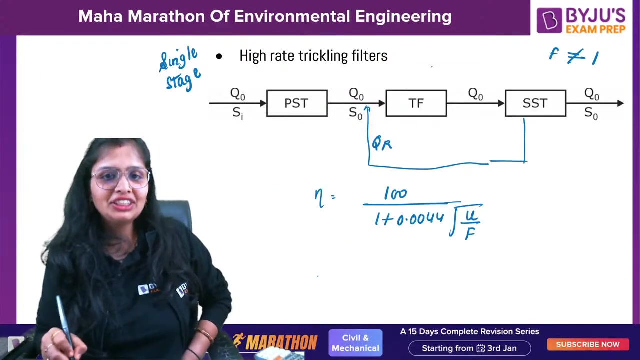 hectare per meter. directly. it is given to me 200 dust formula based how much it is coming. how much it is coming, efficiency, guys. efficiency 74.5 percentage. this is the efficiency, not, is asking me, BOD of the effluent. now see the diagram. another, your efficiency, what? what she is was. 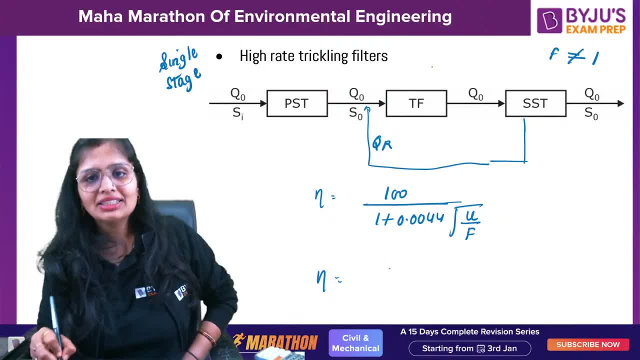 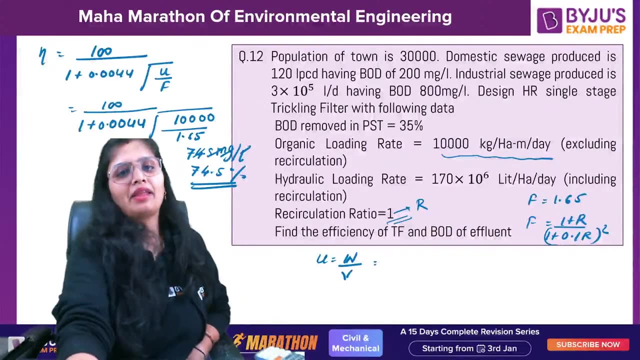 telling me if s naught s naught is the beauty which is entering and s is the BOD which goes out. So influent minus effluent divided by influent BOD into 100.. So this can also be done. Okay, Now see, in this question it is asking me BOD of effluent. Effluent S naught. 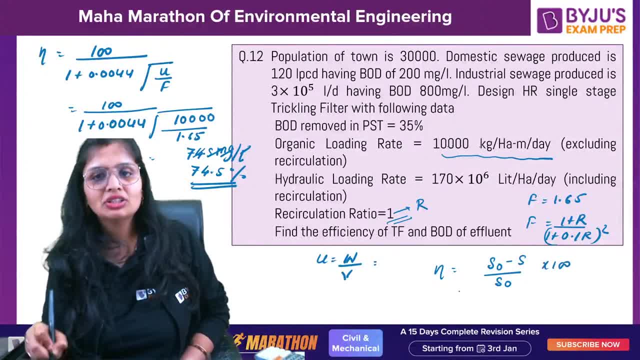 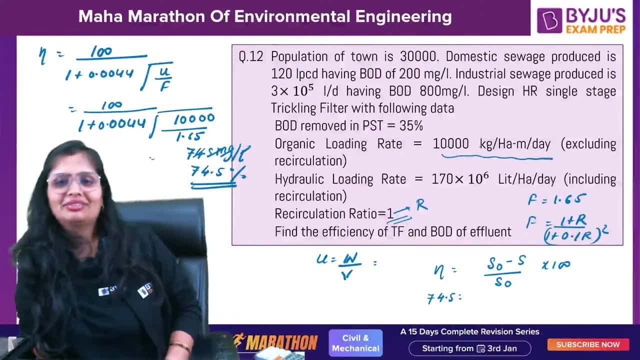 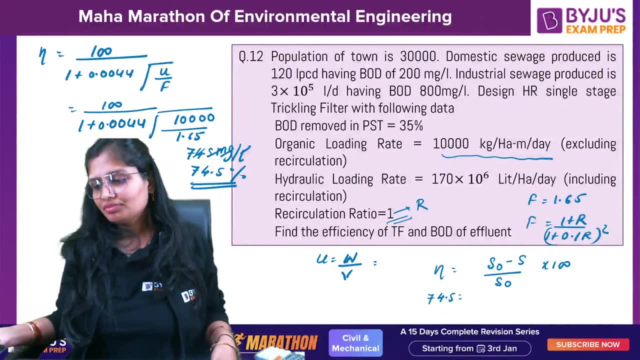 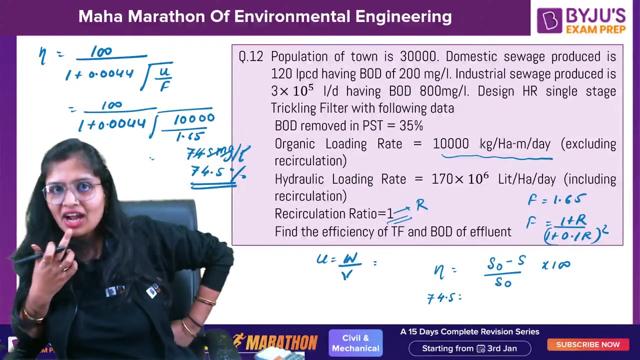 minus S divided by S naught into 100.. Now in this question I have already calculated the efficiency S naught how much BOD is entering. How to calculate? Got stuck. How to calculate, guys. How to calculate now We have to calculate what. We are stuck. We have to calculate BOD mix now. 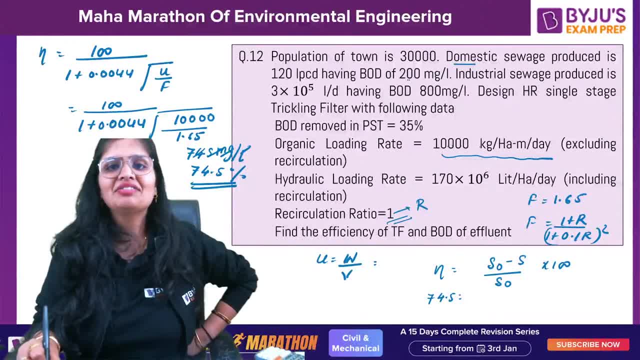 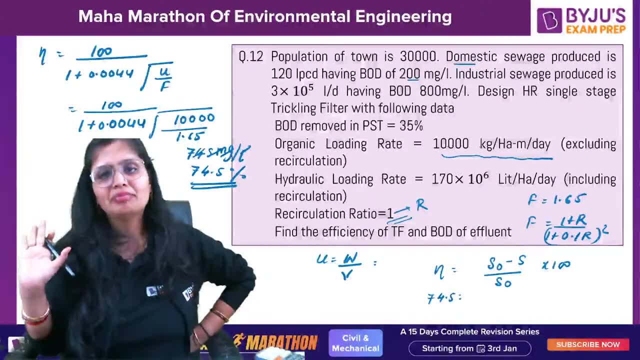 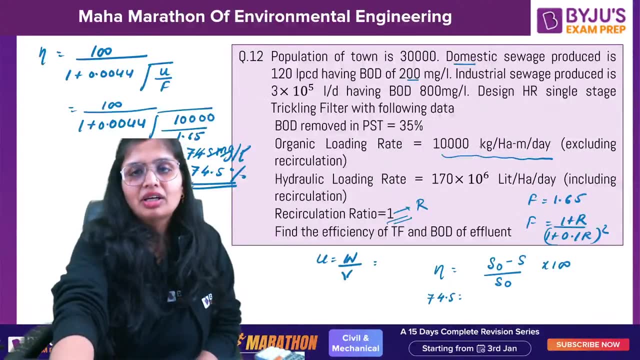 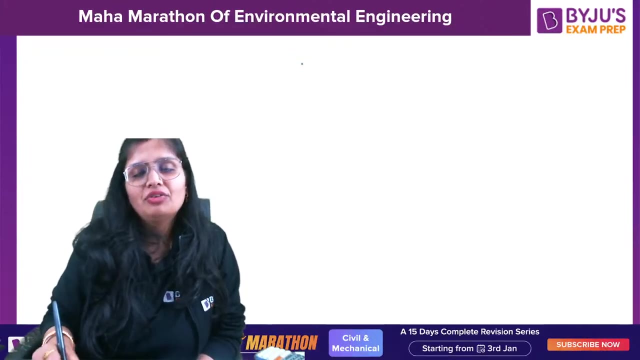 Why? Why we are stuck Because domestic sewage has different BOD, industrial sewage has different BOD. So what we have to do now We have to calculate the BOD, or basically the BOD mix. So, come on, solve this: 30,120 liters, Okay. So we have to calculate BOD. Okay, 30,000 is there? 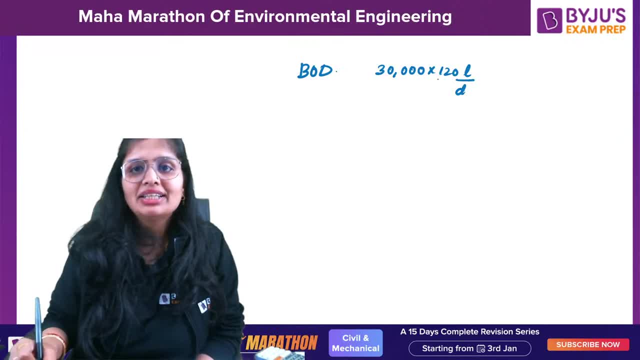 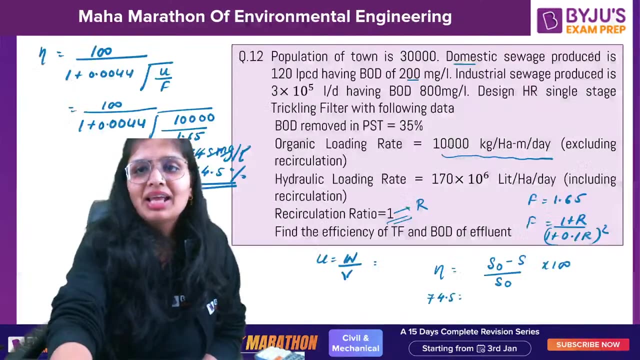 120 liters per day. Okay, This is the discharge. This is the discharge And the BOD is 200 mg per liter, 200.. Domestic sewage: 200. And the industrial sewage is 3 into 10 raised to power, 5 liters per day And the BOD is 800 mg per liter And the total discharge will. 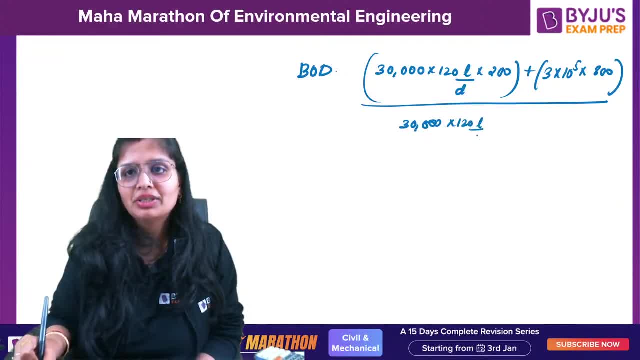 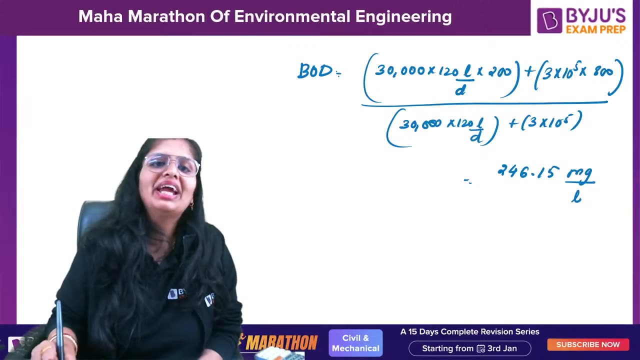 be 30,000 into 120 liters per day, plus 3 into 10 raised to power 5.. How much it is coming the BOD value? So just check it out. This will be the BOD which will be entering into the trickling filter. 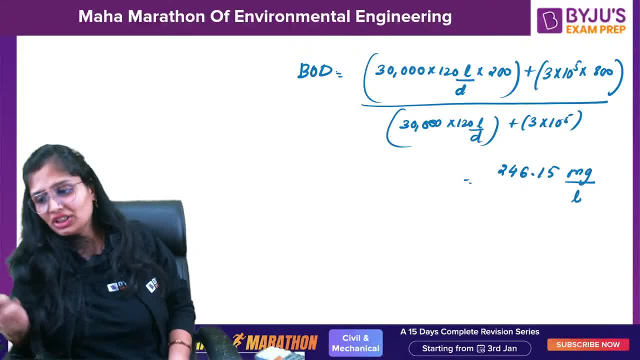 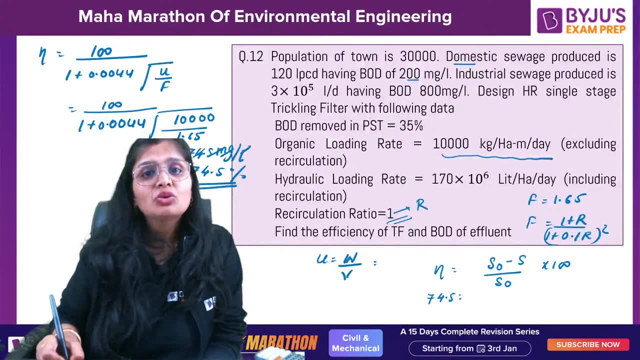 Now why you did that? Because domestic sewage and industrial sewage combined BOD was entering- Okay, But this is not entering the trickling filter. Why? Because it has told that first it will go into the PST and 35 percent is removed. So the BOD which goes into the PST and 35 percent is removed. 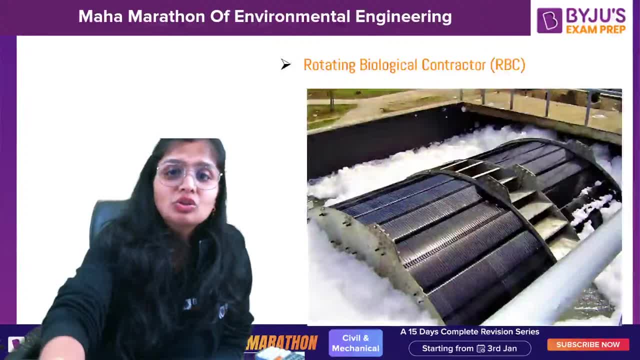 First it will go into the PST and 35 percent is removed. So the BOD which goes into the PST and 3 in labor is ranked, you will find that the BOD is the BOD that the U with trip file into the slip file is able to be stored at the salineor할. 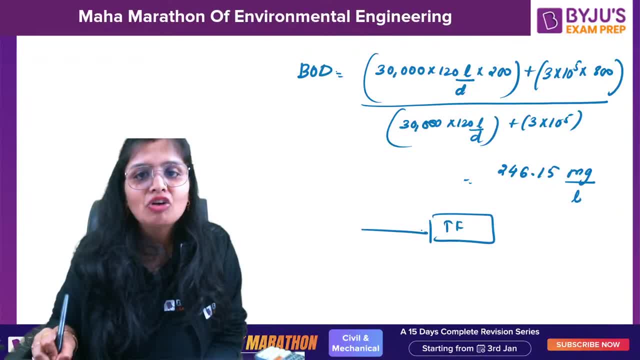 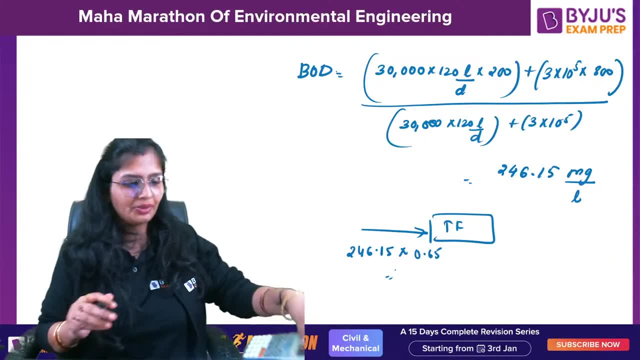 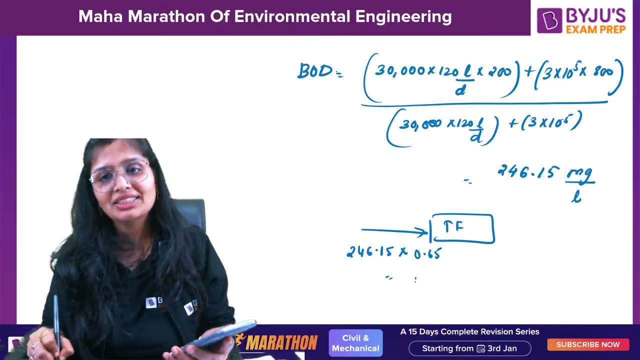 which goes into the tricking filter will be how much 246.15.. 35% is gone there, So here it will go. how much 65%? So it will be 246.15 into 0.65.. This will come out to be 160 mg per litre. 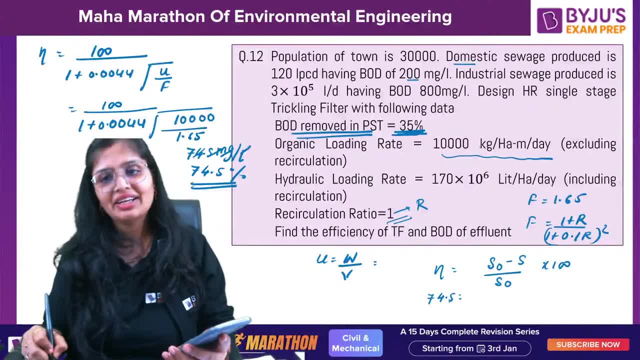 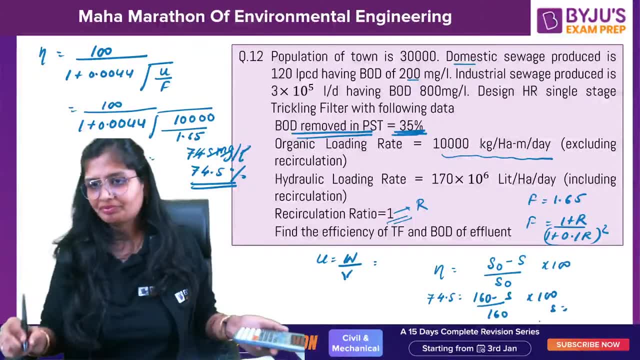 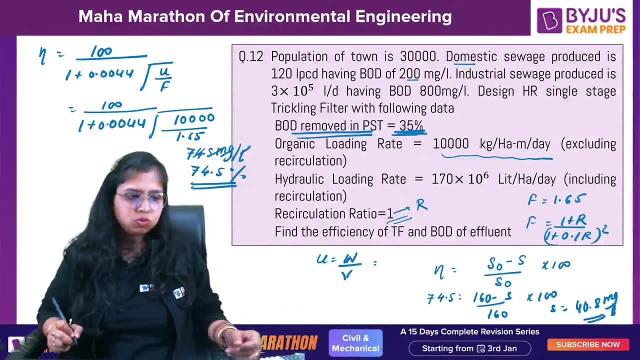 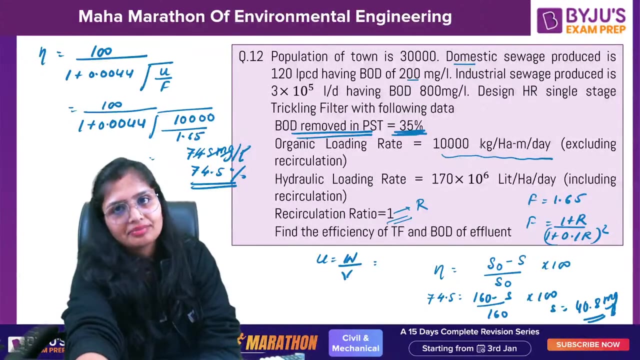 159.99 it is coming. So the BOD which is entering is 160 minus S 160 into 100.. How much is the value of S coming? 40.8 is Clear. Okay, So just let us do rotating. 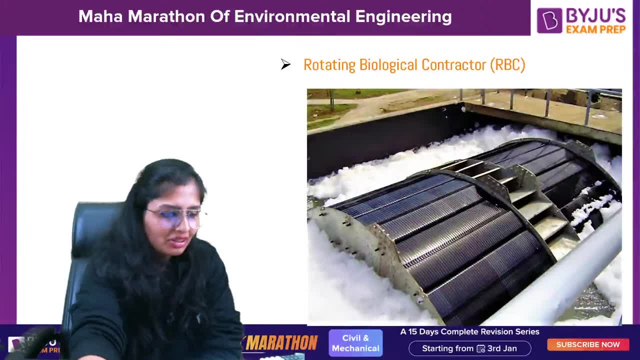 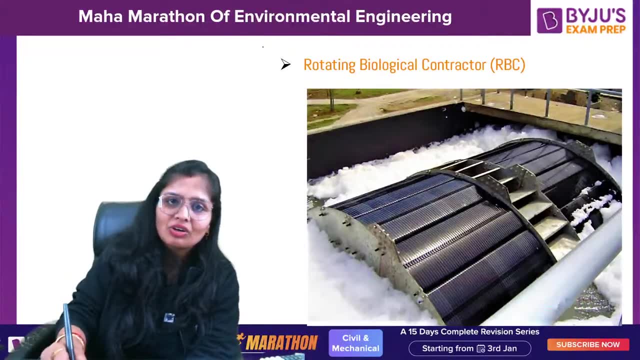 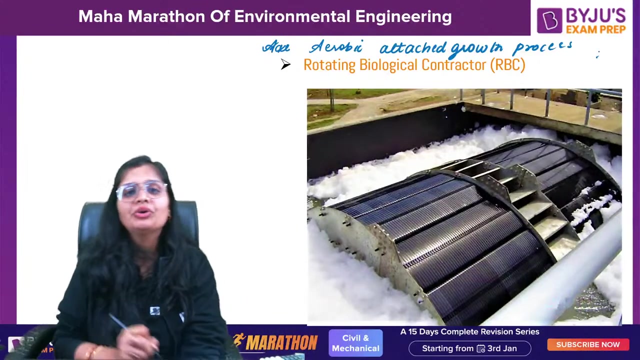 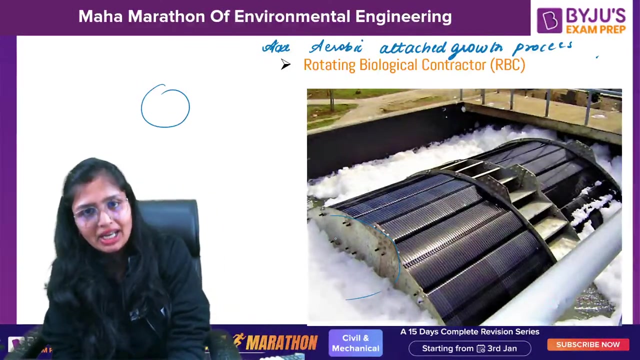 biological contractor, Then I will give you a break. See rotating biological contractor. RBC are also aerobic attached growth process. What you do it here? Here circular disc are provided. Now you can see it here, These circular disc are provided. and here also, you give time for the attachment of the micro. 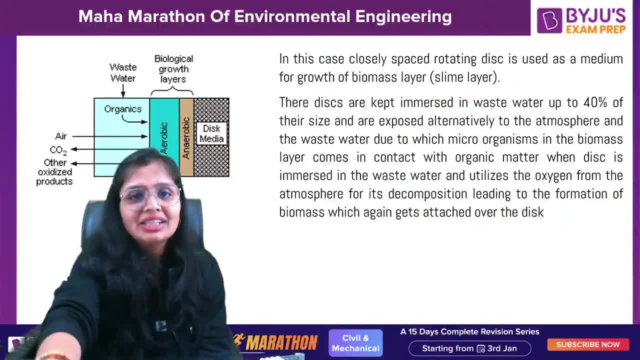 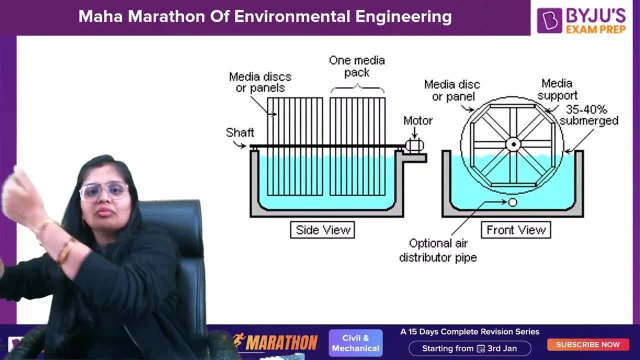 organ: Okay, In this disc. But the problem is here, Here, when you see this disc, Okay, The disc goes down, it goes up, Goes down, goes up. So what is happening? 40% of it is submerged in. 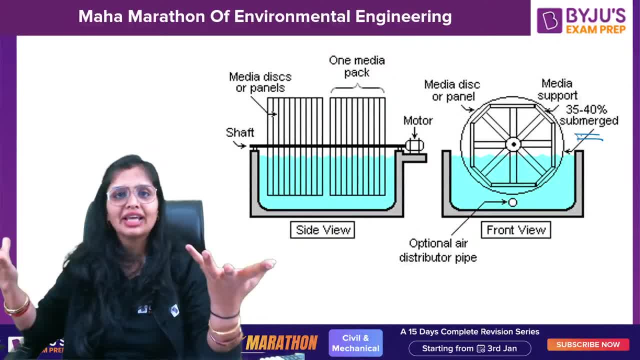 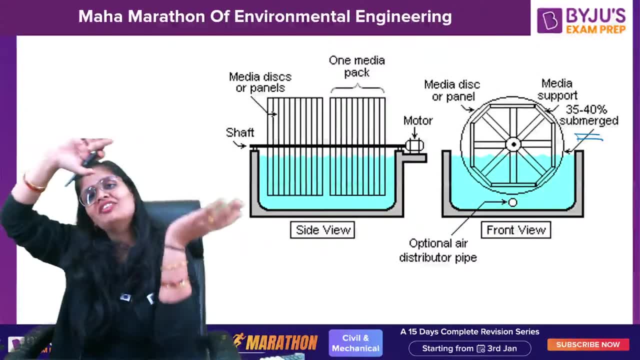 water Rest 60%. about 60% is exposed to the atmosphere. So it will go up. It will carry out the oxygen. It will take the oxygen, carry out the decomposition. The one which was up now, it will go down. The one which was down, it will go up. It will take out the oxygen. 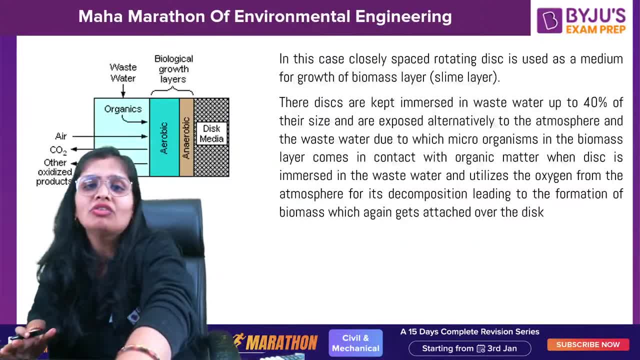 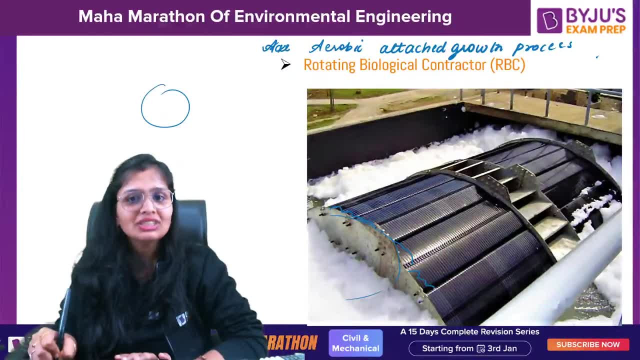 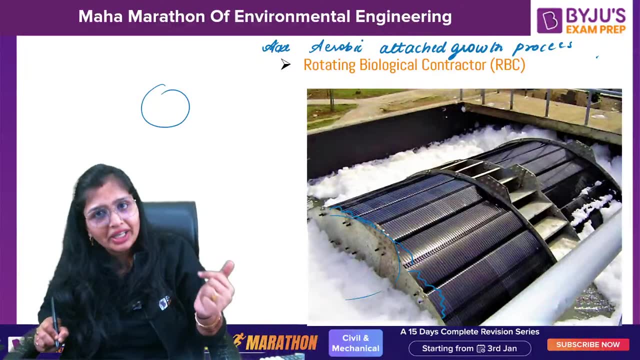 take the oxygen from the atmosphere and carry out the decomposition of biodegradable organic matter. Okay, So here the microorganisms are attached. But you will see, ma'am, the microorganisms are attached, But here they are partially suspended. also, Why? Because 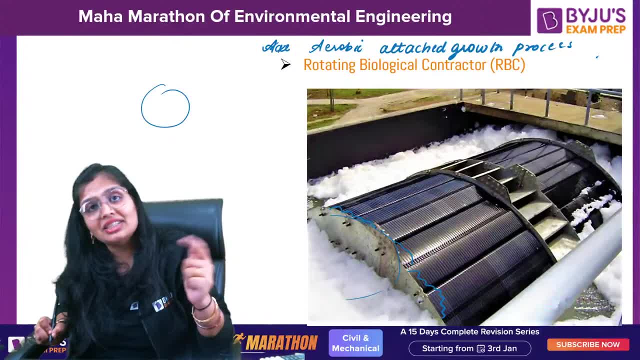 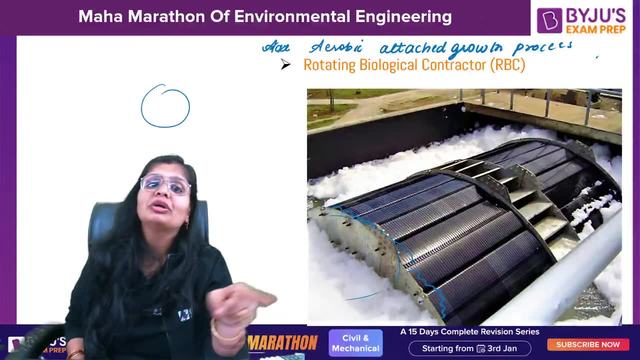 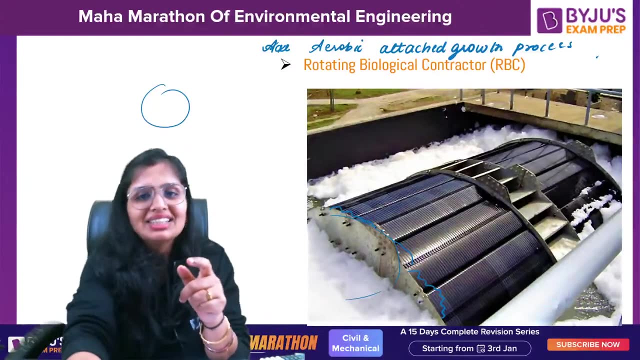 the microorganisms are also moving Because the disc is moving. But since, what is the purpose of disc I gave? I gave the disc for the attachment of biodegradable organic matter. Okay, So that is the reason I will call it as attached growth process. Okay, So this. 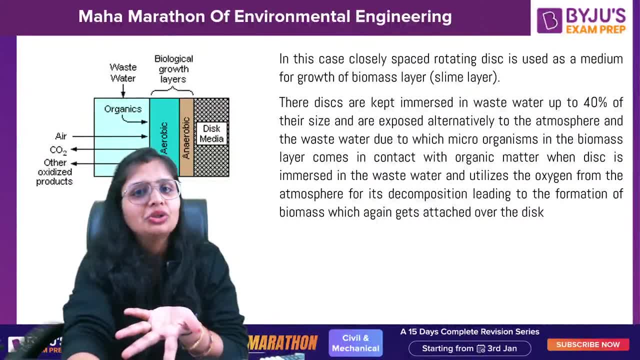 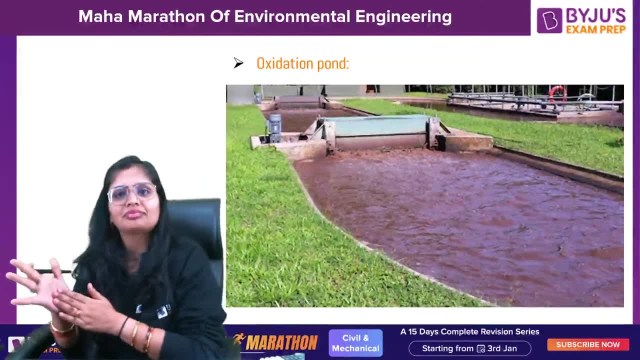 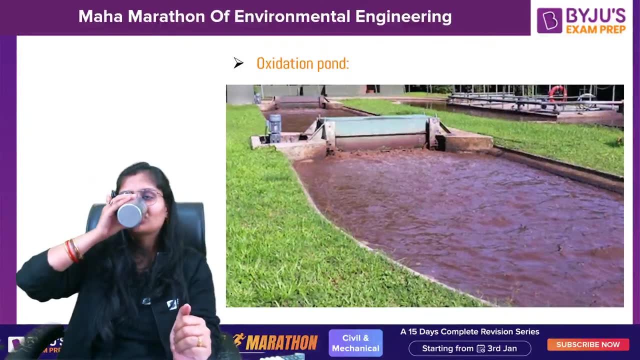 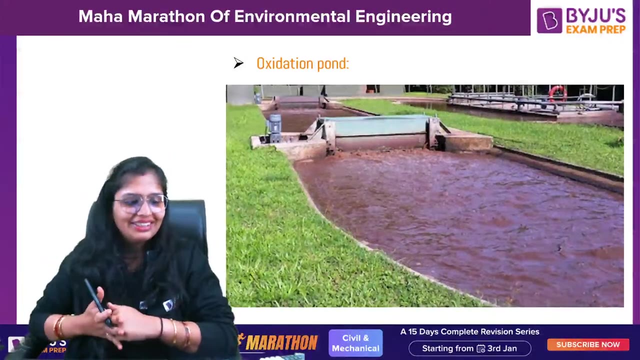 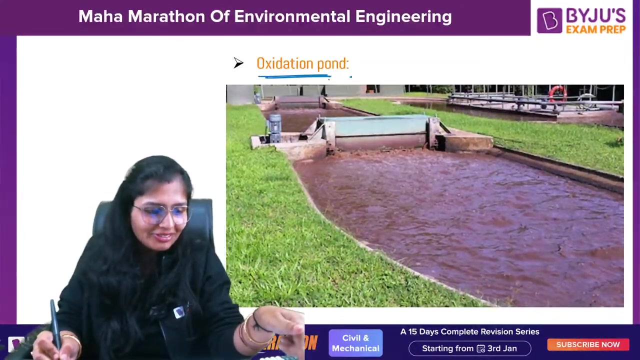 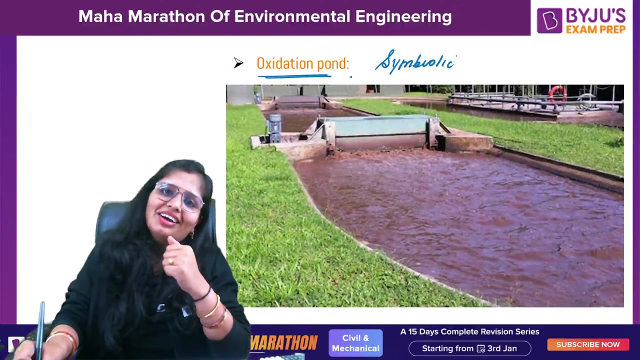 is the process which can also be used, which is mentioned to you here, All the details regarding it. Okay, Any doubts still here? Any doubts still here, guys? Okay, Shall, we do oxidation bond also, or you will kill me. Okay, Oxidation, Shall I. 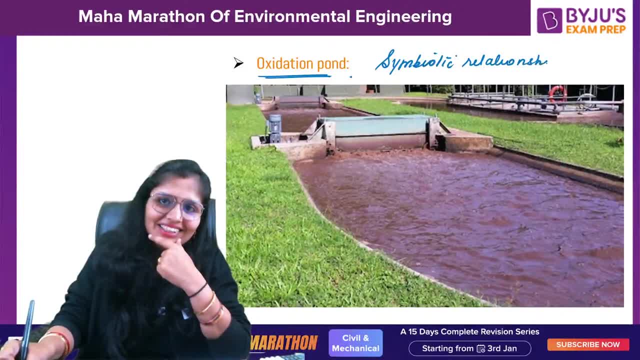 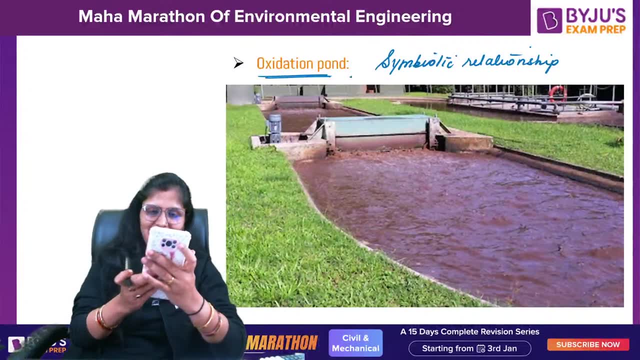 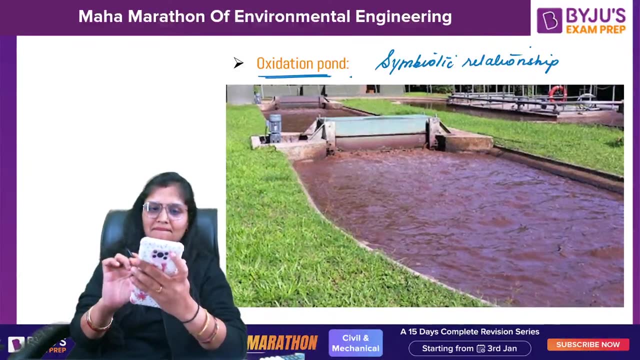 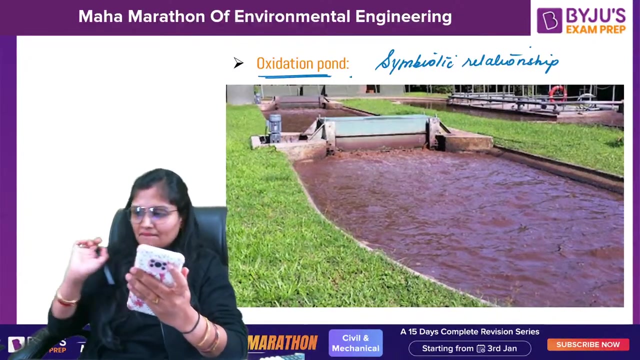 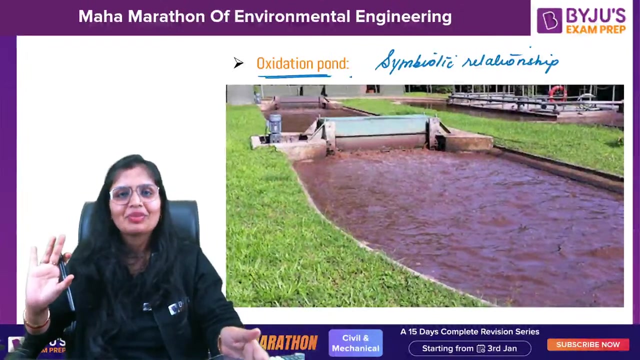 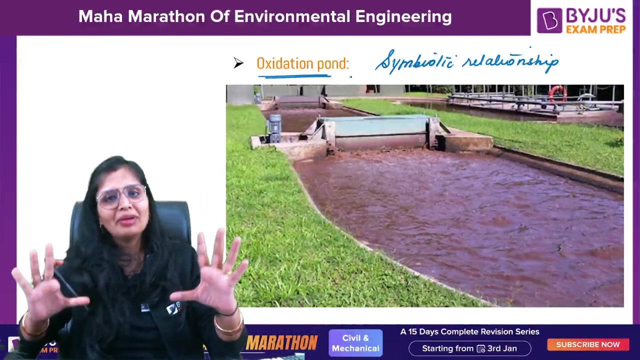 do this, Prashant, Do this Go. I am from 6.. Okay, Oxidation bond is based on symbiotic relationship. that means mutual relationship. Okay, What will happen here? These are the long basins and all where you allow the water, Nothing. So you will have to do this. So you will have. 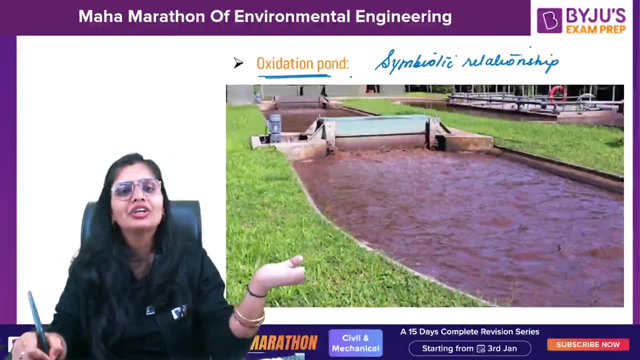 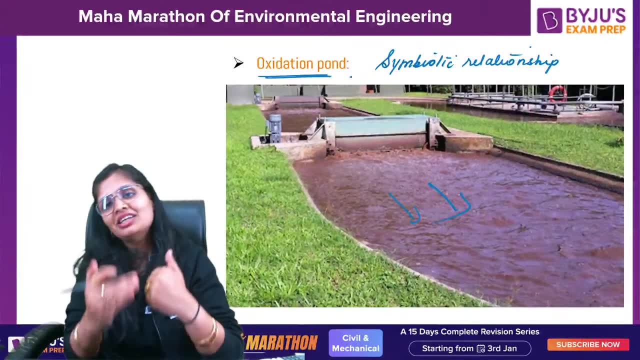 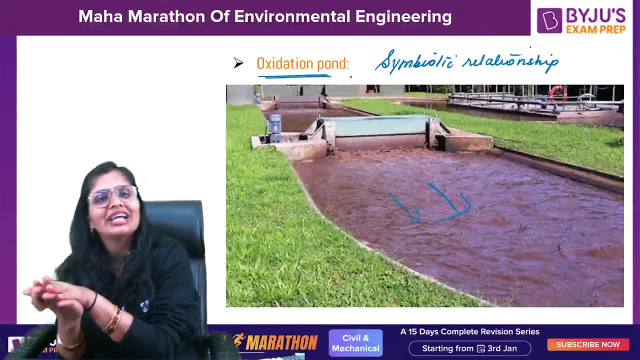 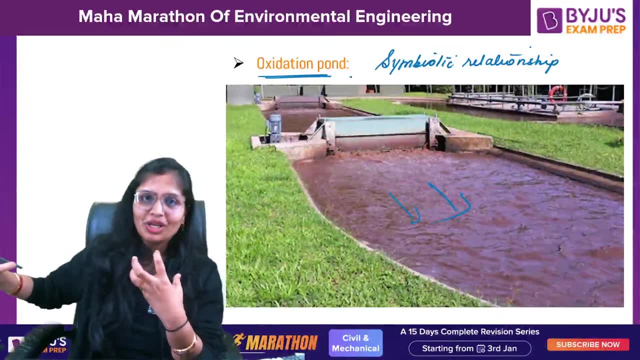 hard for you guys so that you guys can score good marks in your gate examination. When you will top, you will give the credit to me. So that is the reason I am investing on you. So I am giving you and I will take it from you. So that is what mutual relationship. 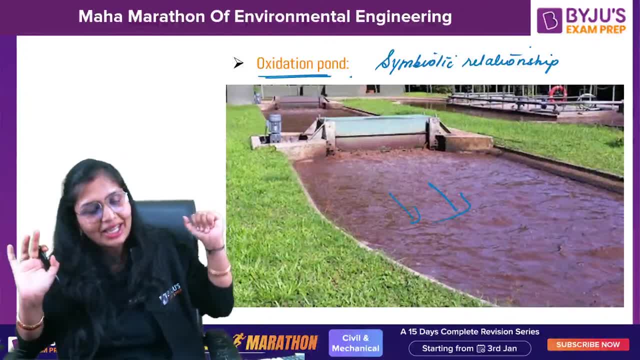 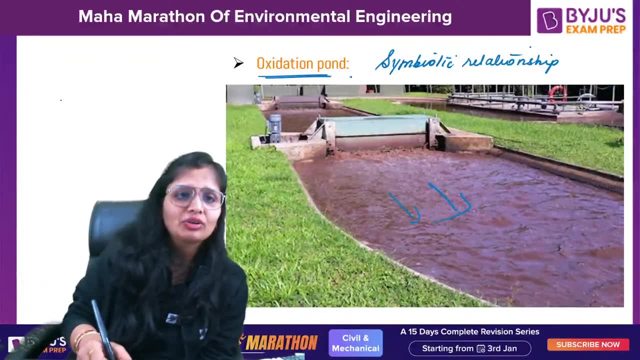 symbiotic relationship. Tumana bhi bhalla ho, mera bhi bhalla ho. So symbiotic relationship. when you talk it about oxidation point has same thing How- Just check it out- Algae does what Algae prepares. food gives oxygen. This oxygen is used by microorganisms and they do the decomposition. 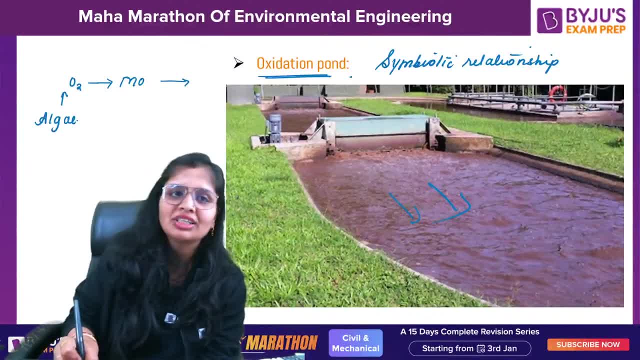 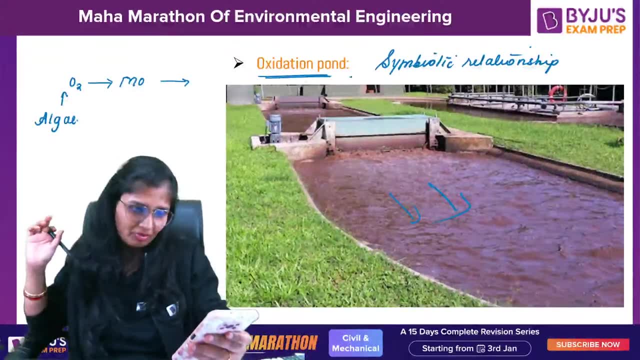 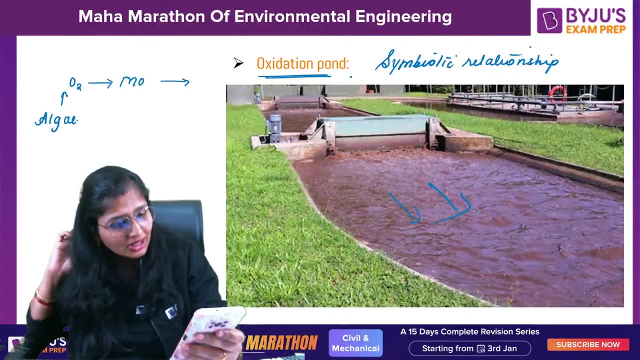 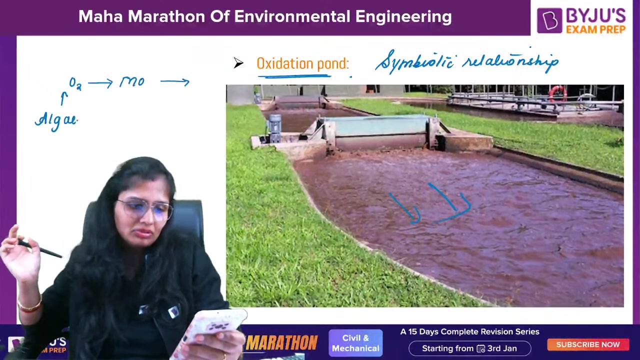 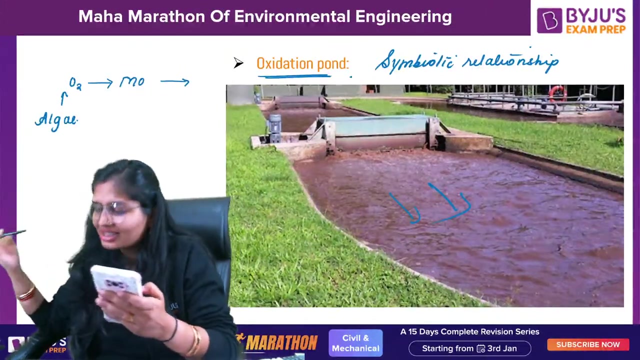 And when aerobic decomposition takes place, what is liberated? What is liberated, guys? I am not going to tell you. Tell me What is liberated. Aerobic decomposition, what is liberated: Carbonates, sulfates, nitrates, This you have to answer me. 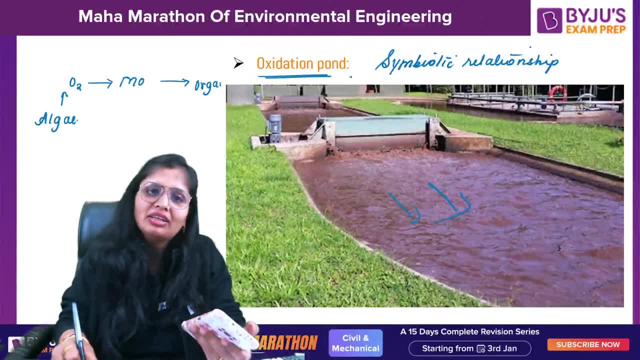 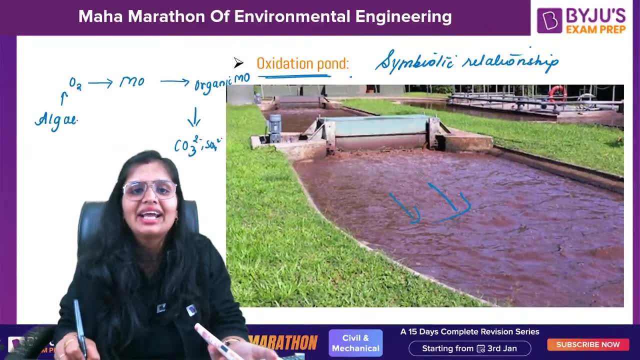 So microorganisms decomposition Organic matter. microorganism decomposes organic matter. It releases carbonates, sulfates, nitrates. Now this is used by algae also and this can be used by anaerobic microorganisms. Here aerobic microorganisms are there, So one relationship is between aerobic microorganisms and algae. 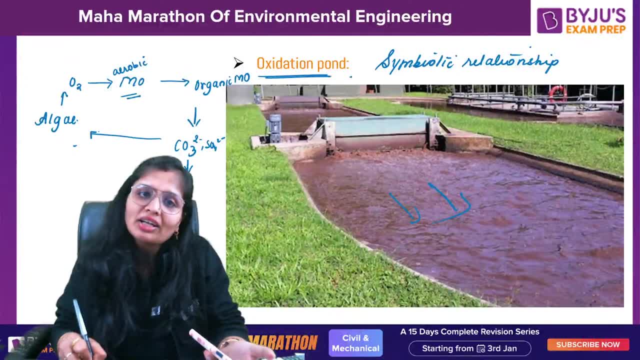 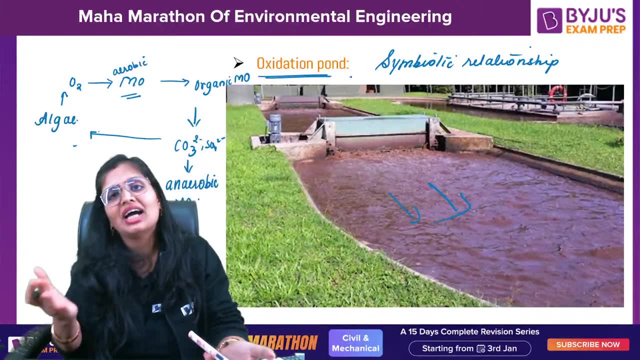 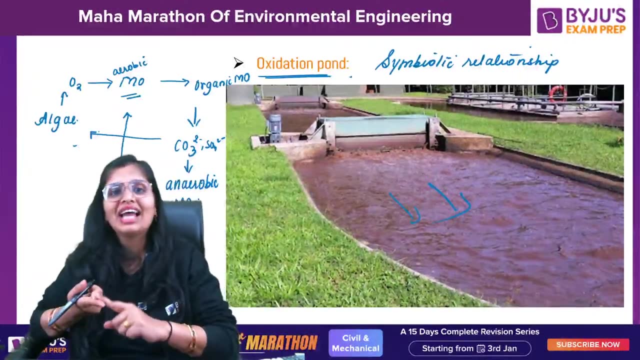 Second is this is also used by anaerobic microorganisms And when they make, when they do the decomposition, Composition and all they release gases like carbon dioxide and all which can be used by aerobic microorganisms. So two relations are going on. One is between algae and aerobic microorganisms. 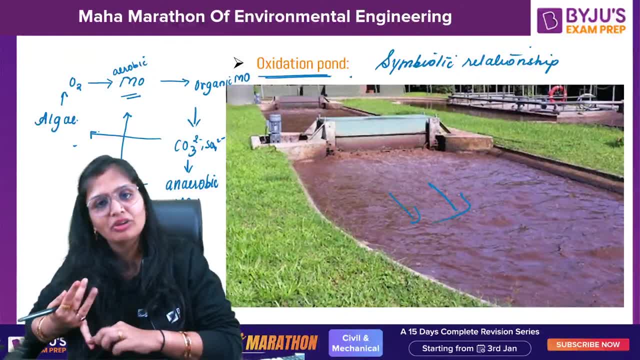 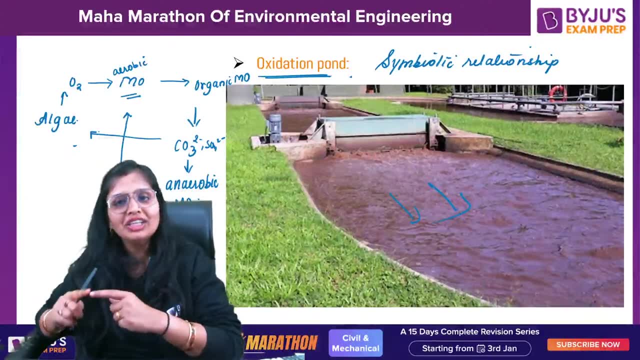 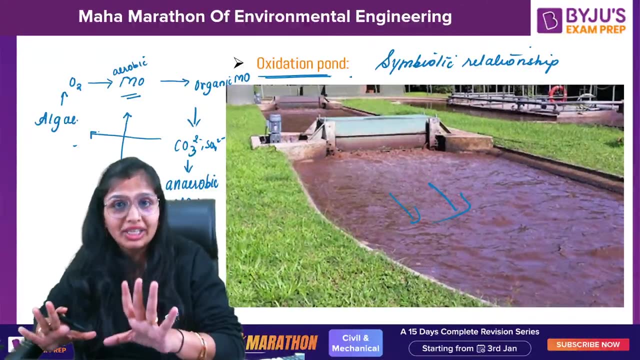 Another symbiotic relationship is going on between aerobic microorganisms and anaerobic microorganisms. Okay, These, these two are going on, with the help of which, when you take out the water, the only problem is large detention time. is there, Ma'am? how much detention time? More than 14.. 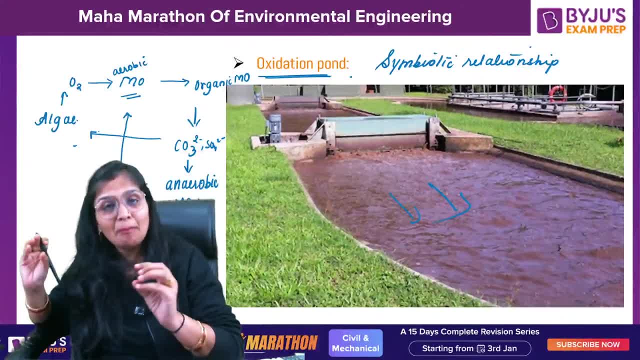 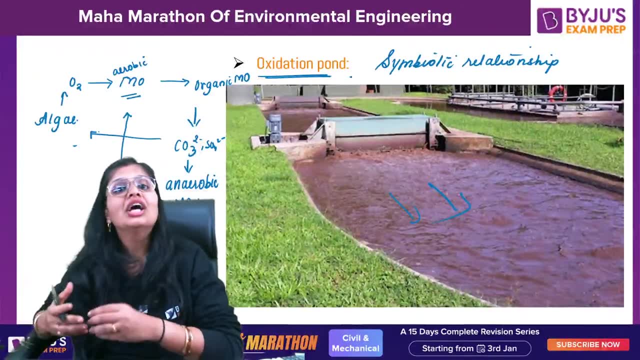 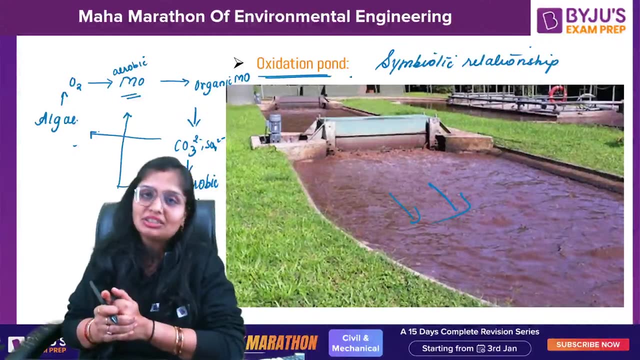 A month. approximately takes a month. So yeah, the main drawback: you can see that a large amount of time is required, but the positive is you see that much lesser quantity of organic matter is there, So large amount of organic matter has been decomposed in this case. 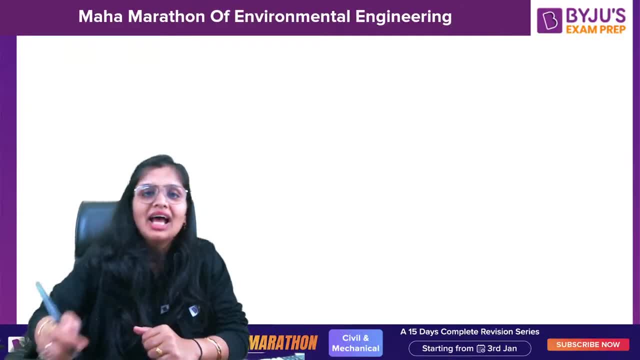 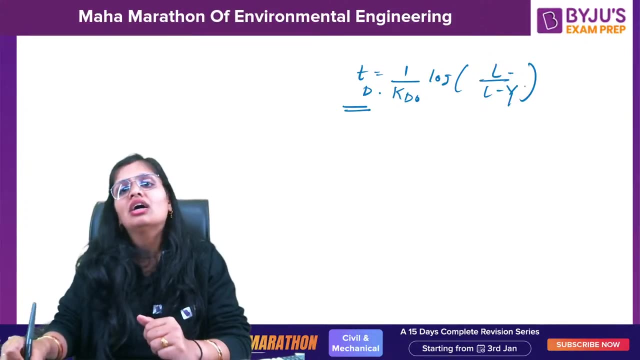 Clear. So this is about oxidation point and there is a formula also: T is equal to 1 KD. log L upon L minus Y, L is the influent BOD. if you want to calculate the detention time and oxidation point, L is the influent BOD, Y is the BOD removed. 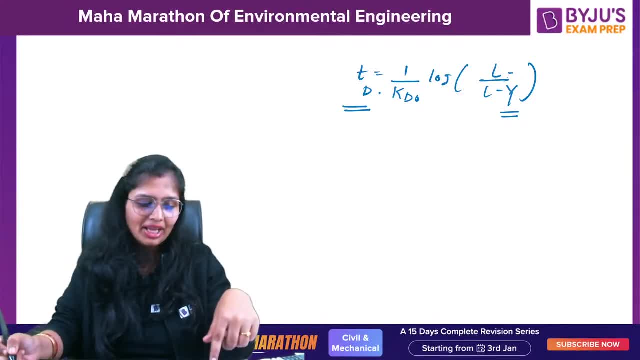 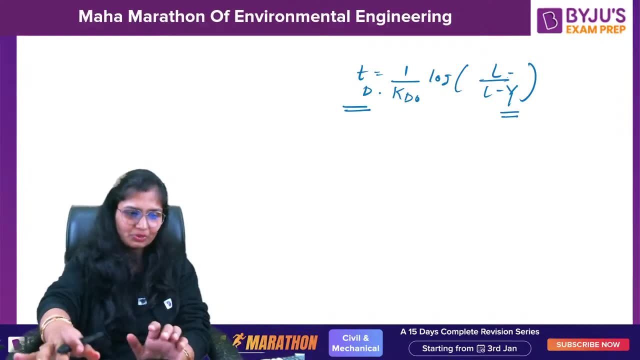 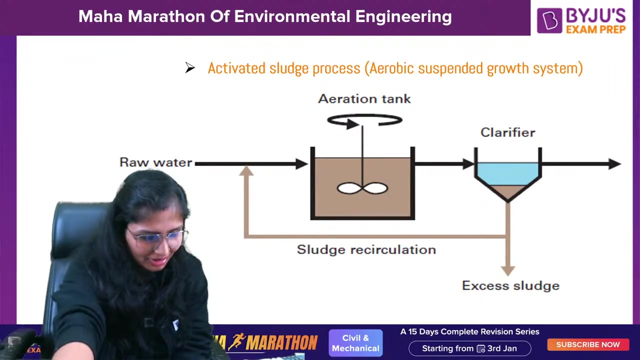 This is the formula for calculating the detention time in the case of oxidation points. Ma'am, move. right of view Now, right Right Now, okay, Now, Now. let it down Now. aerobic is left. large digestion, solid waste management, air pollution. 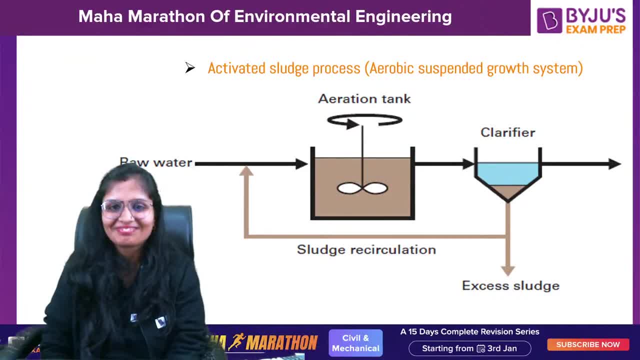 Guys, shall I start or break? Come on, tell me fast, Fast, fast fast. Tiksha, Sheersh and you guys will be coming also, or after break or not. Tell me that also. Okay, Now the subject is not break. 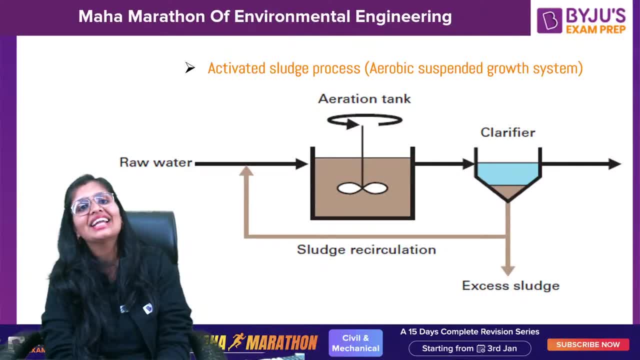 We have ASP left, We have sludge digestion tank left, We have numericals left, We have solid waste management, air pollution. Okay, Okay, Promise me and go break till 6 pm. Okay, We will meet at 6.. 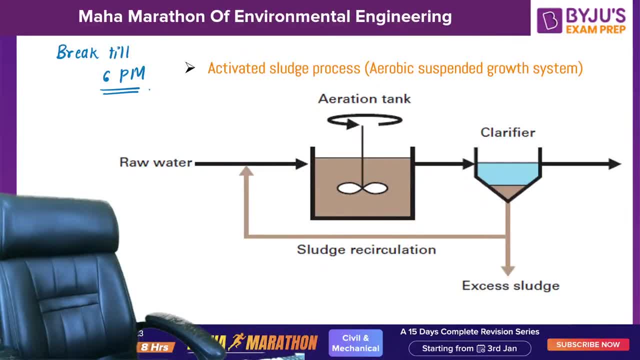 5 pm. We will meet at 7.. Bye-bye, Bye-bye, Bye, Bye, Bye-bye, Bye, Bye, Bye, Bye, Bye, Bye, Bye, Amen, Amen, Amen, Amen, Amen. 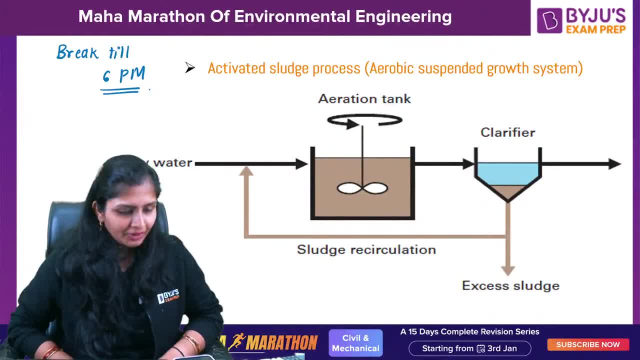 for the case of oxidation ditches, Girish. Okay, So now we will be talking about activated sludge process, which is aerobic. Here we won't take the atmospheric oxygen, We will be supplying oxygen. Moreover, this is a suspended growth system, like the paneer pakoda, and you both are there. 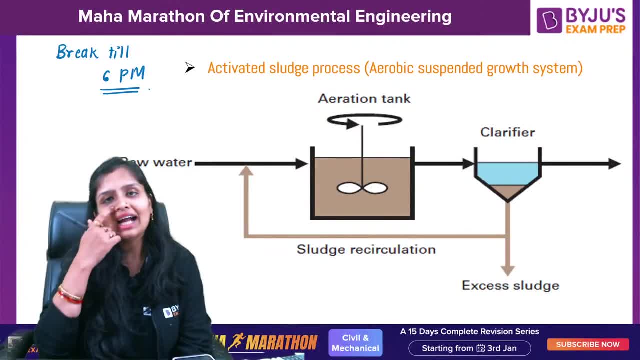 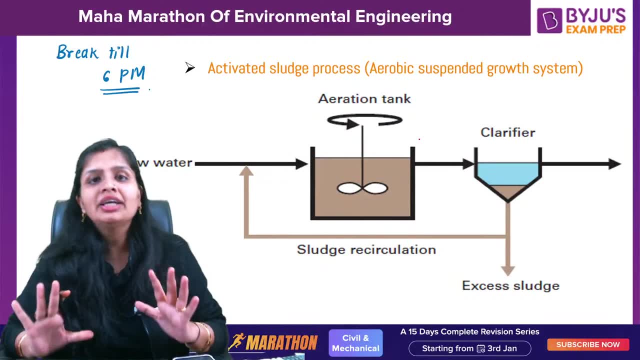 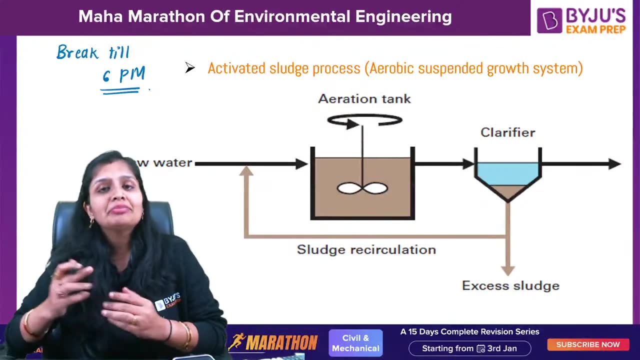 in the party. Okay, So now you can see this activated sludge process. You can see this activated sludge process. Now, what happens is here: the efficiency is quite high, but you are the one who will be supplying oxygen In this. mixing is done. 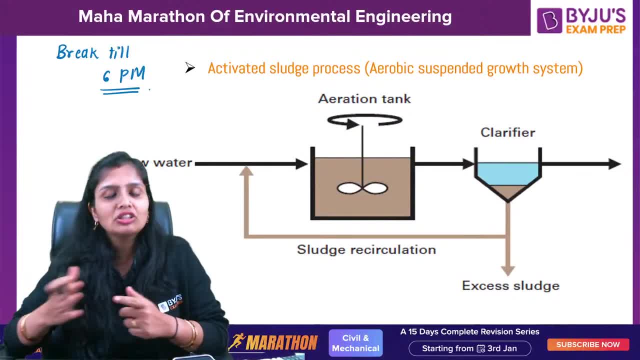 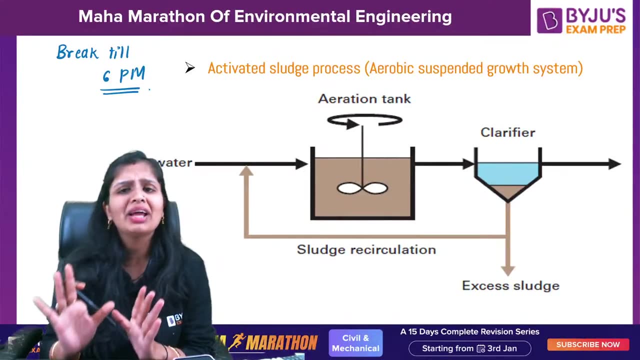 When you do mixing, what you do on the basis of mixing, when you do mixing, the opportunity of contact between microorganisms and organic matter increases. Activated sludge process: Remember: in any treatment unit you don't apply SST, no issues. SST means secondary sedimentation time. 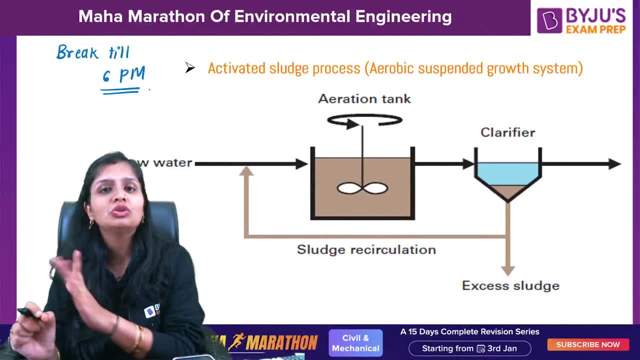 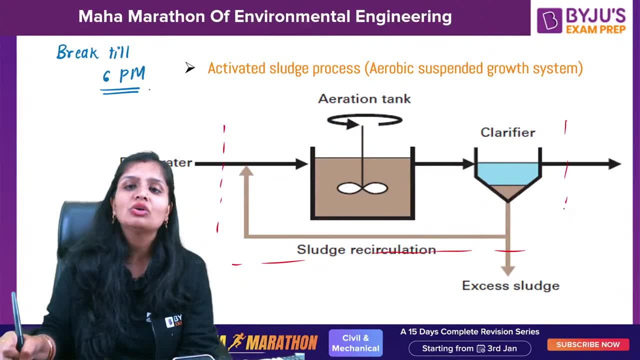 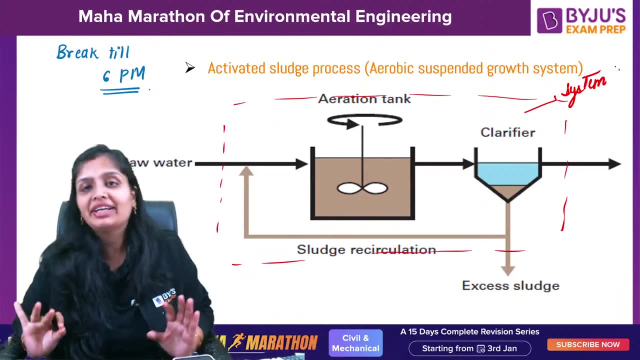 But if, in the case of activated sludge process, you don't apply SST, this activated sludge process will not at all function. So that is the reason. this is the whole system which you will see. This is the whole system of ASP. This is the whole system of activated sludge process. 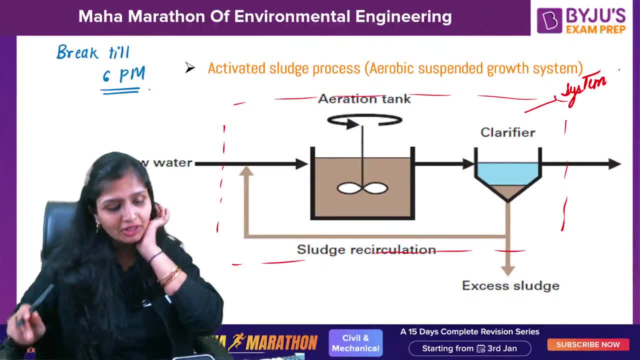 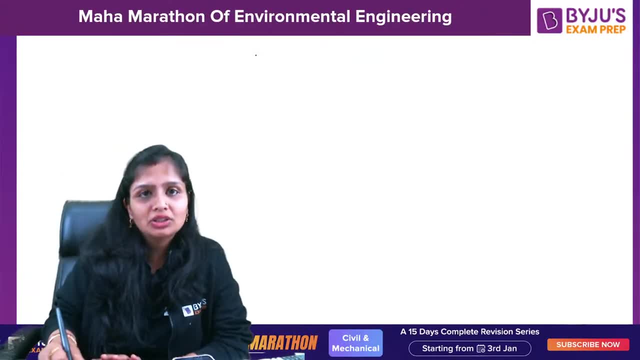 Okay, Now, now talking further. now talking further. When you talk about activated sludge process. when you talk about activated sludge process, let's go. This is the aeration tank, This is the SST. From here, what you are doing? it recycling it, recirculation. 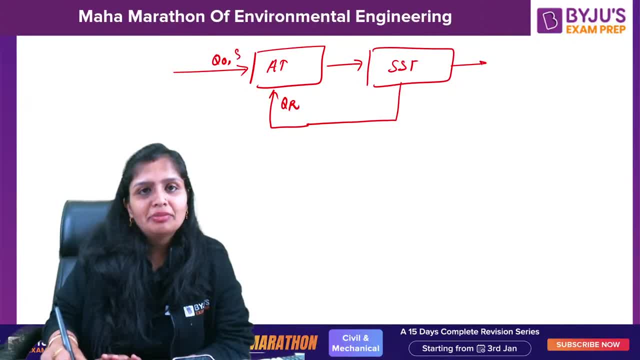 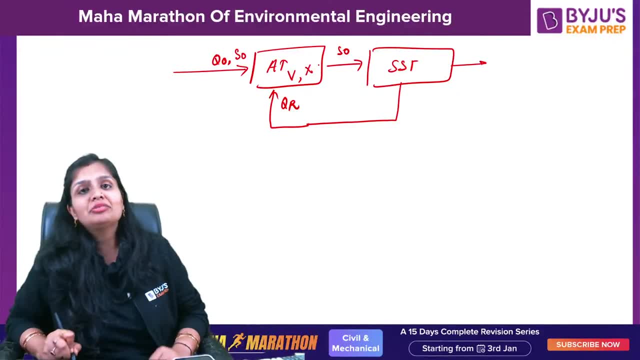 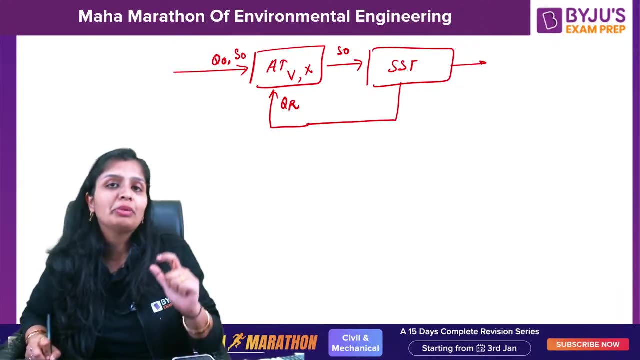 This is Q naught. This is the BOD which is entering The BOD which goes: This is the volume of the aeration tank. This is MLSS. MLSS means mixed liquor, suspended solids For reporting microorganisms. you report it in terms of suspended solids. 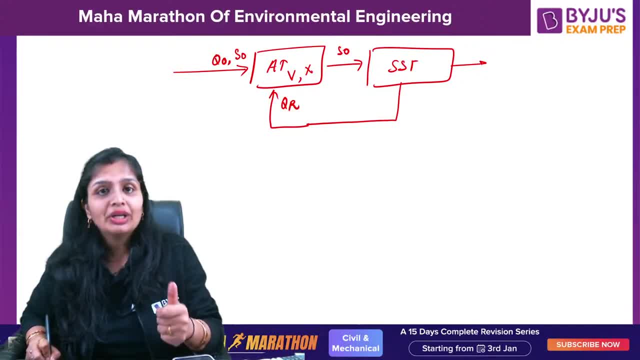 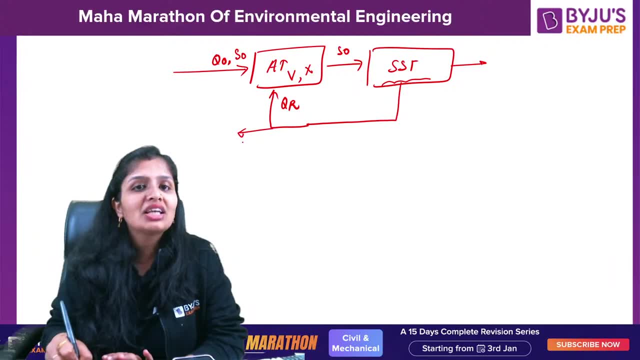 Which is you tell it as MLSS. Okay, mixed liquor suspended solids. A part of the sludge here is recirculated, A part of the sludge is wasted. QU is known as useful sludge. Okay, And this is the QE, the discharge S and this is XC. 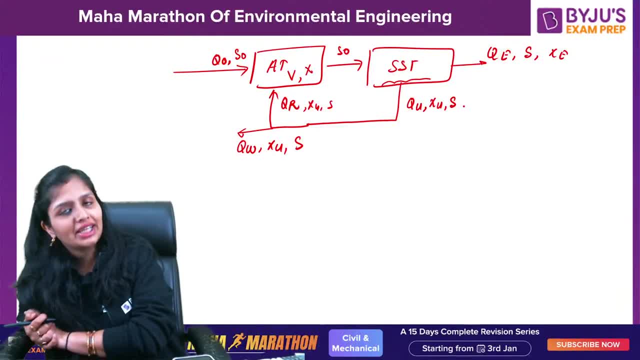 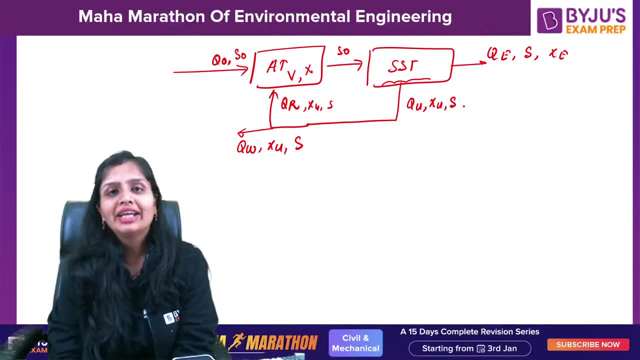 Actually, in SST also, BOD removals takes place. But you assume that no removal of BOD takes place in the case of. No removal of BOD takes place in the case of secondary sedimentation tank. Okay, We assume whatever is the BOD here. 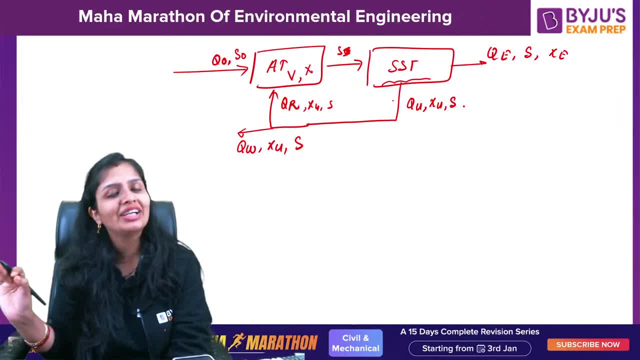 Here the BOD is S, Here the BOD is L. No removal will take place, But the truth is, some amount of BOD gets removed. Now what happens Here? you are recirculating a part of the sludge. Why? 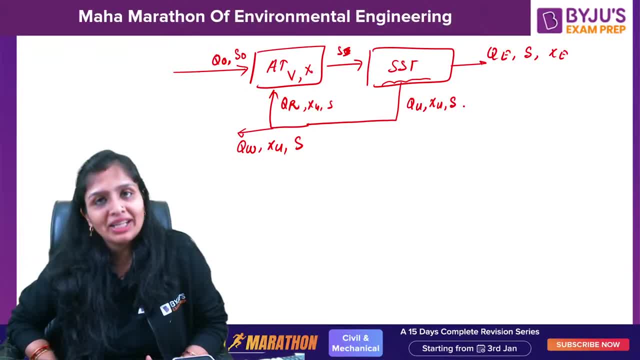 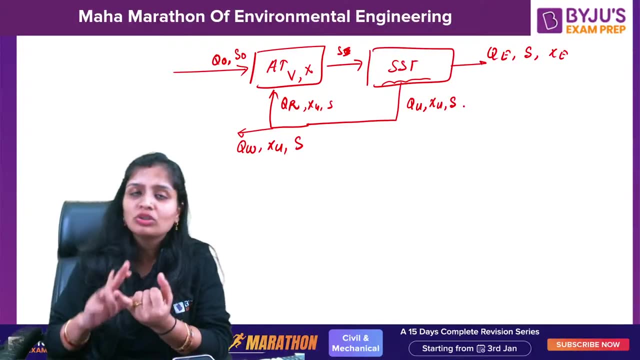 Because if microorganisms will be present, the decomposition will take place at a rapid rate, Means in lesser amount of time, more amount of organic matter will be decomposed. Now, if you don't provide this SST, There will be no recirculation, No recirculation. 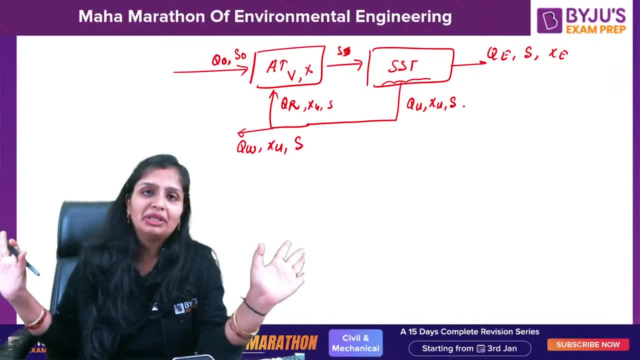 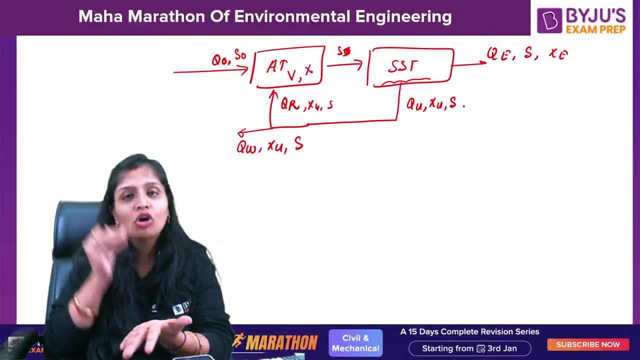 No ASP, No activated sludge process. So if you want the function to take place, If you want the ASP to operate, it is very, very mandatory that you need to do the recirculation. Okay, Now, coming further, there are some parameters which you should know. 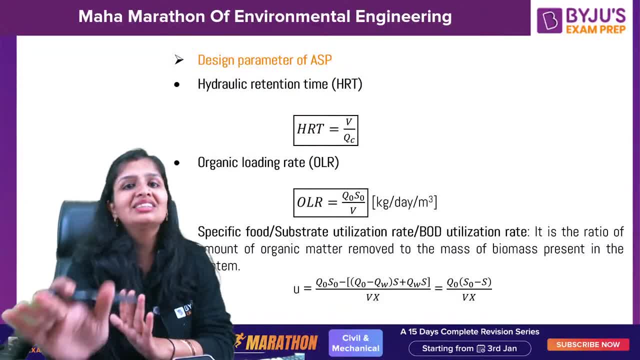 First is the hydraulic retention time. So this hydraulic retention time is equal to the volume by discharge. If Q0 is the discharge and B is the volume, Then Q0 is the discharge, So Q0 is the discharge, So Q0 is the discharge. 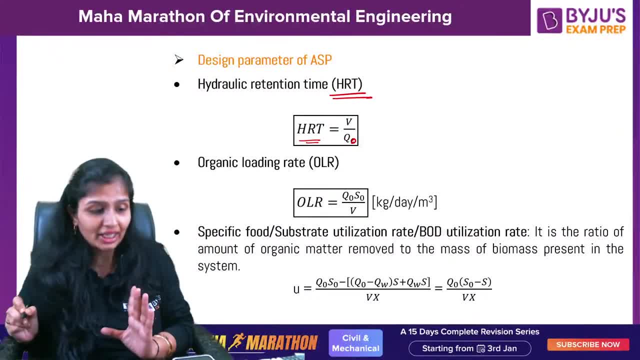 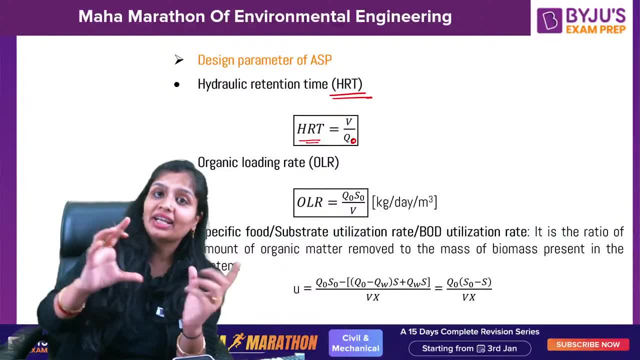 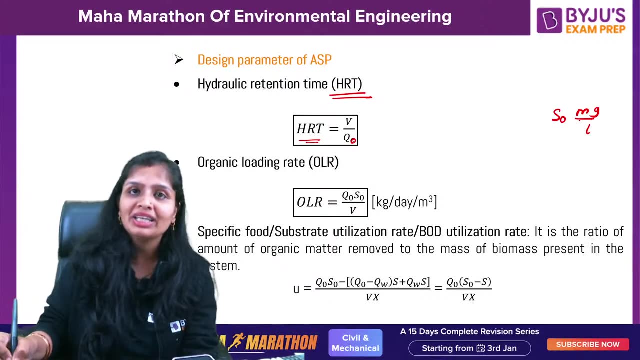 So Q0 is the discharge And V is the volume of the aeration time. So it will become V by Q0.. Organic loading rate means the rate at which organic matter is loaded into the aeration time. If in 1 liter S0 was the BOD, or BOD means BOD, organic matter. 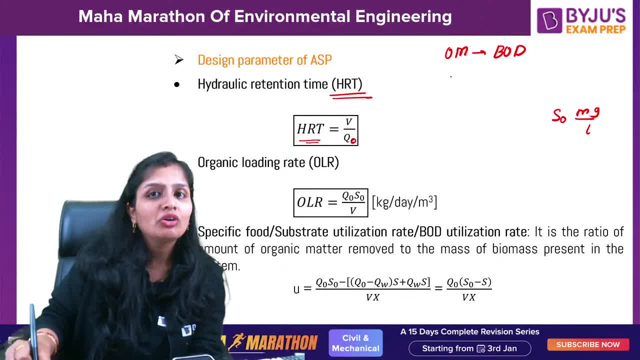 We report in terms of BOD. Microorganisms. we report, If you want to know, quantitative analysis of it. So on quantitative basis, Microorganisms. you report it in terms of MLS. So if in 1 liter S0 is the BOD, 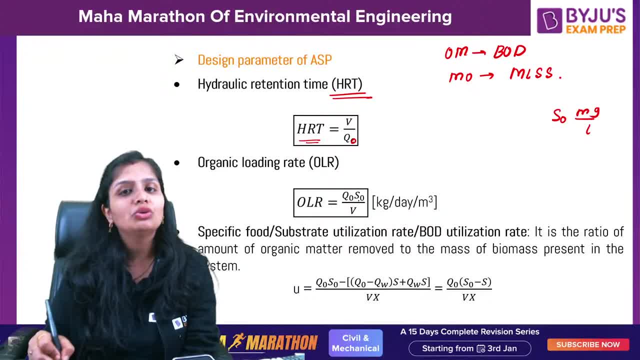 So in Q0, how much will be the BOD? Q0 S0 divided by V? This will be the organic loading rate. Okay, Third is specific food, or you can say BOD utilization rate. So it will tell you how much BOD is removed. 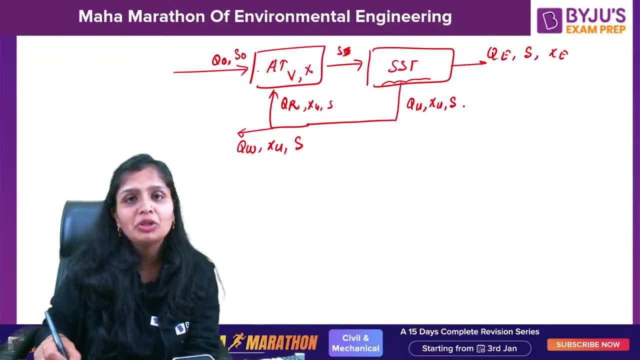 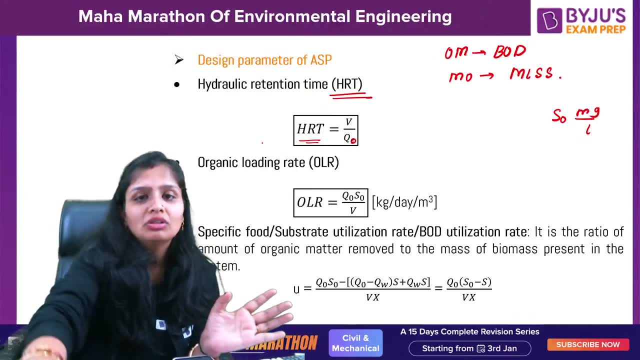 Now see Q0. S0 was the BOD which is coming And which is the BOD which is coming And which is the BOD which is going out. Which is going out. One is QW into XU. QW, it is going out. 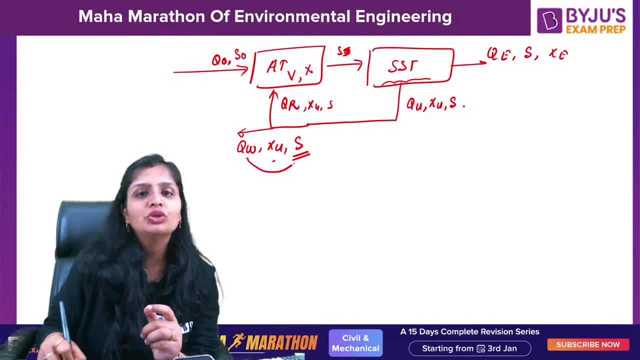 Okay, XU suspended solids. This is BOD, So QW into S. This BOD is going out of the system. You can write it QE or you can write it as Q0 minus QW- Anything you can write Into S. 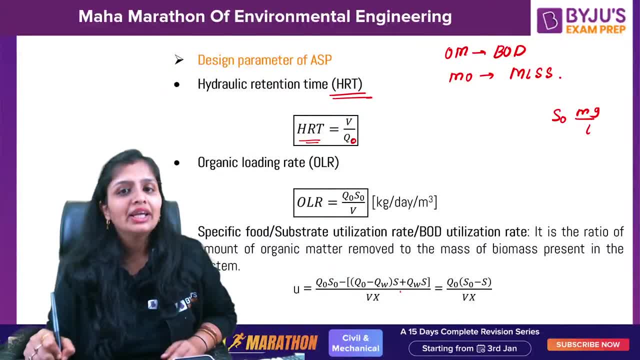 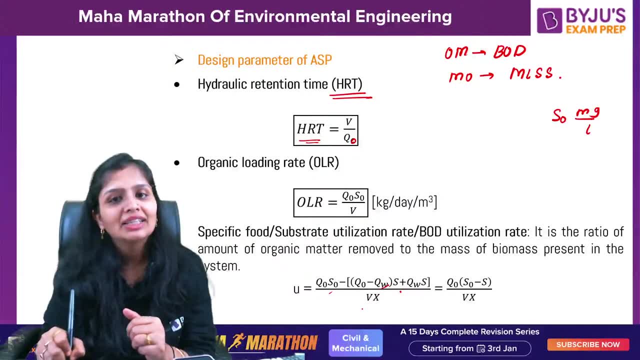 This is going out. This is going out. Okay, So this is the BOD which is going out. So the remaining BOD, So the remaining BOD is the one which is removed, divided by the microorganisms If in one liter, X microorganisms are present. 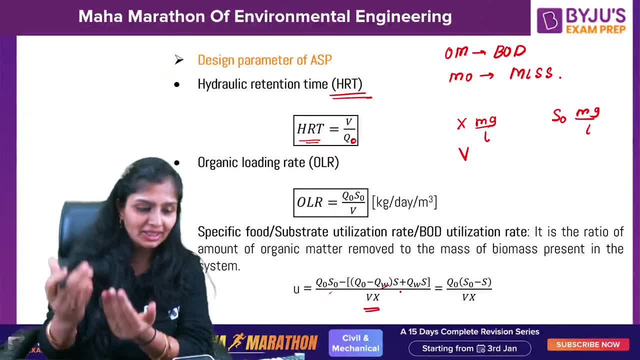 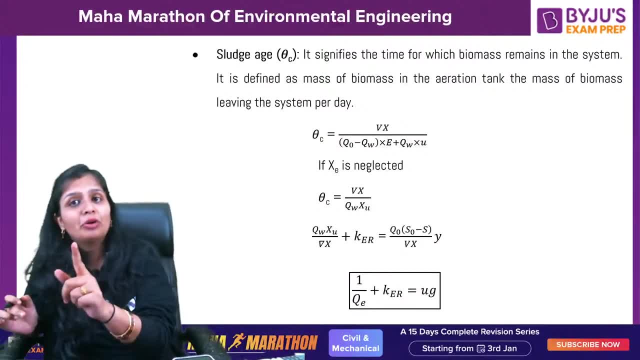 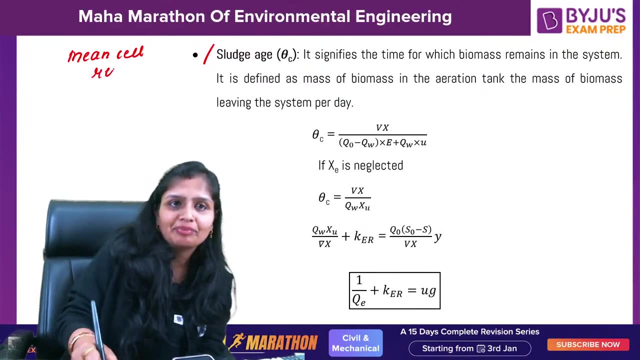 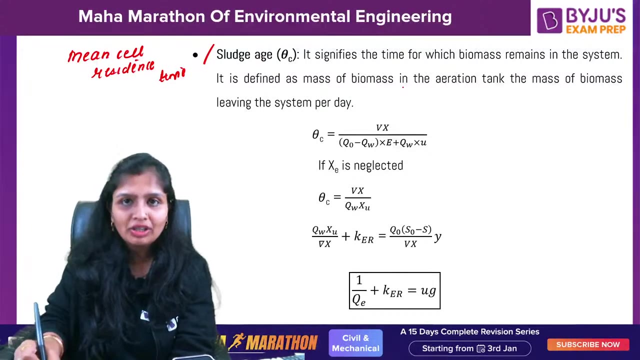 So in total volume, how much microorganisms will be present? V into X, Simple. So this will tell you BOD utilization rate. Large, H, Very important. There is another name for H, or H, which is mean cell residence time. So it will tell you mass of microorganisms. 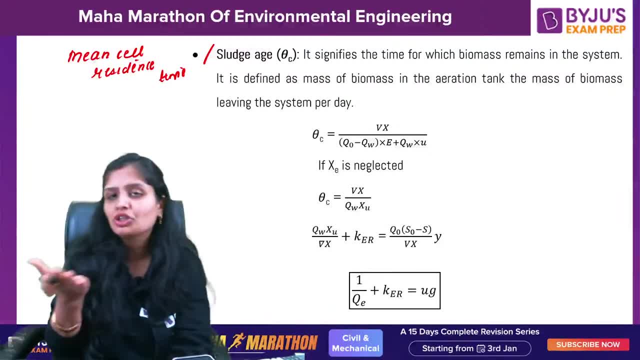 Biomass means microorganisms. Microorganisms, you reported, in terms of suspended solids, So mass of microorganisms in the aeration tank, which is V into X, Divided by those microorganisms which have left the system. They are no more present. So which are the ones? 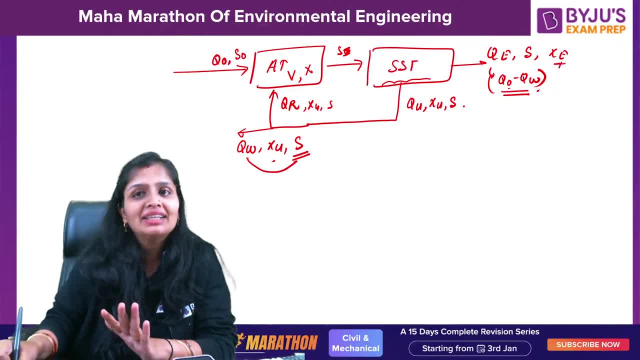 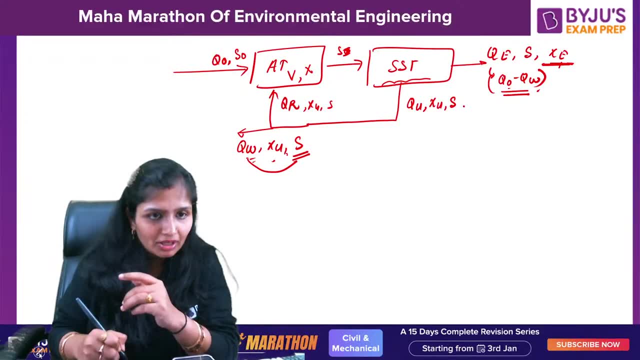 This is Q0 minus QW, XE, Because X you do it for microorganisms, And here QW into XU. This is the system. I will draw it with a double pen. This is the system. Okay, So this is going out. 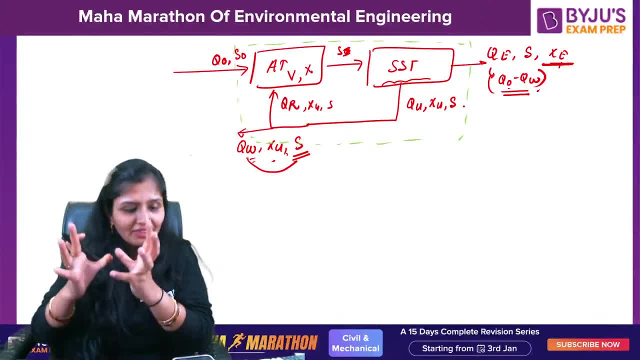 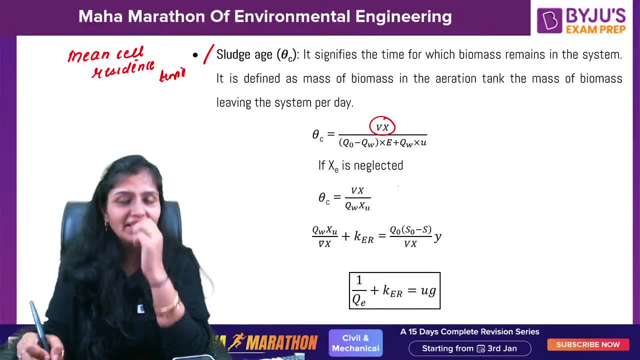 This is going out. So the microorganisms which are there divided by the microorganisms which has left the system. Okay, So this you should know. this is Generally: if in the quotient they haven't given you the value of XC, Takes XC as 0.. 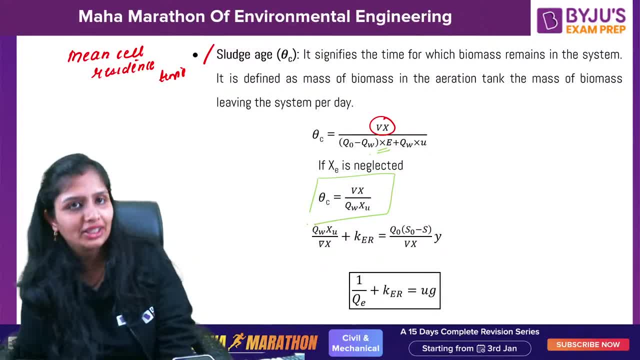 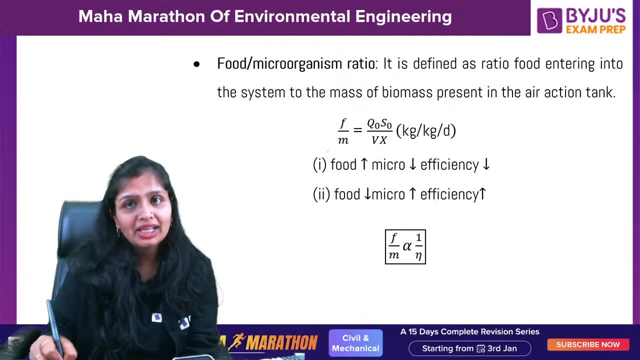 So you will get theta C as VX upon QW X. Okay, Now this is very important: Food for microorganisms ratio. Why? Because it inversely governs the efficiency. How come? Let me tell you See, if food is more, microorganisms is less. 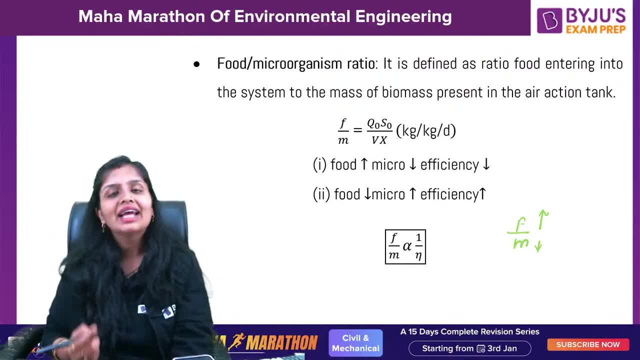 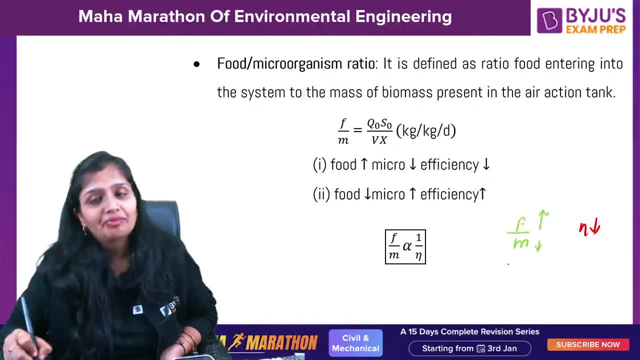 Like khaane wale zyada hai and khana kam hai. Okay, That means what? Composition will not be complete, So efficiency will reduce. Inversely, food by microorganisms is less, Food is more, or food in this case, food is less microorganism. 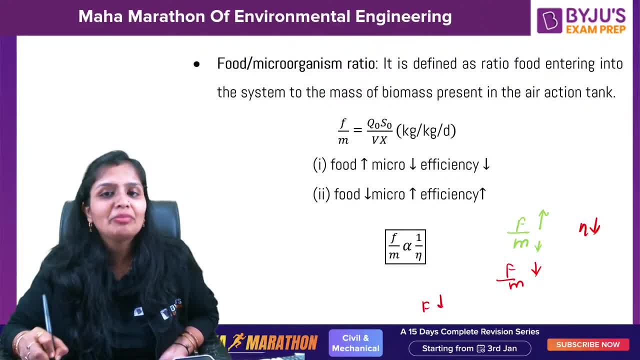 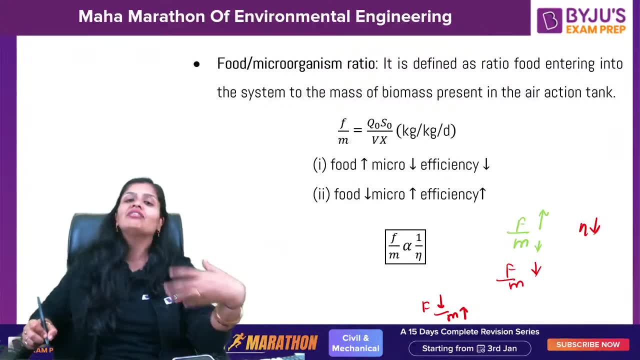 When F by M will become less, When F will be less and M will be more, So this whole ratio will become what Less. So that means khaane wale kam hai, khaane wale zyada hai. So in this case, what will happen? 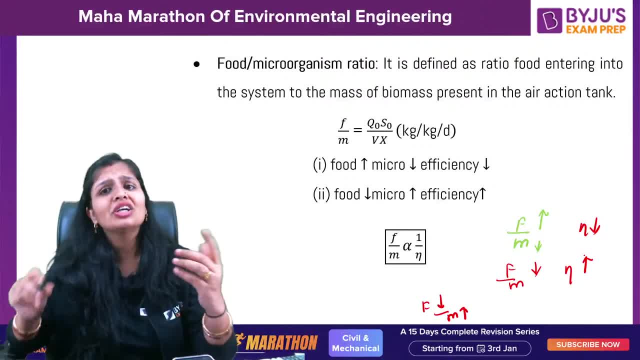 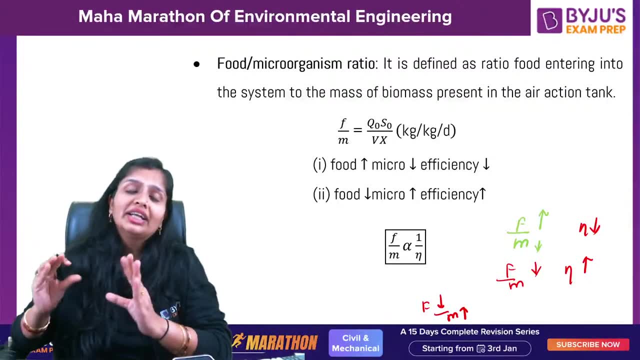 More efficiency will be there. Ma'am, Efficiency you are talking means what you are talking. Efficiency I am talking means I am talking the removal of, or you can say the decomposition of organic matter. So more is the F by M ratio, Lesser is the efficiency. 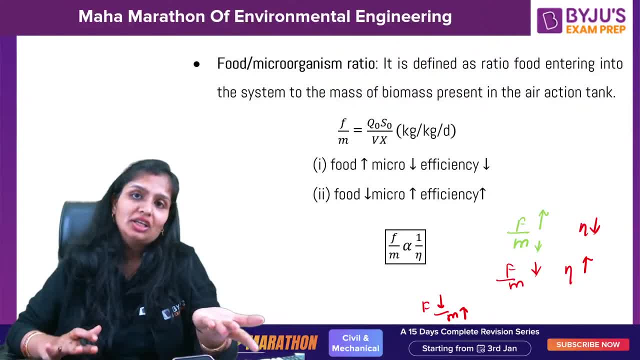 Lesser the F by M ratio, more is the efficiency Clear. So the unit of F by M is day inverse, But technically they write it in terms of kg per kg per day. Food is what If in 1 liters? What is the BOD in the whole discharge? 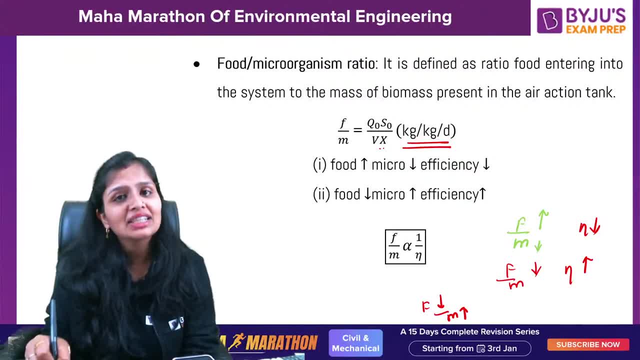 How much will be the BOD Multiply? If X amount of microorganisms are there in 1 liter, How much microorganisms will be there in the whole volume, Just multiply? Okay, This is there. This again recirculation ratio. 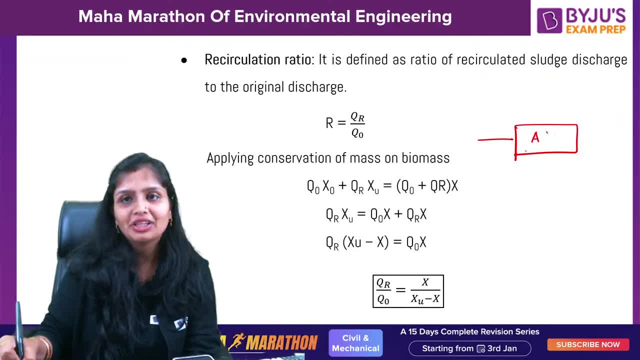 This is important, Everything is important here. Aeration tank is there, Q naught, X naught is the microorganisms Okay, SST is there, Okay, XU. So when you apply conservation of mass here, What you will see? 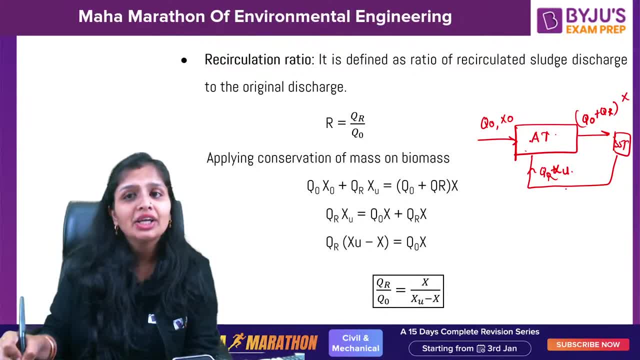 Q naught, X naught is entering into the aeration tank. QRXU is entering into the aeration tank. How much is going out of the aeration tank? Q naught plus QR into X? Okay, So from here you just erased it. 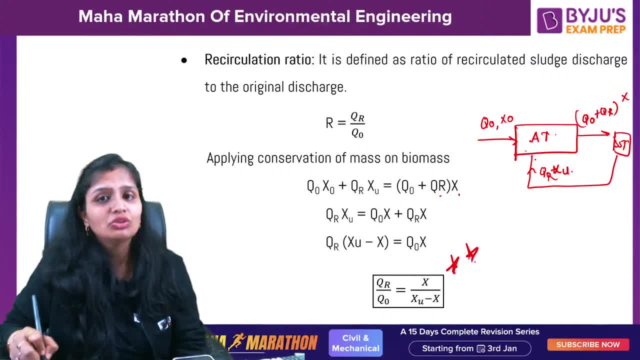 You will get the recirculation ratio. They can ask you. So you should know this. QR by Q naught is X, X is the MLSS concentration, XU is the useful sludge minus X, Which is the MLSS concentration. 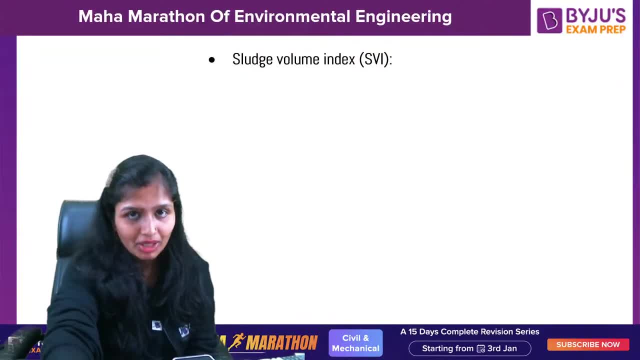 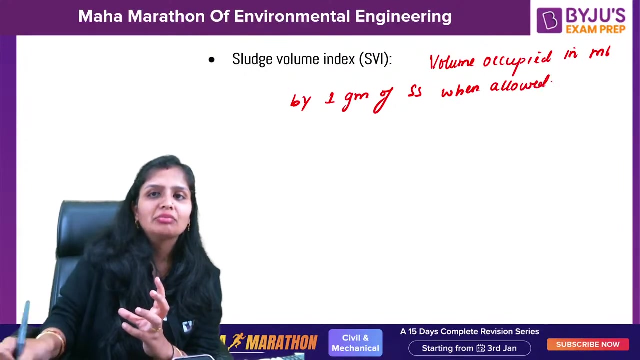 Okay, This is the recirculation ratio. Now Sludge volume index. This tells you the volume occupied in ml. How much volume is in ml? How much volume is occupied in ml By 1 gram of suspended solids When allowed to settle for 30 minutes? 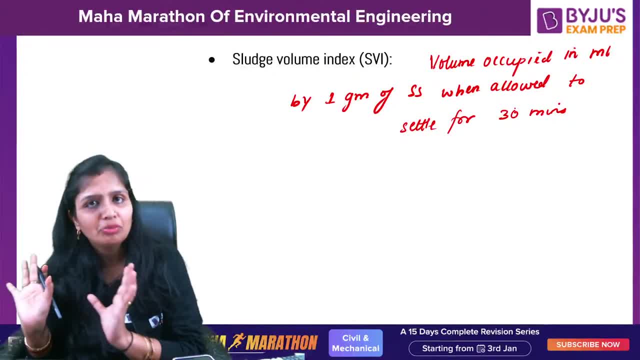 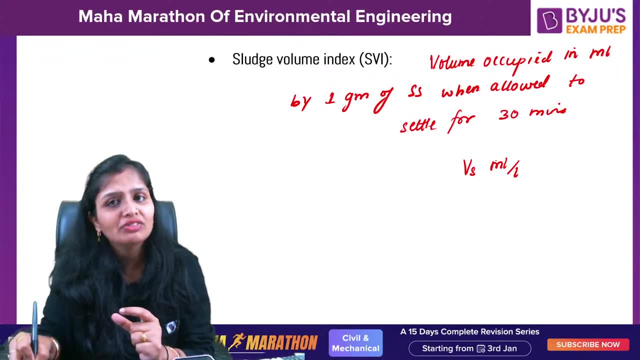 See, You have taken a sample. You have put it How much volume it occupies. Let us suppose it occupies Vs volume 1 liter of the sample you have taken. It occupies Vs volume. Now you take the sample back, Mix it. 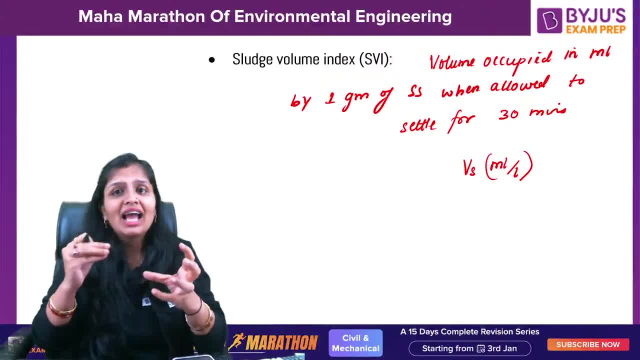 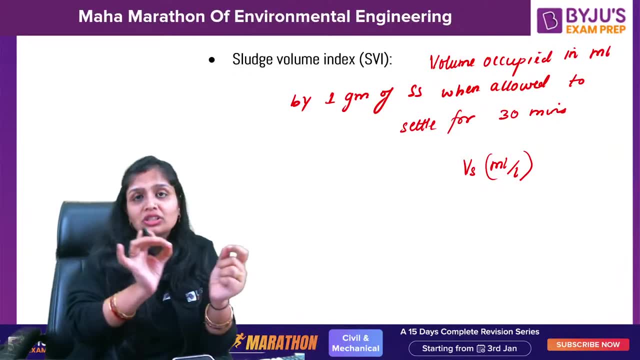 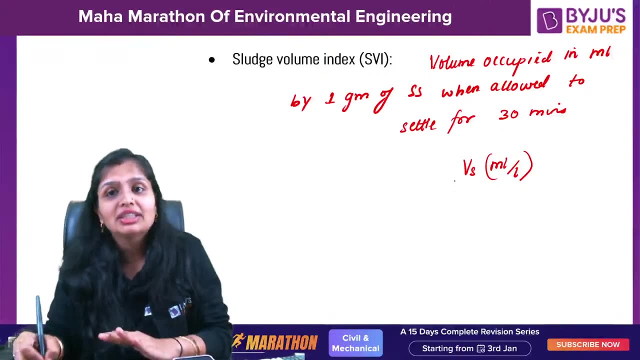 The suspended solids which you have taken, Mix it And calculate the weight of it. Okay, Calculate the weight of it. You will calculate the weight by the similar process how we calculated suspended solids. Okay, How you calculated suspended solids. So let us suppose the suspended solids comes out to be excess. 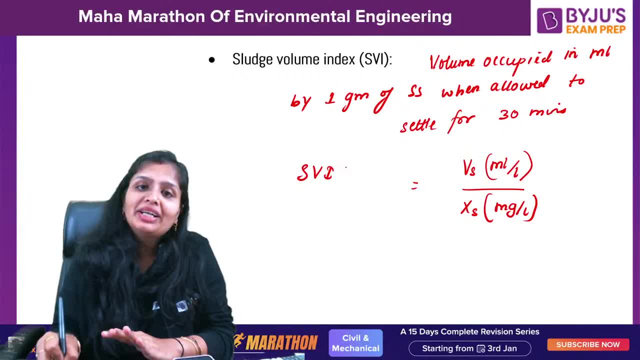 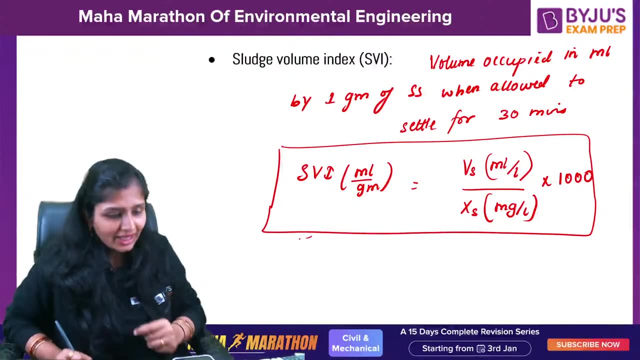 Remember, The unit of sludge volume index is ml per gram And here from here you will get it in ml per mg. So that's why you need to multiply by 1000.. So this is the formula, Mam, you said in ASP. SST is not a function. 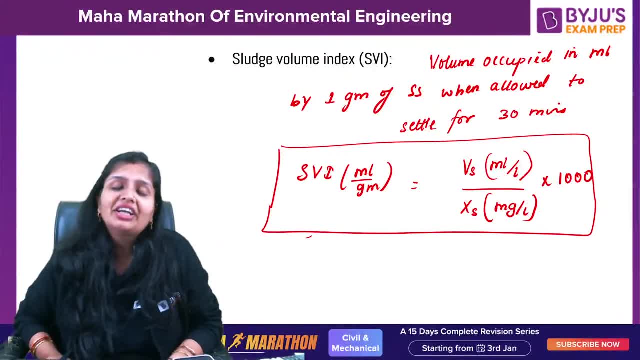 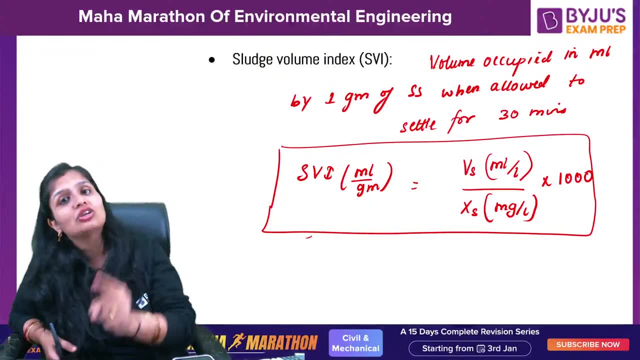 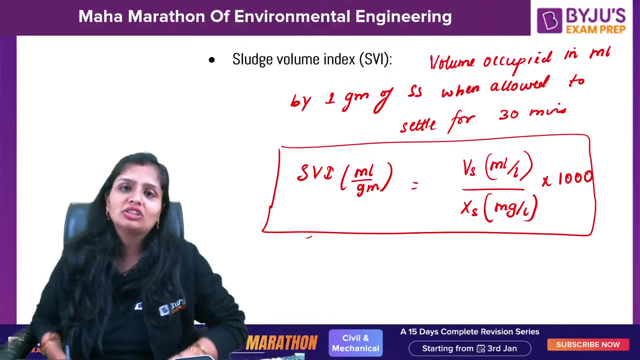 SST is a function. I said MVS. If in any treatment unit you don't apply SST, Not an issue. But in the case of ASP, If SST is not there, It will not function. only Okay, I said that. So it is very, very mandatory to have an SST in the case of activated class process. 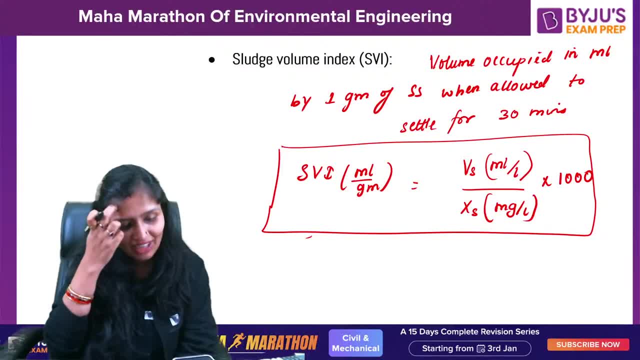 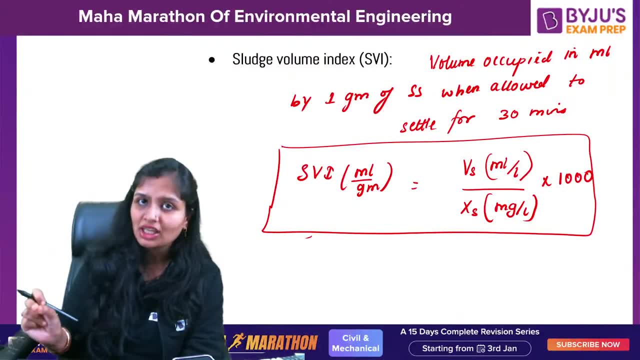 Okay, If MLSS and MLVS- both are given, Then we will take it. MLVS is mixed liquor- volatile suspended solids. Okay, Because it is more accurate. in mixed liquor suspended solids Inert organic matter and dead cells are included, While in MLVS is dead cells are included. 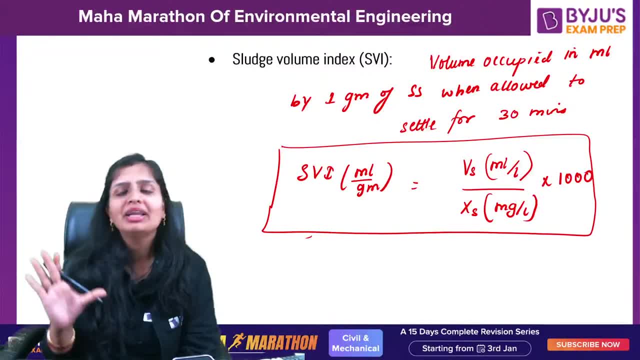 Dead cells are not included. That is the reason we go for MLVS. But MLVS is time consuming to compute. That is the reason. in maximum case they gives you MLSS And we use that. But if it is given, you will use MLVS. 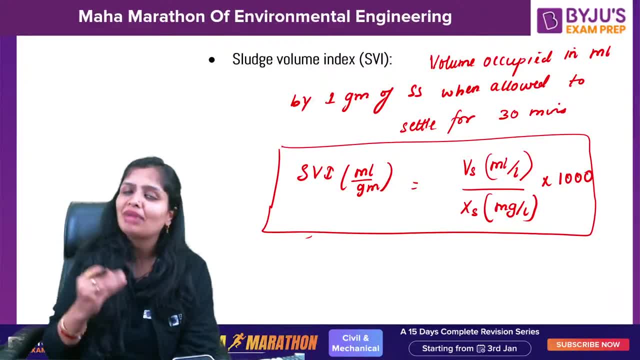 Clear. Okay, Now solve this question. Here you have to calculate hydraulic retention time F by M ratio, BOD removal efficiency, sludge age, Everything you have to calculate. Come on, guys, Waste of time, Waste of time, Waste of time. 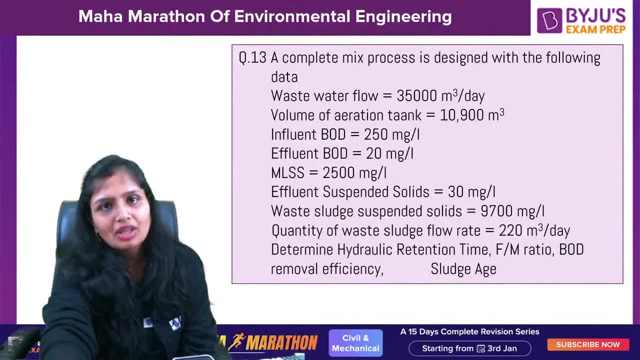 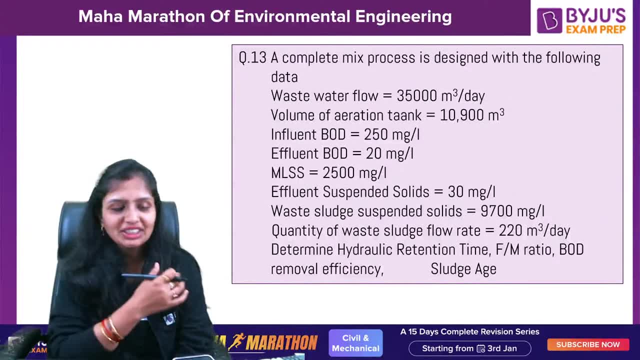 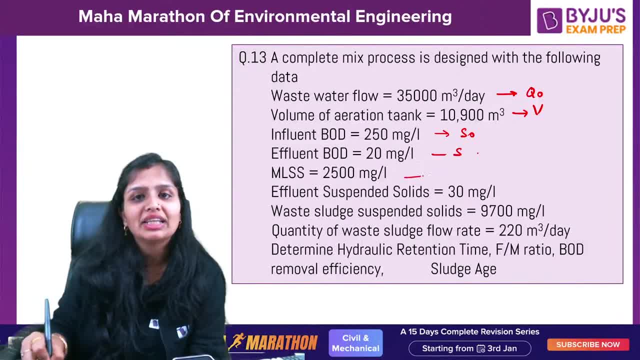 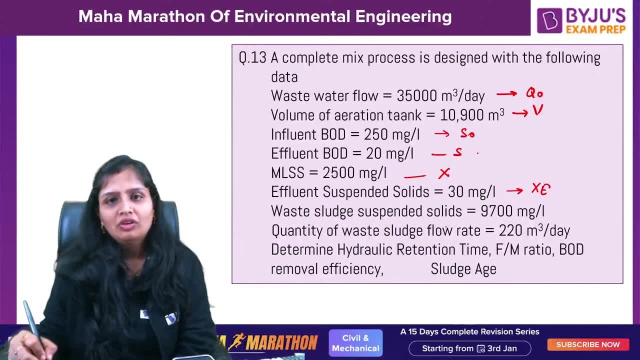 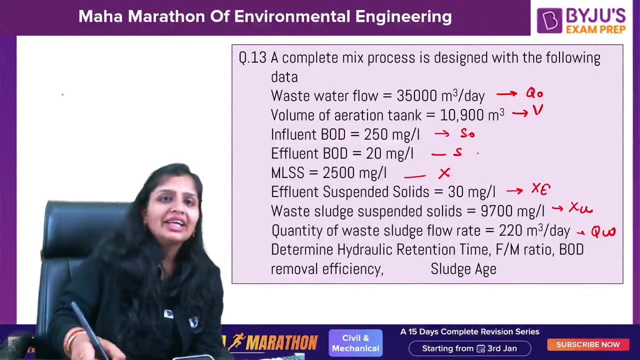 Volume: Influent BOD S, not Effluent BOD S- MLSS. Effluent suspended solids- Wasted sludge. suspended solids Sludge QW. See, I have written everything for you guys. Hydraulic retention time is very simple. 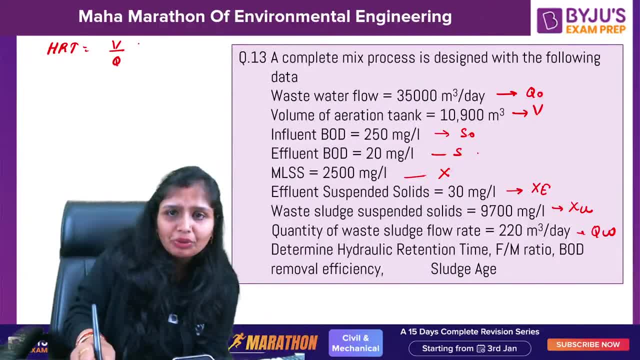 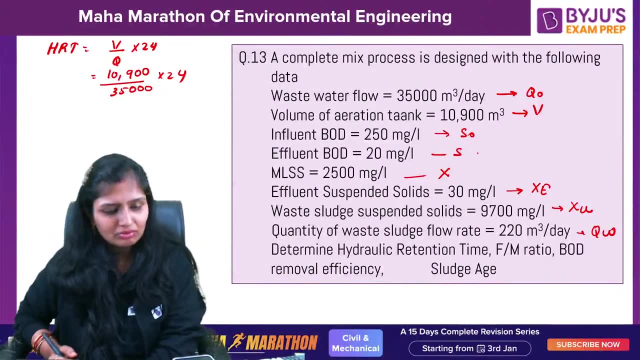 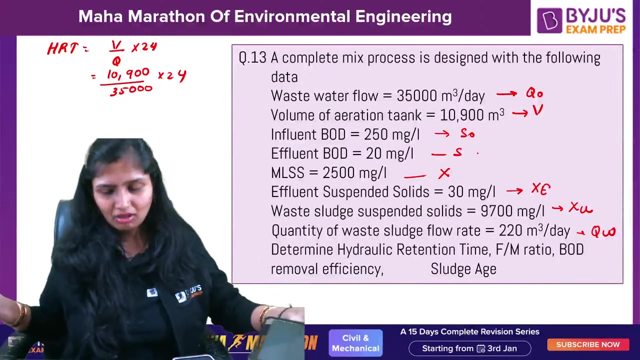 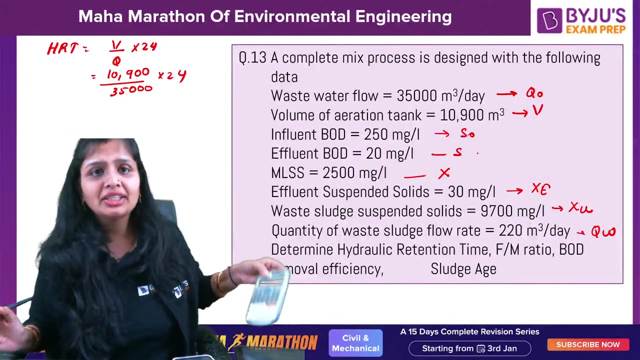 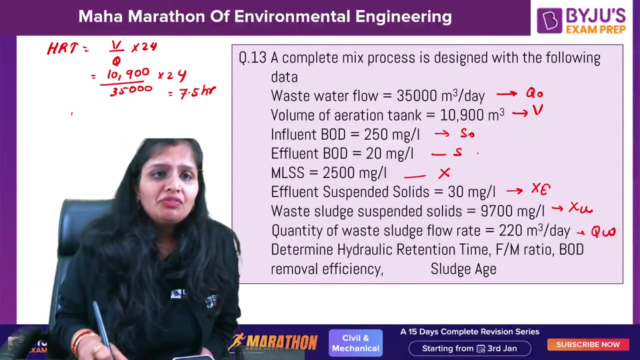 So V by Q into 24.. How much it is coming. How much it is coming. Come on guys, fast. Hydraulic retention time. then food by microorganisms. ratio Q S naught by VX, Q is 35,000, VOD is 250, volume is 10,900 into 250.. 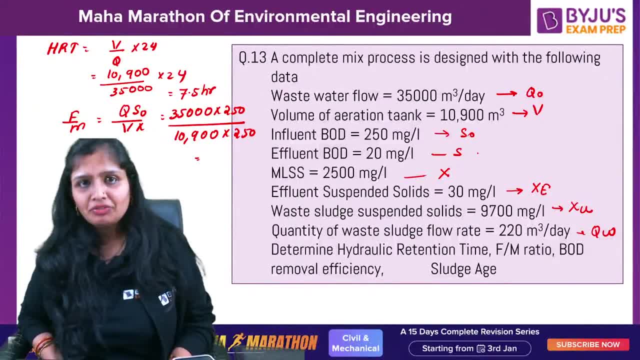 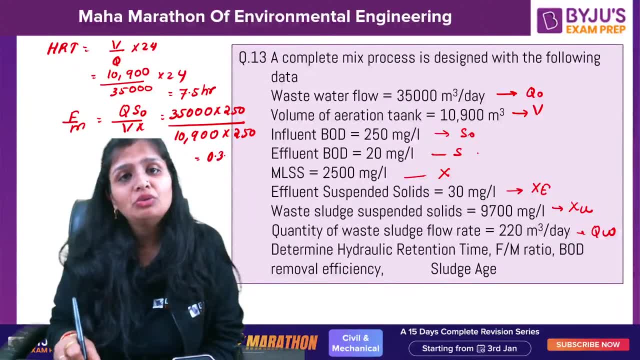 Everything, Everything will get cancelled out, so don't worry. regarding it, 7.47, that is 7.5 I have taken. This comes out to be how much 0.32 day inverse. Next is BOD removal efficiency, which she has already told. 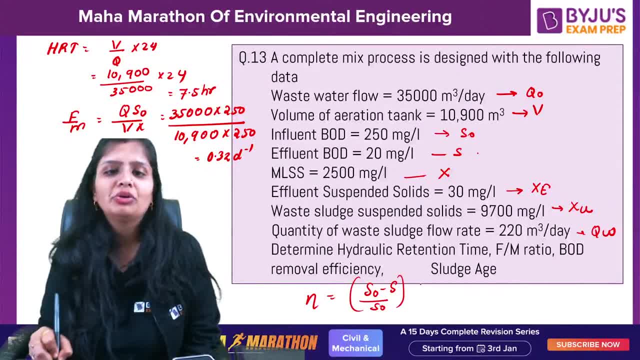 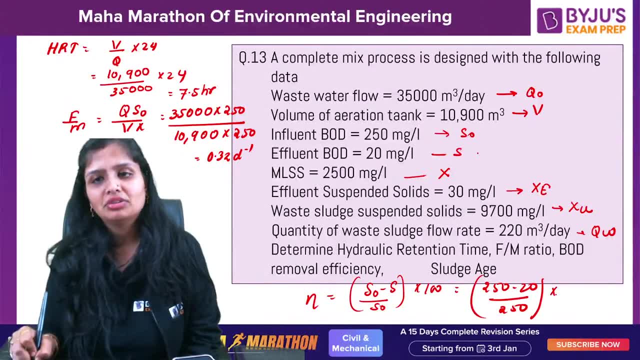 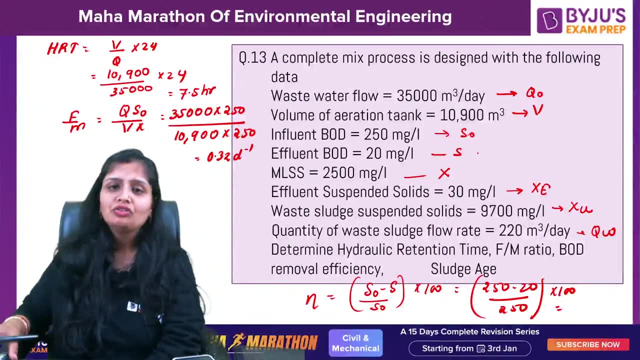 Influent BOD, minus effluent BOD, divided by influent BOD into 100.. So 250 minus 20 divided by 250 into 100.. Simple, How much, How much it is coming 250 minus 20, 230.. 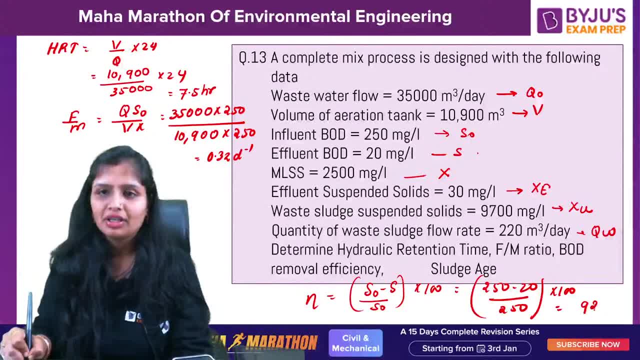 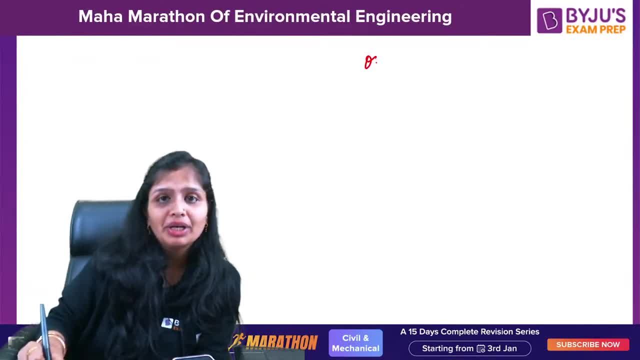 23 into 100, 92%, Fine 92%. Last is sludge age. Remember in this question a sludge age, sludge age. when you do it volume, how much is going? So in the previous case it is Q naught minus QWXC plus QWXU. 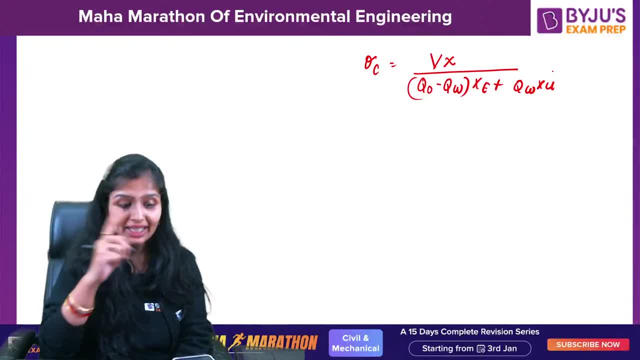 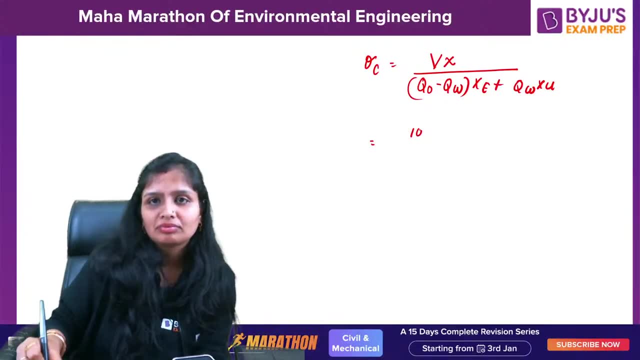 In this question, XC is given to you, So you cannot take it as 0.. You cannot take it as 0.. Remember that Volume is how much: 10,900.. 10,900.. X is how much: 2,500 mg per litre. 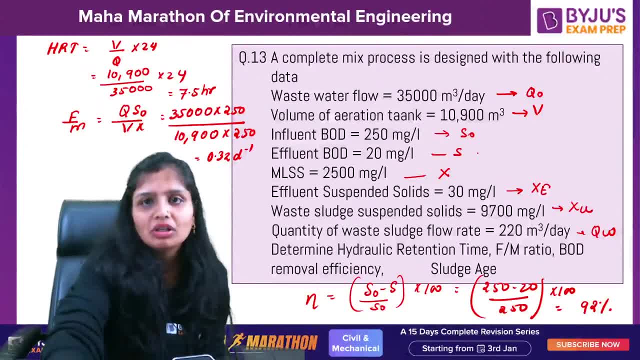 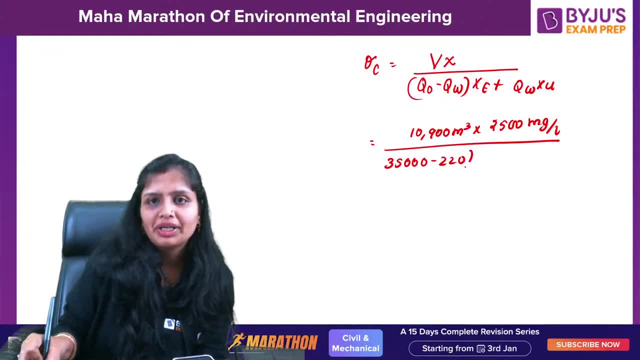 Q naught minus QW. Q naught 3,500 minus 3,500 minus 220.. 3,500 minus 220.. Correct Into XC. XC is given to you as how much: 30. Plus 220 into XU. 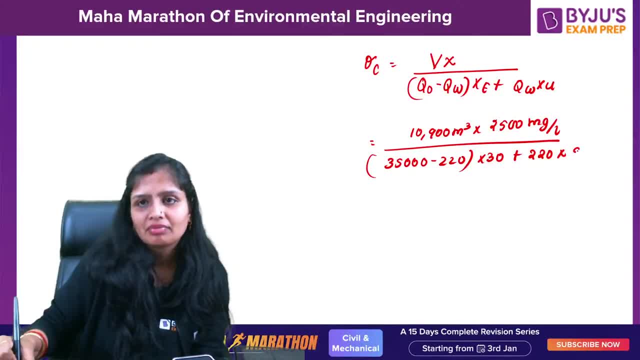 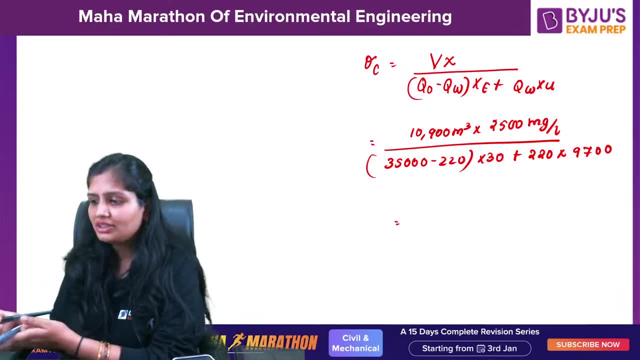 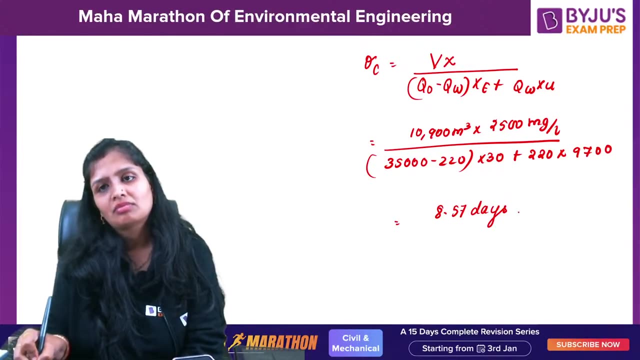 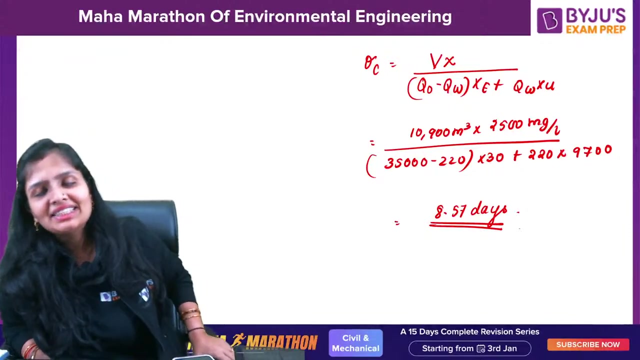 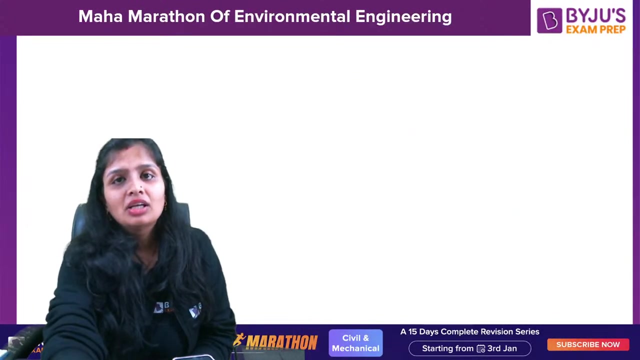 XU is given to you as 9,700.. How much it will come? How much it will come, fine. so it's not necessary that in every case effluent suspended solids is zero. in some cases they can give you. so make sure you know that. okay, so this is the sludge. 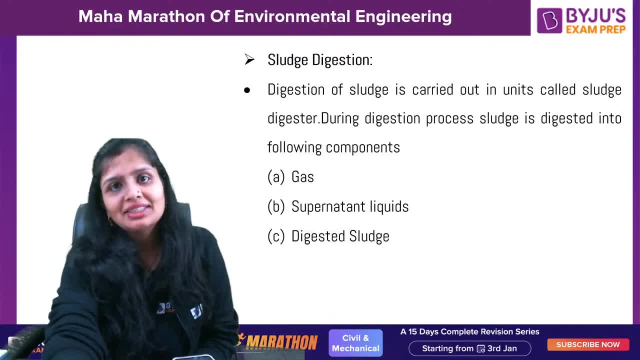 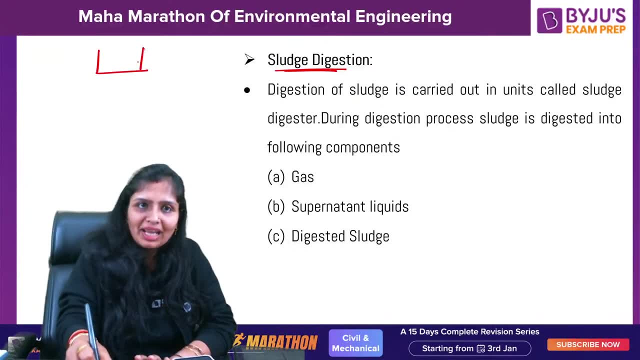 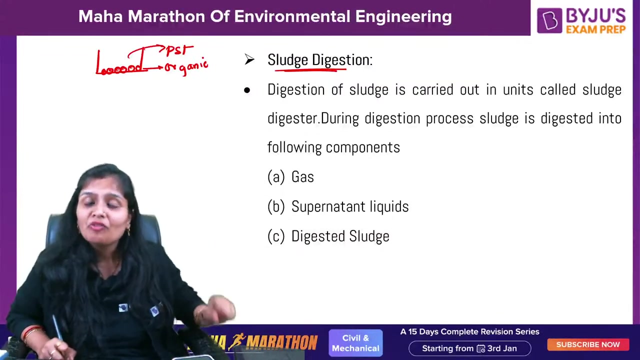 fine. so the last topic, i guess that is the sludge digestion, or the digestion of sludge. okay, so, whatsoever from the primary sedimentation time, whatsoever. suspended solids- organic suspended solids- settle. okay, organic suspended solids, settle. you don't throw it directly. why, ma'am? because if you throw it in the river, microorganisms will take out the rivers. 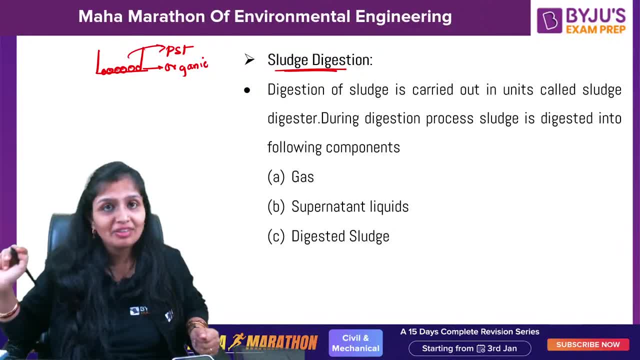 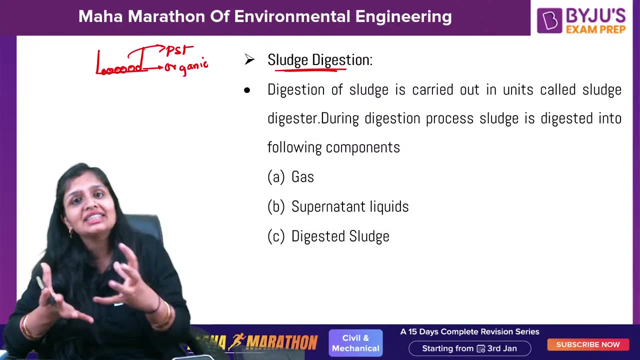 dissolved oxygen, aquatic life. survival will be difficult. if you throw it in the land, it will take atmospheric oxygen. so that is the reason you have to treat it. for treating it, you have to go into the sludge digestion chamber. Now, when you digest it, you reduce it. okay, when you reduce it, it comes into three components. 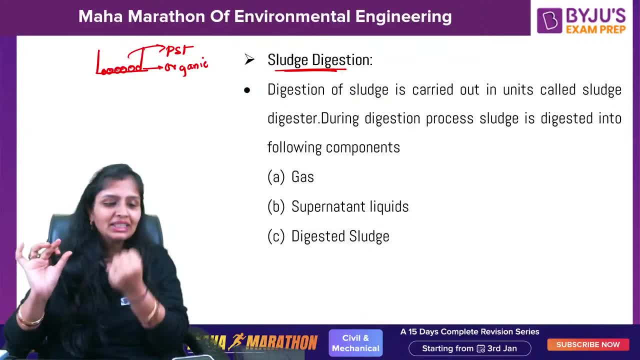 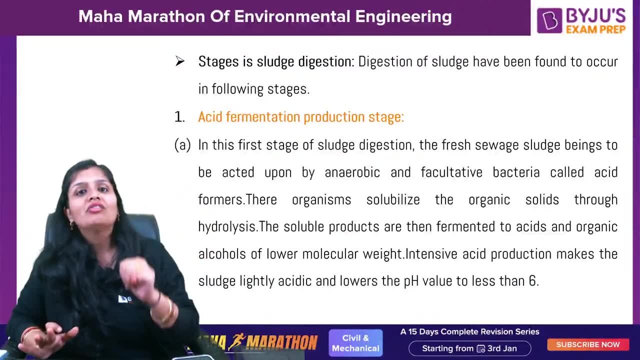 gases, supernatant liquid, digested sludge. basically, you get solid liquid and gas. now, coming further in this, you have three stages. one is acid fermentation. what happens here? acid formers. so what they will do is aerobic and facultative bacteria are there. they will convert the acids. 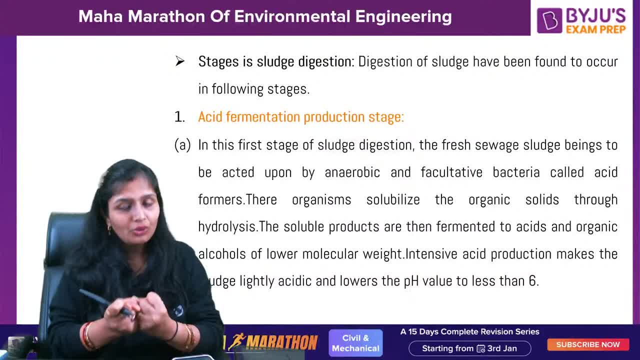 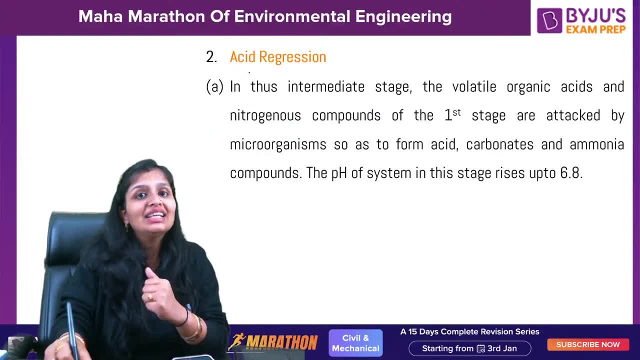 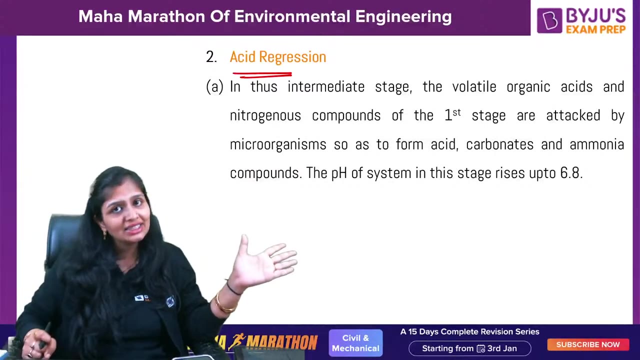 reduce it into lower molecular weight. okay, the ph becomes less than 6.. After acid fermentation, you have acid regression. the acids which are produced in the first stage are attacked by microorganisms and they convert it into carbonates and ammonia compounds. the ph, which was less than six, now the ph, rises up to 6.8. after acid fermentation you 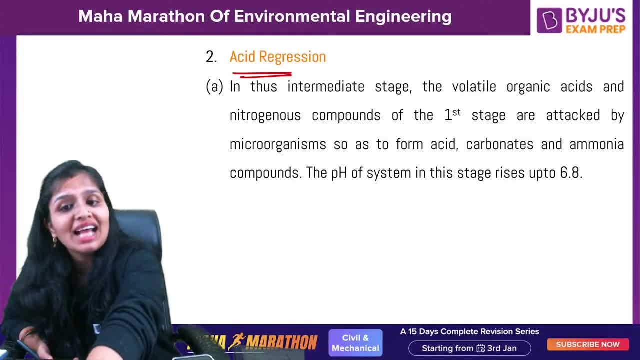 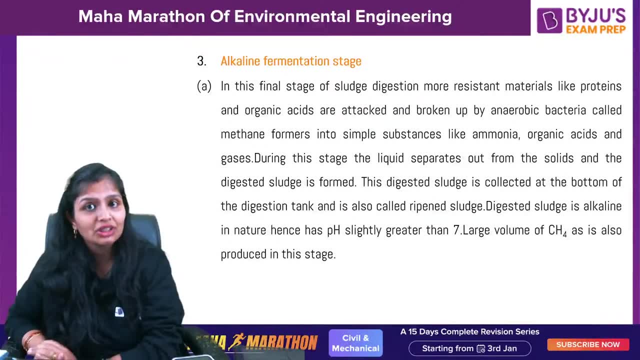 reach acid. that is six-point, six episodes, 6.8.. regression: you have alkaline fermentation. In this stage, methane formers comes into action. What they will do? They will take the acids and oil which is produced in the previous stage. 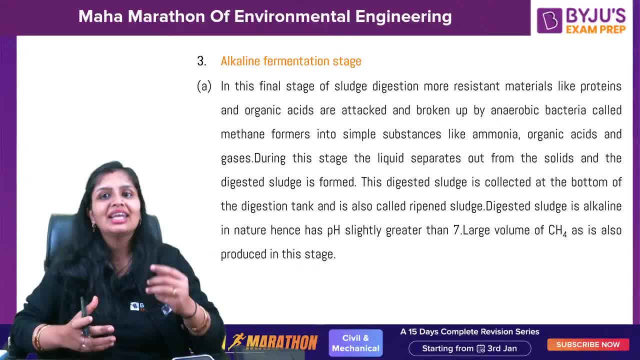 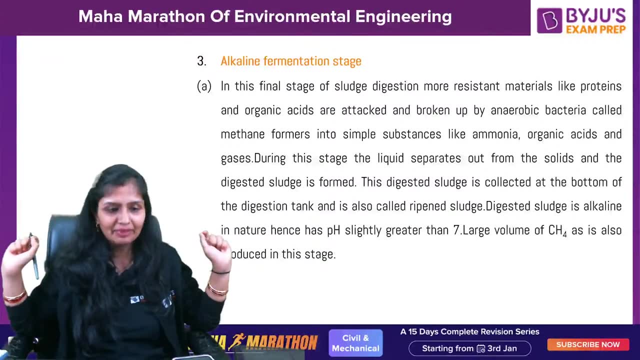 and they will convert it into gases like methane and complex organic matter into simple organic matter. In this stage, you will get the digested sludge at the bottom, then the liquid and the gases at the top, based on their density. This is the last stage. Now, this stage specifically. 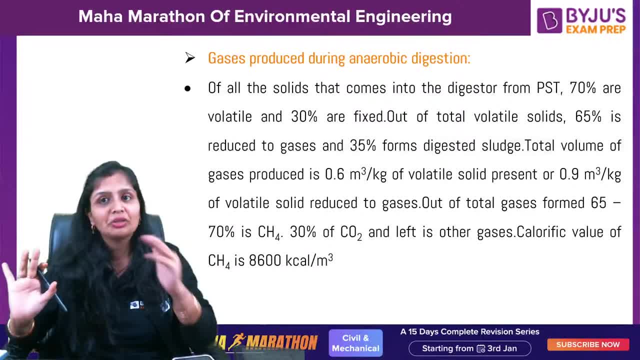 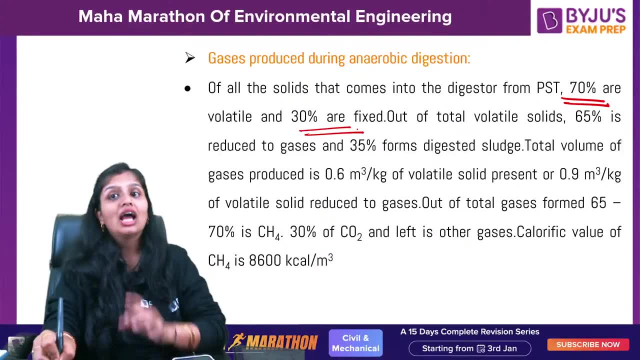 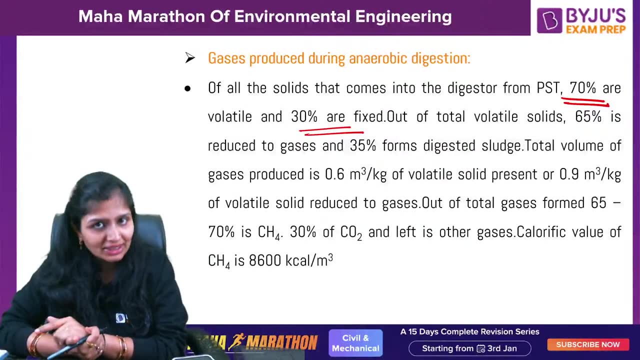 the sludge which you obtain from the digestion chamber. in that 70% is the volatile solids, 30% is the fixed solids. Out of the 70% which is the volatile solids, 65% is reduced to gases, If you want to know how much gases. 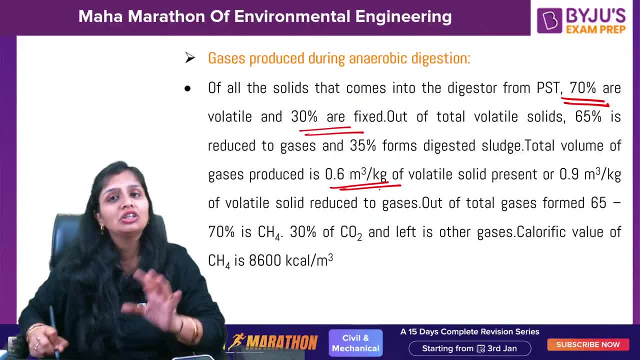 you can say 0.6 m3 per kg of the solids present, or approximately. they give you the same answer: 0.9 m3 per kg of volatile solids reduced to gases. It is that simple. as that Majorly basis methane is released, You can sell the methane. It has a high calorific value of 8600 kilo. 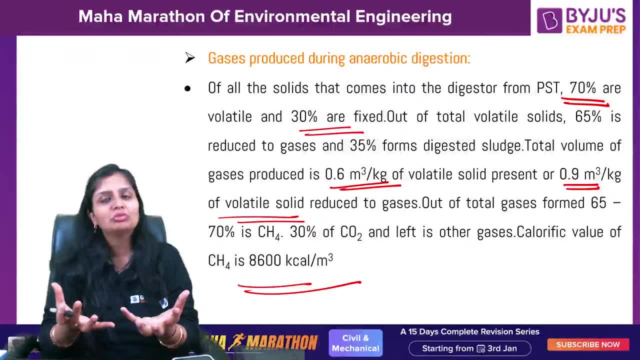 calorie per m3, or the gas which is produced, methane. you can use that for running the plant. So you can use that for running the plant. So you can use that for running the plant. Now, coming further, we have two types of digester here: Standard rate sludge digesters. When you 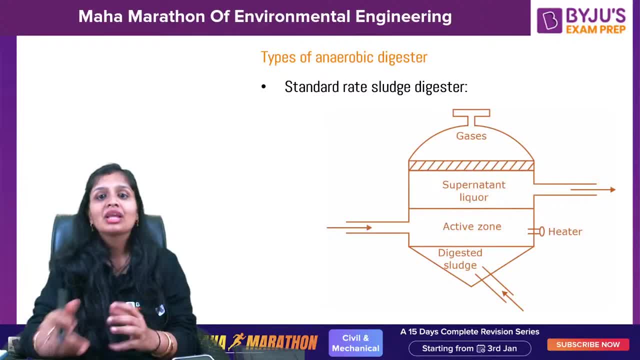 say standard rate, actually the time taken is more. So you feed the sludge here from the primary sedimentation time. What will happen? No mixing, nothing you are doing. You are totally dependent upon the acid formers and methane formers. Methane formers is pH sensitive. It is like a moody person. 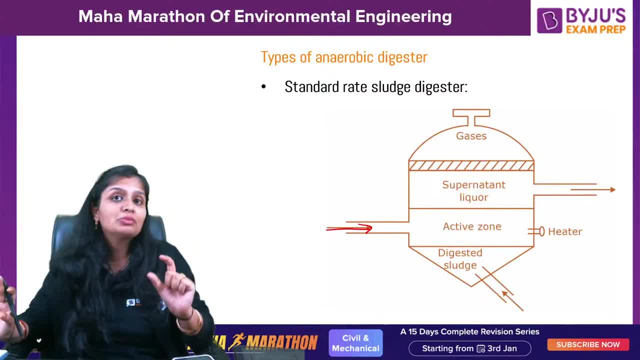 I won't eat that. I won't eat that. It is pH sensitive. It works in a narrow pH range of 6.5 to 7.5 generally. If you increase the pH, it will not function. If you decrease the pH, it will not function. So here, what will? 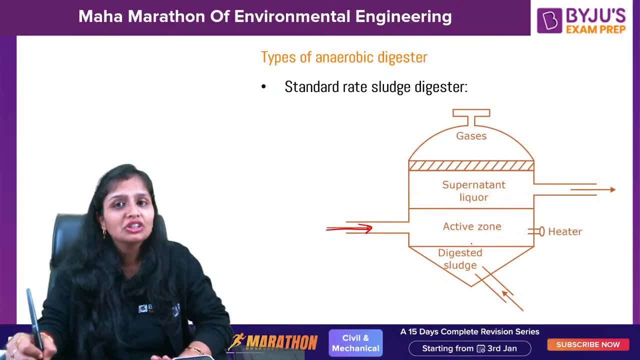 happen Here, the decomposition will take place, The solids which are formed, which will be deposited here, The liquid supernatant liquor which is here. it has a high BOD value. Why? BOD means how much? 1500 to 3000 pp. 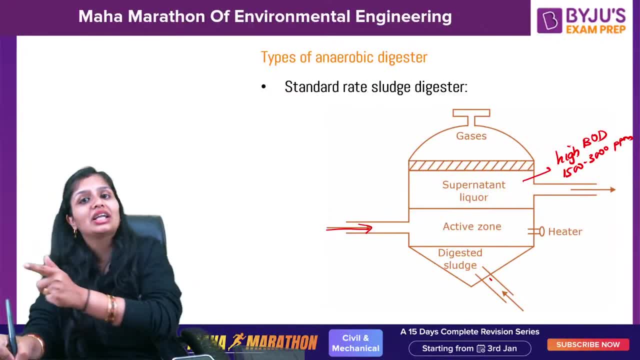 So it is sent back to the primary sedimentation time. Then you have gases released. So from the floating chamber is there from which you collect the gas. That's it. So this is the standard rate sludge digester. Now you want to increase the opportunity of contact This? 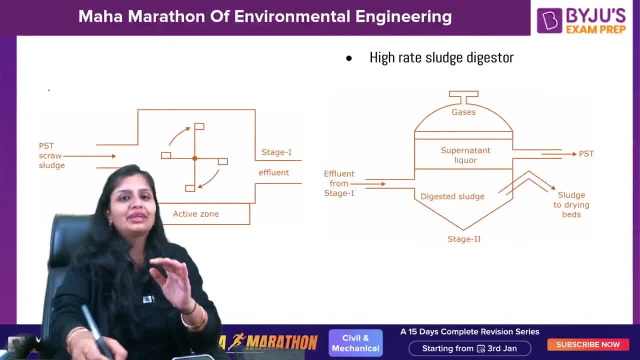 portion of active zone. you take it out and you do mixing. The raw sewage is supplied. You do mixing. When you do mixing, like if in a party I am there and paneer pakoda is there And Prashant is there- You take it out and you do mixing, The raw sewage is supplied. 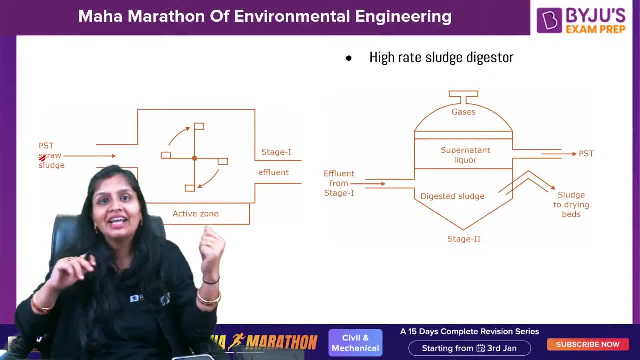 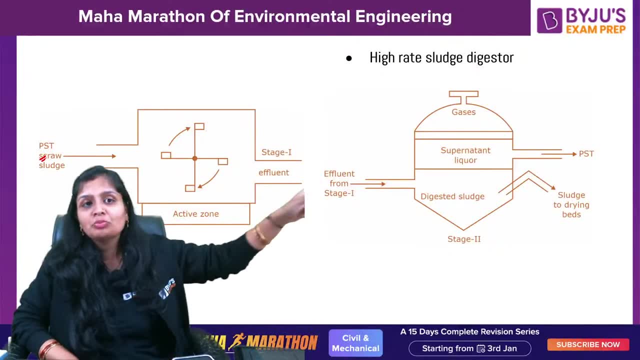 You do mixing. When you do mixing, like if in a party, I am there and paneer pakoda is there, He will come and say: ma'am, paneer pakoda is this side, He guided me, So what, I will go there. So my time for searching the paneer pakoda is reduced. Why? Because Prashant helped. 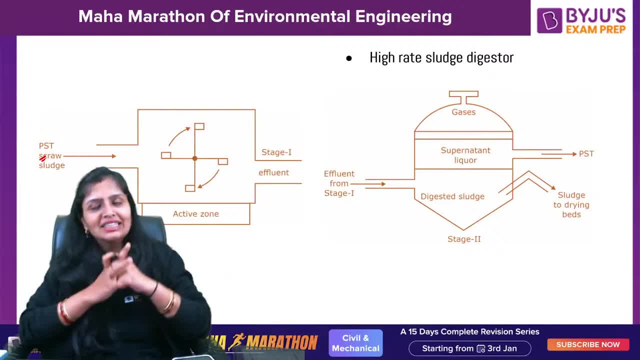 me for telling ma'am paneer pakoda is this side. Similarly, if I have to search, it will take time. So if microorganisms has to search organic matter, it will take time. But if by some external means I am able to get that, it will reduce the time. So here, external, 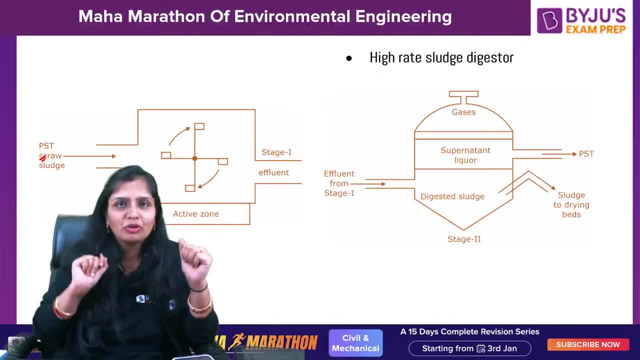 way is my external way was Prashant. He told me: ma'am paneer, pakoda is this side, Don't search in this large acre or party, Okay. Similarly, if you do, the mixing opportunity of contact will increase And so the time required will be less. So, once it is done, 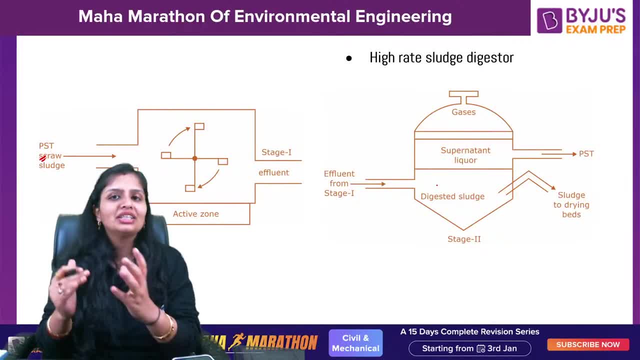 you will feed it Again. here you will get all the three components: digested sludge, supernatant liquor. It has a high BOD. Don't throw it. It is very, very harmful. Okay, So supernatant liquor will go into the PST and you will have gases. So this is the high rate. 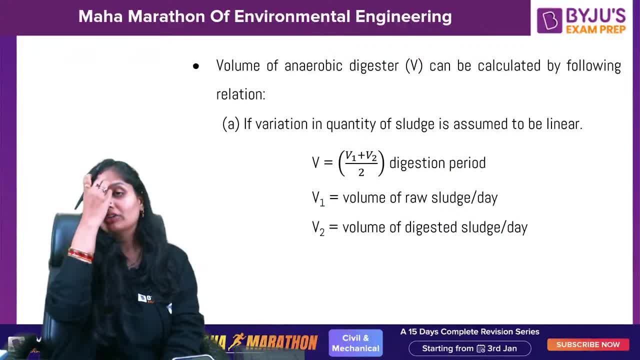 sludge digestion. If you want to calculate the volume, how much sludge is coming and how much digested sludge is going- because the volume of raw sludge is reduced- Gases, you are collecting it in the gas chamber. So this is when you are assuming linear variation. 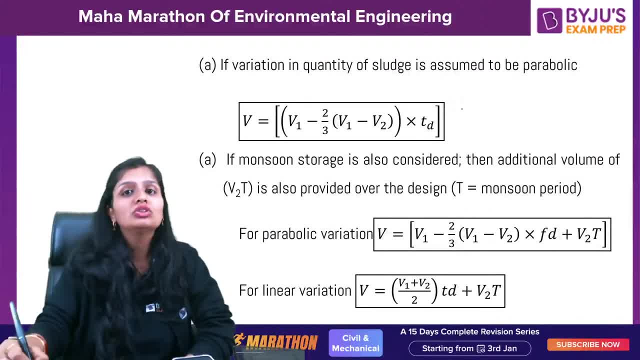 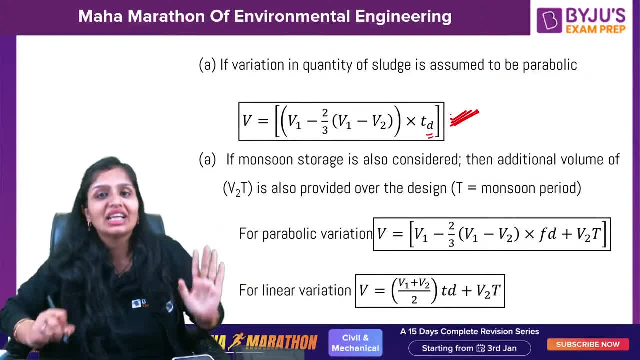 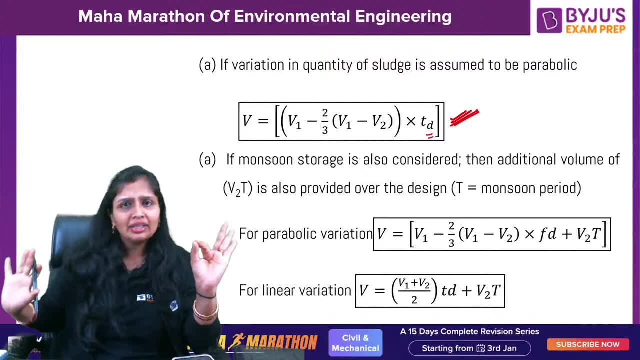 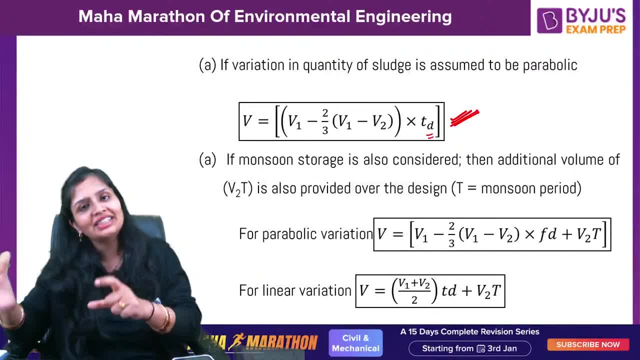 an extra space so that the already digested sludge can also be there. So this is V2 into T Capital. T is the monsoon period. Till that time monsoon period is there, you cannot dispose the digested sludge. Okay, So this is the volume form. 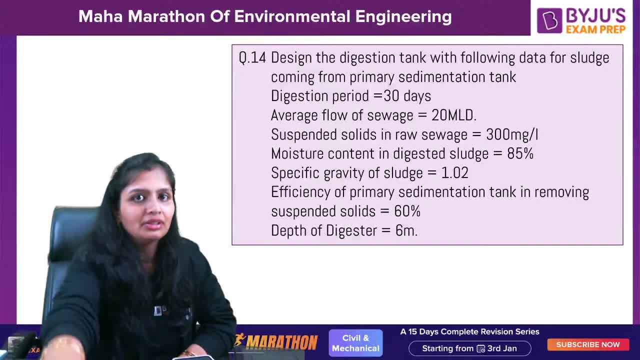 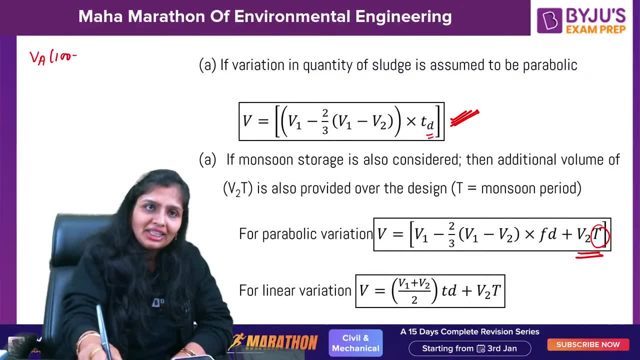 volume problem, any doubts? okay, and there is one prominent relationship: if VA is the volume of raw sludge and initially the moisture content is PA, so ma'am once repeat, while supernatant I'll repeat, that VB is the volume of the digested sludge and the moisture content of the digested sludge. 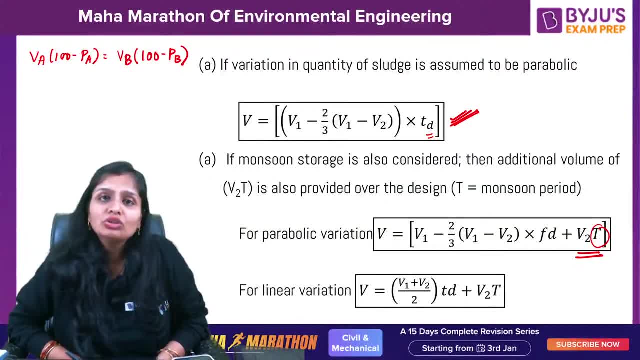 the aim of the sludge digestion tank is to reduce the moisture content. okay, to reduce the quantity of the sewage. supernatant liquor has high BOD. 1500 to 3000, that means in one liters. 1500 to 3000 is the demand of oxygen for the decomposition of biodegradable organic matter. so large quantity. 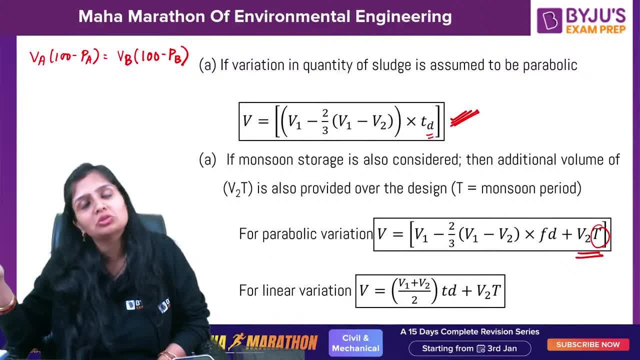 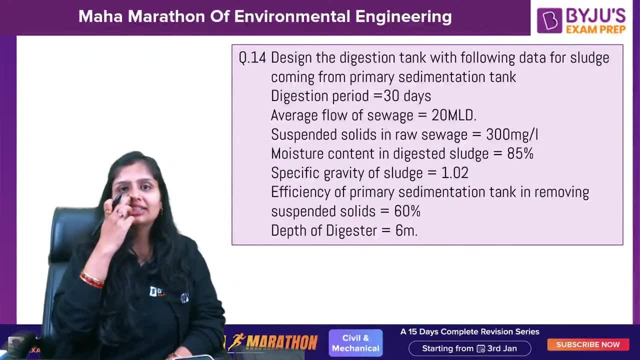 of organic matter is present. that is the reason you cannot dispose it, and it is recirculated back: clear. come on, guys. this is the design for digestion chambers. then we have a septic plant and then we have a biodegradable organic matter. so this is the design for digestion. 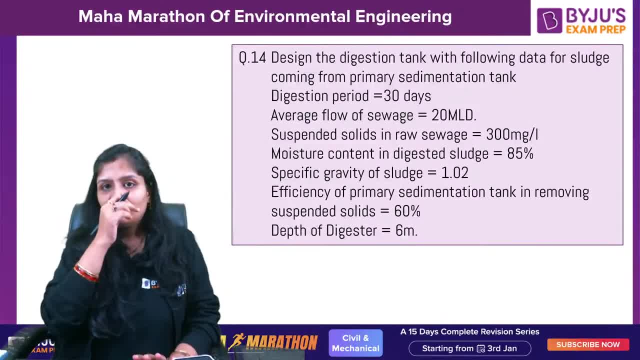 then we have a septic plant and then we have a biodegradable organic matter. so this is the design for digestion chambers. then we have a biodegradable organic matter, so this is the design for digestion tankers. okay, guys, come on, guys, we have to design it first. fastly solve this. 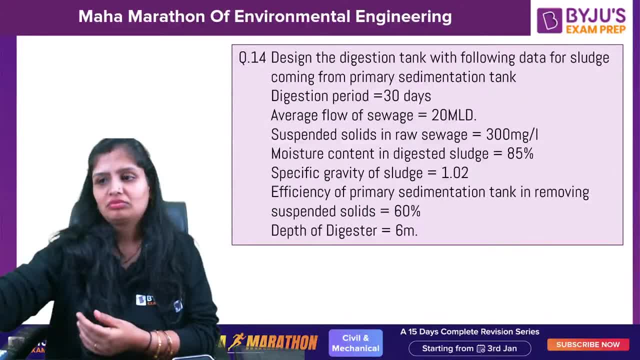 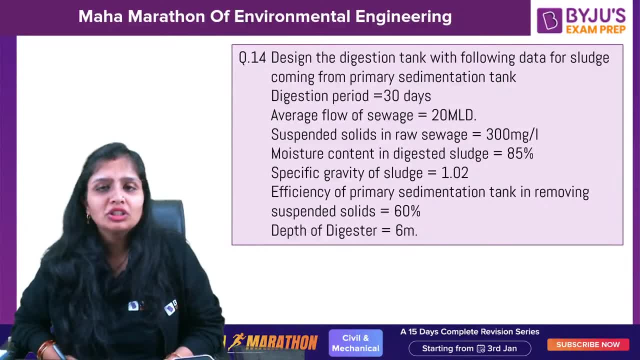 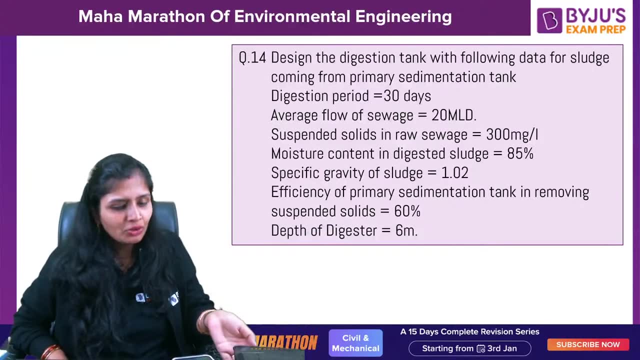 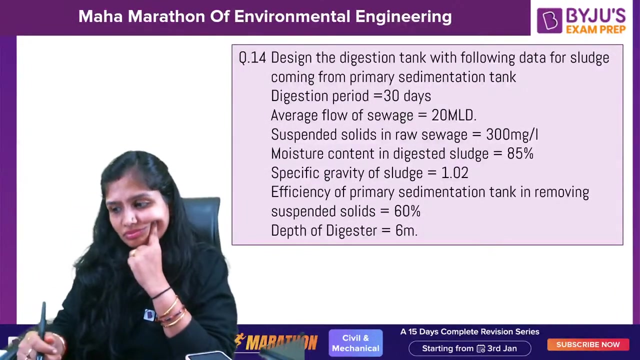 solve this fast. digestion period is given to you, suspended solids. all things are given to you how you solve this. are you going to solve it or I'll be the one who'll be solving it? tell me that also. fastly, fastly, you will be solving it. alright, see here. moisture content in digested. 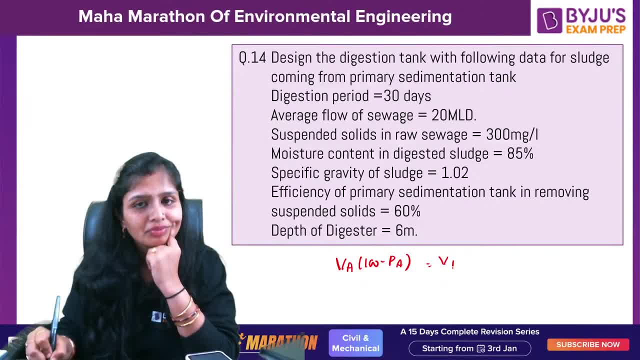 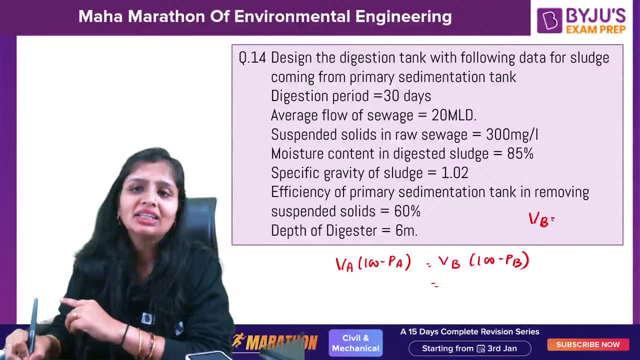 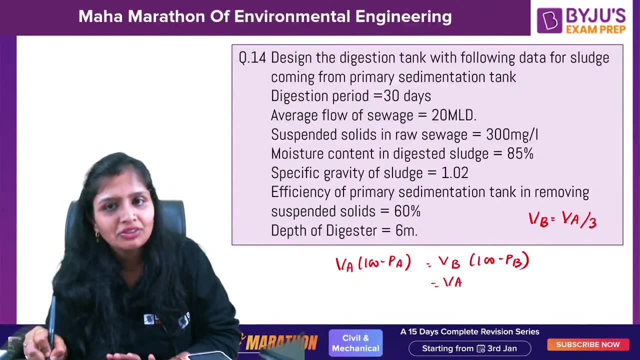 sludge is given to me, digested sludge, VB- is not given to me. I will take it the volume of the digested sludge, VA by 3. so this is VA by 3, 100 minus 85, and this is VA 100 minus. 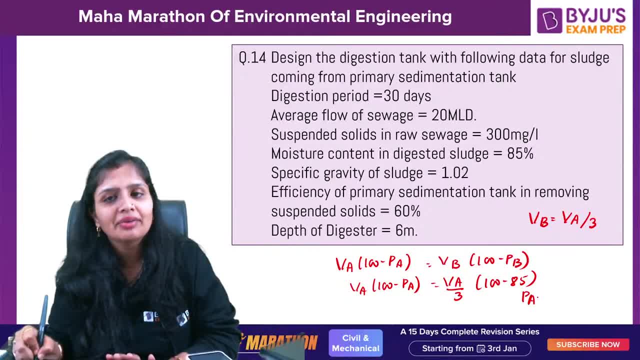 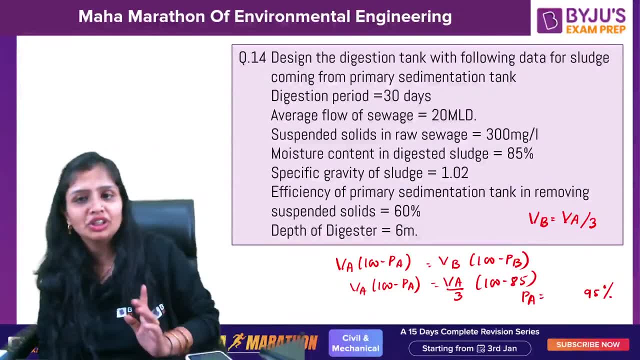 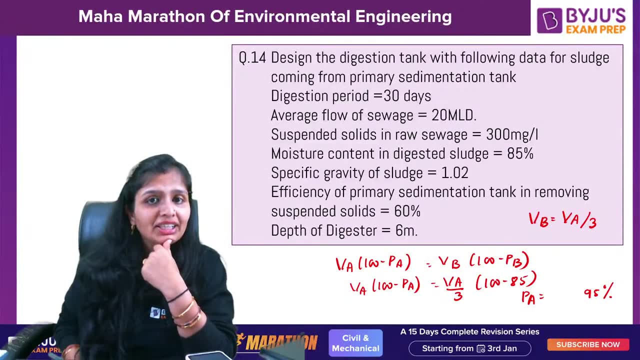 PA, can you tell me how much is the moisture content? calculate and tell me? I think it is 95%. just check it out. 95% is the moisture content. just check it out once. now it is asking me design the digestion tag. so if it is asking me to design, I need to calculate the volume. 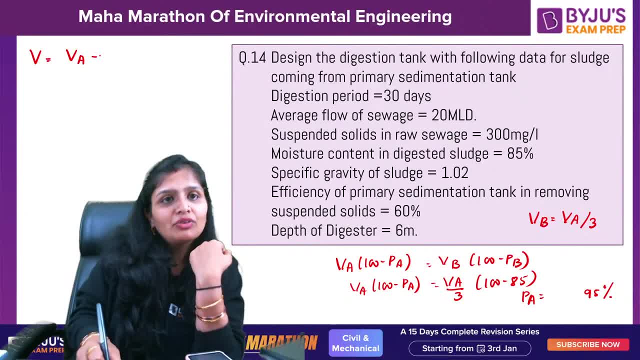 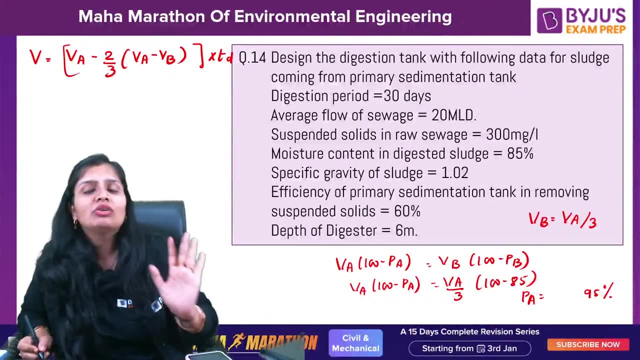 so design, I need to calculate the volume, then I have to calculate the dia. now in the question, I don't know VA, I don't know VB, so I have to calculate the volume. if I am able to calculate the volume of raw sludge, I will get the answer. how will I calculate? 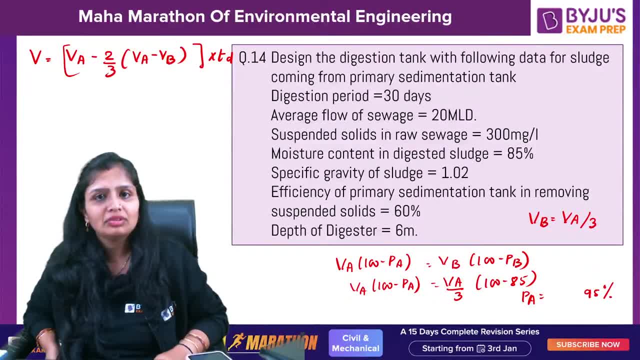 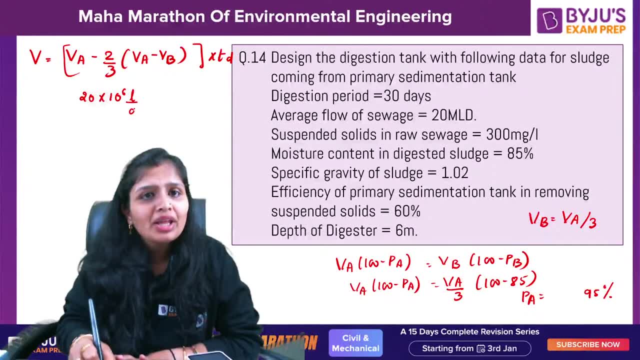 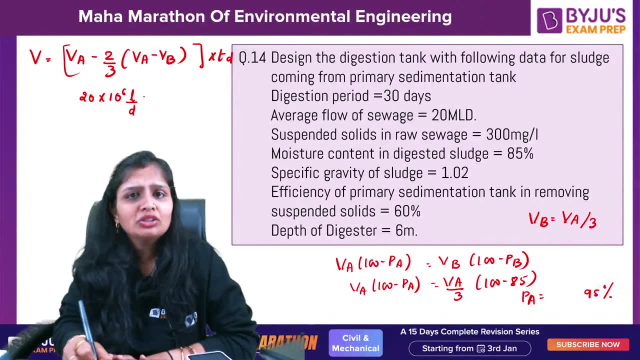 volume of raw sludge. come on, guys see 20 into 10. raised to power, 6 liters was the flow, the solids which were present, suspended solids, which is given. so the suspended solids which are present, was 300 mg per liter. out of this, 60% was reduced. 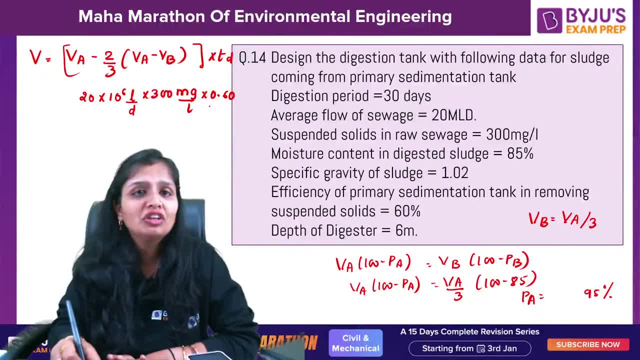 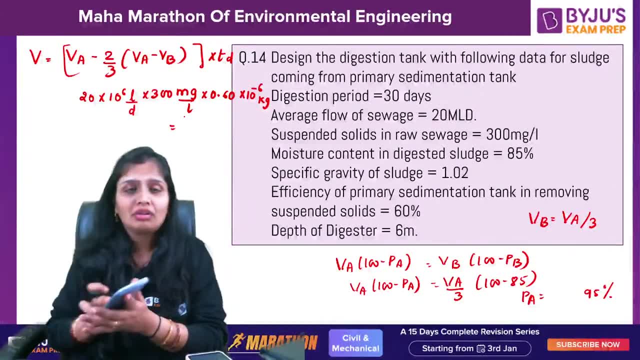 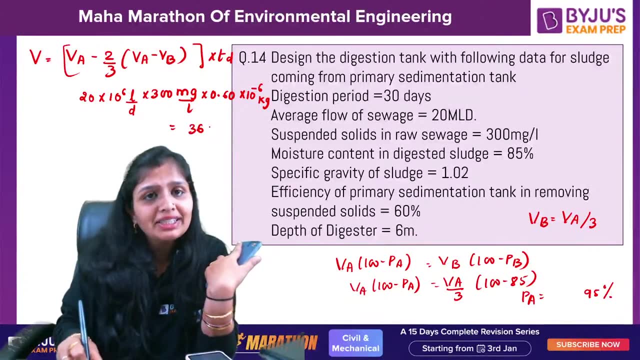 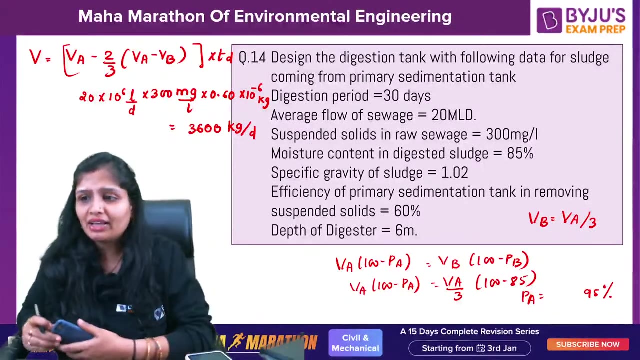 in PST, so this 60% will be the one which will be producing sludge. mg converted into kg, how much it is coming? 3600 kg per day. this is the sludge print. this is the sludge producer. I need to calculate the volume. how will I calculate the volume? anybody? 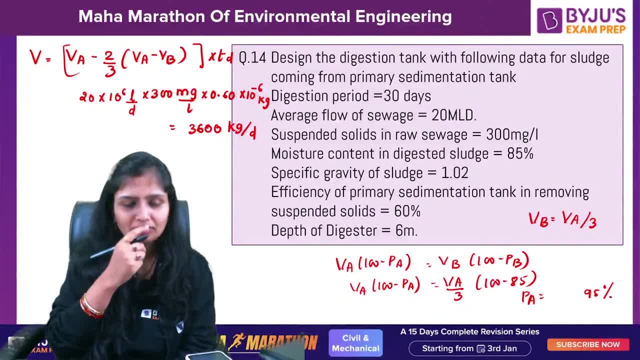 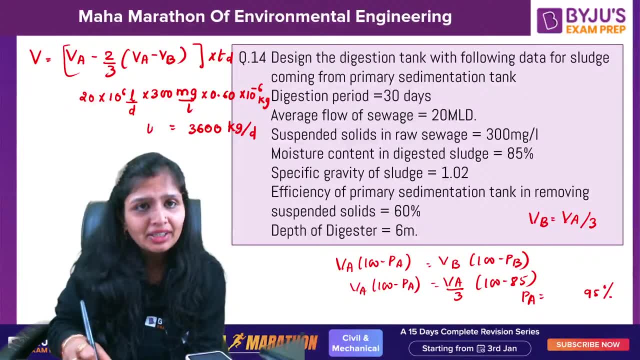 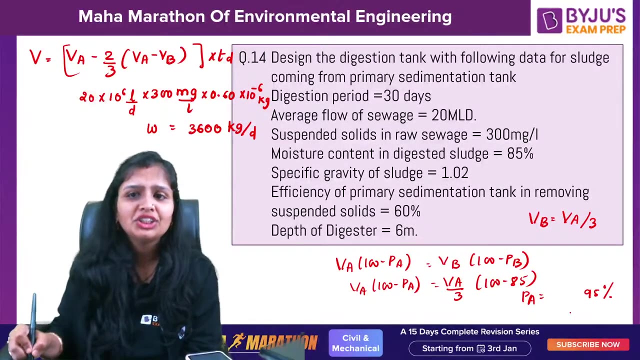 you? come on guys, fast. how can I calculate the volume fastly? I know the weight. how can I calculate the volume? come on guys, fast, fast. moisture content is 95%. that means 5 kg of solid and 95 kg. if I want to write it will be like 50 kg. 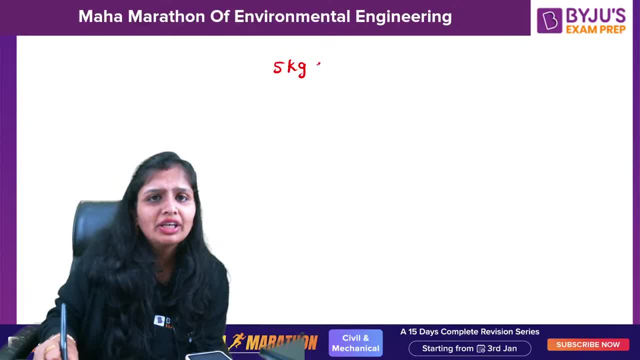 95 kg. if I want to write, it will be like 50 kg. 95 kg. if I want to write, it will be like 50 kg. 5 kg solid and 95 kg of water makes 100 kg of sludge. This is the meaning of it. 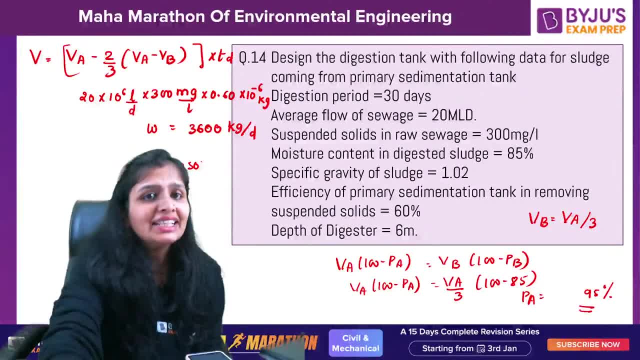 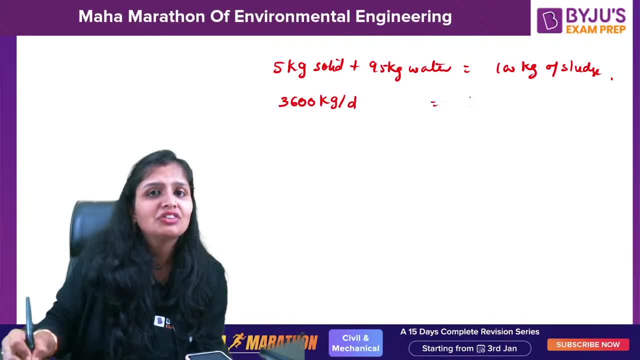 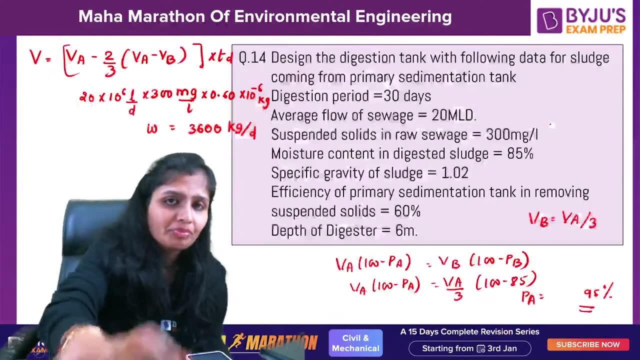 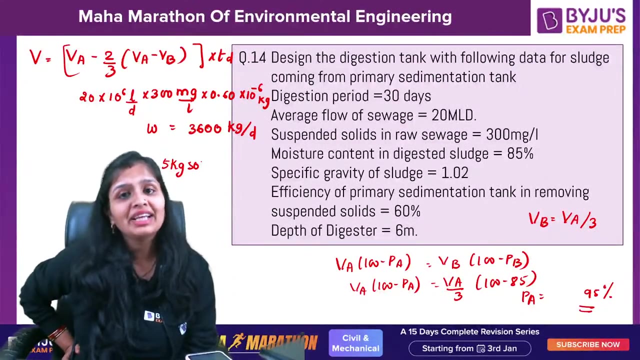 So if 5600 kg per day of solid is there, how much sludge will be made? Can I calculate in this manner? I don't think so, So use specific gravity. Okay, If I take specific gravity, then also I won't get the answer properly. 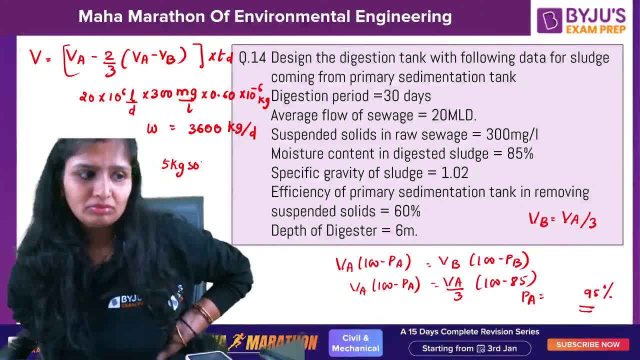 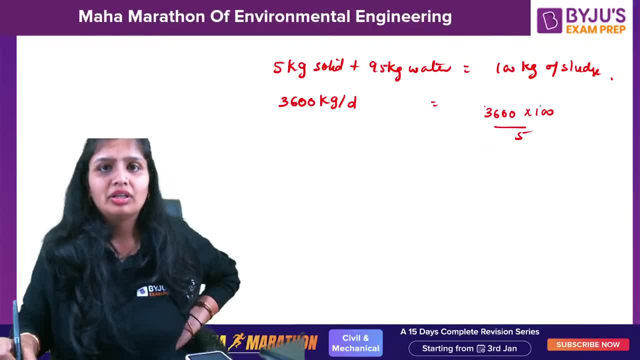 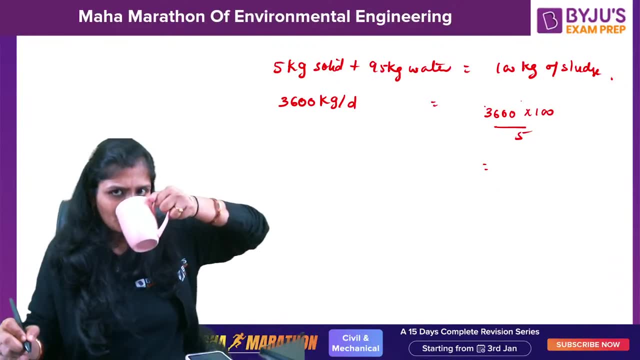 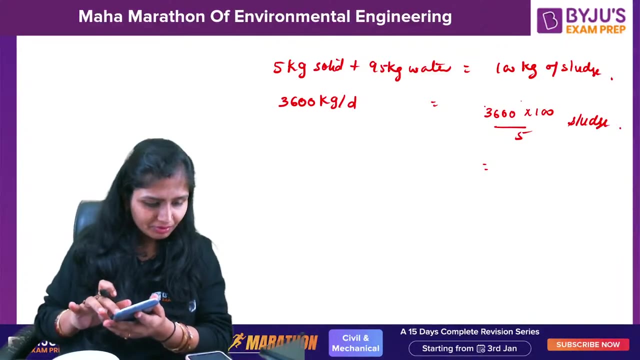 Fast. This is kg per day. How much will I get from here? How much will I get from here? How much will I get from here? How much sludge is produced, Guys? how much sludge is produced? No, we don't go by that method. 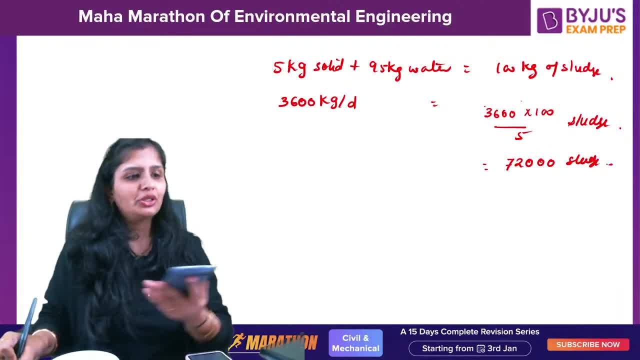 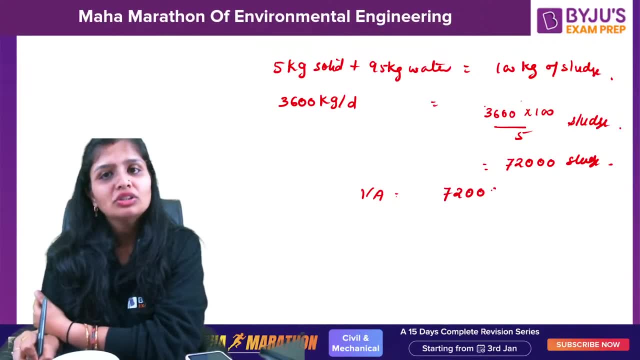 72,000 kg of sludge is produced. I need to calculate the volume. I need to calculate the volume, What I will do: 72,000 divided by the specific gravity, How much it is 1.02, And the specific gravity of water comes out to be: 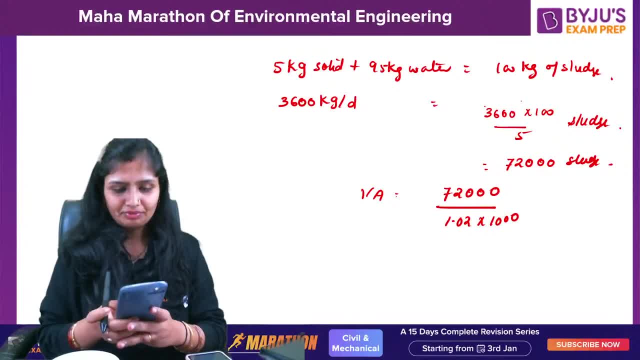 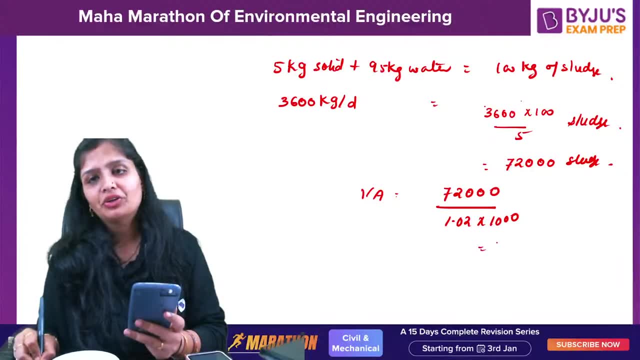 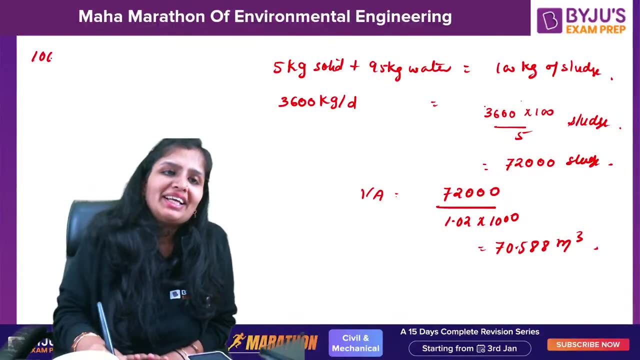 1,000.. So this manner, I will do it: 70.588 m3.. Clear shears: This manner, we will do it. It's like you know the formula. I guess 100 minus Pa kg of solid is there. 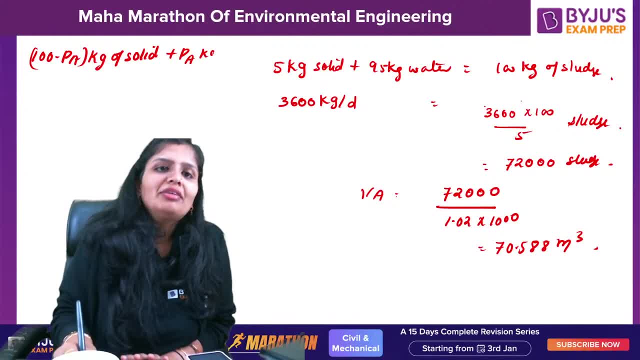 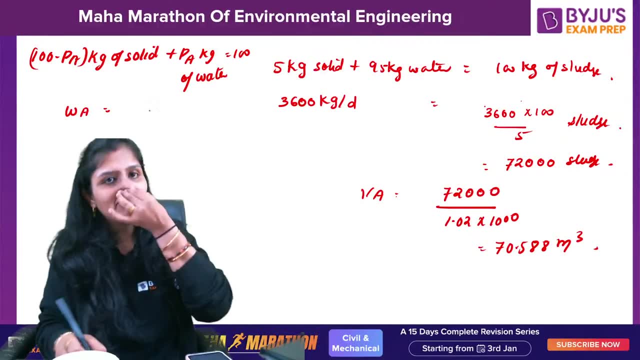 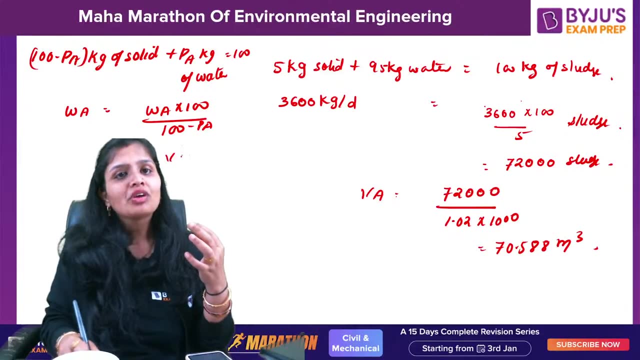 And Pa kg of water is there, So it will make water means moisture, 100 kg of sludge. So if Wa kg of solid is there, how much? it will make? Wa into 100 upon 100 minus Pa. So if you want to get volume, volume will be Wa into 100 divided by 100 minus Pa into the unit weight. 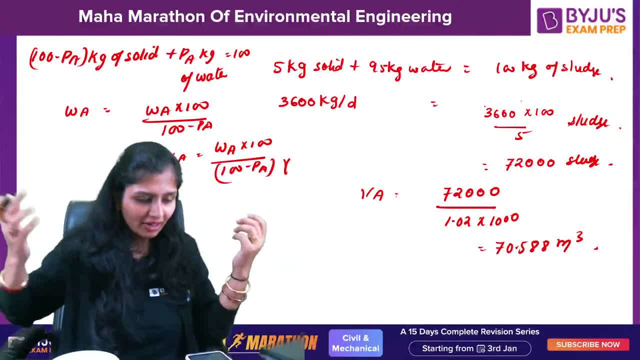 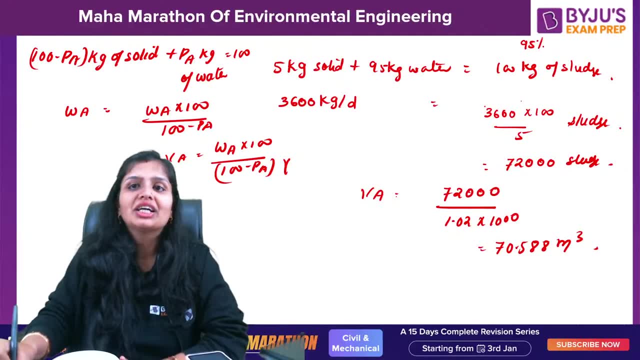 So that's what I have done. That's what I have done, What, Kishalya? See, if it is written 95% moisture content, Moisture means water Percentage means 100. If 100, you know what sludge and sewage are same. 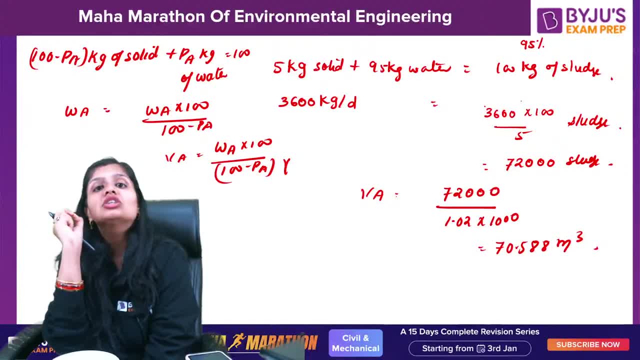 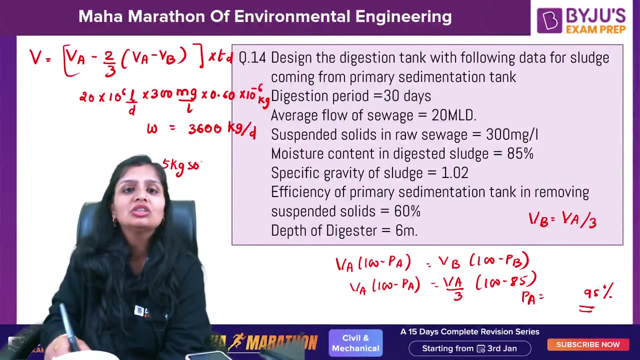 Only difference is the amount of solid content is more in the sludge. So if 95% is the moisture content, that means 95 kg is water rest, 5 kg is solid. So if 3600, which is given to you, this is the solids. 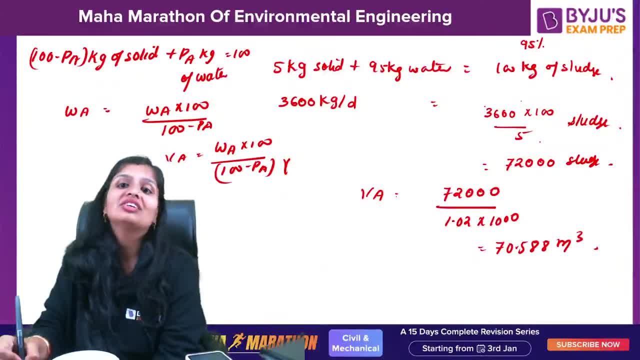 How much sludge will this solid generate? So it will generate 72,000 kg per day of sludge. So it will generate 72,000 kg per day of sludge. So it will generate 72,000 kg per day of sludge. 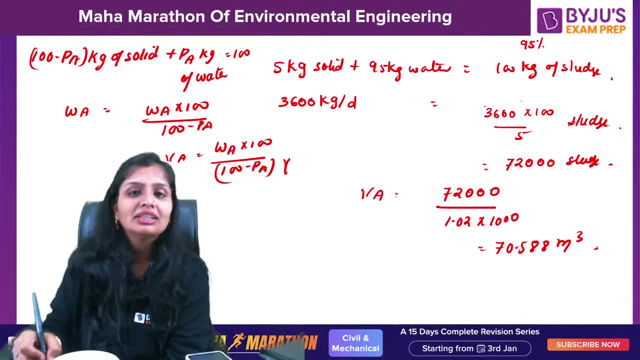 Okay, So this will be the generated sludge. So volume will come out to be what Weight divided by the weight, divided by the specific gravity into the density of water. So generally, this is what Weight by gamma you take, unit weight. 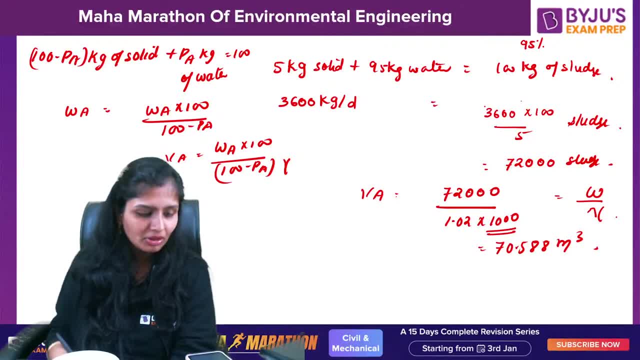 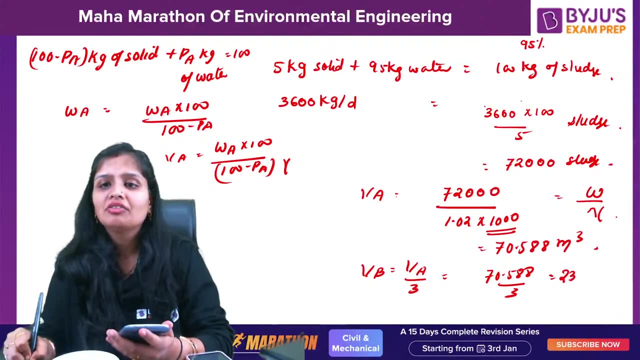 Density is equal to mass by volume. You can go in that manner also, Okay. Okay, VB is equal to VA by 3. How much it will come? 23.529 meters. So from here what you will get. I will just substitute it here only. 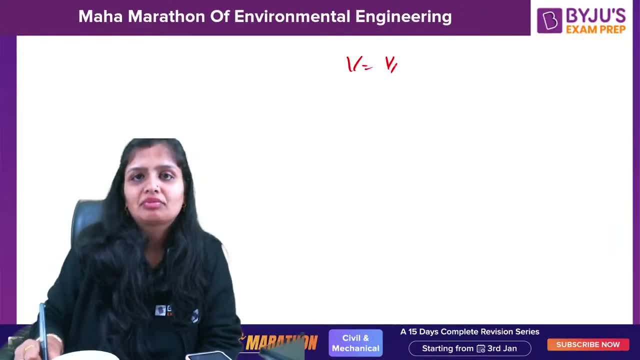 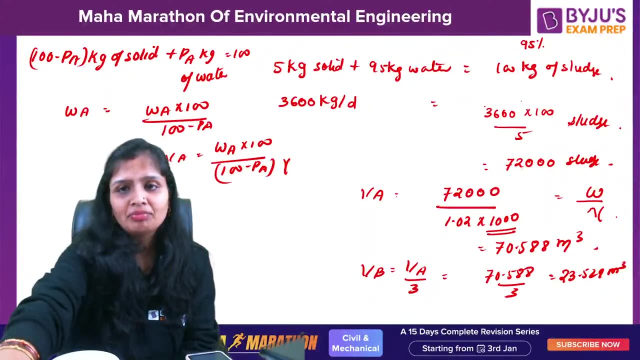 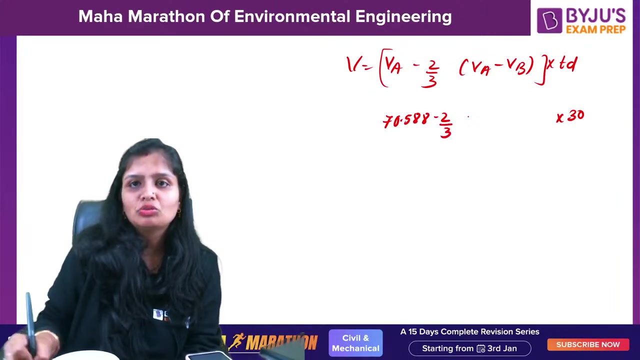 I wrote the formula there In the ancient time. So in this manner we go, She is. you were telling that manner we do not go 30 days. is the detention time? 30 days? 70.588 minus 2 by 3.. 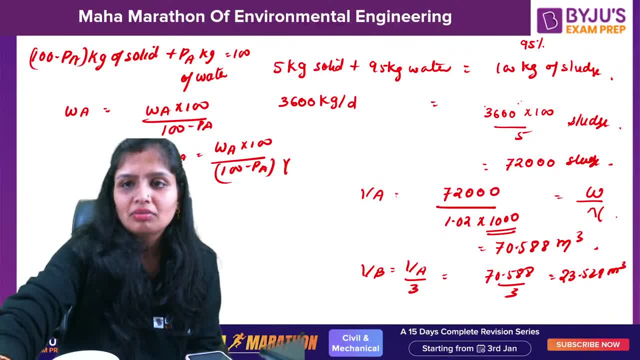 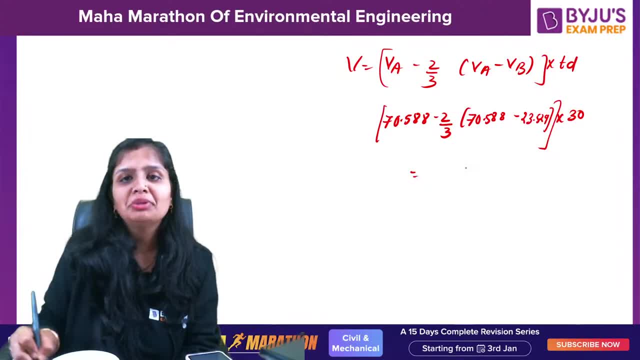 70.588 minus 23.52.. How much meter cube is the volume coming? How much meter cube is the volume coming? The volume is the weight. Now you will do pi by 4 d square h. In the question it has given you the height as 6 meter. 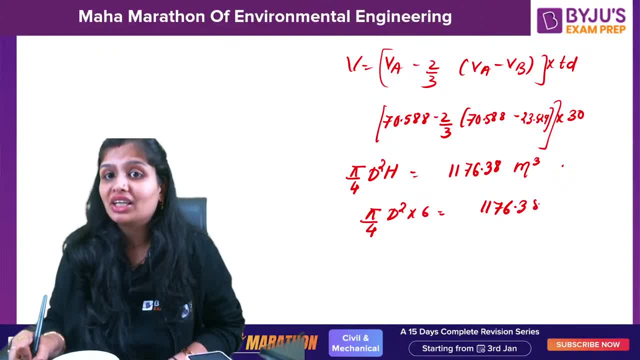 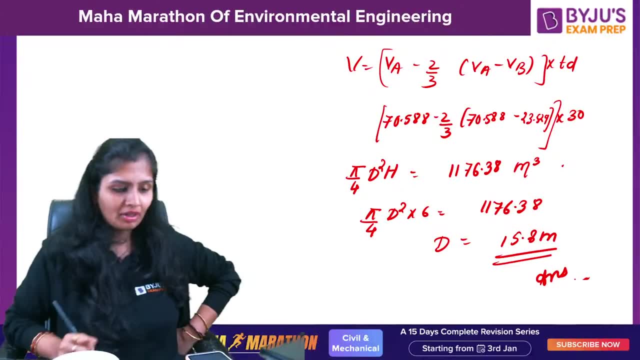 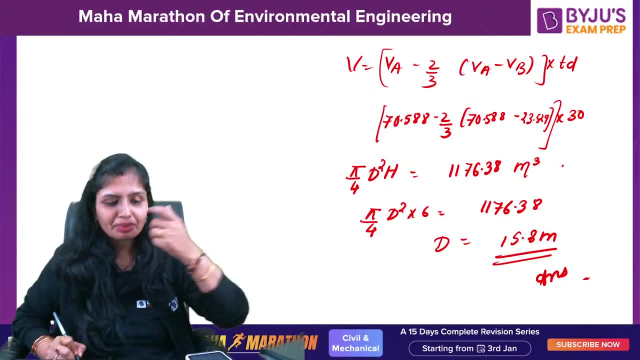 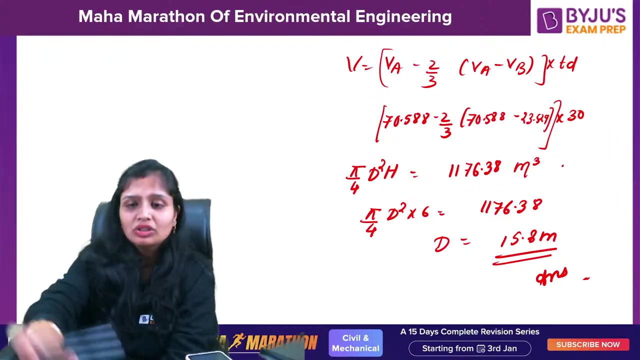 So do it. 6 from here, you will get it and they can ask you in gait examination. It is not that tough that they cannot ask: This will be the dial, This will be the dial, Clear, Clear, this will be the die-off which can they can ask. okay, so this is a volume part and the last, i think 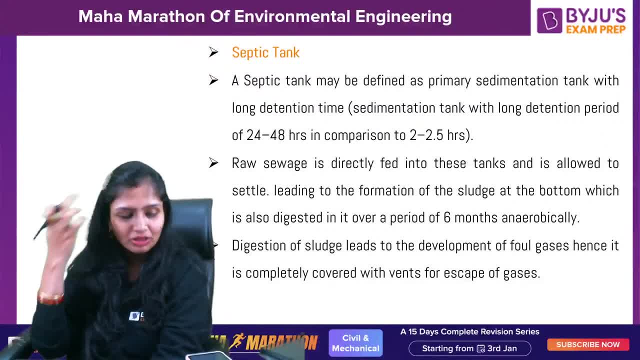 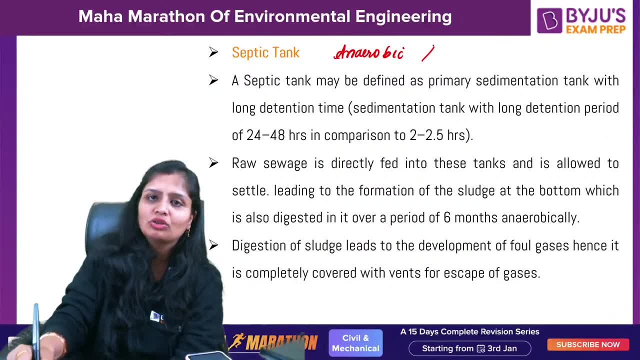 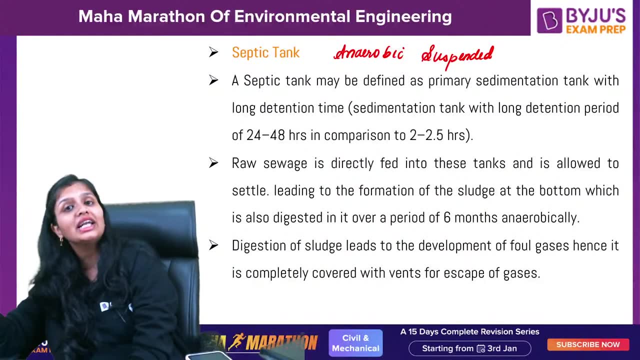 okay, fine, then we'll go to the solid waste management part. so the last one is the septic tank. this is anaerobic, those places, anaerobic suspended growth mechanism, those places like hospitals, and all initially when the sewer pipeline was not laid and they were out of the 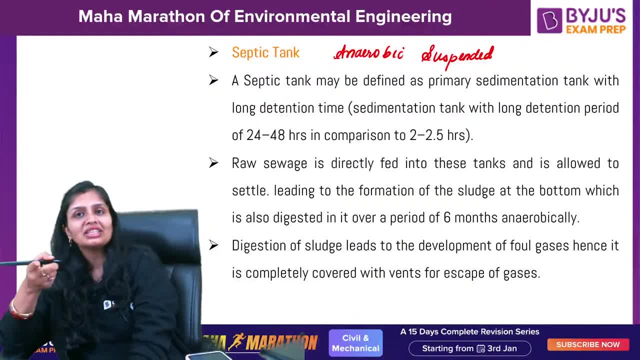 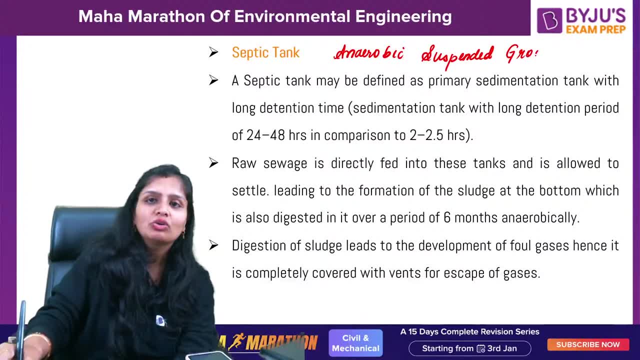 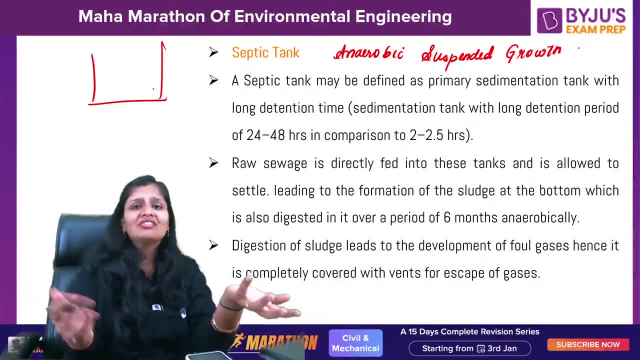 city now also. you guys have seen the septic tank, those places where the sewer facility and all is not there, they go for septic tank. this is anaerobic suspended growth mechanism, normal, no brain, just a sedimentation tank here. you don't do screening anything while you just a connection is there. 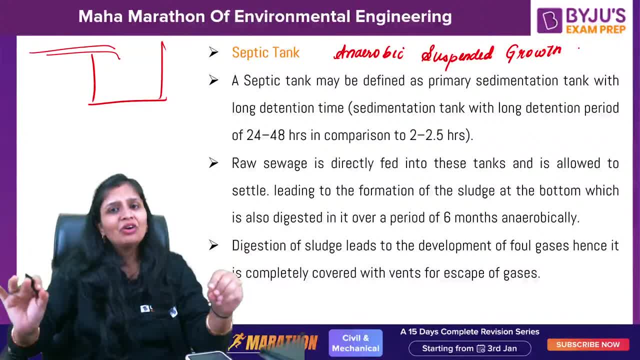 from there the sewage comes. it is being there for 24 to 48 hours in pst. you keep it for 2 to 2.5 hours here. since you haven't done screening, there will not be any further treatment, which will be given you just directly. 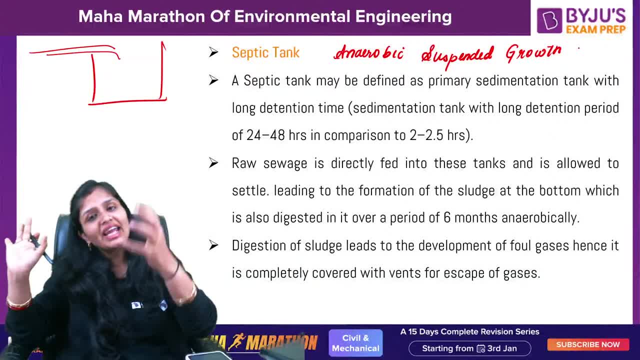 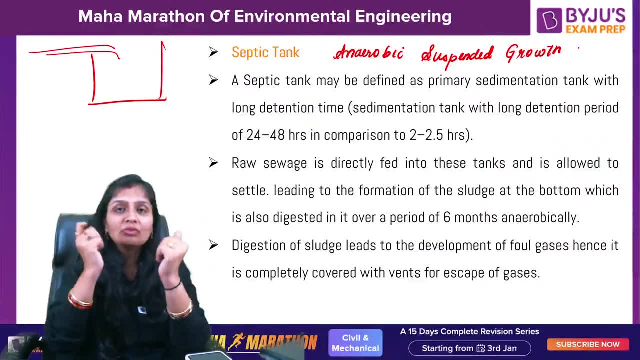 feed it here. okay, now it takes time for digestion, everything it takes time. now when it is digested. that means digestion means what? the decomposition of organic matter takes place, because the sewage which comes out from your homes consists of a large amount of organic matter. so what will happen? 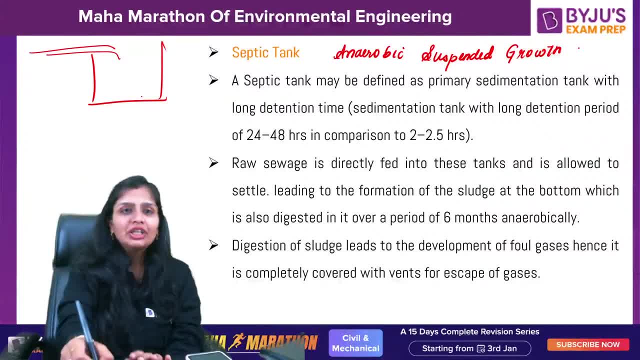 this sewage is fed, eventually you will see the sludge is formed at bottom. you give time for the digestion of this and eventually you reduce it and the gases will go out. on the top vent cover is provided. so technically it functions three things. what first? it functions like primary sedimentation. 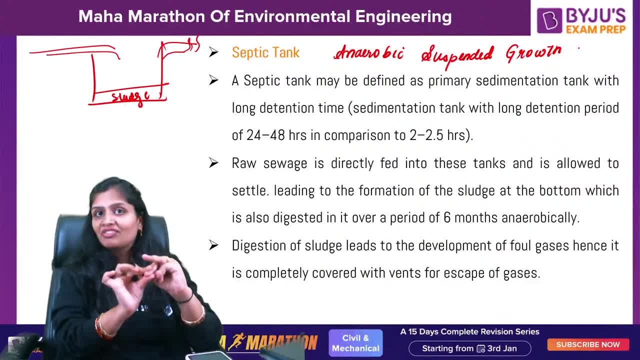 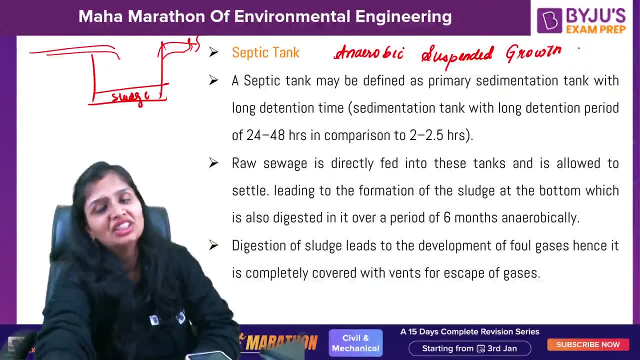 tank. secondly, it functions like biological treatment. why? because suspended organic matter is removed. dissolved organic matter is removed. third, it functions like sludge digestion tank. why? because the digestion of sludge is also carried. moreover, the efficiency is not that much, and you can see this the all those washrooms from there. 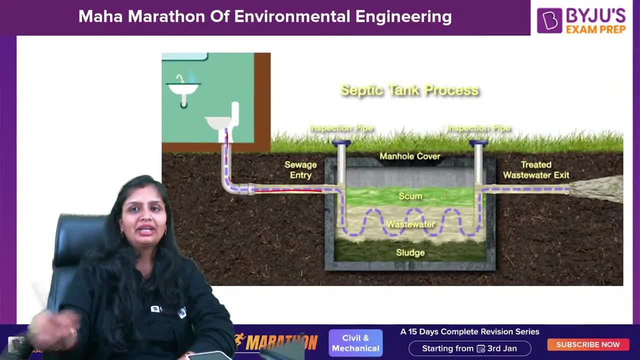 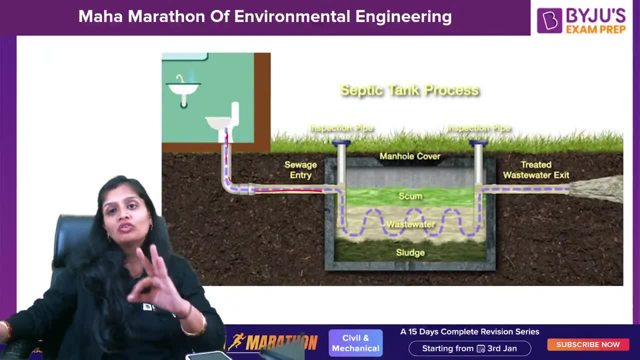 the sewage comes, it goes into this septic tank. this is the process which you can see, and underground pipes is there. so whatsoever is a treated sewage, it is dumped. moreover, make sure that no amount of water table should be near, near should be there near to it, otherwise what? 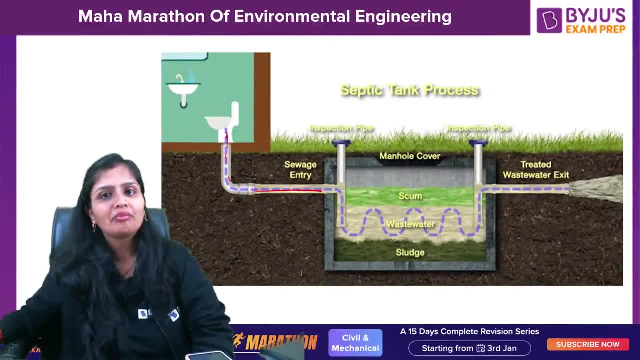 will happen, pollution will happen. so this is the process which you can see. and underground pipes is there. so whatsoever is a treated sewage, it is dumped. moreover, water table should be near near to it, otherwise what will happen? pollution will happen. pollution of that water will take place here. so this is the 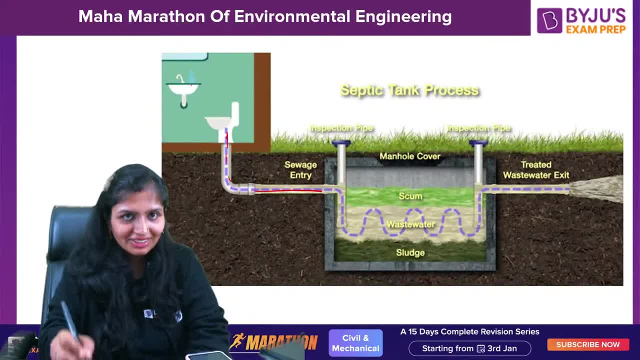 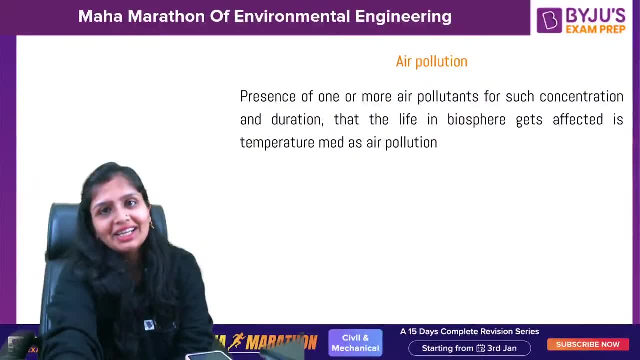 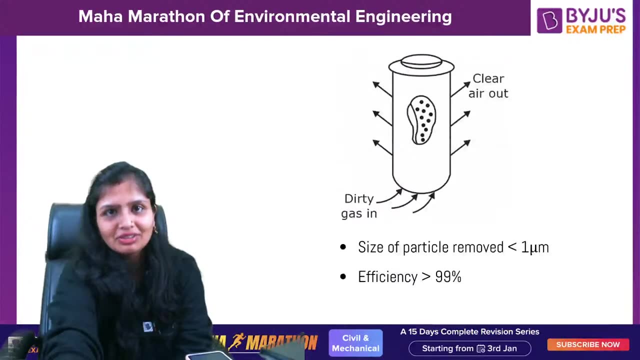 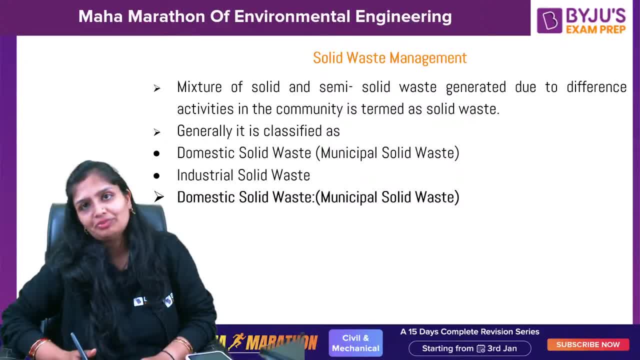 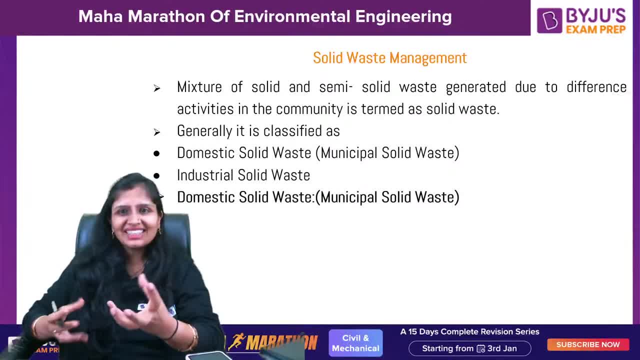 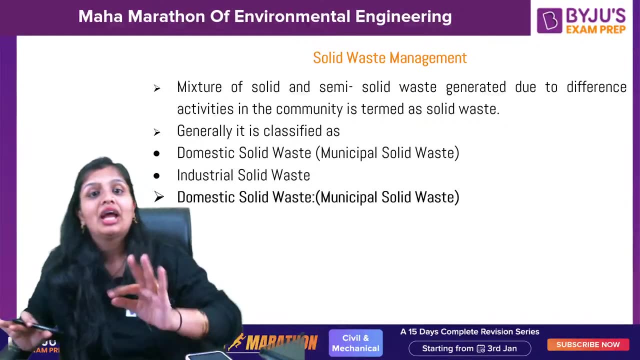 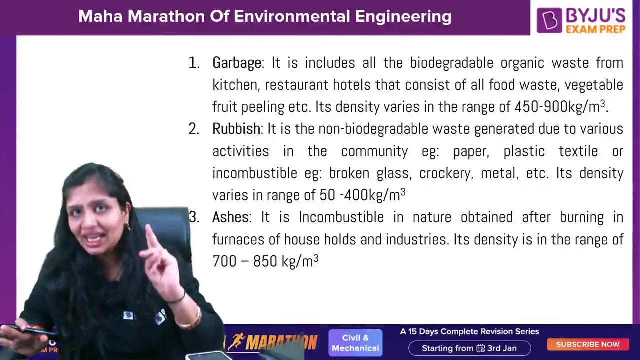 simple, it will be easy, we'll do it fastly. solids and semi-solids which are generated due to domestic activities, industrial activities. they are known as what? solid waste, domestic solid waste, municipal solid waste or refuse. all the three means the same. domestic solid waste is further divided into three things: garbage, rubbish, ashes, till now in your gate. 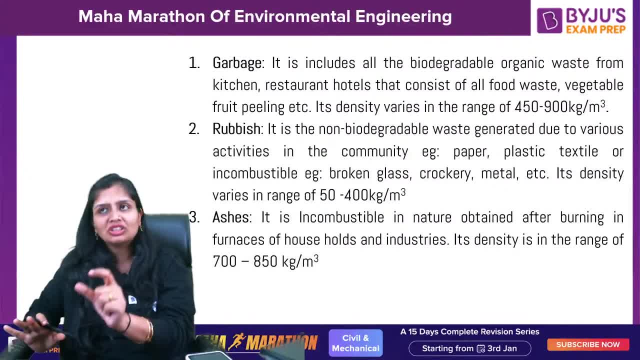 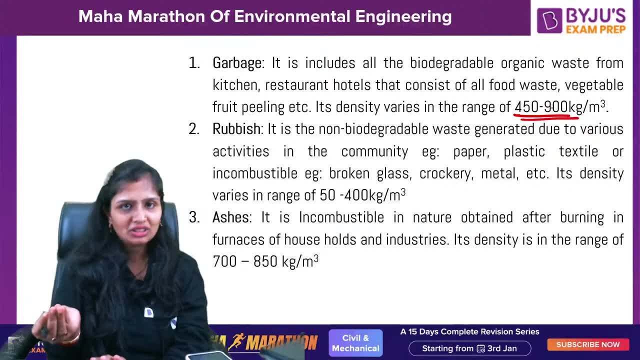 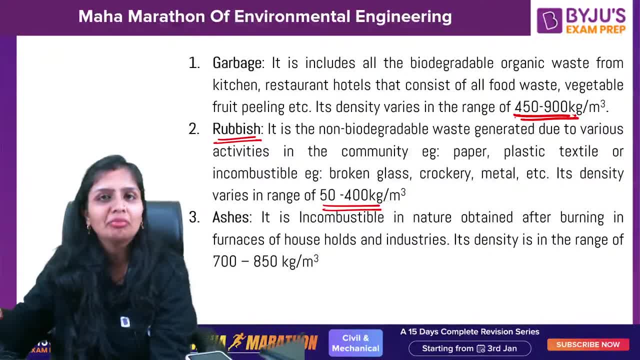 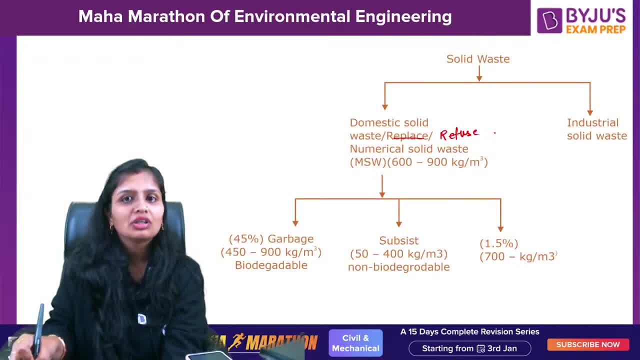 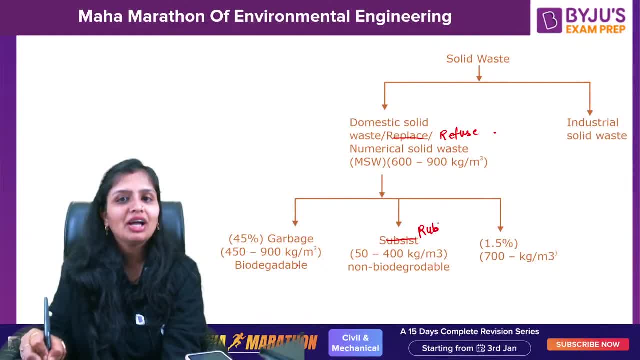 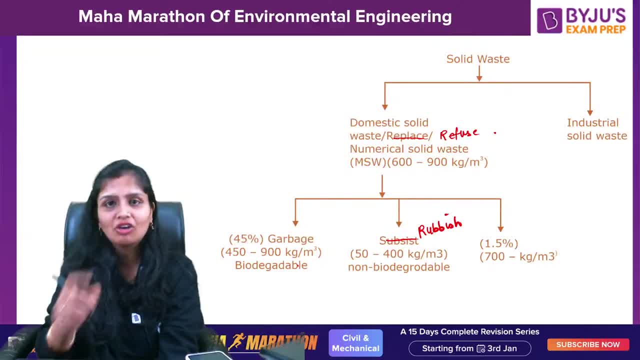 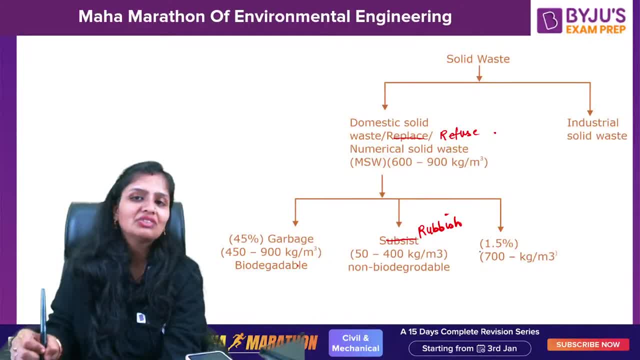 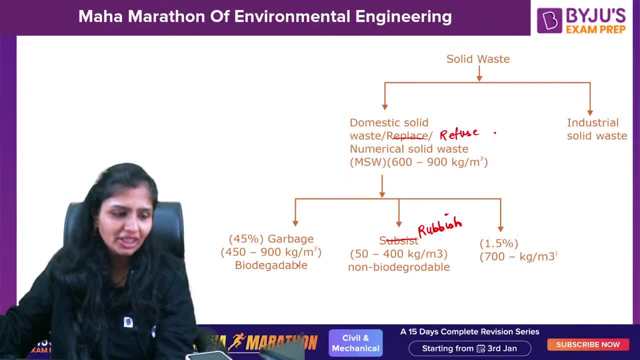 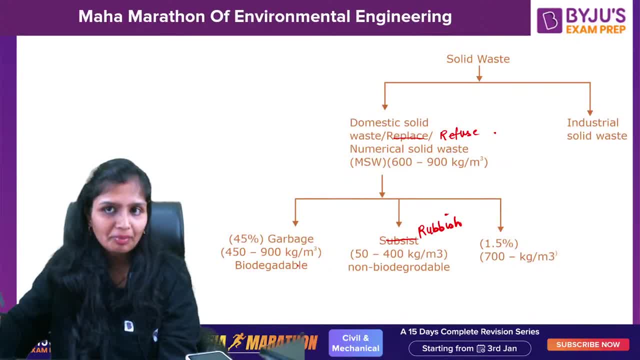 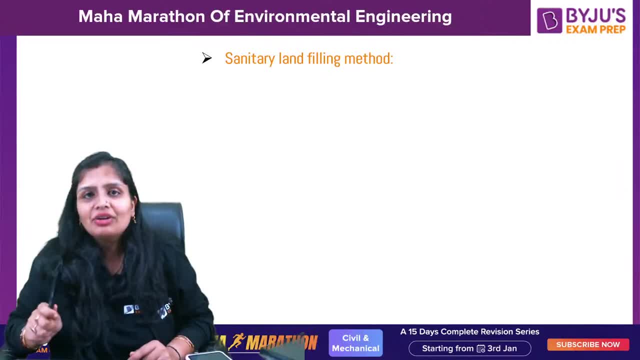 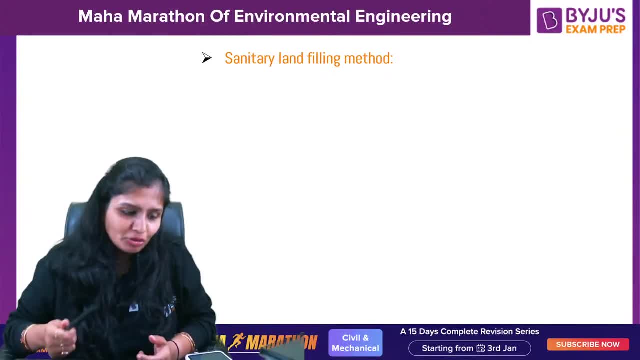 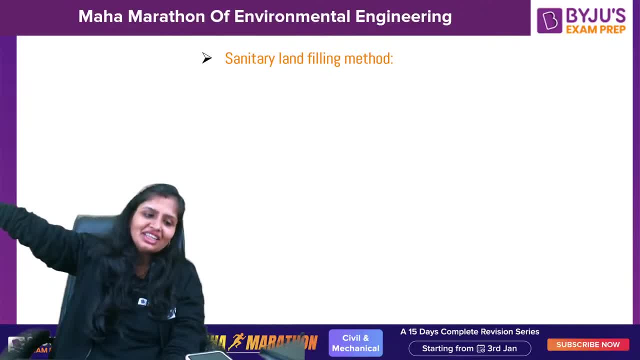 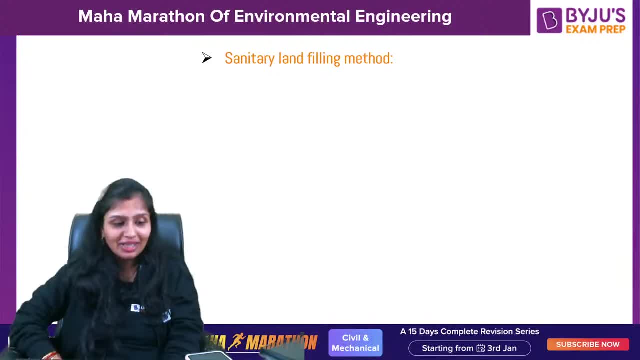 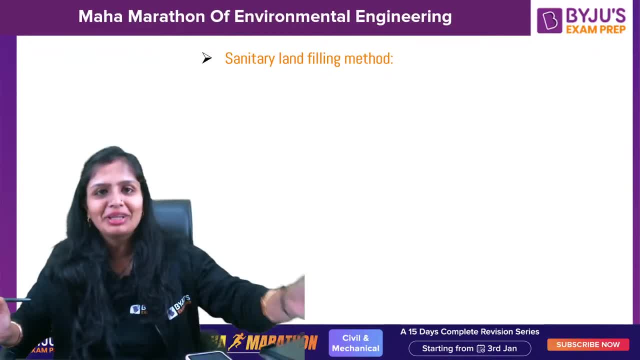 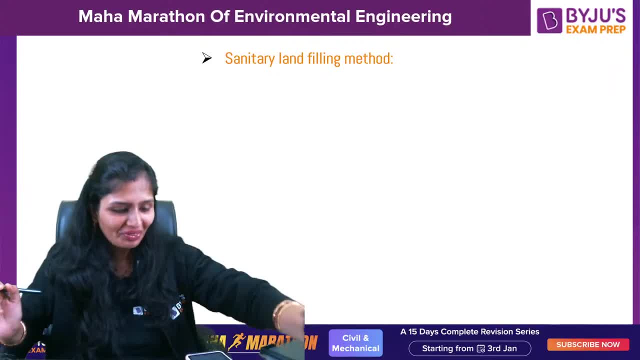 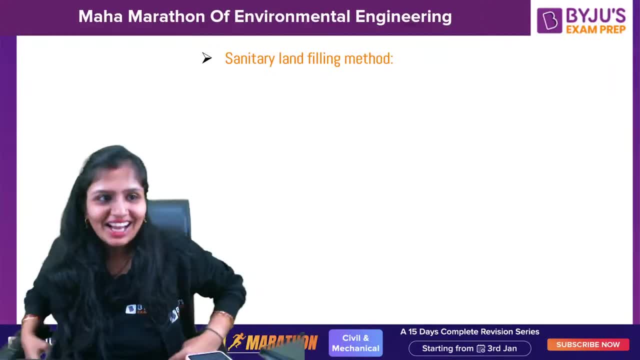 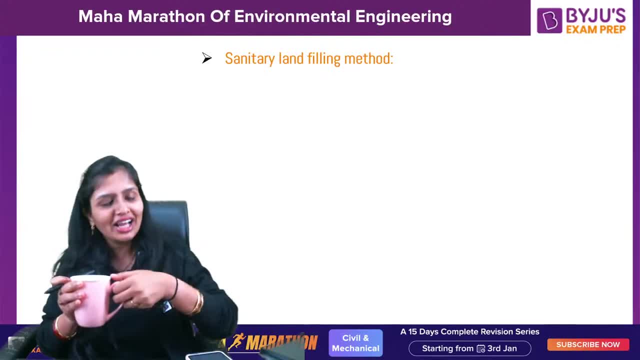 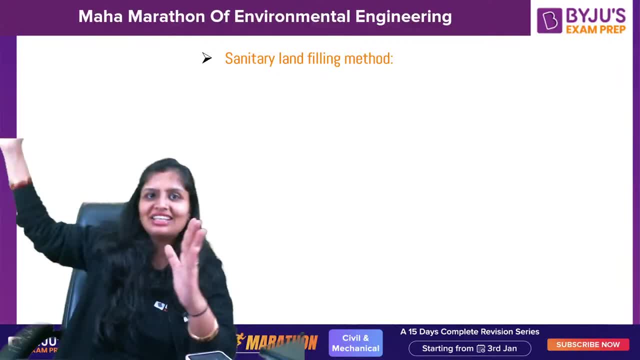 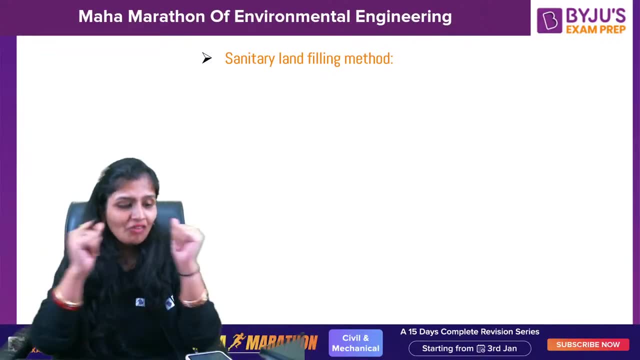 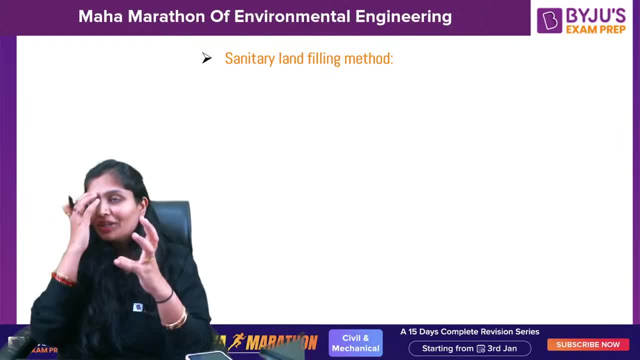 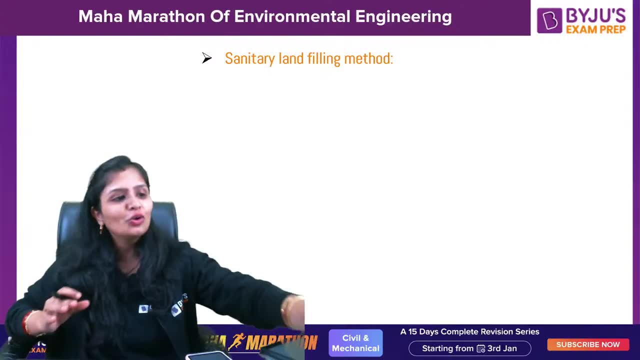 hone se bhi decoration purpose, bilkul sahin bolro pieces hongi main unko colourful, colourful pebbles ke saath mix kar dungi. kuch bhi kar dungi, toad ke chipka dungi aur bol dungi. modern art hai, I can do. 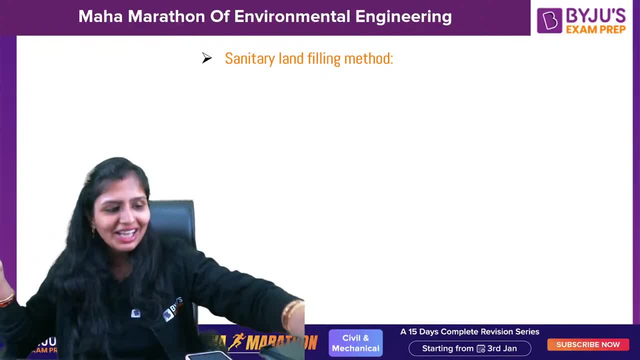 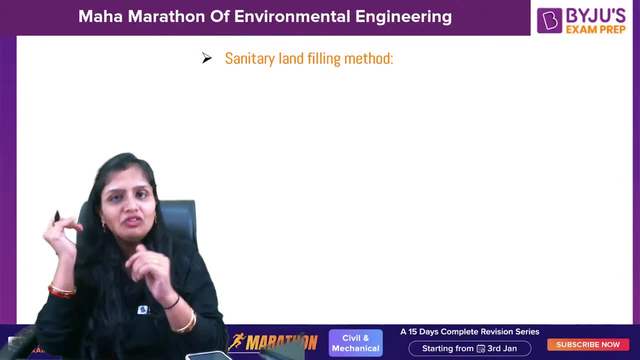 anything that is modern art. I can do that right. so yeah, that's the fact, so this, you know it right. so that's the reason: the energy kilo joule per kg value which you get in India is very less as compared to what you get in. 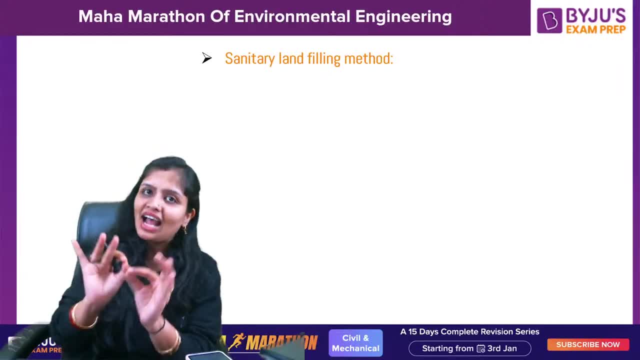 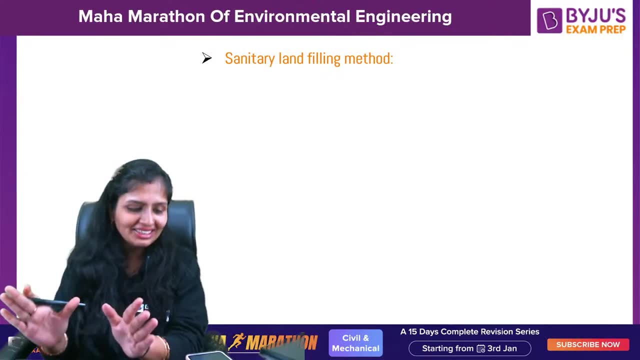 other countries. so if you bring their code and compare it, I have already told you bhai saab nahi ho payega alag hai clear difference. it is there. now let's talking about the methods of treatment, or basically methods of disposal. now talking about the sanitary. 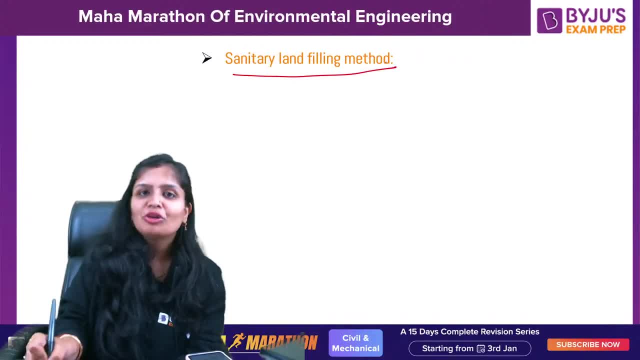 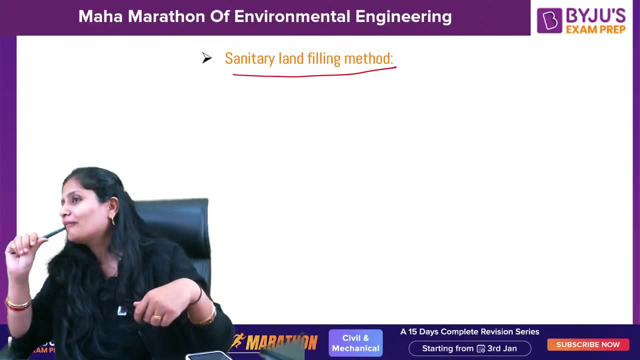 landfilling method, sanitary landfilling method. tum lang bhi bachana, kya kya karto, main kya karti ho. aur ye toh maine k2 kya karta, bote wale ka example de diya aur maine kya kiya hai. 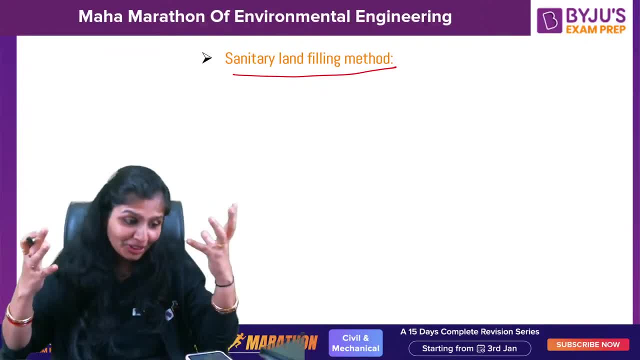 aur maine kya kiya hai? mai soch ke bataungi mujhe instant. mein yaad nahi aara hai ki maine kaunse cheez ka utilization kiya haan, wo jo mug, mug handle which we use for bathing if it breaks out just. 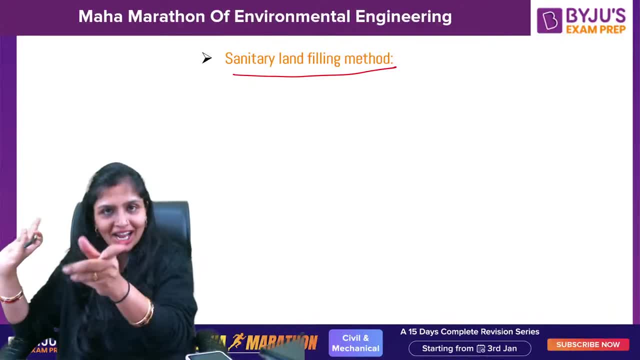 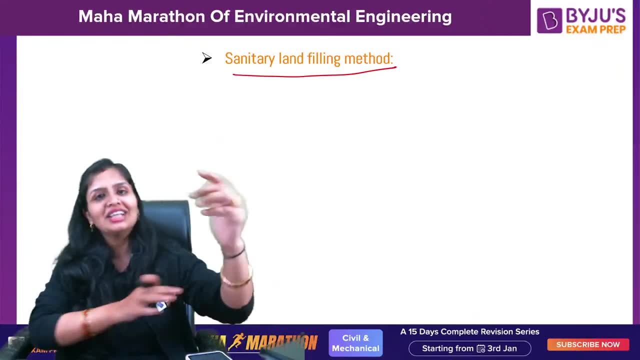 throw it, color it, usme paude laga dete hai. so that work I have done. you guys can also comment and tell me what is the good thing which you have done, being an Indian. okay, so these are the things which I do, it, and I collect the cutleries. 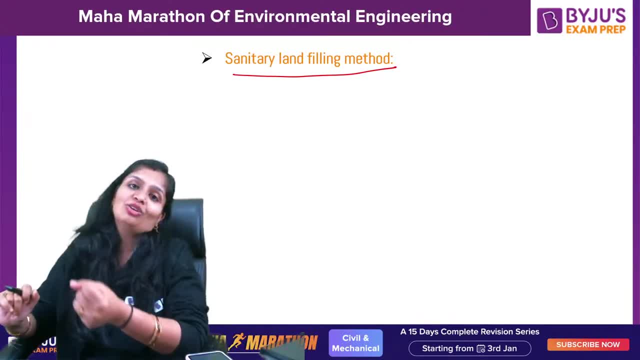 of the hotels and all also. I collect that also. I collect those cutleries and all. and what do I do with that cutleries? phir koi aur aata usko de dete ho thik hai khana dena hai toh. 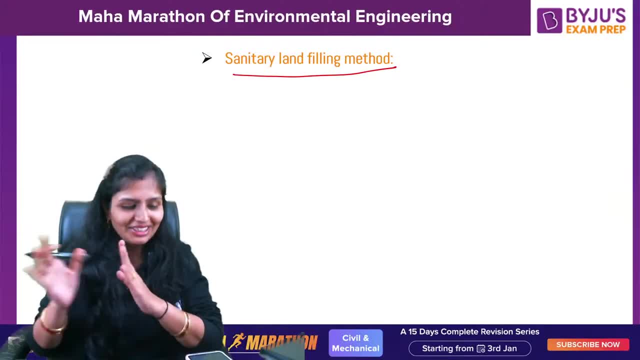 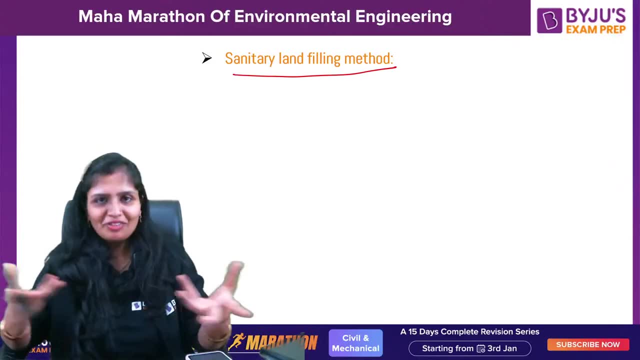 phir apne steel ke dabbe na deke o cutleries de dete hai. so these are the things which I do, Indian things right, and I am proud of it. so, son papdi dibba, we parcel it. all these things, we do it right. 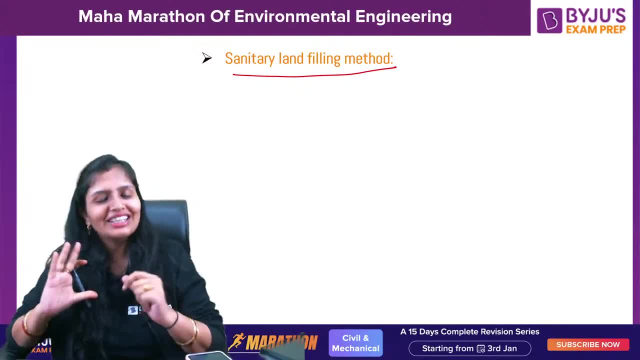 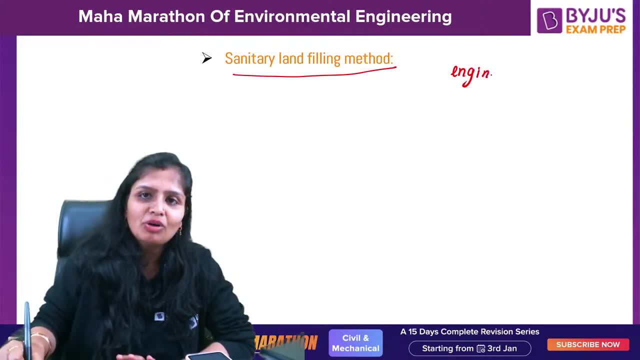 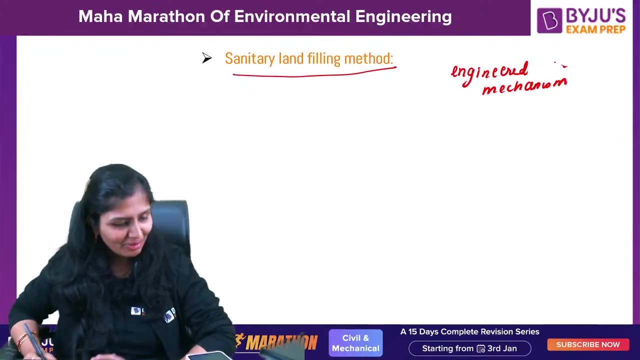 so apnil hus kio raha, yaar, tum nahi karte kya. so this, we do it. so now let's talk about sanitary land filling method. this is a proper, engineered mechanism of engineered mechanism of disposing the solid waste, of solid waste. marriage: cut, convert into something. marriage: 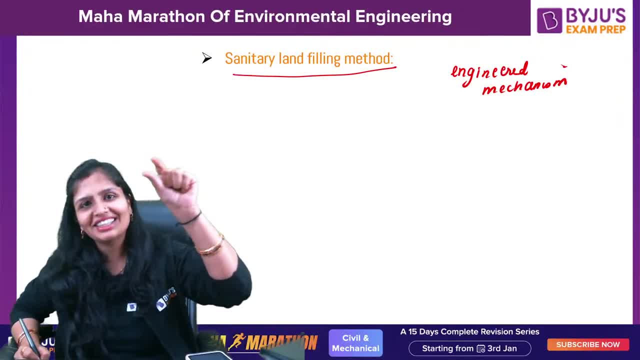 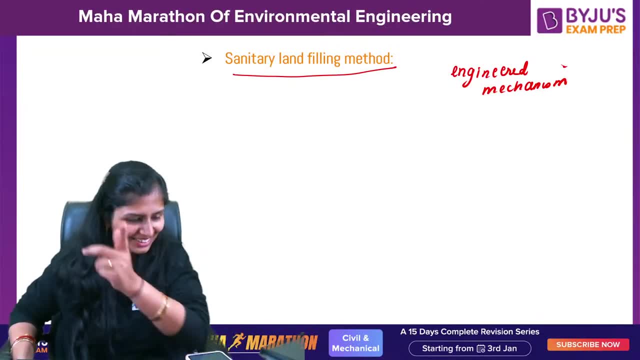 cut kar toh woh pehle chhote the toh Ganesh ji aate the na chipak ke usko use. usko. usko mano phad ke use kar lete the matte wale bowl ko dho ke use correct. 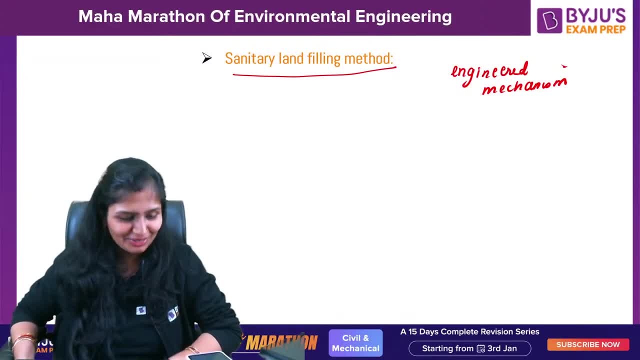 correct humlog bhi mere type ke yo bottle sewaaz bana dete ho. very good, chalo matlab, main akele, hi paagal nahi hu, meri gang bhi paagal hai. chalo so sanitary, ab ye sab kaam karenge. 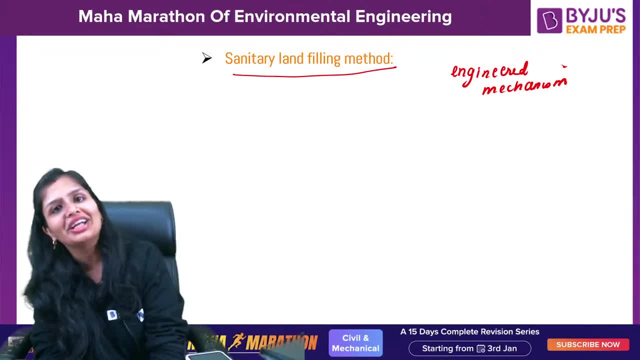 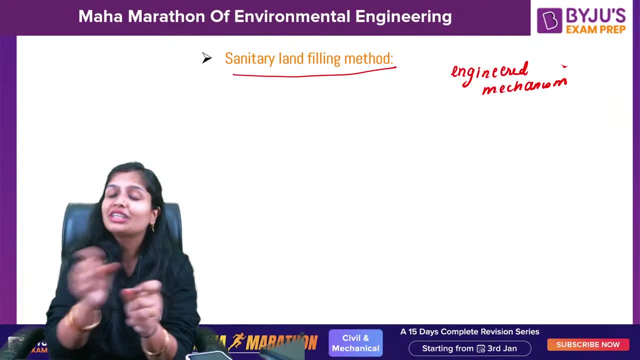 example is: we have taken a toothbrush, we are not throwing it. so this will happen like toothpaste ko antin saath tak hum nikaalenge uske baad bhi. mai kya karte usko kaatte, hum bata hu kyunki. 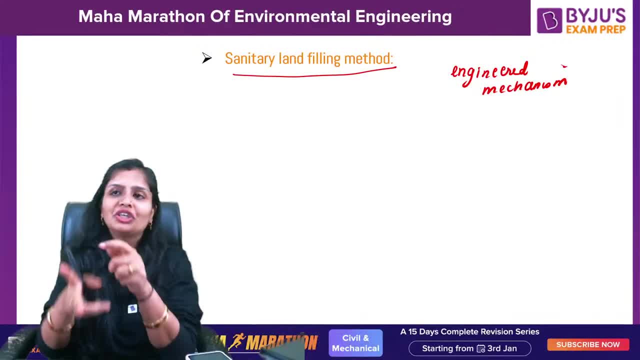 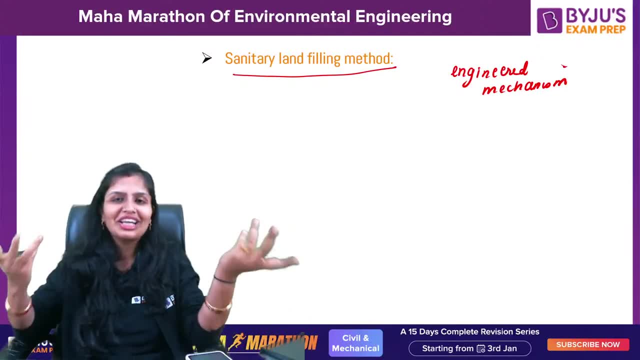 aap usko nikaaloge uske baad bhi usme toothpaste rehta. so what you do? you cut it and you take it out it from the inside steamer bowl as fish tank. see so creative people are there. so this, all things, we do it right. 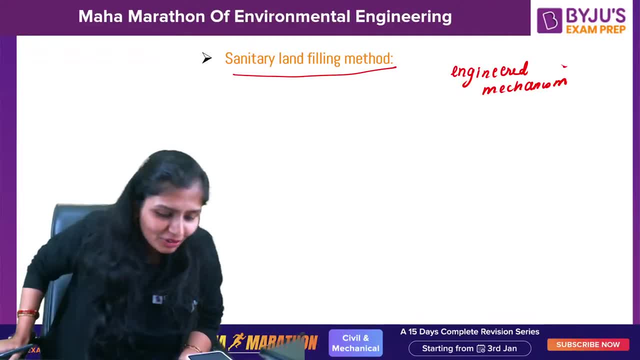 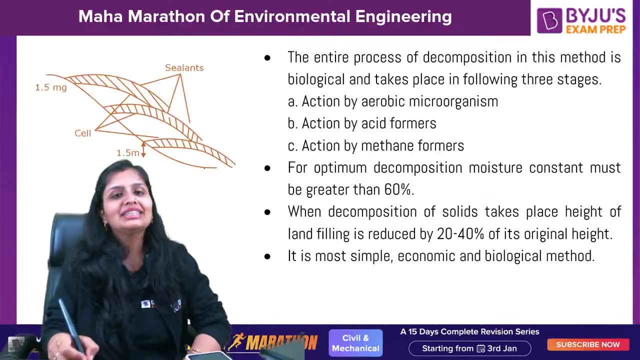 so kaha se milegi energy kilo joule per kg value. toh kam hi nikal ke aayegi na now sanitary land filling. what you do it? you dump it. you can see it here: 0.5 meter. dump it, compact it. 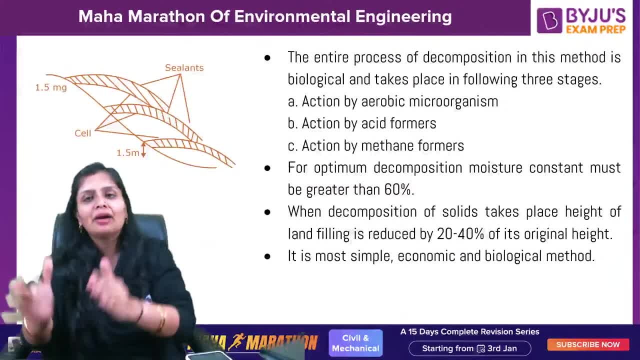 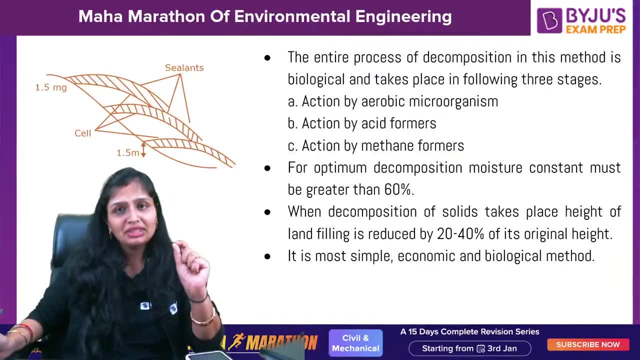 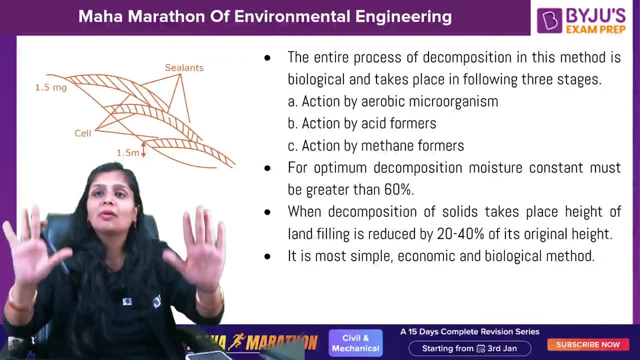 0.5 meter, dump it, compact it. 0.5 meter, dump it, compact it. then spray a good earth soil over it. now what happens is what happens is, technically, in a single day you should do 1.5 meter of compaction, and then you shouldn't compact for. 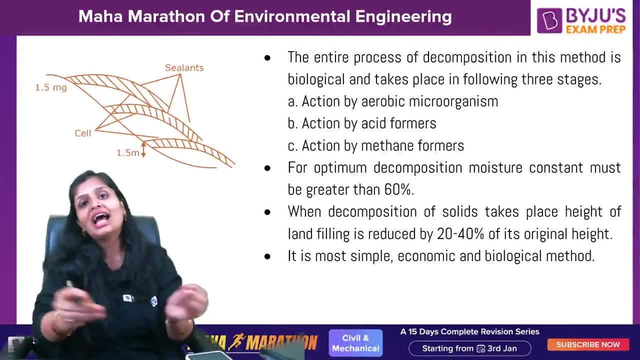 7 days, why you should not basically add any amount of more solid waste there for 7 days, but practically in India they don't wait for a day. also, lao bhai, lao, bring it, bring it, dispose it off. dispose it off. they do like. 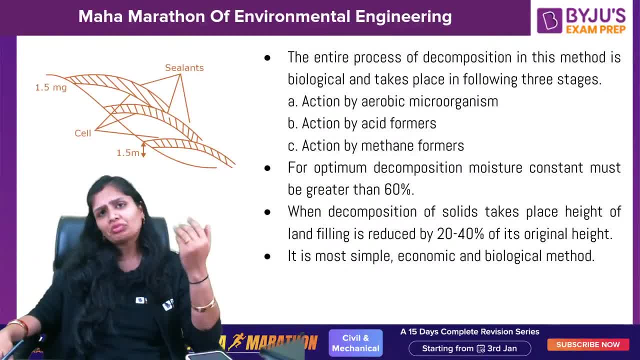 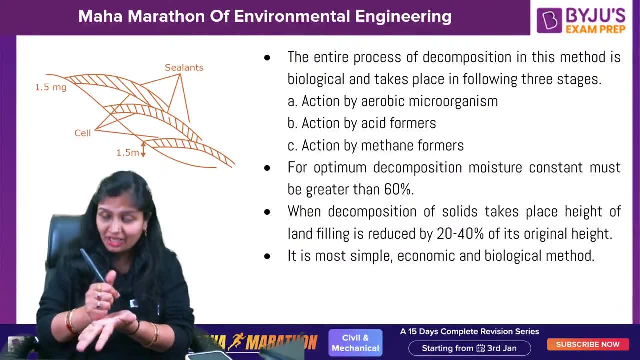 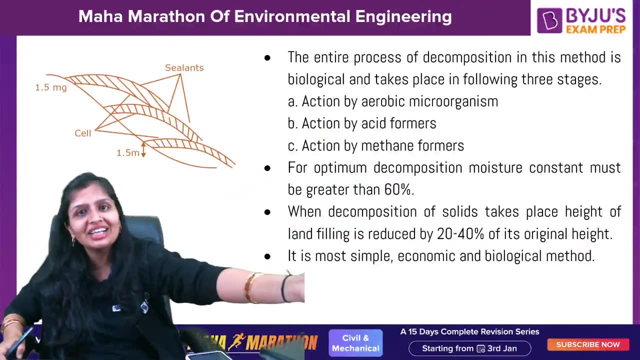 this. so what they do, they are doing it like this. but we say, no, it is a proper engineered mechanism. kitabo mein books. in books it is written like this: but when you go, ma'am, you told wait for 7 days, they are doing it in a single day. 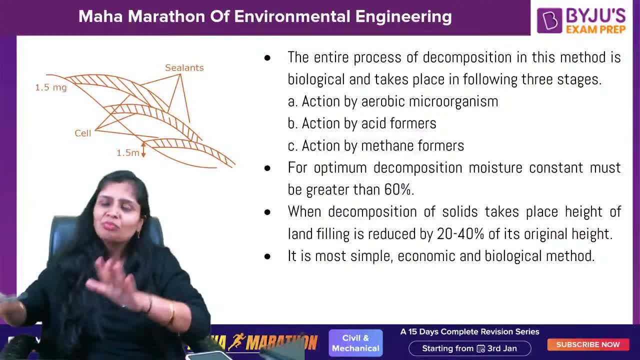 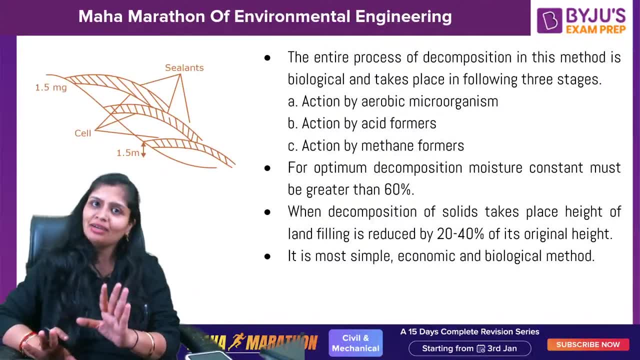 that is the bitter truth. that happens. and you know what? 0.5 meter compact, 0.5 meter compact. they don't do all these things also. so we are starting it, but I told you the ground reality also. so 1.5 meter compaction, you leave. 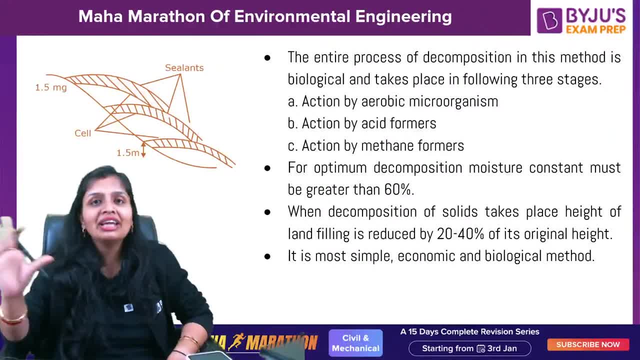 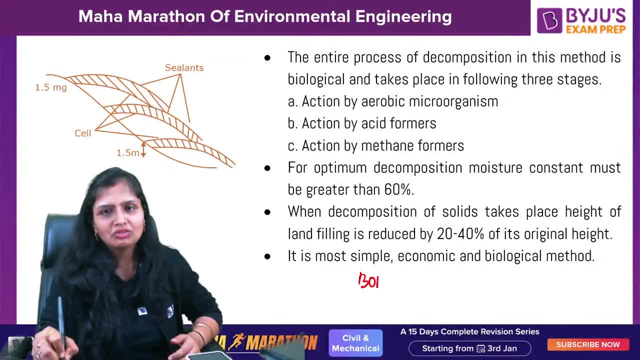 it for 7 days why? example: BOD- maximum amount of BOD value. biochemical oxygen demand is satisfied how I will tell you here also. just wait 7 days. BOD ultimate: 1 minus e to the power. let us take 0.23 into 7. 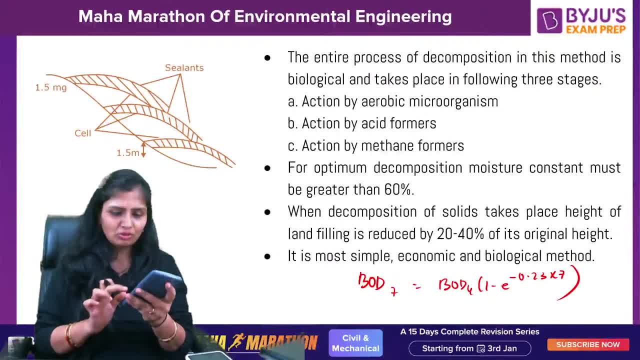 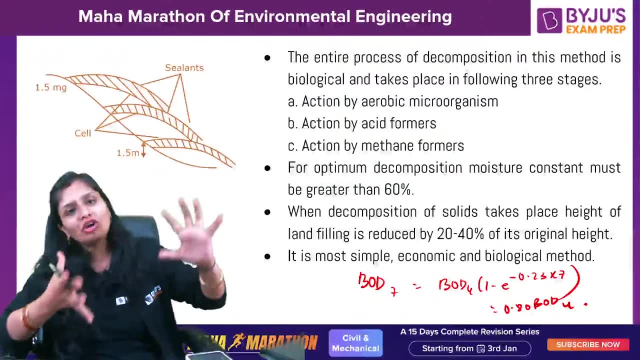 how much it is coming 1 minus e to the power, 0.8, see 80% value of BOD is satisfied, but you don't do it. ok, then again, you compact it, you put good earth soil over it, so what you are doing it. 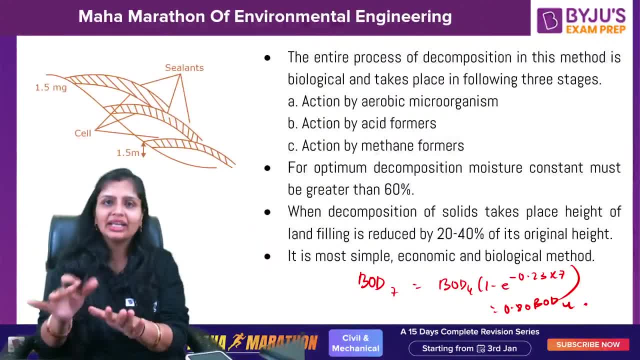 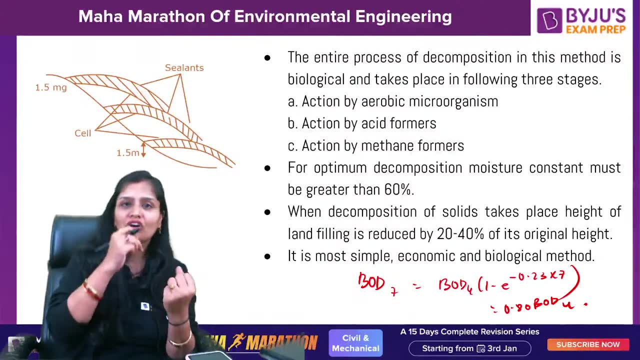 what you are doing it. you are throwing the solid waste, compacting it and allowing the aerobic microorganisms, the acid formers, the methane formers, to attack on this first. initially, oxygen will be there, so aerobic microorganisms will be there. eventually, acid formers will become, which are facultative. 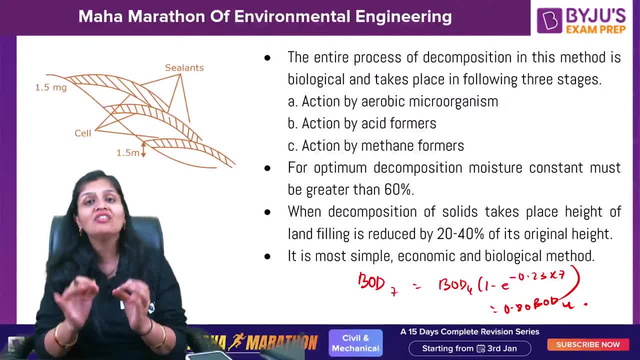 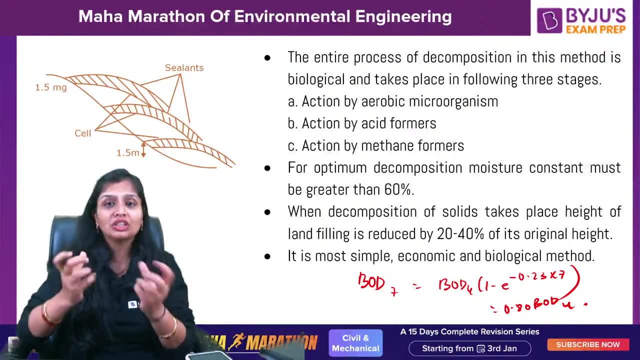 also in nature. after that, methane formers will become, which are strictly anaerobic. it functions in a narrow pH range and they will reduce the solid waste further. ma'am, how come we will know that the solid waste is reduced? you will reduce the height, this height. 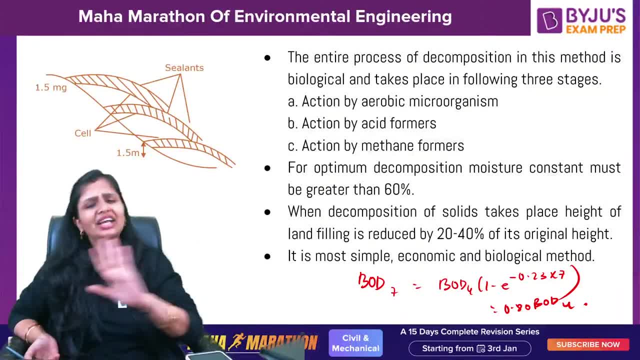 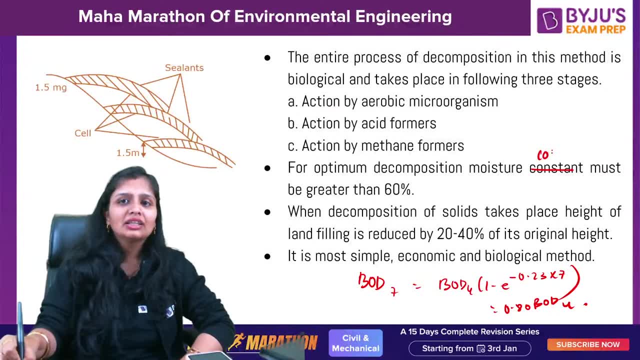 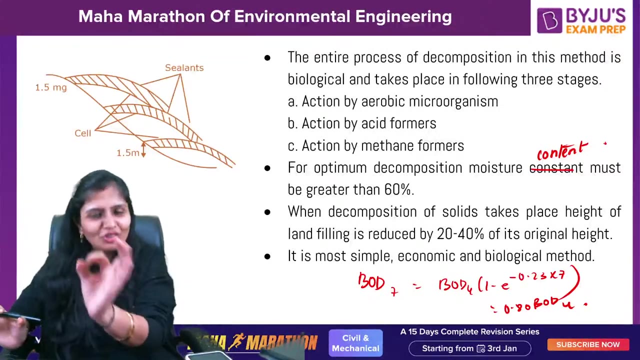 will be reduced to 20 to 40%. simple, economical. you are not doing anything, microorganisms is doing it. ok, and for this the moisture content should be greater than 60%. ok, same same shears is done by my father in law. same big to same. 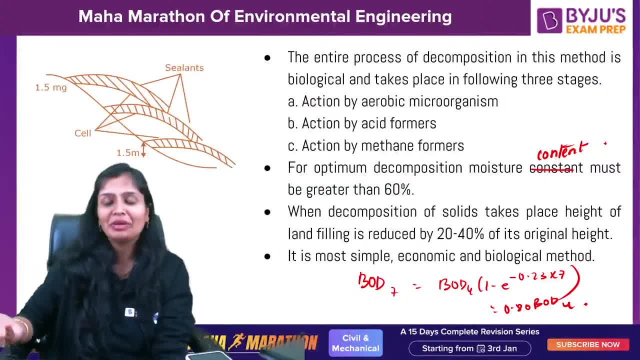 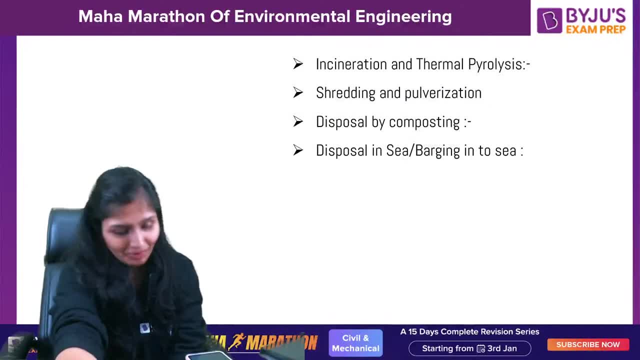 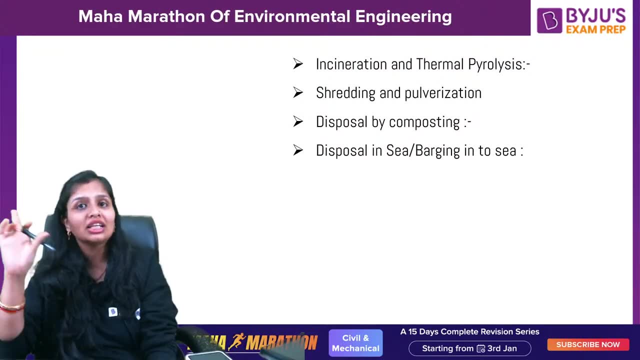 now. we don't have space in our home to keep anything. I am living. that is more than sufficient. so this is the method for sanitary land filling. now incineration and thermal pyrolysis. incineration: you burn it. this question has been asked. incineration: abundant supply of. 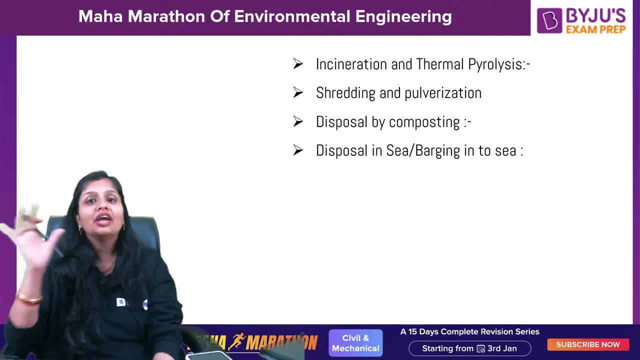 oxygen pyrolysis in the limited supply of oxygen. when you burn it in the limited supply of oxygen specifically you burn, burn only those solid waste which gives you high, which are combustible, and they will give you a high calorific value. ok, so that you can use that for selling. 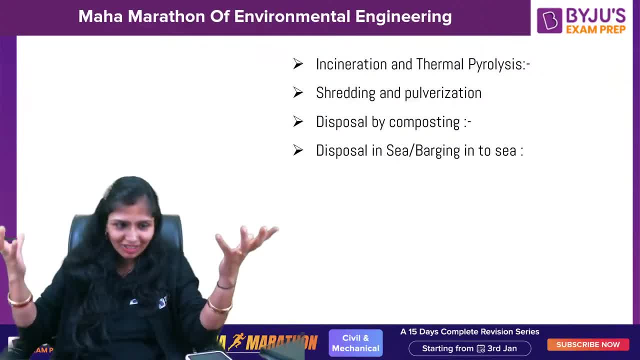 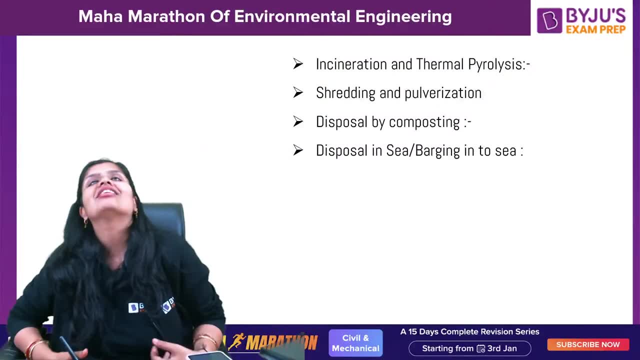 and it will be like money will be money, babu bhaiya. so like that you will get money, money, more money, and then more money, then rich, then super rich, then iphone, then audi, then a bungalow- many things you can have, not that much amount you. 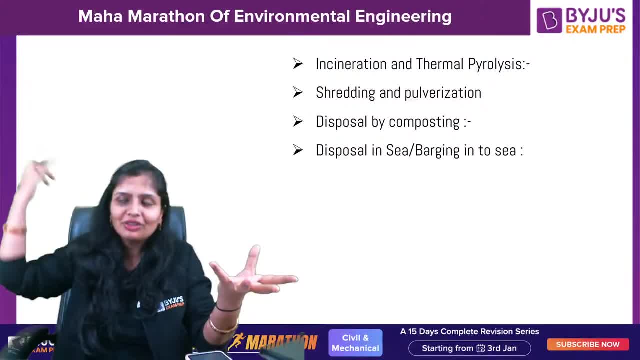 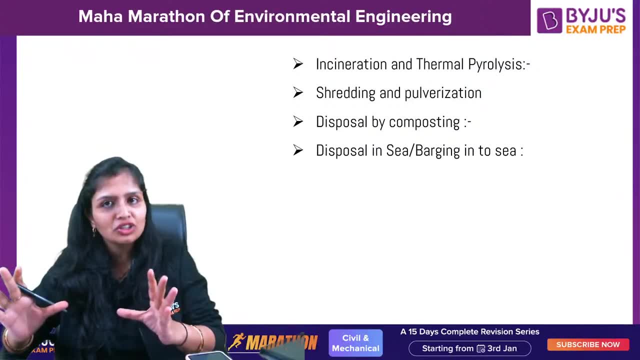 get. but when you burn it you will get that much amount of value that you can run the plant. so that is incineration, thermal pyrolysis. you burn it in a limited supply of oxygen, the by products. you get charcoal, you get tar which you can sell. 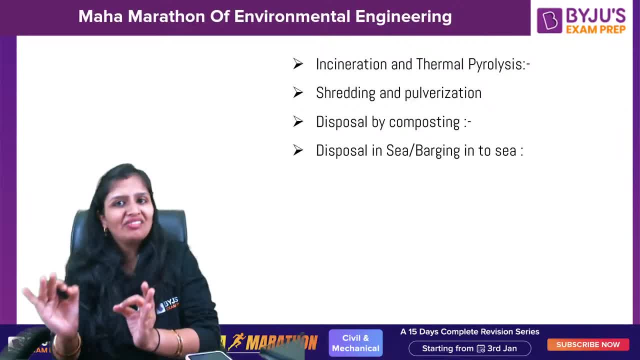 it also ok. shredding and pulverization. basically, this is not any method. higher, basically higher- solids, or the heavy weight solids or the larger solids are reduced into the shorter forms. pulverization and all means: you grind it, you convert it into powdered form. that's it, what you do. 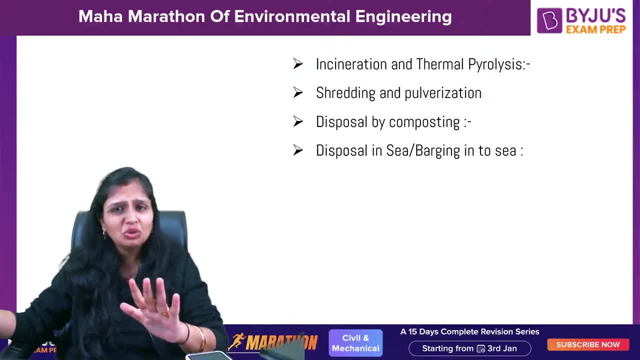 disposal in seas and all dispose it in the seas. nowadays you don't do it. reason for that is it comes back. ok, unsanitary conditions are there, you have to dispose it, and low tides conditions: you have to go deep away from the seashore and 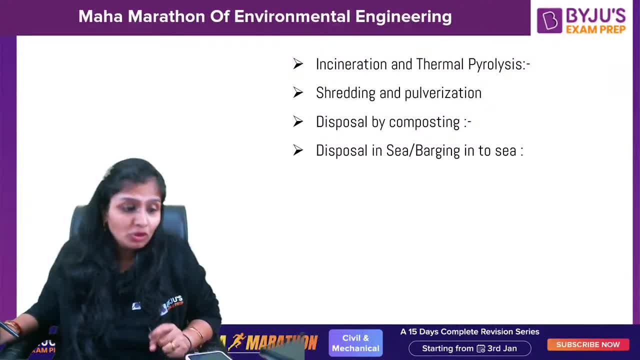 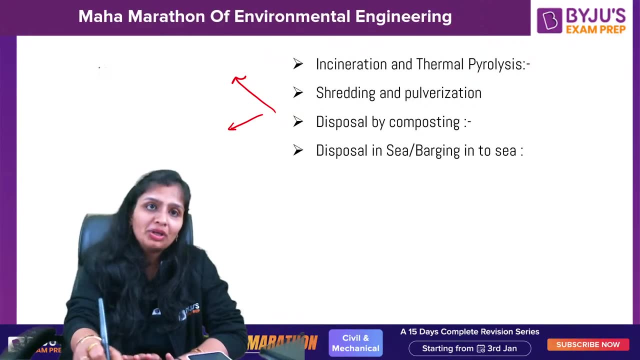 dispose it. so it is a costly process. now, composting, which somebody was telling na that chhilke vilke, they used it for creating a compost. that's a good thing. those things, those biodegradable waste we go for composting very popular is two things. one is bangalore method. 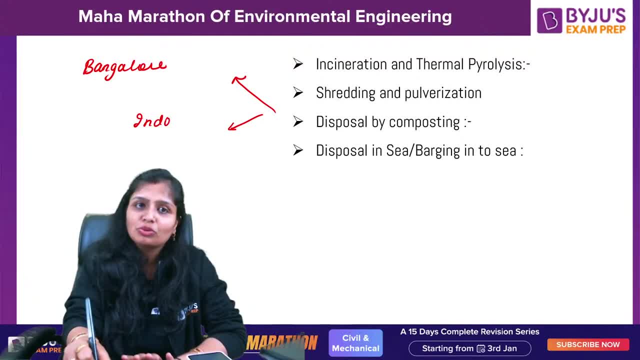 of composting and another one is indore method of composting developed in those cities, so name as that's a blunder, that's a blunder, which is the blunder, which is the blunder: wamsi, bangalore method of composting, indore. 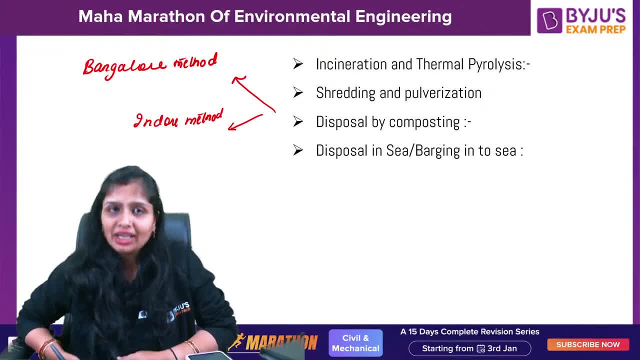 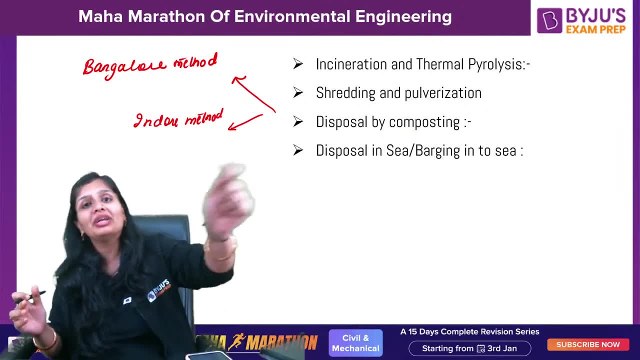 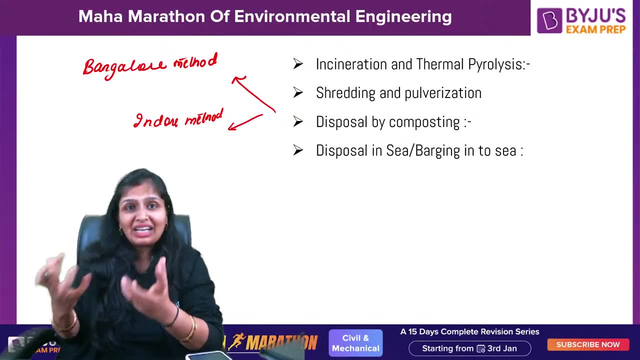 method of composting. bangalore method is an anaerobic method. you break it, just dump it. now you won't turn it and all indore method. what you do, you properly turn it after a suitable intervals so that aerobic condition is maintained. so indore method, practically. 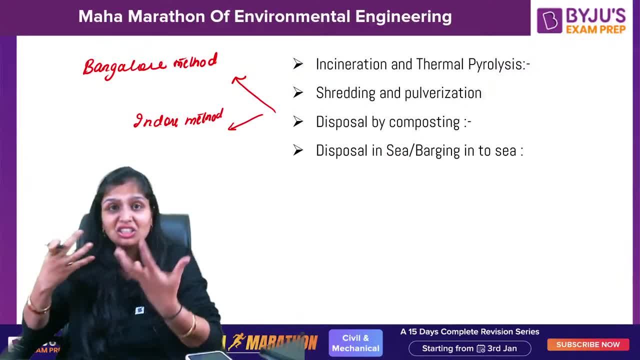 going it and turning it is something which is like, smells right. so that is the reason in many of the municipal corporation: if you will go, they will prefer what. they will prefer what bangalore method? because it is anaerobic. you just keep it, you don't have to turn. 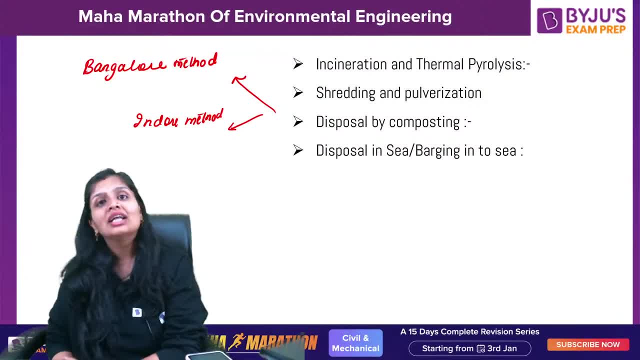 it out, so for maintaining aerobic conditions. but the decomposition will take place, how you will see. you will see the decomposition in terms of height disposal when you do by composting, there will be a thing which is which you will get is humus manure, which you call it as khad also okay. 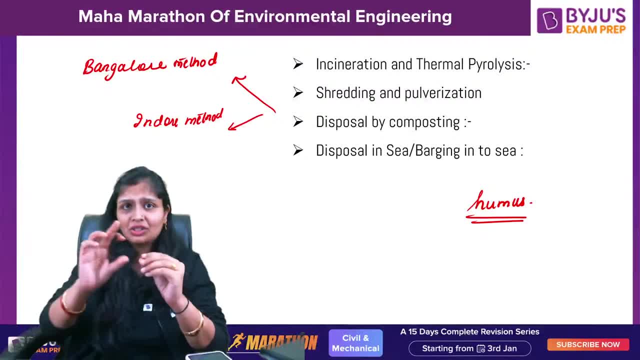 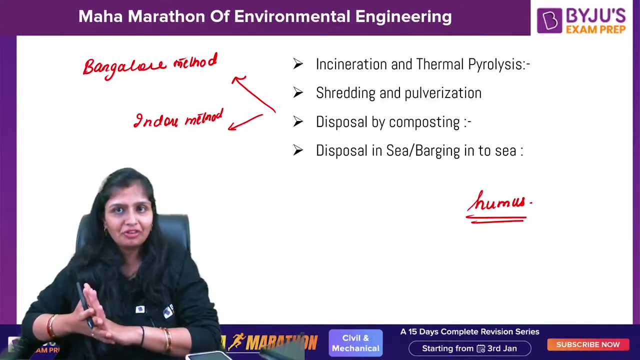 okay. so this humus, you guys, while knowing it, you go and purchase this also because when you use it in your crops and all for sowing it, it gives a higher productivity. so you get it from bangalore method indore, okay. yeah, bangalore method is the preferable. 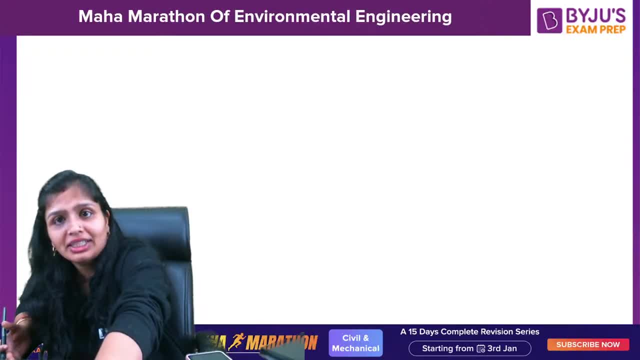 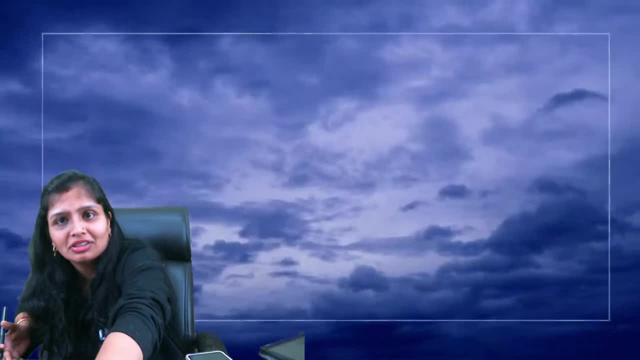 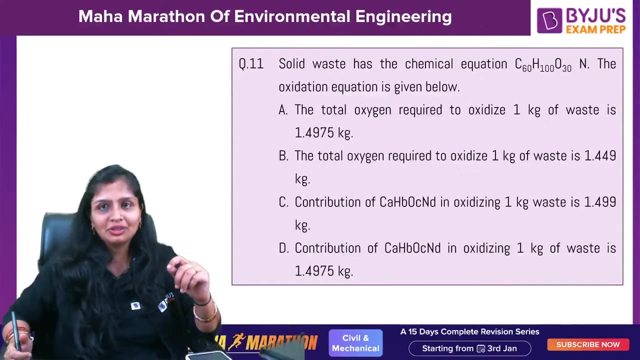 okay, now these are the two questions. where is that question gone? where is one more question? was there? no, just a minute. okay, fine, this is the question. oh, that was for air pollution. okay, this is an msq question. i made banana plant. msq question, msq question. come on, guys. 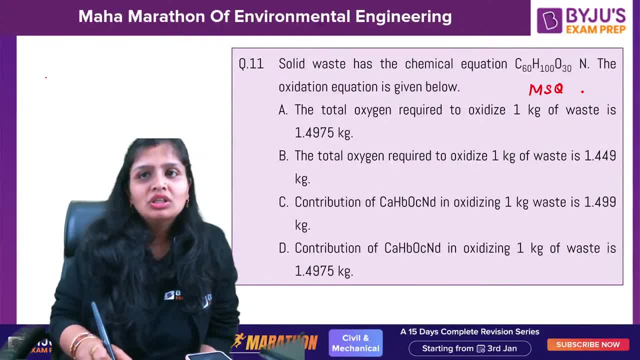 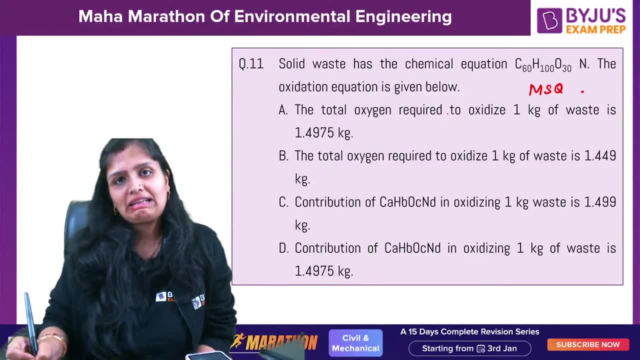 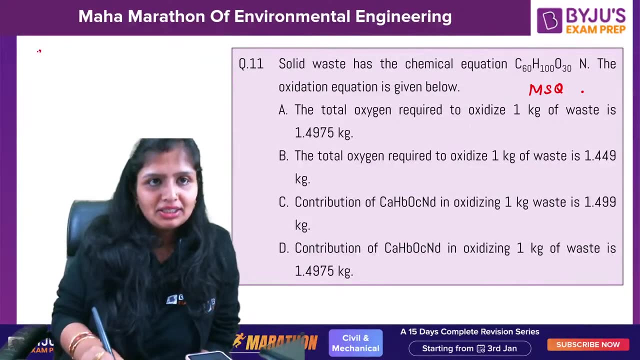 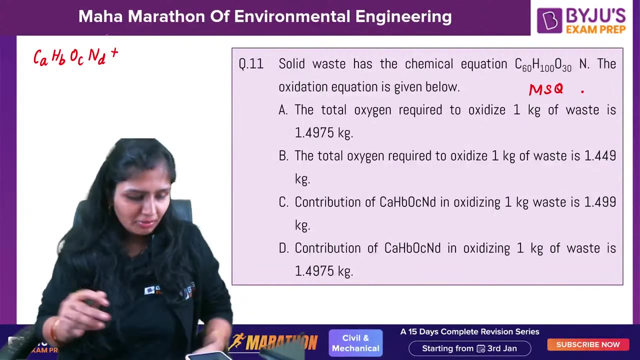 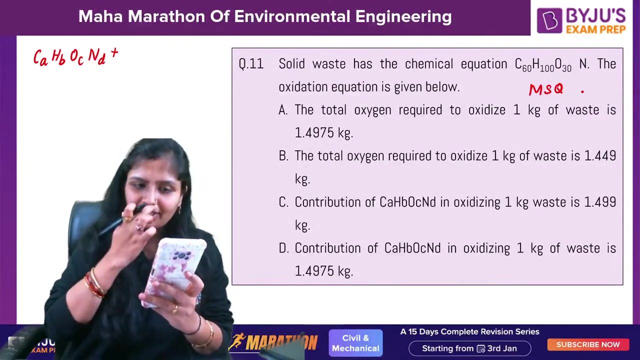 a solid waste is there whose this is given to you. chemical reaction is given to you. oxidation equation: oxidation equation is missing. for this one it will be ca, hb, ocnd plus just a minute. i'll check it out. the oxidation equation should also be there. give me. 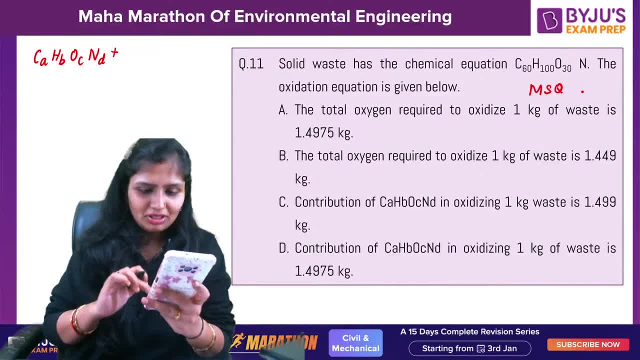 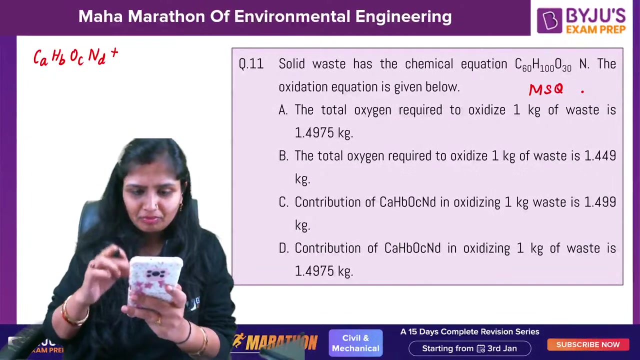 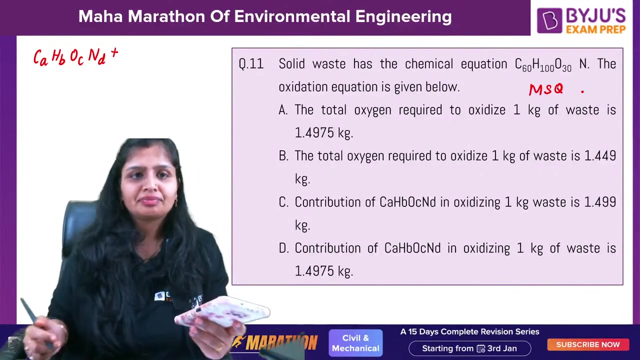 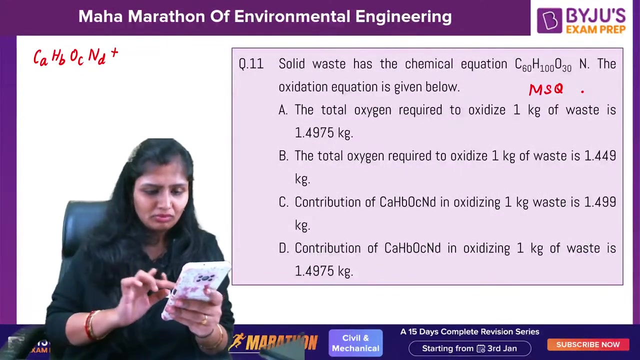 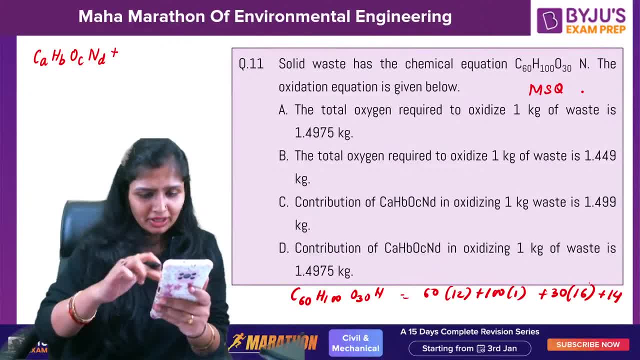 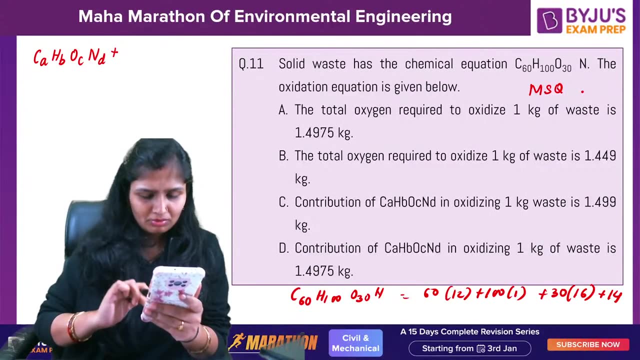 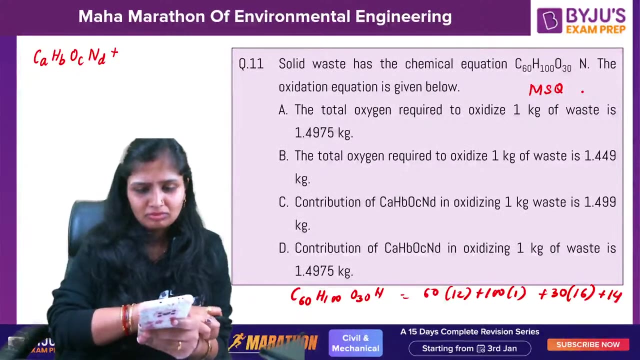 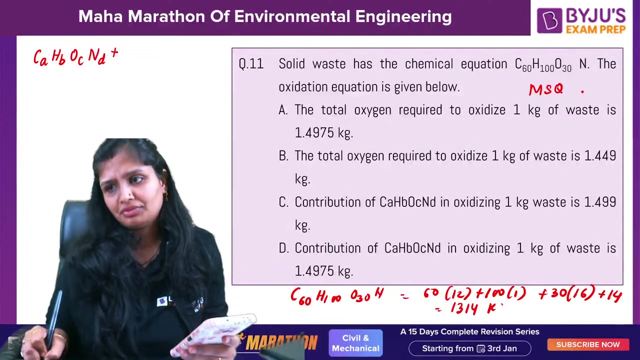 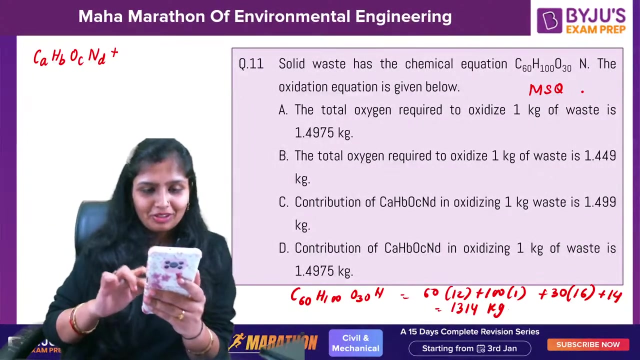 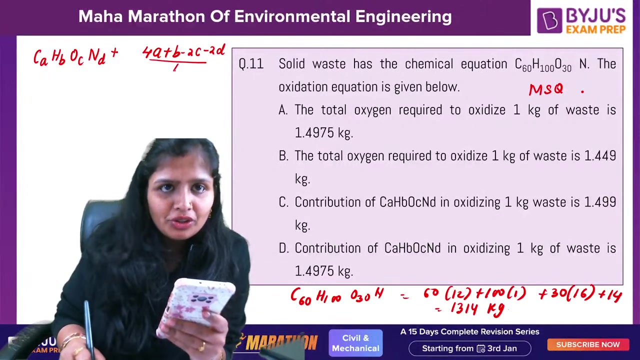 Nitrogen is 14. Come on guys, calculate, Calculate the molecular weight by that time: 1314, 1314- I don't have any quotient in this- Got it? So this is the formula: 4A plus B, minus 2C, minus 2D by 4. 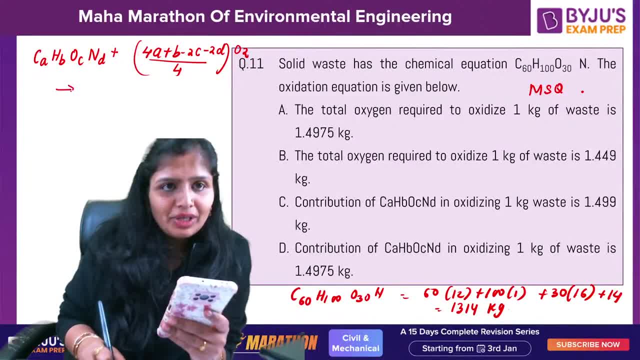 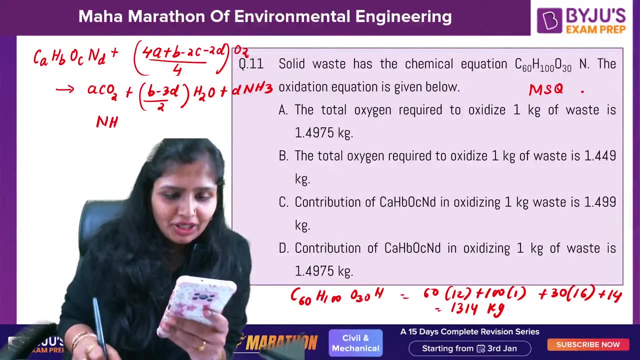 This is O2. This will give you AC. This will give you AC. This is O2 Plus B minus 3D, by 2 H2O Plus the NH3. This is the formula And it is given you. NH3 Plus 2O2 Is H2O plus HNO3. 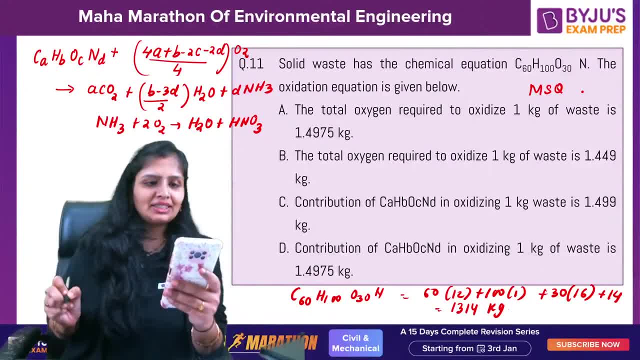 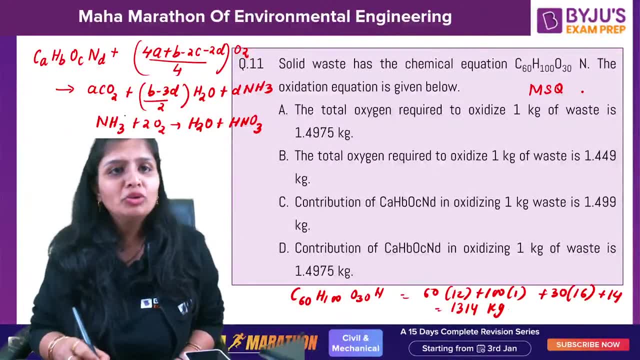 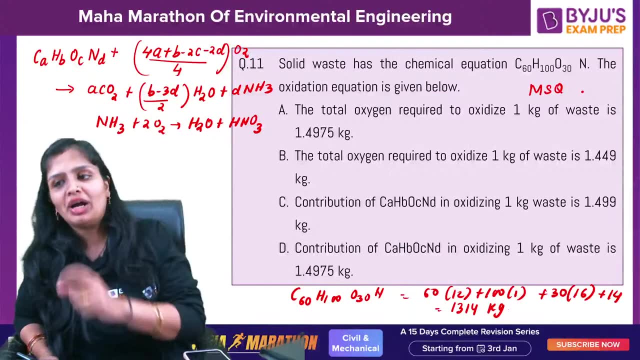 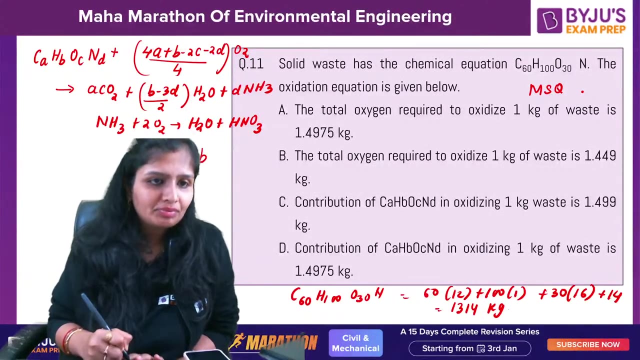 This is the whole question And it is an MSQ question. It is asking you two things: First, contribution of CAAH10 HBOCND in oxidizing 1 kg of waste And the total oxygen requirement. How you will do Now, calculate first the value of 4A plus B. 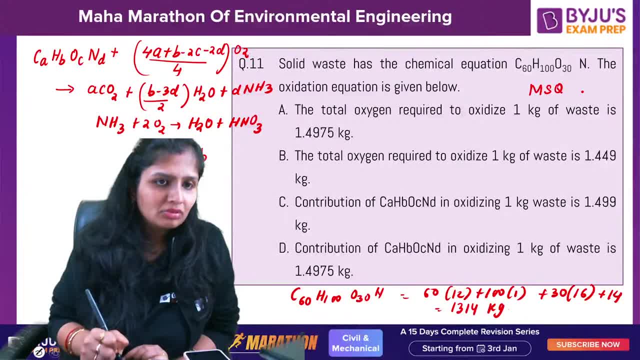 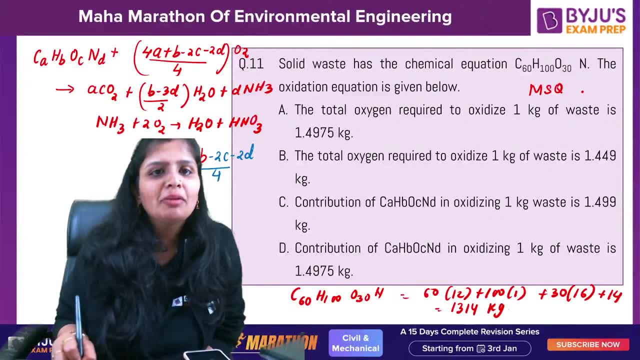 This is a good question. Calculate 4A plus B minus 2C minus 2D by 4 A, B, C, D, you can compare it and you know it: A is 60, B is 100, C is 30 and D is 1. 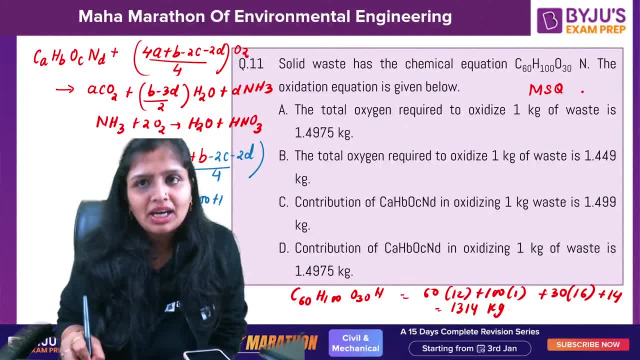 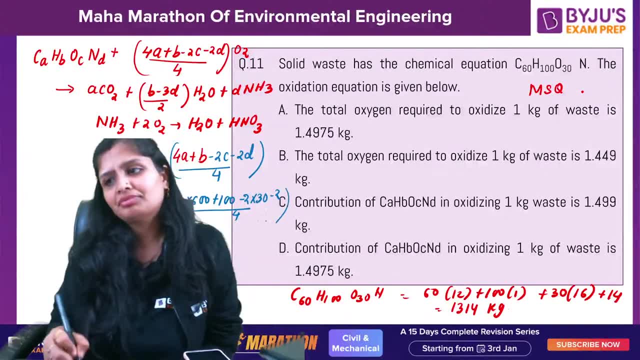 So 4 into C is 100, C is 30 and D is 1. So 4 into C is 60 plus 100 minus 2 into 30 minus 2, divided by 4. How much it is coming. How much it is coming. 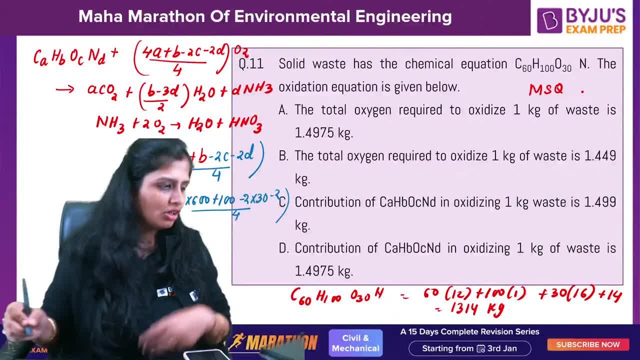 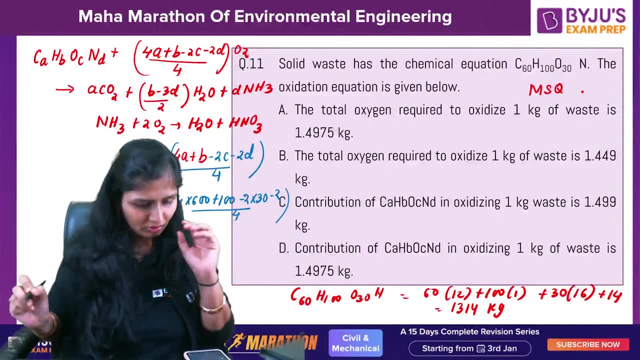 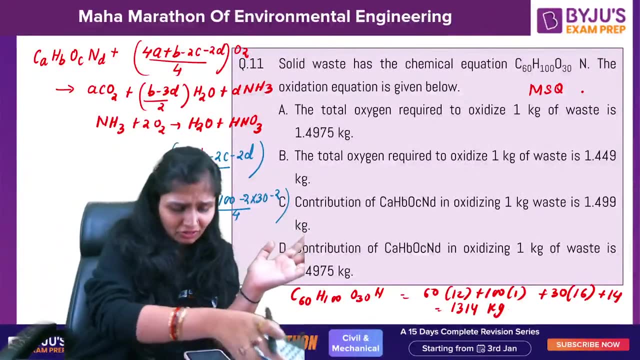 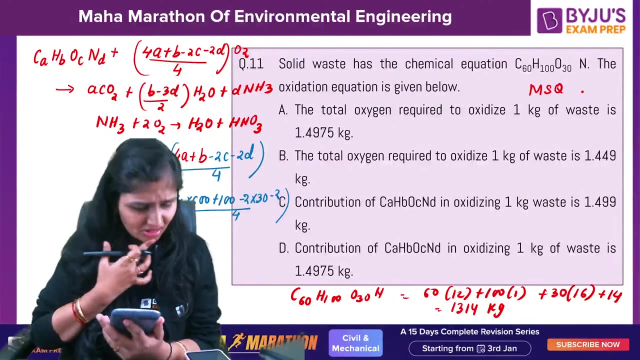 Where it is called How much it is coming: Kg, kg. It is not mentioned. you can take parts also. no issue, Take parts also. Take parts, write kg whatsoever it is. Tell me fast 69.5?. Just check it again. 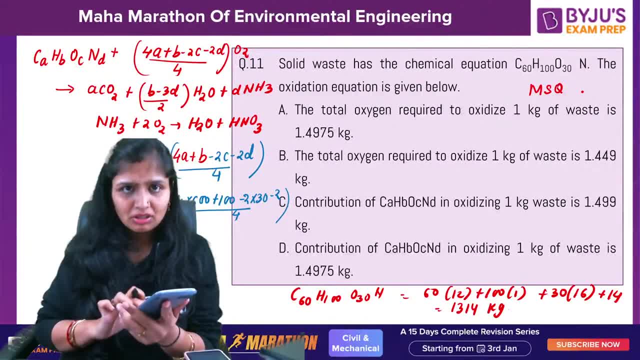 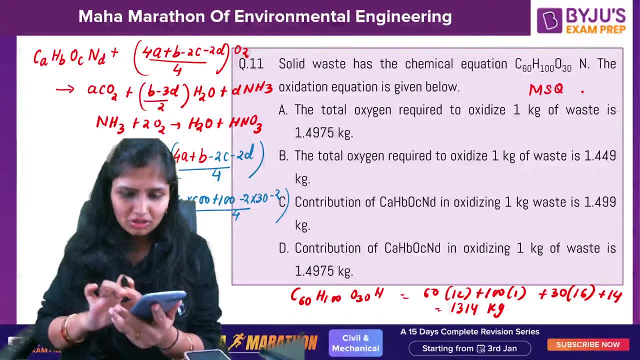 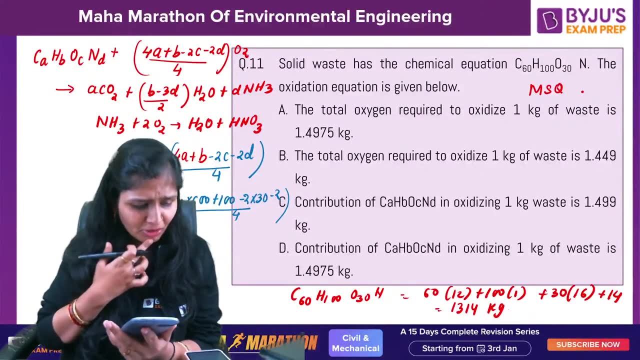 4 into 1600 minus 116.. D is 2, D is there right? 1 by 4.. 559.5 it is coming. How come you are getting 69.5?? Which one you are getting? 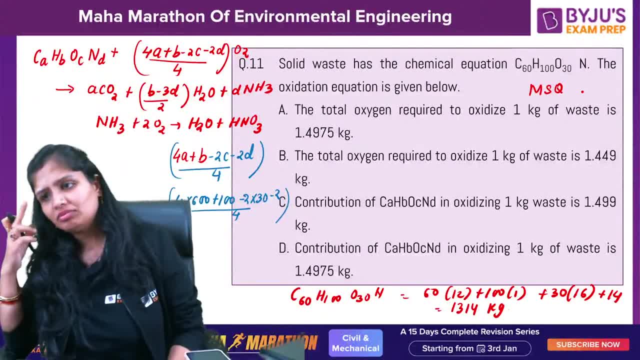 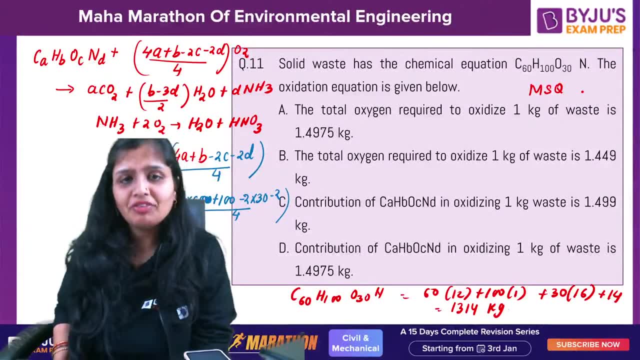 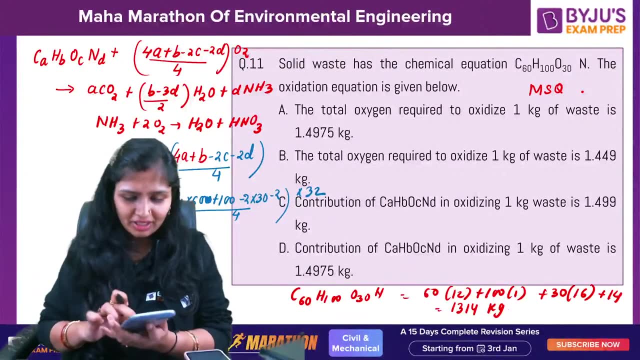 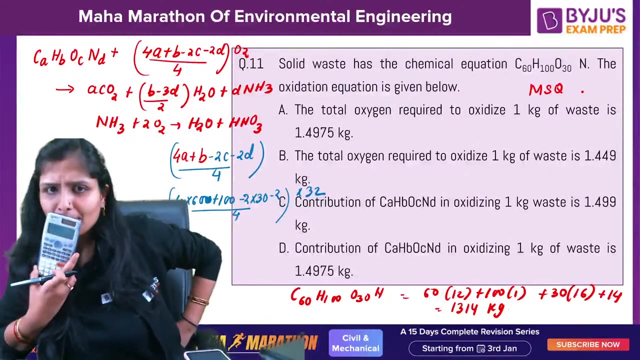 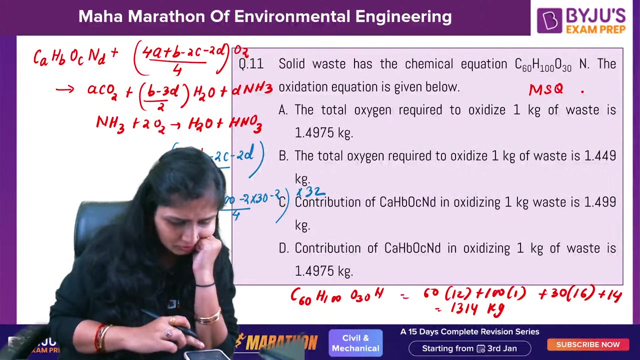 This is 60.. 69.5.. O2 is there? multiply by 32.. Multiply by 32.. I did that mistake. Multiply by 32.. How much you are getting? Just a minute? Just a minute: 360 H100.. 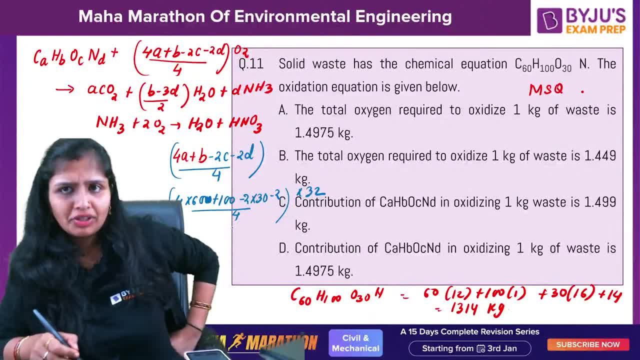 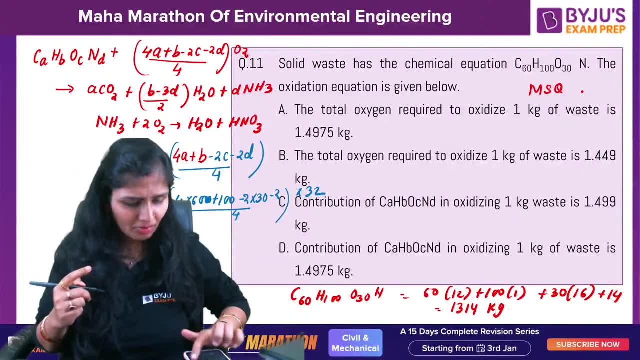 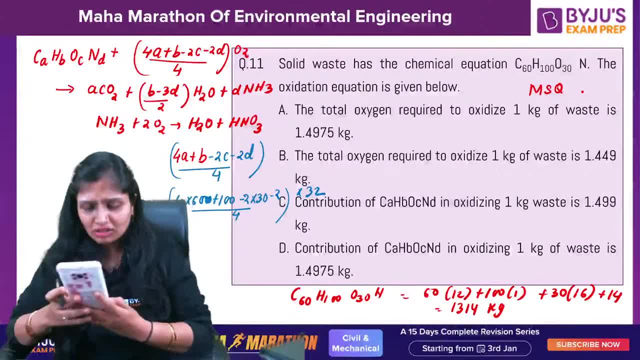 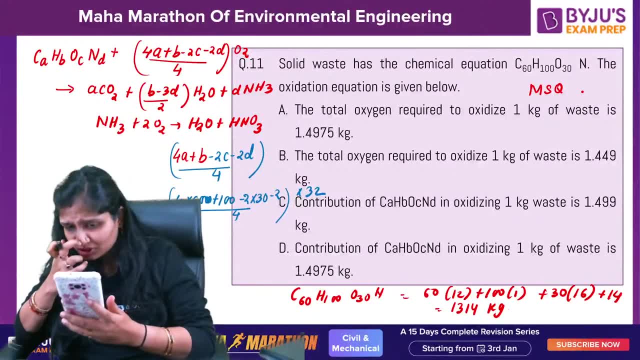 That is what I was just thinking. There is something wrong in this question. This question is not correct. Plus B: According to the question, this is coming, But I am feeling this is wrong. I am feeling this is wrong One second. 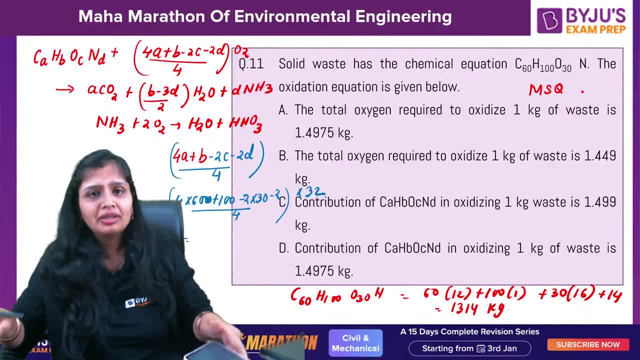 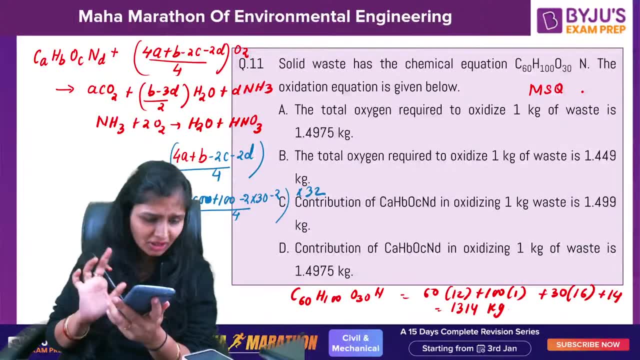 What is Devanshu is telling? Let me do it 4A: 4 into 60.. 4A Question is wrong. Minus B: Minus B is 100.. Minus 2C: Sorry, I am feeling this is wrong. 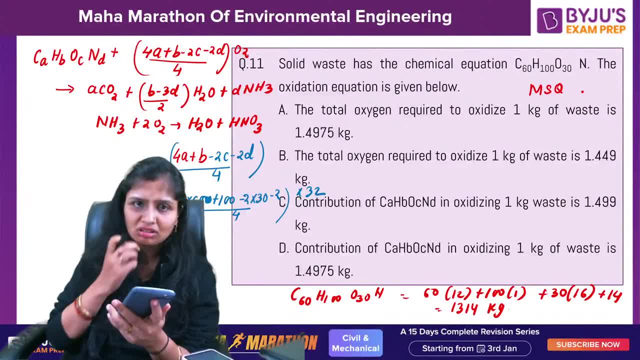 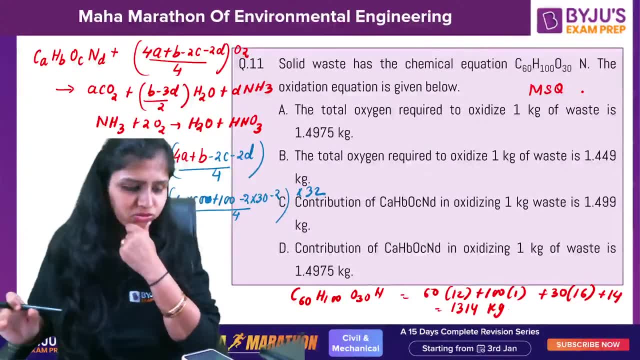 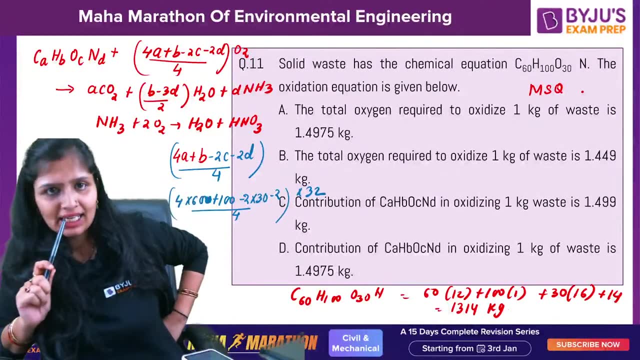 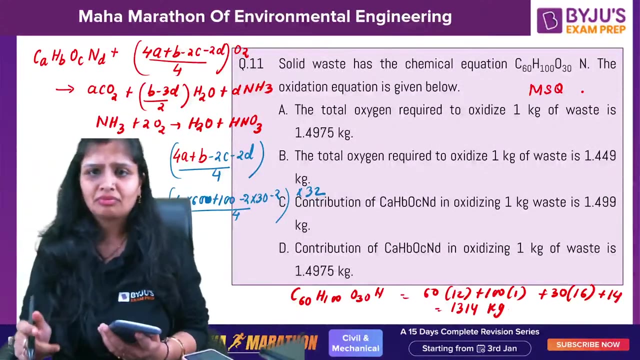 Plus 3D. This is not there. This is not there. This question: there is something wrong with the values. This is not coming correct. Not coming correct. Just do it 50 once, 50.. Take it 50 once. 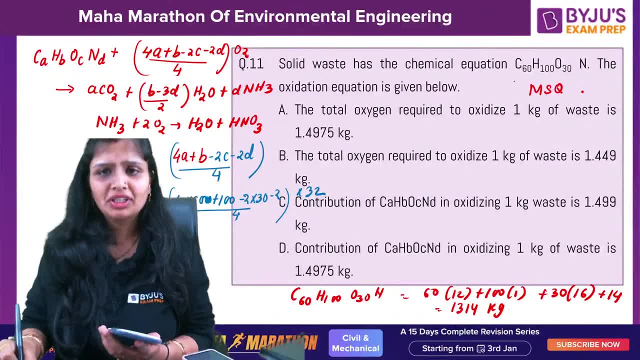 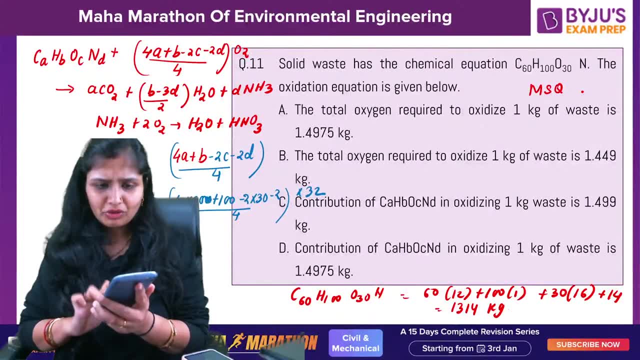 C50.. Take 58.. Just do it once. C50.. C50.. C50.. A value: take it 50.. 4 into 50 plus 100, minus 60 minus 2, divided by 4.. 0, 4.. 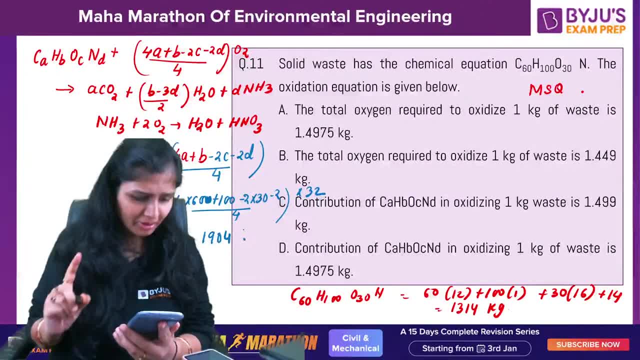 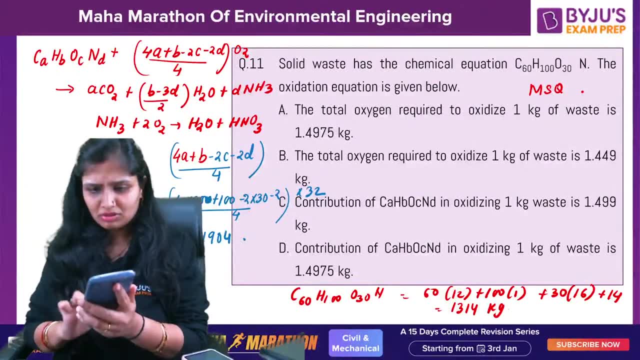 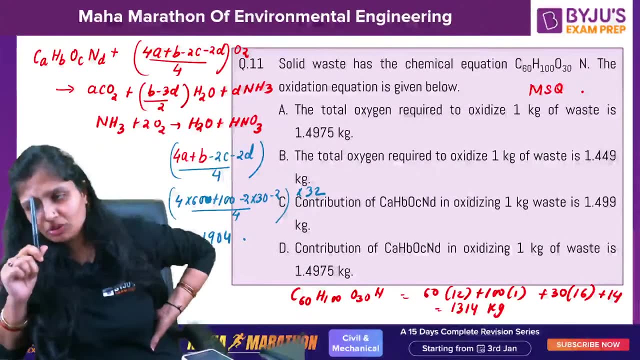 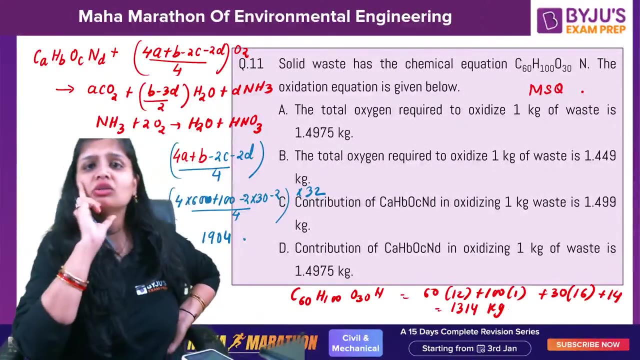 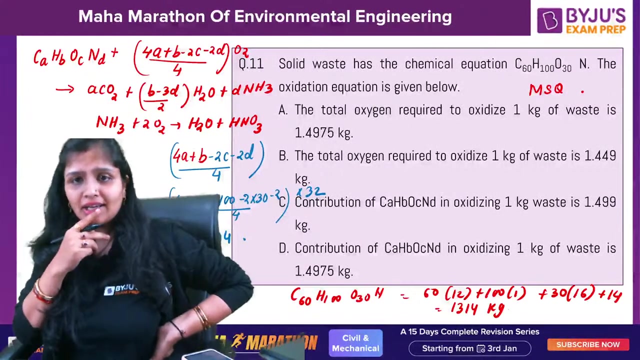 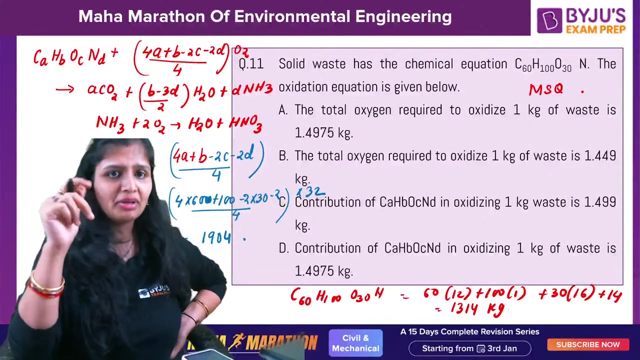 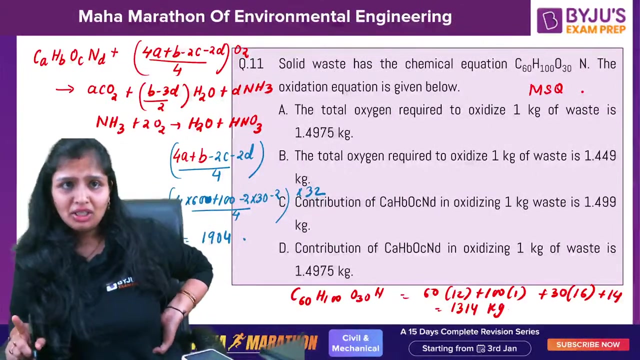 Comes out to be 1, 9,, 0,, 4.. Just a minute, And if I do it here, 50 into 12.. 60. So Okay, So okay, this is a good question, but the values which they have done, they have done some mistakes in this. 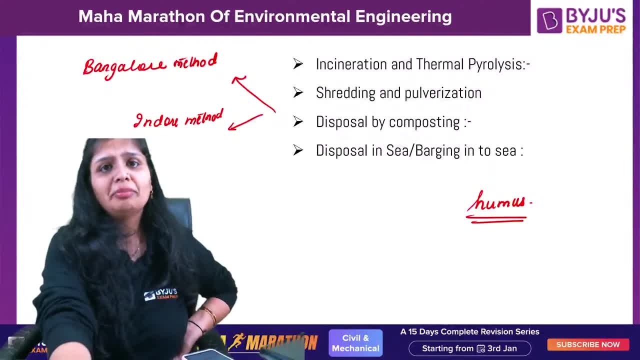 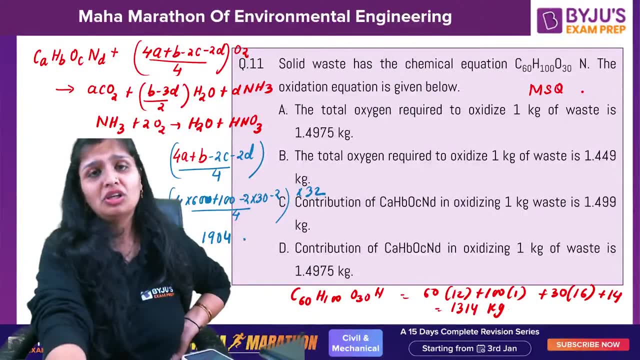 i have to check it out, okay. so who keep it? this question and hold, we'll do this question. simple question is there? only the thing is the balancing is not proper, so you have to balance it out. question that it became wrong. last is the air pollution. so, guys, air pollution. 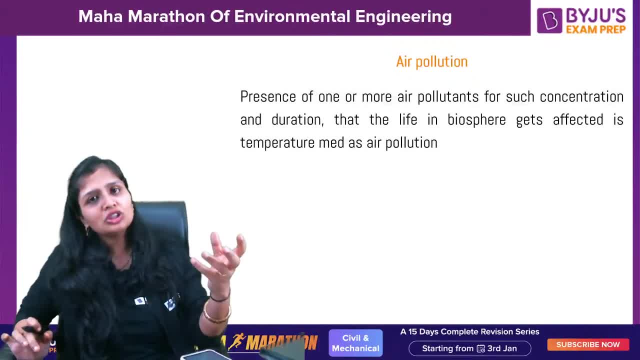 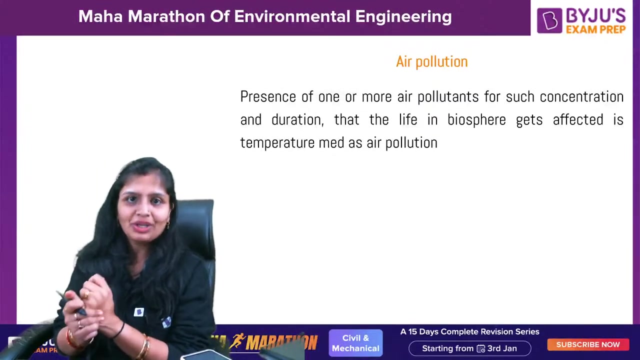 what we do in the air pollution is those pollutants. firstly, what is air pollution? those pollutants which are present. those pollutants which are present in such concentration and in such amounts, which are present in such concentration for a certain time that the life in the biosphere- biosphere is where we are living, where the life persists. persist, okay, it's affected. 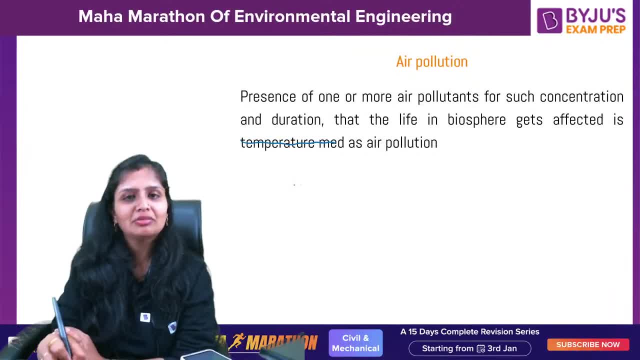 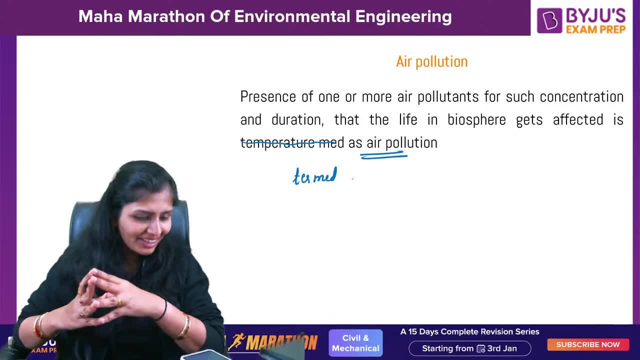 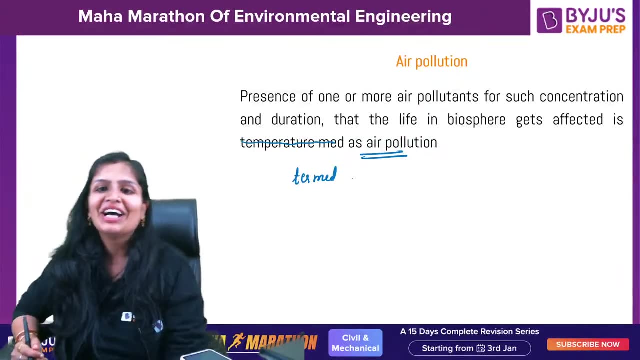 is termed as air pollution is termed as air pollution. okay, now, when you talk about hurry up ma'am, we have to go to panvel in the morning. why do you have to go to panvel? sit quietly and study and leave in the morning. it will be done before an hour. 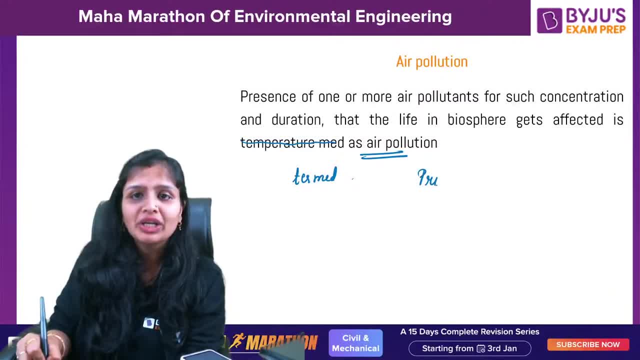 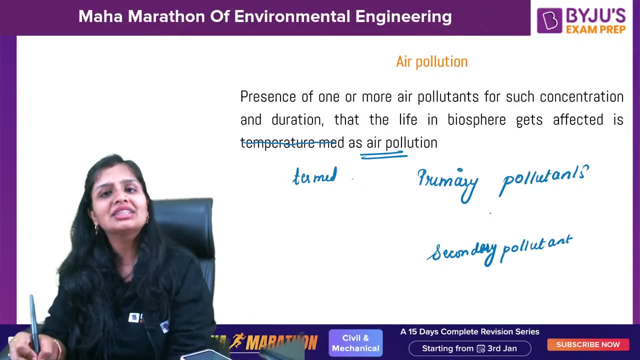 okay, now, when you talk about pollutants, there are two types of pollutants. i don't know which exam is left where they haven't asked this: primary pollutants, secondary pollutants- okay, so the combination, if there are two or more primary pollutants in the say talking about primary pollutants, like example, primary pollutants like the one which you do, профile is suspended. particulate matter. 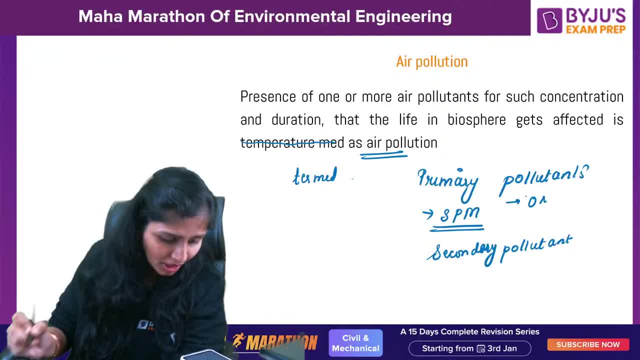 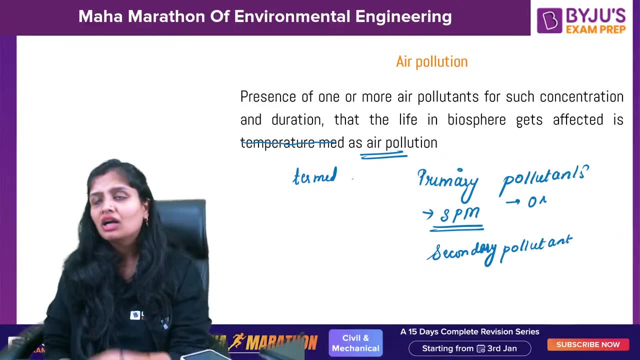 then oxides of nitrogen. uh, mom ask: free basis buffalo for everyone. how do you use it guys? Prashant, that I will take it in that midnight session will happen, Most probably Saturday or Sunday. I will take that session in that I will take it. The questions Questions. 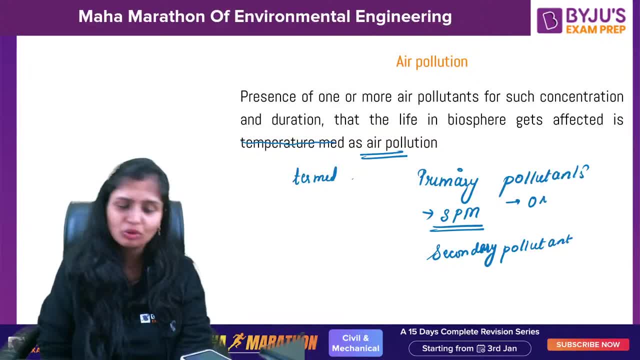 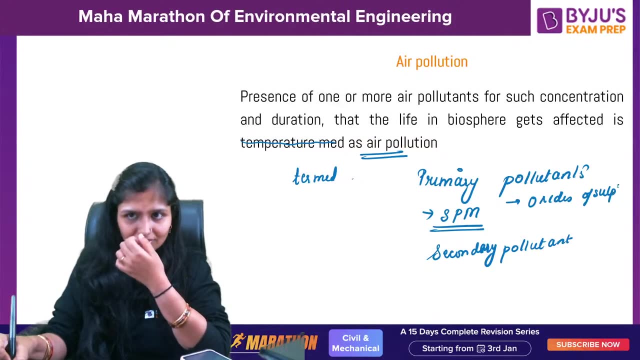 are only there for dry bases and ash free bases, Okay, So don't worry, I won't leave that. Okay. Secondary pollutants we have, like peroxy- Yes, Oxides of sulfur, Oxides of nitrogen. Then secondary pollutants, we have peroxyl acetyl nitrite, We have all these. 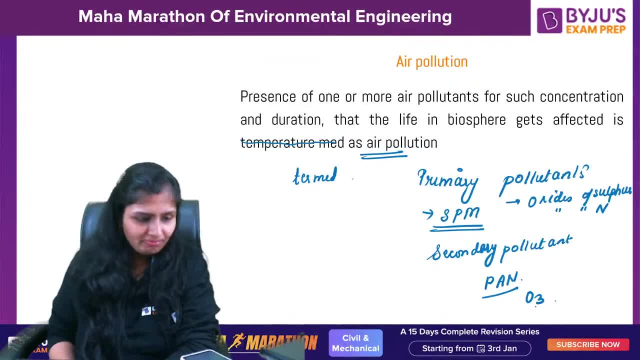 things also For me. it is not buffering, I am checking it. So this is the secondary pollutants. Okay, So these are the secondary pollutants: peroxyl acetyl nitrite and ozone. They give the combination and they ask you which is the primary pollutant. 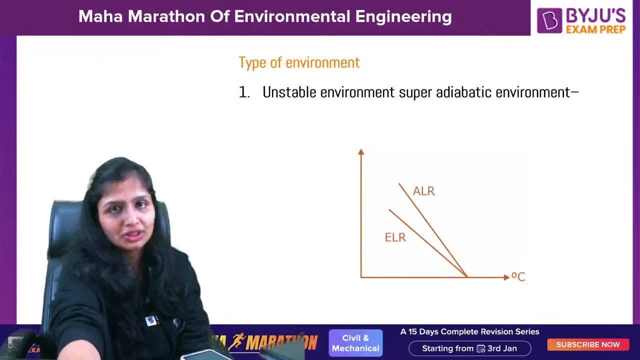 which is the secondary pollutant. So one marks they ask these type of questions. Now, types of environment. First is unstable environment or the super adiabatic environment. What happens? before you study this, you should know two things. One is that you should know that you 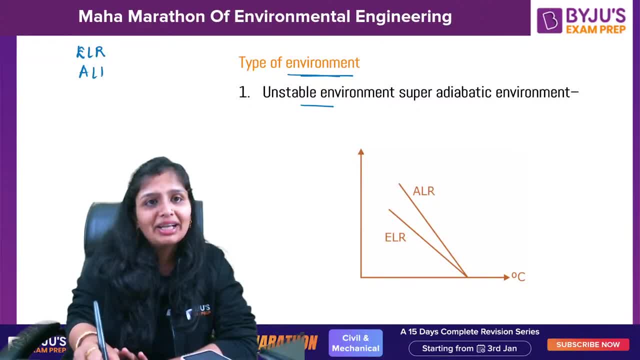 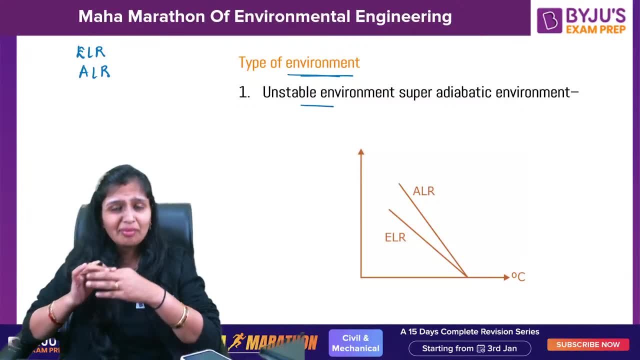 should know that. you should know both of them. First one is environmental lapse state and the other one is adiabatic lapse state. Is it happening now? Is it happening now? also, O3 is secondary. O3 is secondary ozone. Is it buffering now? 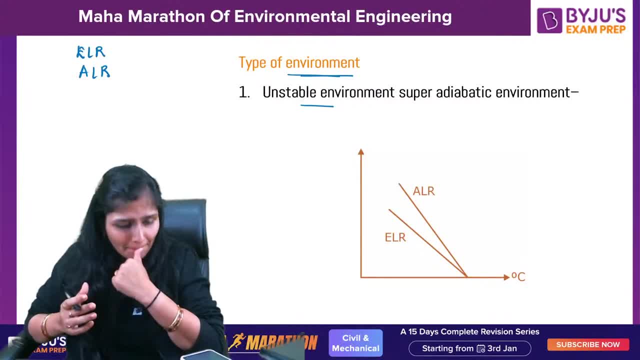 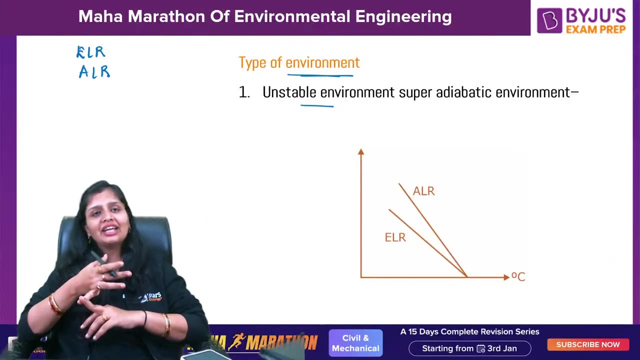 also guys: Yes, Okay, Okay, a good connection, I have checked it out also. just check it out once: is it happening now also, Alec, okay. so first is ELR, environmental lapse rate- what happens? environment means the surrounding area. you talk about only troposphere. troposphere is situated. this is the earth and this is the 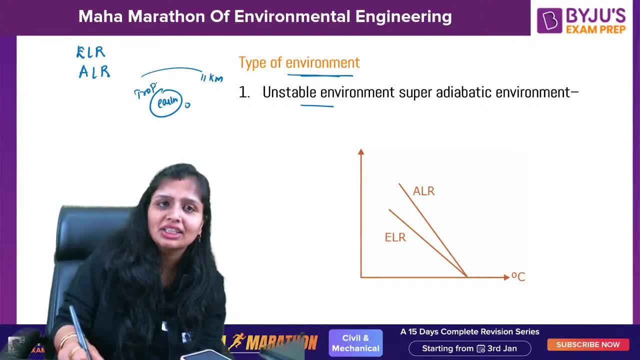 troposphere layer to 11 kilometers and we will all the discussion, which I'll be doing it. I'll that. I'll be talking only about troposphere. temperature of air decreases with increase in height. that is known as what environmental lapse rate. how can you know? take a balloon, okay, insert a thermometer is there and a 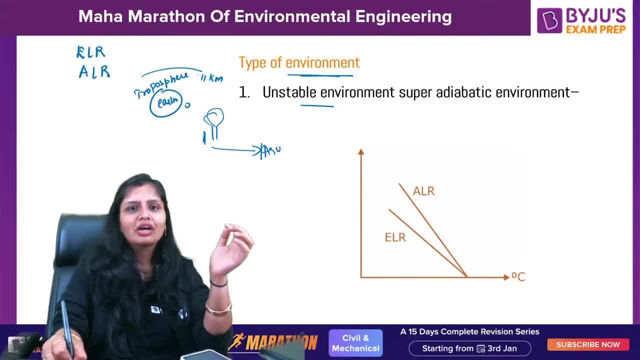 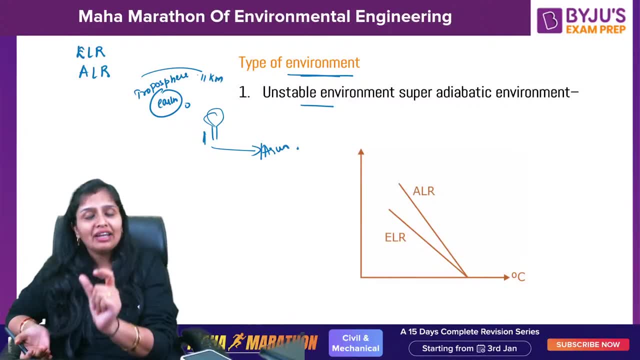 recording mechanism is there and Arun is standing here. Arun is standing here, so the rate it means it does not transfer it heat environmental lapse rate. you use it for the surrounding area. adiabatic lapse rate is for the air parcel or you can say for the polluted. 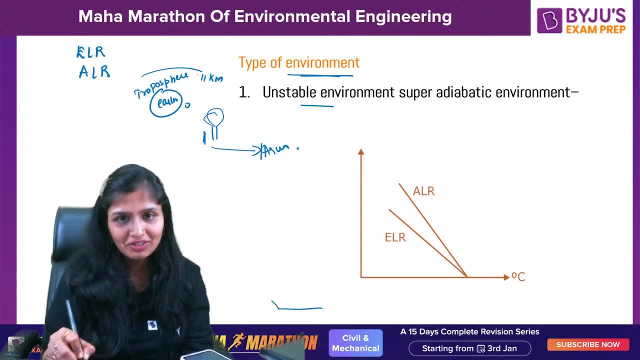 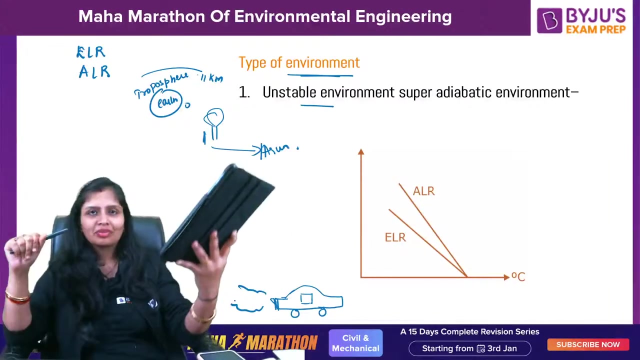 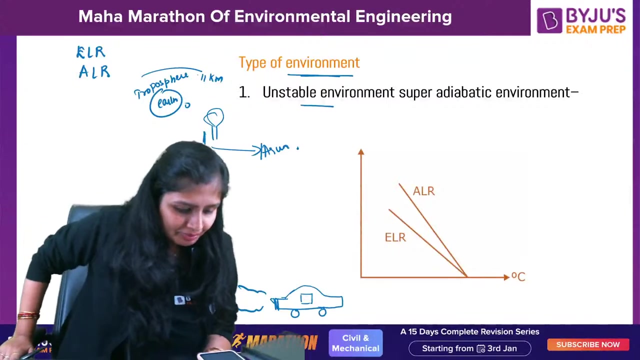 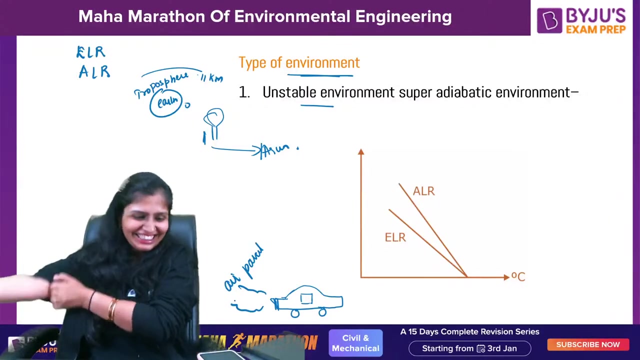 now I'll make a car. this is my car. nobody will laugh. yeah, it's a boat, this is my car. this is my car. bafringa pring- okay now. tangerine- now is it okay? let us check you. do you gear a khara book? okay, if I, you make it okay. 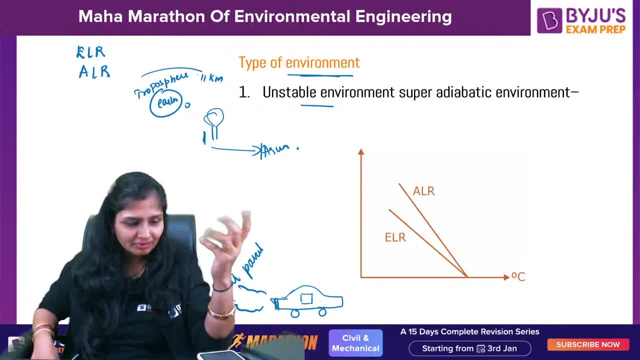 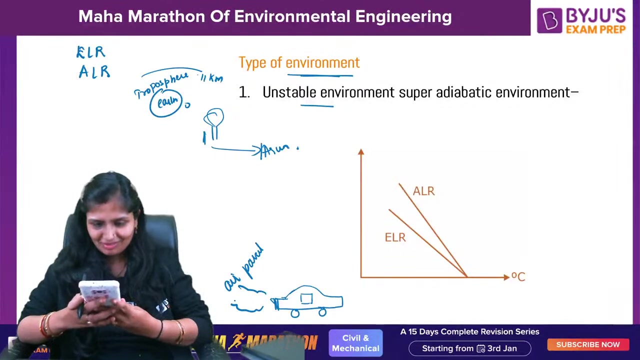 so now what happens? abhooga Tobata, no, hey, our Shaolin abhis make is key. heure to ho ja the time api technical glitch. okay, not, okay, yeah, yes, just a minute, though. nothing is okay, everything. arish allen, you are a bit little bit frustrated. nothing will happen, wait. 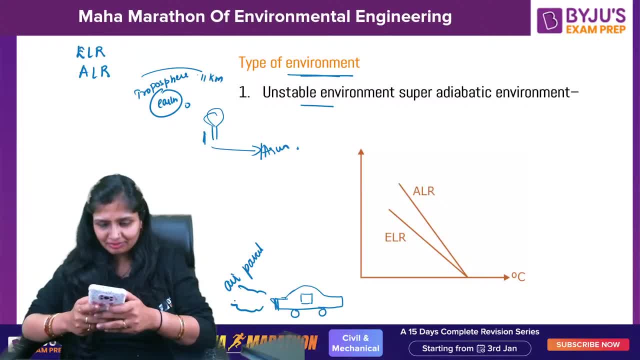 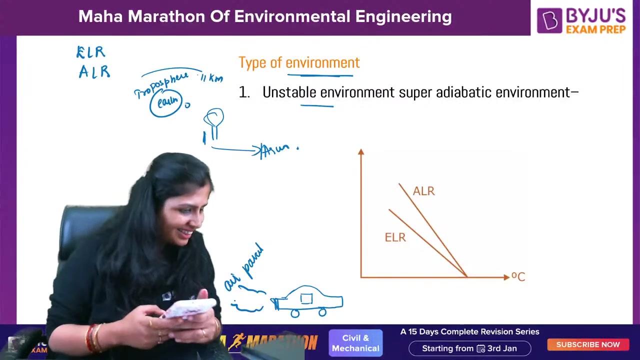 just let me check it out why it is happening. i lost the technical team just a minute wait. 20 minute topic is left and this is the last one i have to follow. is it still happening or not? is it still happening really? yeah, yeah, yeah, yeah, yeah. 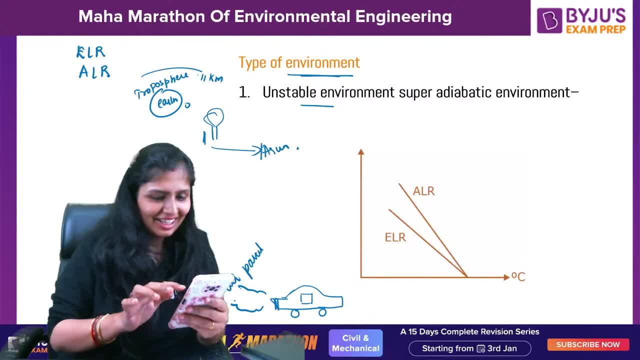 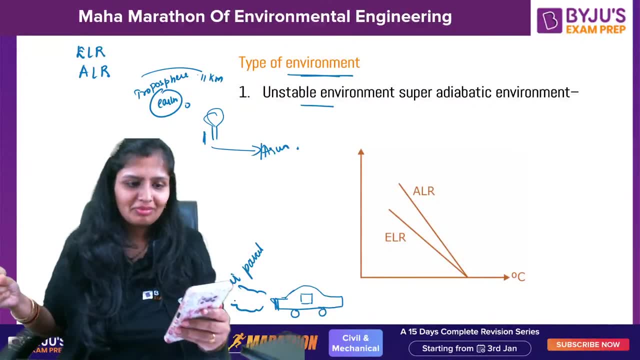 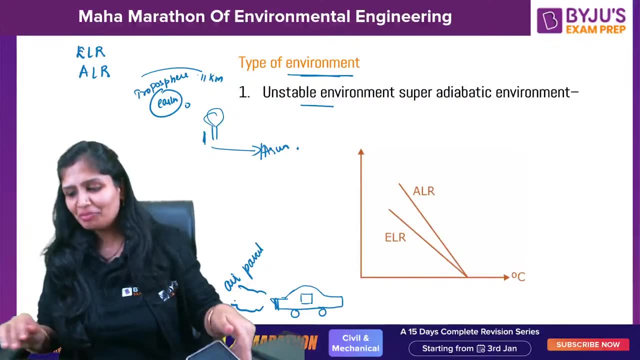 so unlimited, so unlimited, so unlimited. now also it is happening, or what? just check it out. ruko zara, sabar karo, kone mula theek nahi hoga, kone mula theek nahi hoga, kone mula theek nahi hoga. 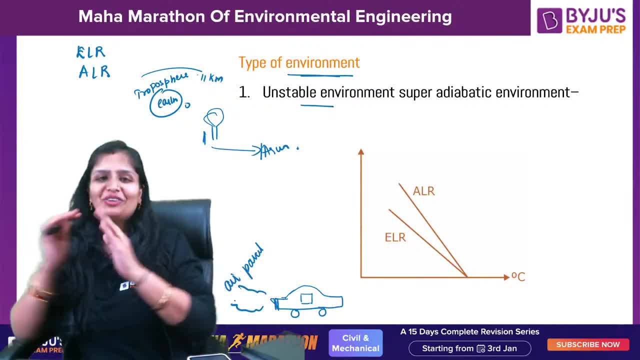 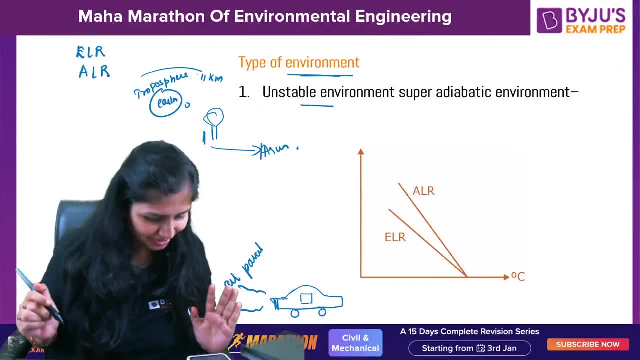 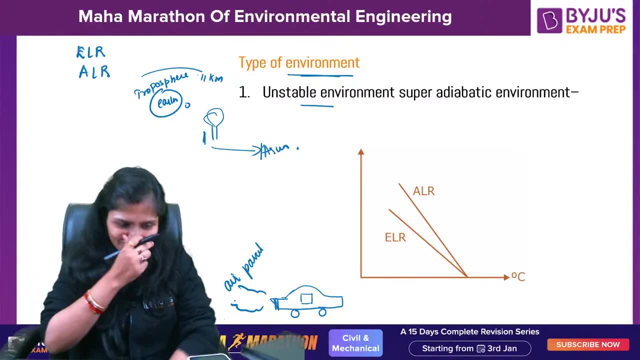 is it oka? is it okay? thik ho gaya. hey, youtube thik kardiya chalo. let's see, ek ghante tak bas thik rahe jaay ab jab padhare ho, toh tabi, tabi hota kone hai vos sathru. 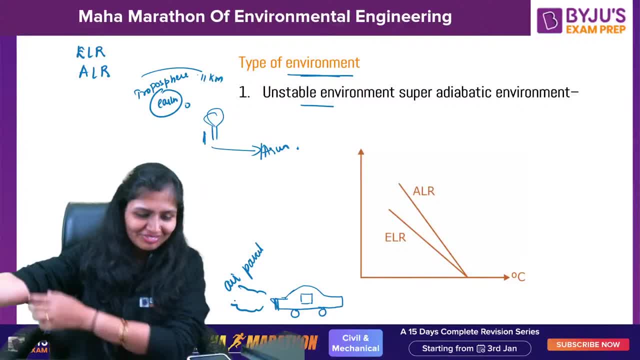 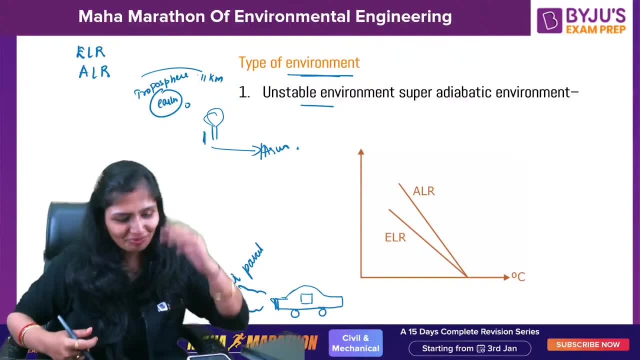 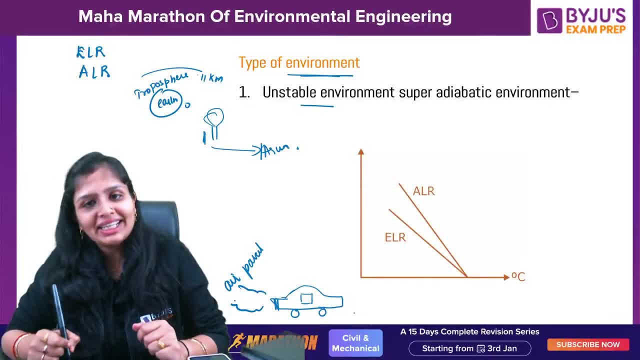 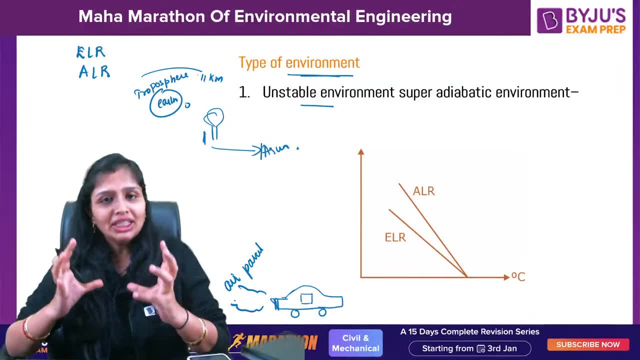 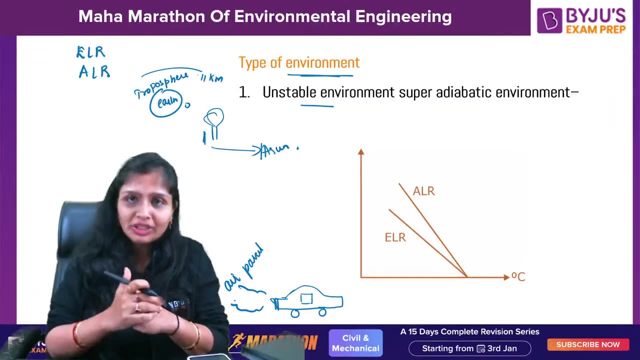 chalo, chalo. so what happens here is basically: this is a car and the pollutants are released. the air parcel is there, that is the pollutant. so this air parcel, when it goes, when the height increases, the air parcels temperature also decreases. the rate at which the rate at which the temperature of 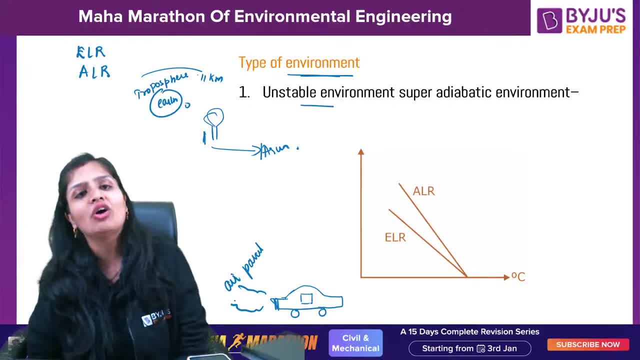 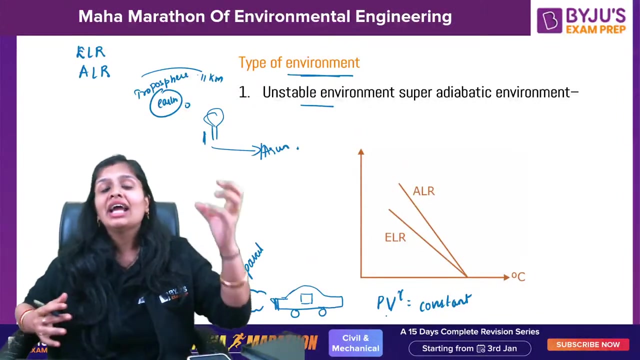 pollutant also decreases with increase in altitude. that is known as adiabatic lapse rate. you guys would have studied in your chemistry. pv gamma is constant. okay, so what happens here? it is not exchanging, it heats, but as the air parcel goes up it tries to expand, and if volume has to expand it will use its internal energy. if it will use its internal 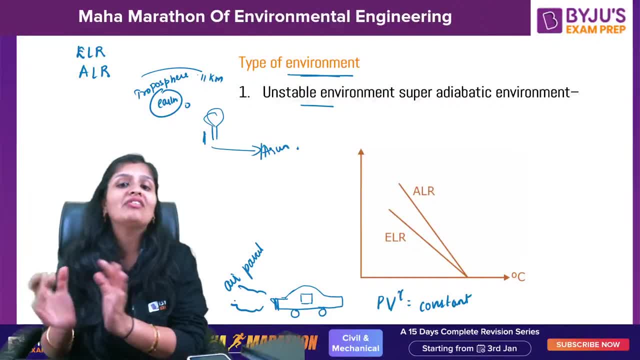 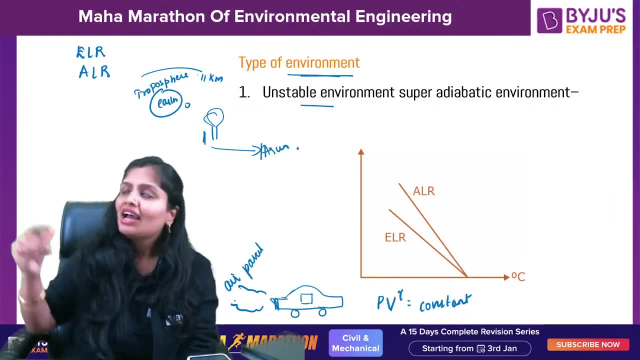 energy volume is expanding, pv to the power gamma is constant. pressure has to reduce. pressure is directly proportional to temperature, so temperature will also reduce a prashant. i said that there is a parcel of air. the pollutant is there. when you go up this pollutant or her temperature. 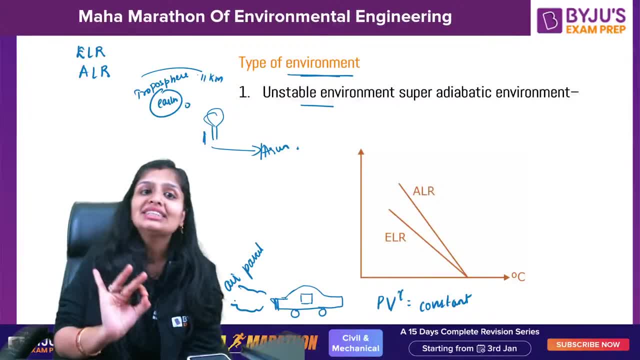 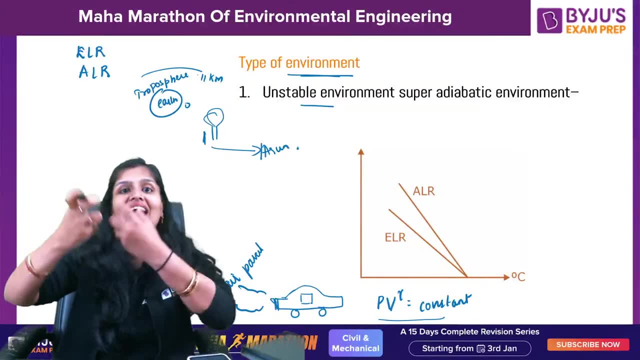 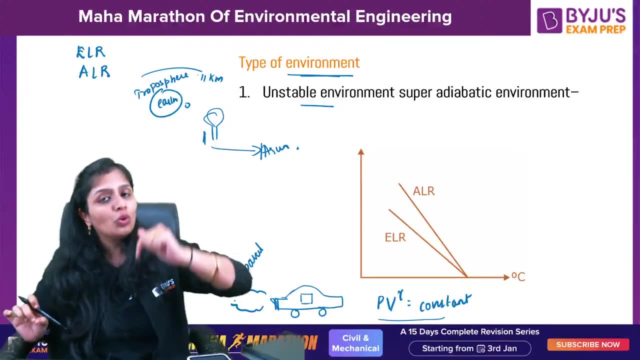 also decreases with increase in altitude. this is an adiabatic process. that means pv to the power. gamma is constant. as the pollutant goes up, it tries to expand. the volume increases. how can it increase its volume? by using its own internal energy. the pressure will decrease and you know the formula: pv is equal to nrt. so if the pressure 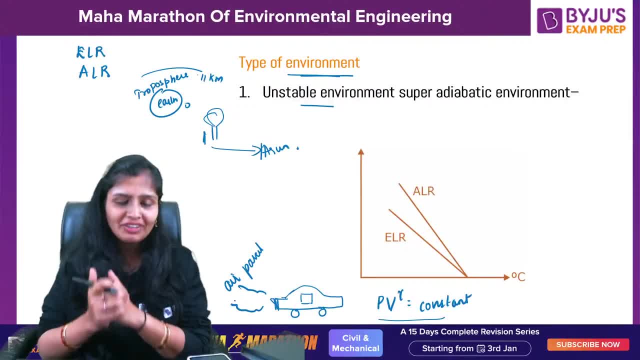 is decreasing, the temperature is decreasing, so what we say is that? so what we say is that that the both the surrounding air and the polluted temperature decreases with increase in altitude. when it decreases for surrounding air, it is environmental relapse rate. when it decreases for air parcel, that is adiabatic love. 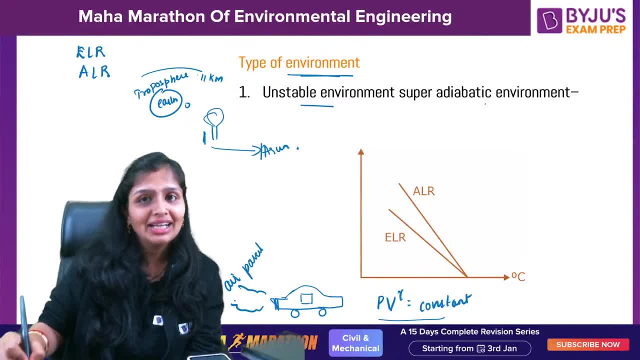 Well, today I have learnt some kind of know- not simple problems- that we see inmeal sympathy balance. so here we will deal with all of these problems in a series of series of previous lectures. then I have tried them out selbst. after say many problems, read them again and write down, and please use these questions for the end of this video. 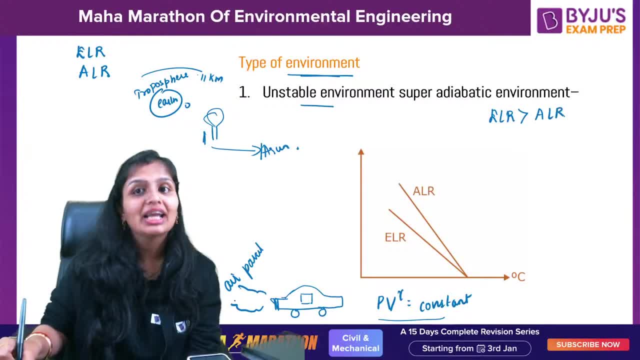 let's re-last complete our computations. when it decreases for the surrounding air, it is environmental relapse rate. when it decreases chor air parcel, that is Ad di mir dec lapse rate. now, unstable environment is this where environmental lapse rate is more than the adiabatic lapse rate. why you? 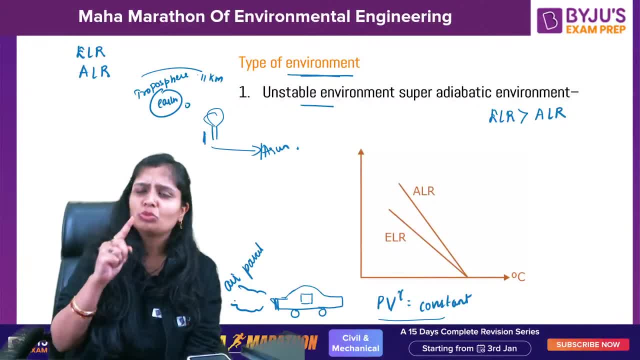 call it unstable. parting say anb to asset price, so it is above the cost to the dt. começar a gelernt short at the place, something like this. why you call it unstable? я Lapse rate is more. That means for both air and pollutant. the temperature is decreasing. 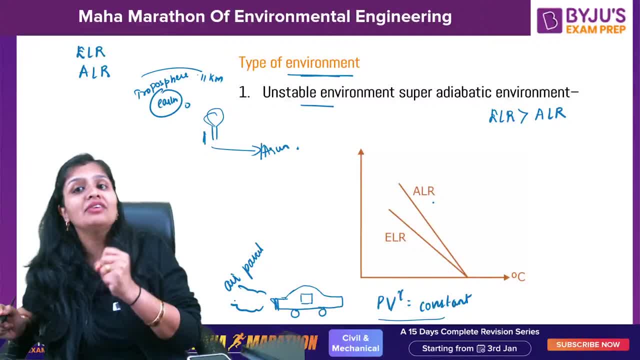 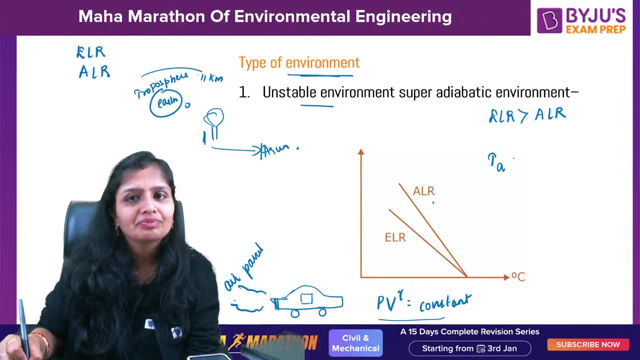 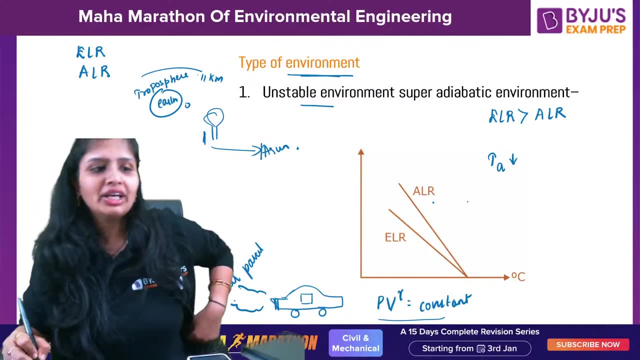 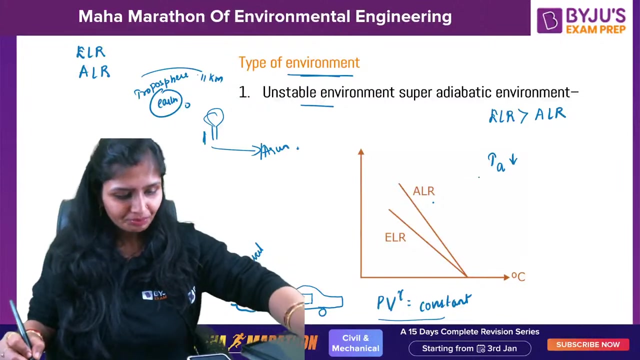 But the temperature is decreasing more rapidly for environmental lapse rate. So temperature is less, Temperature of air is less, Temperature is less, So density will be what Density will be? what More or less? I want to drink it all: Garam, hawa, warm air. 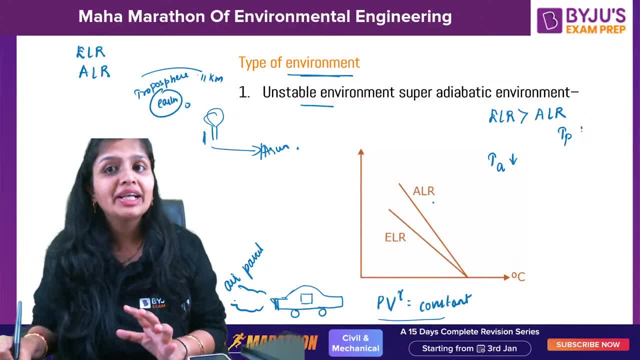 Which is warmer. Pollutant is warmer. Pollutant temperature is more Jiska temperature: zyada. More the temperature. it is lesser in weight. Garam hawa halki hoti hai. Okay, So the density of it will be less. 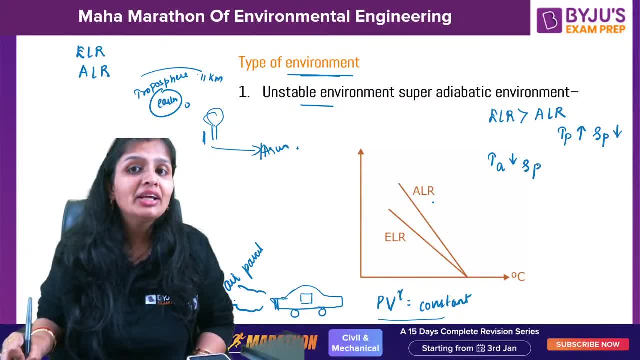 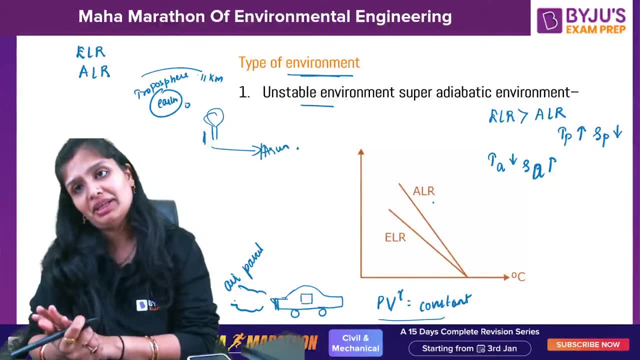 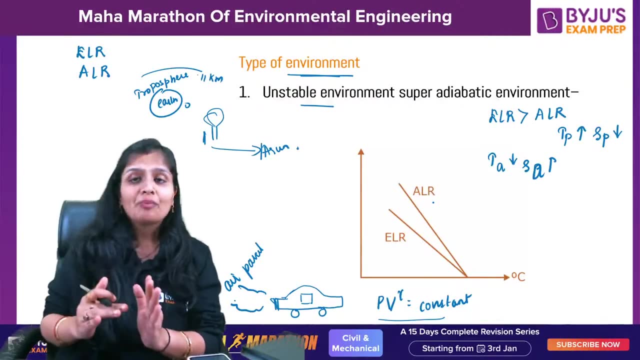 The temperature of air is less, The density will be more. So what will be happening in this case? Rapid mixing of pollutants will take place. Rapid mixing of pollutants will take place, So it creates an unstable environment. Now, since ELR is more than ALR, 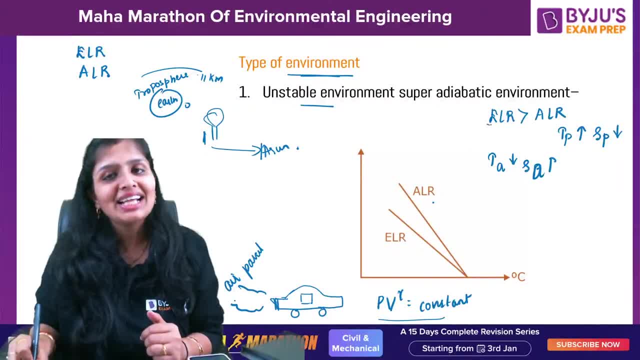 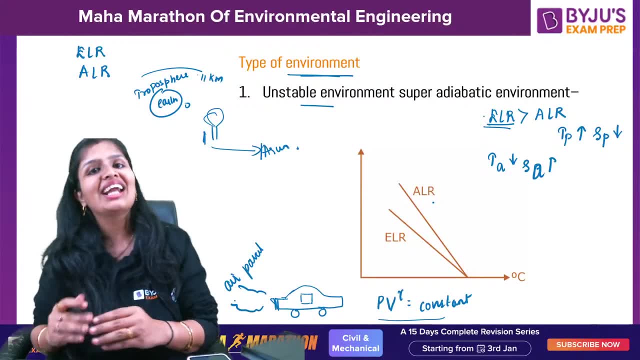 So it is like super se upar. So that's why in place of ELR you call it as super adiabatic lapse rate also. So in some books instead of ALR they write it as SALR, So it is trying to say super adiabatic lapse rate. 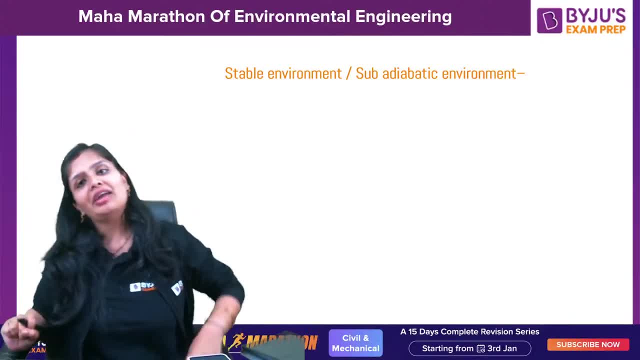 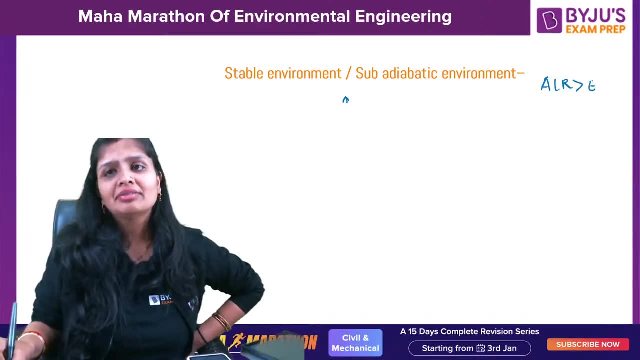 Okay, While in the case of stable environment, or you call it sub adiabatic environment, Why? Because in this case, ALR is more than ELR, ALR, ELR, See here the height is there, Here temperature is there. 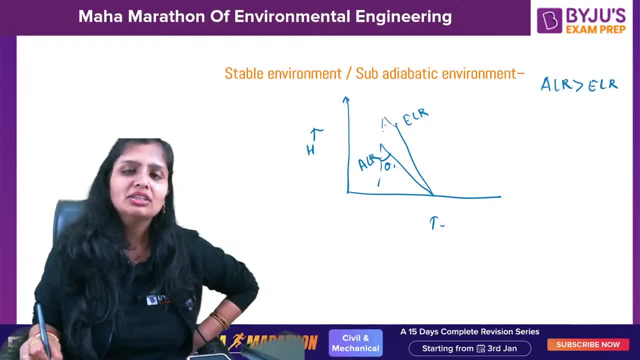 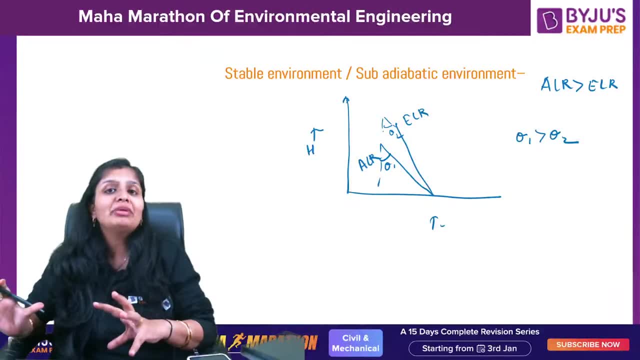 So if you calculate the slope here, theta 1, and you calculate the slope here, theta 2. You will see that theta 1 will be more than theta 2.. So what will be happening? Both temperature will be decreasing, But the temperature will be decreasing rapidly in the case of adiabatic lapse rate. 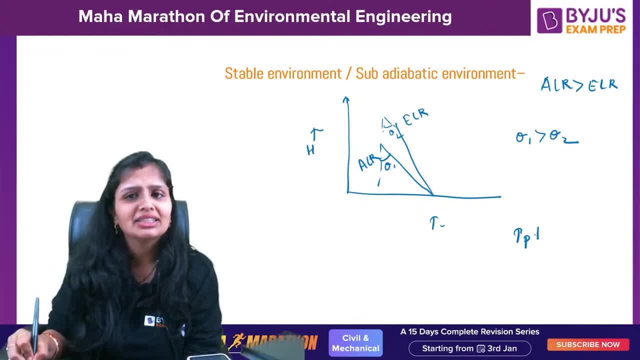 If temperature of pollutant is less, So the density will be more And the temperature of air will be less. So what will happen here? A stable environment will be there. A stable environment will be there. There will be no mixing which will be induced here. 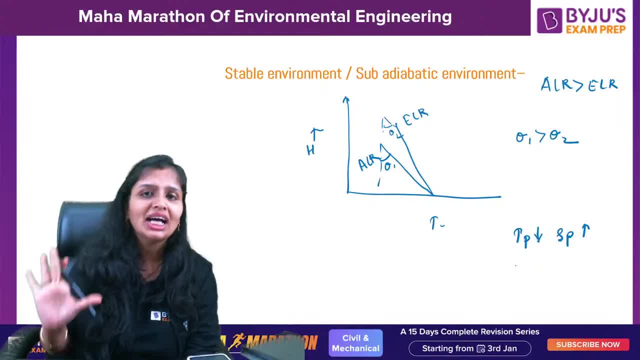 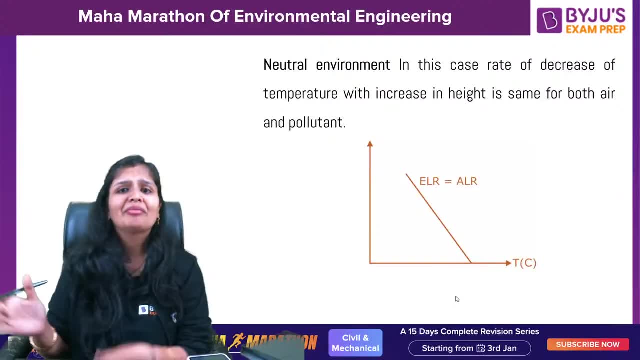 Okay, So this is the stable environment, or you can say the sub adiabatic environment, which you will get it Now talking further, neutral environment. Both are decreasing. The rate is same. ELR is equal to ALR. That is known as what? 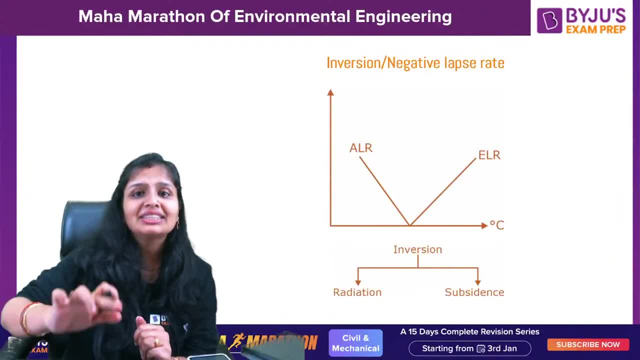 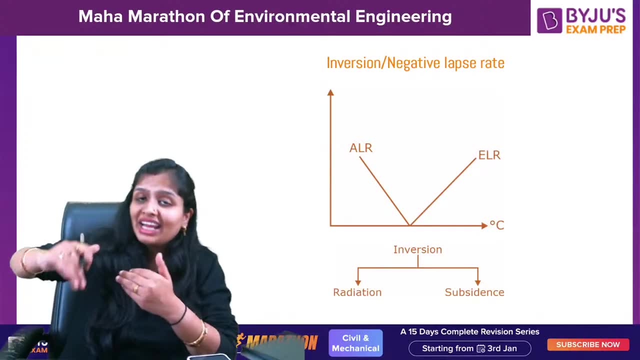 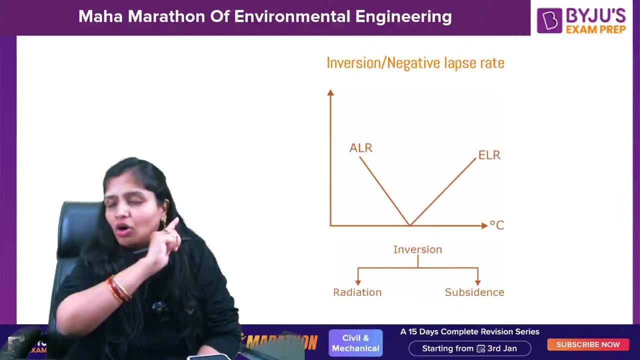 Neutral environment. Coming further is inversion. Inversion means till now we were saying decrease as positive, Decrease was termed as positive. Now, if increasing is taking place, you will call it as negative. So, ALR, remember: pollutant's temperature will always decrease with increase in altitude. 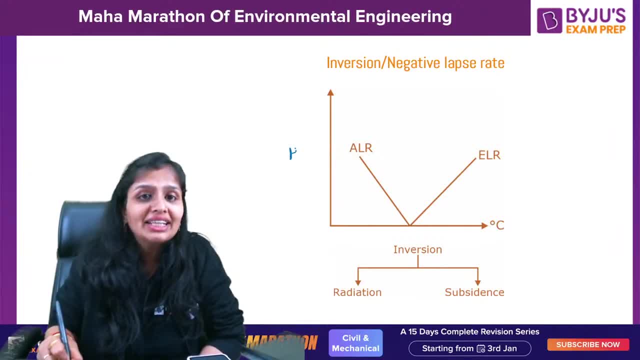 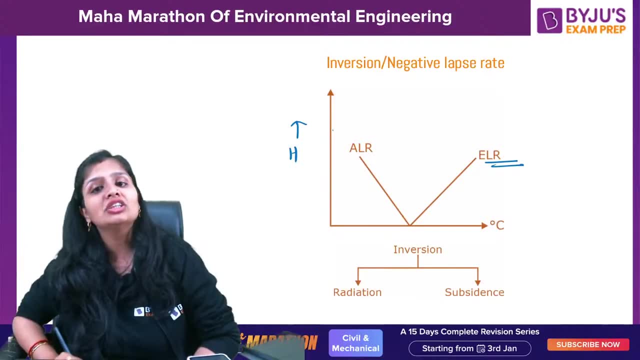 But if the surrounding air temperature increases with increase in altitude, you call it as inversion or you call it as negative lapse rate. Now, inversion is of two types: Radiation inversion, subsidence inversion. Radiation inversion: you call it as surface inversion also because you see it on the surface. 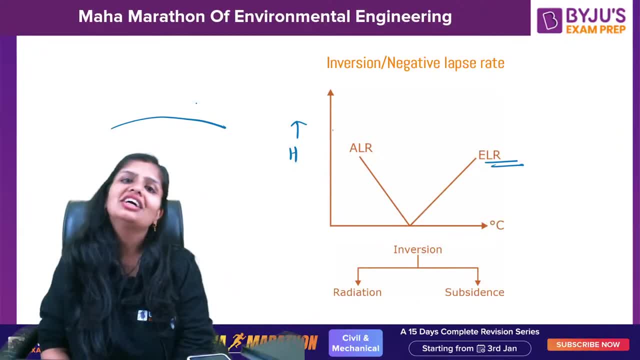 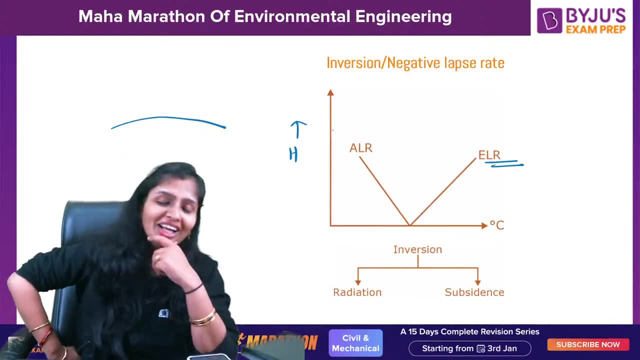 Like you heard that song right: Rata lambi yaa lambi yaa re. So that is for radiation inversion. Tell me I don't sing well, but listen a little. Why Rata lambi ungi. 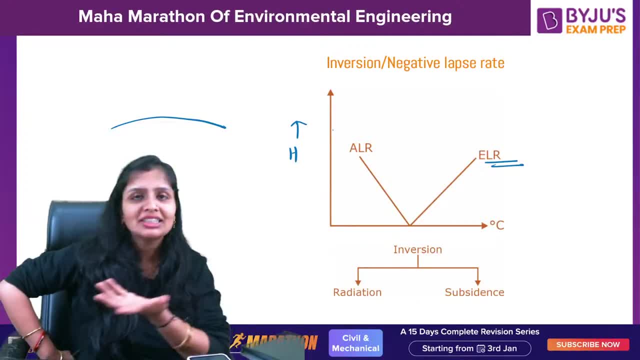 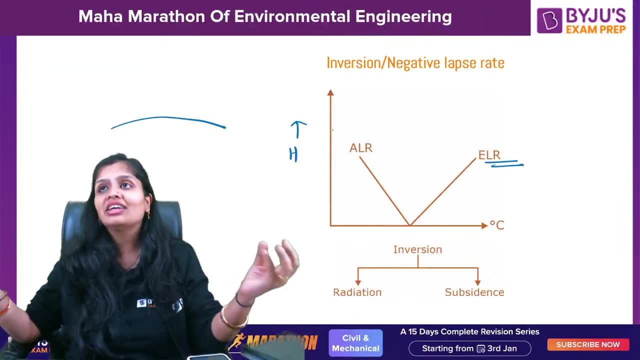 Sardiya Winter nights: rata lambi ho jati hai na 7 pm. you see, you see darkness. 6 pm, 5 pm. So what is there? Darkness is there. Darkness is there, Winter season is there. 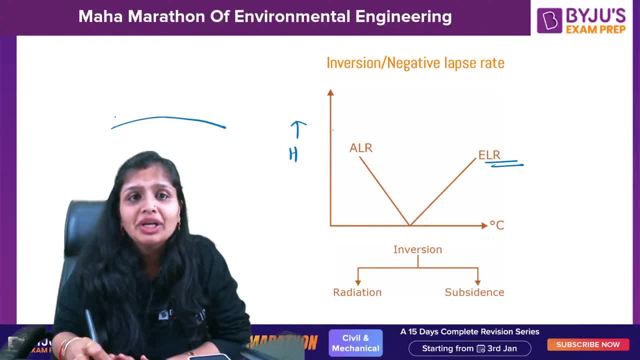 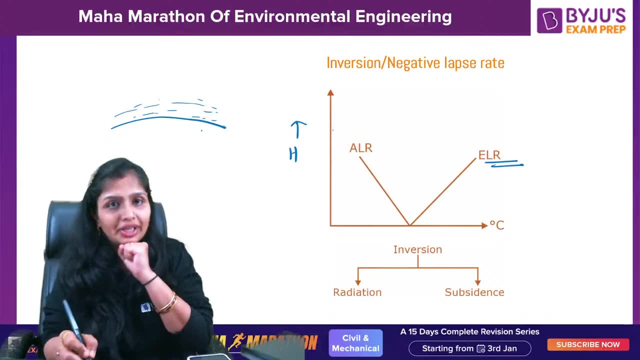 So what happens is the surface near to it. you will see: yahaan pe thandi hawa jati hai Thik hai Land thanda ho jata aur surrounding to it, you will get a colder air, As compared to here, where you get warmer air. 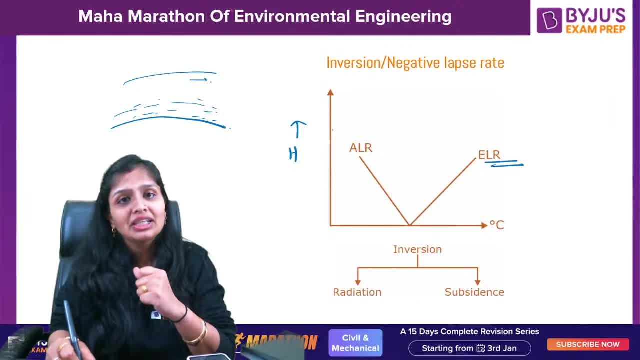 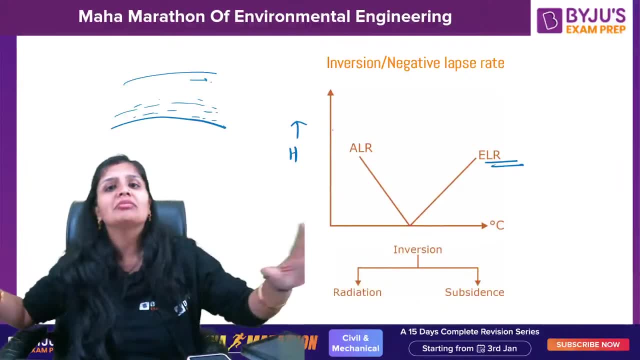 So that is the reason. that is the reason what happens here In radiation inversion. it will happen when long winter nights are there. Jaise subha hogi khattam Tata, bye, bye, goodbye. Radiation inversion gone. 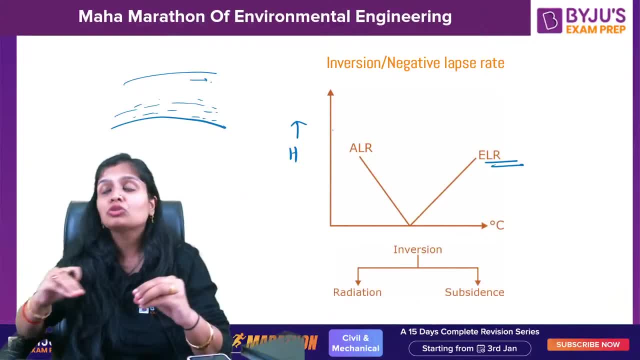 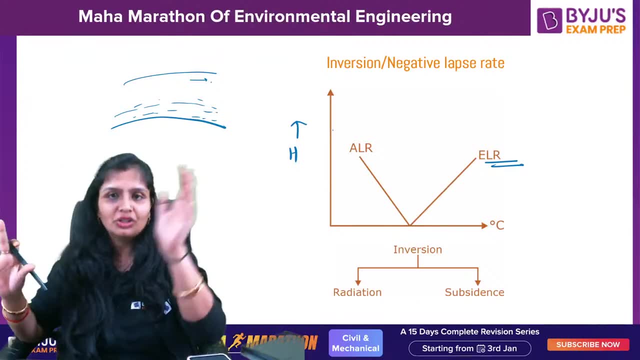 So it happens on long winter nights. Agar aap isko, if you want to see it on prominent basis, toh, then you will see it in the case of, for polar regions, and all You can say this radiation inversion. 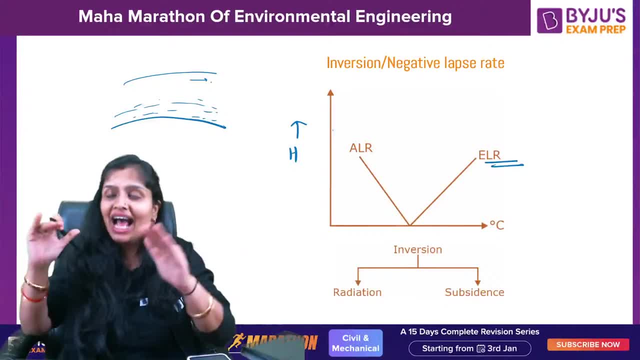 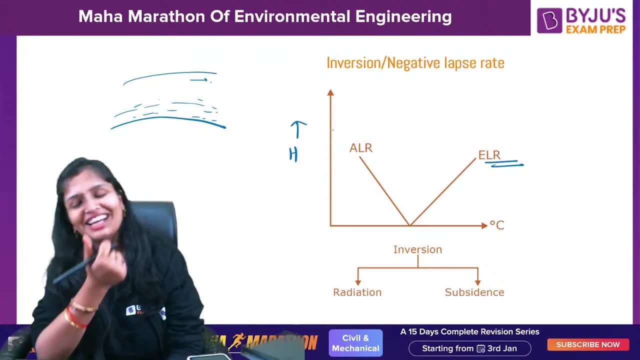 So near to the ground you will see that the temperature is less as compared to the temperature present above it. Raat baaki, Das ji ko bahut gaane ban raha hai. Mere saath melody khel raha hai. 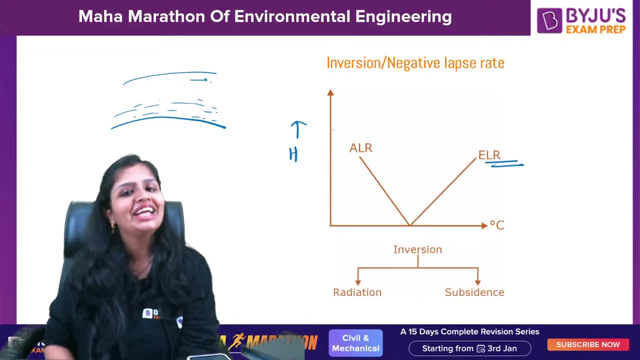 Chalo ek din bette hai. So this is the radiation inversion. Okay, Why? Because as we go up, the temperature is increasing. Okay, Subsidence inversion: this you don't get it in the surface. What happens? 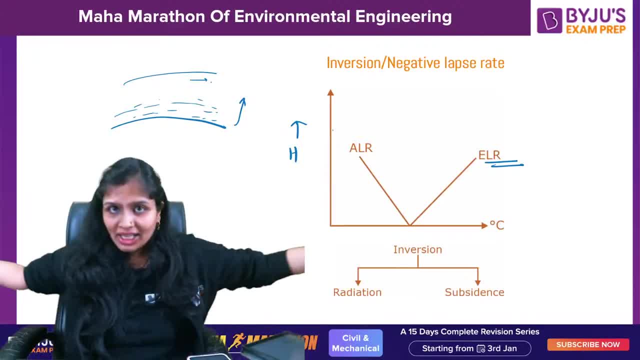 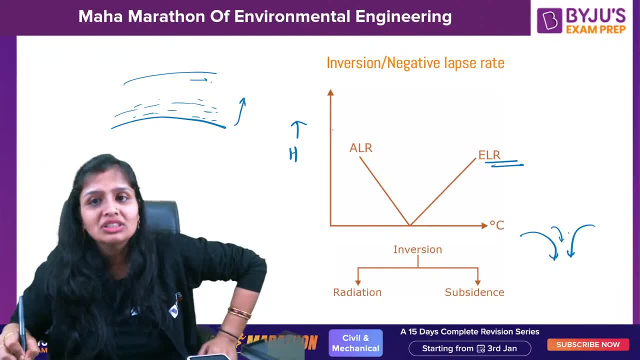 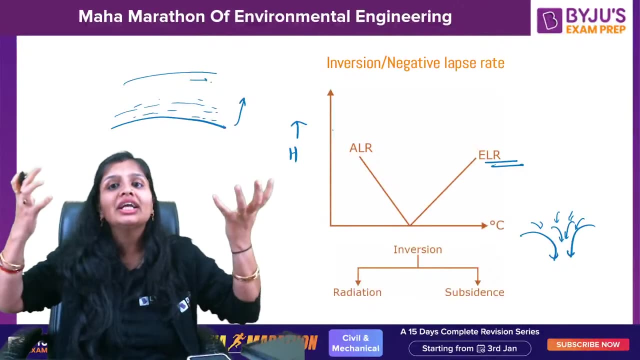 Due to cyclones and all what will happen? The wind subsides, The wind subsides. Okay So the wind, what does? it goes, It goes, subsidence, It goes, subsidence. So what? you will see that, as you go up, the temperature increases. 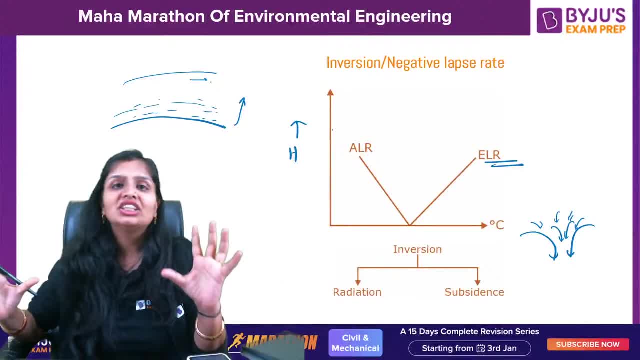 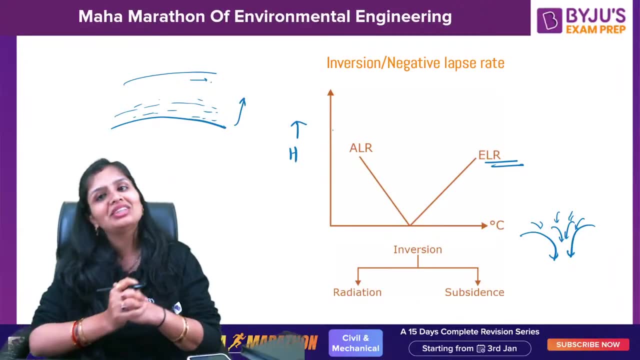 So that is subsidence inversion. Generally it happens in the case of cyclonic conditions and all Okay. So this happens in those conditions: Radiation inversion. you will see it near the surface, As I told you, right now you will be seeing radiation inversion. 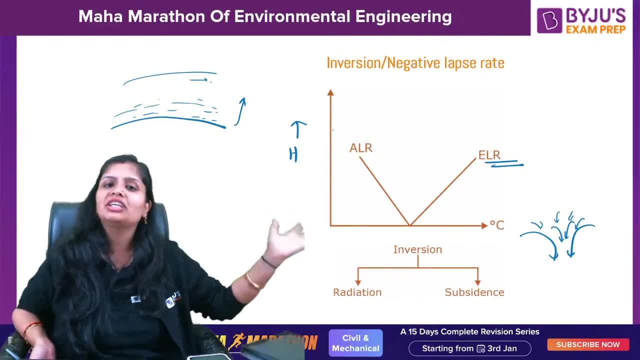 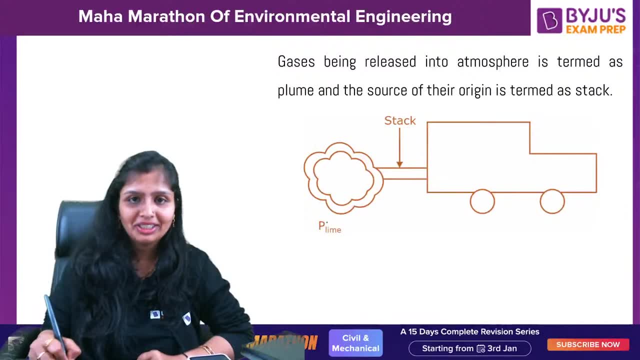 Subsidence inversion during the case when air moves from high pressure to low pressure, Then you will see subsidence inversion. Okay, Now see how good car I have made. Typist will say I have made it. Ma'am is taking credit. 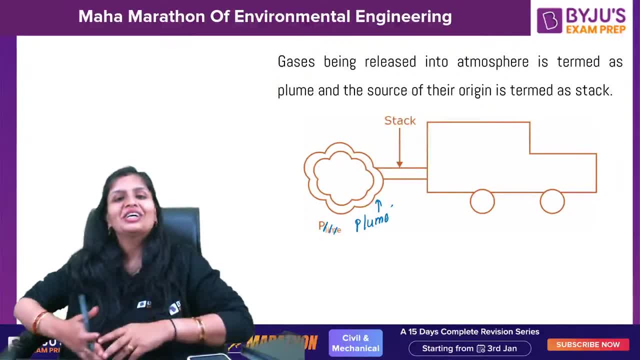 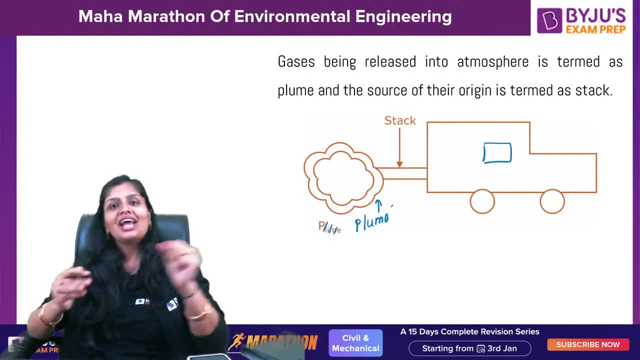 Okay, Thank you, Arun. Okay, So what happens here? This is a car which you can see it. You will say, ma'am, I am not seeing less than a bullock cart. It is a car. So what is happening? 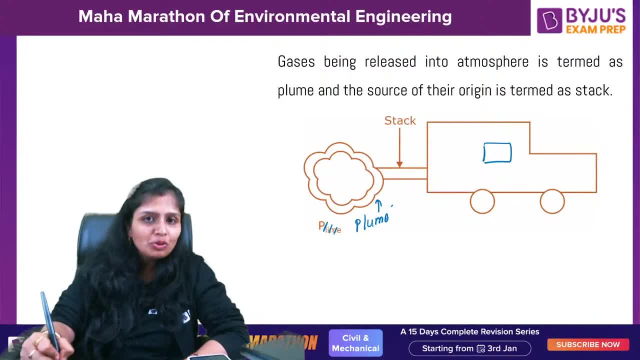 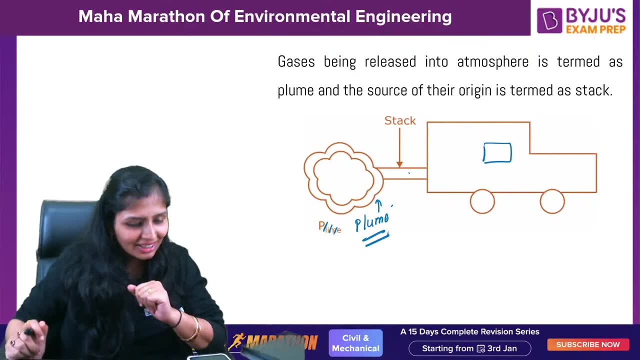 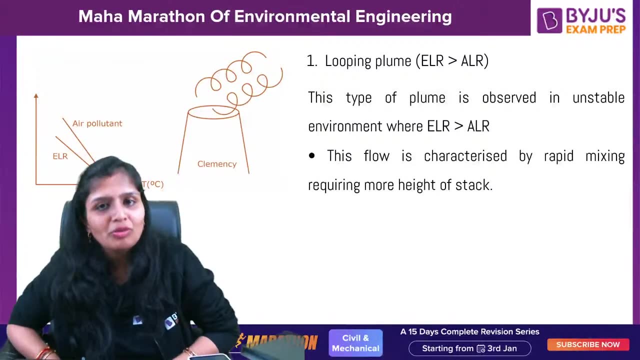 The gas which is released, it is known as plume And the source of their origin is known as stack, Because right now, right now, we will be studying about plume behavior. So first, is the looping plume Highly unstable. 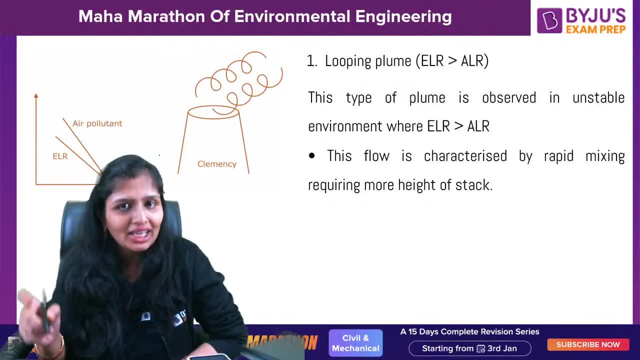 Highly unstable, because here ELR is more than ALR, ALR. Here what will happen? as I told you, rapid mixing will take place, So if anybody is living near to it, the water from the chimney will go to their houses. 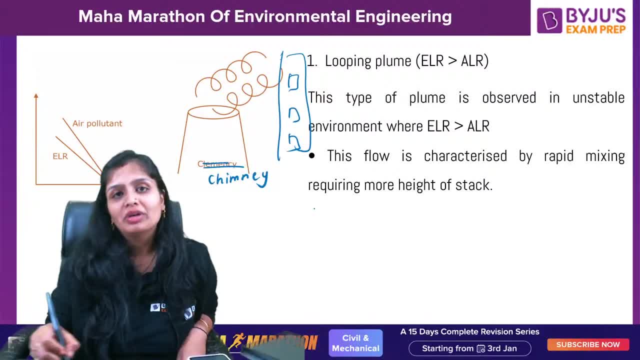 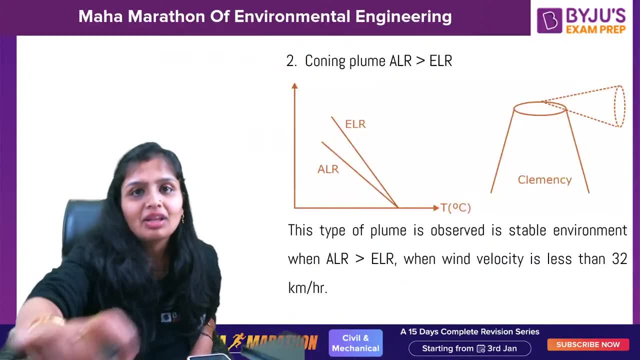 Okay, So this is what. This is what Looping plume. See, these loops are formed, So that's why its name is looping plume. Okay, Coning plume When the wind velocity it depends upon the wind velocity. 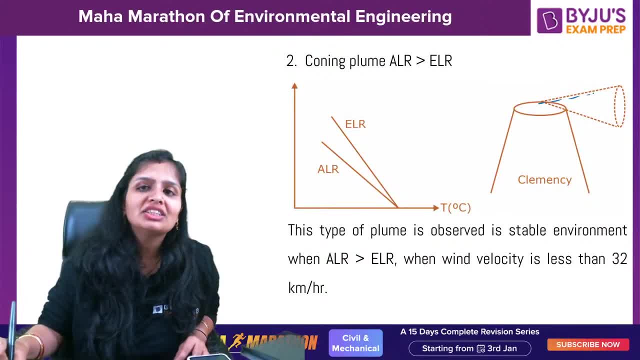 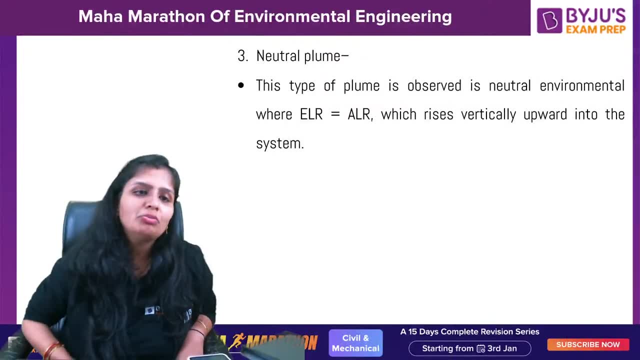 Here. this is a stable environment. The plume which is generated: it is in the air. Okay, The shape of cone, So you can see this is a coning plume. Next talking about is the neutral plume. 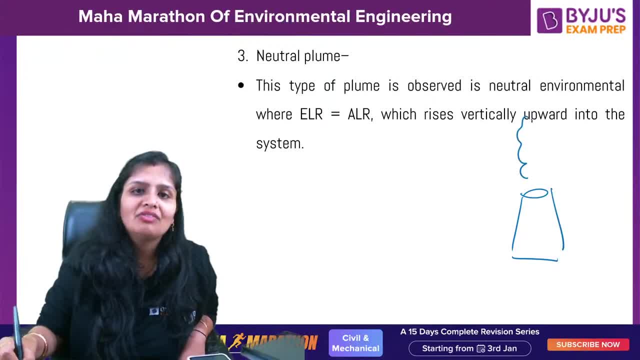 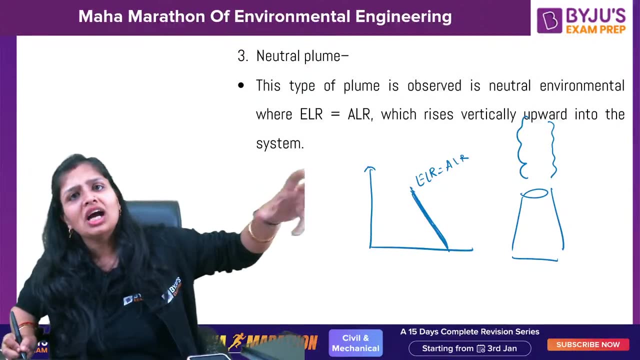 Neutral plume. what will happen? ELR is equal to ALR. Vertical upward movement will take place, Simple See. one time question has been asked in gate examination regarding mass. the following: Now, what they can give you right now is like they can tell you: vertical upward mixing takes place. 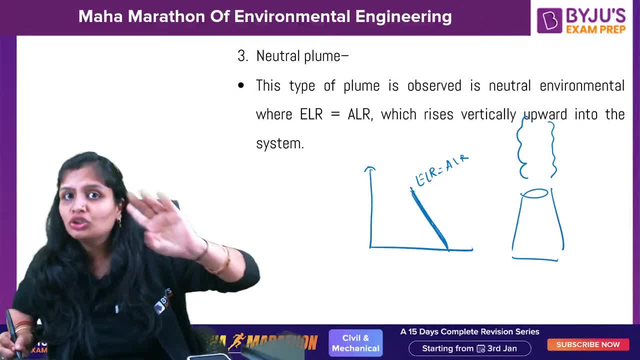 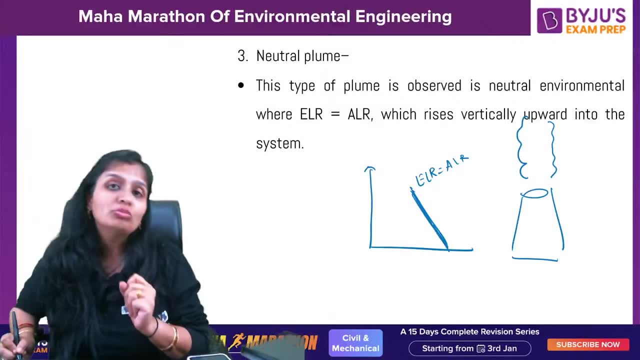 Identify the type of plume And they will give you four options. So you should be able to tell That which is the correct option. Okay, So that's why the features of that plume also you should. Next coming is the fanning plume. 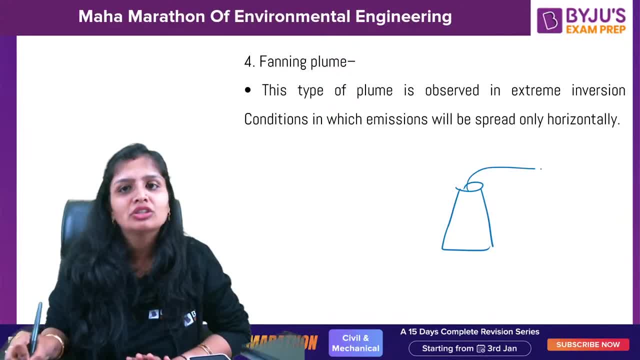 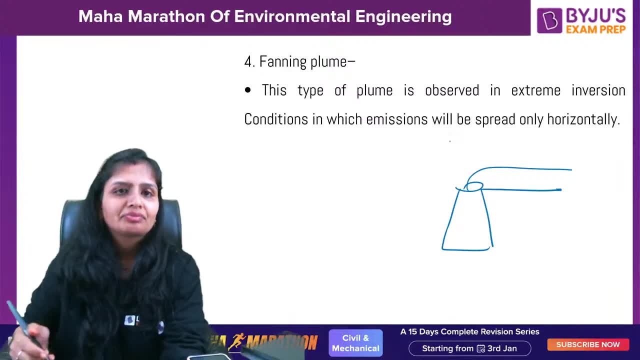 Fanning plume. I can understand from the name It will spread horizontally. How it will happen, How fanning plume will function: Fanning- See ALR always decreases. ALR will always decrease and always decrease. But here inversion. 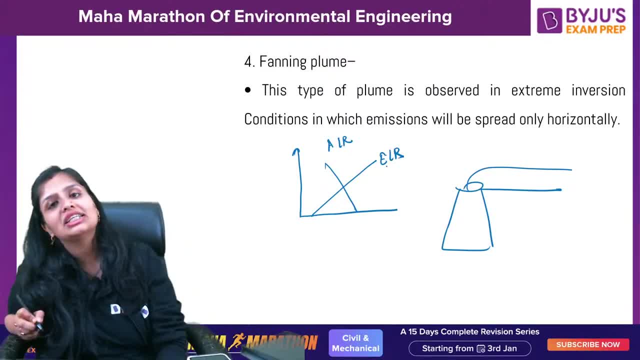 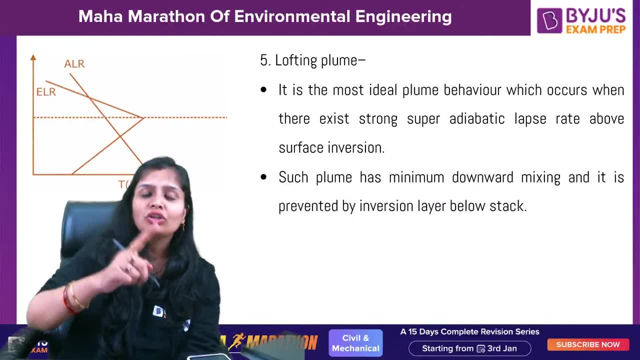 Condition will take place. ELR. This is what This is. fanning plume- Fan Horizontal- Okay. Next, coming to lofting plume. Out of all the types of plume, the best is lofting, The worst is fumigating. 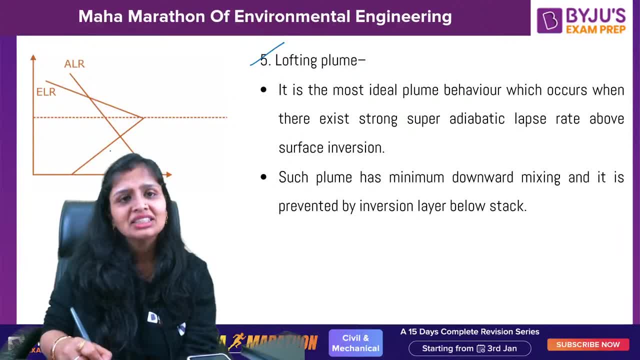 Lofting plume. So see it here. First surface inversion is taking place or afterwards. surface inversion is taking place First, First inversion, Then ELR is greater than ALR. So here it is inversion, Since it is taking place from the surface, this is surface inversion. 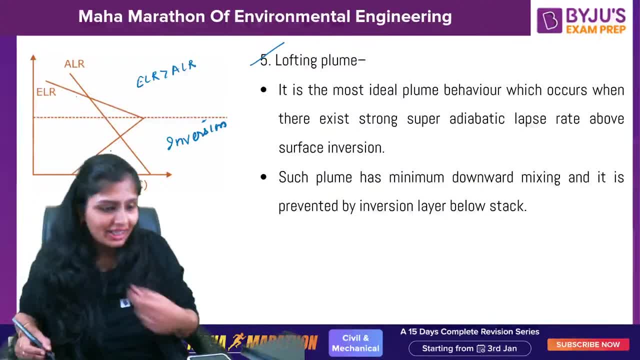 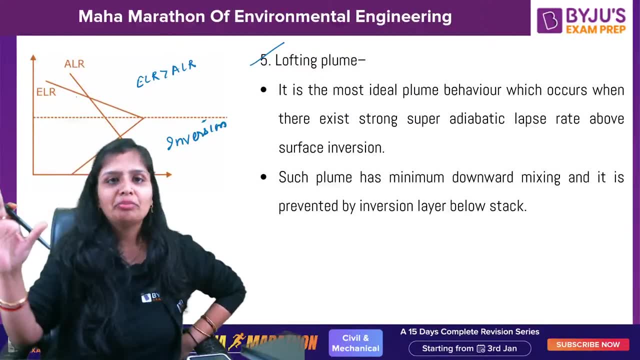 That long, long one. Okay, That one is not inversion. Okay, So this is surface inversion, or you call it as radiation inversion. Okay, This is the best. Pollutants are above. We earthlings don't have any problem. 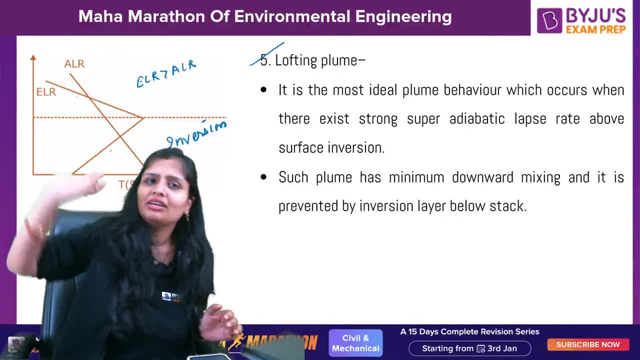 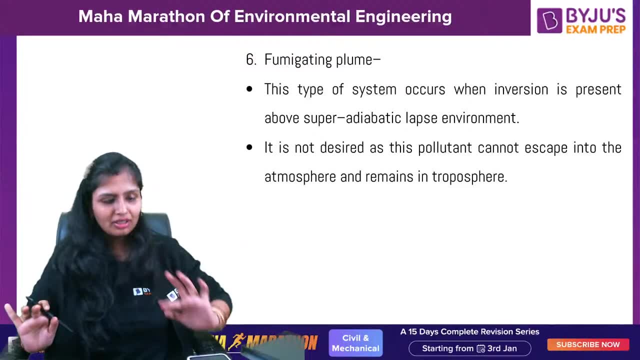 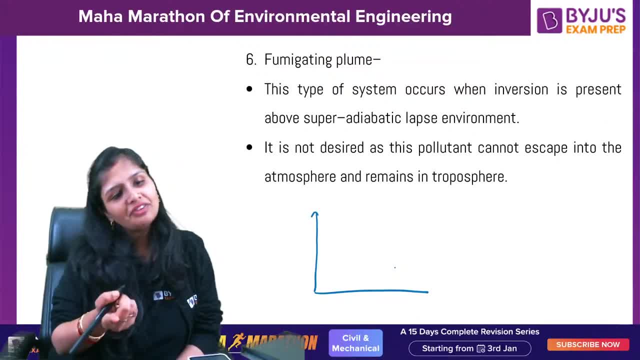 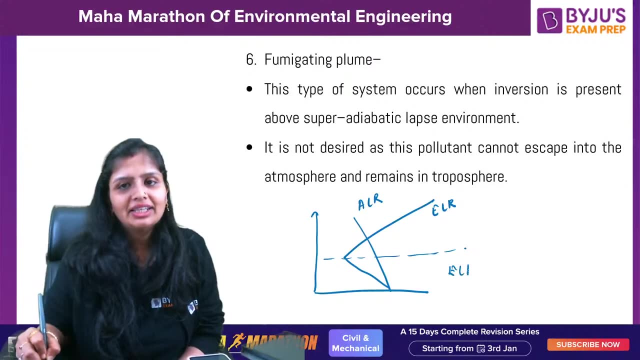 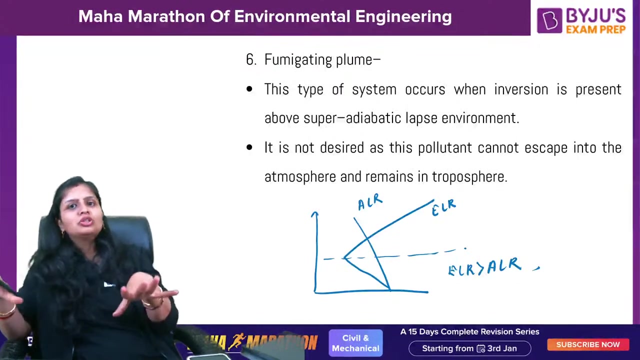 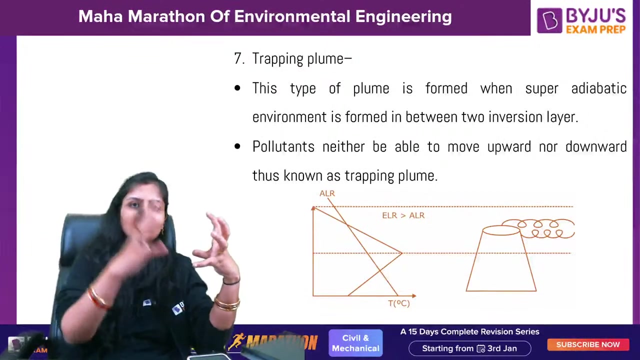 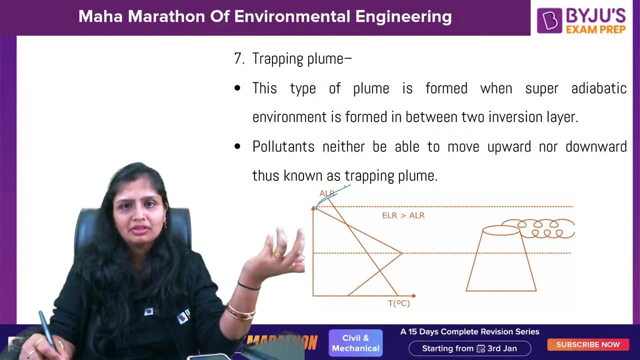 How it is opposite. Earlier surface inversion was happening. Let's keep ELR as it is. It will be in this later. Okay, Here ELR is greater than ALR. and then surface inversion- Okay, these pollutants will remain in the troposphere. it is a problem for us. how will we live? worst, lofting the best, fumigating the worst- okay. now, last is trapping: trapped, first surface inversion, afterwards surface inversion, so trapping is being done. there will be one more trapped, okay, so trapping is done. 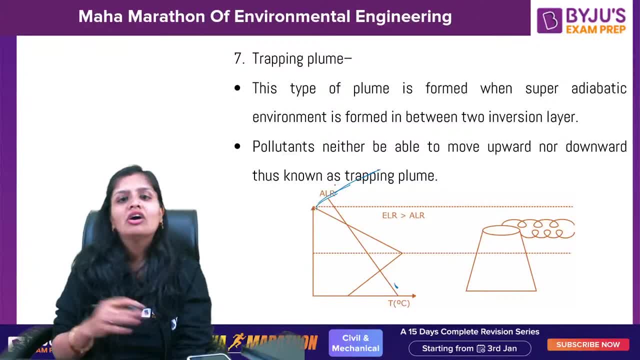 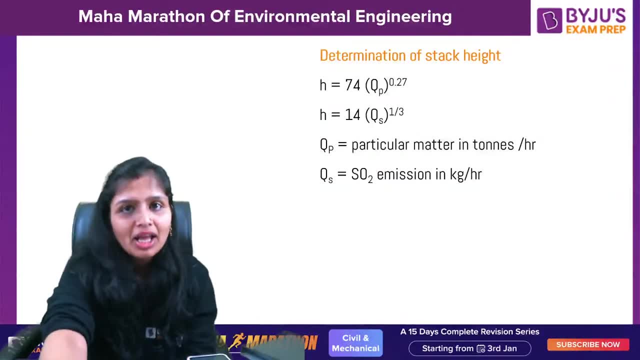 And this inversion earlier, also later also and in between, trapped super adiabatic condition. so this is the trapping, simple types of plumes are there. now let me tell you one thing: very simple questions are there. let me tell you one thing, ELR, there are two dry adiabatic lapse rate. one is dry adiabatic lapse rate and one is wet adiabatic lapse rate. 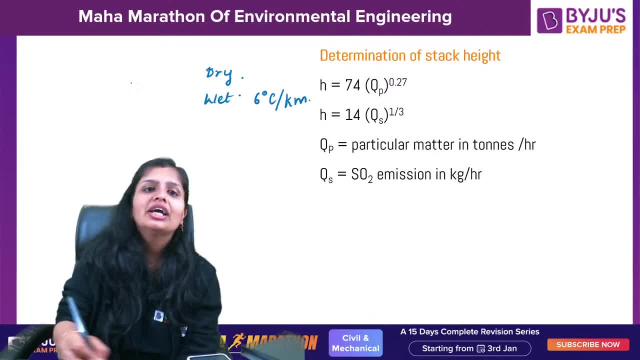 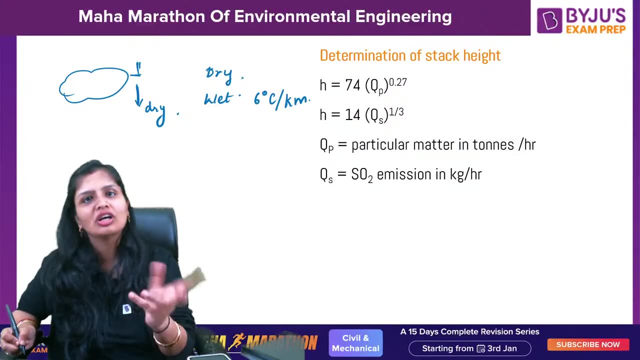 Wet is 6 degree Celsius per kilometer. When we say above the cloud level it is wet and below the cloud level it is dry, the rest is a lie, because below the cloud level, below the cloud level also, you get partial. it is not completely dry, it is not completely wet, it is partially saturated. but in the books it is written, it is followed, so we use it. 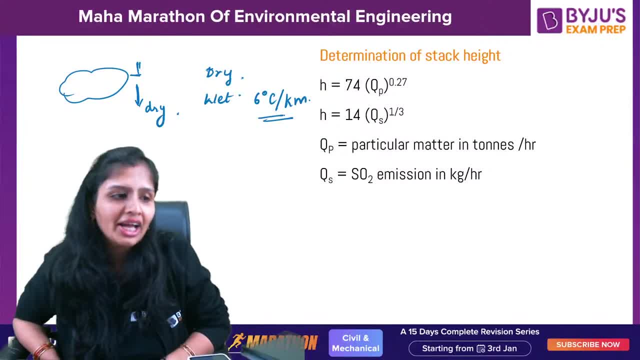 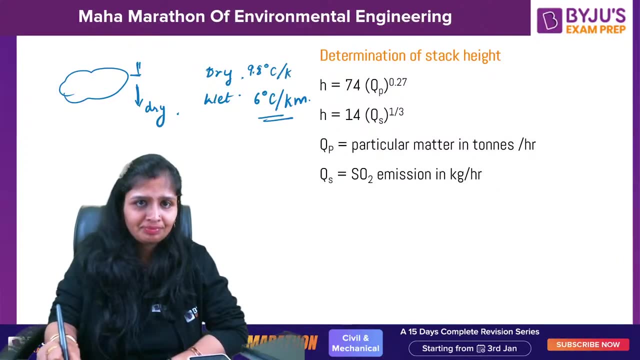 For wet, we use 6 degree Celsius per kilometer. for dry, what we use For dry, what we use, 9.8,. tell me for dry, what we use for dry. Del Paz, Dinesh, Girish, everybody. so simple questions have been asked. let us suppose ground temperature was 40 degree Celsius. okay, so what will be the temperature? what will be the temperature at a height of 0.5 kilometer? 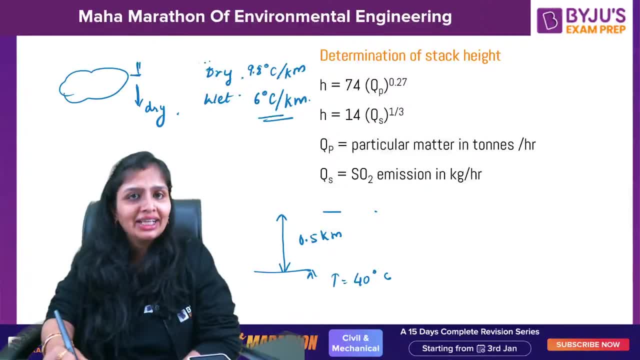 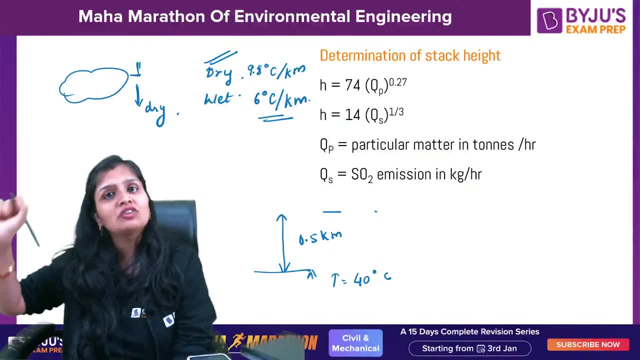 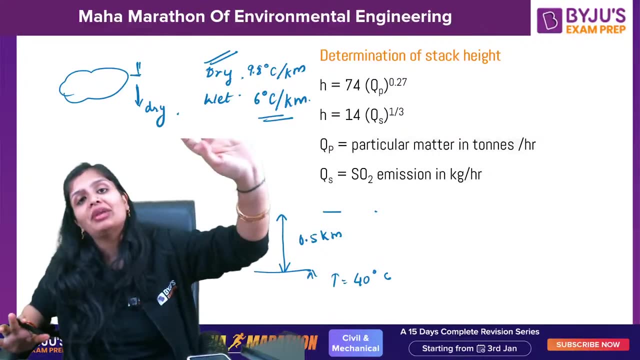 So if not anything, nothing is mentioned- take dry until and unless they mention wet adiabatic, then only take that, otherwise don't take. ELR value varies from place to place. I am living in Bhilai, Dinesh is living in Jalandhar, Dasji is living in Kolkata. everywhere what is happening, ELR will change, but ALR value will remain same. 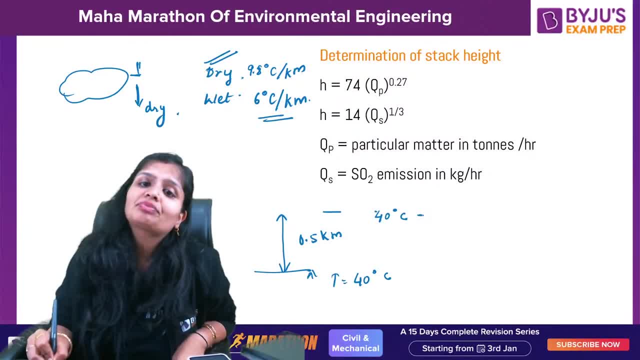 So 40 degree Celsius. let us suppose this is there and IFR is talking about ELR, so 9.8 degree Celsius reduction, So this is taking place. there is a minus sign for 1 kilometer, so 0.5 kilometer. how much will be there? 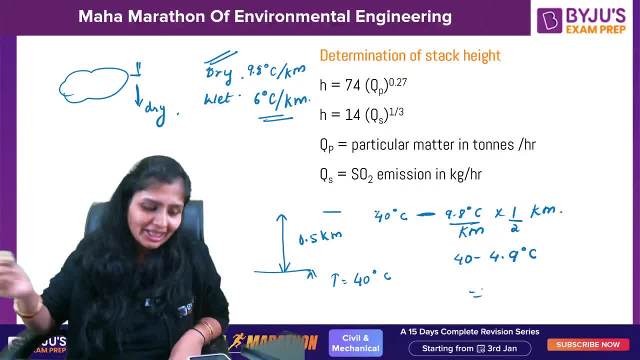 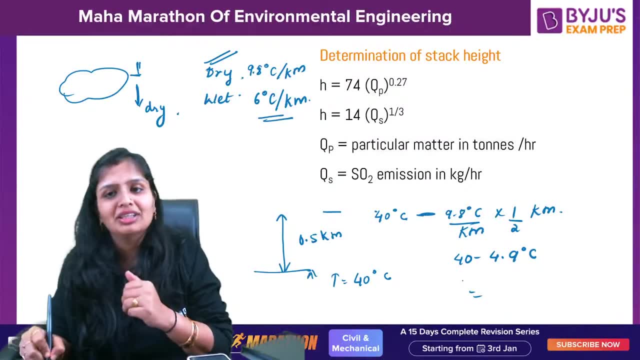 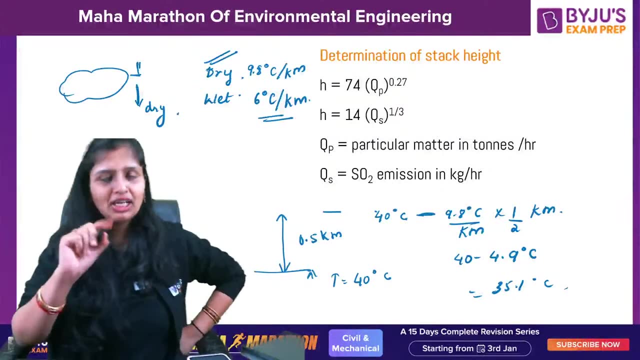 40 minus 4.9 degree Celsius. so this will be the temperature: 40 minus 4.9, 35.1,. this will be there. so such sort of questions are being asked. okay, Now one more type is that: ask that also, I will be doing. 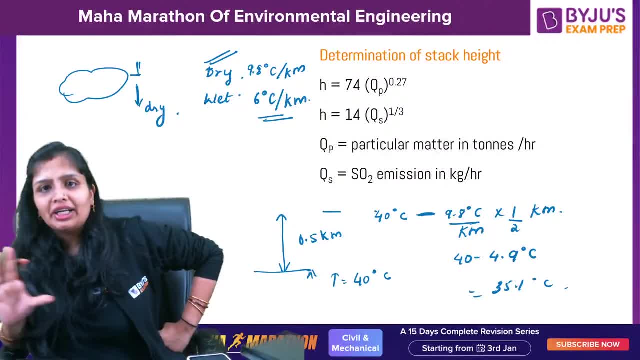 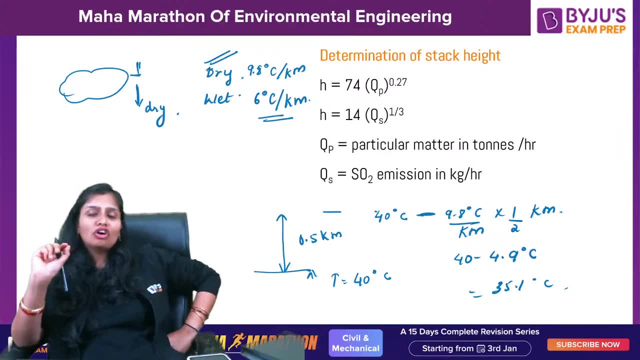 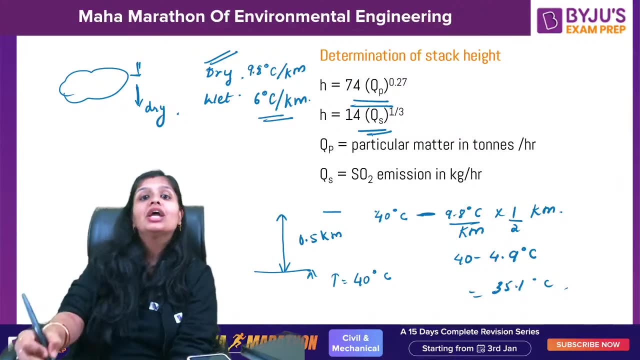 Now, stack means chimney. So if in the question right now they haven't asked, but they cannot, can ask you in one marks questions. if they ask you to calculate the height of the chimney, there are two formulas. one is 74 qp to the power 0.27. another one is 14 qs to the power 1 by 3 qp. 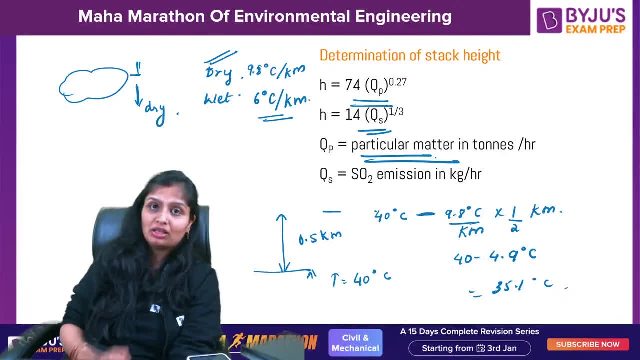 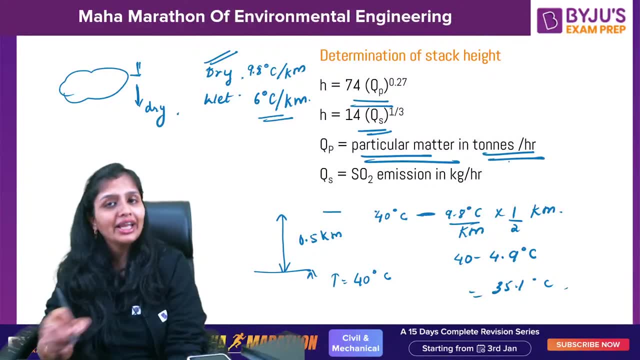 formula you will use when in the question it is giving you particulate matter. but remember, this is an empirical formula. you have to take care of the units particulate matter in tons per hour and qs is sulfur dioxide emission in kg per hour. okay, so you have to use this. 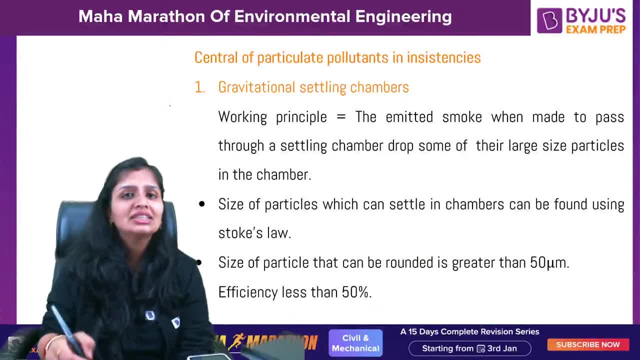 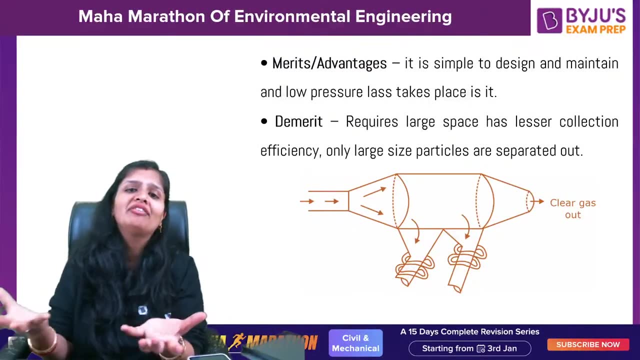 now last is control of particulate pollutants. so first is gravity settling thing, but nothing to apply. no brain to apply. bring the gas. who whatsoever pollutants are there, whose weight will be more, they will settle. simple, simple design. no brain, nothing is there. but the problem is efficiency is less than 50. large, large space is required and only those. 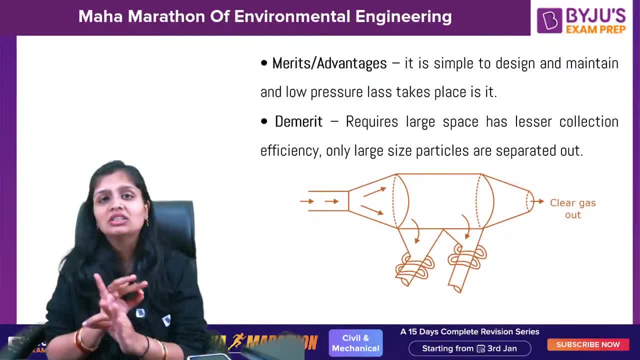 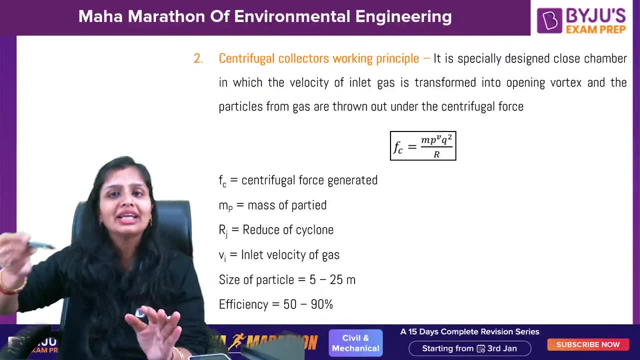 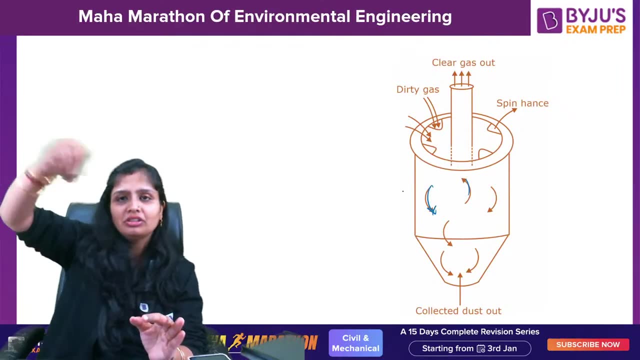 large particles will get settled, so smaller particles will not settle. this is for gravitational settling. centrifugal collectors, centrifugal case. what is that here? closed chamber. is there what you can see? vortex motion. so they will strike to the walls and what's ever particulate matter? straight. 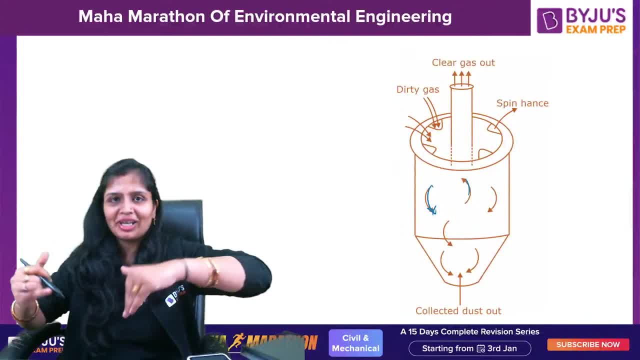 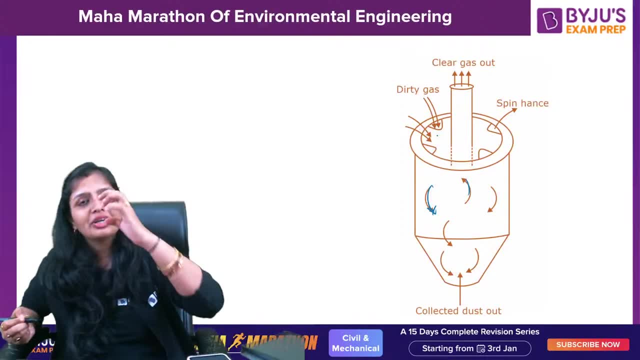 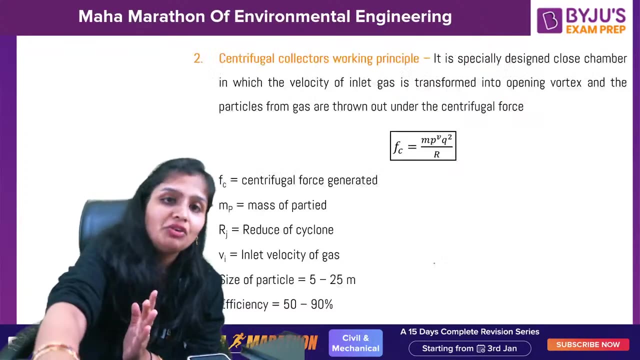 and it will have, like i'm doing the breakdance dance. it will get settled down and the clean gas i will get out. okay, clean gas will be out where it is clean gas is out, and the dust will be collected from water. so if you want to calculate, 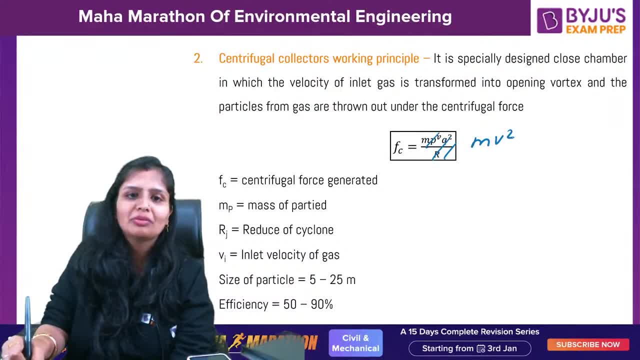 it. this is mv square by r. just simply write mv square by r, that's it okay. so this you can use. considerable efficiency. you will get around 50 times the amount of particulate matter. so this is to 90%. this is for ghooma kar, jhoom bharabar. it is jhoom bharabar, jhoom bharabar, gana ka melody. 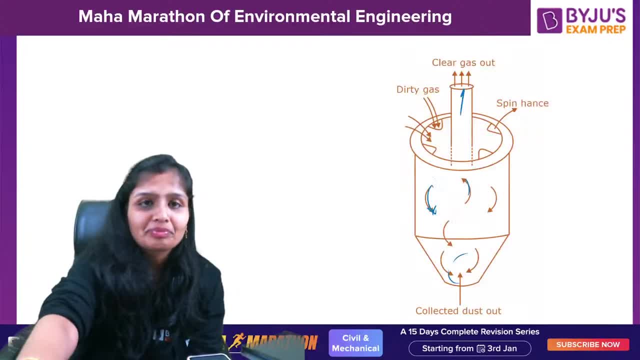 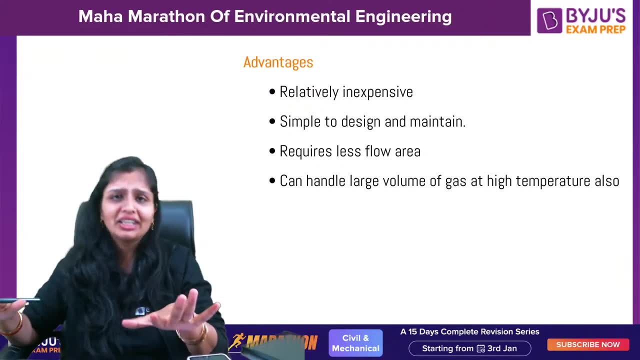 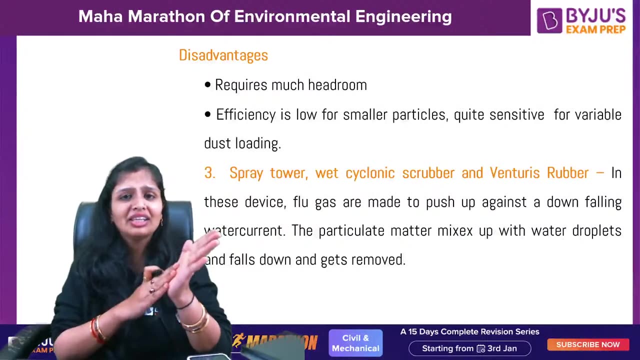 chal raha batao. this is centrifugal collector. okay, now, dimaak nahi inexpensive lesser area is there. efficiency bhi thik thak mil jati hai. achcha banda hai. okay, now, talking about disadvantages: already told you dust and all. are there now three things which function almost equally: spray tower. 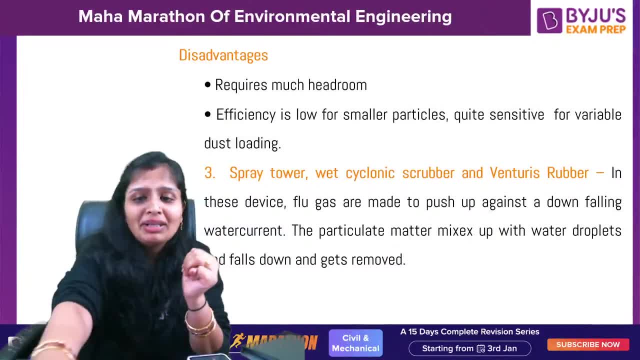 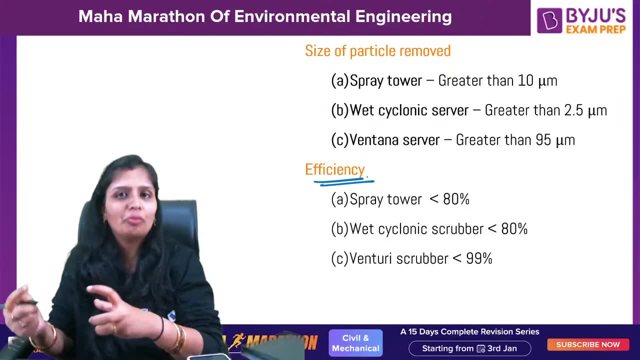 wet cyclonic scrubber, venturi scrubber. what happens here? yaha hum, use karenge pani, but the only difference which you'll get is in the efficiency and their method of operation. you use spray tower particle. this is important because they can ask you once a question, if i'm 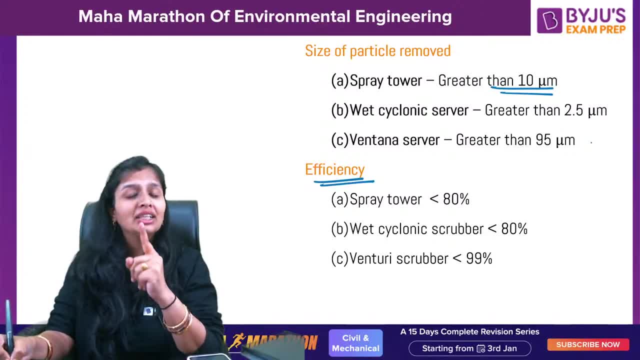 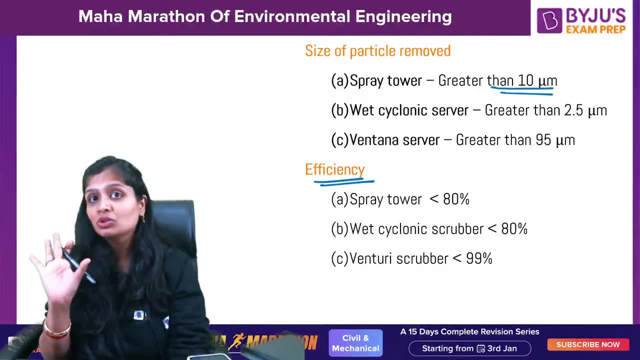 not wrong. 2020, a question regarding this sort of ask: baghouse followed by electrostatic precipitator. this question was asked like this question, so they can ask question. remember one question for sure: they will be asking for air pollution, so you cannot leave it okay. wet cyclonic scrubber- what a mistake. venturi scrubber. 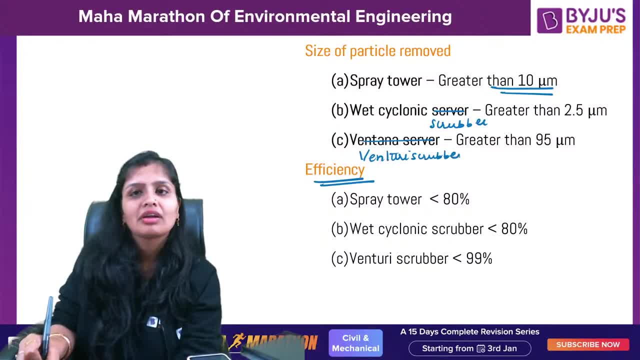 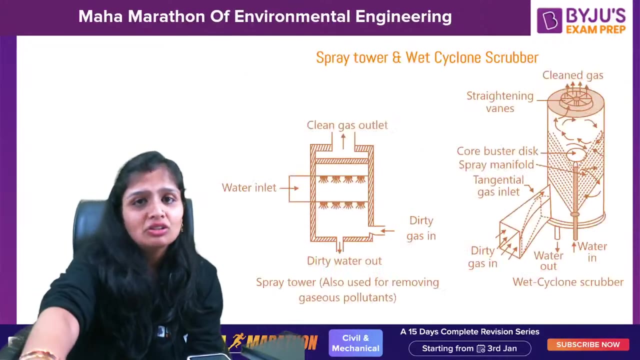 okay, this is different. this is not. the 95 micrometer is very big at 9.5. i'll check it out once. okay, venturi scrubber. is there now talking legs? venturi scrubber, if i talk about next is what has been done. so first i'll show you. 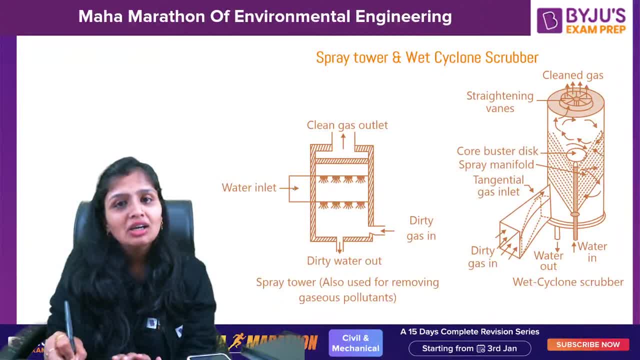 this is the spray tower. you can see the water. dirty gas goes here. clean water we will take. so what will happen here? absorption technique has been followed. dirty gas goes. whatsoever particulate matter, dust is there, water will absorb it. so clean gas will go out and the dirty water will go out from here. same thing, which will. 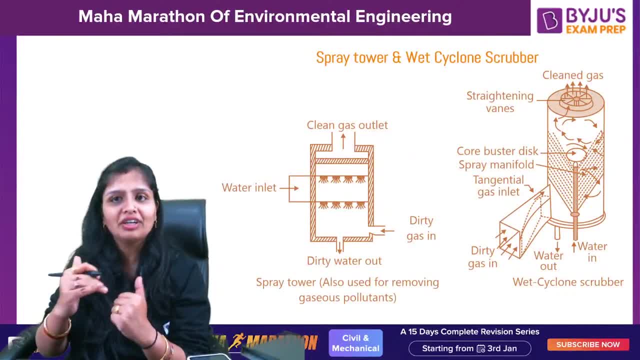 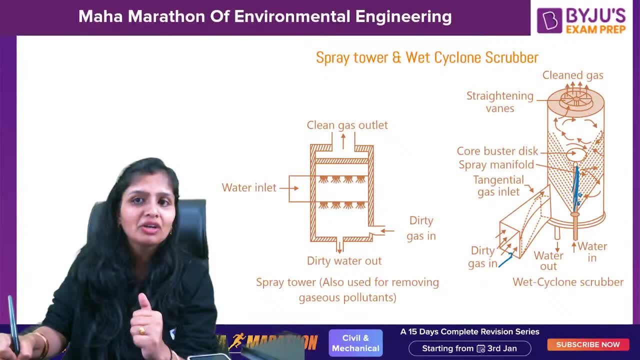 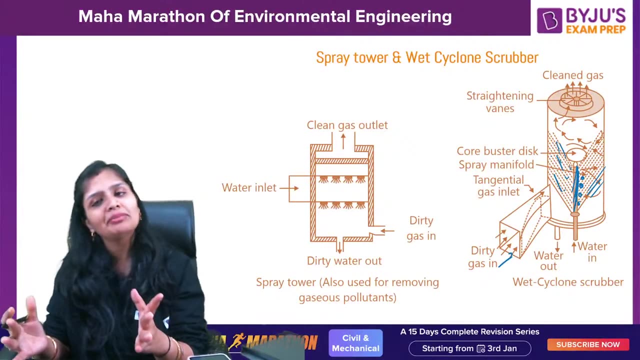 happen in which cyclonic scrubber, the method is different, but the thing is safe. what will happen here? the dirty gas will go and here the water will go. but here, perforations are there, small, small holes are there from which the water goes. okay, and now what we'll do again here: absorption. 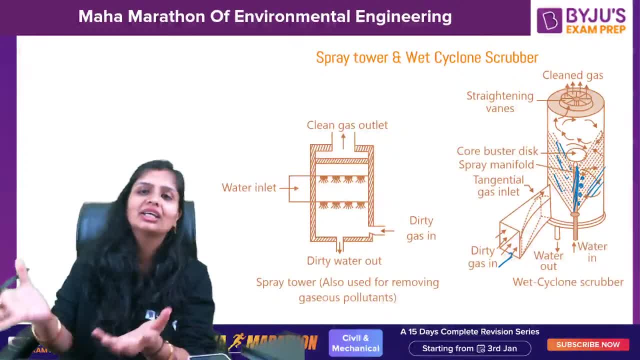 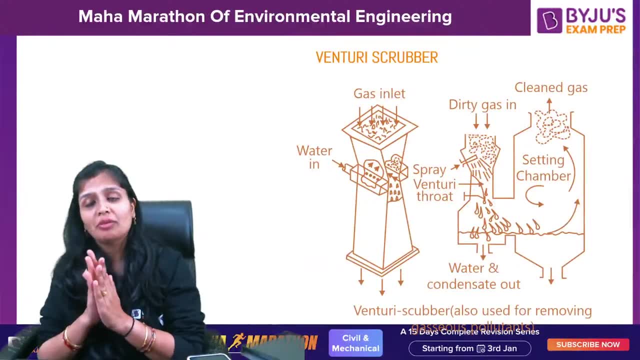 principle whatsoever: pollutants are there, they will get absorbed and the clean gas will go, will go out. okay, so this is wet cyclonic scrubber. now the most important is the venturi scrubber, because you are doing the same operation two times if you do the same times. 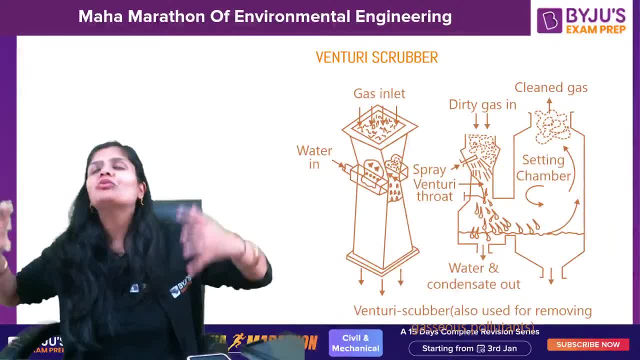 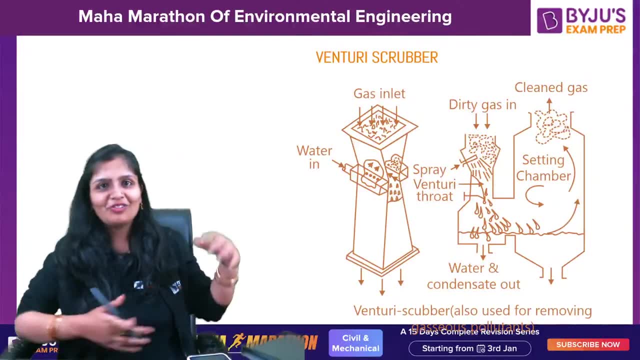 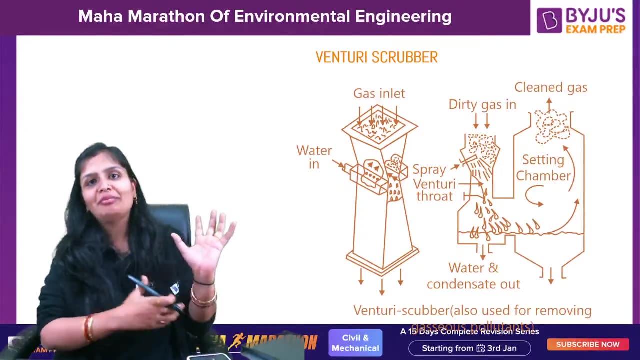 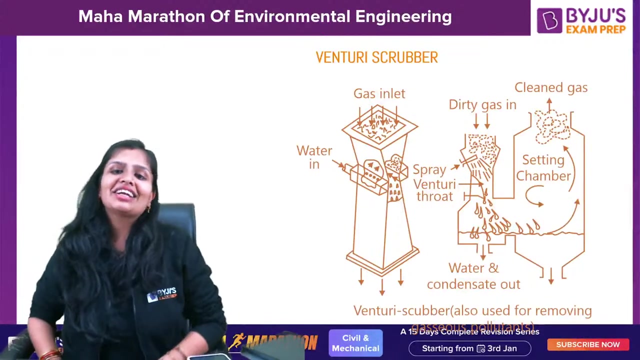 let's talk about venturi scrubber. so what will be happening is dirty gas will be here in the first chamber. you will be providing water. so what will be happening? what will be happening here? absorption principle. second, you are doing what? so that whatsoever, or gravitational, basically. so what will happen? you have provided a settling. 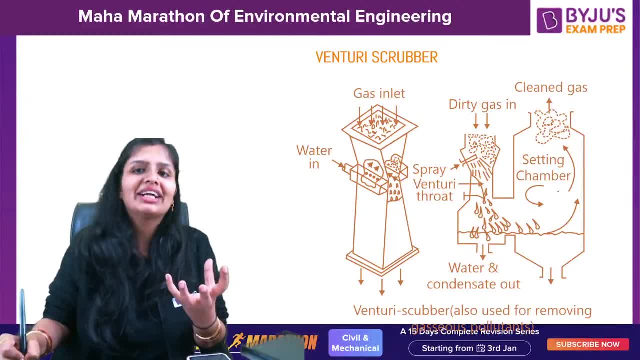 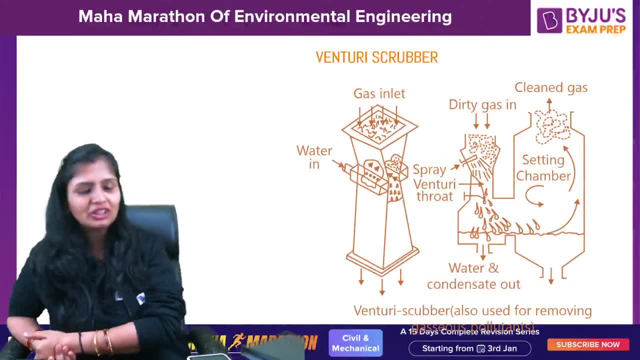 chamber. so those impurities which are heavy, they will settle down. so actually the operation is done twice. so comparatively greater efficiency is obtained for the case of venturi scrubber. that's why if you see it venturi scrubber, you get 99 percent of the 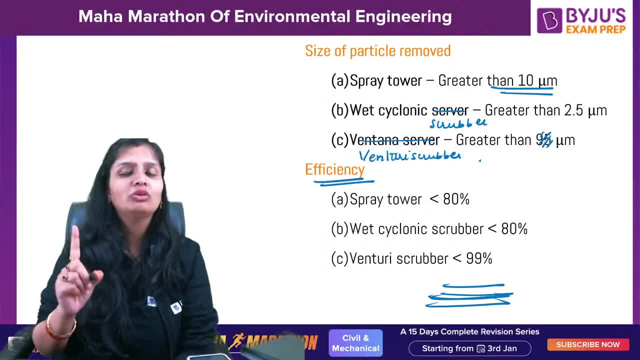 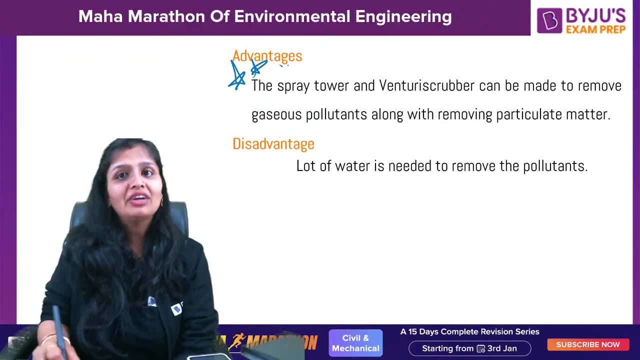 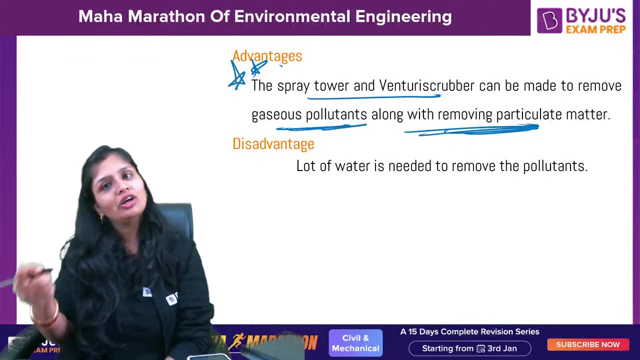 efficiency okay, as compared to any other. now talking about one more thing important. this is very important: the spray tower and venturi scrubber. they not only reduce, remove gaseous pollutants, they remove particulate matter also, both- right now every removal- we were talking about particulate matter. venturi scrubber and spray tower remove particulate matter, but they're 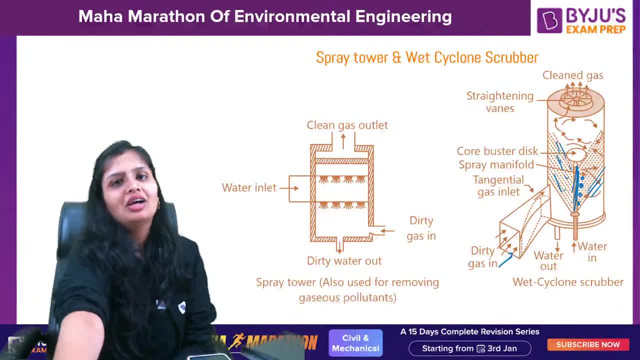 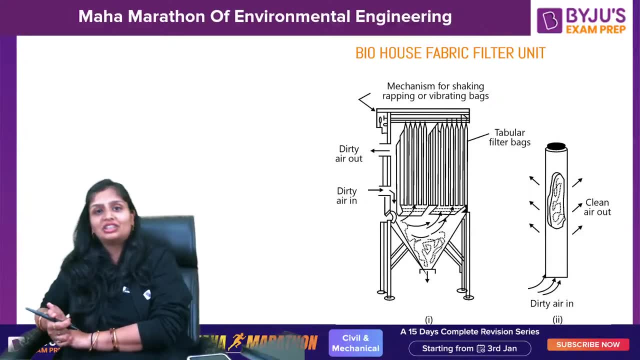 also now, this is the best one: dry air. so what will happen? dry, dirty air will pass through it. whatsoever is the clean air will go out and that particulate matter and all will get trapped. so this is a. it has shown you one fabric filter. multiple number of filter bags are there, okay, so this is big house filter bag. 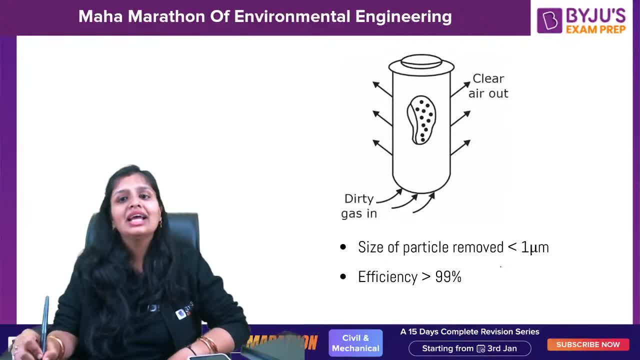 So this is big house filter. You can see less than 1 micrometer particles are also removed, Highest efficiency and even the smallest particle size is being removed. Okay, The thing is it has to be in dry state That you have to maintain. 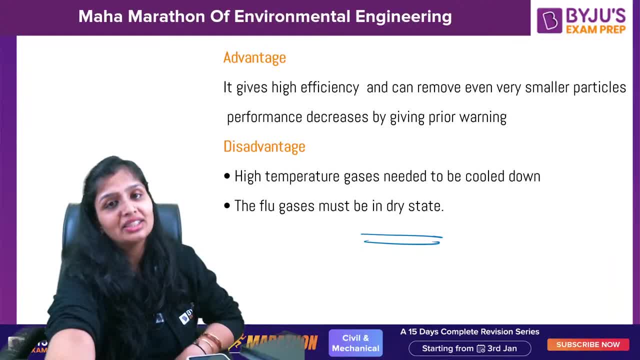 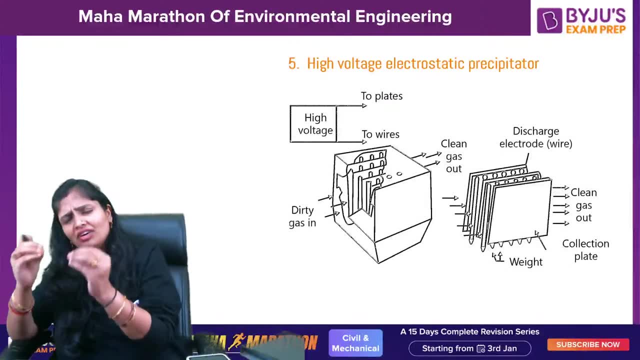 And the high temperature gases may not burn the cloth, So that is the reason temperature is also to be maintained. Okay, Meet Electrostatic precipitator. In every power plant you go, you will see this electrostatic precipitator, ESP. 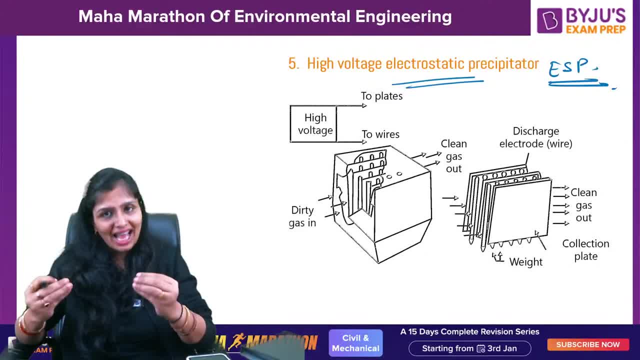 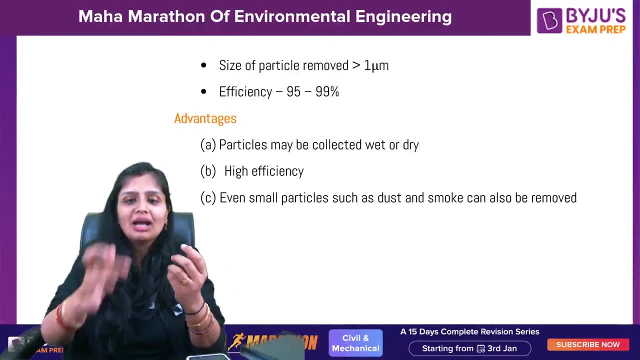 What we do it here. you pass the gas. they gain the charges. Then you will pass it through the plates, So the charges attract and eventually those particles are removed. As simple as that. So what is happening? The flue gas is made to pass through this highly ionized plates. 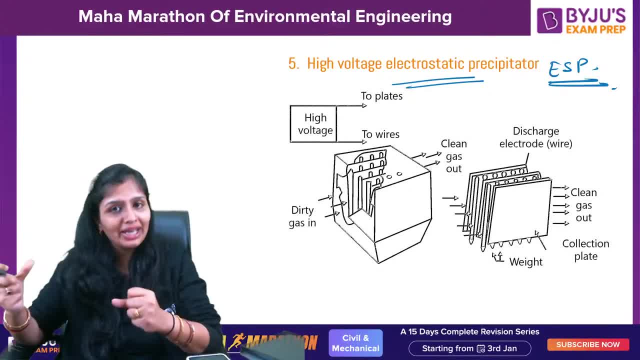 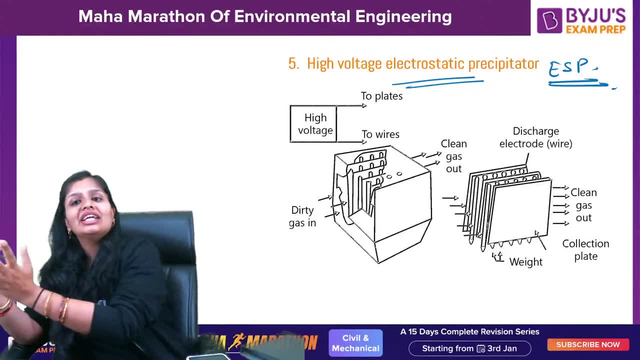 This is there. So they get the charges. They go through the plates. Okay, The dirty gas will go in, They will attach to the respective electrodes and you will get the clean gas out. So this happens in the case of electrostatic precipitator. 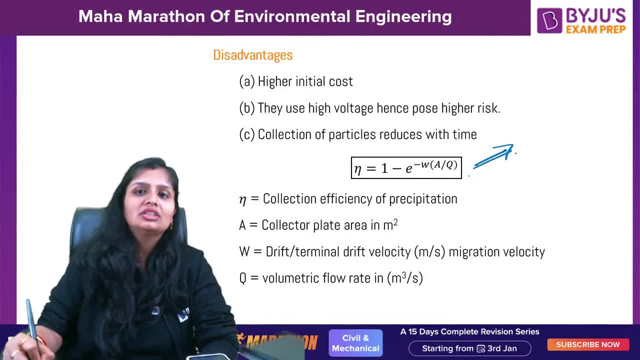 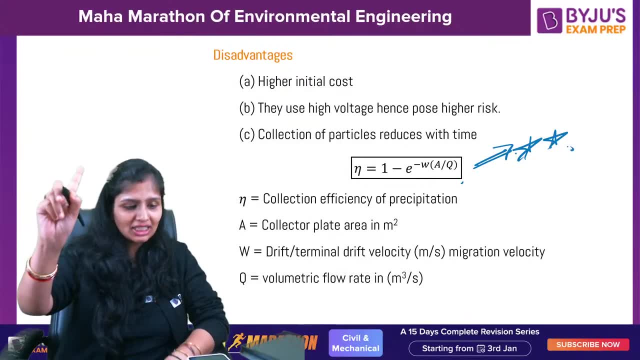 There is the one formula which is used. This is the formula 1 minus e to the power, minus w a by q. Very important. Remember this because questions has been asked twice. The best will be done by planting trees and plants. It will be done by planting trees and plants. 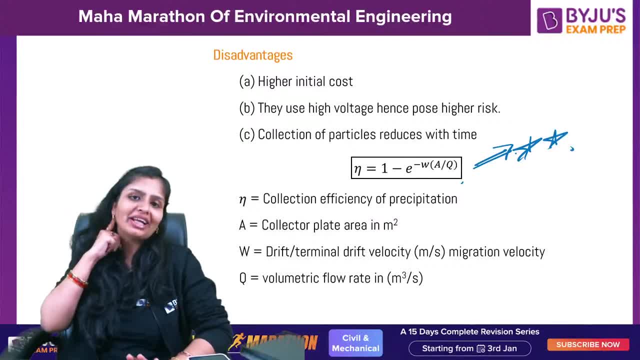 So efficiency is 1 minus e to the power, minus w, a by q. E tells the efficiency, A is the collector area, Q is the discharge And w is the migration velocity. Okay, Simple questions are being asked from this efficiency. 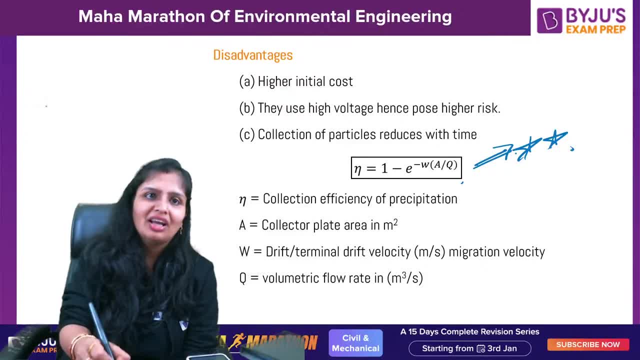 Let us suppose example Questions. These are small questions. Okay, If 96% Is the efficiency Collector area, is this much? If 97% is the efficiency Collector area, is this much? What will be the collector area if 99% efficiency? 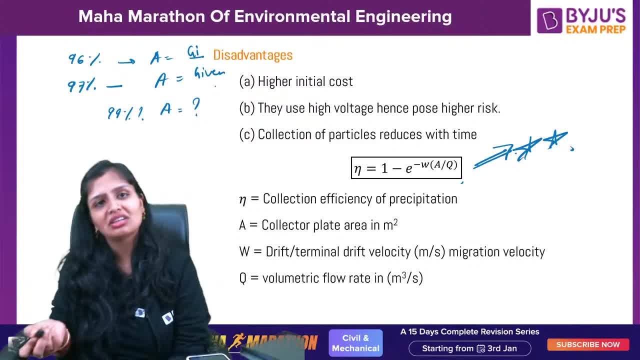 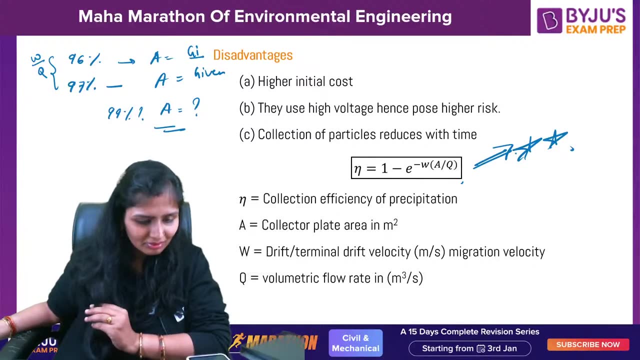 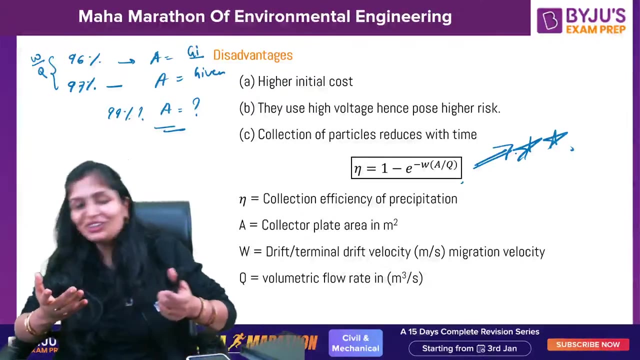 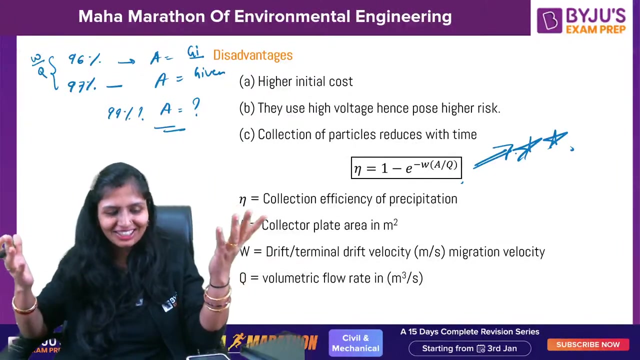 This is given. This is given And this is asked. Two equations, not needed also From any one equation. calculate what w by q, Substitute it here, You will get the answer. Such simple questions are there. So if this is the answer, then now the answer is: 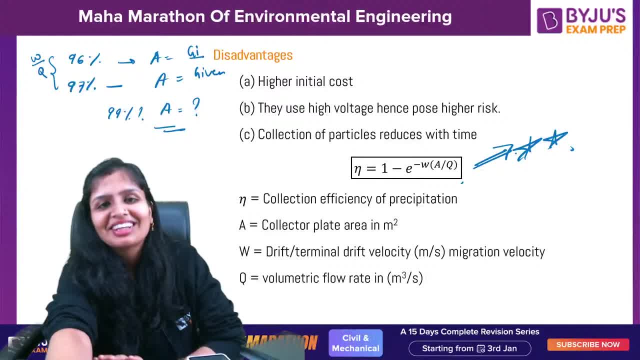 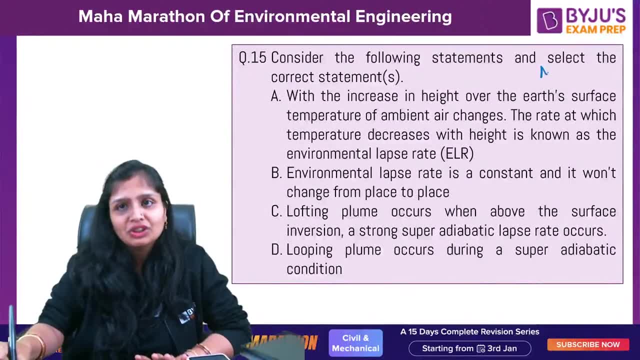 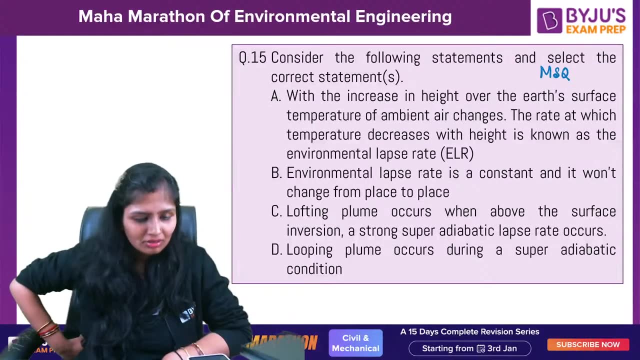 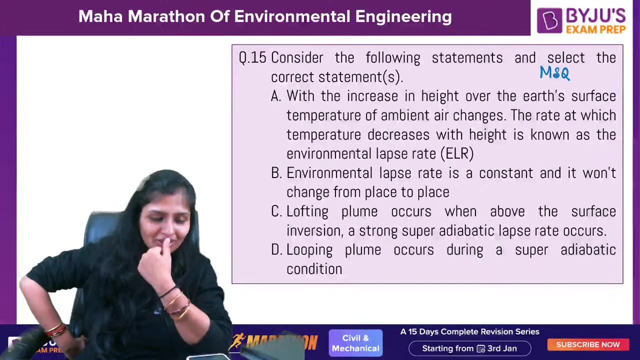 I want to calculate this for the height. This is the right answer. It should be the right answer as well. So let me have one more question. So this is the right answer. It should be the right answer as well. tomorrow is my hydrology paper. how can i take class today? which class you want? 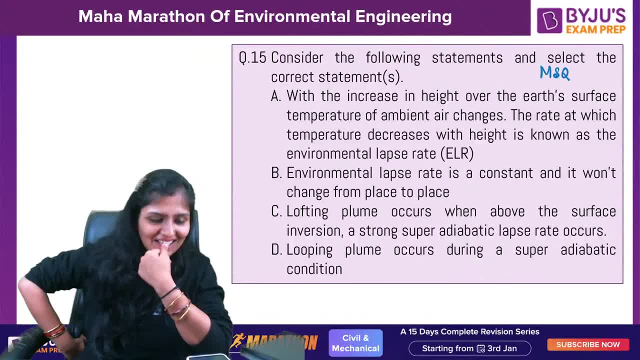 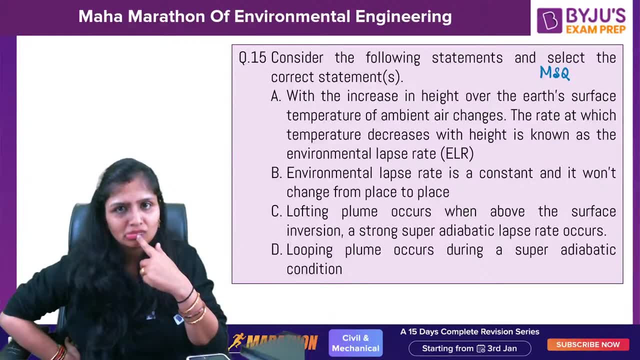 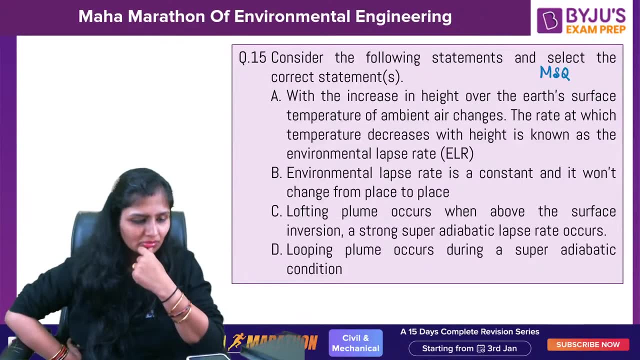 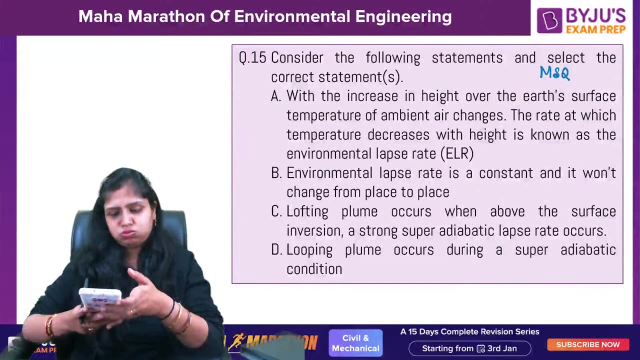 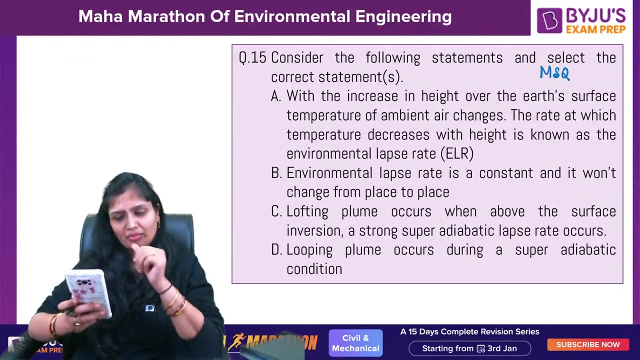 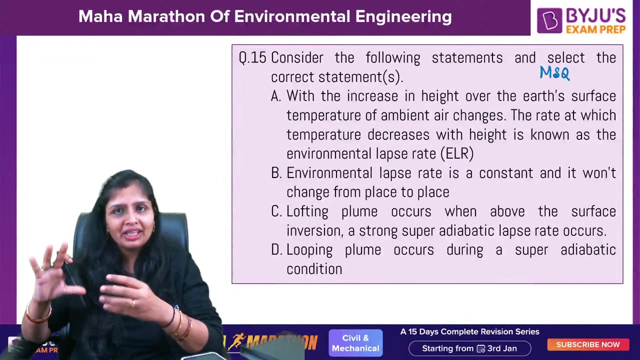 come on guys. msq question. drift will drift velocity? see electrostatic precipitators. you are charging the particles. you are passing it through an high ionized plate where they get charges. you are passing it through an ionized plate where they get charges, so the velocity which those charged particles attain, that is known as the drift velocity. 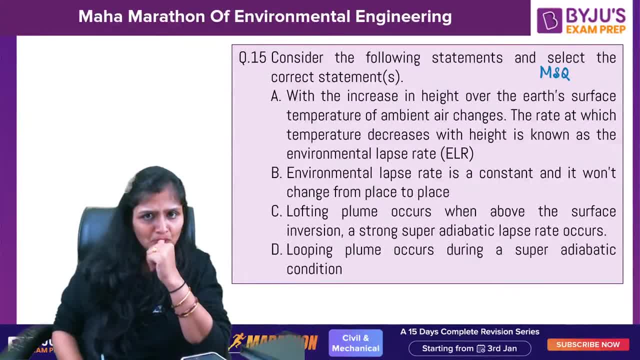 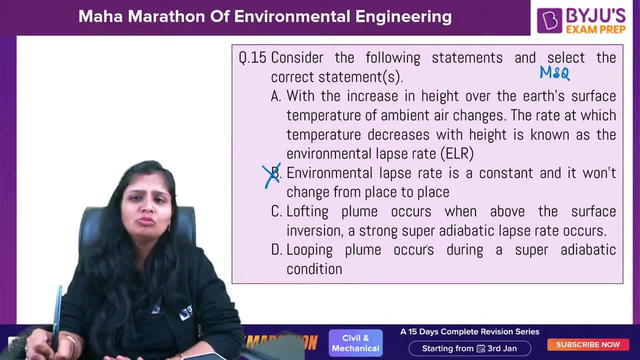 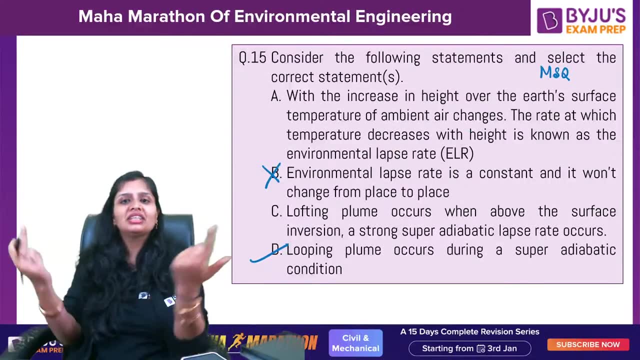 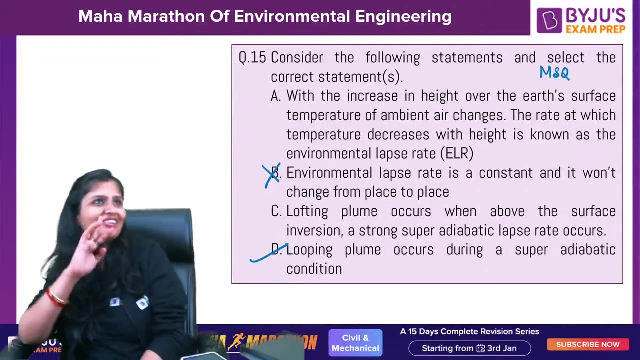 okay, a and d see this is wrong. environmental rap state changes. looping flume occurs during a super adiabatic. this is correct. with increase in height, temperature of ambient ambient air means the surrounding air changes. okay, uh, this you know. when you say the ambient such when we go to the hotels and all. 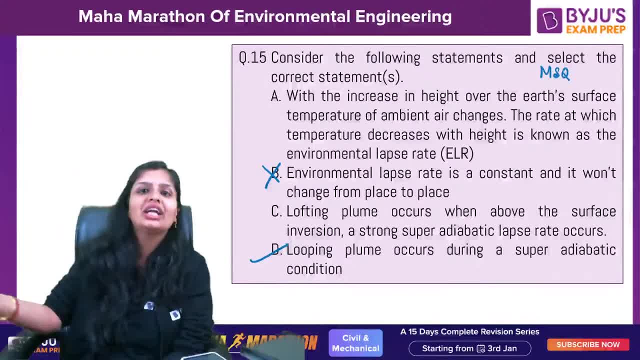 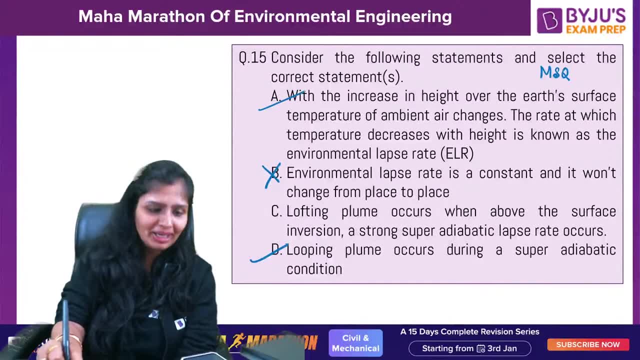 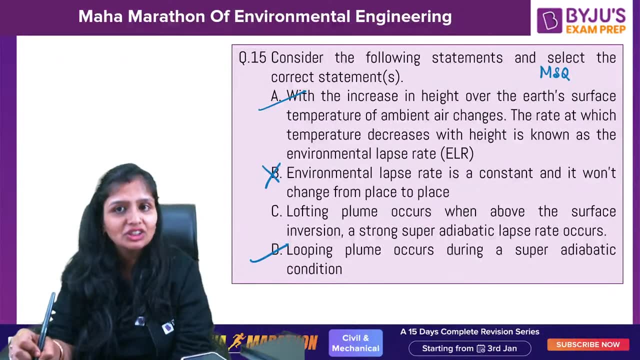 very so. the velocity which those charged particles attain, that is known as the drift velocity. selfie Clicker: ambience, so it is good. ambience means surrounding, so that is ambient, is the surrounding air changes. so when the temperature decreases. so this is environmental lapse rate correct, isn't too late. also correct: laughting flume occurs when above the surface inversion a strong. 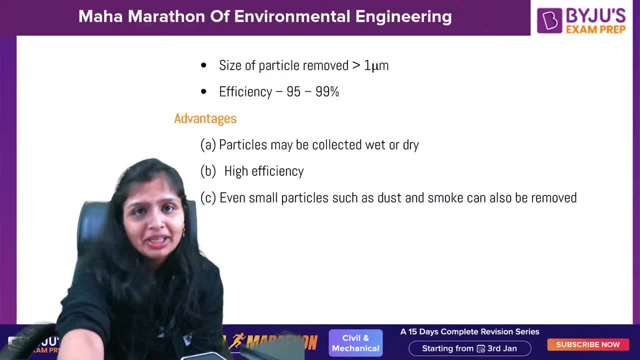 adiabatic condition. this is also true. who said: not picture you forgot c1, lofting and fumigating beta where it is size, where it is civilizing rather than ex. còn the buyers tix not anymore. no problem, elisa, you did not miss it when i worked your life. 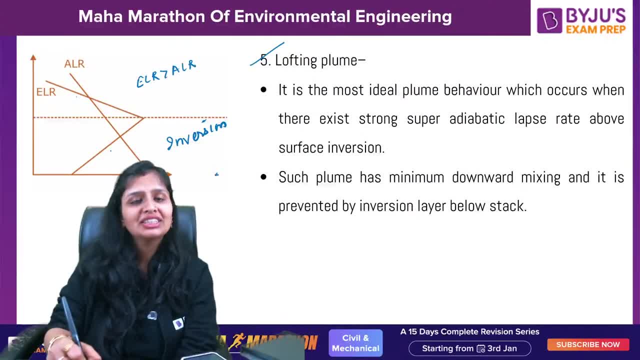 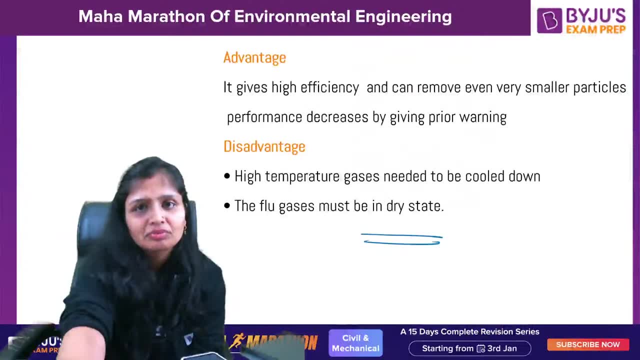 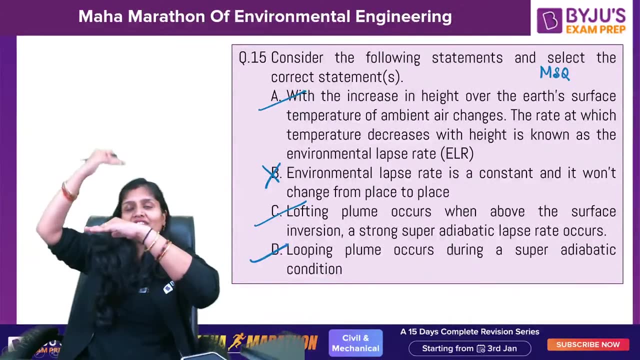 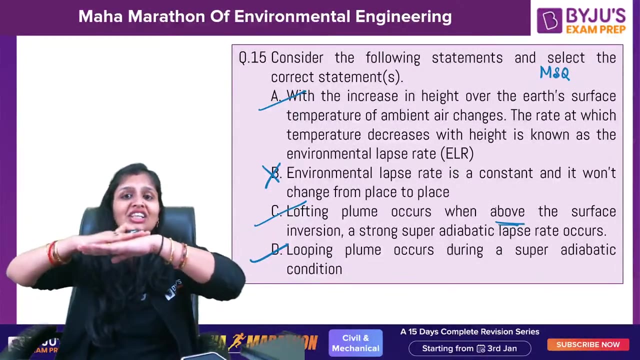 it is Locking first inversion, then super adiabatic, Pumigating opposite. So that is only written here. Just check it out. Above the surface inversion. Above the surface inversion: strong super adiabatic condition. Order is mentioned na When: above the surface inversion. 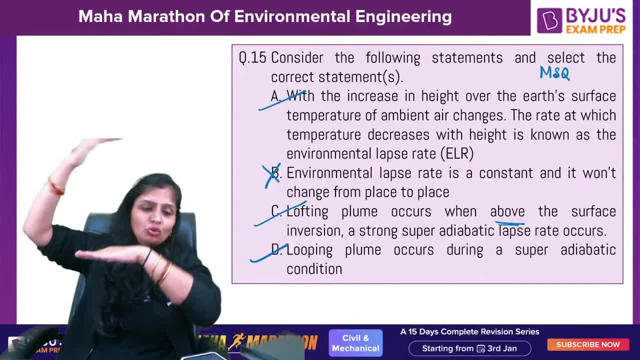 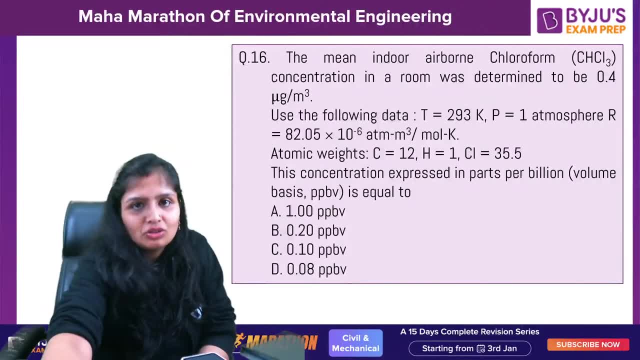 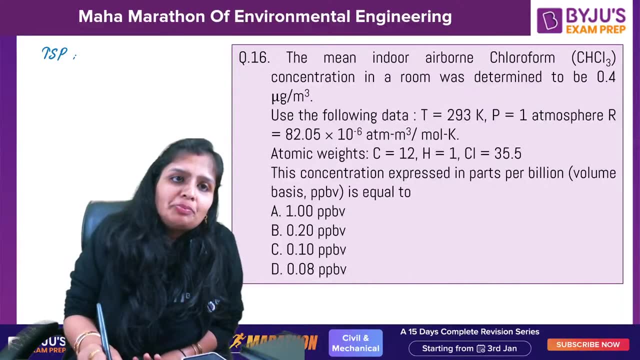 ke upar Surface inversion. ke upar, Got the Girish Fine. The last question. So I tell you the formula. first, Total suspended particulate matter in microgram per meter cube. if you need The concentration of that total suspended particulate matter particle in ppm is: 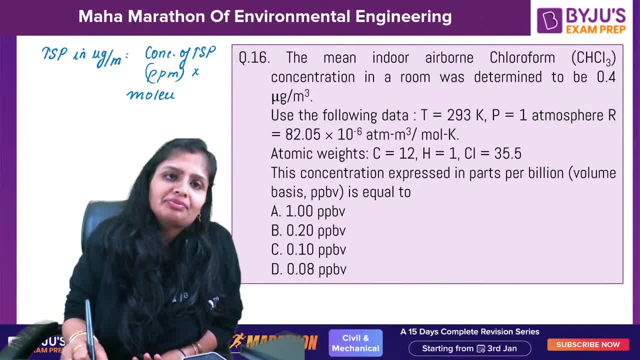 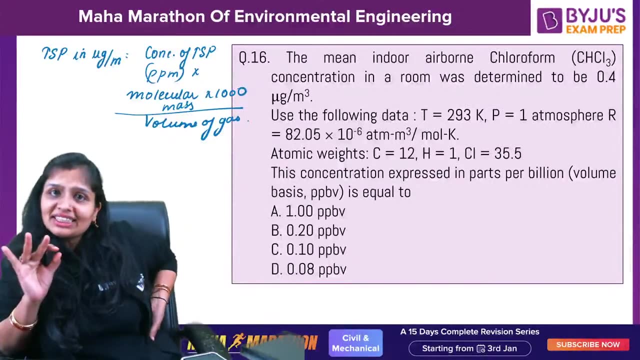 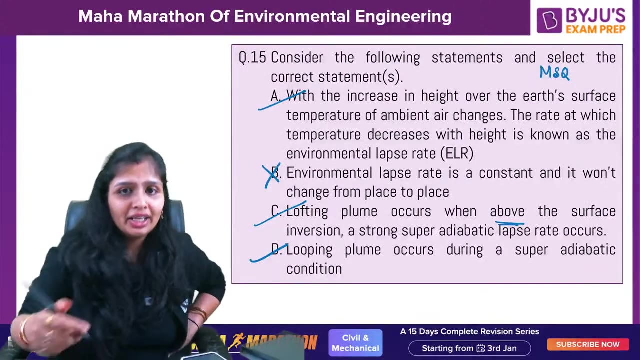 into the mass. Technically it is molecular mass Into 1000 divided by volume of gas. This is the formula Now: volume of gas at standard temperature and pressure condition. Which one is above, Which one is below? Diya to hai Dikho na Girish. Above surface inversion. 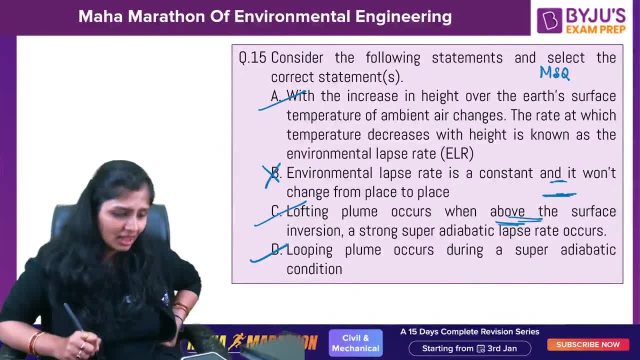 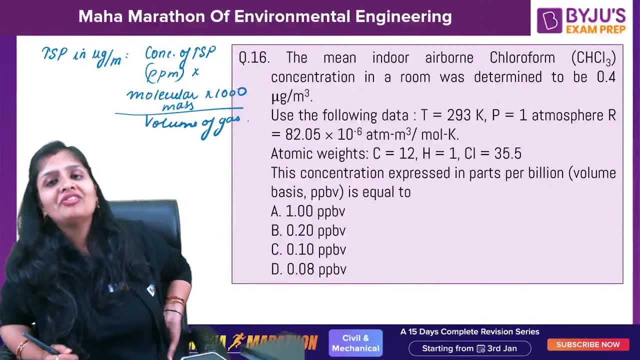 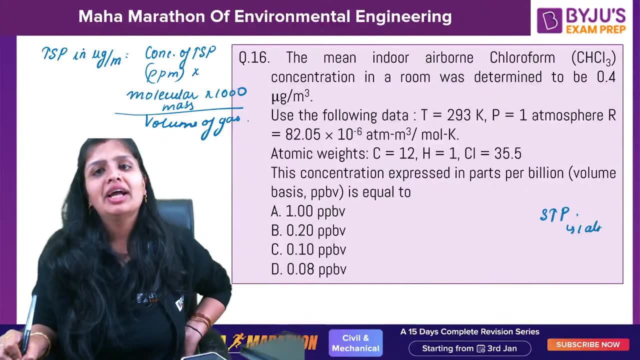 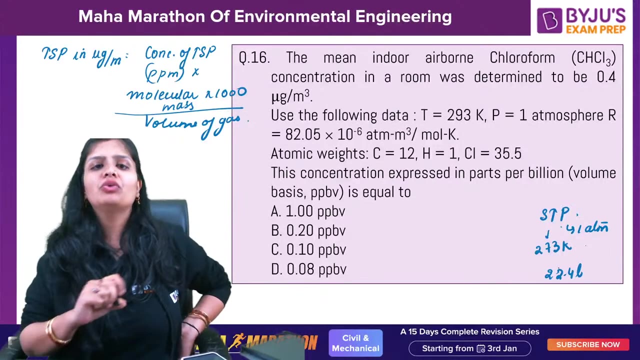 Surface inversion, Ke, upar. It is mentioned beta, Fine, So the volume of gas at standard temperature and pressure Pressure is 1 atmospheric Temperature, 273 Kelvin. Okay, So the volume occupied will be 22.4.. If any other, If any one of the thing changes, If pressure changes, Temperature, 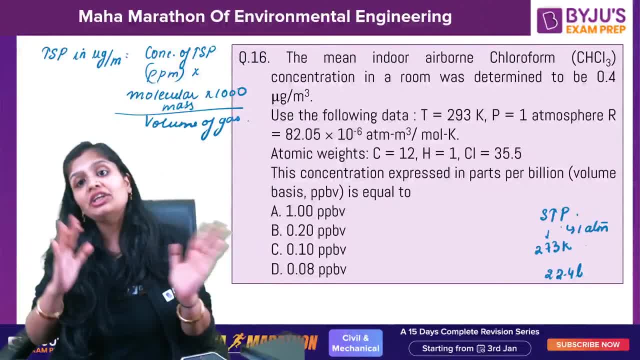 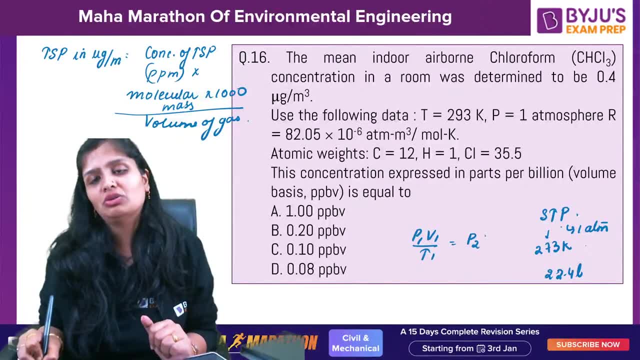 changes. If any one of the thing changes, The volume will not remain same. Then you have to calculate the volume. There is a relationship. once upon a time in chemistry you would have studied: P1, V1 by T1 is equal to P2, V2 by T2.. So from this relation you can calculate. 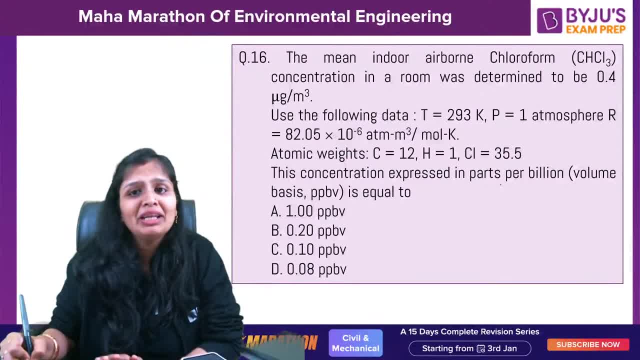 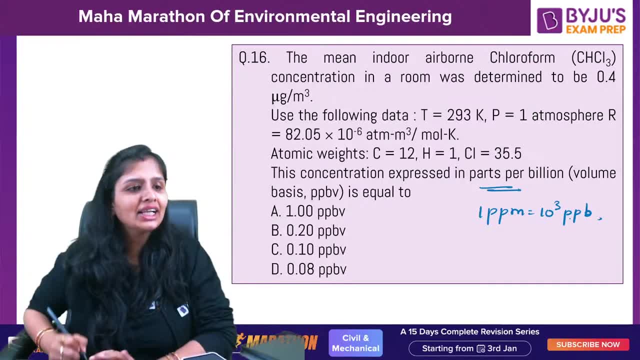 it. Now. see this question. It is asking: mean parts per billion. 1 parts per million is equal to 10. raise to power 3 parts per billion. Is it correct? Kam kalak bhi likh sakte. So now. 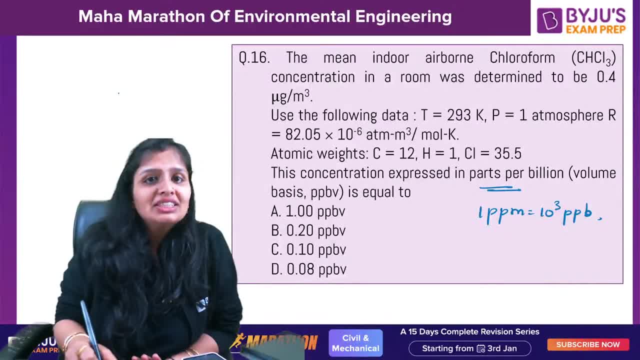 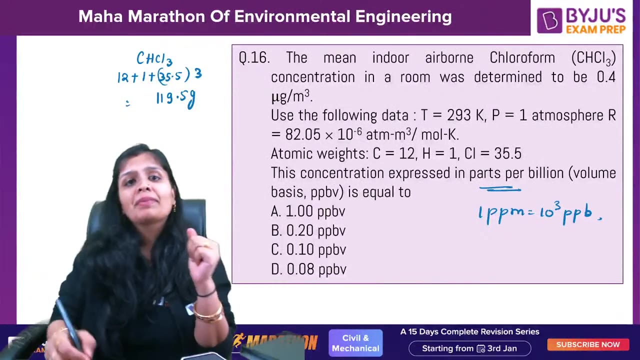 Now the concentration it has asked. First calculate the weight of CHCl3.. CHCl3 weight is. Carbon is 12.. Hydrogen is one. Fluorine is 35 point 5 into 3.. How much is the weight coming? This is the waste, This is coming. Okay, Now this is the 119 point 5 grams which 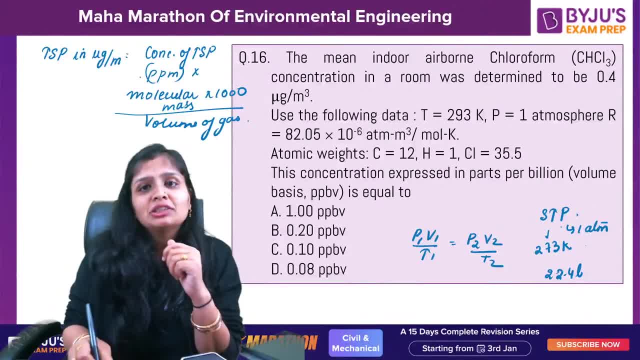 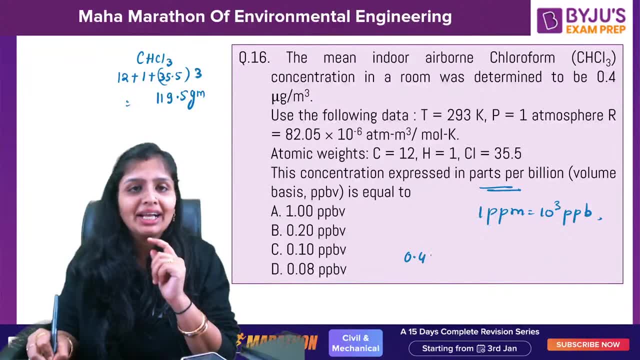 is the waste coming Now this TSP will be how much TSP? TSP is given to me directly, 0.4.. 0.4 value: it is given to me directly. Concentration in ppm. first I will calculate Molecular weight. I know 119.5. 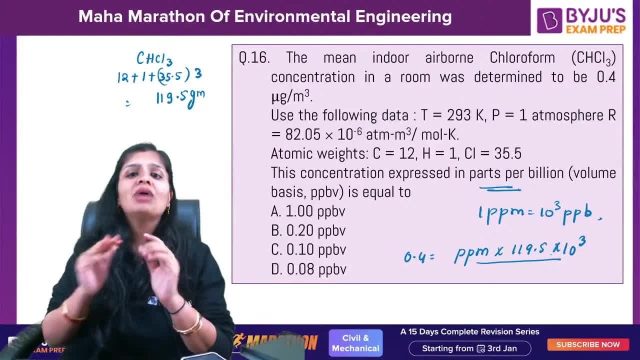 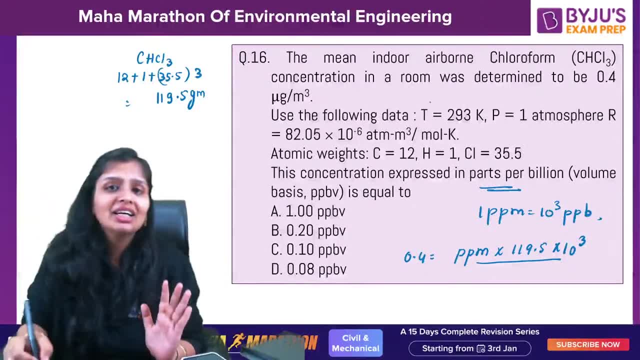 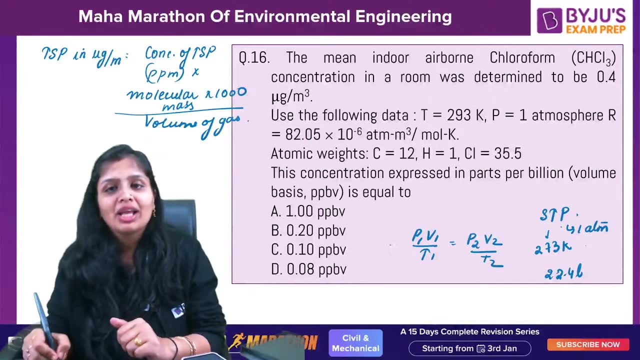 divided by 1000.. Volume I have to calculate. I cannot put 22.4 liters. Why? Because pressure is standard but temperature is 293 Kelvin. So first, what I need to do, I need to calculate the volume. So here the pressure was 1.. Here the volume is 22.4.. Temperature is 273 Kelvin. 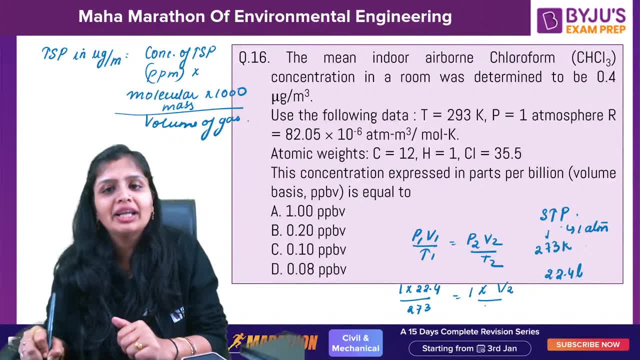 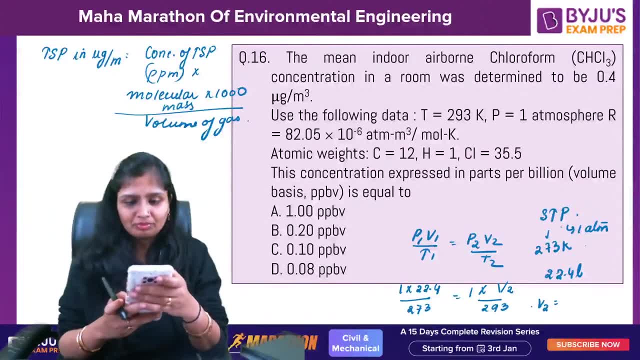 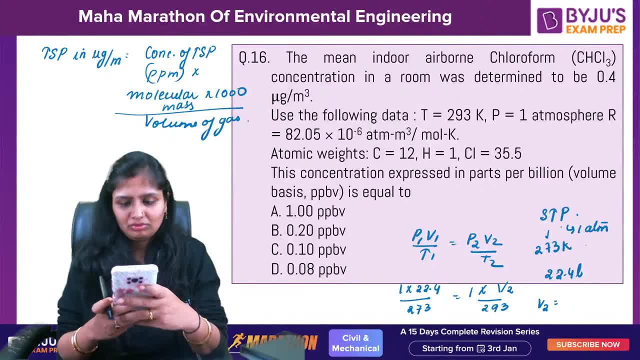 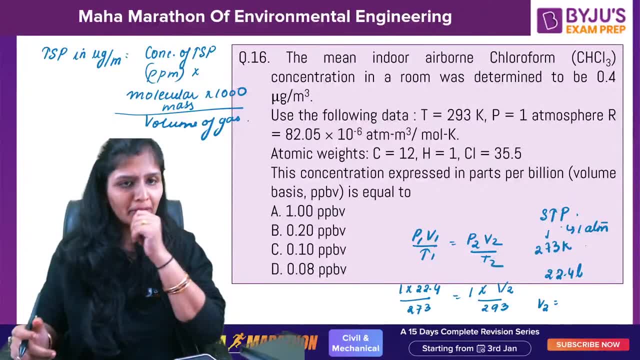 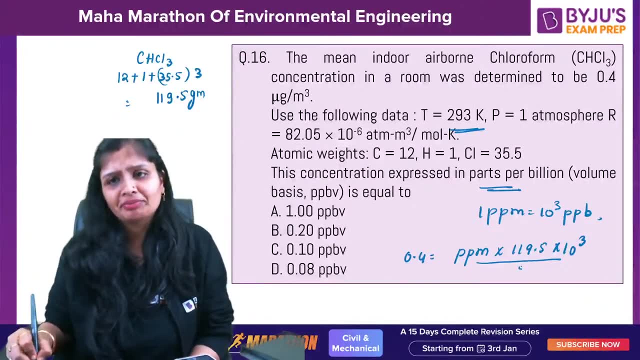 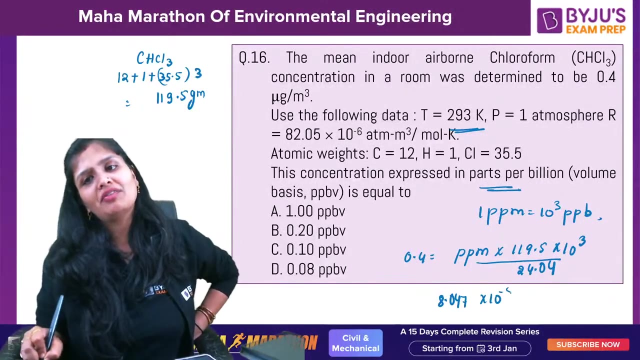 Come on guys. what is the volume? How much is the volume coming Bhas khatam Tata, bye, bye From here. what you will get? 8.047 into 10 raised to power minus 5 ppm. So multiply by 10 raised to power, 3 for 4.. 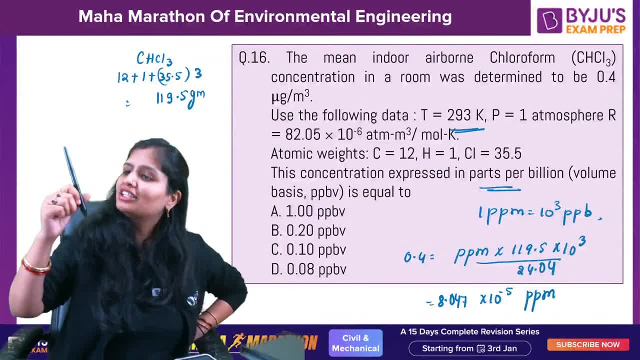 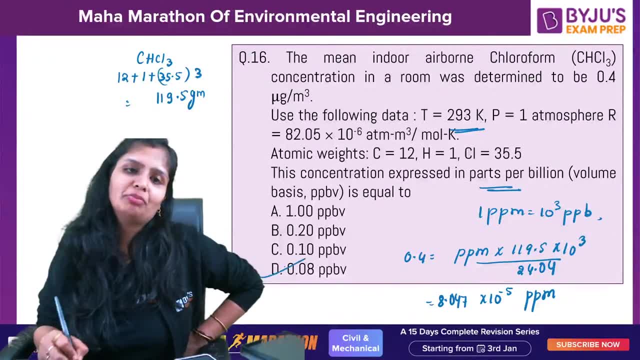 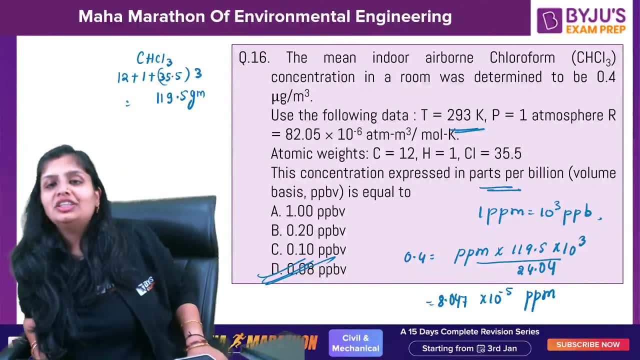 What magic happens? It is a magic pencil. The slide moves forward automatically. So parts per million multiplied by 10, raised to power 3, you will get 0.08.. That's it. So this completes your entire environment marathon. 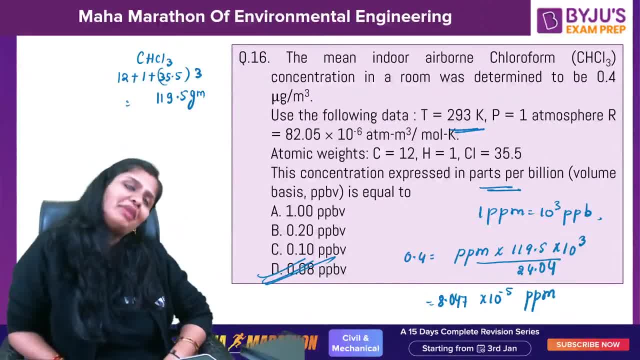 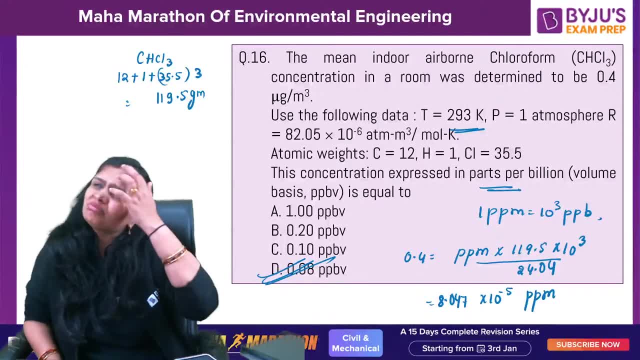 Any doubts? Now we will take a midnight session tomorrow. Today I think you guys are exhausted also, So we will take it on Sunday. I guess Salute hai jitni lambi class lene ke liye. Thank you, Knowledge Adda. 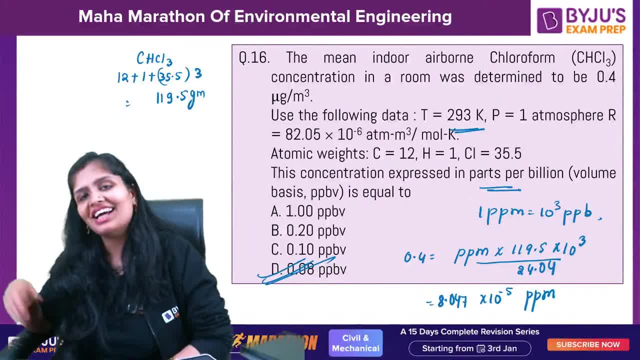 Aapse hi knowledge le rahe hain. Aapka pyaari hai. Start gaya 90.. Dekho, Thank you, Arun, Arun, thank you, Apni ESC ki preparation ke sath sath aapne mujhe dekha. 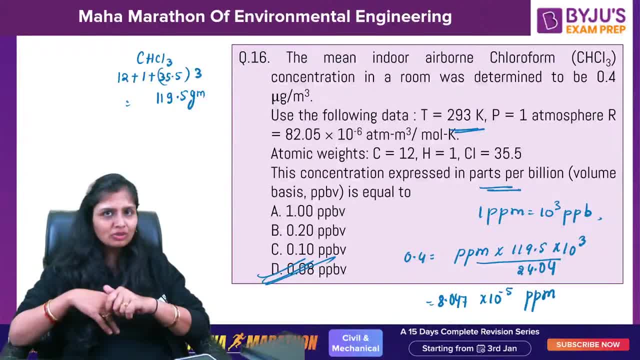 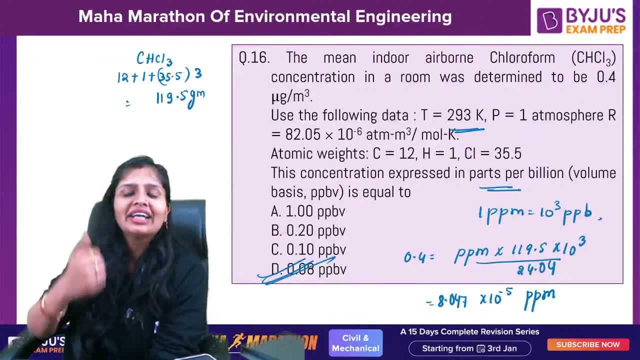 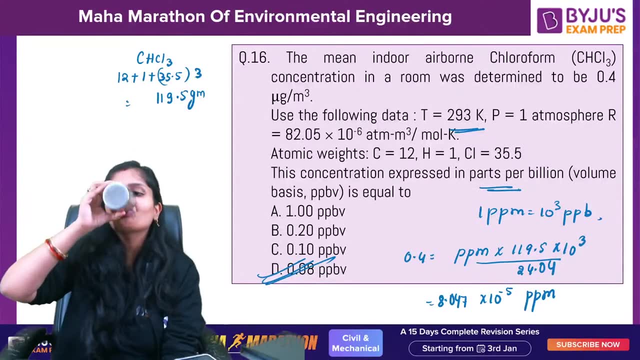 Thank you everybody. So any doubts You can ask to me in my telegram group. TB related calculation problem. aati hai Girish. this is a gate problem, only bitta. This is gate problem, only Calculations. aati hai aur IBI hai. 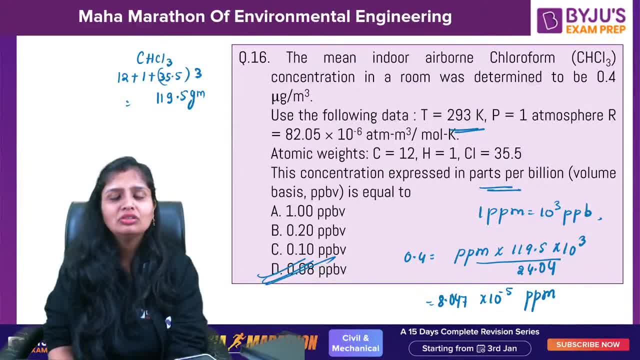 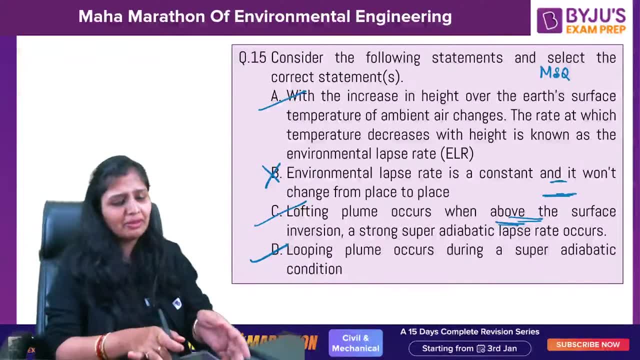 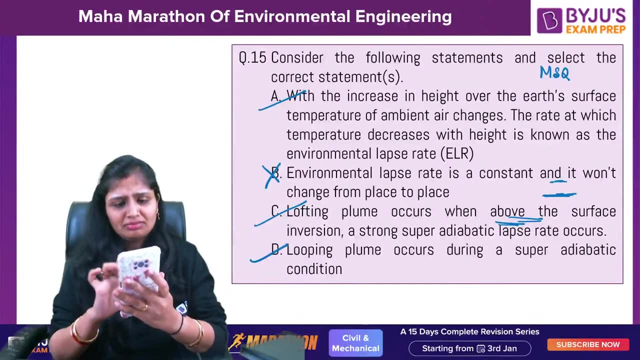 Gate mein questions. Okay, So this type of questions they ask And one more type questions are being asked. This is my thought of telling Just one. One more type question are being asked: Where is that PDF? Just a minute. 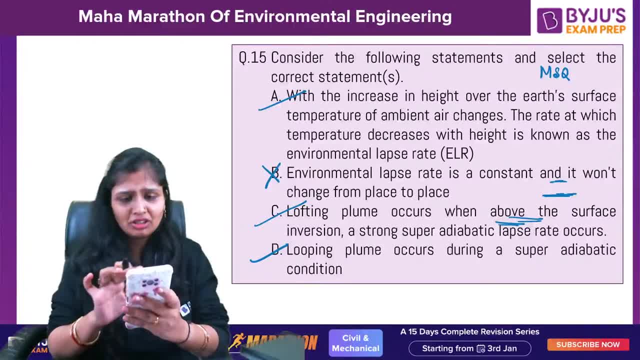 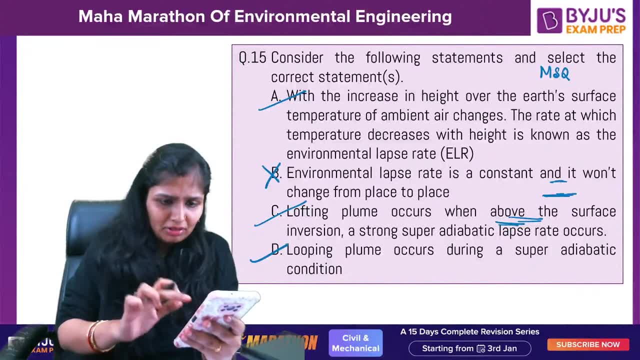 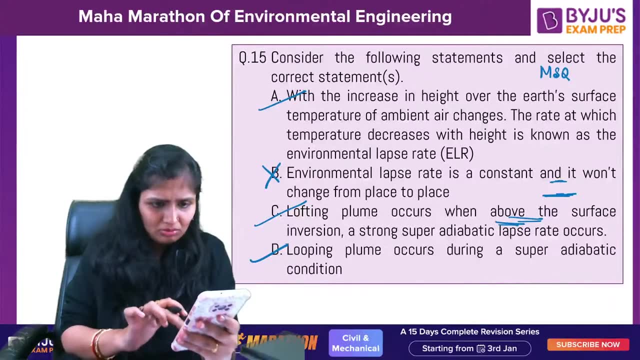 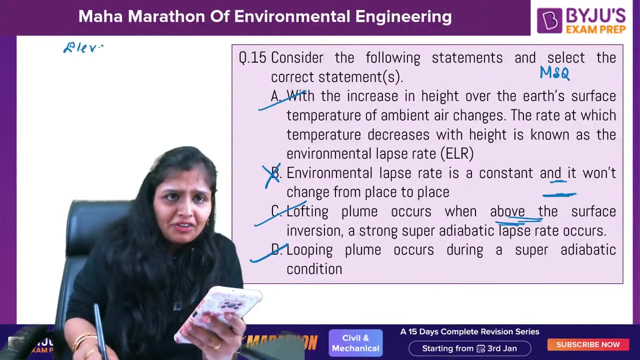 This is a patent question asked 2-3 times in your gate examination. Last isko bhi kar leta Chhoda hai kyo. Air pollution. Air pollution Elevations in meters- it is given to you as how much. 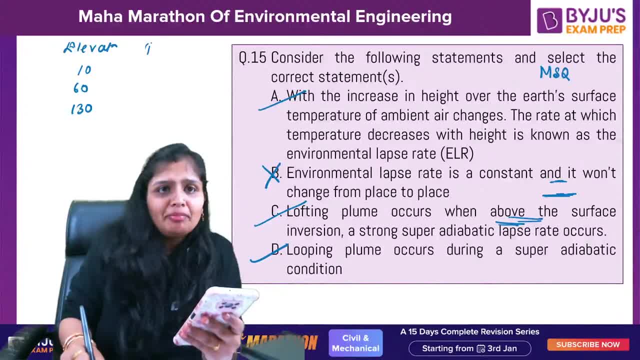 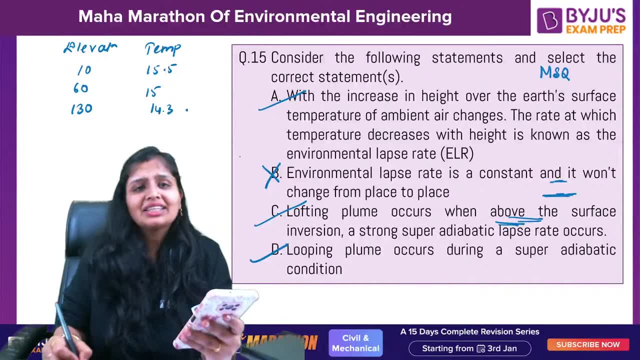 10,60,130, and temperature is given to you as 15.5,, 15 and 14.3.. And it is asking you: the atmosphere is classified as stable, unstable, neutral, inverse. 2017 IIT Roorkee. 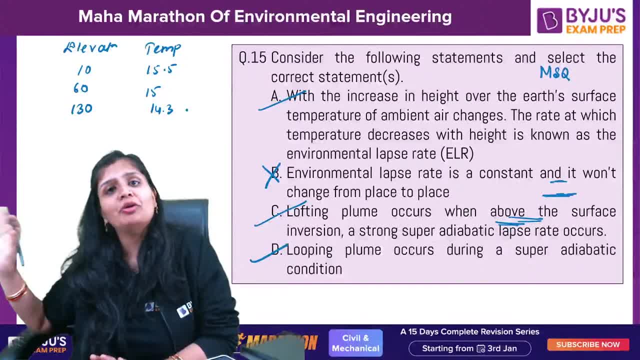 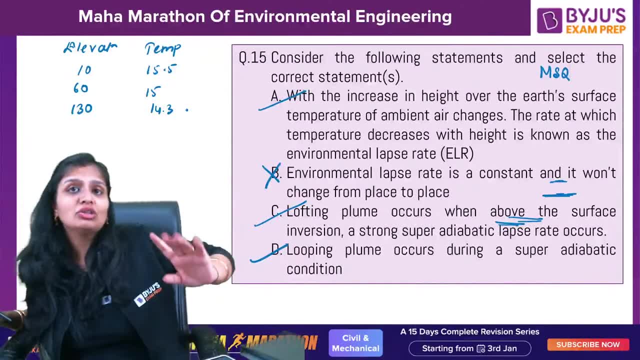 See If this thing comes. Always remember: ALR is 9.8 degree Celsius. but one thing: if in the quotient it is telling you to take ALR as 10 degree Celsius, in that case you have to take ALR as 10 degree Celsius. Okay, so you calculate ALR. 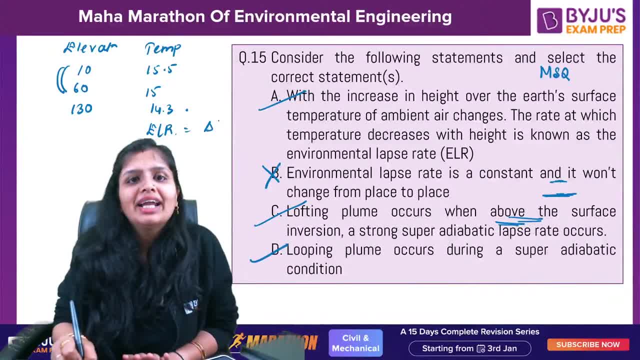 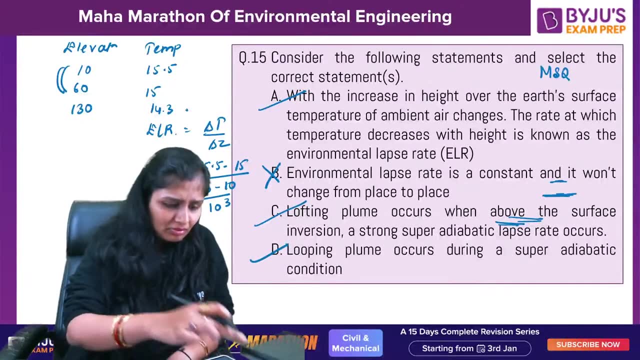 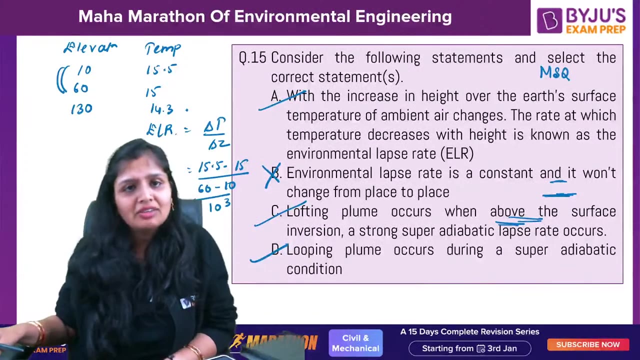 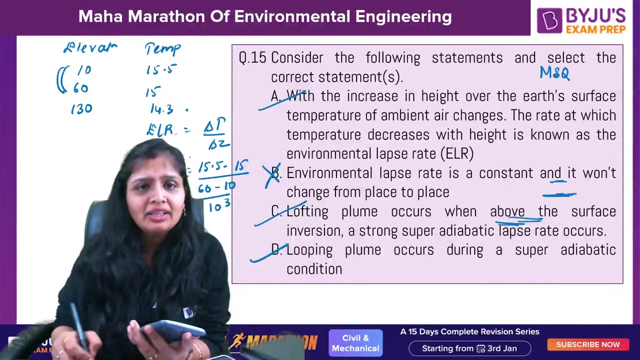 for first this condition: ALR. you will calculate, you know, delta T by delta Z. So how much is the change in temperature? 15.5 minus 15, I know decrease is taking place. 16 minus 10 divided by 1000.. How much it is coming? Yes, I will do it, Just do it quickly: 0.5 into 1050. 10. 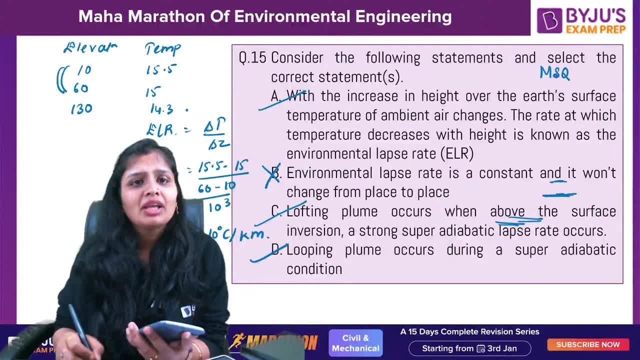 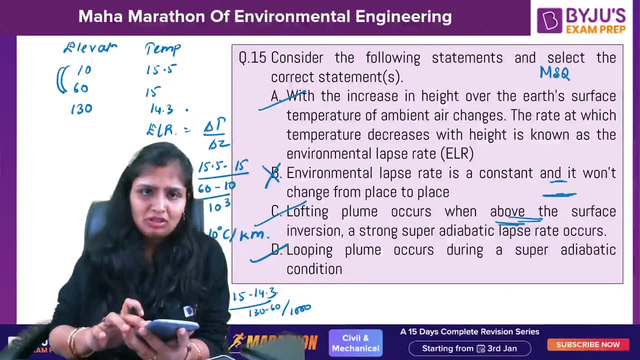 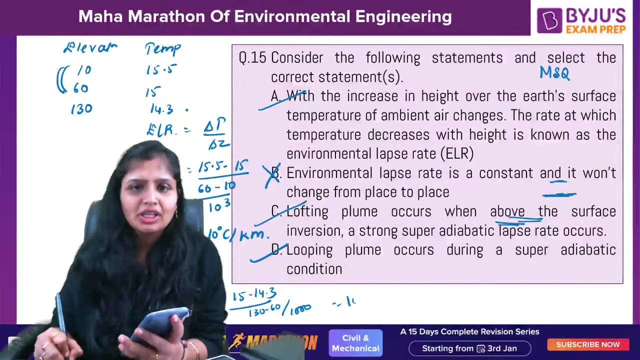 10 degree Celsius per kilometer. Okay, you can do it for 15 minus 14.3, 130 minus 60 divided by 1000.. So this will 15 minus 14.3, 10 degree Celsius. So ALR is 10 degree Celsius, which is greater than ALR. So this is an unstable. 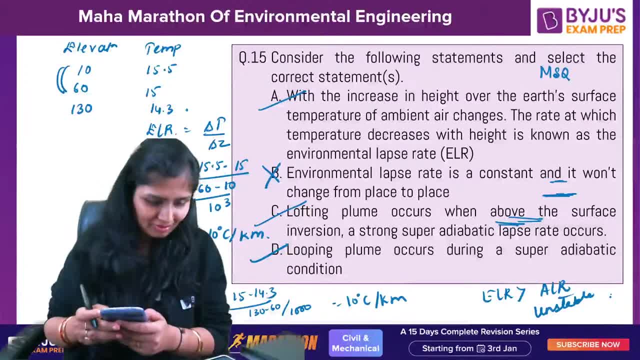 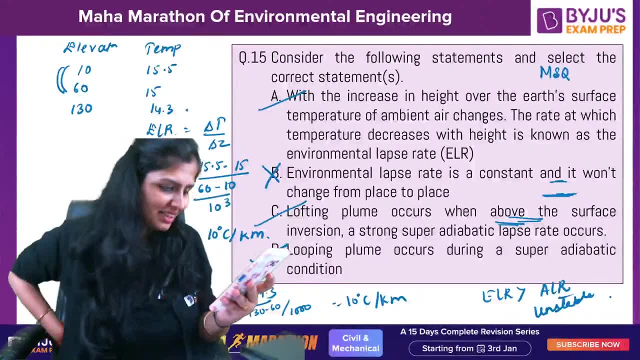 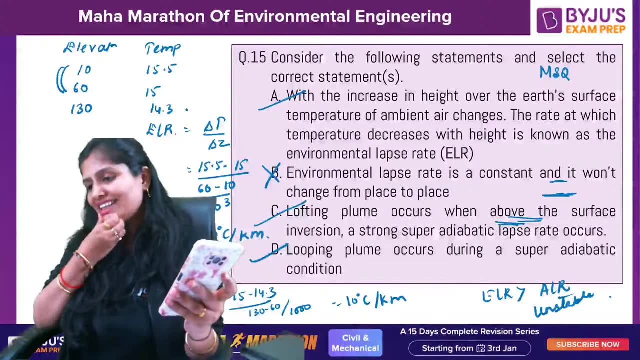 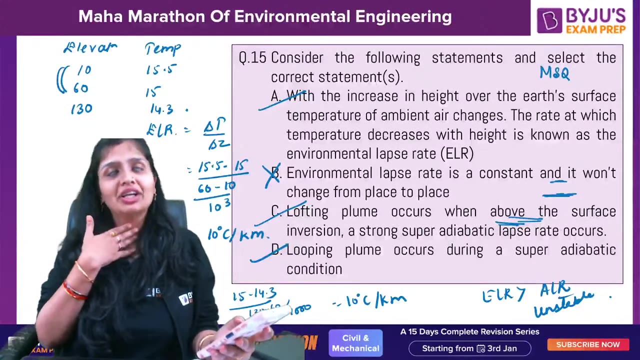 environment. Wow, Arun, Thank you, Thank you, Thank you. 95 hours, Very good, ma'am. Thank you, Vamsi. You will get its PDF Now. I will convert it to PDF, So I will give you its PDF. You will get the PDF in my telegram group also. 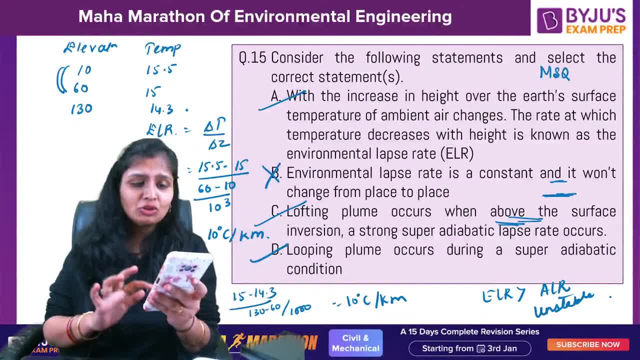 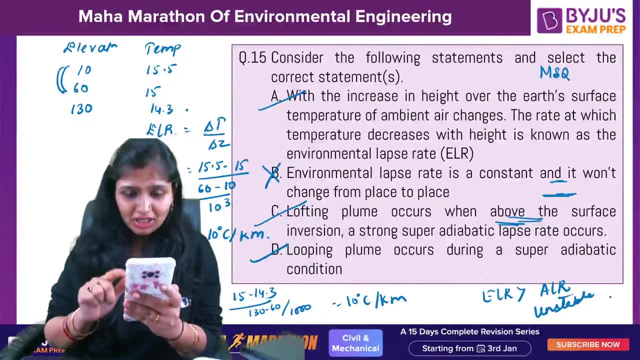 Everywhere you will get it. Okay, and I guess you guys know my telegram group So you can join me, tag me wherever somebody asked me. doubts also, but I was in the class So so. so. So I'll give you my telegram group also in case you want to join. 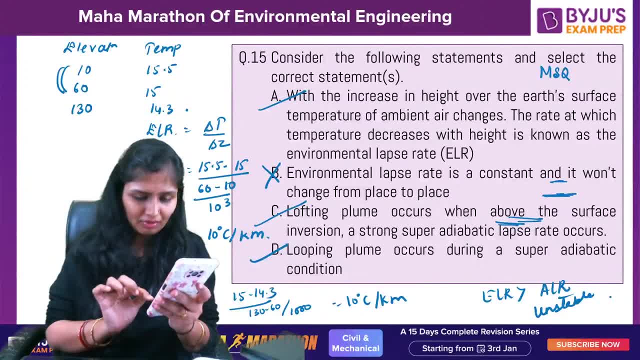 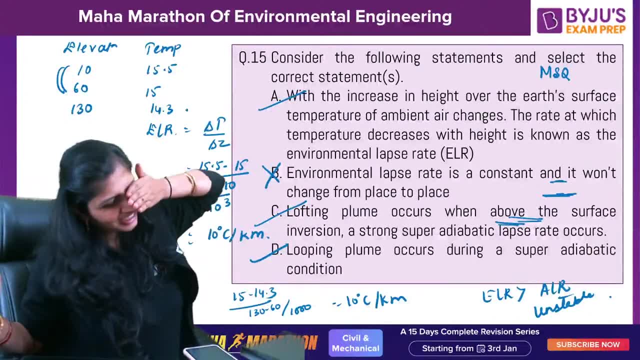 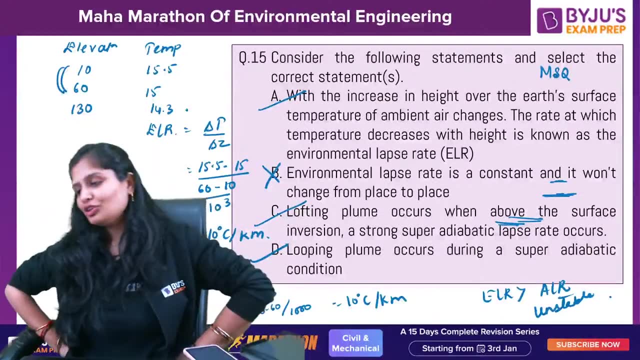 You can join it, Okay, Okay. So any more thing? Or should we say bye-bye, I don't feel like going, I don't feel good, I feel like that's it. Let's go Anything more? So tell me. 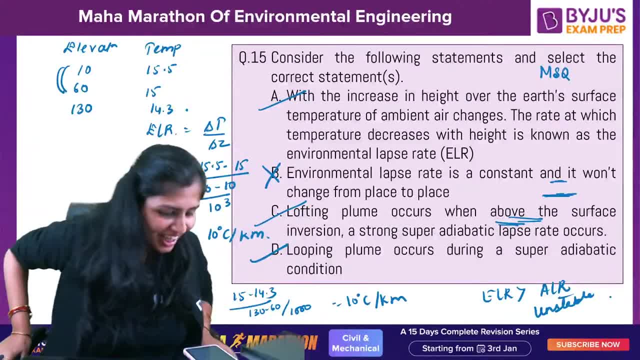 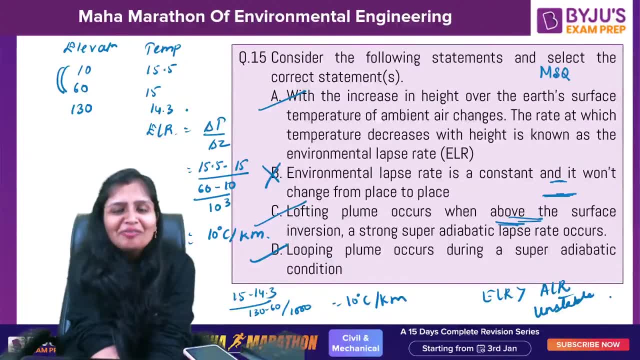 Otherwise we'll say bye-bye. Krishna Das, Kishaila Das will sing: Acha chalta ho, Dua ho, mein yaad rakhna Aisa kuch Acha, Yes, tomorrow. Abhinav sir's. 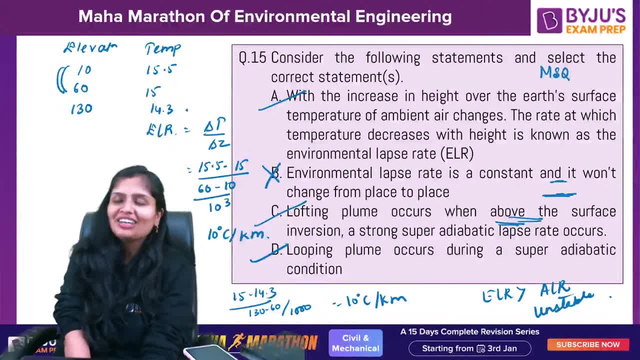 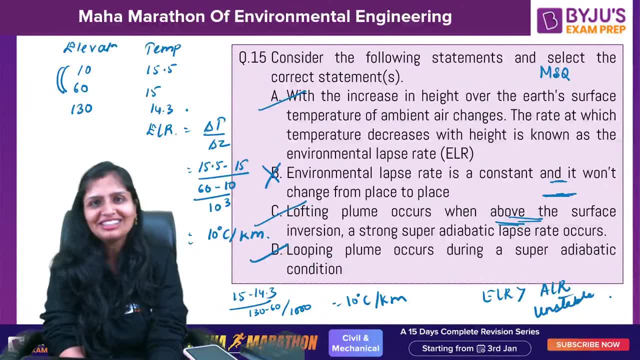 Good evening, sir. Tomorrow Abhinav sir's Geotech soil plus foundation is there, Sir, I'll also come to attend. Then I'll also learn soil. So 10 am session: is there guys? Link already ban chuki hai. 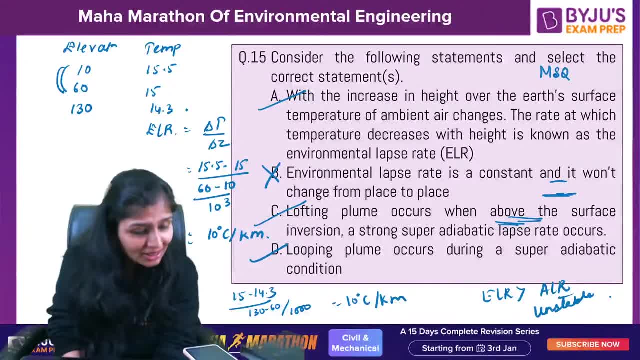 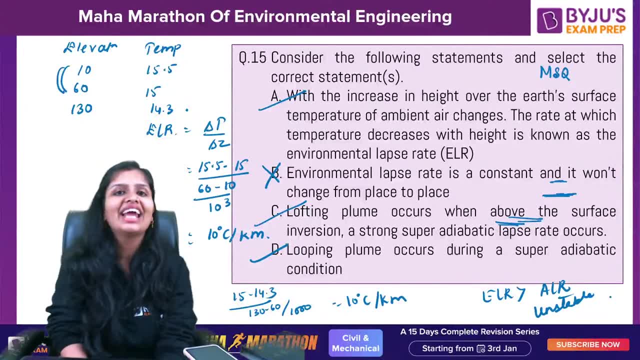 Set a reminder. Okay, Zero hardness method. ek baad Giri Sharma's zeolite method gives you zero hardness, in that you take salts like Na2OAl2O3.XSiO2.YH2O. That method gives you zero hardness, but use only sodium zeolite. 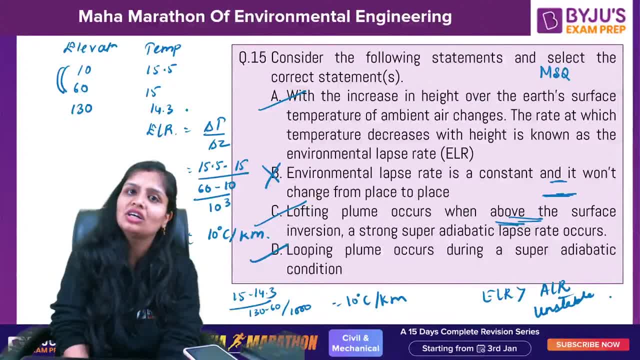 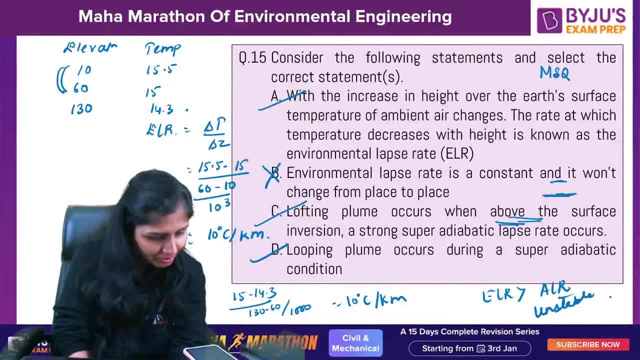 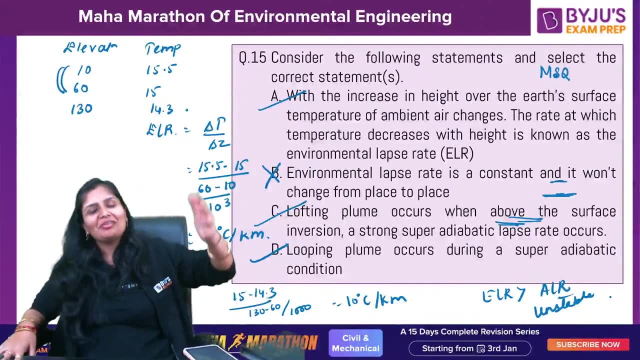 Regeneration can also take place in that Okay Of sodium, zeolite, Calcium and magnesium hardness are completely Okay. Okay, Okay, Okay, Acha to hum chaltay Kishala. ek din hum log na melody create karte hai. 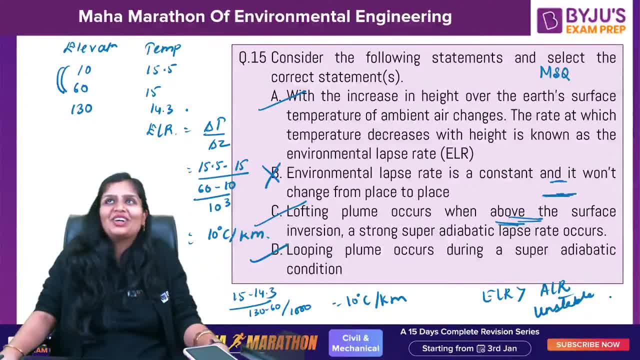 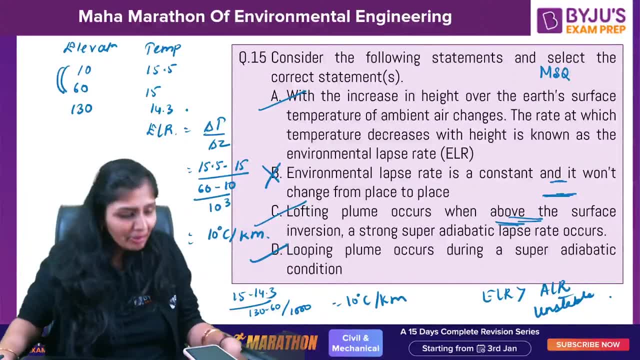 14 minutes remaining to complete 10 hours. Oh my God, Fine Ma'am environment. ka small quotient state easy karwa diye. Next session: Okay, fine, I'll take a midnight session and, Girish, I will include quotient of. 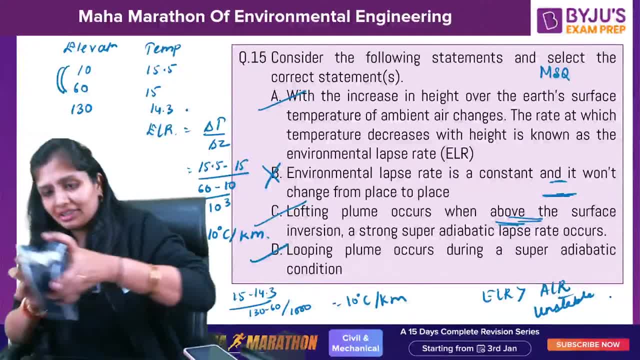 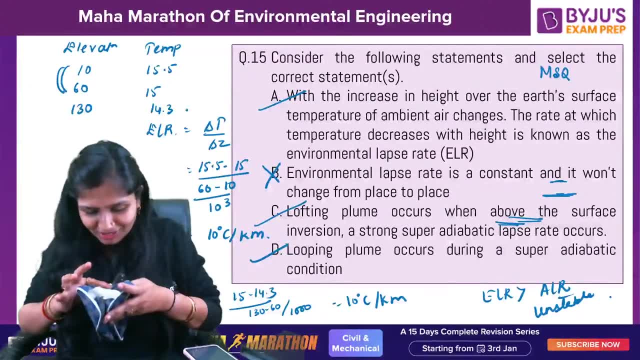 Ek minute. I'll write it down first, Otherwise I'll forget Itte saare pen hai par, phir bhi pen nahi mil raha. likhne ko, Dekh rahe ho, Dekh rahe ho, Binod. 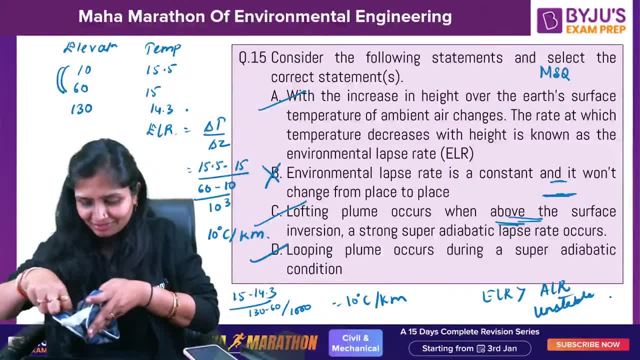 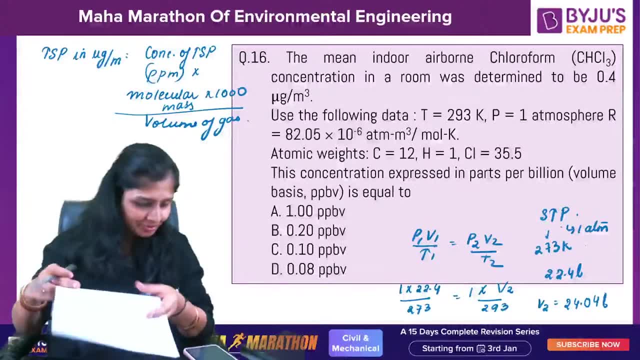 Just a minute, Tell me kya kya cheez include karna hai. Chalo pen ko sahi likh le Kuch Batao. What's the things I need? Firstly, solid waste ash free bases wale quotients. 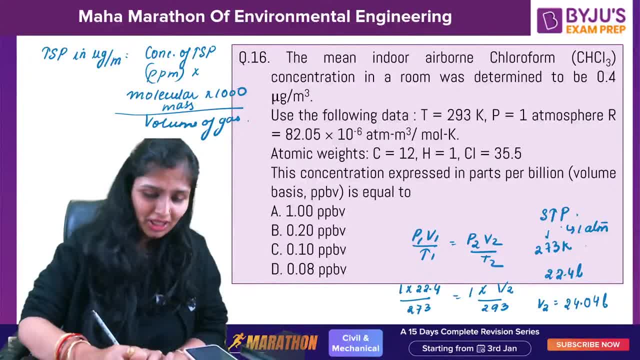 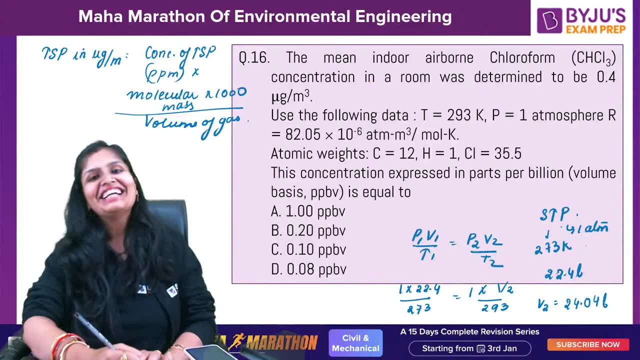 And what else? Zero hardness, wale quotients, What Be fast Up to 8 so that we can make 10.. I'll continue up to 8.. 10 hour session. Okay, What else guys? Tell me fast. 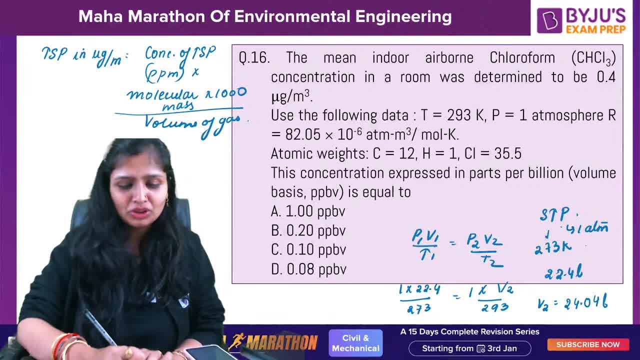 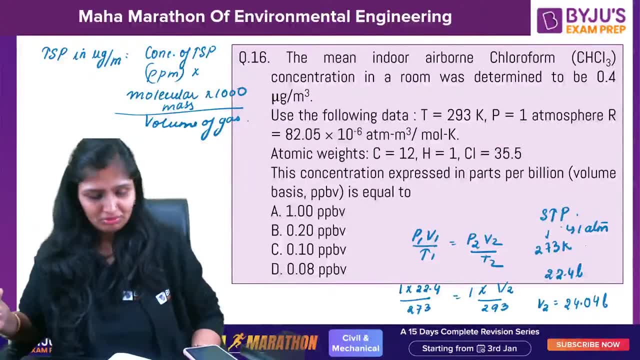 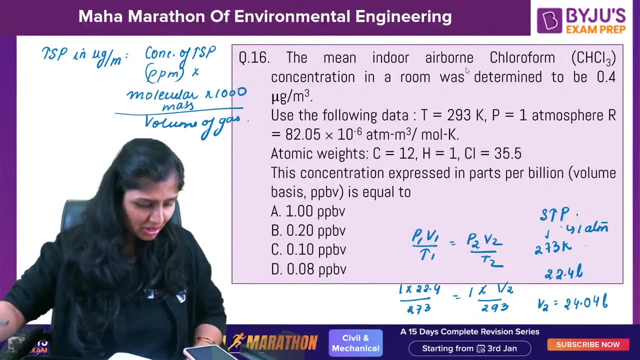 What else you want in the quotient series? I will prepare quotients: Ash, free bases, zero hardness. What else you want? Fast, fast, fast. Microgram to Pivometer convolution in unit BOD quotients: Okay. 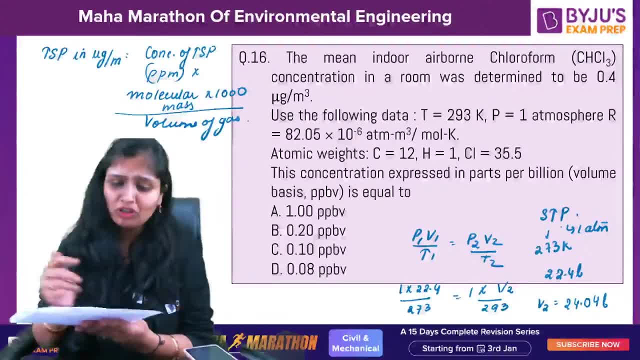 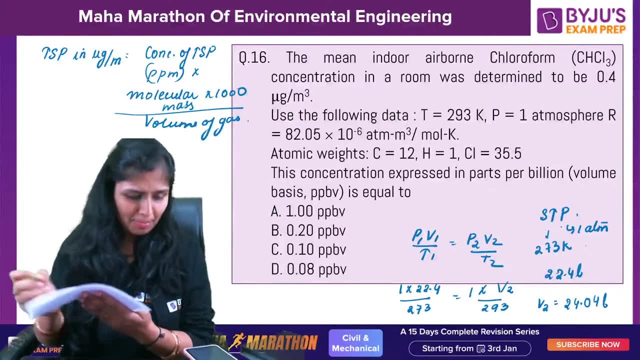 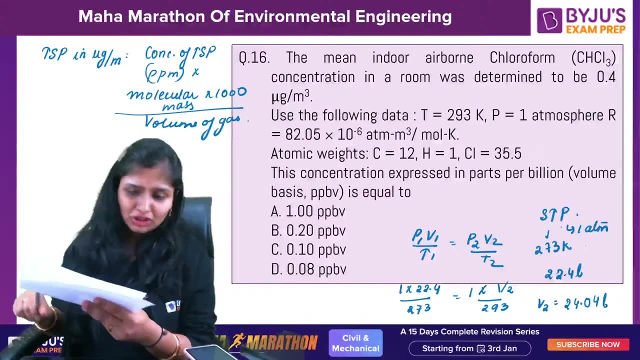 Have you got quotients for Streather-Phelps equation also? You want Streather-Phelps equation quotients also, Streather-Phelps BOD done, Okay, fine, So there's quotients and Girish told me regarding zero hardness. 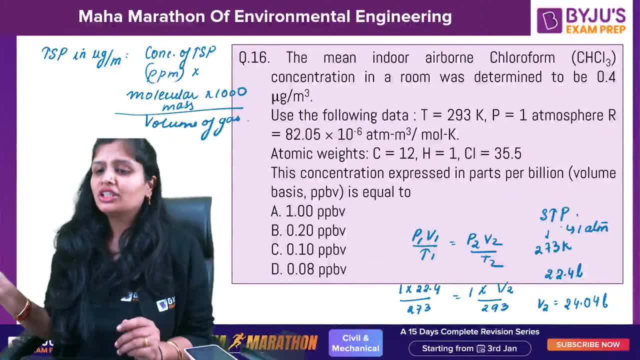 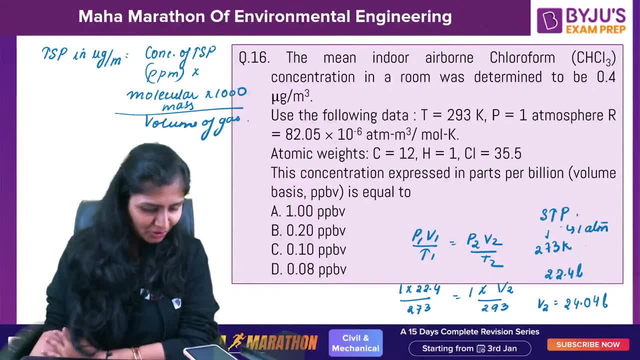 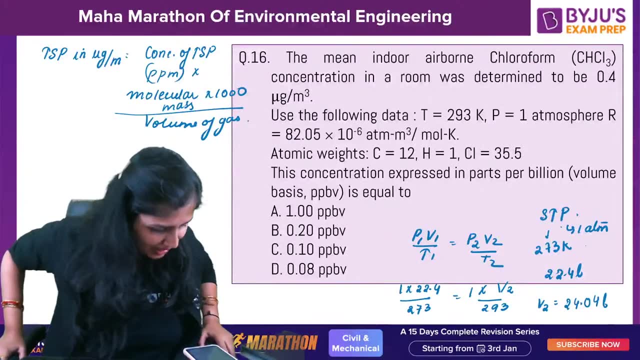 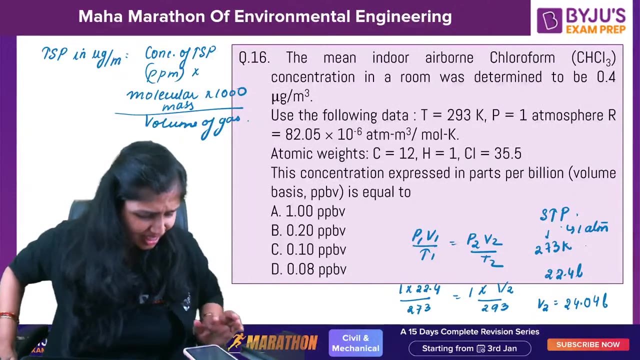 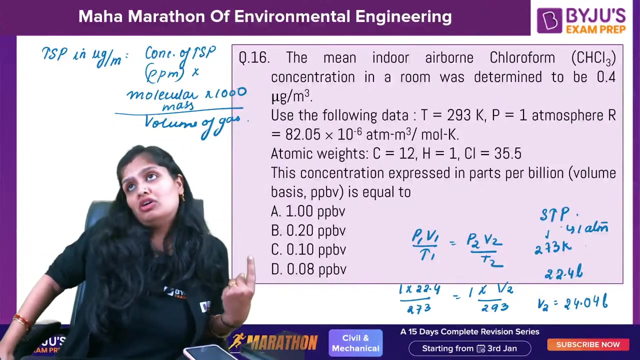 Okay, fine, Mentioned. So we'll take all these quotients into account. more number of questions for you and there will be a question series also coming, so don't worry, maximum questions. we know sabine genius. if you talk about velocity over flow rate, the plan area or the surface area is b into l. 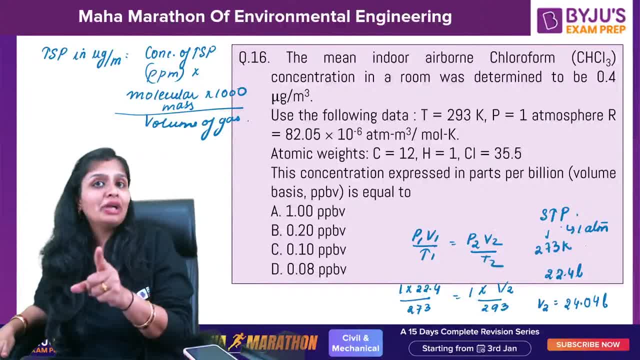 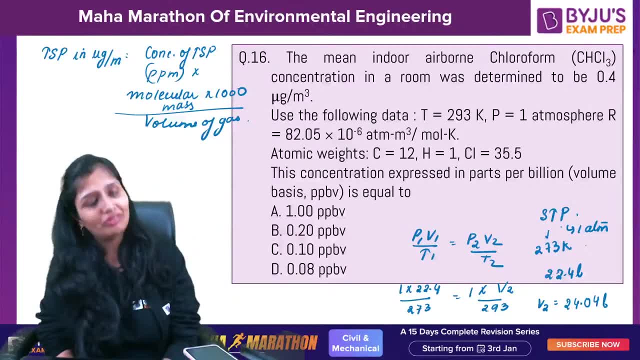 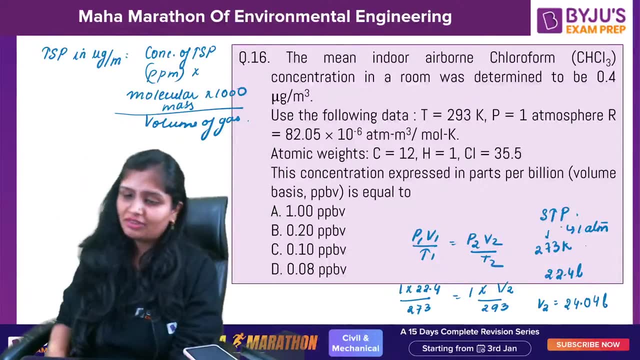 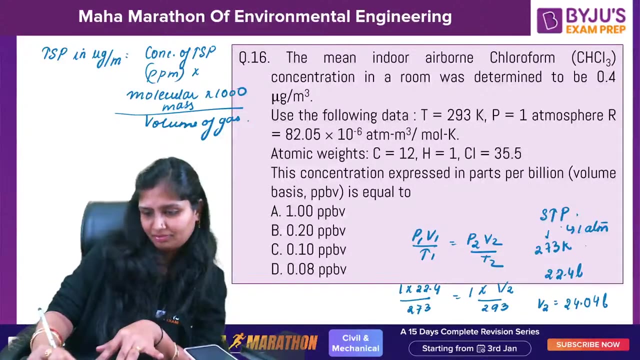 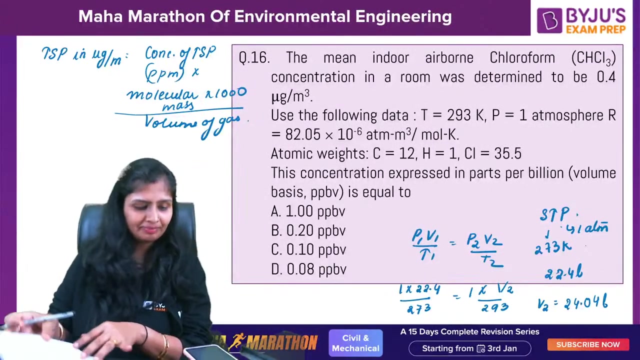 cross-sectional area is b into h. if you talk about sedimentation, the plan area is b into l. noise pollution is also done. it is not in gate, but i will do it. ok, prashant, i will do short questions. one max questions. ok, any more doubts? 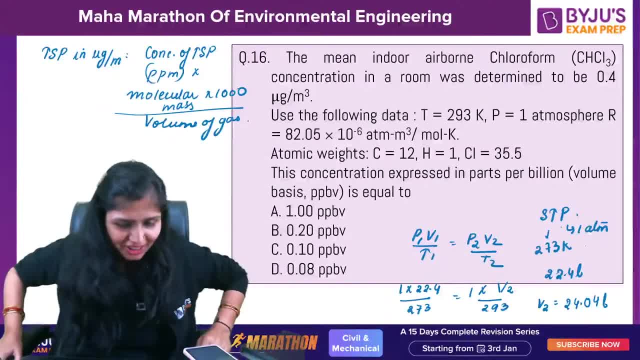 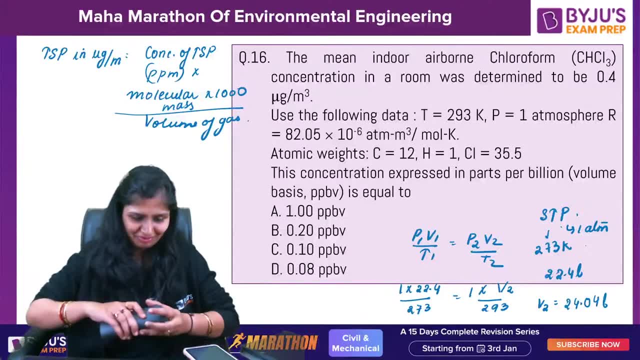 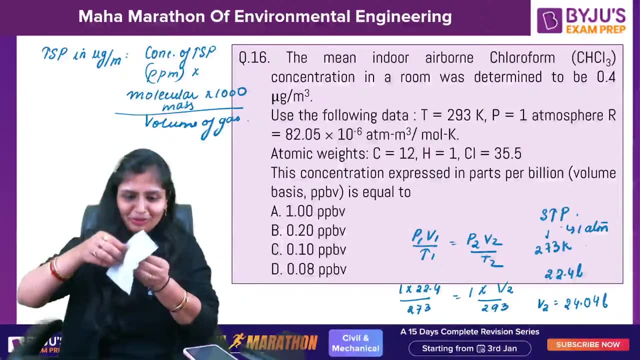 read by indian��. come on, lets continue. lets do something else. very more creativity. do you know indians? second thing happens when somewhat things are involved, 嗎 it Chooses to take care of the things. first thing: i broke 1 glass, so am i holding the other glass? very well. 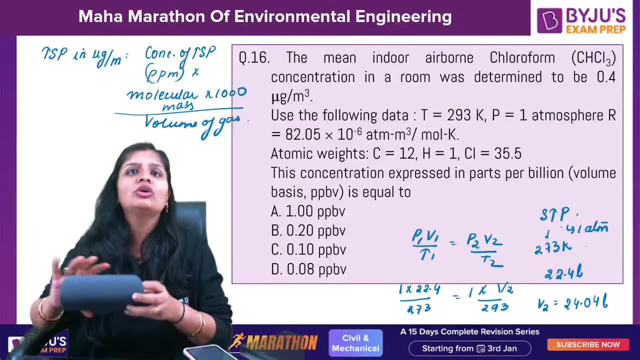 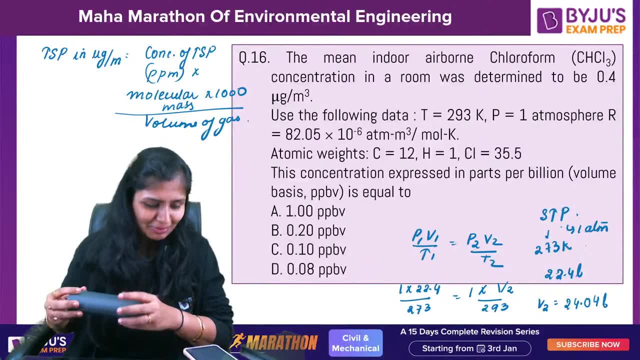 daily dose: continuous to learn. the time is now 8 pm. meet the match date. master is 6 or better than at 8 pm. Okay, I will make you fail. sometimes. I will make you do everything. Now I just have to study GS. 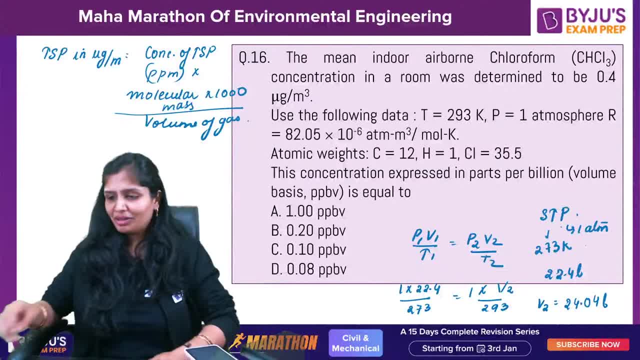 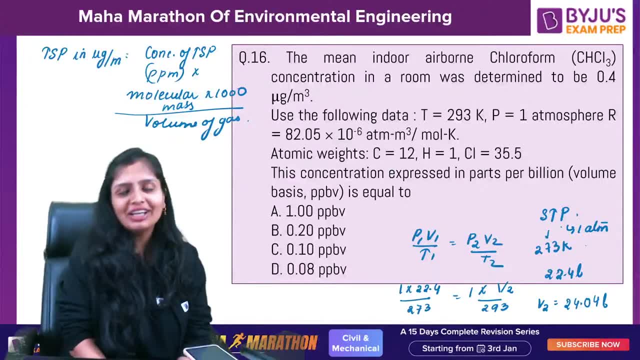 So let's meet now. Oh, it's been a long time, I don't want to pass the time. Okay, never say goodbye. Okay, I am not saying goodbye. You will get the PDF of this class. Okay, The calculation mistakes and all. check it out. 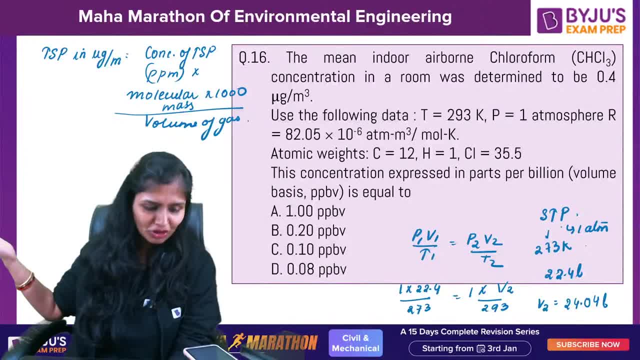 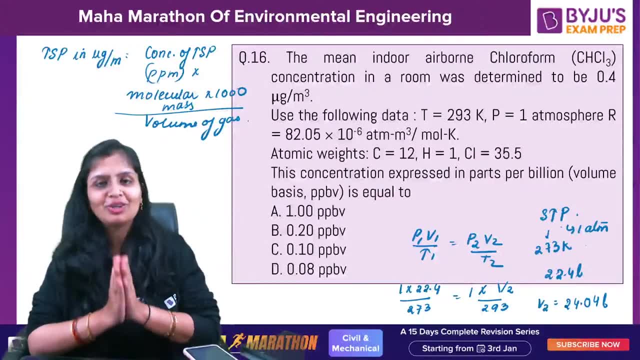 If there is a little bit, then somewhere. you only told the answers. I don't have anything in it. Okay, thank you. Thank you so much, everybody. I didn't felt like I will be able to take such a long class. But Prashant Aayushi Sachin. there are n number of names. 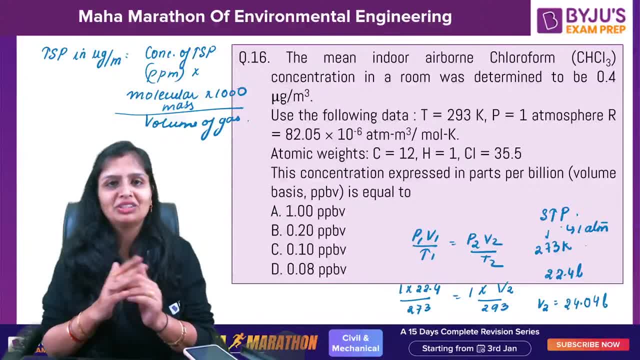 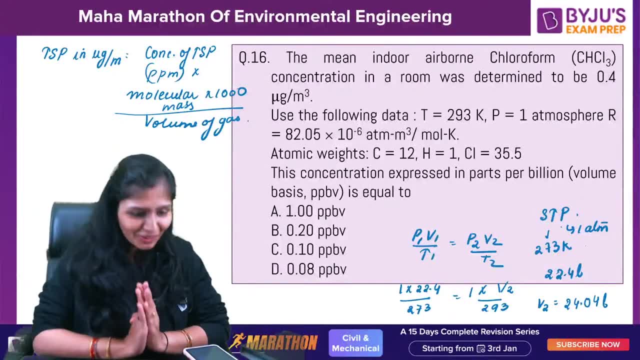 Devanshu Sopnil Ronan, everybody. Okay, Das ji, thank you so much for being with me patiently and listening to me. Arun's blood also came out of his ears. even then he listened to me Okay. 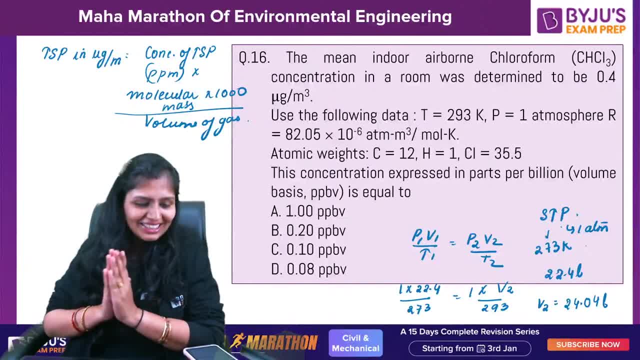 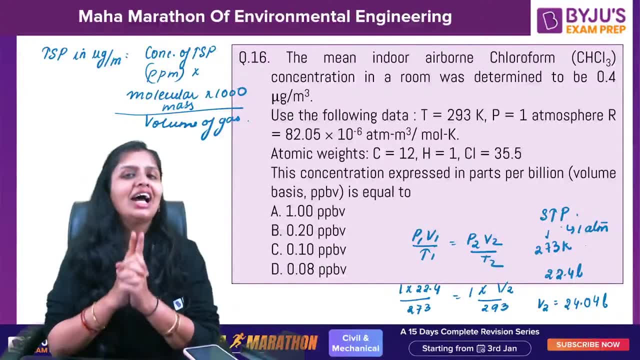 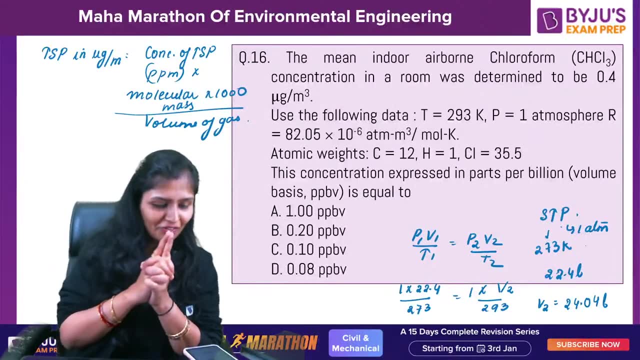 So, guys, knowledge adha. thank you, Thank you everybody. Lots of love to you. Similarly, I will be coming on Wednesday with hydrology and irrigation marathon. You have to be there with me. Promise me, Love you, Love you everybody. 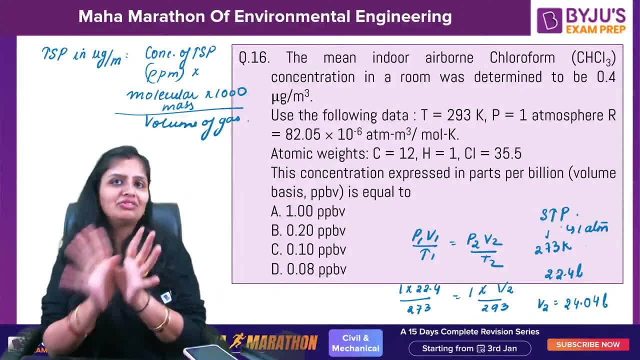 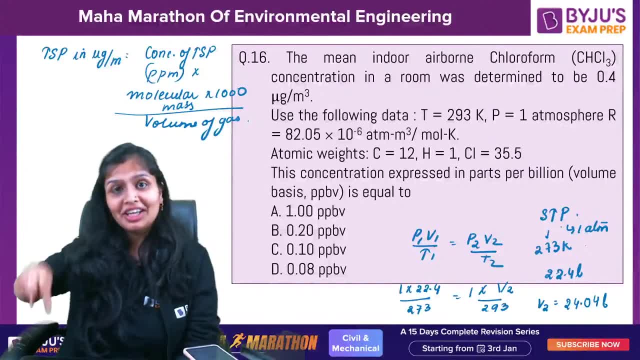 And promise me you will be there. Okay, hydrology first, then we will go for irrigation. Okay, Okay, you have to rock it and gate. See, I was there with you. You know, I woke up in the morning because of you guys. 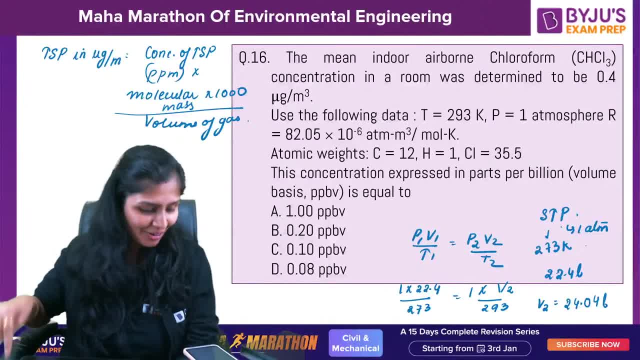 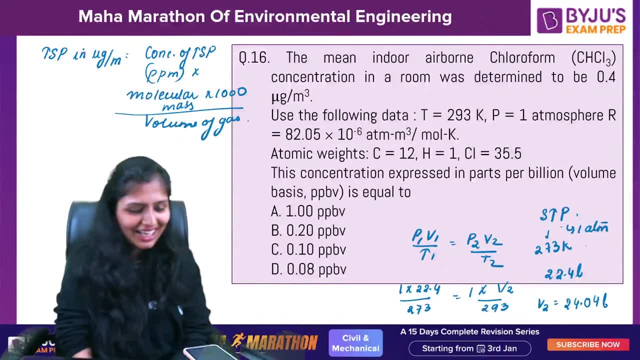 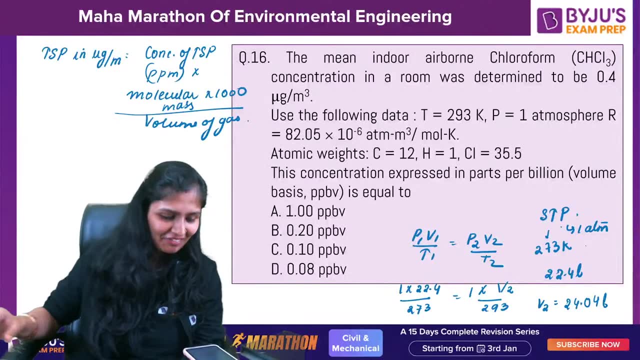 So you have to crack gate at any cost? Okay, fine, So we will meet you. Thank you so. so so much, guys. Now will you make me cry, you fool. Come on, keep it. Okay, guys, Sachin, everybody. 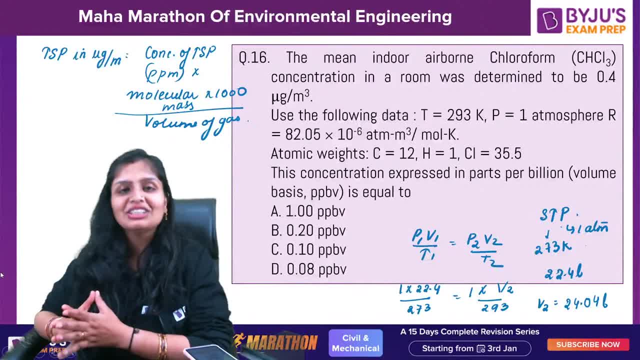 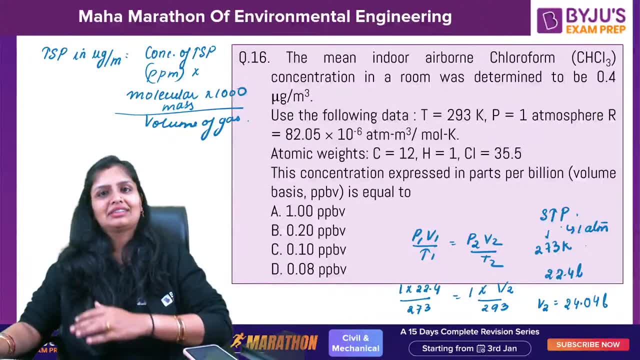 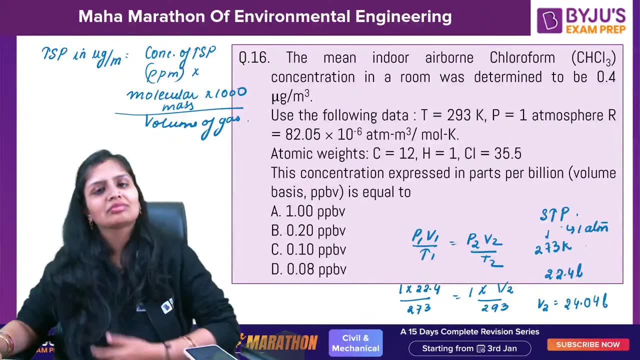 Thank you so much, guys. Good night, Take care of yourself, Bye, bye and study hard. Bye, Bye, Bye, Bye, Bye, Bye.